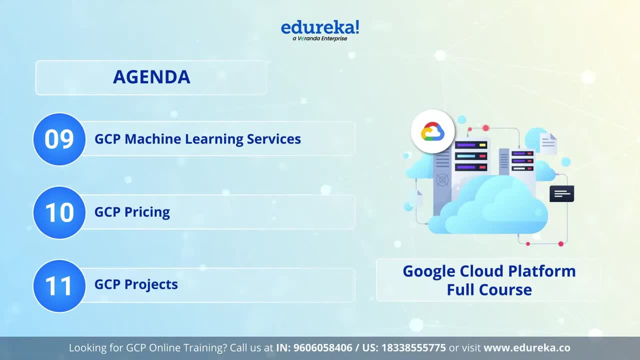 In order to accomplish this, we will look at how to start a career in Google Cloud Platform, where we will see the different certifications in Google Cloud Platform, followed by some essential GCP interview questions with answers. So stick till the end. What is cloud computing? 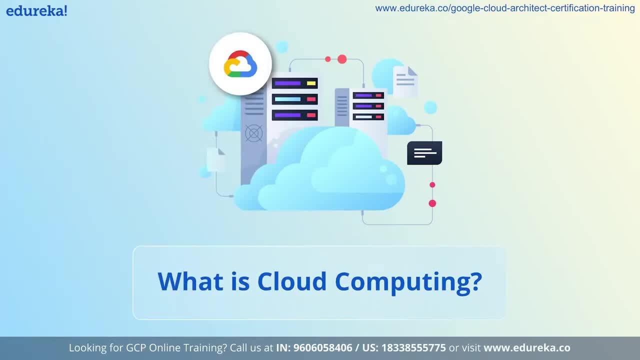 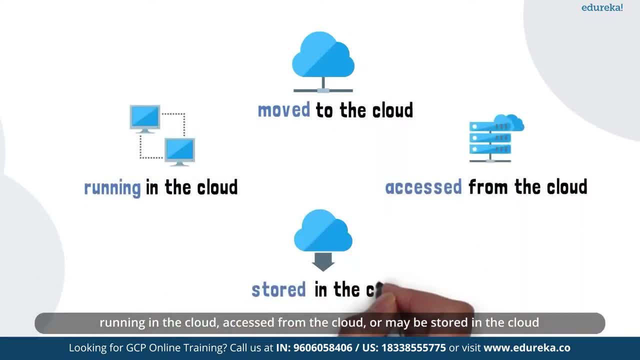 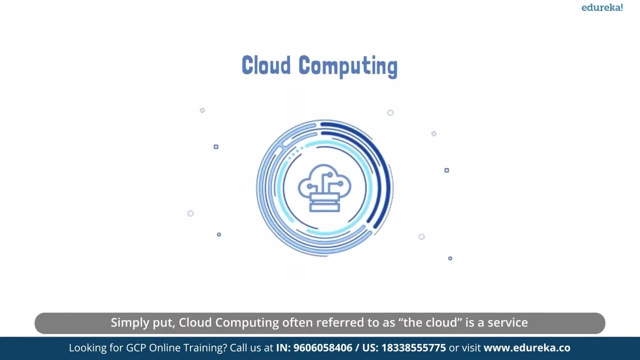 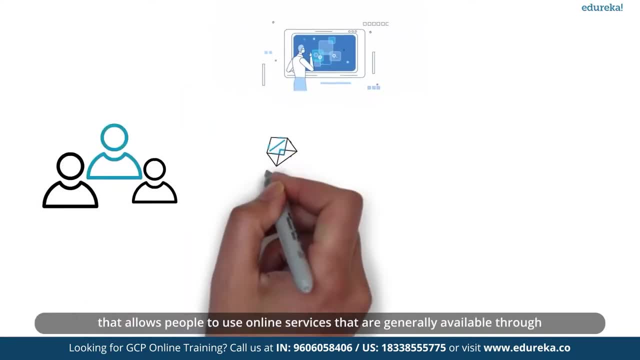 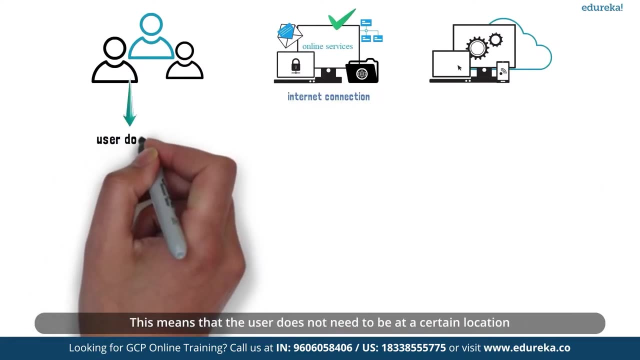 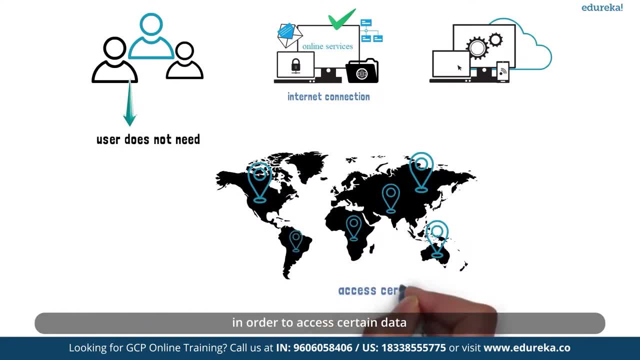 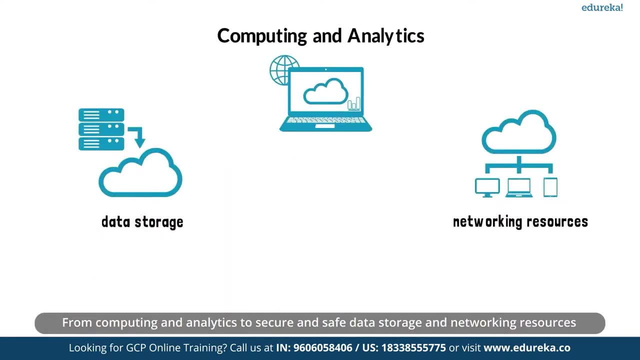 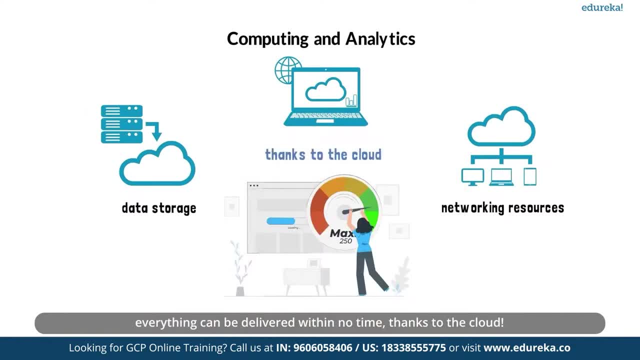 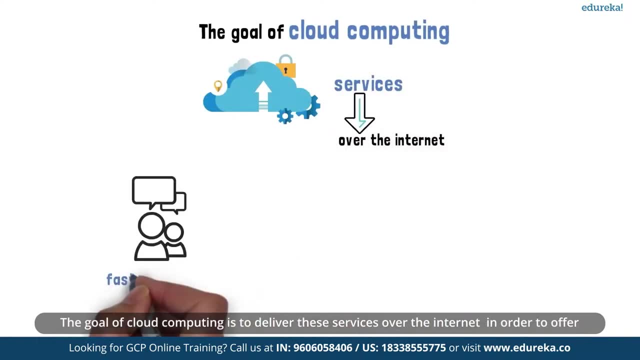 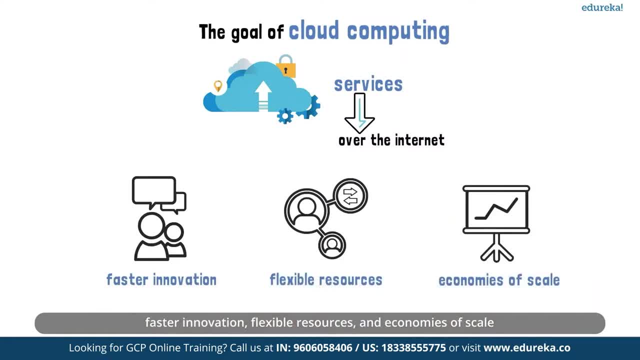 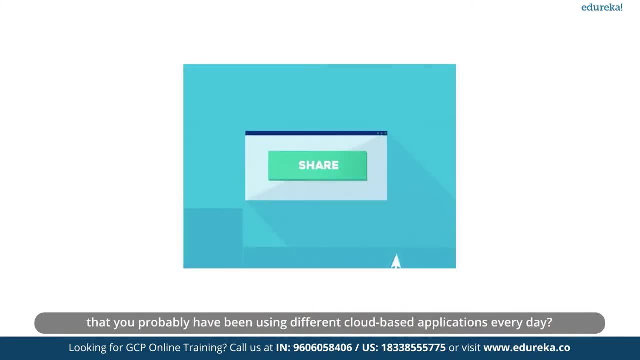 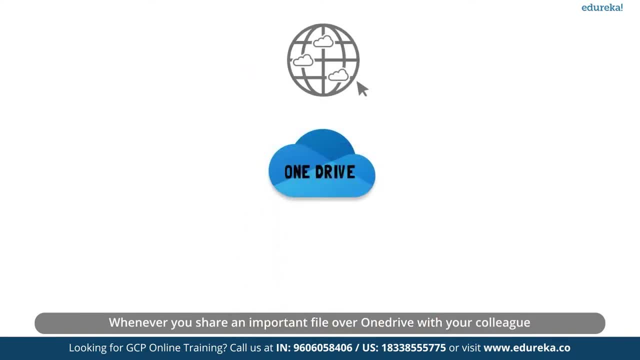 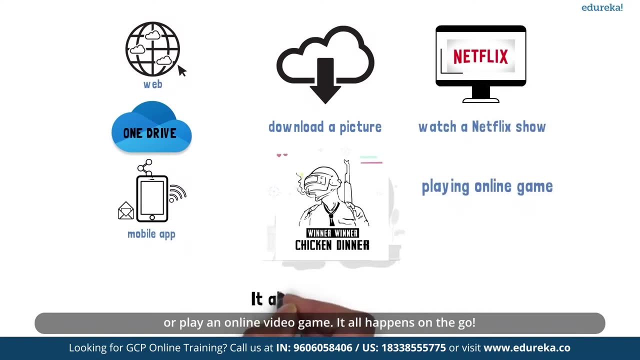 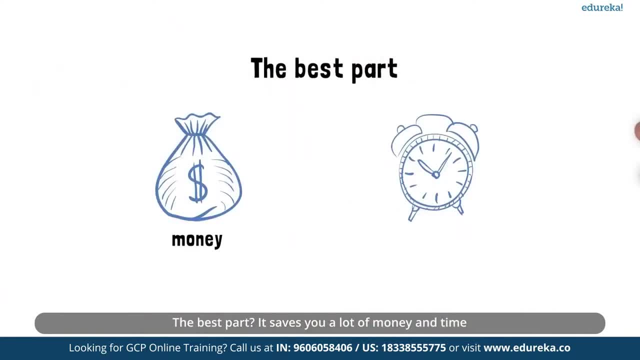 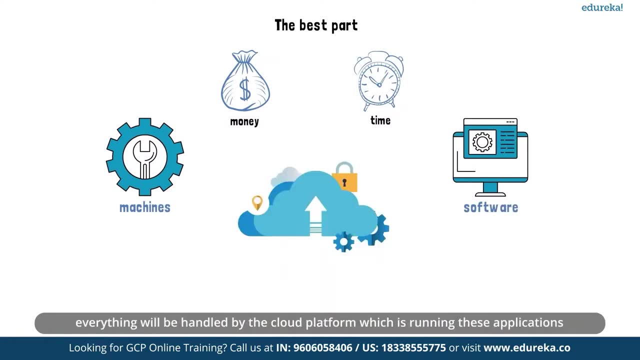 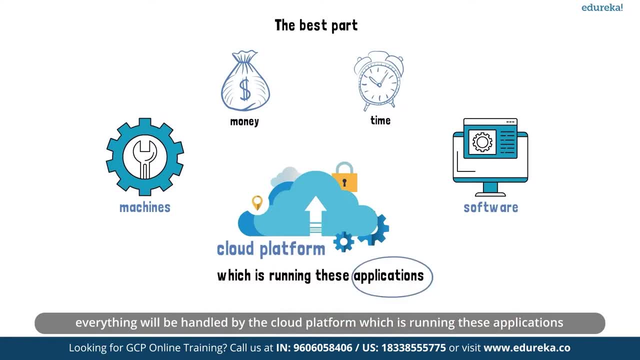 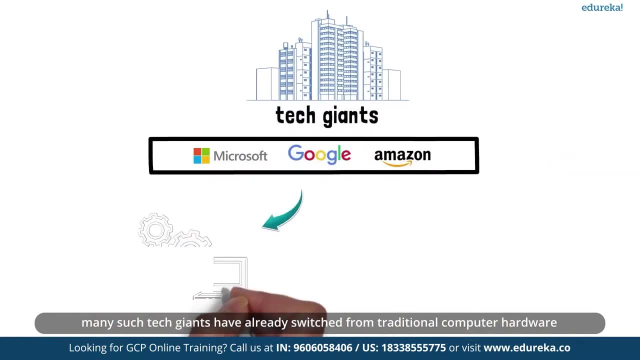 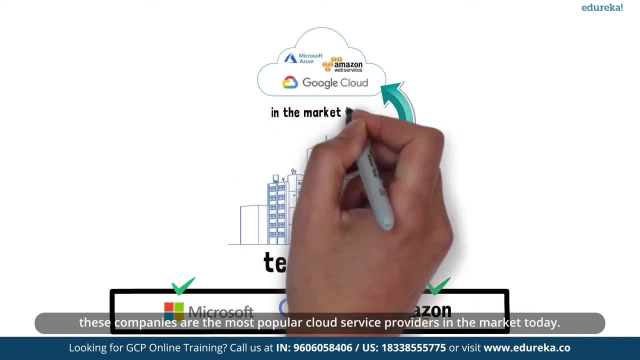 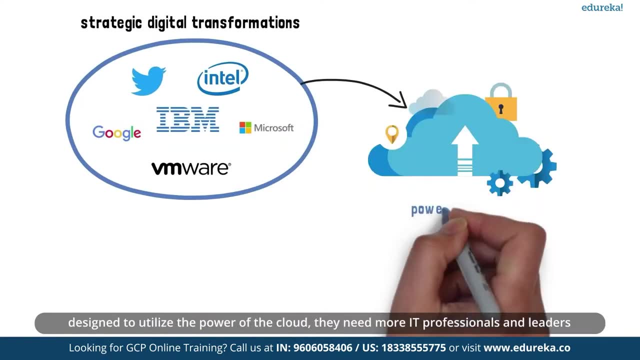 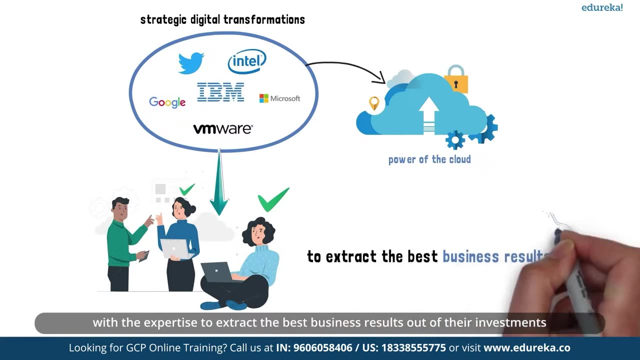 these companies are also the most popular cloud service providers in the market. today, As more and more companies undergo strategic digital transformations designed to utilize the power of the cloud, they need more IT professionals and leaders with the expertise to extract the best business results out of their investments. 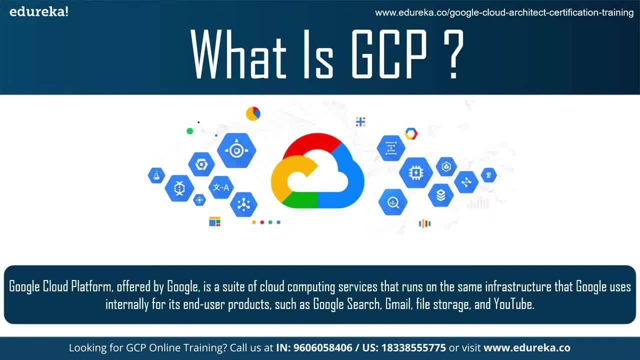 What is Google Cloud Platform? Offered by Google, it is a suite of cloud computing services that runs on the same infrastructure that Google uses internally for its end-user products, such as Google Search, Gmail, File Storage and YouTube, Along with a set of management tools. 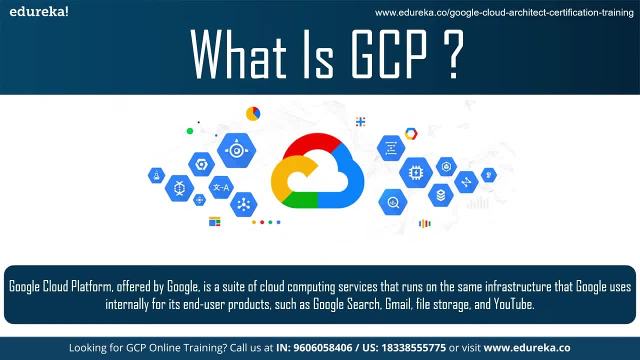 it provides a series of modular cloud services, including computing, data storage, data analytics and machine learning, For organizations with large amounts of data to store or analyze. Google Cloud storage prices are up to 20% cheaper than AWs and the price of database services. 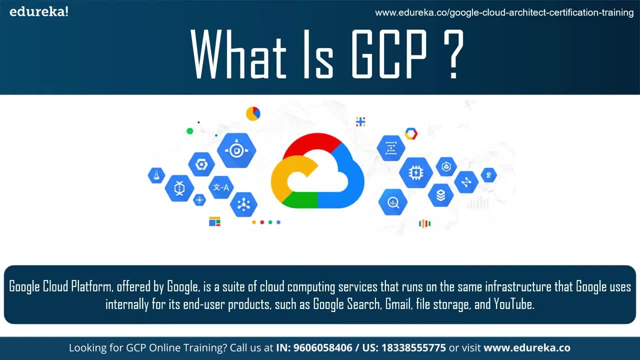 also compares favorably, While there is no difference in the price of container services. Google Cloud is an industry leader in the field and is also investing heavily in AI and machine learning technologies. Many small and large enterprises are increasingly adopting Google Cloud Cloud Platform for end-user cross- graduated. 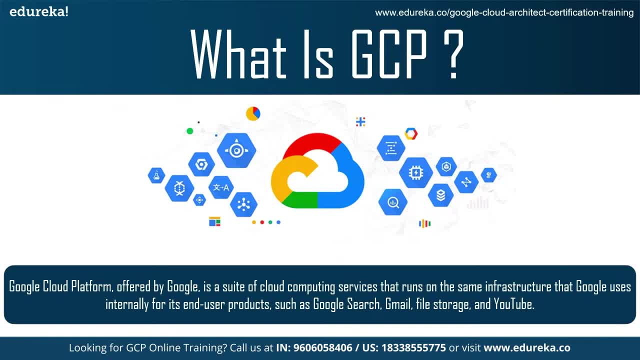 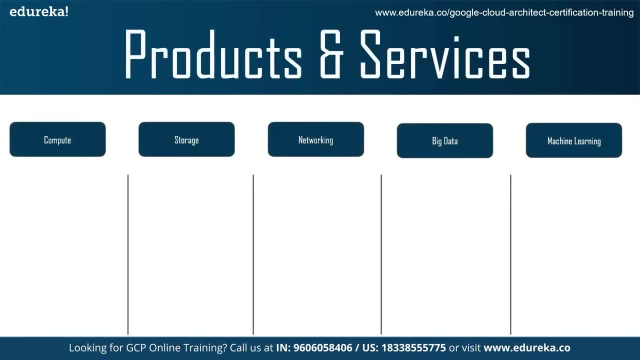 dawn, kind and VR. This network is a great hub for machines cloud platform since it engages things and makes them more secure at reasonable costs. let's now understand different products that google cloud platform offers. we can divide google cloud products and services into five major categories, that is, compute, storage, networking, big data and machine. 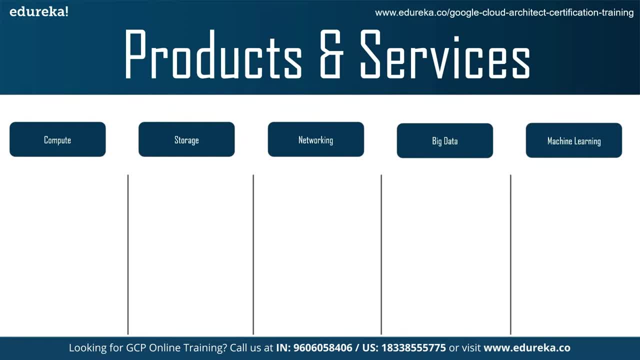 learning. so let's first understand what compute does. the secure and customizable compute service lets you create and run virtual machines on google's infrastructure. these are the subcategory of products provided in compute. so first in the category is compute engine, which offers platform to run your virtual machines, your virtual servers, on google cloud. 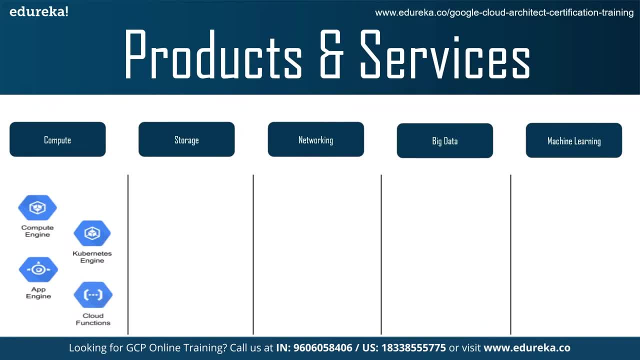 so suppose if you have a server sitting in a house and if you want to deploy a similar server on google cloud, okay, you would use compute engine to do so. so next is google kubernetes engine, which provides a managed environment for deploying, managing and scaling your containerized applications using google infrastructure: the google kubernetes engine. 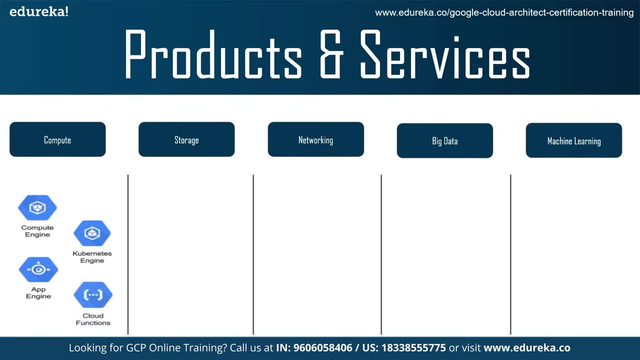 environment consists of multiple machines grouped together to form a cluster Moving on App Engine. as the name suggests, it is an application engine where you can deploy your web applications, your large-scale applications, without any headache of managing the backend infrastructure. Now, moving on to the last category in compute, that is, Cloud Function. 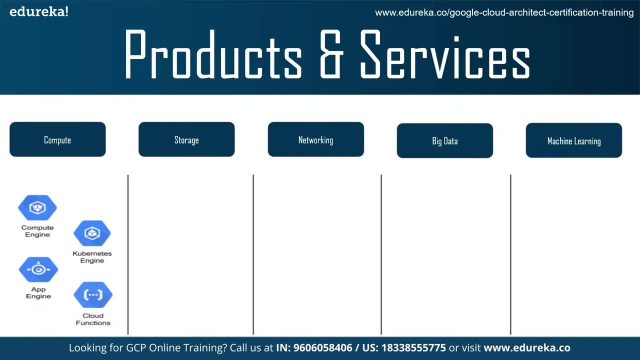 which allows you to trigger your code from Google Cloud Firebase and Google Assistant, or call it directly from any web, mobile or backend application via Hypertext Transfer Protocol. Moving on to storage, this is the USP of Google Cloud, because ever since Google came into the market, 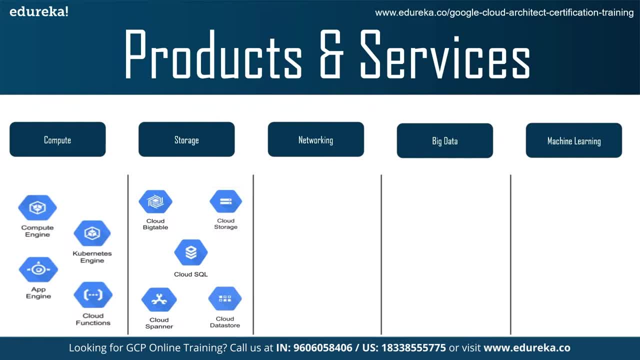 its storage and how it deals with the data has always been its USP. So these are the subcategories under storage. The first major product provided under storage is Cloud Bigtable, So it is a NoSQL database. For people who don't know what is NoSQL database is: 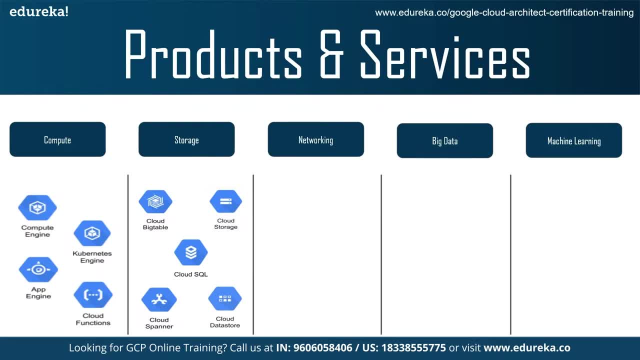 it simply means it's a database where you cannot apply concepts of traditional relational databases to data which is not structured, which is big data, which is sparsely populated. All such kind of data can be stored and you can simply consider the second category. 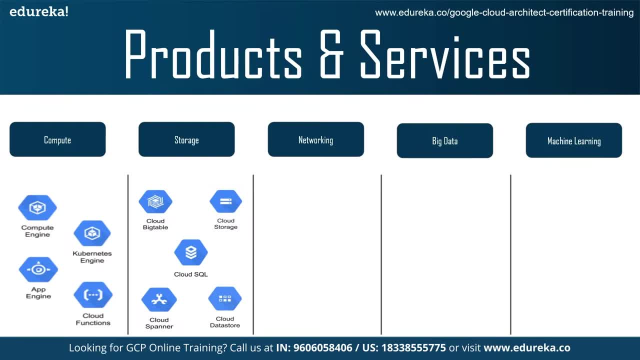 which is Cloud Storage as a C or D drive on your laptop. It is an object store where you can store all kinds of objects like images, videos, documents, etc. It is a concept of buckets, So within storage you have multiple buckets. 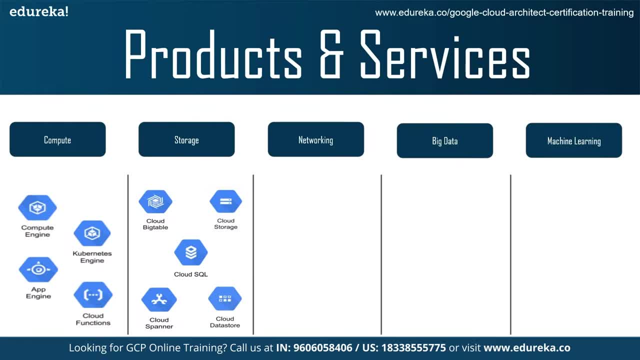 like you have folders in your drive right, And within those buckets you can store your files, just like you store files in your folders in your hard drives right In your laptop. So moving on to the next one, that is, Cloud SQL. 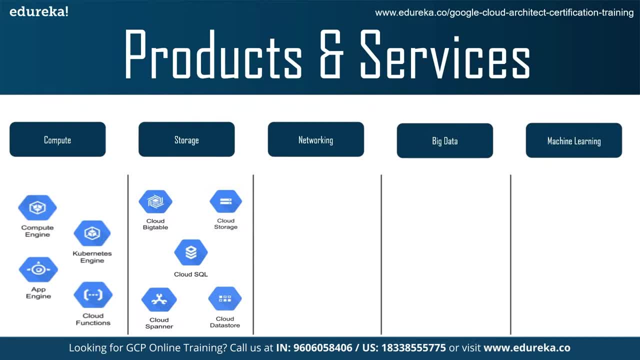 So Cloud SQL is a relational database. So Cloud SQL is a relational database product. It's very efficient if your database is not very large and it's very good for database analysis. It is a fully managed database service which makes it easy to set up, maintain, manage. 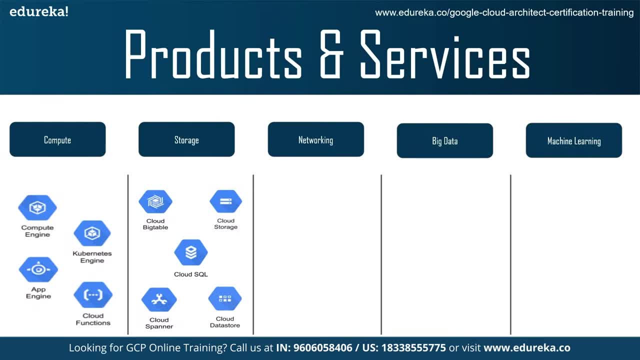 and administer your relational databases on Google Cloud platform. Cloud Spanner can be considered as a big brother for Cloud SQL, So Cloud Spanner is a relational database with big data capabilities. So you can consider it as if you combine Cloud SQL and big data capabilities. that make Cloud Spanner 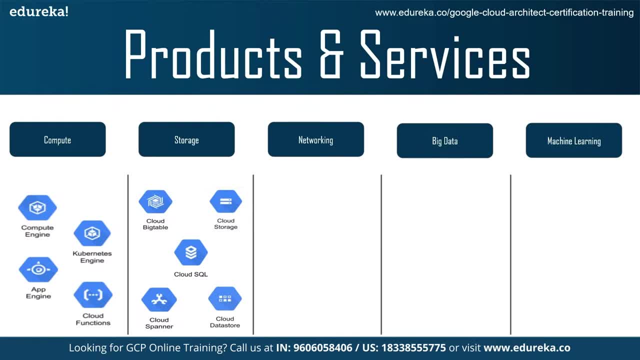 So Cloud Spanner is similar. It's a way to run SQL with massive scale and massive capabilities to run big data loads with SQL support. Now moving on to the last one in this category, that is, Cloud Datastore, which is a subset of BigTable. 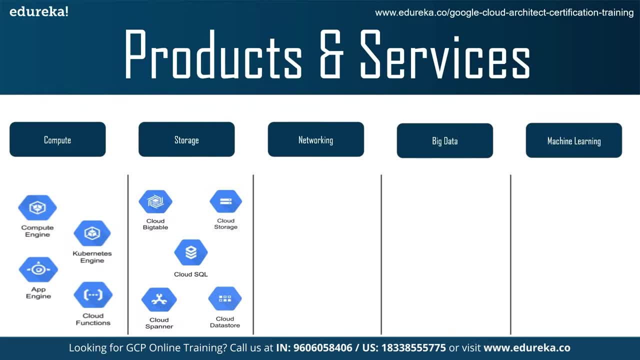 because what BigTable cannot provide is somewhat provided by Cloud Datastore. So Cloud Datastore sits on BigTable technology with a slight SQL support. Although it is a no SQL database, it still gives you some flexibility of using SQL and doing your analysis. 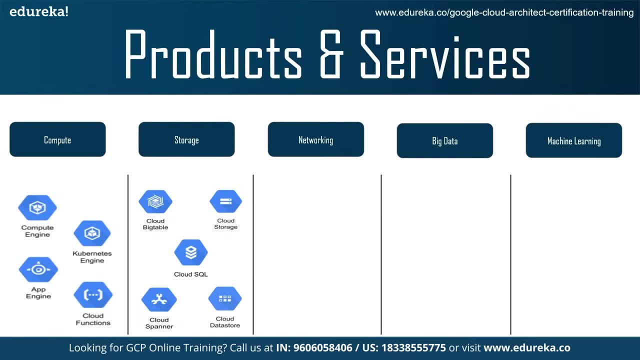 Now coming to the third category, that is, networking. So Google Cloud Networking has tools that make it easy to manage and scale your networks, and these are the subcategories under networking provided. so first in the category is cloud load balancing, from which you can scale your applications on. 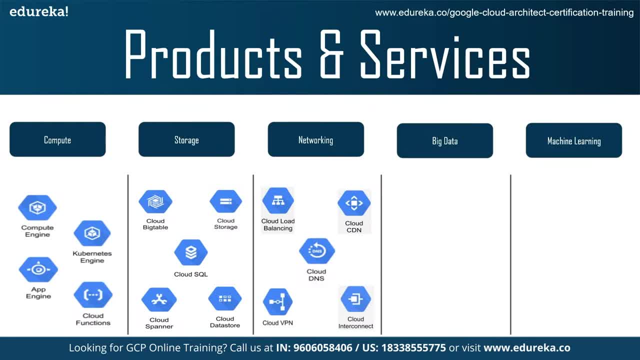 compute engine from zero to full throttle with no pre-warming needed. it is a fully distributed software defined managed service for all your traffic. now moving on to cloud cdn. extended as content delivery network, it offers connectivity to more users everywhere. and next is cloud dns, a service which provides you a network of dns servers- dns extended as domain name servers. you. 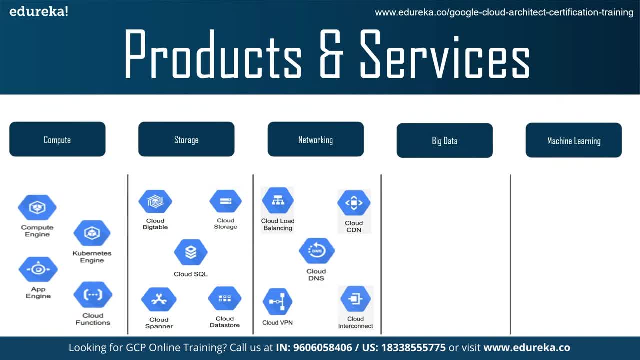 can easily manage your dns report through its interface. now moving on to the next one, that is, cloud vpn. vpn is extended as a virtual private network, so cloud vpn securely connects your peer networks to your virtual private cloud network through an ip secure vpn connection. now moving on to the last one in the category, that is cloud interconnect. so cloud interconnect establishes: 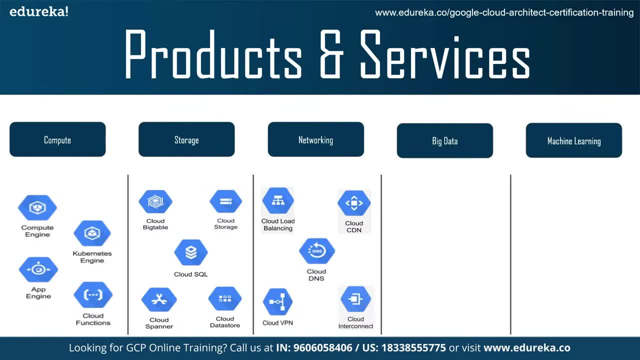 private connectivity from your data center, office or co-location environment to reduce your network costs, increase bandwidth throughput and provide a more consistent network experience than internet based connections. so moving on to the fourth one in the major product, that is big data. so it is natural if you see to host a big data infrastructure in the cloud, because 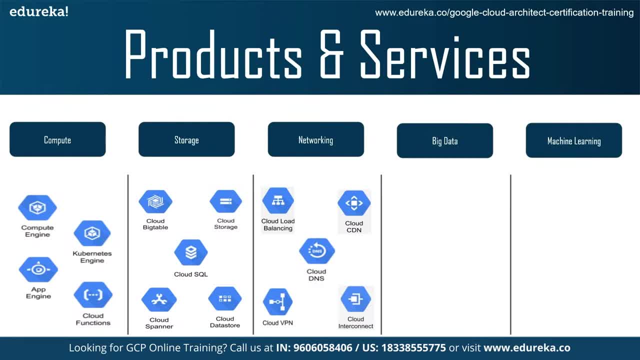 the google cloud platform provides multiple services that support big data storage and analysis. so these are the subcategory under big data. so first in the category is big query, which can run your data analytics and data loads, and you can, like store your massive amount of data under data warehouse. so whatever data warehouse or data lake needs you have, you can get it fulfilled. 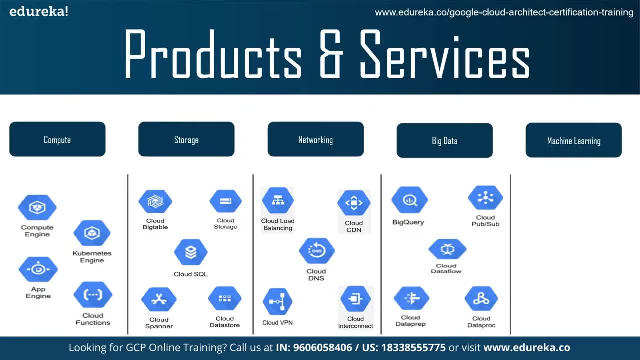 by bigquery. so next is cloud pub sub, which is a technology which is used to ingest streaming data into google cloud platform. it is a middleware which sits between source and google cloud platform. okay, now moving on to the next one, that is, cloud data flow, which can simply be considered as an 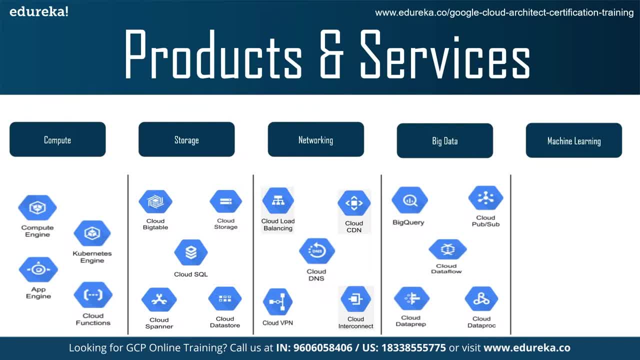 etl product. this helps you in extract, transform and load data, helps you extract batch data and streaming data in the same time, and you can create data flows within google cloud platform so you can process your data and massage your data and load it into the target. okay, so this is pretty much what data flow does. next is cloud data prep, which 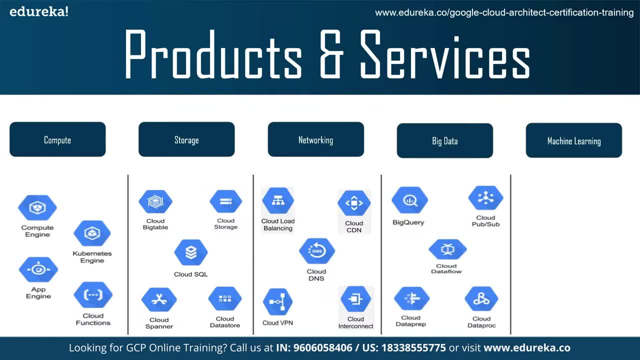 is like an intelligent cloud service to visually explore, clean and prepare data for analysis and machine learning. so now, moving on to the last one in the category, that is, a cloud data prop, which is a fully managed and highly scalable service for running apache spark, apache flink. 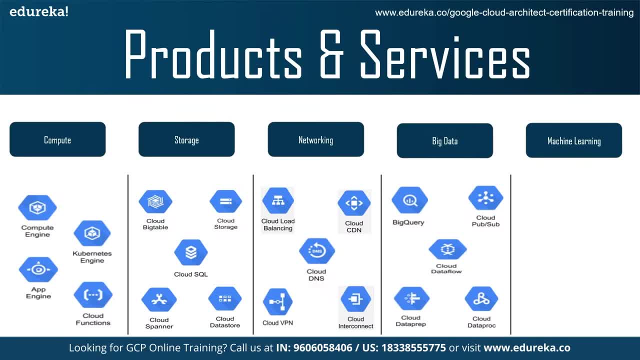 presto and 30 plus open source tools and frameworks. so use data proc for data lake modernization, etl and secure data science at planet scale, fully integrated with google cloud at a fraction of cost. now moving on to the last major product, that is, machine learning. 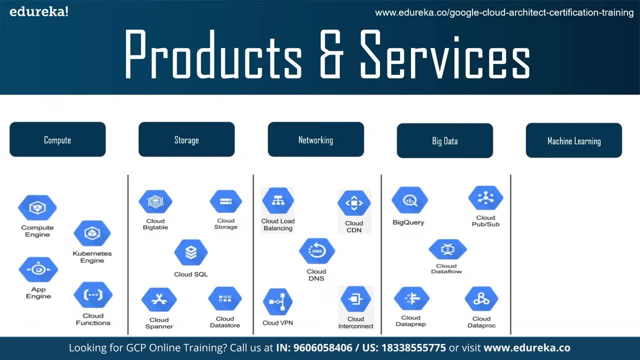 so google cloud platform provides several machine learning tools and products for developers, data scientists and data engineers to take their projects from ideation to deployment that took quickly and cost efficiently. so all the products under this are based on different auto machine learning models which are developed by google cloud platform and are 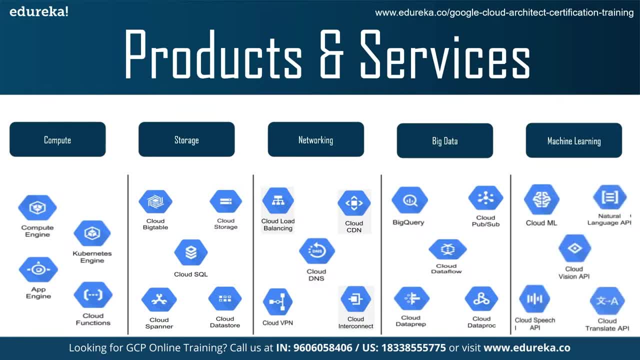 readily available. these are the subcategories of the products provided under machine learning. first in the category is google cloud ml engine, which is a hosted platform to run machine learning, training, jobs and predictions at scale. cloud ml engine automates all resource monitoring for running the jobs okay, so it can also manage the life cycle and deployed models and their versions. 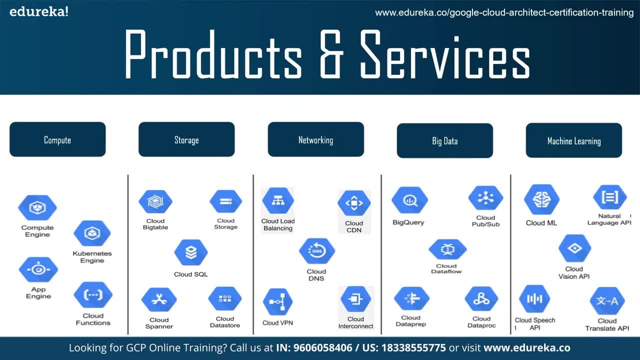 so moving on to the next one, that is, the natural language. api like this is a very famous product. okay, now moving on to the next one, which is like cloud vision api. so vision api and machine learning model helps you read images. so if i upload an image under vision api, by just reading that image, the 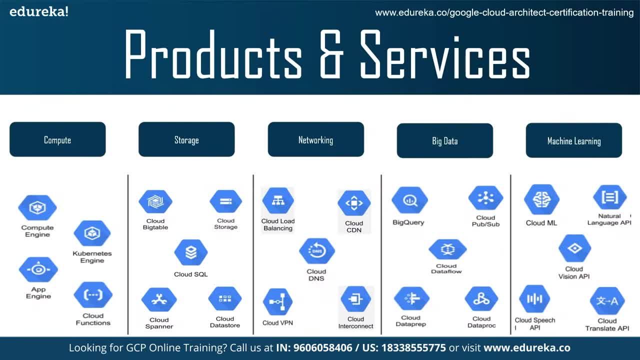 google cloud platform can help you identify the data points which can relate it to the particular image, so it's very efficient for image data processing. next is speech api, so this gains helps in converting your speech. so suppose someone is speaking and at the same time, you want a particular speech to be converted into a text. okay, then in. 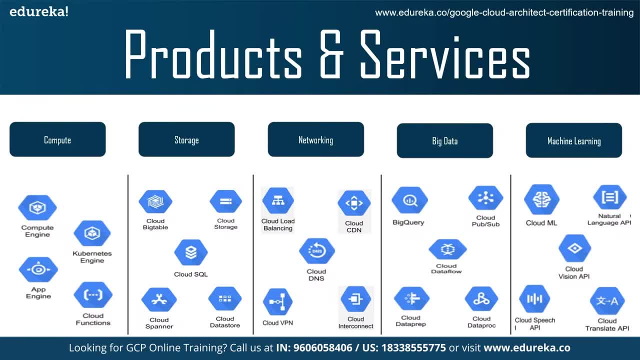 case, this particular api and ml model comes handy and it helps you do that analysis. now, moving on to the last one in the category, that is a translate api. so this helps you convert one particular language to another. suppose you have something written in japanese and you feed that. 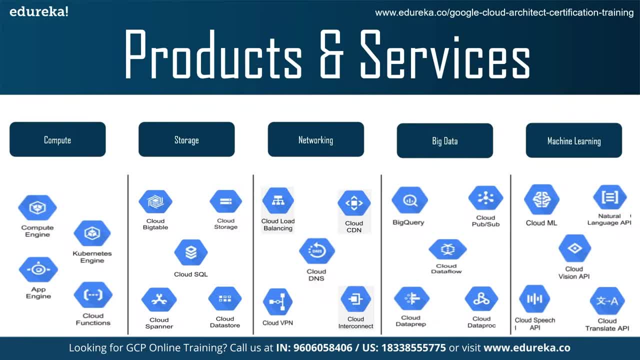 and translate api and it can get converted into english or any other language of your choice. okay, so all these machine learning models need data to train itself. remember that. okay, any machine learning model cannot work unless it has a training data and based on that only it can run those statistics and come out with some predictive analysis. 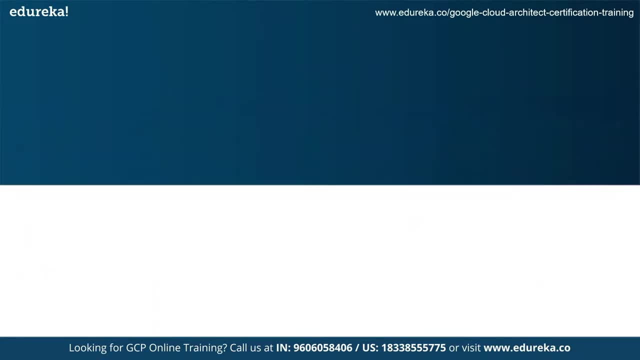 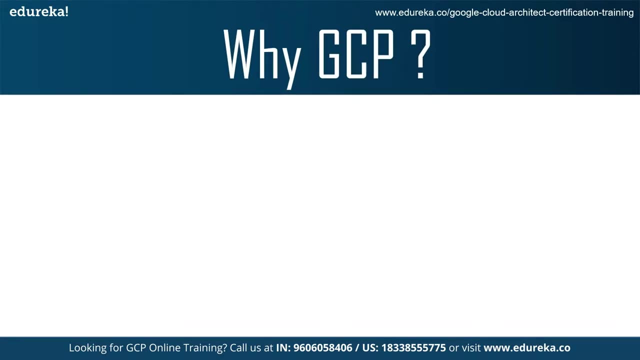 okay, i hope it's clear. now. the products and services. so now let's move on to understand why we should prefer google cloud platform. so now that you have a brief idea of what is cloud computing is and what is google cloud platform, let's understand why one must go for google cloud. 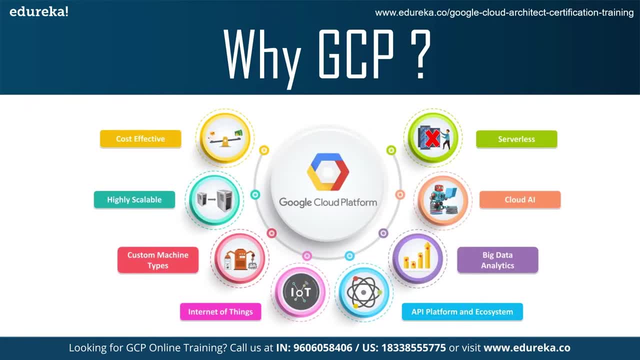 platform. we all know how big is the database of gmail, youtube and google search is, and i don't think in recent years google servers has gone down. it's actually one of the biggest in the world, so it seems an obvious choice to trust them right. so now let's take a. 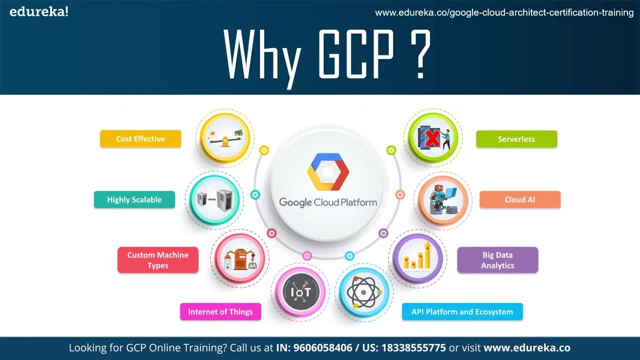 look at some of its features of google cloud platform. what really gives it an upper hand over other vendors? so first one is: it has a better pricing than its competitors. it is highly scalable and it uses auto scaling to automatically adjust the sum of virtual machine instances that are. 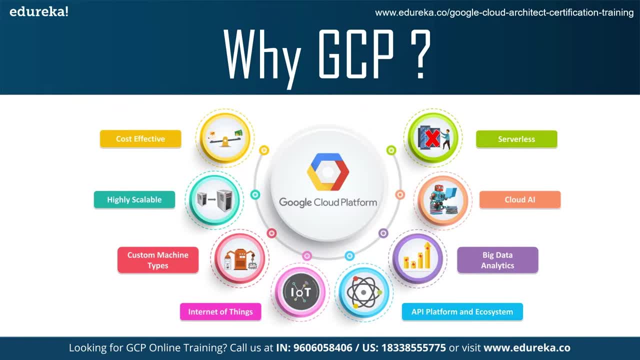 hosting your application. so what it does is it allows your application to adapt to different, varying amounts of traffic. now, if you see the third one, with custom machine types, you can create compute engine virtual machines with optimal amounts of virtual cpu and memory. now coming to google cloud's iot code, which is a fully managed service to easily and 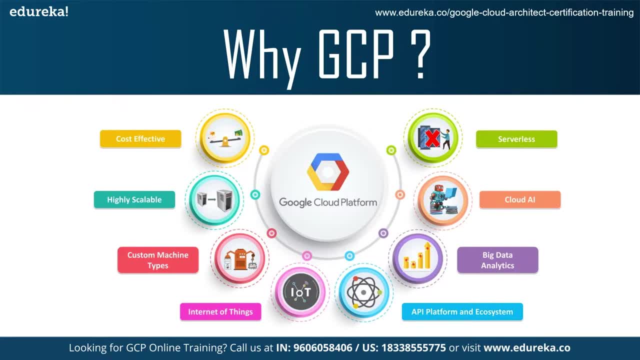 securely connect, manage and ingest data from globally dispersed devices, google cloud apis, if you see like they allow you to automate your workflows by using your favorite language. so this google cloud api ecosystem consists of compute api, storage api, big data analytics api, networking api and several, several others. now moving on to the sixth one, it is like 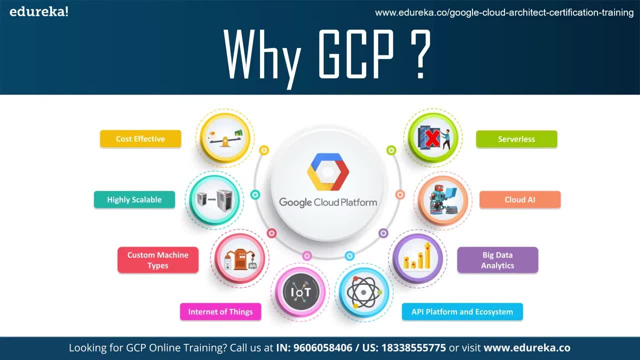 big data analytics, so google cloud smart analytics solutions are fully managed. this multi-cloud analytics platform empowers everyone to get insights while eliminating constraints of scale, performance and cost. big data analytics use real-time insights and data apps to drive decisions and innovation. with cloud ai, gcp cloud functions is the 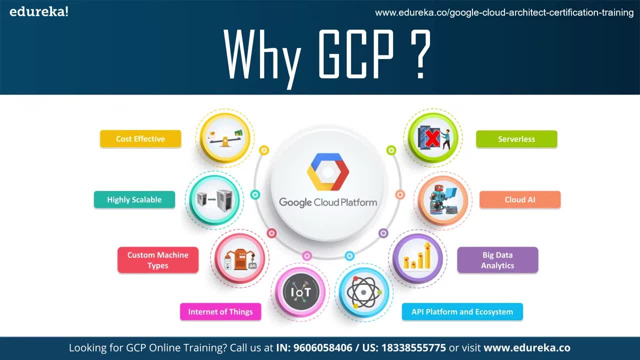 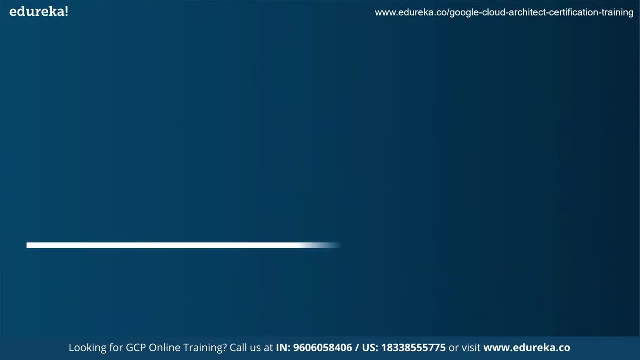 easiest way to run your code in the cloud. so, moving on to the last one, that is, serverless, google cloud platform is highly available and fault tolerant. let's now look at some popular advantages of google cloud platform. so first one is like: customers gets a higher time. 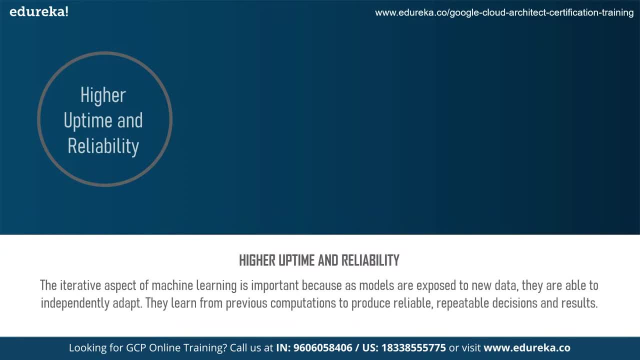 and reliability. if a data center is not available for some reason, the system immediately falls back onto the secondary center without any service interruption being visible to users. moving on to the next one: economic pricing. so google's economies of scale. let customers spend less, so it works in. 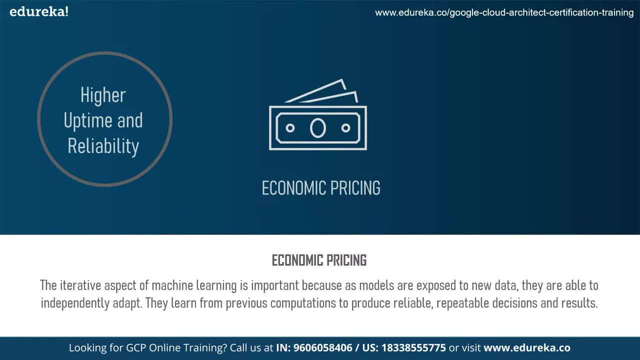 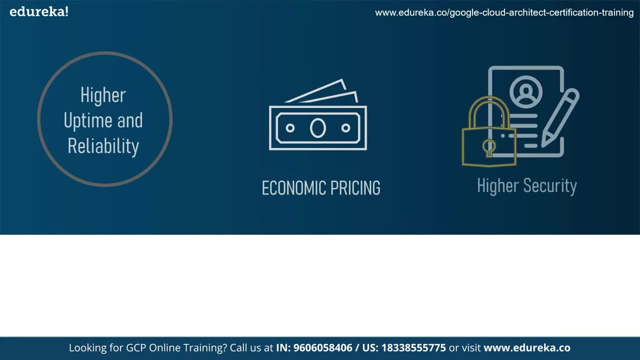 a way, like google, minimizes overheads and consolidates a small number of server configurations, which is these, through an efficient ratio of people to computers. now moving on to the last popular advantage, that is, of course, the higher security. so google's investments in security to protect. 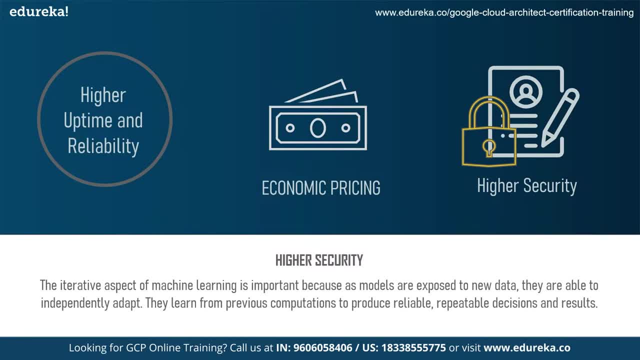 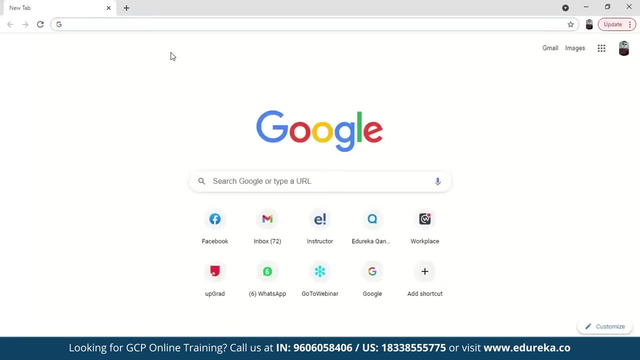 customers. so customer benefit from process based and physical security investments made by google. so google highest leading and security experts. that's how google provide a higher security to its customers. so let's take a quick demo now on google cloud platform. okay, so just simply go to google. 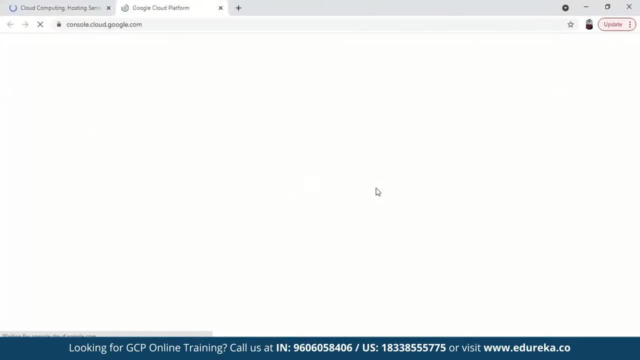 cloud platform and go to the console. what you can do is you can just directly go to the console. if you don't have an account on google cloud platform, then create one, because it's a good platform to have your account on, and it will ask for your credit and debit card details, while 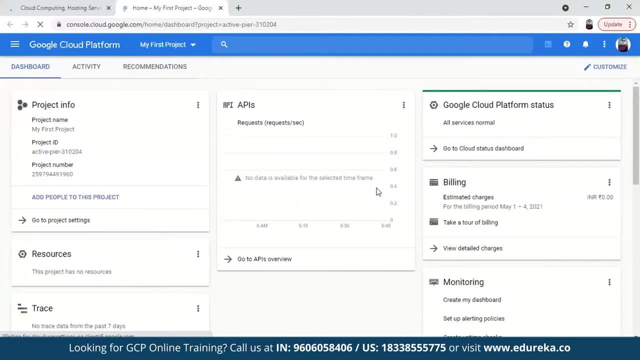 creating the account just for the verification purpose only. let me first introduce you to the platform that the google has to offer to us. okay, before that, remember one thing: like google cloud platform provides you like a free trial for like 90 days, okay, and it has certain limitations also. 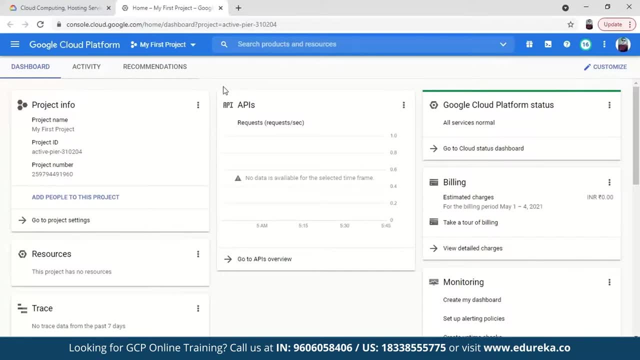 but if you like need the complete package and need complete access, then you can like go for a paid version also. so that's how it starts. this is how interface looks like. you can see there's a project information is here. like when you create the account, there will always be a inbuilt project will be there. but you can like go here to my first. 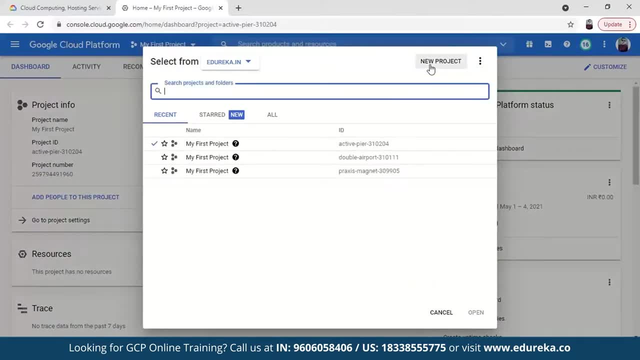 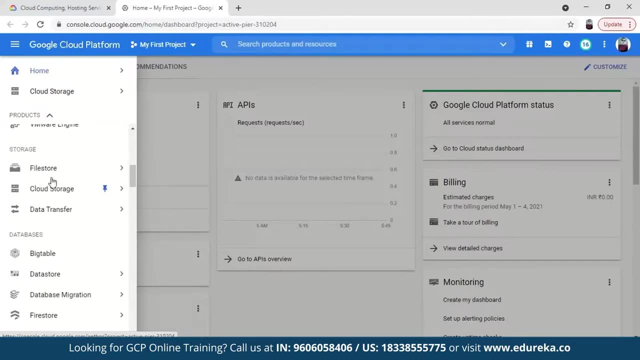 project and here you can like go to new project and you can create a new project with whatever name you want to give. okay, now coming to the dashboard. so i have like explained you previously right products and services. so here are like production services provided as of networking. 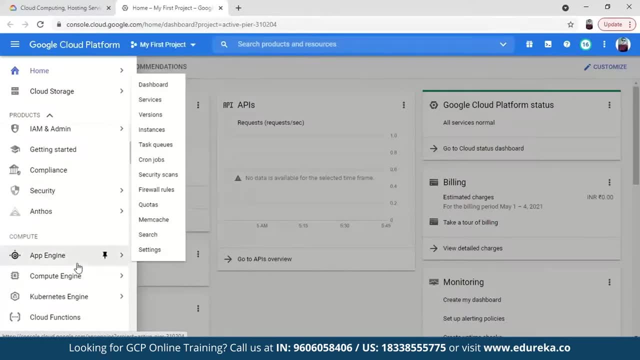 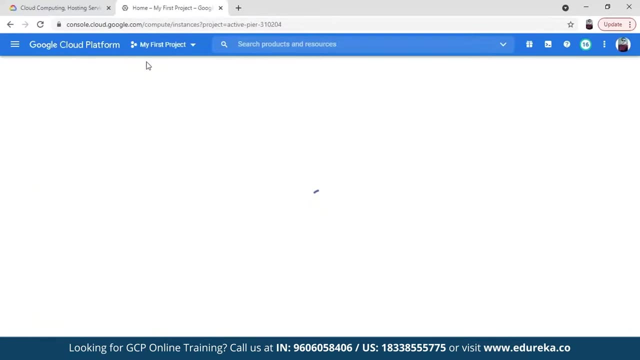 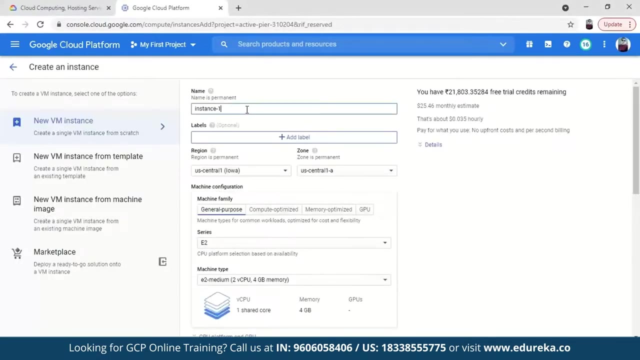 and of storage and of compute. okay, so let's see how to create an instance in google cloud platform. so just go to compute engine and you can go to vm instances. will take a little time, okay, so you can create an instance from here. you can like, name your instance whatever name you want to give to the instance. okay, 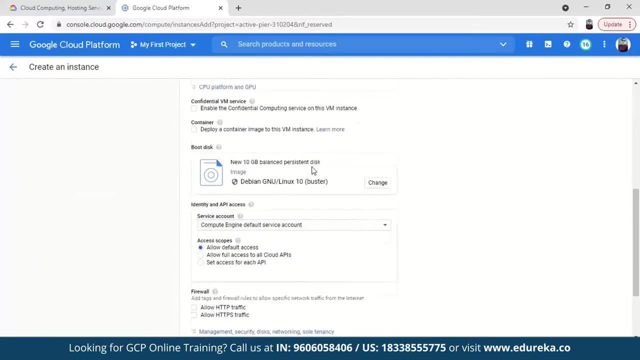 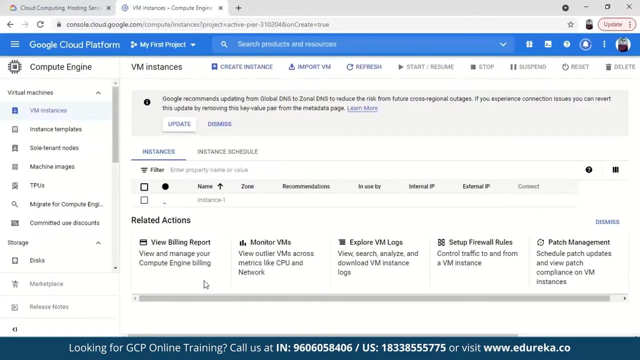 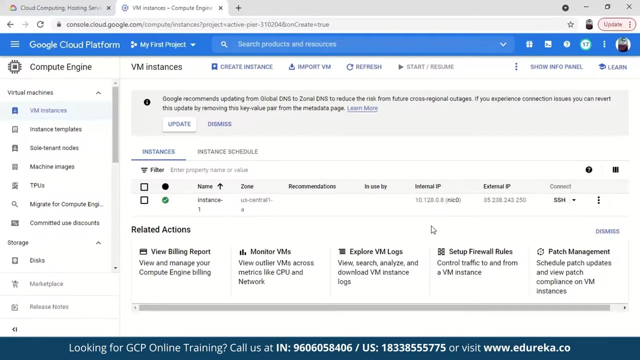 then you can fill in the details. if you want to do some customization, you can do from here and you can then just go as per your requirement, create it so the instance will be created. it will take a little time, but it will be created, so the instance is being created. so remember one thing: like, uh, as i have told you, like i have a free. 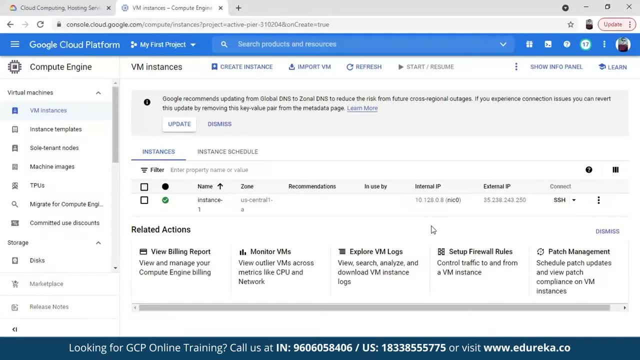 trial. so it has a little limitation, right. so here. limitation is that i cannot create an instance for windows from here. okay, i have a like window os, so for linus, always only. that's the limitation. so if you want to get it for the complete access for windows also so you can go for a paid version, okay. 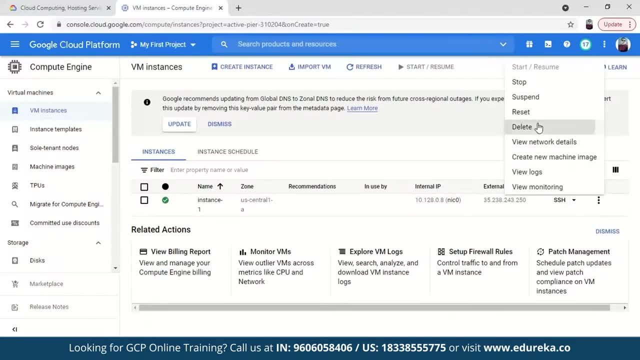 so right now i'm just deleting this. you can just go here and eat the instance. i am not able to launch it here. we can just go here and delete the instance. i am not able to launch it here. we can go to some other service and we can use that service of google cloud platform. not, if not the 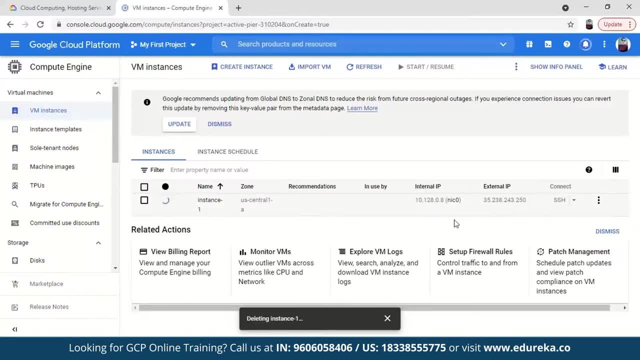 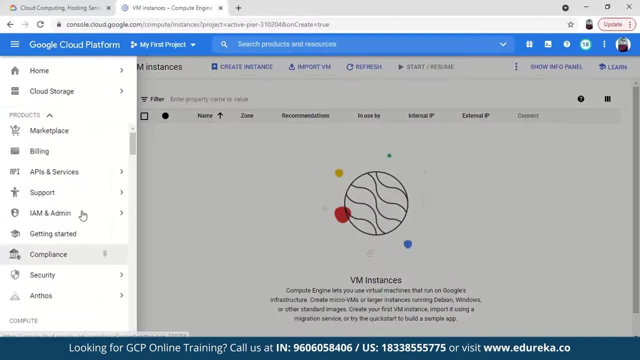 instance thing. you can go for the other one. let's just get this deleted. let it get deleted, takes a little time, so you can just go out of compute engine. we can use the service of a storage. okay, like we can store files or whatever kind of files you want to store, you can use the storage. 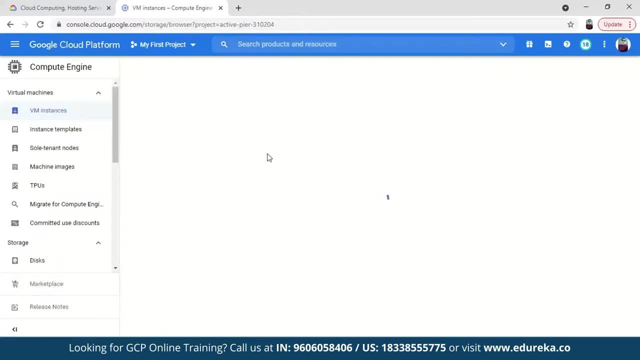 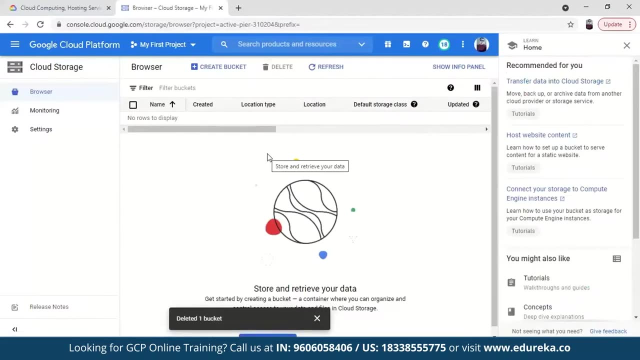 for that? okay, cloud storage. so yeah, remember, i have like explained you about storage. there is this, a bucket system in cloud storage. if you remember, like we have the drives in our laptop, we have folders and we can store files in that. similarly, here is the bucket system so you can. 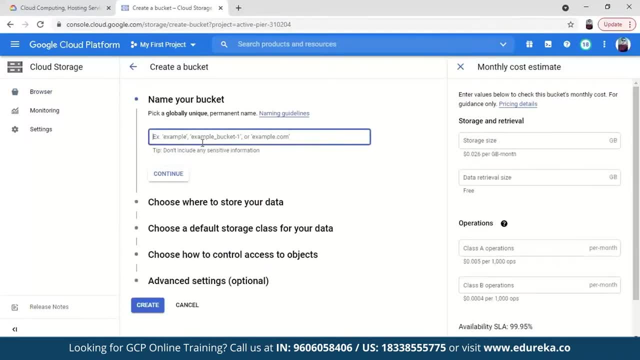 create a bucket from here and remember that, while naming the bucket, its name should be globally unique. okay, like the similar name of any bucket is there, like anywhere in the world they have created with the same name. then you can't create that. okay, use some unique word for that. okay, like. 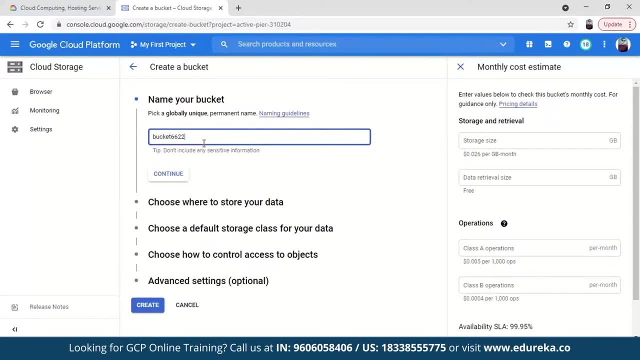 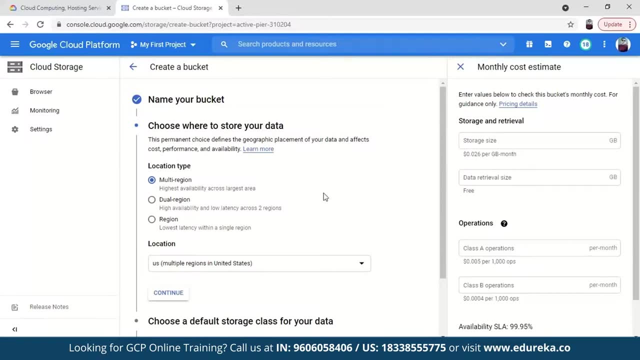 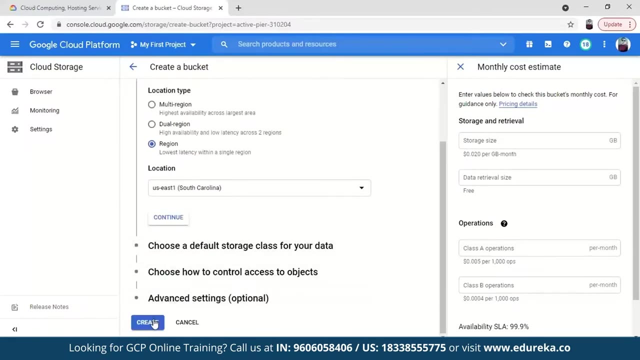 i am using here bucket 6622. okay, continue. so you can see like there is no bucket name 6622 here. you can see like there is no bucket name 6622. here you can see like there is no bucket name 6622. so here i am choosing single region and then i will just create it. it takes a little time, yeah. 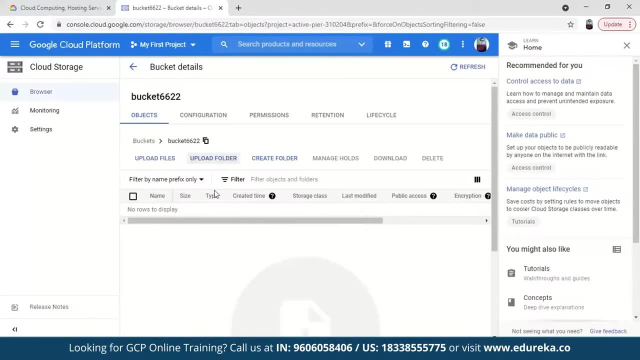 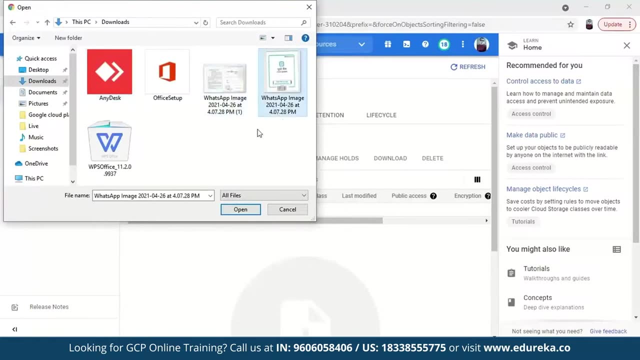 okay, done. so remember that here you can like create folder, upload folder, just like your hard drive. okay, or you can upload files. so let's upload a file. so this is like an exe file, this is an image file. whichever file you want to upload, you can upload. so, yeah, let's upload a exe file here. 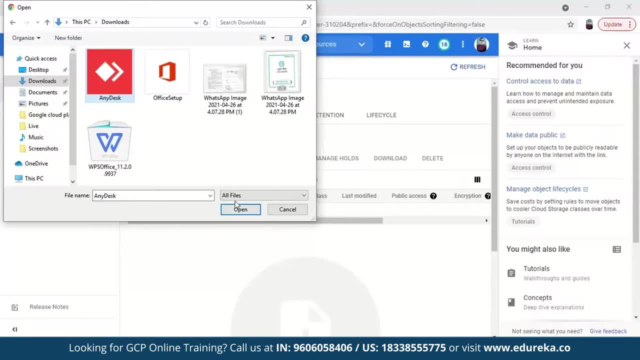 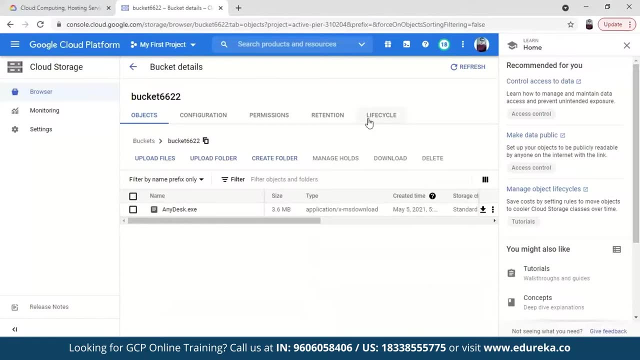 and any kind of like video file or any csv file, txt file, whatever kind of file. you can upload any file either. okay, yeah, so it got uploaded, and remember that this is the life cycle thing. okay, what you can do is retention permissions. everything is there. so in life cycle, what? 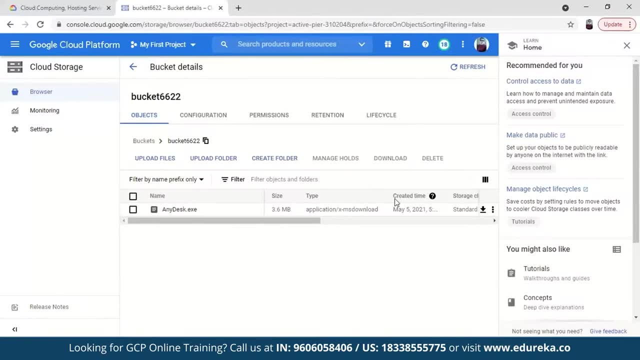 you can do is, uh, while you are storing a file or anything, any kind of file- but you feel like you want to delete it after 15 days or 30 days or any kind of days, any number of days. so you can go to life cycle and you can like choose its time period. okay, so what happens is if you forget, like you, 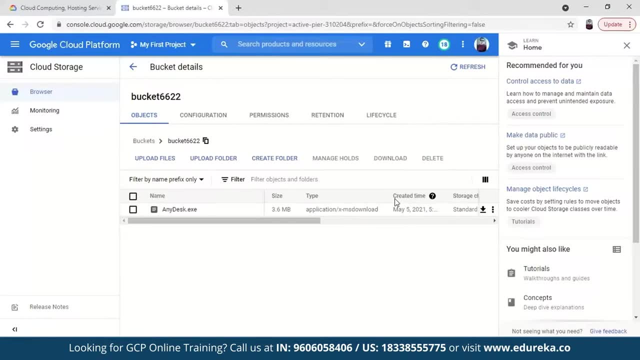 want to delete it, it will automatically get deleted after some days. so, given for 30 days or 15 days, it automatically get deleted in. also you can delete it from here like you can select it and you can delete it from here, or also you can download it if you want to download, whenever you want to download. 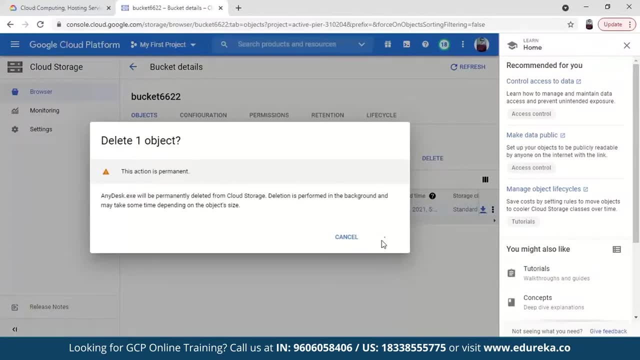 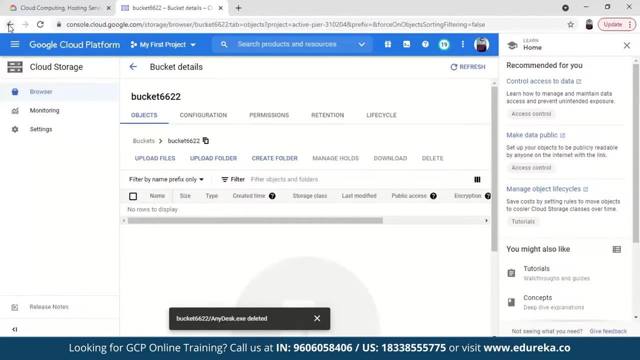 you can download it from the download option. now we are deleting it. so yeah, it's permanent action, so it's permanently got deleted. okay, also, if you want to like, delete the bucket also, you can just go back here, the bucket section. we can go. all the buckets are given. so here we have created. 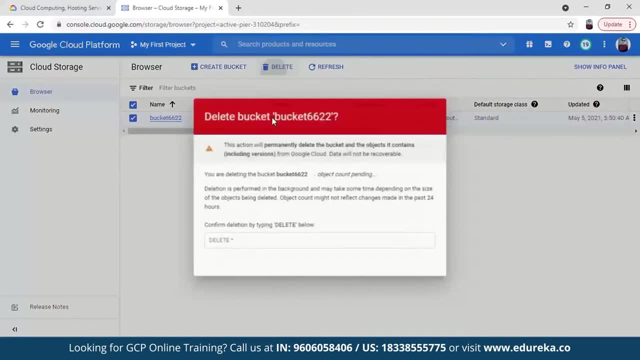 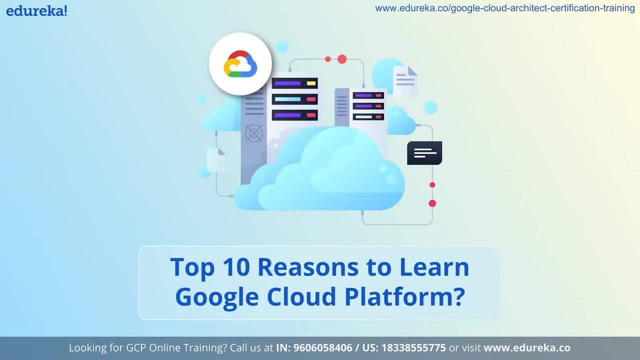 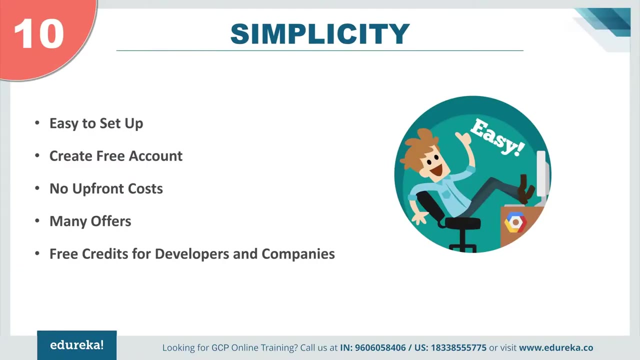 this bucket. we can just go select this and delete it. all you have to do is just click delete here, just delete it. so, starting at number 10, we have simplicity. now google has made setting up an account and using the google cloud services very easy. just by creating a google account, you can access the whole google cloud platform. 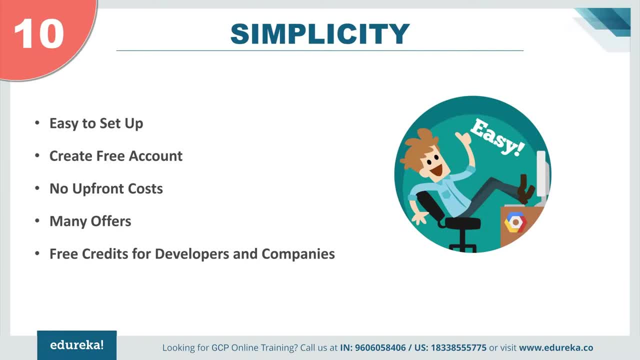 now, if you already have a google account, which i think most of you might be having, just go to cloudgooglecom and tap on the try for free button and you'll have the freedom to choose any of the services of the google cloud platform. there are no upfront costs required to use these services. 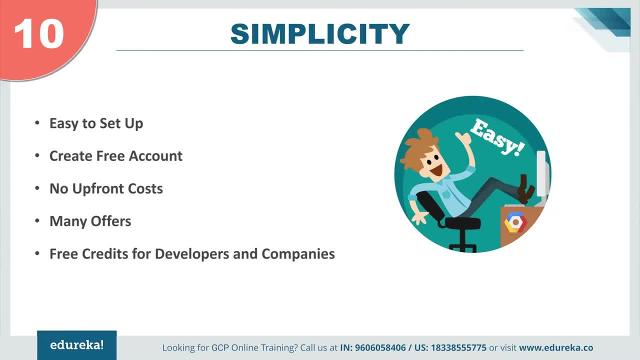 you get a 300 worth credit, which you can use over a time period of 12 months. now for startups, it's beneficial to work, play around and get to know the google cloud platform services before investing heavily in it, as they provide a hundred thousand dollars with credit for startups and $500 in credit for developers as well. 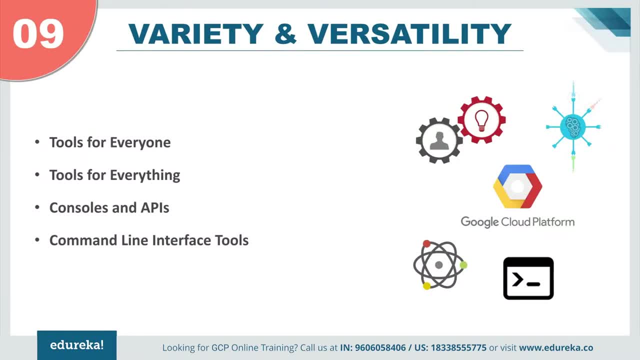 Coming up to reason number nine, we have variety and versatility. So once you get started on the Google Cloud platform, there are tools for everyone and for everything in the IT industry. Now you can use all these products for development, like the developers console, web UI and the command line interface tools. 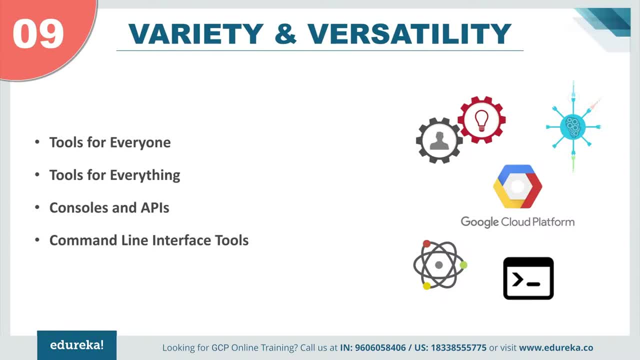 to work for the command line, Be it the Windows, Mac or the Linux environment. Now you also have the option to use the RESTful APIs. Now Google has its own set of managed APIs that can be used in different applications for different purposes. 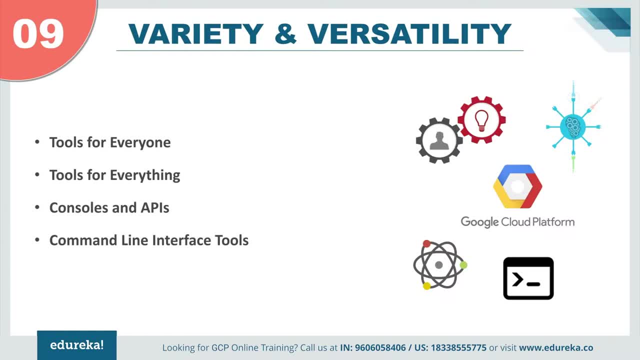 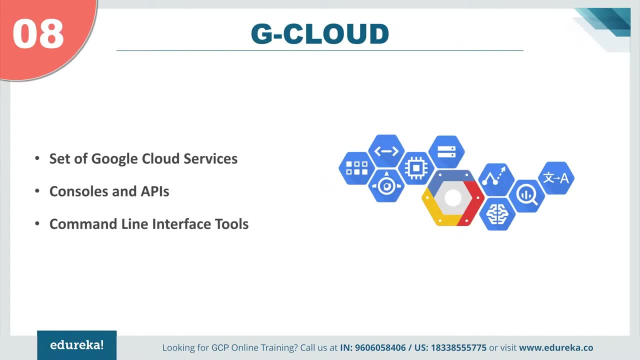 Now, needless to say that these APIs are very easy to work with. Coming up to reason number eight, we have the Google Cloud, which is the G Cloud. Now, G Cloud is basically the set of Google services Services that can be integrated with one another. 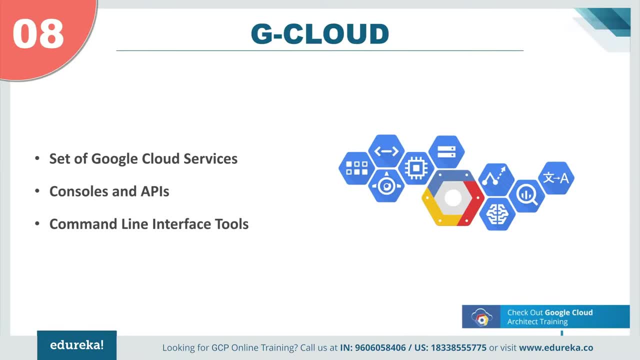 to create applications and run websites. Now. they are very easy to work with. You can use them separately as well as together for different types of applications, according to your needs. Now, Google stands out when compared to other cloud providers here, as they specialize in modularity. 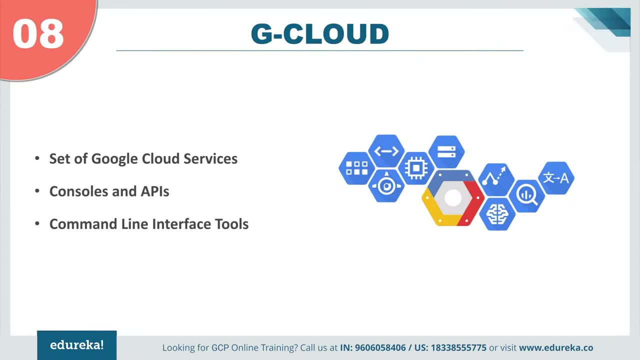 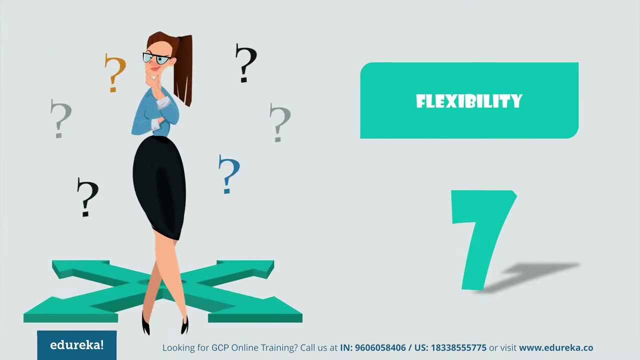 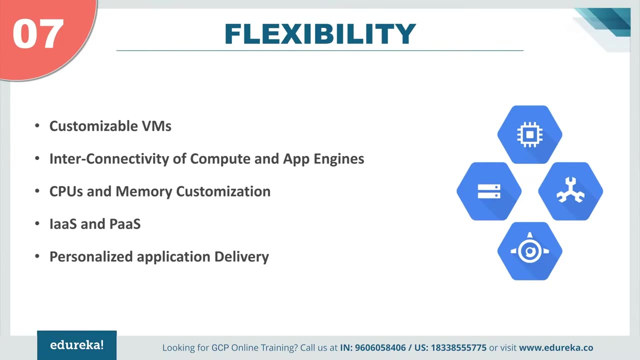 Now you can use these different pieces of the Google Cloud into various products, and you can mix and match these pieces according to your requirements. Now, at number seven, we have the flexibility. So custom machine types is a feature of Google Compute Engine that lets you easily create a machine type customized to your needs. 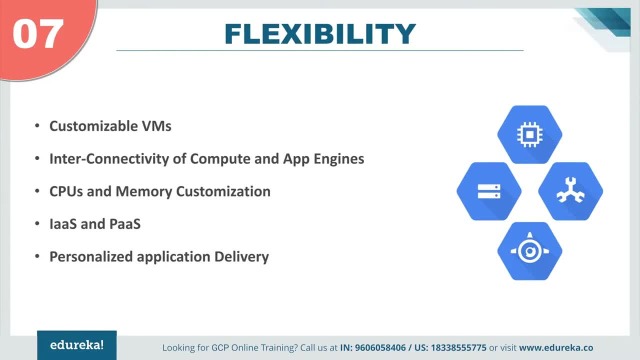 With custom machine types, you can create virtual machines with the optimal amount of CPU and the optimal amount of memory required for your workloads. Now you can create a machine type with as little as one virtual CPU to as much as 64 virtual CPUs. 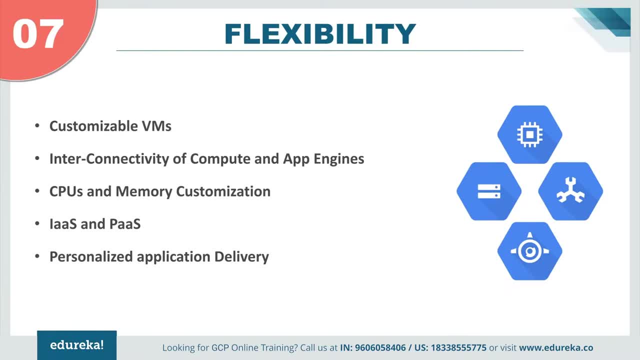 With Compute Engine, you are getting infrastructure as a service and with App Engine, you're getting platform as a service, all under one roof of Google Cloud. Now, the flexibility of the Compute and the App Engine allows to create a fully managed, customizable machine which can be scaled up or down. 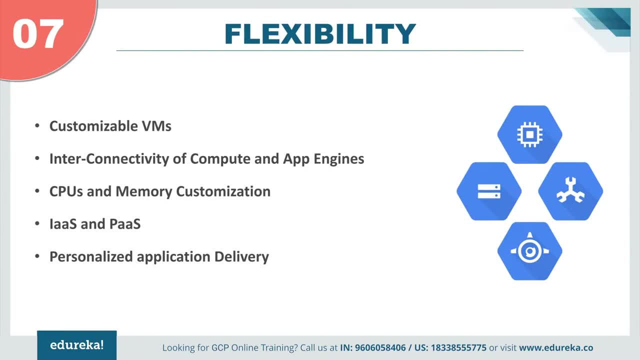 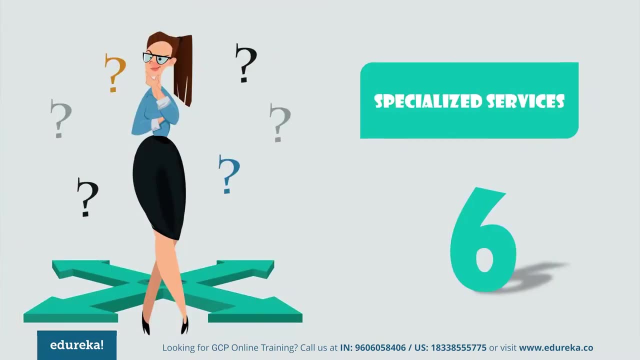 according to the traffic it receives or according to our requirements. So we can say that they are breaking down the barriers of the infrastructure as a service and platform as a service by bringing them together all along, making things simpler for us as well. Now coming to number six. 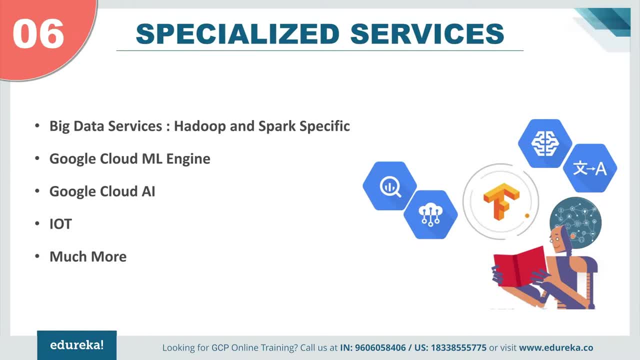 we have the big data, machine learning and the artificial intelligence services. A Google Cloud platform provides fully managed data warehousing facility with batch and stream processing, along with added Hadoop and sparse specific configurations. Now GCP has an IoT specific intelligent platform that unlocks business insights. 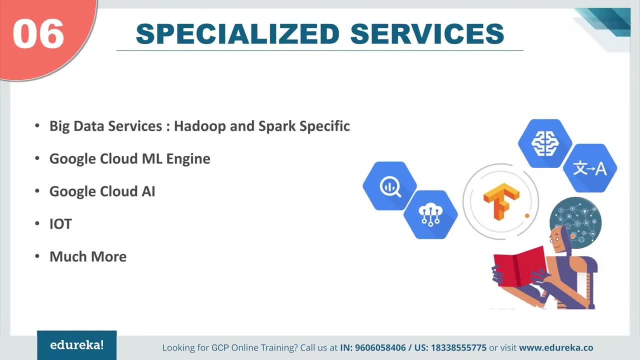 from your global device network. Google Cloud's artificial intelligence provides model machine learning services with pre-trained models and a service to generate your own tailored models as well. Their neural net based machine learning service has better training performance and increased accuracy as compared to other large-scale deep learning system. 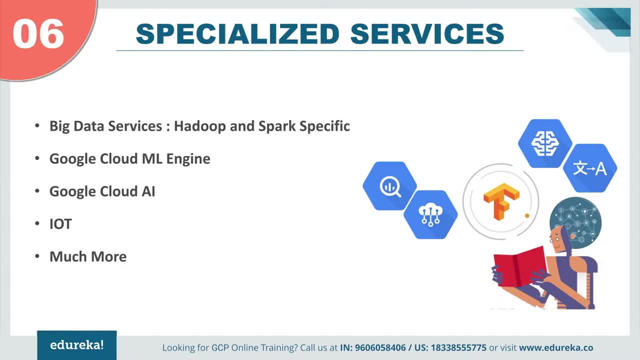 And with the introduction of TensorFlow, everything we do on the machine learning engine is taken up to a whole another level. Their services are fast, scalable and very easy to use. Now major Google applications use cloud machine learning, including the photos We have: image search, the Google app. 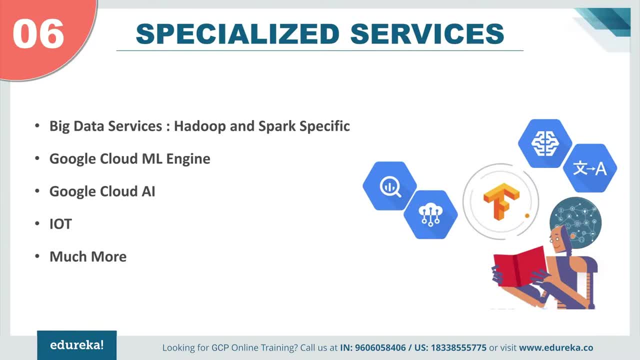 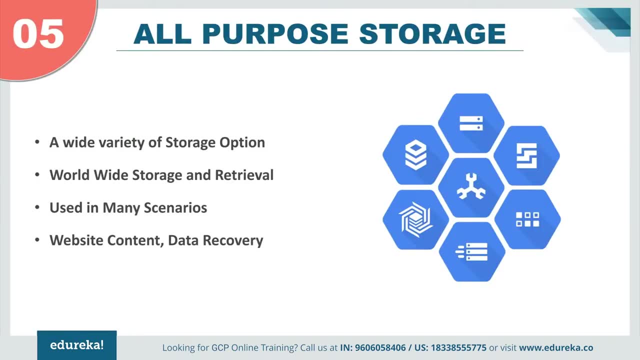 which is the voice search. We have translate and inbox reply, which is the smart reply. Now, coming up to reason number five, we have storage and database option. Now, Google Cloud storage is a set of various storage services offered by Google for different domain scenarios. 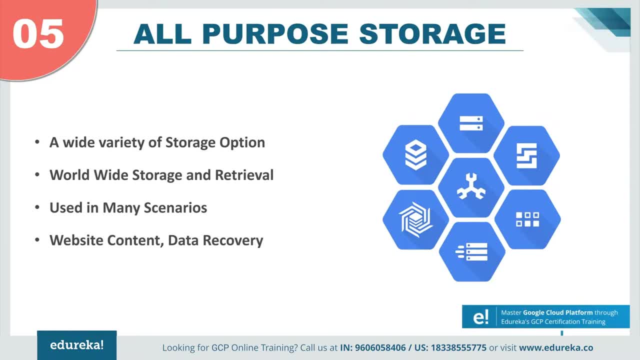 It allows worldwide Storage and retrieval of any amount of data at any time. They can use this cloud storage services for a range of scenarios, including serving website content, storing data for archival and disaster recovery, or distributing glass data objects to users via direct download. Now here we have so many options like the cloud sequel, the cloud big table, cloud data. 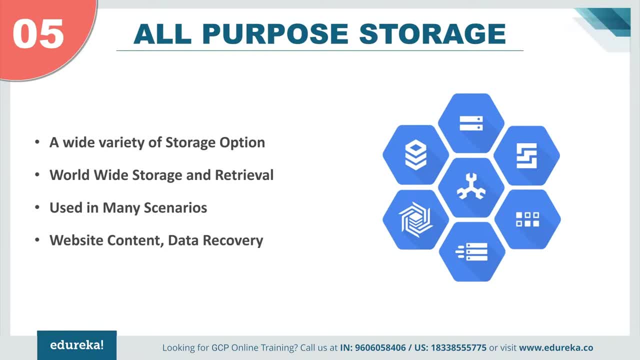 So persistent disk, cloud, BigQuery and there are many other more options. The cloud sequel is used for my sequel and PostgreSQL big table is used for scalable No sequel databases. Now data stores is the document oriented database as a service. persistent Disk is a high-performance block storage. 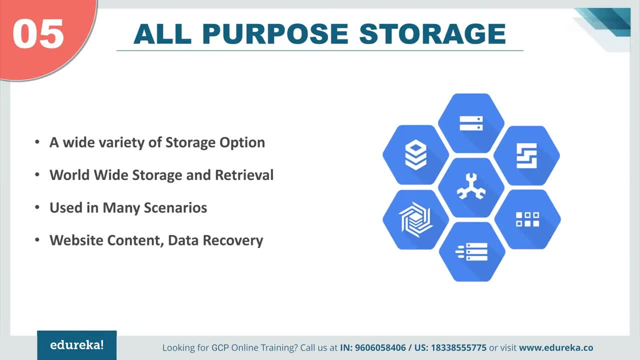 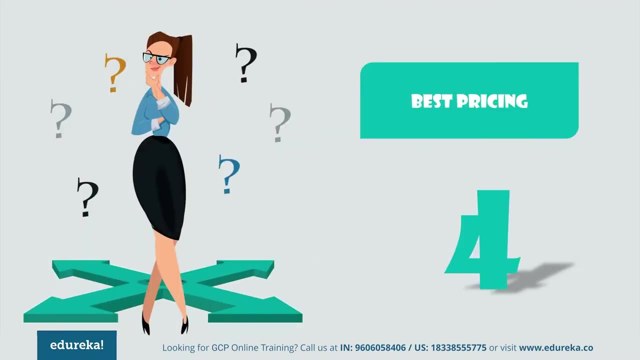 which is very suitable for the virtual machines and the container storage. Now BigQuery is Google's fully managed, low-cost analytics data warehouse. So you can see here that Google has mastered this storage domain and no one can defeat them here Now. reason number four is pricing. 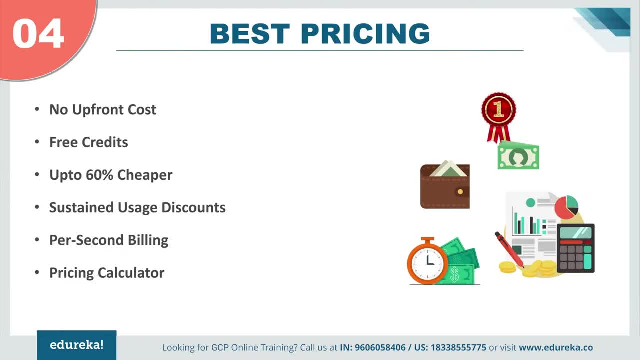 This is another domain where Google is way ahead than other cloud providers. They have no upfront cost required to set up an account or use these services. They also provide lots of free credits to explore these services. on an average, It is 60% cheaper as compared to the other cloud providers. 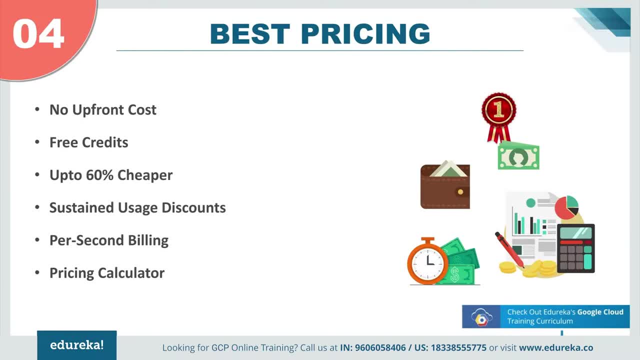 Plus, if you use the services for a longer period of time, Google also provides discounts. The billing is done on a per second basis, which is how a cloud service should work. The- finally, the most amazing feature is the price calculator, which you can use to find out the estimate of the services that you are going to use. 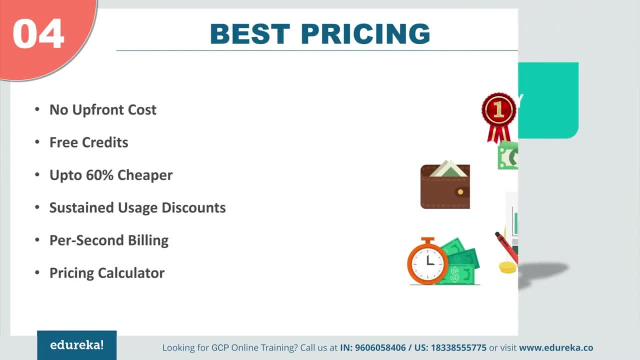 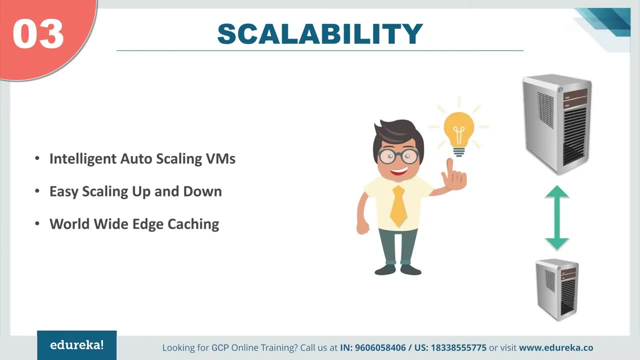 so that they aren't any shocking bills or invoices later. So, coming down to the top three reasons, at number three we have scalability. You can easily scale up or down your machines depending upon your requirements. Everything is made simpler by Google plus. the Google VMS are auto scalable. 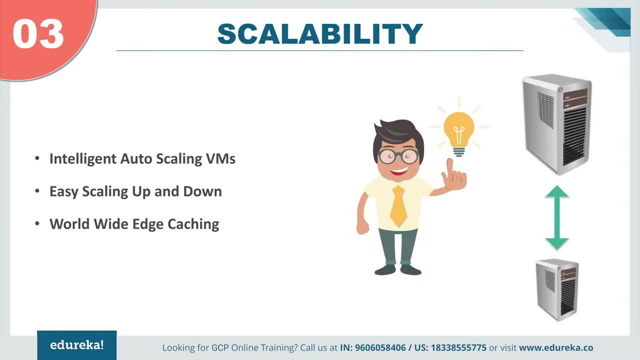 They have auto scale, of which scales up or down your instances according to the traffic It receives all along, saving money for you and making tasks simpler as well. So this is really a cool feature, as it decreases the overhead and also the engagement effort required for this job. 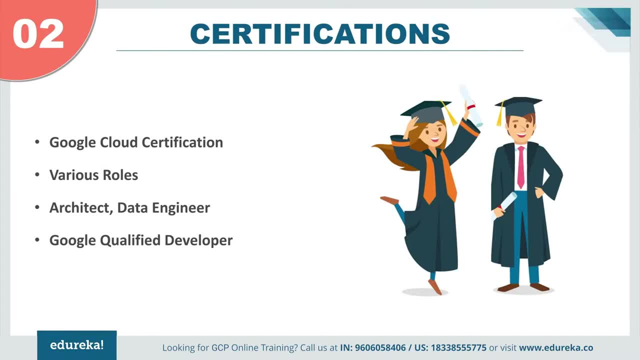 At number two, we have the certifications. Now, Google provides lots of certifications that are very important and very useful If you are looking for a good certification in the cloud Department. they provide four types of cloud certification, which are: the professional cloud architect. the professional data engineer. 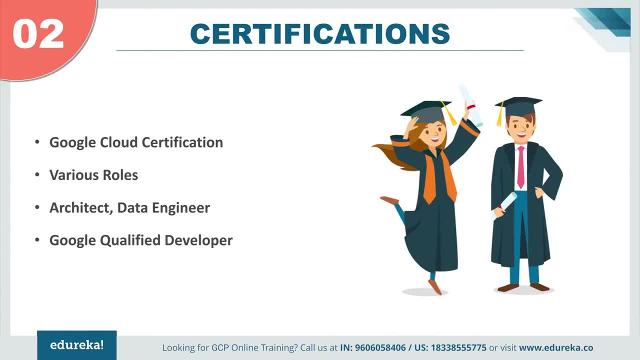 the G Suite administrator and the G Suite Now. these certifications are very good for people who are working in the cloud industry. apart from these certification, They also provide the Google qualified developer certifications. So in order to get certified, you need to clear these four exams. 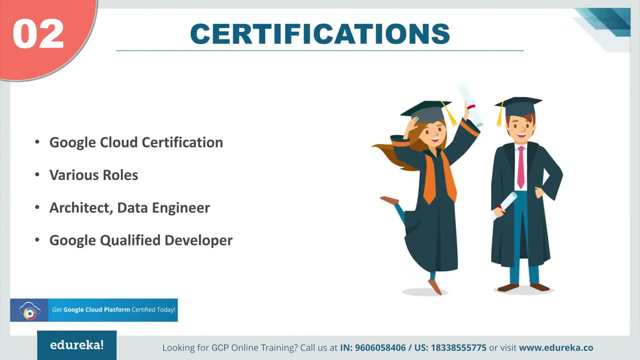 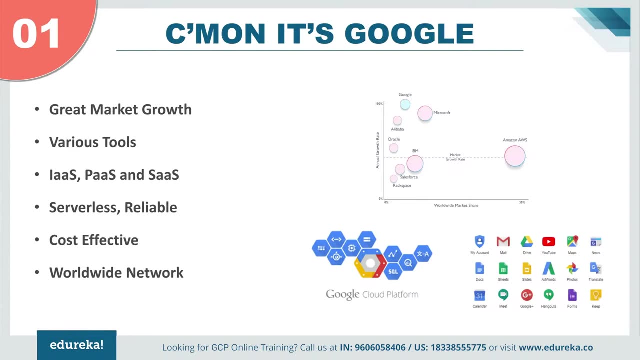 which are the app engine exam, the cloud storage exam, the compute engine exam. Clearing all these exams will certainly provide you with an upper hand over the others while applying for a job anywhere. Now coming down to our top reason, Come on. 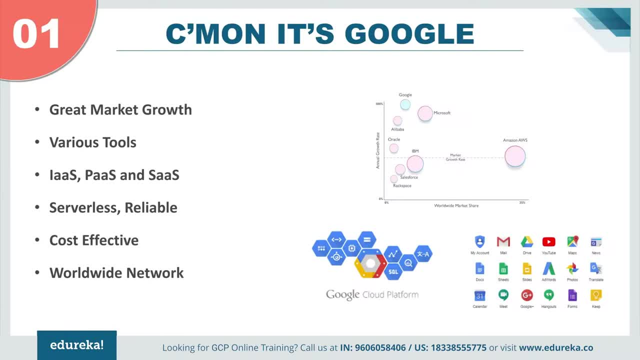 It's Google. We all know how big is the database of Gmail, YouTube and the Google search and I don't think in the recent years Google Server has ever gone Down. It is one of the biggest company in the world and the worldwide Network is phenomenal. 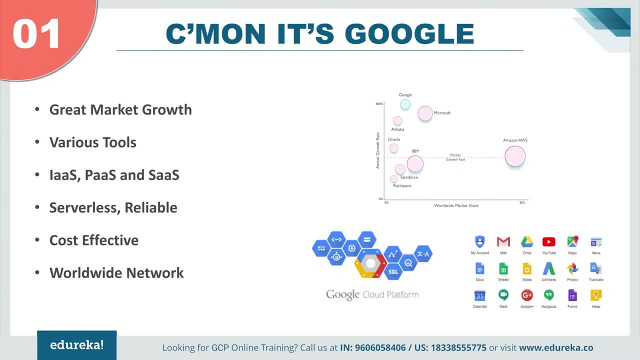 You get everything you expect from Google: It's reliability, scalability, the infrastructure and lots more. you get everything under one roof and managing services is really, really easy. You can think of it as working alongside the world leaders in innovation and technology. So, as I mentioned earlier, 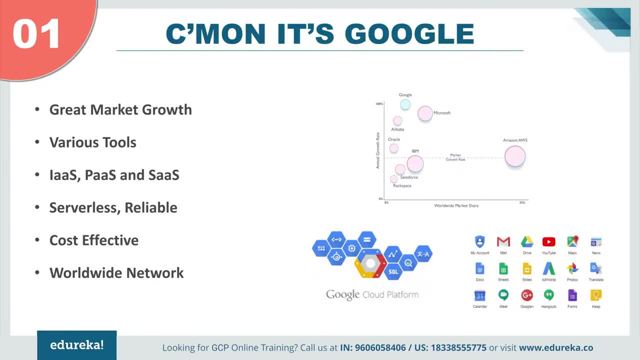 they are so cost-effective and reliable and also they are serverless, which means You do not need to manage the servers. Everything is taken care of by Google. and, most importantly, being a little new to this cloud market, The annual growth rate are off charts already. 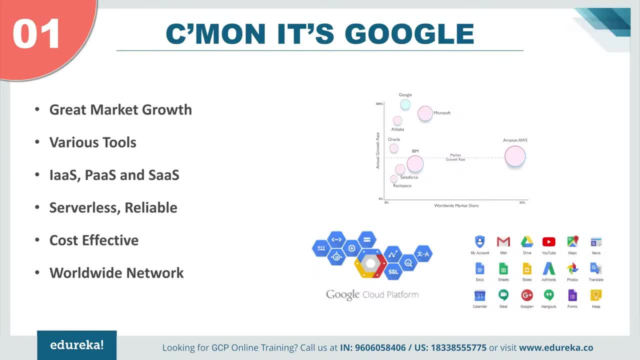 I is over 100%. now You can also relate it to the amount of services provided by Google for its normal Gmail users, which is YouTube, the Google Mail, the Google Drive. We have Maps, sheets, translates, Hangouts, and the list goes on and on. 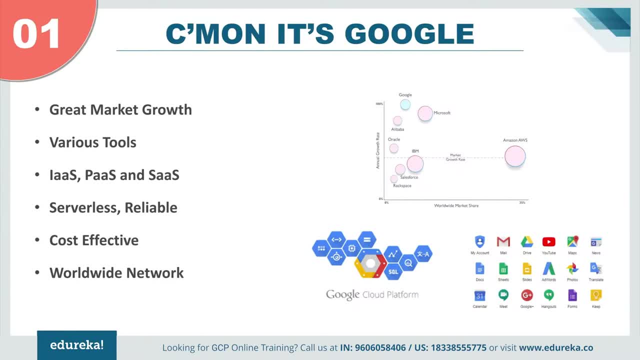 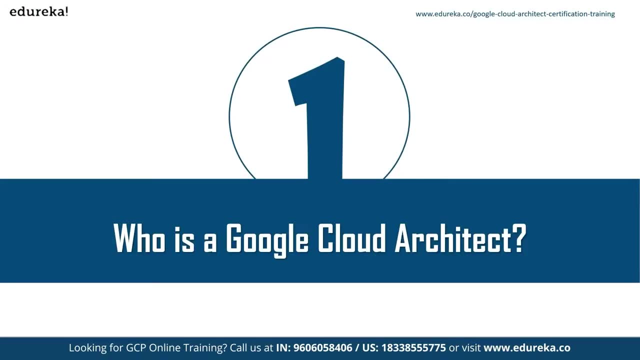 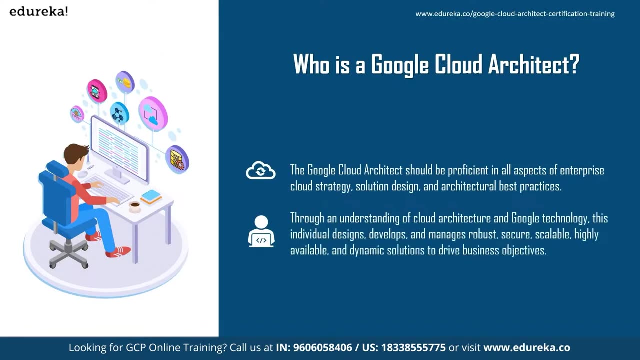 So you did not worry about the quality of the services provided by Google. Who is the Google cloud architect? A Google cloud certified professional cloud architect enables organization to leverage Google cloud technologies through an understanding of Google technology and cloud architecture. The individual designs, develops and manages robust, secure, scalable, highly available and dynamic solutions to drive business. 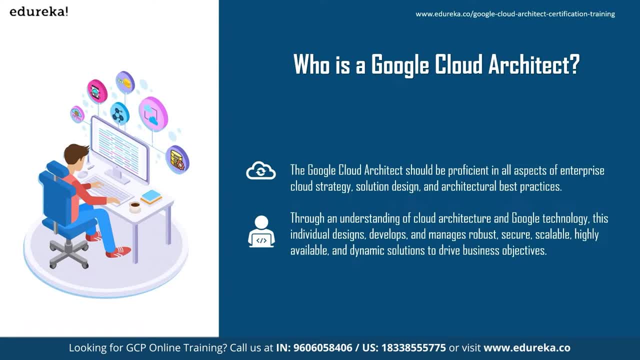 Objectives: The cloud architect should be proficient in all aspects of Enterprise cloud strategy, solution design and architectural best practices. Also, the cloud architect should be experienced in software development methodologies and approaches, including multi-tiered distributed applications which span multi-cloud or hybrid environments. 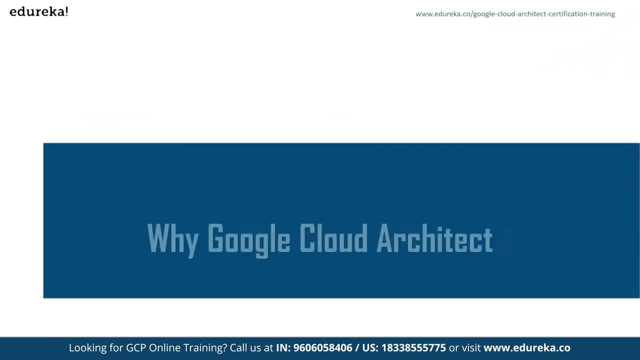 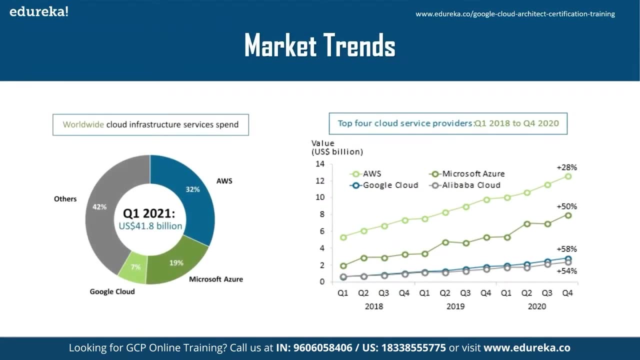 Now that you have understood who is a Google cloud architect, Let's understand why there's a need for Google cloud architect. First of all, let's look at the market trends for Google cloud platform. If you see for the first pie chart in this, you can see like the data is for quarter one of 2021, where we can see the top three cloud service providers. 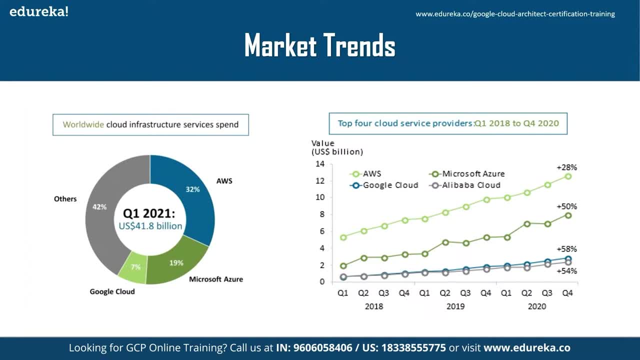 Like the first one. you can see the AWS- 32% market share, and then Microsoft Azure for 19% and Google cloud for 7%, and then there are various others and make a lot of cloud service providers, which constitutes to 42% of the market share. 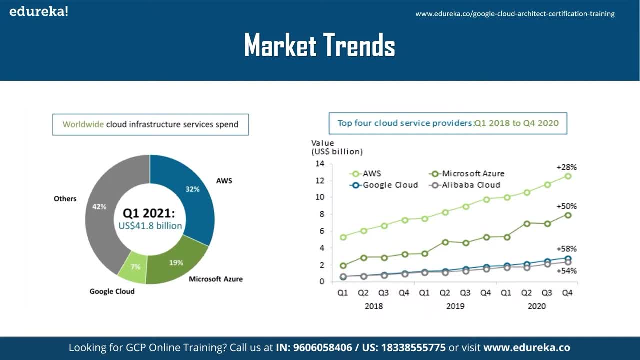 Now, if you see, AWS is actually the biggest cloud player because it was launched like way back in 2004, and after that Microsoft Azure and then after that Google cloud in 2010 was launched. But if you see, like initially it wasn't that much growing. but if you see, in the last three years, 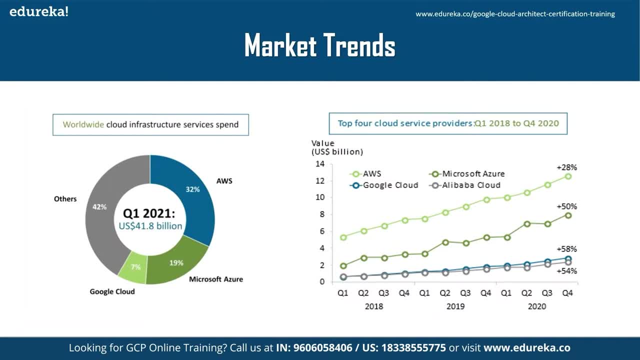 if you see the second graph from quarter one 2018 to the quarter of 2020,, you can see that AWS has 28% surge in market and then Azure has 50%, where Alibaba cloud has 54% and the highest You can see. 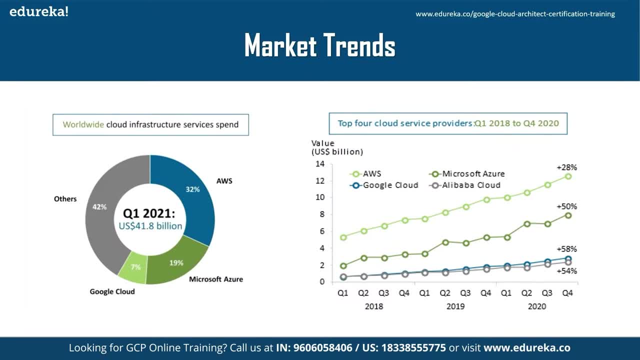 is of Google cloud, which is 58%, and Google cloud is that's how grabbing the market like aggressively. It's because of its various services, like ML and AI also, and of cloud AI, like various big query services. These are like the unique services to Google cloud provide. 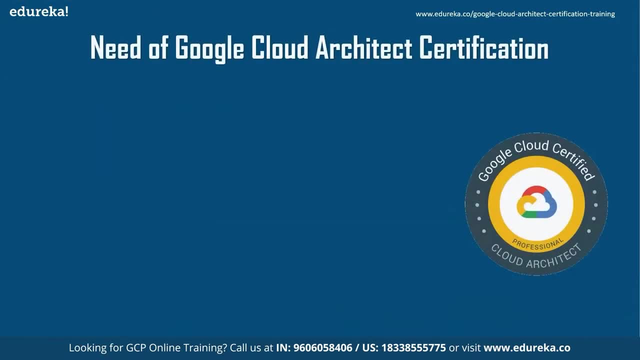 We will talk about it later on. Okay, now let's talk about the need of Google cloud architect certification. So the Google cloud certification validator expertise and showcase your ability to transform with Google cloud technology. And it enables organization to leverage Google cloud technologies. 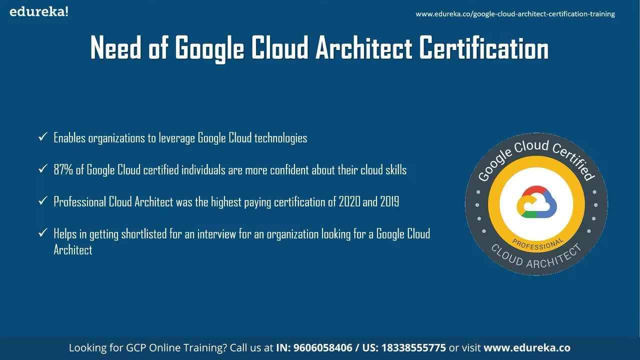 Also, like 87% of the Google cloud certified individuals are more confident about their cloud skills and professional cloud architect was the highest-paying certification of 2020- 2019.. More than one in four of Google cloud certified individuals took on more responsibility or leadership roles at work. 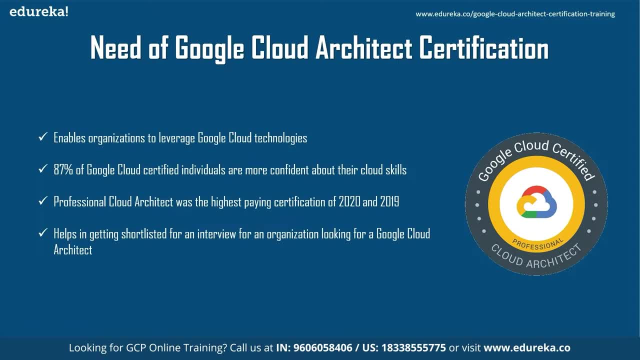 Also one of the major factor of Google cloud architect certification. It helps in getting the candidate shortlisted in the company which is looking for a cloud architect. So this first of all they what they see in a resume is whether you have a Google cloud architect certification or not. 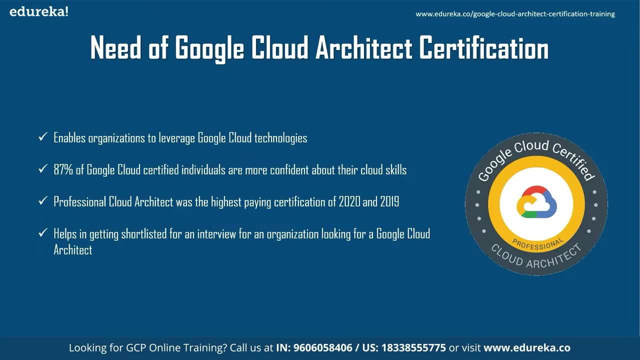 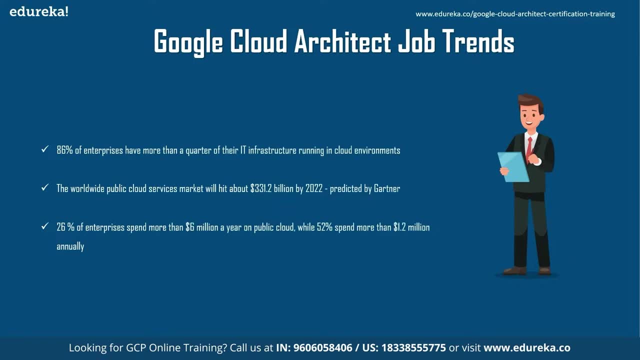 If you have it, then you will get shortlisted for sure. That's the major needs of a Google cloud architect certification. Now let's look at the job trends for Google cloud architect. So if you look at the IT sector, 86% of the enterprises have more than a quarter of the IT infrastructure running in cloud environments. 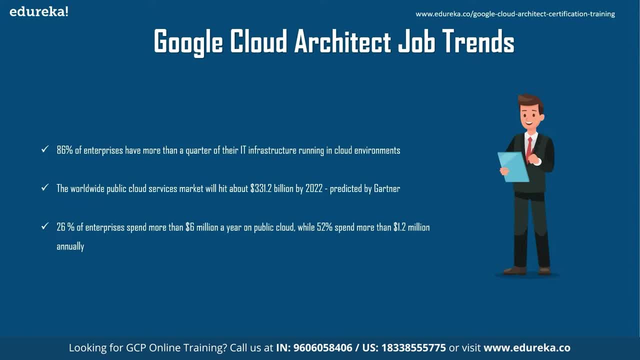 And, according to the study done by Gartner, the public cloud services market will like hit 12%- about 31.2 billion dollar- by 2022, and 52% of the enterprises spend more than 1.2 million dollar annually on public cloud, as well as 26% of the enterprises spend more than 6 million dollar, which is like really huge. 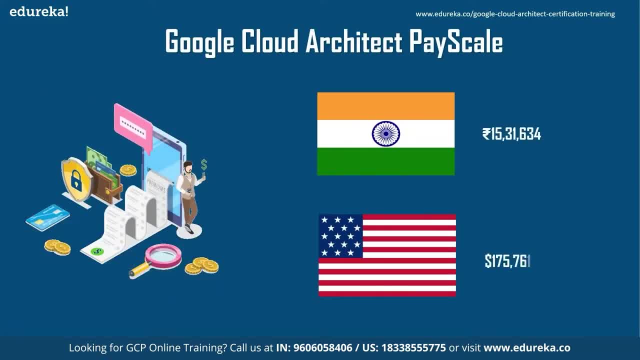 Now let's look at the salary, or say pay scale, for a Google cloud architect. So, according to global knowledge, the average pay for a Google cloud architect in India is 15.3 lakhs, Whereas in US it is 175,000 US dollars. 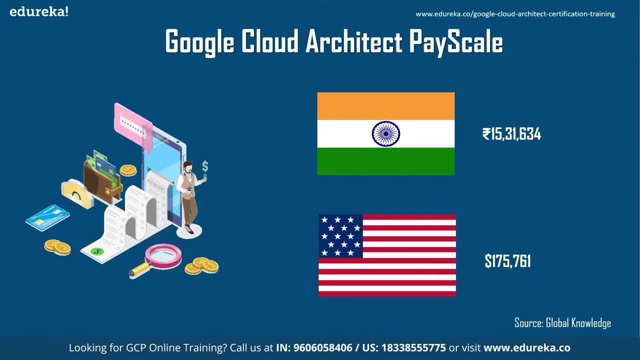 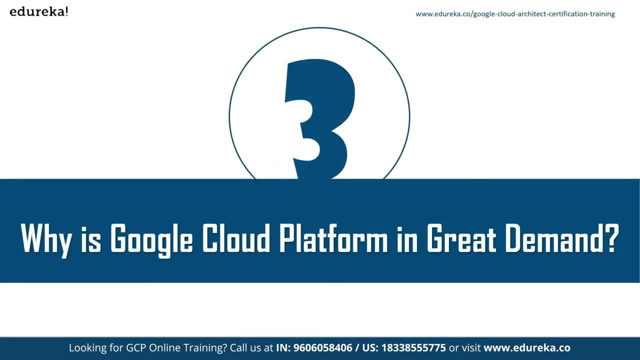 which is, you can Understand, like a very high scale salary has been provided to Google cloud architects. Now let's understand why Google cloud platform is in great demand. We all know how big the database of Gmail, YouTube and Google search is and I don't think in recent years, 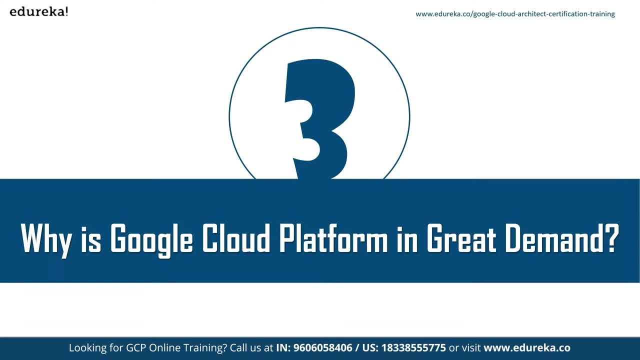 Google server has gone down. It's actually one of the biggest in the world, So it seems an obvious choice to trust them right. So now let's look at what really gives Google cloud an upper hand over other vendors. The first of all. 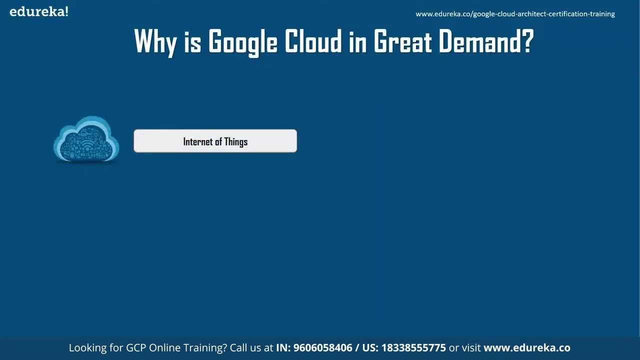 the major advantage Google cloud has is of Google clouds IOT, which is a fully managed service to easily and securely connect, manage and ingest data from globally dispersed devices. Also, Google cloud has a better pricing than its competitors, which means it's cost effective. 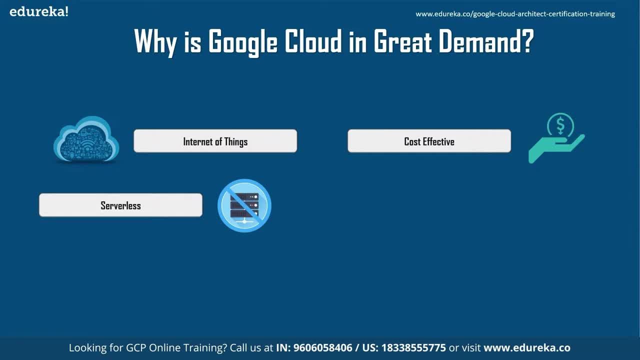 Third, due to serverless computing, it is highly available and fault tolerant. With cloud AI, cloud functions in GCP is the easiest way to run your code in the cloud, integrated with machine learning technologies. Also, it is highly scalable as it uses auto scaling to 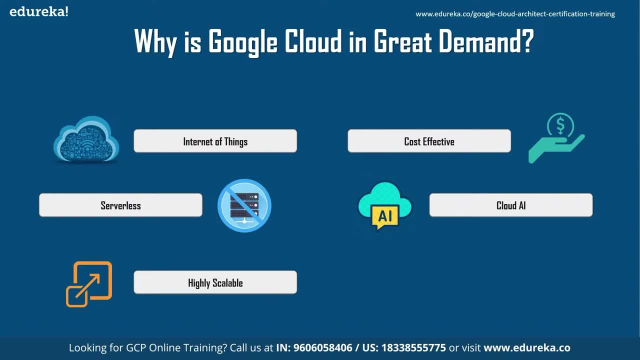 automatically adjust the number of virtual machine instances that are hosting your application. So what it does is it allows your application to adapt to different, varying amounts of traffic. Lastly, Google cloud smart analytics solutions are fully managed means big data analytics solutions. This multicloud analytics platform empowers everyone to get insights while eliminating constraints of scale. 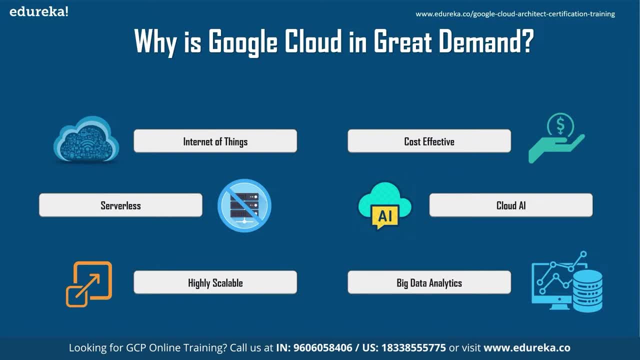 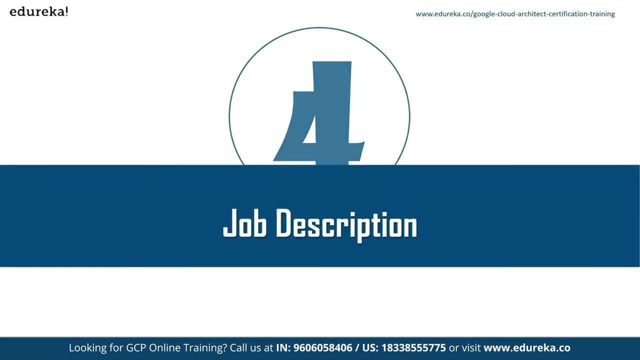 performance and cost. It uses real-time insights and data apps to drive decisions and innovation. Now let's look at the job description of a Google cloud architect. So you can see here the job description of a Google cloud technical architect of Accenture company. 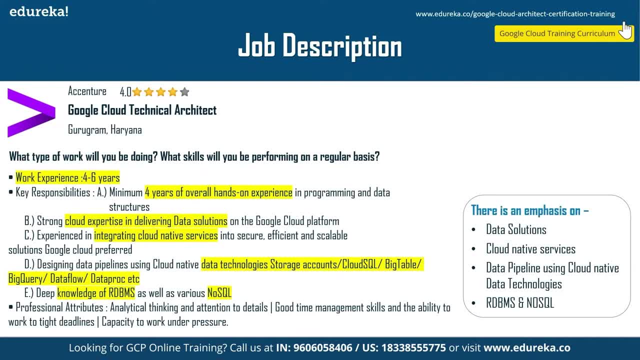 and the location you can see is Gurugram Haryana. So now let's understand what type of work will be required by the company and what skills will you be performing on a regular basis? So the work experience, first of all, is required: four to six years. 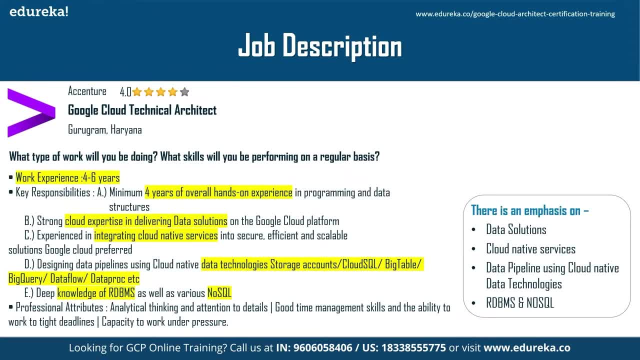 a minimum of four years of overall hands-on experience in programming and data structures, then strong cloud expertise in delivering data solutions, especially like database services and big data services on the Google cloud platform. Also, Google cloud architect should be experienced in integrating cloud-native services. 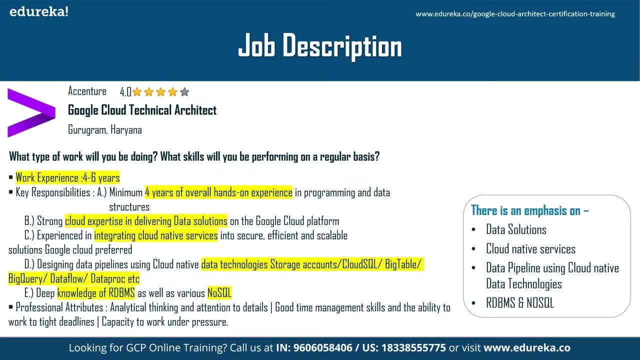 Cloud-native services are the like. unique services for that particular cloud service provider means unique services which are in Google cloud platform. The Google cloud architect should know about it and should know how to work on it and how to execute and make an output through it. 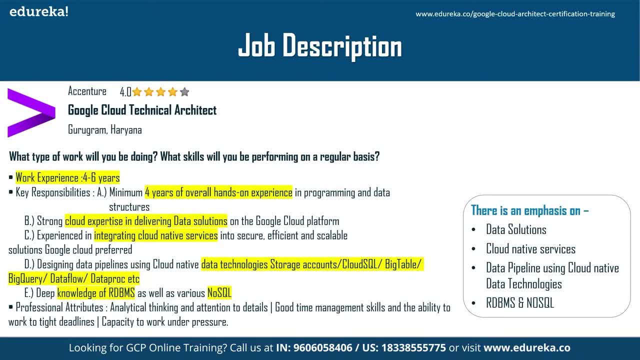 So Google cloud architect should be like integrating cloud-native services into secure, efficient and scalable solutions. Also, Google cloud architect should know how to design data pipelines using cloud-native data technologies. means cloud-native data technologies can be like storage accounts, cloud SQL. 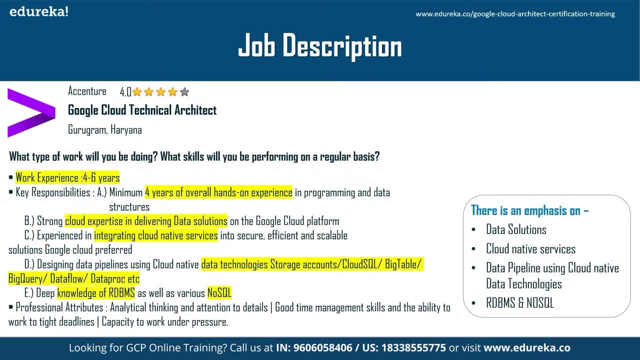 Bigtable, BigQuery, Dataproc, Dataproc, etc. Also, the Google cloud architect should have a deep knowledge of RDBMS, as well as of NoSQL, for like database programming And other non-technical, or say professional, attributes that the Google cloud architect should carry is analytical thinking and attention to details. 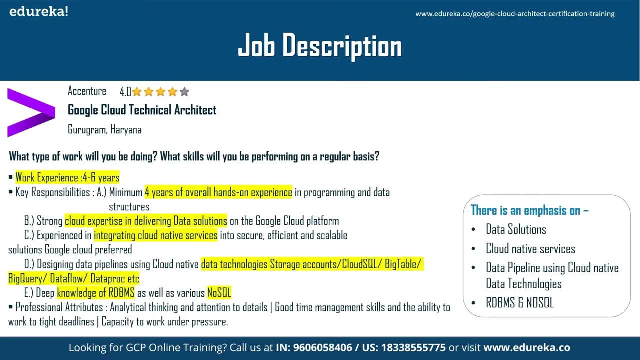 good time management skills and the ability to work to hide too tight deadlines and then capacity to work under pressure. These all things are required by a Google cloud architect. You can see the emphasis as a main of data solutions, cloud-native services, data pipeline. 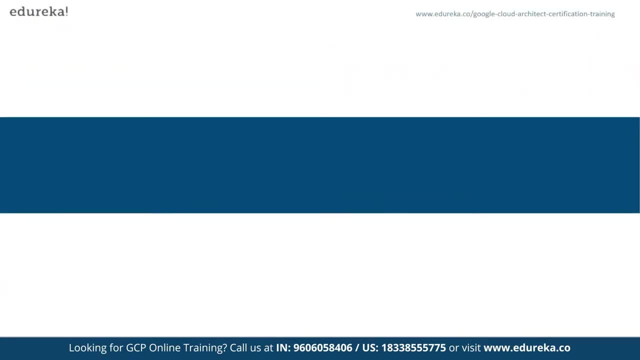 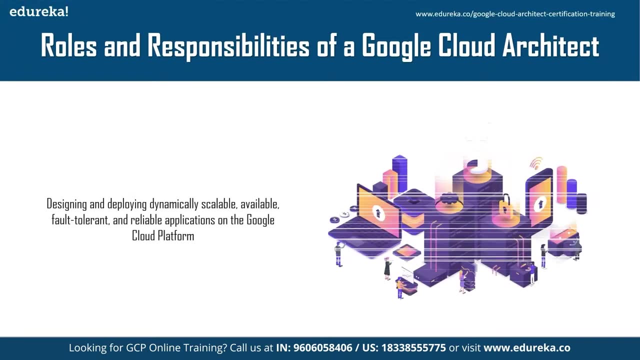 cloud-native data technologies, also of RDBMS and SQL. Now let's understand the roles and responsibilities of Google cloud architect, which he performs on a daily, weekly or monthly basis. So the Google cloud architect should know how to design and deploy applications on Google cloud platforms. 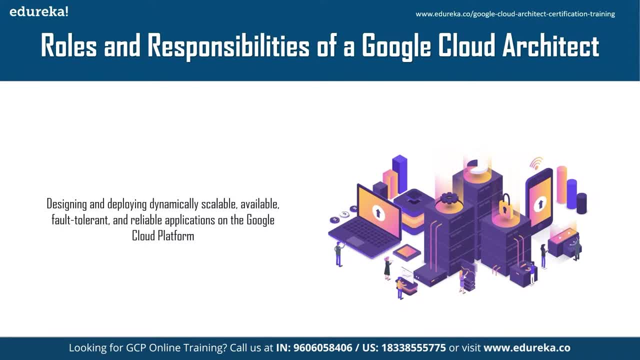 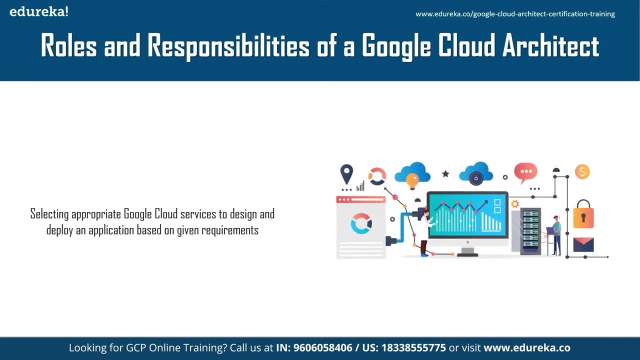 which are dynamically scalable and available, fault tolerant and also, like it should be, very much, reliable And secure as well. Also, if the Google cloud architect is going to deploy an application, then he should know what kind of Google cloud services should be used for it. 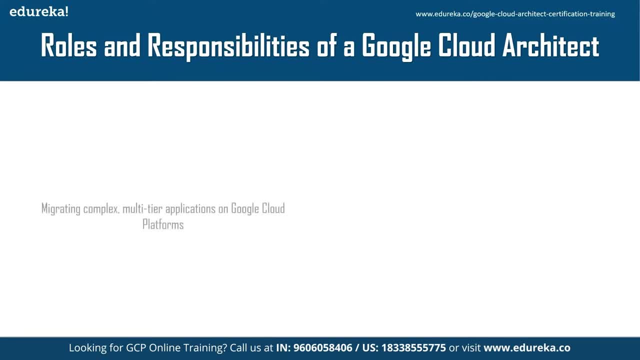 for that kind of a deployment based on the given requirements. Especially, he should also know like how to migrate application also like multi-data application, say the databases and a heavy database, also on Google cloud platform. One more thing is he should make a strategy of how to work on Google cloud platform with the most optimization and cost saving techniques. 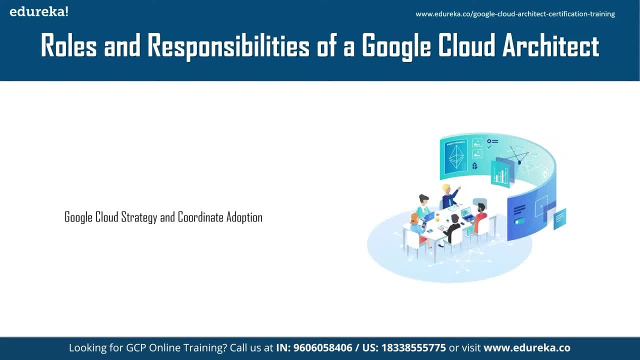 And he should also know how to coordinate. If there are new things are coming, he should be easily adaptable to the changes. Okay, Also, he should know how to implement multiple Google cloud services and use multiple products of Google cloud platform in a way that it shouldn't cost much to the company or, say, organization. 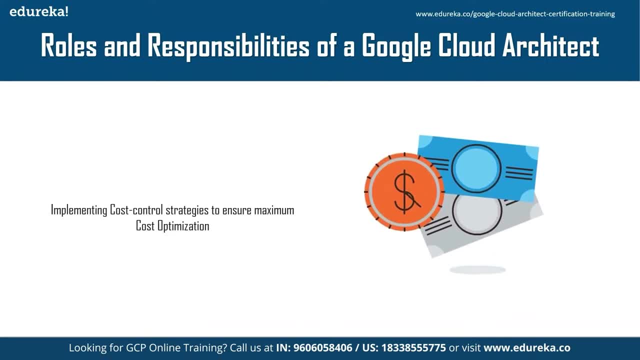 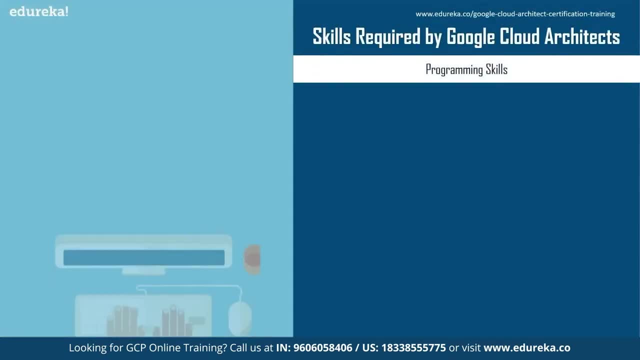 That means he should be well aware with the cost optimization techniques in Google cloud platform. Now let's understand the skills required by the Google cloud architect. So first of all, let's see the programming Skills required by the Google cloud architect. 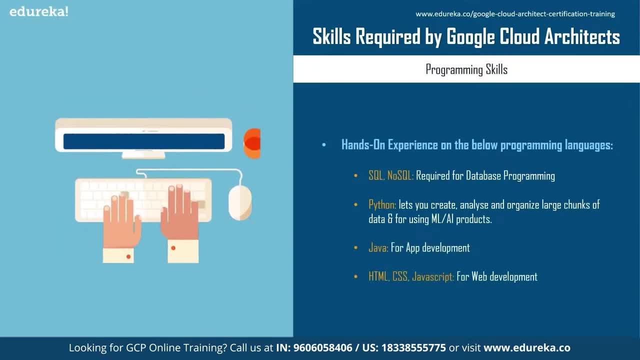 So he should have an hands-on experience of SQL as well as NoSQL, which are, like, majorly required for database programming and database migration and for querying purposes. He should also know the Python programming language, maybe not to the expertise or in very advanced level. 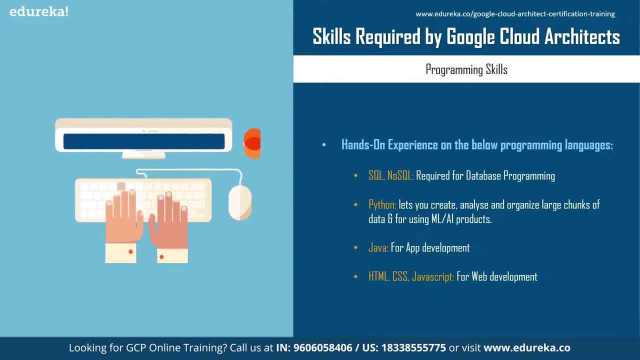 but at least at an intermediate level, so that he can create, analyze and organize large chunks of data as well, as it's very useful for using ML and AI products like natural language, language processing and means, natural language understanding and auto ML products For these purposes. 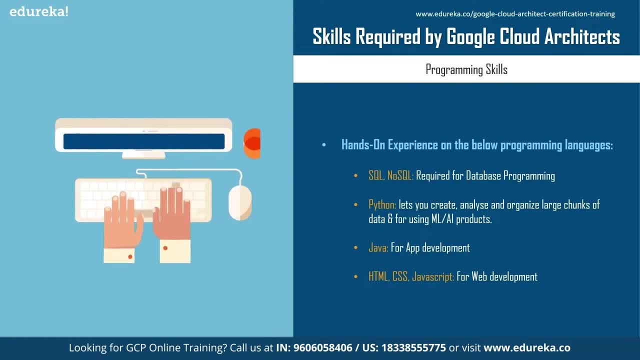 Python is like very much required, Also for the application development purposes. he should know the Java programming language, Also for web development purposes. he should carry a good knowledge of HTML, CSS and JavaScript. Now let's see the operating systems. 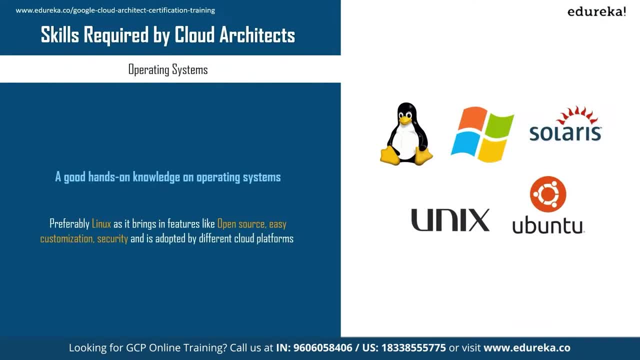 which the Google architect should be well aware of and should have a good knowledge of, like Linux, Solaris, Ubuntu, Windows, Unix, but preferably I would say he should have a good knowledge of Linux, As it brings the features like open source, security, customization and is adopted by different cloud platforms as well. 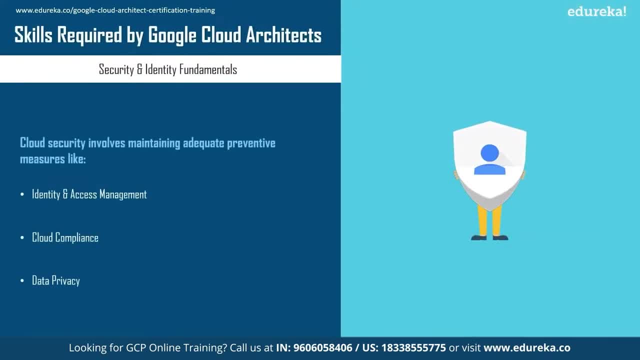 He should also have a very good knowledge of security and identity fundamentals in Google cloud platform, like identity and access management, like how to provide certain access management to certain users. If an employee is working under him and if he is handling any team, then he should know what kind of access he should provide to that person, to that employee. 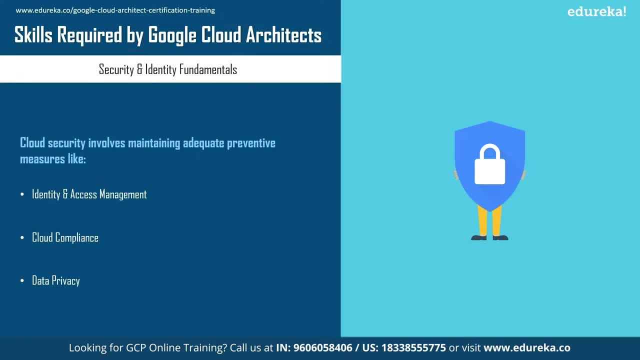 I mean, and what are the roles and policies of identity and access management? Also, he should be well aware of cloud compliance techniques. So cloud compliance is like the principle that cloud lever systems must be compliant with the standards their customers require, and cloud compliance ensures that cloud computing services meet compliance requirements. 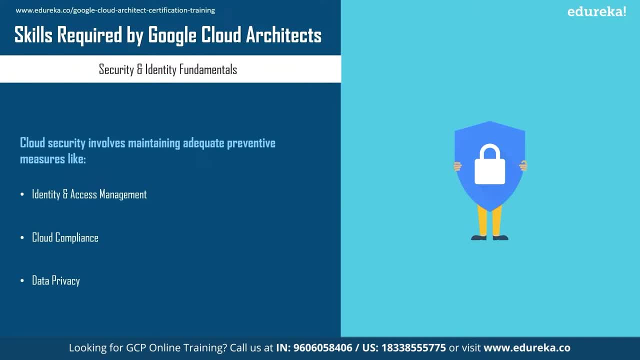 Lastly, he should be well aware of data privacy if he is uploading any data on cloud or if he is extracting any data from the cloud- import, export everything. So he should be well aware of the data privacy and how to protect and secure data from exploitation. 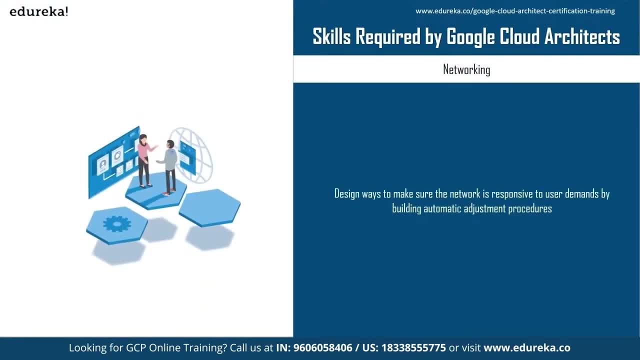 So Google cloud architect is also required to have a good knowledge of networking as well means networking in Google cloud platform. Like you, should have a very good knowledge of cloud CDN, which is a cloud delivery network for service web and like video content, and also for cloud DNS. 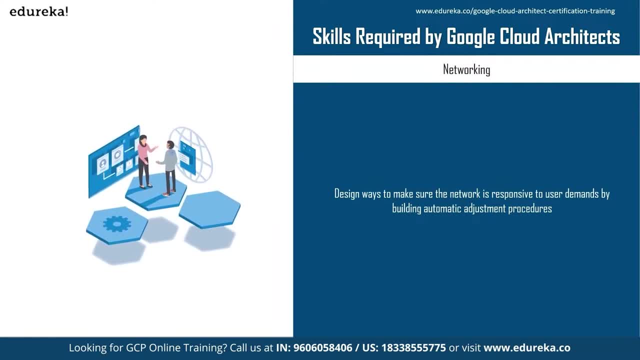 which is a domain name system for reliable and low latency name lookups, as well as of hybrid connectivity options for VPN peering and enterprise needs On a whole. Google cloud architect should know how to design networking ways to make sure the network is responsible to user demands. 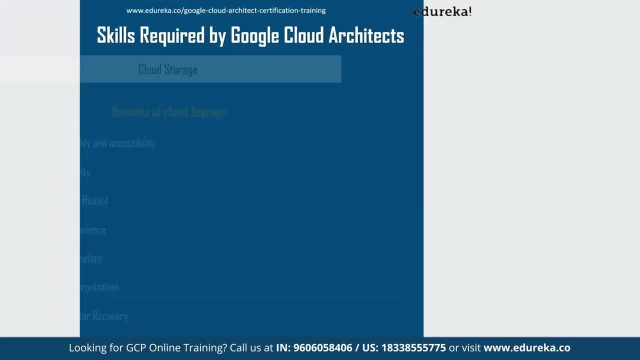 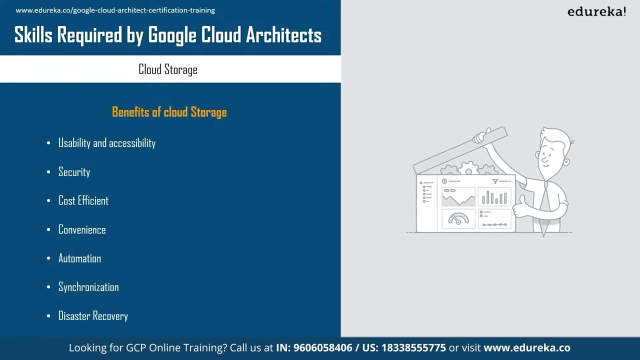 by building automatic adjustment procedures. Lastly, he should be very well aware of cloud storage techniques in Google cloud platform and especially like usability and accessibility through cloud storage- How easily cloud storage can be used and accessed. Secondly, he should ensure the security for storage. 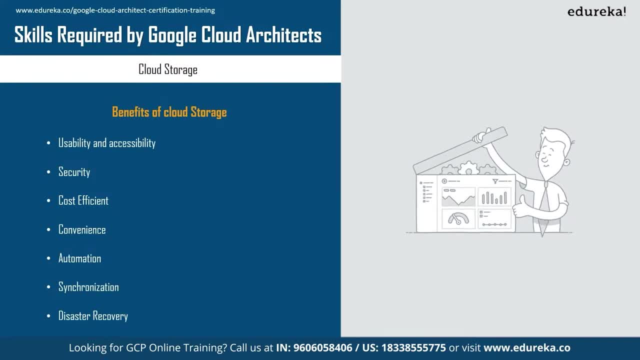 If he is storing any data, he should be ensuring that how he can use security techniques to secure the data and whatever services he is combining with cloud storage. he should be ensuring that how he can use security techniques to secure the data and whatever services he is combining with cloud storage. 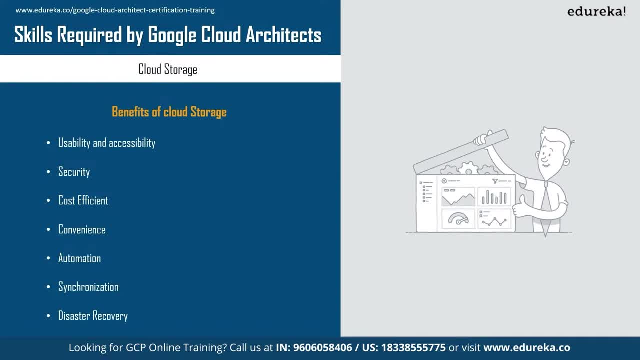 it should be cost efficient, as well as the service he is using, like cloud storage service. if he is using, he should be able to optimize it in a way that it should cost the least to the organization, as well as he should be using it. that it's very portable, or you can say like very easily usable. 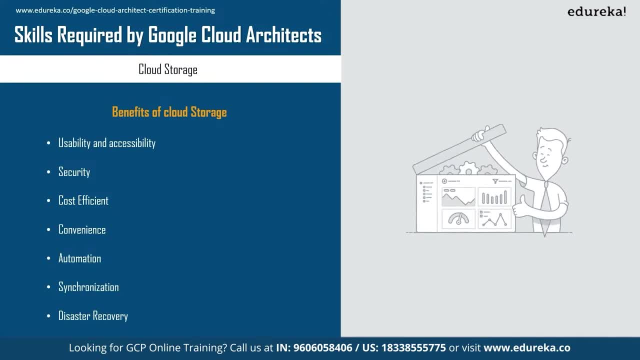 so that will be convenient for the organizations and for the client also. he should know how to automate the data he is storing- cloud storage- and the data should be synchronized with the multiple devices or we can say with the lead device of the organization. and also he should 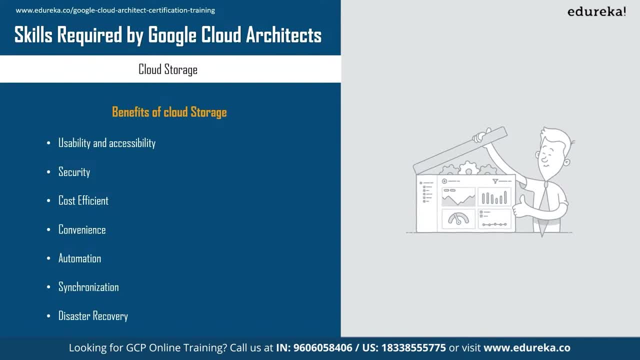 be well aware of the disaster recovery in cloud storage so that if the data gets lost, then it can be backed up later on. now, when we come to data storage, so there are like four types of storage. so the first is a standard storage, which is good for hot data that's accessed frequently, including 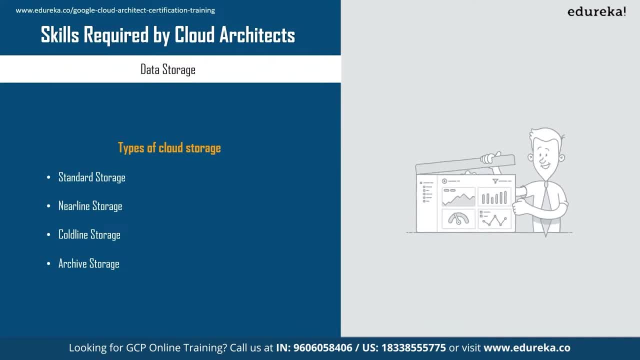 websites, streaming videos and mobile apps. second is nearline storage, which is like for low cost, good for data that can be stored for at least 30 days, including data backup and long-term multimedia content. then there's cold line storage, which has a very low cost, good for data that can be stored for at least 90 days. 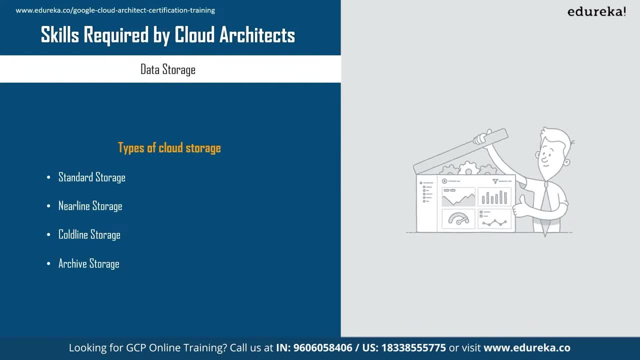 including disaster recovery. then there is archive storage, so which has a lowest cost, good for data that can be stored for at least 365 days, including regulatory archives. now, these are the non-technical skills required by the google cloud architect, that he should be flexible in working, and he 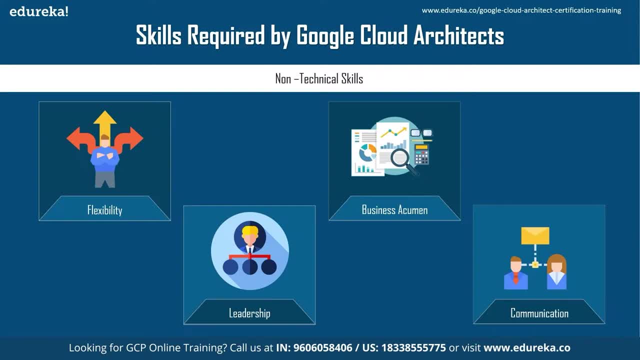 should have a leadership skills as well, as he should be able to work in the cloud as well, as he should be able to work in the cloud as well, as he should be able to work in the cloud as well as well- to lead a team, and he should be business oriented. that how to profit the organization. if 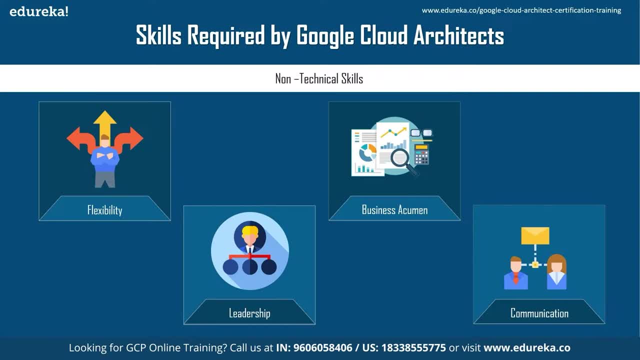 he is working on any project or something, he should know that how to extract out the maximum leads or you can say, the maximum profit for the business. also, he should have very good communication skills so that he can lead a team or he can connect multiple teams or he can easily handle the. 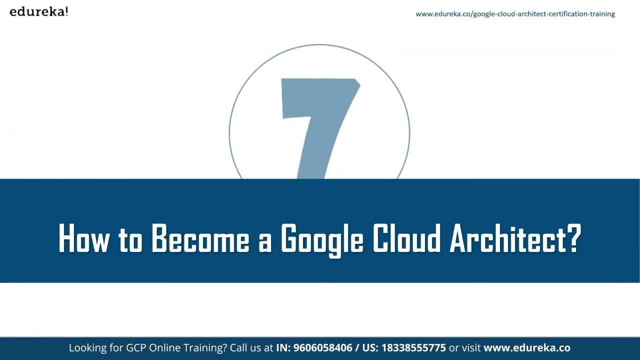 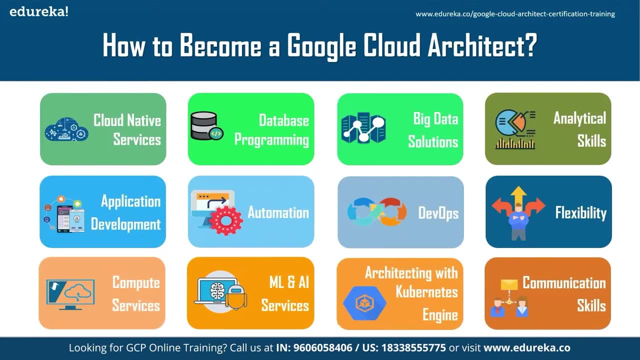 clients as well. now let's understand how one can become a google cloud architect. for becoming a google cloud architect, you should know cloud native services means which are the cloud native services means which are the unique services. you can say like firebase firestore app unique services. you can say like firebase firestore app engine or google kubernetes engine. cloud run. 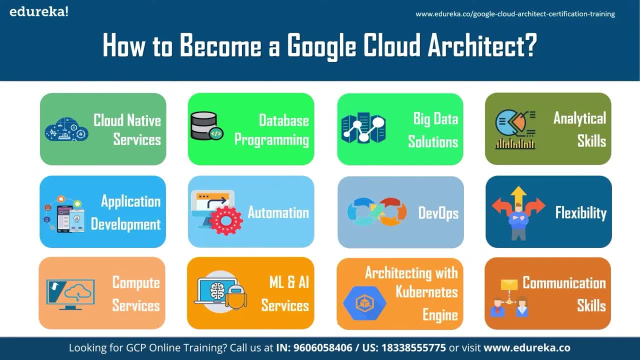 engine or google kubernetes engine, cloud run. you should have a good hands-on experience, or say a. you should have a good hands-on experience, or, say, a very deep knowledge of these cloud native, very deep knowledge of these cloud native services. also, you should be well aware of database. 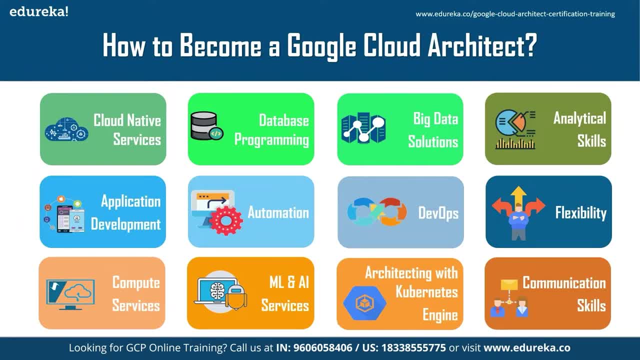 services. also, you should be well aware of database programming like both sql and no sql, so that you can programming like both sql and no sql, so that you can handle sql databases as well as no sql databases, handle sql databases as well as no sql databases, like there is a cloud sql and then there is a cloud. 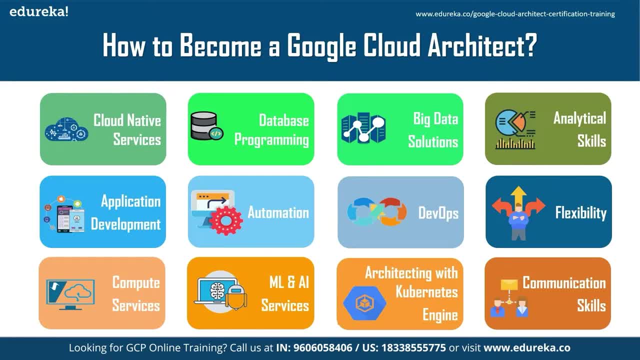 like there is a cloud sql and then there is a cloud big table fire store, also like memory store. cloud big table fire store, also like memory store. cloud spanner- all these are database services provided. spanner- all these are database services provided in google cloud platform also. you should be well. 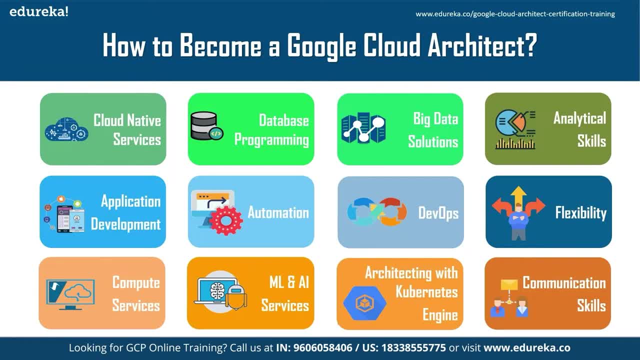 in google cloud platform. also, you should be well aware of big data solutions so that big data, aware of big data solutions, so that big data services in google cloud platform can be easily. services in google cloud platform can be easily managed, like bigquery and dataproc or cloudpub. 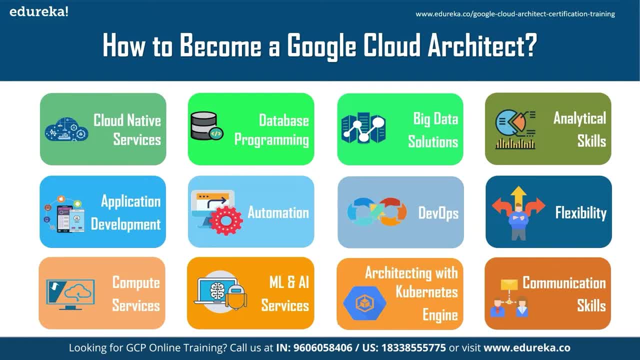 managed, like bigquery and dataproc or cloudpub sub or data flow. these are big data solutions. sub or data flow. these are big data solutions you should be well aware of also. you should carry- you should be well aware of also. you should carry- very fine analytical skills also. you should be. 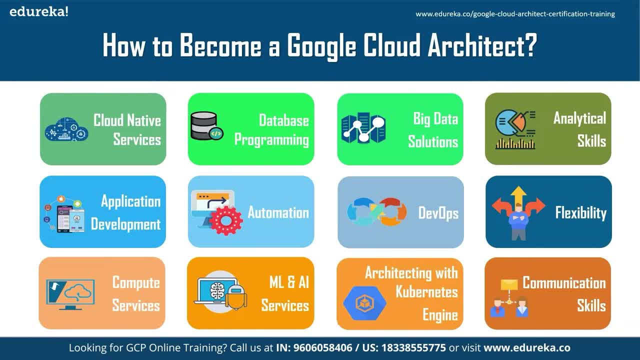 very fine analytical skills also, you should be well aware of application development, like you can use, well aware of application development, like you can use- app engine, google cloud platform for developing app engine, google cloud platform for developing the applications for deploying, also for deploying the applications for deploying, also for deploying purposes also. also, you should know the automation. 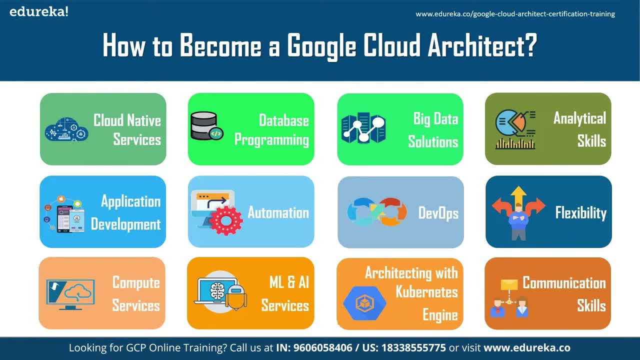 purposes also. also, you should know the automation process in google cloud platform. like there is a process in google cloud platform, like there is a free google cloud platform automation software. free google cloud platform automation software. from park my cloud, so park my cloud is a like tool. from park my cloud, so park my cloud is a like tool for scheduling non-production instances on google. 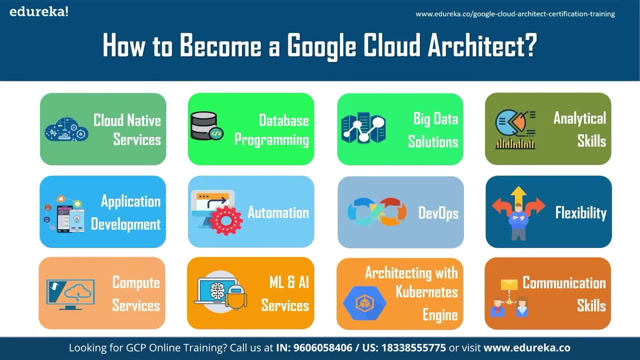 for scheduling non-production instances on google cloud platform. it helps companies reduce their cloud cloud platform. it helps companies reduce their cloud computing costs. also like improve their id computing costs. also like improve their id governance, increase accountability and optimize their governance, increase accountability and optimize their cloud computing resources as well. also. you. 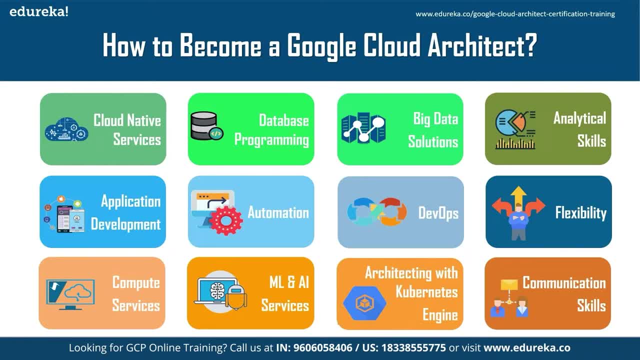 cloud computing resources as well. also, you should be well aware and have a good knowledge of devos, should be well aware and have a good knowledge of devos products, products and integrations so that you can build and deploy new cloud applications or store artifacts and monitor app security. 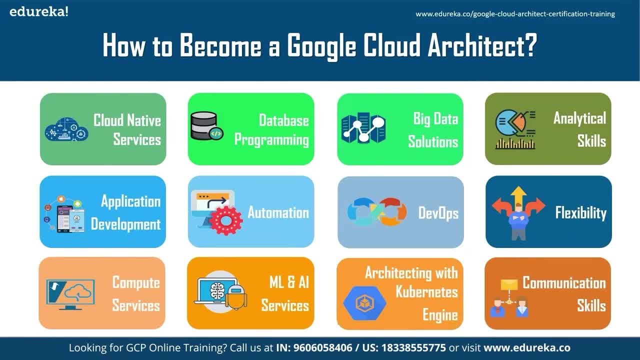 and reliability on google cloud. like there is a cloud build and artifact registry. like cloud builder, you can see like it defines custom workflows for building, testing and deploying across multiple network environments. and artifact registry is used for storing, managing and securing your container, images and language packages. all these things you should be well aware of. also, you should be. 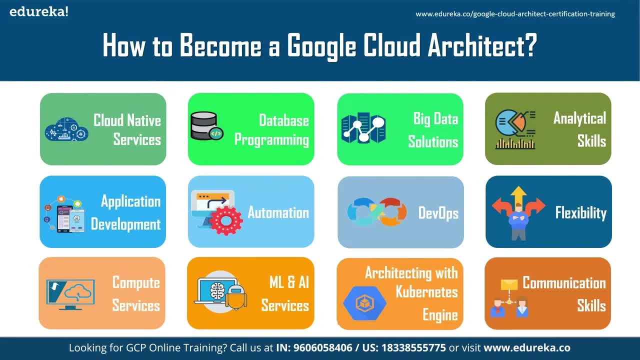 flexible enough to work in a fast-paced environment. flexible enough to work in a fast-paced environment as well, as well. also, you should be well aware of the compute services as well. like this also. you should be well aware of the compute services as well, like this compute engine where you can run virtual machines in. 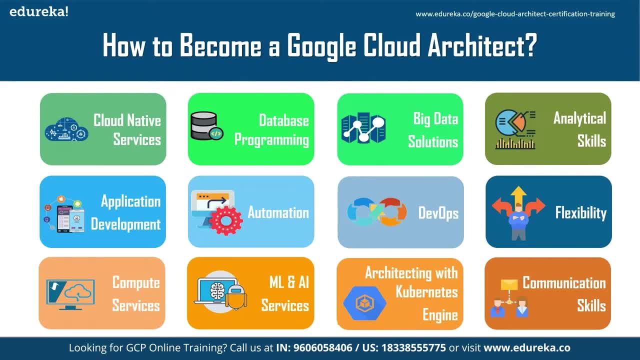 compute engine where you can run virtual machines in google's data center, and also like there is a google app engine, google's data center, and also like there is a google app engine, which is a serverless application platform for apps, which is a serverless application platform for apps. 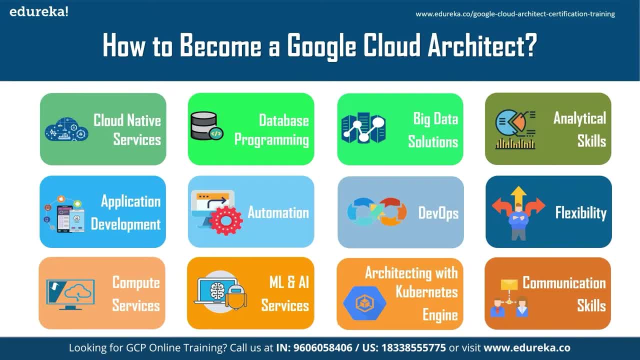 which is a serverless application platform for apps and backends, also like cloud gpus and backends also like cloud gpus and backends also like cloud gpus. mpreemptible virtual machines and mpreemptible virtual machines and mpreemptible virtual machines and shielded virtual machines. you should be. 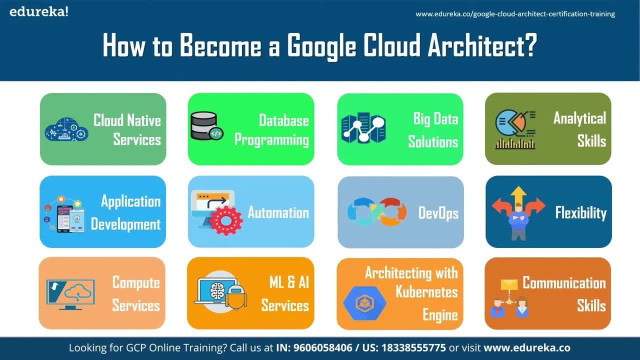 shielded virtual machines. you should be shielded virtual machines you should be well aware of, well aware of, well aware of, and should also have a like hands-on and should also have a like hands-on and should also have a like hands-on experience also, experience also. 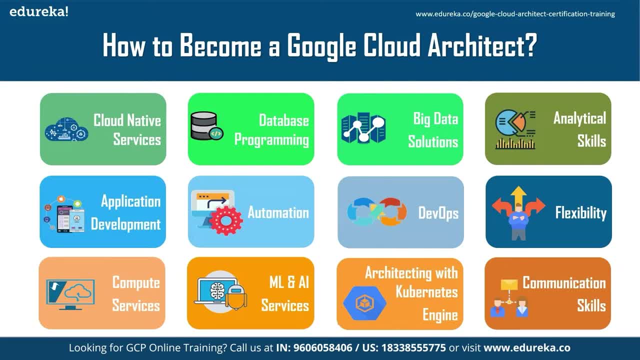 experience also other than that. there are also like mln other than that. there are also like mln other than that. there are also like mln. ai services, which is very unique in ai services, which is very unique in ai services, which is very unique in like google cloud, and google cloud is. 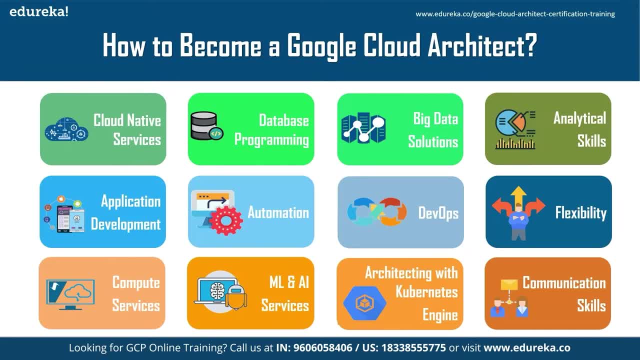 like google cloud and google cloud is like google cloud, and google cloud is actually famous for its mln services. so actually famous for its mln services. so actually famous for its mln services. so that is something you should be like you. that is something you should be like you. 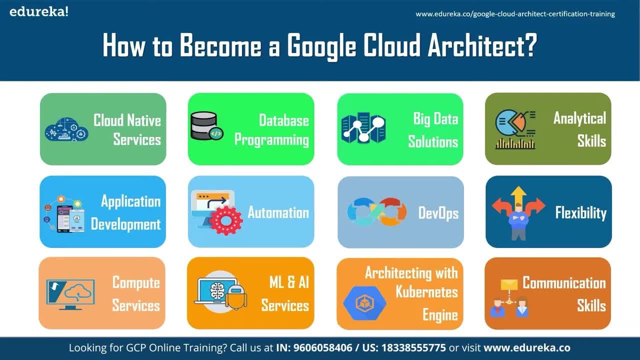 that is something you should be like. you should have a deep knowledge and a should have a deep knowledge and a should have a deep knowledge and a hands-on experience, and you should really hands-on experience and you should really hands-on experience and you should really be well aware of it. 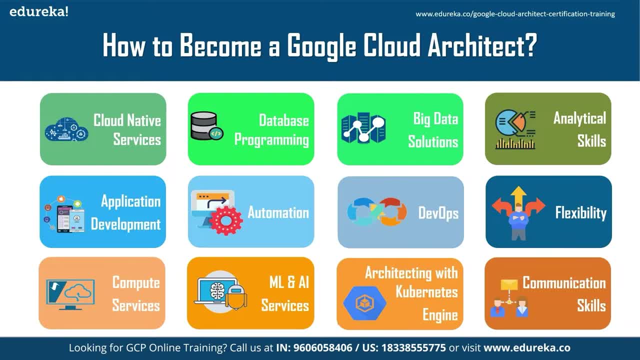 be well aware of it. be well aware of it so you can see like there are certain. so you can see like there are certain, so you can see like there are certain services like auto ml vision ai, services like auto ml vision ai, services like auto ml vision ai, and like this cloud translation for. 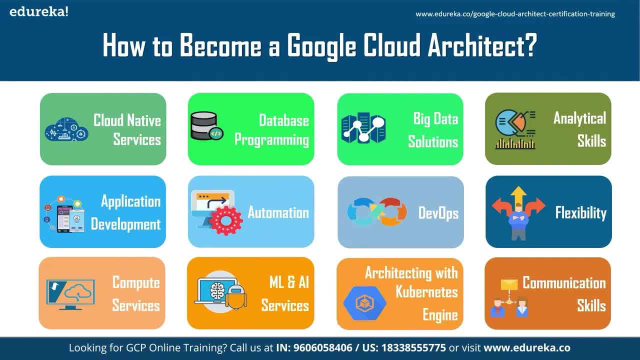 and like this cloud translation for, and like this cloud translation for language detection translation and language detection translation and language detection translation, and there is a cloud natural language for there is a cloud natural language, for there is a cloud natural language for sentiment analysis and sentiment analysis, and 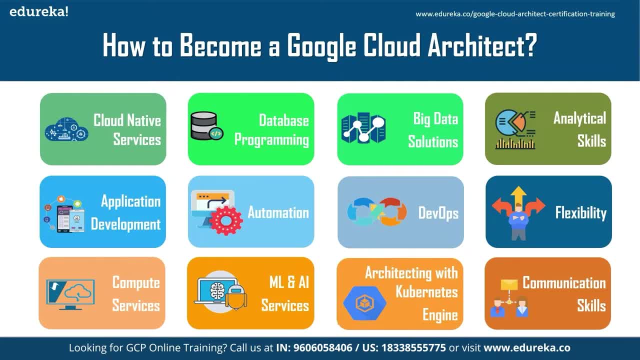 sentiment analysis. and video is also there for video. video is also there for video. video is also there for video. classification recognition: this is like classification recognition. this is like classification recognition. this is like for deep learning: all these things, this for deep learning, all these things, this for deep learning, all these things, this- and you should know about the. 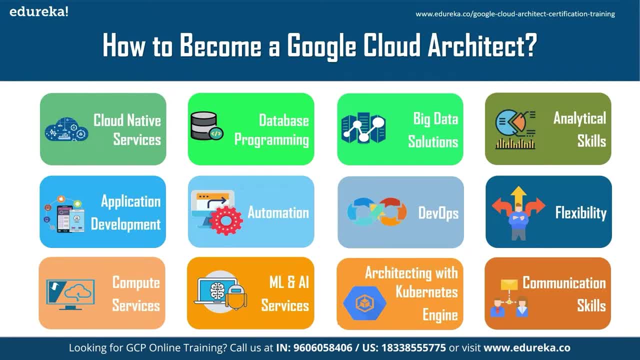 and you should know about the and you should know about the architectural working of kubernetes, architectural working of kubernetes, architectural working of kubernetes engine. so they are like two modes of engine. so they are like two modes of engine. so they are like two modes of google kubernetes engine. 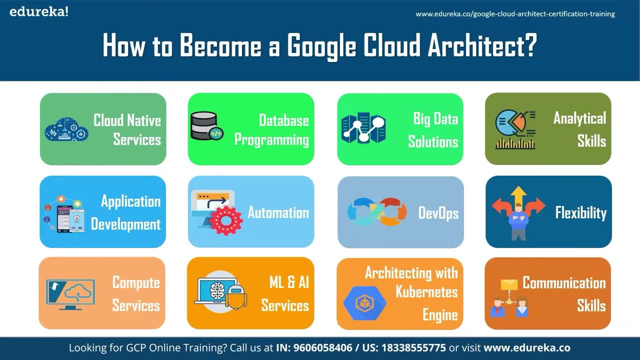 google kubernetes engine. google kubernetes engine means there are two modes of operation, means there are two modes of operation, means there are two modes of operation. google kubernetes engine. they are like google kubernetes engine. they are like google kubernetes engine. they are like standard and autopilot. and 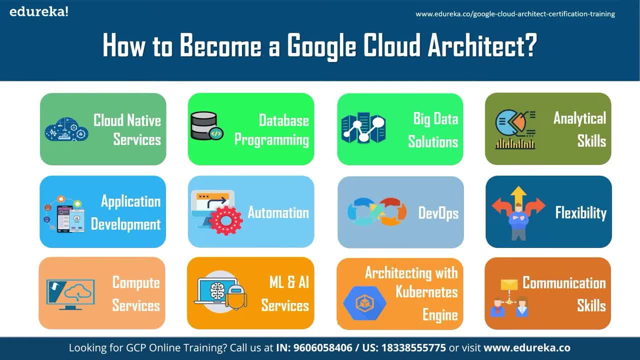 standard and autopilot and standard and autopilot. and like there's also podding cluster auto, like there's also podding cluster auto, like there's also podding cluster auto scaling in it and there is like pre-built scaling in it and there is like pre-built. 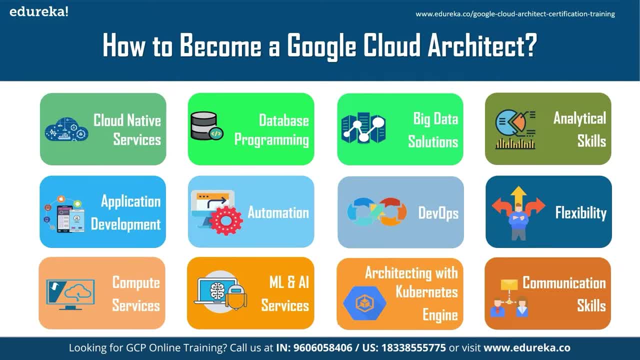 scaling in it and there is like pre-built kubernetes applications and templates, kubernetes applications and templates. kubernetes applications and templates are also there, also like a container, are also there, also like a container, are also there, also like a container. native networking and security is also. 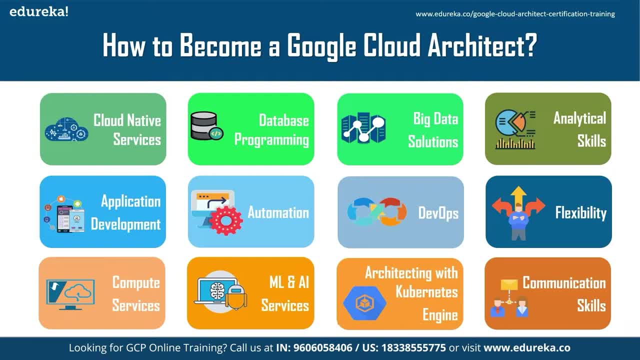 native networking and security is also. native networking and security is also being provided by gk, being provided by gk, being provided by gk. sandbox means google kubernetes engine sandbox, means google kubernetes engine sandbox, means google kubernetes engine sandbox, sandbox, sandbox. so these are some of the concepts you so these are some of the concepts you, so these are some of the concepts you should be well aware of, other than that should be well aware of, other than that should be well aware of, other than that you should also have a very. you should also have a very. 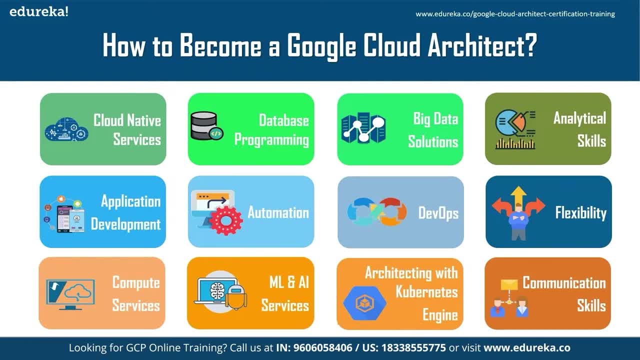 you should also have a very good communication skills to handle good communication skills. to handle good communication skills to handle clients and handle teams and multiple clients and handle teams and multiple clients and handle teams and multiple teams as well. now let's see the google teams as well. now let's see the google. 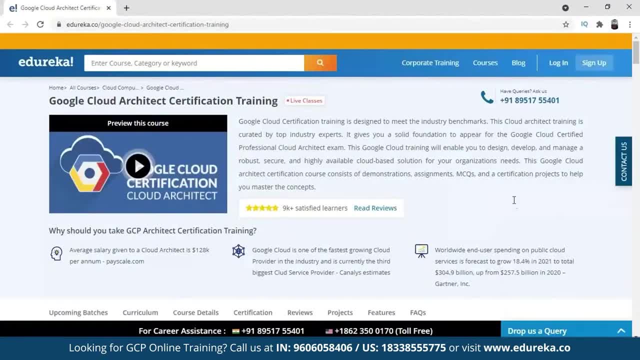 teams as well. now let's see the google cloud certification provided by edureka. cloud certification provided by edureka, cloud certification provided by edureka as well, as well, as well. so you can see how i have explained you. so you can see how i have explained you. 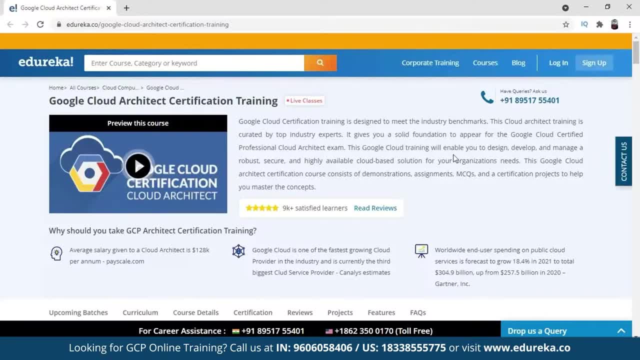 so you can see how i have explained you a step by step. like google certification, a step by step. like google certification, a step by step. like google certification, training is designed to meet, the training is designed to meet, the training is designed to meet the industry benchmark. it's, of course, the 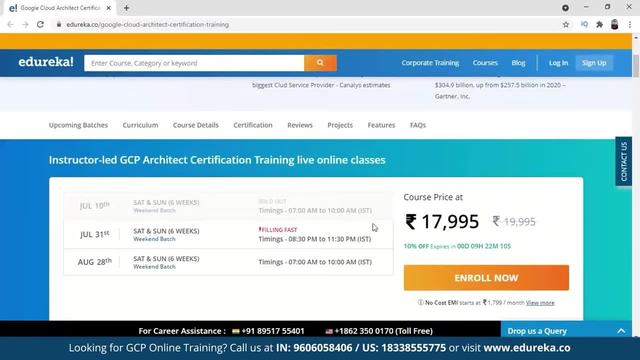 industry benchmark. it's of course the industry benchmark. it's of course the industrial event course, industrial event course, industrial event course. and then there are multiple batches for, and then there are multiple batches for, and then there are multiple batches for it. right now there's a july 31. 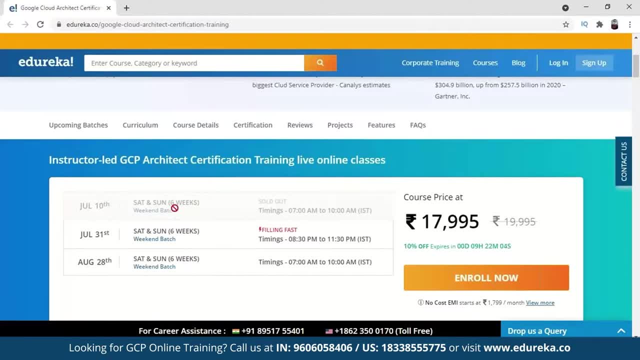 it right now there's a july 31. it right now there's a july 31 batch which is filling paths, then it's batch which is filling paths, then it's batch which is filling paths. then it's also like august 28 patch. they are like 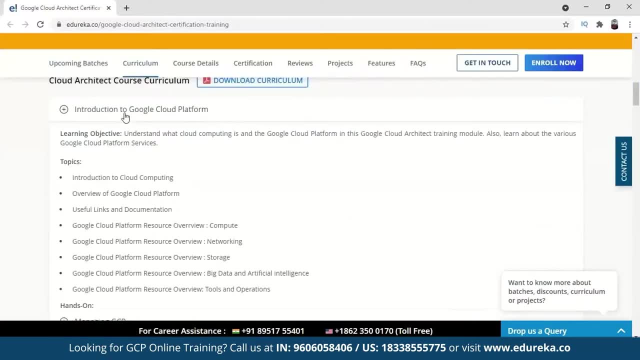 also like august 28 patch. they are like also like august 28 patch. they are like monthly batches. you can register for monthly batches. you can register for monthly batches. you can register for them. as i have like explained, you step them. as i have like explained, you step. 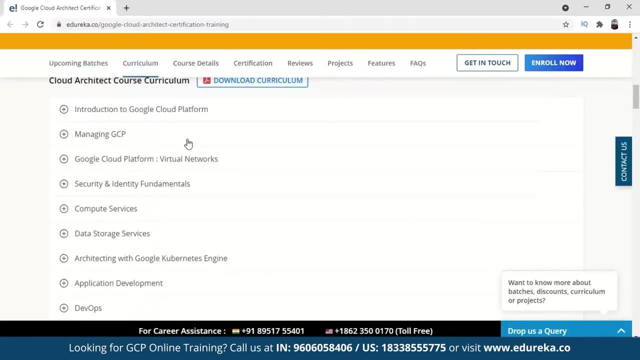 them as i have like, explained you step by step how google certification is by step. how google certification is by step, how google certification is needed and why you need to be certified needed and why you need to be certified needed and why you need to be certified google cloud. 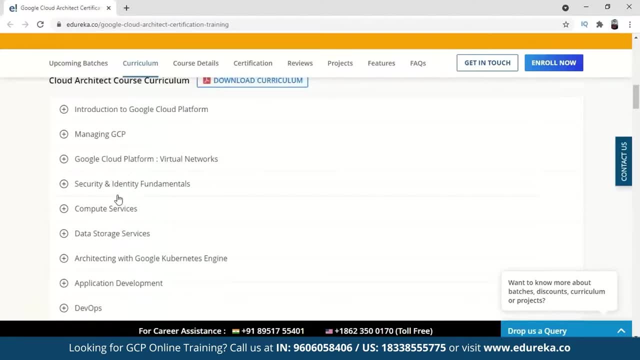 google cloud: google cloud architect. you can see i've explained to architect. you can see i've explained to architect. you can see i've explained to compute services for like virtual compute services, for like virtual compute services, for like virtual networks, all these things and compute networks, all these things and compute. 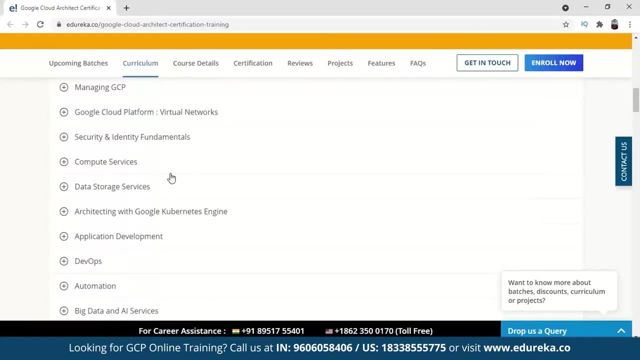 networks, all these things, and compute services and security and identity services and security and identity services and security and identity fundamentals, like i've explained you fundamentals, like i've explained you fundamentals, like i've explained you, like the entity access management and like the entity access management and 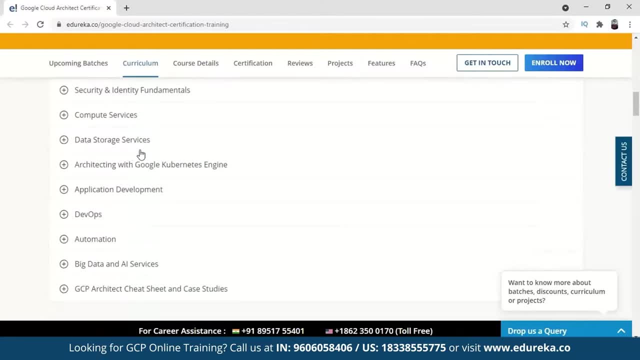 like the entity access management and cloud compliance and data privacy things. cloud compliance and data privacy things, cloud compliance and data privacy. things other than that data storage services. other than that data storage services, other than that data storage services- and these are like the fundamentals like. and these are like the fundamentals like. 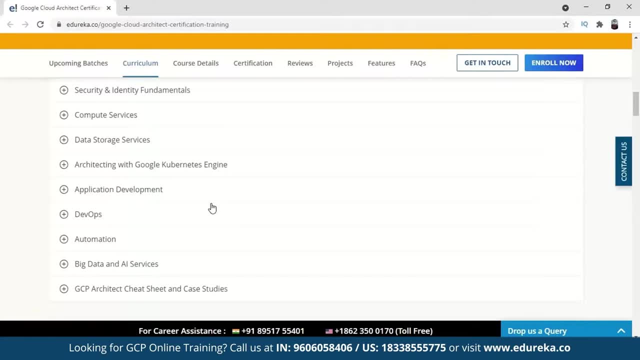 and these are like the fundamentals, like these services, you should actually be these services. you should actually be these services. you should actually be knowing and how, where you should knowing and how, where you should knowing and how, where you should implement these services for what? implement these services for what? 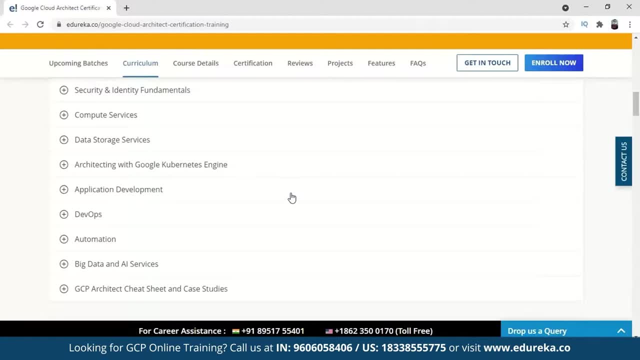 implement these services? for what requirement? this is how the industrial requirement. this is how the industrial requirement. this is how the industrial event- google cloud platform architect event. google cloud platform architect event- google cloud platform architect course- has been constructed by edureka. course has been constructed by edureka. 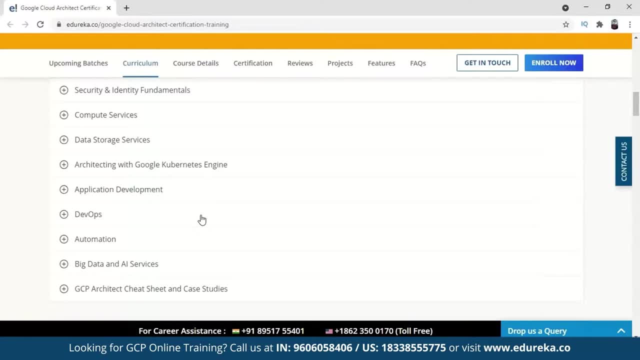 course has been constructed by edureka, and it can surely help you in also, and it can surely help you in also, and it can surely help you in also- cracking the google cloud platform exam, cracking the google cloud platform exam, cracking the google cloud platform exam that we are going to talk about then. 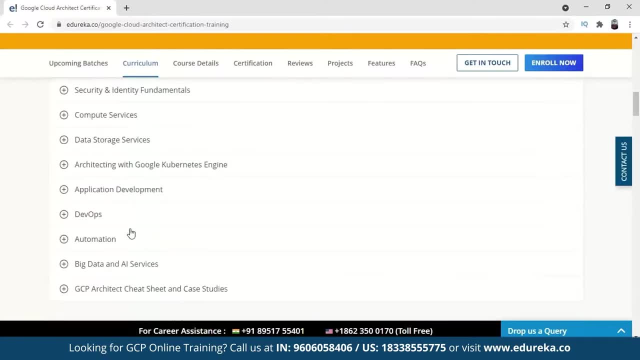 that we are going to talk about then, that we are going to talk about then. there's you can see like i have there's you can see like i have there's. you can see like i have explained to devops automation. explained to devops automation, explained to devops automation: everything i have explained you. 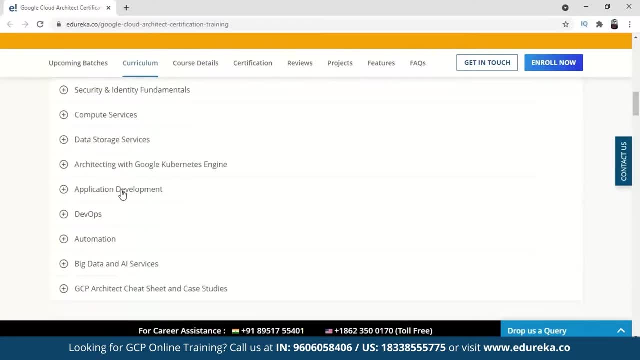 everything i have explained you, everything i have explained you, so as i have told you how these services, so as i have told you how these services, so as i have told you how these services are very much important, are very much important, are very much important, and these are the services you should. 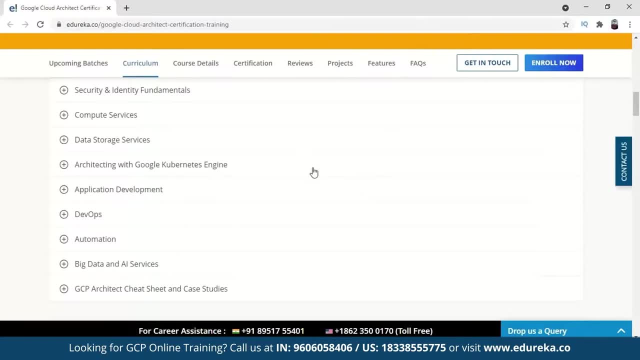 and these are the services you should and these are the services you should target for, target for, target for: so you can register for edureka google. so you can register for edureka google. so you can register for edureka google. cloud platform architect certification. cloud platform architect certification. 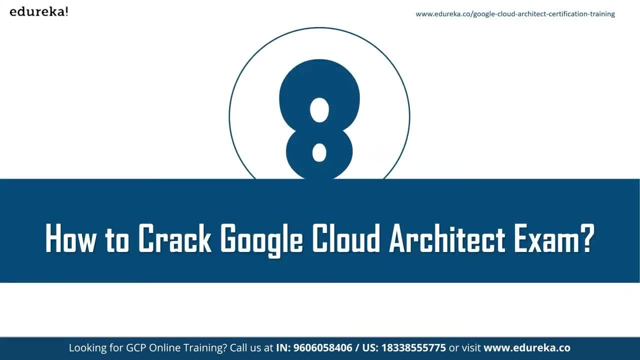 cloud platform architect certification. so this was all about how to become a. so this was all about how to become a. so this was all about how to become a google cloud architect. google cloud architect- google cloud architect. now, let's understand how to crack google. now, let's understand how to crack google. 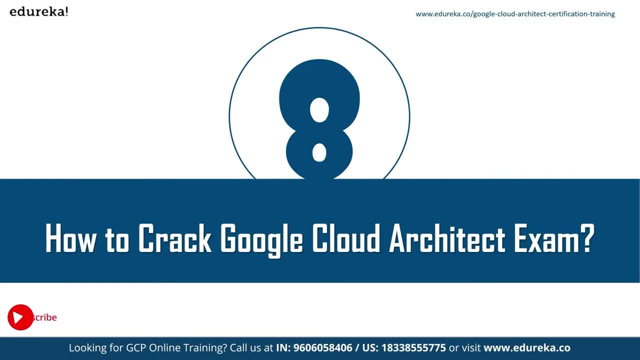 now let's understand how to crack google cloud architect exam. cloud architect exam. cloud architect exam: if you don't know much about google cloud, if you don't know much about google, if you don't know much about google architect exam, it is valid for two years. architect exam. it is valid for two years. 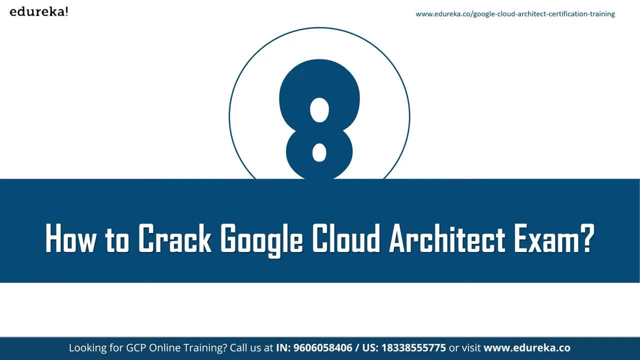 architect exam. it is valid for two years and it's a two hour exam when you have, and it's a two hour exam when you have. and it's a two hour exam when you have prepared for it, you can actually apply. prepared for it, you can actually apply. 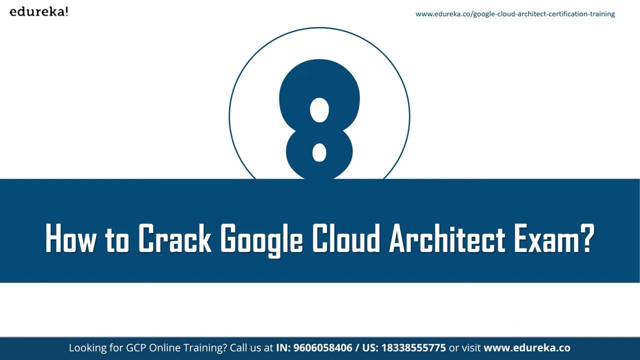 prepared for it. you can actually apply for it, for it, for it that you can look at the documentation. that you can look at the documentation that you can look at the documentation. part of a google cloud platform. part of a google cloud platform. part of a google cloud platform for cracking google cloud architect exam. 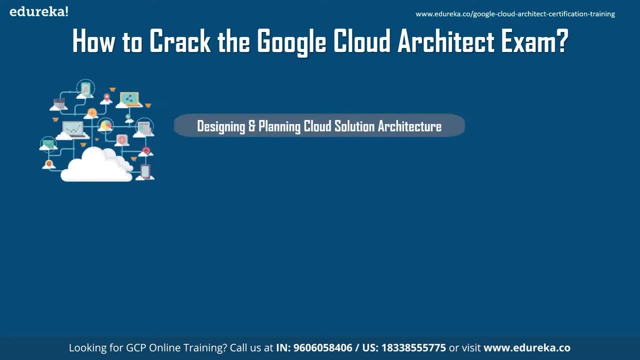 for cracking google cloud architect exam. for cracking google cloud architect exam, you should know how to design and plan a. you should know how to design and plan a. you should know how to design and plan a google cloud solution architecture. google cloud solution architecture. google cloud solution architecture like designing a solution infrastructure. 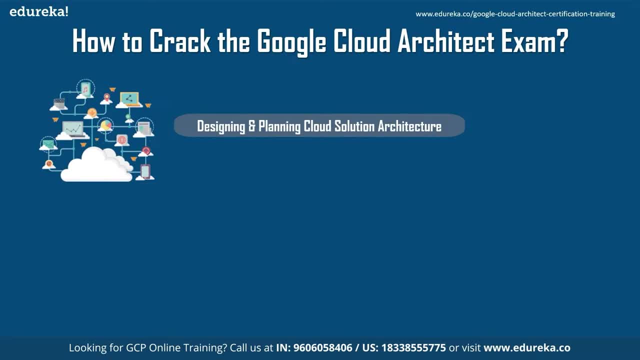 like designing a solution infrastructure. like designing a solution infrastructure that needs business requirements, that needs business requirements, that needs business requirements, and consideration for that includes, and consideration for that includes, and consideration for that includes, business use cases and product strategy. business use cases and product strategy. business use cases and product strategy: cost optimization: supporting the 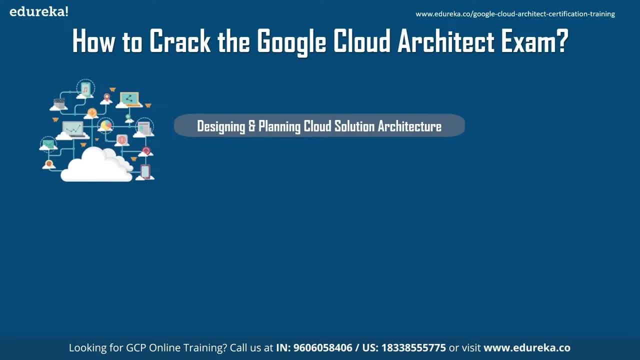 cost optimization: supporting the cost optimization, supporting the application design. application design. application design. integration with external systems. integration with external systems. integration with external systems. movement of data- as well as like movement of data. as well as like movement of data as well as like design, decision, trade-offs and build. 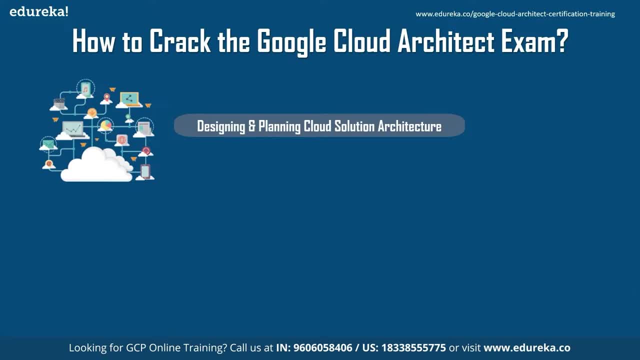 design decision, trade-offs and build design decision, trade-offs. and build by modify or depreciate also the. by modify or depreciate also the. by modify or depreciate also the compliance and observability as well. compliance and observability as well. compliance and observability as well, other than that designing a solution. 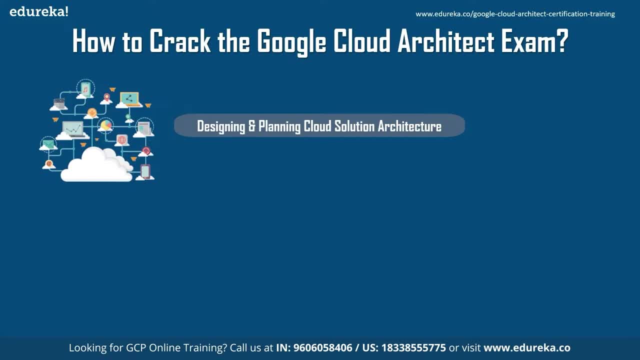 other than that designing a solution, other than that designing a solution. infrastructure that meets technical infrastructure that meets technical infrastructure that meets technical requirements. requirements, requirements like high availability and failover, like high availability and failover, like high availability and failover. design scalability to meet growth. design scalability to meet growth. 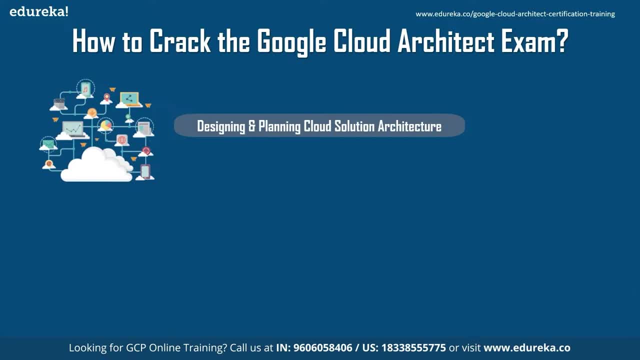 design scalability to meet growth requirements and performance and latency requirements and performance and latency requirements and performance and latency. and while designing in network storage and while designing in network storage. and while designing in network storage and compute services and compute services and compute services, you should consider integration with 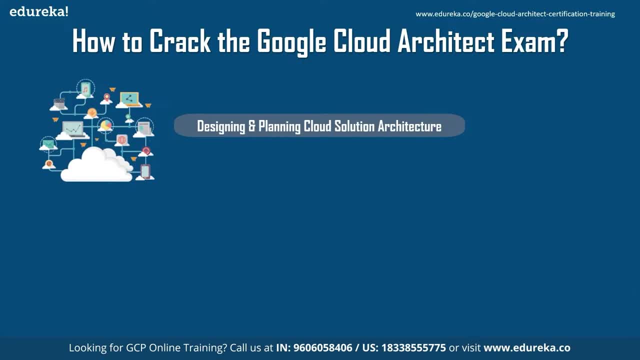 you should consider integration with. you should consider integration with on-premises or multi-cloud, on-premises or multi-cloud, on-premises or multi-cloud environments. choosing data processing environments. choosing data processing environments, choosing data processing technologies as well, and choosing technologies as well and choosing. 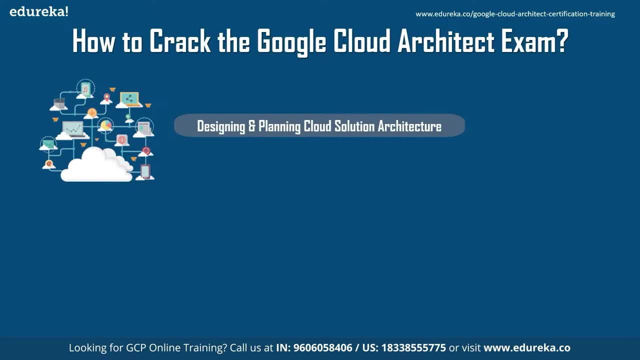 technologies as well, and choosing compute resources and mapping compute- compute resources and mapping compute, compute resources and mapping compute needs to needs, to needs, to platform products. then also like creating platform products, then also like creating platform products. then also like creating a migration plan that is documents, a migration plan that is documents. 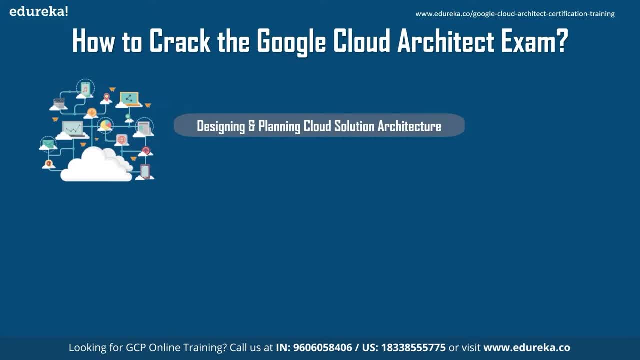 a migration plan, that is, documents and architectural diagrams for which the and architectural diagrams for which the. and architectural diagrams for which the considerations include integrating considerations include integrating considerations include integrating solutions with existing systems. solutions with existing systems. solutions with existing systems. migrating systems and data to support. 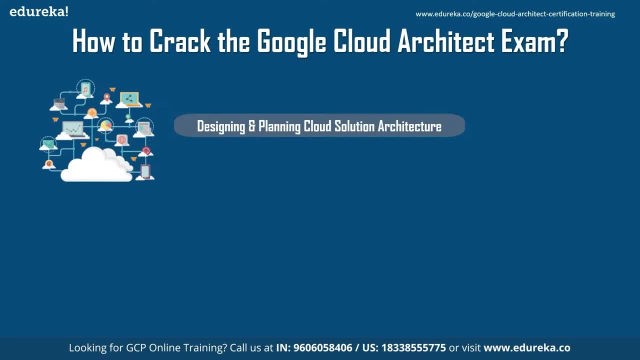 migrating systems and data. to support migrating systems and data. to support the solution also for software license, the solution also for software license, the solution also for software license. mapping and network planning: also like mapping and network planning. also like mapping and network planning, also like demanding management planning. and. 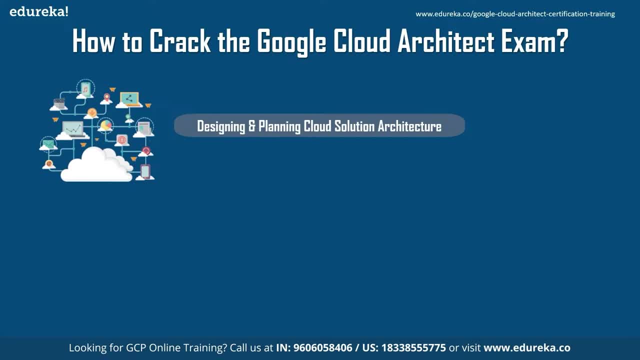 demanding management planning and demanding management planning and envisioning, especially like envisioning, envisioning, especially like envisioning, envisioning, especially like envisioning future solution improvements, future solution improvements, future solution improvements, considerations for that that include considerations for that, that include considerations for that, that include cloud and technology improvements, and 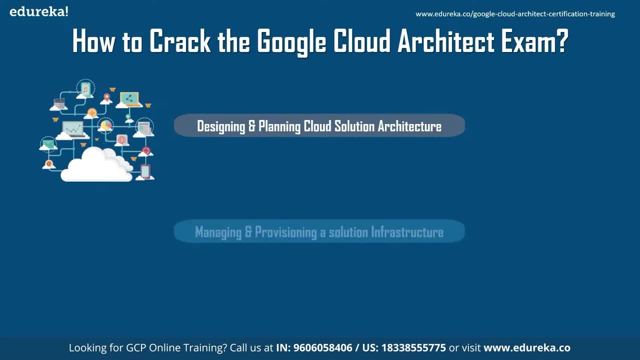 cloud and technology improvements and cloud and technology improvements and evolution of business needs and evolution of business needs and evolution of business needs. and evangelism and advocacy. second thing is evangelism and advocacy. second thing is evangelism and advocacy. second thing is: you should know how to manage and 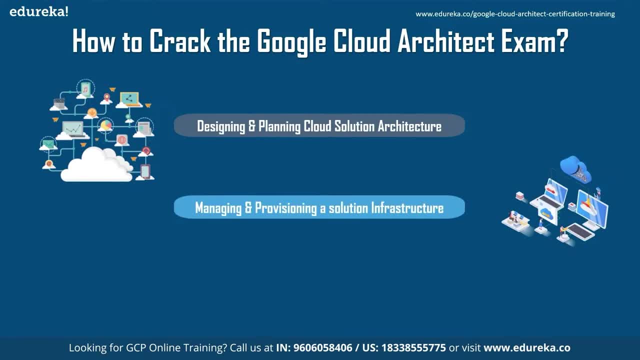 you should know how to manage, and you should know how to manage and provision of solution infrastructure. so provision of solution infrastructure, so provision of solution infrastructure. so for that you need to configure network, for that you need to configure network, for that you need to configure network topologies. 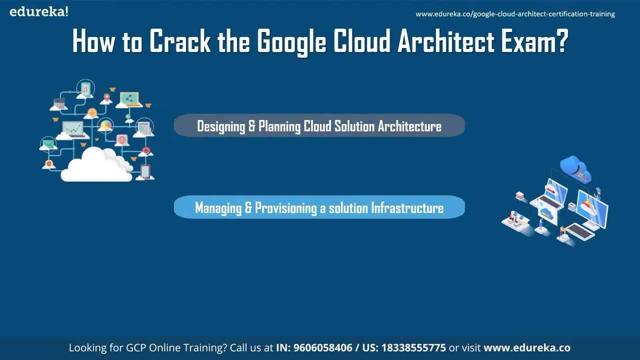 topologies, topologies, and you should consider extending to and you should consider extending to and you should consider extending to on-premises environments and extending on-premises environments and extending on-premises environments and extending to a multi-cloud environment that may, to a multi-cloud environment that may. 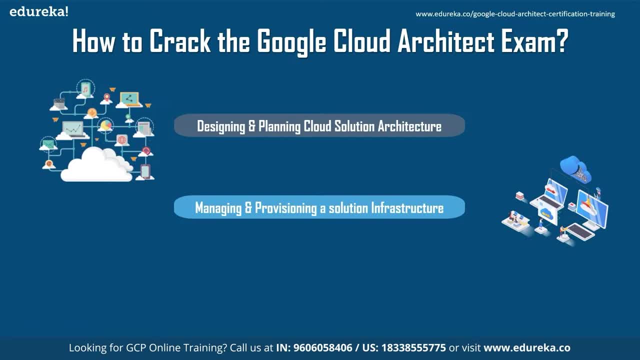 to a multi-cloud environment that may include google cloud to google cloud, include google cloud to google cloud, include google cloud to google cloud. communication, communication, communication. so one more thing is there, while so one more thing is there, while so one more thing is there while configuring network topologies, that is. 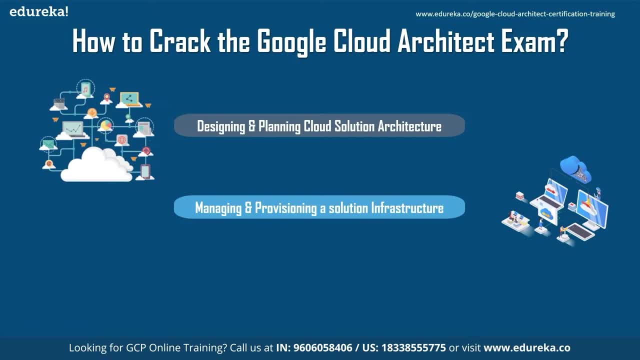 configuring network topologies. that is configuring network topologies. that is security protection also, while managing security protection also, while managing security protection also, while managing security and access management, as well as security and access management, as well as security and access management, as well as data growth planning also, like you. 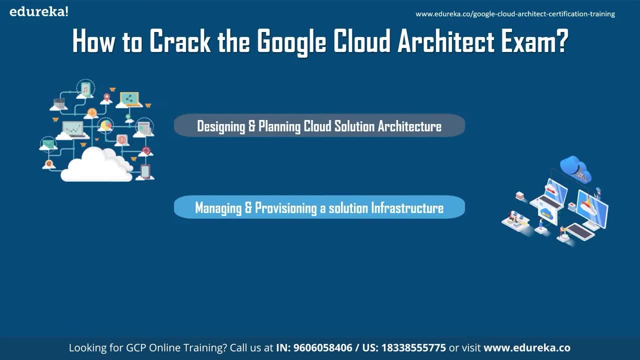 data growth planning also, like you. data growth planning also like you. should configure compute systems as well. should configure compute systems as well. should configure compute systems as well, while managing and provisioning. and you while managing and provisioning, and you while managing and provisioning, and you should consider compute resource. 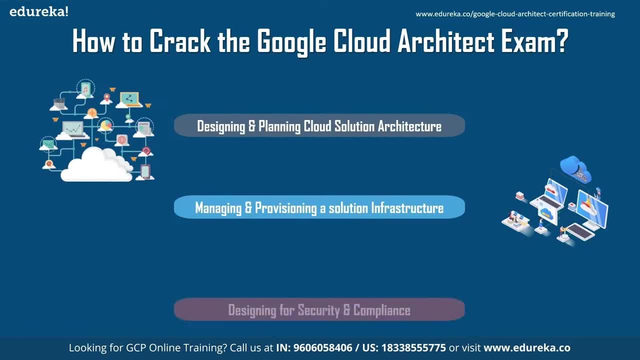 should consider compute resource, should consider compute resource provisioning for that and compute provisioning for that, and compute provisioning for that and compute volatility configuration as well, volatility configuration as well. volatility configuration as well. now, the third thing is: you should know. now, the third thing is: you should know. 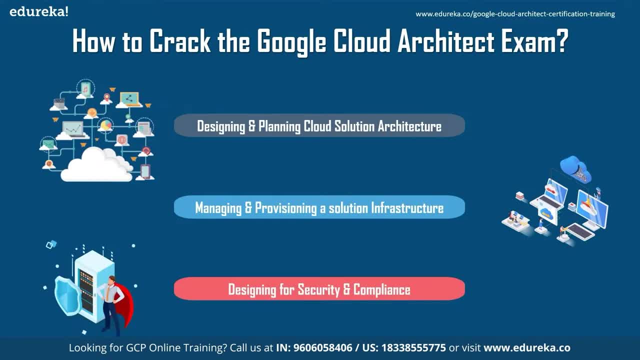 now the third thing is: you should know how to design for security and how to design for security and how to design for security and compliance. while designing for security, compliance, while designing for security, consider identity and access. consider identity and access. consider identity and access. management also like resource hierarchy. 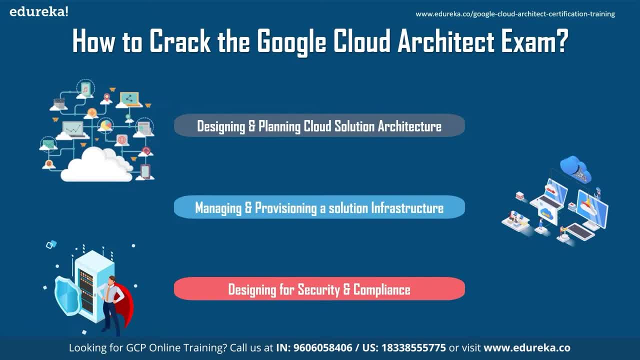 management also like resource hierarchy management also like resource hierarchy and data security and separation of and data security and separation of and data security and separation of duties and security controls like duties and security controls like duties and security controls like auditing vpc service controls, etc. auditing vpc service controls, etc. 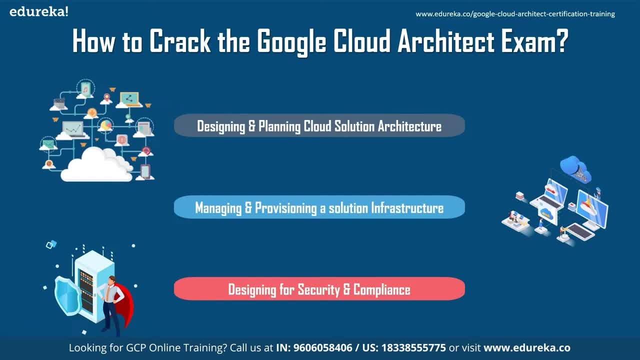 auditing vpc service controls, etc. and also like managing the customer. and also like managing the customer. and also like managing the customer: managed encryption keys with managed encryption keys, with managed encryption keys, with cloud key management services and cloud key management services and cloud key management services and remote access as well. 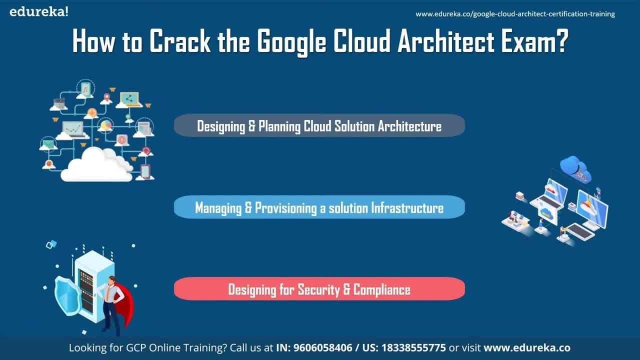 remote access as well. remote access as well. and second thing under designing and and second thing under designing and and second thing under designing. and security compliance is designing for security compliance, is designing for security compliance, is designing for compliance for that. consider compliance for that. consider compliance for that. consider legislation and commercial as well as. 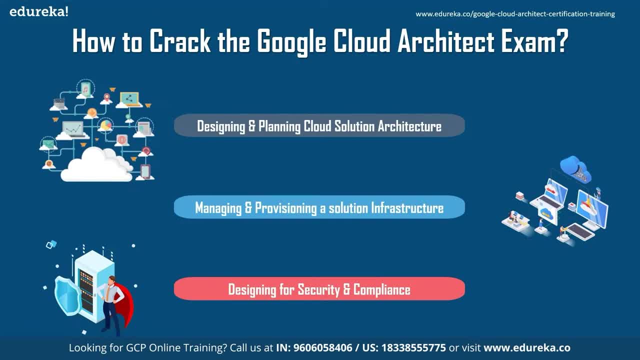 legislation and commercial, as well as legislation and commercial, as well as industry certifications and audits, as industry certifications and audits, as industry certifications and audits as well, well, well, like including logs. so the fourth step is like including logs. so the fourth step is like including logs. so the fourth step is analyzing, optimizing a technical and 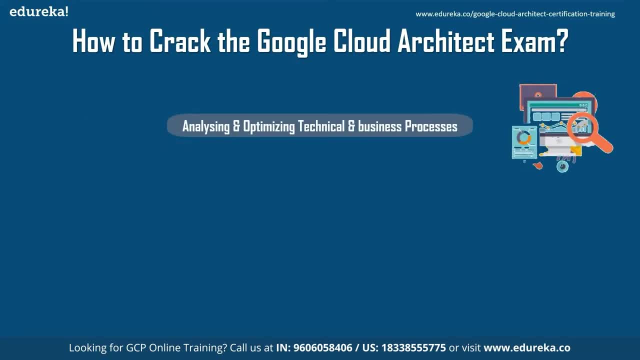 analyzing, optimizing a technical and analyzing, optimizing a technical and business process. so while analyzing and business process. so while analyzing and business process. so while analyzing and defining, defining, defining skill process, consider software skill process, consider software skill process, consider software development life cycle and development life cycle. and 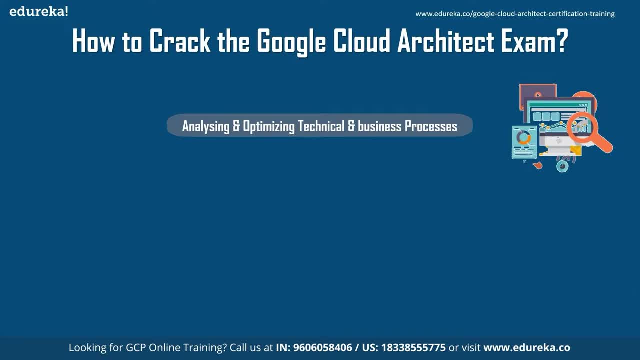 development life cycle and continuous integrations, or continuous continuous integrations, or continuous continuous integrations, or continuous deployment, as well as troubleshooting deployment, as well as troubleshooting deployment, as well as troubleshooting, and testing and validation of software, and testing and validation of software, and testing and validation of software infrastructure other than that service. 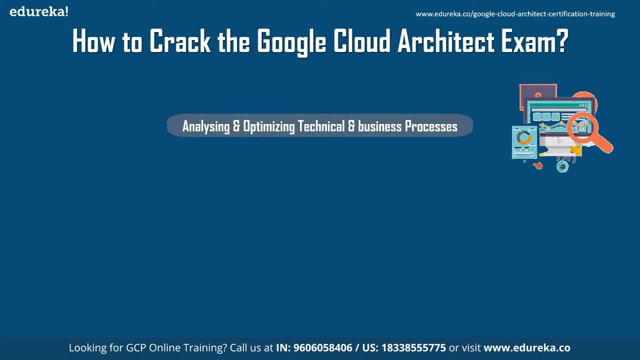 infrastructure other than that service infrastructure other than that service catalog and provisioning and business catalog and provisioning and business catalog and provisioning and business continuity and disaster recovery as well. continuity and disaster recovery as well. continuity and disaster recovery as well. second step is to analyze and define. second step is to analyze and define. 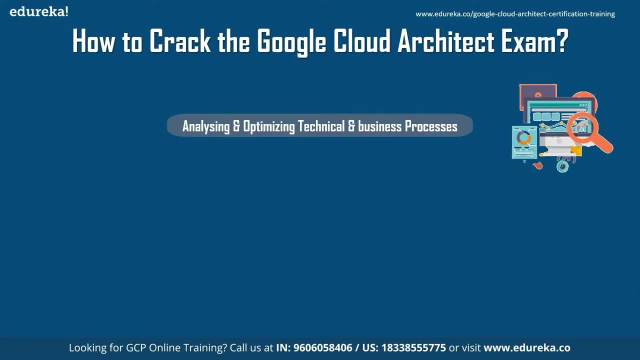 second step is to analyze and define business processes, and for that you need business processes, and for that you need business processes. and for that you need to consider, to consider, to consider stakeholder management, change management, stakeholder management, change management, stakeholder management, change management, team assessment, decision making. 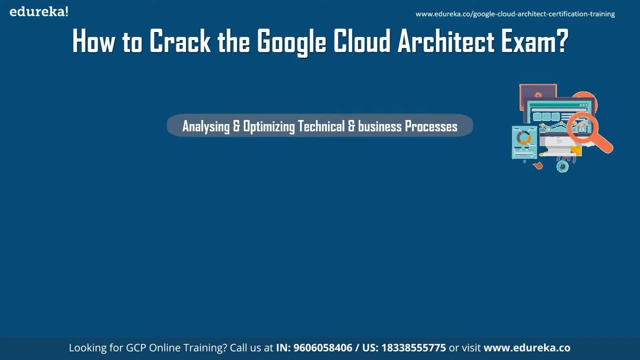 team assessment, decision making. team assessment, decision making processes. customer success management processes. customer success management processes, customer success management, cost optimization resource as well. cost optimization resource as well, cost optimization resource as well. third thing: under analyzing: optimizing. third thing under analyzing: optimizing. third thing: under analyzing: optimizing technical business processes developing. 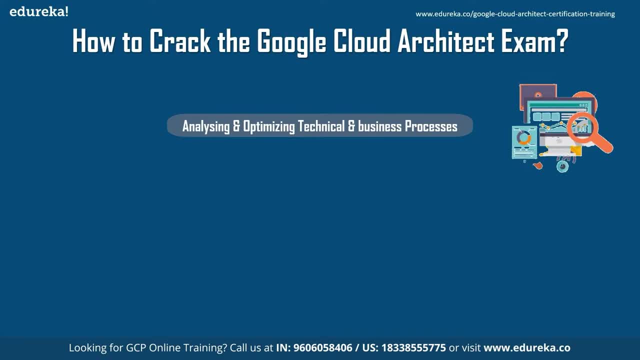 technical business processes, developing technical business processes, developing procedures to ensure reliability of procedures, to ensure reliability of procedures, to ensure reliability of solutions in production. like you can, solutions in production. like you can solutions in production, like you can take for example chaos engineering. and take for example chaos engineering and 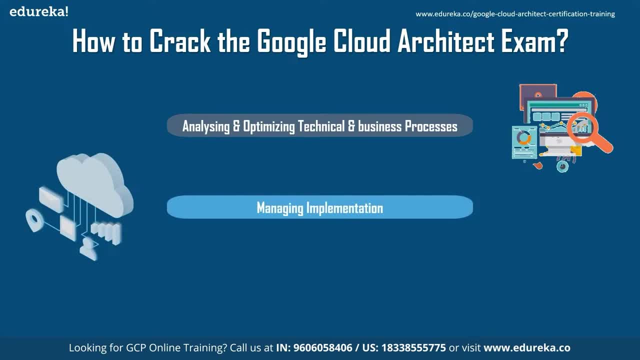 take, for example, chaos engineering and penetration testing. fifth step is penetration testing. fifth step is penetration testing. fifth step is managing implementation. so that can be managing implementation, so that can be managing implementation, so that can be done by advising development, or done by advising development, or done by advising development or operation teams, to ensure successful. 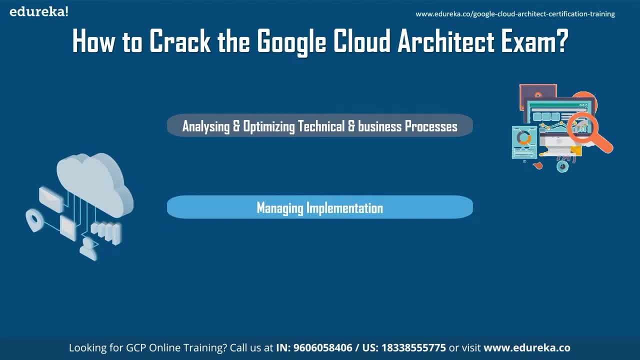 operation teams to ensure successful operation teams, to ensure successful deployment of the solutions and for deployment of the solutions and for deployment of the solutions and for that purpose. you need to consider that purpose, you need to consider that purpose. you need to consider application development api best. application development api best. 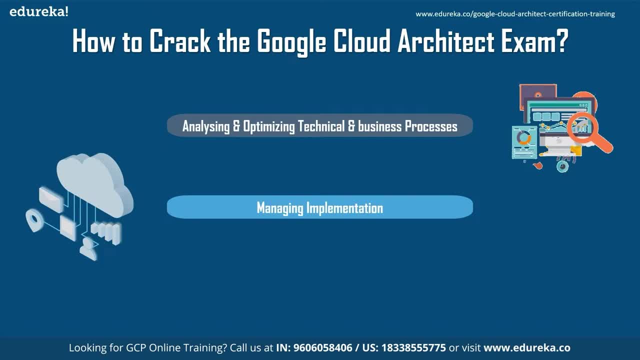 application development, api best practices, practices, practices, test framework and data and system test framework and data and system test framework and data and system migration and management tooling. so migration and management tooling. so migration and management tooling. so implementation can be managed also by. implementation can be managed also by. 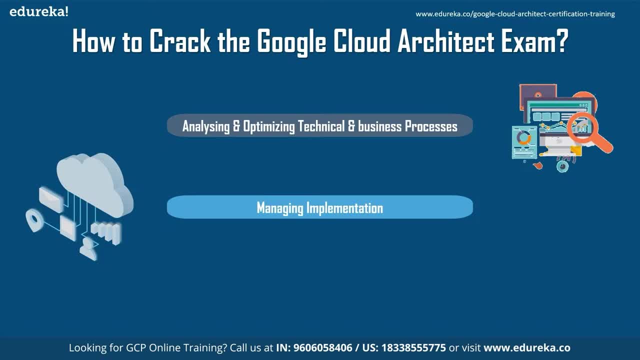 implementation can be managed also by interacting with the google cloud. interacting with the google cloud, interacting with the google cloud programmatically- and for that you need programmatically, and for that you need programmatically, and for that you need to consider google cloud shell google. to consider google cloud shell google. 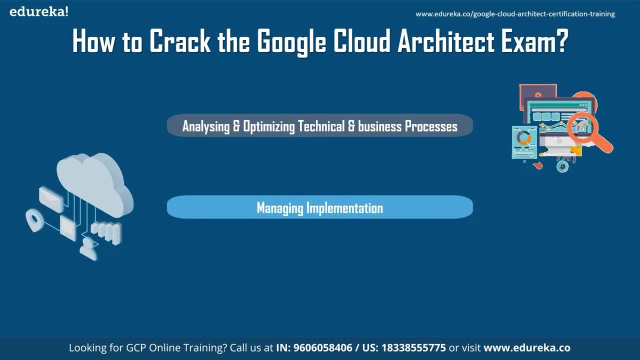 to consider google cloud shell, google cloud sdk also like cloud emulators. cloud sdk also like cloud emulators. cloud sdk also like cloud emulators means cloud bigtable data store spanner. means cloud bigtable data store spanner. means cloud bigtable data store spanner, pub server and fire store as well, etc. 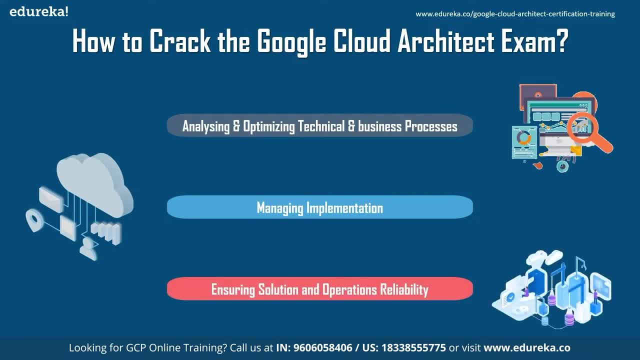 pub server and fire store as well, etc. pub server and fire store as well, etc. so the last step is ensuring solution, and so the last step is ensuring solution. and so the last step is ensuring solution and operations reliability, and for that operations reliability, and for that operations reliability. and for that you need to consider monitoring logging. 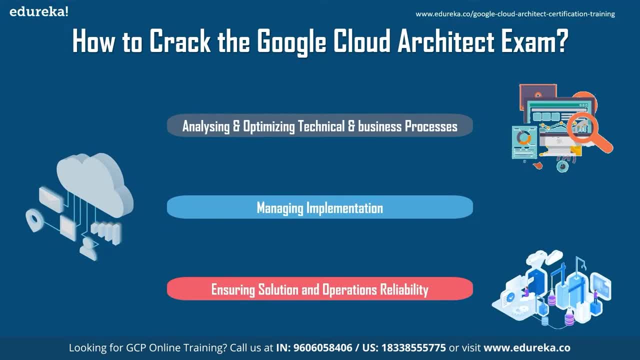 you need to consider monitoring logging. you need to consider monitoring logging. profiling editing solutions. as well as profiling editing solutions. as well as profiling editing solutions, as well as deployment and release management. deployment and release management. deployment and release management: assisting with the support of deployed. assisting with the support of deployed. 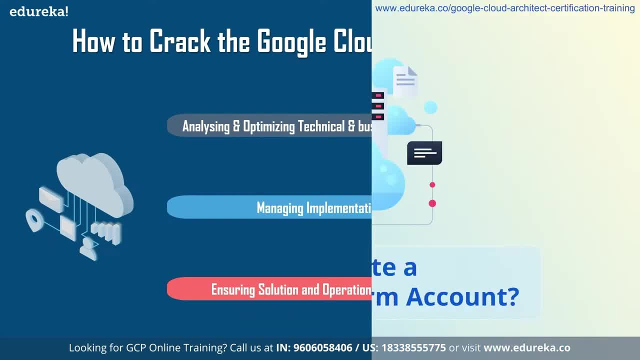 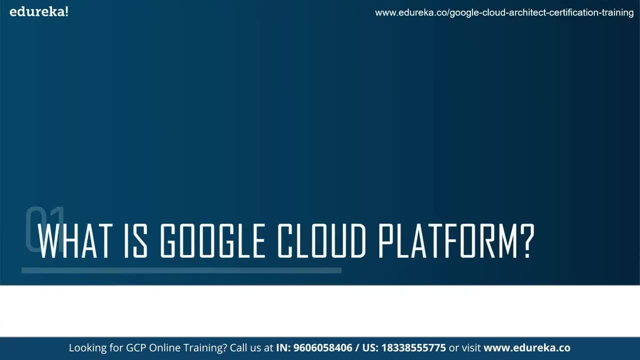 assisting with the support of deployed solutions and evaluating quality control solutions and evaluating quality control solutions and evaluating quality control measures. what is google cloud platform now google? what is google cloud platform now google? what is google cloud platform now google cloud platform is basically the cloud. cloud platform is basically the cloud. 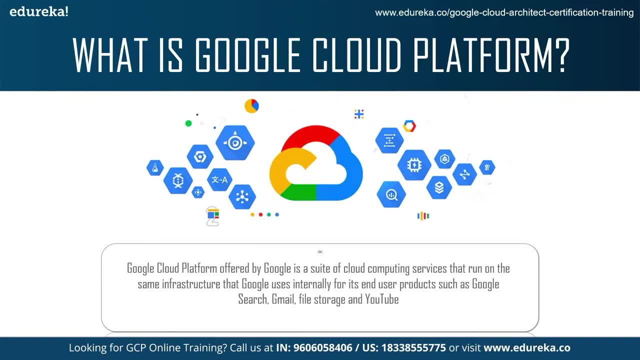 cloud platform is basically the cloud computing suite offered by google. so this computing suite offered by google, so this computing suite offered by google. so this suite basically consists of various. suite basically consists of various. suite basically consists of various cloud computing services that run on the cloud computing services that run on the. 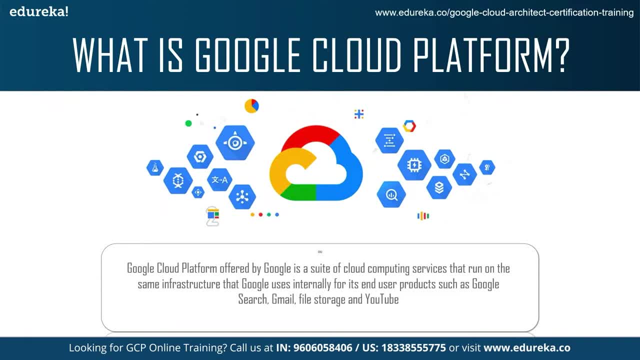 cloud computing services that run on the same infrastructure as all the other same infrastructure, as all the other same infrastructure, as all the other google services run on like, for example, google services run on like, for example, google services run on like, for example, let's say, google search, gmail and youtube. 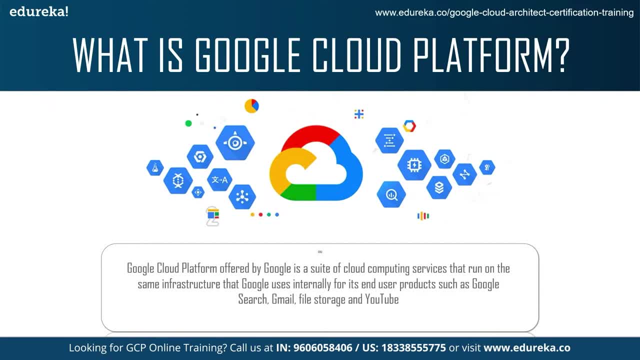 let's say google search gmail and youtube. let's say google search gmail and youtube. all of these services internally have all of these services internally have all of these services internally have certain structures and certain services, certain structures and certain services, certain structures and certain services that they run on, and google cloud. 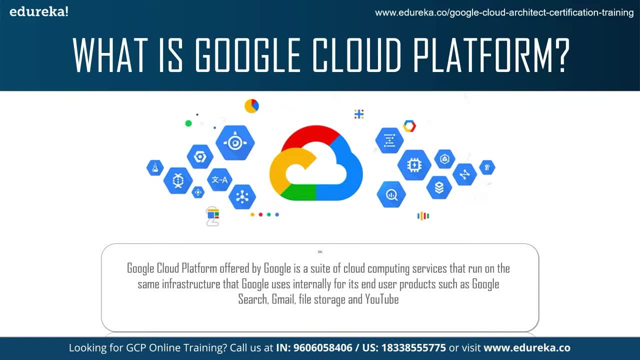 that they run on and google cloud that they run on, and google cloud platform has enabled us to basically use platform has enabled us to basically use. platform has enabled us to basically use the same services that they use, the same services that they use, the same services that they use internally. right, so next up, we come to. 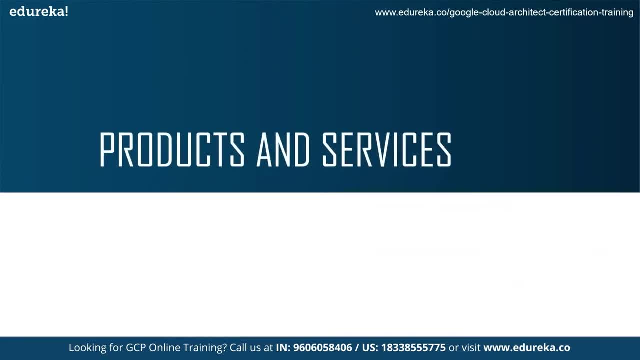 internally right. so next up, we come to internally right. so next up, we come to various products and services, that various products and services, that various products and services that google cloud platform has to offer, google cloud platform has to offer, google cloud platform has to offer. now, there are various products and 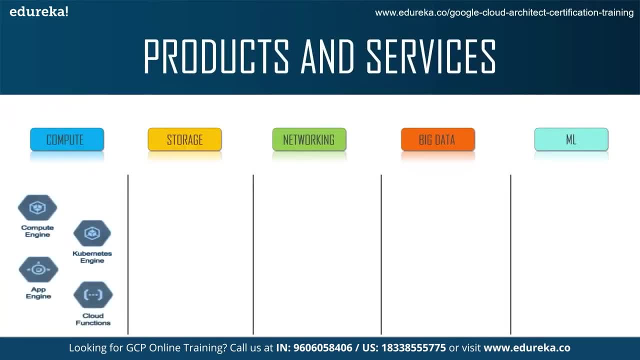 now there are various products and now there are various products and services, such as compute storage services, such as compute storage services, such as compute storage, networking, big data and machine learning, networking, big data and machine learning, networking, big data and machine learning. so, out of the compute products and 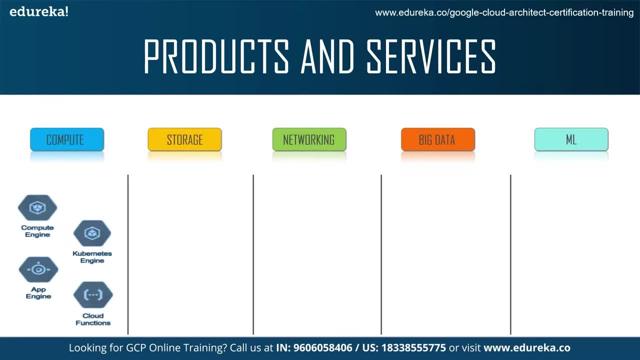 so, out of the compute products and services that there are, there is services that there are. there is services that there are. there is compute engine, the kubernetes engine, the compute engine, the kubernetes engine, the compute engine, the kubernetes engine, the app engine and the cloud functions. 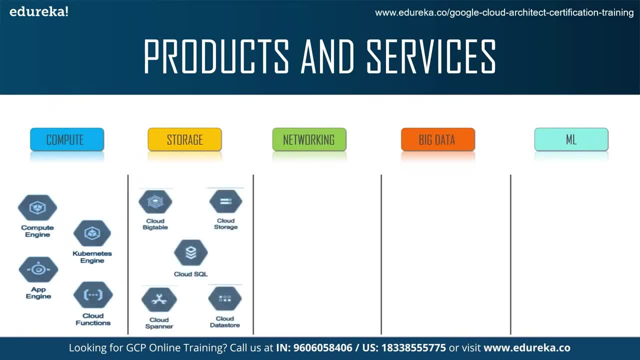 app engine and the cloud functions app engine and the cloud functions service when it comes to storage. google service when it comes to storage. google service when it comes to storage. google cloud platform offers its users. the cloud platform offers its users. the cloud platform offers its users the cloud big table, cloud storage, cloud sql. 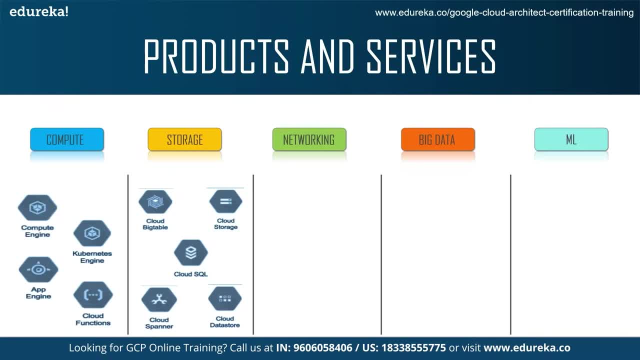 cloud big table, cloud storage, cloud sql- cloud big table cloud storage, cloud sql cloud planner. and finally the cloud data cloud planner and finally the cloud data cloud planner and finally the cloud data store. when we're talking about store, when we're talking about store, when we're talking about networking, there are various services. 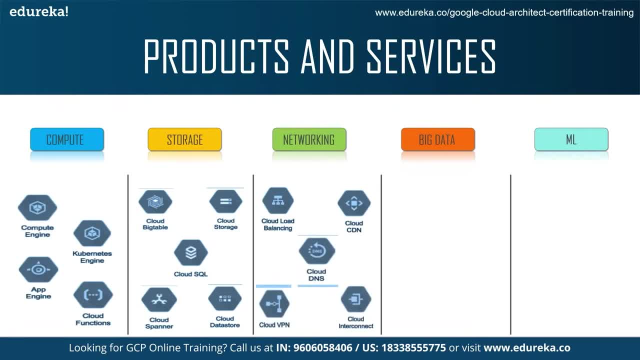 networking. there are various services networking. there are various services that are there, such as the cloud load that are there, such as the cloud load that are there, such as the cloud load balancing, cloud cdn, cloud dns, cloud vpn, balancing cloud cdn, cloud dns, cloud vpn balancing cloud cdn, cloud dns, cloud vpn and, finally, the cloud interconnect right. 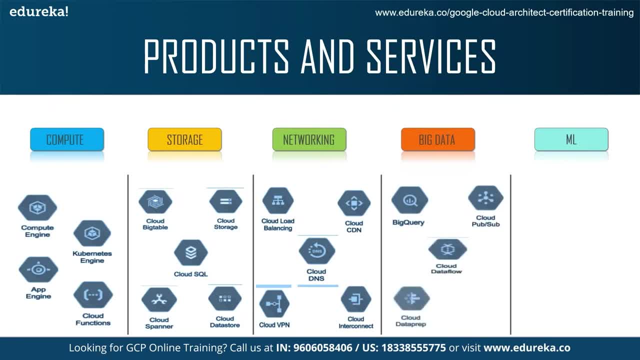 and finally the cloud interconnect right and finally the cloud interconnect right. and when it comes to big data, there are, and when it comes to big data, there are, and when it comes to big data, there are services such as bigquery pub sub data, services such as bigquery pub sub data. 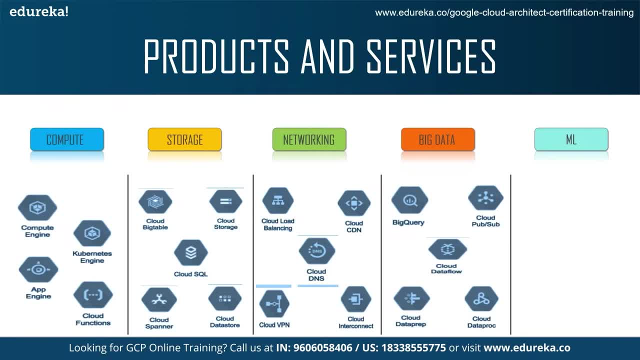 services such as bigquery, pub, sub data flow, etc. and finally we have the flow, etc. and finally we have the flow, etc. and finally we have the machine learning services, such as the machine learning services, such as the machine learning services, such as the cloud, ml, the vision, api, the google text. 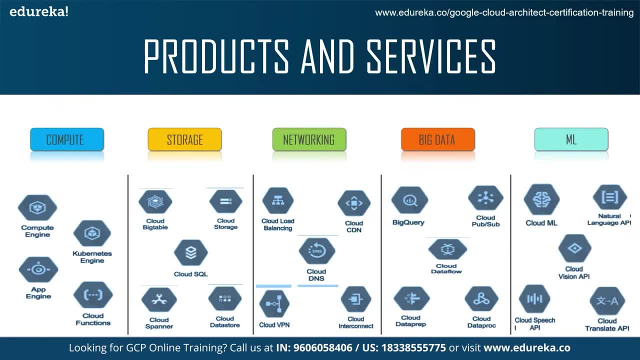 cloud ml, the vision api, the google text cloud ml, the vision api, the google text speech api, speech api, speech api and other such services. right so these and other such services. right so these and other such services. right so these are the various products and services. are the various products and services. 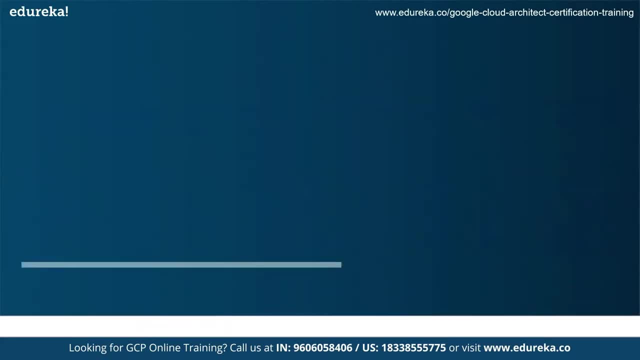 are the various products and services that are present in google cloud, that are present in google cloud, that are present in google cloud platform, platform platform. next, we talk about google cloud free. next, we talk about google cloud free. next, we talk about google cloud free tire. now, free tire is basically: 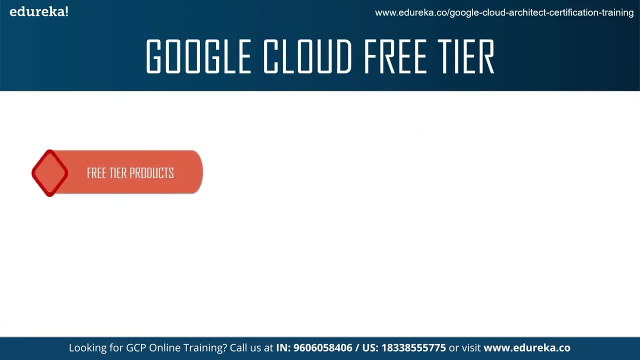 tire. now, free tire is basically tire. now, free tire is basically something that is accessible to users, something that is accessible to users, something that is accessible to users which allows users to use various, which allows users to use various, which allows users to use various services, services, services- free, of course, for a certain time. 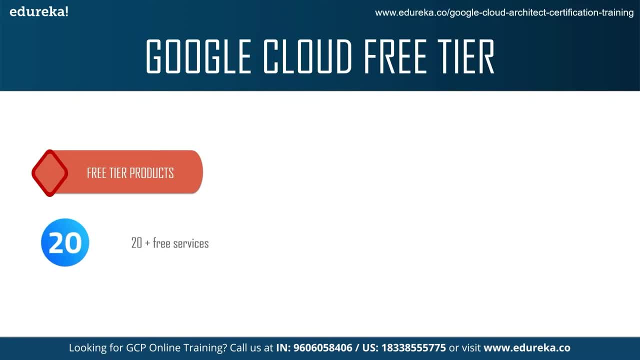 free, of course, for a certain time. free, of course, for a certain time limit. now there are over 20 free services limit. now there are over 20 free services limit. now there are over 20 free services and there is 300, and there is 300. 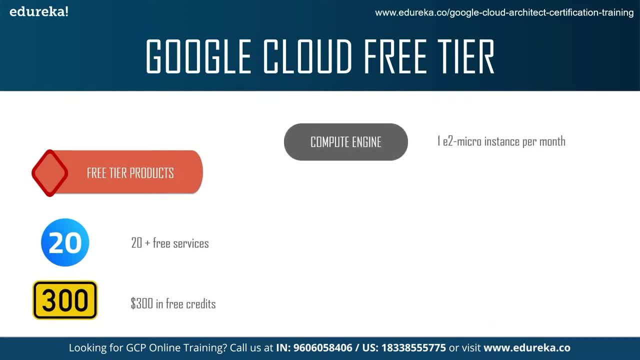 and there is 300 in free credits for every user, some of in free credits for every user, some of in free credits for every user. some of the services are the compute engine. the services are the compute engine. the services are the compute engine. now the free tire limit for compute. 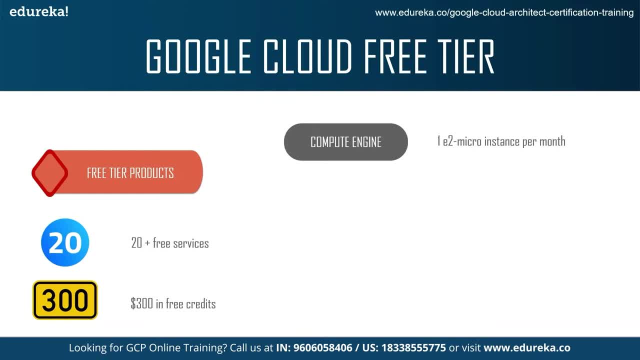 now the free tire limit for compute. now the free tire limit for compute engine engine engine is one e2 micro instance per month. is one e2 micro instance per month. is one e2 micro instance per month. next, we come to cloud storage- now free. next, we come to cloud storage- now free. 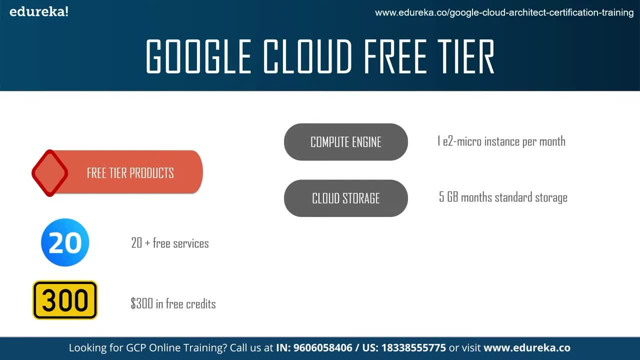 next we come to cloud storage. now, free tire limit for cloud storage. similarly, tire limit for cloud storage. similarly tire limit for cloud storage. similarly, is 5gb month standard storage right. so is 5gb month standard storage right. so is 5gb month standard storage right. so, for each month, there is 5gb free storage. 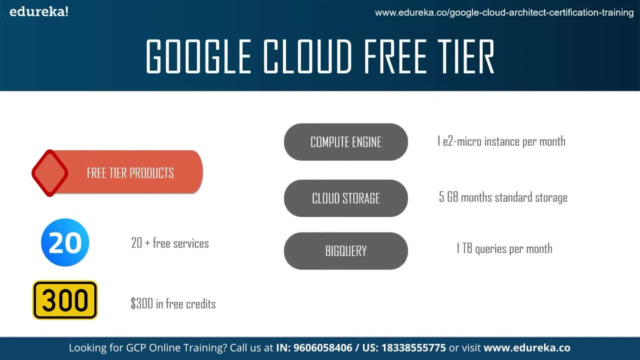 for each month. there is 5gb free storage for each month. there is 5gb free storage with google cloud storage, with google cloud storage, with google cloud storage. next up. we have bigquery now with next up. we have bigquery now with next up. we have bigquery now with bigquery. it basically 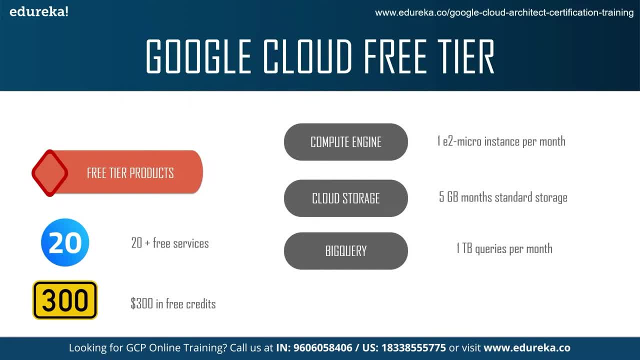 bigquery. it basically bigquery. it basically allows you to have one tb queries per. allows you to have one tb queries per. allows you to have one tb queries per month and, it being a big data month, and it being a big data month and it being a big data service, it has to have a lot of queries. 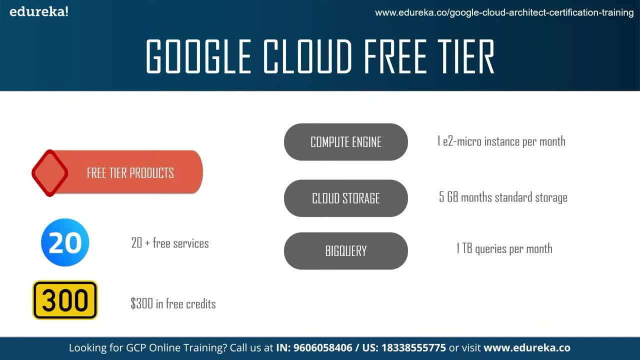 service. it has to have a lot of queries service. it has to have a lot of queries and a lot of analytics and insights, and a lot of analytics and insights, and a lot of analytics and insights every month. so it allows every month. so it allows every month. so it allows every user one tb queries per month. 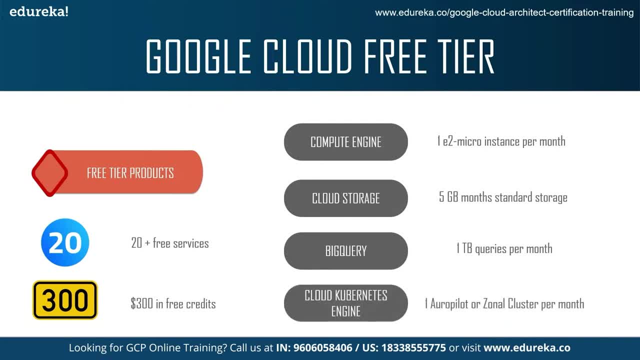 every user: one tb queries per month. every user: one tb queries per month. and then we have basically the cloud, and then we have basically the cloud, and then we have basically the cloud kubernetes engine, kubernetes engine, kubernetes engine and this cloud kubernetes engine will. 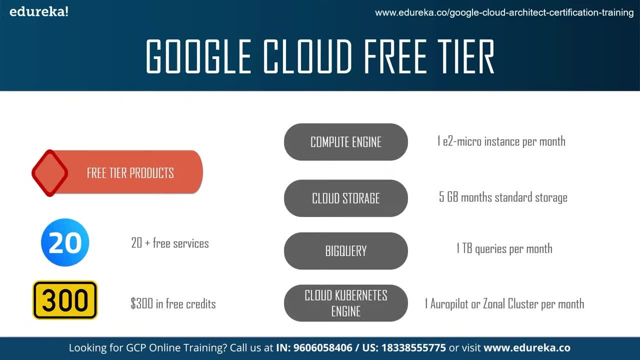 and this cloud kubernetes engine will. and this cloud kubernetes engine will basically have a free tire limit for basically have a free tire limit, for basically have a free tire limit for one autopilot or one zodon cluster per one autopilot or one zodon cluster per. 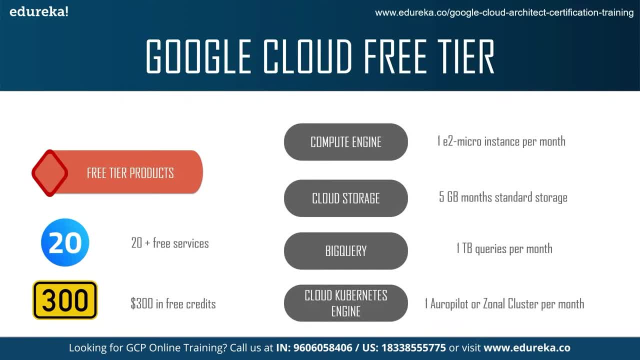 one autopilot or one zodon cluster per month, month, month. so these are the basic free tire. so these are the basic free tire. so these are the basic free tire limitations for some of the services limitations for some of the services limitations for some of the services that are present in google cloud. 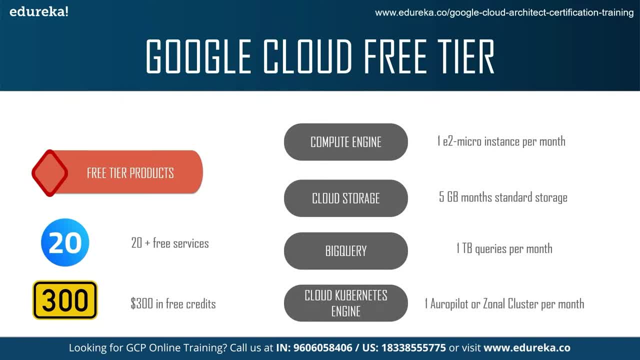 that are present in google cloud, that are present in google cloud platform, and the basic gist of what platform and the basic gist of what platform and the basic gist of what google cloud free tire has to offer its google cloud free tire has to offer. its google cloud free tire has to offer its users. 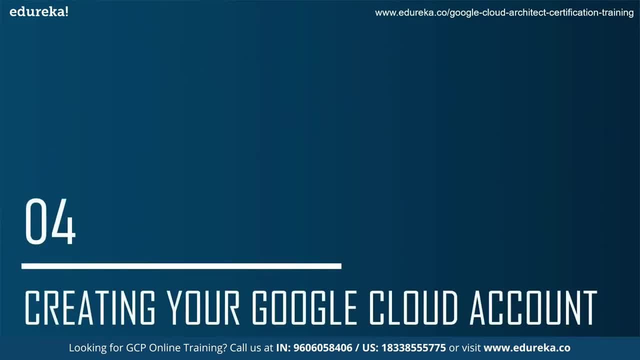 users, users. next, we come to creating your own google. next, we come to creating your own google. next, we come to creating your own google cloud account, cloud account, cloud account. so basically, when you type google cloud, so basically when you type google cloud, so basically when you type google cloud platform on google, you get something. 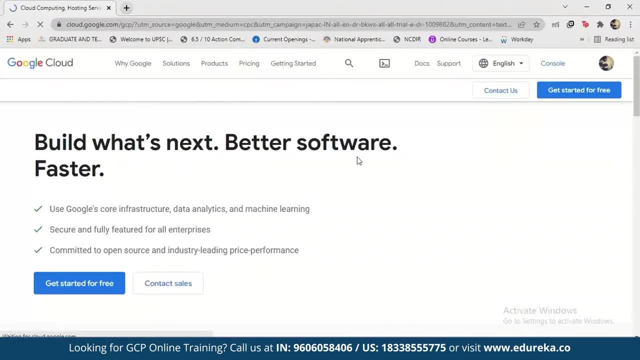 platform on google, you get something. platform on google, you get something like this, like this, like this: go on the first link and this is what go on the first link and this is what go on the first link, and this is what you get. you get, you get. now, what you need to do here is just 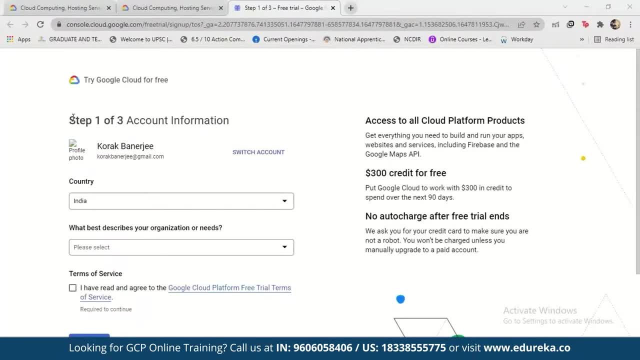 now. what you need to do here is just now. what you need to do here is just click on get started for free. click on get started for free. click on get started for free. uh, so basically, when you click on this, uh, so basically, when you click on this. 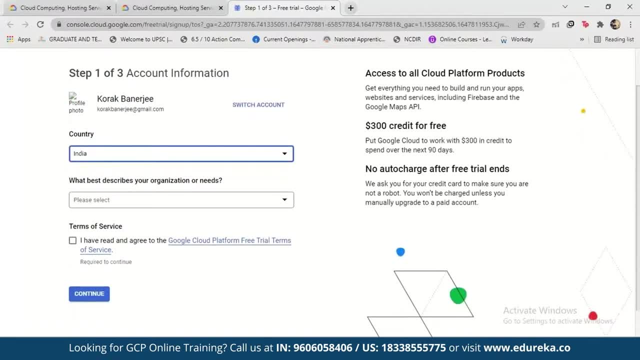 uh, so basically, when you click on this, you'll get this page, you'll get this page, you'll get this page. and here it asks some basic information. and here it asks some basic information. and here it asks some basic information for you, for you, for you like your country, and what you need to. 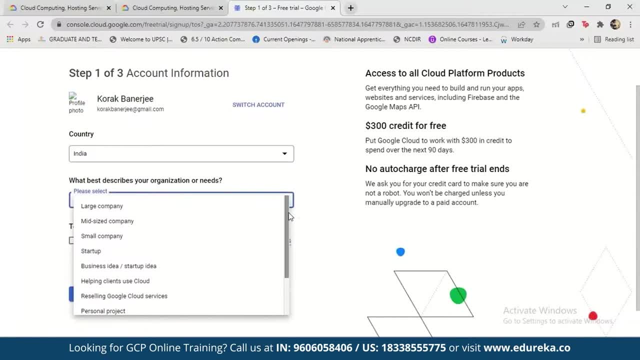 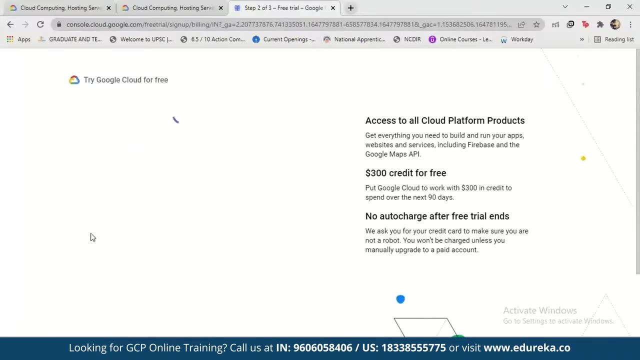 like your country and what you need to like your country and what you need to do now. if you need organization, do now. if you need organization, do now. if you need organization, just click on continue and just click on continue and just click on continue and basically just. 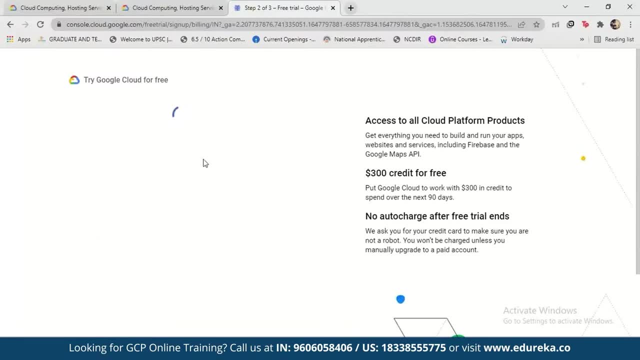 basically, just, basically, just go ahead, add your number and click on. go ahead, add your number and click on. go ahead, add your number and click on. continue again, continue again, continue again, right, right, right. so what you have to do here is just add. so what you have to do here is just add. 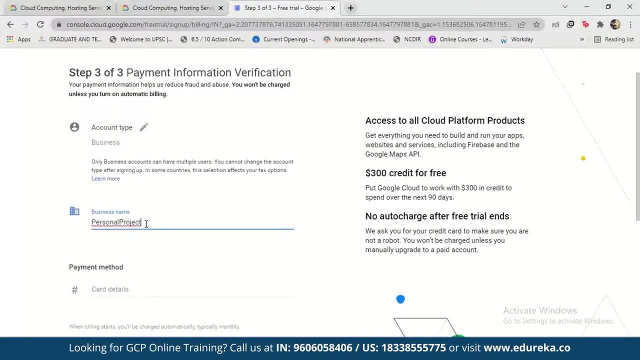 so what you have to do here is just add your method of payment, your method of payment, your method of payment now. this is the part where you have to now. this is the part where you have to now. this is the part where you have to basically add the payment information. 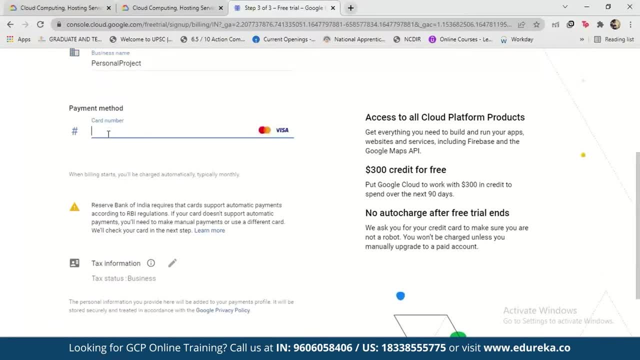 basically add the payment information, basically add the payment information and let's just say: put the card details. and let's just say: put the card details and let's just say: put the card details in here, in here, in here, right and just right and just right, and just select these. so, basically, once you've 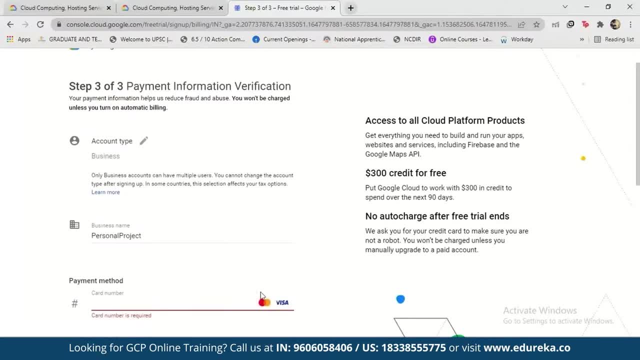 select these. so, basically, once you've select these, so basically, once you've done with your card details, done with your card details, done with your card details and you've made the transaction there'll, and you've made the transaction there'll, and you've made the transaction, there'll be two rupees deducted from your. 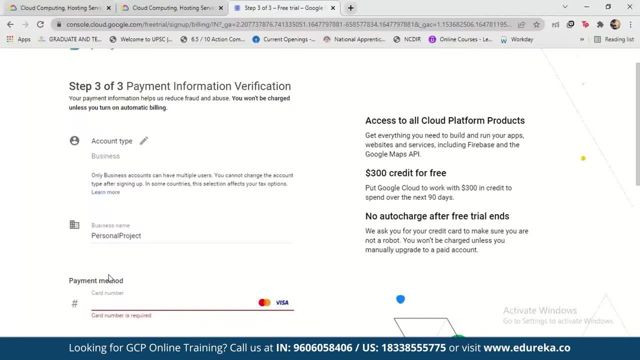 be two rupees deducted from your, be two rupees deducted from your account, account, account. that is basically the basic amount of. that is basically the basic amount of that is basically the basic amount of money that google has to money that google has to money that google has to make first time. verifying that it is you. 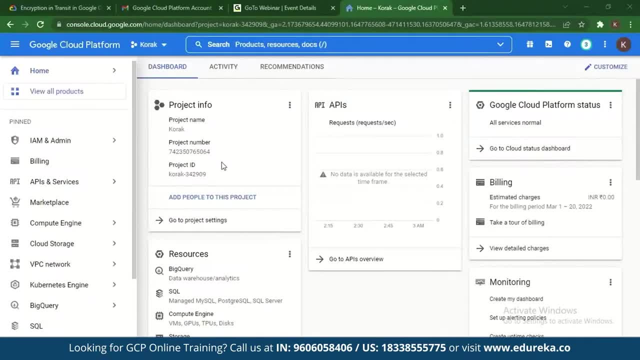 make first time, verifying that it is you make first time, verifying that it is you who's basically making the transaction, who's basically making the transaction, who's basically making the transaction? and so, finally, when you've actually made, and so, finally, when you've actually made, and so, finally, when you've actually made the payment. 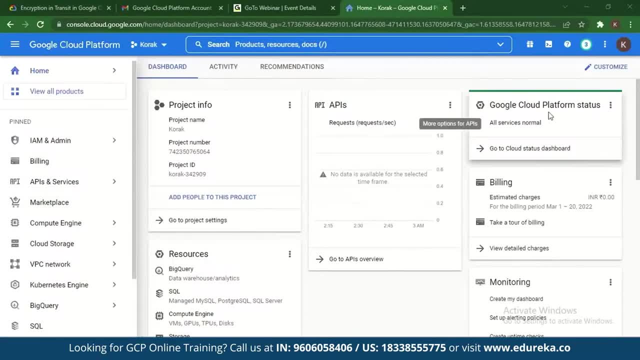 the payment, the payment. what you can see is you can log into the. what you can see is you can log into the. what you can see is you can log into the console, and this is what the dashboard console and this is what the dashboard console and this is what the dashboard looks like and what you can do here is. 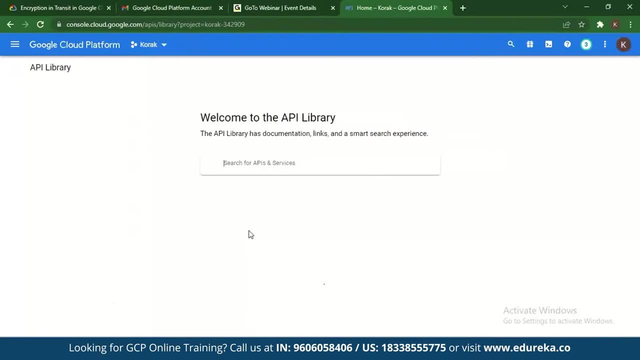 looks like and what you can do here is looks like and what you can do here is: you can go to apis and services go to. you can go to apis and services go to. you can go to apis and services. go to library, library, library and check out the various services that. 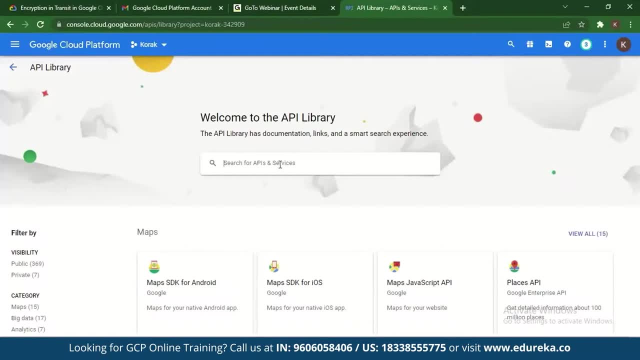 and check out the various services that and check out the various services that google cloud platform has to offer. google cloud platform has to offer. google cloud platform has to offer. let's check out. let's say, for example: let's check out. let's say, for example: let's check out. let's say, for example, compute engine. 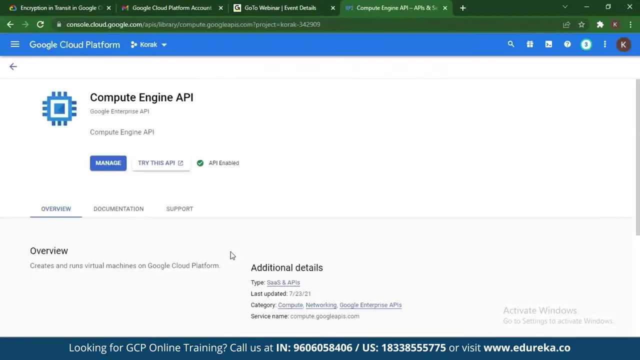 compute engine, compute engine. right, so this is a compute engine api. right, so, this is a compute engine api. right, so this is a compute engine api and i can just manage this and try and, and i can just manage this and try and, and i can just manage this and try and enable this. so what you have to do, 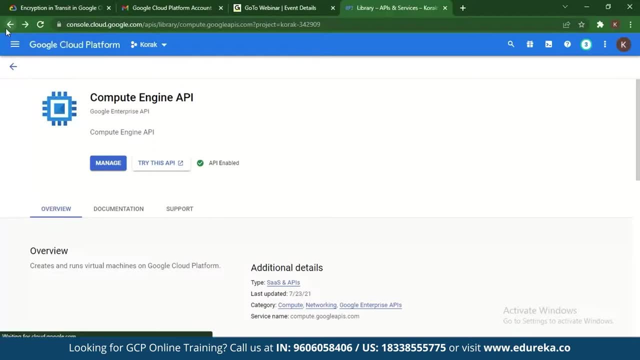 enable this. so what you have to do, enable this. so what you have to do basically is basically, is basically is: try and enable any api that you use. try and enable any api that you use. try and enable any api that you use, and that is how you basically use. 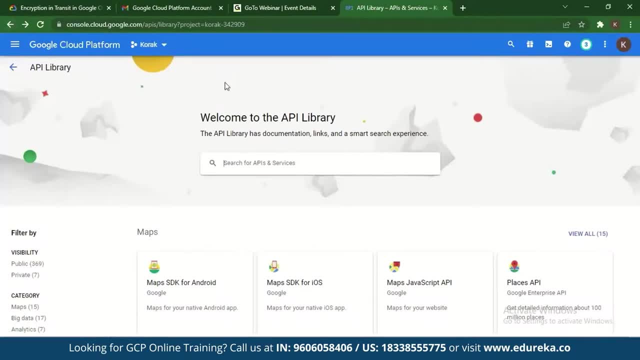 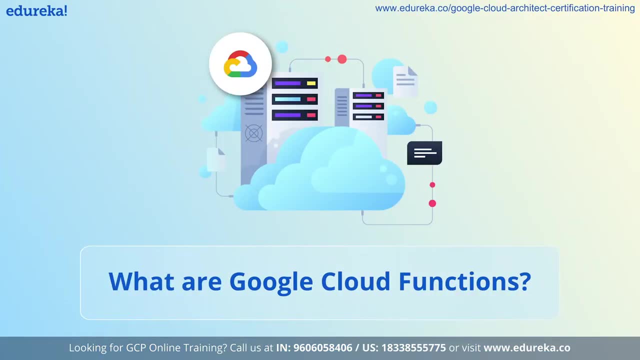 and that is how you basically use. and that is how you basically use google cloud platform in general and google cloud platform in general and google cloud platform in general, and this is how you create your google. this is how you create your google. this is how you create your google cloud platform account. 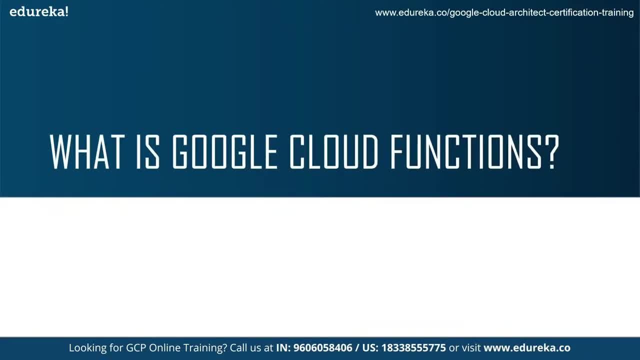 what is google cloud functions now when? what is google cloud functions now when? what is google cloud functions now? when we talk about google cloud functions, we, we talk about google cloud functions. we we talk about google cloud functions. we need to know that cloud functions is an need to know that cloud functions is an 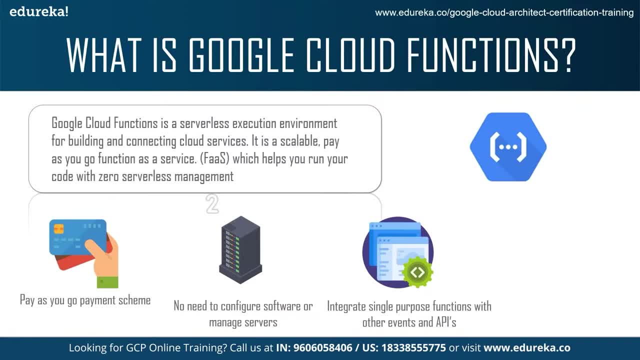 need to know that cloud functions is an api which is provided by google cloud api, which is provided by google cloud api, which is provided by google cloud platform. so this is basically a platform. so this is basically a platform. so this is basically a serverless execution environment for. 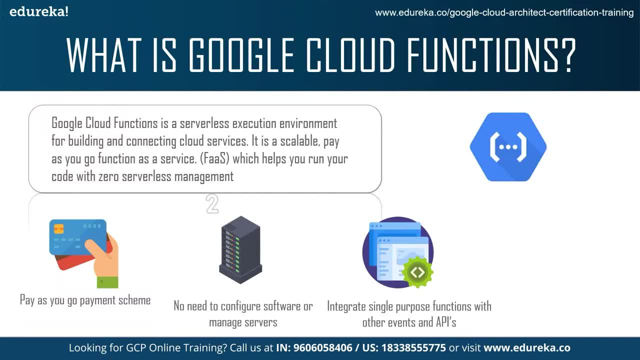 serverless execution environment for serverless execution environment for building and connecting cloud services. building and connecting cloud services. building and connecting cloud services- right, so it's scalable. and pay as you. right, so it's scalable. and pay as you. right, so it's scalable. and pay as you go, so you need to only pay for the. 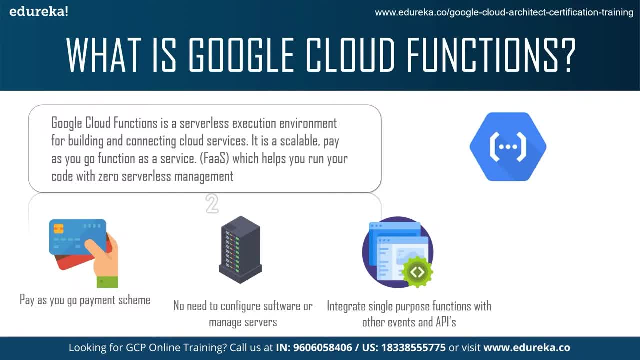 go. so you need to only pay for the go. so you need to only pay for the amount of time that you use the function, amount of time that you use the function, amount of time that you use the function for. so it is basically a function as a. 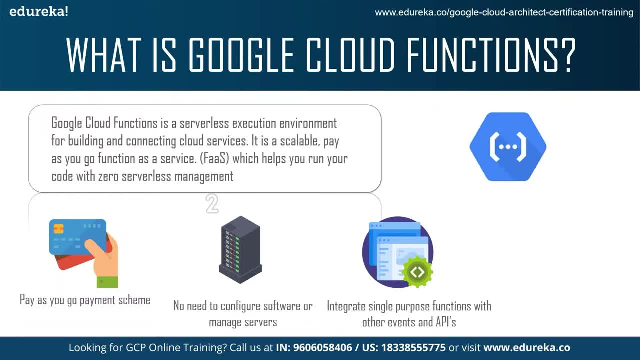 for, so it is basically a function as a for. so it is basically a function as a service that is provided by google cloud service. that is provided by google cloud service. that is provided by google cloud platform, which allows you to pay as you platform, which allows you to pay as you. 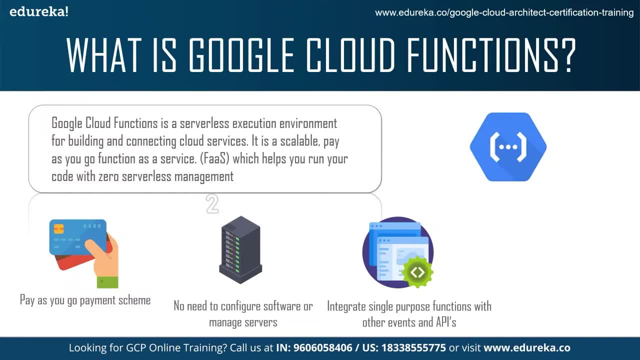 platform which allows you to pay as you go, which basically means that you only go, which basically means that you only go, which basically means that you only have to pay for the amount of time and have to pay for the amount of time, and have to pay for the amount of time and the amount of data and resources that 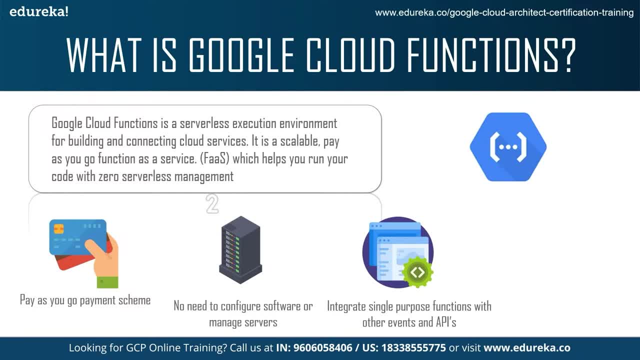 the amount of data and resources, that the amount of data and resources that you use for your cloud functions and you use for your cloud functions and you use for your cloud functions, and nothing extra. next, we talk about the nothing extra. next, we talk about the nothing extra. next, we talk about the fact that it you do not need to configure. 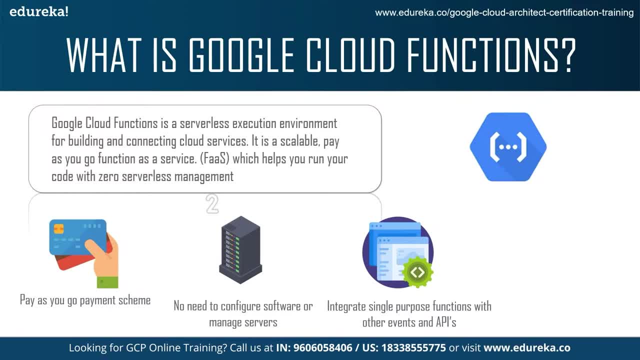 fact that it you do not need to configure, fact that it you do not need to configure the software and manage the service as the software, and manage the service as the software and manage the service as well. it is basically allowing you. well, it is basically allowing you. 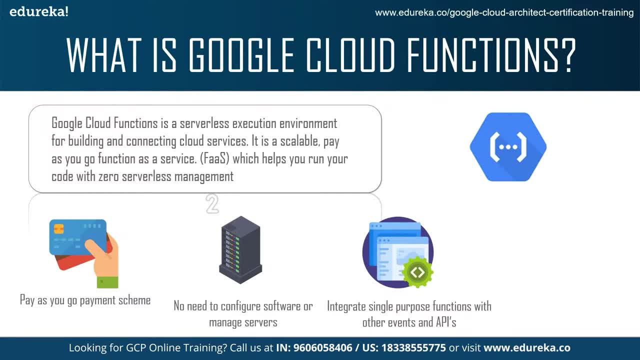 well, it is basically allowing you serverless management and you can serverless management and you can serverless management and you can basically integrate single purpose, basically integrate single purpose. basically integrate single purpose functions with other events and apis as functions with other events and apis as functions with other events and apis as well. so this is basically a brief. 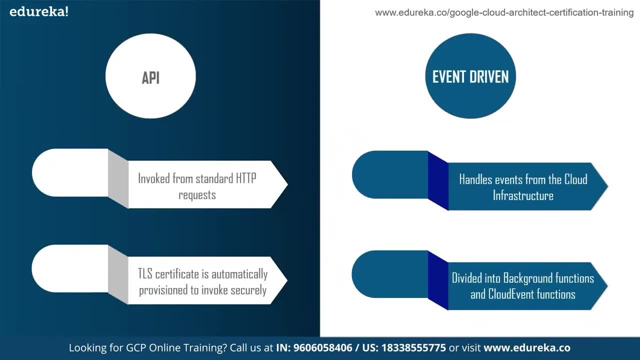 well, so this is basically a brief. well, so this is basically a brief overview of what cool cloud functions is. overview of what cool cloud functions is. overview of what cool cloud functions is. next we talk about the different kinds. next we talk about the different kinds. next we talk about the different kinds of cloud functions that are present. so 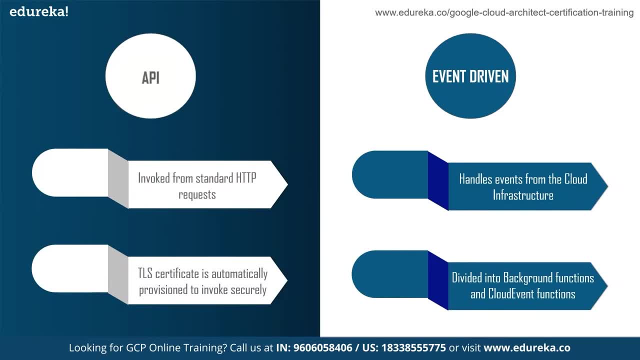 of cloud functions that are present. so of cloud functions that are present. so there are basic two different kinds of. there are basic two different kinds of. there are basic two different kinds of cloud functions present, namely api cloud cloud functions present, namely api cloud cloud functions present, namely api cloud functions and event-driven cloud. 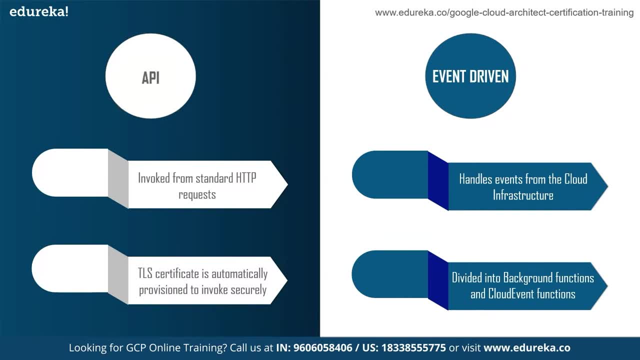 functions and event-driven cloud functions and event-driven cloud functions. so basically api cloud functions functions. so basically api cloud functions functions. so basically api cloud functions are invoked from standard http. are invoked from standard http. are invoked from standard http. requests: event-driven cloud functions. requests: event-driven cloud functions. 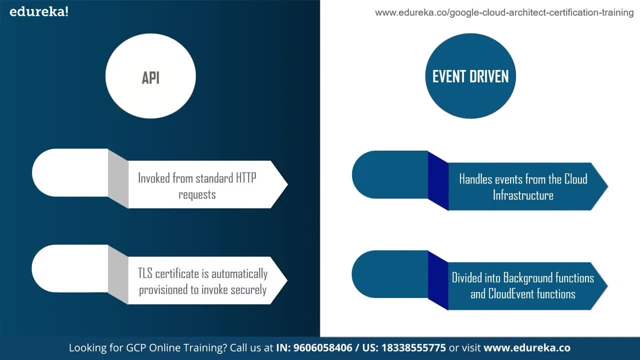 requests, event-driven cloud functions, handles events from the cloud. handles events from the cloud, handles events from the cloud infrastructure and basically can be infrastructure and basically can be infrastructure and basically can be invoked apart from http requests as well invoked apart from http requests as well invoked apart from http requests as well. then we see that the tls certificate is. 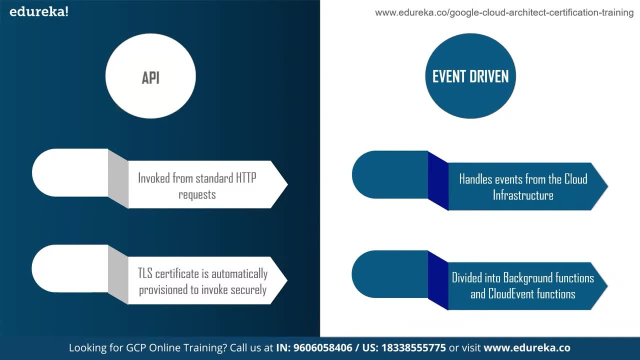 then we see that the tls certificate is, then we see that the tls certificate is automatically provisioned to invoke, automatically provisioned to invoke, automatically provisioned to invoke securely, which is basically for api securely, which is basically for api securely, which is basically for api cloud functions. now, when it comes to 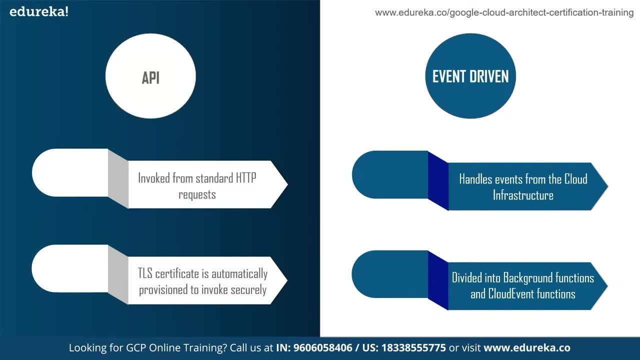 cloud functions. now, when it comes to cloud functions, now, when it comes to event-driven cloud functions, it is event-driven cloud functions. it is event-driven cloud functions. it is divided into background functions and divided into background functions and divided into background functions and cloud event functions. now, these are the. 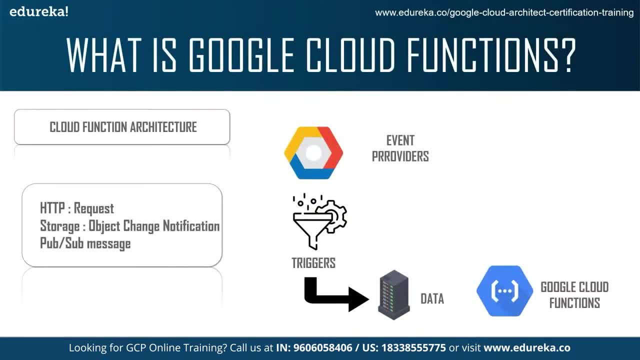 cloud event functions. now, these are the cloud event functions. now. these are the two basic types of cloud functions. next, two basic types of cloud functions. next, two basic types of cloud functions. next, we see the basic infrastructure of cloud. we see the basic infrastructure of cloud. we see the basic infrastructure of cloud functions. we see that the event 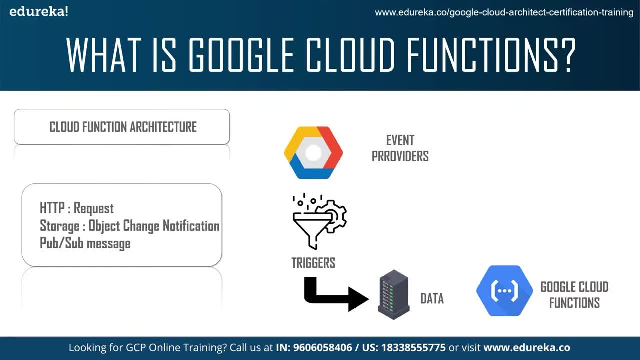 functions. we see that the event functions. we see that the event providers provide you with a trigger. providers provide you with a trigger. providers provide you with a trigger which then goes and gets stored in that, which then goes and gets stored in that, which then goes and gets stored in that, in the data, and this trigger will then 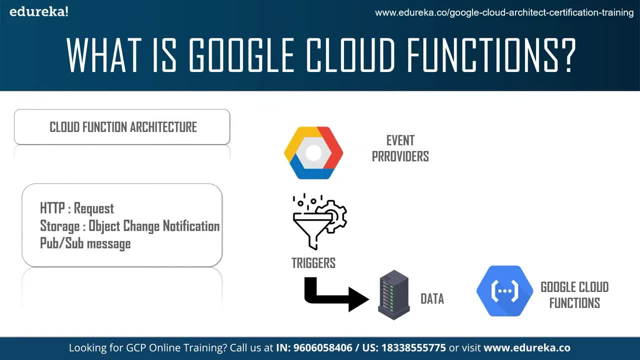 in the data and this trigger will then in the data and this trigger will then send you a response according to your. send you a response according to your. send you a response according to your function, that you have, and that is function that you have, and that is. 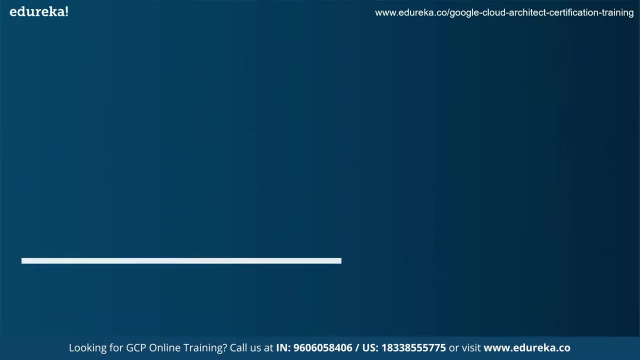 function that you have, and that is basically how cloud functions work. basically how cloud functions work. basically how cloud functions work- okay. next up, we see why use cloud. okay. next up, we see why use cloud. okay. next up, we see why use cloud functions at all. now, here we talk about. 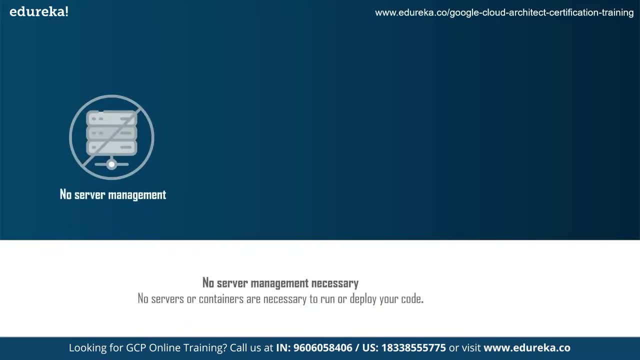 functions at all. now, here we talk about functions at all. now, here we talk about most of the things that are the features, most of the things that are the features, most of the things that are the features of cloud functions, or why do we need them- of cloud functions, or why do we need them. 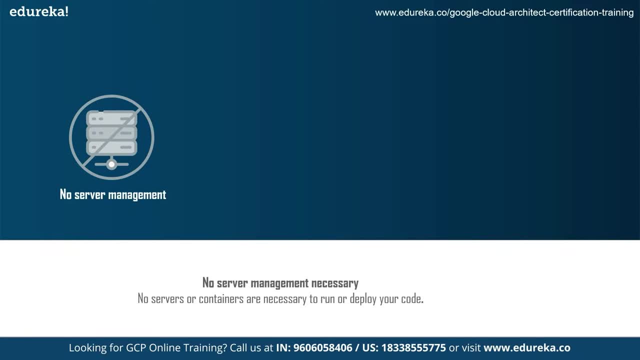 of cloud functions, or why do we need them at all? what does cloud function have to at all? what does cloud function have to at all? what does cloud function have? to? provide us with right, so the first. and provide us with right, so the first. and provide us with right, so the first, and the most important thing we see is that 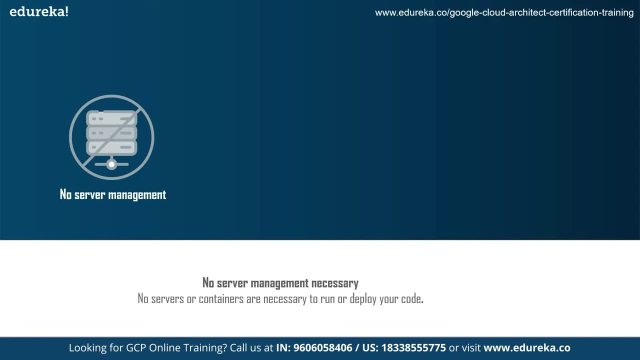 the most important thing we see is that. the most important thing we see is that you do not need server management. no, you do not need server management. no, you do not need server management. no, server management is necessary. or server management is necessary, or server management is necessary, or containers as well, to run or deploy your 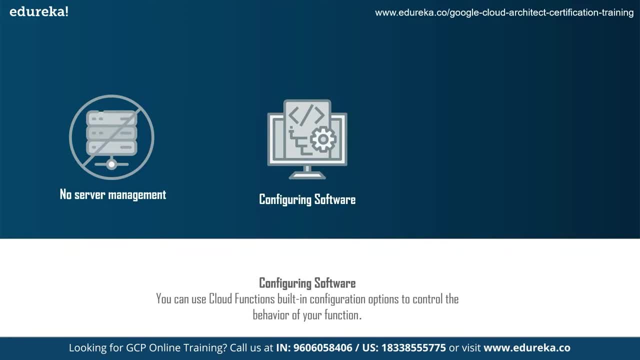 containers as well. to run or deploy your containers as well. to run or deploy your code. next, we see that configuring code. next, we see that configuring code. next, we see that configuring software is extremely important. so you software is extremely important. so you software is extremely important so you can configure cloud functions built-in. 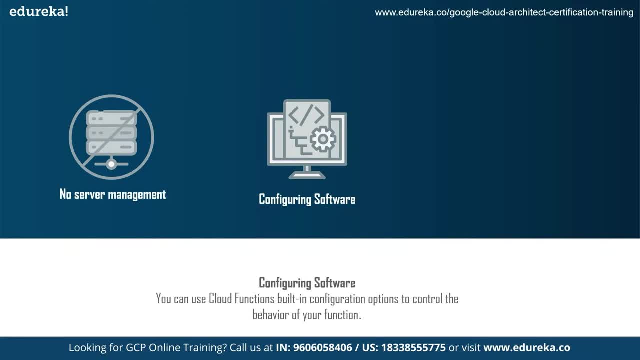 can configure cloud functions built-in, can configure cloud functions built-in configuration options to control the configuration options, to control the configuration options, to control the behavior of your functions. so you can behavior of your functions. so you can behavior of your functions. so you can basically configure it based on. 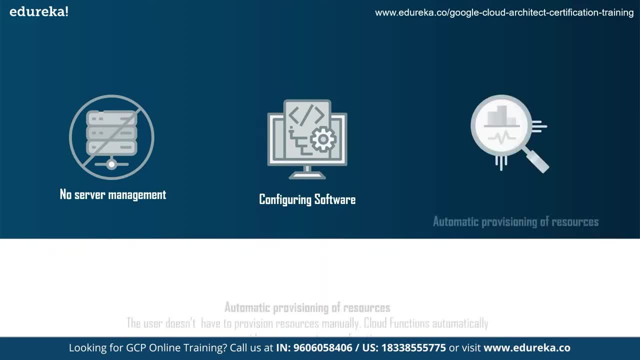 basically configure it based on: basically configure it based on whatever you feel like is the best for whatever you feel like is the best for. whatever you feel like is the best for your function. next up, we see the your function. next up, we see the your function. next up, we see the automatic provisioning of resources. now 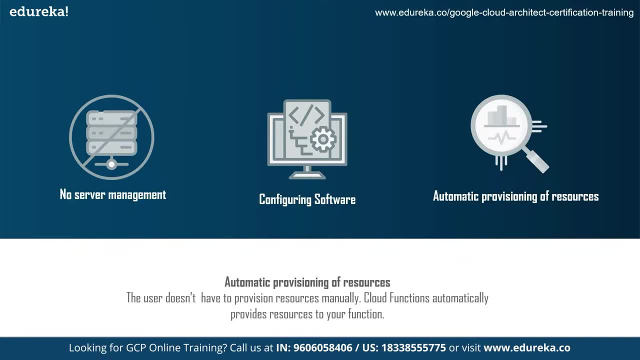 automatic provisioning of resources now. automatic provisioning of resources now. the user does not have to provision. the user does not have to provision. the user does not have to provision resources manually. cloud functions resources manually. cloud functions resources manually. cloud functions automatically provisions resources for. automatically provisions resources for. 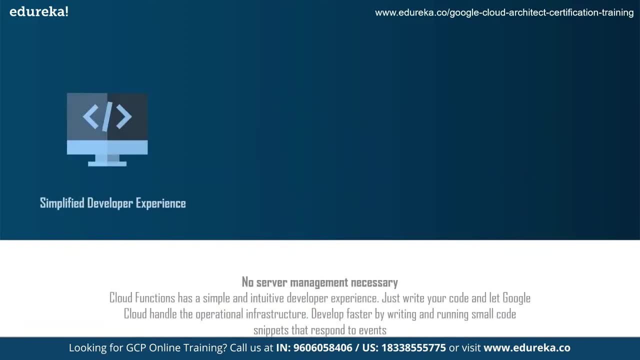 automatically provisions resources for your cloud functions. right, so next up, your cloud functions. right, so next up, your cloud functions. right, so next up. we talk about simplified developer. we talk about simplified developer. we talk about simplified developer experience. that experience, that experience that google cloud functions provides us with. 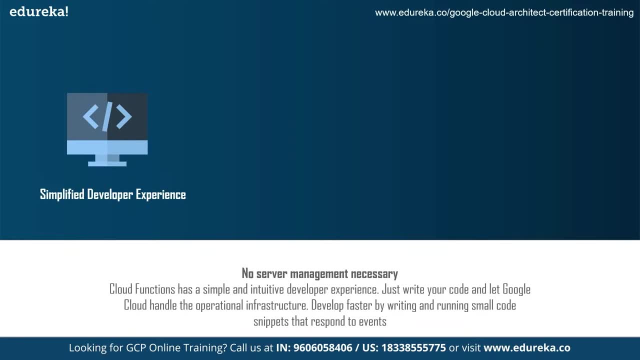 google cloud functions provides us with. google cloud functions provides us with. now cloud function has a simple and now cloud function has a simple and now cloud function has a simple and intuitive developer experience. just intuitive developer experience. just intuitive developer experience. just write your code and let google cloud. 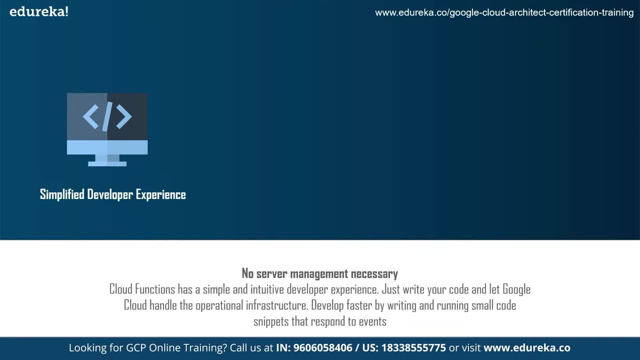 write your code and let google cloud write your code and let google cloud handle the operational infrastructure. so handle the operational infrastructure, so handle the operational infrastructure. so you do not need to think about all the, you do not need to think about all the, you do not need to think about all the operational infrastructure. that is there. 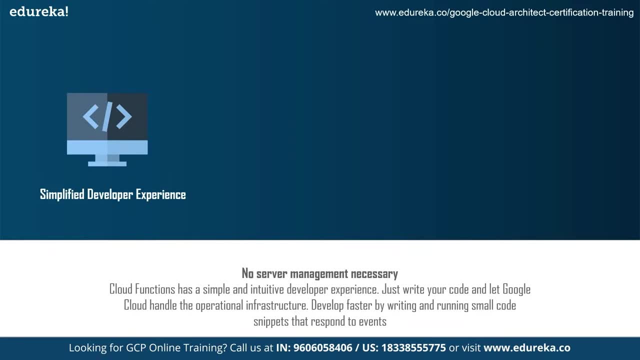 operational infrastructure, that is there. operational infrastructure: that is there, you just have to write your code and you just have to write your code and you just have to write your code and basically develop faster by running small. basically develop faster by running small. basically develop faster by running small code snippets that respond to various 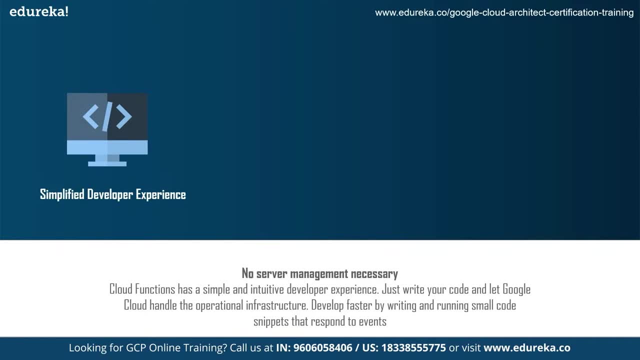 code snippets that respond to various code snippets that respond to various events that google functions provides, events that google functions provides. events that google functions provides: right next up, we see that it is the pay. right next up, we see that it is the pay. right next up, we see that it is the pay as you go model. so you are only built. 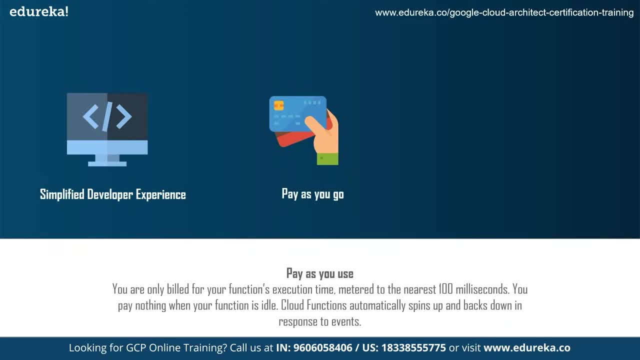 as you go model, so you are only built as you go model, so you are only built for the functions executing time meter, for the functions executing time meter, for the functions executing time meter to the nearest 100 milliseconds. so to the nearest 100 milliseconds, so to the nearest 100 milliseconds. so basically, you pay nothing when your 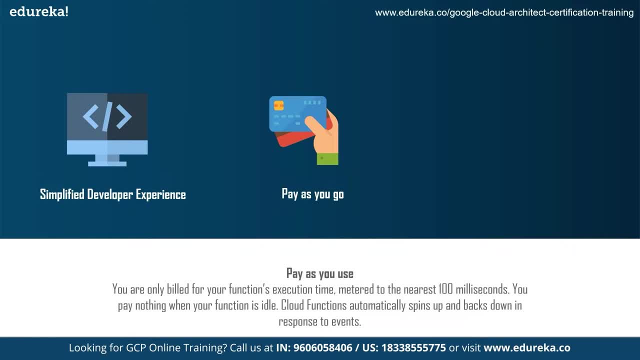 basically you pay nothing when your basically you pay nothing when your function is idle right, so cloud functions function is idle right. so cloud functions function is idle right. so cloud functions automatically spins up and back, automatically spins up and back, automatically spins up and back down with the response to events. so 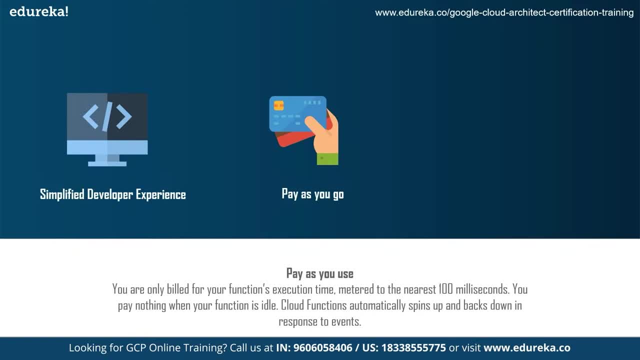 down with the response to events, so down with the response to events. so, basically, whenever you use your function, basically whenever you use your function, basically whenever you use your function, that is the only time where you are, that is the only time where you are, that is the only time where you are charged, and you are not charged if your 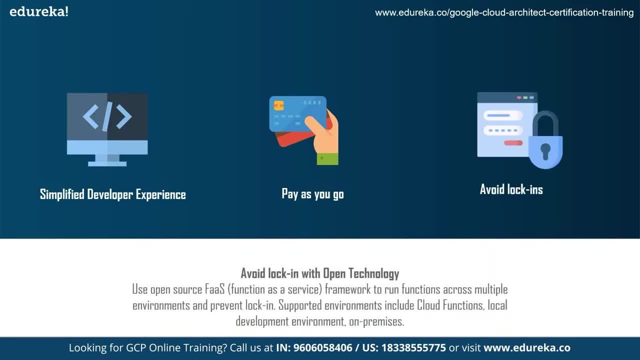 charged and you are not charged, if your charged and you are not charged if your cloud function is inactive. and finally, cloud function is inactive and finally, cloud function is inactive. and finally, we see that you can avoid logins. so we see that you can avoid logins. so 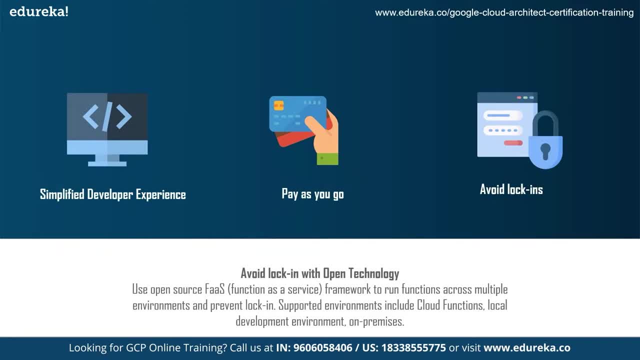 we see that you can avoid logins. so basically use open source fas, which is basically use open source fas, which is basically use open source fas, which is basically function as a service, basically function as a service, basically function as a service: framework to run functions across, framework to run functions across. 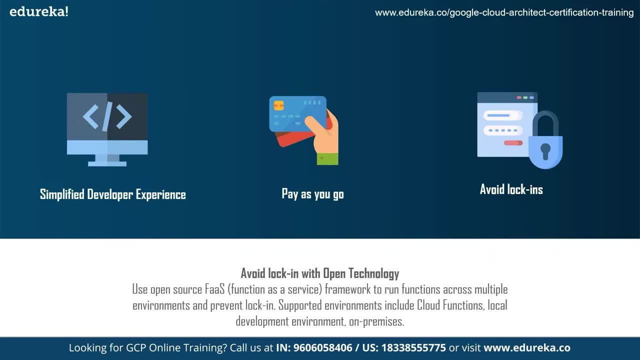 framework to run functions across multiple environments and prevent multiple environments. and prevent multiple environments and prevent logins. supported environments include logins. supported environments include logins. supported environments include cloud functions, local development cloud functions. local development cloud functions, local development environment, on-premises, etc. right, so you? 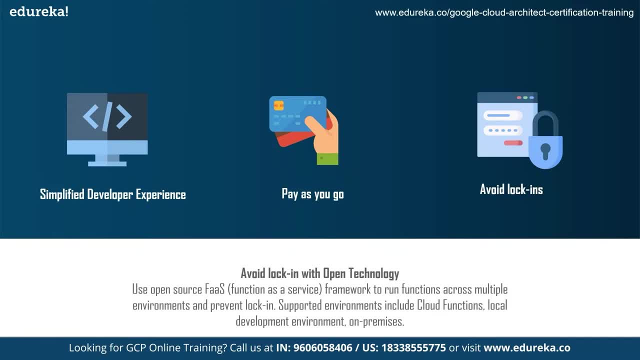 environment, on-premises, etc. right, so you environment on-premises, etc. right, so you can avoid logins using cloud functions, can avoid logins using cloud functions, can avoid logins using cloud functions with open technology. so this is why you with open technology. so this is why you. 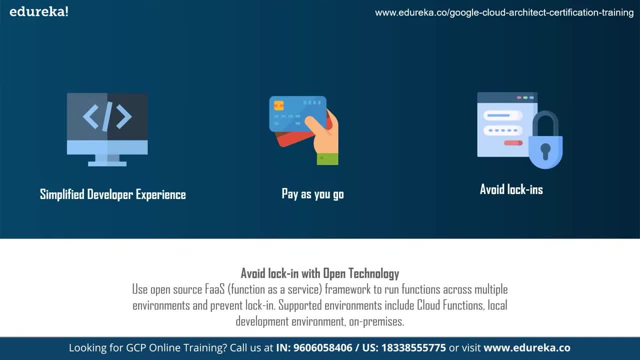 with open technology. so this is why you should use cloud functions and the should use cloud functions and the should use cloud functions and the various features it's providing next up, various features it's providing next up, various features it's providing next up. we talk about the integration with other. 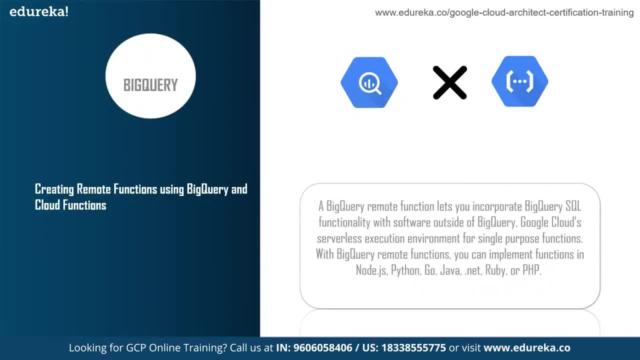 we talk about the integration with other. we talk about the integration with other apis that cloud functions has. so the apis that cloud functions has, so the apis that cloud functions has. so the first integration we talk about is the first integration we talk about is the first integration we talk about is the bigquery integration with cloud functions. 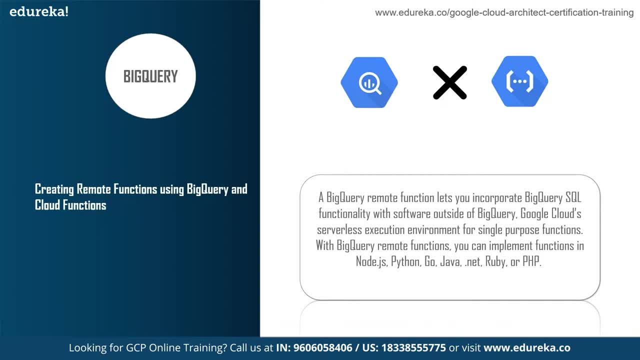 bigquery integration with cloud functions. bigquery integration with cloud functions. so bigquery remote function will let you. so bigquery remote function will let you. so bigquery remote function will let you create a bigquery sql functionality and create a bigquery sql functionality and create a bigquery sql functionality and software outside bigquery with the help. 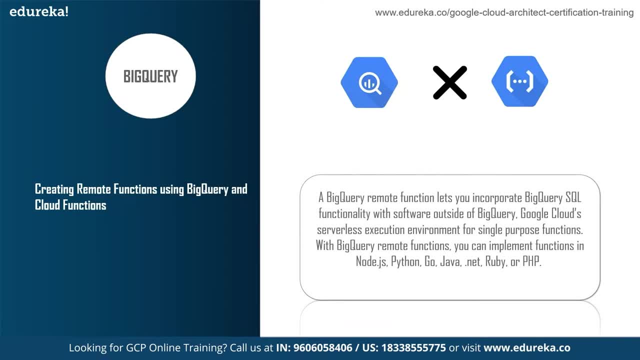 software outside bigquery with the help, software outside bigquery with the help of cloud functions. right. so the of cloud functions right, so the of cloud functions right. so the serverless execution environment, serverless execution environment, serverless execution environment basically allows bigquery to do this. 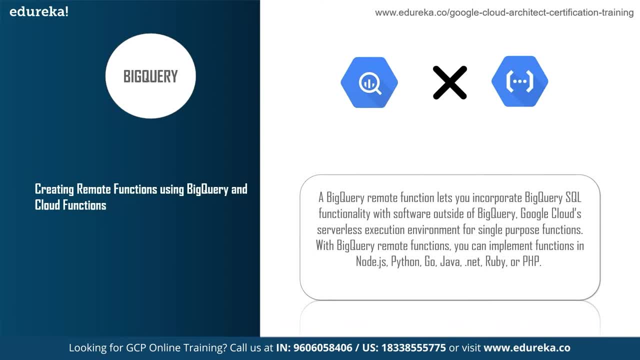 basically allows bigquery to do this, basically allows bigquery to do this and make remote functions as well. so, and make remote functions as well. so, and make remote functions as well. so this is one of the integrations that. this is one of the integrations that. 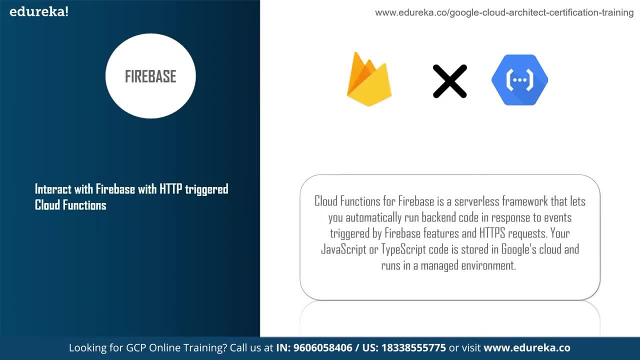 this is one of the integrations that google cloud functions has. google cloud functions has. google cloud functions has. so next up, we talk about the integration. so next up, we talk about the integration. so next up, we talk about the integration with firebase. now google cloud can be. 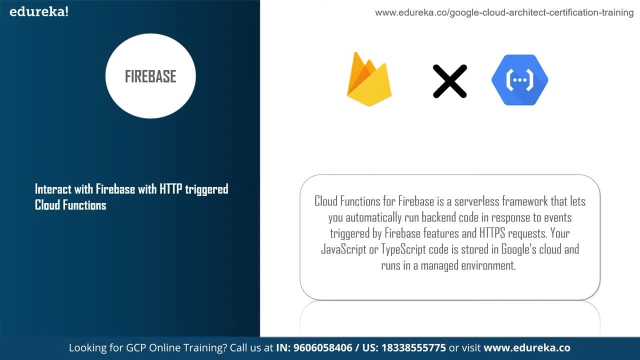 with firebase. now google cloud can be with firebase. now google cloud can be integrated with firebase, provided that integrated with firebase, provided that integrated with firebase, provided that, basically, basically, basically, you use it for the serverless framework, you use it for the serverless framework, you use it for the serverless framework and it lets you automatically run back. 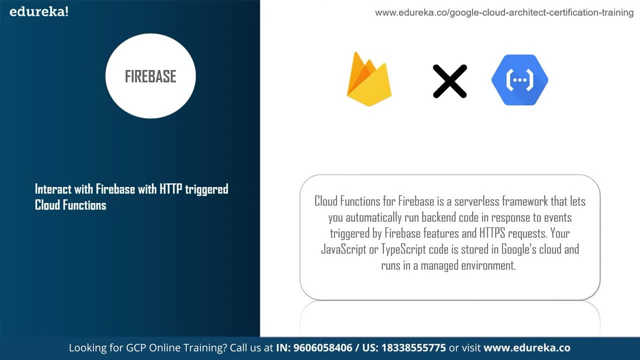 and it lets you automatically run back. and it lets you automatically run back and code in response to events. and. and code in response to events. and and code in response to events. and triggers. so these triggers are provided triggers. so these triggers are provided triggers. so these triggers are provided in the format of http requests or api. 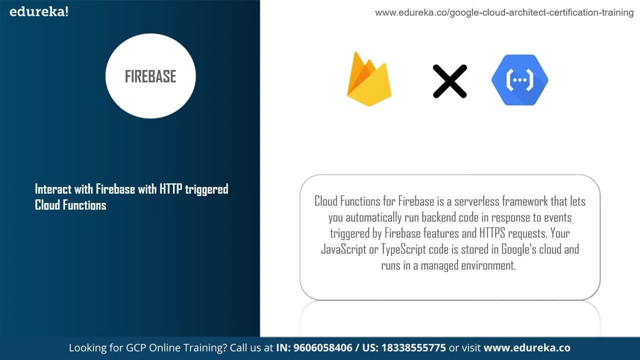 in the format of http requests or api, in the format of http requests or api requests or something like that requests or something like that requests or something like that. so, basically, what firebase does with so, basically what firebase does with. so basically what firebase does with google cloud functions is that you can 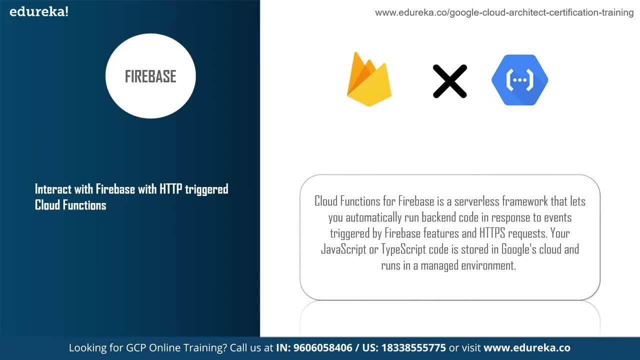 google cloud functions is that you can. google cloud functions is that you can interact with firebase using http. interact with firebase using http. interact with firebase using http. triggered cloud functions. right, so this triggered cloud functions. right, so this triggered cloud functions. right, so this basically requires the first kind of 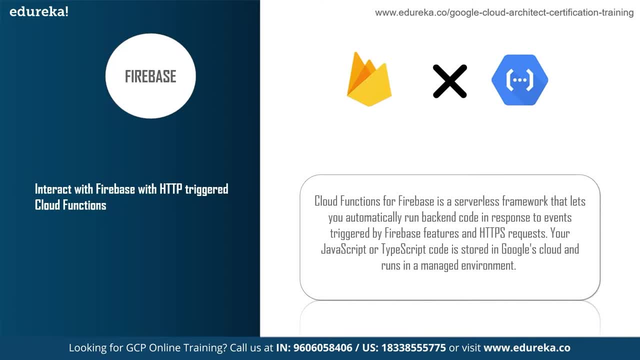 basically requires the first kind of, basically requires the first kind of cloud functions. that is the api kind of cloud functions. that is the api kind of cloud functions. that is the api kind of cloud functions. not the event during cloud functions, not the event during cloud functions, not the event during once when it comes to interacting with. 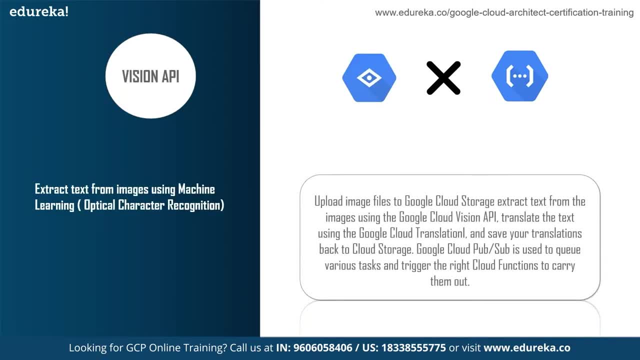 once when it comes to interacting with, once when it comes to interacting with firebase, firebase, firebase. so next up, we talk about vision api. so next up, we talk about vision api. so next up, we talk about vision api. integration with cloud functions: cloud. integration with cloud functions- cloud. 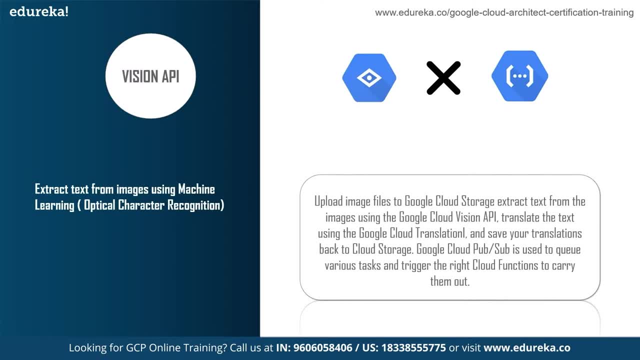 integration with cloud functions. cloud vision api is another api that provides vision. api is another api that provides vision. api is another api that provides us with facial recognition and us with facial recognition and us with facial recognition and photographic recognition: optical photographic recognition, optical photographic recognition, optical character recognition and all of that. 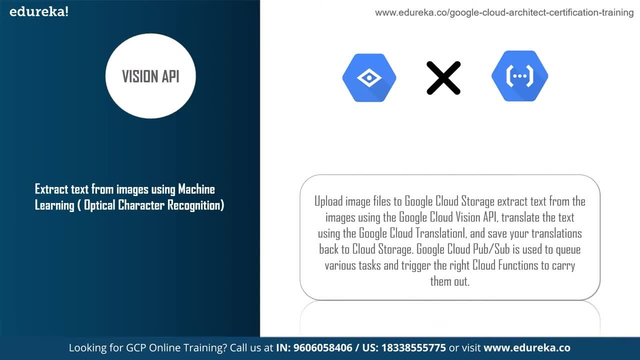 character recognition, optical character recognition and all of that. character recognition, optical character recognition, and all of that, and if you want to check out more on and if you want to check out more on and if you want to check out more on cloud vision api, you can check out. 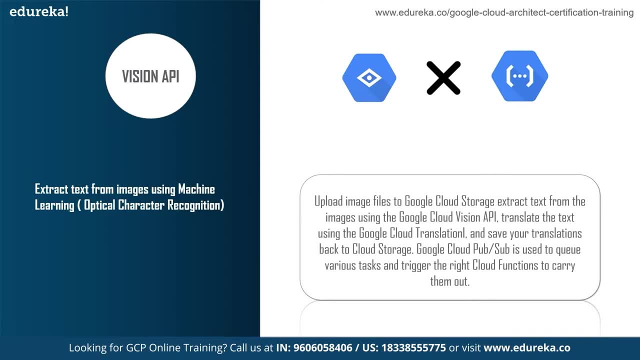 cloud vision api. you can check out cloud vision api. you can check out edureka's video on vision api as well. edureka's video on vision api as well. edureka's video on vision api as well. now, when it comes to cloud functions. now, when it comes to cloud functions. 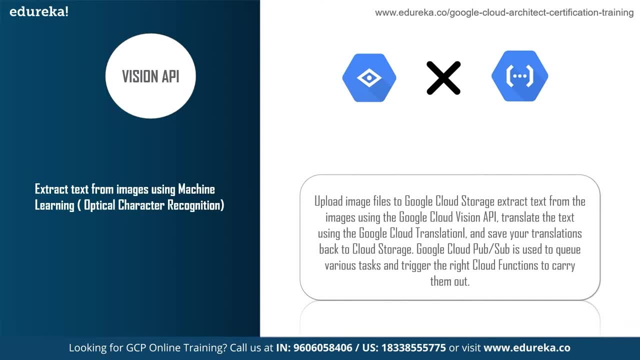 now, when it comes to cloud functions with vision api, we can see that, when it with vision api, we can see that when it with vision api, we can see that, when it comes to optical recognition, of comes to optical recognition of comes to optical recognition of characters, which is basically something. 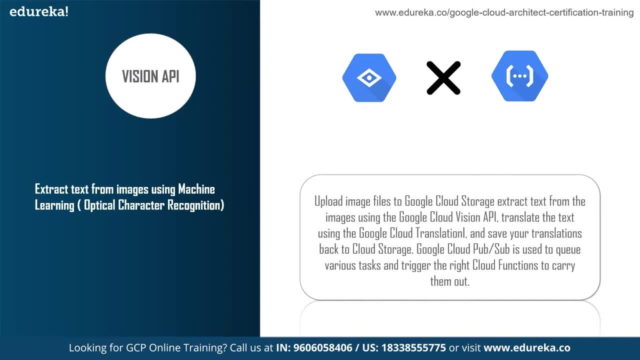 characters, which is basically something. characters, which is basically something that, in layman terms, can be explained as that, in layman terms, can be explained as that, in layman terms, can be explained as reading the text that is present in. reading the text that is present in. 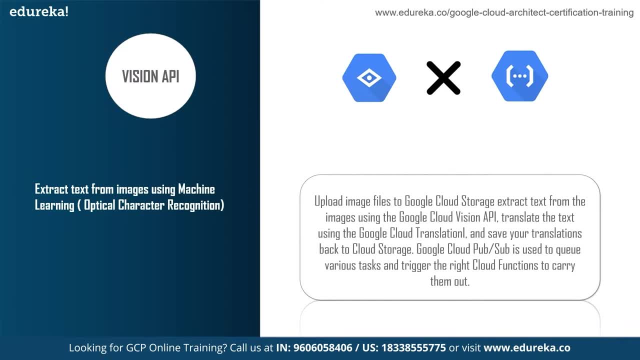 reading the text that is present in images and then printing that out right images and then printing that out right images and then printing that out right so you can basically read whatever. so you can basically read whatever. so you can basically read whatever image that you have and if it has some, 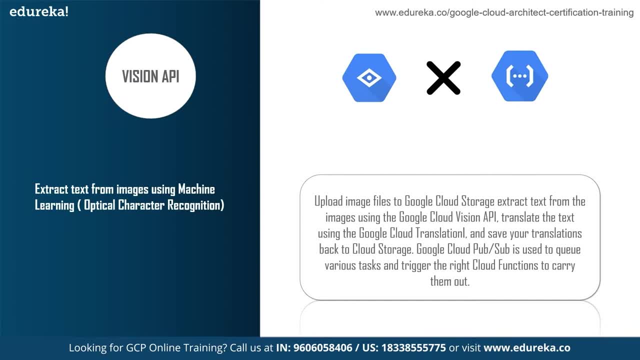 image that you have and if it has some image that you have and if it has some sort of text, sort of text, sort of text. optical character recognition will optical character recognition, will optical character recognition will basically print that text out to you, basically print that text out to you. 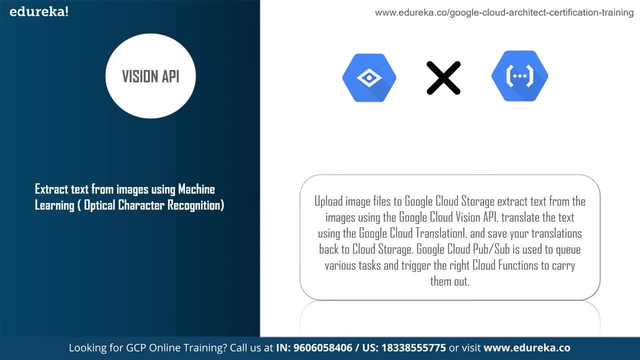 basically print that text out to you, right? so this is what vision api, right? so this is what vision api right. so this is what vision api integration with cloud functions is used. integration with cloud functions is used. integration with cloud functions is used for. next up, we come to the pricing of 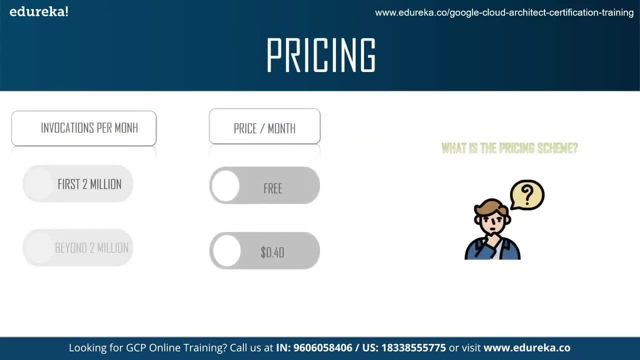 for next up, we come to the pricing of. for next up, we come to the pricing of google cloud functions. so when it comes google cloud functions, so when it comes google cloud functions, so when it comes to pricing, we can see that pricing is to pricing, we can see that pricing is. 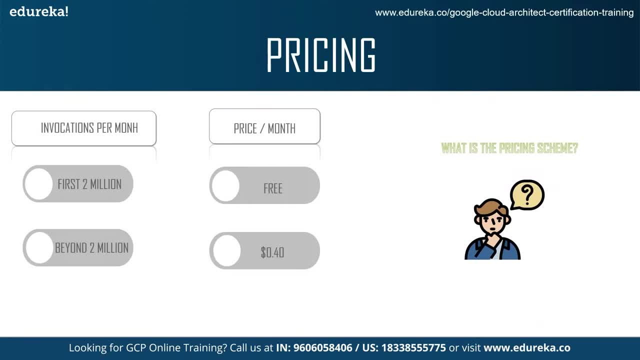 to pricing, we can see that pricing is based on various things, such as based on various things, such as based on various things, such as invocations per month and the price per invocations per month and the price per invocations per month and the price per month. so, for the first two million, 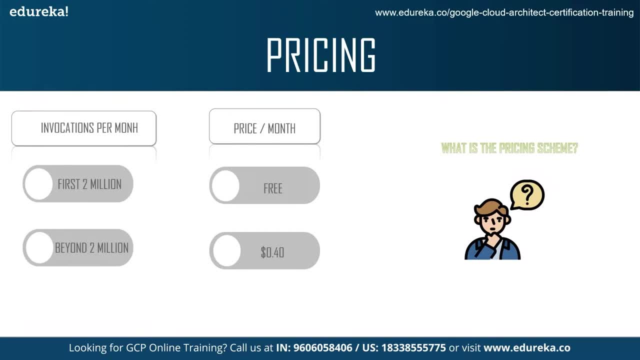 month. so for the first two million month. so for the first two million invocations, the price is free. and if you invocations, the price is free. and if you invocations, the price is free. and if you go beyond 2 million invocations, the price. go beyond 2 million invocations, the price. 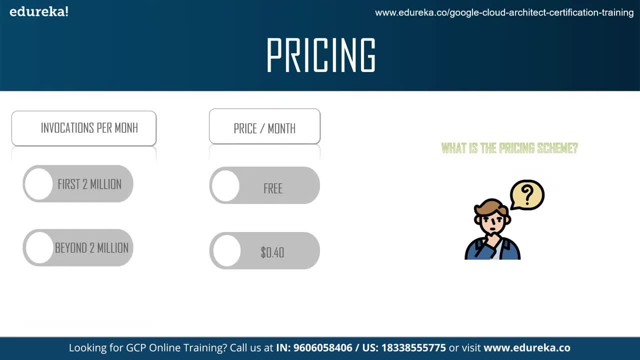 go beyond 2 million invocations. the price is 0.40 dollars per month, is 0.40 dollars per month, is 0.40 dollars per month. so, apart from all of this, we can see. so, apart from all of this, we can see. 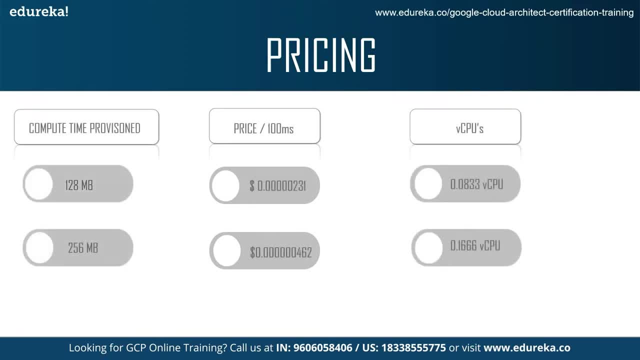 so, apart from all of this, we can see that pricing is also based on the, that pricing is also based on the, that pricing is also based on the compute time provision, the price per compute time provision, the price per compute time provision, the price per 100 millisecond and the virtual cpus. 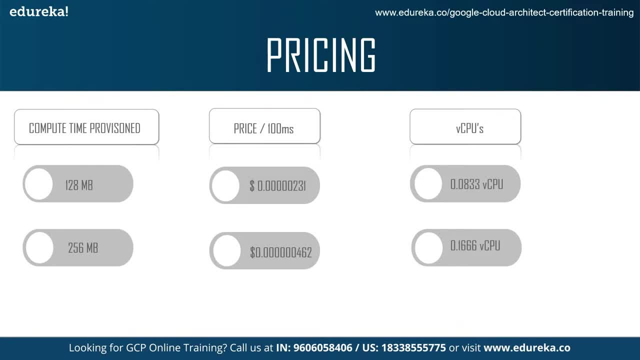 100 millisecond and the virtual cpus: 100 millisecond and the virtual cpus present. so 128 mb compute time will be present. so 128 mb compute time will be present. so 128 mb compute time will be priced at around 0.0000231. 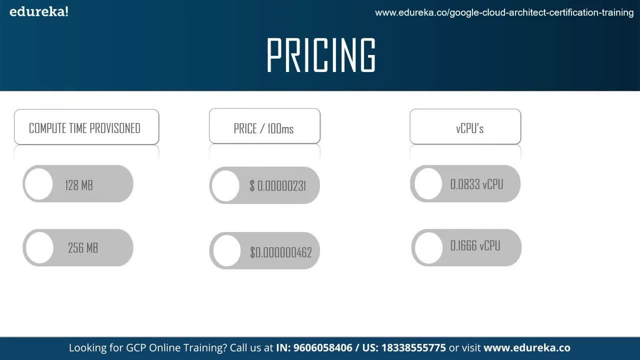 priced at around 0.0000231. priced at around 0.0000231 dollars, whereas virtual cpus required will dollars whereas virtual cpus required. will dollars, whereas virtual cpus required will be 0.0833 be 0.0833. 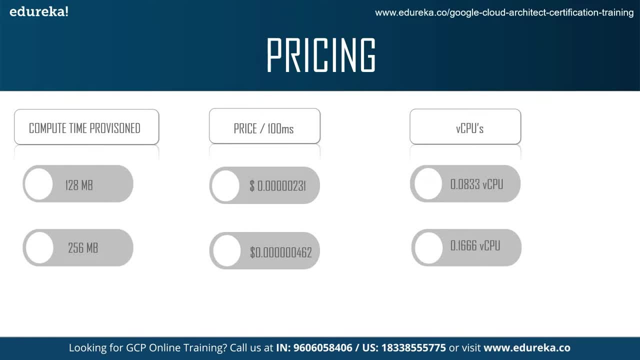 be 0.0833, right, so similarly, it is exactly the double right. so similarly, it is exactly the double right. so similarly, it is exactly the double of what 128 mb needs for 256, of what 128 mb needs for 256, of what 128 mb needs for 256, right. so the virtual cpu is required in. 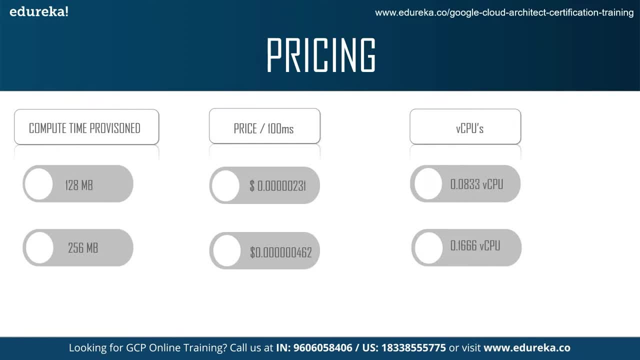 right, so the virtual cpu is required. in right, so the virtual cpu is required. in the 256 mb computer provision will be: the 256 mb computer provision will be: the 256 mb computer provision will be 0.166 virtual cpu is required. 0.166 virtual cpu is required. 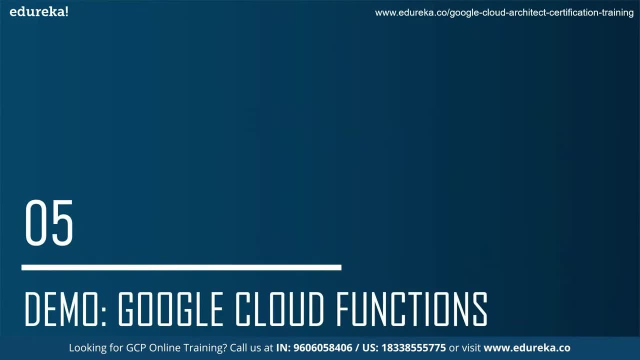 0.166 virtual cpu is required. so next up, we see a demo on google. so next up, we see a demo on google. so next up, we see a demo on google cloud functions, cloud functions, cloud functions. so i have a github repository with. so i have a github repository with. 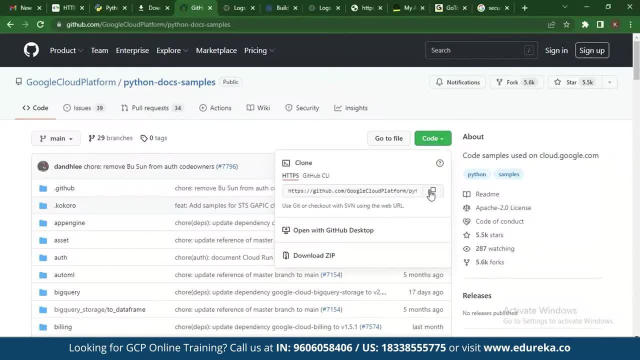 so i have a github repository with python code which will go for google python code which will go for google python code which will go for google cloud platform, cloud platform, cloud platform, and let's just copy this repository and let's just copy this repository and let's just copy this repository and try including it on our system, on our. 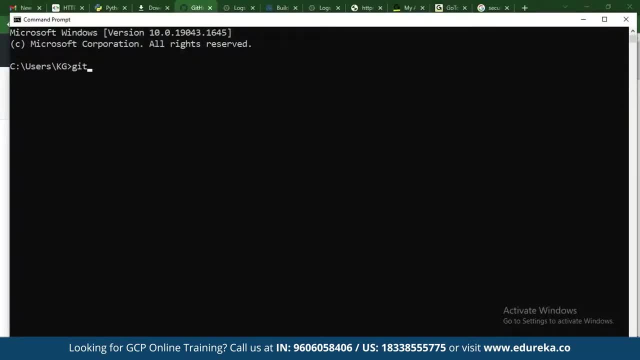 and try including it on our system, on our, and try including it on our system, on our local system, local system, local system. so do that. what you need to do is so do that. what you need to do is so do that. what you need to do is it clone? 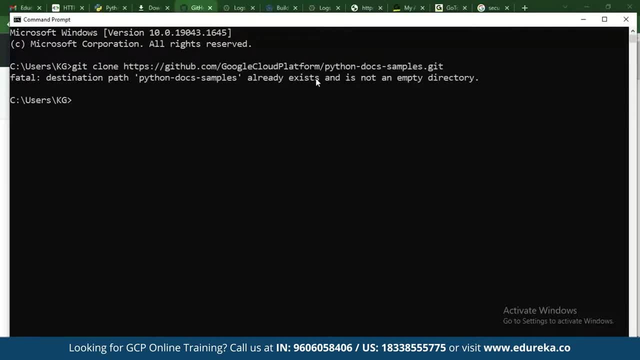 it, clone, it, clone and copy that here, and copy that here, and copy that here so you can see that this repository is. so you can see that this repository is. so you can see that this repository is already cloned in my system, already cloned in my system, already cloned in my system, and all i need to do is find the path for. 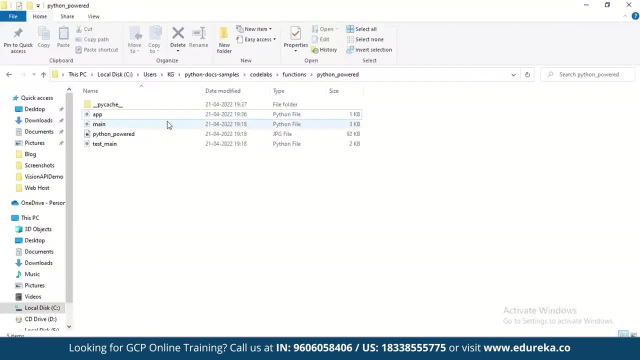 and all i need to do is find the path for, and all i need to do is find the path for it, it, it, so let's go search for the path for it. so let's go search for the path for it. so let's go search for the path for it, and this is basically my path. 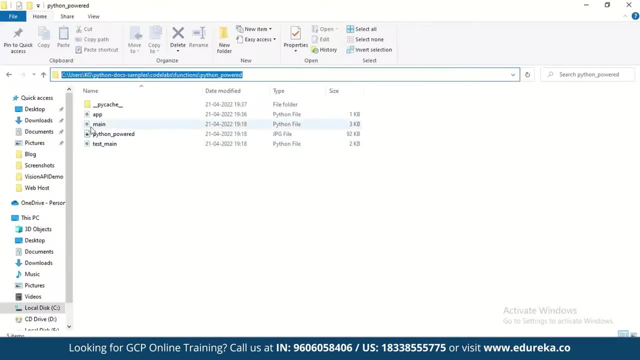 and this is basically my path and this is basically my path for my repository. just copy this path for my repository. just copy this path for my repository. just copy this path. so once you copy that path, so once you copy that path, so once you copy that path, basically all you have to do is cd and 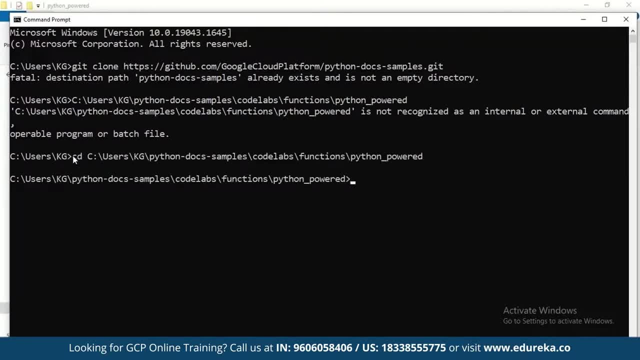 basically all you have to do is cd and basically all you have to do is cd and paste that path here, paste that path here, paste that path here and you will basically go into your and you will basically go into your and you will basically go into your directory. 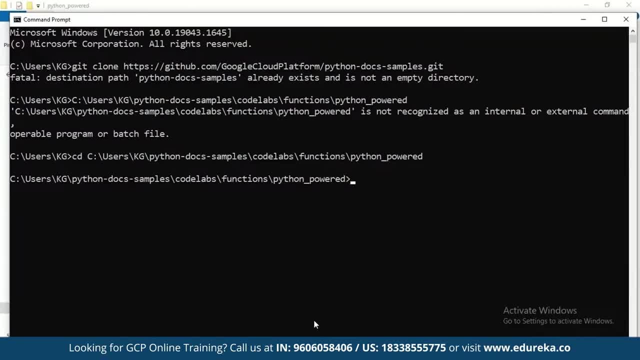 directory, directory, right. so this is how you change the right. so this is how you change the right. so this is how you change the directory. now, once you've changed the directory, now, once you've changed the directory, now, once you've changed the directory, you can see: 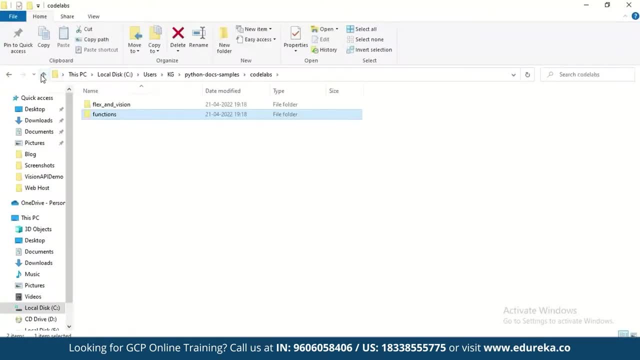 directory. you can see directory. you can see that your file that you've downloaded the. that your file that you've downloaded the. that your file that you've downloaded the github repository that you've downloaded, github repository that you've downloaded. github repository that you've downloaded has various files in it. so what you need. 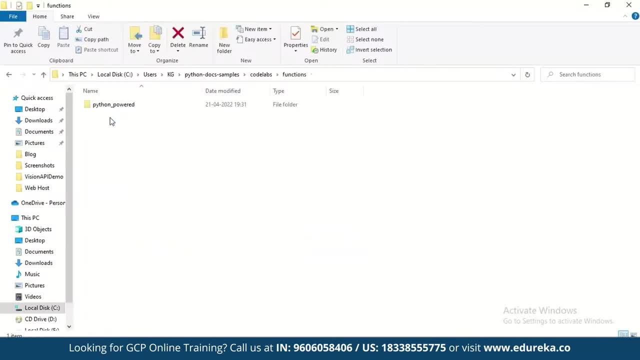 has various files in it. so what you need has various files in it. so what you need to do is open up the python file. to do is open up the python file. to do is open up the python file into your vs code, right? so open up the. 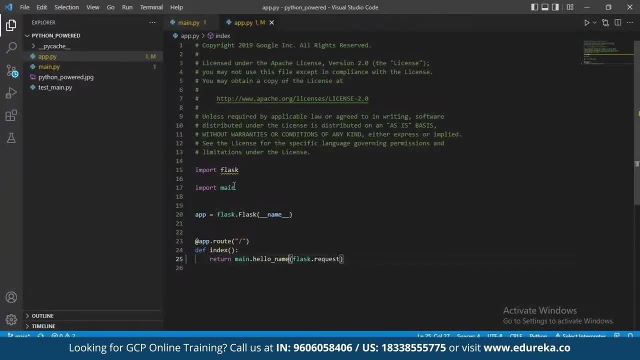 into your vs code, right, so open up the into your vs code, right, so open up the python file in your vs code. python file in your vs code. python file in your vs code. and, as you can see, this is the python. and, as you can see, this is the python. 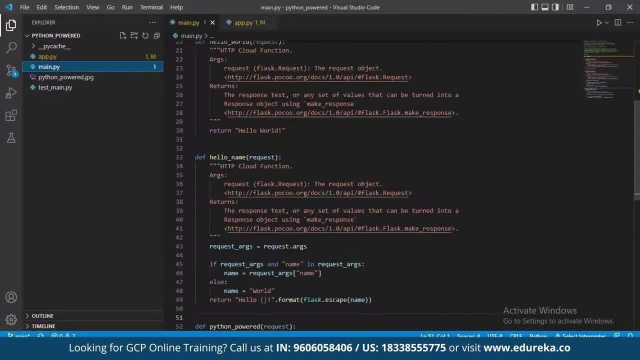 and, as you can see, this is the python file, which is the apppy file, which is the apppy file, which is the apppy, and this is the main function, which is, and this is the main function, which is, and this is the main function which is the mainpy. 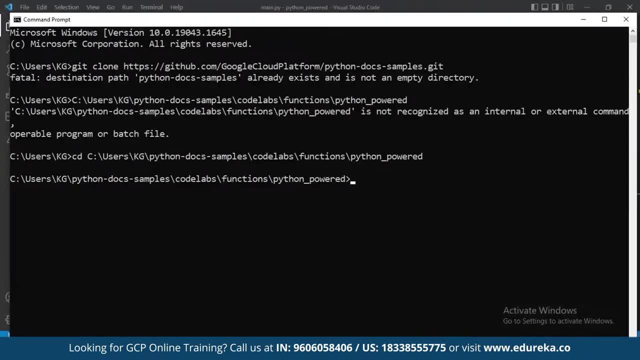 the mainpy, the mainpy, right. so what you need to do now is test, right. so what you need to do now is test, right. so what you need to do now is test it on your local system, right so you it on your local system, right so you. 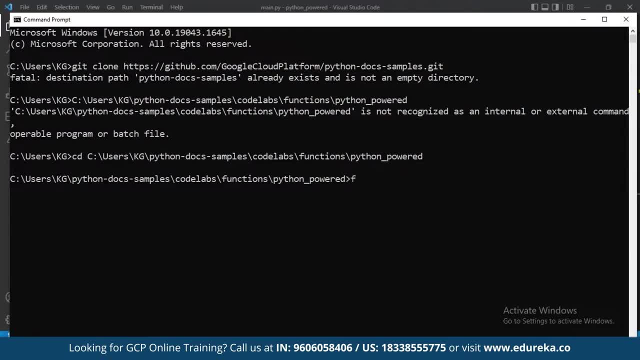 it on your local system, right? so you have the python file. you have the. have the python file. you have the. have the python file. you have the repository. all you need to do is run repository. all you need to do is run repository. all you need to do is run flask, right? so this is basically running. 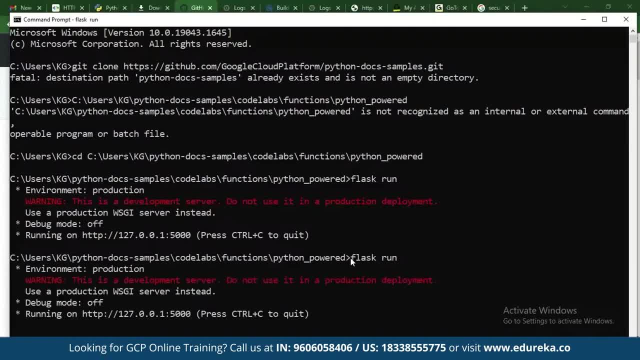 flask, right, so this is basically running. flask, right, so this is basically running. let's try it out again, just one last. let's try it out again, just one last. let's try it out again, just one last time. time time, right, it is running on this local machine. 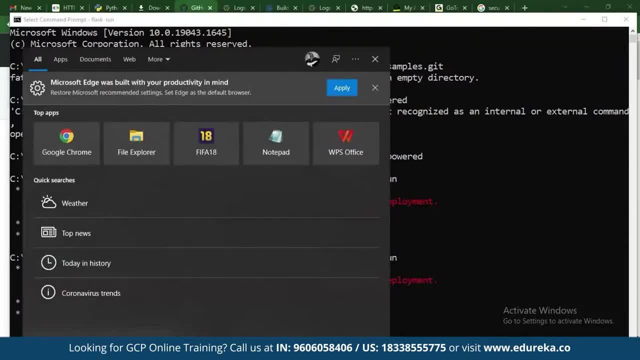 right, it is running on this local machine. right, it is running on this local machine, local host, right. so what we need to do, local host right. so what we need to do, local host right. so what we need to do is let's check it out. so go to postman. 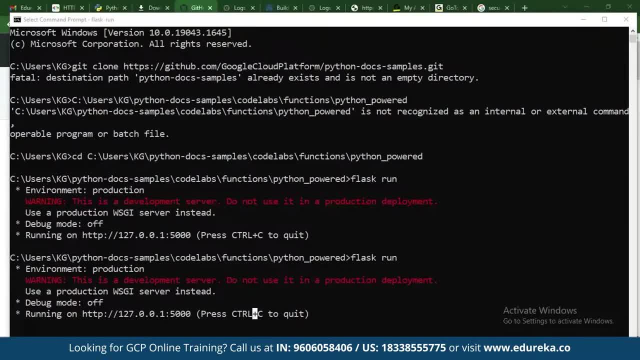 is: let's check it out, so go to postman. is: let's check it out, so go to postman. and postman basically allows you to see: and postman basically allows you to see, and postman basically allows you to see that, if your http triggered functions. 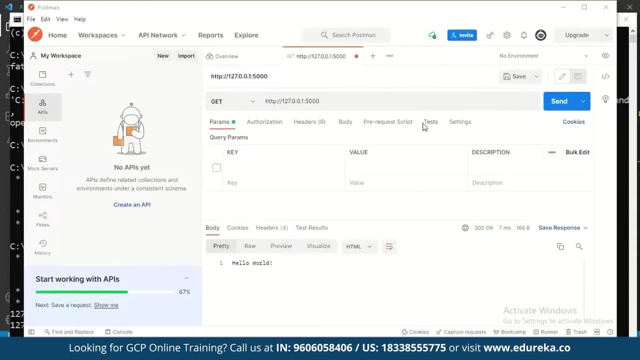 that if your http triggered functions, that if your http triggered functions is working right, so when you go to is working right, so when you go to is working right. so when you go to postman, you basically type in postman, you basically type in postman, you basically type in this trigger that you have the url. 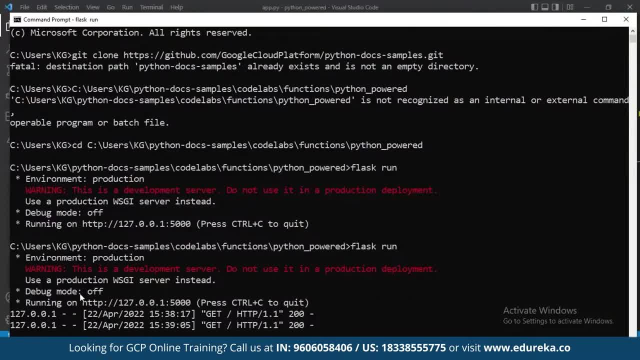 this trigger that you have the url. this trigger that you have the url, which is basically this. which is basically this, which is basically this: this is running on this localhost. you, this is running on this localhost. you, this is running on this localhost. you can just go back to postman. 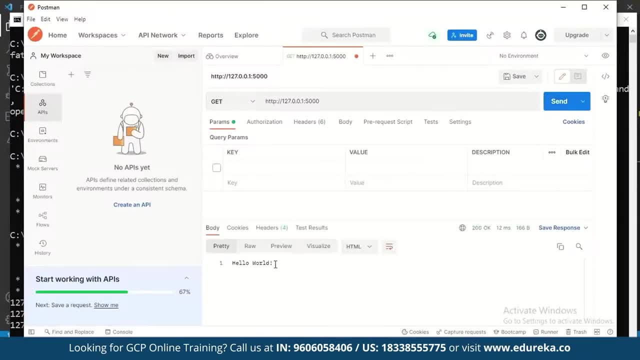 can just go back to postman. can just go back to postman. copy paste this, copy paste this. copy paste this. do this and you can see hello world out. do this and you can see hello world out. do this and you can see hello world out here. so this is running on my local host. 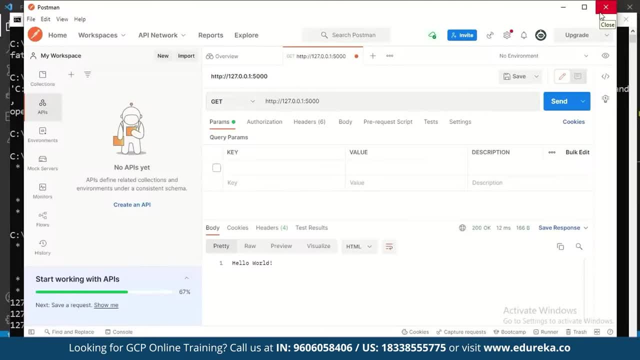 here. so this is running on my local host here, so this is running on my local host now. let's try doing this on google now. let's try doing this on google now. let's try doing this on google cloud functions, cloud functions, cloud functions- right. so once you go to google cloud, 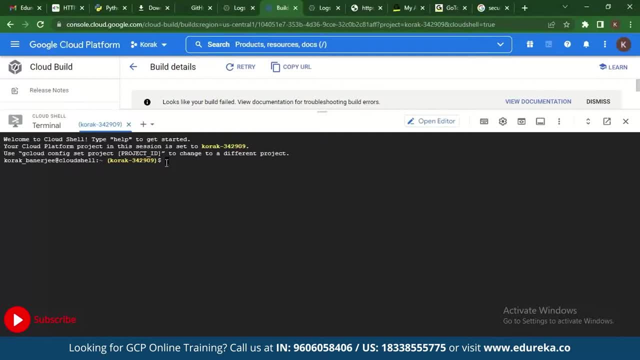 right. so once you go to google cloud, right. so once you go to google cloud, functions, you can basically just functions. you can basically just functions. you can basically just open up cloud shell. and since you now open up cloud shell, and since you now open up cloud shell, and since you now have the github repository in your 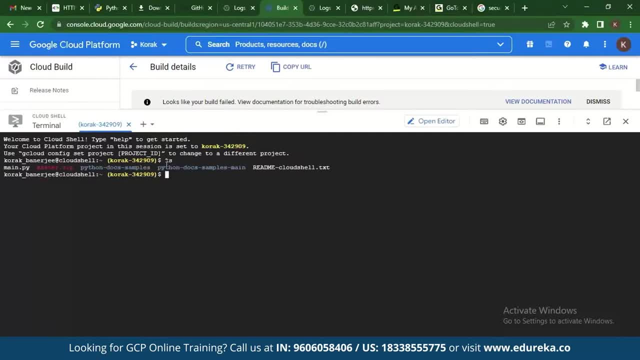 have the github repository in your have the github repository in your system. you can just check the directory system. you can just check the directory system. you can just check the directory. so this is the directory that we have. so this is the directory that we have. so this is the directory that we have and our repository is called. 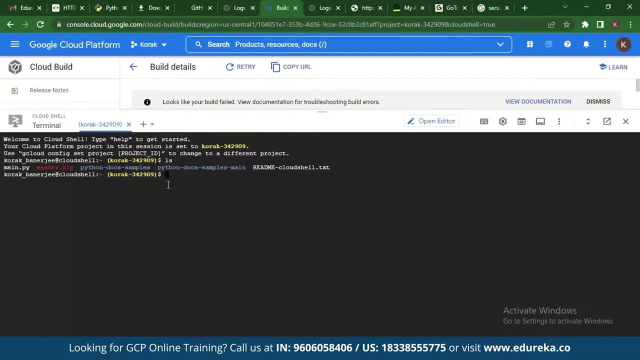 and our repository is called. and our repository is called: python doc- samples- right, so python doc. python doc- samples- right, so python doc. python doc- samples- right, so python doc- samples, samples, samples. so we can just move into the python doc. so we can just move into the python doc. 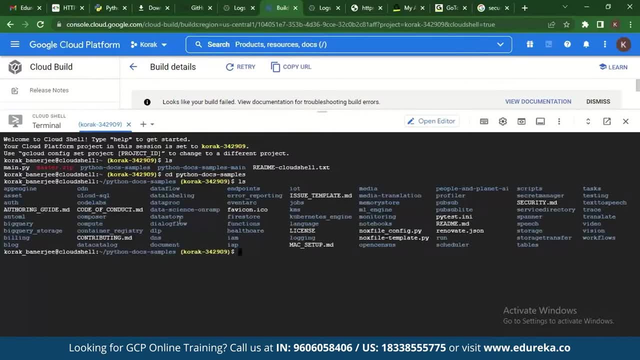 so we can just move into the python doc. samples, samples, samples. right, and now we're in. we'll check out. right, and now we're in, we'll check out. right, and now we're in. we'll check out the files in here, the files in here, the files in here and now. what we need to do is go into. 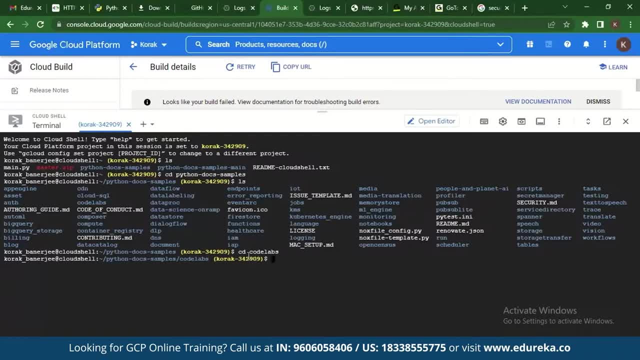 and now what we need to do is go into, and now what we need to do is go into the repository with the code, the repository with the code, the repository with the code, right now, once you've moved into the right now, once you've moved into the 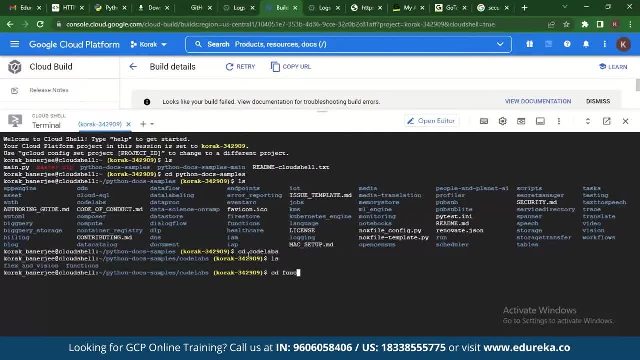 right now. once you've moved into the repository with the code, check out the repository with the code. check out the repository with the code. check out the files in it, files in it, files in it and move into the folder with the. and move into the folder with the. 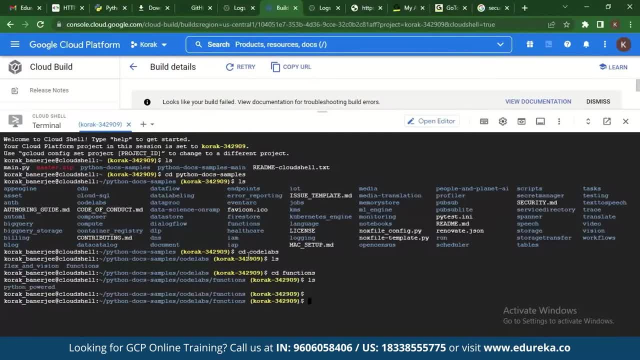 and move into the folder with the function in it and check out the function in it. and check out the function in it and check out the repository again. repository again. repository again. move into python part. now you move into. move into python part. now you move into. move into python part. now you move into python part. check out the repository. 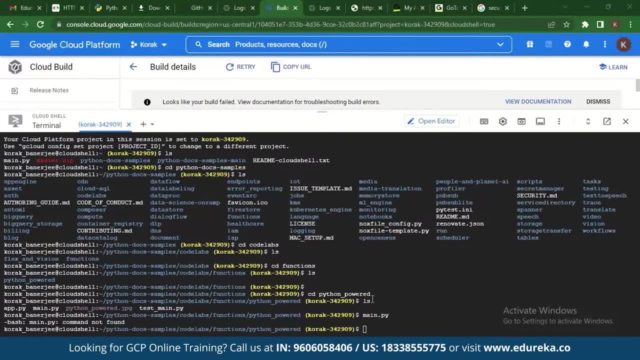 python part. check out the repository. python part. check out the repository. and you have mainpy here, right, and you have mainpy here, right, and you have mainpy here, right? so once you've found your mainpy file. so once you've found your mainpy file. 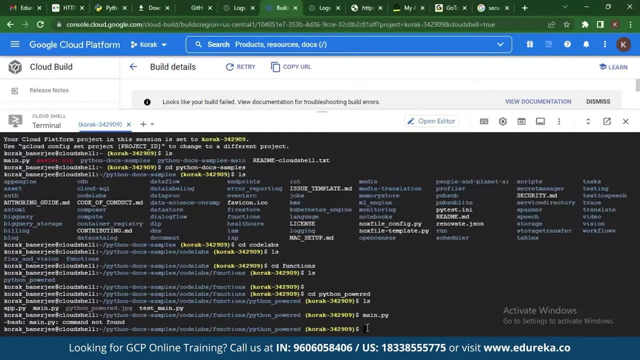 so, once you've found your mainpy file, what you need to do, what you need to do, what you need to do is basically create a function with a is basically create a function with a. is basically create a function with a trigger and endpoint, and all of that. so 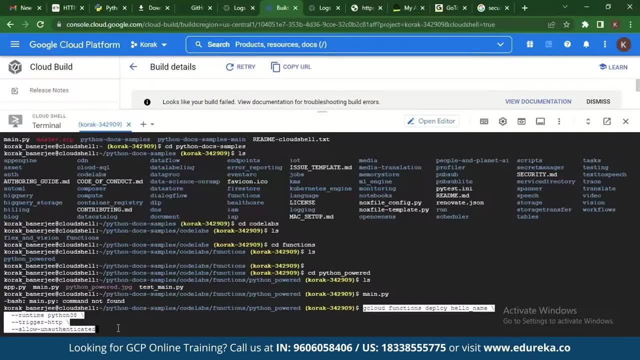 trigger and endpoint and all of that. so trigger and endpoint and all of that. so just this is basically the code for just this is basically the code for just this is basically the code for creating a cloud function with the creating a cloud function with the. creating a cloud function with the runtime, the trigger and the. 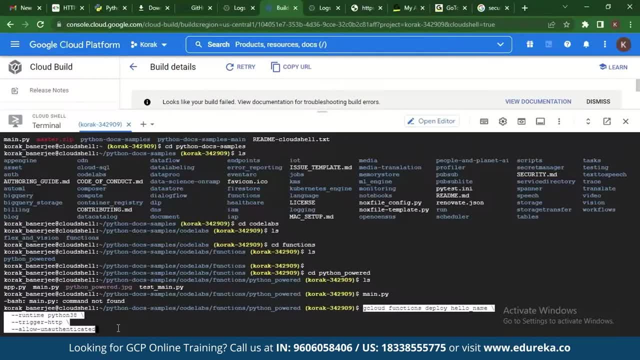 runtime, the trigger and the runtime, the trigger and the unauthentication specified. so what unauthentication specified? so what unauthentication specified? so what happens if you basically do not specify happens, if you basically do not specify happens, if you basically do not specify that unauthenticated functions will be? 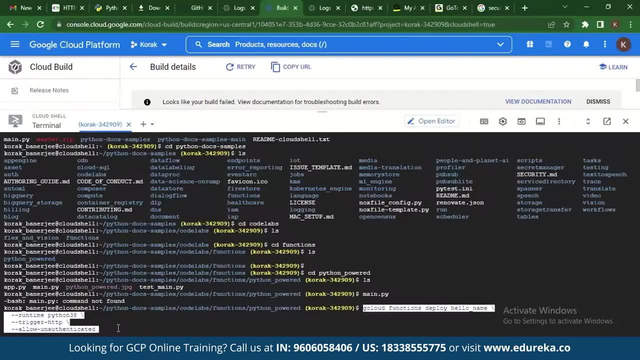 that unauthenticated functions will be. that unauthenticated functions will be available. is that every cloud functions available? is that every cloud functions available? is that every cloud functions that you create will be authenticated. that you create will be authenticated. that you create will be authenticated if you don't disallow authentication in. 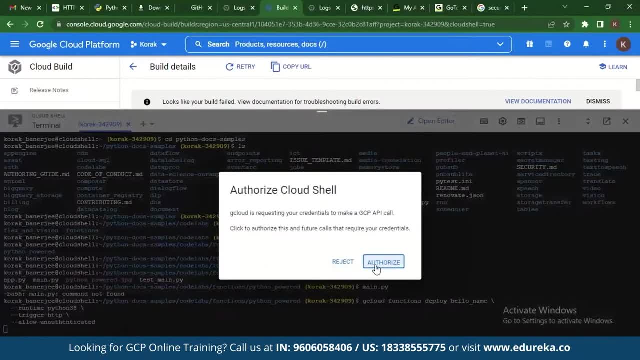 if you don't disallow authentication in, if you don't disallow authentication in general. so let's just try deploying this general. so let's just try deploying this general, so let's just try deploying this, and it will basically ask you for, and it will basically ask you for. 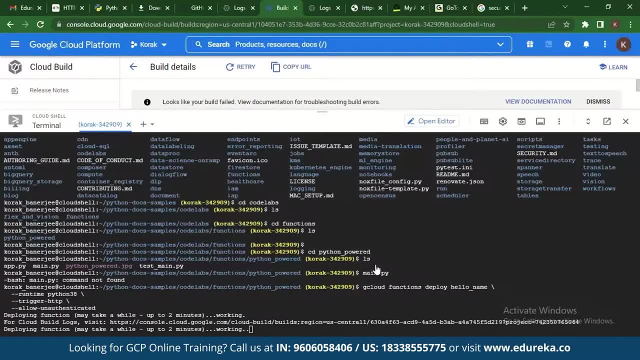 and it will basically ask you for authorization. right, so it is deploying now this. right, so it is deploying now this. right, so it is deploying now. this basically takes a bit of time for you to basically takes a bit of time for you to basically takes a bit of time for you to deploy a cloud functions maybe around. 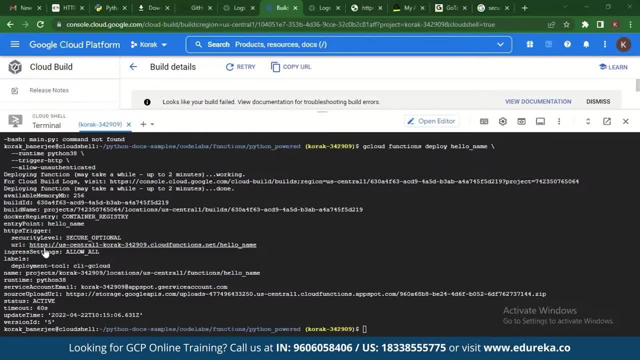 deploy a cloud functions, maybe around. deploy a cloud functions maybe around two to three minutes, two to three minutes, two to three minutes, right? so once you've deployed your cloud, right? so once you've deployed your cloud, right? so once you've deployed your cloud function, you can go check it out on this. 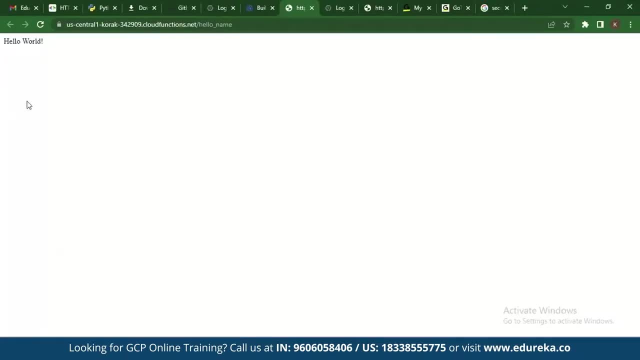 function. you can go check it out on this function. you can go check it out on this: url, url, url, right, so this is basically showing me right. so this is basically showing me right. so this is basically showing me. hello world right now. this is an http. hello world right now. this is an http. 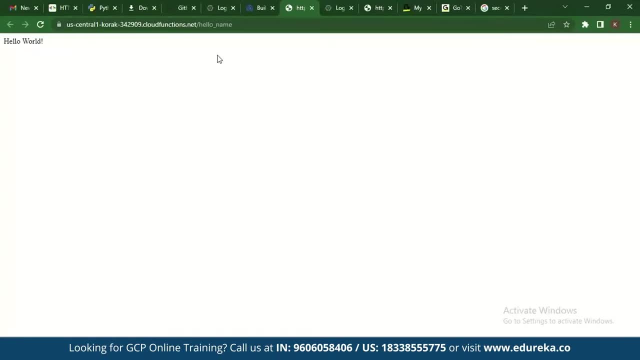 hello world. right now, this is an http triggered cloud function that allows you triggered cloud function that allows you triggered cloud function that allows you to take arguments in. so what we can do to take arguments in, so what we can do to take arguments in, so what we can do is we have our code here. 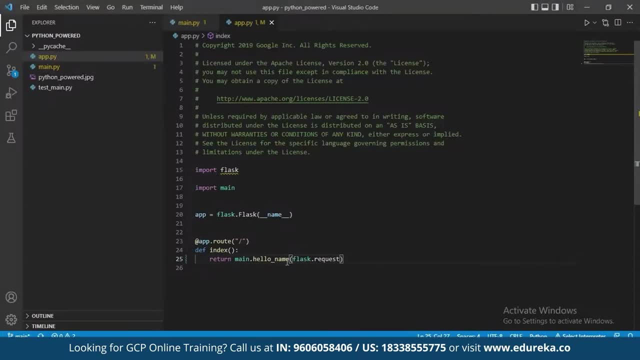 is we have our code here, is we have our code here. and if we go into the apppy thing, and if we go into the apppy thing, and if we go into the apppy thing we can see it is hello name, right. so we can see it is hello name, right. so 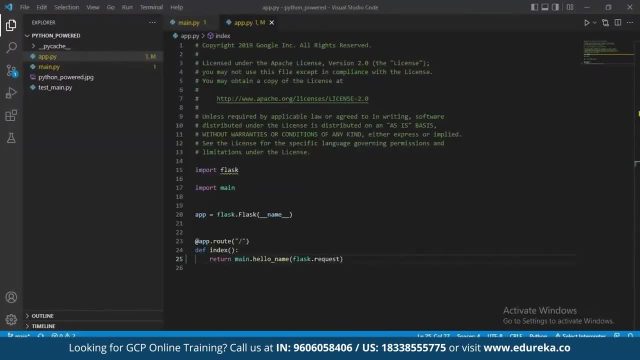 we can see it is hello name, right? so let's just go back to postman here, and let's just go back to postman here, and let's just go back to postman here and try something out, try something out, try something out. so what we will be aiming to do here is 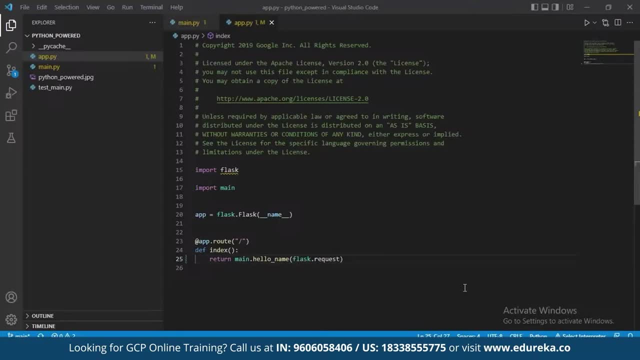 so what we will be aiming to do here is so what we will be aiming to do here is that we'll be aiming to change that. we'll be aiming to change that. we'll be aiming to change the arguments that we give in and see the arguments that we give in and see. 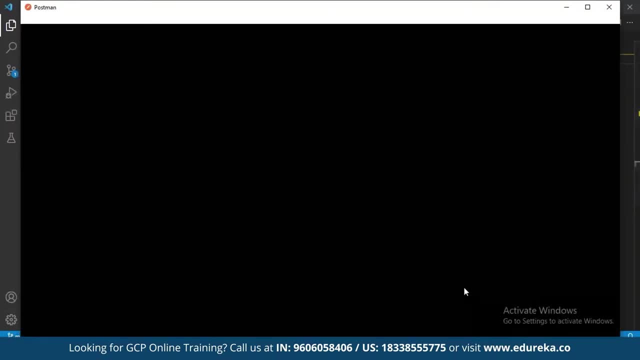 the arguments that we give in and see if our http triggered a back end is if our http triggered a back end is if our http triggered a back end is still working, so these are not still working. so these are not still working, so these are not, let's say, if you go back to this, so 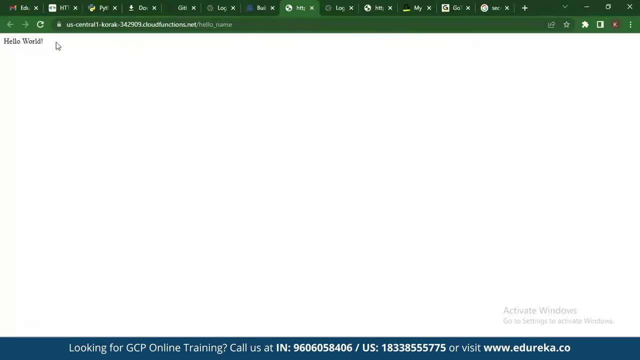 let's say, if you go back to this, so let's say, if you go back to this, so this is not really a web page. this is, this is not really a web page. this is, this is not really a web page. this is basically, basically, basically a serverless backend, right? so? 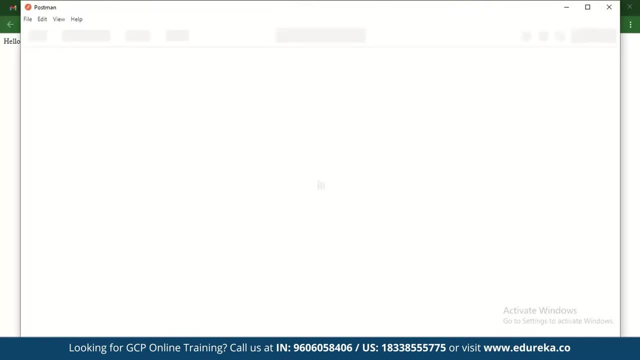 a serverless backend- right. so a serverless backend- right. so this is the basic difference, and this is the basic difference and this is the basic difference. and let's check it out on postman now. let's check it out on postman now. let's check it out on postman now. right, so postman is up and all you need. 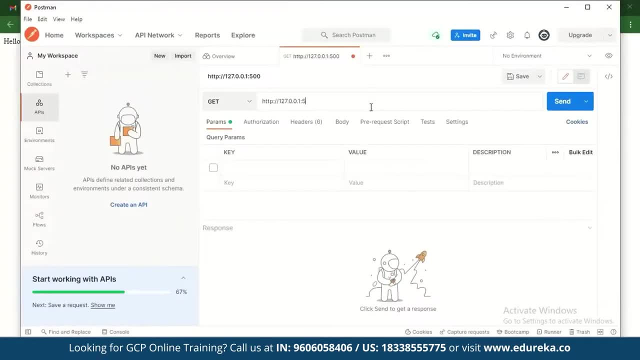 right, so postman is up, and all you need right, so postman is up, and all you need to do to do to do is take in this, put it in here. is take in this, put it in here, is take in this, put it in here and check if it's working. 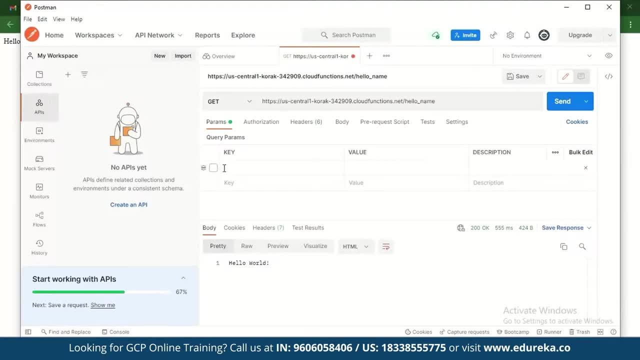 and check if it's working. and check if it's working right. so right now it shows me hello right. so right now it shows me hello right. so right now it shows me hello name. but this is a function which allows name, but this is a function which allows. 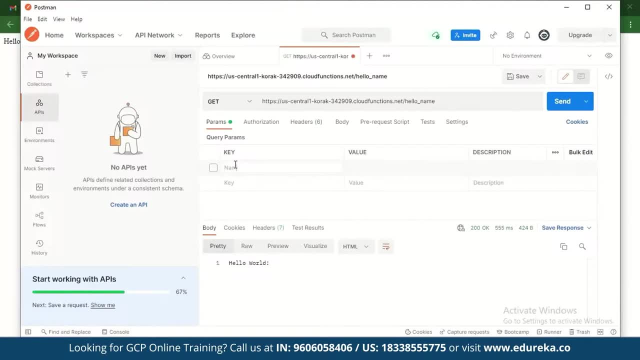 name. but this is a function which allows you to you, to you, to take in arguments, so let's just give it take in arguments. so let's just give it take in arguments, so let's just give it an argument like an argument, like an argument like name, and this can be a eureka. 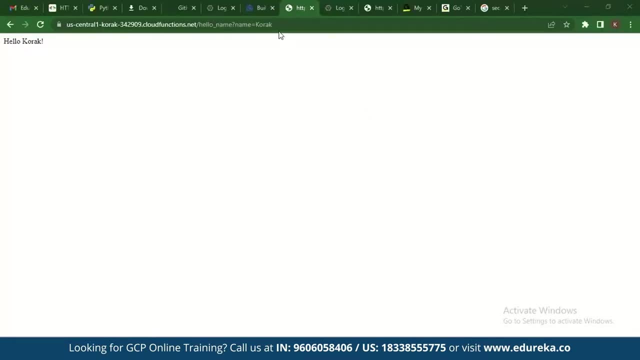 name, and this can be a eureka name, and this can be a eureka, right? so let's just check it out now, right? so let's just check it out now, right? so, let's just check it out now. so, basically, what happens is, if we can, 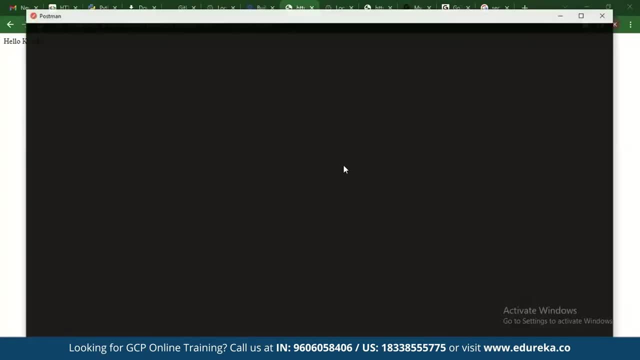 so, basically, what happens is if we can. so, basically, what happens is if we can see, see, see. this is the argument that we gave in, this is the argument that we gave in, this is the argument that we gave in. and go back to postman, and go back to postman. 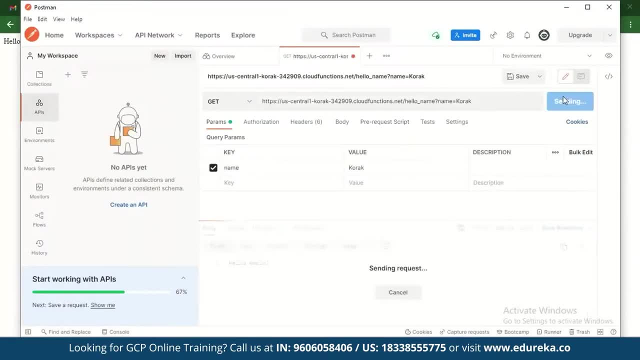 and go back to postman: change this and paste this. change this and paste this. change this and paste this, change it. it says hello cora, change it. it says hello cora, change it. it says hello cora because i have put in arguments here, because i have put in arguments here: 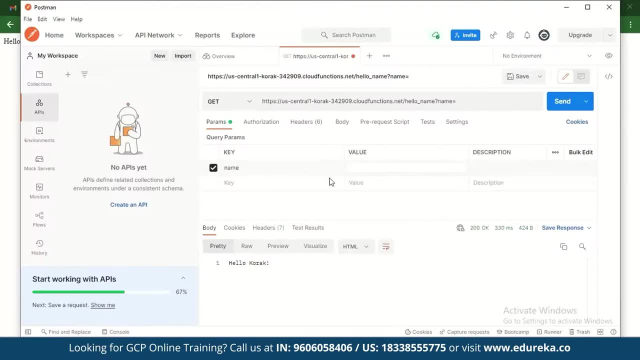 because i have put in arguments here: which has name and value of code now. which has name and value of code now. which has name and value of code now, let's, let's, let's change this to. let's say it will go. change this to: let's say it will go. 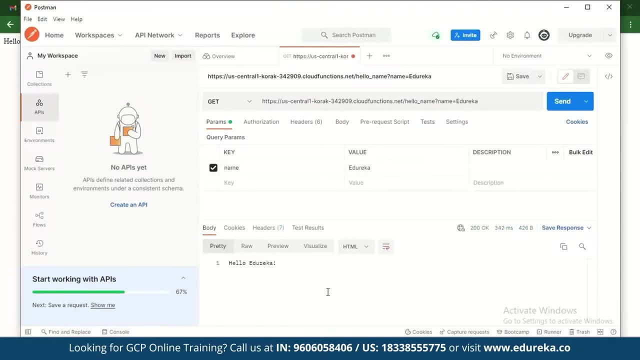 change this to, let's say, it will go and check if it's still working, and check if it's still working, and check if it's still working. right, so it is working. and this is right, so it is working. and this is right, so it is working. and this is basically how you create. 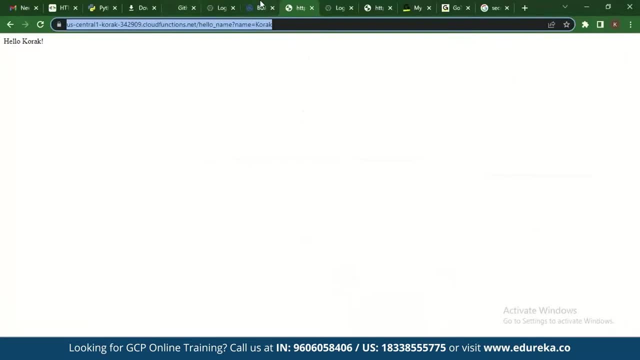 basically how you create, basically how you create an http triggered cloud function, an http triggered cloud function, an http triggered cloud function. now, with that, we come to the end of the now, with that, we come to the end of the now. with that, we come to the end of the demo. so the last thing we talk about is: 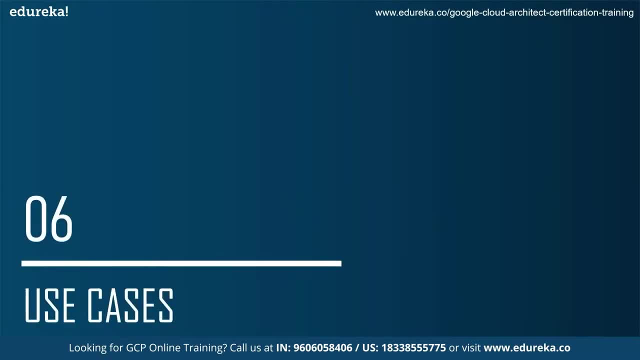 demo. so the last thing we talk about is demo. so the last thing we talk about is the different use cases that cloud, the different use cases that cloud, the different use cases that cloud functions has with different integrated functions, has with different integrated functions, has with different integrated apis. so we'll be talking about two use. 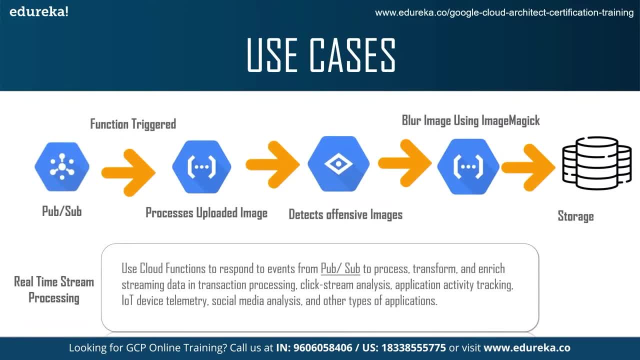 apis, so we'll be talking about two use apis. so we'll be talking about two use cases here. so the first use case- we talk cases here. so the first use case- we talk cases here. so the first use case we talk about is the real-time stream processing. 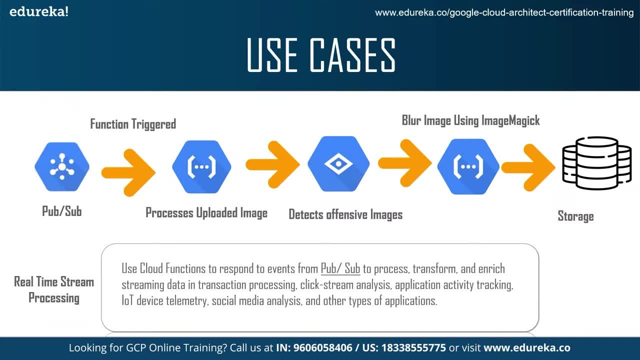 about. is the real-time stream processing about. is the real-time stream processing now. real-time stream processing is pub. now. real-time stream processing is pub. now. real-time stream processing is pub. sub will basically trigger a function. sub will basically trigger a function. sub will basically trigger a function now. this function will basically process. 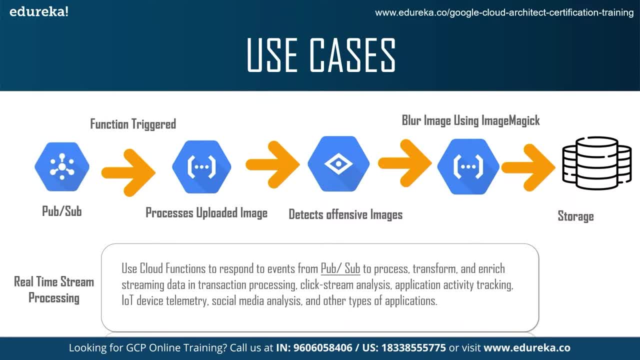 now this function will basically process. now. this function will basically process the uploaded image and detect the. the uploaded image and detect the. the uploaded image and detect the offensive images. if they are there now- offensive images. if they are there now- offensive images. if they are there now, this offensive image detection is done. 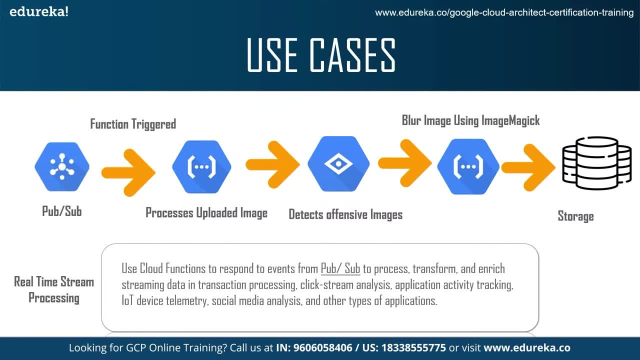 this offensive image detection is done. this offensive image detection is done using google cloud vision api. and if using google cloud vision api, and if using google cloud vision api, and if there is some offensive content- google, there is some offensive content. google, there is some offensive content- google cloud vision api sends a cloud. 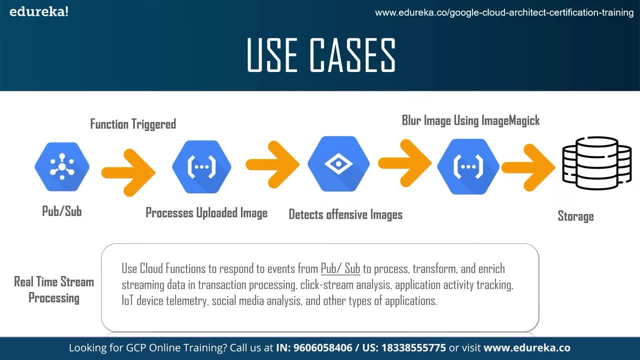 cloud vision api sends a cloud. cloud vision api sends a cloud function request to blur the image out function. request to blur the image out function- request to blur the image out, and this is then stored as a blurred. and this is then stored as a blurred and this is then stored as a blurred image in storage. and finally we talk. 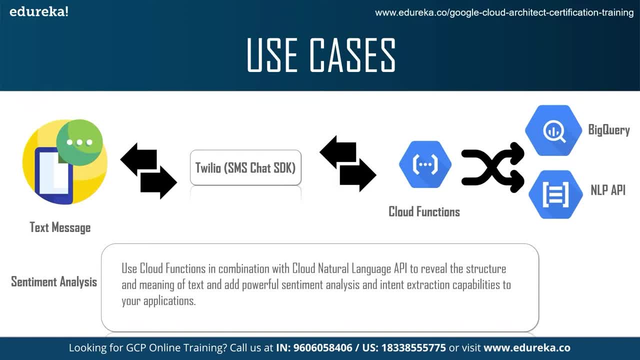 image in storage. and finally we talk image in storage and finally we talk about sentiment analysis now. so about sentiment analysis now. so about sentiment analysis now. so sentiment analysis, basically sentiment analysis, basically sentiment analysis, basically understanding the requirements or the understanding, the requirements or the understanding, the requirements or the behavior of the user in general. so 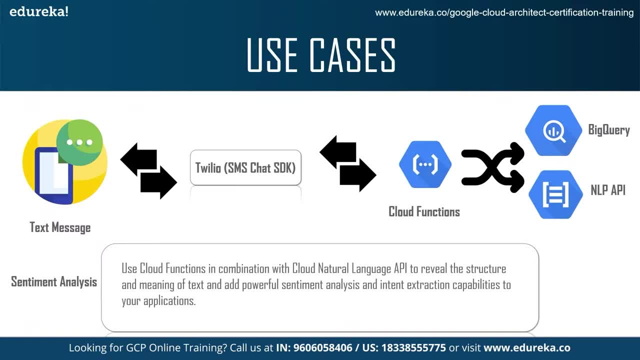 behavior of the user in general. so behavior of the user in general. so basically what we do here is basically what we do here is basically what we do here is: we see a text message and with that text we see a text message. and with that text we see a text message. and with that text message we use twillow, which is: 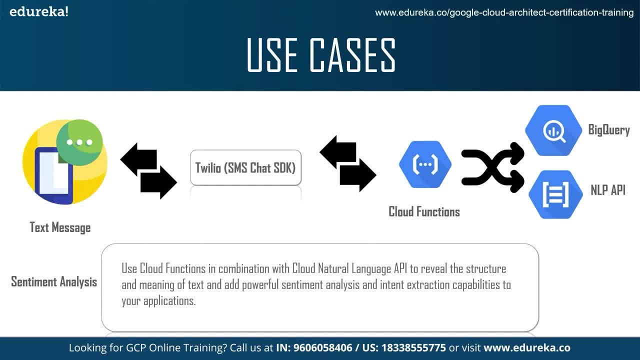 message. we use twillow, which is message. we use twillow, which is basically a chat sdk, and with cloud basically a chat sdk and with cloud basically a chat sdk and with cloud functions bigquery and mlp what it functions, bigquery and mlp what it. 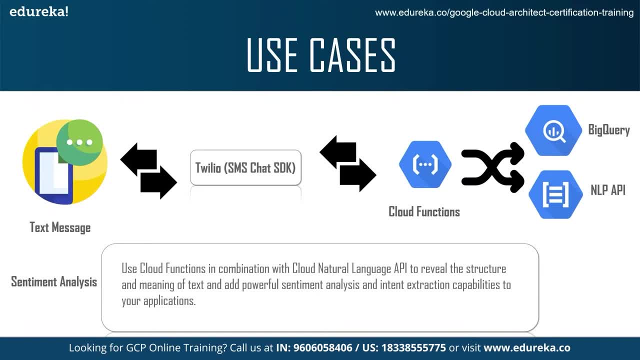 functions: bigquery and mlp. what it basically does is that it adds, basically does. is that it adds, basically does is that it adds sentimental analysis and intent, sentimental analysis and intent, sentimental analysis and intent, extraction capabilities to your extraction capabilities, to your extraction capabilities, to your application. right? so there is a lot of. 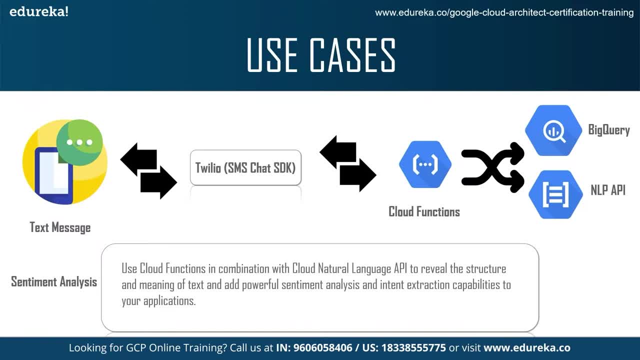 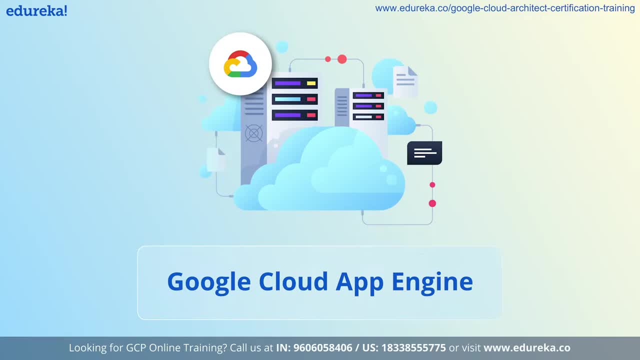 application right. so there is a lot of application right. so there is a lot of natural language processing involved, natural language processing involved, natural language processing involved here. so there is an integration with here. so there is an integration with here. so there is an integration with bigquery and nlp api as well. 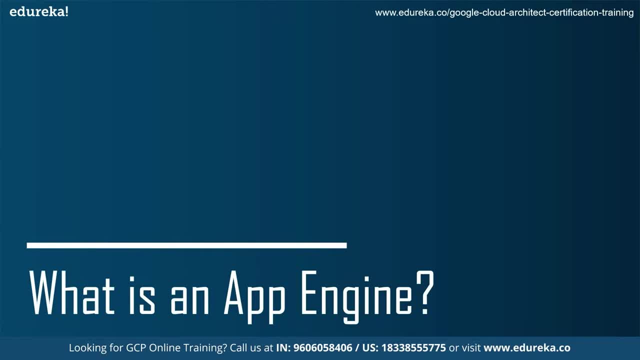 bigquery and nlp api as well. bigquery and nlp api as well. so you might be thinking, what an app? so you might be thinking what an app. so you might be thinking what an app? engine is, so let's have a little. engine is so let's have a little. 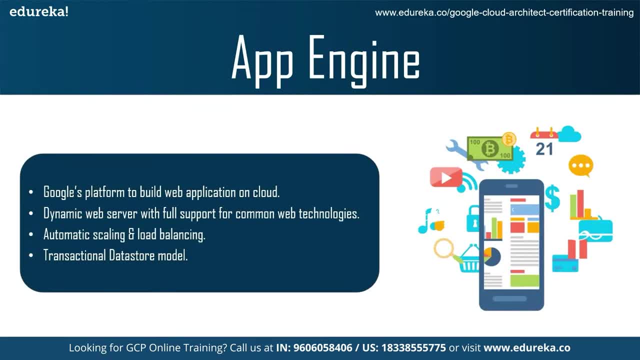 engine is. so let's have a little introduction to app engine. it is a fully introduction to app engine. it is a fully introduction to app engine. it is a fully managed serverless platform for managed serverless platform, for managed serverless platform for developing and hosting web applications. 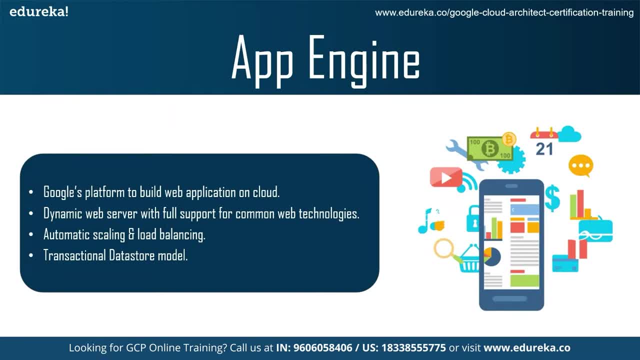 developing and hosting web applications. developing and hosting web applications at scale. you can choose from several at scale. you can choose from several at scale. you can choose from several popular languages libraries and popular languages libraries and popular languages libraries and frameworks to develop your apps. then let frameworks to develop your apps. then let 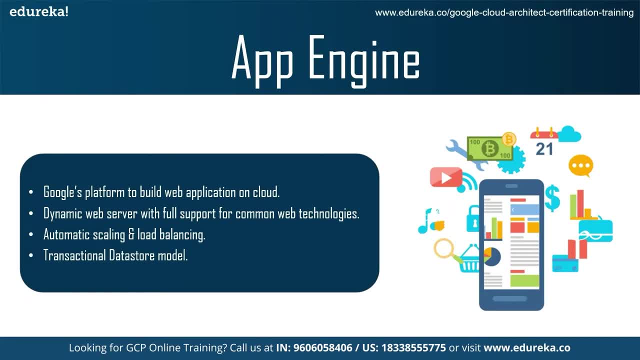 frameworks to develop your apps, then let app engine takes care of provisioning. app engine takes care of provisioning. app engine takes care of provisioning servers and scaling your app instances servers and scaling your app instances servers and scaling your app instances based on demand. based on demand, based on demand. now let's understand app engine service. 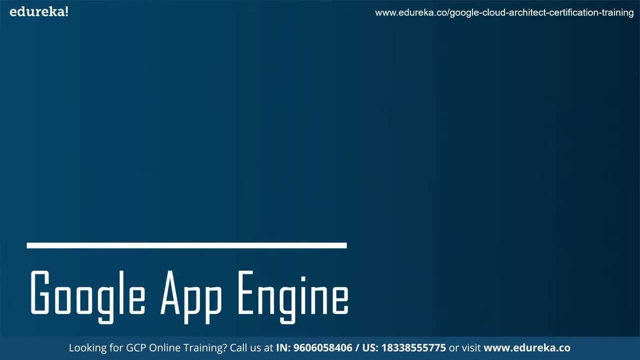 now let's understand app engine service. now let's understand app engine service provided by google cloud platform. that is provided by google cloud platform. that is provided by google cloud platform. that is google app engine, google app engine, google app engine. if i talk about google, then we all know. 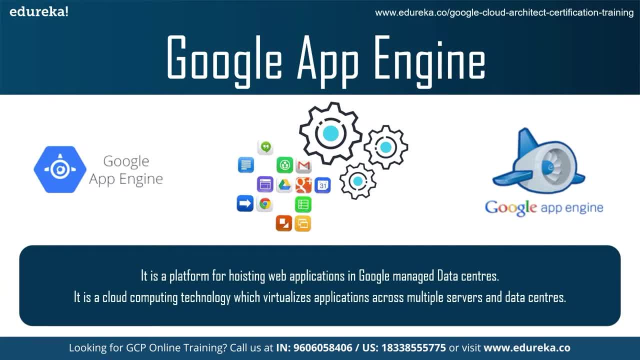 if i talk about google, then we all know. if i talk about google, then we all know that it provides an enormous range of that. it provides an enormous range of that. it provides an enormous range of tools, products and services in the tools, products and services in the. 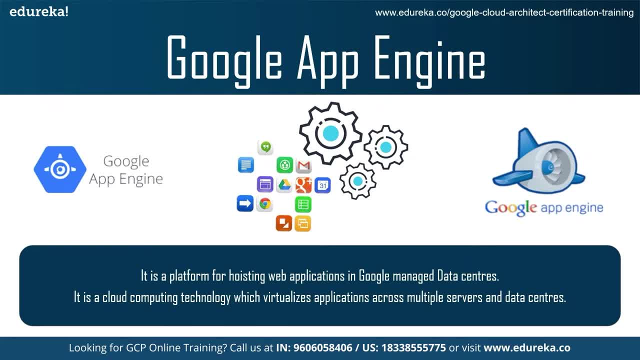 tools, products and services in the running market. google has scored high running market. google has scored high running market. google has scored high percentile and left the footprint in the percentile and left the footprint in the percentile and left the footprint in the list of world's top four companies. 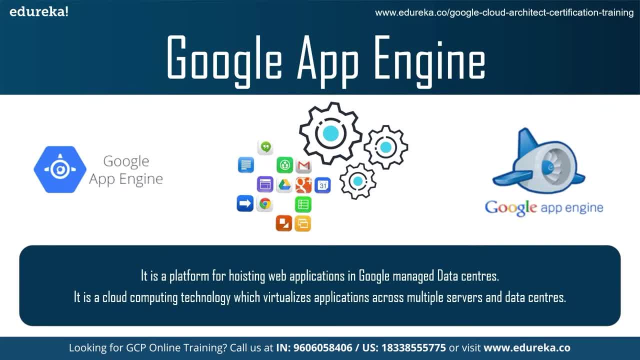 list of world's top four companies. list of world's top four companies. so google app engine by the name. only we so google app engine by the name. only we so google app engine by the name. only we can recognize that google has created an, can recognize that google has created an. 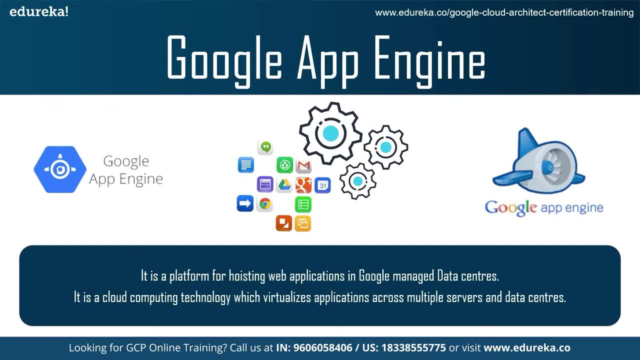 can recognize that google has created an app engine. the name is similar to a app engine. the name is similar to a app engine. the name is similar to a search engine, but its search engine, but its search engine, but its purpose is of course different app engine purpose is of course different app engine. 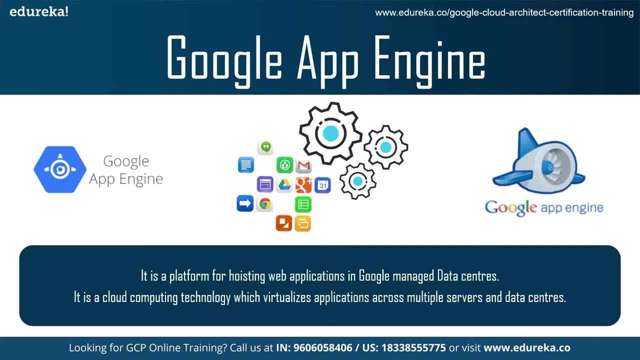 purpose is, of course, different: app engine is a service and cloud computing is a service and cloud computing is a service and cloud computing platform employed for developing and platform employed for developing and platform employed for developing and hosting web applications. hosting web applications. hosting web applications: it is a platform as a service- cloud. 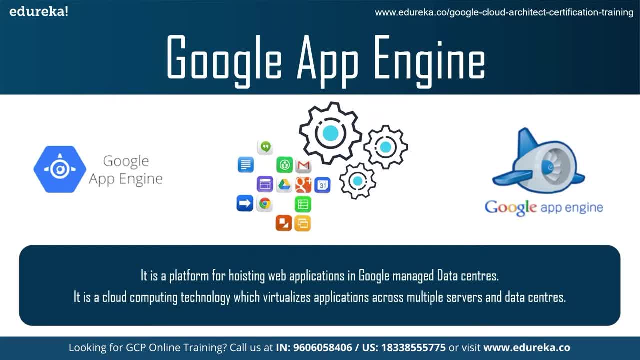 it is a platform as a service cloud. it is a platform as a service cloud computing platform that is entirely computing platform. that is entirely computing platform that is entirely managed and utilizes inbuilt services to managed and utilizes inbuilt services to managed and utilizes inbuilt services to drive the apps. 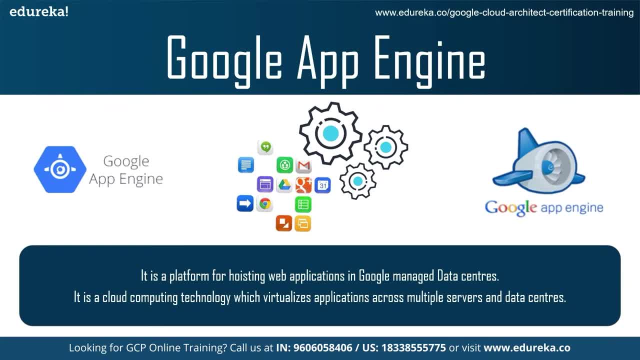 drive the apps. drive the apps once after downloading the sdk. that is once after downloading the sdk. that is once after downloading the sdk. that is software development kit. you can software development kit. you can software development kit. you can instantly start the development process. instantly start the development process. 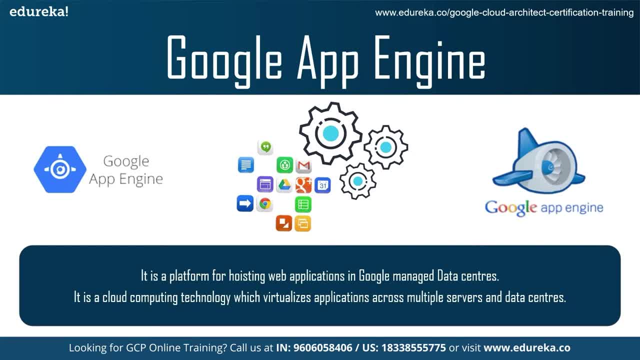 instantly start the development process, but for this it is mandatory to use. but for this it is mandatory to use. but for this it is mandatory to use technical knowledge. if you don't know technical knowledge, if you don't know technical knowledge, if you don't know the technical terms, then there is no. 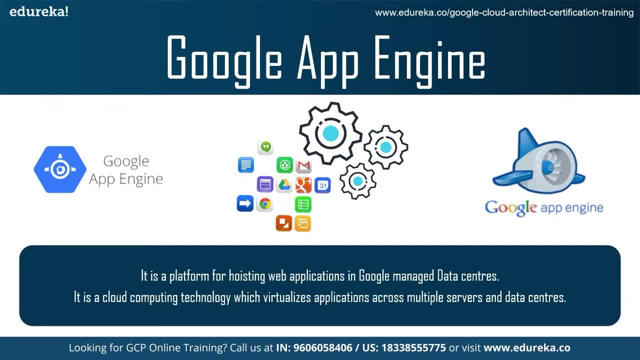 the technical terms, then there is no the technical terms, then there is no need to take tension. okay, as there are need to take tension. okay, as there are need to take tension. okay, as there are many id industries in the market, that many id industries in the market, that. 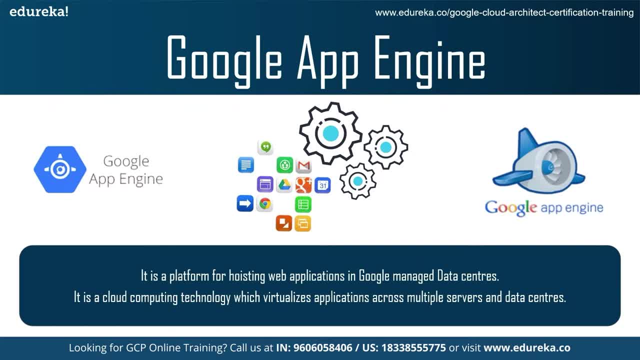 many id industries in the market that are providing google app engine are providing google app engine. are providing google app engine development services, development services. development services. app engine. lets you build highly app engine. lets you build highly app engine. lets you build highly scalable applications on a fully 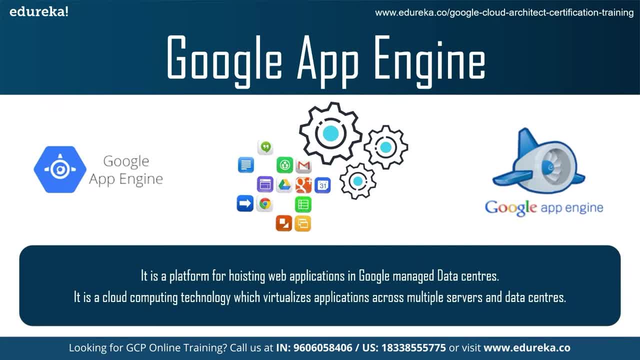 scalable applications on a fully scalable applications on a fully managed serverless platform also. you managed serverless platform also. you managed serverless platform also. you can scale your applications from zero to. can scale your applications from zero to. can scale your applications from zero to planet scale without having to manage. 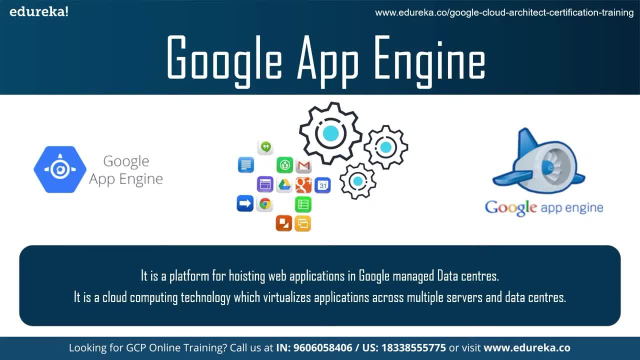 planet scale without having to manage planet scale without having to manage infrastructure. okay also, you can free up infrastructure. okay also, you can free up infrastructure. okay also, you can free up your developers with zero server, your developers with zero server, your developers with zero server management and zero configuration. 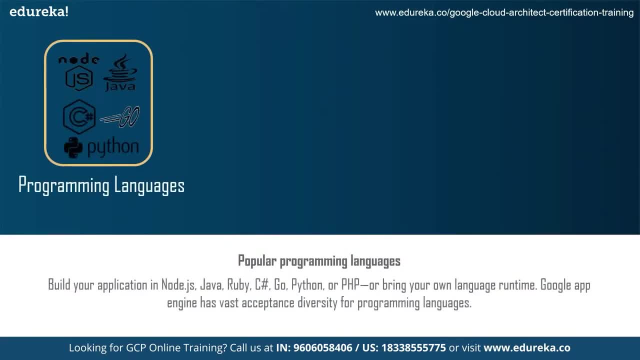 management and zero configuration. management and zero configuration of google app engine of google app engine of google app engine. if you see the programming languages: the. if you see the programming languages: the. if you see the programming languages: the platform supports php, c, java, python, go. platform supports php, c, java, python, go. 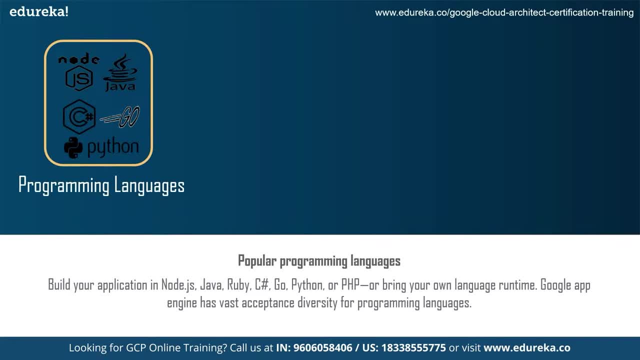 platform supports php, c, java, python, go, nodejs dot net and ruby applications, nodejs dot net and ruby applications, nodejs dot net and ruby applications, and, apart from this, it also supports, and apart from this, it also supports, and apart from this, it also supports, other programming languages through. 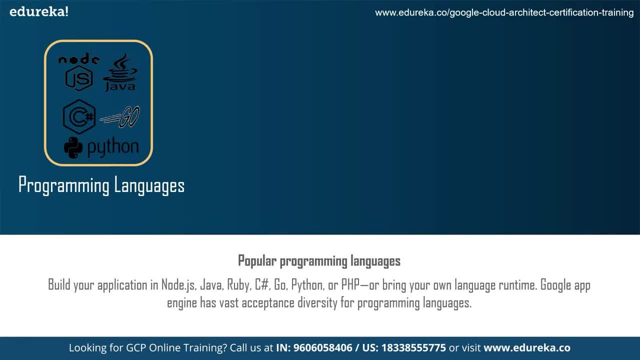 other programming languages through other programming languages, through custom runtimes, custom runtimes, custom runtimes. the app engine serves 350 plus billion. the app engine serves 350 plus billion. the app engine serves 350 plus billion requests per day. requests per day. requests per day. now, if you see, like how google app 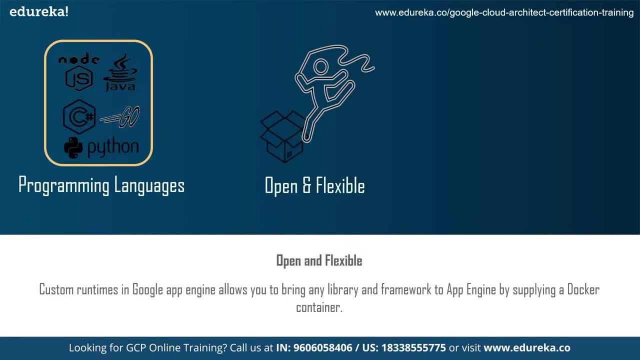 now, if you see, like how google app, now if you see like how google app engine is actually open and flexible, so engine is actually open and flexible, so engine is actually open and flexible. so so custom runtimes in google app engine, so custom runtimes in google app engine. 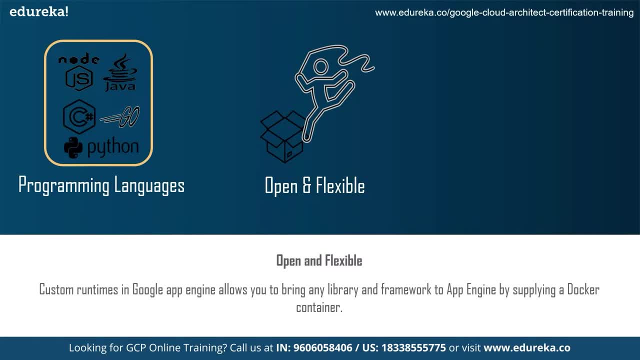 so custom runtimes in google app engine allows you to bring any library. and allows you to bring any library. and allows you to bring any library and framework to app engine by supplying a framework to app engine, by supplying a framework to app engine, by supplying a docker container. 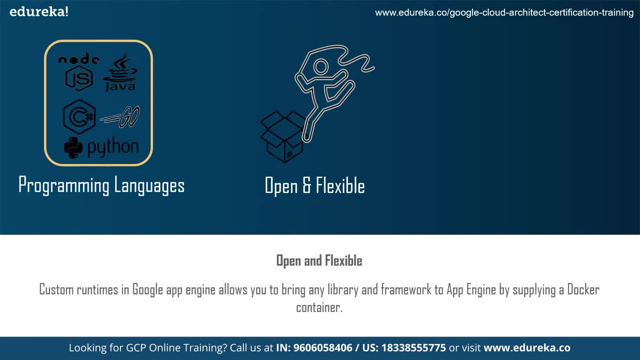 docker container- docker container so you can customize runtimes or provide. so you can customize runtimes or provide. so you can customize runtimes or provide your own runtime by supplying a your own runtime. by supplying a your own runtime by supplying a customer docker image or docker file from 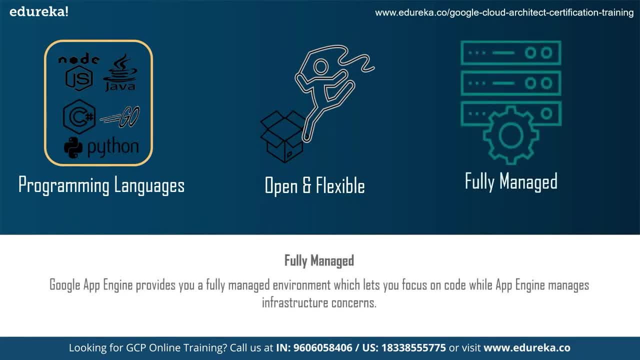 customer docker image or docker file from customer docker image or docker file from the open source community, the open source community, the open source community. then you can see like google app engine. then you can see like google app engine. then you can see like google app engine is actually fully managed. 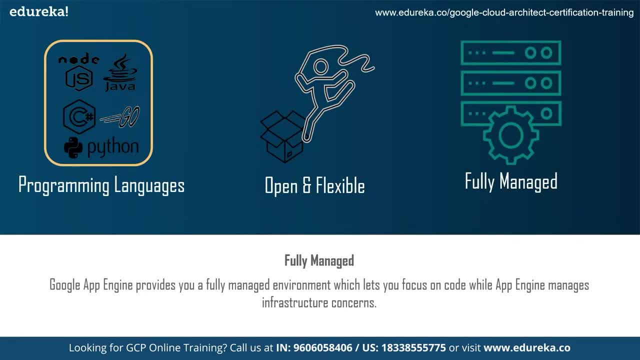 is actually fully managed, is actually fully managed. so google app engine's fully managed. so google app engine's fully managed. so google app engine's fully managed environment, which makes it easy to build environment, which makes it easy to build environment, which makes it easy to build and deploy an application that runs. 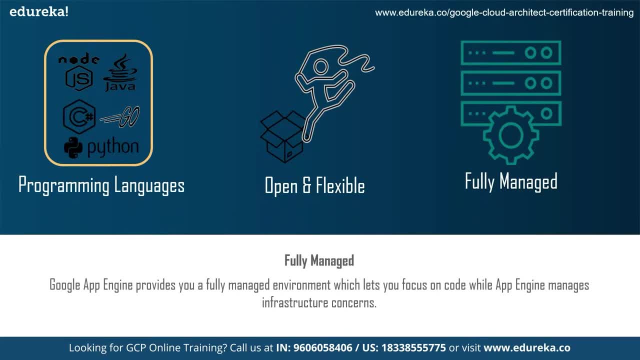 and deploy an application that runs and deploy an application that runs reliably, even under heavy load, and with reliably, even under heavy load, and with reliably, even under heavy load, and with large amounts of data, large amounts of data, large amounts of data, and which lets you focus on code while 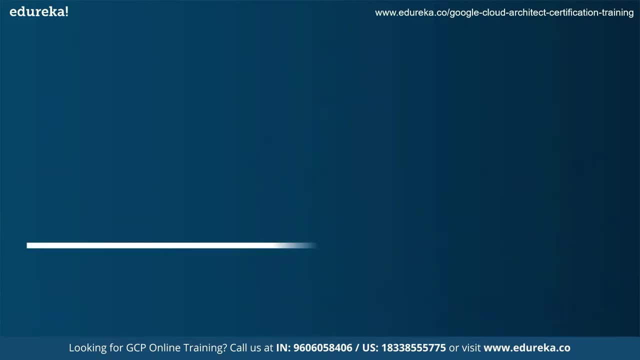 and which lets you focus on code while. and which lets you focus on code while. app engine manages infrastructure. app engine manages infrastructure. app engine manages infrastructure, concerns, concerns, concerns. let's now see the architecture of google. let's now see the architecture of google. let's now see the architecture of google app engine. 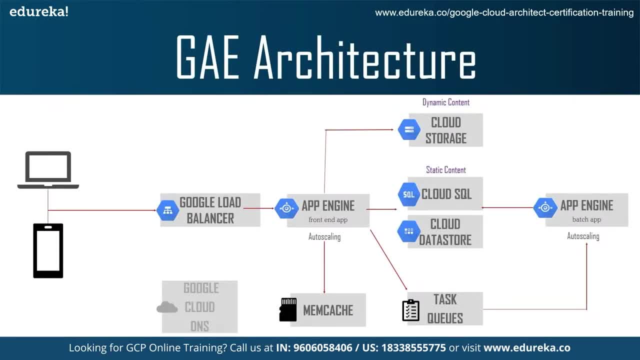 app engine. app engine. so this is how a simplified architecture. so this is how a simplified architecture. so this is how a simplified architecture looks like among the main services. and looks like among the main services and looks like among the main services and structures available are google load. 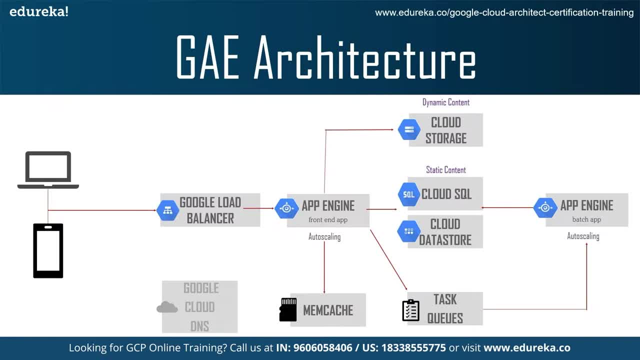 structures available? are google load structures available? are google load balancer which manages the load balancer, which manages the load balancer, which manages the load balancing of the applications? then we balancing of the applications, then we balancing of the applications, then we have front-end app which is responsible. 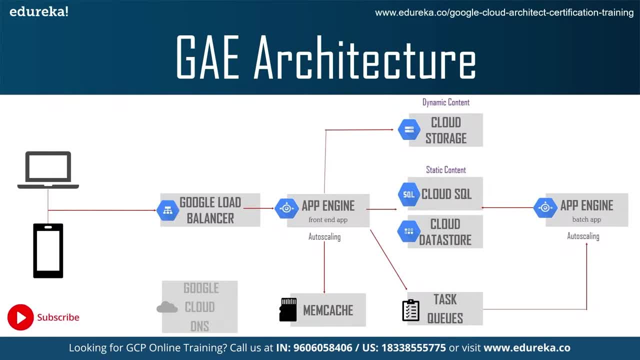 have front-end app, which is responsible. have front-end app which is responsible for redirecting requests for appropriate for redirecting requests for appropriate for redirecting requests for appropriate services, services, services. then we have main cache. that is a cache. then we have main cache, that is a cache. 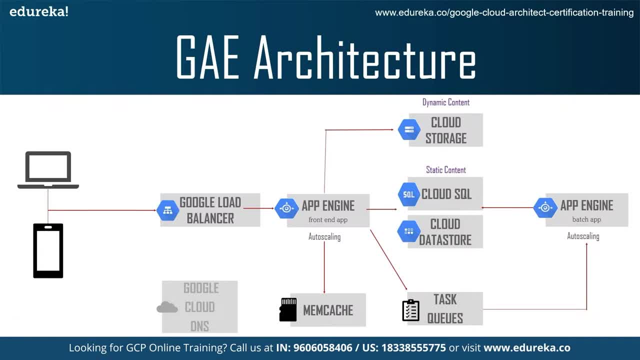 then we have main cache, that is, a cache memory shared between instances of memory, shared between instances of memory, shared between instances of google app engine generating high speed google app engine. generating high speed google app engine. generating high speed in the availability of the. in the availability of the. 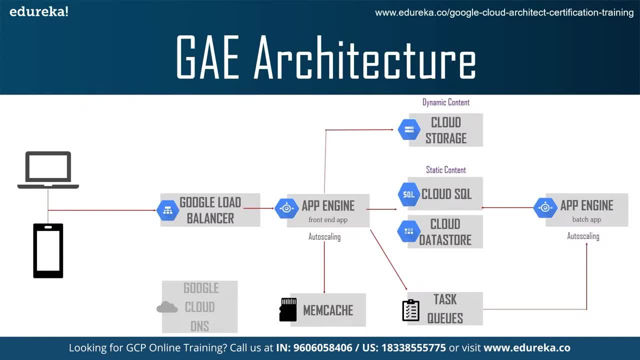 in the availability of the information on the server and task use. information on the server and task use. information on the server and task use is used, which is like a task use, if you is used, which is like a task use if you is used which is like a task use, if you see, that is a mechanism that provides. 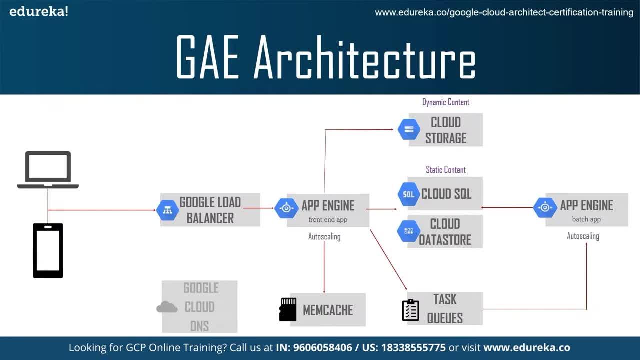 see, that is a mechanism that provides. see, that is a mechanism that provides: redirection of long tasks to back-end. redirection of long tasks to back-end. redirection of long tasks to back-end. servers, servers, servers. making front-end servers free for new. making front-end servers free for new. 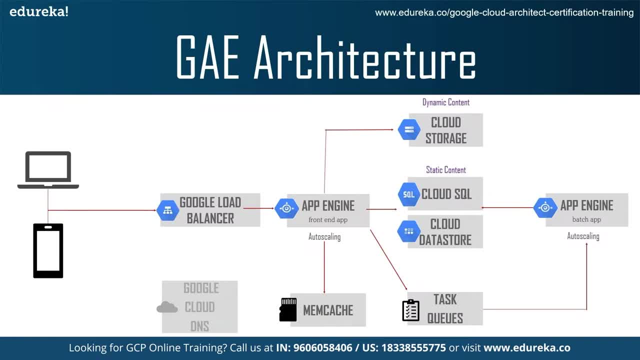 making front-end servers free for new users requests: users requests: users requests. in addition, google app engine also has: in addition, google app engine also has: in addition, google app engine also has: static and dynamic storage. static and dynamic storage. static and dynamic storage solutions. the static storage solution. 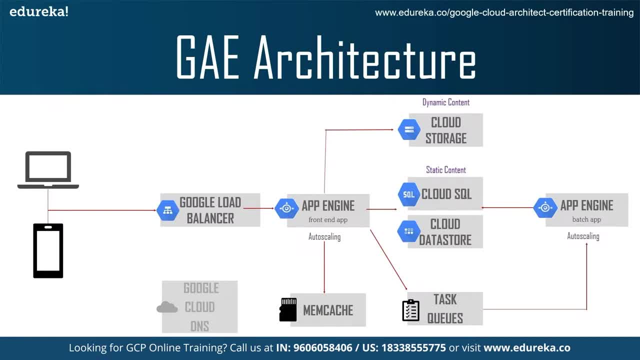 solutions: the static storage solution solutions. the static storage solution provides the file storage service, provides the file storage service, provides the file storage service called cloud storage, whereas the dynamic called cloud storage, whereas the dynamic called cloud storage. whereas the dynamic storage solution provides relational storage solution, provides relational. 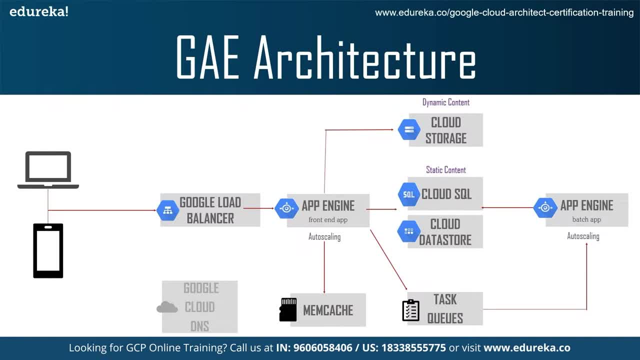 storage solution provides relational database services, database services, database services such as the cloud sql and no relational such as the cloud sql, and no relational such as the cloud sql, and no relational- no sql such as cloud data store. no sql such as cloud data store. no sql such as cloud data store. now let's see the development cycle of 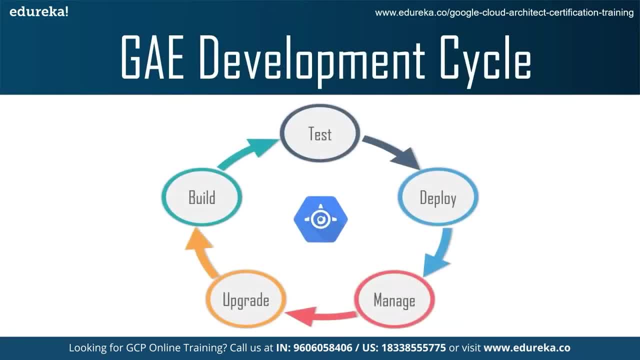 now let's see the development cycle of now. let's see the development cycle of google app engine. google app engine. google app engine- here, if you see test build and deploy is here. if you see test build and deploy is here. if you see test build and deploy is the software development kit. 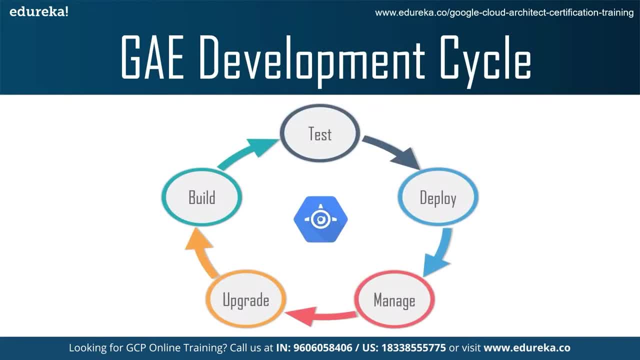 the software development kit. the software development kit means sdk, so sdk is a set of software, means sdk, so sdk is a set of software, means sdk, so sdk is a set of software development tools that allows the development tools, that allows the development tools, that allows the creation of applications for a certain 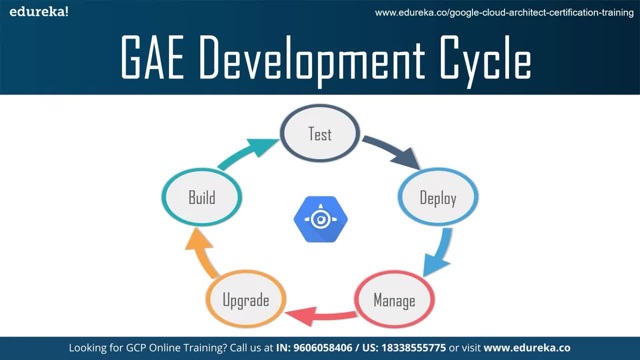 creation of applications for a certain. creation of applications for a certain software package: software framework software package, software framework software package, software framework hardware platform, computer system, video hardware platform. computer system, video hardware platform, computer system, video game console, game console, also operating system or similar, also operating system or similar. 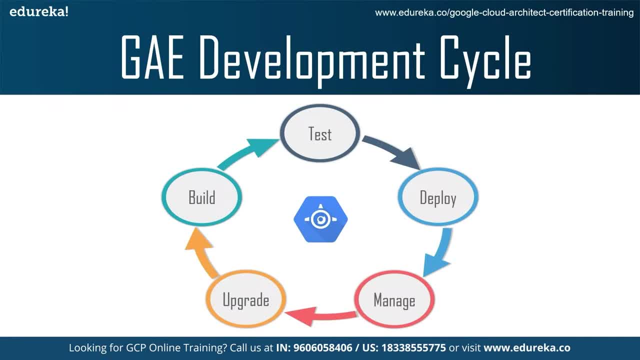 also operating system or similar development platforms, development platforms, development platforms. the next one cycle is managed, which is the next one cycle is managed, which is the next one cycle is managed, which is an app engine administration control, an app engine administration control, an app engine administration control, and then we have upgrades, like all the 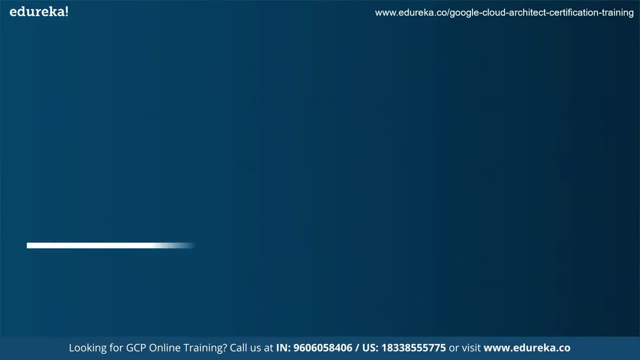 and then we have upgrades like all the. and then we have upgrades like all the. updates are being provided for. updates are being provided for. updates are being provided for: deployment to software development kit. deployment to software development kit. deployment to software development kit. now let's look at the components of an 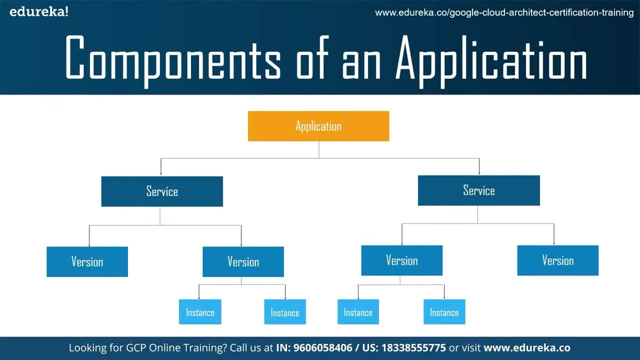 now let's look at the components of an. now let's look at the components of an application: the app engine application application. the app engine application application, the app engine application, is created under your google cloud project, is created under your google cloud project, is created under your google cloud project when you create an application resource. 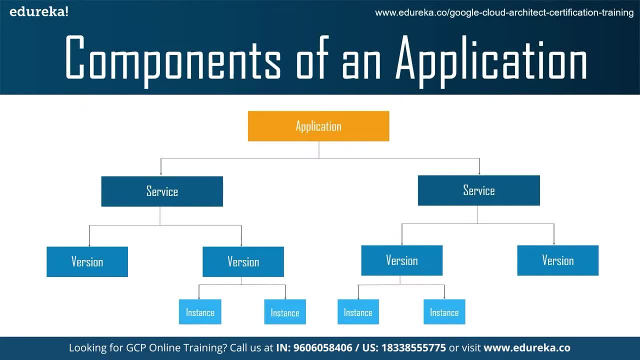 when you create an application resource. when you create an application resource, the app engine application is a top level. the app engine application is a top level. the app engine application is a top level container. that includes the service container, that includes the service container, that includes the service version and instance resources that make 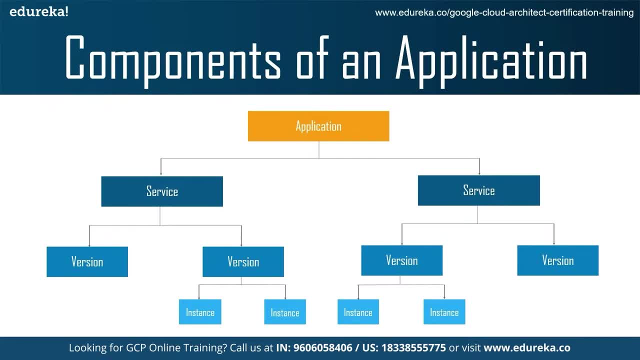 version and instance resources that make version and instance resources that make up your app. up your app, up your app. when you create your app engine app- all when you create your app engine app- all when you create your app engine app- all your resources are created in the region. 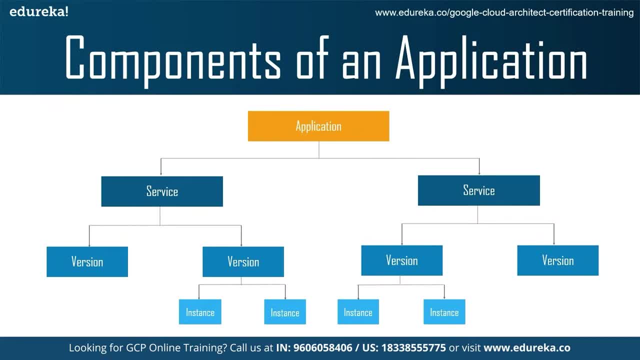 your resources are created in the region. your resources are created in the region that you choose, including your app code that you choose. including your app code that you choose. including your app code along with a collection of settings, along with a collection of settings, along with a collection of settings, credentials and your apps metadata. 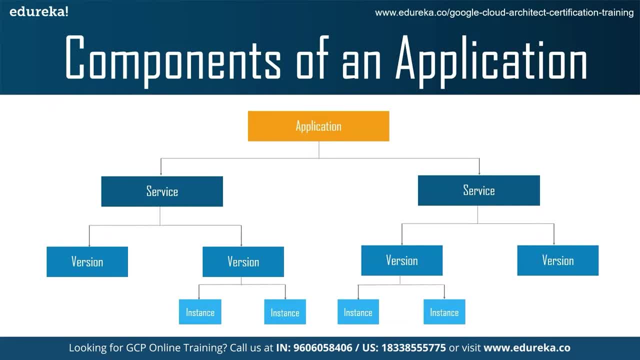 credentials and your apps metadata. credentials and your apps metadata: each app engine application includes: each app engine application includes: each app engine application includes at least one service: the default service. at least one service. the default service. at least one service. the default service, which can hold many versions. 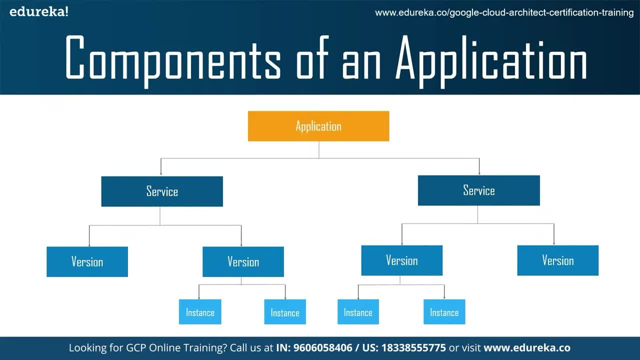 which can hold many versions. which can hold many versions, depending on your app billing status. depending on your app billing status. depending on your app billing status. the following diagram illustrates the. the following diagram illustrates the. the following diagram illustrates the hierarchy of an app engine application: hierarchy of an app engine application. 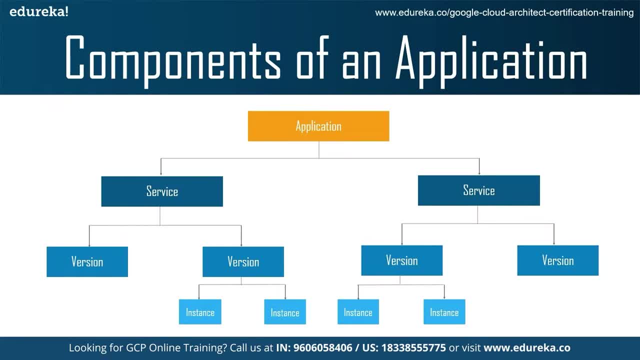 hierarchy of an app engine application running with multiple services in the running, with multiple services in the running, with multiple services. in the diagram, the app has two services that diagram. the app has two services that diagram. the app has two services that contain multiple versions and two of. 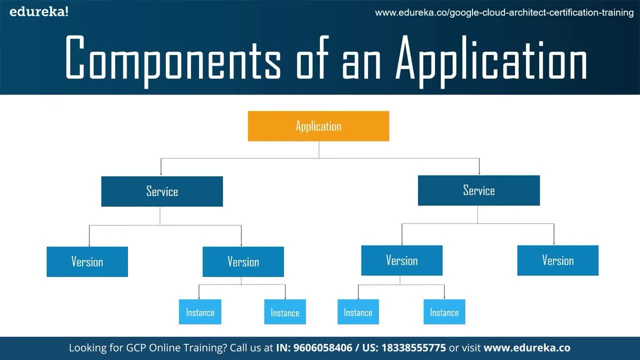 contain multiple versions and two of contain multiple versions and two of those versions are actively running on. those versions are actively running on. those versions are actively running on multiple instances, multiple instances, multiple instances. so let's understand service inside is so let's understand service inside is so let's understand service inside is so you can use services in app engine to 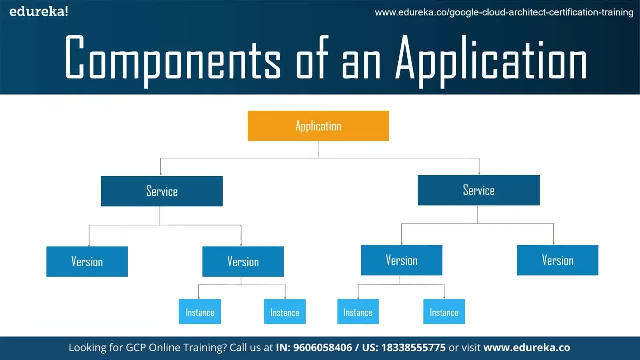 so you can use services in app engine to. so you can use services in app engine to factor your large apps into logical factor, your large apps into logical factor, your large apps into logical components that can, components that can, components that can securely share app engine features. and 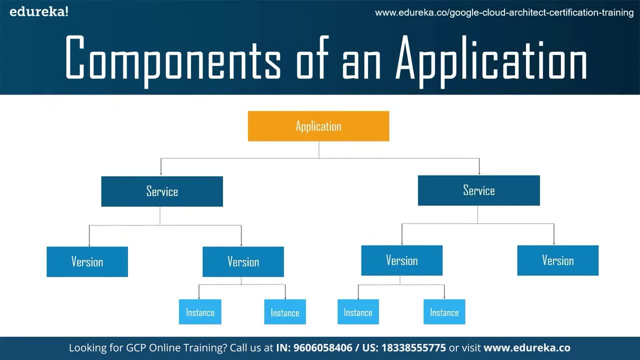 securely share app engine features and securely share app engine features and communicate with one another. communicate with one another. communicate with one another generally. your app engine services generally, your app engine services generally, your app engine services, behave like micro services. therefore, you behave like micro services. therefore you 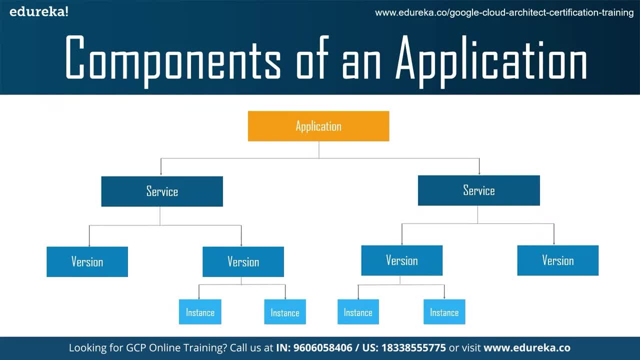 behave like micro services. therefore, you can run your whole app in a single, can run your whole app in a single, can run your whole app in a single service, or you can design and deploy service, or you can design and deploy service, or you can design and deploy multiple services to run as a set of. 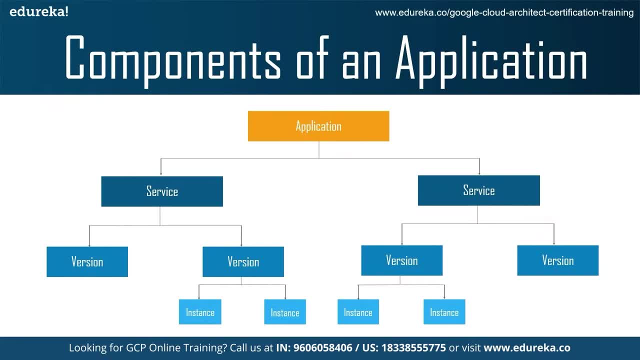 multiple services to run as a set of multiple services. to run as a set of micro services, micro services, micro services- for example, an app that handles your, for example, an app that handles your, for example, an app that handles your customer request might include separate. customer request might include separate. 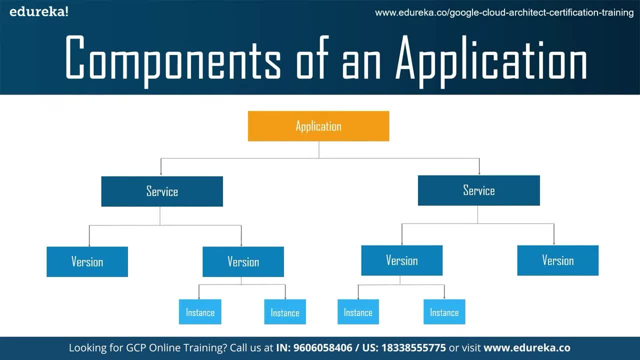 customer request might include separate services that each handle different tasks. services that each handle different tasks. services that each handle different tasks, such as api requests from mobile devices, such as api requests from mobile devices. such as api requests from mobile devices. internal administration type requests. internal administration type requests. 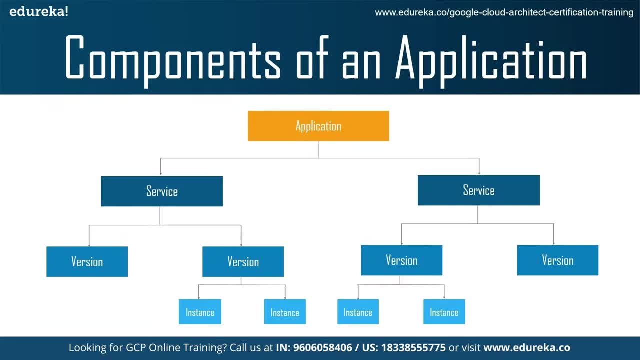 internal administration. type requests: backend processing, such as billing. backend processing, such as billing. backend processing, such as billing pipelines and data analysis pipelines and data analysis, pipelines and data analysis. each service and app engine consists of. each service and app engine consists of each service and app engine consists of the source code from your app and the. 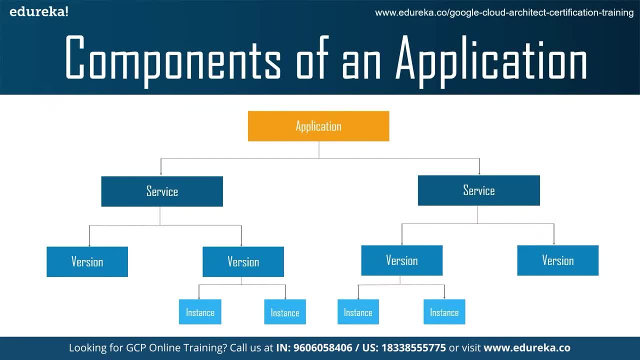 the source code from your app and the. the source code from your app and the corresponding app engine configuration. corresponding app engine configuration. corresponding app engine configuration files. the set of files that you deploy files. the set of files that you deploy files. the set of files that you deploy to your service represent a single. 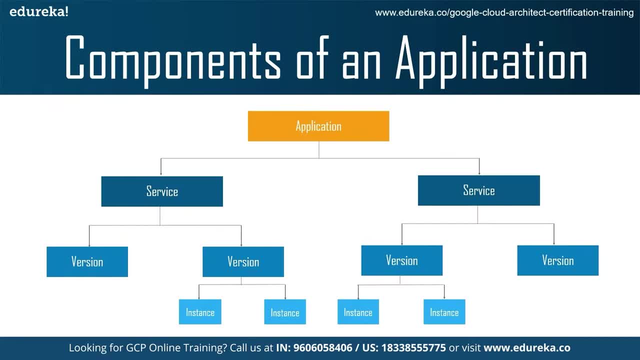 to your service. represent a single to your service. represent a single version of that service and each time version of that service and each time version of that service. and each time that you deploy to that service, you are that you deploy to that service. you are that you deploy to that service, you are creating additional versions within that. 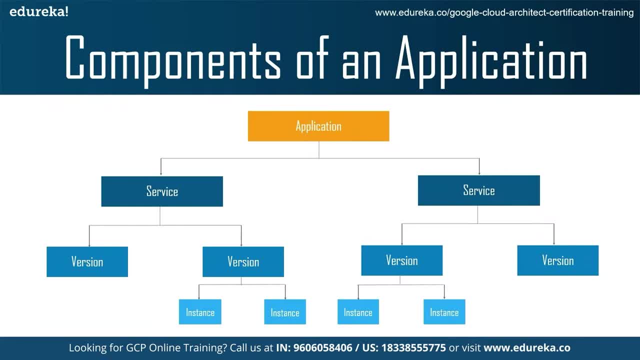 creating additional versions within that, creating additional versions within that same service. then we have versions having same service, then we have versions having same service, then we have versions having multiple versions of your app within multiple versions of your app, within multiple versions of your app within each service. allows you to quickly switch. 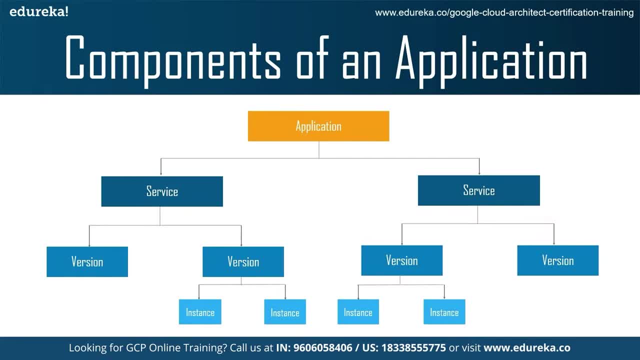 each service allows you to quickly switch. each service allows you to quickly switch between different versions of the app, between different versions of the app, between different versions of the app for rollbacks, testing or other temporary for rollbacks, testing or other temporary for rollbacks, testing or other temporary events. you can route traffic to one or 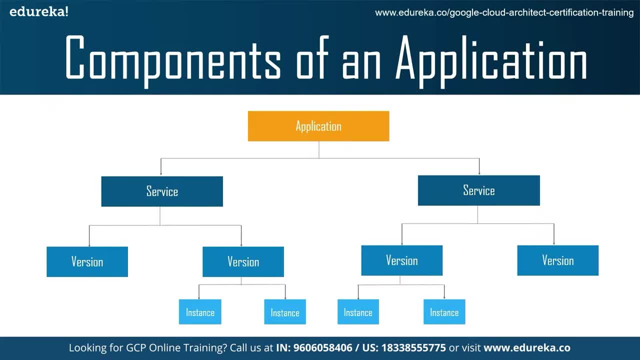 events you can route traffic to one or events you can route traffic to one or more specific versions of your app by more specific versions of your app, by more specific versions of your app, by migrating or splitting traffic, then we migrating or splitting traffic, then we migrating or splitting traffic, then we have instances. so the versions within. 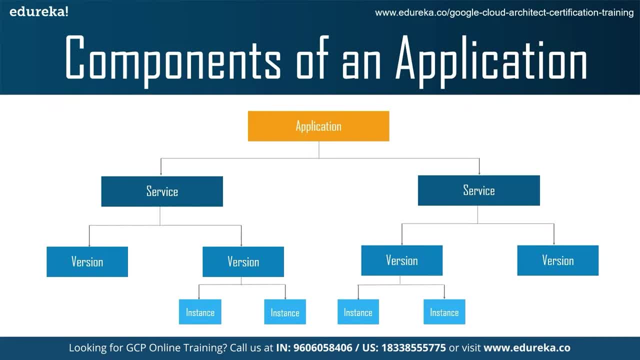 have instances. so the versions within have instances. so the versions within. your services run on one or more. your services run on one or more. your services run on one or more instances. okay, by default. app engine instances. okay, by default, app engine instances. okay, by default. app engine scales your app to match the load your 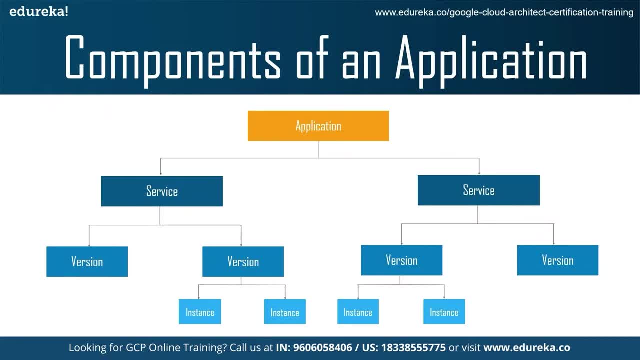 scales your app to match the load. your scales your app to match the load. your apps will scale up the number of apps will scale up the number of apps will scale up the number of instances that are running to provide instances that are running. to provide instances that are running to provide consistent performance, or scale down to. 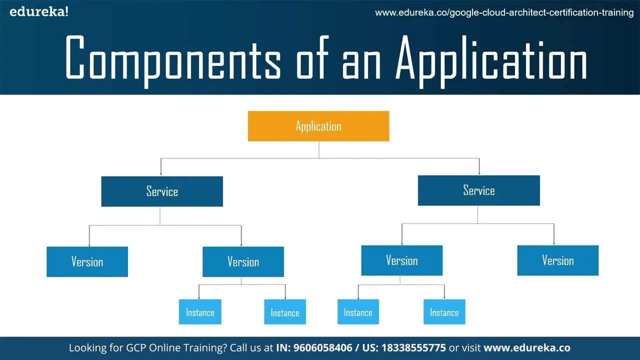 consistent performance or scale down to consistent performance or scale down to minimize idle instances and reduces minimize idle instances and reduces minimize idle instances and reduces costs. for more information about costs: for more information about costs. for more information about instances: see how instances are managed. instances: see how instances are managed. 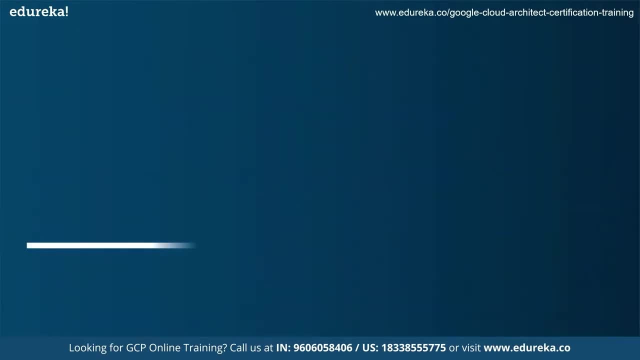 instances, see how instances are managed. okay, I will explain you that in the demo. okay, I will explain you that in the demo. okay, I will explain you that in the demo. so, now that you have a theoretical, so, now that you have a theoretical, so now that you have a theoretical understanding of Google App Engine, let's 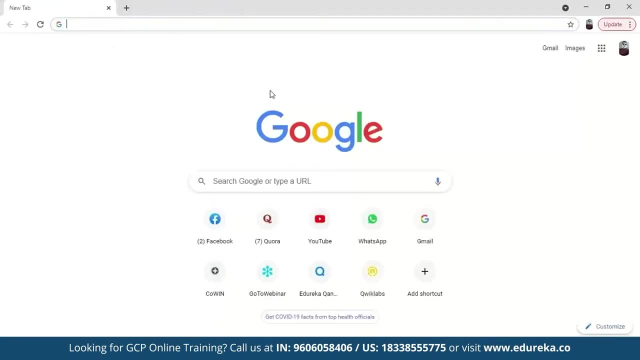 understanding of Google App Engine. let's understanding of Google App Engine. let's implement a simple app through Google. implement a simple app through Google. implement a simple app through Google App Engine. App Engine, App Engine, so you can just go to Google Cloud. so you can just go to Google Cloud. 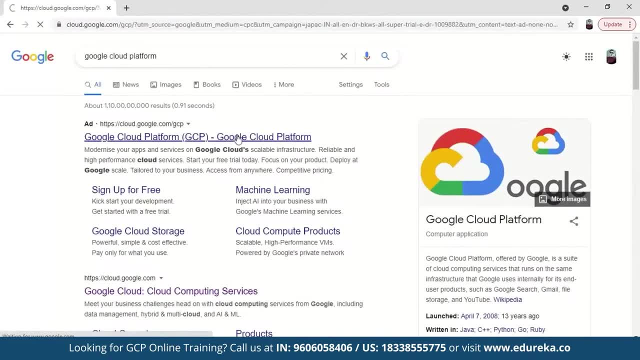 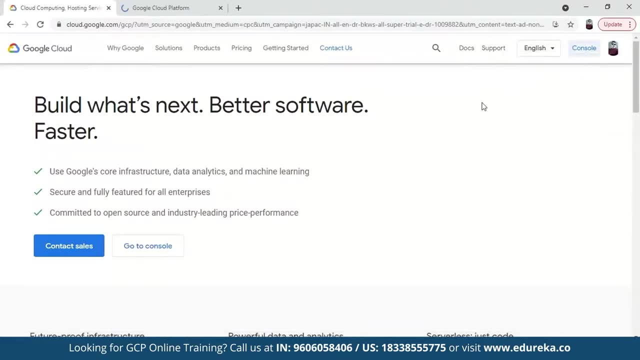 so you can just go to Google Cloud platform, platform, platform. open it, open it, open it. you have console and we have documents. you have console and we have documents. you have console and we have documents also. open the console also. yeah, also open the console also. yeah, also open the console also. yeah, remember that if you don't have an account, 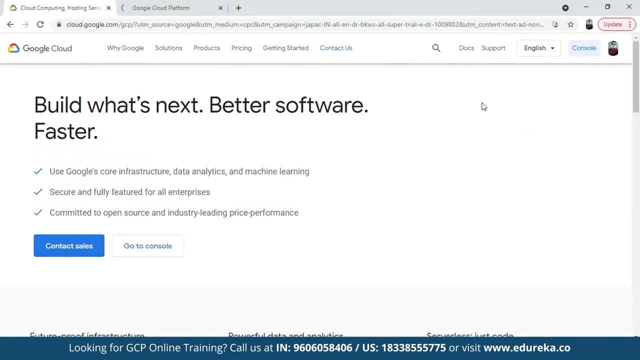 remember that if you don't have an account, remember that if you don't have an account on Google Cloud platform, it's a very good on Google Cloud platform. it's a very good on Google Cloud platform. it's a very good platform to have your account on. just, platform to have your account on. just platform to have your account on. just create your account. it will ask for your create your account. it will ask for your create your account. it will ask for your some basic details of your name and phone. some basic details of your name and phone. 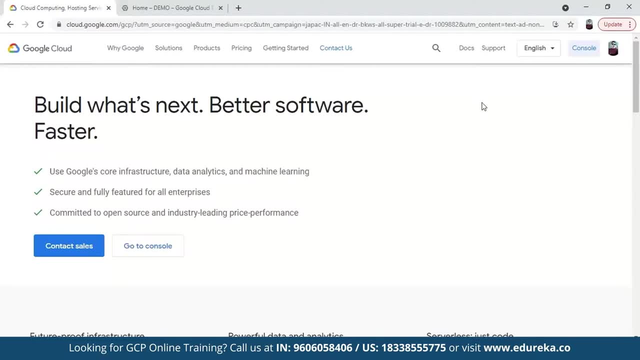 some basic details of your name and phone numbers and address and it will also numbers and address. and it will also numbers and address and it will also ask for your credit and debit card. ask for your credit and debit card. ask for your credit and debit card details. it will just deduct one rupee. 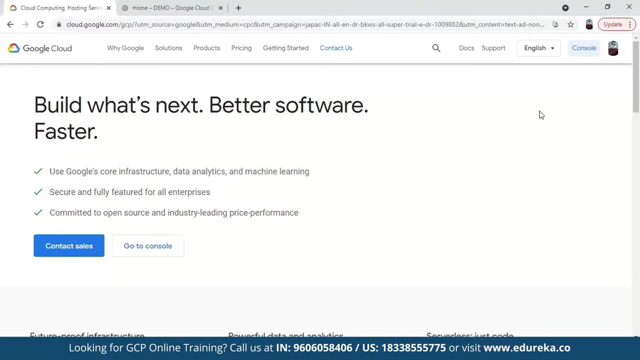 details: it will just deduct one rupee. details: it will just deduct one rupee and that will also be refunded within a. and that will also be refunded within a. and that will also be refunded within a while and free trial: you will get 300 while and free trial: you will get 300. 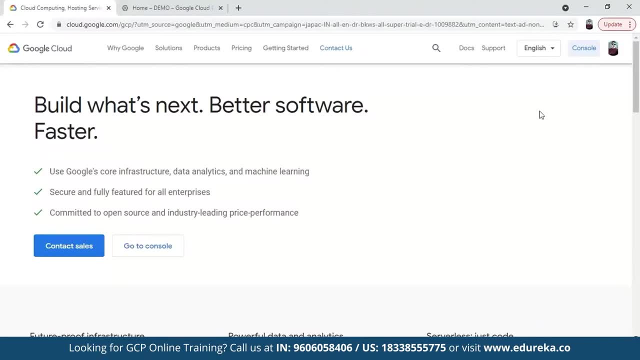 while and free trial, you will get 300 dollar credit for 90 days and you can dollar credit for 90 days and you can dollar credit for 90 days and you can use that credit for like i'm showing you, use that credit for like i'm showing you. 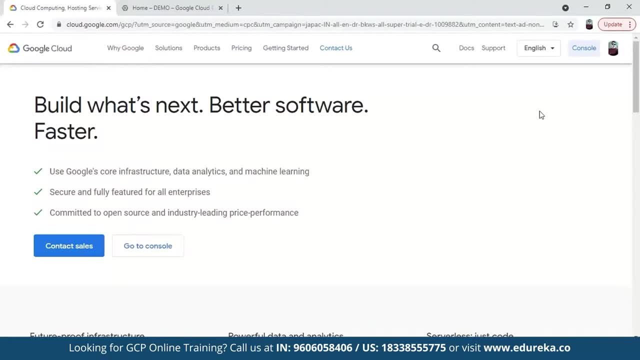 use that credit for, like, i'm showing you some exercises inside app engine. you can some exercises inside app engine. you can some exercises inside app engine. you can perform those exercises using those, perform those exercises using those. perform those exercises using those credit. okay, so you can just show, we have. 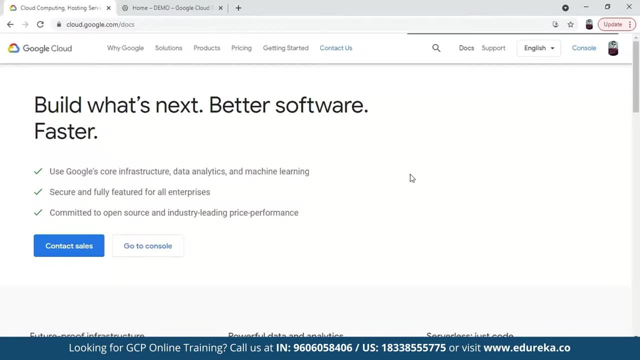 credit. okay, so you can just show we have credit. okay, so you can just show we have opened the dashboard and let's go to the opened the dashboard. and let's go to the opened the dashboard and let's go to the documents: part documents. part documents: part inside this. we have to go to the compute. 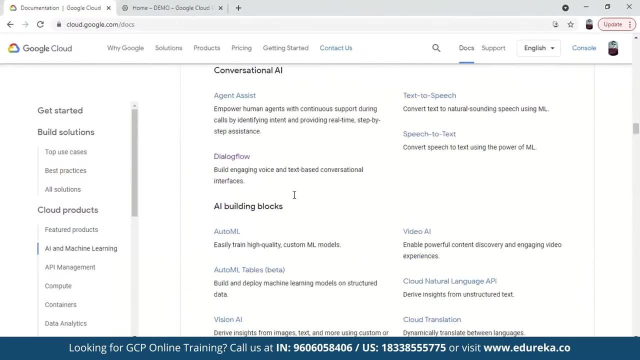 inside this we have to go to the compute. inside this we have to go to the compute. product under compute. we have app engine product under compute. we have app engine product under compute, we have app engine. so so, so here it is compute app engine, here it is compute app engine. 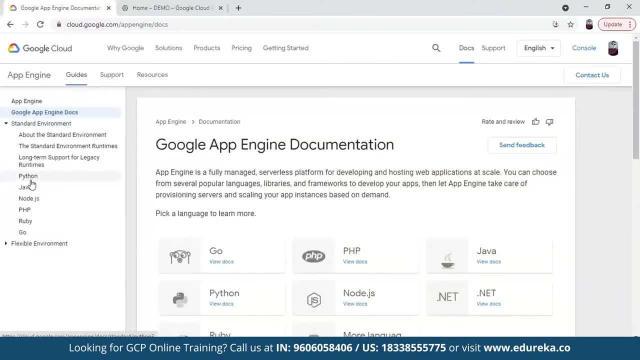 here it is compute app engine, then go to standard environment, then go to standard environment, then go to standard environment to python. we are going to implement a to python. we are going to implement a to python. we are going to implement a simple app of hello world using python. 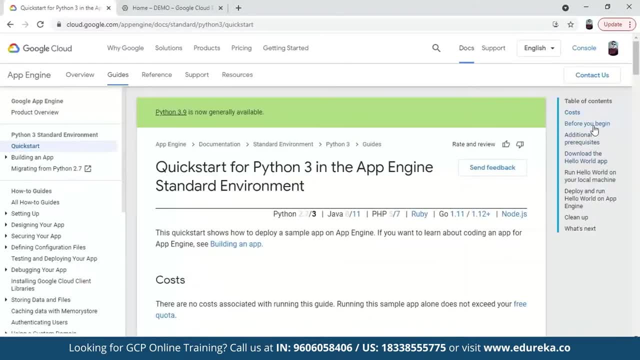 simple app of hello world using python. simple app of hello world using python: quick start, quick start, quick start. these are the table of contents for how. these are the table of contents for how. these are the table of contents for how we are going to implement the app. 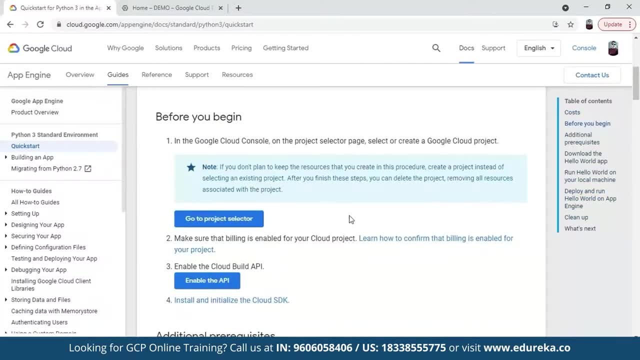 we are going to implement the app. we are going to implement the app. okay. so inside, this is the first step- is okay. so inside, this is the first step is okay. so inside, this is the first step- is: you have to create a project in. you have to create a project in. 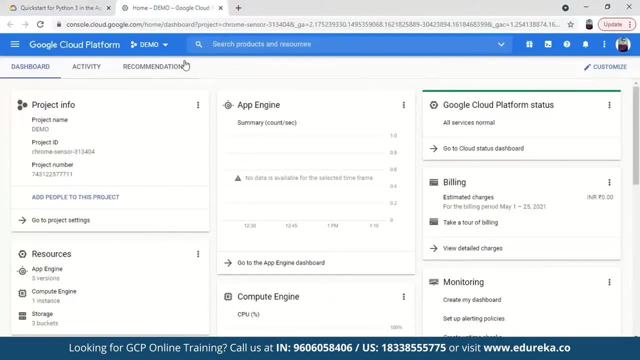 you have to create a project in google cloud platform. this is how the google cloud platform. this is how the google cloud platform. this is how the dashboard of google cloud platform looks. dashboard of google cloud platform looks. dashboard of google cloud platform looks like, like, like, and you go here. this is the demo means. and you go here. this is the demo means. and you go here. this is the demo means. it's written because it's the name of my. it's written because it's the name of my. it's written because it's the name of my project. these are the same number of 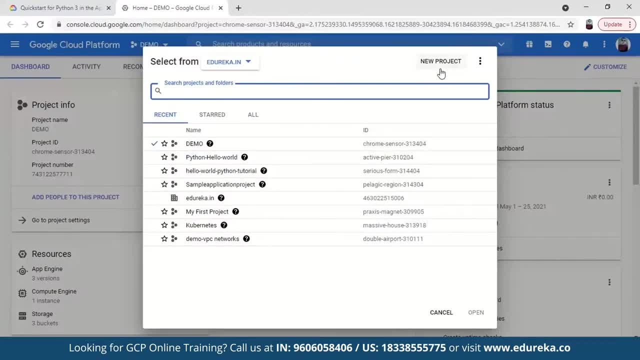 project. these are the same number of project. these are the same number of projects. i've been here, but you can also projects. i've been here, but you can also projects. i've been here, but you can also go to go to go to new project and create. okay, so let's go. new project and create. okay, so let's go. new project and create. okay, so let's go to here, to here, to here. second step is remember when you are. second step is remember when you are. second step is remember when you are creating the project, creating the project. 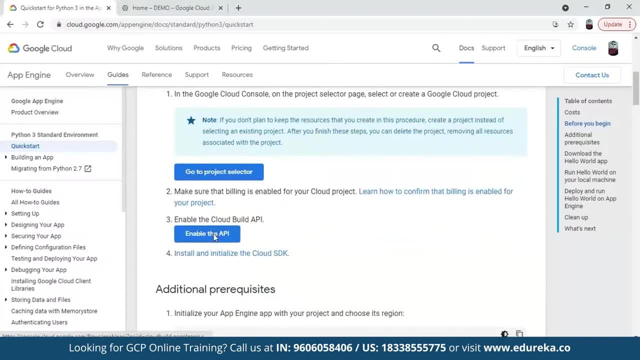 creating the project. ensure that billing is enabled for that. ensure that billing is enabled for that. ensure that billing is enabled for that. okay, okay, okay. then. third step is just open it from here. then third step is just open it from here. then third step is: just open it from here. enable the api. 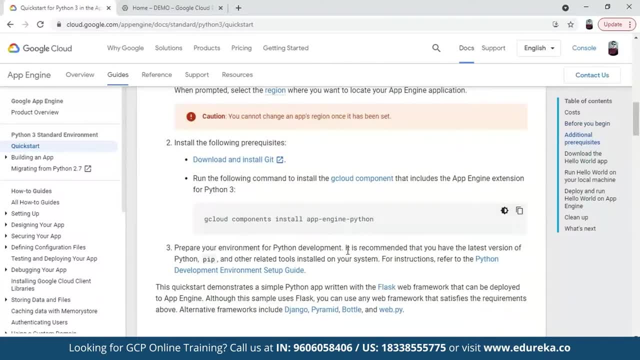 enable the api, enable the api, open this and just enable the api. then we open this and just enable the api. then we open this and just enable the api. then we just remember the next step additional, just remember the next step additional, just remember the next step: additional prerequisites. 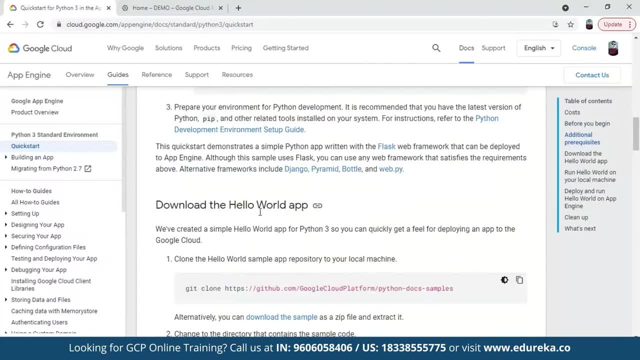 prerequisites: prerequisites: it's not required, okay, so yes, it's not required. okay, so, yes, it's not required, okay, so yes, then you go to the hello world app, then you go to the hello world app, then you go to the hello world app. so what we have to do is we just have. 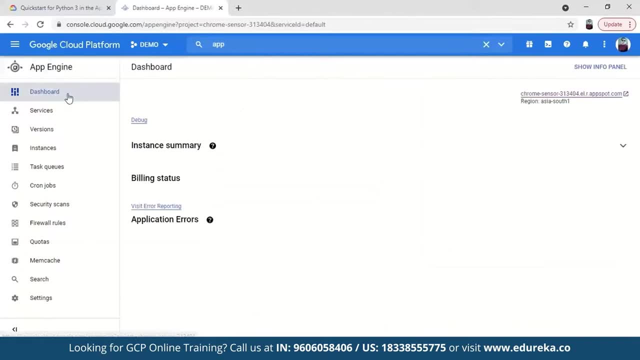 so what we have to do is we just have. so what we have to do is we just have to go to the app engine here, to go to the app engine here, to go to the app engine here. remember i explained you on the. remember, i explained you on the. 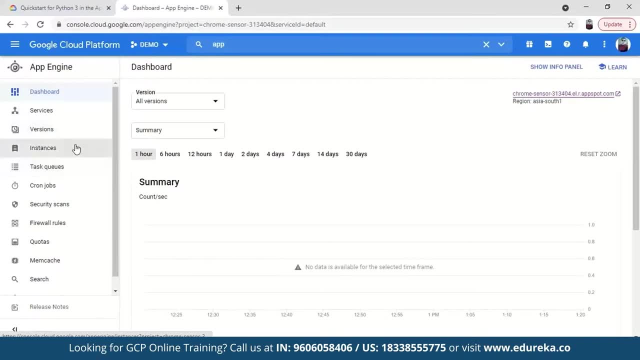 remember, i explained you on the application components. application components, application components inside which we have services versions, inside which we have services versions, inside which we have services versions and instances and instances, and instances. this is the same thing when you create. this is the same thing when you create. 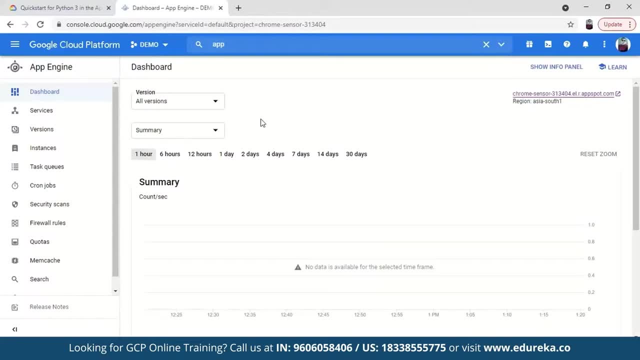 this is the same thing: when you create an app, the services will be provided, and an app, the services will be provided, and an app, the services will be provided and the versions will be created, and also the versions will be created, and also the versions will be created, and also the instances will be created for that. 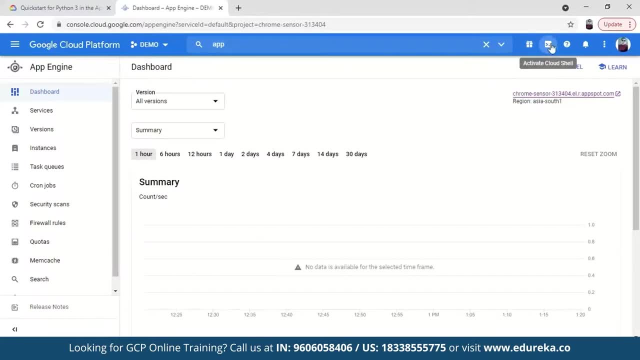 the instances will be created for that. the instances will be created for that. so what we have to do is just open the. so what we have to do is just open the. so what we have to do is just open the cloud shell from here: activate cloud cloud shell from here: activate cloud. 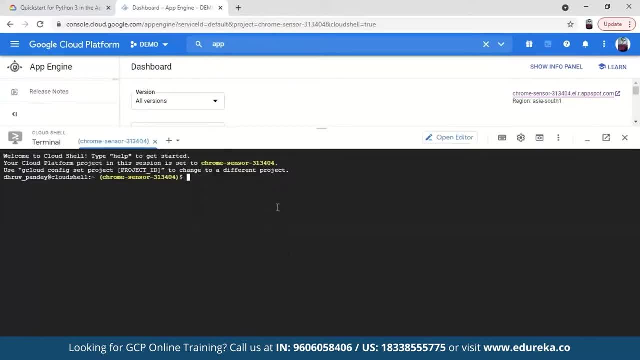 cloud shell from here. activate cloud shell. so what we have to do is go to the. so what we have to do is go to the. so what we have to do is go to the documents part. remember this documents part. remember this documents part. remember this. these steps are here. download the hello. 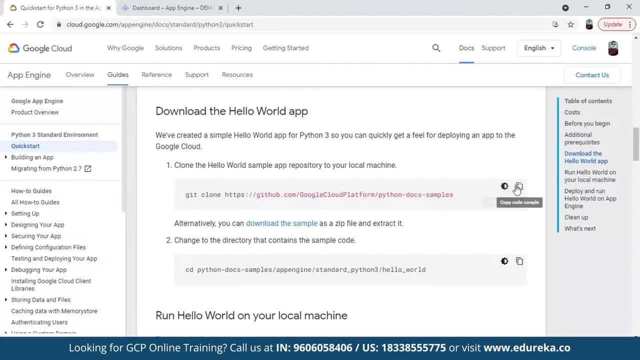 these steps are here. download the hello. these steps are here. download the hello. world- yeah, how we have to implement it. world- yeah, how we have to implement it. world- yeah, how we have to implement it. you have to copy this. you have to clone a. you have to copy this. you have to clone a. 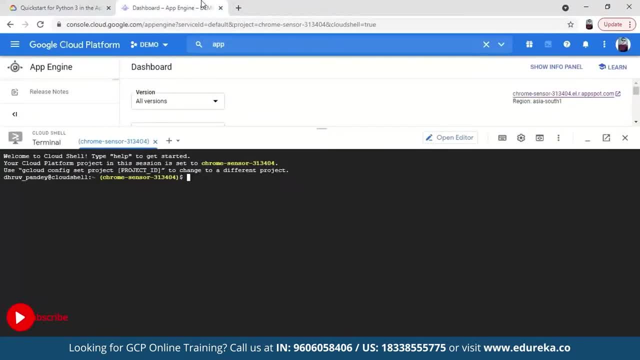 you have to copy this. you have to clone a github depository. okay, inside which the github depository? okay, inside which the github depository. okay, inside which the hello world program is already present. hello world program is already present. hello world program is already present. so, yeah, just have to clone it. so just 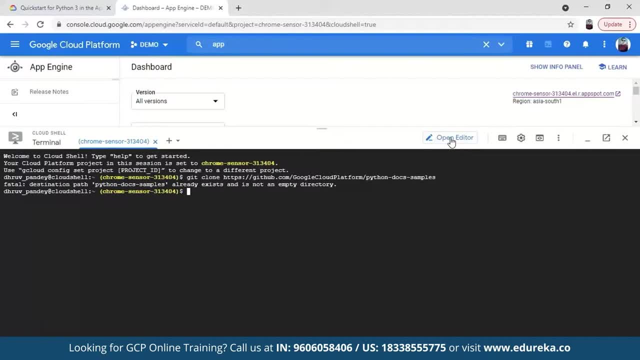 so yeah, just have to clone it. so just so, yeah, just have to clone it. so just paste it here, paste it here, paste it here. just enter, then we can go to the editor. just enter, then we can go to the editor. just enter, then we can go to the editor here. 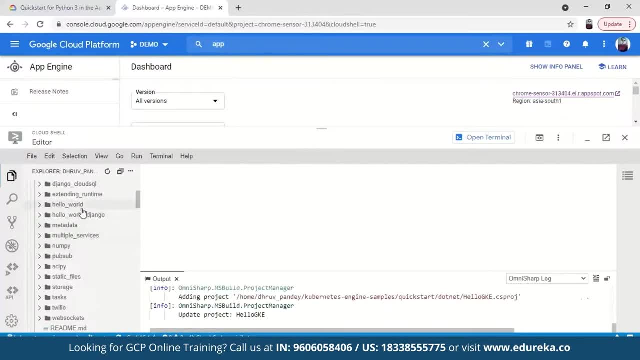 then the hello world program? where is uh then the hello world program? where is uh then the hello world program? where is uh? yeah, hello, yeah, yeah, yeah, in hello world we have uh mainpy in hello world. we have uh mainpy in hello world we have uh mainpy, yeah. this is the 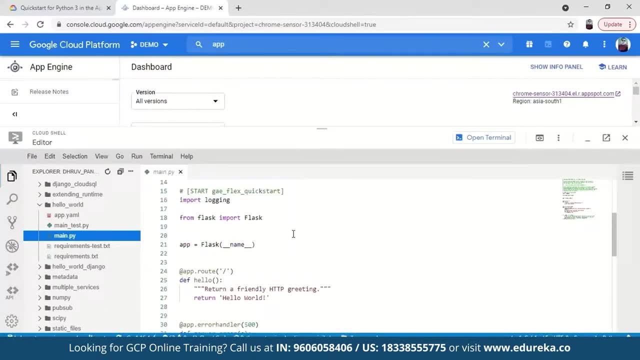 yeah, this is the. yeah, this is the python program, all the. we are going to python program all the. we are going to python program all the. we are going to use flask for it. so, using class, we are use flask for it. so, using class, we are use flask for it. so, using class, we are creating this. we don't. you don't have to. 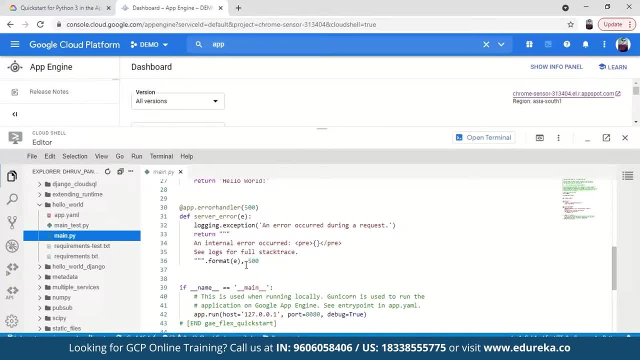 creating this. we don't. you don't have to creating this, we don't you don't have to code of it. we can just use it uh like code of it. we can just use it uh like code of it. we can just use it uh like this. only, it's just a simple demo. 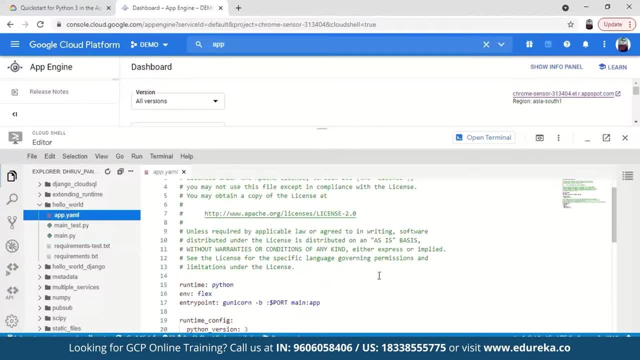 this only, it's just a simple demo. this only it's just a simple demo. and then we have a appyml file with and then we have a appyml file with: and then we have a appyml file with. all the specifics are being given here. all the specifics are being given here. 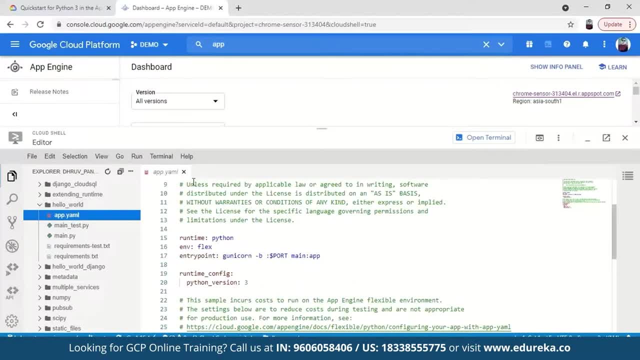 all the specifics are being given here. so what you can do is you have. so what you can do is you have. so what you can do is you have understood the path here, okay. understood the path here, okay. understood the path here, okay. so we can just go back to the terminal. 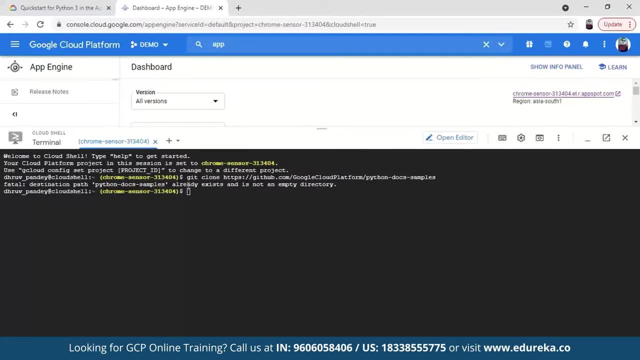 so we can just go back to the terminal. so we can just go back to the terminal, the repository. we have already cloned the repository. we have already cloned the repository, we have already cloned. what you can see here is that the. what you can see here is that the 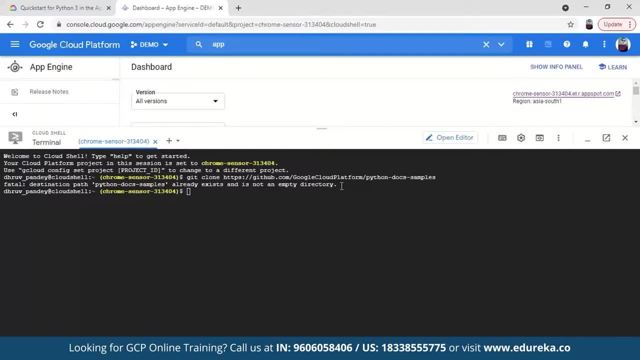 what you can see here is that the repository is already cloned. repository is already cloned. repository is already cloned, but the thing is when you're doing when. but the thing is when you're doing when, but the thing is when you're doing when you're going to do it for the first time. you're going to do it for the first time. you're going to do it for the first time. the directory won't be existing, so it, the directory won't be existing, so it, the directory won't be existing, so it will clone and it will take a little. 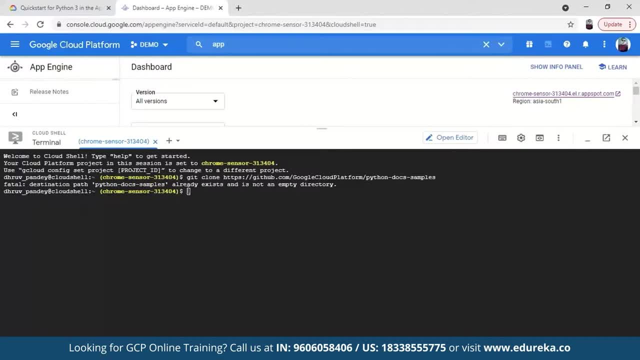 will clone and it will take a little will clone and it will take a little time, so it will get cloned. okay time, so it will get cloned. okay time, so it will get cloned. okay, mine is already showing that it already. mine is already showing that it already. 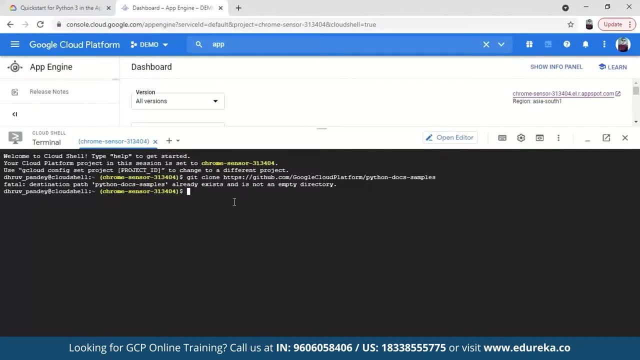 mine is already showing that it already exists, because i have already tried exists, because i have already tried exists, because i have already tried the demo here. okay, so yeah. so what we can the demo here? okay, so yeah. so what we can the demo here? okay, so yeah. so what we can do is, uh, we can go to. 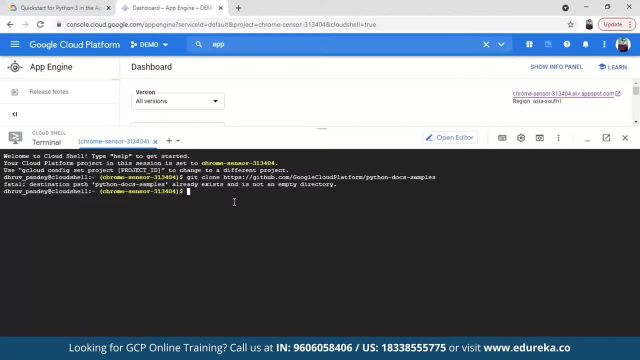 do is: uh, we can go to do is. uh, we can go to. we can type here, for we have to input the. we can type here, for we have to input the. we can type here, for we have to input the path. right, so for inputting the path, we. 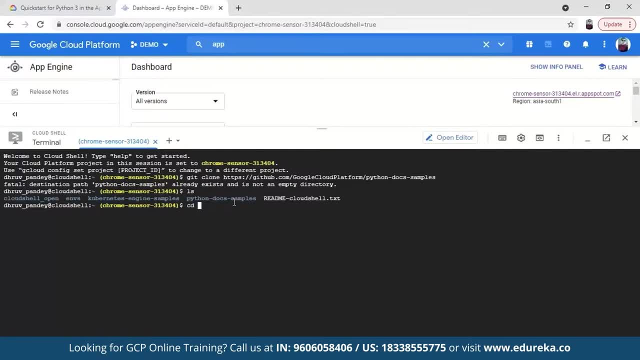 path right. so for inputting the path, we path right. so for inputting the path we can just type. can just type. can just type: ls then cd. what was the location? python ls then cd. what was the location? python ls then cd. what was the location python docs. 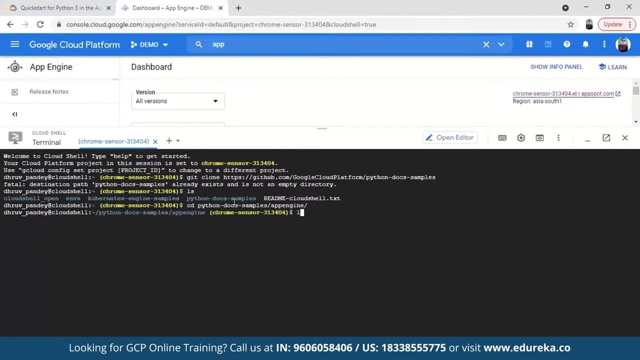 app engine, app engine, app engine. the further path will be given by again. the further path will be given by again. the further path will be given by again: ls cd- flexible hello world. ls cd- flexible hello world. ls cd- flexible hello world. then we just have to deploy the app. so 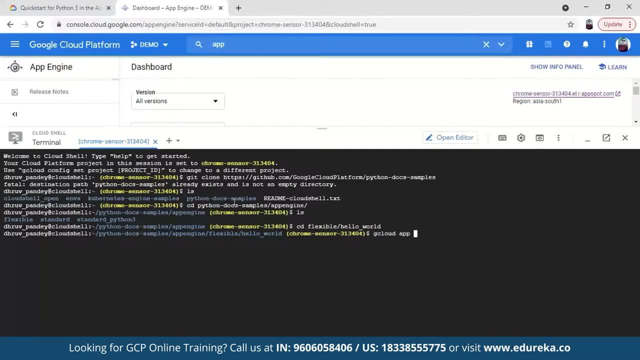 then we just have to deploy the app. so then we just have to deploy the app. so just give the command g cloud, just give the command g cloud, just give the command g cloud, app deploy, app deploy, app deploy, just authorize it, just authorize it, just authorize it. what have? so what happened here is it's. what have so? what happened here is: it's what have so. what happened here is it's asking for me to continue. but if you are asking for me to continue, but if you are asking for me to continue, but if you are going to do it for the first time, it. 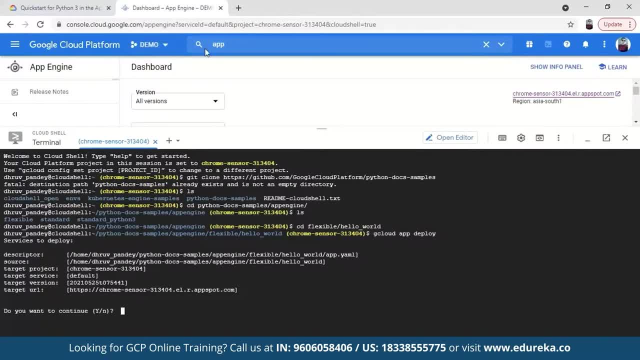 going to do it for the first time. it going to do it for the first time. it will ask you to select your project. like will ask you to select your project. like will ask you to select your project like. my project name is demo with the billing. my project name is demo with the billing. 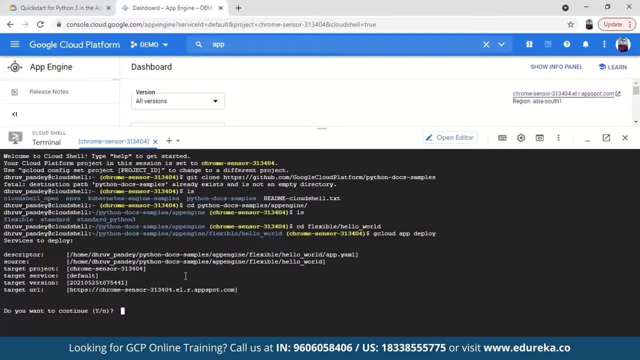 my project name is demo with the billing enabled. so remember that you have to enabled. so remember that you have to enabled. so remember that you have to. there will be a certain list of projects. there will be a certain list of projects. there will be a certain list of projects, so you have to select one project. 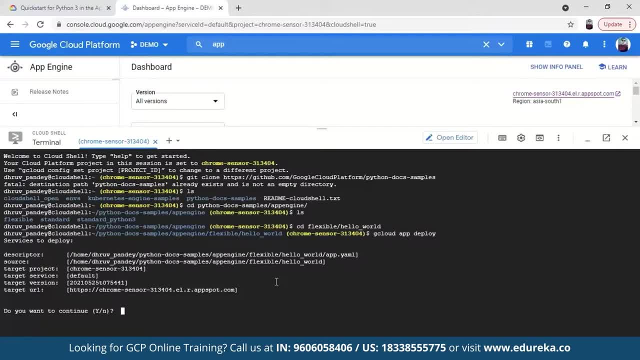 so you have to select one project. so you have to select one project, and then there will be another option of, and then there will be another option of, and then there will be another option of. you like, press enter after that by. you like, press enter after that by. 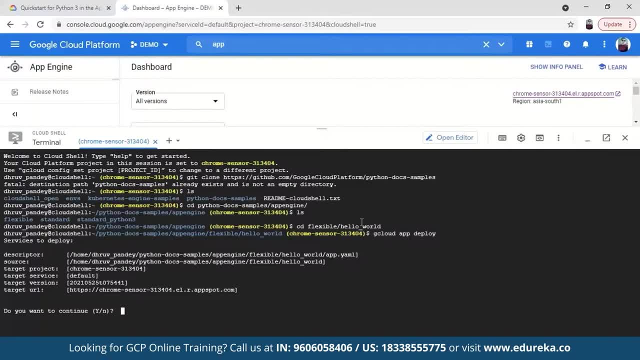 you like, press enter. after that, by selecting the project. it will ask for the selecting the project. it will ask for the selecting the project. it will ask for the region. so you have to select a region. region, so you have to select a region. region, so you have to select a region. okay, like, my region is a asia south, so okay, like my region is a asia south. so okay, like my region is a asia south. so you have to select your region, and then you have to select your region, and then you have to select your region and then it will ask for you to continue. so you 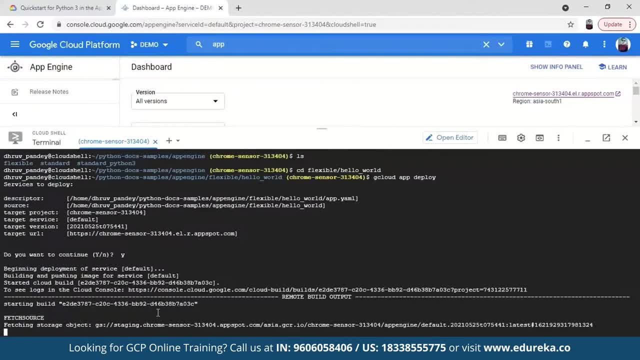 it will ask for you to continue, so you, it will ask for you to continue, so you just have to type the, just have to type the, just have to type the wire here. it doesn't usually take this long, but it doesn't usually take this long, but 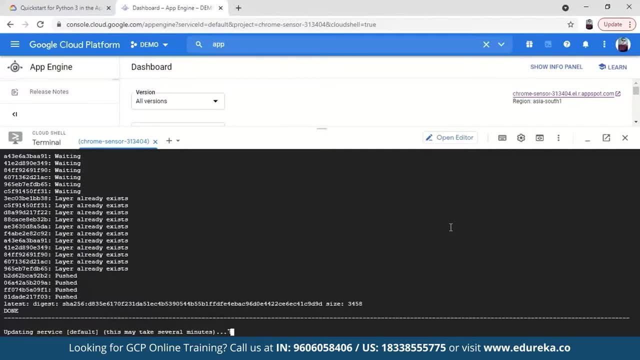 it doesn't usually take this long, but today there's a little server problem. today there's a little server problem. today there's a little server problem. that's why it's taking this long. that's why it's taking this long. that's why it's taking this long. i hope you have understood till now the. 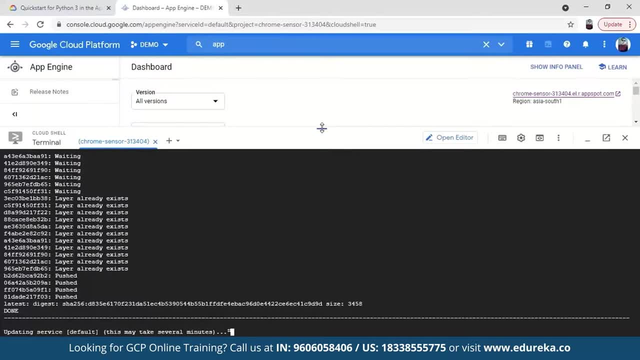 i hope you have understood till now the. i hope you have understood till now the like the theoretical part also, and also like the theoretical part also, and also like the theoretical part also. and also the the the like this implementation also till now. like this implementation also till now. 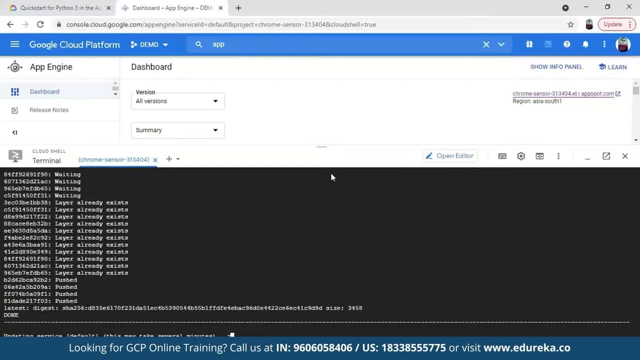 like this implementation also till now. remember those codes which i have told. remember those codes which i have told. remember those codes which i have told you: right for the path one and also for you. right for the path one and also for you, right for the path one and also for the cloning one. cloning one will be given. 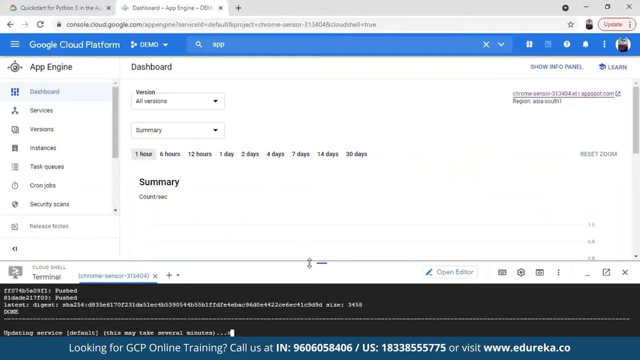 the cloning one. cloning one will be given the cloning one. cloning one will be given for the path, when you have to remember, for the path, when you have to remember, for the path, when you have to remember that okay, that okay, that okay, so you can see here. uh, like services and 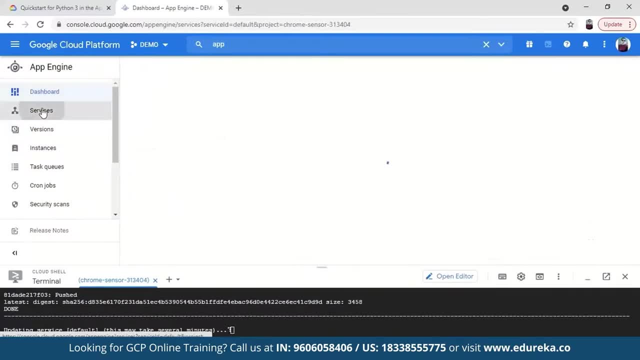 so you can see here: uh like services. and so you can see here, uh like services, and versions and instances are given, when versions and instances are given, when versions and instances are given, when you create this project a service, will you create this project a service? will you create this project? a service will be created. 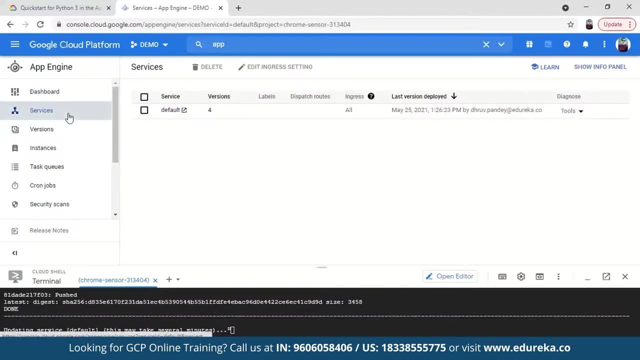 be created, be created and yeah, this is a single service is and yeah, this is a single service is and, yeah, this is a single service is being created and said that the versions being created, and said that the versions being created, and said that the versions will be created. so i have created a new. 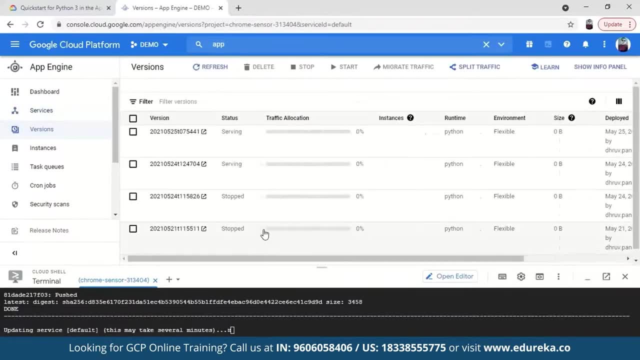 will be created, so i have created a new will be created, so i have created a new version. in that, like this one through version, in that, like this one through version, in that, like this one through cloud shell, i have created a new version. cloud shell, i have created a new version. 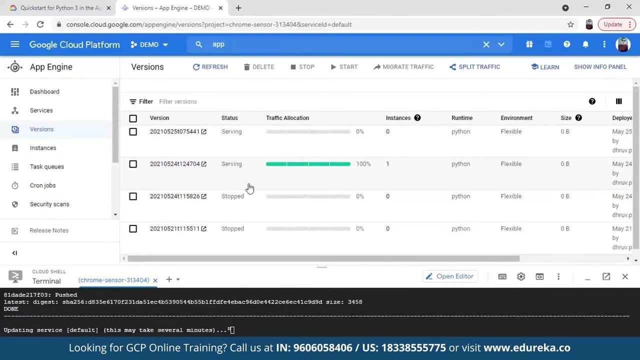 cloud shell. i have created a new version. this one. it is just serving right. this one. it is just serving right. this one, it is just serving right. now. right needs to have stopped this. i now right needs to have stopped this. i now right needs to have stopped this. i have already. 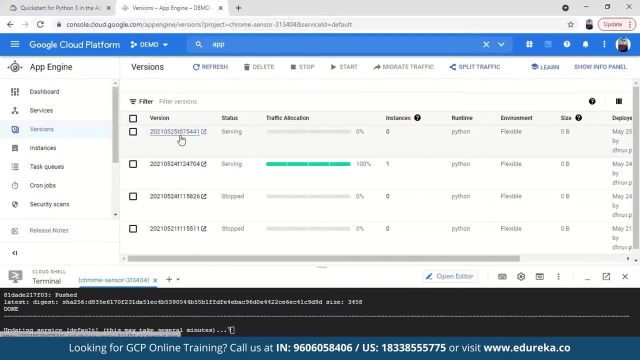 have already, have already run ran before. this one is ours, run ran before this one is ours, run ran before this one is ours. two zero two one. this five four four. two zero two one. this five four four two zero two one. this five four four one. this is the version we have created. one. this is the version we have created one. this is the version we have created. okay, so in instance, this is not showing. okay, so, in instance, this is not showing. okay, so in instance, this is not showing right now, but this shows when you just right now, but this shows when you just. 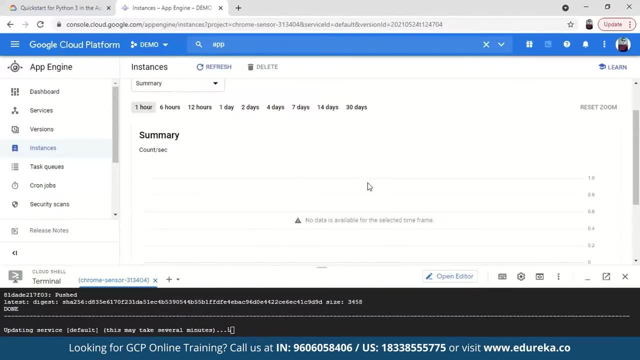 right now, but this shows when you just get implemented now, when in this app get implemented now, when in this app get implemented now, when in this app starts running, it shows all the starts running. it shows all the starts running. it shows all the information regarding that. information regarding that. 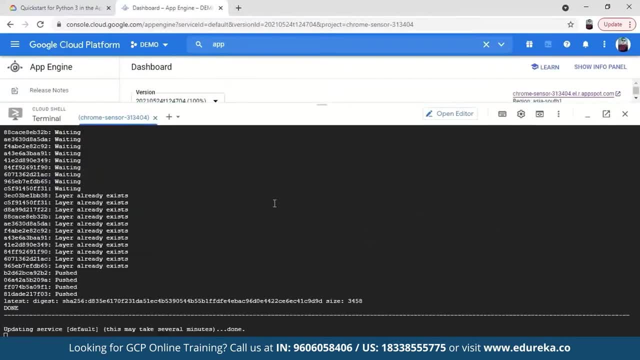 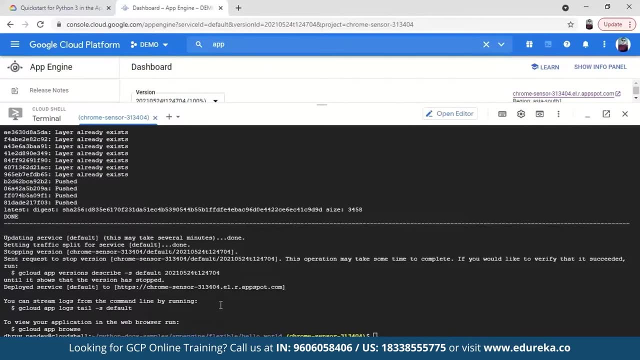 information regarding that. okay, so yeah, okay so yeah, okay so yeah, so yeah, the service is updated. yeah, it's so. yeah, the service is updated. yeah, it's so yeah, the service is updated. yeah, it's almost done now, almost done now, almost done now. yeah, so what you can do is: yeah, here is. 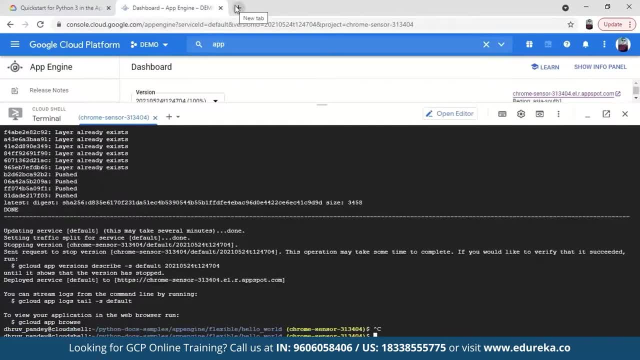 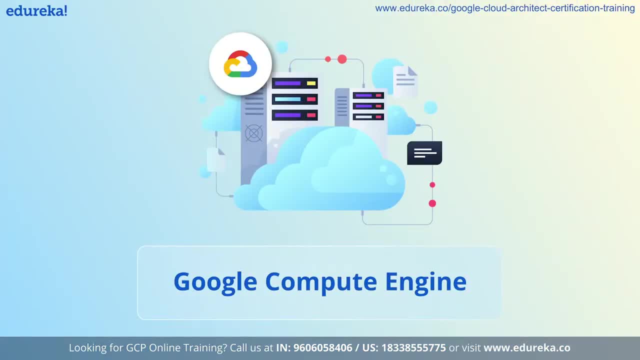 yeah. so what you can do is: yeah, here is yeah. so what you can do is: yeah, here is the link. you can just the link. you can just the link. you can just copy the link. copy the link. copy the link. go to the go to the. go to the. yes, we got it, hello. 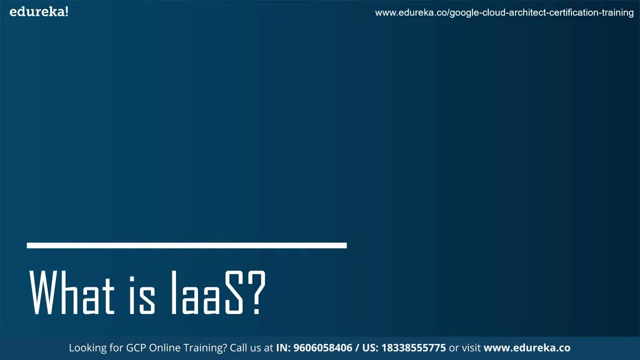 yes, we got it, hello. yes, we got it, hello. so now, let's first. so now, let's first. so now let's first understand what infrastructure is a, understand what infrastructure is a, understand what infrastructure is a service that is iaas is, service that is iaas is. 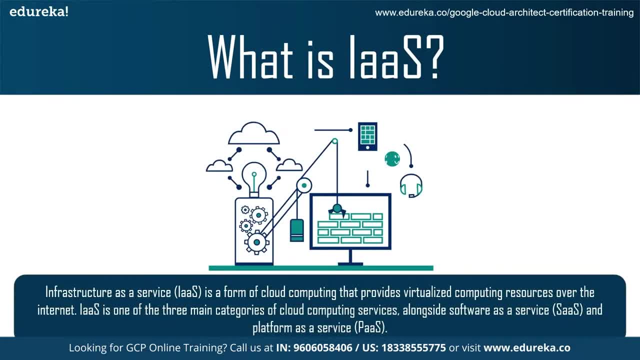 service that is iaas is so infrastructure as a service are so infrastructure as a service are so infrastructure as a service are online services that provide high level online services that provide high level online services that provide high level apis, which are used to deliver various apis, which are used to deliver various. 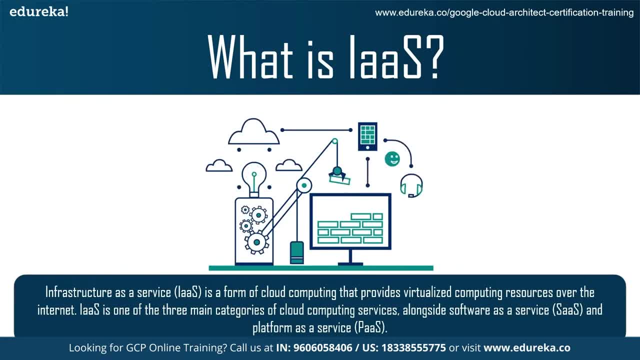 apis, which are used to deliver various low-level details of underlying network. low-level details of underlying network. low-level details of underlying network infrastructure, like physical computing infrastructure, like physical computing infrastructure, like physical computing resources, location data partitioning resources, location data partitioning resources, location data partitioning, scaling, security, backup, etc. a. 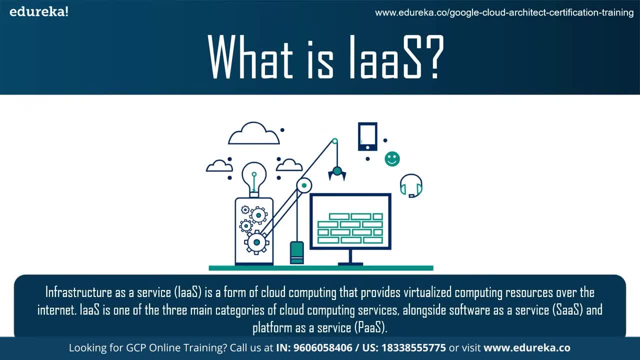 scaling, security, backup, etc. a scaling, security, backup, etc. a hypervisor which is nothing but a hypervisor which is nothing but a hypervisor which is nothing but a physical host, such as zen oracle virtual physical host, such as zen oracle virtual physical host, such as zen oracle virtual box, oracle, vm, kvm or vmware runs the. 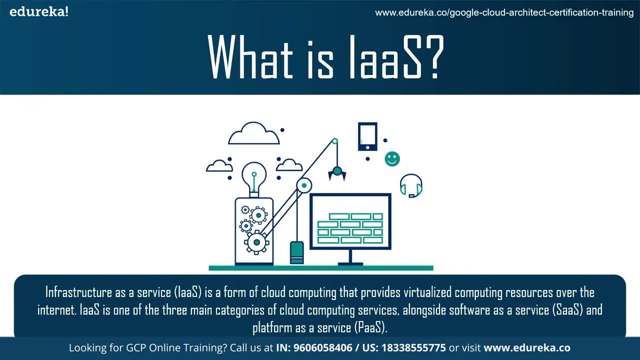 box. oracle vm, kvm or vmware runs the box. oracle vm, kvm or vmware runs the virtual machines as guests. so pools of virtual machines as guests. so pools of virtual machines as guests. so pools of hypervisors within the cloud. hypervisors within the cloud. 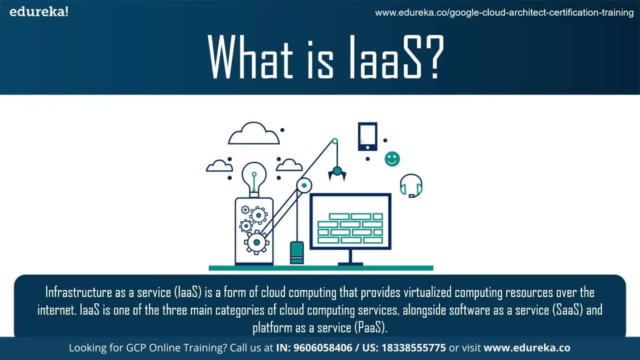 hypervisors within the cloud operational system. can support large operational system. can support large operational system. can support large number of virtual machines and the number of virtual machines and the number of virtual machines and the ability to scale services up and down. ability to scale services up and down. 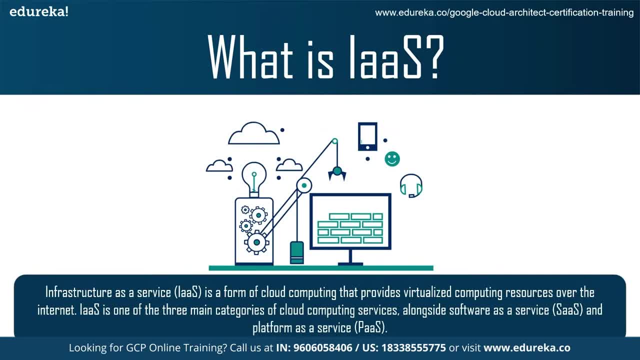 ability to scale services up and down according to customers reading. according to customers reading. according to customers reading requirements. typically, iaas involves the requirements. typically, iaas involves the requirements. typically, iaas involves the use of cloud orchestration technology. use of cloud orchestration technology. use of cloud orchestration technology like open stack, apache, cloud stack or 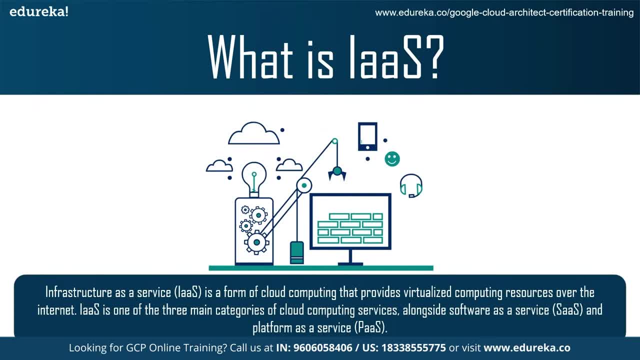 like open stack, apache cloud stack, or like open stack, apache cloud stack or open nebula. this manages the creation of open nebula. this manages the creation of open nebula. this manages the creation of a virtual machine and decides on which a virtual machine and decides on which. 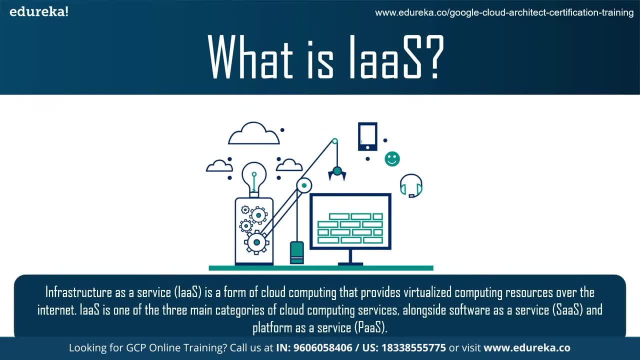 a virtual machine and decides on which hypervisor to start it. which enables hypervisor to start it. which enables hypervisor to start it. which enables virtual machine migration features. virtual machine migration features. virtual machine migration features between hosts also. it allocates storage between hosts also. it allocates storage. 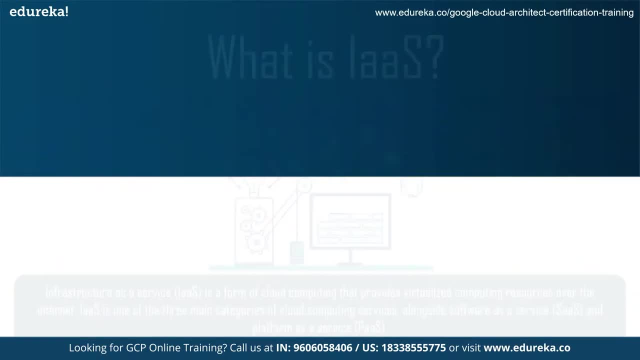 between hosts. also, it allocates storage volumes and attaches them to virtual volumes and attaches them to virtual volumes and attaches them to virtual machines and correct usage information machines and correct usage information machines and correct usage information for billing and more now let's get an for billing and more. now let's get an. 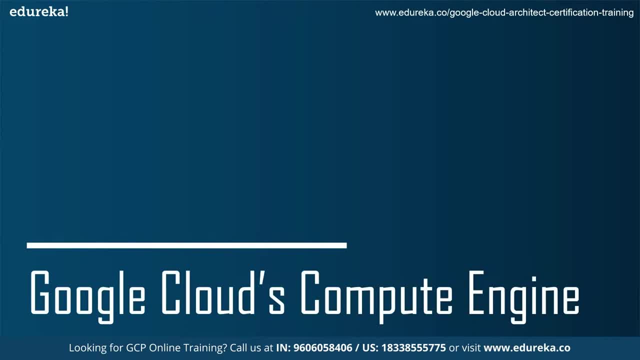 for billing and more. now let's get an overview of google cloud's compute engine. overview of google cloud's compute engine. overview of google cloud's compute engine. so google's compute engine is google's. so google's compute engine is google's. so google's compute engine is google's infrastructure as a service, virtual. 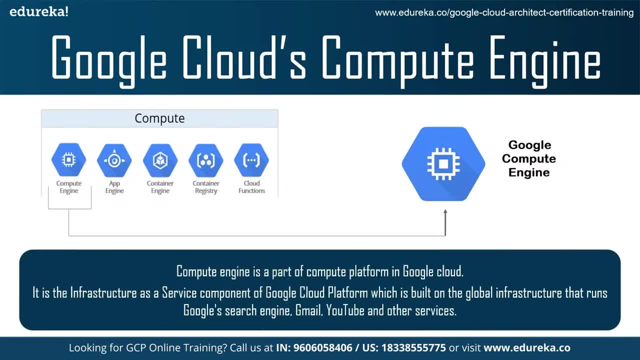 infrastructure as a service. virtual infrastructure as a service- virtual machine offering. it allows customers to machine offering. it allows customers to machine offering. it allows customers to use virtual machines in the cloud as use virtual machines in the cloud as use virtual machines in the cloud as server resources instead of acquiring and. 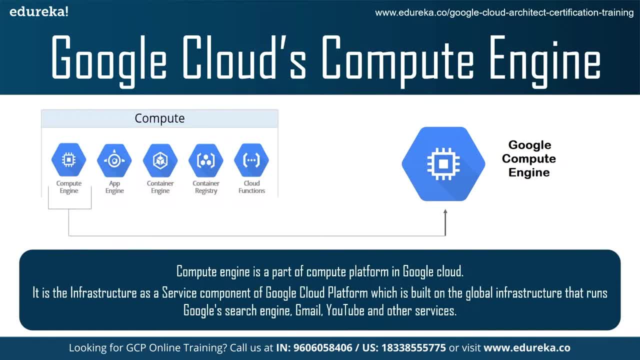 server resources instead of acquiring and server resources instead of acquiring and managing server hardware. google's managing server hardware. google's managing server hardware. google's compute engine offers virtual machines. compute engine offers virtual machines. compute engine offers virtual machines running in google's data centers- running in google's data centers. 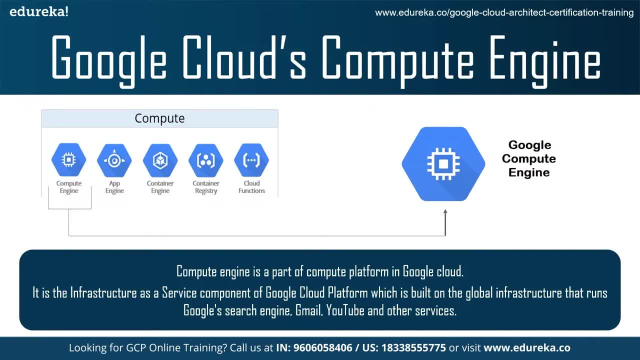 running in google's data centers connected to the worldwide fiber network. connected to the worldwide fiber network. connected to the worldwide fiber network. the tooling and workflow offered by the, the tooling and workflow offered by the. the tooling and workflow offered by the compute engine enables scaling from. 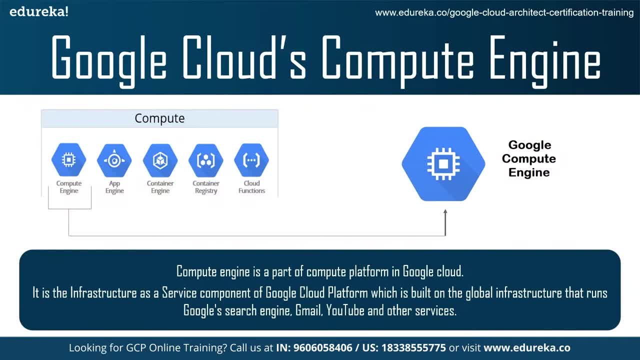 compute engine. enables scaling from compute engine. enables scaling from single instances to global google, single instances to global google, single instances to global google. compute engine enables users to launch compute engine. enables users to launch compute engine. enables users to launch virtual machines on demand- virtual virtual machines on demand- virtual. 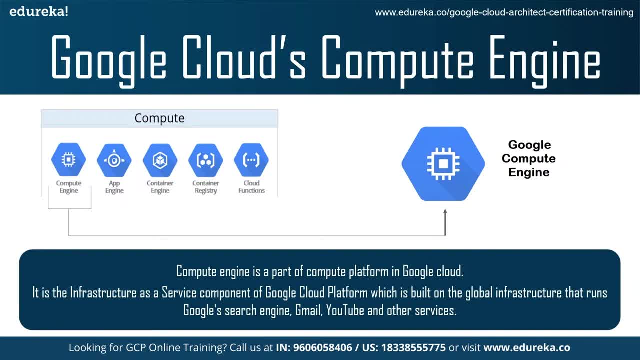 virtual machines on demand. virtual machines can be launched from the machines. can be launched from the machines. can be launched from the standard images or custom images created. standard images or custom images. created standard images or custom images created by users: the google compute engine. by users: the google compute engine. 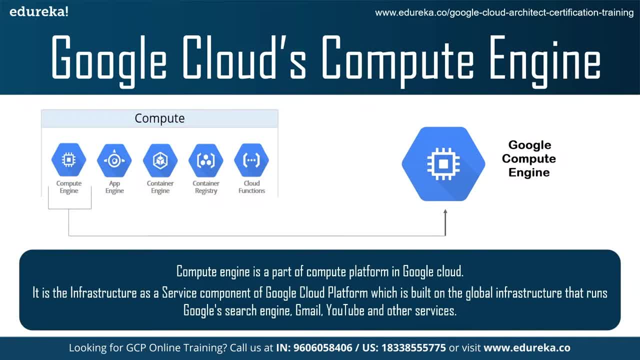 by users. the google compute engine users must authenticate based on auth 2.0. users must authenticate based on auth 2.0. users must authenticate based on auth 2.0 before launching the virtual machines, before launching the virtual machines, before launching the virtual machines. so what auth 2.0 here is? so, if you see, 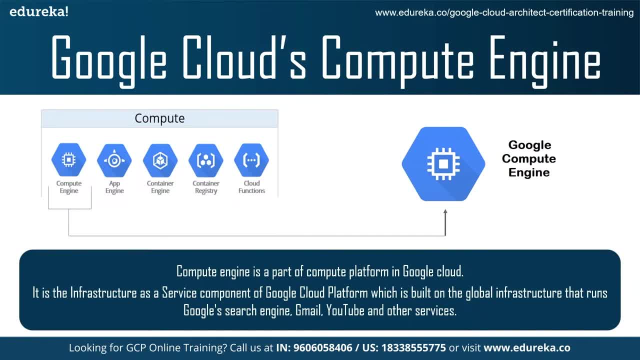 so what auth 2.0 here is? so if you see? so what auth 2.0 here is? so, if you see, auth is an open standard for access. auth is an open standard for access. auth is an open standard for access delegation, commonly used as a way for. 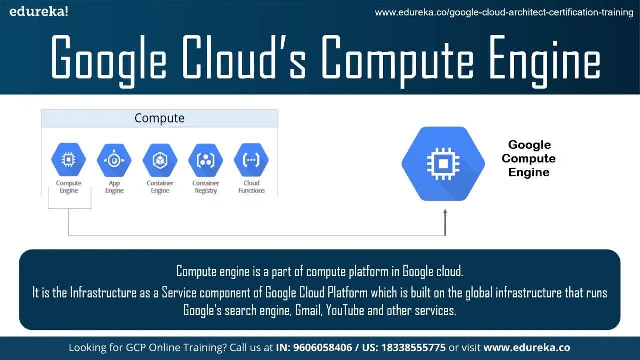 delegation. commonly used as a way for delegation. commonly used as a way for internet users to grant websites or internet users to grant websites or internet users to grant websites or applications access to their information applications, access to their information applications, access to their information on other websites, but without giving 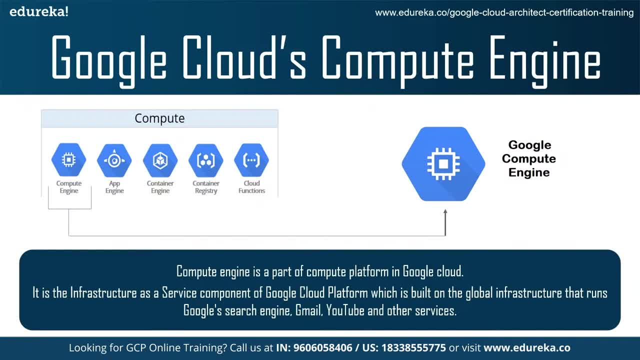 on other websites, but without giving on other websites, but without giving them the passwords. the mechanism is used, them the passwords. the mechanism is used, them the passwords. the mechanism is used by companies such as amazon google, by companies such as amazon google, by companies such as amazon google, facebook, microsoft, twitter, to permit. 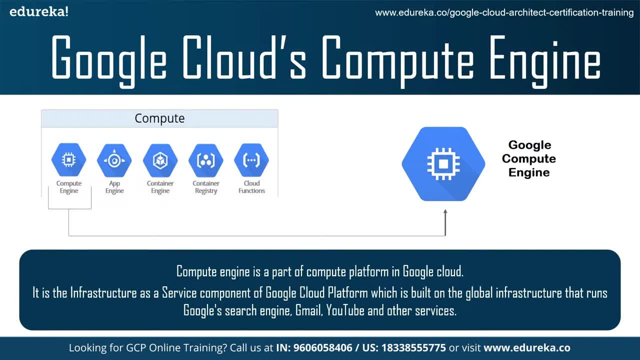 facebook- microsoft twitter. to permit facebook- microsoft twitter. to permit users to share information about their users. to share information about their users, to share information about their accounts with third-party applications. accounts with third-party applications. accounts with third-party applications. of websites now going back to google. of websites now going back to google. 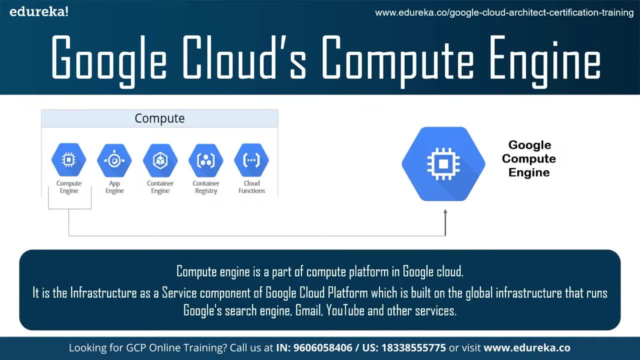 of websites. now, going back to google compute engine, which can be accessed. compute engine which can be accessed. compute engine which can be accessed via the developer console or sful api, or via the developer console or sful api, or via the developer console or sful api or command line interface. 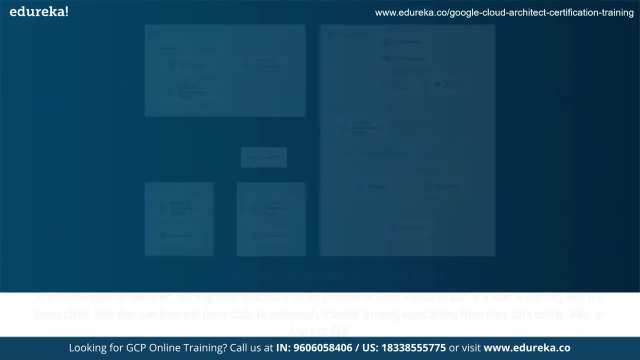 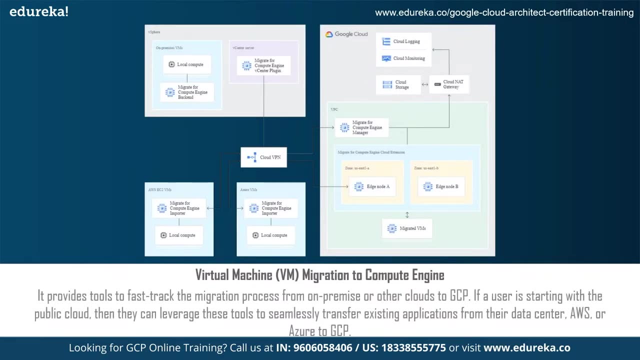 command line interface. command line interface. now, let's have a look at some of its now. let's have a look at some of its now. let's have a look at some of its user like: is it starting with the public? user like: is it starting with the public? 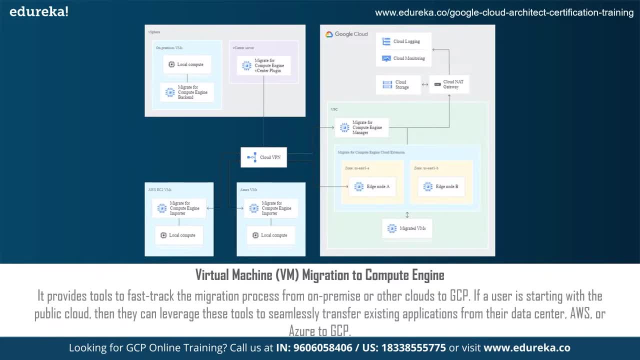 user like: is it starting with the public cloud? then they can leverage these tools cloud. then they can leverage these tools cloud. then they can leverage these tools to seamlessly transfer existing. to seamlessly transfer existing. to seamlessly transfer existing applications from their data center or applications from their data center. or. 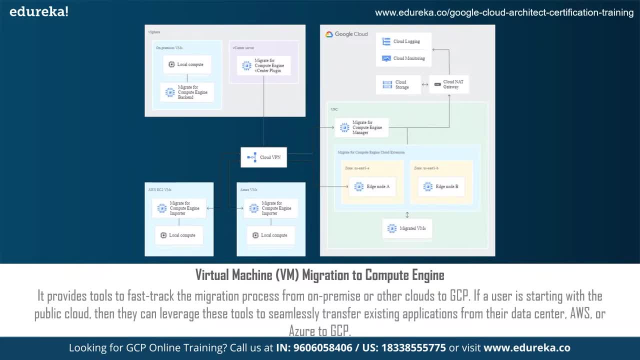 applications from their data center or aws or echo to google cloud platform. aws or echo to google cloud platform, aws or echo to google cloud platform. users can then have their applications. users can then have their applications. users can then have their applications running on compute engine within minutes. 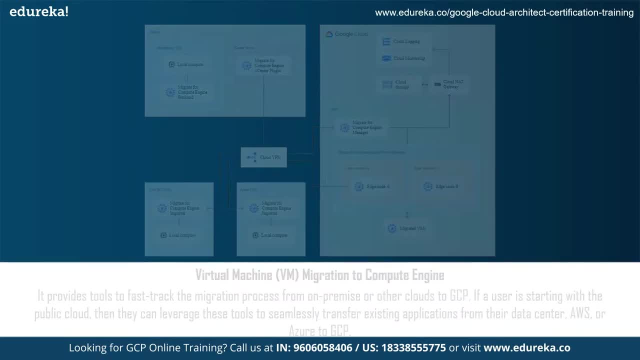 running on compute engine within minutes. running on compute engine within minutes. while the data migrates transparently in. while the data migrates transparently in, while the data migrates transparently in the background. that's how virtual the background. that's how virtual machine migration works. then we have genomics data processing, as you can see in the chart. that how it. 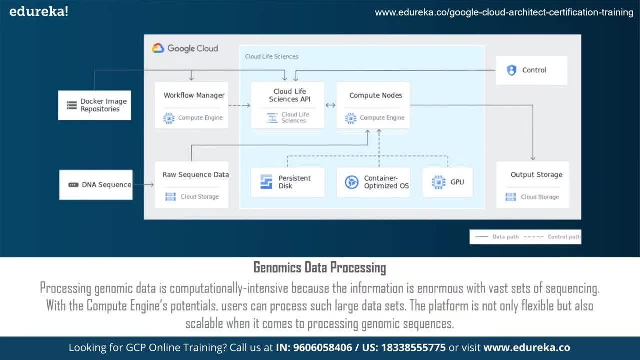 works. so processing genomic data is like computationally intensive process, because the information is enormous, with the vast sets of sequencing, so with the compute engines, potentials, users can process such large data sets. so what it do is it processes petabytes of dynamic data in seconds with compute engine and high performance computing solution, so google cloud's. 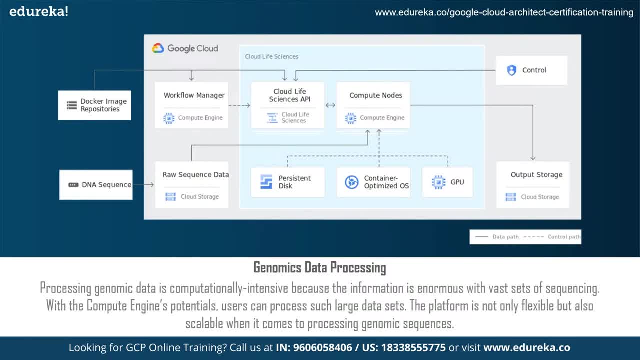 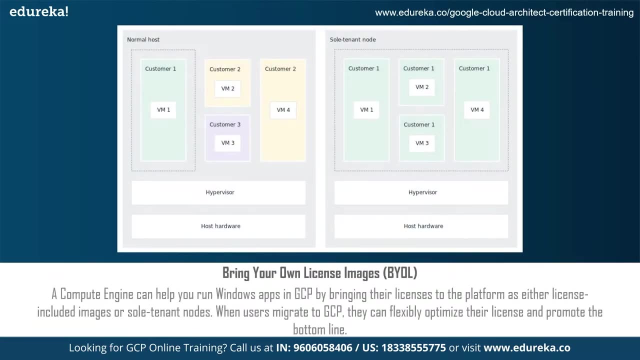 engines. scalable and flexible infrastructure enables research to continue without disruptions. okay, also like it's like: competitive pricing and discounts help you stay within the budget to convert ideas into discoveries or hypothesis into kiosks, and also like inspirations into products. then we have byol, also known as bring your own license images. so in this, how the normal. 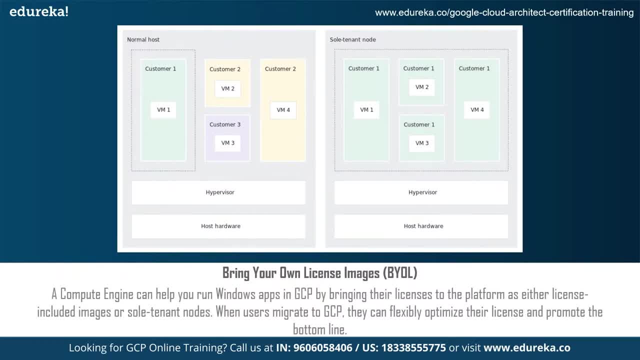 host and then we have a soltenet node. you can see how this chart is given for its working. so what it do is a compute engine can like help you run windows apps and google cloud platform by bringing their licenses to the platform as either licensing through the images or soldering. 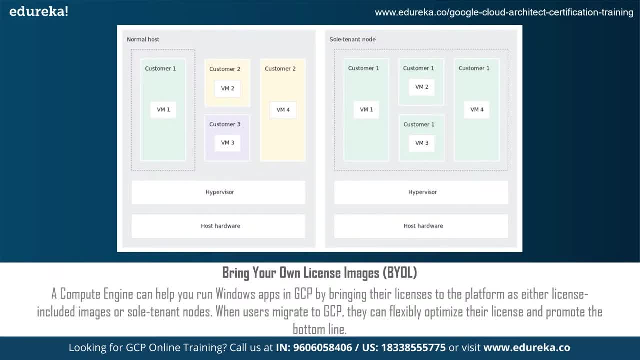 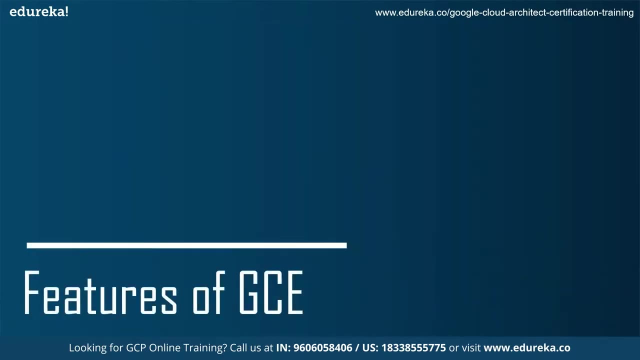 images as shown. so, after you migrate to google cloud, optimize or modernize your license usage to achieve your business goals. take advantage of the many benefits available to virtual machine instances, such as reliable storage options, the speed of the google network and also like auto scaling. now let's look at some of the key features of google computation. the first is machine types. 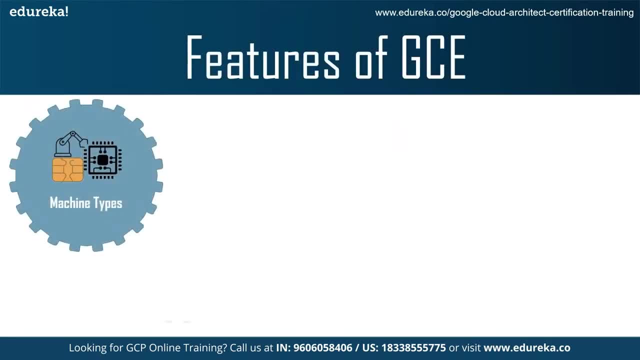 it describes the virtual hardware that is attached to an instance, which also includes ram and cpus. there are like two types of machines. first is a predefined and second is a custom machine types. so predefined machine types are like there are pre-configured virtual machine templates that can be used to set up the virtual machines. the configurations have been. 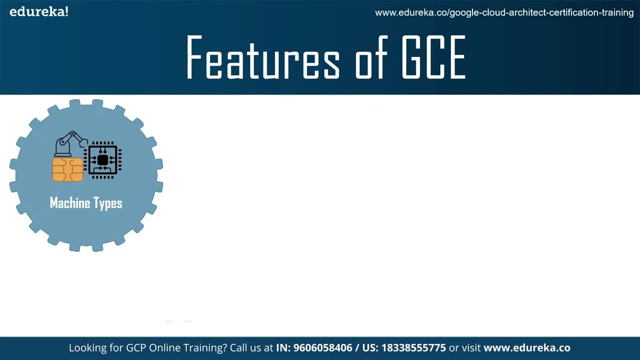 pre-optimized by google and like meet most of the requirements. so the pdf machine types are further divided into four subcategories. so they are like standard virtual machines, which are like balanced between processing power and memory, and then we have high memory virtual machines. in this like 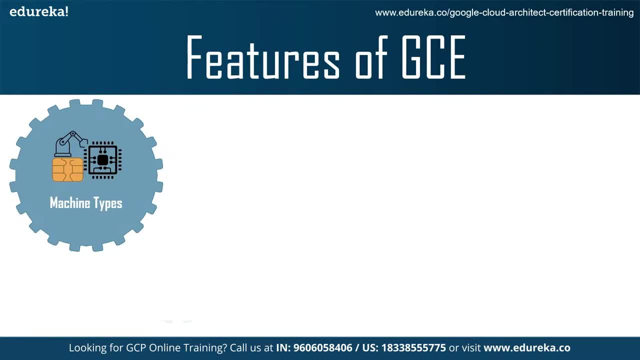 emphasis is put on memory over processing power for tasks that needed accessible non-disk storage. then we have high cpu virtual machines, so high cpu usage for like high intensity applications that require processing over memory. then the fourth subcategory, that is the shared for virtual machines. so if you see a single virtual cpu backed by a physical cpu that can run for a period of time. 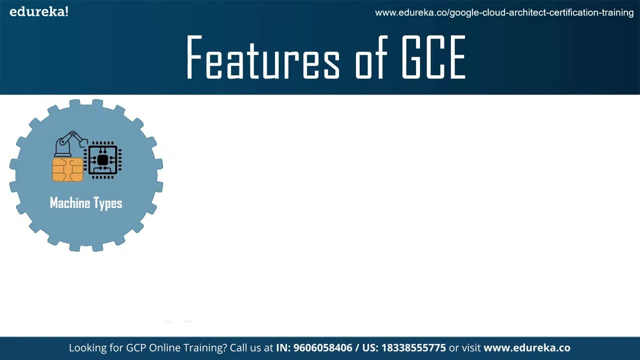 these machines are like not for use cases that require an ongoing server significant power. so the second main category under machine types is a custom machine types. in this the virtual machine can be configured manually for a compute engine virtual machine instance. so users can like select the number of cpus and memory, provided they are within google's set limit. 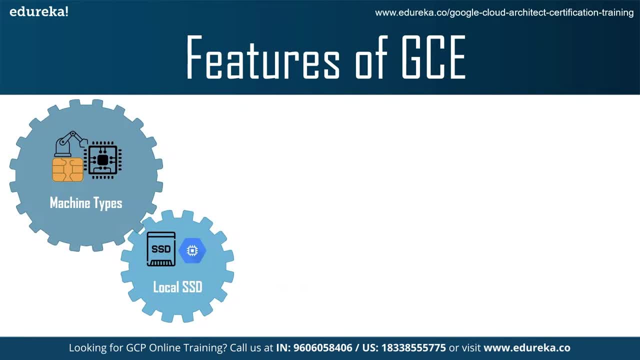 so the second one is a local ssd. so google compute engine offers always encrypted local solid state drive block storage which is physically attached to the virtual machine running it. it improves performance and also, like, reduces latency. now the third one is persistent disk. so these are durable, high performance block storage for virtual machine instances which 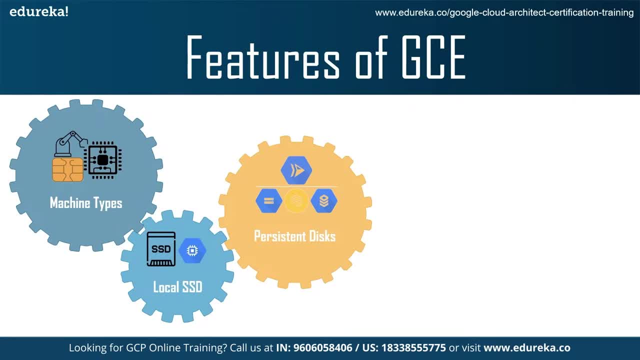 can be created in hard disk or ssd formats, so users can make snapshots and create a new persistent disk from the snapshot. if a virtual machine instance is terminated, the data is retained by the persistent disk, which can be attached to another instance. there are two types of persistent disks. first is shared, second is ssd. then we have gpu accelerator. 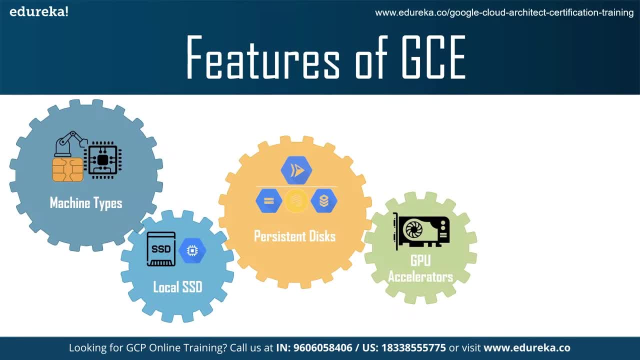 so gpus are added to accelerate computationally intensive workloads like machine learning or virtual workstation applications, etc. also the fifth one is images. so an image contains the operating system of the root file system that uses leverage to run virtual machine instance. so google cloud platform provides two main types of images. first one is public image and second is 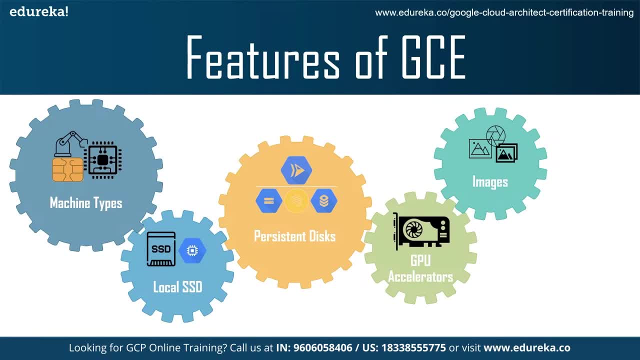 custom images. so public images are like collection of open source and proprietary options. this is the starting point for most virtual machine instances and come packaged with only the operating system. the second one is the custom images. so public images, if you see, are a good starting point, but 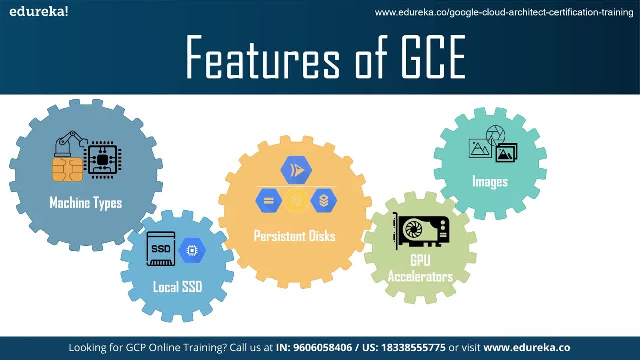 they are designed to be built upon and turned into custom images to match the needs of the customers. custom image has the software needed, along with all the scripts necessary for the user to be able to use the images to work automatically, without administrator intervention. these are automatically brought up and shut down for load balancing or recovery needs. 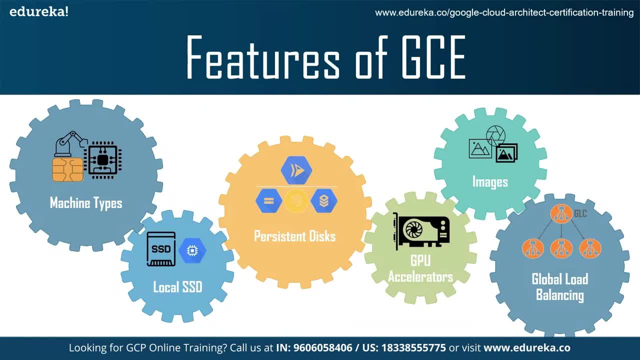 so the last one is global load balancing, so it helps in distributing incoming requests across pools of instances, across multiple regions, so that users can achieve maximum performance, throughput and availability at a cost. similarly, there are many other features like linux and windows support, container reservations, os patch management, live migration for virtual machines and many more. 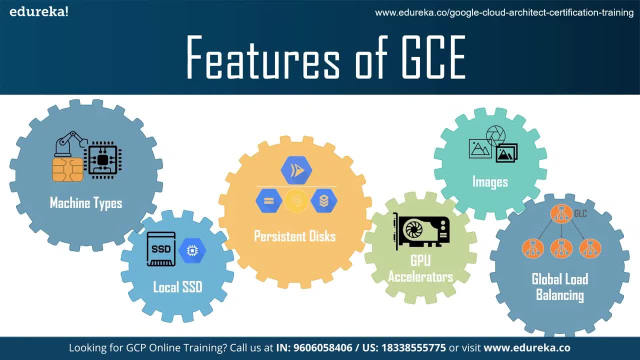 google compute engine has many pros, such as the improved fertilizer access, like smooth integration with other google services, and few cons, as, uh like, most components are based on proprietary technologies and the choice of programming languages is limited. so now that you know the applications and features of google, 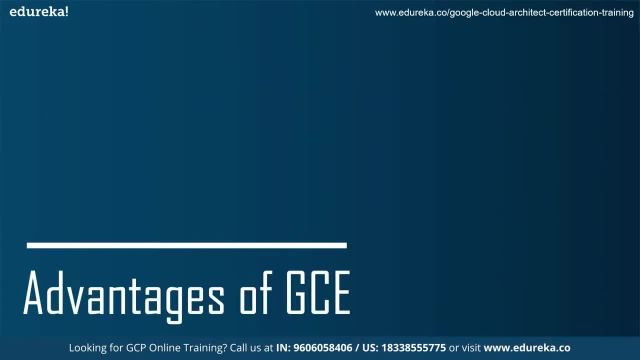 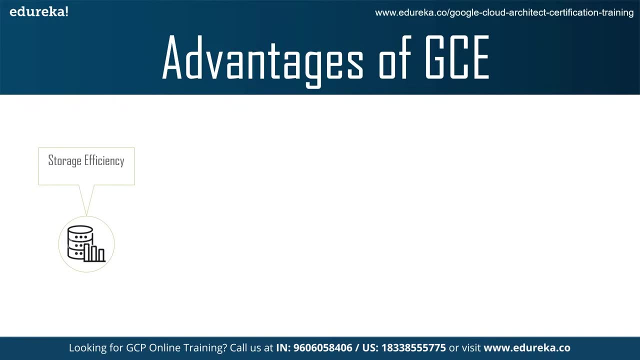 compute engine. let's now look at some major advantages of it. okay, so the first is storage efficiency. so the persistent is support up to 257 terabyte of storage, which is more than 10 times higher than what amazon elastic block storage can accommodate. organizations that require more scalable storage options can go for computing. then we have 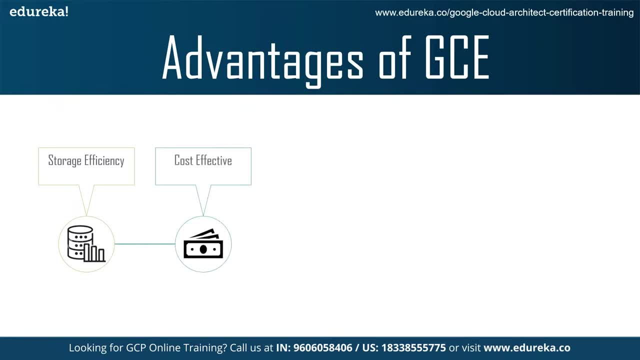 costs as it is cost effective. so within the gcp ecosystem we just pay only for the computing time that have consumed. so the first second billing plan is what used by the google computing. then we have instability. google compute engine offers stable services because of its ability to provide live migration virtual machines between the hosts. also, google cloud platform has a robust and inbuilt and redundant backup system, so the compute engine can provide high standard of load balancing in your field and in its BI system. and also we can provide a very wide diversity of alerts from another branch ecosystem as well as, for example, back-up system, so the compute engine can 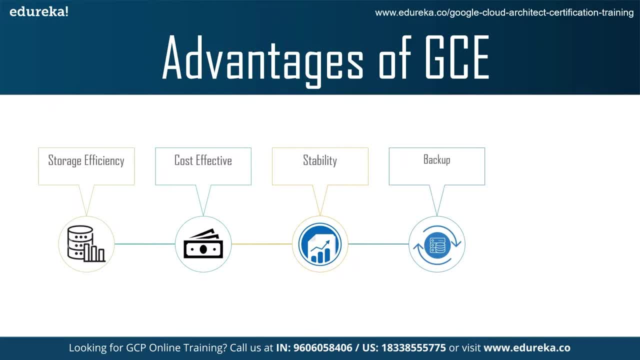 provide a lot of research and data, as well as a lot of data that can be used for the input and use for the various systems, for example. so the co-authorization of all the systems in the geocompâlter, for example, for the uses this system for flagship products like search engine and gmail. also, coming to security, 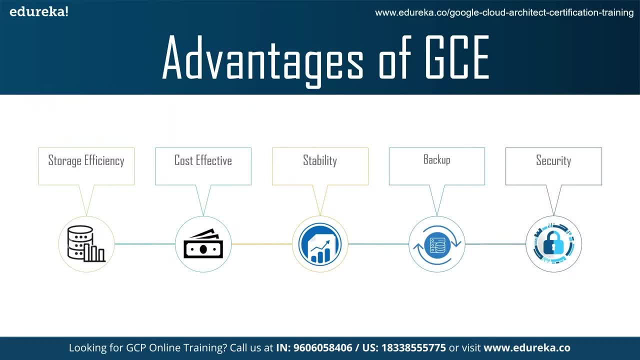 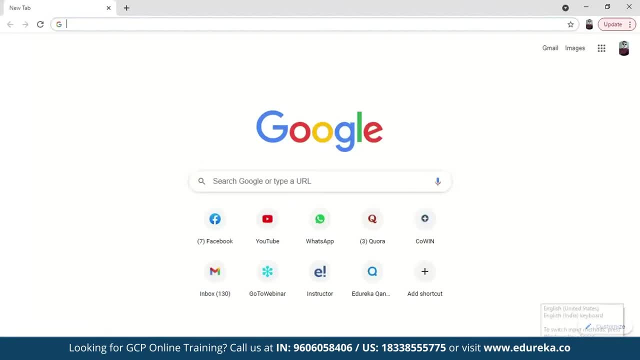 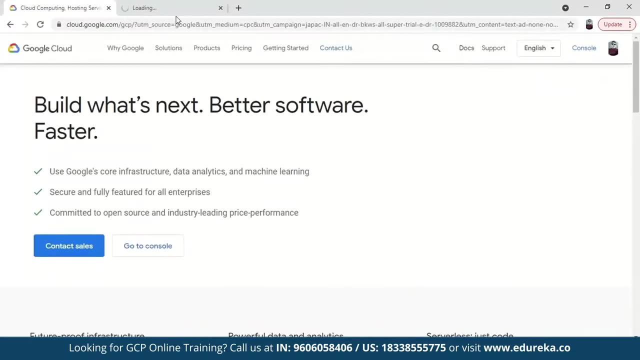 so google compute engine is the most secure and safe place for cloud applications. so now that you have a theoretical understanding of google compute engine, let's practically try our hands on it. so you can just directly go to google cloud platform. let's open it first. let's go to the documents part, so in this also you can open the console. 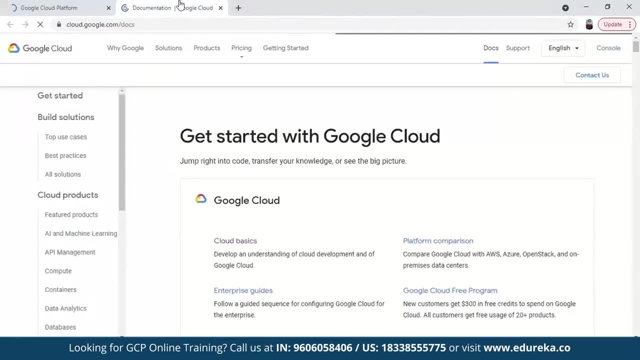 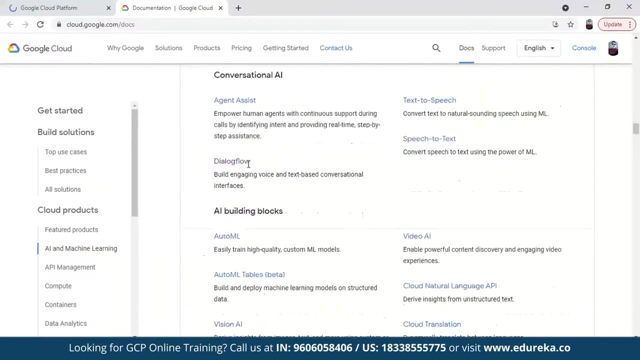 also this one. this tab only we can open. okay, so for support purpose you can just go through this documentation part, though i'm going to explain you still. if you need any in support, you can uh go to this computer part and here the compute engine is given. from here you can. 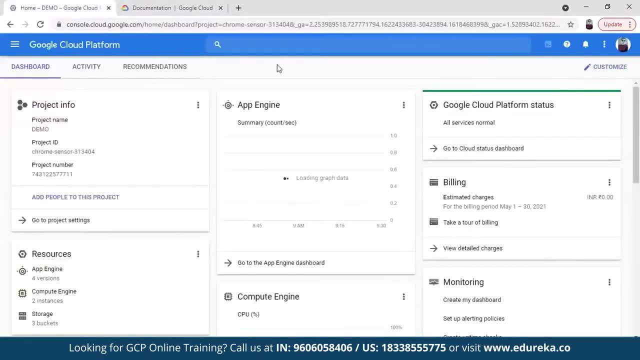 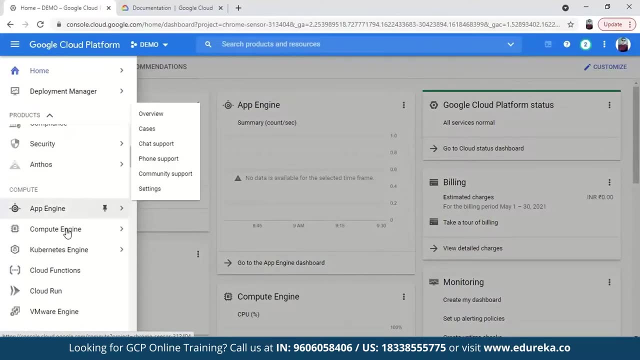 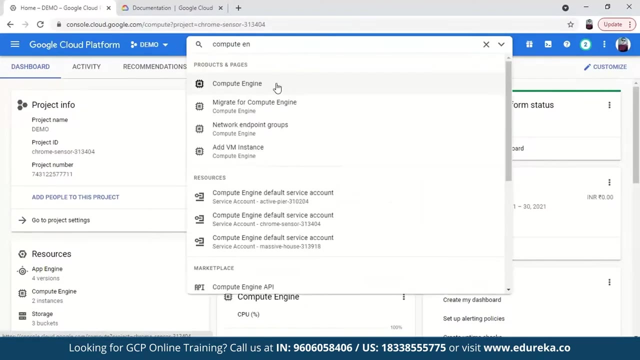 like much more understanding of google compute engine. so let's come back here. we have opened the console. this is how the google cloud platform dashboard looks like. you can either go from here to compute engine, from here we can open, or you can just search here compute engine. okay, so these are the virtual machine instance templates. so these are different kind. 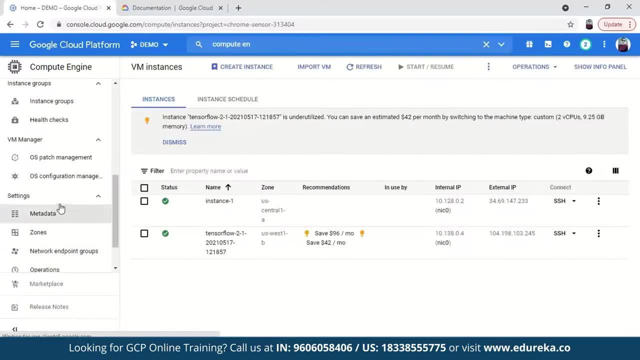 of virtual machines are given. then we also have storage. under that we have a stamina. we have this snapshots, or images, as i've told you like. there are built-in images also and they are like custom images also. so here's the dis. these are discreet, already been created. and then we also have 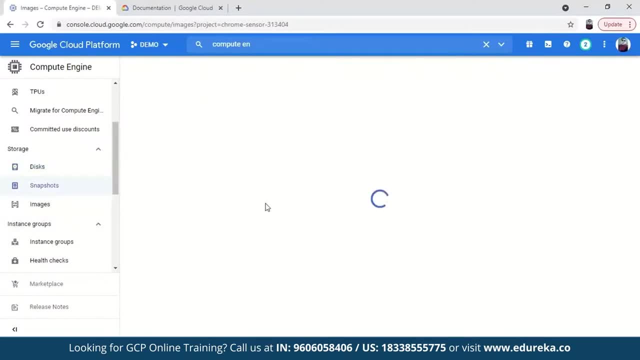 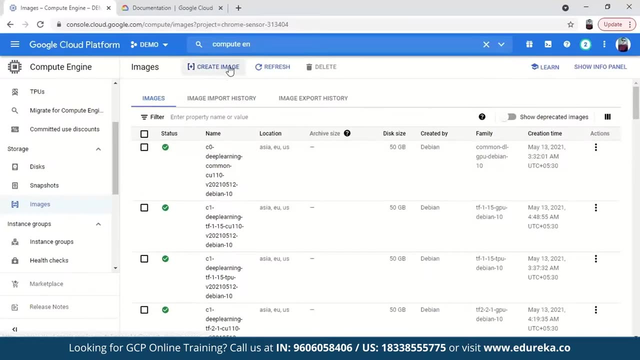 snapshots. one of the snapshot is also there. so then we have images. so these are the built-in images. you can use any of them, or, if you want to make your own custom type images, you can create image from here. okay, now let's finally go to virtual machine instances and let's see how we can launch an instance. 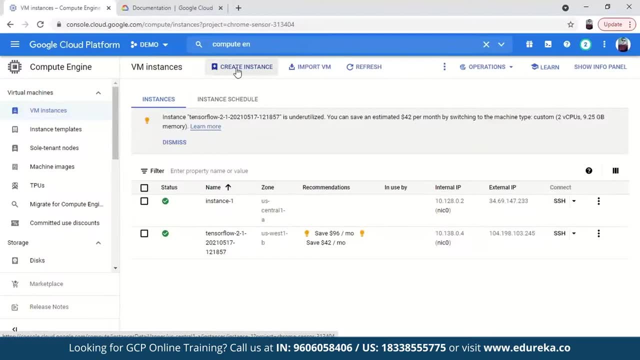 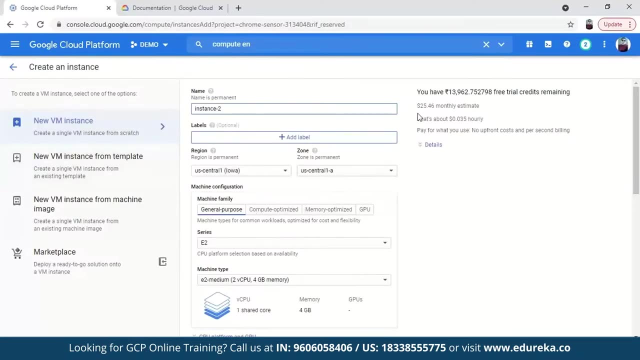 so these are the two instances which i've already created, so let's go and create a new one. okay, so you can name your instance here and here's. whatever configurations you're gonna give now the price will change. okay, like i can show you, just for showing. 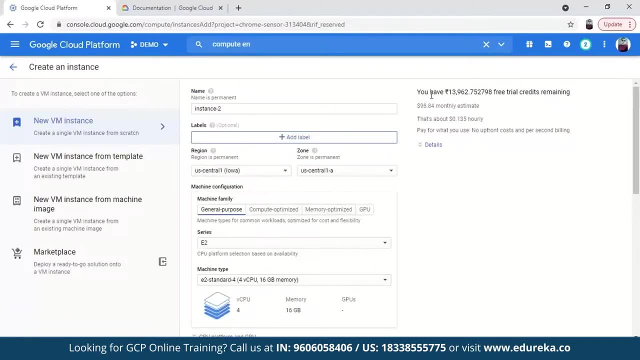 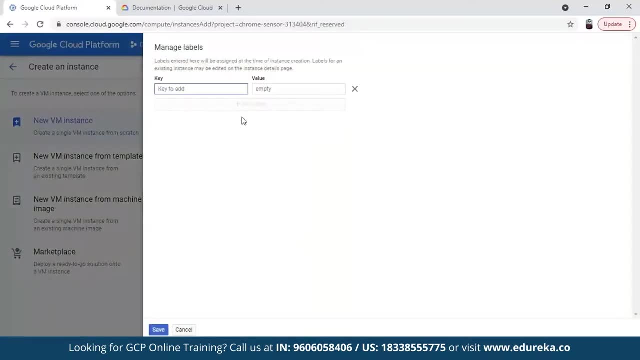 purpose. i'm just showing you. if you change it to four virtual cpus, see the price has changed right again. go to the small one, okay. so you can also add label here and give it a key environment and give testing, okay. or you can add much more label, then okay, you can add more labels like: 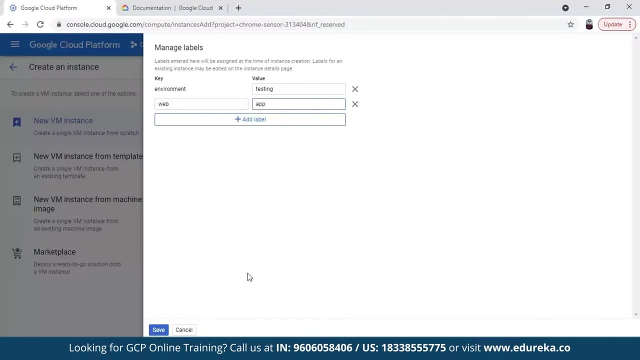 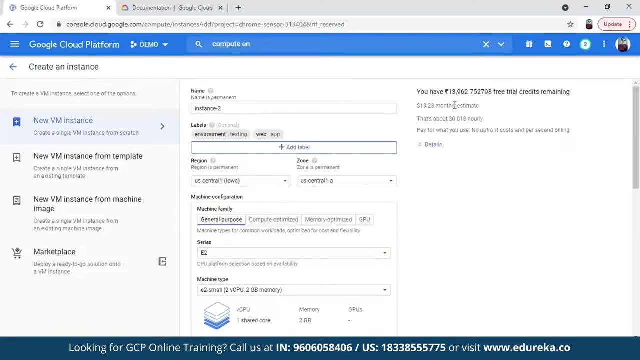 i can give the value for it like app. okay, you have to do that. and then you can like save it. okay. then we have like: see, i'm changing the configuration, that's why the price is changing, okay, and then we have to see the region also, under that region and zone you have. 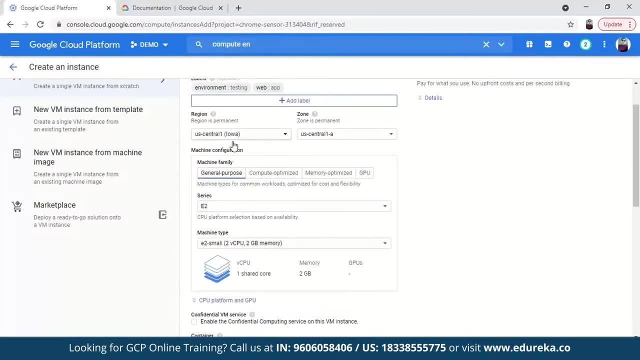 to select and that we have different services. okay, like right now, the under this, these services are there: general purpose, compute optimized, memory optimized and gpu. okay, like you can see in this e2 series, we have for general purpose, we have series and we have machine types of four cpus and 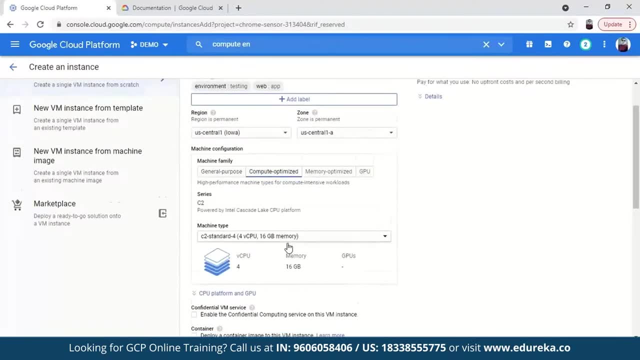 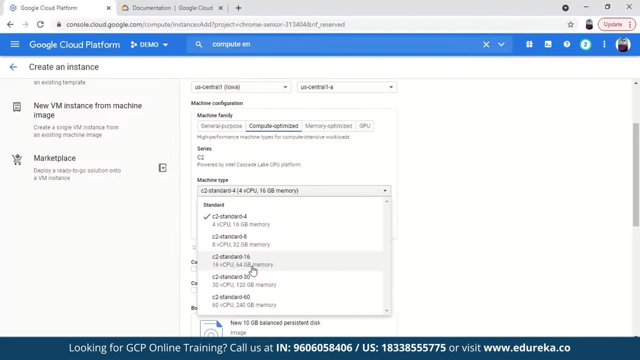 8gb memory and all this like that. then we also have a compute optimized. also under this. we have 4 cpu 16 gb and then 8 cpus. we have 32 gig for 16 cpus. we have 64 gig, these kinds of cpus. 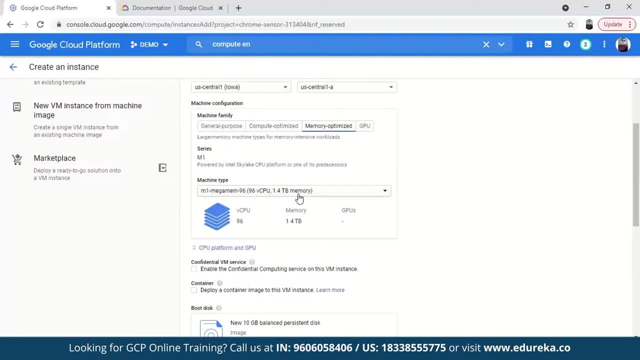 and memory is given and if you come to memory optimized, these are the large ones, these are the ultra level ones. so there are like 96 cpus and one 4 point tv of memory, also 40 cpus and then 60 memory, and then we also have gpus for it, for 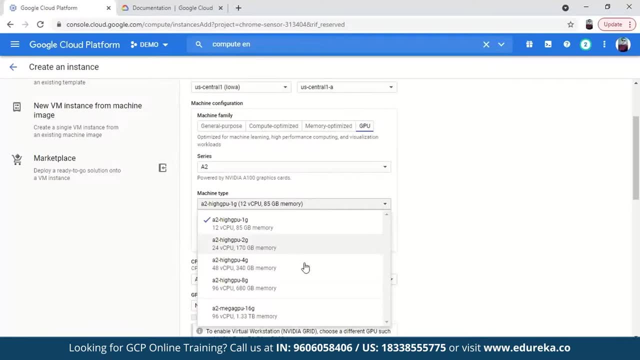 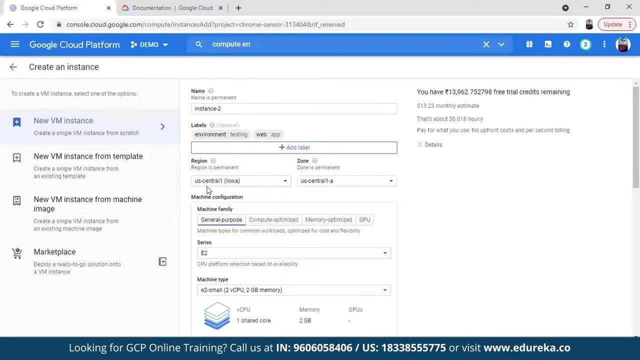 different machine types. we have these kinds of 424 virtual cpu, 170 gb memory and this way it is given, but remember that you don't get it in every region and zone, like i can show you right now. it is selected as ua, central one and usb. 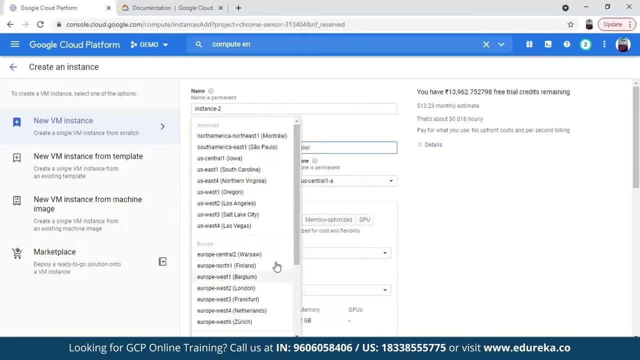 central one a right. and if we change it to europe west, okay, let's see. if we change it to europe west, see, now you can see, gpu is already gone. if we see for c1, now even the memory optimizer is also gone. so that's how it works, okay. so let's go to the default one only, which v1? yeah, okay, then we have. 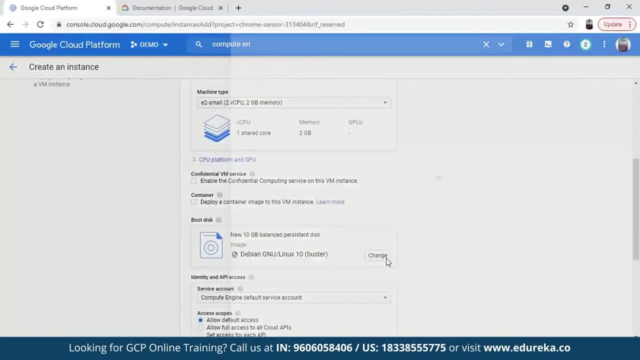 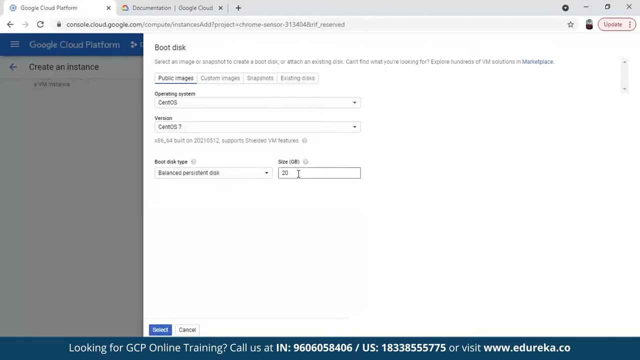 boot disk also. you can change this boot disk also, like you can go to change. you can select a public image or anything for different one. you can use this and then yes, oh, seven, okay, let's go to 50 also, we can do that and then we can select it. okay, or we can go to custom images, if you want to. 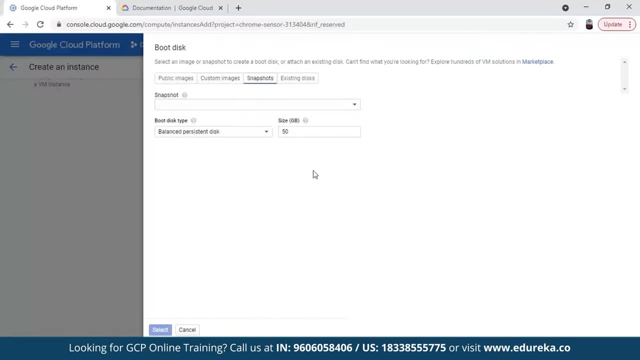 use any custom image of yours. you can use it here. if you have any step shots taken, you can also use app shots here. also if you have an existing disk or a like, if you have made some existing disk from a previous virtual machine, then you can use it, but right now we don't have one. also i've shown 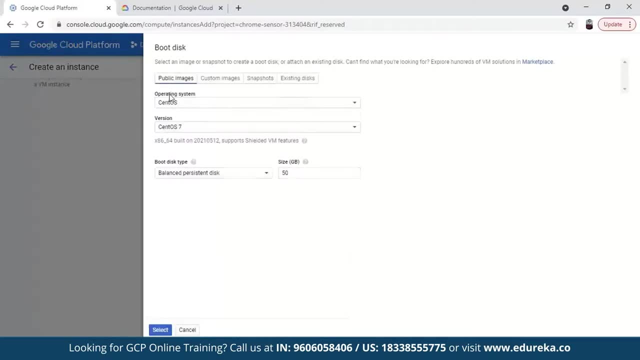 this here. you can select it here. okay, you can change it again. you can just go to db and only. okay, linux is selected, balance persistent disk or ssd persistent, which one you can select. give it then only and just select it. this is the depositing we have done again, and then you can. 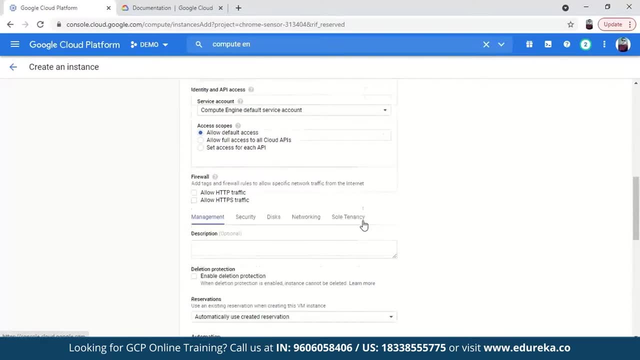 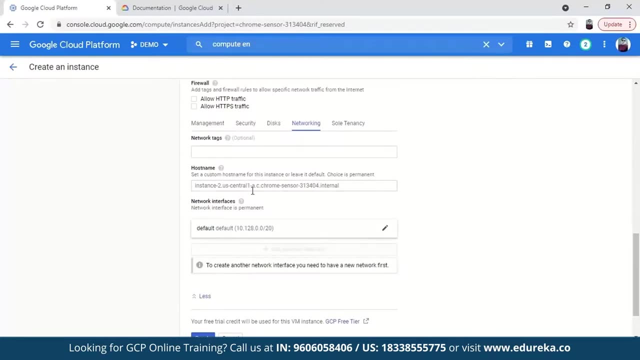 come to this management security, this network household tendency and just select it. let's come to the networking part. if you already have a network tag or something, you can select it here also you can change the host name, or whatever host name you updated, you can give a different one also. 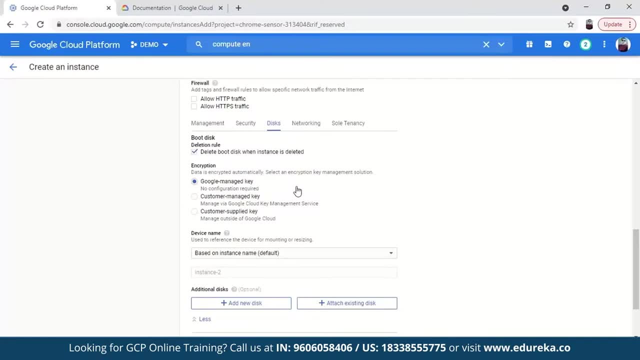 okay, and then we have discs. it's like if you have creating virtual machine you can, if you delete a virtual machine also you can retain your disk. also there is an option here: delete boot disk when instance is deleted, so you can just deselect it. so if a virtual machine is deleted, then also a disk. 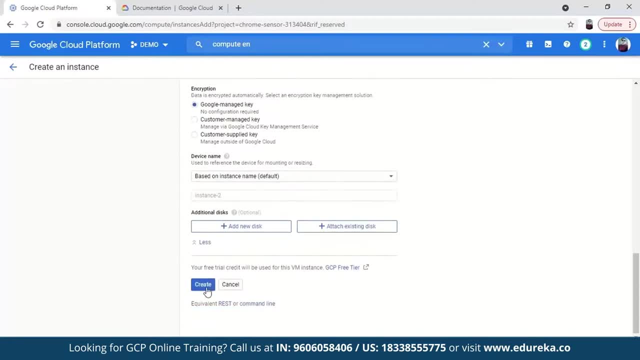 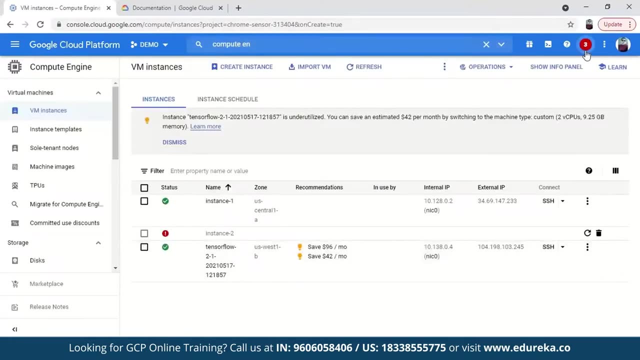 will be like retained, stuck in doing it. so let's create it. well, i think there is a problem. there's some problem with virtual machine strength and it's boot disk instance. yeah, okay, they don't support. what you can do is early. this is something. there are certain limitations, there are certain 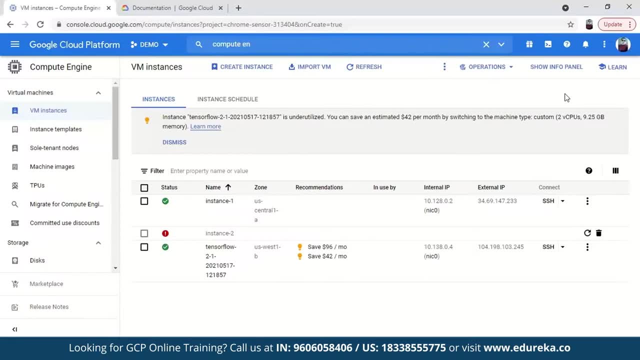 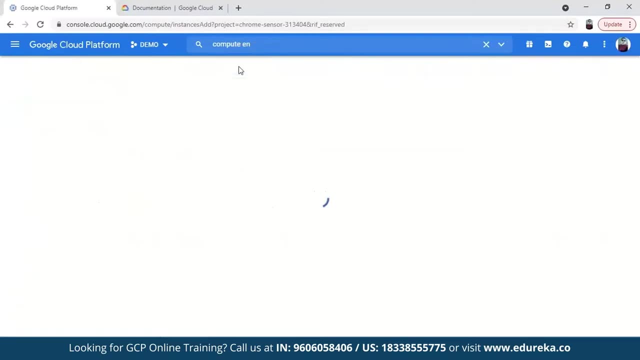 limitations of, i want to say for free trial, because this is a free trial. okay, so you can buy one or you get. there are certain limitations. you have to follow those limitations. so you can like simply create a default one with default settings. you can like: right now i'm not doing any. 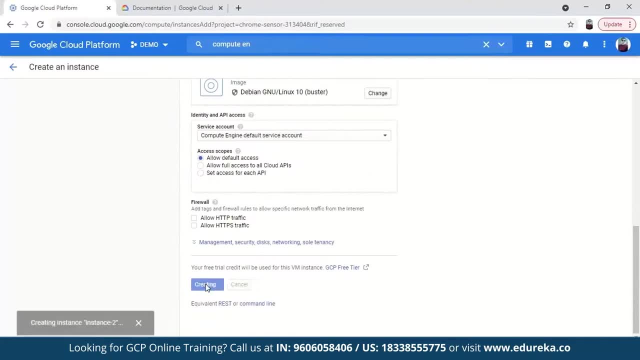 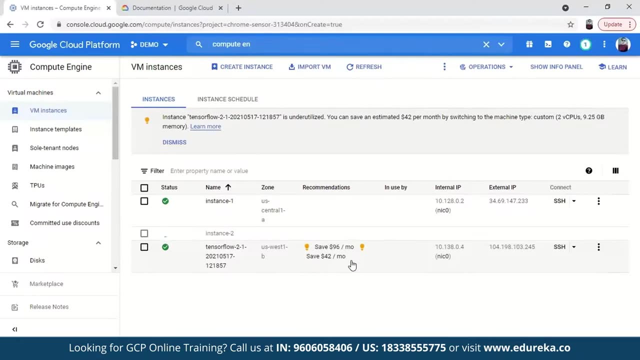 customizations and everything. so you can just create that for now. so it will take a few times because i've changed some settings now. that's why it wasn't able to run and there are certain limitations. i hope you understand. yeah, now it's been created. also, let me tell you this: like suppose, if you have created this instance and you have working, 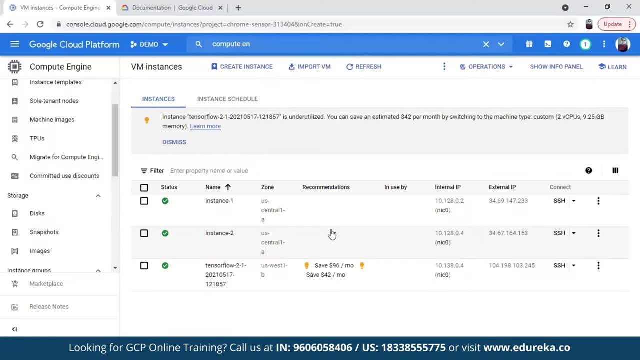 on it. you have created this one server, we've created this virtual machine, i mean, and you're working on it for a long time. you work and then suppose a teammate comes and he sees that and he feels like okay, this is a lot of mess up, so he deletes the instance. now what happens is: 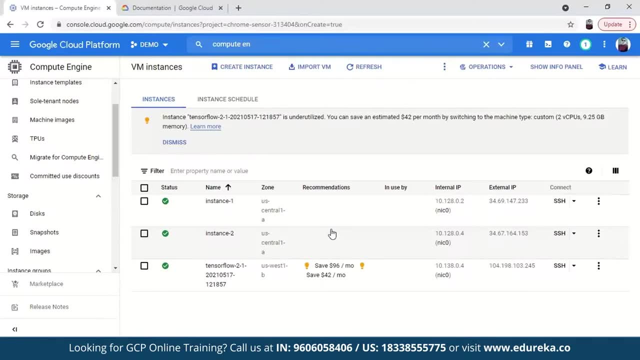 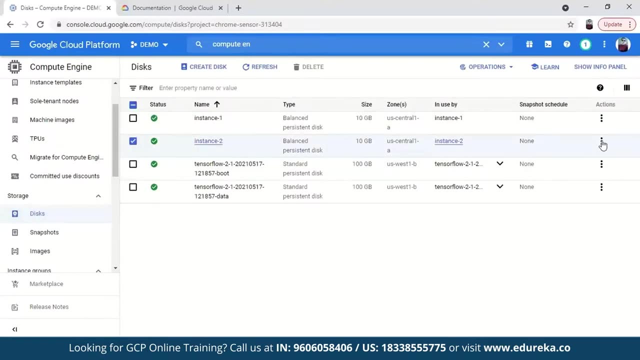 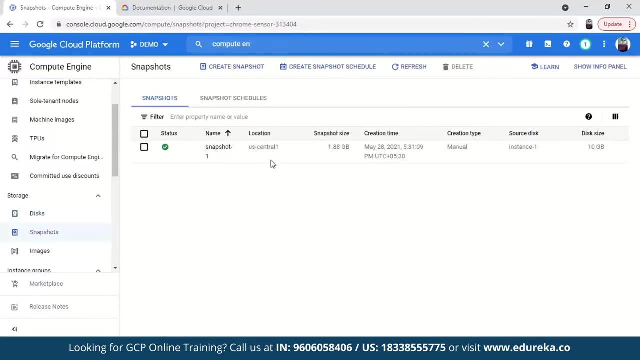 it will be like: oh, your work is gone, all the work you have done is gone. but what you can do is: or you can go to disk only, okay, so this is the instance too. what you can do is create a snapshot from here, okay, or you can just: snapshot is created, it will be created here. 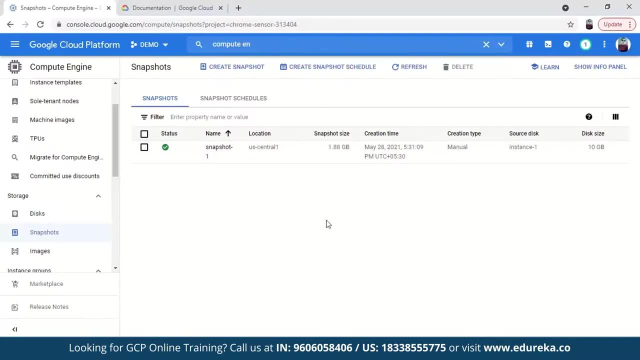 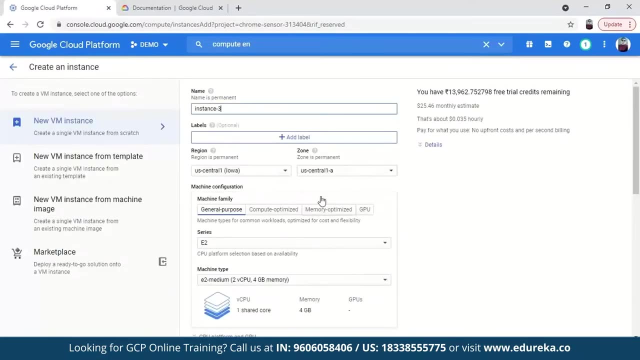 okay, like another snapshot is here, for instance one. if youりateit for instance two, it will be created here itself. so, while creating the instance, what you can do is if you have taken the snapshot, okay. so what you can do is, from here, you can change it and you can go and select a snapshot. 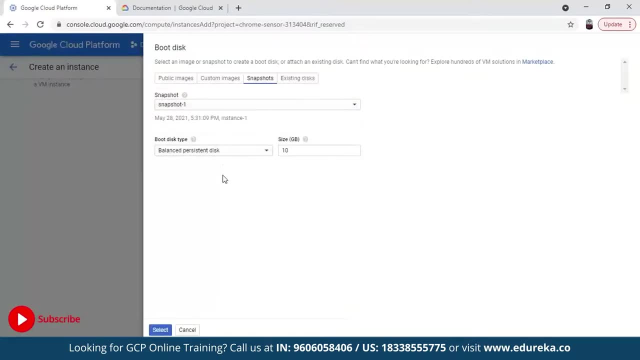 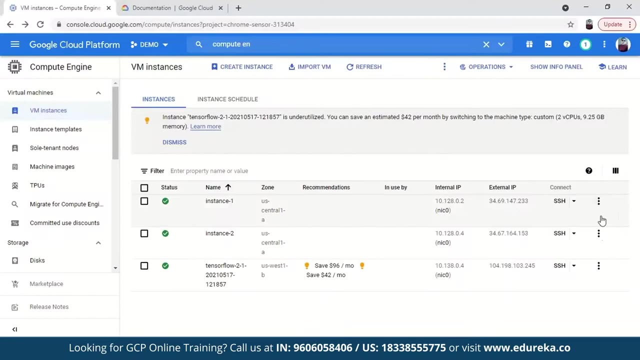 from here. okay, like right now, snapshot is given. now, for instance, one just given. if you use it, all your work will be retained, how it works. also, you can, like you want, to delete an instance. you can just go here and delete the instance from here. it will take a few seconds. 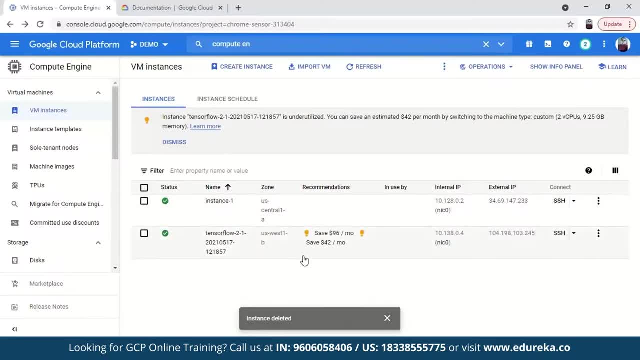 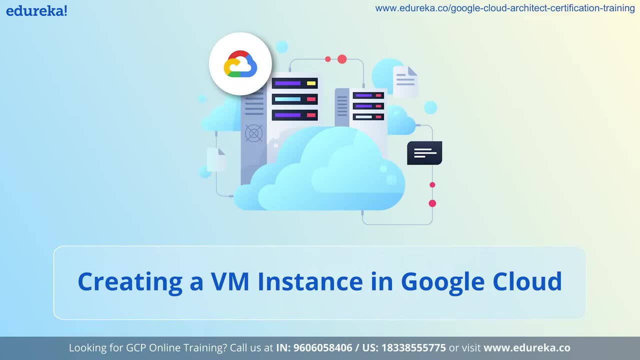 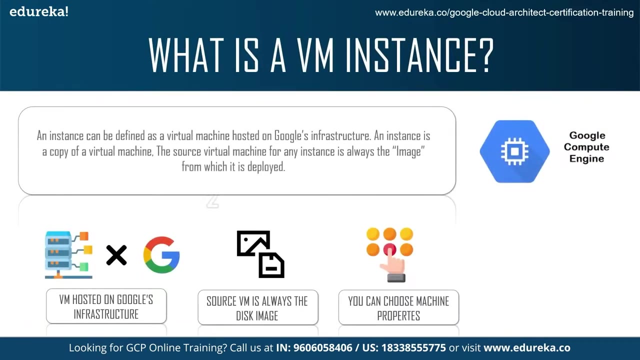 yeah, then chance got deleted. I hope you have understood now. this is the basic demo. so what is a VM instance? as we all know that a virtual machine is a digital version of a physical computer, right? so a virtual machine, software, can run applications, operating systems and all of that. so, virtual machine being a copy, 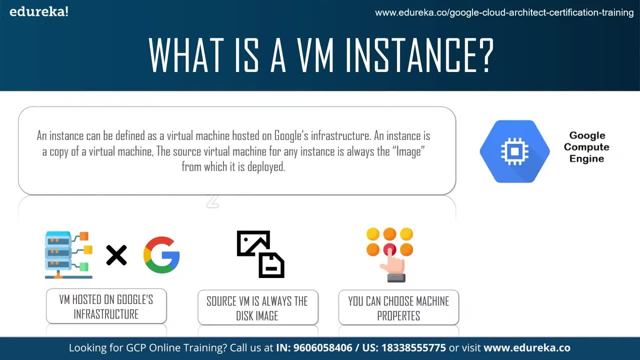 of the physical machine. when it comes to VM instance, an instance can be defined as a virtual machine hosted on Google Cloud Platform infrastructure. right, since we're talking about Google Cloud Platform, one machine instance is here. so a VM instance is nothing but a virtual machine that is hosted on Google. 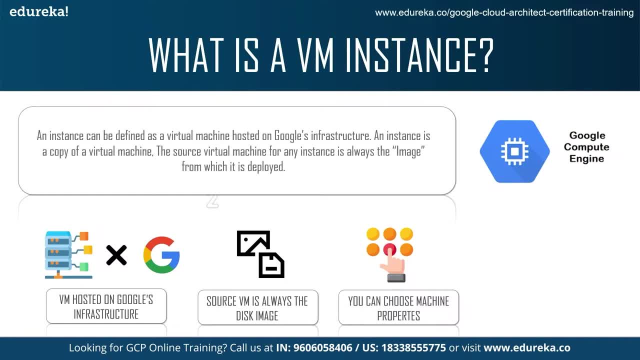 Cloud Platform. so the source virtual machine for any instance is always the image from which it is deployed, right? so VM hosted on Google Cloud Platform infrastructure is a VM instance. the source VM is always the disk image that is available and fact that you can choose your various machine properties. 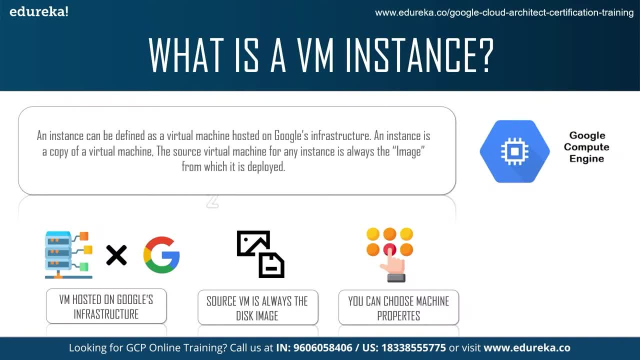 that are there. so when you create a virtual machine, you get to choose the kind of properties your virtual machine will have, let's say, for example, the kind of networking properties your VM has, or let's say the kind of storage capabilities, the instance type that you choose. all of these can be chosen by the user when 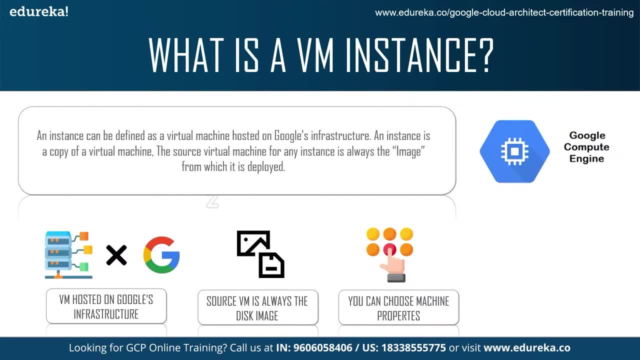 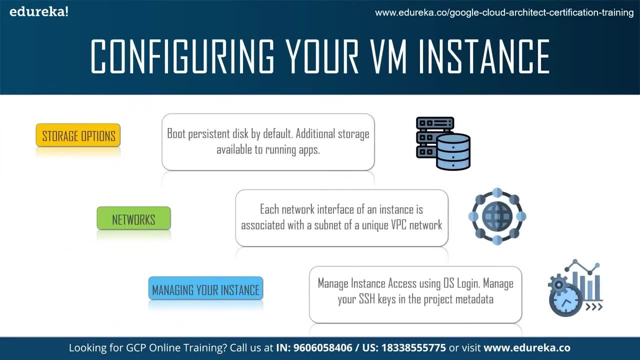 you're creating a virtual machine instance on Google Cloud. so next we come to configuring your VM instance. now, when it comes to configuring your very own VM, there are many options that you have when it comes to configuring your VM instance, such as you can configure the storage that your VM provides, the networking. 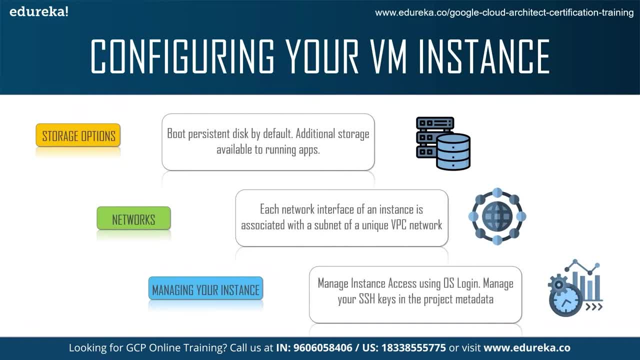 capabilities that your VM has, and also you can manage your instance overall. so storage options are various and most important thing is that, when it comes to storage, boot persistent disks are there by default, so additional storage is always available to run apps. next up, we have networks. now each network interface. 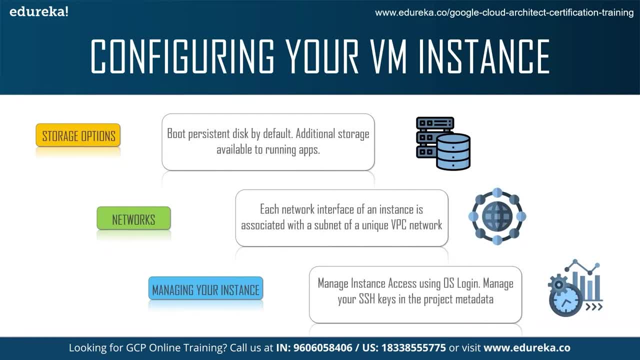 of an instance is associated with a subnet or a VPC unique network that you have now. that is basically the fact that when you create an instance, if you have certain subnet for a certain instance, your virtual private cloud will basically connect to that subnet that you have created before. so for this you 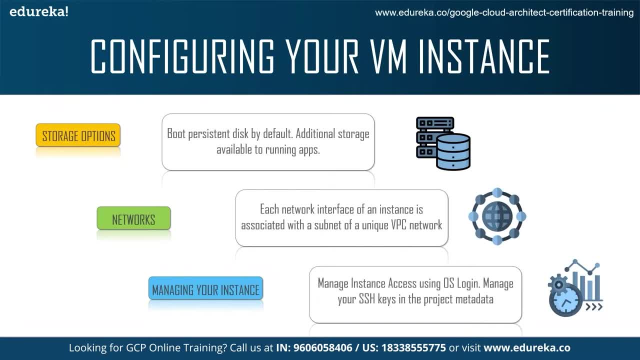 can use labels that you can have that you can also add during your VM creation process. so another thing that users can choose to do is add different labels to the VM instances that they create and finally, we come to managing your instance instance. now, managing instances comes with the manage instance access during 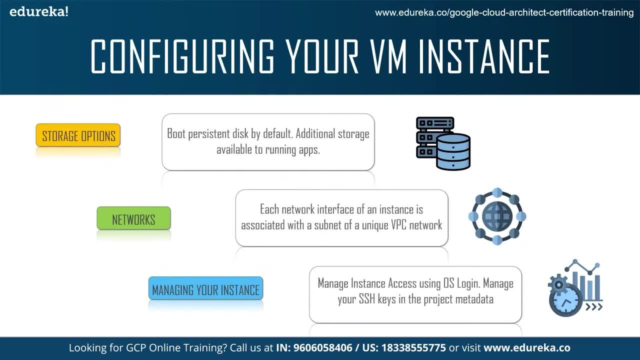 all OS login right, so you manage your SSH keys in the project metadata. now these keys will basically help you log into and connect to your VM when it has been created. now these keys are generally private keys and basically, if you want to log into your OS and access the VM, what you have to do is generate. 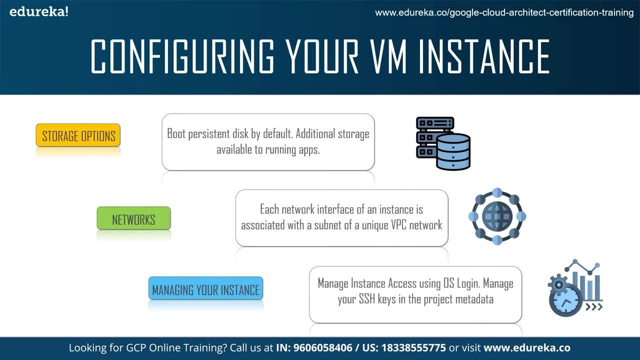 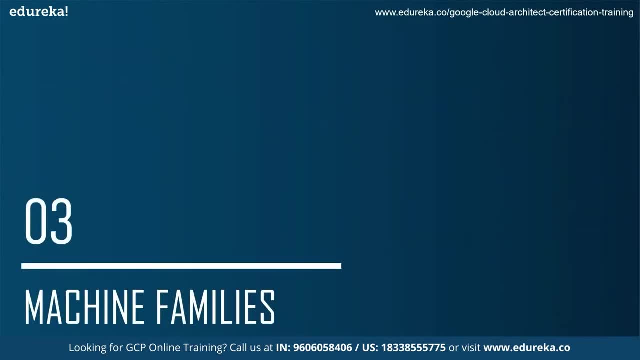 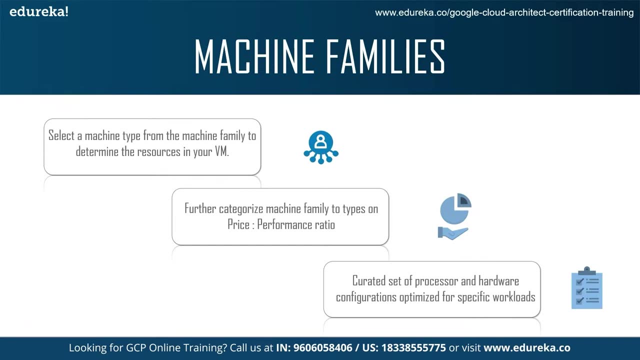 certain private keys that will be able to access your VM. this is all about configuring your VM instance. next up, we come to the machine families. now, what is a machine family? a machine family is nothing but a curated set of processor and hardware configurations that you have, which are optimized for specific 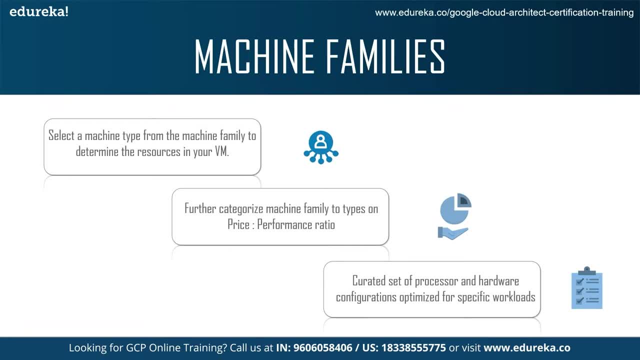 workloads right. so when you talk about Google Cloud Platform and the virtual machine instances that they have, there are various different machine instances that they provide because of the different machine families that they belong to. let's say, for example, there are machine families such as the n1, n2d and the n2. 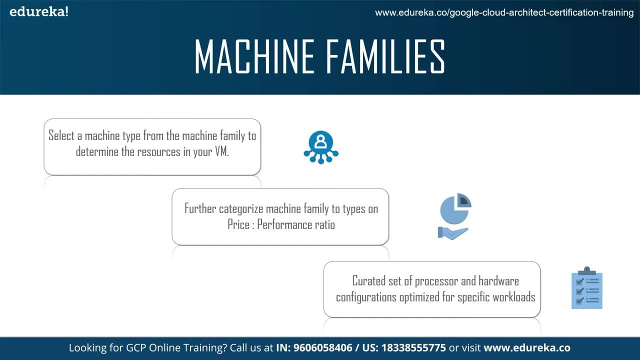 available. now. each different instance is optimized separately for a separate workload and the pricing will be based separately on that as well. so machine instances: when we talk about it, let's see that first we select a machine type from the instance family to determine the resources in the VM right, and then 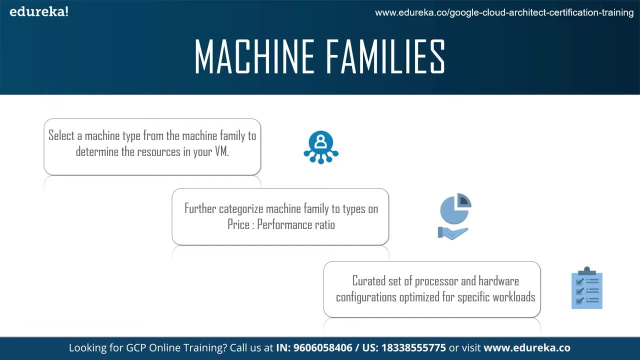 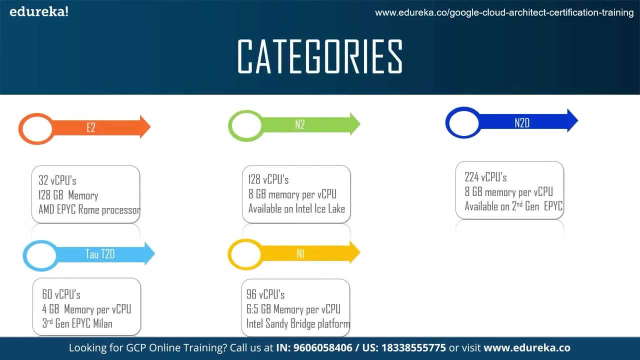 we further categorize the machine family to types on the price to performance ratio that they have. and finally, the curated set of processor and hardware configurations is optimized for the workload that is there. so next up we can talk about the different categories that are there now. the first category is the e2. now e2 has around 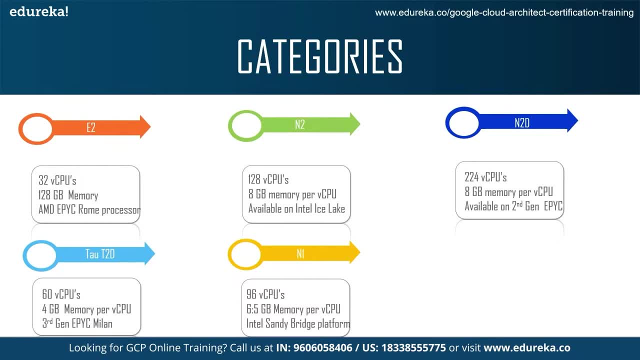 32 virtual cpus, 128 gb memory and the amd etyc rom processor right, whereas when we talk about n2, we can see that, compared to e2- 32 virtual cpus, n2 has around 128 virtual cpus, whereas there is around 8 gb memory per virtual cpu and it is available on intel isolate. when we talk about n2d, we can. 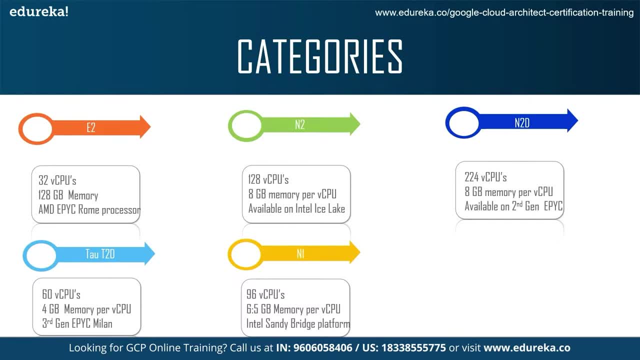 see that, compared to n2 and e2, n2d has 224 virtual cpus. the 8 gb memory per virtual cpu is the same as n2, whereas it is available only on second gen computers. let me talk about the tau t2d now. the tau t2d offers the users around 60 virtual cpus. 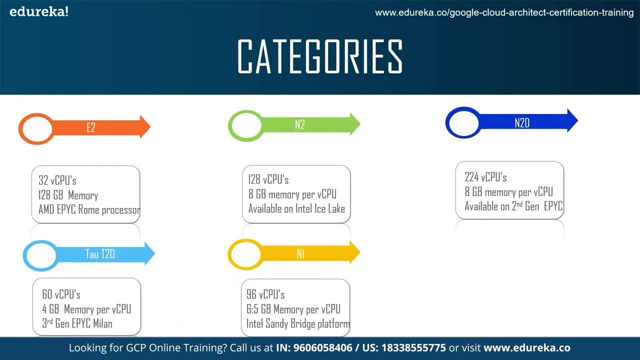 4 gb of memory per vcpu, which is different from the n2 and n2d and third generation epyc milan and the last one we talk about here is n1. now, n1 offers you 96 virtual cpu, 6.5 gb memory per. 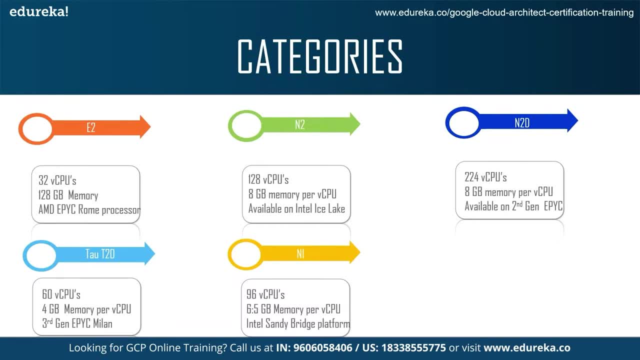 virtual cpu and it's available on the intel sandy bridge platform, right? so these are the various machine instances and the categories that they have and, as you can see, these are basically different and can be used for different workloads and basics, on the basis of which need needs to be optimized. for example, you can optimize the amount of virtual. 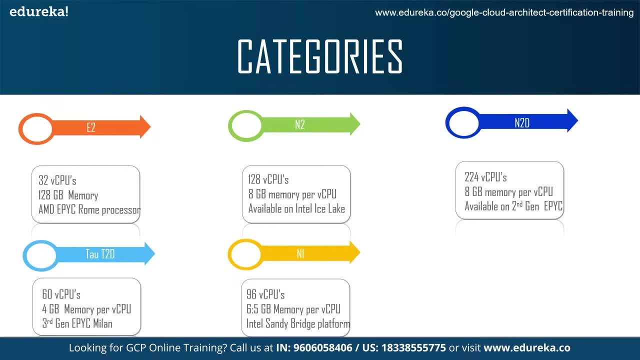 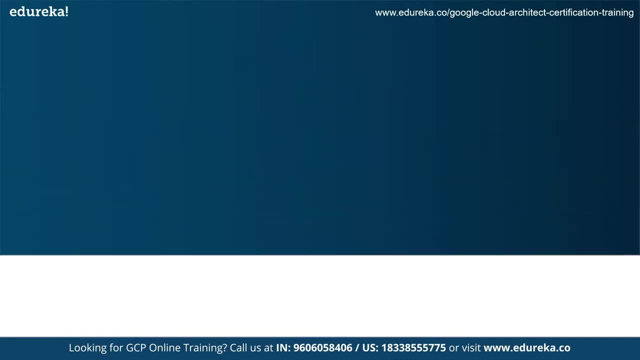 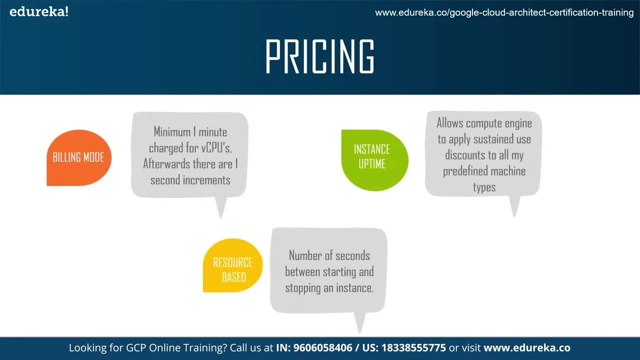 cpus, you can optimize the amount of memory. you can optimize other things as well, such as networks and all of that. so this is basically all about machine families. next up, we talk about the pricing. when it comes to pricing, it's based on three major points. basically, pricing is based on the billing mode, the instance, uptime and the resource, which is based on. 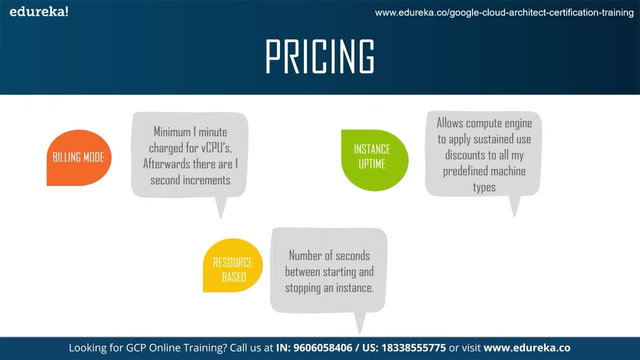 when it comes to billing mode william, one minute is charged for virtual cpus. afterwards there are one second increments for whatever vm has been used. instance uptime allows the compute engine to apply sustained use for discounts to all the predefined machine types that are there. and finally, there is the resource-based pricing model, which talks about the number of seconds. 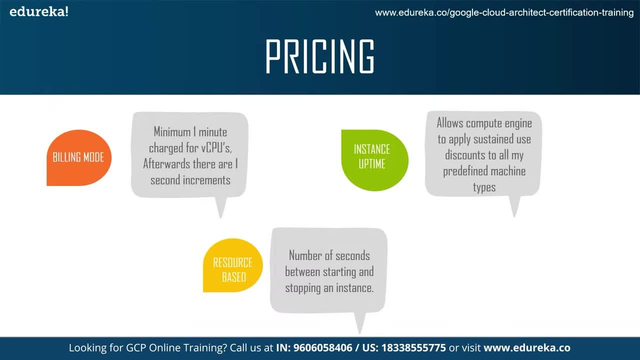 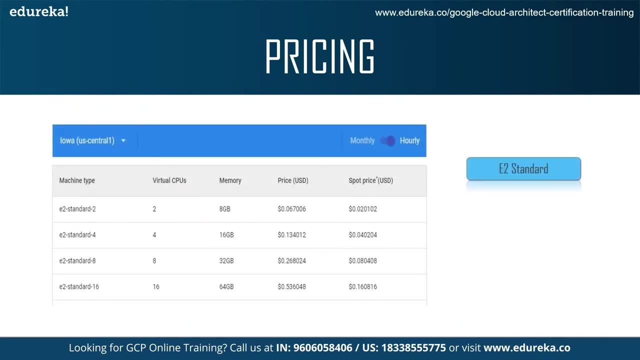 between starting and stopping an instance, and that is how you determine the price of your vn, right? so this basically gives you an idea about the e2 standard pricing, where we can see that the e2 standard 2 has two virtual cpus- 8gb memory- and is around 0.067 dollars per month, and the spot 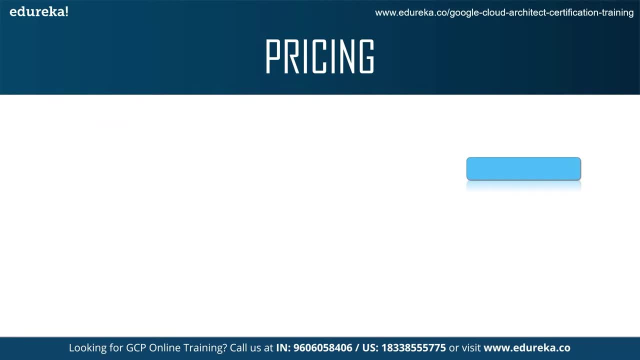 price is around zero point, zero, zero, zero, zero, zero two. so that is basically your pricing model. So likewise it's the same for N2, where you can see that there are different virtual CPUs for the different types of N2- standard machine types, And these are the different prices. 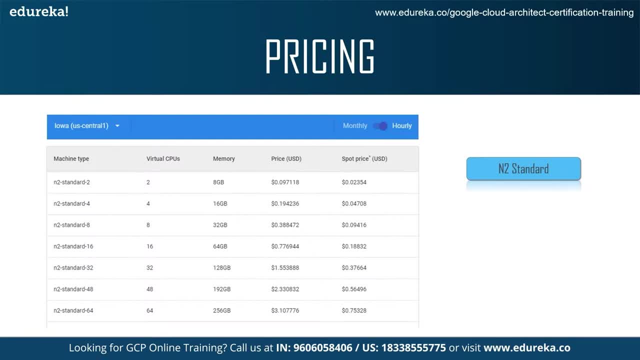 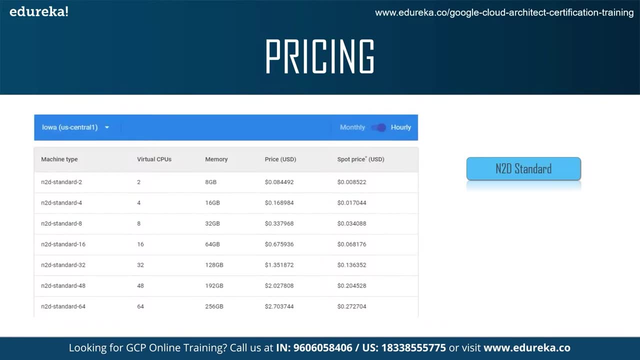 For example, N2 standard 2 has two virtual CPUs, 8GB memory, etc. And finally we can see the N2D standard pricing. Now, all of this is different for the different machine families that are there right? 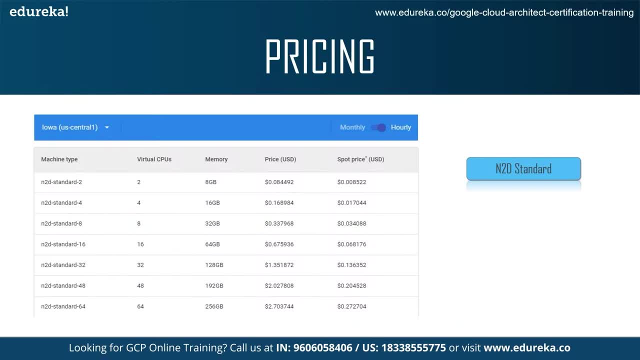 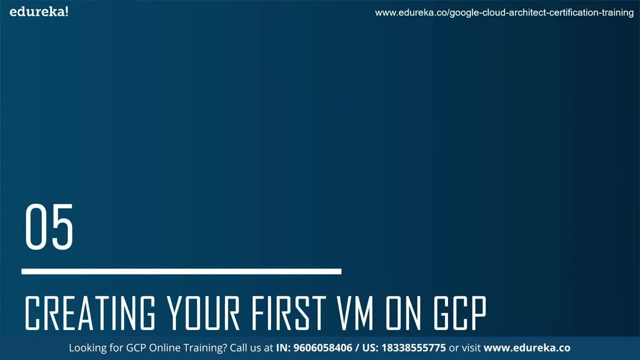 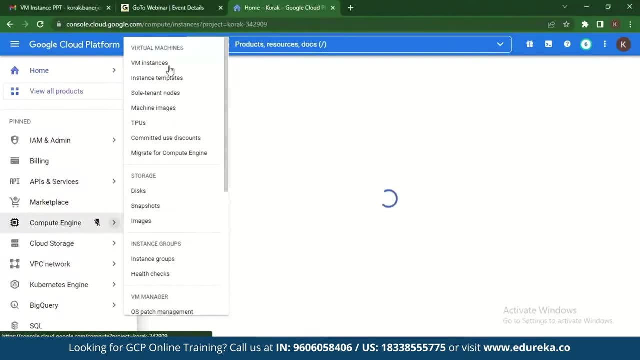 So this is how you basically see the pricing for what VM you are using. Finally, we come to creating your first VM on Google Cloud Platform. So let's get started. So log into your console and make sure you go to Compute Engine. So this is where you want to go. 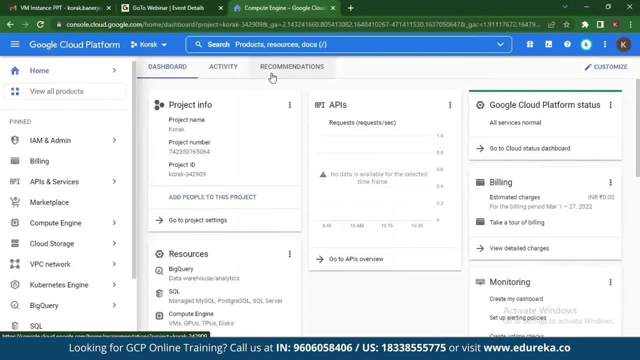 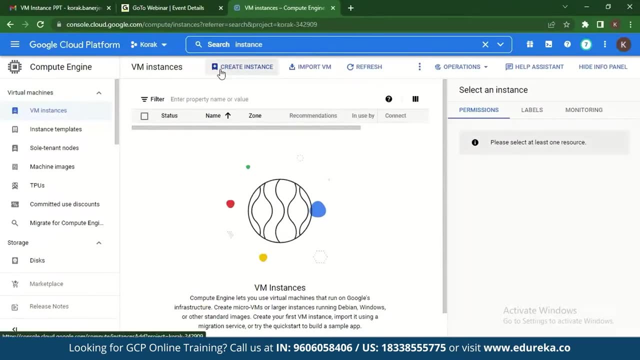 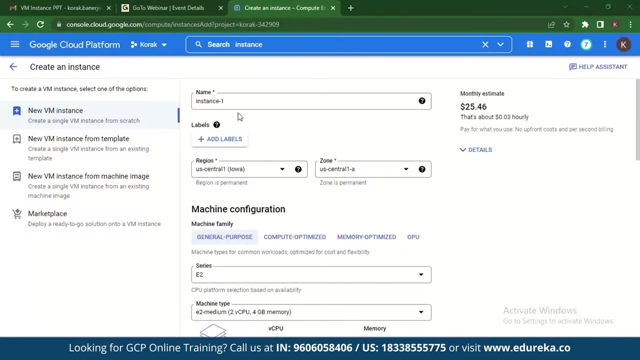 Once you go to Compute Engine, you have to go to VM Instances. Just try and go back here, Right? So once you go to VM Instance, what you have to do is go to Create Instance Now, as soon as you do that, so when you see you have Create Instance, you can name your instance. 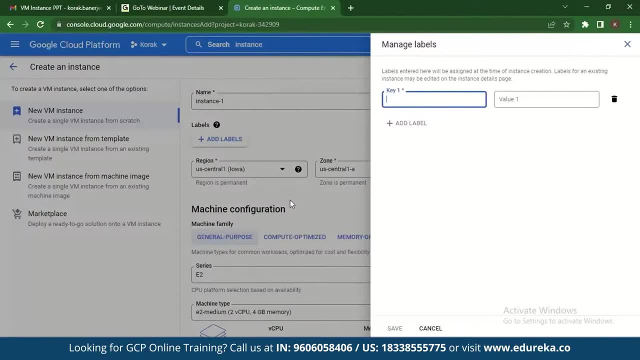 Let's say Instance 1. You can add labels to it. So next we come to labels. Now labels will basically help you identify the whatever instance resources are there. So you can help manage labels. So the labels will help you identify the resources that are there. 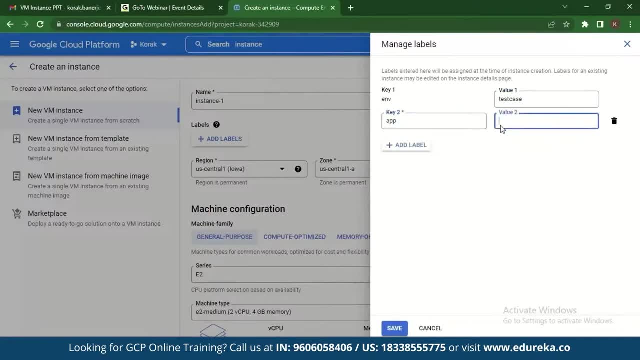 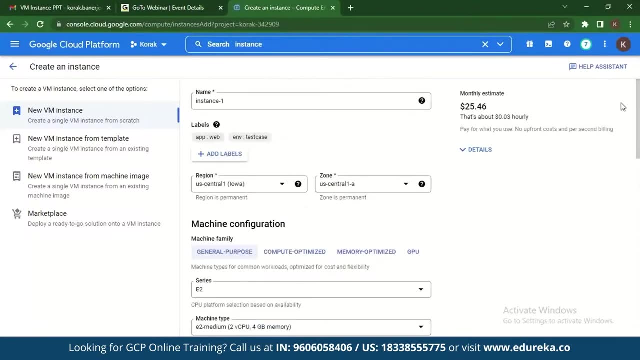 Let's say, for example: So you've now added your labels, So let's check out the other things that we can do Now. the region: let's see the regions we can do. So this is US Central right now. You can change this to a lot of things. 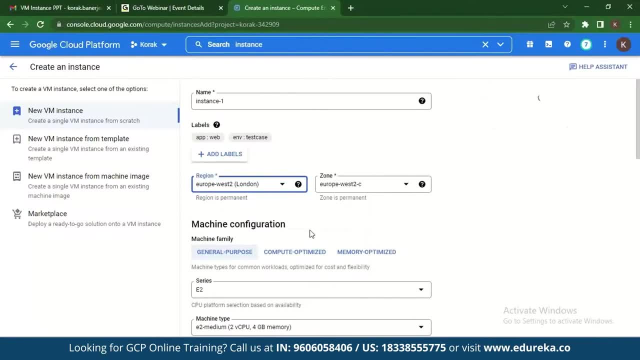 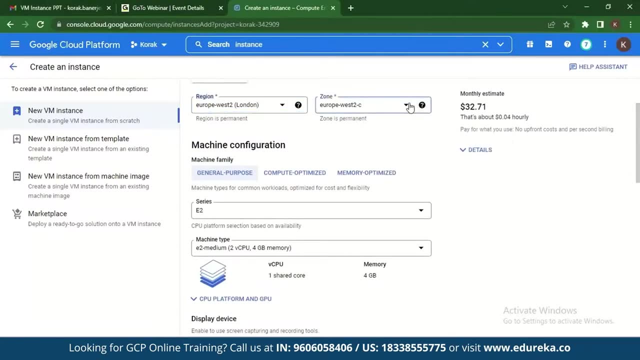 Let's change it to Europe and London. So if you change it to London, you can see here the different kind of machine configurations that you have Now. this has two hosted two to three hosted zones. Yeah, it has three hosted zones. 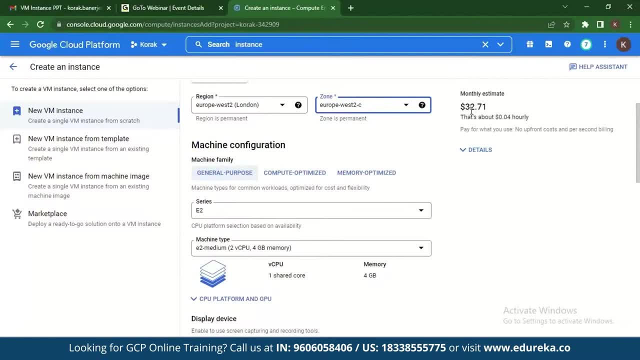 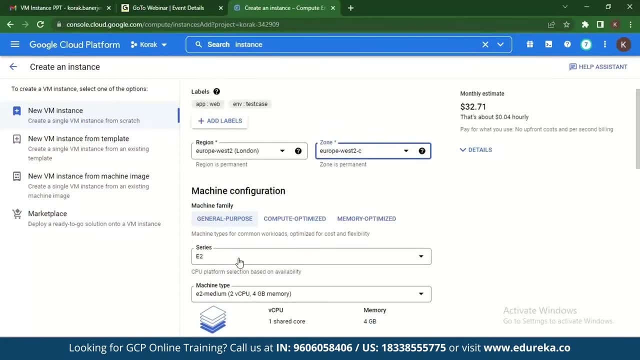 And, as you can see, there's a mastery estimate of you Having Around thirty two point seven one dollars per month, right? So machine configuration: Now this, by default, is set to E2.. What you have to do here is check out the other ones that are there. 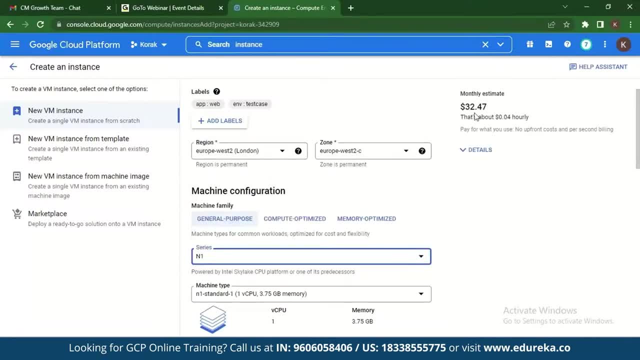 Let's say, let's check out N1.. So, as you can see, the price has just gone down by a little bit And you have to make sure that the prices for your VM are low so that you can have it free to, accessible and the machine type that you have here. 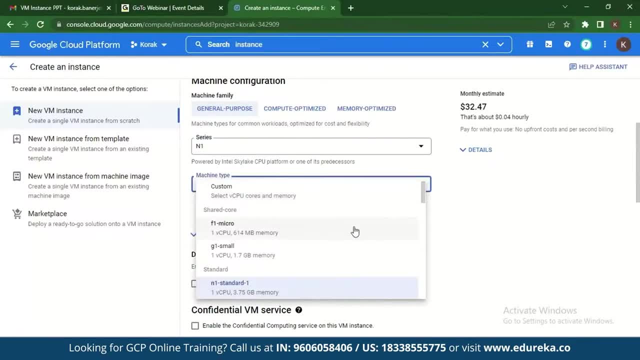 Is the N1 standard, but that is around thirty two dollars per month. You can change it to F1 micro. Let's see. Yeah, So once you do that, you can see that the monthly estimate is around six point one one dollars and it is free to access. 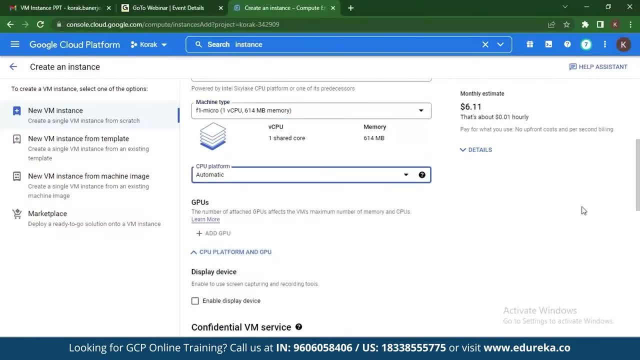 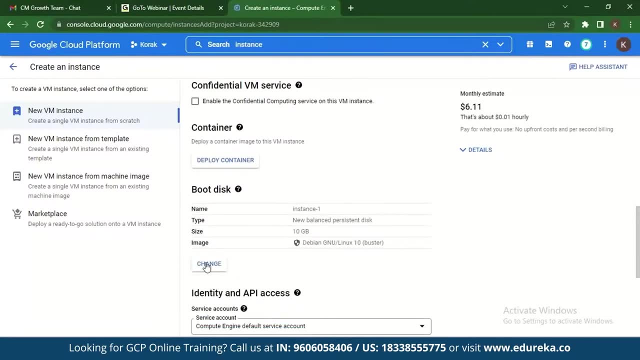 And the other things that you can do is the CPU platform and the GPU that is there. after that, If you don't have other things, you can check out the boot disk that is there. Now you can change your boot disk. Let's say it is by default set to Debian. 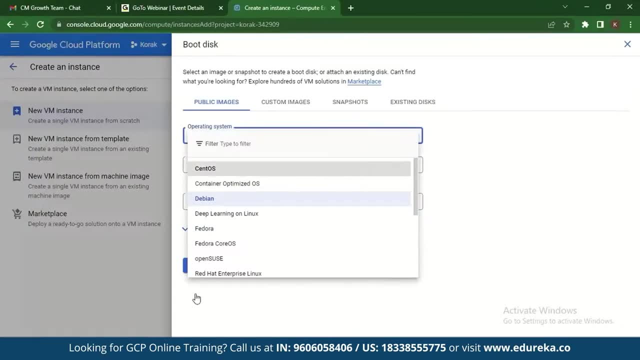 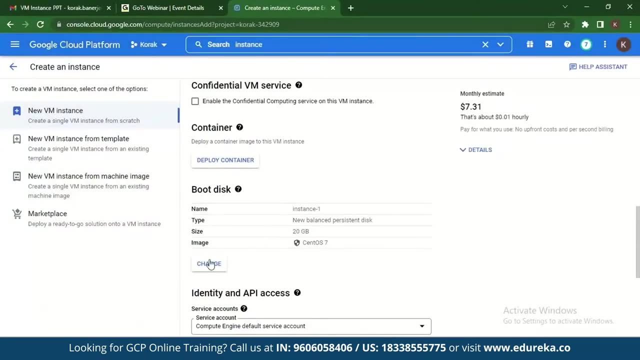 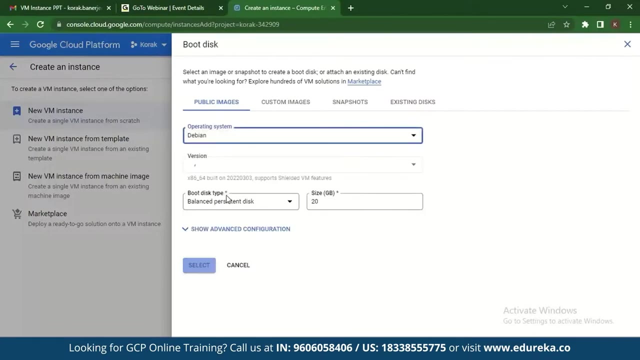 You can change it to CentOS. and once you change it to CentOS, let's check it out. The pricing changes and it has changed to seven point three one. So we don't want that. We want our VM to have the least possible cost. and we change it back to Debian and you go. 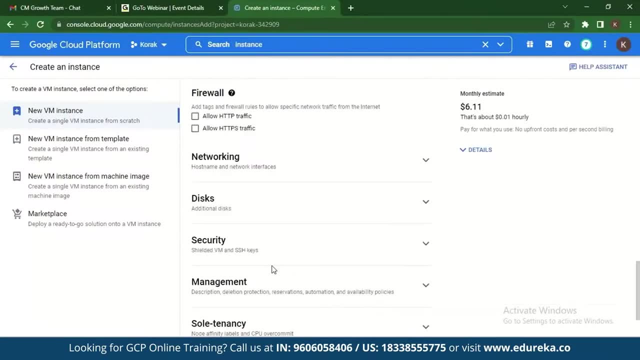 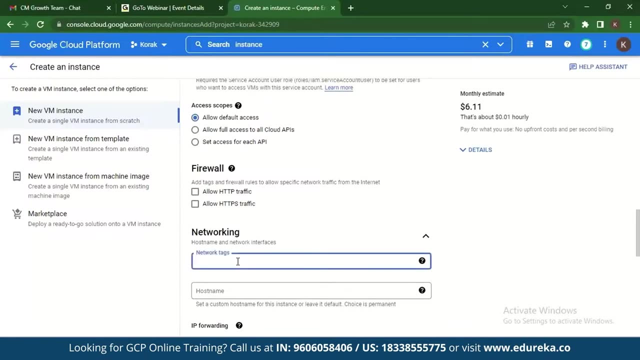 So we're back to six point one one. All you have to do now is go to the advanced settings. So once you go to these advanced settings, you have to go to networking And let's say you can add these tags, Let's say the web that you had. 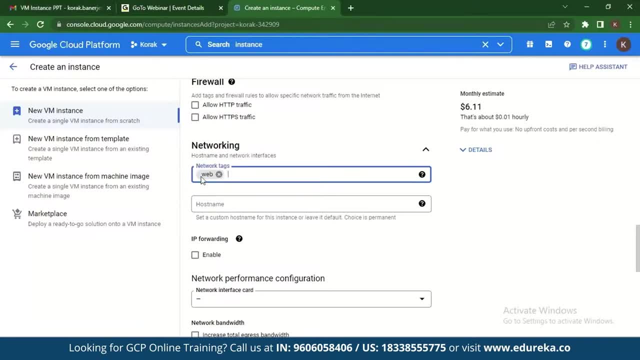 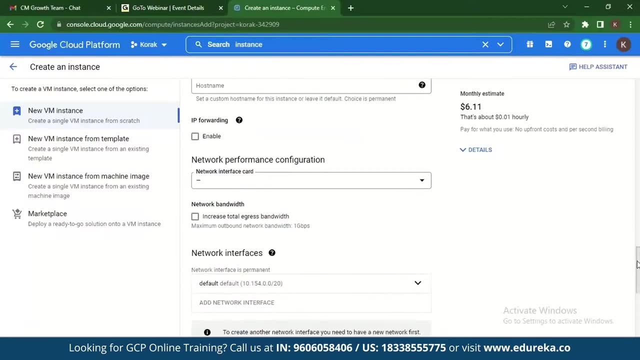 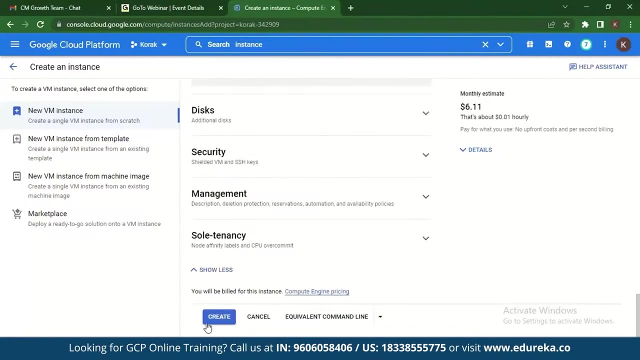 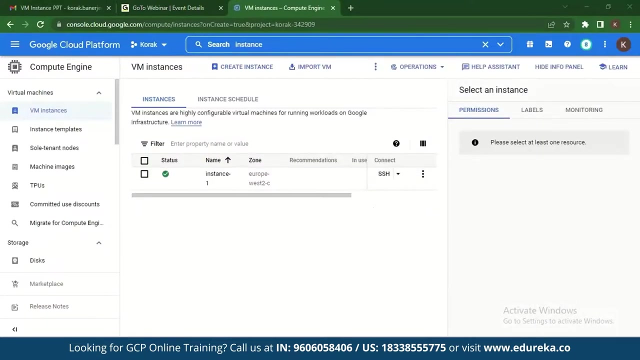 So this networking tag will basically have any resources, as the web tag will have to be rerouted towards this network traffic After this. that's just so. all you have to do now is create the instance. So, as you can see, your instance has been created. 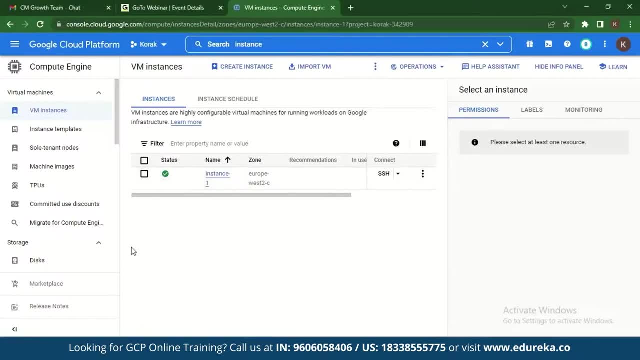 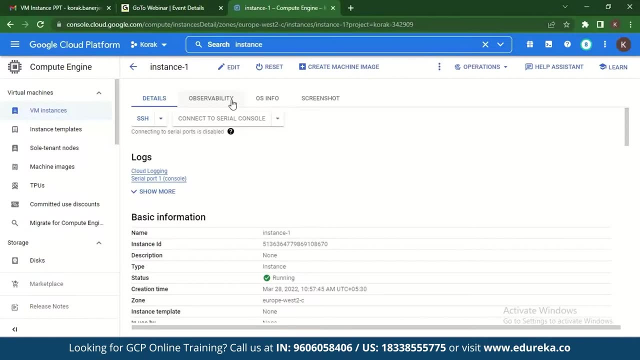 Now what you need to do is connect to your instance and you can check out your instant details over here. You click on your instance, You can check out the different details of your instance and you can check out the observability and all of that logs. 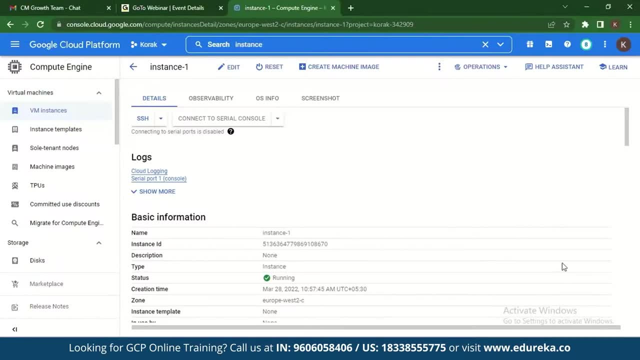 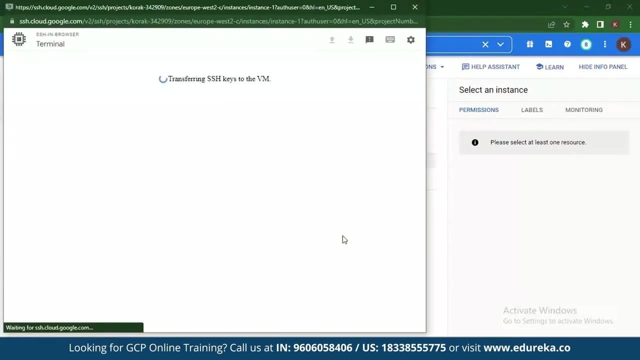 So, as you can see, this is basic information: Instance one instance, ID, the type of instance, the status, all of that with zone and the templates. So let's go back. I can try connecting to our instance. So if you go to basic SSH, let's try this one out. 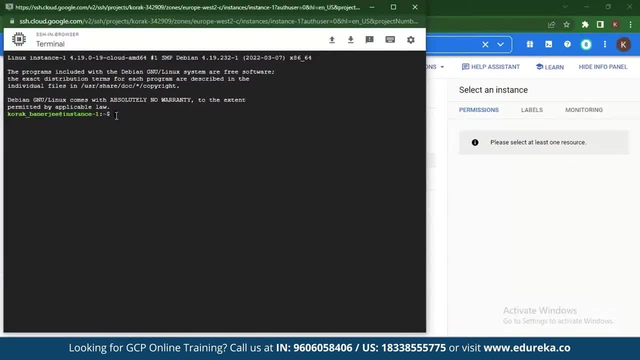 So, as you can see, the SSH terminal has opened up, so all you need to do is right now, type in LSB. So if you do LSB, you'll basically check out the name and the size of your disk And after this, just: 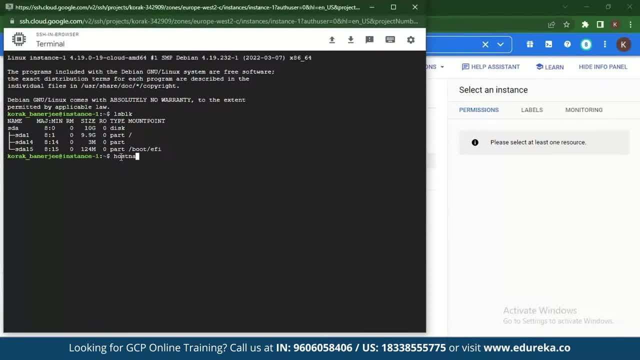 Put it to host name and instance one is the host name, So let's now check if we can sudo into this. Yes, we can. So right now, after this, all you need to do is cat, etc. slash, OS release And you can check the name of your Linux VM. 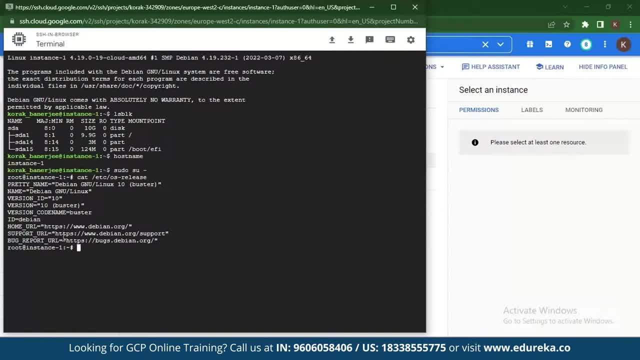 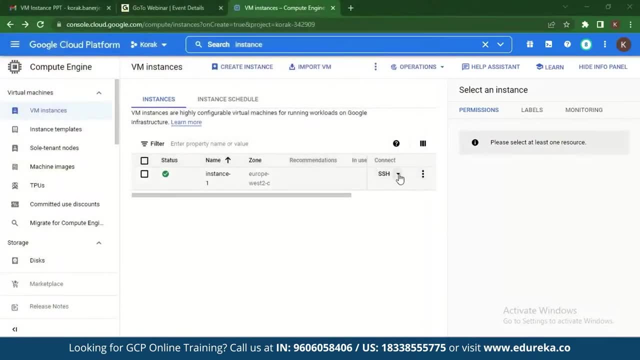 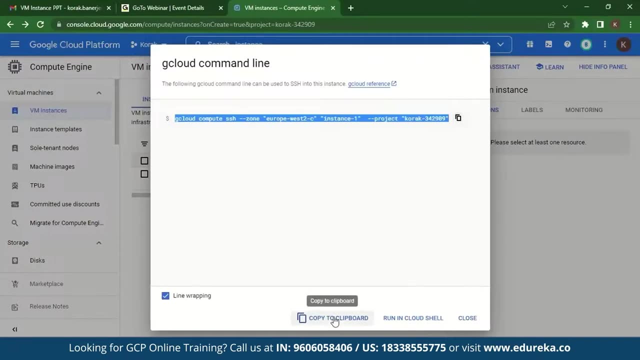 And ID, the instance type, all of that. So this is how you check it with SSH, right? So what you can do now is try and check it with the others as well. You can check it in gcloud command. All you need to do is copy this and run in cloud shell. 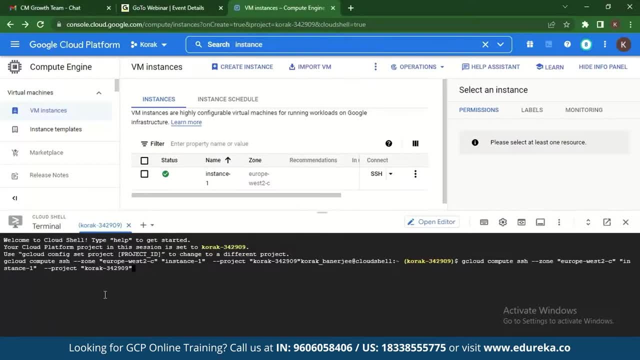 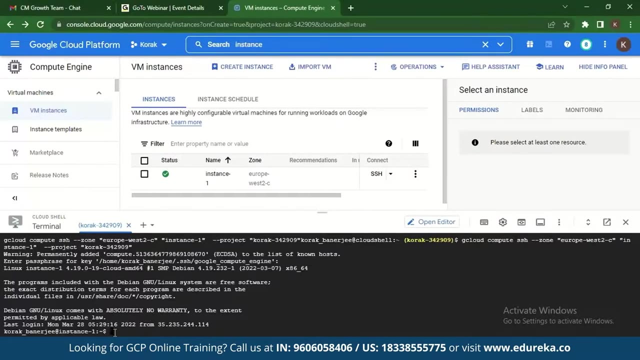 Right. So this is the command that you've used to connect to your cloud shell, And all you need to do is enter And authorize Right. So this is basically your connecting to the instance, And all you have to do here is the same command: cat, etc. OS release. 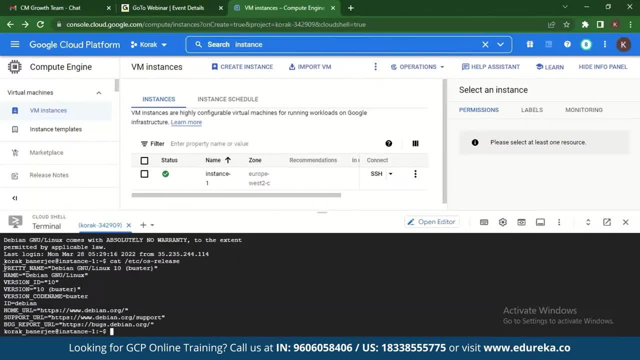 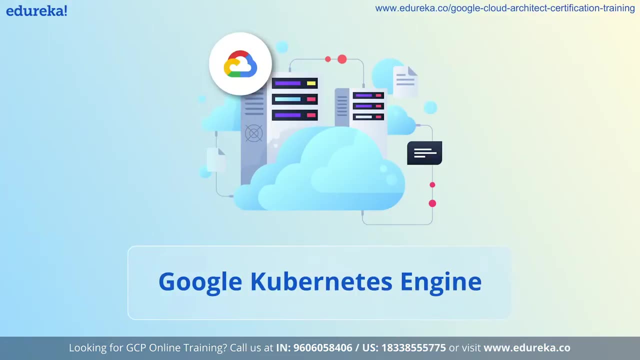 Enter Right. So once you do the cat dot, etc. you can see that these are all the names of the VM and the version and the ID that you have. So this is how you can connect to your VM instances in Google Cloud. What is Google Kubernetes engine? 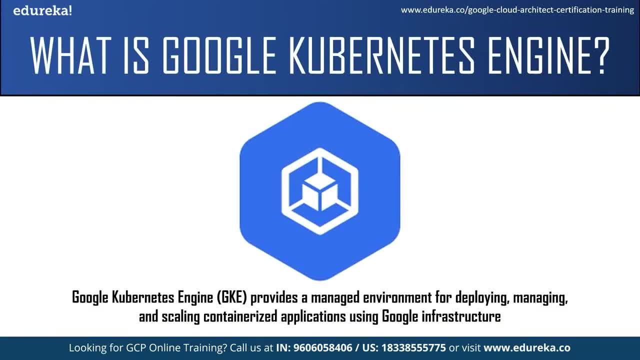 Google Kubernetes engine provides a managed environment for deploying, managing and scaling your containerized application using the Google infrastructure. The GKE environment consists of multiple machines, specifically compute engine instance, which are grouped together to form a cluster. Now, a cluster is the foundation of Google Kubernetes engine. the Kubernetes 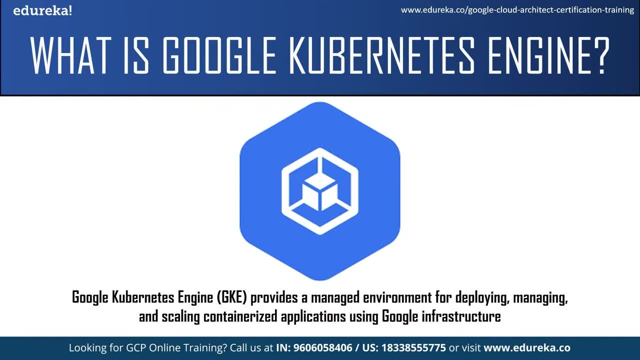 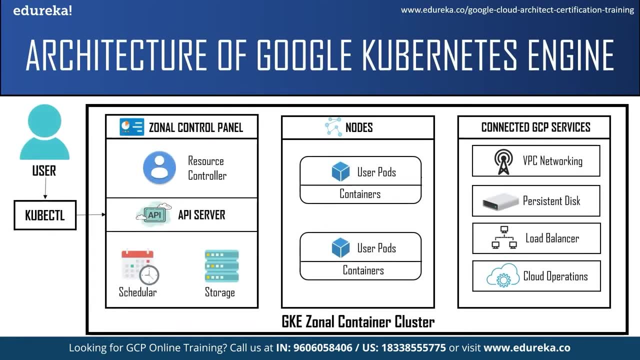 objects that represent your containerized application- all run on top of your cluster. Now to understand GKE better, let us understand its architecture and its working. As you know, all Kubernetes- objects that represent your containerized application- run on top of a cluster. 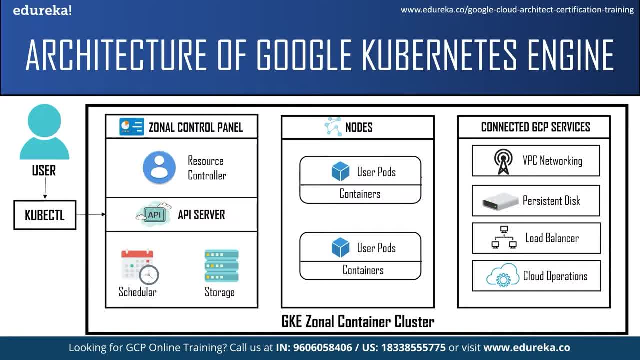 It is the foundation of GKE. a cluster consists of at least one control plane and multiple worker machines called nodes. These control plane and node machines run on Kubernetes cluster orchestration system. The control plane runs the control plane processes, including the Kubernetes API servers, scheduler and core resource controllers. The control plane is 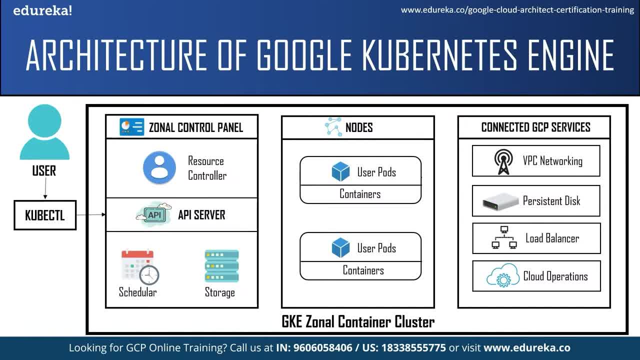 responsible for deciding what runs on each and every node. This can include scheduling workloads, like containerized applications, and managing the workloads, lifecycle, scaling and upgrades. The control plane also manages network and storage resources for those workloads. Now all the interaction with the clusters are done via Kubernetes, API calls and the control. 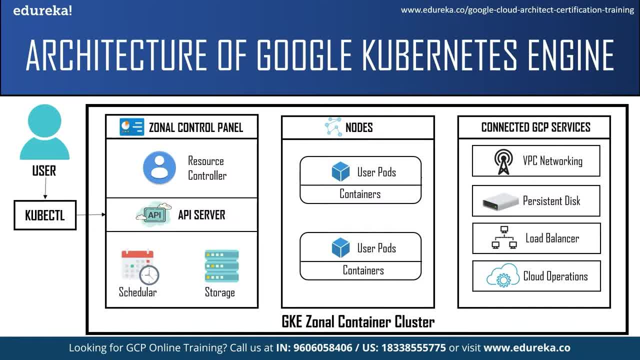 plane runs the Kubernetes API server processes to handle those requests. You can make Kubernetes API calls directly via http, slash, grpc, or indirectly by running commands from the Kubernetes command line client, that is, kubectl, or interacting with the UI in the cloud console. Now coming to the nodes: 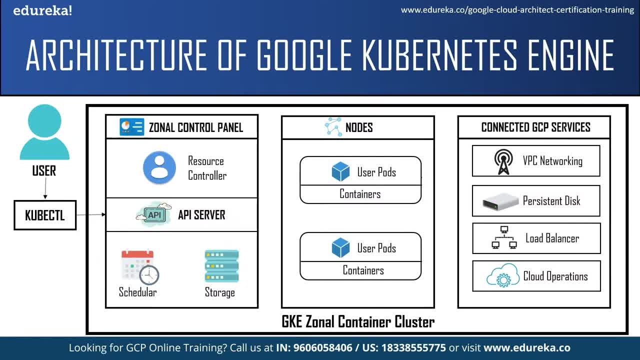 Now, nodes are the worker machine that run your containerized application, which is a containers and other workloads. They run the services that are necessary to support the containers running in workloads. Each node is managed from the control plane, which receives update on each node self-reported status. Next we have something called the user port. 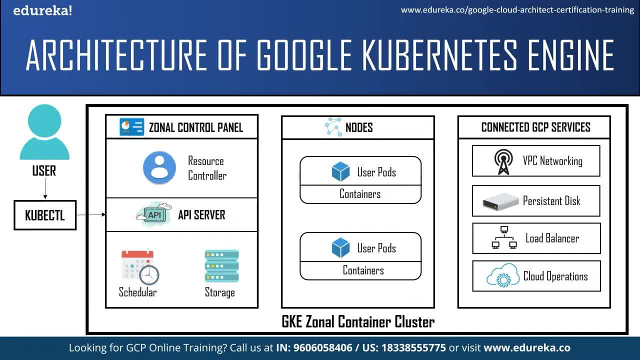 Now parts are the most basic and smallest deployment object in Kubernetes. It can contain one or more containers. So now, when the pod runs multiple containers, the containers are managed as a single entity and it shares the pods resources such as networking and storage. They're connected to various GCP services such as VPC networking persistent. 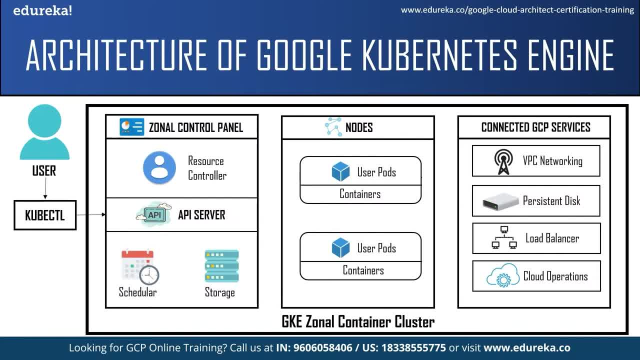 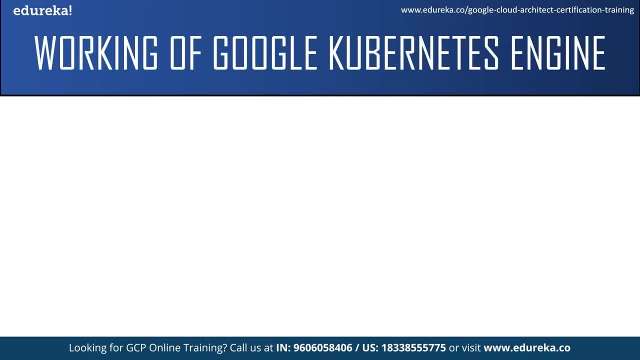 disk load balancer and other cloud operations. This was the architecture of GKE. Now let us understand it's working. GKE works with containerized applications. These containers, whether for application or batch jobs, are collectively called as workloads, And before. 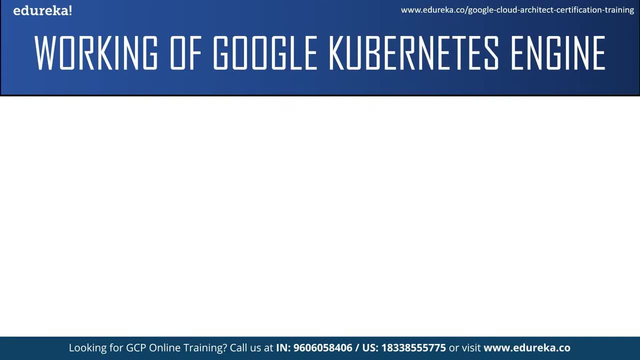 you deploy this workloads on GKE, you need to have a containerized, containerized application. To deploy the workloads on GKE, you must first package it into a container. Now to create a continuous integration and continuous delivery pipeline, you can use Cloud Code to write. 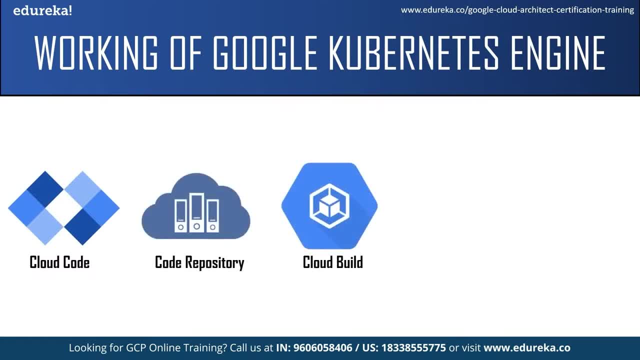 your application, then send the code to a repository which launches a build process in Cloud Build This build process build container images from a variety of source code repository. These container images are stored in container registry and are ready to be deployed in the Google Kubernetes engine. You can then create a GKE Cluster using Cloud Console UI- Gcluster. 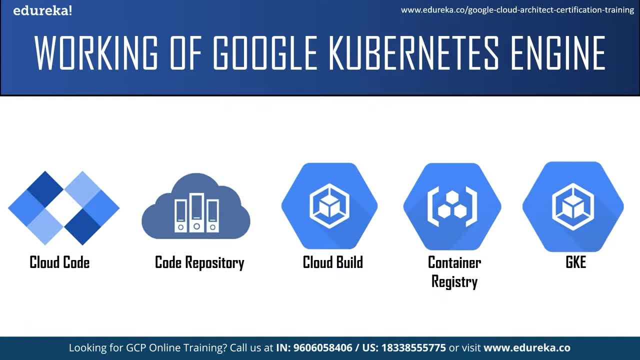 and the others. If you want to deploy all of your code files online, you need to be in the gcloud command-line interface or the apis. after this, with a few clicks, you can deploy your application on GKE. Now I guess you have some idea about Google Kubernetes engine. 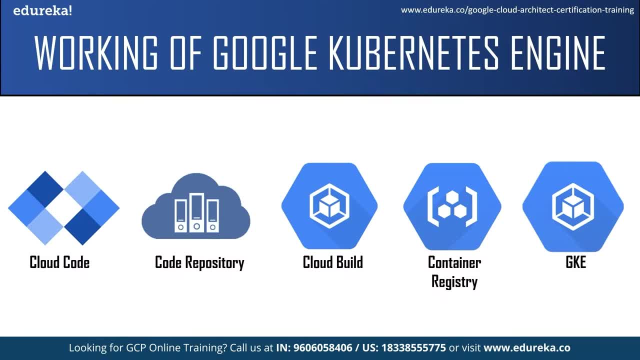 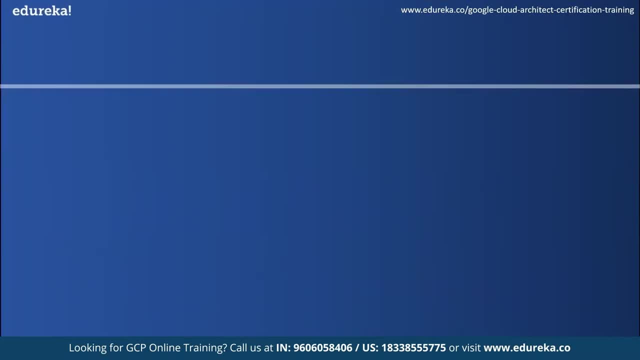 Now let us move on to the next topic and see some of the advantage of Google Kubernetes engine. with Google Kubernetes engine, You gain the benefits of advanced cluster management features that Google Cloud provides. first is load balancing for compute engine instance. Google Cloud offers server-side load. 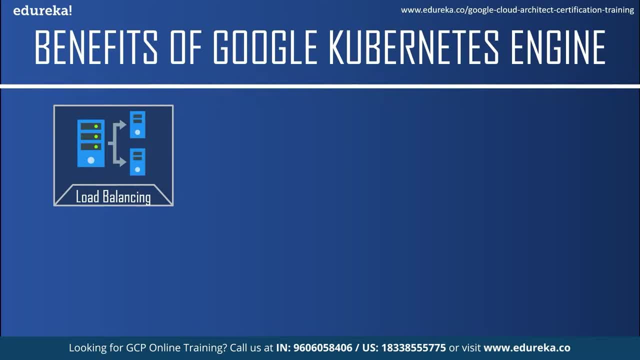 balancing so you can distribute incoming traffic across multiple virtual machine instances. load balancer can scale your application, support heavy traffic, detect and automatically remove unhealthy virtual machine instances using health checks and route traffic to the closest virtual machine. This is a managed service, which means its component are redundant and highly available. 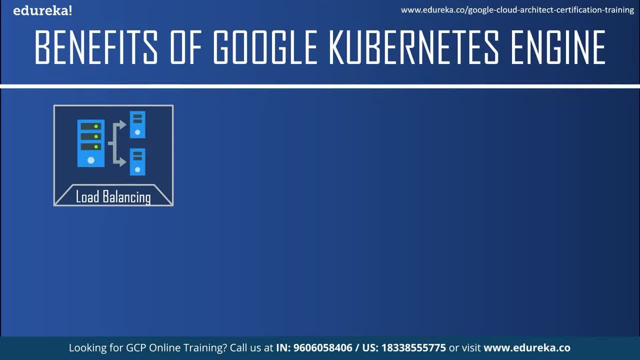 So if a load balancing component fails, it is restarted or replaced automatically and immediately. The next benefit is auto scaling. GKE's cluster autoscaler automatically resizes the number of nodes in a given node pool based on the demand of your workloads. You don't need to manually add or remove nodes or over provision. your node pools instead. 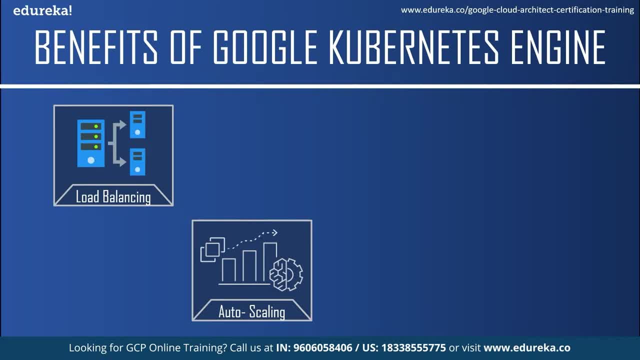 you specify a minimum and maximum size for the node pool, and the rest is automatic. The next benefit is auto updating. auto upgrades will help you keep the nodes in your cluster up to date with the cluster control plane version when your control plane is updated with auto. 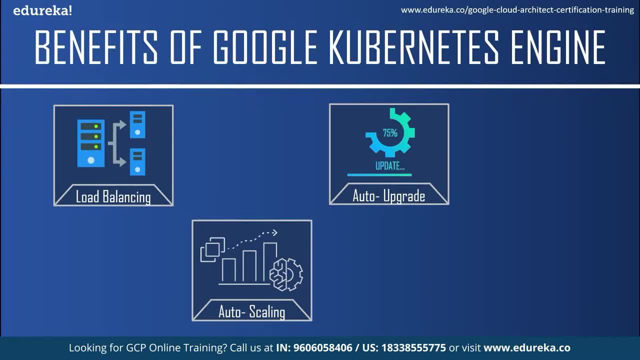 To update. you don't have to manually track and update your nodes when the control plane is updated on your behalf. It also provides better security by automatically ensuring that security updates are applied and kept up to date with the latest Kubernetes features. The next benefit is monitoring and logging. Google Kubernetes engine includes native integration. 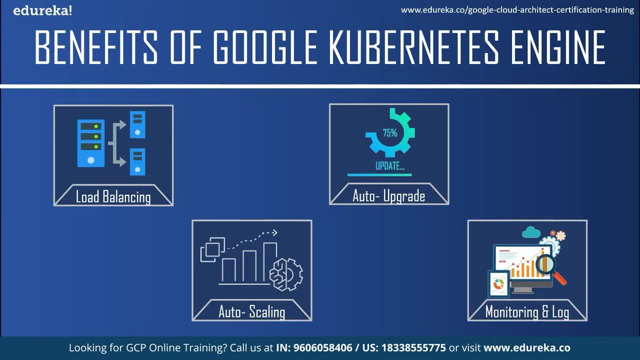 with cloud monitoring and cloud logging. When you create a GKE cluster running on the Google cloud, cloud operations for GKE is enabled by default And provides a monitoring dashboard specifically tailored for Kubernetes with cloud operations for GKE. you can control whether or not cloud logging collects application logs. 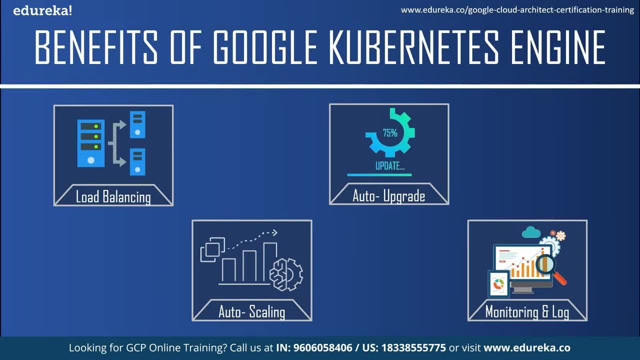 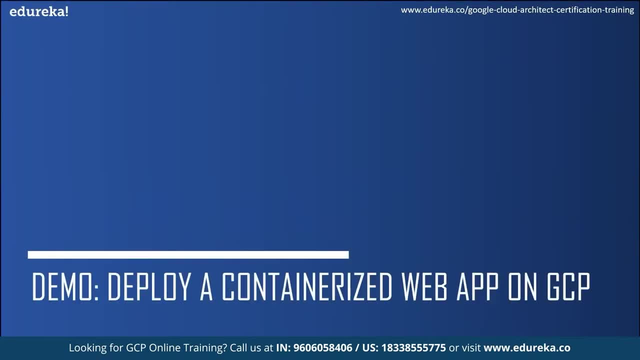 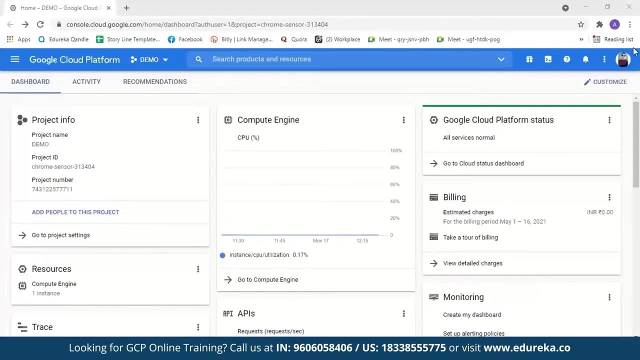 You also have the option to disable the cloud monitoring and cloud logging integration altogether. These were some of the benefits of Google Kubernetes engine. Now let us move on to a demo part and see how to deploy a containerized application on Google Cloud Platform. So now demo. we are going to package a sample web application into a docker container. 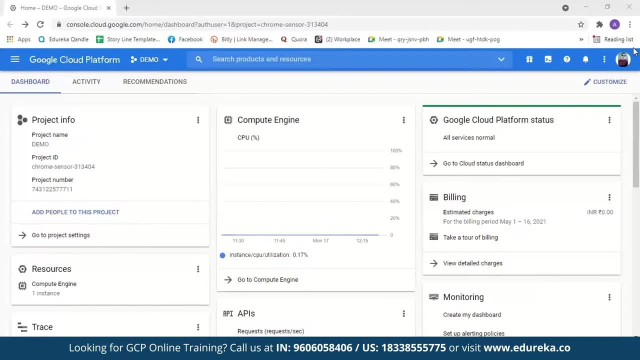 And then run that container image on a GKE cluster. So for that I've logged in into a GCP account. Now it is very simple to create a new GCP account. All you have to do is enter your debit card or credit card detail and give your address. 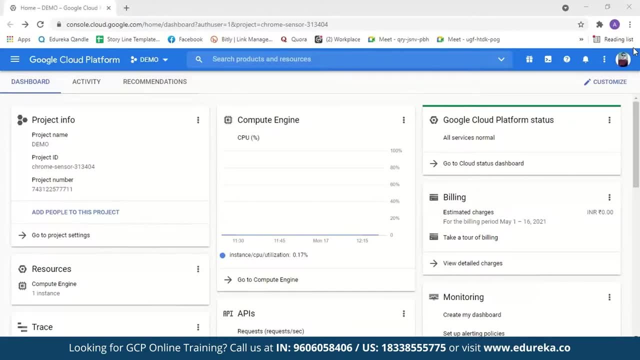 Then you might be charged maybe a rupee for it, But even that will be refunded later. Now, as you sign into a new account, GCP will provide you $300 of free credit. You can use this amount to explore Google Cloud services. You won't be charged until you choose to upgrade. 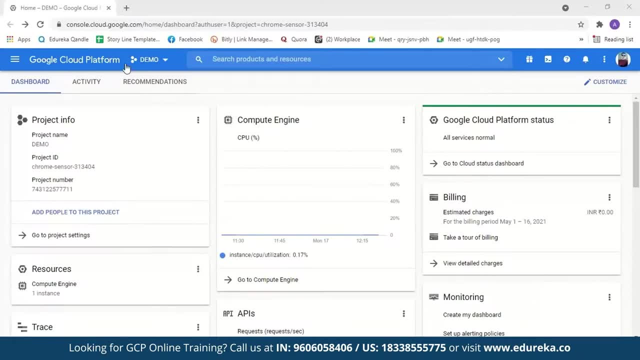 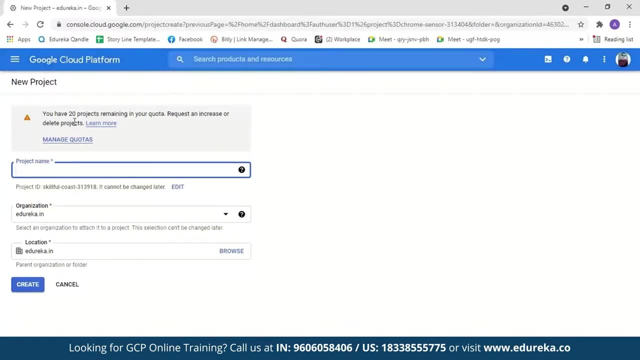 And it will be valid for 90 days. So first, let us create a new project. So we'll just go here, Select a new project. We can name a project anything we want, So we'll just name it Kubernetes. Let the rest be same and we'll just create it. 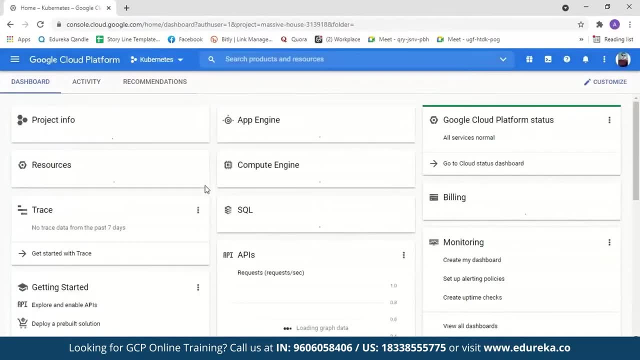 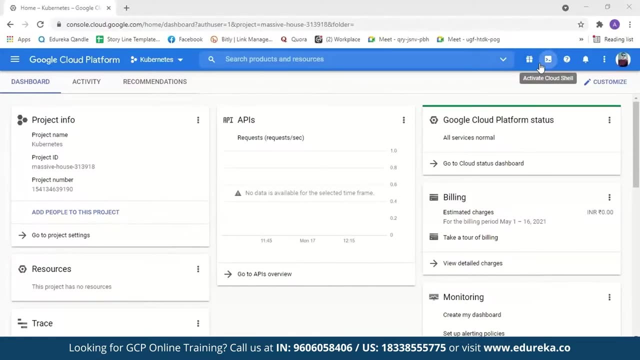 Now a project is created, we'll just select it. So for a demo, we're going to use Cloud Shell Now. Cloud Shell is an online development and operational environment. It can be accessed from anywhere with the browser. The reason we are using Cloud Shell is we do not have to install any command line tools. 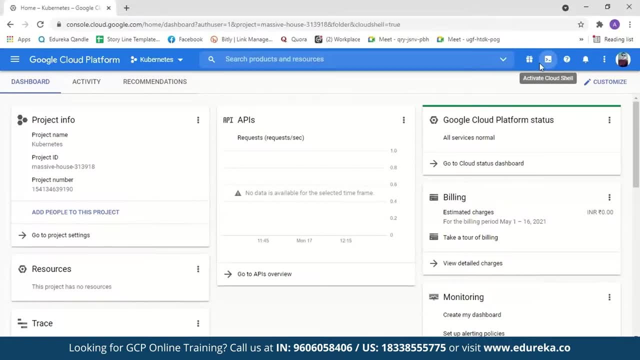 for a demo. So we'll just click on activate Cloud Shell over here And you can see a Cloud Shell terminal which is being created at the bottom of a screen. So the first step, as I've mentioned before, is to build a container image. 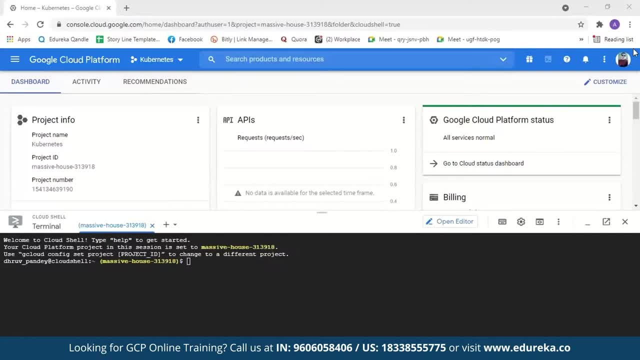 For this tutorial. We're going to deploy a sample web application Called hello app, which is a web server written in go programming language. It responds to all requests with the message Hello world on port 8080. before we deploy the hello app to GKE, we must package the 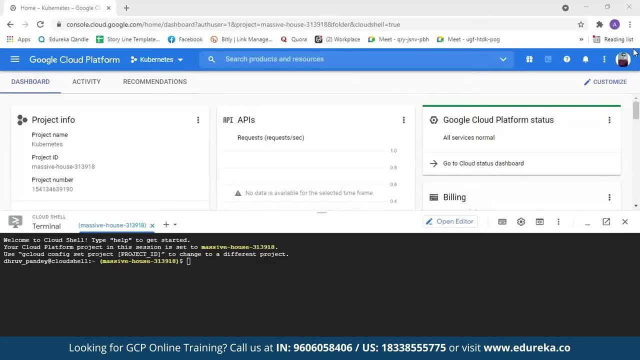 hello app source code as a docker image, and to do that we need the source code and the docker file. Now, the docker file contains information about how the image is built. So first let us download the source code and docker file for the hello app application. 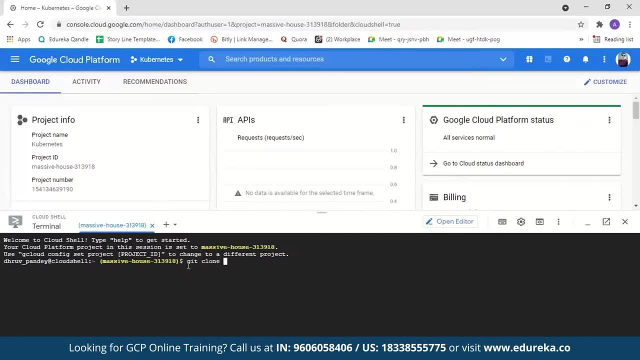 Get Hello App clone HTTPS, Githubcom, Google Cloud Platform, Kubernetes, engine samples. So the hello app application is available in this website, So we've just mentioned the website URL over here. Let's click on enter So it says that the directory already exists. 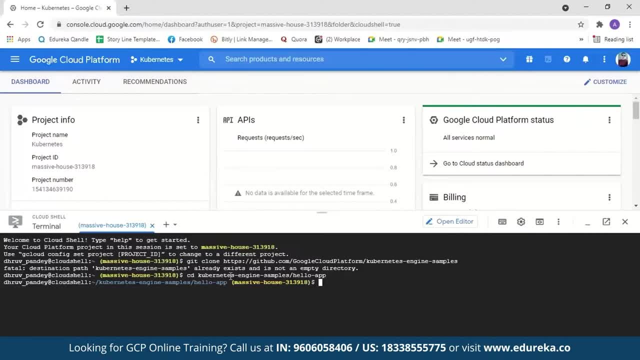 So we get a message saying the directory already exists, So we'll just change the directory. Next we have to set the project ID environment variable to the Google Cloud project ID. You can find the project ID over here, But I guess my project ID is the project ID. 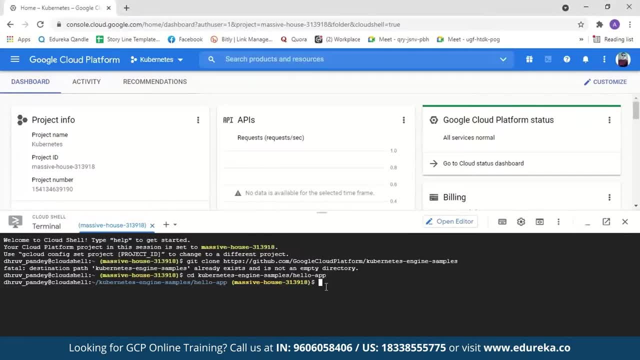 environment variable. So let's just confirm it. So for that we'll just type echo dollar sign. Next, you have to set project ID environment variable to a Google Cloud project ID. for that you have to type export Project ID is equal to. you can find your project ID over here: 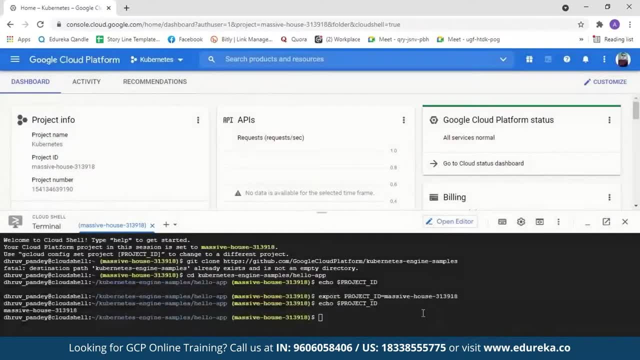 You can just copy it from here And paste it over here. the project ID variable associates the container image with your projects container registry. now to confirm a project ID, We'll just type Echo dollar project ID here. You can see this is a project ID. after confirming the project. 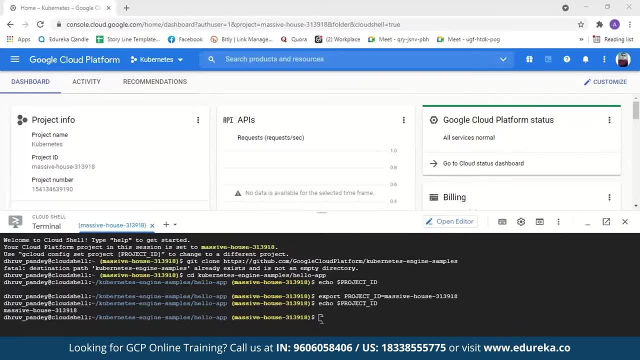 ID. It is time to build docker image for the hello app, So for that will type Docker, build space. I've been T space, GCR, dot, IO, slash dollar project ID. slash hello app version one. Now, this is a name given to a docker image and GRE refers: 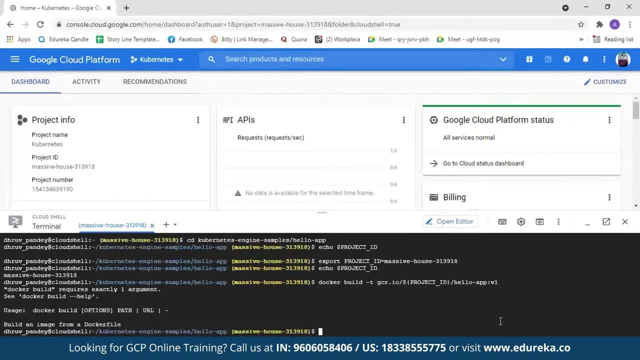 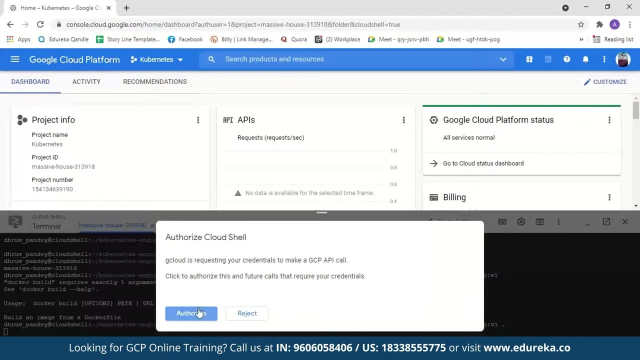 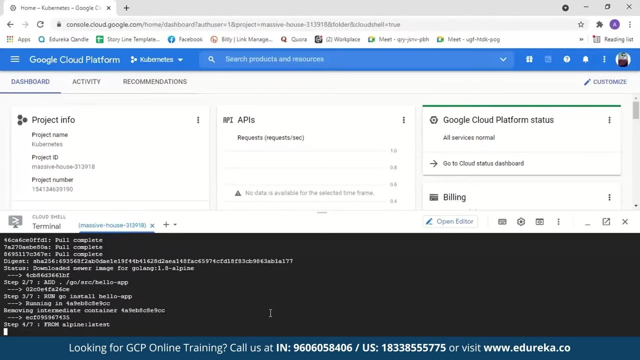 to the container registry. We just forgot one more thing over here. that is space a dot. now it will ask you to authorize cloud shell. You can just select authorize over here. You can see a docker Image is being created. We just extend this. 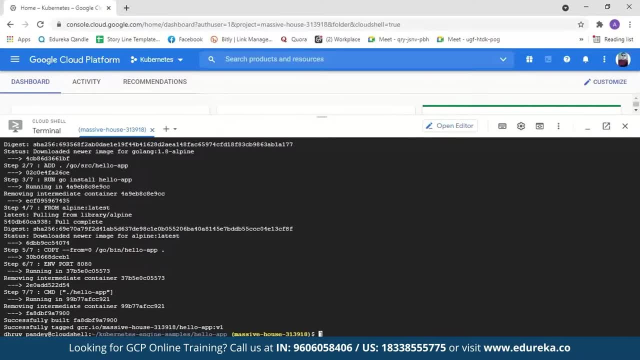 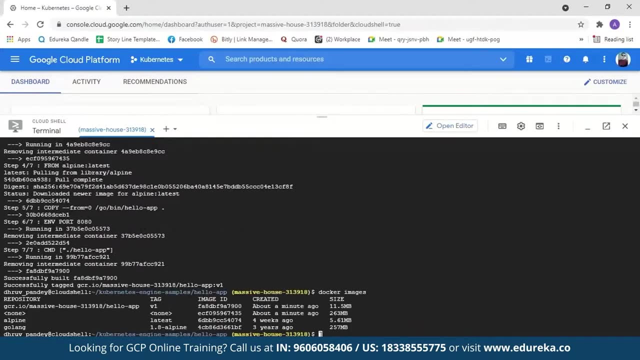 You can see our docker image was successfully built. How to just confirm if a docker image was built with just type Docker images. Now you can see a docker image is built. It was created a minute ago and the size of it after this. 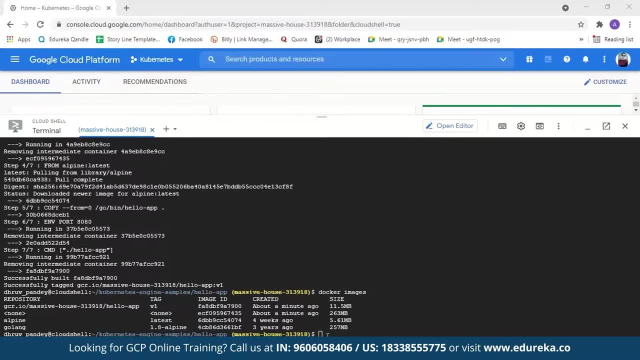 We have to push a docker image to the container registry So GKE clusters can download it and run the container Image. So for this we are going to enable the container registry API will just type G cloud Services. Enable Container registry dot. 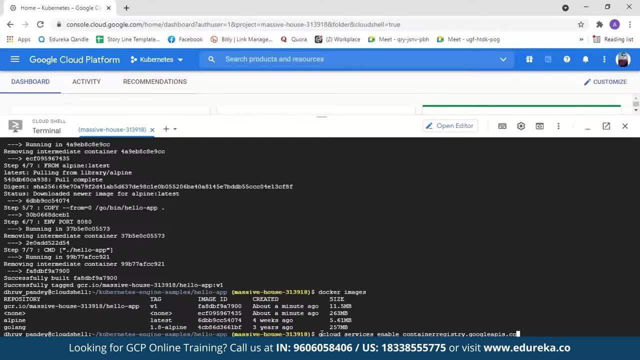 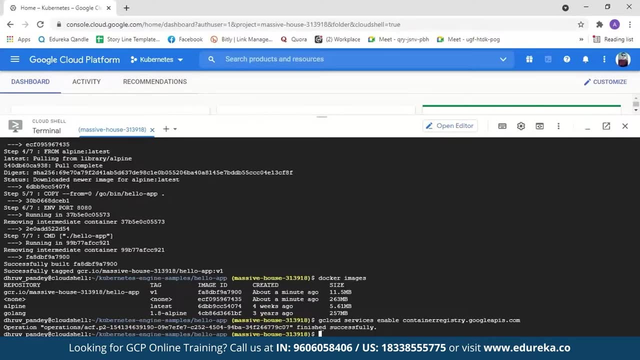 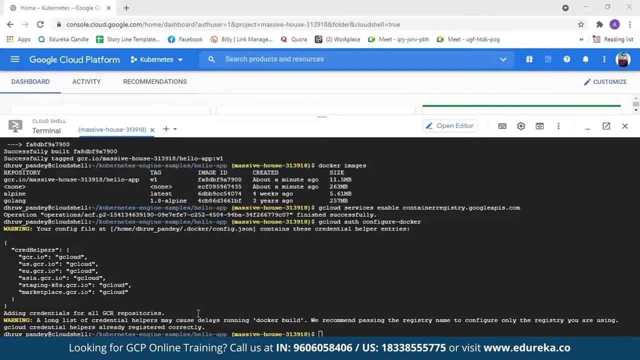 Google API is Dot com. Next, we have to authenticate to container registry by configuring the docker command line tool. for that We're going to type G cloud Authenticate, Configure Docker. Now, this is just a warning message saying that we have a. 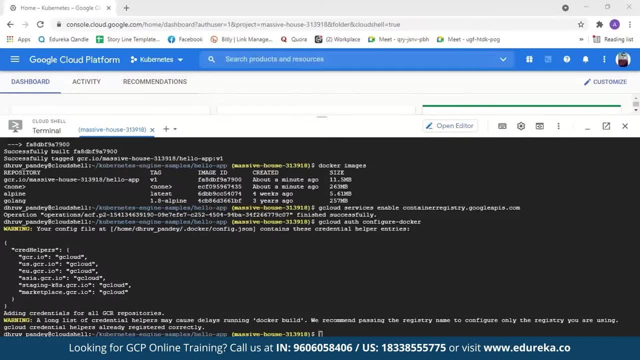 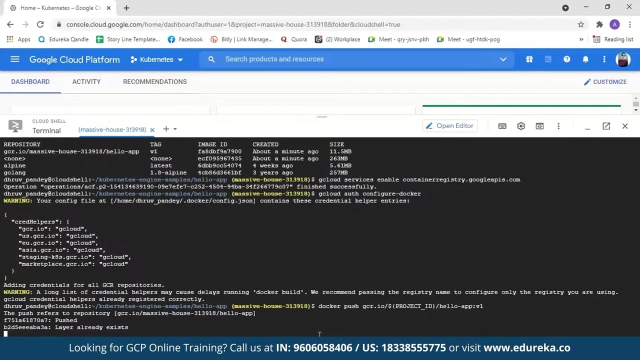 lot of credential and it might be slow. So now we have authenticated our container registry, Now we have to push the docker image to the container registry. So for that we're going to type Docker, push- The name of our docker image. Now a docker image is being built in the container registry. 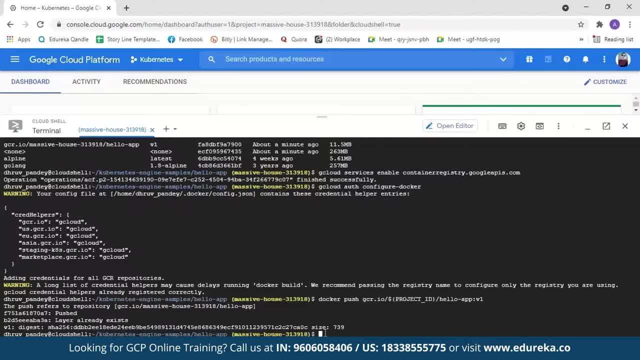 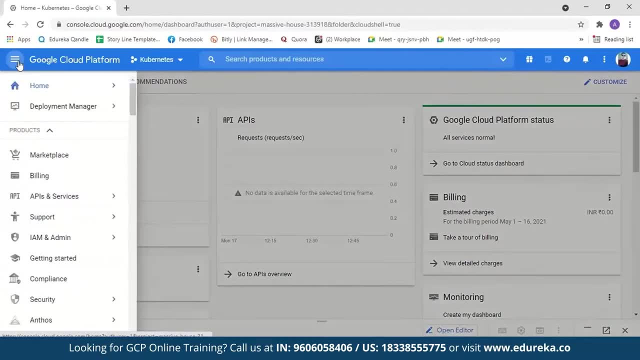 Now you can see a docker image is pushed to our container registry. Now the next step is to create a Google Kubernetes engine cluster. So for this we're just going to minimize it and just go to Kubernetes. You can either select Kubernetes engine from here or you can. 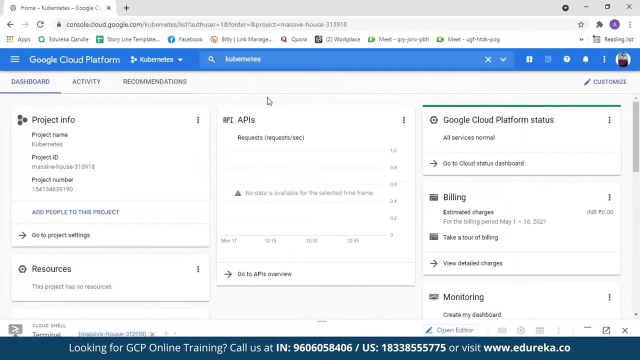 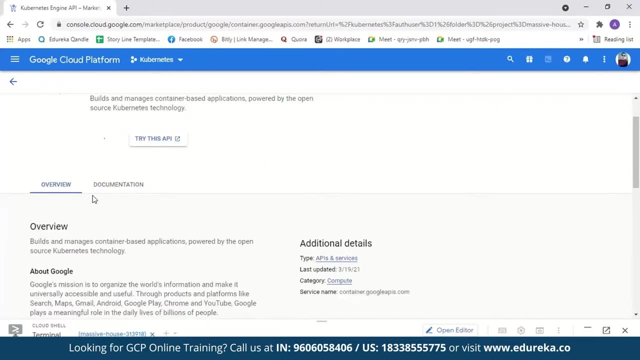 just type Kubernetes over here: Kubernetes engine. We just click on enable over here. Now this might take a couple of seconds. You can scroll down and read our overview about it. We can read about Google and the various other products which are offered by them. 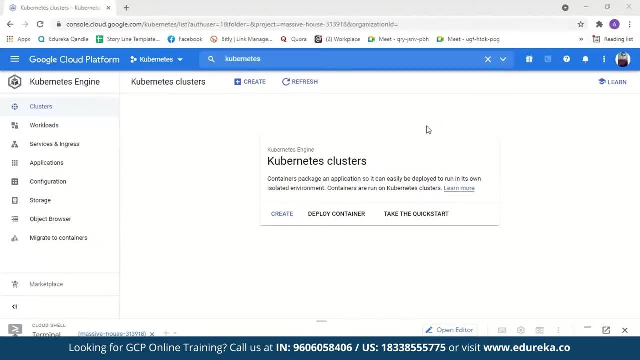 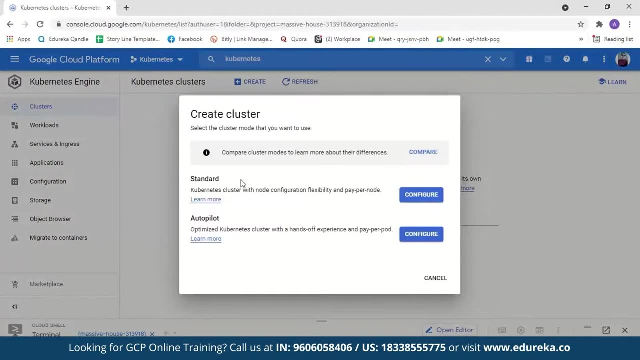 Now, this is what the Google Kubernetes engine console would look like, So it'll ask us to first create a Kubernetes cluster, So we'll just go ahead and create one Now. we have two options over here when the standard and the other one is autopilot. 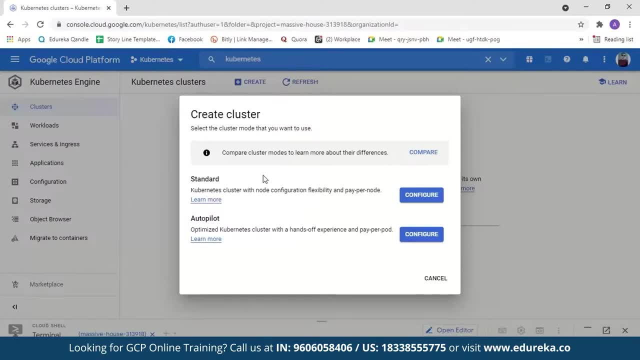 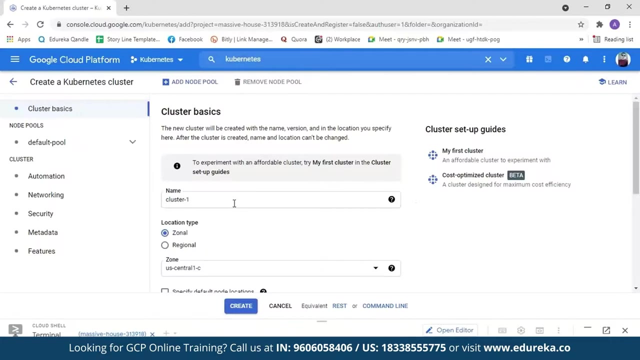 In standard, you manage your clusters underlying infrastructure, which will give you node configuration flexibility and in autopilot, GKE provisions, and manages the clusters underlying infrastructure. So we'll just go with standard over here and click on configure So we can name our cluster whatever we want. 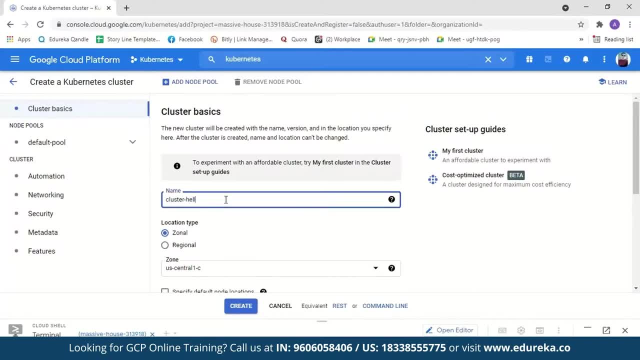 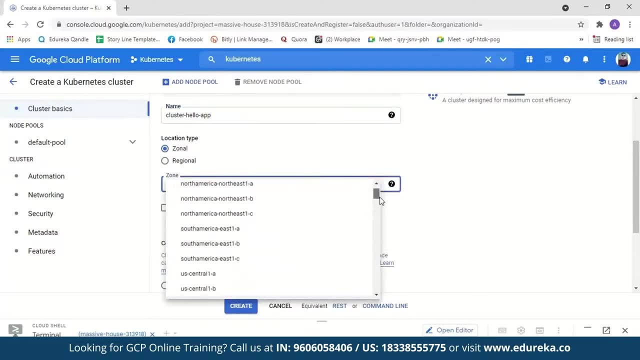 We'll just name it Cluster Hello app. You can select any zone from here. These are the available zones, So we'll just select a maybe us-west one. Now you can select the zone which is nearest to you. You can select the version which is go to static version. 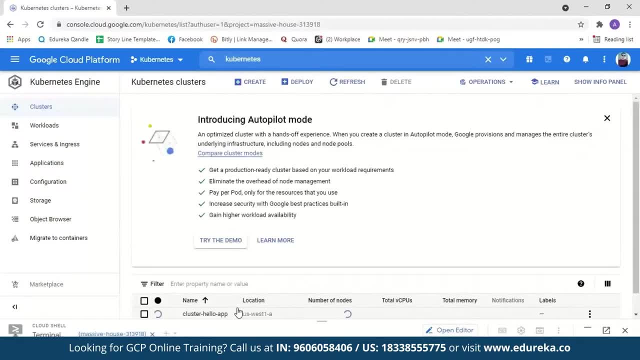 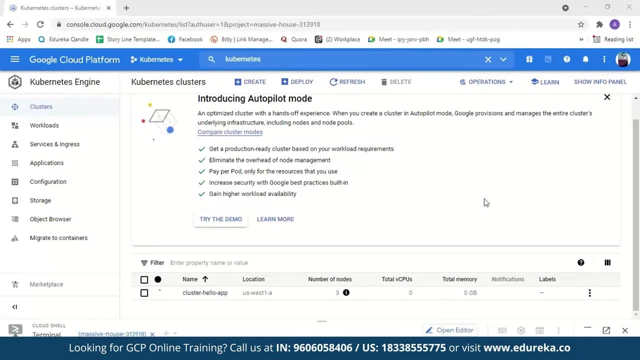 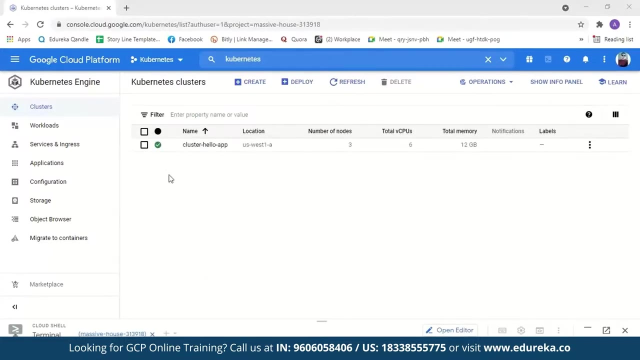 and just create a cluster. Now. creating a cluster might take a couple of minutes, So we'll wait for some time and refresh it to see if it is created or not. You can see there is a green tick over here, which means our cluster is successfully created. 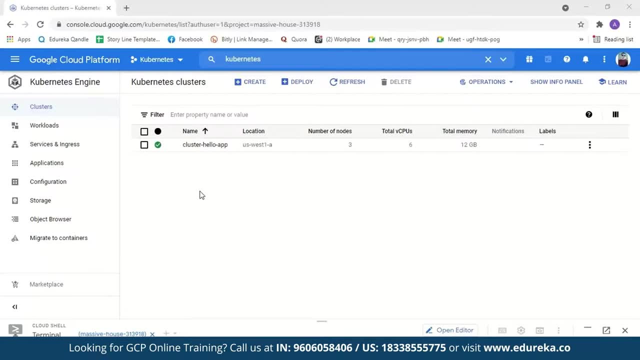 We have already pushed the docker image to a container registry. The next step is deploying the sample application to Google Kubernetes engine. for this step You have to create a kubernetes deployment to run the application on the cluster and also create something called the horizontal pod autoscaler, which scales the number of pods. 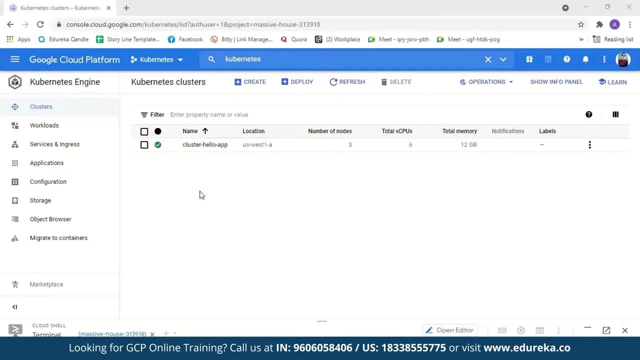 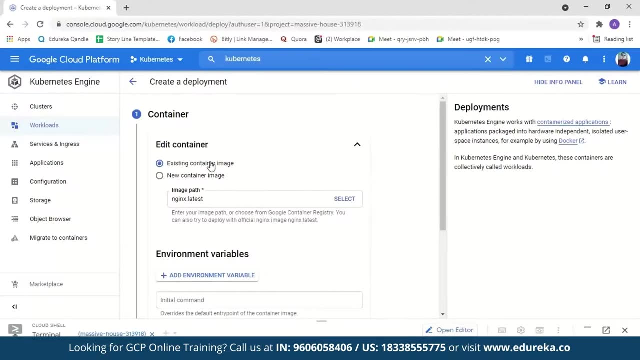 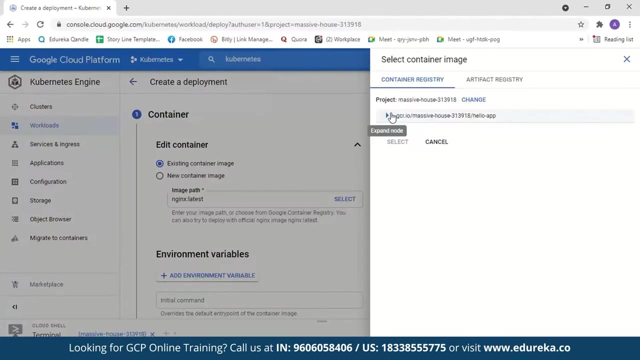 It can be anywhere from 1 to 5 based on the CPU load. So for that we'll go to workloads. Click on deploy. We have an existing container image, So we'll just select it. go to select. This is a project ID and this is the name of the docker image. 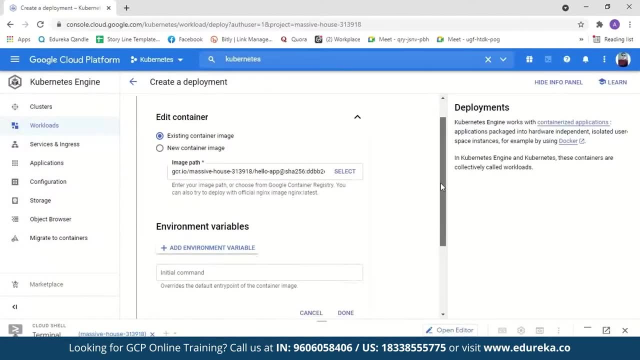 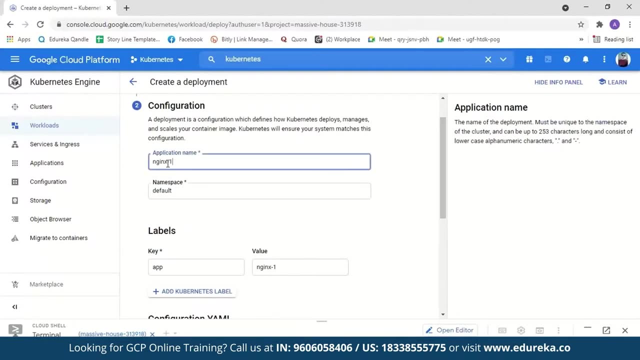 So we'll just expand it and select this. A docker image is selected, Click on continue and we have to configure it so we can name our application anything we want. So we'll just name it: Demo application. We let the namespace be default. 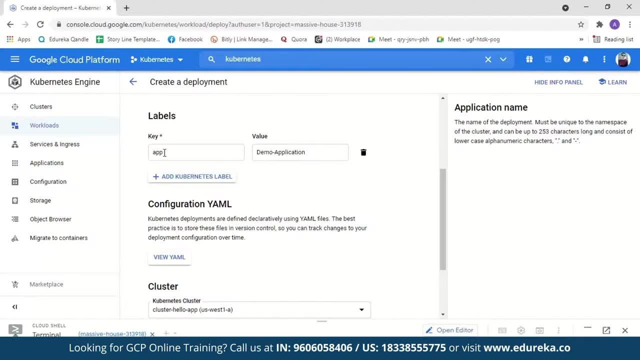 Next, we have label, which is basically for identification, So let the key be app and the value be demo. application will not make any changes in that, and this is our cluster on which the demo application is going to be deployed. Now, when we see the yam, 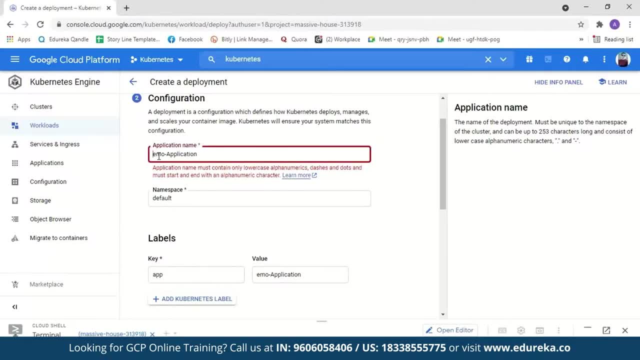 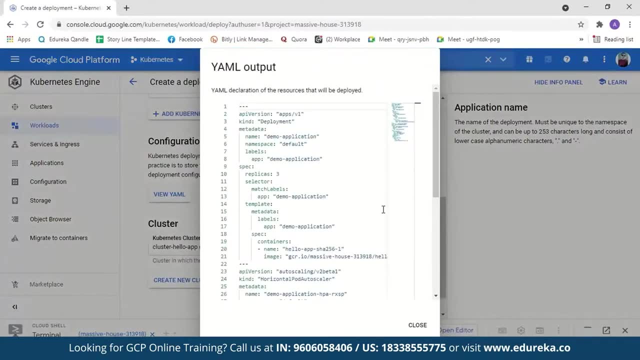 Okay, so we have a error here. We cannot use uppercase, So we'll just make it lowercase. demo application. Now, when we see the yaml file, you can see two kubernetes API resources About to be deployed into your clusters. The first one is deployment. 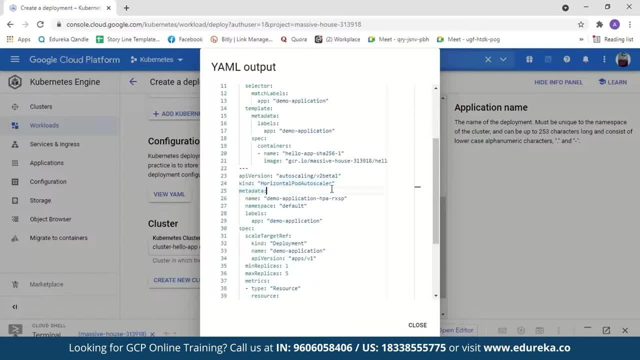 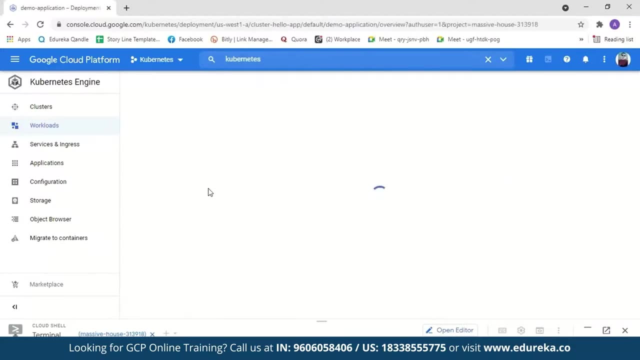 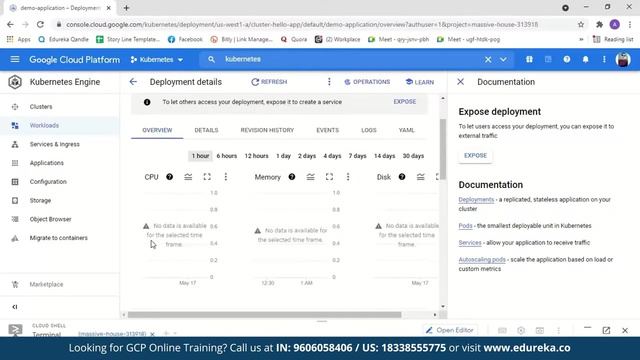 And next is the horizontal pod autoscaler. Next we'll just click on deploy And our deployment is being created now. This might take only a couple of seconds. Here You can see the CPU usage, memory usage and a disk usage, but as of now there is no data available. 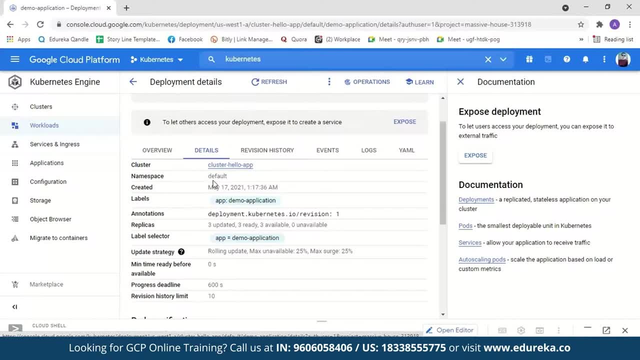 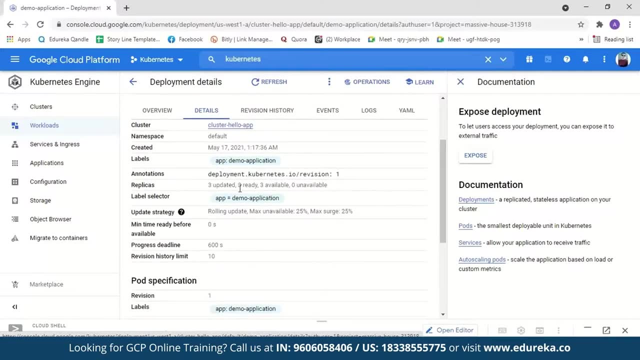 Now, if you go to details, you see a cluster name, the namespace which I have mentioned. When was it created and at what time. the labels: how many replicas were made. there were three replicas which are made, So after the deployment we are going to expose the sample. 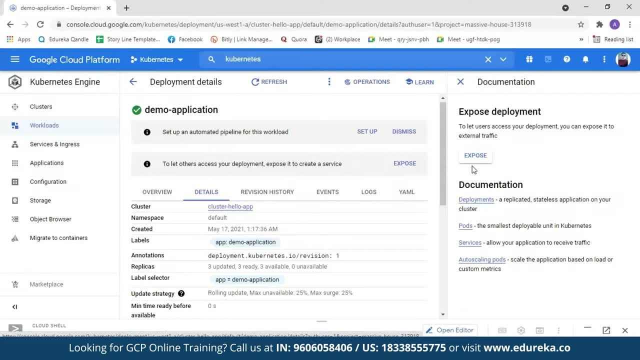 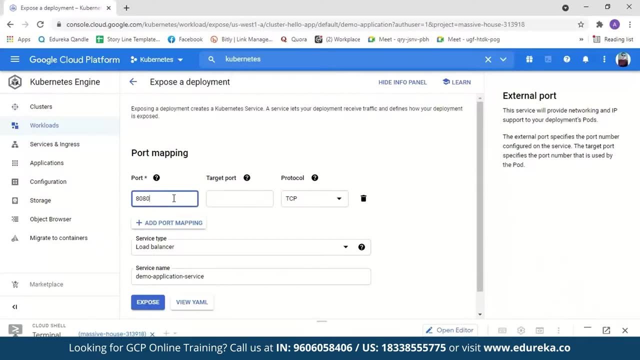 application to the internet. So for that we have an option here called as expose. So we'll just click on this in the target port will select 8080.. Now this is the port the hello app container listens to, as I had mentioned at the starting of the demo, the service type: 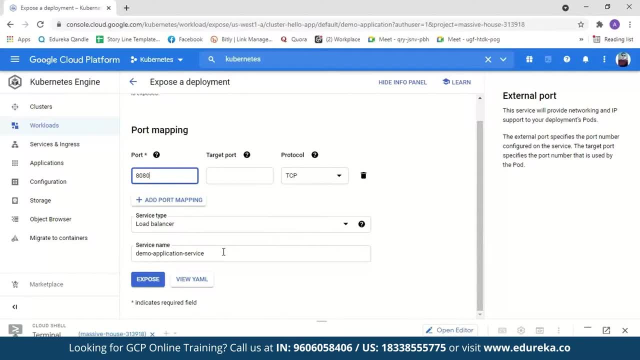 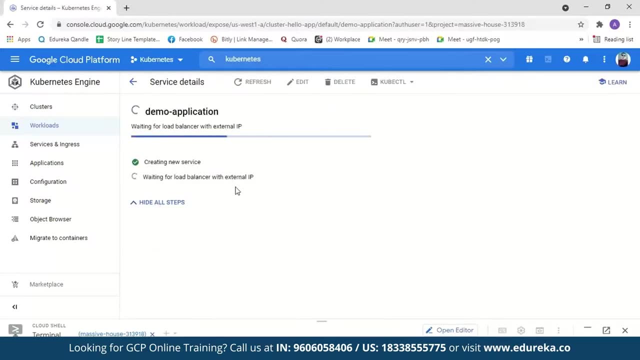 Let it be load balancer itself, and we can name our service anything We want. let it be demo application service itself, and we're just going to click on expose over here. Now, a new service has been created and it is waiting for a load balancer with an external IP to be created. 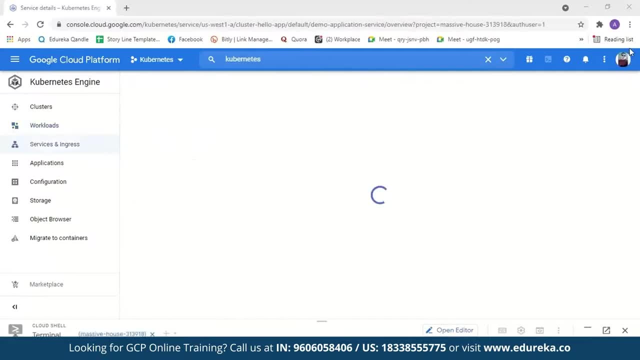 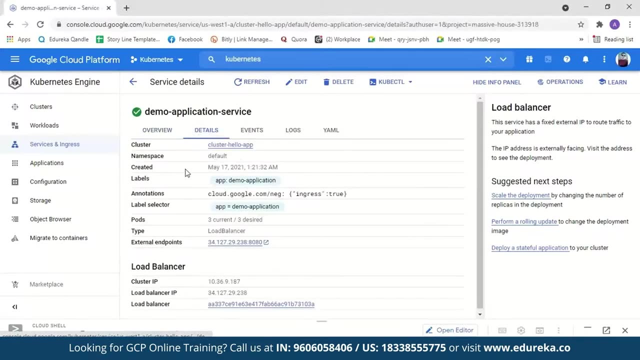 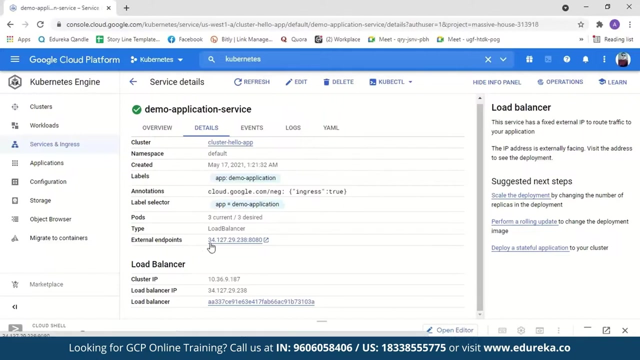 Now this might also take a couple of seconds. Now a service has been created, So when we go to details, you can see the cluster name, the namespace, when was it created, the label, the ports, the type, load balancer and external endpoint. So we'll just click on this or you can just copy this and 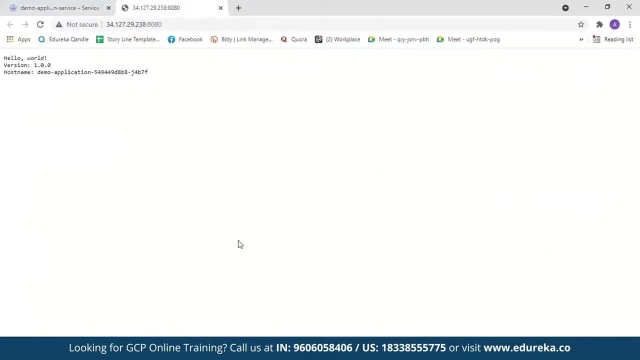 paste it in the new tab. So when I click on this, we are directed to a sample application. So here is a sample web application. Now you see, a sample application is exposed to the internet through Kubernetes service, and here is the hello world message. 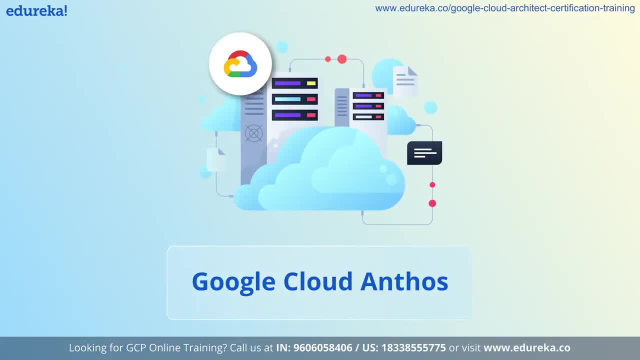 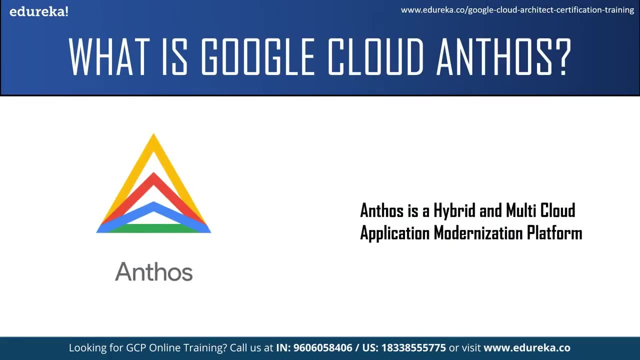 with the version and the host name. What exactly is Google Cloud? and those and those is a hybrid, A multi-cloud application modernization platform. It was launched in June 2019 and can help in rapidly building hybrid and multi-cloud application without compromising on security, as well as not increasing the complexity. 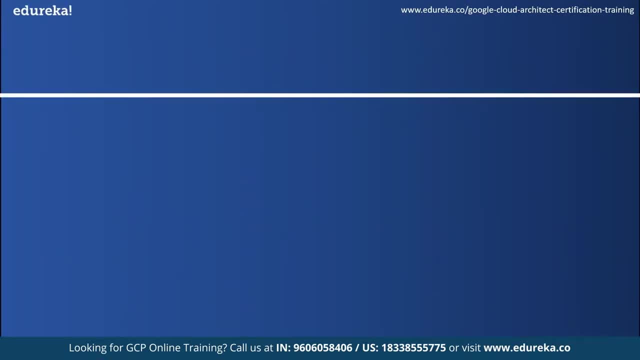 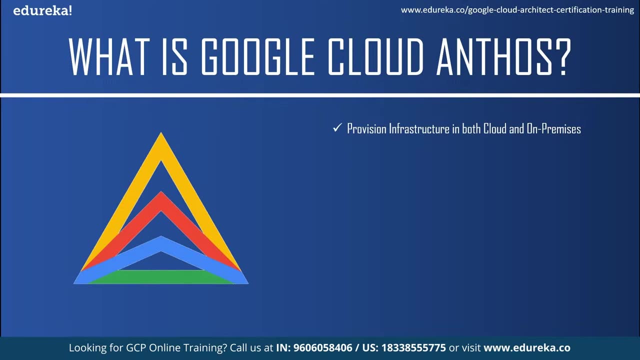 Now, if you're wondering what Anthos can be used for, here are a few cases where you can use Anthos. Firstly, it helps in provisioning infrastructure in both cloud and on-premises as well. Next, it provides infrastructure management tooling security. 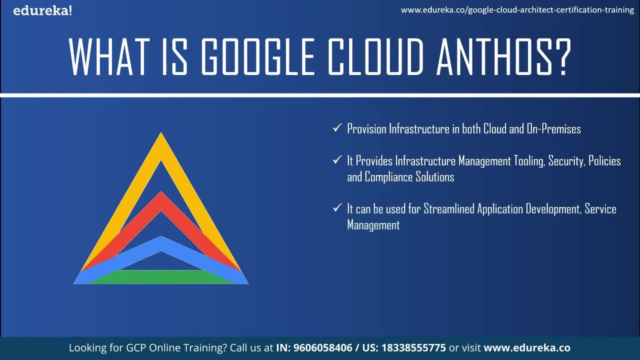 policy and compliance Solutions. It can also be used for streamlined application development, service management and workload migration from on-premises to the cloud. Next, one of the core functionality of using Anthos is to easily deploy container-based application in a hybrid or multi-cloud. 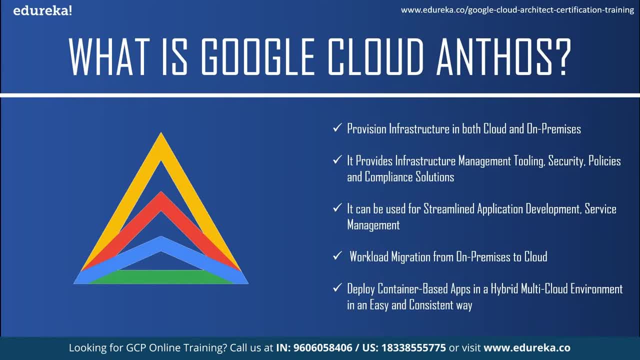 environment in an easy and consistent way. clients can choose from various deployment options, such as on-premises bare metal, Google Cloud platform, AWS or Kubernetes clusters. Google Cloud Anthos allows developer to focus on Innovation and create new features, software or products for the company instead. 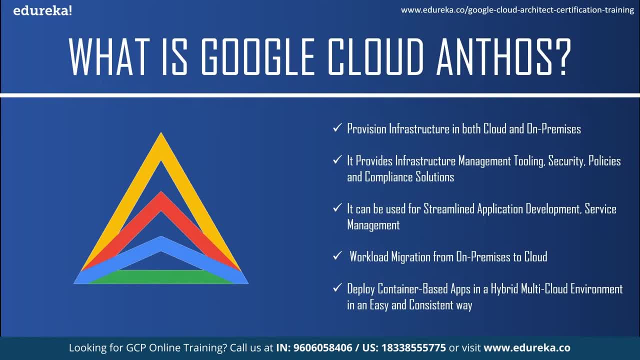 of spending time on managing complex hybrid environment. This will be taken care by Google Cloud Anthos. Now I guess you have some idea about what Google Cloud and those can be used for. in order to understand Google Cloud Anthos better, Let us take a look at its components. 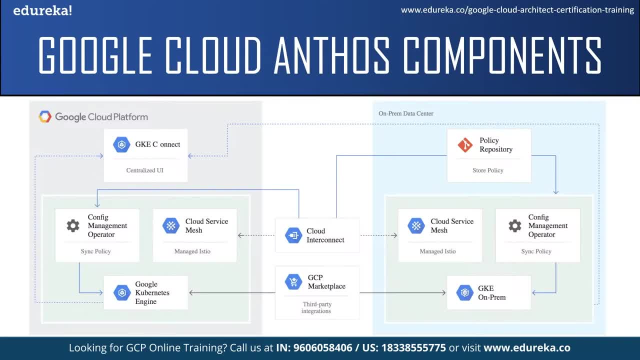 Basically, Anthos is a platform composed of several technologies integrated together, rather than a single product. It is powered by Kubernetes, Along with other technologies like Google Kubernetes engine, Google Kubernetes engine, on-prem, Istio service, mesh and others. Let us talk about each of these components one by one. 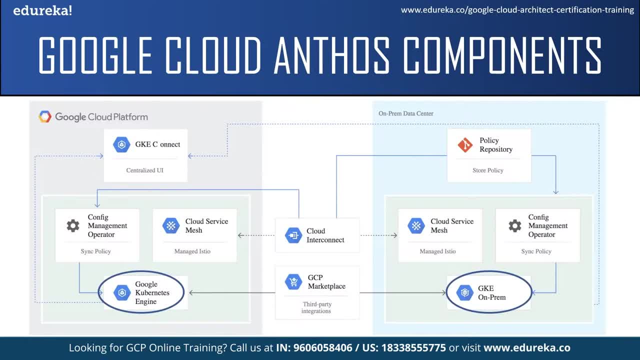 Now the Google Kubernetes engine and Google Kubernetes engine on-prem are the main computing components which enables Anthos. now GKE is nothing but a managed environment for deploying, managing and scaling containerized application using the Google infrastructure. Now, if a company already have the data center or the IT infrastructure, 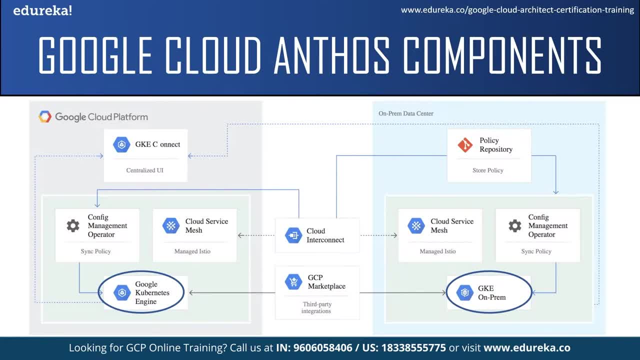 they can use GKE on-prem, which will provide them all the benefits of GKE, like Auto updates, Auto node repair and many more. then, to connect the on-premises data centers and workloads on GCP, There is Google Cloud interconnect now Google Cloud interconnect. 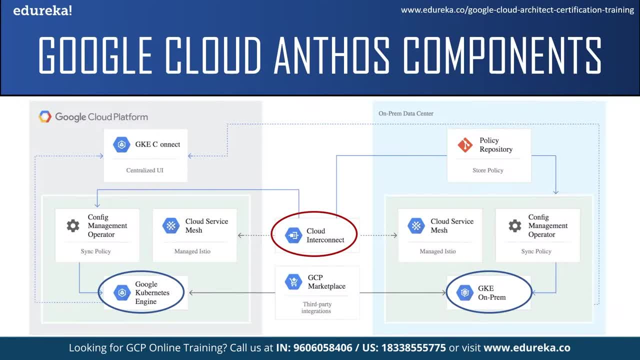 is a service which provides direct connectivity between on-premises data centers and the workloads on Google Cloud platform with consistent latency and high bandwidth. now Google Anthos service mesh enables fully managed service meshes for complex microservices architecture, Which would include traffic management mesh, telemetry and securing. 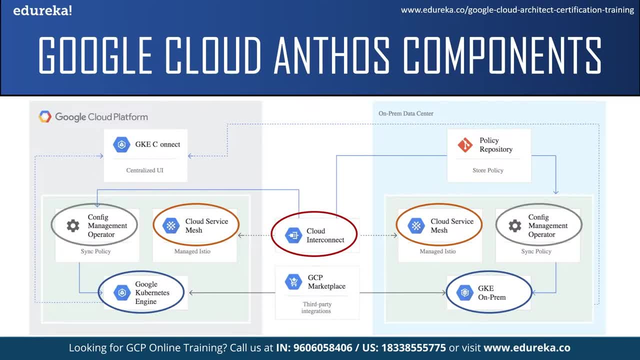 service communications, and with Anthos config management, you can create configuration which will allow you to easily and consistently manage your resources globally across clouds and data centers. next, the GKE connect allows you to register GKE on-prem based clusters to the GCP console. 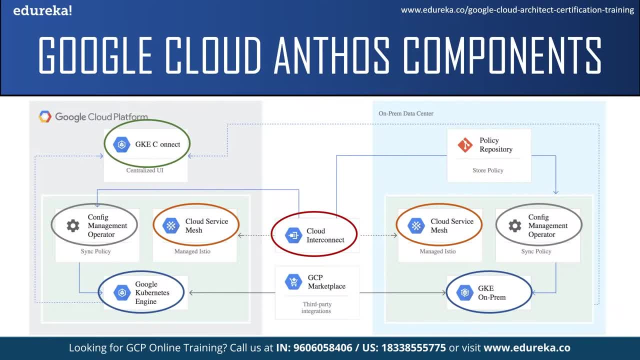 This can help in securely managing the resources and workloads running on them together with the rest of the GKE clusters. This can be enabled by installing the GKE Connect agent organization can simultaneously migrate the virtual machine applications to Google Kubernetes engine with Anthos migrate. 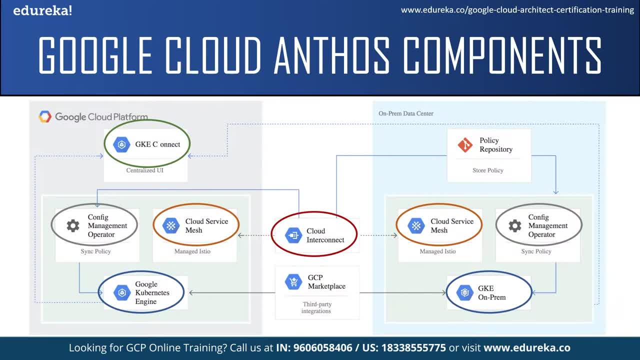 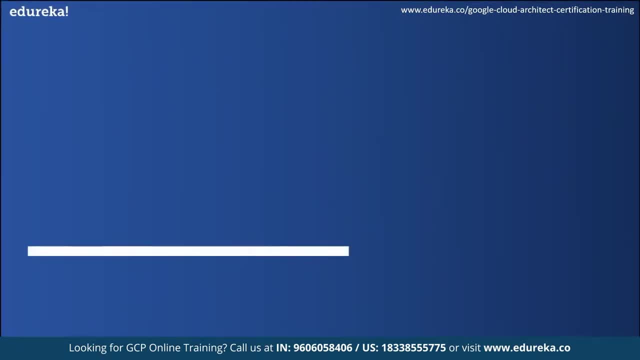 So the apps can be run and managed through GKE with is your service mesh capabilities. So now I guess you have some idea about Anthos components and what is Anthos. Let us move on to the next topic and see some of the features of Google Cloud Anthos. 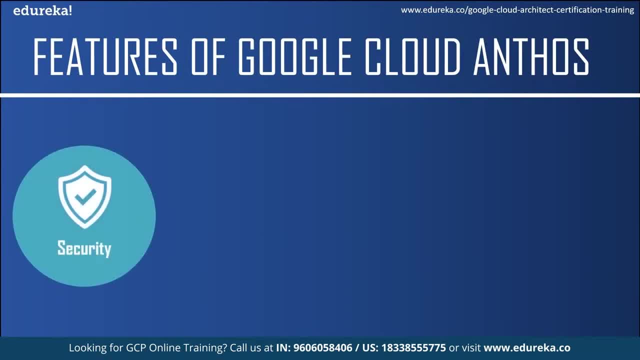 The first feature is Google Cloud Anthos integrate security into each stage of application lifecycle, from developing to building and running. Anthos enables defense in-depth security strategies with a comprehensive portfolio of security control across all the deployment models. The next feature is it offers a fully managed service mesh with 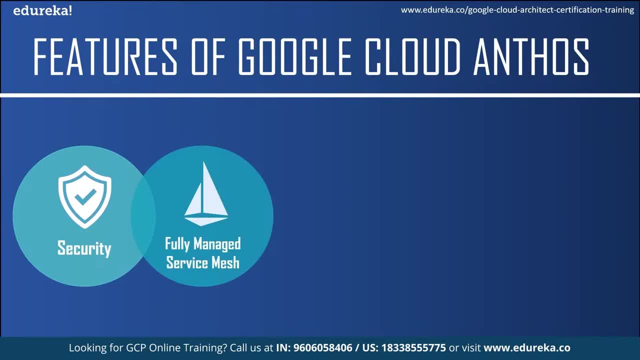 built-in visibility. Google Anthos service mesh unburdens the operational and the development team by empowering them to manage and secure traffic between services, while monitoring, troubleshooting and improving application performance. The next feature is it provides container orchestration and management service. Google Cloud Anthos enables you to run Kubernetes clusters. 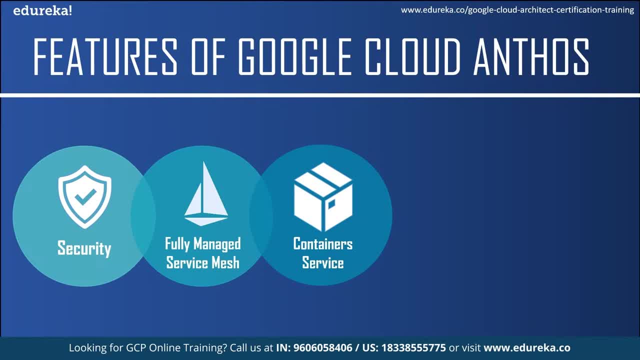 anywhere in both cloud and on-premises environment. Anthos can also run on your existing virtualized infrastructure and bare-metal servers without a hypervisor layer. It simplifies your application stack, reduces the cost associated with licensing a hypervisor and decreases time spent learning. 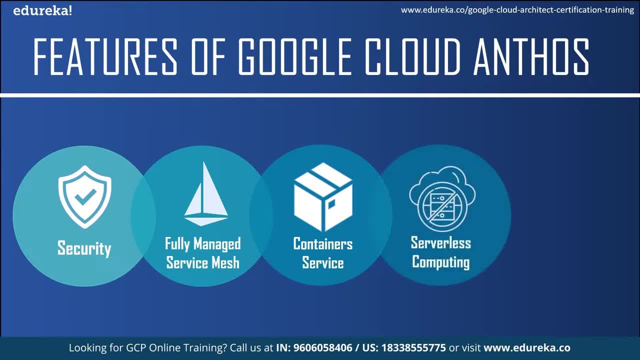 new skills. The next feature of Google Cloud Anthos is serverless computing. Anthos provides a serverless deployment platform called Cloud Run for Anthos, which allows you to deploy workloads to Anthos cluster running, on-premises or on Google Cloud, all with the same consistent. 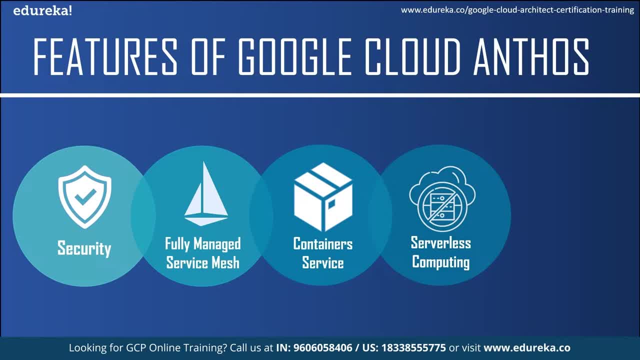 experience. Cloud Run for Anthos is powered by native, which is an open-source project that supports serverless workloads on Kubernetes. The next feature is migrating existing workloads to containers. You can use the migrate for Anthos service that minimizes the manual effort required to move and convert existing application. 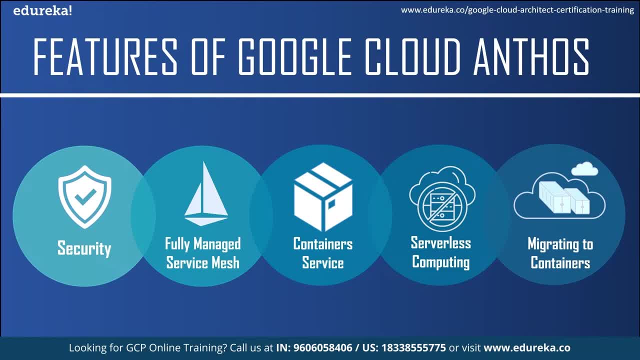 into containers. with migrate for Anthos, You can easily migrate and modernize your existing workloads to containers on a secure and managed Kubernetes service. These were some of the features of Google Cloud Anthos. Now let us move on to the next topic and see some of the benefits. 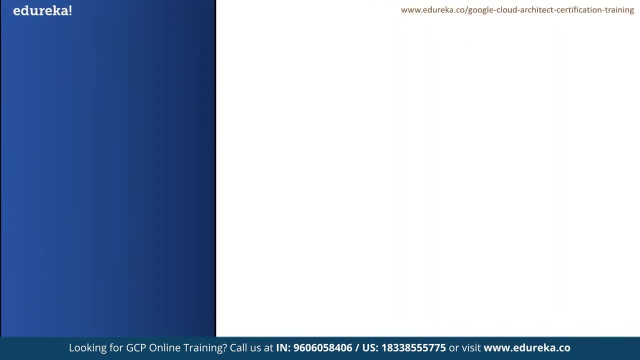 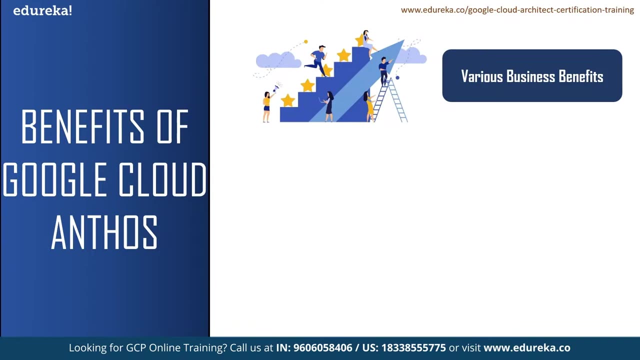 of using Google Cloud Anthos. The first benefit is it provides various business benefits. Now, according to a Forrester Research Anthos report, which is commissioned by Google, It was found that overall Anthos business benefits include operational efficiency, developer productivity and security productivity. 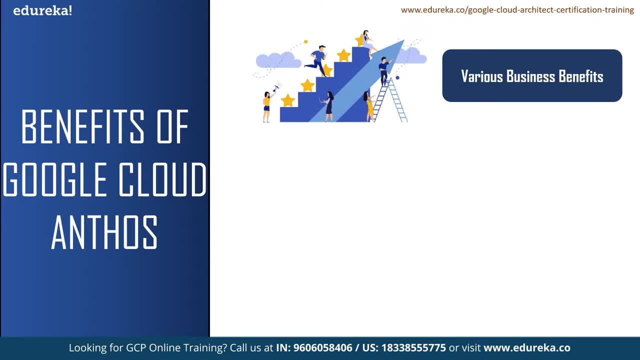 On an average, organization saw 4.8 times return of investment within three years of adopting the Anthos cloud platform. The developers can use this platform to quickly and easily build and deploy existing container based application and microservices based architectures. They can use git compliance management and CICD workload. 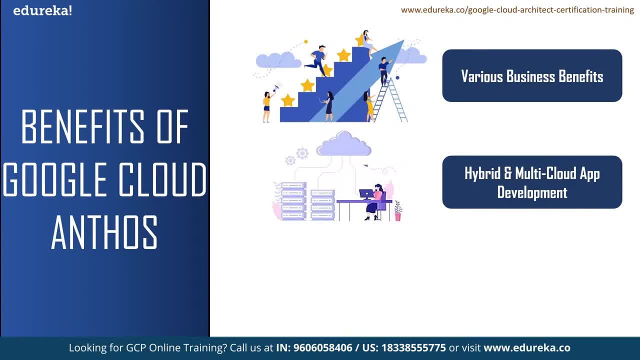 for configuration as well as code using Anthos configuration management. It also supports for Google Cloud Marketplace To easily and quickly deploy functional software packages or products into clusters. The next benefits of Anthos is it provides enhanced security. Anthos protects apps with high standard for reliability. 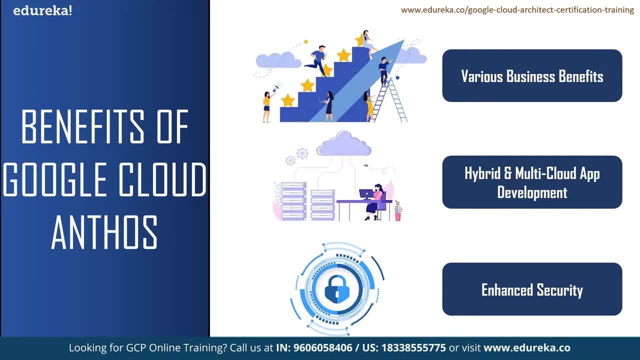 availability and vulnerability. from a security perspective, Anthos also offers a high level of control and alertness for your services: health and performance with a comprehensive view. Now these were just some of the benefits of Google Cloud Anthos, And let us take a look at the pricing of Anthos. 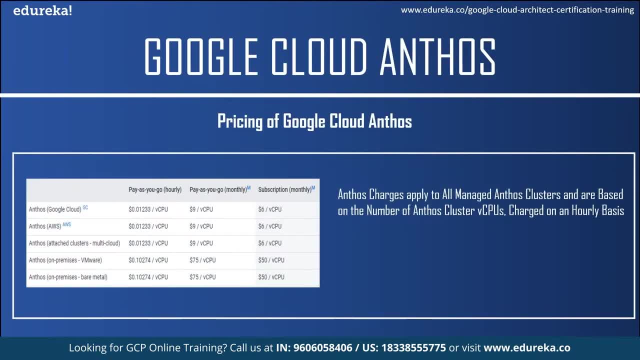 Anthos charges applies to all managed Anthos clusters and are based on the number of Anthos clusters- virtual CPUs- charged on an hourly basis. There are two types of pricing option for Anthos. The first one is pay-as-you-go pricing model. where you are 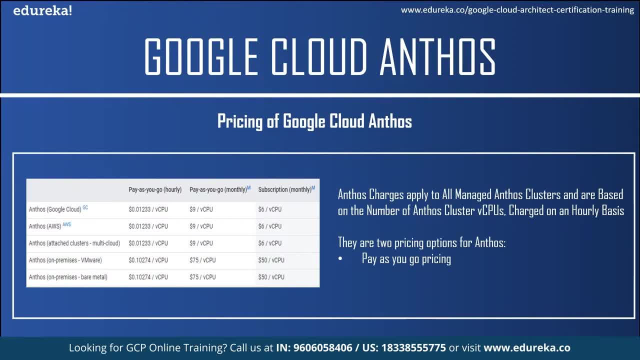 built for Anthos managed clusters as you use them Now. if you want to try Google Anthos or use it infrequently, you can choose pay-as-you-go pricing model. The next type of pricing option is a subscription pricing, which provides a discounted price for a committee. 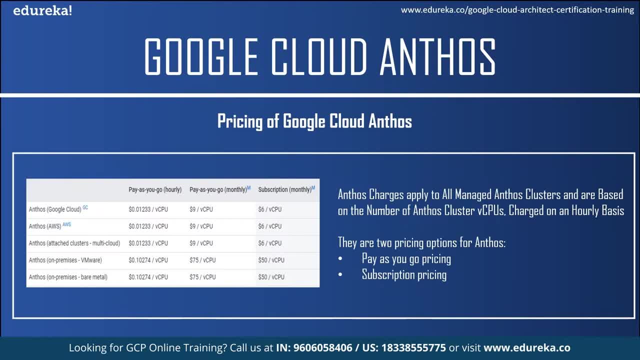 The term. your monthly subscription covers all Anthos deployment, irrespective of environment, at their respective billing rates. any usage over your monthly subscription fees will show as an overage in your monthly bill at the pay-as-you-go price listed here. Now you can see in the image over here: 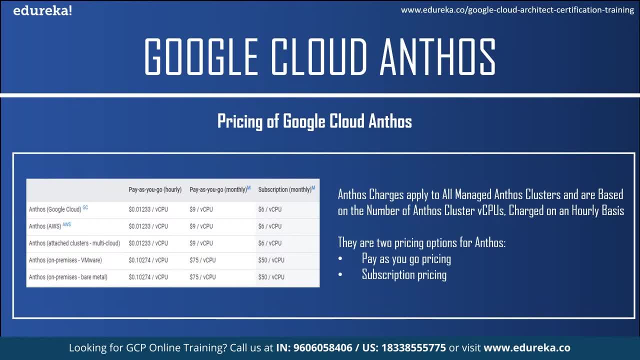 There are three payment option. First one is pay-as-you-go in an hourly basis, The next one is pay-as-you-go in a monthly basis and the subscription for monthly, and you can see the rates for each virtual CPU in various deployment Models, such as Google Cloud, AWS, multi-cloud, on-premises, VMware. 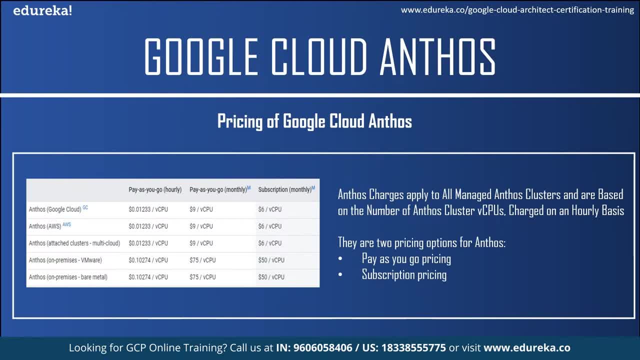 and on-premises bare metal. The good news is, if you are a new Anthos customer, you can try Anthos on Google Cloud for free, up to $900 worth of usage or for a maximum of 30 days, whichever might happen earlier. 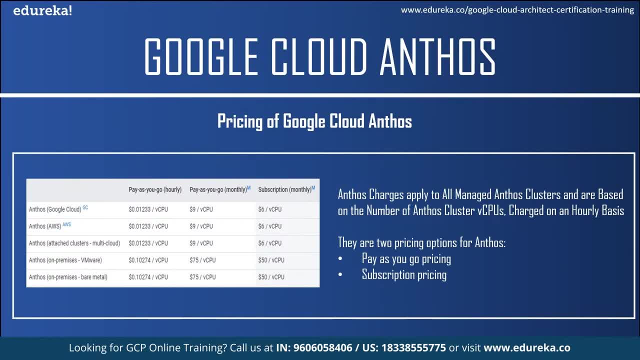 Now, during this trial period, you're only billed for the applicable fees and then credited at the same time for those fees- up to $900, but is still billed for the applicable infrastructure usage during the trial. This was about Google Cloud Anthos pricing. Now let us move on to the next topic and see a case study on. 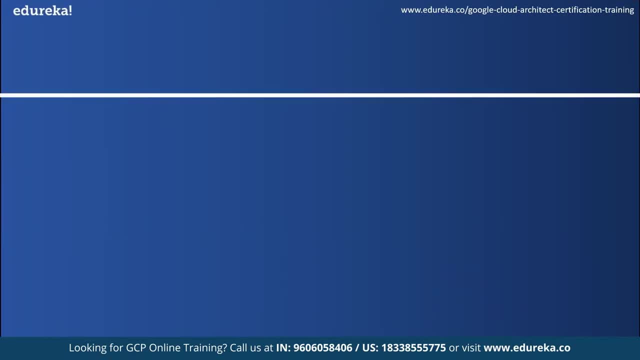 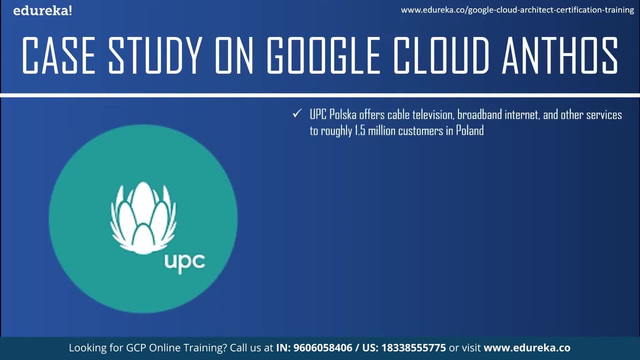 Google Cloud Anthos. So for a case study, we'll be talking about UPC Polska. Now, UPC Polska is a Polish telecommunication arm of Liberty Global Europe, which offers cable television, broadband internet and other services to roughly 1.5 million customers in Poland. 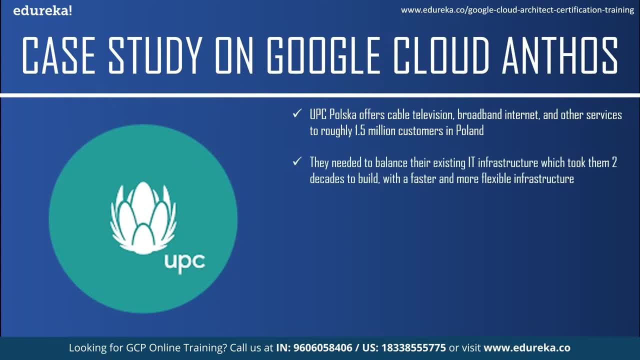 The problem they faced was they needed to balance their existing IT infrastructure, which took them two decades to build, with a faster and more flexible infrastructure. So when they were looking for the solution, they decided to opt for hybrid IT, which would give them the speed to market the needed 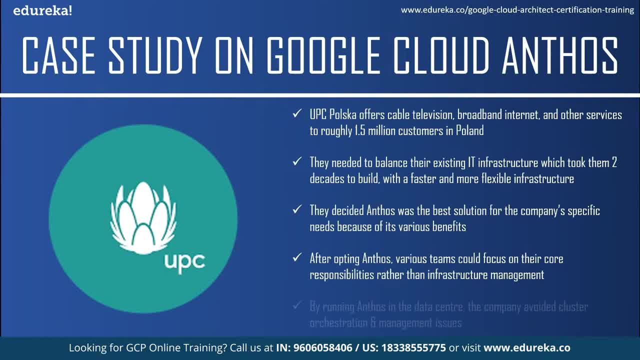 as well as maintain the existing infrastructure which they value. Now, deciding about the hybrid approach, they thought Anthos was the best solution for the company's specific needs because of the consistent experience across environment, agility enabled by modern CICD and the ability to set policy and ensure security at scale. 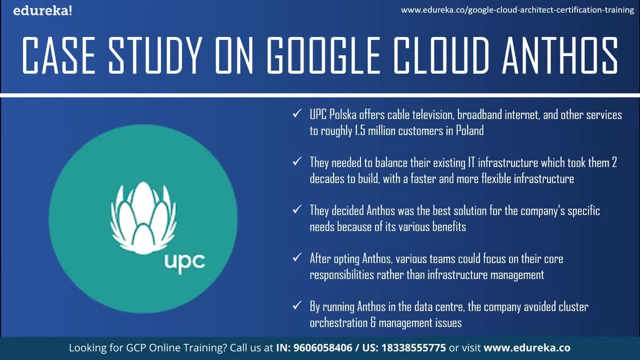 Then they partnered with Accenture and focused on the cultural and organizational element involved in rolling out a new solution. When they opted for Anthos, it provided them with the following benefits: Their various team could focus on the core responsibility rather than infrastructure management. 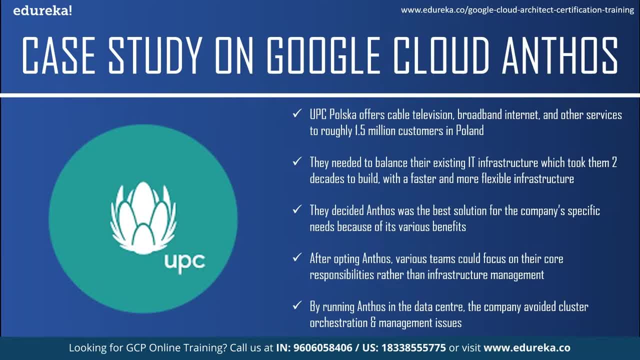 For example, developers could focus on writing greater codes, while the operational team could use Anthos to effectively manage and run those applications anywhere. Also, the on-premises nature of the company's existing infrastructure made scaling and general maintenance difficult By running Anthos in. 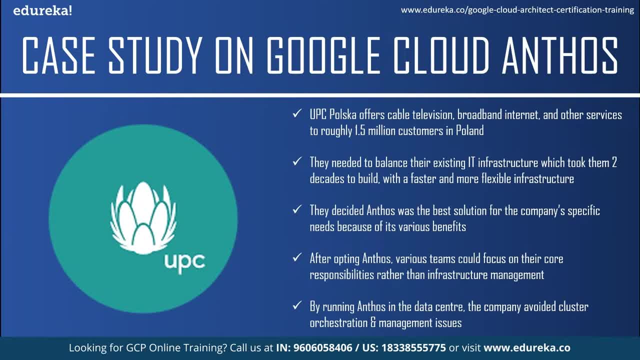 the data center, the company gained the fully compliant Kubernetes experience necessary to avoid cluster orchestration and management issues, which included managing and scaling the containers. They also improved the scalability and resilience through containerized GKE clusters. on Anthos: Now, this was a case study on Google Cloud Anthos. 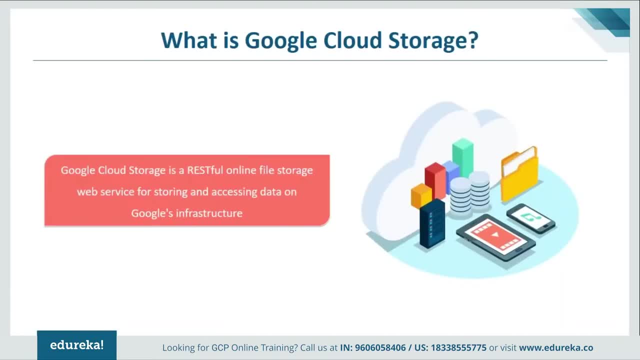 What is Google Cloud Storage Now? Google Cloud Storage is a set of various storage services offered by Google for different domain scenarios. It is a restful online file storage web service for storing and accessing data on the Google's infrastructure. Google Cloud Storage allows worldwide storage and retrieval of. 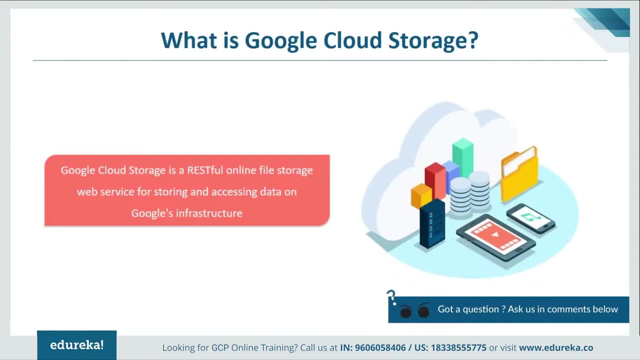 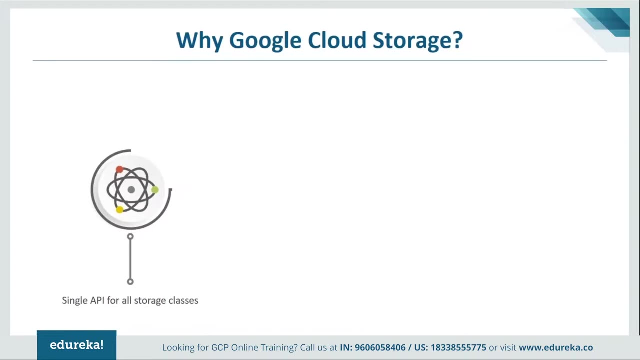 any amount of data at any time. You can use the cloud storage for a range of scenarios, including servicing website content, storing data for archival and disaster recovery, or distributing last data objects to users via direct download. So let's understand why we need Google Cloud Storage First of all. 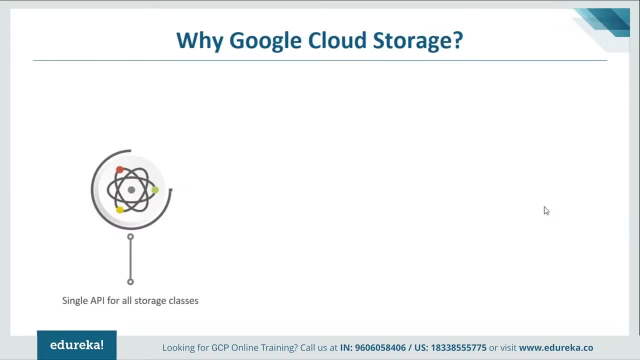 it has a single API for all storage classes. The cloud storage, consistent API latency and speed across storage classes simplifies development integration and reduces code complexity. You can set custom policies to transition data seamlessly from one storage class to the next, depending on your cost and availability needs. 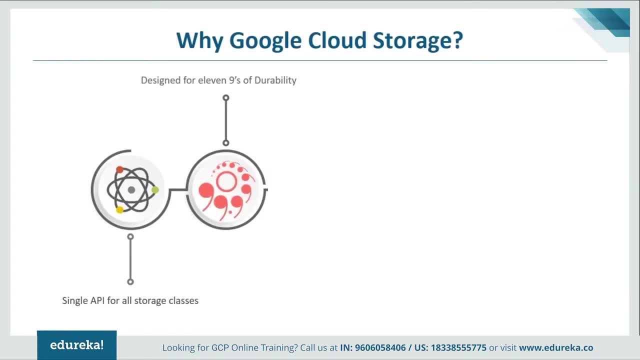 at the time. It is designed for 11 lines of durability. Google Cloud Storage is designed for 99.99. that are 11 lines annual durability. It stores the data redundantly with automatic checksum to ensure data integrity With multi-resource storage. 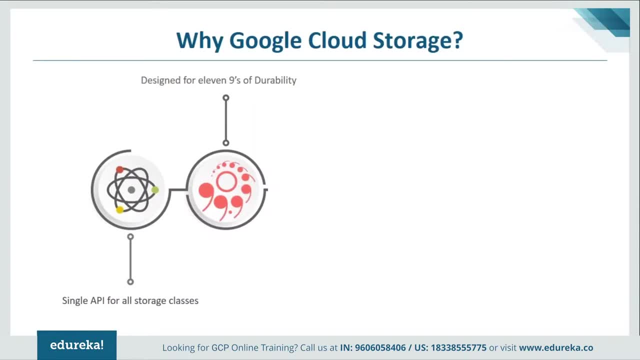 your data is maintained in geographically distant locations. It is highly scalable and performant. Now, Google Cloud Storage is practically infinitely scalable. Whether you are supporting a small application or building a large exabyte scale system, Google Cloud Storage can handle anything. 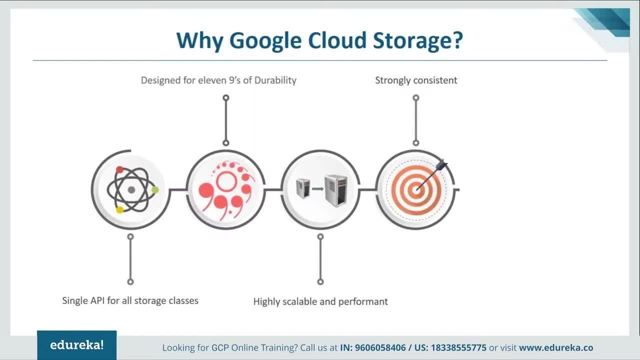 It is strongly consistent: When a ride succeeds, the latest copy of the object is guaranteed to be returned to any get globally. Now coming to the zero carbon emission, you have many things to consider in the cloud platform you choose. First of all, it's the 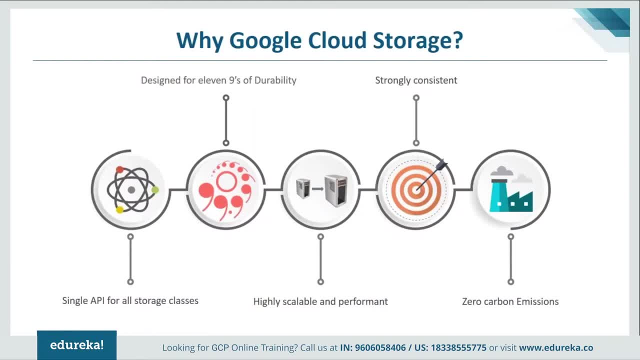 price, the security, the openness and, of course, the products available Now. Google believes you should consider the environment too. A sustainable cloud is not only good for the environment, but also good for your business By moving storage from a self-managed 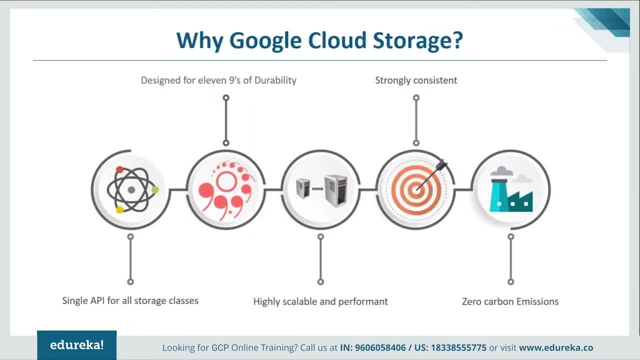 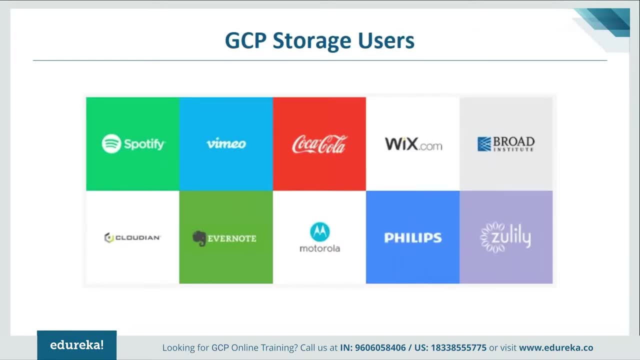 data center to GCP, the emission directly associated with the company's data storage will be zero. Now, here you can see, we have certain users who use Google Cloud platform for the storage services. We have Spotify, Coca-Cola, Evernote, Motorola. 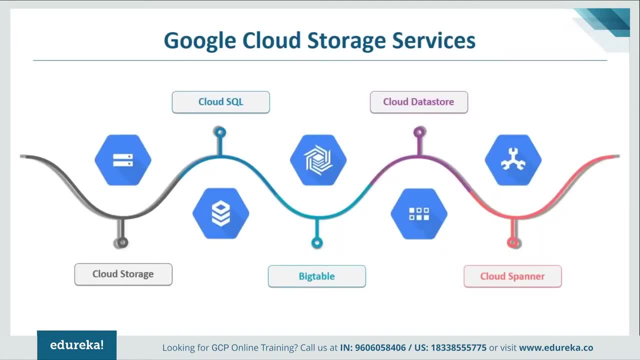 Philips and many more. Now let's have a look at the various Google Cloud Storage services provided by Google. We have the cloud storage. We have cloud sequel. Next we have the big table, the cloud data store and cloud spanner. We'll look into the details of each and every. 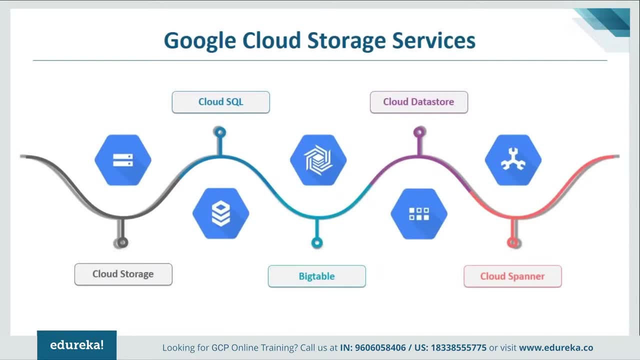 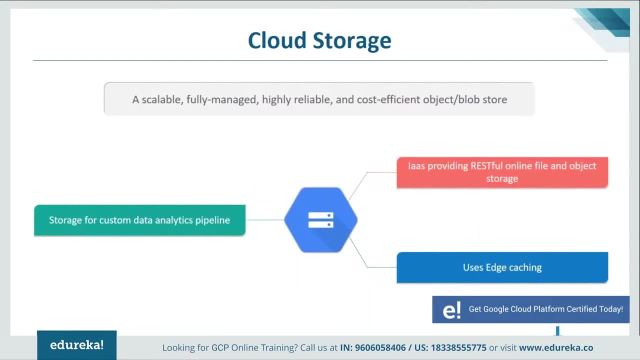 one of these services in this video. So let's get started with the cloud storage. The cloud store is a scalable, fully managed, highly reliable and cost-efficient object or blob store. It redefines what the industry can expect from online storage by providing a unified offering across the availability spectrum From live. 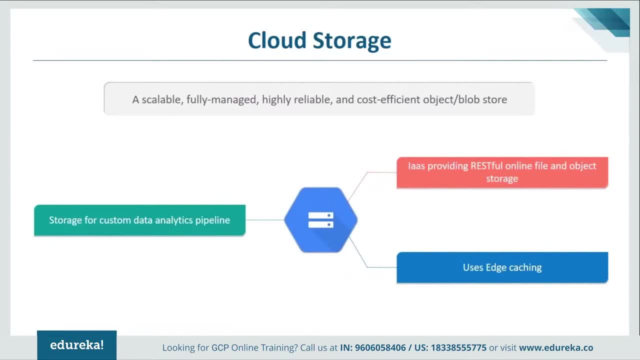 data tapped by today's most demanding application to cloud archival solution: near line and code line. It has many features, such as single API across storage, scalable to exabytes of data. very high availability across all storage classes, As we saw earlier that Spotify was one of the users. 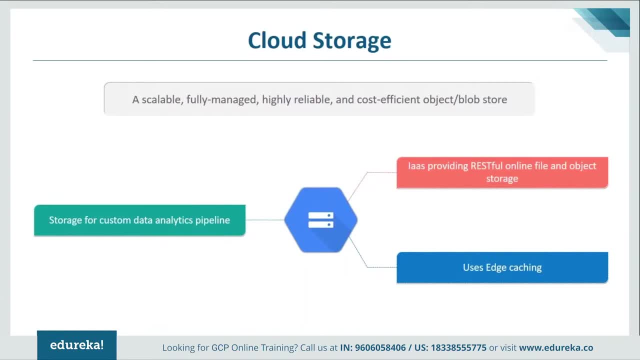 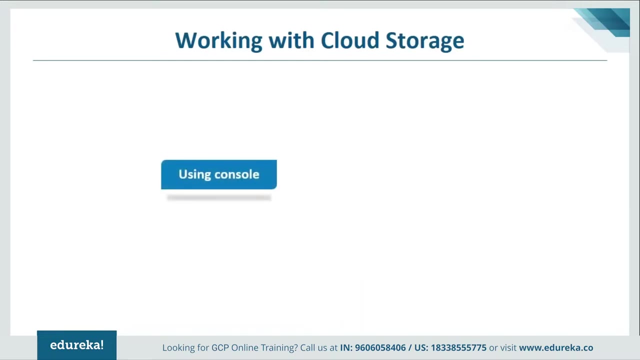 of the Google Cloud storage. Now Spotify uses Google Cloud storage for storing and serving music. using regional storage allowed them to run audio transcoding in Google's compute engine close to project storage. Now working with cloud storage, There are two different methods. We have the console and we have the gsutil tool. Now console is 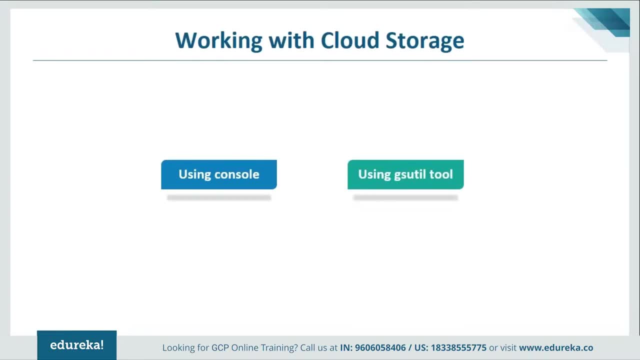 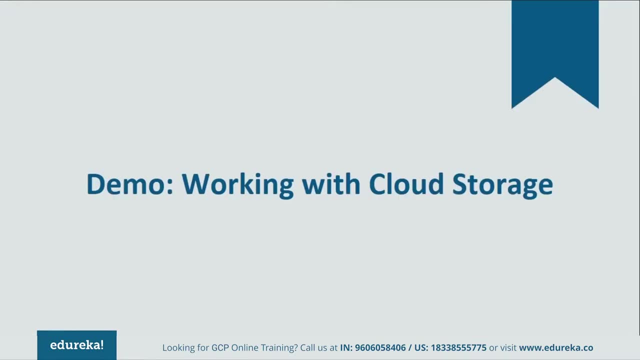 provided by Google on the web page or the web UI itself, and gsutil is a set of commands or tools which are used in the cloud SDK. So let's go ahead and see how we can work with the Google Cloud storage. First of all, you need to log in into your Google Cloud. 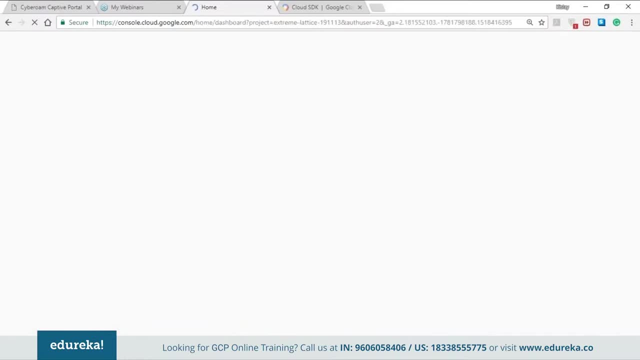 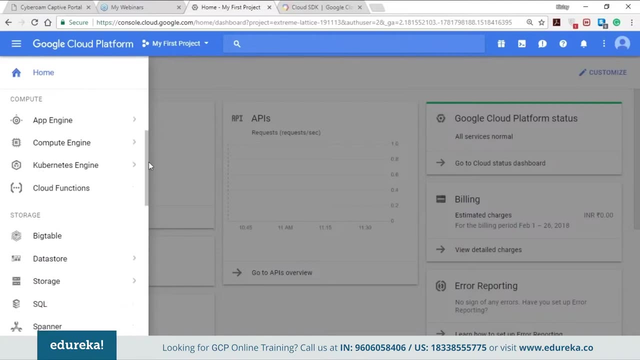 platform account and you need to go to the console In the left hand side. in this toolbar you can see we have the various services, which are the compute, storage, networking, monitoring and the development tools and the big data tools. So today we will focus on the storage services. So let's go to the storage section, as 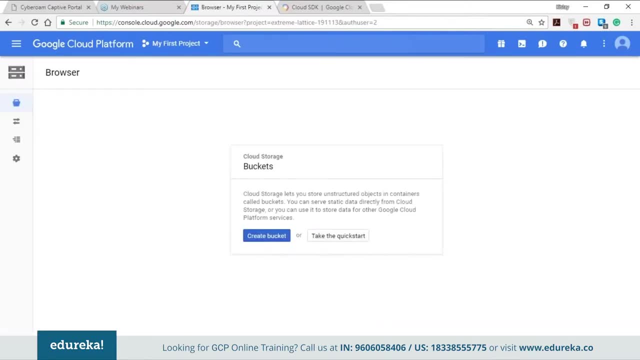 you can see, here I have the option to create a bucket. So let's understand what is a bucket. the cloud storage lets you store unstructured data objects in containers, which are known as buckets. You can serve static data directly from cloud storage or you can use it to store data. 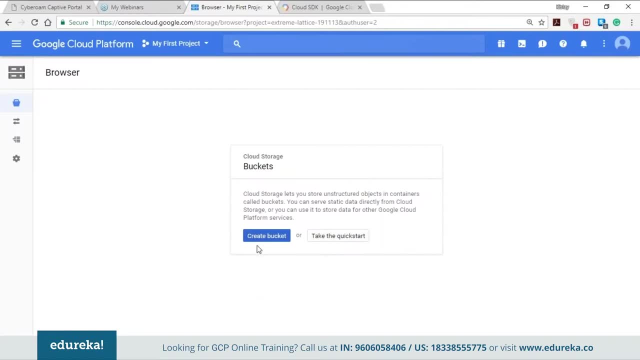 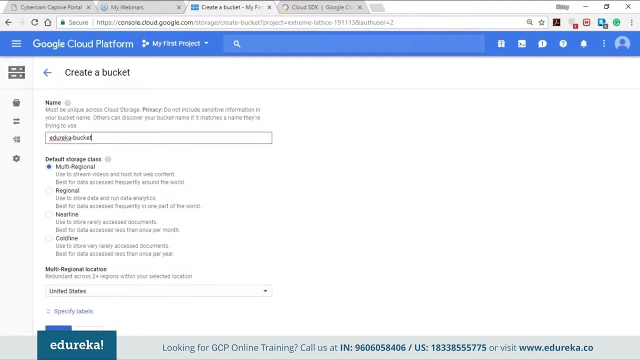 Other Google Cloud platform services. So let's go ahead and create a bucket. So first we need to input the bucket name, Next we have to select the storage classes. Now there are four types of storage classes, which are: multi-regional, regional. 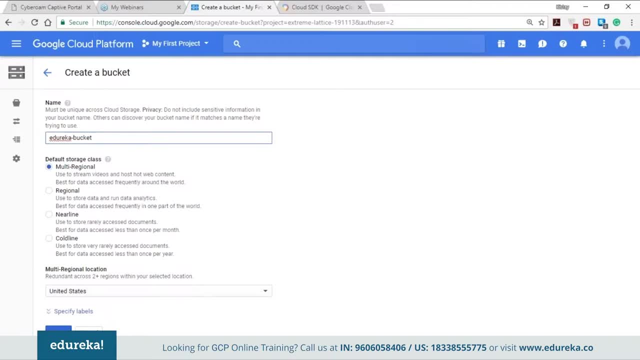 near land and code line. out of these two, the multi-regional and regional are based on the geographic regions, Whereas near line and code line are based upon the usage. Now, multi-regional is used for the data which is accessed frequently around the world. 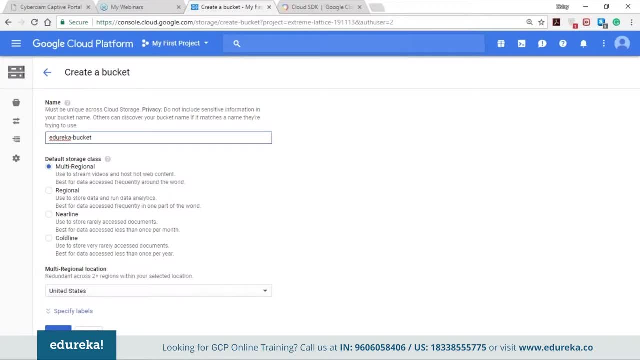 Regional is used For the data which is accessed frequently in only one part of the world. coming on to near land and code line near land is best suited for the data which is accessed less than once per month. That means you can access it maximum once per month. Now code. 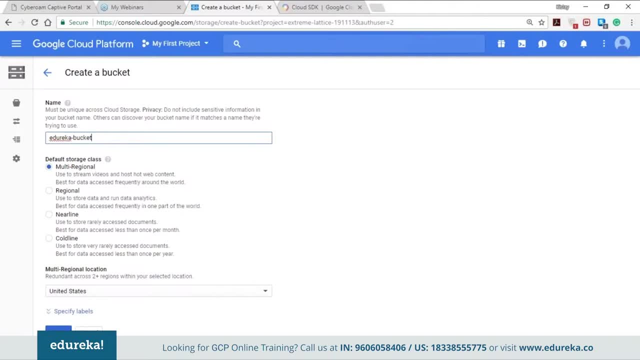 line is best used for the data which is accessed less than once per year. So now I'm going to select the regional storage class. next we have to select the regional location And just tap on the create button, and within seconds your bucket will be created. 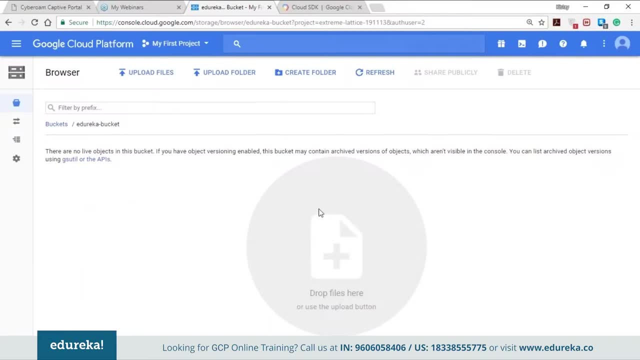 As you can see that there is nothing inside this bucket here. You can directly drop your files here from your PC or your laptop and you have the option to upload files, upload a folder or create a folder. Let me just upload one file. Within seconds, the file is uploaded and it's shown here. 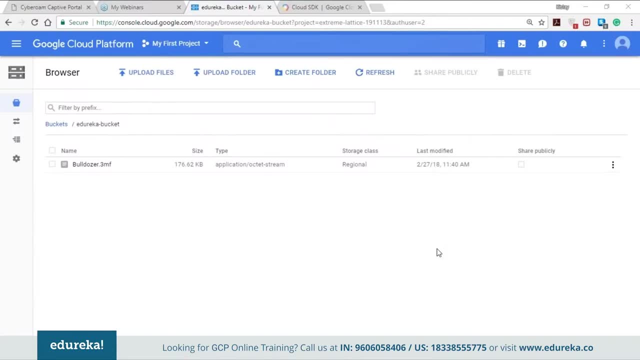 Now that you have seen how to create a bucket and upload a file, the same can be implemented using the gsutil commands. for that, we need to download the cloud SDK. now, cloud SDK can be downloaded from Google. tap on on the first page and you'll be redirected to this page. Now you can. 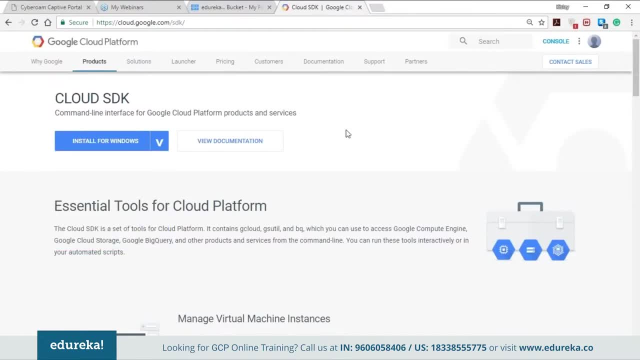 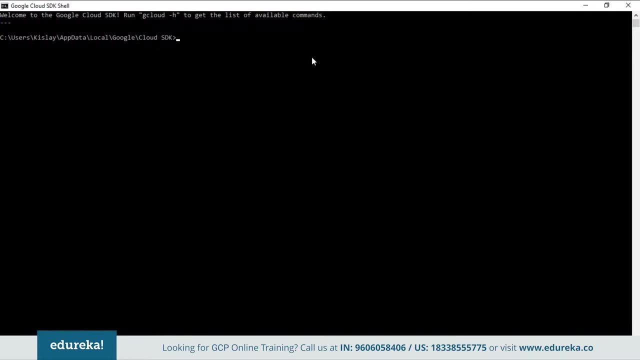 install it for Windows, Mac OS, Linux or other operating systems. I have already downloaded, so I'll just fire up the cloud SDK shell. Now. just to create a bucket, All you need to do is type in the command gsutil mb, which is make bucket. hyphen C, which stands for the class, the storage class, which 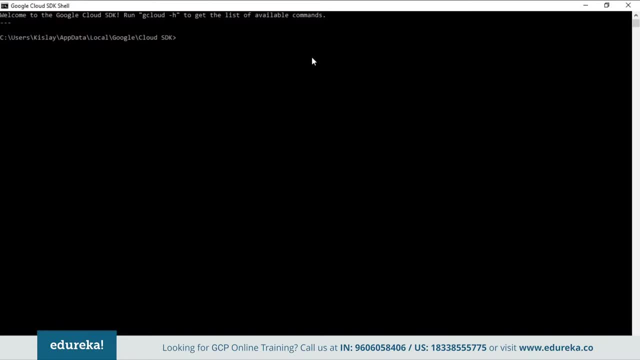 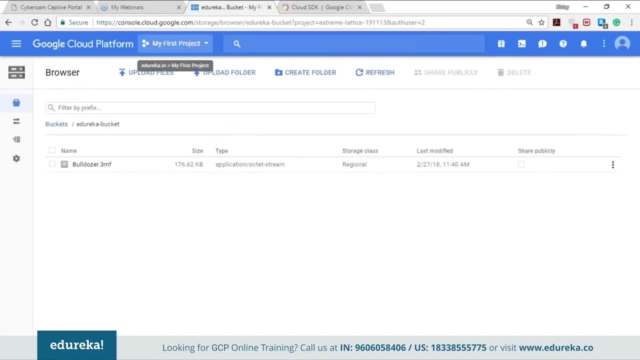 I'm going to select as regional. hyphen L stands for location and hyphen P, which stands for the project ID. and finally, you have to input the name of the bucket For project ID. you can refer to the my first project or whatever be your project. just copy your ID from here. 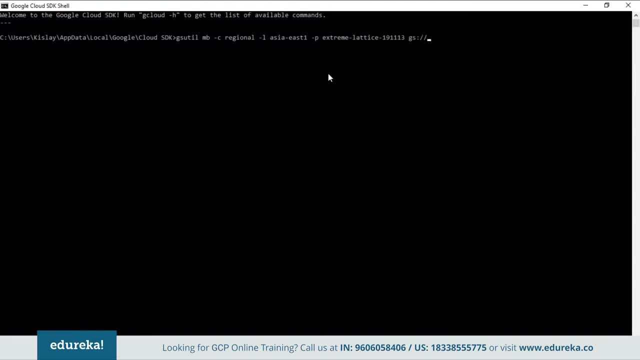 Paste it and then, finally, you need to input the name of the bucket. So now, to list the buckets, All you need to type in is gsutil ls. As you can see, we have two buckets, which is edureka bucket and edureka bucket 2. the same will be reflected on the website itself. 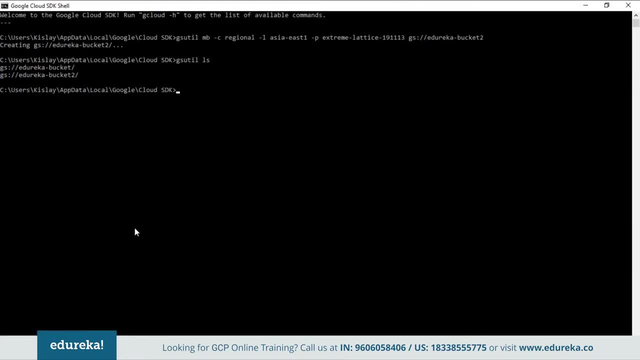 As you can see here, edureka bucket 2 is also here Now. to list the contents of a bucket you need to tap in the commands gsutil ls, hyphen R and the name of the bucket. So, as you guys saw earlier that I uploaded an image to the first. 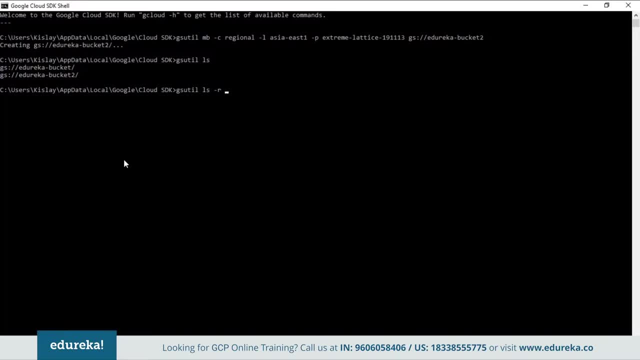 bucket which I created, edureka bucket. So let me list the contents of that one. As you can see, it's showing me the image which I uploaded not to delete a bucket. We have an easy command of gsutil rm, hyphen R and the name of the. 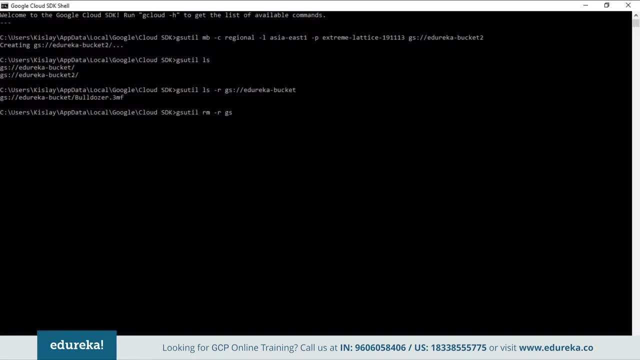 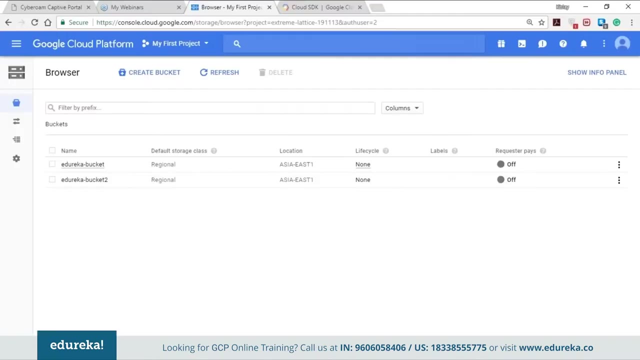 bucket. Here. I'm deleting the Second bucket I created and after that will list the buckets to see whether it was deleted or not. The same will be reflected on the website. Let me refresh this page. As you can see, we have only one bucket, which is the edureka bucket. 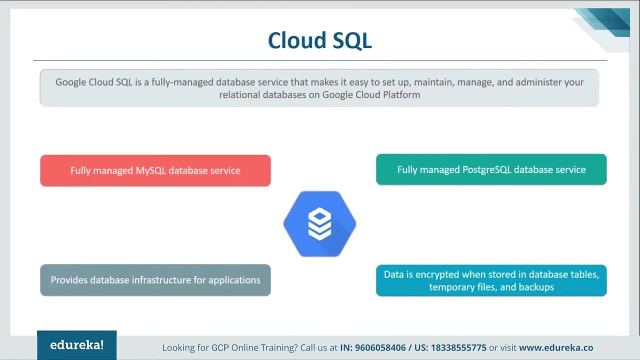 So now let's go ahead with cloud sequel. the cloud sequel is a fully managed database service that makes it easy to set up, maintain, manage and administer your relational MySQL or postgreSQL database in the cloud. the cloud sequel offers high-performance, scalability and convenience, hosted on the Google. 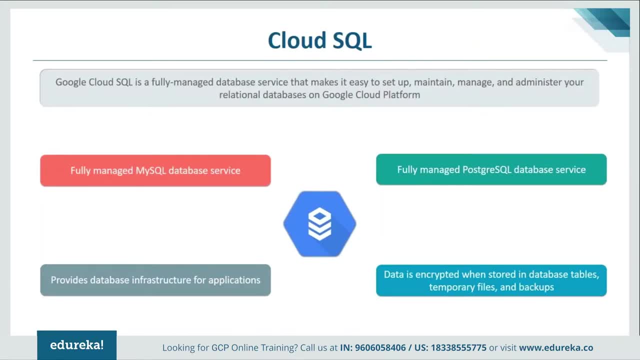 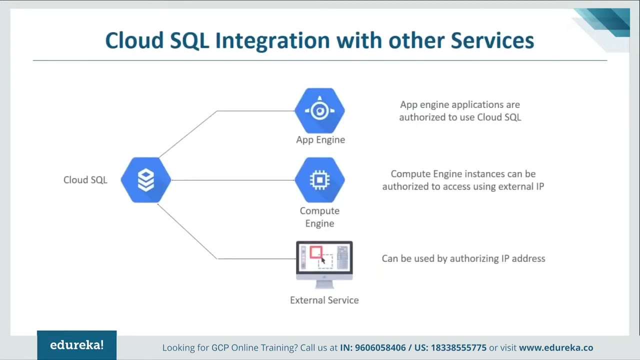 Cloud platform. The cloud sequel provides a database infrastructure for application running. Anyway, it is fully managed postgreSQL database service and my sequel database service. The data is encrypted when stored in the database table. Now cloud sequel can be integrated with other services such as app. 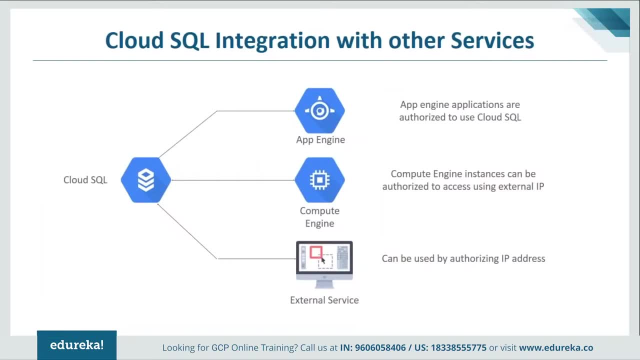 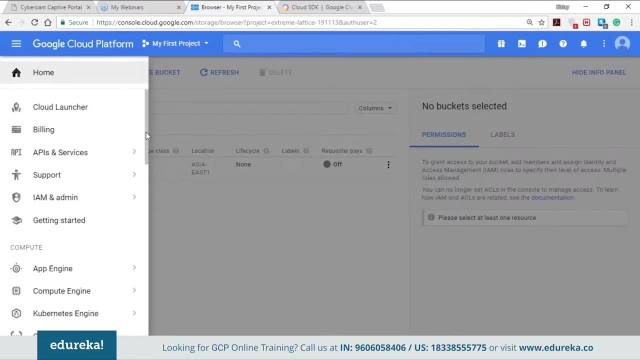 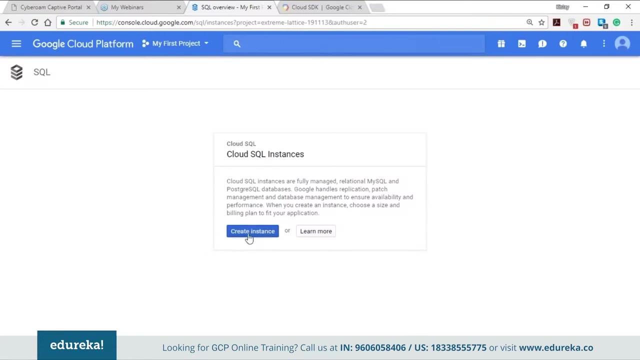 engine, the compute engine, And external services via the external IP. Let's go ahead and see how we can work with the cloud sequel. Go to the taskbar on the left hand side, tap on the sequel button and here you'll be asked to create an instance which will be our sequel. 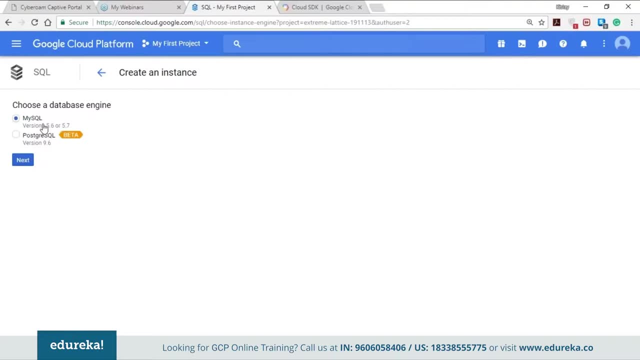 instance. just tap on the button here You have the option to choose between my sequel and postgreSQL. the postgreSQL is in beta format, So I'll select my sequel now. There are two options. first We have the first generation and the second generation now. second, 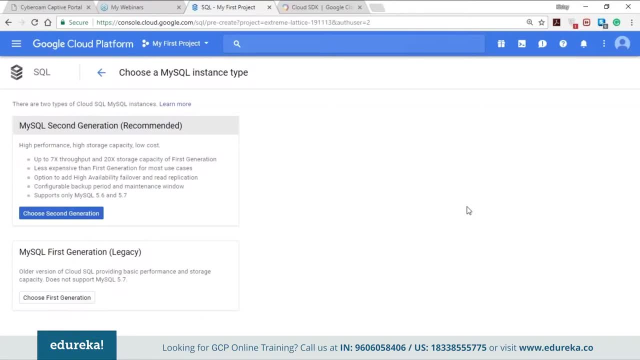 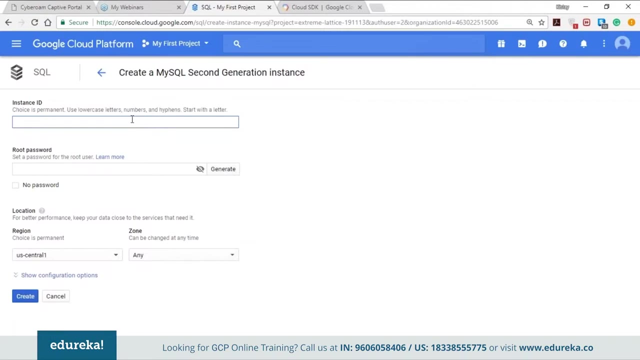 generation has seven times the throughput and 20 times the storage capacity than the first generation. It is less expensive and it supports my sequel 5.6 and 5.7. now, in order to create your sequel instance, All you need to provide is the instance ID and set a root password. 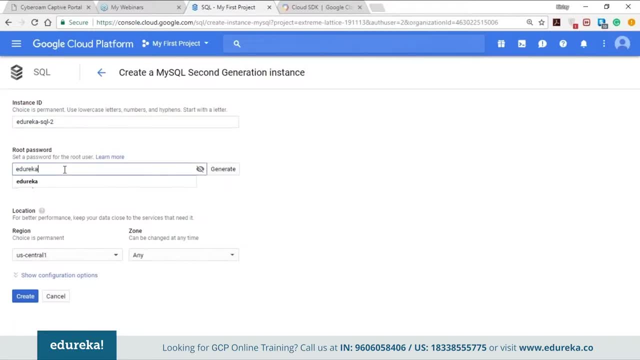 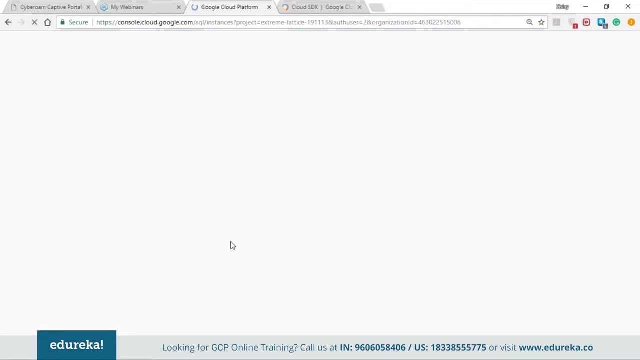 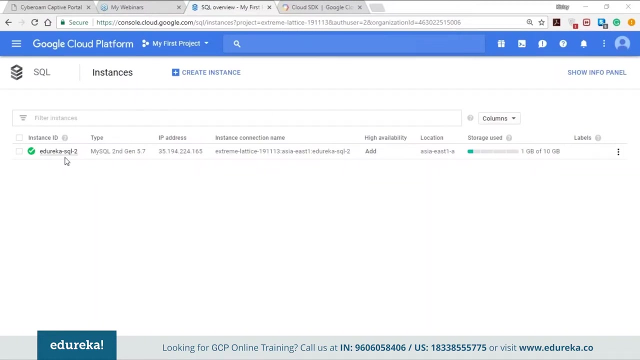 So the instance ID here is a really good sequel to and the password. now You need to select the region And the particular zone In this, tap on this create button and your sequel instance will be created within minutes. So now that our instance is created, let's go ahead and click on the. 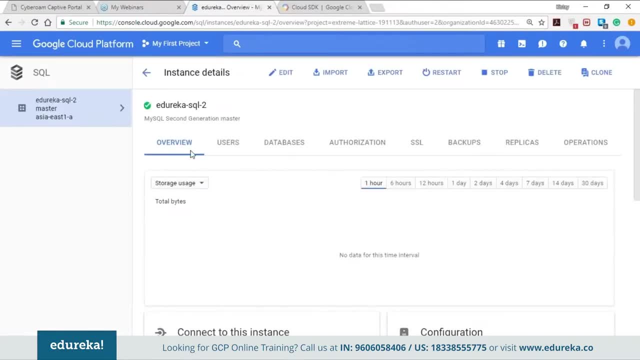 instance ID. Now, as you can see, here we have so many options like user databases, authorization, SSL, backups, replicas and operation. Now let's get to the User part. here we can create a user account. by default, We have a root user. 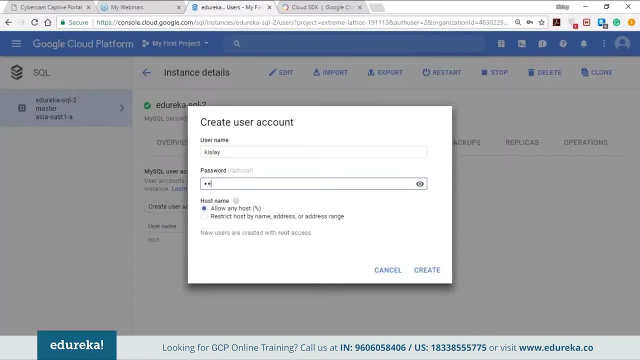 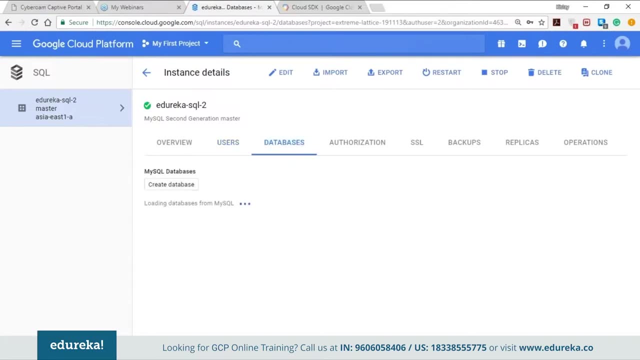 So let's create a user. just input your user name and put in the password, and within seconds your user will be created. Now, coming on to the database part. here We have the option to create a database. by default, We have three databases, which are: the information schema, my sequel. 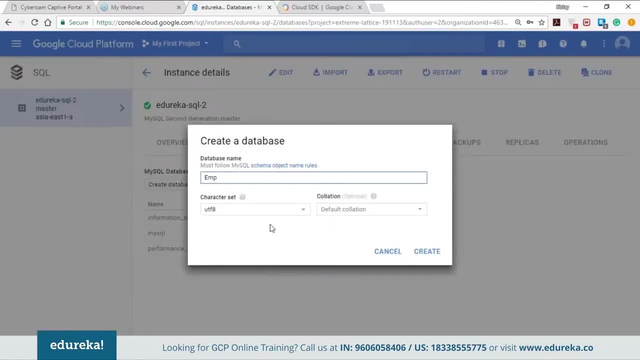 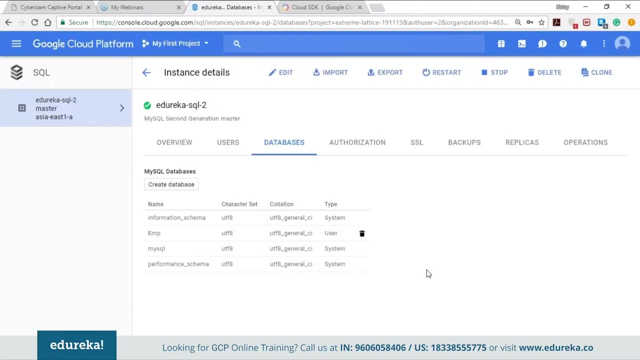 and the performance schema. Let me create a database. employee. as you can see, creating a database Is so easy. Now, the database which we created and the instance we created can be accessed using the Google Cloud Shell as well as the cloud SDK, So we'll see how we can access the same using the cloud shell. 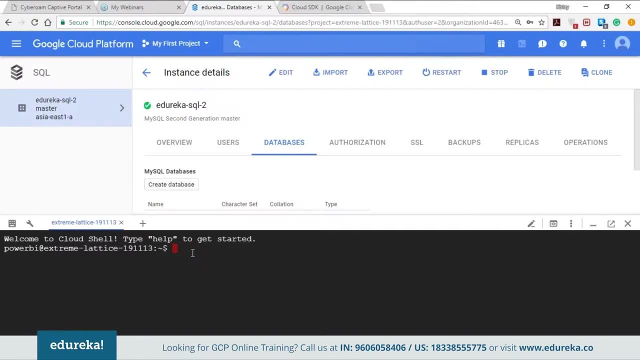 Now, in order to connect your sequel instance to the cloud shell, All you need to type is G- cloud sequel- connect the name of the instance and your username. The instance name is Edureka, SQL to, and the username is crystal. As you can see, within minutes I was redirected to the my sequel. 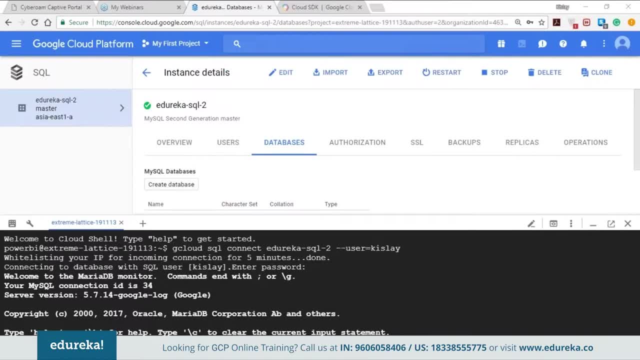 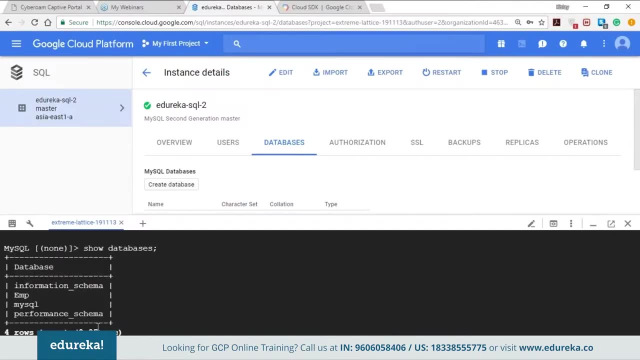 shell of the instance. Now, this my sequel shell works in the same way as any other my sequel. So let's first check the databases. So, as you can see, we have the EMP database which I created just now. you can use this database And perform the same function. 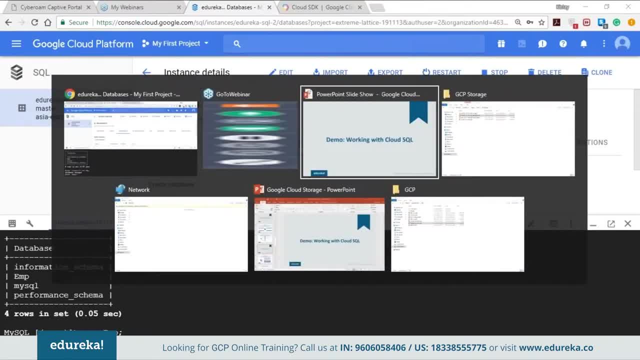 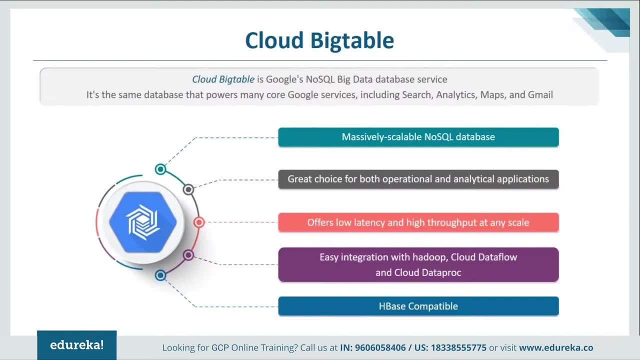 As a my sequel shell. now, coming back to our services, Next we have the cloud big table. The cloud big table is Google's no sequel big data database service. It is the same database that provides many core Google services, including search analytics, maps and Gmail. 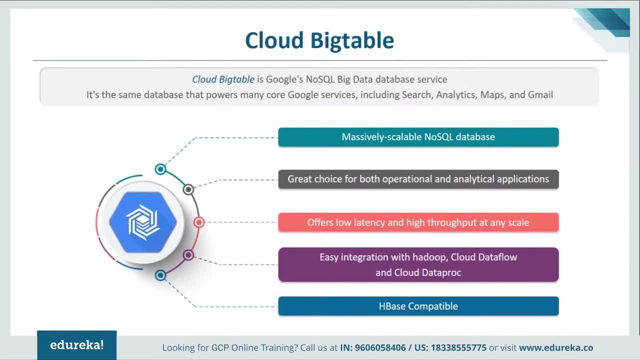 It provides massively scalable, no sequel database suitable for low latency and high-throughput workloads. It integrates easily with popular big data tools like Hadoop and spark, And it supports the open-source industry based standard HBase API. Now cloud big table is a great choice for both operational and 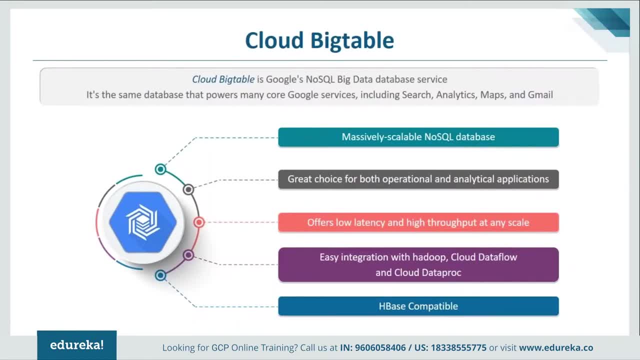 analytical applications, including IOT user analytics and financial data analytics. You can use big table as the storage engine for large-scale low latency applications, as well as throughput intensive data processing and analytics. the big table provisions and scales 200 of petabytes automatically, and it can smoothly handle millions of operations per 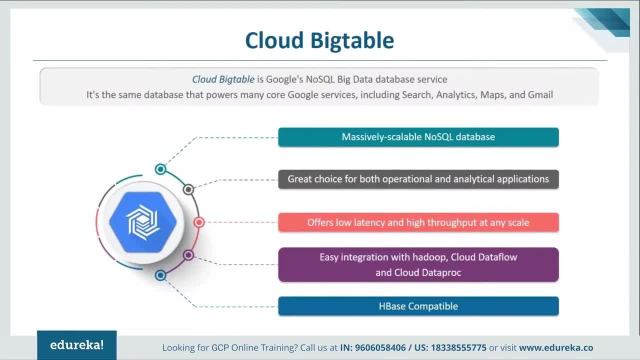 second, changes to the deployment configuration are immediate, So there is no downtime during the reconfiguration. cloud big table stores data in tables which contains row. each row is identified by a row key. It is the same as any no sequel database. now data in a row is 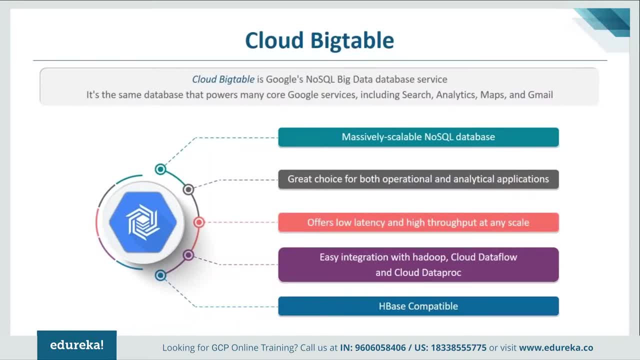 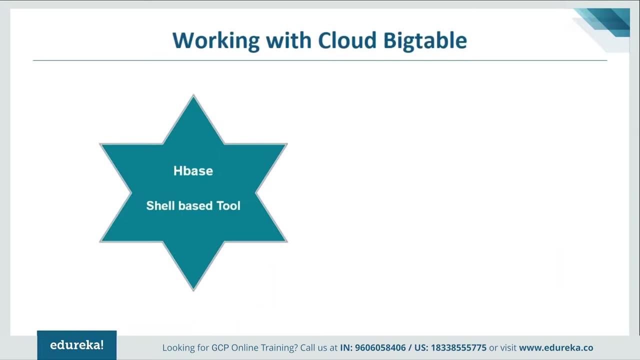 organized into column families or a groups of column. a column qualifiers identifies a single column within a column family. a cell is the intersection of a row and a column, and each cell can contain multiple versions of a value. Now, working with cloud big table, There are two ways. we have the HBase, which is the shell based tool. 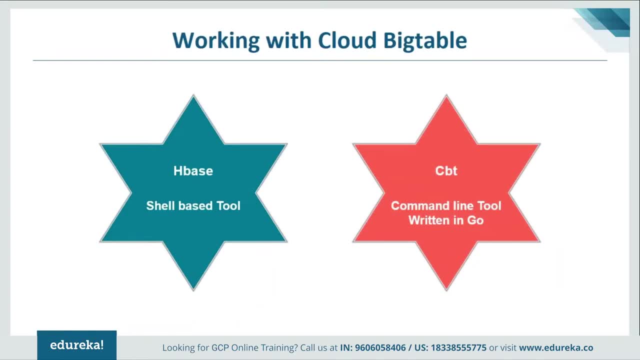 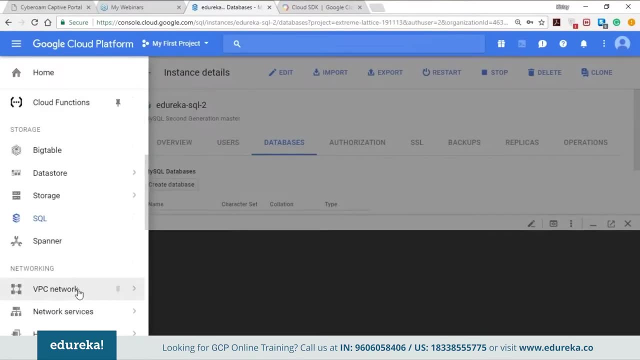 and we have CBT, which is the command line tool, written in. go now Let's go ahead and see how we can work with cloud big table. Just go to the storage section, Click on big table And here you can have the option to create an instance. the step on: 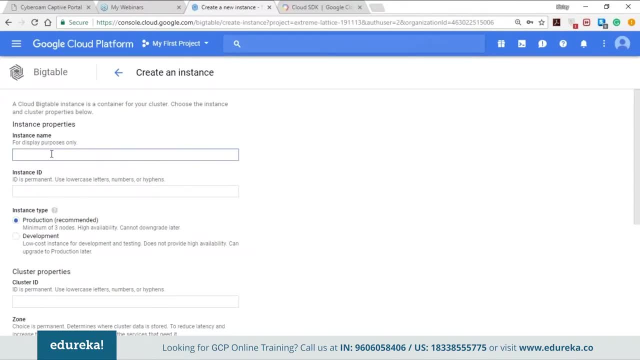 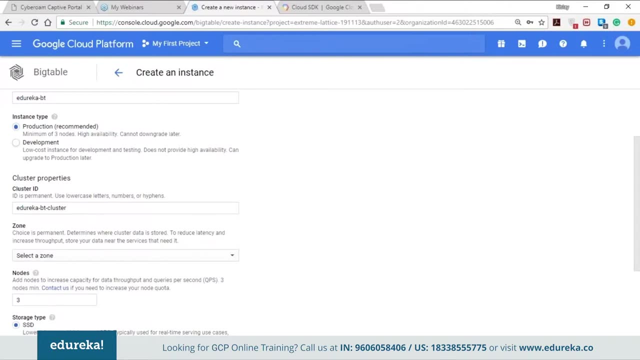 that button and here you can see you have to provide your instance name. instance ID is automatically created. Now you have the instance type, which is either production or development. now production is not preferred unless and until you have a very high availability requirement with a minimum number. 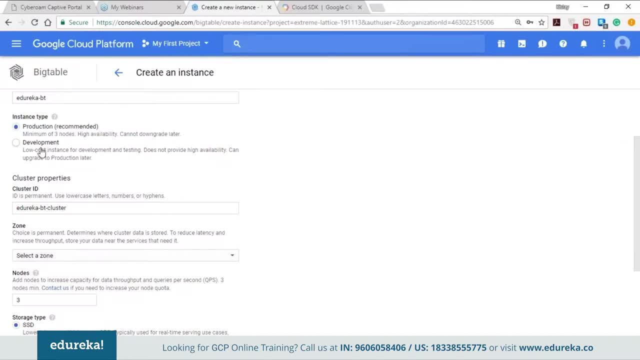 of three nodes plus. it cannot be downgraded. now. development seems to be the best choice If you want a low-cost instance for development and testing, though it does not provide high availability, but it can be upgraded to production later. Now we need to select the zone. 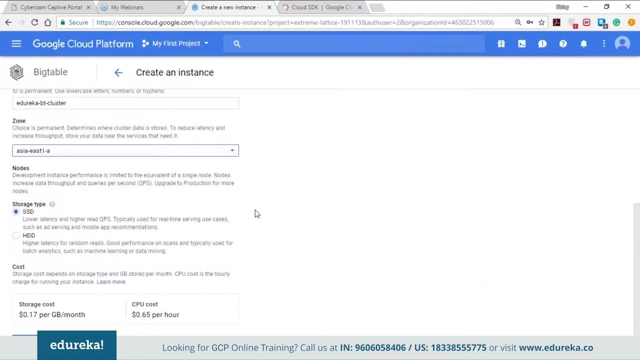 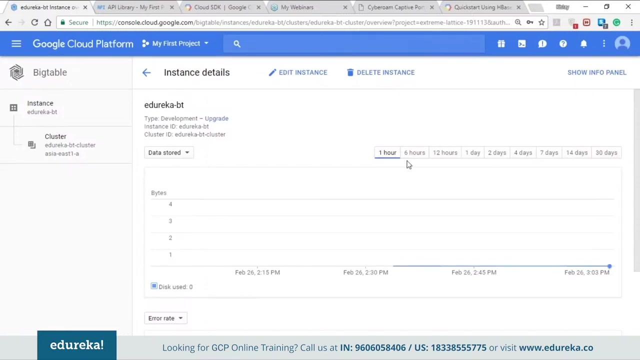 You have to select the storage type, which can be the SSD or SDD. Now, SSD is has a lower latency and higher read QPS, which is query per second. to stop on the create button and within seconds, your instance will be created. So, guys, as you can see here that I have created an instance which 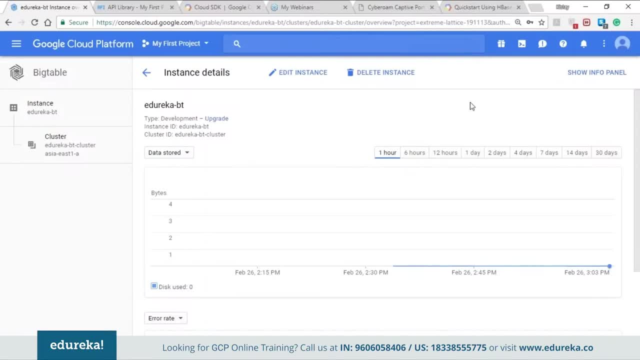 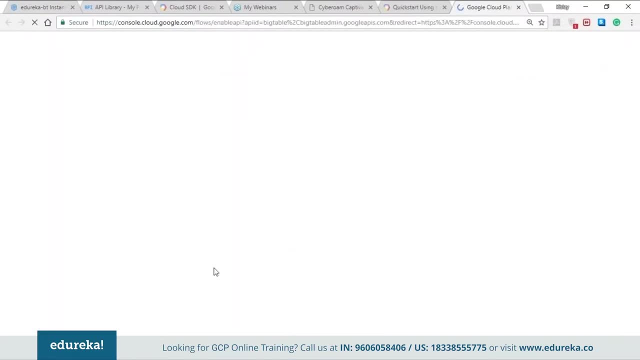 is Edureka hyphen BT, the big table instance. Now let's go ahead and fire up this instance using the cloud shell. First of all, we need to enable the API's, which is the cloud big table API and the cloud big table admin API. 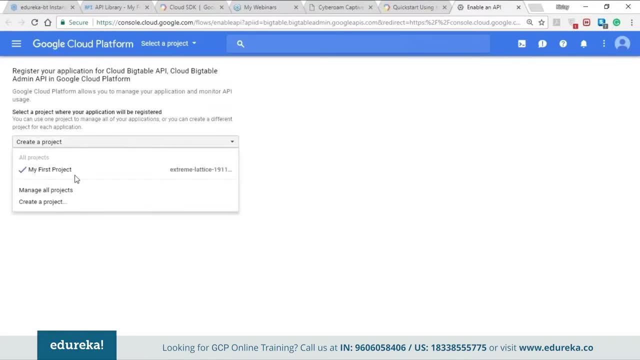 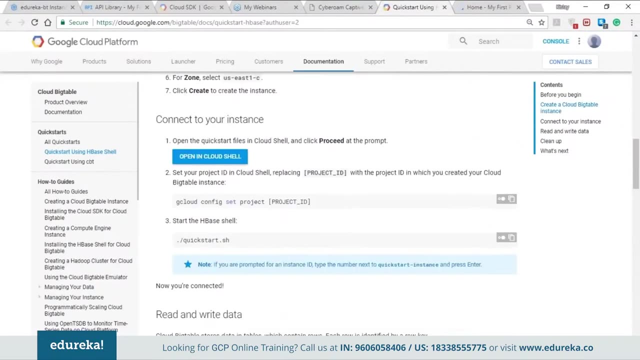 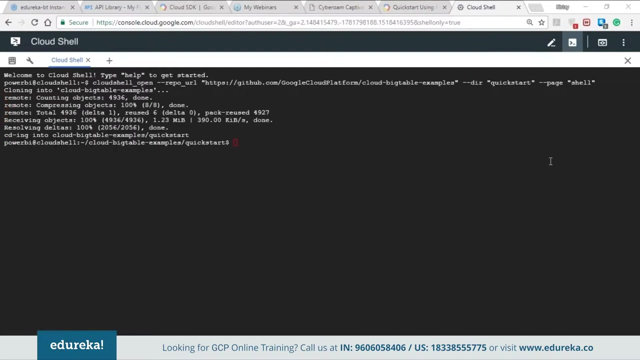 For that we need to select the project here. Let me select my project. Now, the API's are enabled And I've created the instance. All we need to do is open the cloud shell now. So, guys, as you can see here, it automatically connects to the. 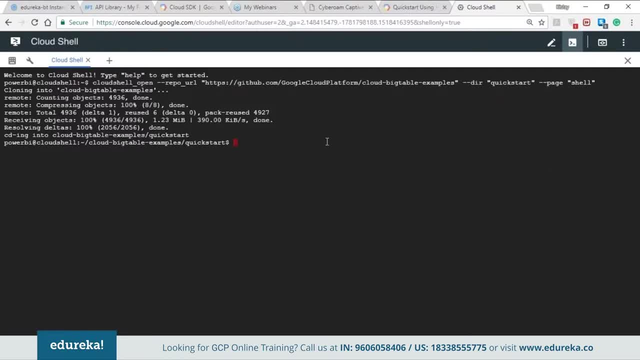 github repository of the Google Cloud Platform. and now to connect our project to the Google Cloud Platform, All we need to do is type in the command G Cloud config, set project and the project ID. Let me just copy the project ID. And now to start the HBase shell, we need to type in the command: 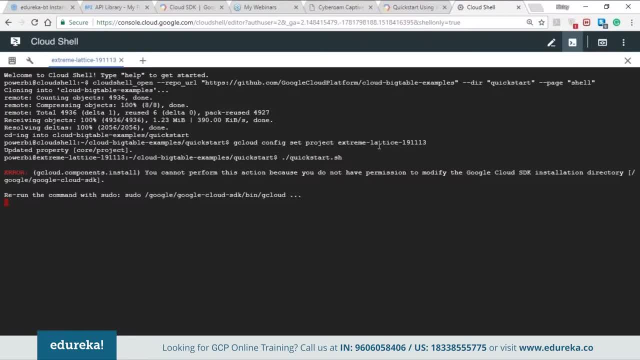 quickstartsh. As you can see, it throws an error that you cannot perform this action because you don't have the permission to modify the Google Cloud SDK installation directly. But instant they read on the command with sudo. as you can see, it is scanning for the projects. 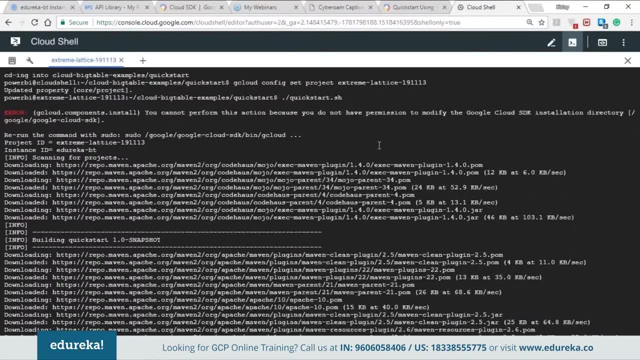 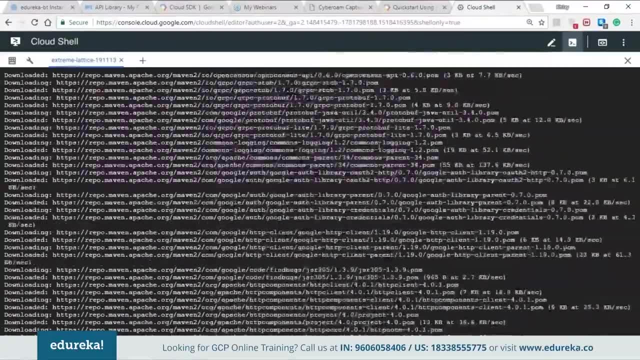 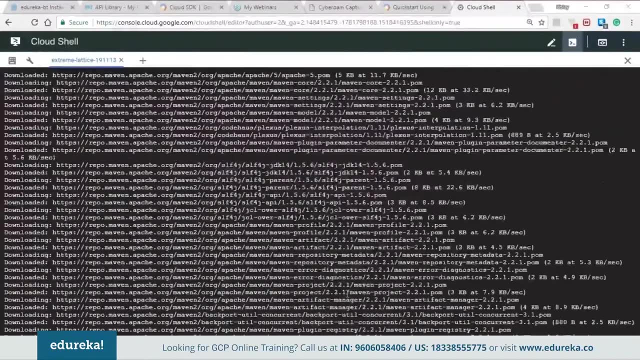 And downloading the projects from the maven repository. It's building the quick start with the snapshots And in a moment you will be connected to the HBase shell. So, guys, as you can see here, now that we have entered the HBase shell, 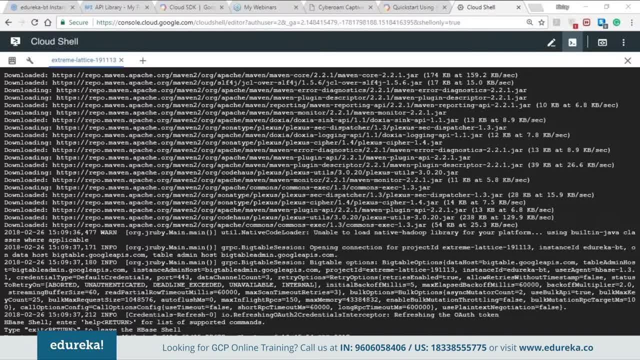 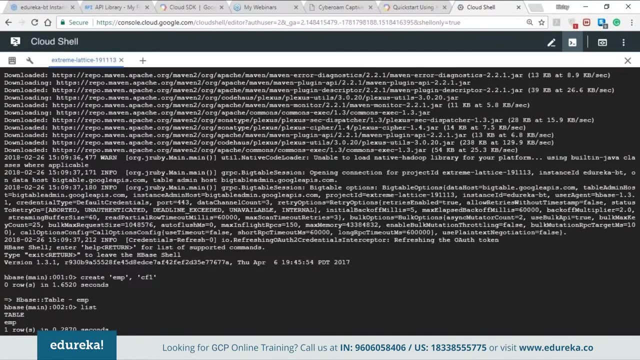 Now we need to create a table with a column family, CF1. all we need to do is type in this command: create the name of the table, which is EMP, and the column family name. Now to list it, all we need to type is list. 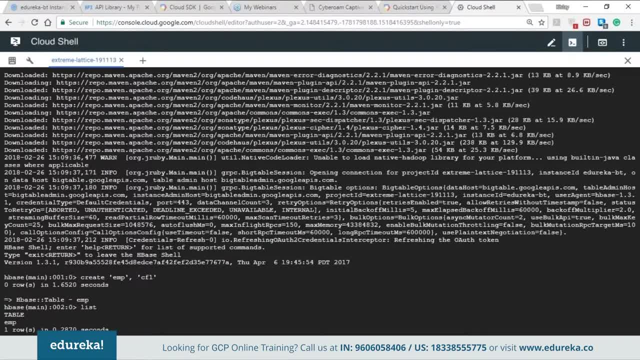 I will list one row in the table EMP. now, to put the value of any value in a row- R1, suppose, using the column family CF1 and the column qualifier C1, all we need to do is put in this command The row number, which is R1, the column family, which is CF1 column. 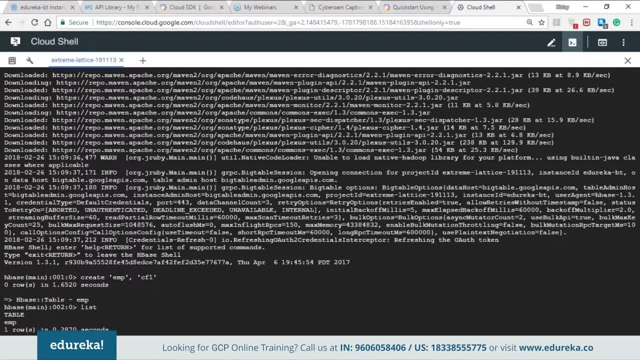 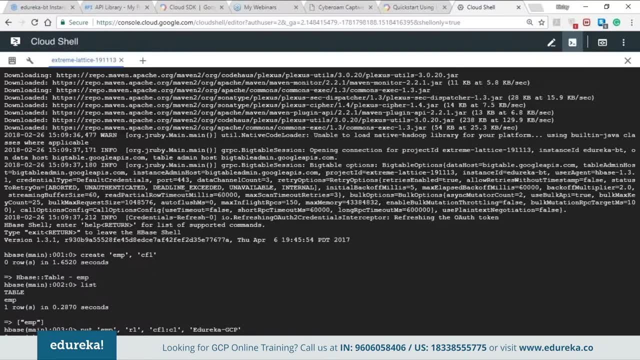 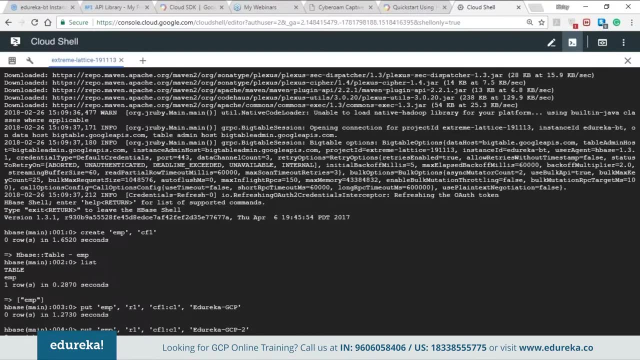 qualifier C1 as the value to be inserted. First of all, I'll be inserting a value. Okay, Now let's insert another value And to see the values inside a particular table, all you need to do is type in the command scan and the table name, as you can see here. 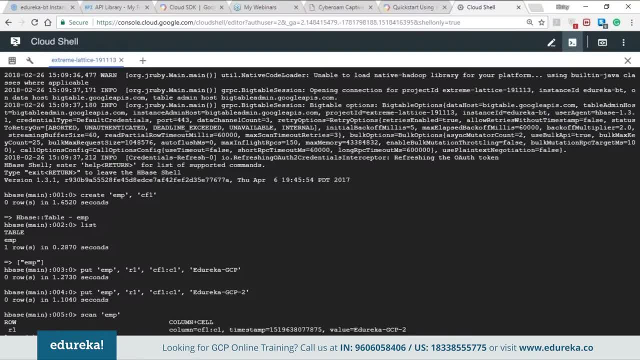 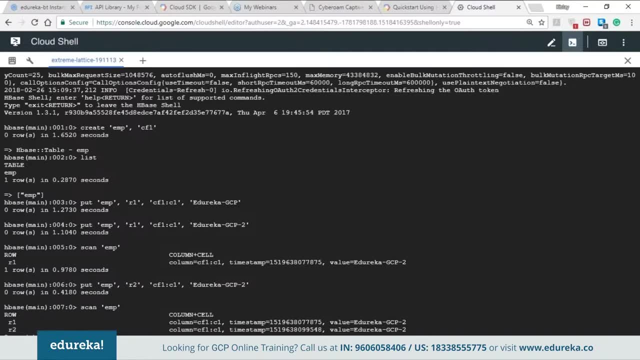 in the R1 row. Let me put in another value in the row R2 and scan again. You'll see that we have two rows, each of which have the values in the column family one. We have the timestamp and the value written as Edureka GCP 2.. 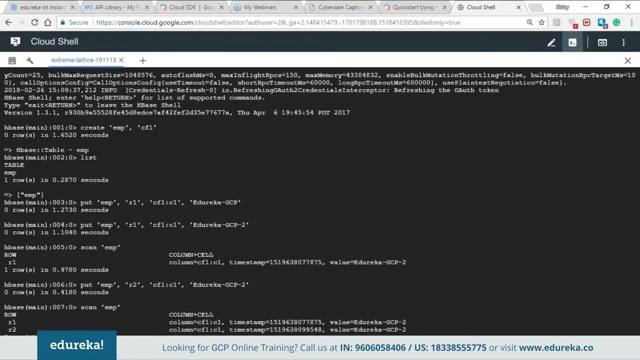 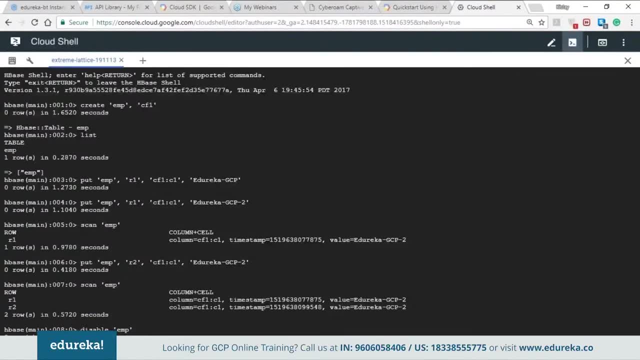 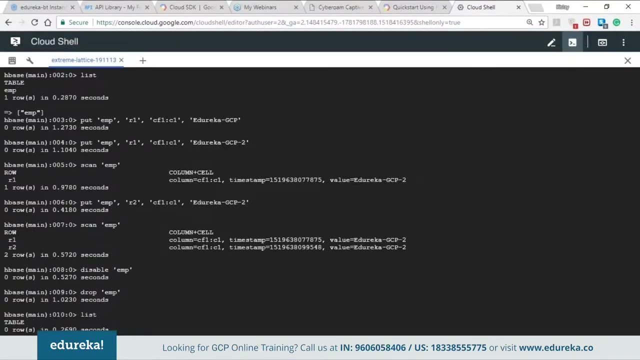 Now to drop the table, There are two commands to be inserted: which is disable the table name and put in as disable EMP, And the second one is drop EMP. Now, when I list the tables, it will show me zero tables. So the same can be implemented via the CBT, which is the command line. 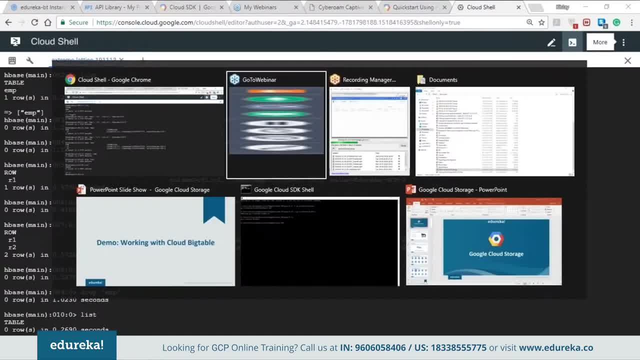 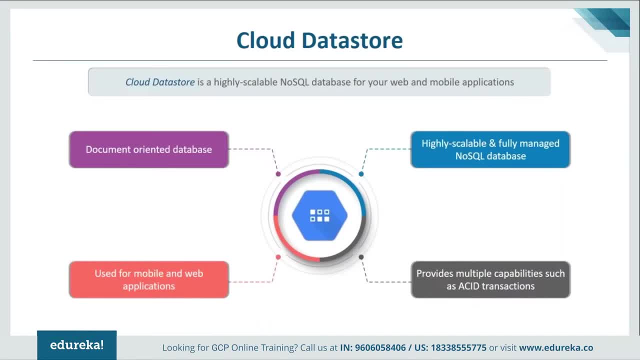 using the go command. So let's go back to our presentation Now. next we have the cloud data store. The cloud data store is a NoSQL document oriented database build for automatic scaling, high performance and ease of application development. Cloud data store features. 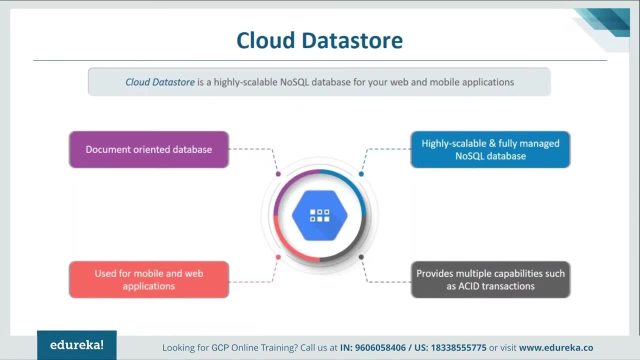 Include automatic transaction, which implies that operations will either all succeed or none will occur. high availability of reads and writes. massive scalability and high performance. flexible storage and querying of data. We have the balance of strong and eventual consistency encryption addressed. the cloud data store automatically encrypts all the data. 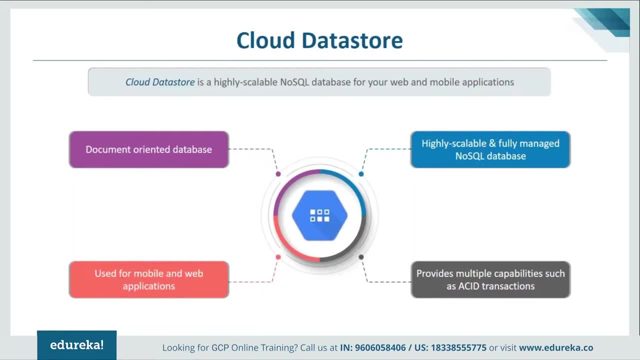 before it is written to the disk and automatically decrypts the data when read by an authorized user. The cloud data store Is ideal for application that rely on high availability structure data at scale. You can use the cloud data store to store and query all types of 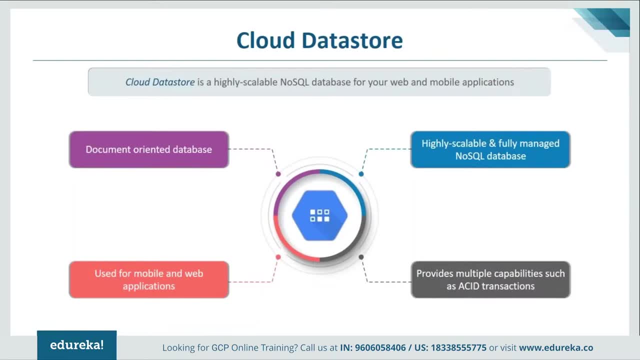 data. You can use it for: product catalogs that provide real-time inventory and product details for a retailer. user profiles that deliver a customized experience based on the users past activities and preferences. the transactions based on asset properties, For example, transferring funds from one bank account to another. now data. 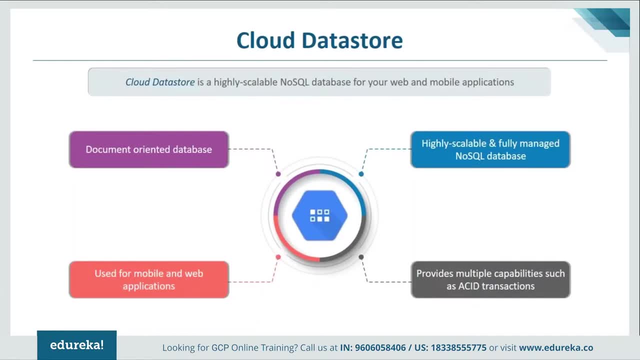 objects in cloud Data store are known as entities, and an entity has one or more named properties, Each of which can have one or more values. entities of the same kind do not need to have the same properties, and an entity's value for a given property do not need to be of the same data type- cloud data. 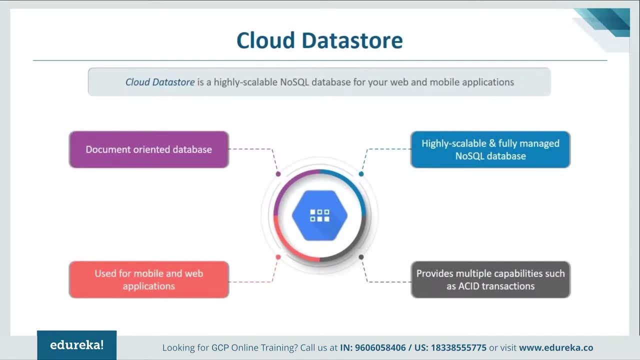 store supports a variety of data types for property values. These include the integers, floating point, number strings, dates and binary data. each entity in the cloud data store Has a key that uniquely identifies it. The key consists of the following components. Let us see. 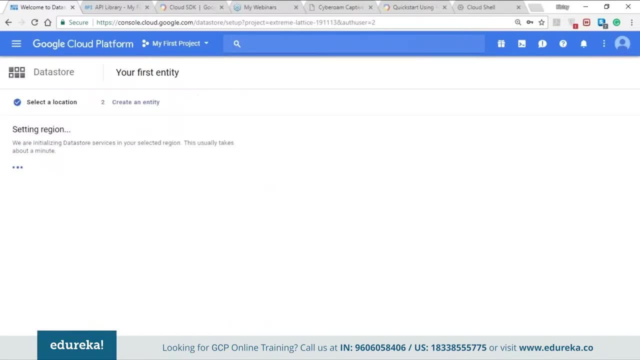 So first let's select a location- Now, entities are nothing but data objects in the cloud data store, As I mentioned earlier- or it is setting the region and we'll have to input the following identifiers for a particular entity. We have the namespace of the entity, which allows it for multi tenancy. 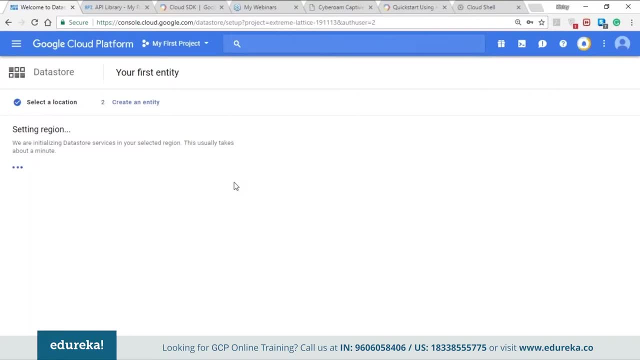 The kind of the entity which categorizes it for purposes of cloud data store queries. We have an identifier for the individual entity, which can either be a key or an integer, an optional ancestor path locating the entity within the cloud data store hierarchy. As you can see, here we have the namespace, the kind, the key identifier. 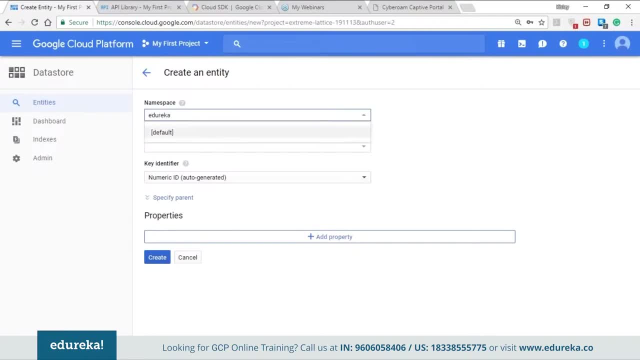 and the properties to be added. So let's input the name- The kind I'm entering is at demo, which will easily help me categorize it for future purposes. Now, key identifier can be numeric ID or a custom name- and just tap on the create button. 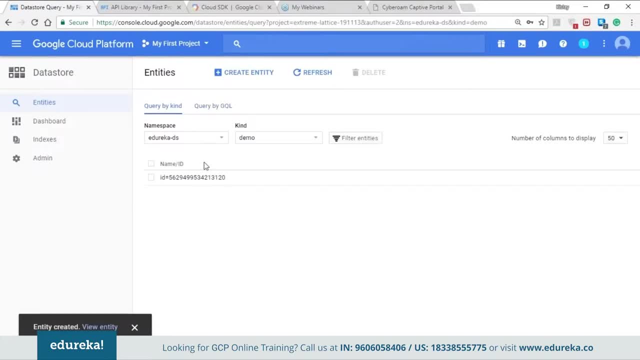 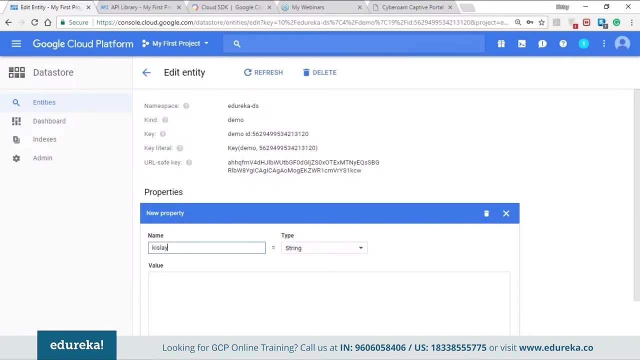 Now you have two options, which are query by kind or query by GQL. You can add properties such as for the name, I'll enter type string. You can add another property. Just click on the Save button. Now you have two options here: query by kind or query by GQL. 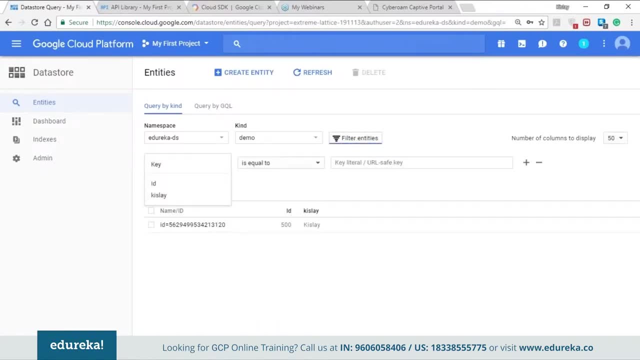 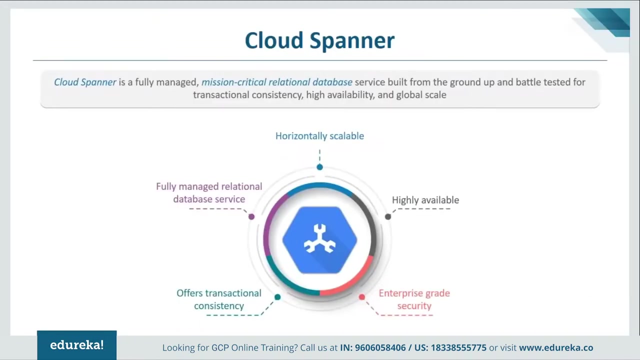 You can filter the entities here. apply filter, which is the key ID, is an integer equal to 500.. Applying filters, you will get the following output: Now that we have seen cloud data store, Let's go ahead and have a look at the cloud spanner. 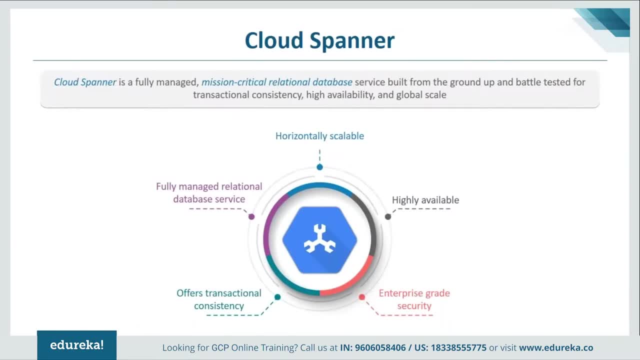 A cloud. spanner is a fully managed, mission-critical relational database service that offers transactional consistency At a global scale, schema SQL and automatic synchronous application for high availability. Cloud Spanner is the only enterprise-grade, global, distributed and strongly consistent database service built for the cloud specifically to combine 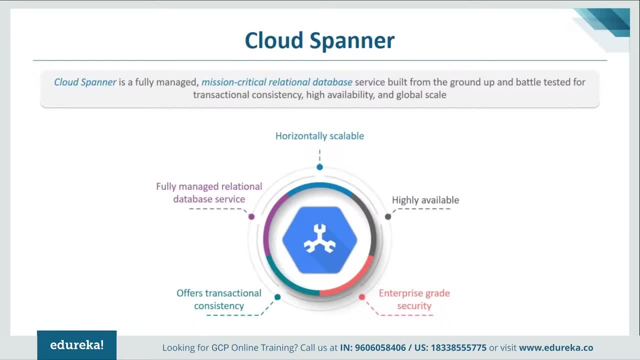 the benefits of both relational database structures with the non-relational based horizontal scale. This combination delivers high-performance transactions and strong consistency across rows, regions and continents, with an industry-leading 99.99% availability, SLA, No planned downtime and enterprise-grade security. 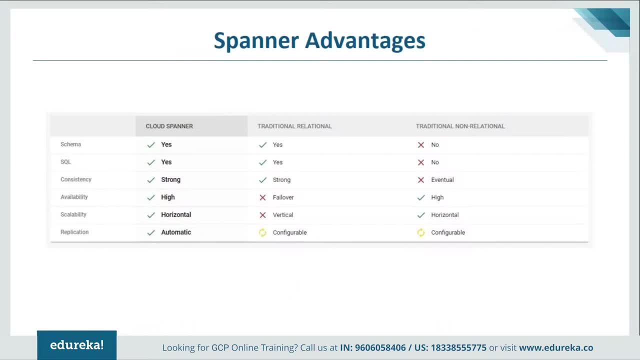 Now, as you can see here, the spanner gives a certain advantages over traditional relational database as well as traditional non-relational database. As you can see, in the traditional relational we cannot have high availability as well as scalability, And in traditional, non-relational. 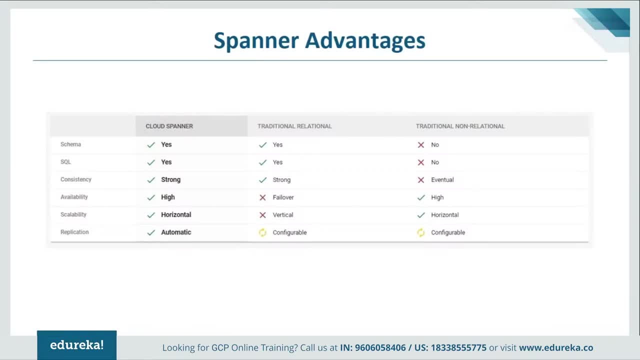 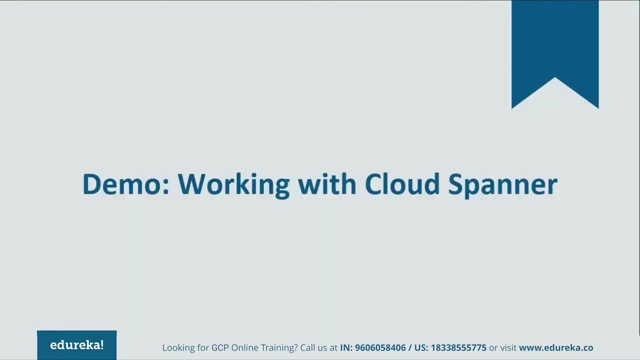 we cannot have a particular schema and we do not use SQL. But in cloud spanner we have the benefits of both the traditional relational and the traditional non-relational. Now let's go ahead and work with Google Cloud Spanner. Just go to the spanner. 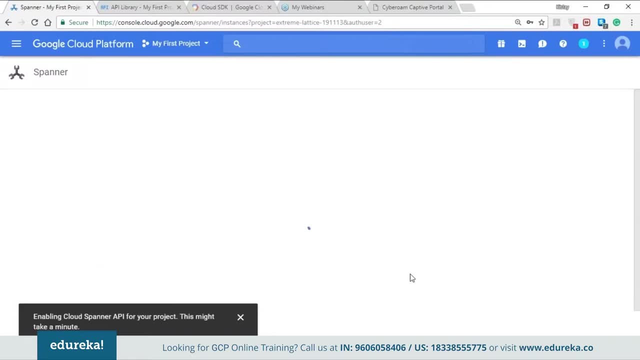 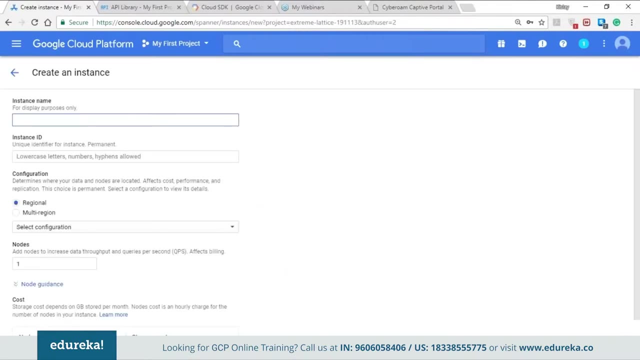 It automatically enables the cloud Spanner API for your project, So you do not have to do it manually. So now let's go ahead and create an instance. You can write the instance name. You can set up the configuration of regional or multi-regional. 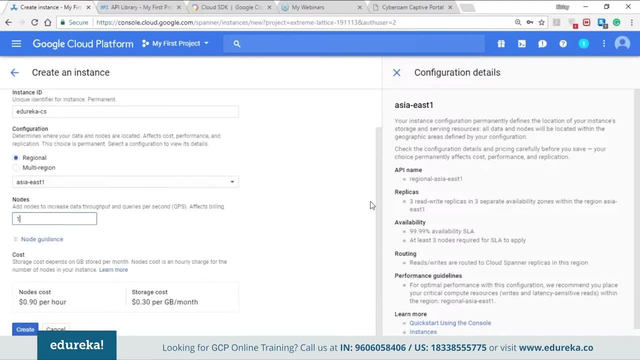 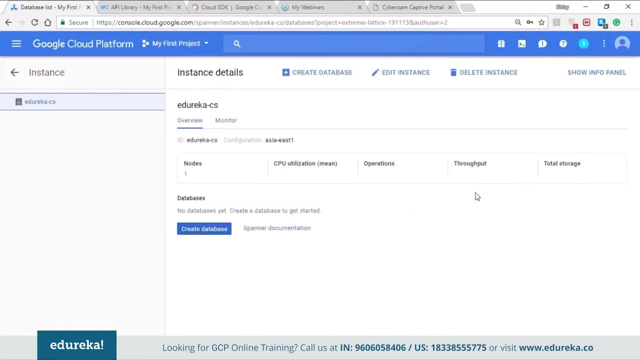 You can select the number of nodes. Just tap on the create button and it will create a cloud Spanner instance for you. So Spanner is very easy. You just need to tap on create database button and it will create a database. You can add a table. 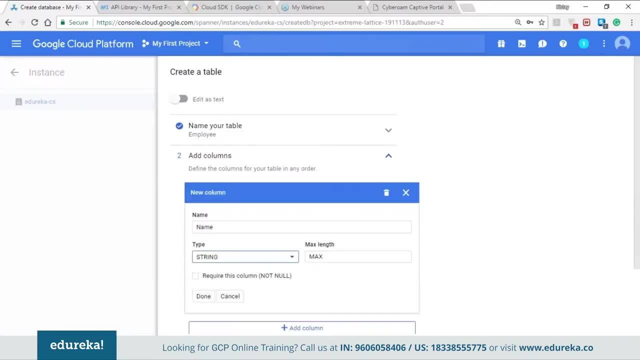 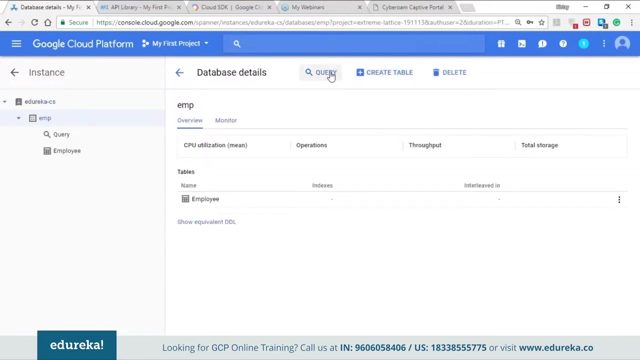 You can add columns here. You can also add columns here. So suppose you want to add the ID Also. you can set the primary key. Just tap on the create button And Spanner will automatically create the database for you. You can monitor your database or you can change the database. 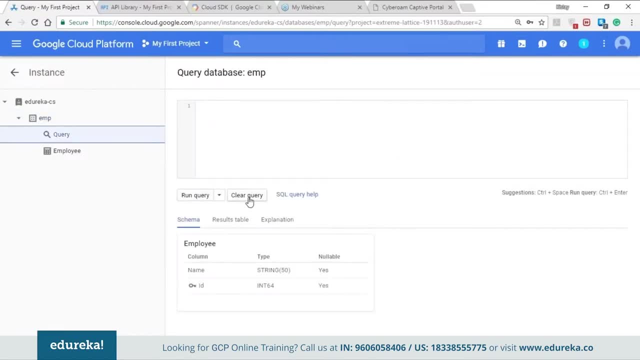 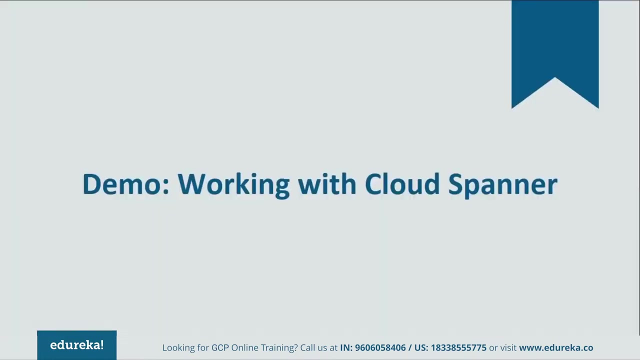 You can also query in a database. You can run a query from here or you can add it just by selecting the particular database and you can edit the schema. You can either add a column Or delete a column, or you can add values. Now that we have seen the cloud Spanner, 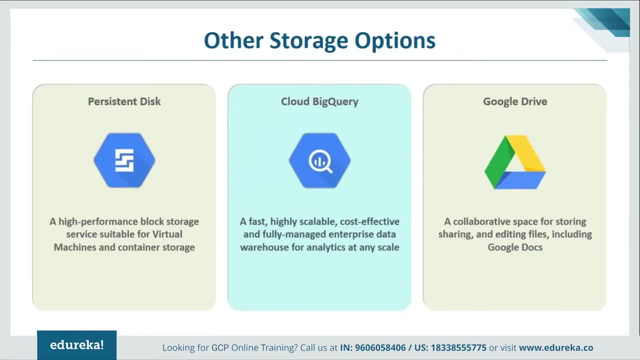 Here are some other useful cloud storage options. We have the persistent disk, cloud, BigQuery and the Google Drive. Now, persistent disk is a high-performance block storage service suitable for virtual machines and container storage. It offers unmatched price to performance ratio. You only pay for the capacity and you are never charged for the provisioned IOPS. 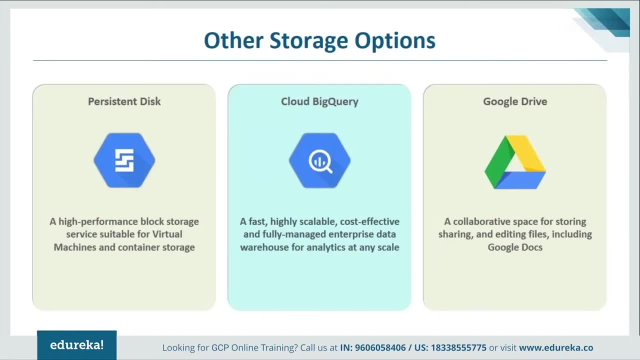 Additionally, persistent disk offers multi-readers, mounts and on-demand volume resizing to simplify operations. Now BigQuery is Google's fully managed, low-cost analytics data warehouse. It is serverless and there is no infrastructure to manage. No need to guess the needed capacity or over provision. 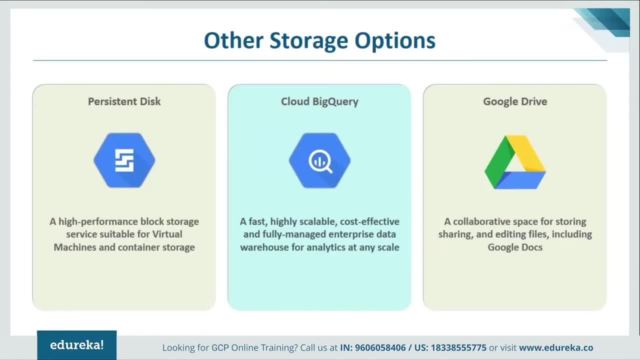 and you do not need a database administrator. You can focus on analyzing data to find meaningful insights. Now, finally, Google Drive is a collaborative space for storing, sharing and editing files, including Google Docs, with a 15 GB of space- 15 GB of storage space available for free accounts. 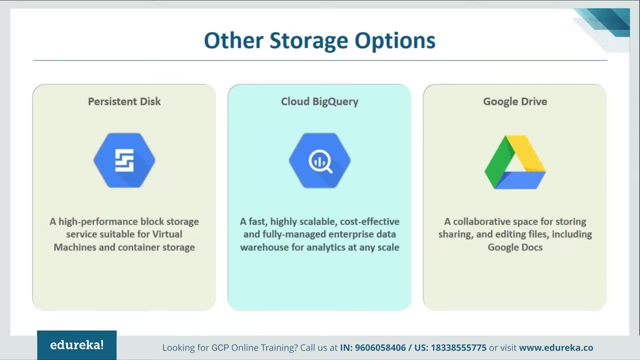 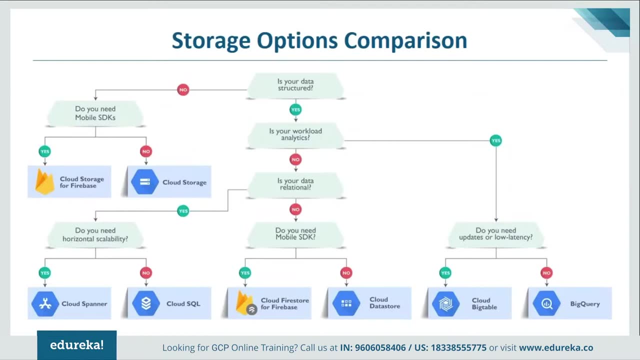 Now that we have seen all the services provided by GCP, Let's see exactly where and when these services are being used, As different application and workloads require different storage and database solution. Google offer a full suit of industry-leading storage services that are price performance. 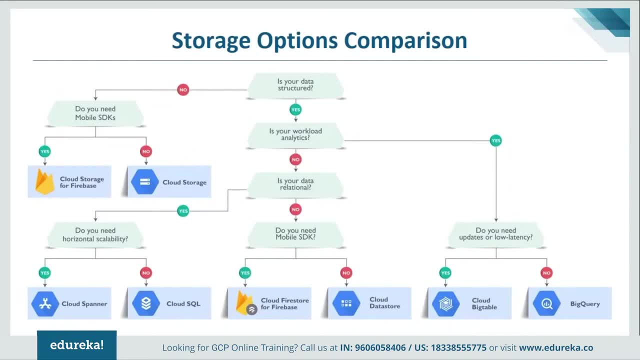 and meet your needs for structured, unstructured, transactional and relational data. The image given here helps you identify the solution that fit your scenarios, whether they are mobile applications, authentication, hosting commercial software data pipelines or storing backups. Now you might be wondering: what is Google Cloud Storage for Firebase? 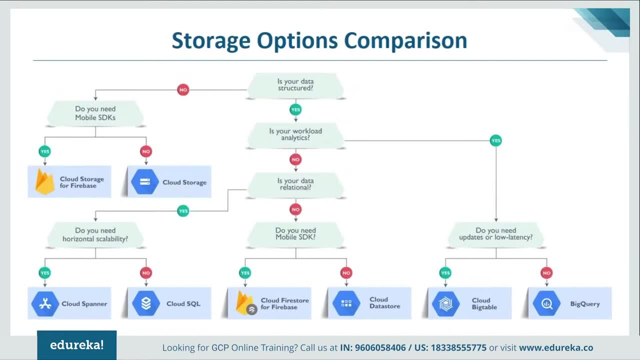 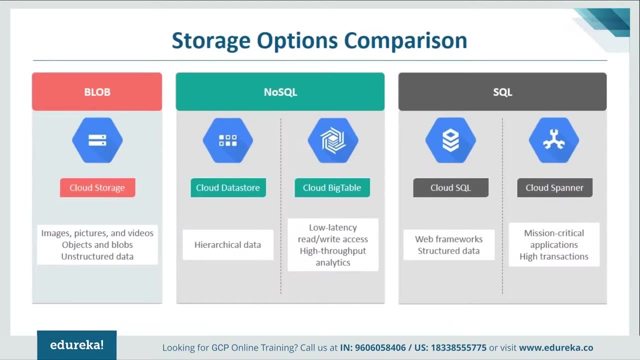 Now Firebase, mobile and web access to Google Cloud Storage with serverless third-party authentication and authorization. Now let us see when these storage are used and in which scenarios. First, if we want to store a blob type, we use the cloud storage to use images, pictures, videos, objects. 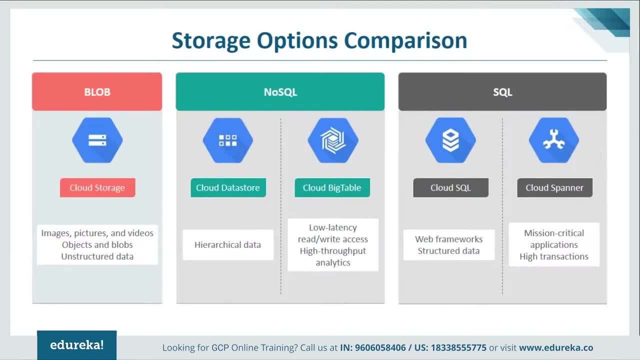 and unstructured data. When we come to NoSQL, we have the Cloud Datastore and the Cloud Bigtable. Cloud Datastore is used for hierarchical data and Cloud Bigtable is used for low-latency read and write access and high-throughput analytics. 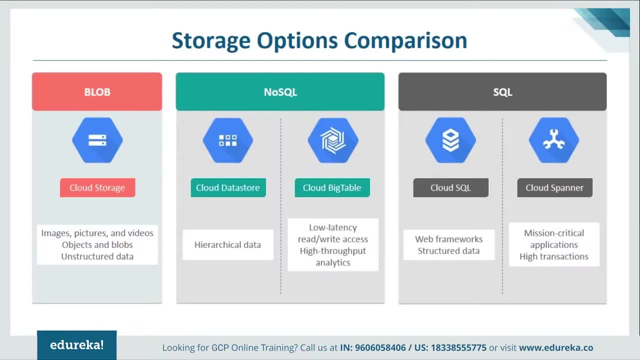 Coming to SQL, we have the Cloud SQL, which is the web framework for structured data, and Cloud Spanner, which is used for mission-critical applications and high transactions. Now Cloud Storage: the examples are storing and streaming multisystems, multimedia storing for data analytics load and disaster recovery. 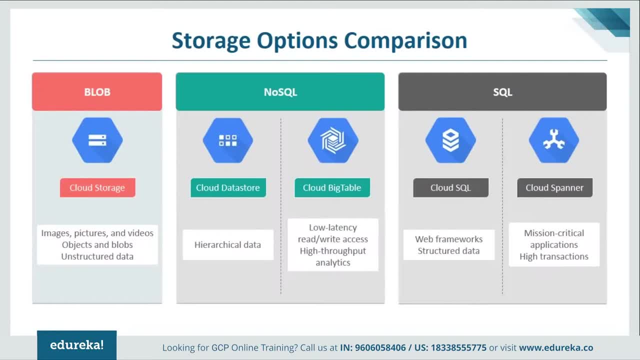 Coming on to Cloud Datastore. it is used for user profiles, product catalogs and game state. Now Cloud Bigtable is used for IoT finance personalization, recommendation, monitoring and graphs. Cloud SQL is used for blogs, content management websites. 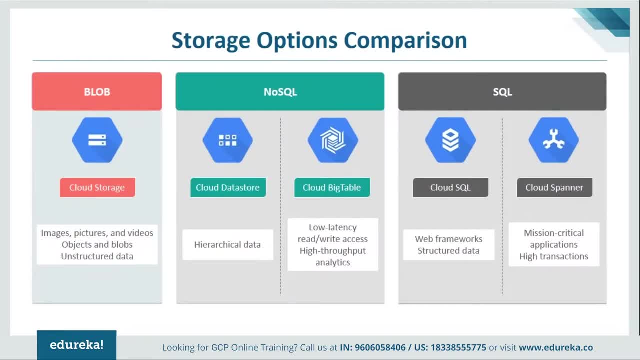 business intelligence application, CRM, ERP and e-commercial application. Coming on to Cloud Spanner, it is used for financial service, which are mission-critical- global supply chain and retail. Now we are left with the persistent disk. A persistent disk are used for virtual machines to share read-only access data across VMs. 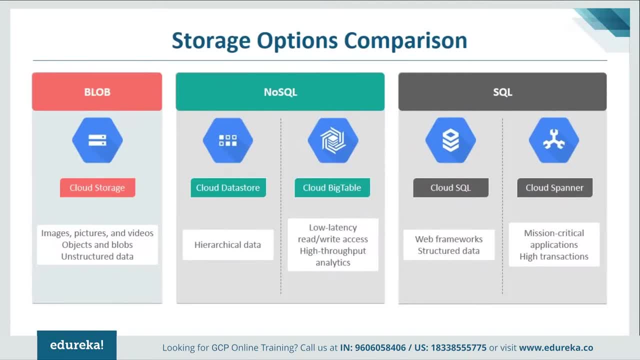 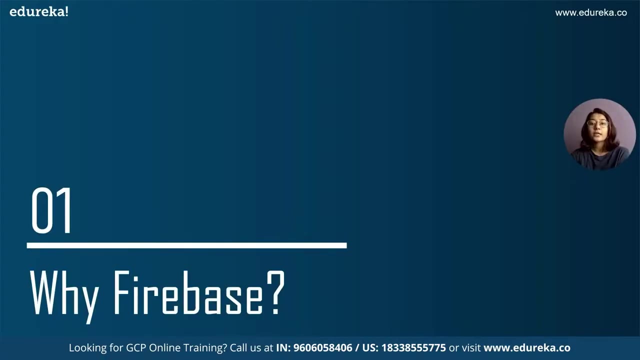 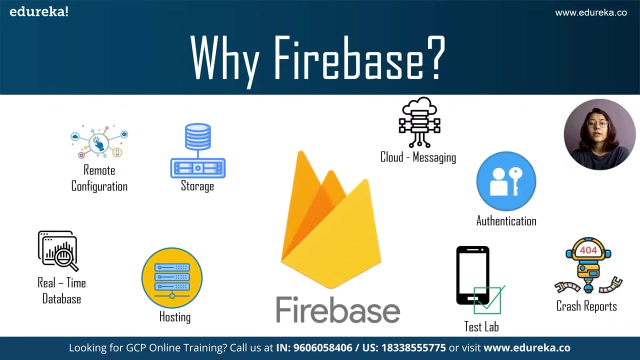 It is used as a backup of running VMs. Now BigQuery is used for large data analytical reporting, data science and analysis and big data processing using SQL. Why Firebase is used? Firebase is a Google-backed application development software that enables developers to develop iOS, Android and web applications. 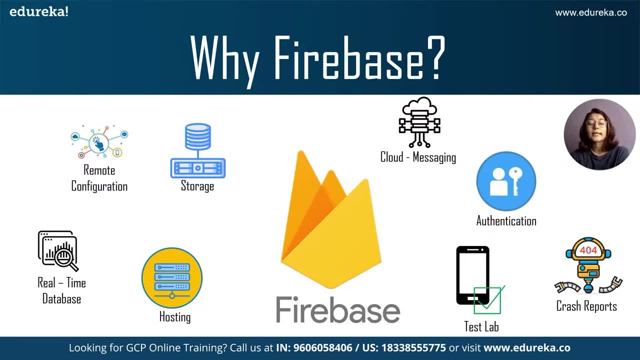 When you will get into the depth of application development on any platform, you will realize that you have some great ideas, but you don't have the resources to make those ideas a reality. Consider this: you want to make a web page and you will need to host it at some point. 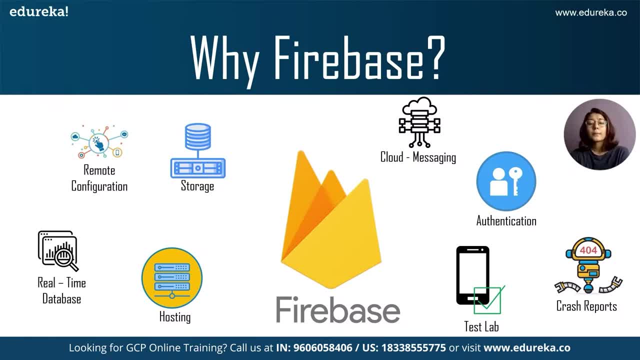 of the time for which you will need a server, But building your own custom server is a lot of pain for a front-end developer. Not only will you have to buy and keep your server online 24 by 7, but also create and manage the databases. 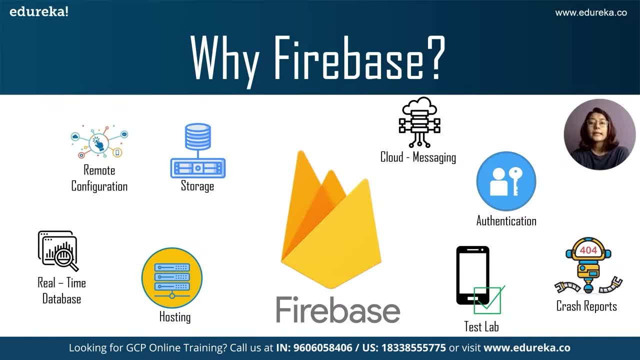 This is where Firebase comes to rescue. It not only takes care of all the problems that I just mentioned, but also provides you with lots of features that you can play with. Let's take a brief look at some of them. Firebase is based on a data structure used by the NoSQL database. 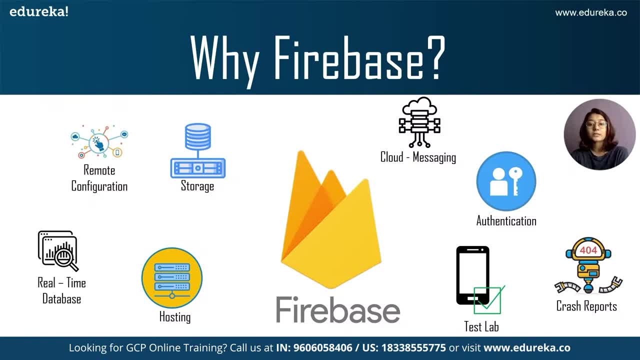 which is vastly different from those used in relational databases. Some operations are faster in NoSQL than relational databases like MySQL. As developers, you don't need to worry about the server-side software. Mobile and web SDKs enable this. The main offering is real-time sync of data between client apps and Firebase via. 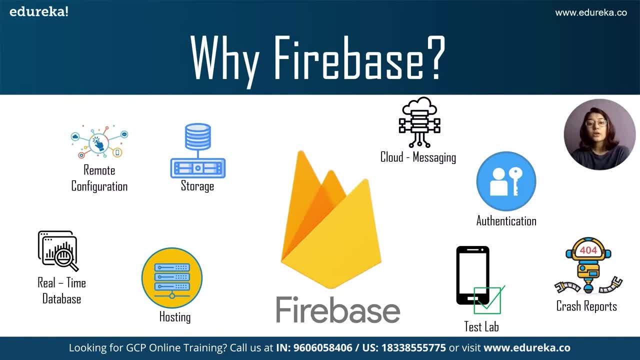 real-time database and cloud firestore Using authentication. user authentication feature is easy to build, even if it involves third-party providers such as Facebook or Twitter. Messaging and notifications are efficiently done using Firebase cloud messaging or FCM, Unlike native apps updated via app stores. remote config can update Firebase apps. 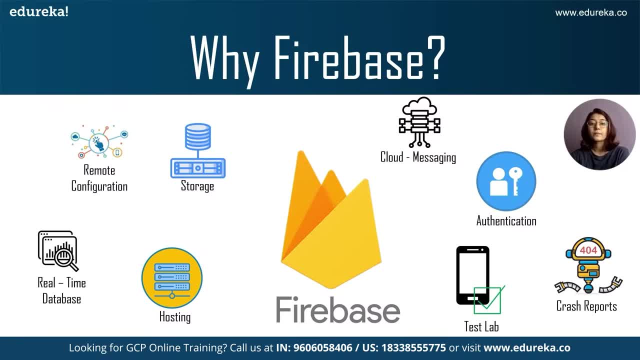 without asking the user to update their installation. In addition to this, web-based analytics and performance monitoring, app stability and performance can be improved. There's a good integration with AdWorbs and AdMob. Even UI testing across multiple devices is simplified via test labs. 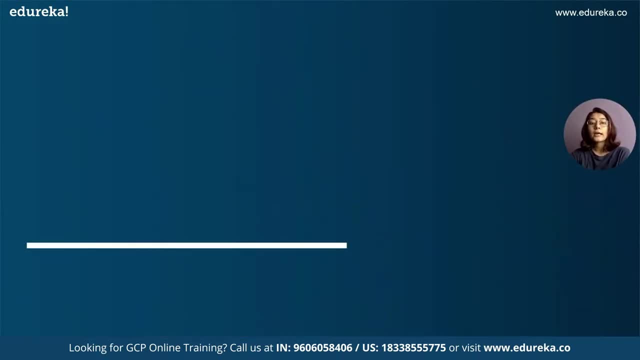 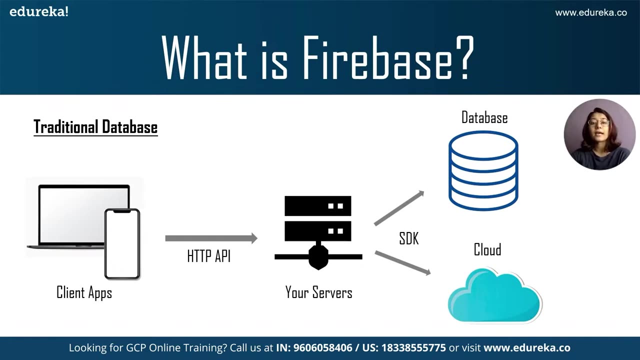 Now that we know why Firebase is so extensively used, let's take a look at what is Firebase. Modern web and mobile apps are typically built with a mix of backend services and frontend frameworks. Wouldn't it be nice if there was a way for developers to focus on just the frontend and user experience? 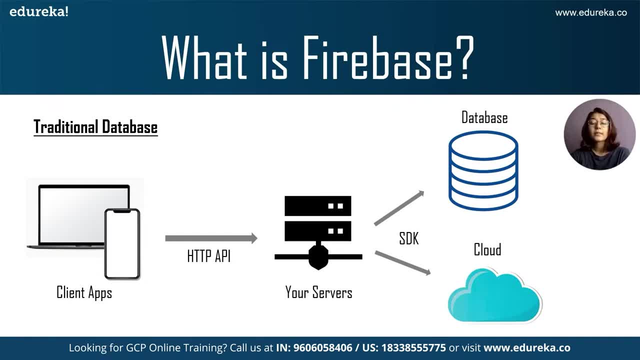 and let someone else take care of all the backend requirements. It's exactly in this context that backend as a service has emerged, that is, Firebase. Traditional app development typically involves writing both frontend and backend software. The frontend code just invokes the API endpoints exposed by the backend, and the backend code actually does the work. 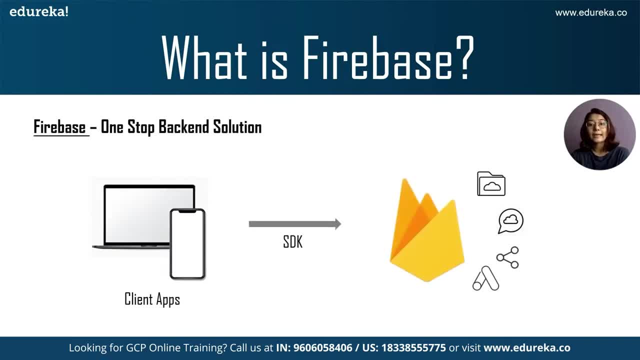 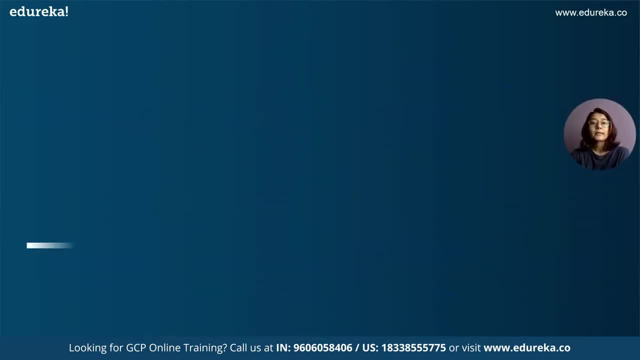 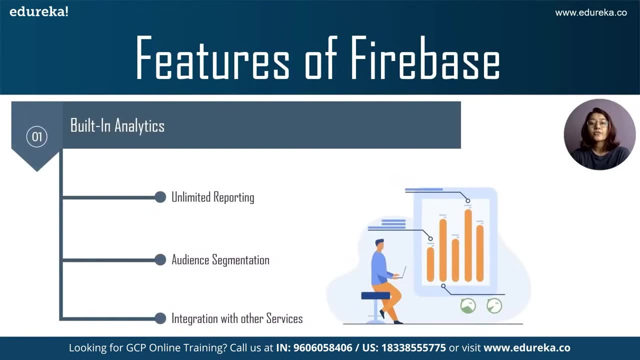 But with Firebase, your app accesses those servers directly or allows you to write APIs to handle that, if needed. Now that we know what Firebase is, let's take a look at the features of Firebase. First is built-in analytics. Google Analytics for Firebase is a free app measurement solution that provides insight on app usage and user engagement. 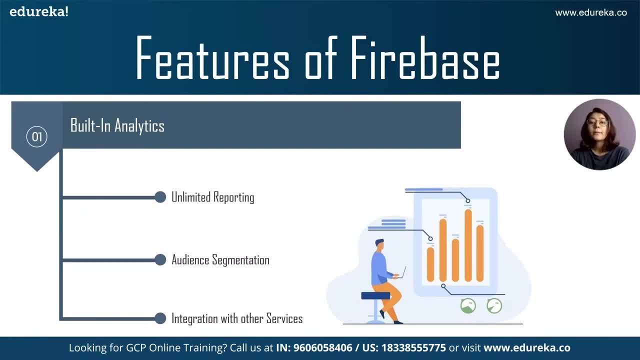 After you integrate the Firebase SDK with your app, basic app usage data is collected automatically and is available in Google Analytics and Google Analytics for Firebase. You don't need to add any code to enable automatically collected events, such as how many first opens, session starts or in-app purchases you've had. 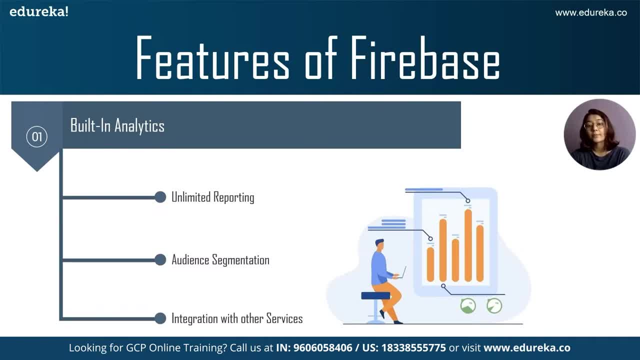 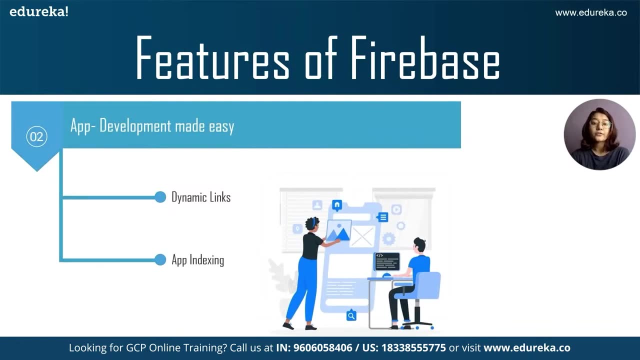 This lets you see how much time users have spent in your app, how many users were active during a certain period of time and how often in-app purchases were made. Next feature is app development made easy. Firebase offers a suite of tools required for businesses to build powerful applications. 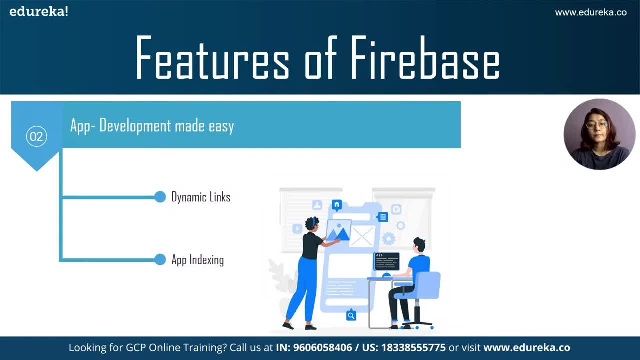 without having to worry about the management of infrastructure. It is designed to support backend developers at all stages of development and helps in improving the quality of the overall app development exercise. It provides a host of features and modules that an app developer needs as a service. 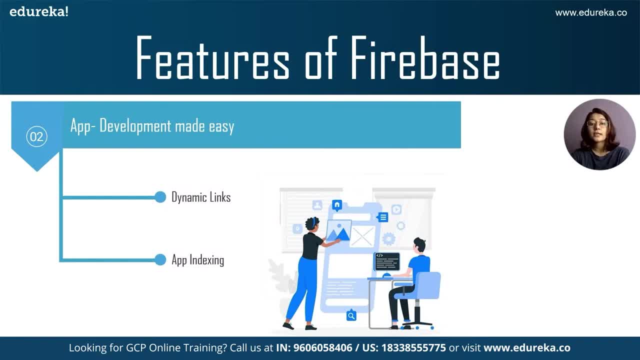 thereby eliminating the need to create these from scratch. Firebase is in no way a replacement for backend development activity, but it is rather a platform to help backend developers and engineers enhance the experience of the app without stressful coding and architectural planning. Our next feature is growth and user management. 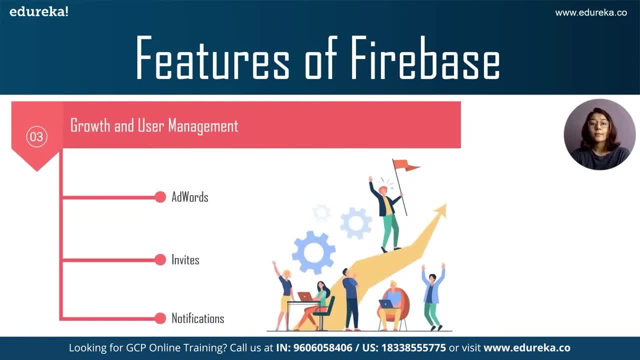 When you link your ads account to a Firebase project, you can create mobile application marketing lists based on analytics audiences. You can create audiences in Firebase using any combination of events and user properties and then use those audiences to run targeted ad campaigns. For example, you can create an audience of Android users who live in Canada. 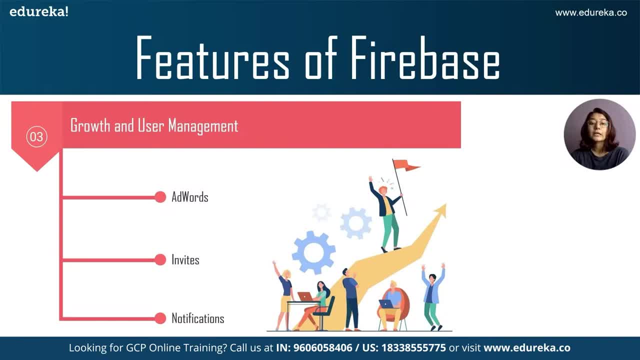 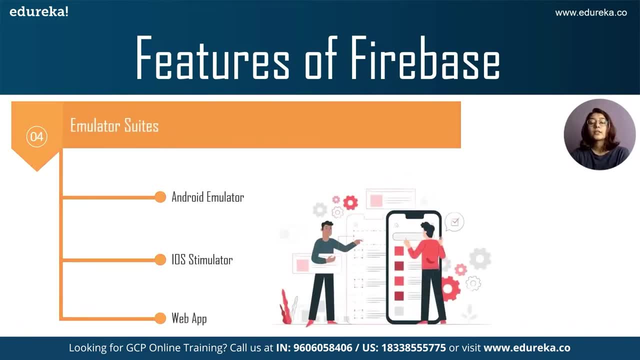 and then run ad campaigns directed at the users included in this audience. Yes, it's that simple. Our next feature is emulator suits. The Firebase local emulator suit consists of individual service emulators built to accurately mimic the behavior of Firebase services. This means you can connect your app directly to these emulators. 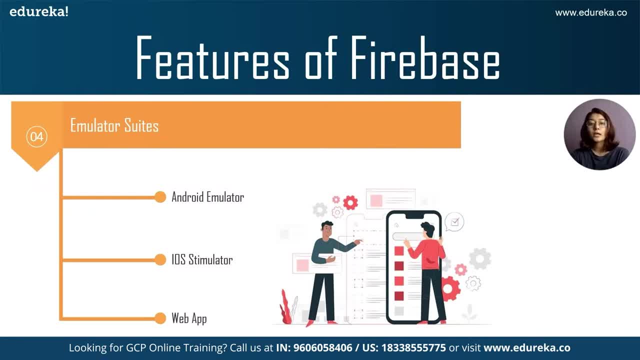 to perform integration testing or QA without touching production data. We need the Firestore emulator to safely read and write documents in testing. Since all services are connected to the local environment, these triggers the event, So these triggers the event in each other's services. 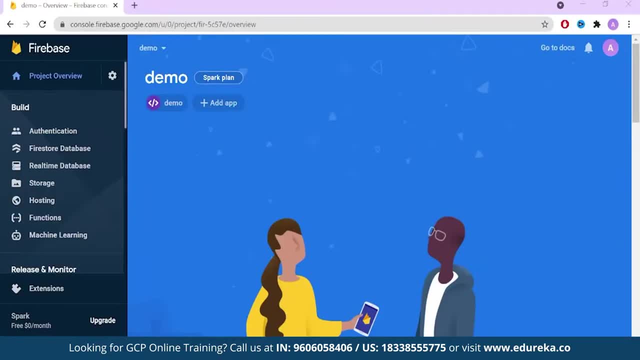 Now let's take a look at the Firebase interface After you make a project. this is what your interface will look like. I'll be showing you how we got here, but for now let's understand what all Firebase has to offer. 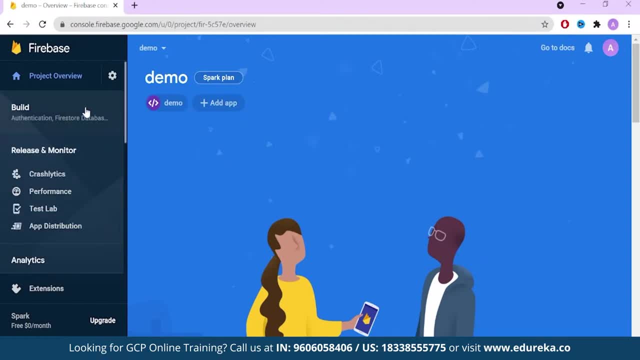 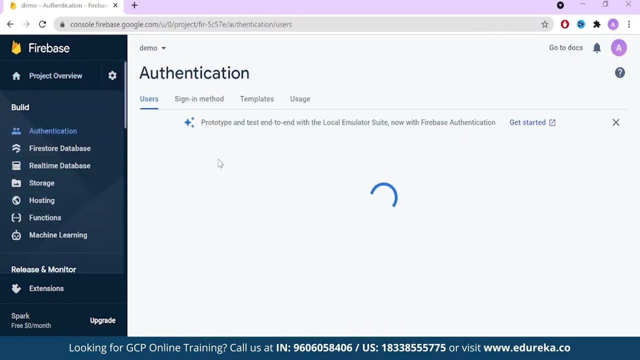 First, what we see here is build In build. we have authentication, Firestore, database and so on. First is Firebase authentication. Firebase authentication provides backend services, easy-to-use SDKs and ready-made UI libraries to authenticate users to your apps. 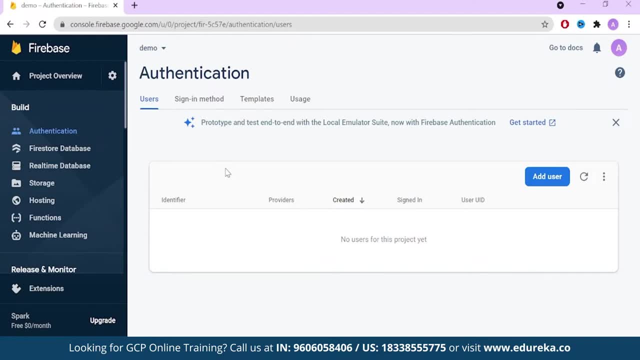 Normally it would take you months to set up your own authentication system And even after that you would need to keep a dedicated team to maintain that system. But if you use Firebase you can set up the entire system in under 10 lines of code. 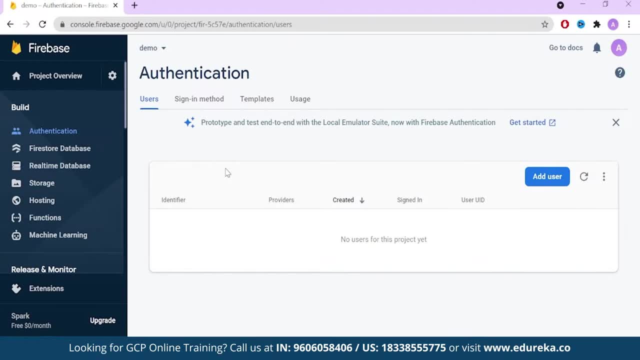 that will handle everything for you, including complex operations like account merging. Let's click on authentication. We can see here users, sign-in methods, templates and usage. Users are nothing but the number of people logged in to your database. Every single user has a unique ID which we can use to change the rules. 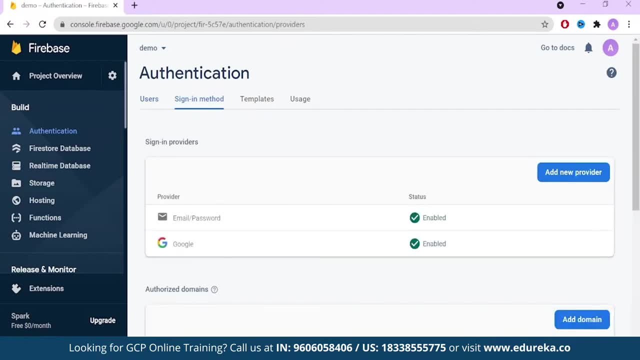 In sign-in methods, we can see a number of providers which we can incorporate in our applications, and it's really easy. All we have to do is add a new provider and enable it. Let's take a look at the Firestore database. 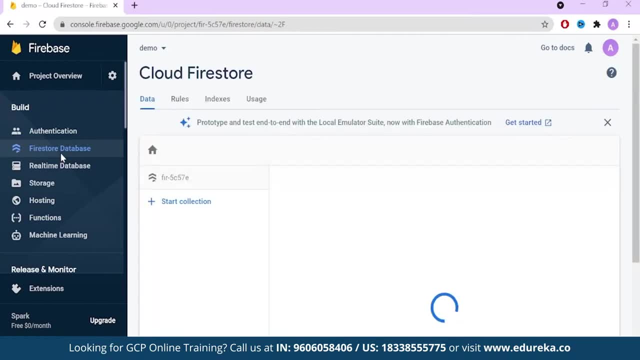 Firestore database is nothing but the Cloud Firestore, which is a no-SQL document database that lets you easily store sync and query data for your applications. Since this is a no-SQL document-oriented database, there are no tables or rows. Instead, you can store data in documents which are organized in collections. 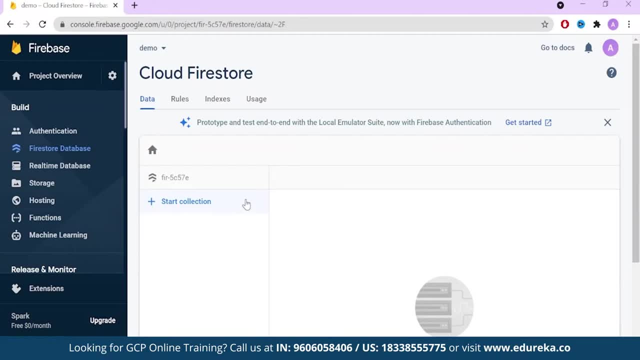 Each collection contains a set of key-value pairs. We also have security rules here. Security rules provide access control and data validation in a simple yet expressive format To build user-based and role-based access systems that keeps your users' data safe. 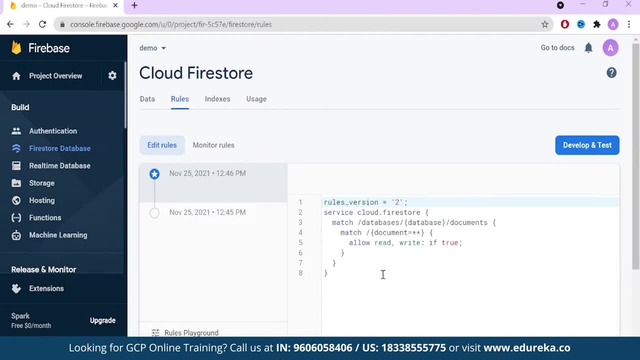 you need to use Firebase authentication with Cloud Firestore security rules. All Cloud Firestore security rules consist of match statements which identify documents in your database and allow expressions which control access to those documents. Every database request from a Cloud Firestore, mobile or web client library. 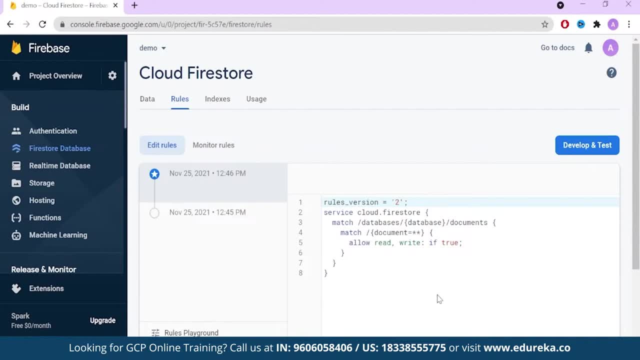 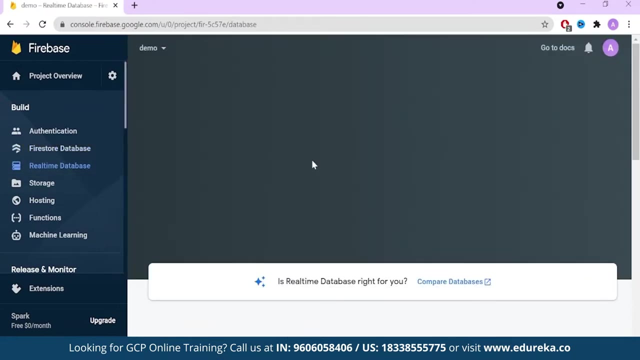 is evaluated against these security rules before reading or writing any data. If the rules deny access to any of the specified document paths, the entire request fails. Next is a real-time database. The real-time database is really just one big JSON object that allows you to access the data. 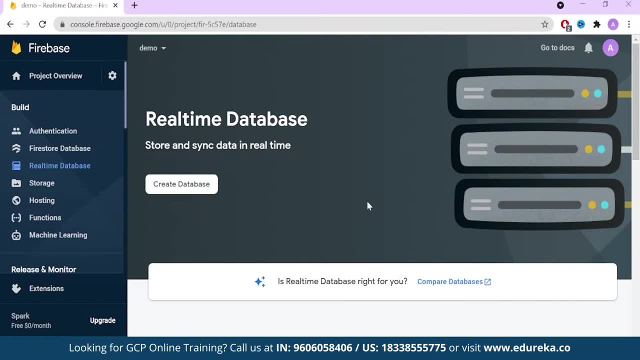 Next is a real-time database. The real-time database is really just one big JSON object that allows you to access the data With just a single API. the Firebase database provides your apps with both the current value of the data and any updates to that data. 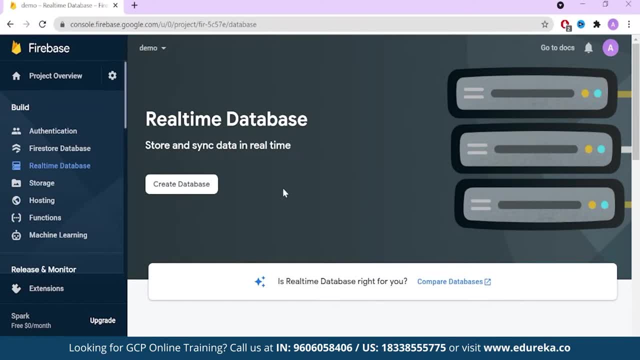 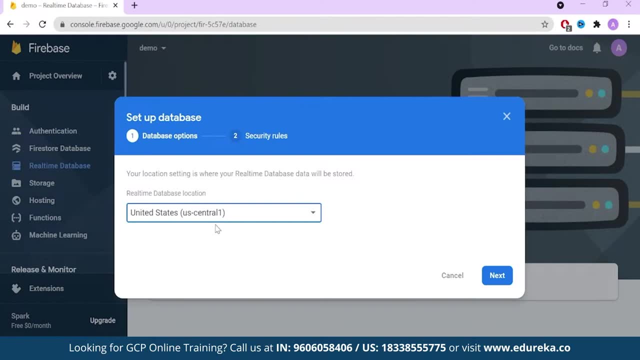 Real-time syncing makes it easier for your users to access their data from any device, So let's create a database here. So let's create a database here. We can select the location as. We can select the location as. We can select the location as. 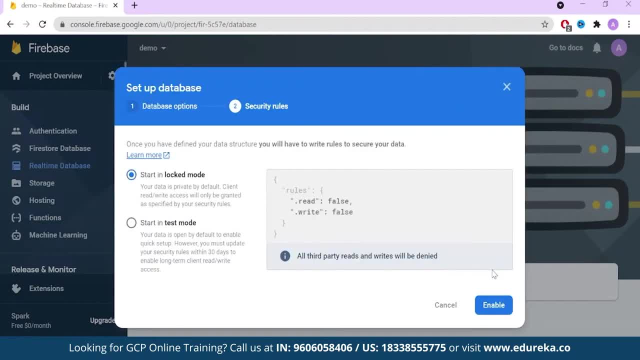 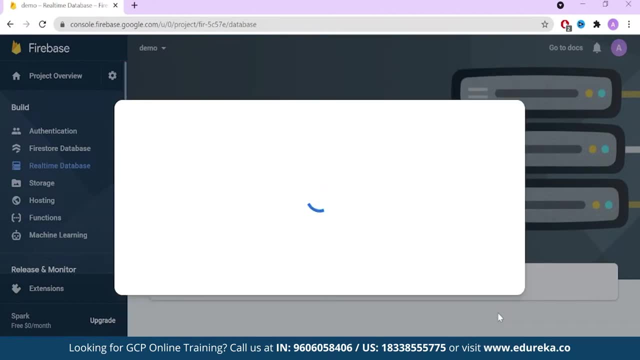 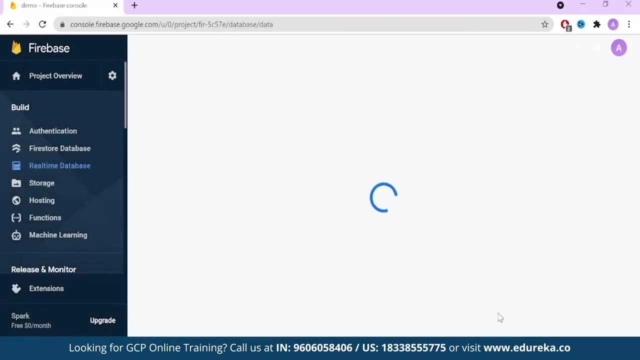 Let's keep it default for now. Let's keep it default for now. Click on next and we'll start this in test mode and enable this. So this will create our real-time database. Real-time syncing makes it easy for your users to access their data from any device, be it. 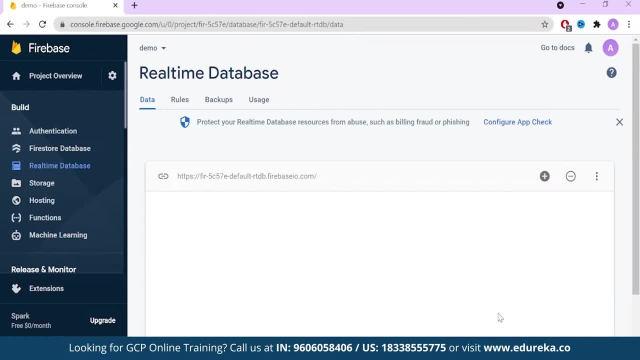 web or mobile Meaning. it lets you sync your data on any platform When your users go offline. the real-time database SDKs use local cache on the device to serve and store changes. When the device comes online, the local data is automatically synchronized. 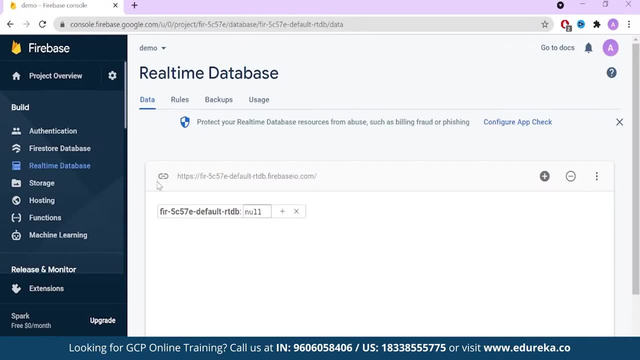 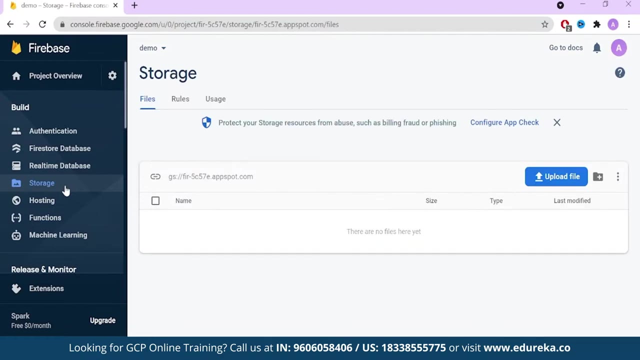 Its interface is similar to that of Cloud Firestore, consisting of data data security rules which we can change according to the need of our project. Next is storage Firebase. Storage is a standalone solution for uploading user-generated content like images and videos from an iOS and Android device, as well as the web. 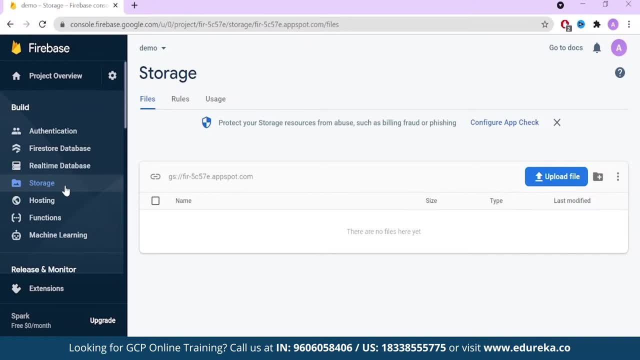 Firebase Storage is designed specifically for cloud storage. Firebase Storage is designed specifically for cloud storage, as well as the web. Firebase Storage is designed specifically for cloud storage, as well as the web. Firebase Storage is designed specifically to scale your apps, provide security and. 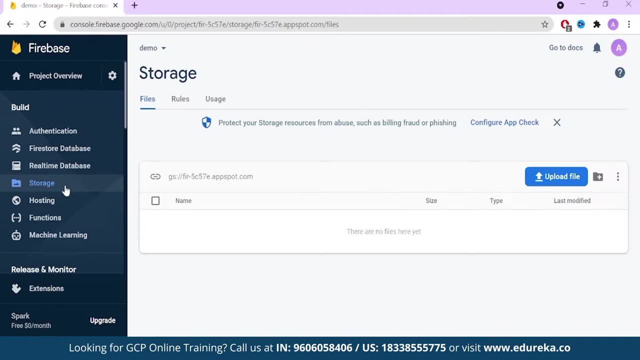 ensure network resiliency. Firebase Storage uses a simple folder or file system to structure its data. You can easily upload the required files from your system and it can be accessed from any device. We can also have rules here which play the same function as we saw in the Cloud Firestore. 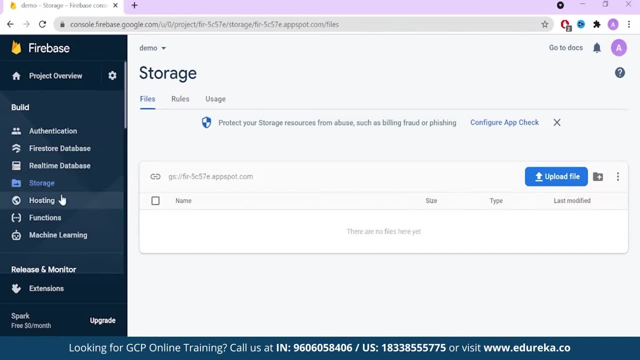 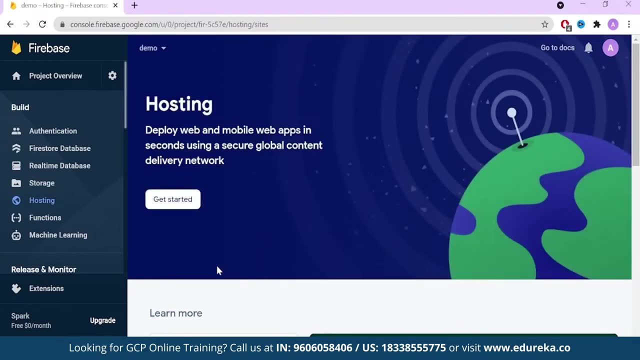 and real-time database. Next is Firebase Hosting. It is a secure global web-based database. It is a secure global web hosting CDN or content delivery network, which is really good at quickly delivering static content like HTML, CSS or JavaScript. 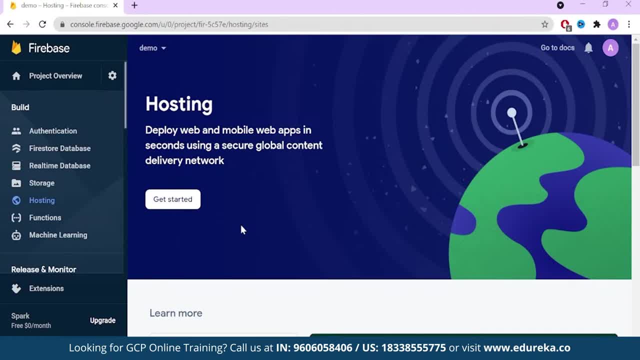 Next is Firebase Hosting. It is a secure global web hosting CDN or content delivery network, which is really good at quickly delivering static content like HTML, CSS or JavaScript using servers that are close to your users, And you can get it set up quickly with or without a server. Next is mailbox also, which is a secure global web-based database. It is a secure global web hosting CDN or content delivery network, which is really good at quickly delivering static content like HTML, CSS or JavaScript using servers. 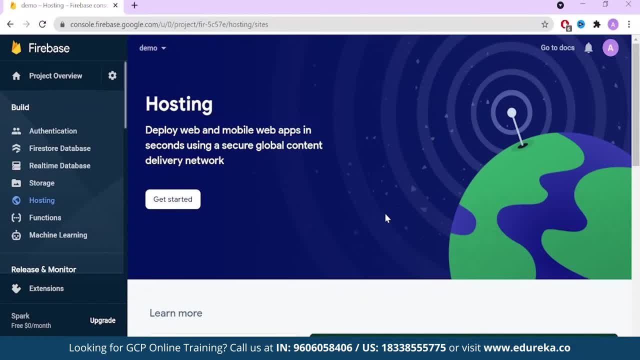 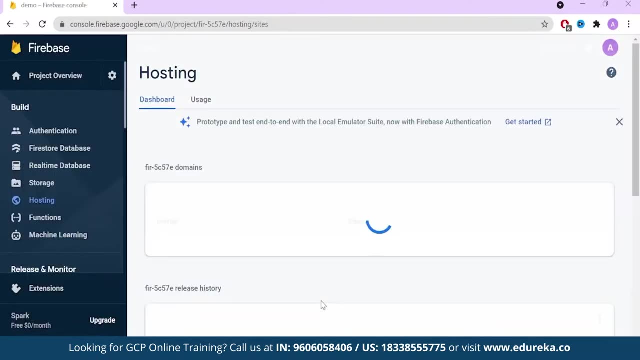 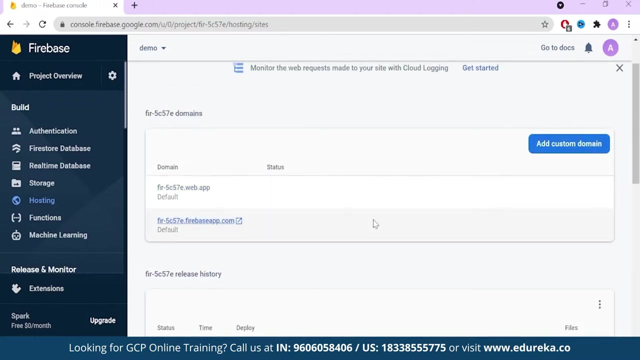 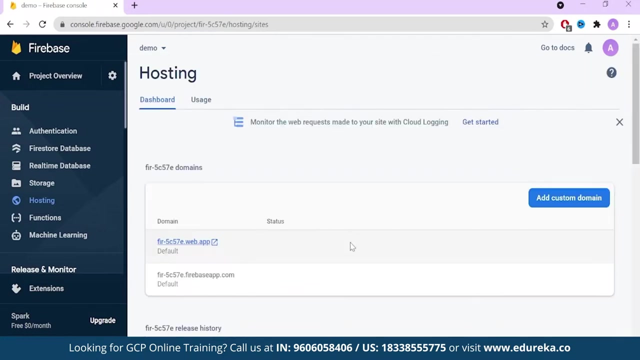 that are close to your users. Next is Microsoft Stylized Administrator. Almost all users in the language will be able to access that dashboard. Next is Cooldown. Next is SAP Storage. Next is AppStore. Next is Salesforce: status of your application- okay, next we have here is the cloud functions: firebase cloud functions. 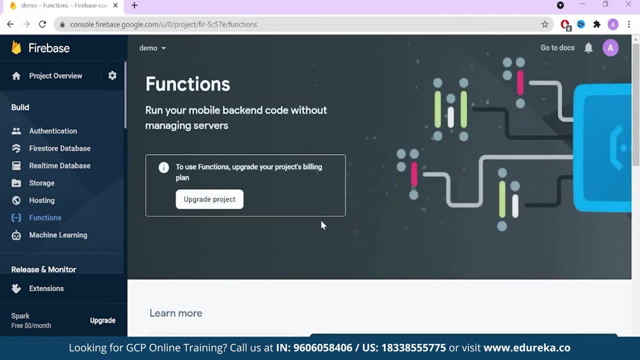 refer to a serverless framework that enables developers to execute back-end code for responding to https and firebase feature triggered events. google cloud is used for storing typescript or javascript code and can be executed within a managed environment. this reduces the requirement for scaling and managing servers. cloud functions are only available on the blaze plan and a user. 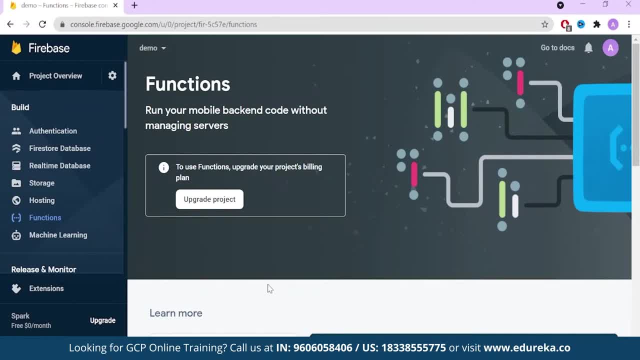 cannot try the service under the spark plan. it is important to emphasize a free quota for cloud functions, but charges will happen under the blaze plan as soon as the user exceeds the free limit. we will learn more about blaze and spark plans as the session progresses. for now, you just need: 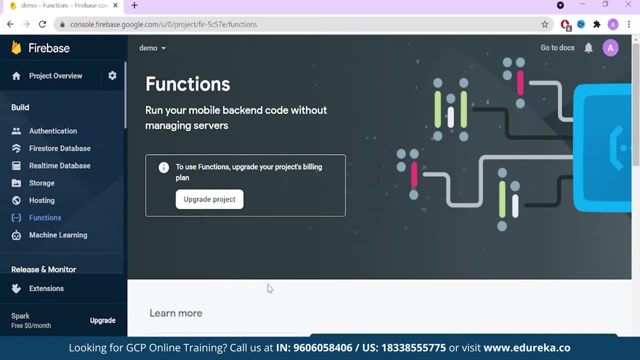 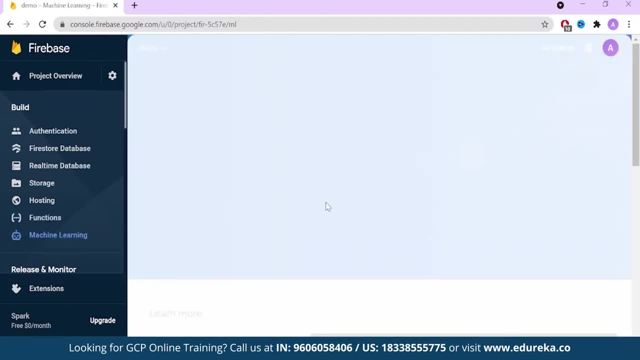 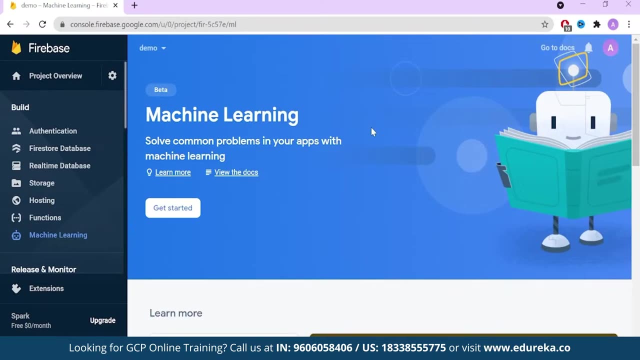 to understand that to use cloud functions you need to upgrade your project from the spark plan to blaze plan. next we have is machine learning. firebase machine learning is a mobile sdk that brings google's machine learning expertise to android and apple apps. it is a powerful yet easy. 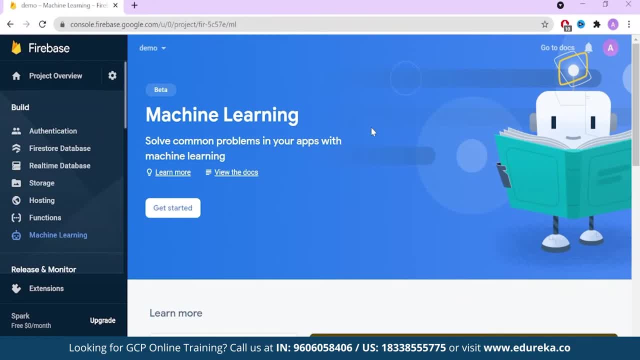 to use package. whether you are new or experienced in machine learning, you can implement the functionality you need in just a few lines of code. let's move on under release and monitor. we have a lot of applications like test labs and app distribution. crashalytics is a real-time crash. 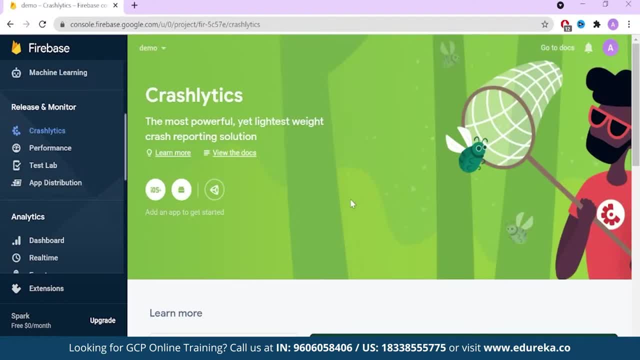 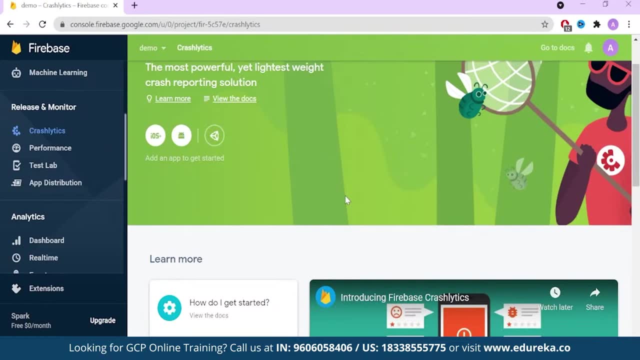 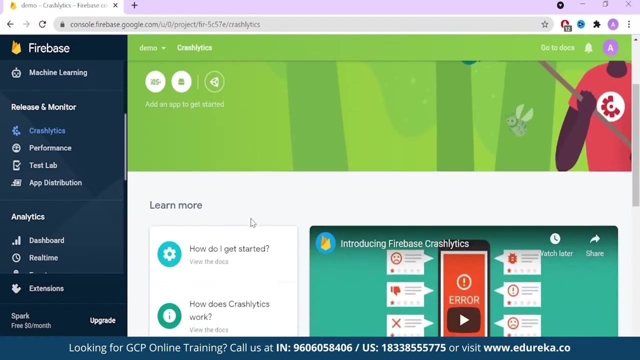 reporting tool that helps you prioritize and fix your most pervasive crashes based on the impact on real-time users. crashalytics can also be easily integrated into your android, ios, mac os, tv os or and watch os applications. next is test labs. firebase test labs have this amazing service. 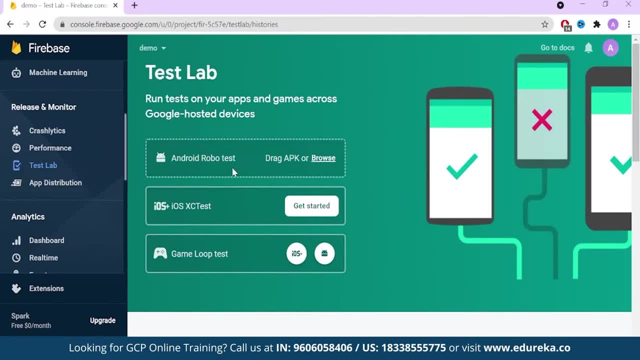 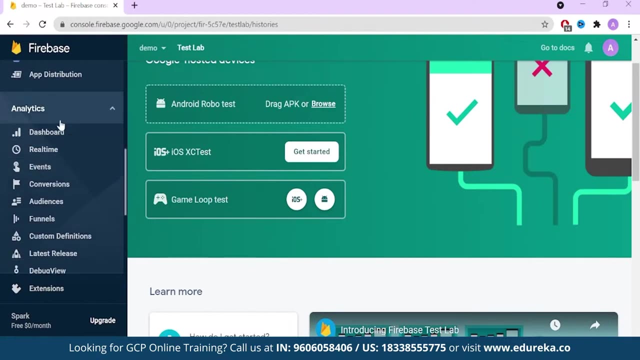 robotest. this allows us to test our app without having to write any test scripts. with robotest, we can have firebase test your app completely, even fill in specific form fields and push buttons. moving along under analytics, we have dashboard, real-time events, conversations and so on. analytics surfaces data about user behavior in your ios and android applications, enabling 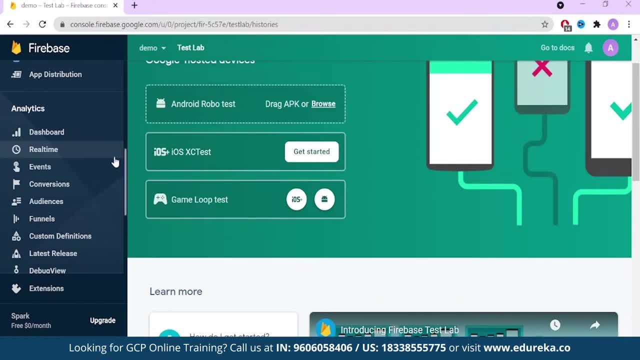 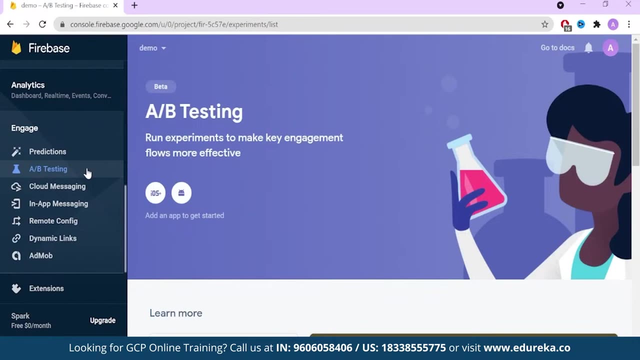 you to make better decisions about your product and marketing optimization. in engage we have tabs like prediction, a b testing, cloud messaging, etc. under a b testing. this helps you improve your app by making it easy to run, analyze and scale products and marketing experiments through firebase you can. 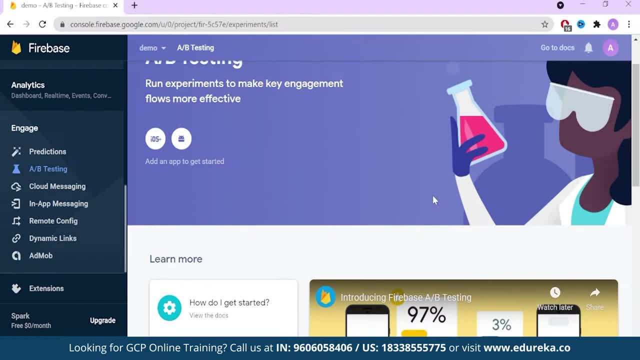 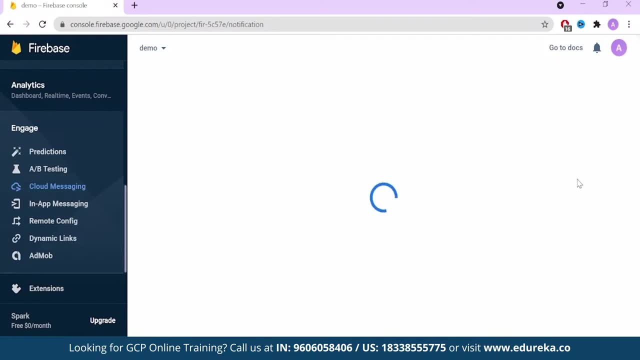 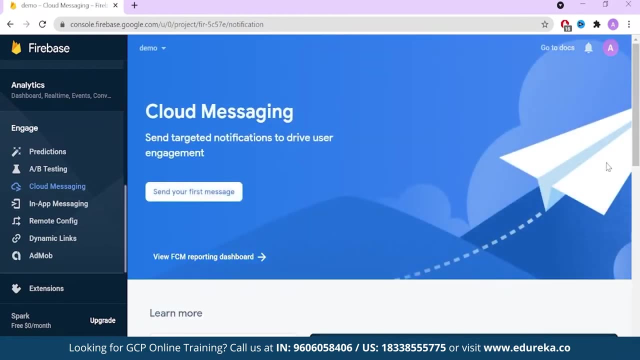 test your applications user interface features that you might have added. let's move on to cloud messaging. our firebase cloud messaging, or fcm, provides a reliable and battery efficient connection between your server and devices that allows you to deliver and receive messages and notifications on any device for free. next is remote config. remote configuration essentially allows us to publish. 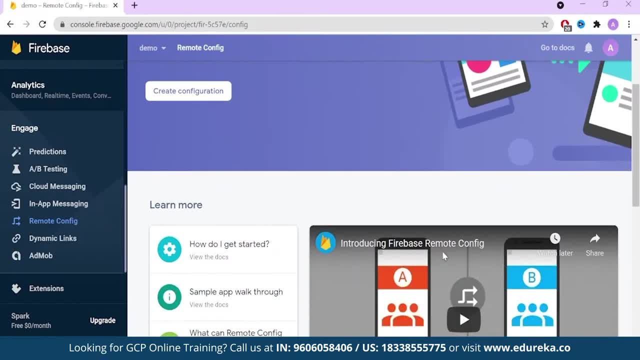 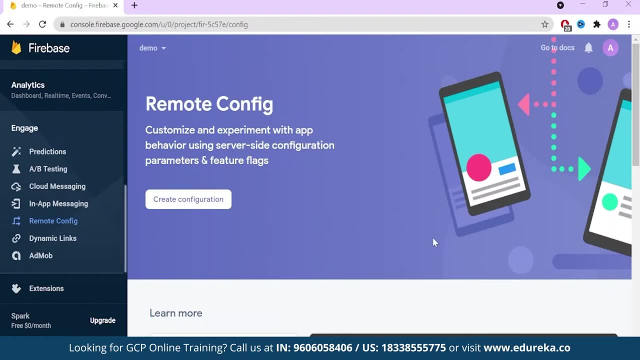 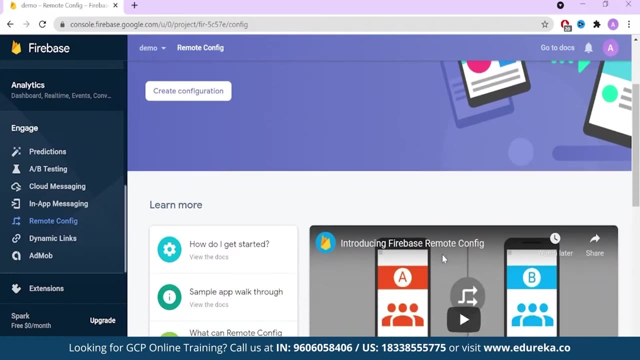 updates to our users immediately. whether we wish to change the color scheme for a screen, the layout for any particular section in our application or show promotions, we can change the color scheme for show promotional or seasonal options. this is completely doable using the server side parameters without the need to publish a new version. now that we know the firebase console, let's take a look at a 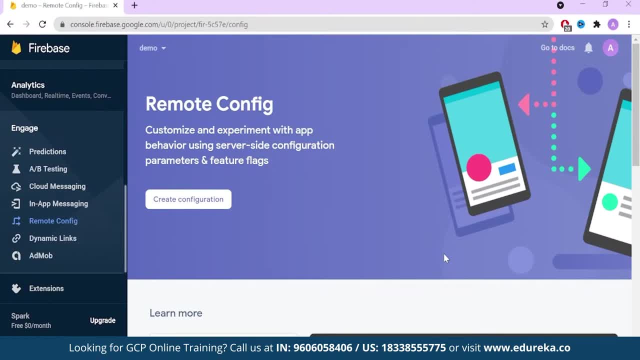 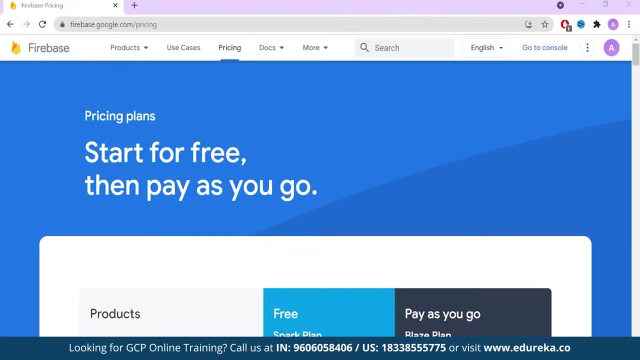 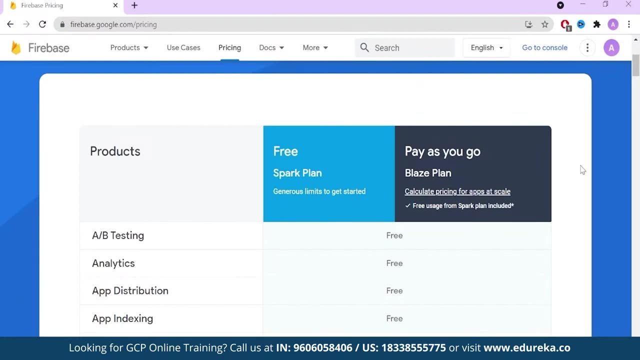 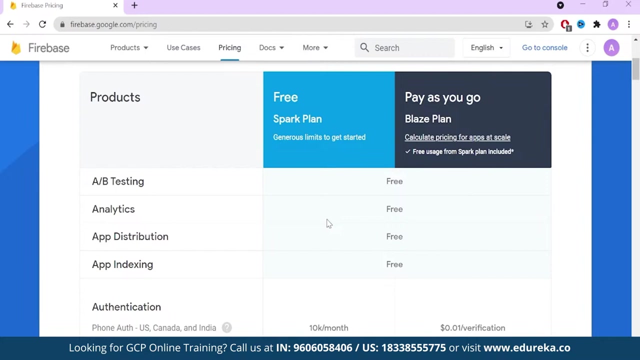 little hands-on in which we will build a website from scratch and use firebase functions on it. let's take a look at the firebase pricing plans. so firebase has two major plans. uh, one that is free is called a spark plan and the other one is called the blaze plan, which is pay as you go. spark plan offers 1 gb total storage- 22k writes. 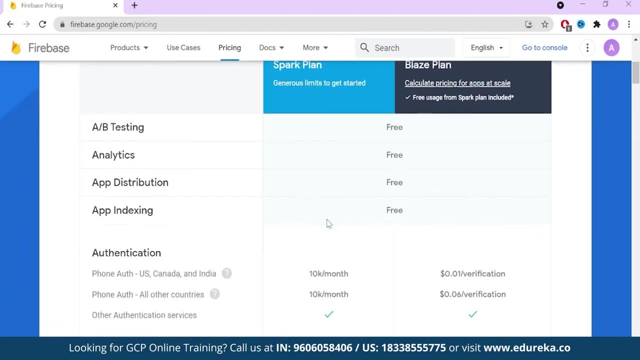 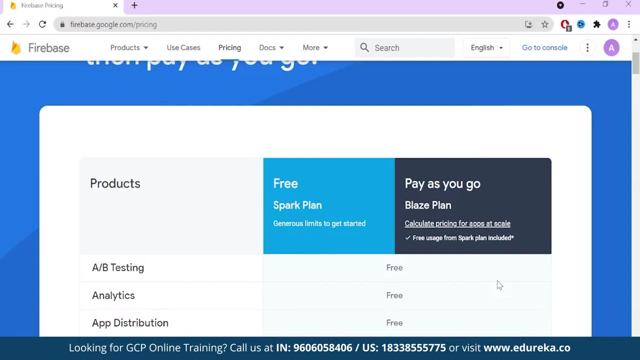 per day, 52k reads per day and 22k deletes per day. blaze plan charges 0.18 per gb, which is 13 rupees per gb, for database storage, 0.026 per gb, which is roughly 2 rupees per gb, for application storage. and additional charges for database storage and low source. thank you, someone for supporting an account. i've put the link in the description for you. that's why i put this link in the description, so that you do not miss any. Connect action next asks a few questions, especially in a build over system. 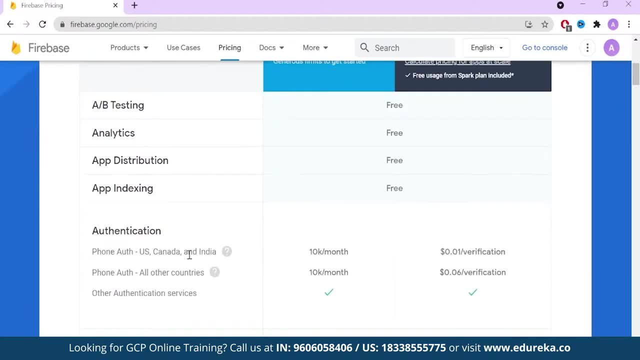 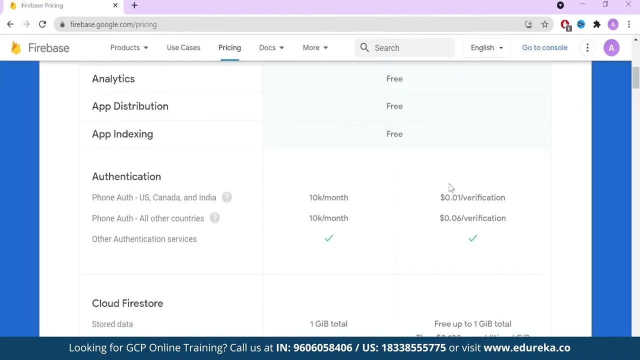 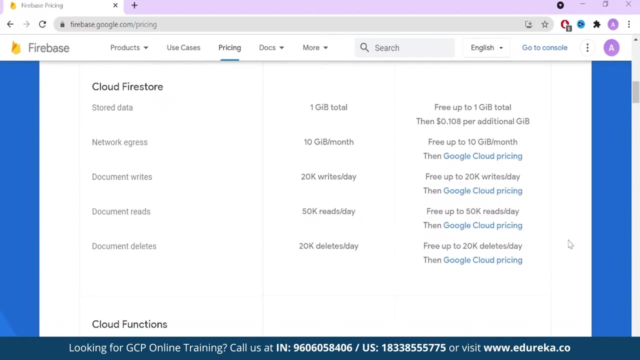 database operations and data transfer. Firebase provides 10,000 authentications per month And beyond that it charges a different rate depending on our region. Cloud Firestore provides a total of 1 GB storage In the Blazendan. there is a charge for storage. 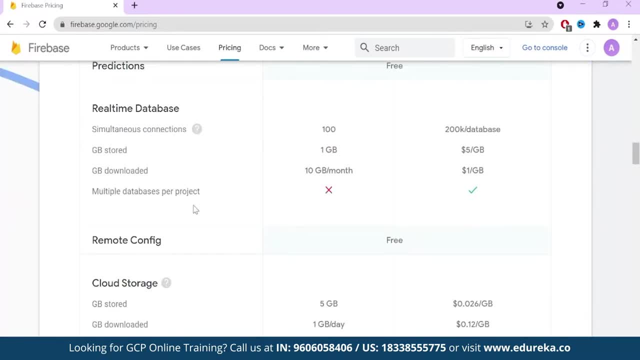 Space and database operations are priced separately. The Firebase Realtime Database provides free and unlimited reads and write operations. Google hosts your Firebase app free in the Spark plan And in the Blazendan. charges a modest fee per GB of application data stored and data transferred. 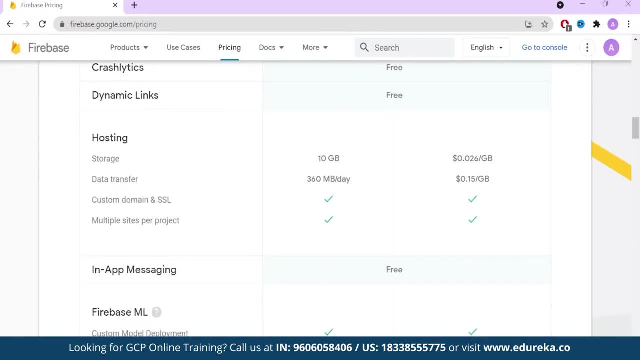 Both plans provide free SSL and multiple sites per project. The Google Machine Learning Kit is available in Firebase for up to 1,000 images per project and can be useful for a variety of image processing tasks. Google Test Lab is available five times a day. 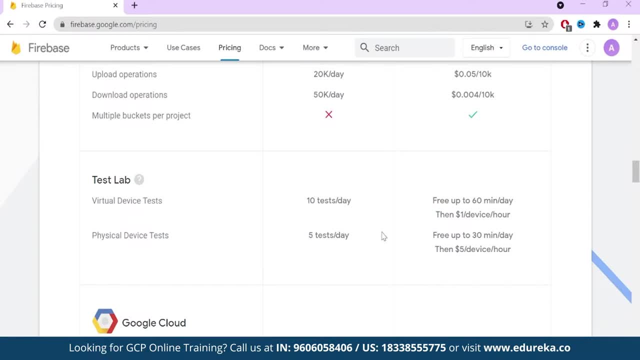 for real devices And 10 times a day for virtual devices. Firebase provides the Usage tab in its console, which shows the status of your payment and uses for various Firebase services. To sum it up, the pricing plan, that is, the Spark plan. 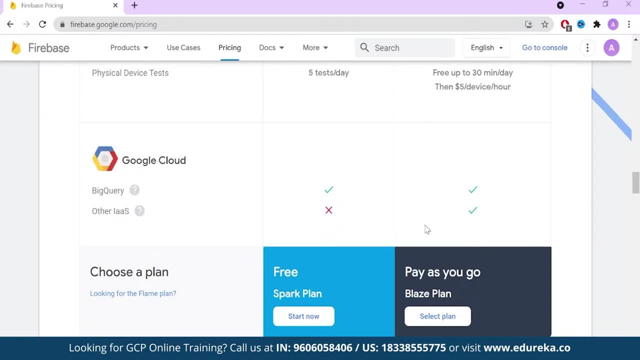 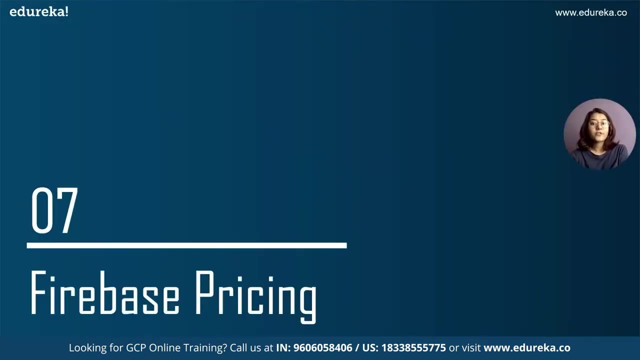 incorporates a limited free tier And it's an excellent option for development and small applications. The second tier, which is the Blaze plan, works on a pay-as-you-grow model And it's ideal for production applications. Now let's take a look at the companies using Firebase. 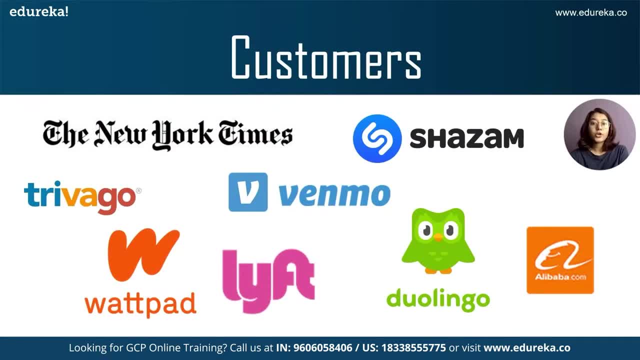 Famous companies like Trivago, Duolingo, the New York Times, use Firebase for application development, analytics and other database features. One of the reasons why Firebase is so widely used is because Firebase needs minimal coding knowledge and recommends integration through its user interface. 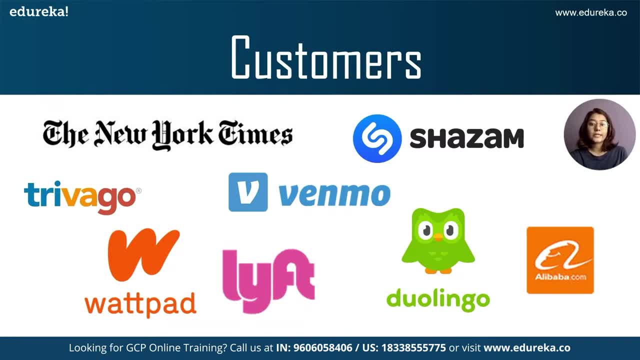 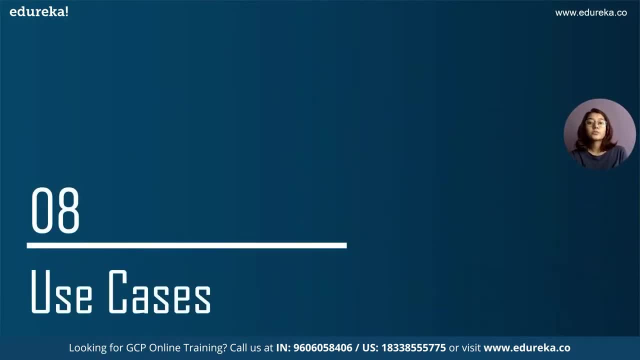 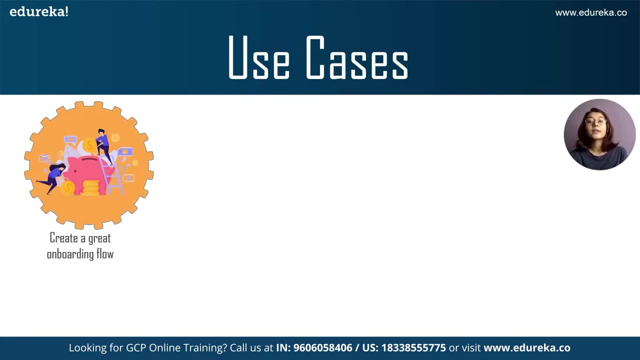 This feature eliminates the requirement for complex configurations and allows you to easily set up the platform. Now let's take a look at some of the use cases. Creates an onboarding flow Firebase. enables the developers to programmatically create dynamic links with custom parameters. 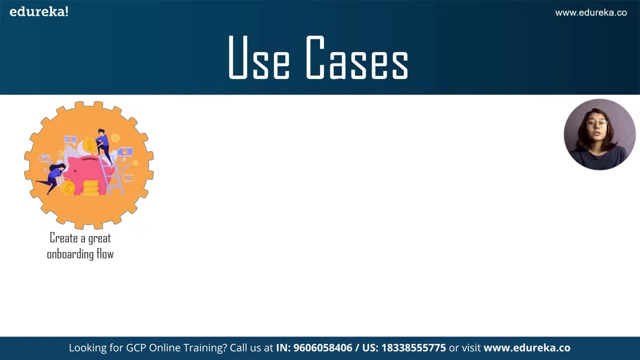 Creating a tailored custom onboard UI for the user when he or she navigates to the application by clicking on the custom link. With open authorization on Earth feature users can sign into your app via Facebook, Twitter, GitHub or Google. This cuts down the hassle of manually inputting user details. 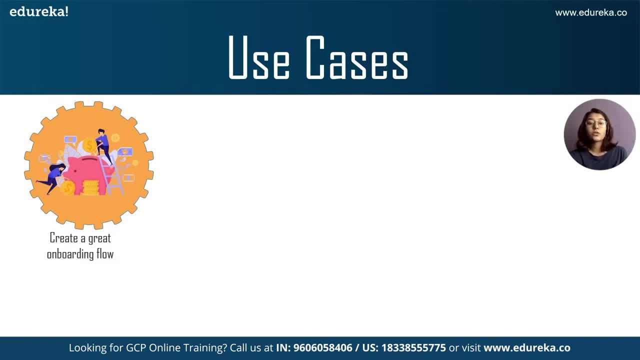 in the signup form, eventually improving the user onboarding rate by lots. Rolling out new features progressively. Development teams can roll out new features to a limited group of users, Get user feedback, run a thorough testing and, when everything is fine, roll out the features. 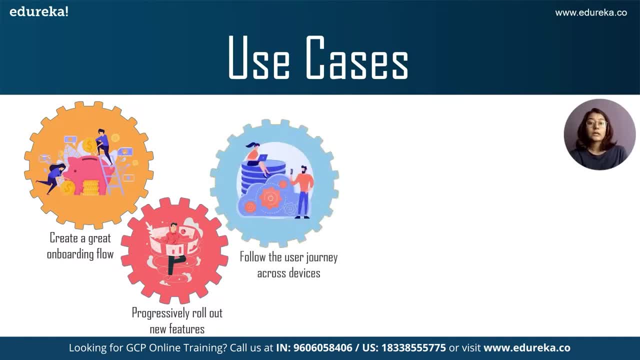 on a larger scale. Follow the user journey across devices. We often or always, use the same applications via mobile desktops and tabs or any devices. Firebase facilitates the smooth management of user sessions and user activity across several devices. Optimize ads based on user behavior. 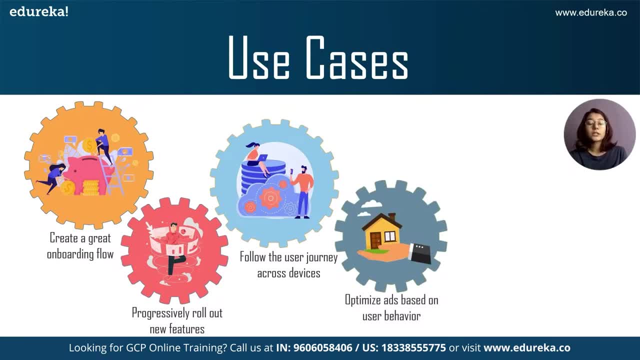 With the help of Google Analytics, development teams can monitor the user behavior and accordingly display related advertisements in their applications. Manage third-party payments without setting up your own servers To enable in-app purchases. Firebase helps developers streamline the third-party payment API integration process without any need for setting up and managing our own servers. 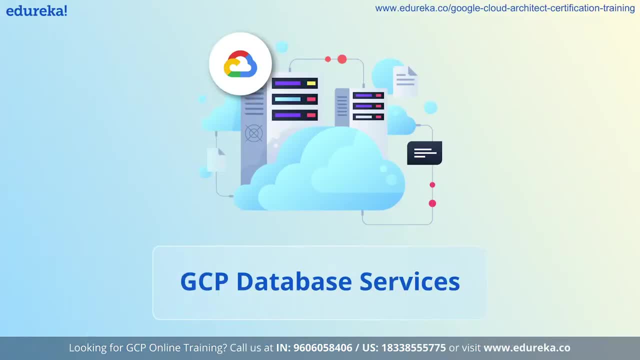 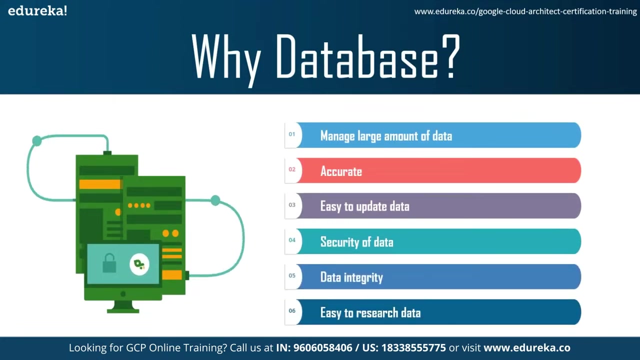 to run the payment feature. Now let's have an introduction of database. First, let's understand. why do we need a database? A good database is crucial to any company or organization. This is because the database stores all the pertinent details about the company, such as employee records. 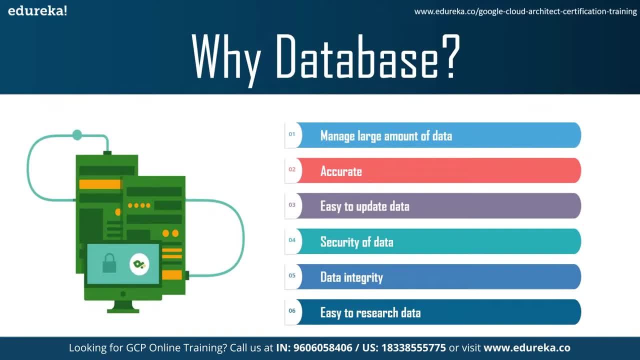 transactional records, salary details, etc. The various reasons a database is important are: it manages large amounts of data. A database stores and manages a large amount of data on a daily basis. actually, This would not be possible using any other tools, such as a spreadsheet, as 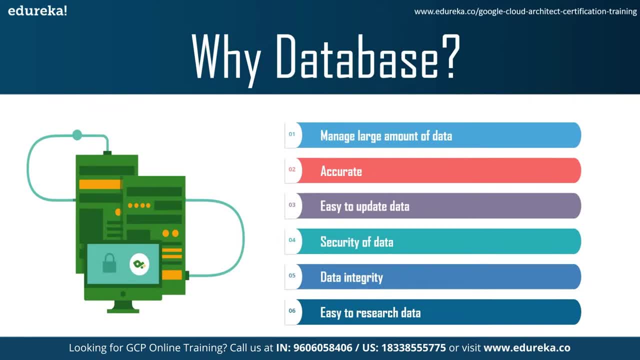 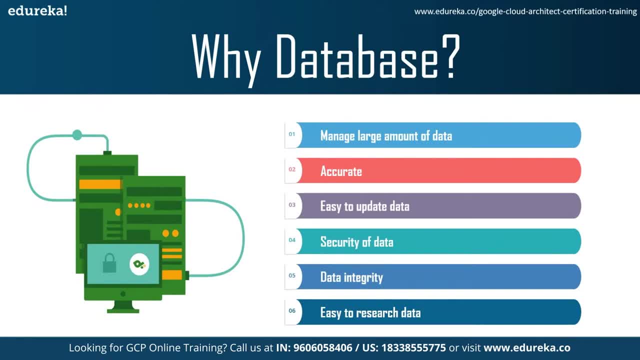 guaranteed to be correct in most cases. Third: it's easy to update. So in a database it is easy to update data using various data manipulation languages available. One of these languages is SQL. Fourth, the security of data. So databases have various methods to. 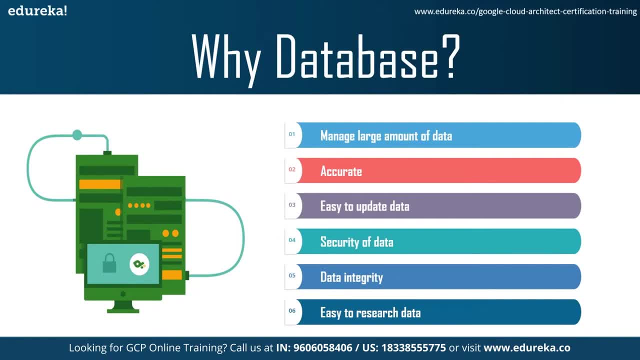 ensure security of data. There are user logins required before accessing a database and various access specifiers. These allow only authorized users to access the database. Fifth is data integrity. So this is ensured in databases by using various constraints for data. Data integrity in databases makes sure that the data is accurate and consistent in a database. 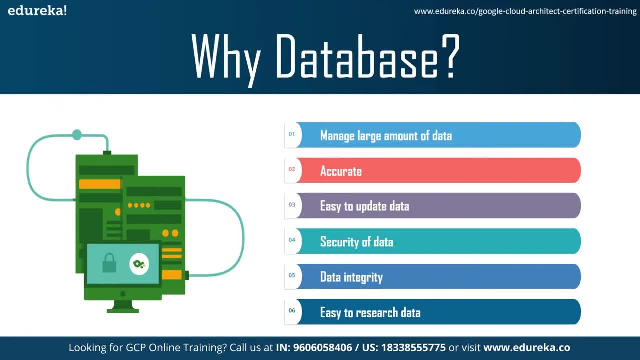 Last one that is easy to research database. So if you see like it's very easy to research and access the data in database, This is done using a data query language which allows searching of any data in the database and performing computations on it. Now that you have, 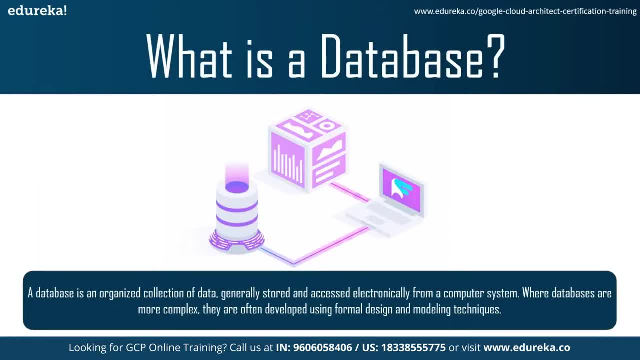 understood the need of a database, let's briefly understand what actually it is. So a database is an organized collection of structured information or data, typically stored electronically in a computer system. A database is usually controlled by a database management system, Together the data and the database management system, along with the applications that are associated. 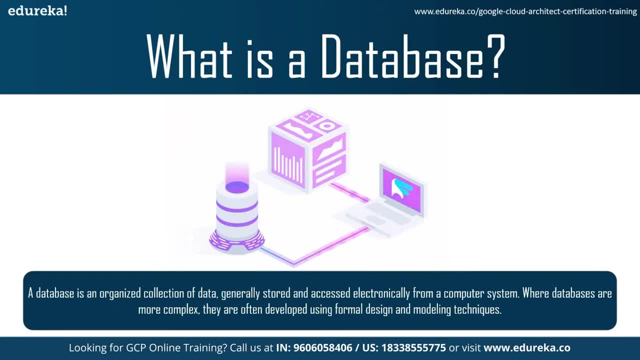 with them are referred to as a database system, often shorted to just database. Data within the most common types of databases in our operation today is typically modeled in rows and columns In a series of tables to make processing and data querying efficient. the 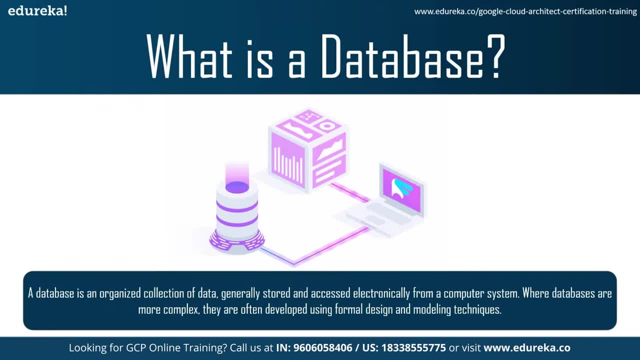 database can be accessed, managed, modified, updated, controlled and organized. Most databases uses structured query language means SQL for writing and querying data. Databases are used to support internal operations of organizations and to underpin online interactions with customers and suppliers. Databases are used to hold administrative information and more specialized 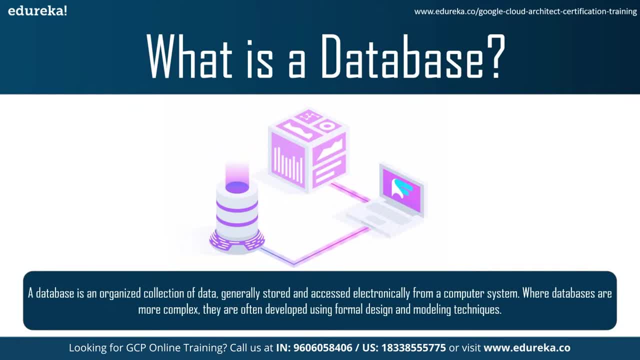 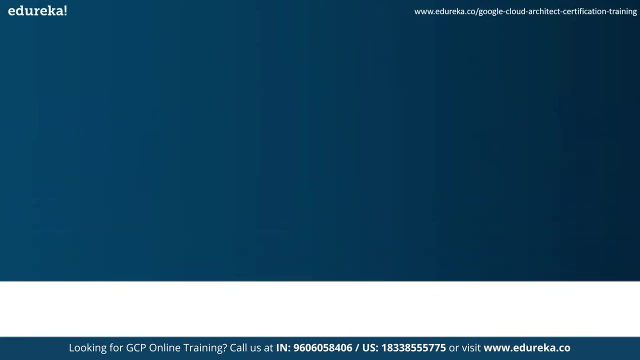 data, such as engineering data or economic models. Examples include computerized library systems, flight reservation systems or computerized parts inventory system, and many content management systems that store websites as collections of web pages in a database. Now that you have an overview of Google Cloud Platform, as well as of a database, now let's understand the different types of GCP. 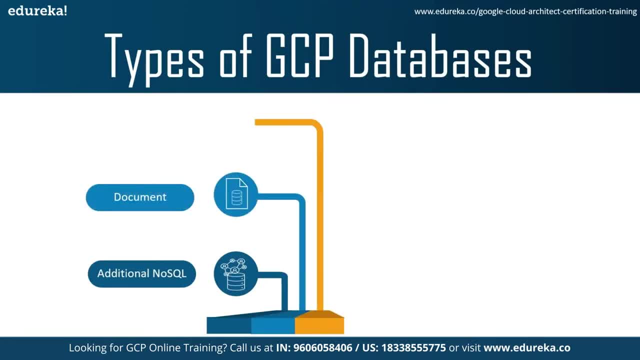 databases. So the first is relational databases. A relational database is a type of database that stores and provides access to data points that are related to one another. Relational databases are based on a relational model, an intuitive, straightforward way of representing data in tables. In a relational database, each row in the table is a record. 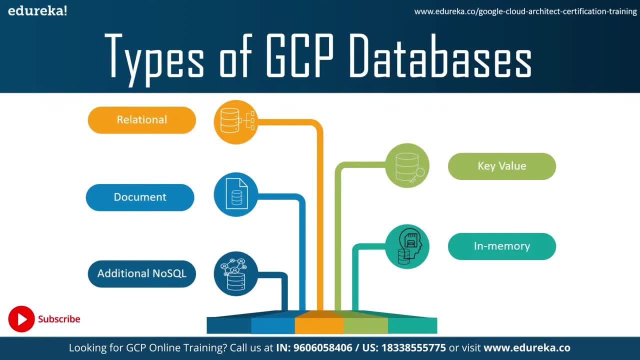 with a unique ID called the key Columns of the table hold attributes of the data and each record usually has a value of each attribute, making it easy to establish the relationships among data points In a relational database. all data is stored and accessed via relations Relations. 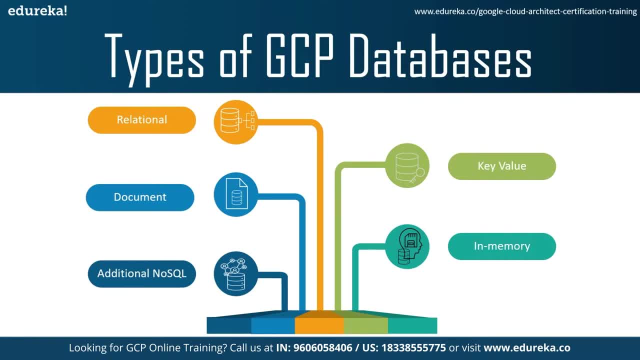 that store data are called base relations and in implementations are called tables. Other relations do not store data but are computed by applying relational operations to other relations. These relations are sometimes called derived relations. In implementations these are called views or queries. Derived relations are convenient in that 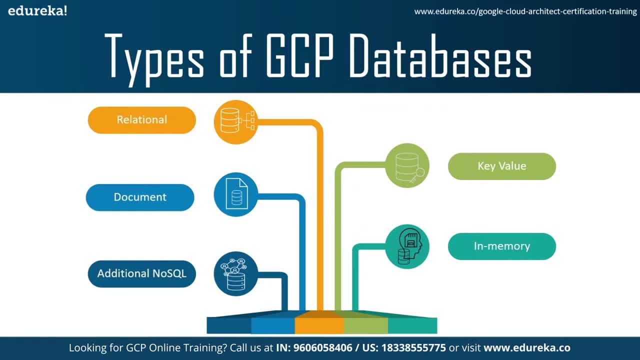 they act as a single relation, even though they may grab information from several relations. Each relation or table has a primary key, this being a consequence of a relation being a set. A primary key uniquely specifies a tuple within a table, While natural attributes 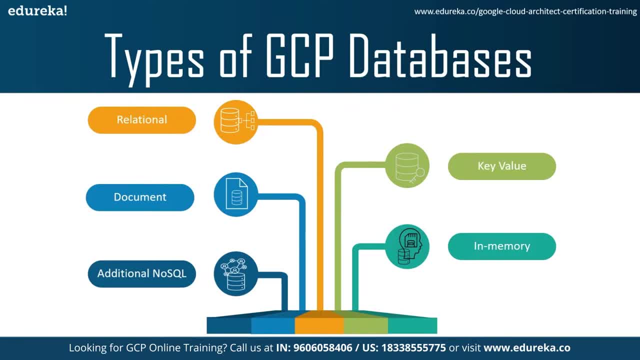 I mean attributes used to describe the data being entered are sometimes good primary keys. A foreign key is also there in a relational database management system. So a foreign key is a field in a relational data table that matches the primary key column of another table. It relates the two. 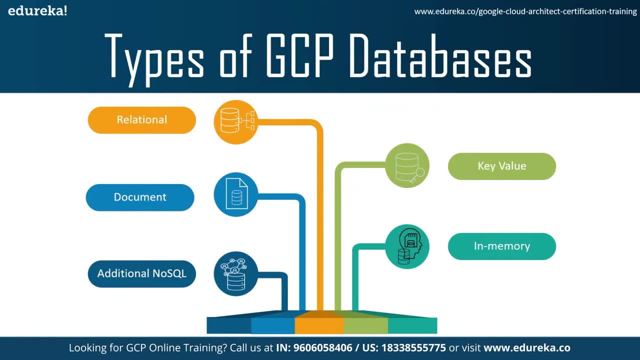 keys. Foreign keys need not have unique values in the referencing relation. A foreign key can be used to cross reference tables and it effectively uses the values of attributes in the reference relation to restrict the domain of one or more attributes in the referencing relation. Second is key value. 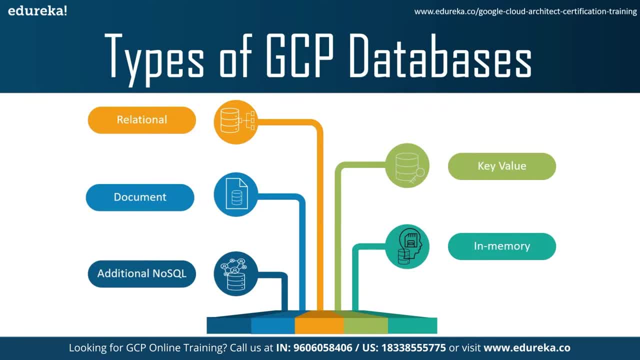 databases. So a key value database or key value store is a data storage paradigm designed for associative arrays and a data structure more commonly known today as a dictionary or hash table. Dictionaries contain a collection of objects or records which, in turn, have many different fields. 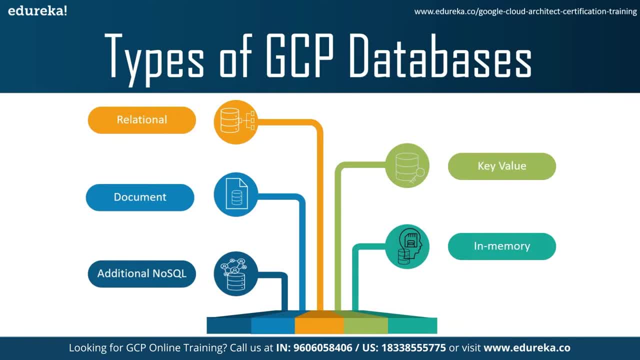 within them, each containing data. So these records are stored and retrieved using a key that uniquely identifies the record and is used to find the data within the database. So key value databases work in very different fashion from the better known relational databases. Relational databases pre-define the data structure in the database as a series. 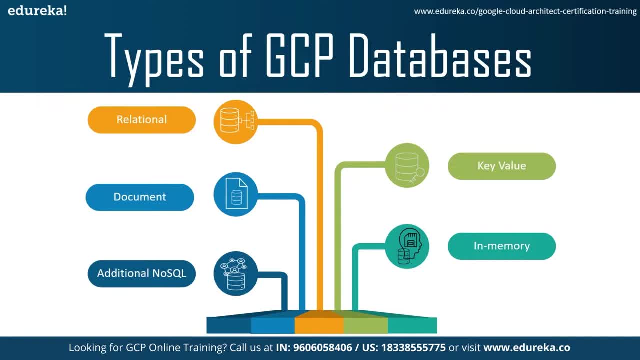 of tables containing fields with well-defined data types. Exposing the data types to the database program allows it to apply a number of optimizations. In contrast, key value system treats the data as a single, opaque collection which may have different fields for every record. 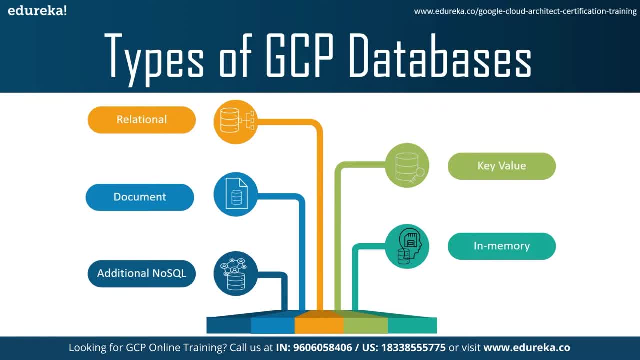 This offers considerable flexibility and more closely follows modern concepts like object-oriented programming. Because optional values are not represented by placeholders or input parameters as in most relational databases, key value databases often use far less memory to store the same database, which can lead to large performance gains in certain 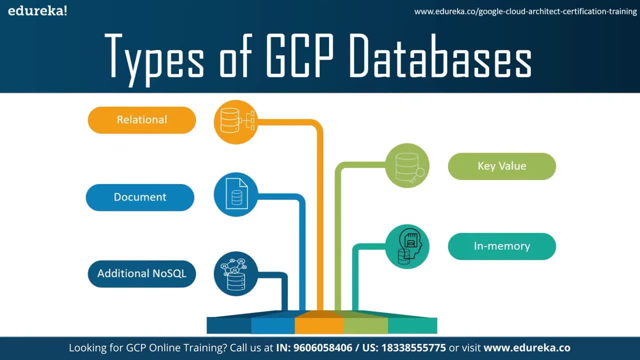 workloads Because optional values are not represented by placeholders or input parameters as in most relational databases. key value databases often use far less memory to store the same database, which can lead to large performance gains in certain workloads' performance. A lack of standardization and other issues limited key value systems to niche users for. 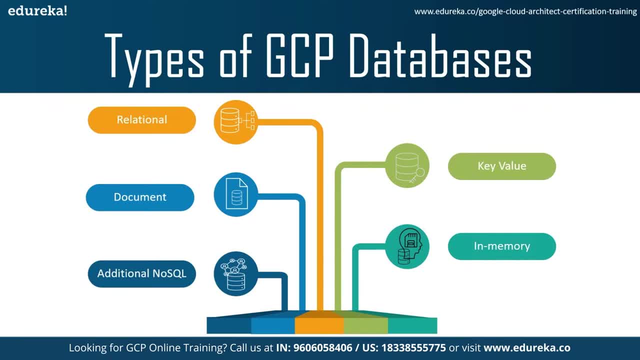 many years, But the rapid move to cloud computing after 2010 has led to a renaissance as part of the broader NoSQL movement. Now the third one is document database. So a document-oriented database, or document store, is a computer program and data storage system designed for storing. 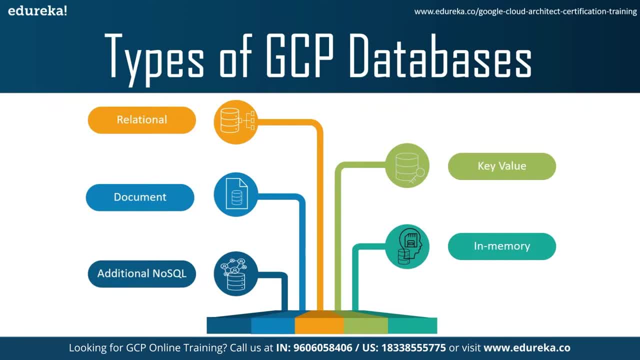 retrieving and managing document-oriented information, also known as semi-structured data. Document-oriented databases are one of the main categories of NoSQL databases, and the popularity of term document-oriented database has grown with the use of the term NoSQL itself. XML databases are a subclass of document-oriented databases that are optimized. 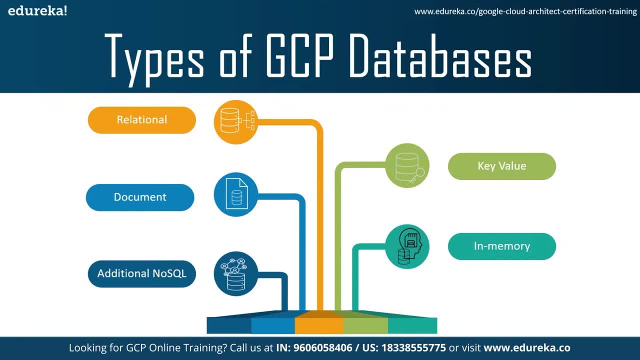 for XML documents. Graph databases are similar but add another layer, the relationship which allows them to link documents for rapid traversal. Document-oriented databases are like inherently a subclass of the key value store, another NoSQL database concept. So the difference lies in the 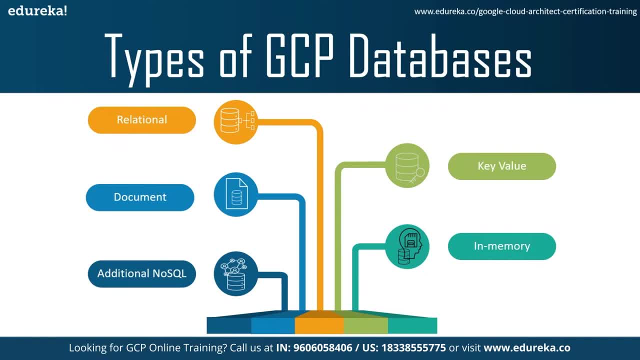 way the data is processed. In a key value, the data is considered to be inherently opaque to the database, whereas the document-oriented system relies on internal structure in the document in order to extract metadata that the database engine uses for further optimization. Although the difference is often negligible due to tools in the systems, conceptually, 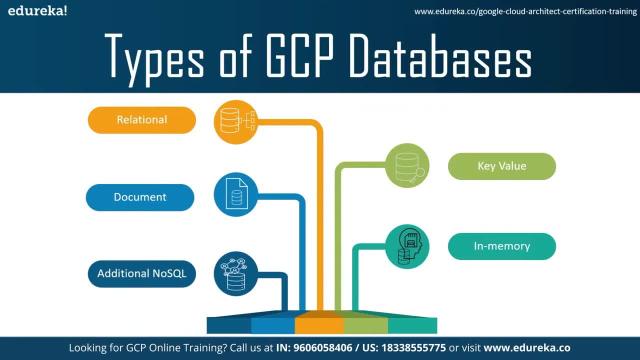 the document store is designed to offer a richer experience with modern programming techniques. So document databases contrast strongly with the traditional relational database. like, relational databases generally store data in separate tables that are defined by the programmer, and a single object may be spread across several tables. So document databases 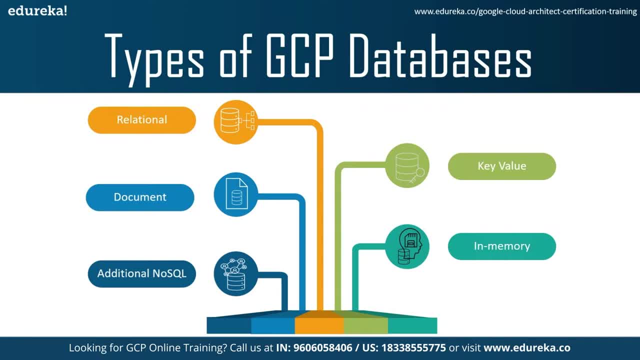 store all information for a given object in a single instance in the database, but a very stored object can be different from every other. This eliminates the need for object relational mapping while loading data in the database. So the fourth we have is in-memory database And in-memory database, IMDB, also a main memory database system, or MMDB, you can say. 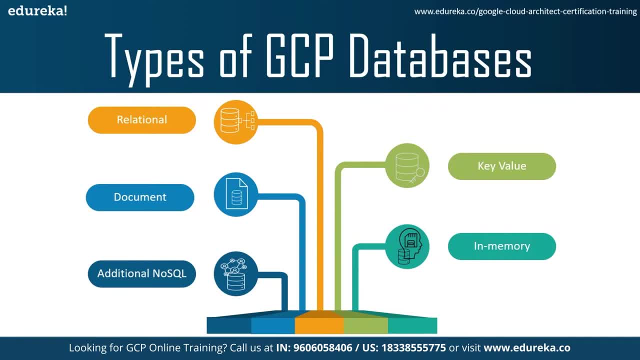 it like a memory resident database is a database management system that primarily relies on main memory of a computer data storage. It is contrasted with the database management system that employ a disk storage mechanism. So in-memory databases are like faster than disk optimized databases, because 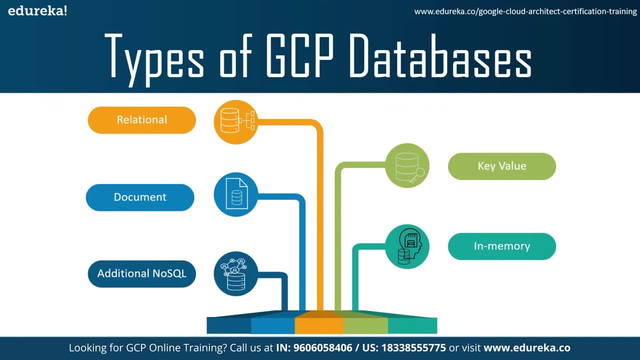 disk access is slower than memory access. The internal optimization algorithms are like simpler and execute fewer CPU instructions, So accessing data in memory eliminates seek time when querying the data, which provides faster and more predictable performance than disk Applications where response time is critical, such as those running telecommunication. 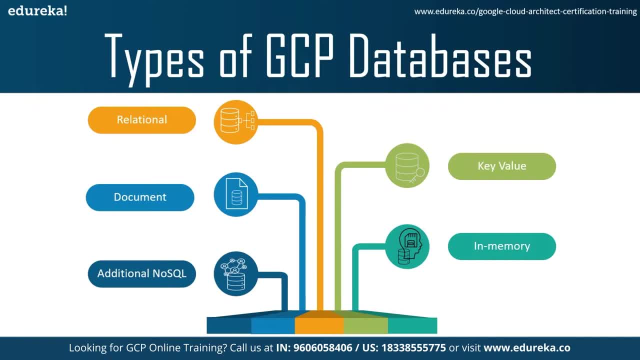 network equipment and mobile advertising networks, often main memory databases. So in-memory databases have gained much traction, especially in the data analytics space and in the mid 2000s, mainly due to multi-core processors that can like address large memory and due to less expensive RAM, A potential technical hurdle with in-memory data storage. 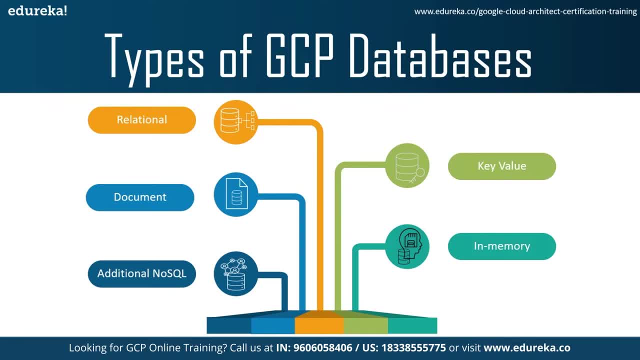 is the volatility of RAM. So, specifically in the event of a power loss, intentional or otherwise, data stored in the volatile RAM is lost. With the introduction of non-volatile random access memory technology, in-memory databases will be like able to run at full speed and maintain data. 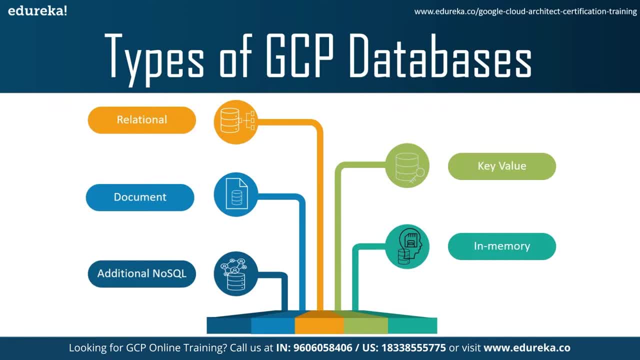 in the event of power failure. Now, the last one is additional NoSQL databases. Like, a NoSQL database provides a mechanism for storage and retrieval of data that is modeled in means other than the tabular relations used in the relational databases. So there are additional NoSQL databases. 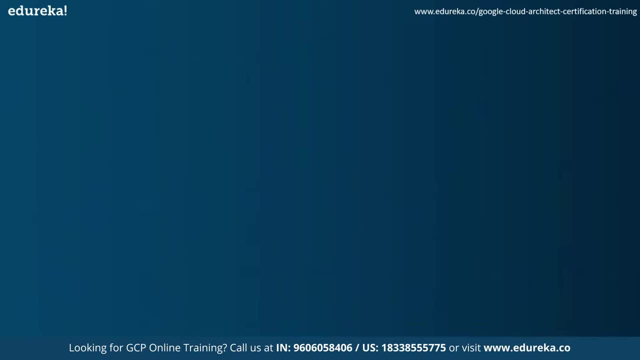 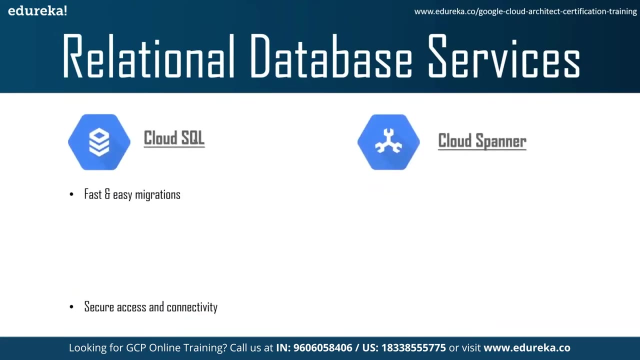 present in GCP, like MongoDB and others. So now that you have understood the types of databases, let's now understand services under these types of databases. So first we have relational databases, under which we have Cloud SQL and Cloud Spanner. So Cloud SQL is a fully managed database service. 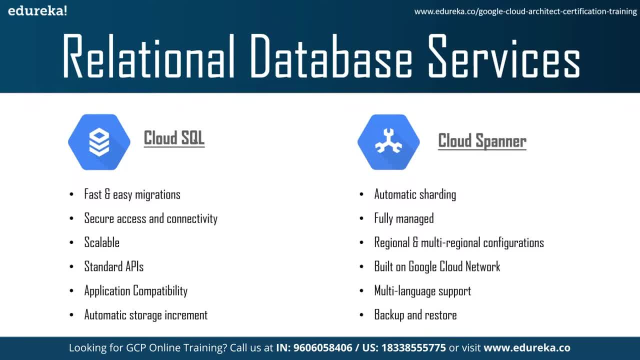 that makes it easy to set up, maintain, manage and administer your relational MySQL databases on cloud platform. The Cloud SQL for MySQL connector allows you to access data from Cloud SQL for MySQL databases within Data Studio, So its key features are like fast and easy migration, So database. 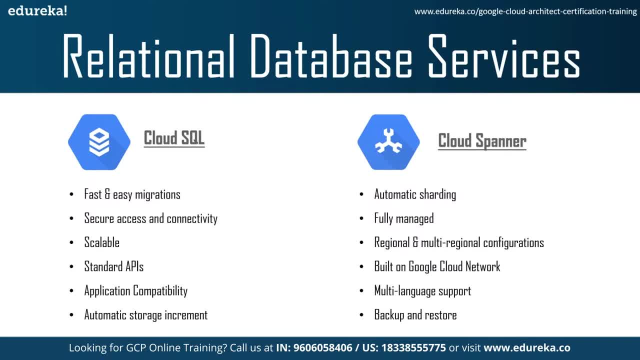 migration service makes it easy to migrate databases from on-premises compute engine and other cloud to Cloud SQL with minimal downtime. So second is the secure access and connectivity. So Cloud SQL data is encrypted when on Google's internal networks and when stored in database tables or temporary files and backups. 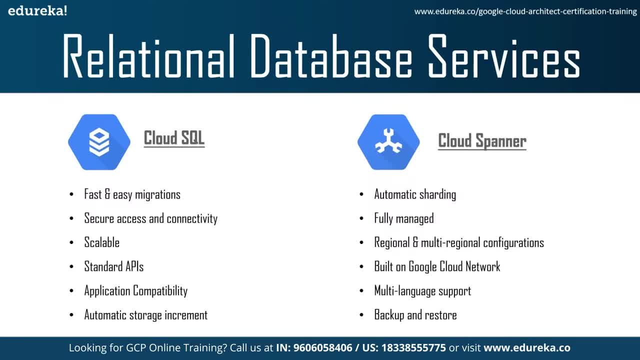 So Cloud SQL supports private connectivity with virtual private cloud And every Cloud SQL instance includes a network firewall allowing you to control public network access to your database instance. Third is easy integration. So access Cloud SQL instance from just about any application. Easily connect from App Engine, Compute Engine, Google Communities Engine. 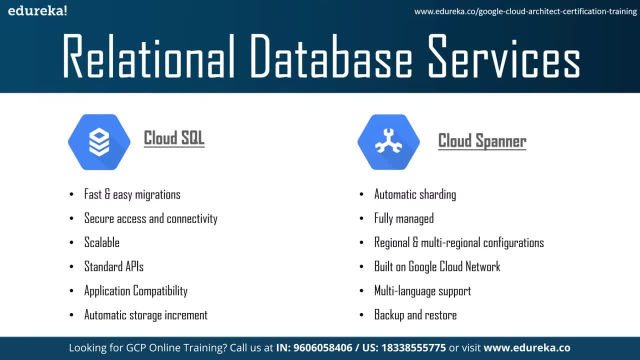 and your workstation. Open up analytics possibilities by using BigQuery to directly query your Cloud SQL databases. Then fourth is standard APIs. So build and deploy for the Cloud faster, because Cloud SQL offers standard MySQL or PostgreSQL and SQL server databases, Ensuring application compatibility. So 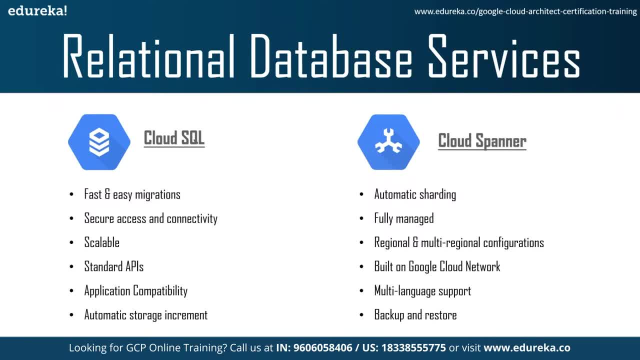 use standard connections drivers and build migration tools to get started quickly. Then fifth is application compatibility. So build and deploy for the Cloud faster because Cloud SQL offers standard MySQL or PostgreSQL SQL and Microsoft SQL. Then the last one is automatic storage increment, So Cloud SQL can automatically scale up storage capacity. 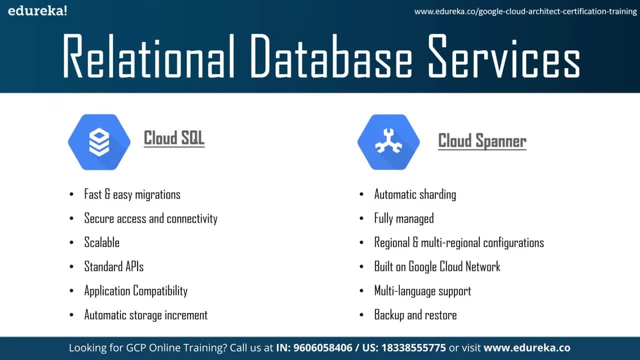 when you are near your limit. This way, you don't have to spend time estimating future storage needs or spend money on capacity until you need it. Now the question is when to choose Cloud SQL From lift and shift of on-premise SQL databases to the cloud, to handling large SQL. 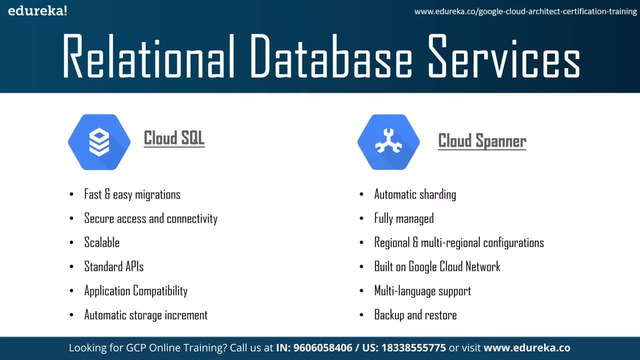 data analytics to supporting CMS data storage and scalability and deployment. So Cloud SQL can automatically scale up storage capacity when you are near your limit. So Cloud SQL can automatically scale up storage capacity when you are near your limit. In the cloud environment of microservices, Cloud SQL has many uses and is a better option. 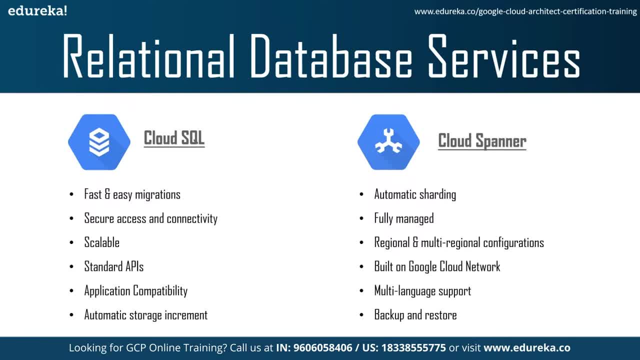 when you need relational databases capabilities but don't need storage capacity over 10 TB. I mean 10 terabytes. Now coming to Cloud Spanner. So Spanner is a distributed SQL database developed by Google. Spanner is a globally distributed database service and storage solution. It provides 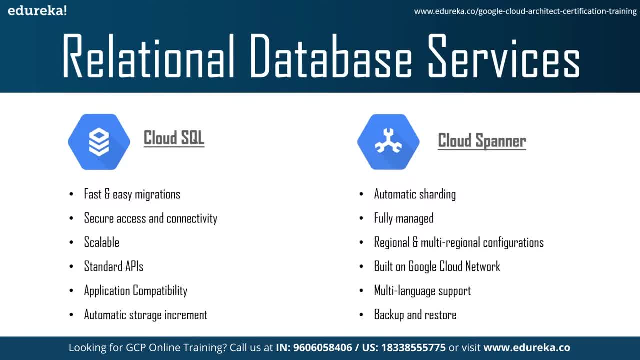 features such as global transactions, strongly consistent reads and automatic multi-site replication and failover. Its key features are first auto-sharing, Cloud Spanner optimized, and then the second is performance, by automatically sharing the databases on request load and size of the data. As a result, you can spend less time worrying about how to scale. 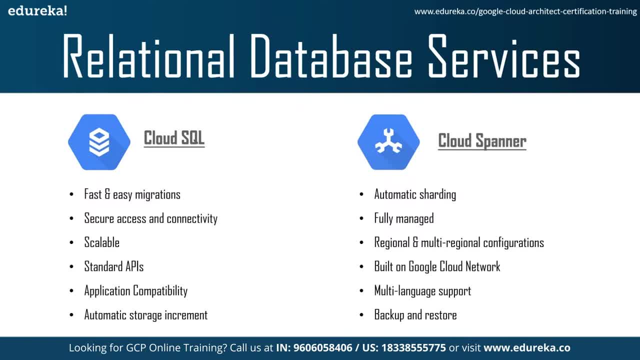 your database and instead focus on scaling your business. The second is it is fully managed, which means easy deployment at every stage and for any size databases. Synchronous replication also like synchronous replication, and maintenance, are automatic and built-in. The third one is it has regional and multi-regional configurations, No matter where your 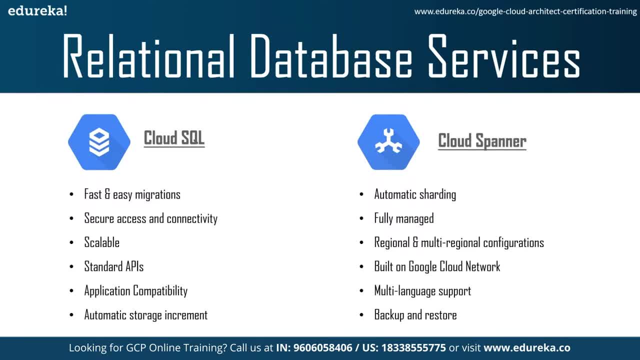 users may be. apps backed by Cloud Spanner can read and write up-to-date, strongly consistent data globally. Additionally, when running a multi-region instance, your database is able to survive a regional failure and offers industry-leading 99.99% availability. So fourth is built on Google Cloud. 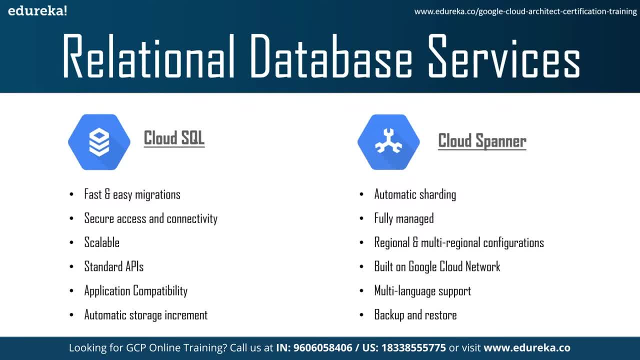 network. Cloud Spanner is built on Google's dedicated network that provides low latency, security and reliability for serving users across the globe. Fifth is it provides multi-language support. So client libraries in C, C++, Go, Java, NodeJS, PHP, Python and Ruby JDBC drivers for connectivity with popular 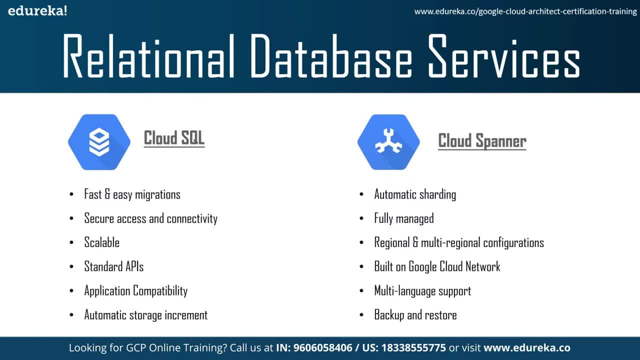 third-party tools. Last is backup and restore. Backup and restore recovers the database to the last state when the backup or the export was taken. PITR provides continuous data protection, with the ability to recover your past data to a microsecond granularity. Now the question is when to choose Cloud Spanner. 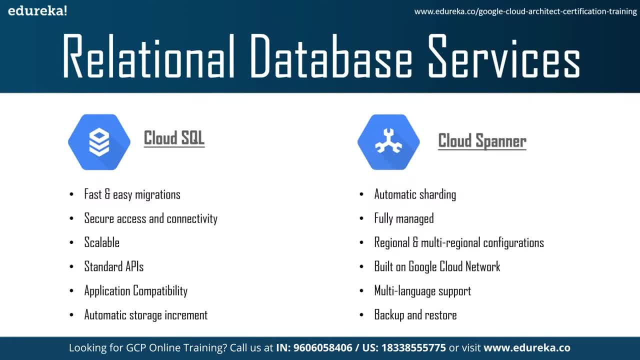 So Cloud Spanner should be your go-to option. if you plan on using large amounts of data- more than 10 terabyte- So Cloud Spanner should be your go-to option. if you plan on using large amounts of data- more than 10 terabyte- So Cloud Spanner should be your go-to. 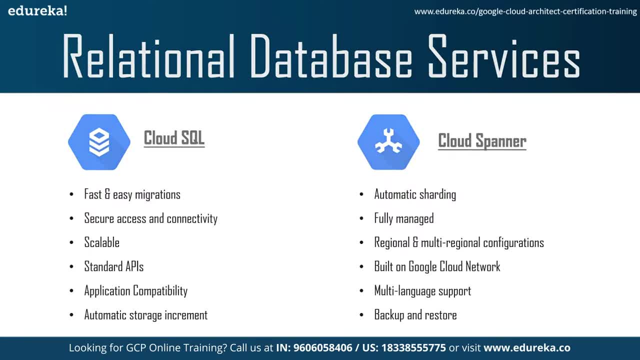 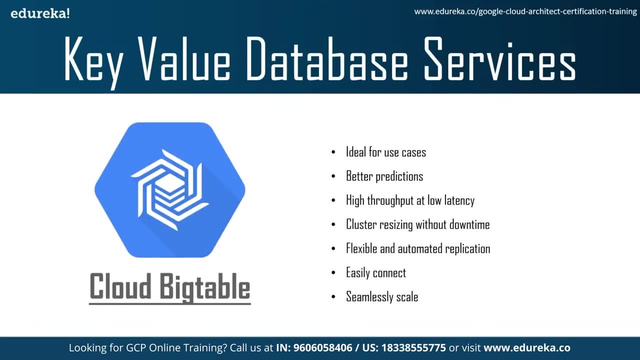 option if you plan on using large amounts of data, more than 10 terabyte. Now, the next is a key value database under which Google provides Bigtable service. So Bigtable is a compressed, high-performance proprietary data storage system built on Google file system. chubby log service SSD table. 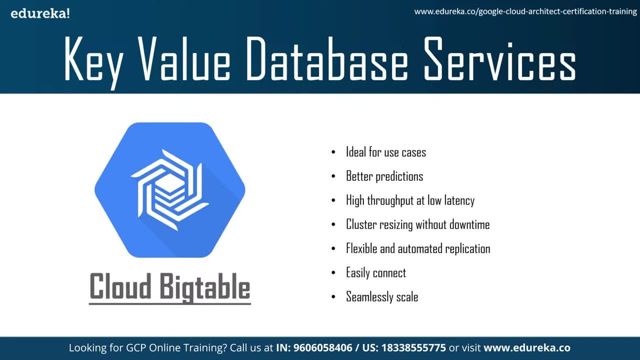 and a few other Google technologies. Some of its key features are: it is built for use cases such as personalization, edtech, fintech, digital media and IoT. Second is: it gives better prediction, Designed with a storage engine for machine learning applications leading to. 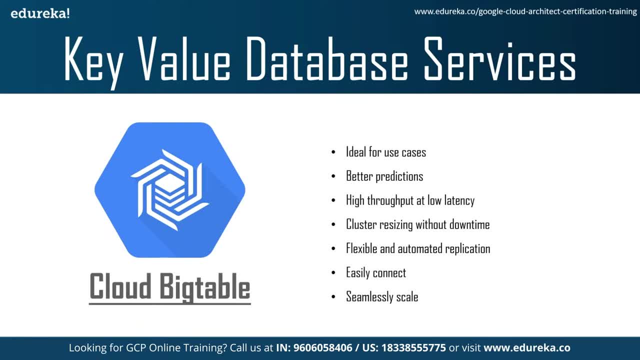 better prediction. Third is high throughput at low latency. So Bigtable is ideal for storing very large amounts of data in a key value store and supports high read and write throughput at low latency for fast access to large amounts of data. Throughput scales linearly. You can increase QPS means queries per. 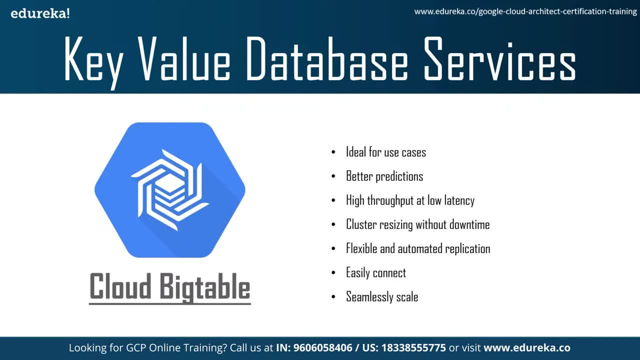 second, by adding Bigtable nodes. So Bigtable is built with proven infrastructure that powers Google products used by billions, such as search and maps. Then fourth is a cluster resizing without downtime. It scales seamlessly from thousands to millions of reads or writes per second. Bigtable. 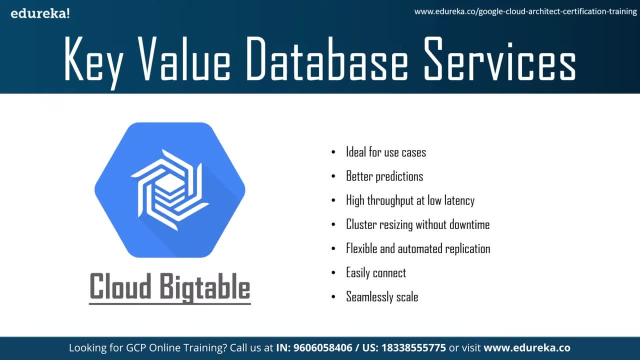 throughput can be dynamically adjusted by adding or removing cluster nodes without restarting, meaning you can increase the size of a Bigtable cluster for a few hours to handle a large load, then reduce the cluster's size again, all without any downtime. Like it's, flexible and automatic replication to optimize. 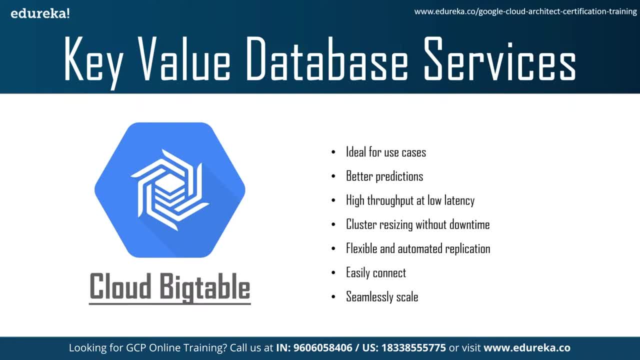 any workload, So write data once and automatically replicate where needed, with eventual consistency, giving you control for high availability and isolation of read and write workloads. No annual steps needed to ensure consistency or repair data or synchronize writes and deletes. Benefit from a high availability. SLA of. 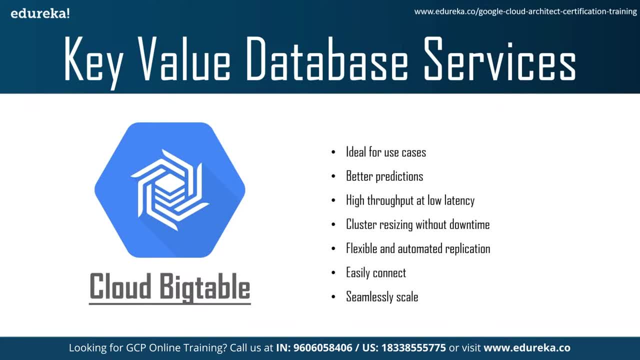 99.999% for instances with multi-cluster routing across three or more regions. 99.9% for single cluster instances. So next is like it easily connect to Google Cloud services such as BigQuery or the Apache ecosystem. Last, is it seamlessly? 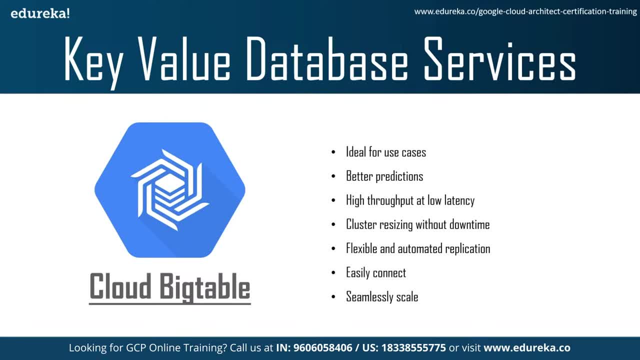 able to match your storage needs. So no downtime during reconfiguration. Now the question is when to choose Bigtable. So Cloud Bigtable is a good option if you are using large amounts of single key data and is a preparable for. 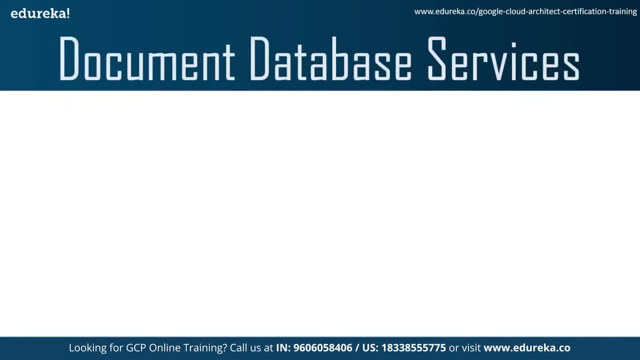 low latency, high throughput workloads. Moving on to the next type of services, that is, document database services, under which we have Cloud Firestore and Firebase. So Cloud Firestore is a cloud-hosted, no SQL database that your iOS, Android and web apps can access directly via native SDKs. 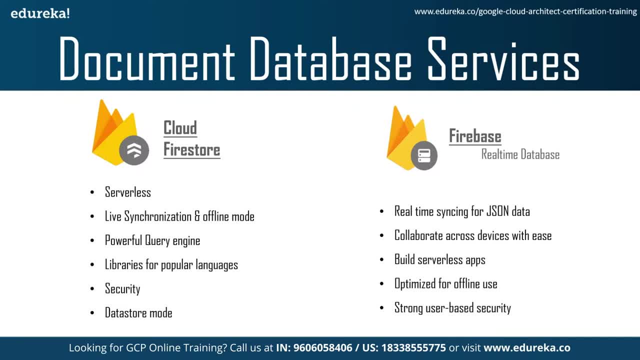 Cloud Firestore is also available in native Nodejs, Java, Python, Unity, C++ and Go SDKs. in addition to REST and RPC APIs, It is a flexible, scalable database for mobile web app and server development from Firebase and Google Cloud. Some of its key features are: first of all, it is serverless, which helps. 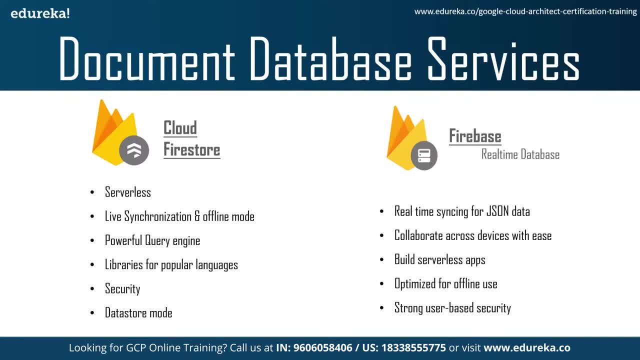 you in focusing on your application's development using a fully managed serverless database that effortlessly scales up or down to meet any demand, with no maintenance windows or downtime. Second is live synchronization and offline mode. Built-in, live synchronization and offline mode makes it easy to build multi-user collaborative applications on. 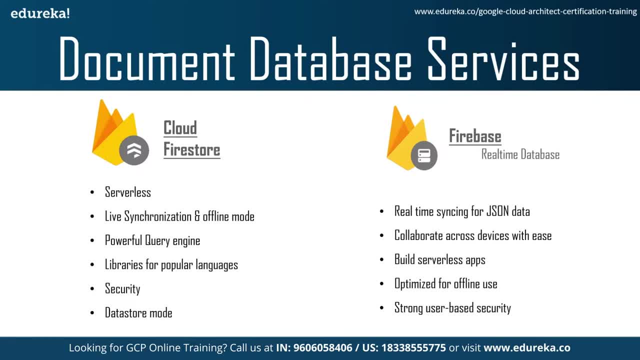 mobile web and IoT devices, including workloads consisting of live access tracking, activity tracking, real-time analytics, media and product catalogs, communications, social user profiles and gaming leaderboards. Third is powerful query engine. Firestore allows you to run sophisticated ACID transactions against your document data. This gives you more. 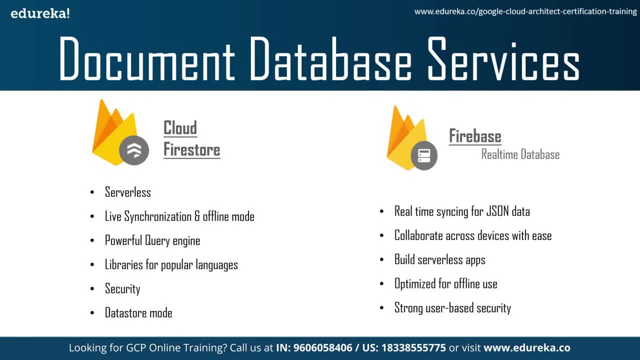 flexibility in the way you structure your data. Fourth is libraries for popular languages. Focus on your application development using Firestore client-side development libraries for web, iOS, Android, Plutter, C++ and Unity. Firestore also supports traditional server-side development libraries using 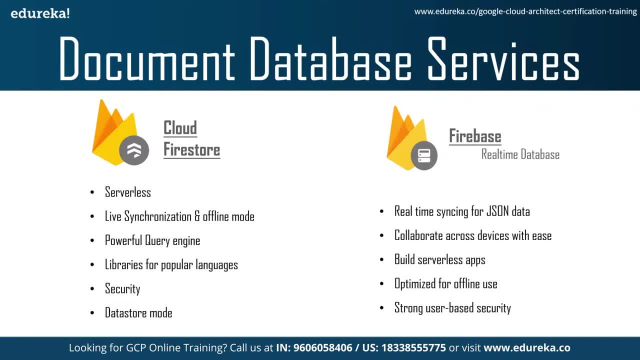 Nodejs, Java, Go, Ruby and PHP. Fifth is security. Firestore seamlessly integrates with Firebase authentication and identity platform to enable customizable identity-based security access controls and enables data validation via a configuration language. So the last one is Datastore. 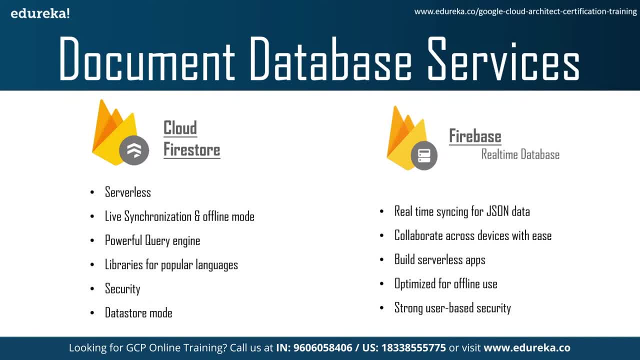 In Datastore mode. Firestore supports the Datastore API. You won't need to make any changes to your existing Datastore apps and you can expect the same performance, characteristics and pricing, with the added benefit of strong consistency. Existing cloud Datastore databases will be. 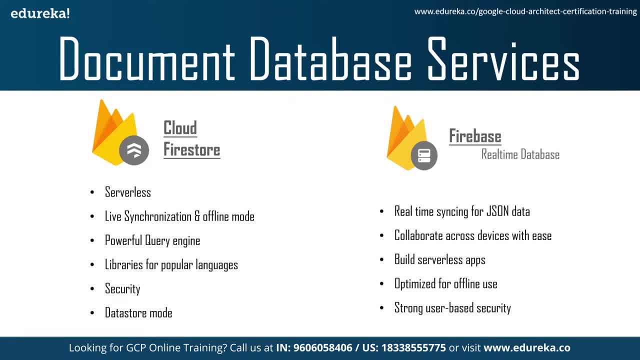 automatically upgraded to Firestore in the next like year of 2022 also. So now the question is when to choose Firestore, When you focus live on app development and you need live synchronization and offline support. Now coming to Firebase real-time database. Over the last few years, Firebase 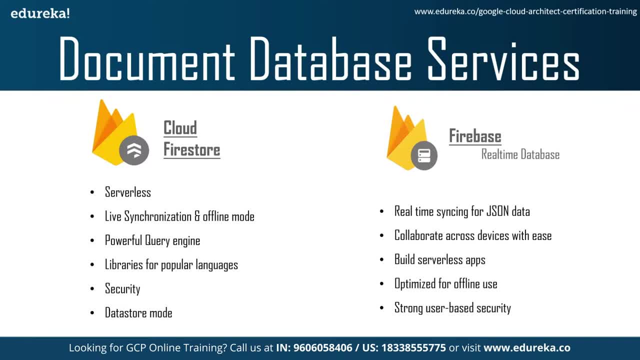 has grown to become Google's app development platform. It now has 16 products to build and grow your app. If you have used Firebase before, you know it already offer a database, which is the Firebase real-time database. So the Firebase real-time database, with its client SDKs and real-time 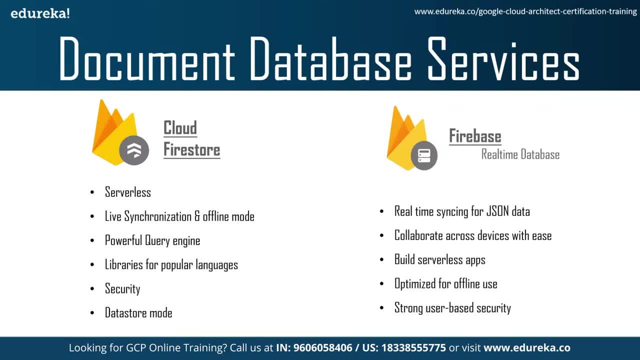 capabilities is all about making app development faster and easier. Since its launch, it has been adopted by hundreds of thousands of developers, and as its adoption grew, so did usage patterns. Let's discuss some of its key features. So, first of all, it provides real-time synchronization for JSON data. 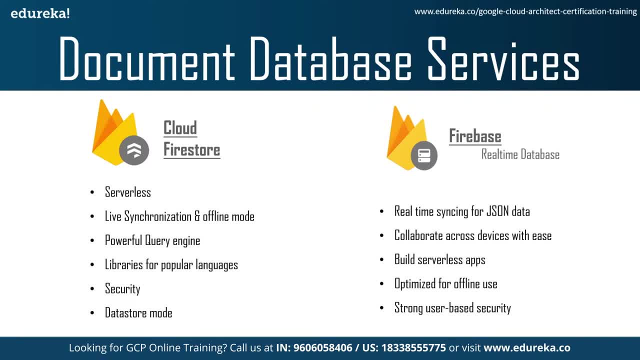 So developers began using the real-time database for more complex data and to build bigger apps, pushing the limits of the JSON data model and the performance of the database at scale. The Firebase real-time database is a cloud-hosted NoSQL database that lets you store and synchronize data between your users in 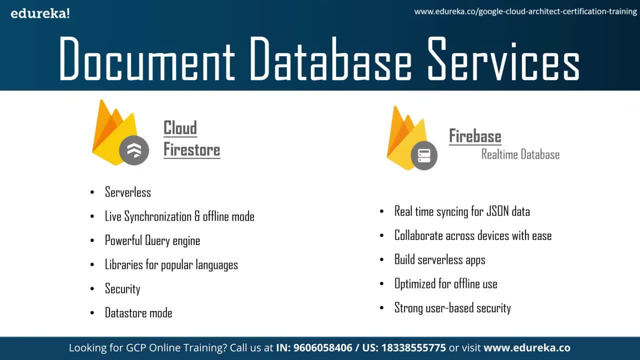 real-time. In its new update, Cloud Firestore enables you to store, synchronize and query app data at global scale. Second is like collaborate across devices with ease. So real-time synchronization makes it easy for your users to access their data from any device, web or mobile, and it helps your users collaborate with one another. 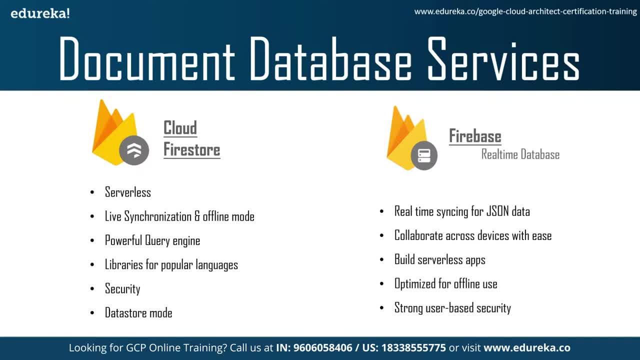 Third is build serverless apps. So real-time database ships with mobile and web SDKs so you can build applications without the need of servers. You can also execute backend code that responds to events triggered by your database using cloud functions for Firebase. Fourth is optimized for online use. 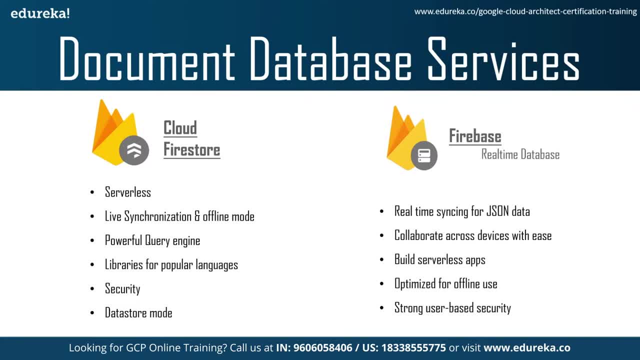 So, when users go offline, the real-time database SDKs use local data cache on the device to solve and store changes. When the devices come online, the local data is automatically synchronized. The last one is strong user-based security. The real-time database integrates with Firebase authentication. 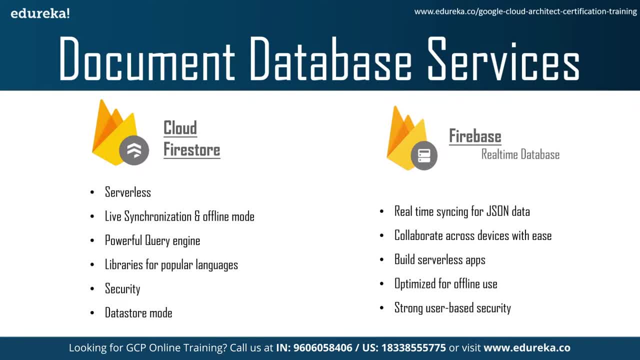 to provide simple and intuitive authentication for developers, You can use Google's speculative security model to allow access based on user identity or with pattern matching on your data. So the use cases for Firebase real-time database involve development of applications that work across devices, advertisement, optimization and personalization, and third-party. 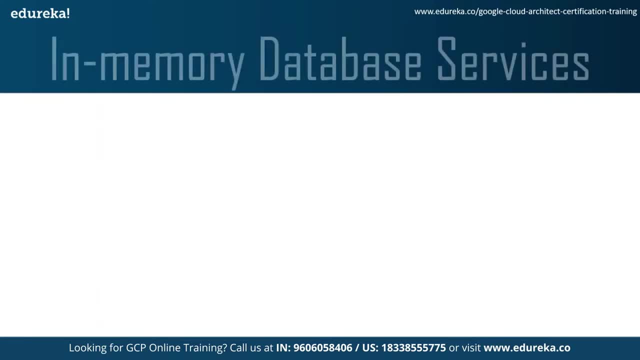 payment processing. Now moving on to the next type of service, that is, in-memory database services, under which Google provides memory store. So memory store reduces latency with scalable, secure and highly available in-memory service for Redis and memcached. Memory store automates complex tasks for open-source. 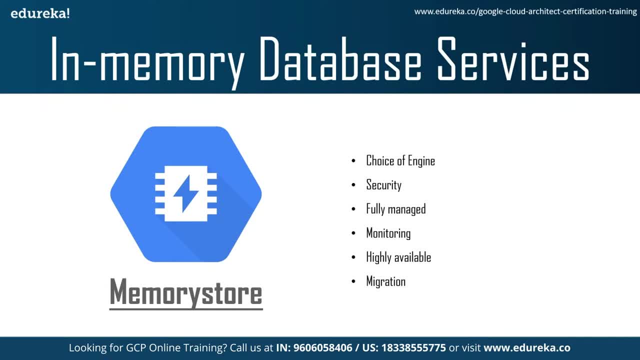 Redis and memcached like, enabling high availability payload patching monitoring so you can spend more time coding. Start with the lowest tier and smallest size and then grow your instance with minimal impact. Memory store for memcached can support clusters as large as 5 terabytes, supporting millions of. 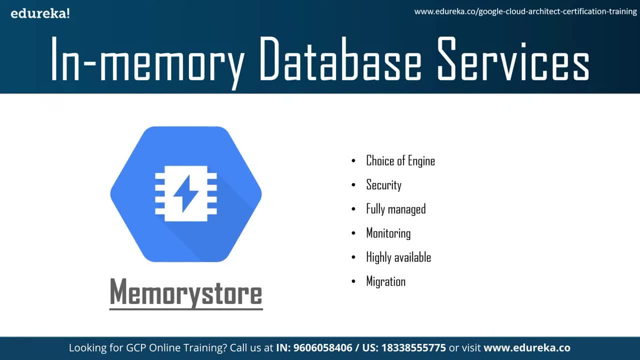 QPs at very low latency. So memory store for Redis instances are replicated across two zones and provide a 99.9% availability. SLA Instances are monitored constantly and, with automatic failover, Applications experience minimal disruption. Some of its key features are choice of engines, So choose from the two. 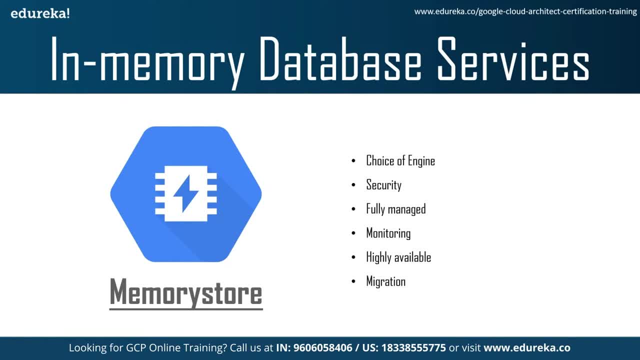 most popular open-source caching engines to build your applications. Memory store supports both Redis and memcached and is fully protocol compatible. Choose the right engine that fits your cost and availability requirements. Second is security, So memory store is protected from the internet using virtual. 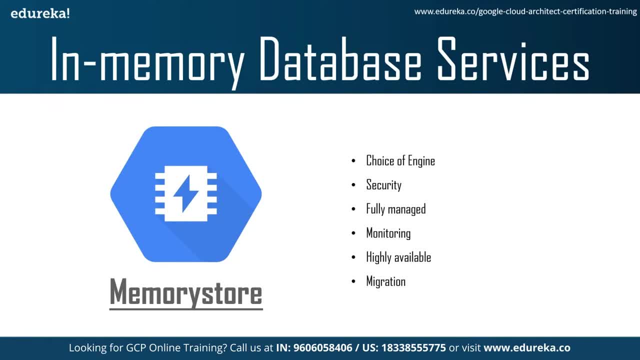 private cloud networks and private IP, and comes with IAM integration, all designed to protect your data. Systems are monitored 24, 7 and 365 days, ensuring your applications and data are protected. Third is it's fully managed. So provisioning, replication, failover and web patching are all 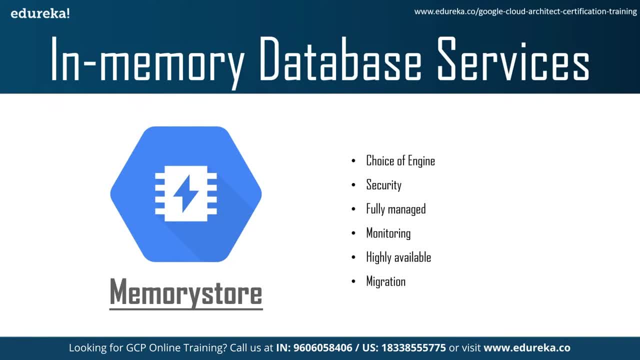 automated, which drastically reduces the time you spend doing DevOps. Fourth is monitoring, So monitor your instance and set up custom alerts. with cloud monitoring, You can also integrate with the open sensors to get more insights to client side metrics. Fifth is it's highly available, So standard tier. 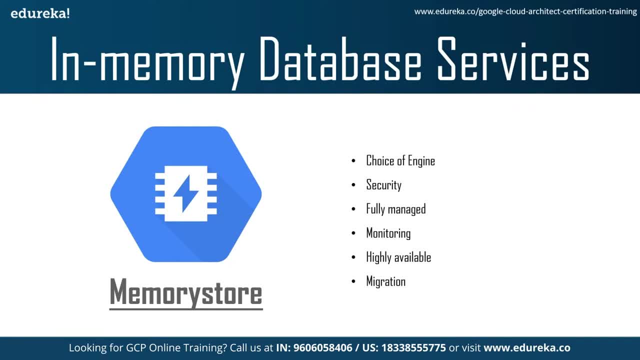 memory store for Redis instances provide an 89.9% availability SLA with automatic failover to ensure that your instance is highly available. You also get the same availability SLA for memcached instances. Last is migration. So memory store is compatible with open source protocol, which makes it. 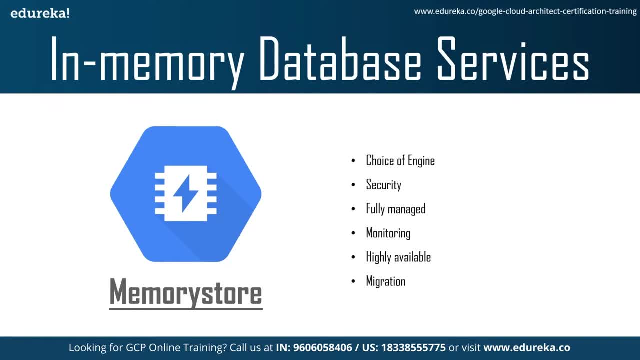 easy to switch your applications with no code changes. You can leverage the import and export feature to migrate your Redis and memcached instance to Google Cloud. Now the question is when to choose a memory store. If you are using key value datasets and your main focus is transaction latency, then 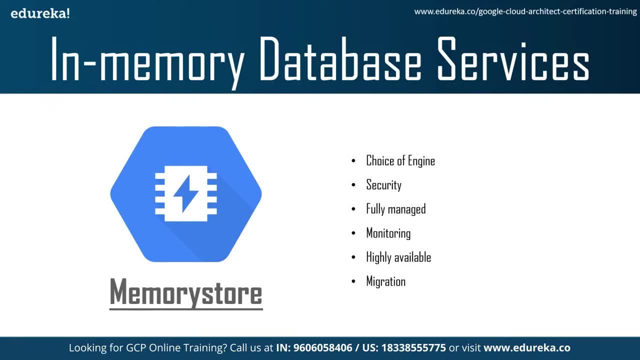 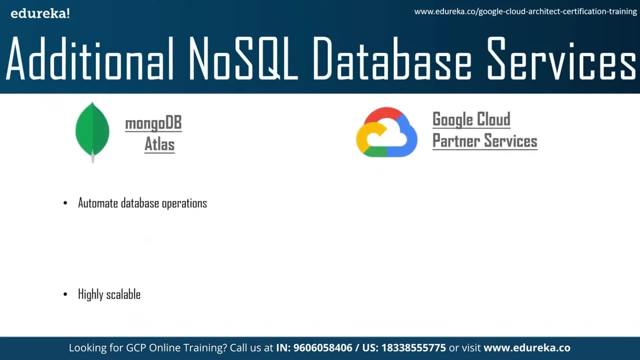 you can go for memory store. Now, moving on to the last type of database services, that is, additional NoSQL database services, under which we have MongoDB, Atlas and Google Cloud partner services. So MongoDB is a source available cross-platform document-oriented database program classified as a. 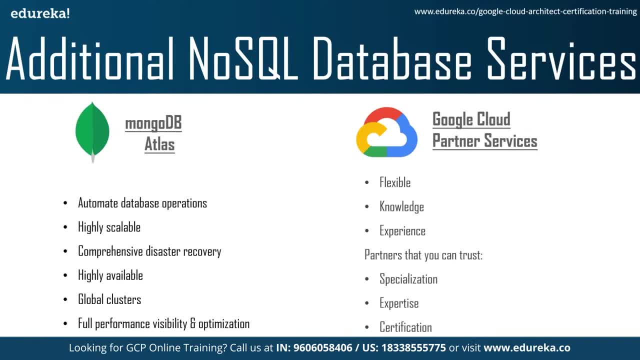 NoSQL database program. MongoDB uses JSON-like documents with optional schemes, and MongoDB Atlas is the best way to deploy, manage and grow MongoDB on Google Cloud, Engineered and run by the same engineers that build the database. Atlas incorporates best practices developed from support. 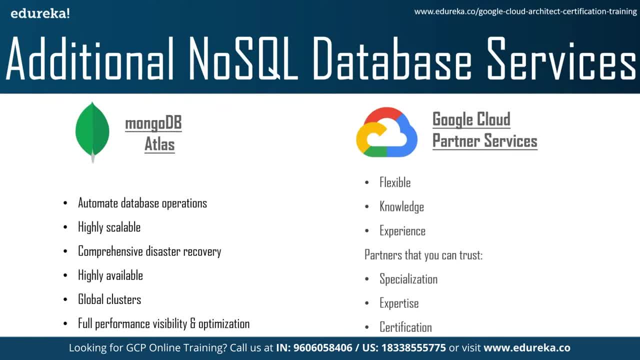 and support. It is a platform that can support thousands of distributed deployments into an easy to use, fully automated service that grants you the power and freedom to focus on what really matters: building and optimizing your applications. Its key features are: first, its database operations are 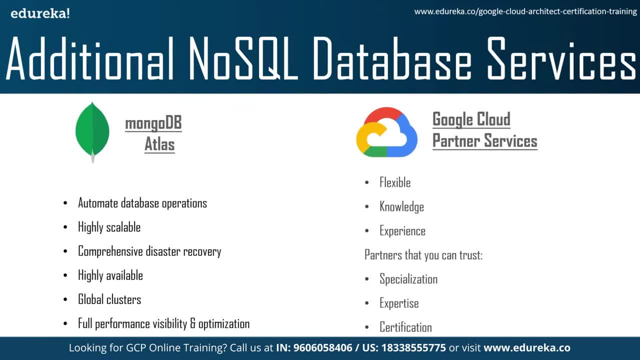 automated, as database operations take time, and so MongoDB Atlas lowers your stress by orchestrating the moving parts, deploying clusters in minutes, modifying them on demand with zero downtime, and taking advantage of automated operations. Second, it is highly scalable. So add storage, scale up. 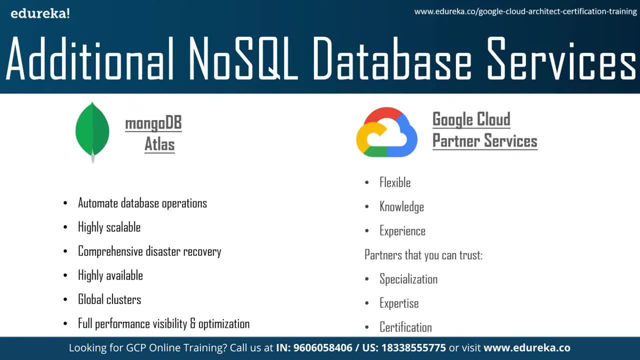 scale out or scale down with the push of a button or a simple API call. MongoDB Atlas allows you to easily tweak the dimensions of your deployment with no impact to your applications. Third is a comprehensive disaster recovery. So MongoDB Atlas includes an optional, fully managed backup service that 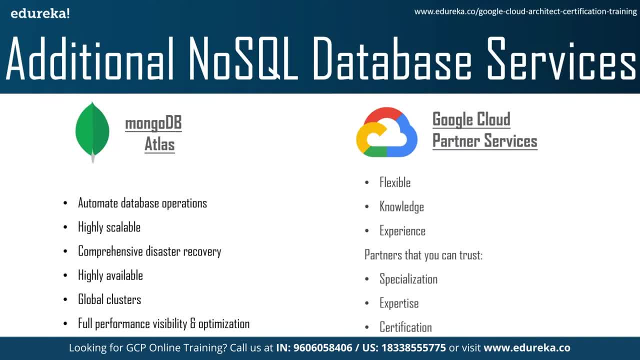 provides continuous backups with point-in-time recovery. Query your backup snapshots and restore granular data sets in a fraction of the time. Easily restore snapshots to different projects to rapidly spin up developer or test environments. Fourth, it's highly available, backed by uptime SLAs. 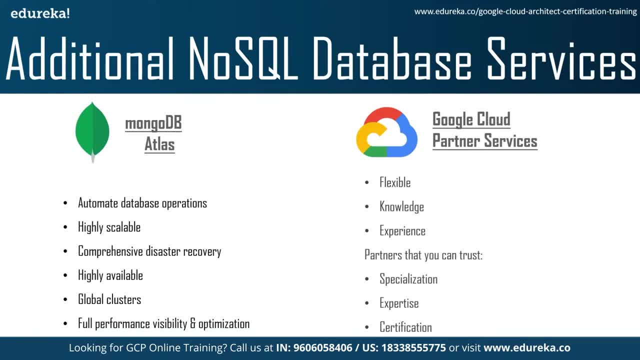 Each cluster is distributed across the zones in a Google Cloud region, ensuring no single point of failure. Should your primary fail, MongoDB Atlas will automatically trigger the election and failover process, with no manual intervention required. Production databases are backed by 99.9% uptime SLA. 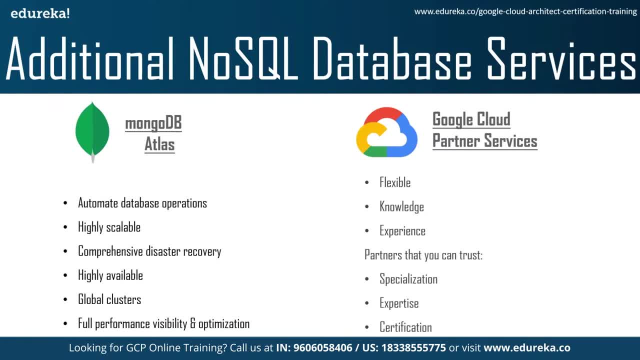 Fifth is global clusters. So global clusters are built into MongoDB Atlas, and MongoDB Atlas allow you to deploy a geographically distributed database that provides low latency, responsive reads and writes to users anywhere, with strong data placement controls to satisfy emerging regulations. And the last one, 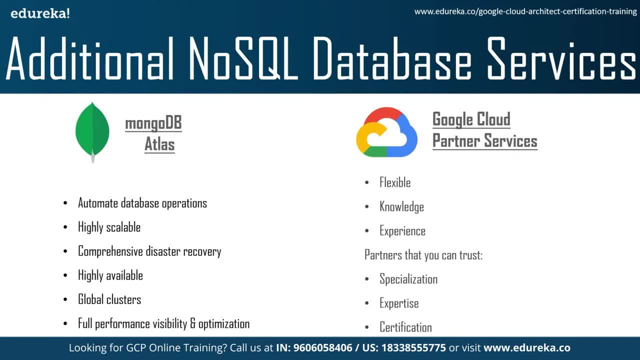 is full performance, visibility and optimization. So MongoDB Atlas includes optimized dashboards that highlight key historical metrics, view performance in real-time, customize alerts or dig into the details with ease. So built-in tools such as the Performance Advisor highlight flow-running queries and suggest. 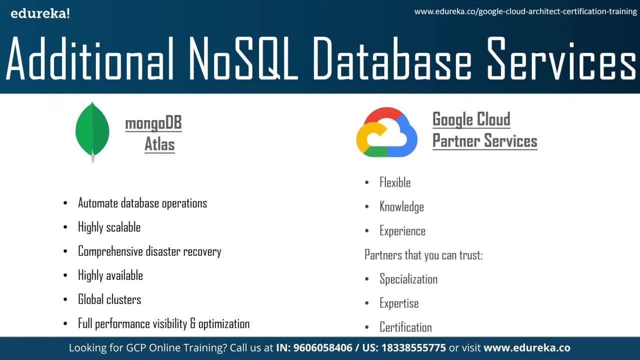 indexes to help optimize your database. Now the next we have is Google Cloud partner services. So you can choose Google Cloud partner service on the basis of regions, specialization, expertise, initiatives and products. But why work with a Google Cloud partner? So? first of all, it's flexible, So Google Cloud's 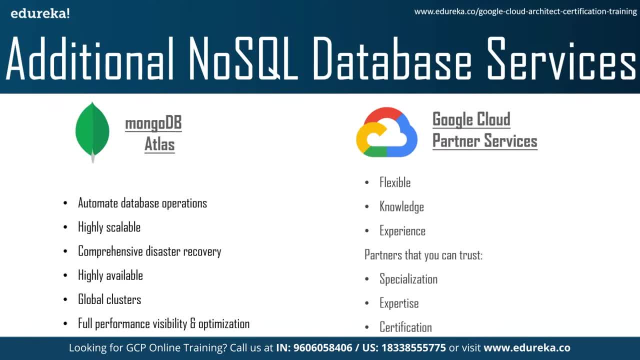 global network means you can work with a Google Cloud partner that best fits your organization's needs. The second is for the knowledge purpose- like collaborate with a partner that has the right industry background to unlock your next level of business growth. And the third and the last one is experience. So 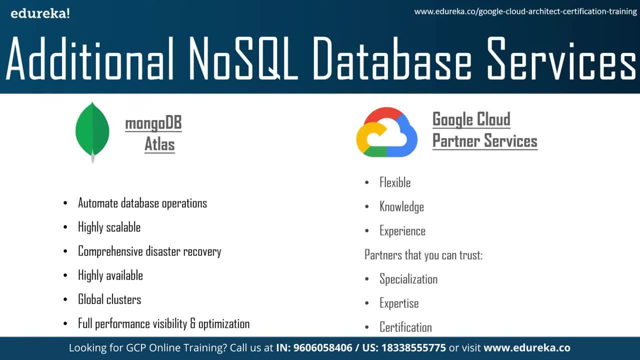 have the confidence to tackle your toughest business challenges with the support of a partner with proven success. So one more thing is: like Google, partners are the ones you can trust, actually. So partners that have certified their teams, earned expertise and achieved specialization have the Google validated skills to. 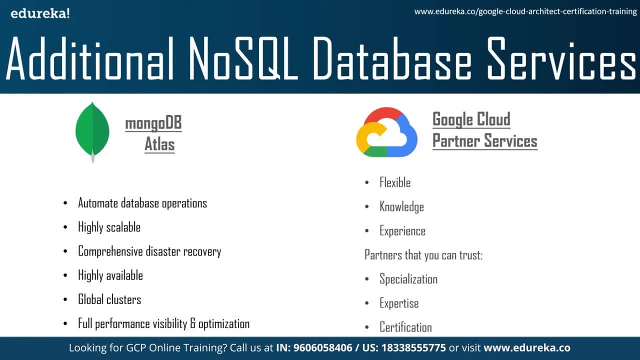 help you achieve your goals. So partners are divided in like in three forms. So first is the specialization. So specialization is the highest technical designation a partner can earn. Partners who have achieved a specialization in a solution area have an established Google Cloud service practice consistent. 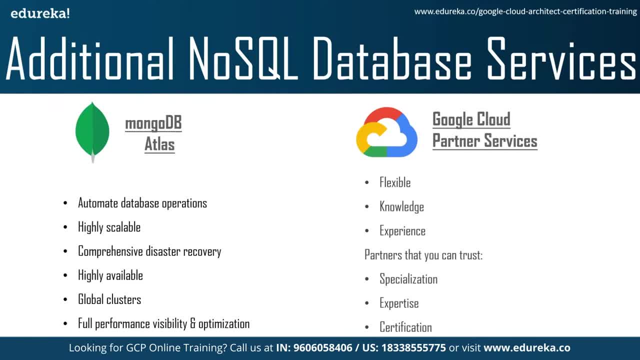 customer success and proven technical capabilities vetted by Google and a third party accessor, Like there is a specialization in application development, cloud migration, data analytics, data management, internet of things, machine learning, marketing analytics, etc. Second is expertise, So partners with the expertise. 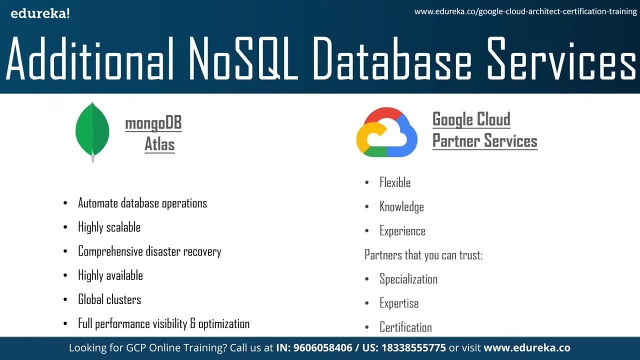 designation have demonstrated proficiency and have exhibited customer success through the combination of expertise and proven technical capabilities. So partners who have achieved a combination of experience in a specific industry, workload or product. So, for example, like there is an expertise in industry. 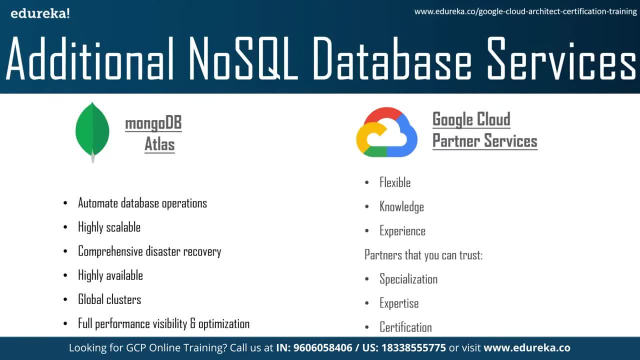 and expertise in Google Cloud product or technology and workload. Third is certification. So partners with teams of Google Cloud certified individuals have the validated technical knowledge and advanced skills to address your business's needs through implementing Google Cloud technologies. There are a lot of certifications, like foundational data cloud leader, associate cloud engineer. 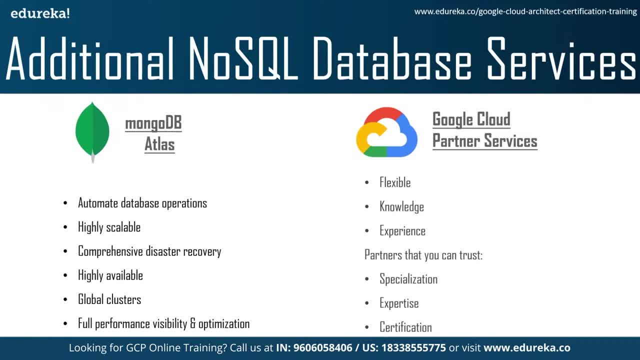 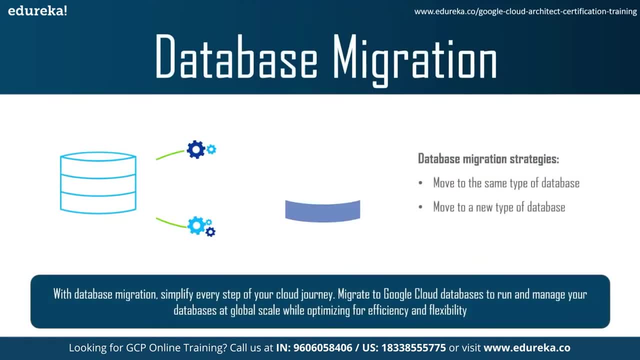 professional cloud architect, professional cloud developer and cloud developer, professional data engineers and various others. Now let's look at some solutions provided by the GCP database. So the first one is the database migration. Database migration is the process of selecting, preparing, extracting. 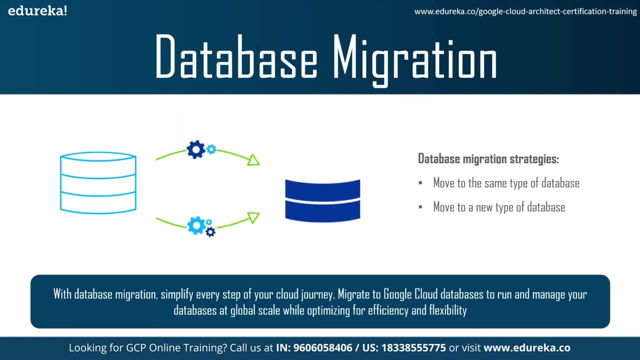 and transforming data and permanently transferring it from one computer storage system to another. With Google Cloud, you can simplify your database migration at every step of your cloud journey. So migrate to Google Cloud databases to run and manage your databases at global scale, while optimizing for efficiency and 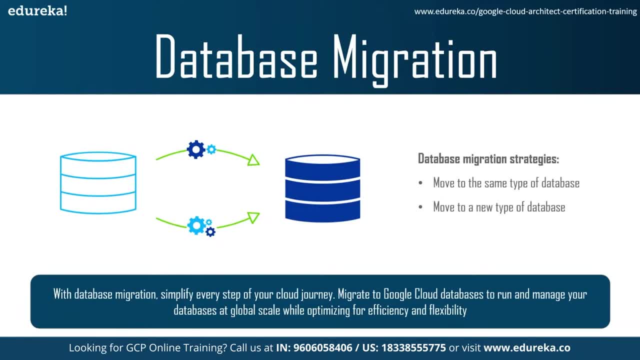 flexibility. There are two database migration strategies. First one is move to the same type of database, So lift and shift databases to Google Cloud using databases like Cloud SQL for MySQL, Cloud SQL for PostgreSQL, Cloud SQL for MySQL Server, Cloud Memorystore for Redis and Cloud Bigtable, along with Google's open source partner. 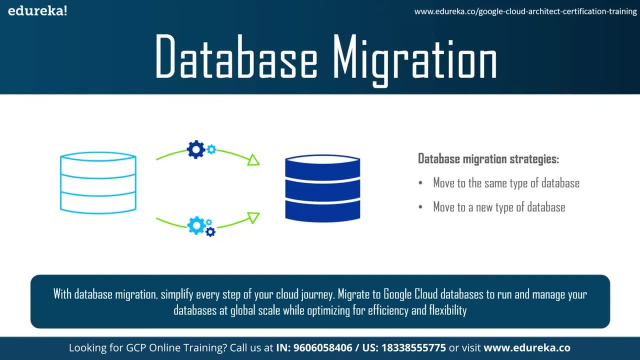 databases like MongoDB Datastacks, Elastic, Neo4j, Influx Data and Redis Enterprise Database migration service for Cloud SQL can help to minimize downtime during migration. Second strategy is move to a new type of database, Whether you are moving from. 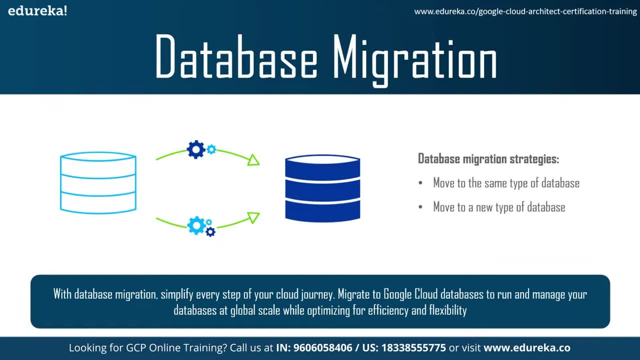 proprietary to open source databases, or modernizing from traditional databases to scalable cloud native databases. we have a solution for you. Leverage your serverless change data capture and replication service data stream to synchronize data across databases, storage systems and applications. Google's 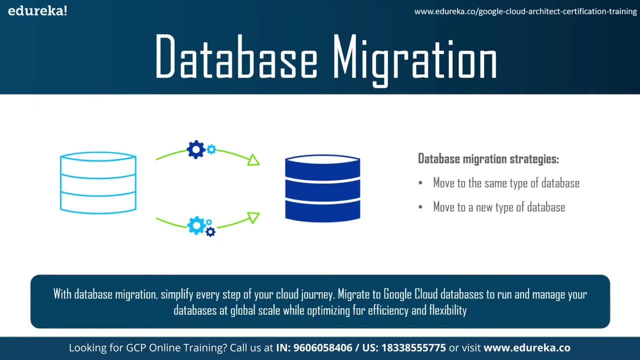 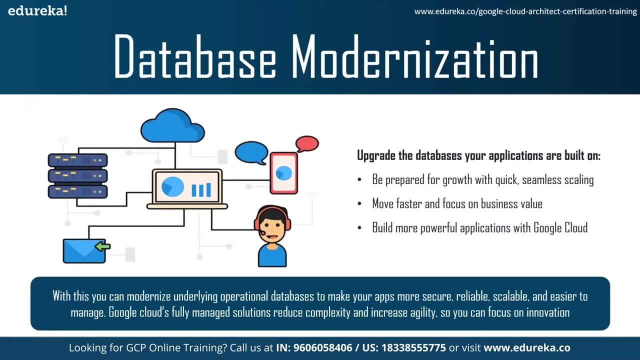 migration assessment guides and partners can help you get started. Now moving on to the next solution, that is, database modernization. So database modernization is primarily about changing applications to work around functional discrepancies between old and new databases. With Google Cloud, you can modernize. 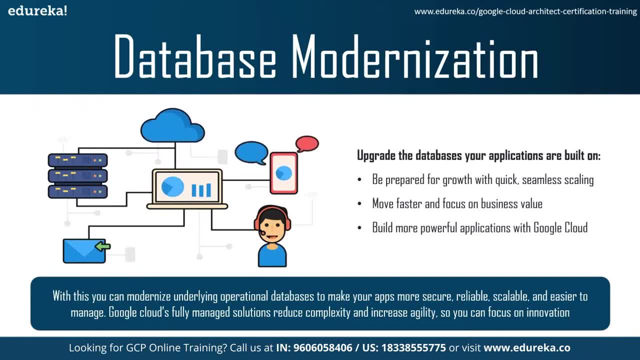 underlying operational databases to make your apps more secure, reliable, scalable and easier to manage. Our fully managed solutions reduce complexity and increase agility so you can focus on innovation, So you can upgrade the databases on which your applications are built on, by being prepared for growth with quick, seamless. 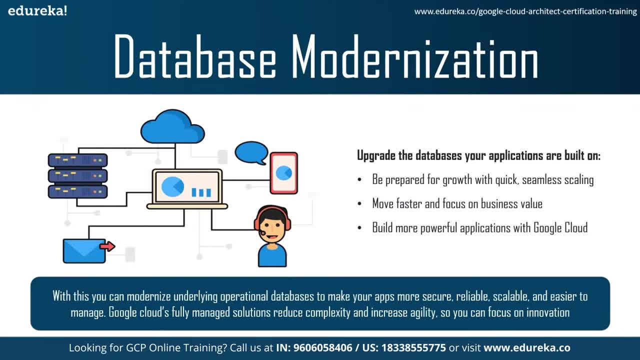 scaling, which means scale Google Cloud databases seamlessly And build cloud native apps that are prepared to handle seasonal surges or unpredictable growth. Second, move faster and focus on business value, which means enable developers to ship faster and perform less maintenance with database features like serverless management, auto scaling and deep integrations, And the 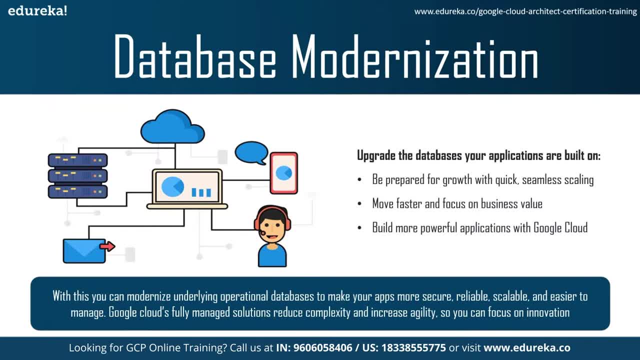 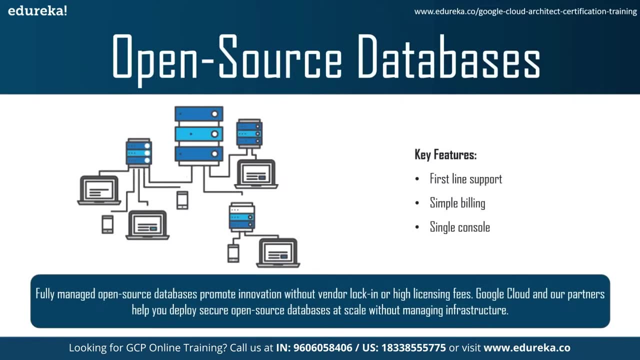 third one is build more powerful applications with Google Cloud To transform your business. with robust ecosystem of services like Google Kubernetes engine easily access data for analytics and AIML with big data. So the third database solution is open source databases, An open source database. 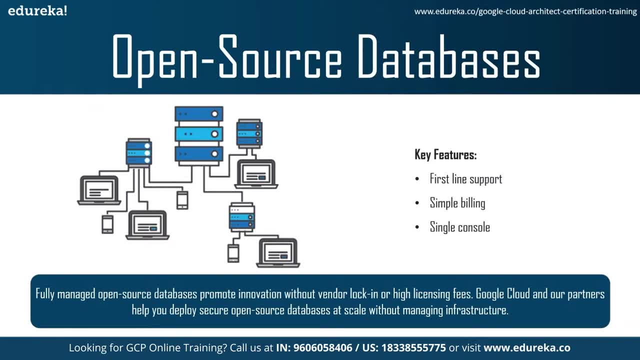 allows users to create a system based on their unique requirements and business needs. It is free and can also be shared. The source code can be modified to match any user preference. So open source databases address the need to analyze data from a growing number of new applications at lower cost, With Google Cloud fully. 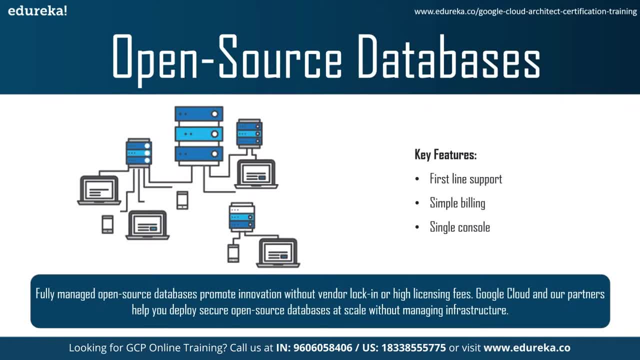 managed open source database. promote innovation without venturing out of the organization, without vendor log in or high licensing fees. Google Cloud and our partners help you deploy secure open source databases at scale without managing infrastructure. So make the most of Google Cloud's commitment to open. 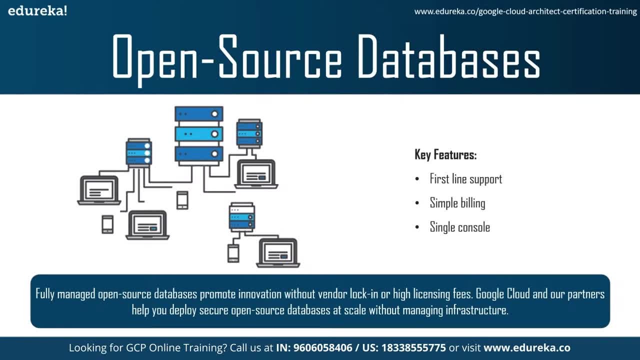 source by first line support. So Google provide first line support for open source databases so you can manage and log support tickets from a single window. Second is the simple billing. So whether you are using NoSQL or relational databases, you will only see one bill from Google Cloud. Third is single. 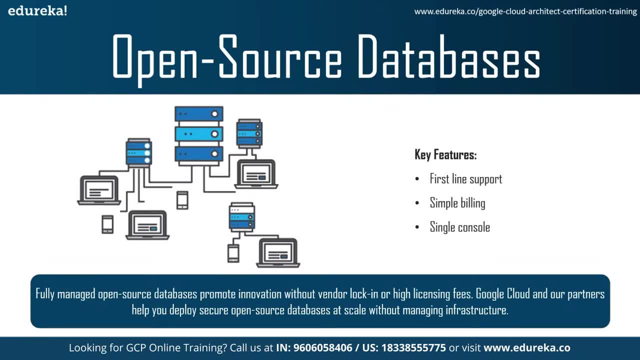 billing. So if you are using NoSQL or relational databases, you will only see one bill from Google Cloud. So you will only see one bill from Google Cloud. Now, the last major GCP database solution is the SQL Server on Google Cloud. 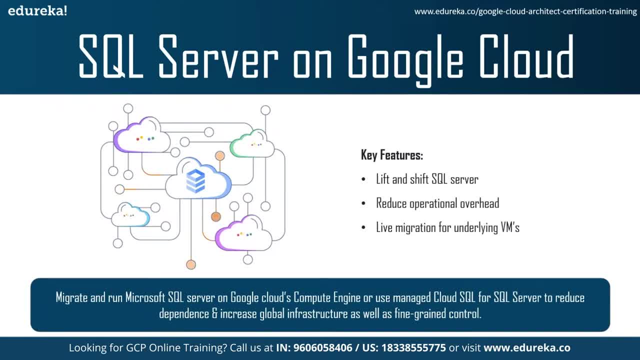 So SQL Server is a relational database management system developed by Microsoft. As a database server, it is a software product with the primary function of storing and retrieving data as requested by other software applications, which may run either on the same computer or on other computer across a network. Its key feature: 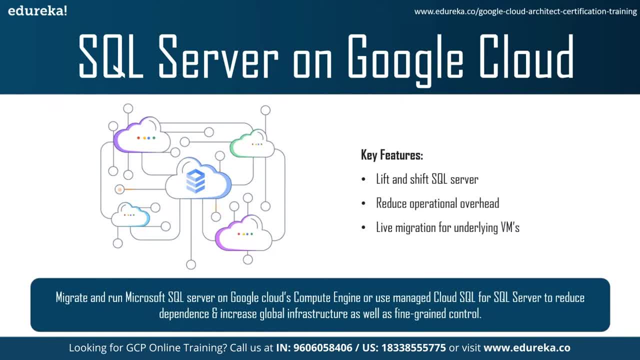 are lift and shift SQL Server, So migrate your existing workloads to Cloud SQL or Cloud Server running on Compute Engine with full compatibility. SQL Server running on Google Cloud works with all of your familiar tools like SSMS and Visual Studio. Connect your existing workloads to the best of what Google Cloud. 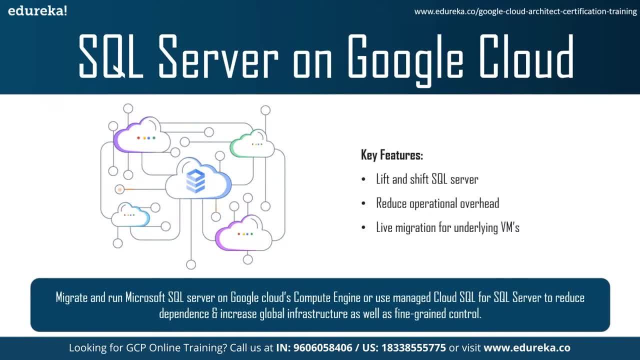 has to offer. Second is reduce operational overhead. So Cloud SQL for SQL Server is a fully managed database service with a 99.95% SLA. Being fully managed includes upgrades, patching, maintenance, backups and tuning regional availability in. 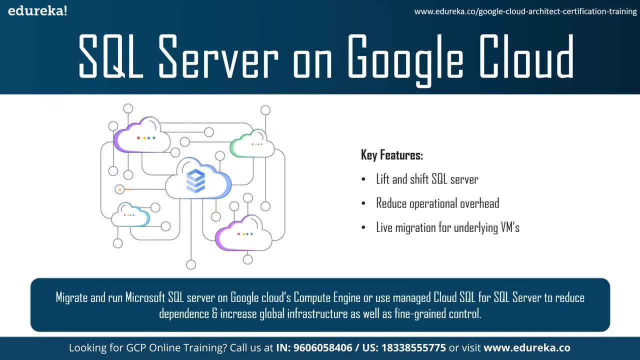 various virtual machine shapes, with memory from 3.75 GB up to 416 GB and storage up to 30 GB for all workloads, provide flexible scaling options to eliminate the need to pre-provision or plan capacity before you get started Now. the last one is the live migration for underlying virtual machines. When you 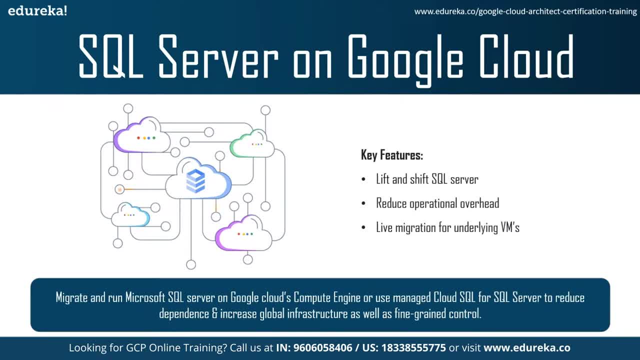 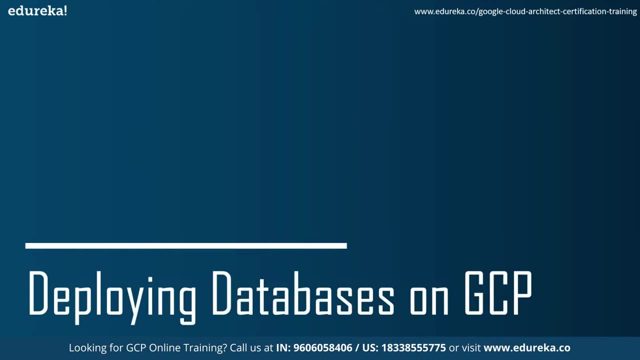 run SQL Server on Compute Engine. the virtual machines can live migrate between host systems without rebooting, which keeps your applications running even when host systems require maintenance. Now let's understand the methods of deploying databases on Google Cloud Platform. So GCP predominantly offers three types of. 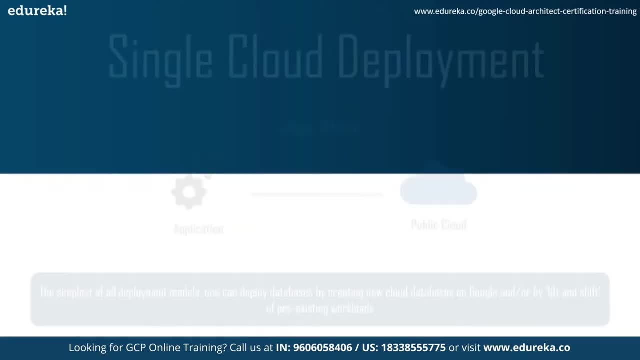 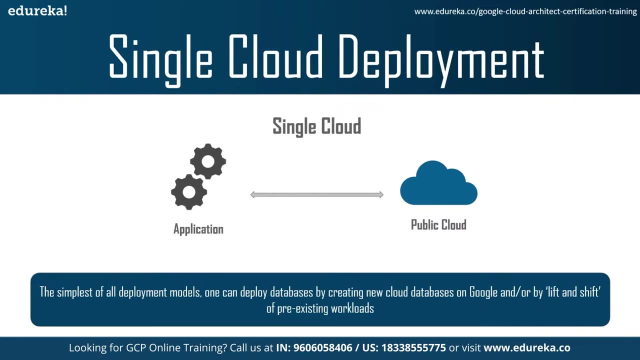 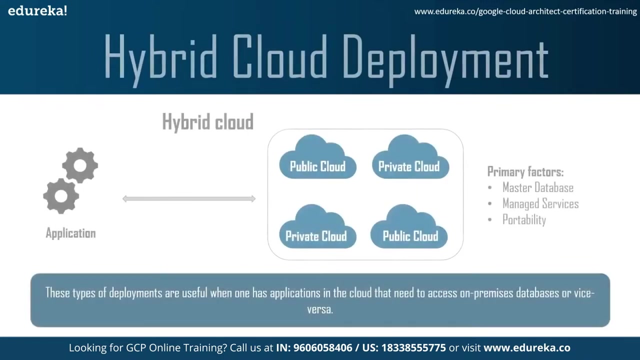 reference architecture model for Google data distribution, In that the first one is single cloud deployment, The simplest of all deployment models. one can deploy databases by creating new cloud databases on Google and or by lift and shift or pre-existing workloads. So the second is hybrid cloud deployment. These types of deployments are useful. 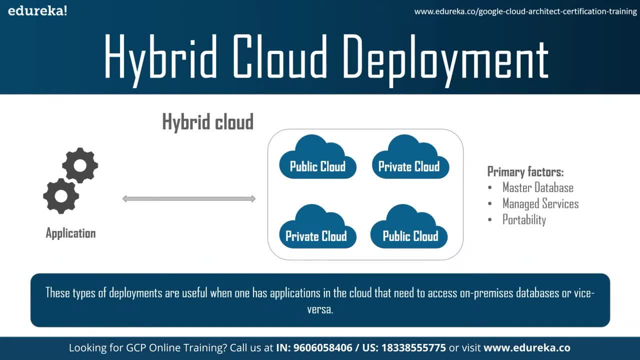 when one has applications in the cloud that needs to access on-premises databases or vice versa. There are three primary factors to be considered when deploying a hybrid model with some data on cloud platform and some on-premises. So that's why it's been shown like a public cloud and private cloud, And so, in primary, 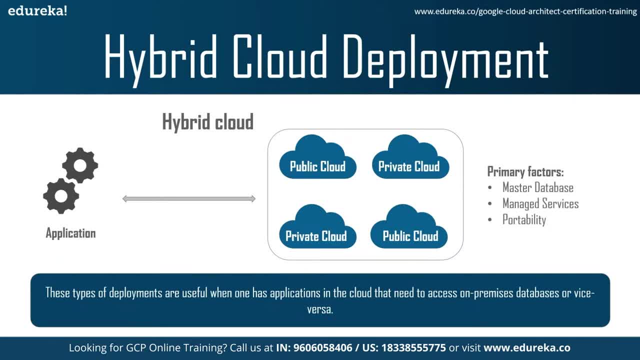 factors. first, one is a master database. First and foremost, you need to decide whether your master database is stored on-premises or on-premises. So that's why you need to decide whether your master database is stored on-premises or. 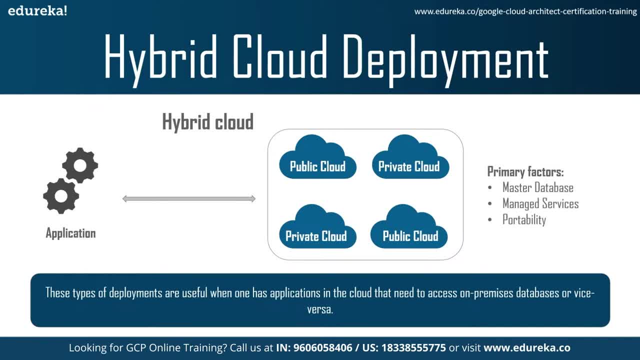 on-the-cloud. Once you choose the cloud, GCP resources act as a data hub for on-premises resources, whereas if you choose on-premises, your in-house resources synchronize data to the cloud for remote use or backup. Second is: 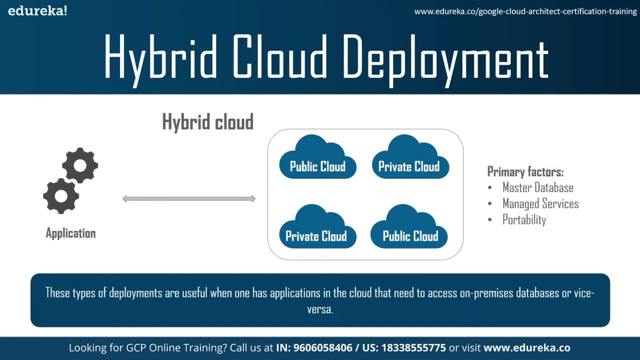 managed services, So available for resources in the cloud. these services comprise scalability, redundancy and automated backups. You, however, have an option of using third-party managed services. Third is portability, So, based on the type of data store you choose, you can use third-party managed services. 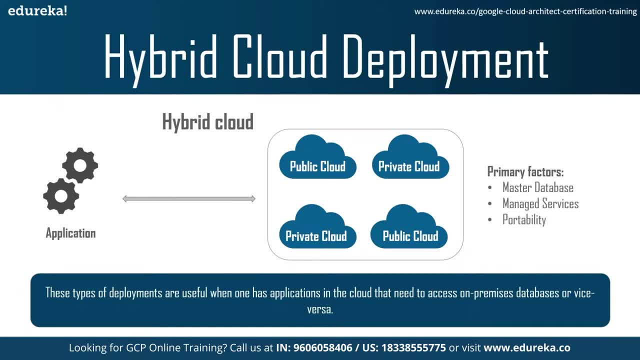 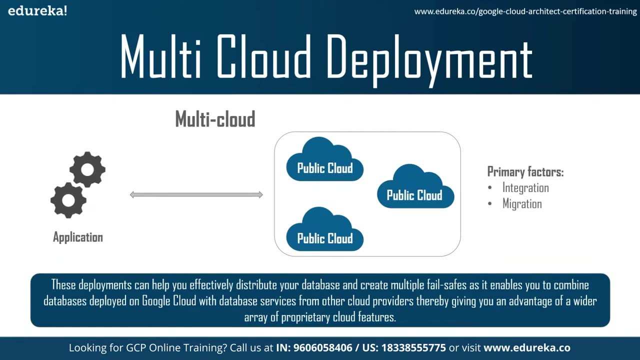 The portability of your data is affected too. To ensure reliable and consistent transfer of data, you need to consider a cross-platform store such as MySQL. So the third kind of deployment is multi-cloud deployment. These types of deployments can help you effectively distribute your database and create multi-fail. 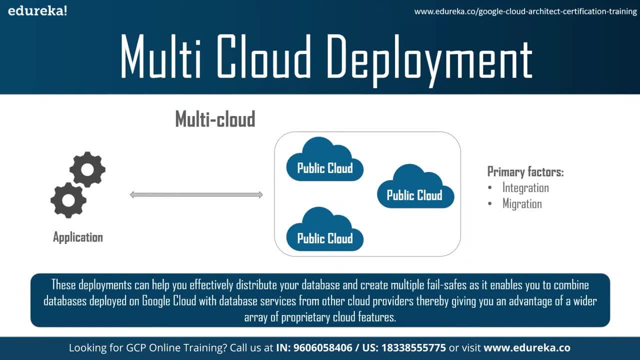 saves, as it enables you to combine databases deployed on Google Cloud with database services from other cloud providers, thereby giving you an advantage of a wider array of proprietary cloud features. And there are two primary factors to be considered when deploying this model. First is integration, So ensuring that client 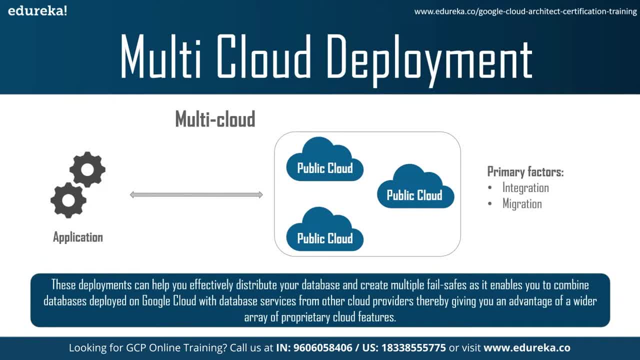 systems can seamlessly access databases, regardless of the cloud they are deployed on. For instance, use of open-source client libraries to make databases smoothly available across clouds. Second is migration. So, since there are multiple cloud providers, one may need to migrate data between clouds with the help of database. 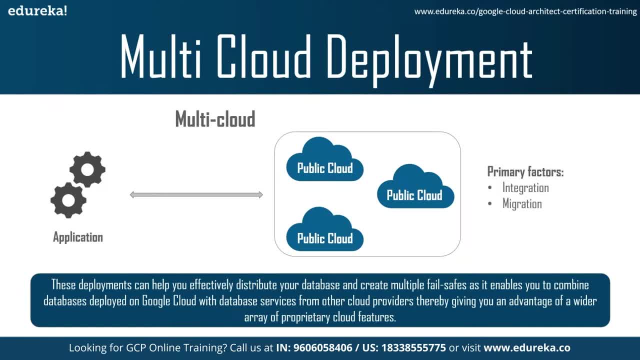 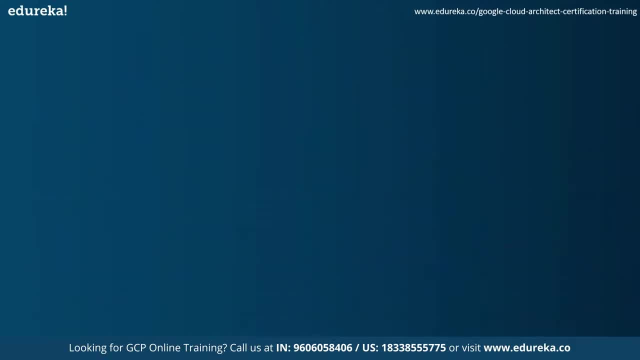 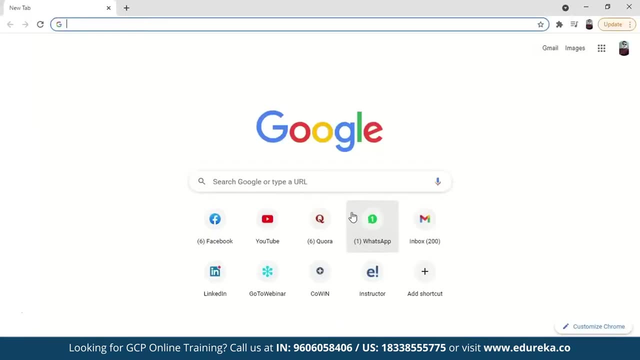 replication tools for export or import processes. So Google Storage Transfer Service is one such tool to help you with database migration. Now that you have a theoretical understanding of GCP database services, let's now deploy a database service on Google Cloud Platform, So you can just go. 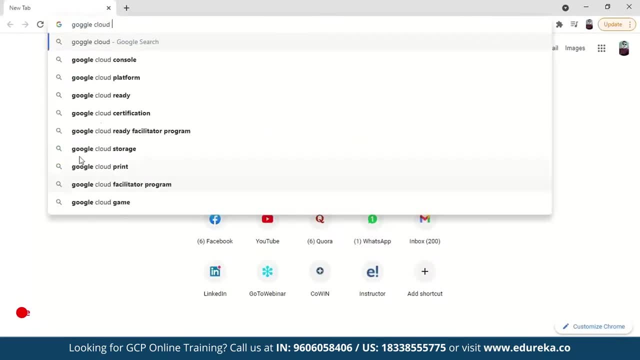 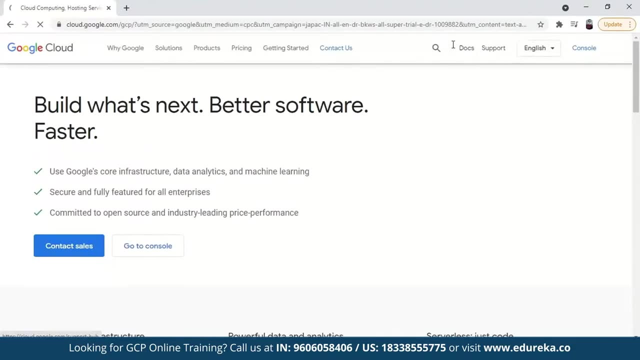 to this: to search for Google Cloud Platform, Just open this link and go to the console. You can also go to the documents part and you can understand more about the database services quite briefly. But right now let's- because we are working on this, we are going to like demonstrate it practically. Let's go to the console. 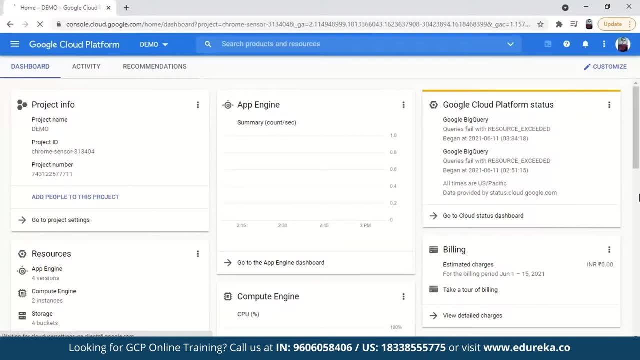 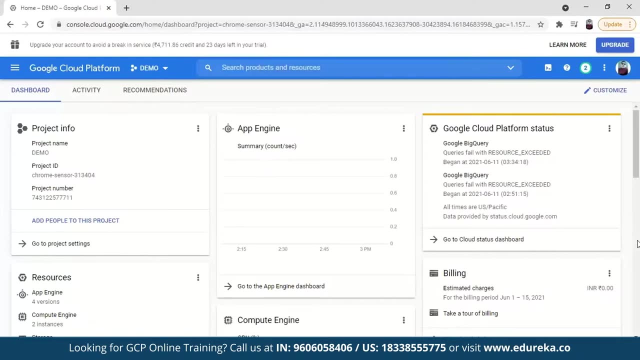 So this is how the Google Cloud Platform console looks like. Also, if you don't have an account on Google Cloud Platform, then create one Like. Google Cloud Platform is a very nice platform to have your account on. You get a free tier in it, Like you can. 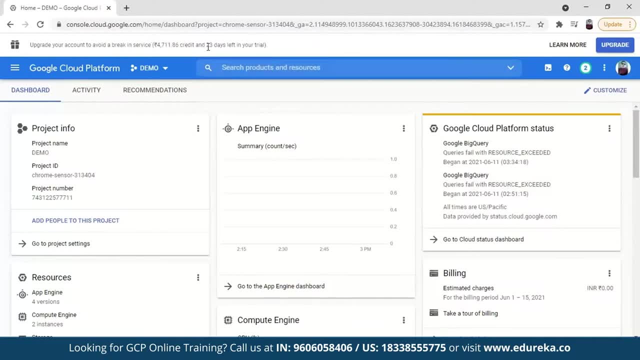 see here, my free trial has like 4711 credits and 23 days left in it. What happens is you get a free trial of 90 days in which you get the 300 US dollars of credit So you can use that credit Like during the exercise. I'm going to explain how to use that credit. 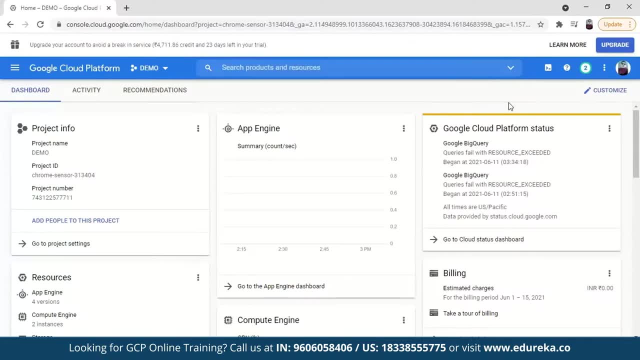 I'm going to explain you in this Also. like, when you create this account, it will just debit one rupee and it will also get refunded to you quite soon, So you just have to give your credit and debit card details also for it. Okay, So let's start, You just. 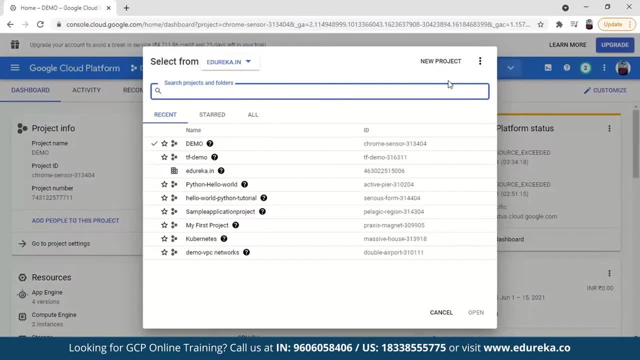 go to my demo. this place, This demo is just the name of my project. You have to create your own project. You can just go to new project and create your project, Give it a name and that's it. I have this demo and several other projects, So I will go with demo only So. 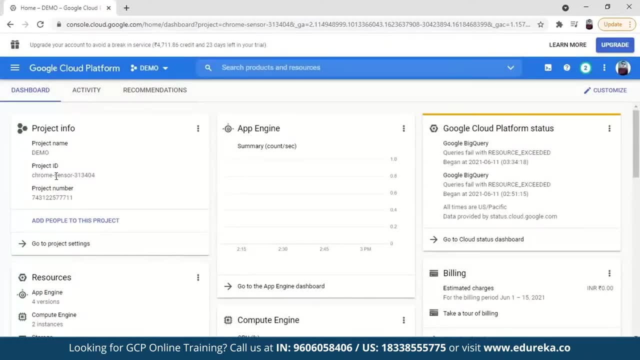 that's the name of my project, So these are the project name. project ID, name of the project. project number is given. So what I'm going to explain here today is like this: database services, Cloud SQL, So Google Cloud SQL service. So where I will be creating 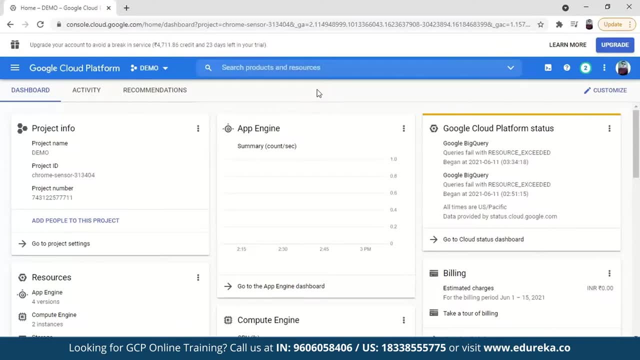 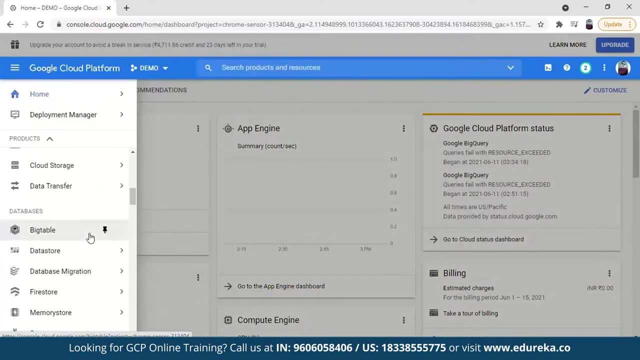 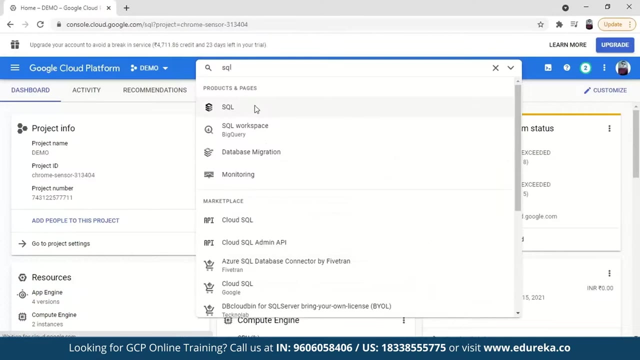 an SQL instance and also, like the database also, I will be creating in it and also a user account. Okay, So you can just go here and go to databases. From here, you can go to SQL, or you can search from here. Just search here, SQL. So yeah, we are here, Let's go. 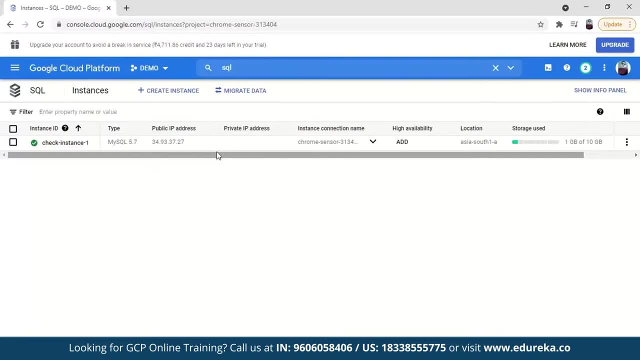 to SQL. So this is like one of the instance which I have already created. So that's why it's showing like this. But when you open it for the first time, it asks for what kind of instance you want to create, like MySQL or the Postgres SQL or any other. So, because I have already 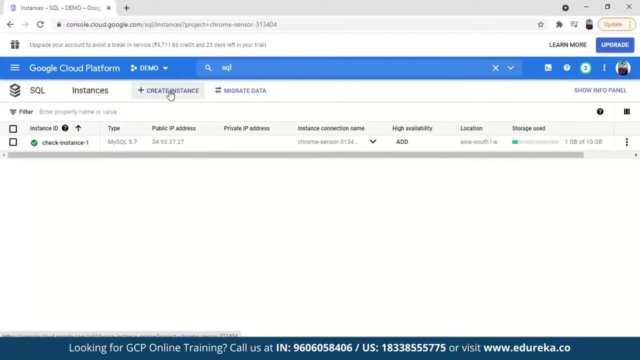 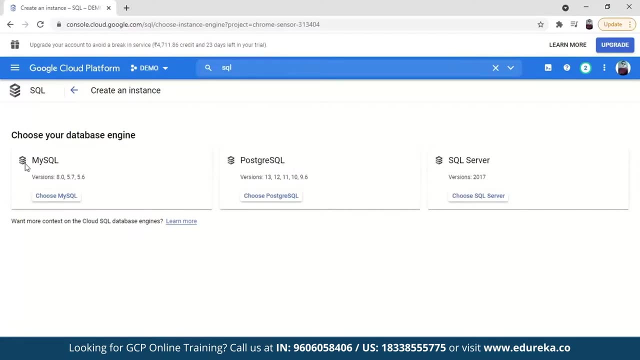 created one, So it's not asking me. I will just go and create the instance from here. Yeah, This page you will get. Okay, That's what I was saying: MySQL, server, Postgres, SQL or MySQL. Okay, So I will be creating MySQL So you can give a name. One more thing: It. 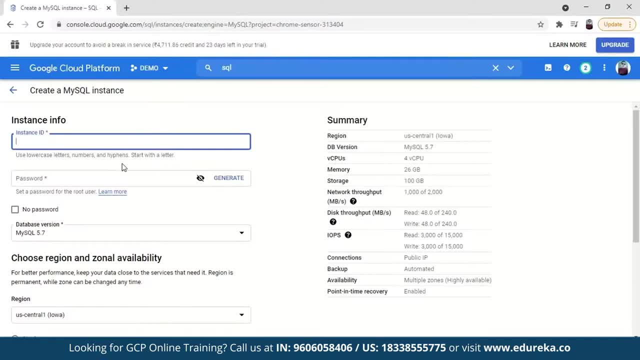 should be unique. It should not like cannot repeat the same thing, So you can give a unique name. So I will just give database service demo. Also, there should be one number. So yeah, database service demo 1.. Okay, Also give the password if you want to Right now. 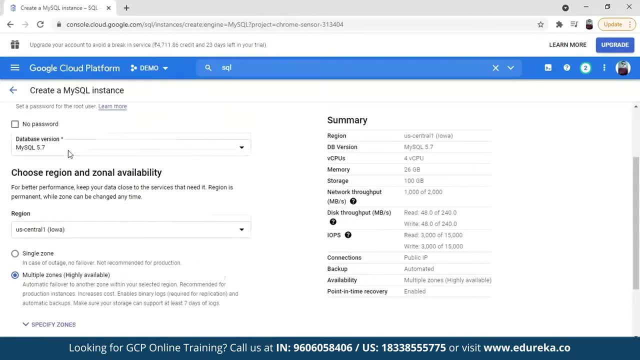 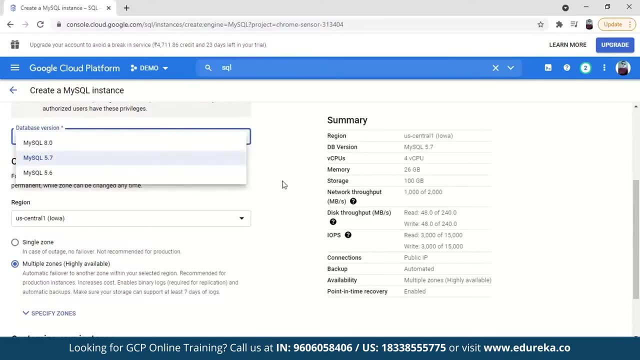 we are just demo, So I will choose no password. Also, choose the version from here for it. Right now I am going with MySQL 5.7 only. Also, select your region. Like I have this region nearest to you. Like I have, region nearest to me is Asia-South. So I will just. 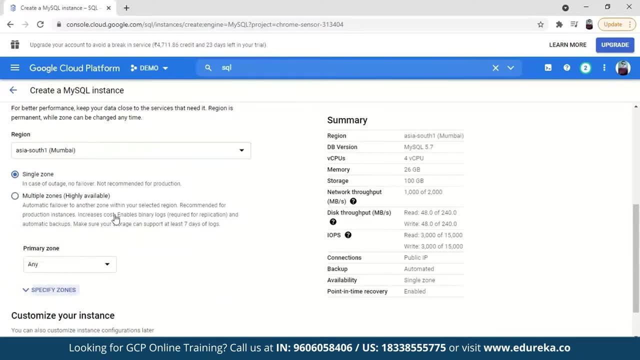 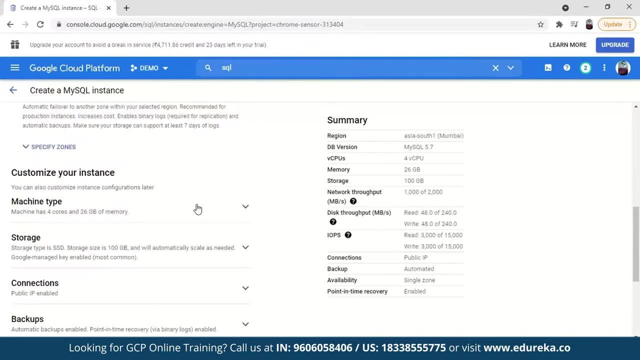 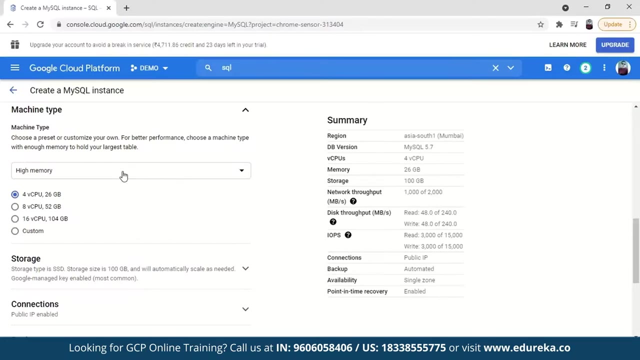 select your zone, So Asia-South for me, Okay. Also, you can like do further customizations. So let's see the machine type, So select whichever is suitable for you Like. right now I don't require quite a high one Like, so I will go for a standard one, But like. 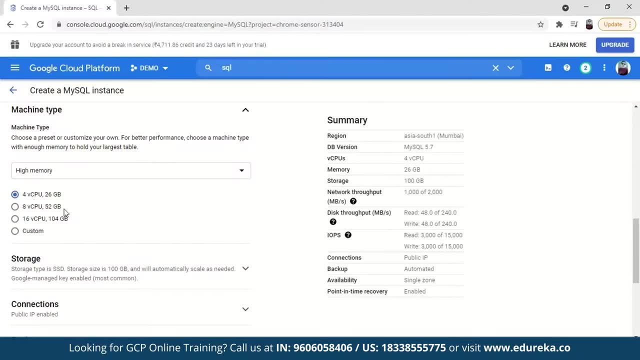 here we have like, in high memory we have 4 virtual CPUs and 26 GB memory, 52 GB memory with 8 virtual CPUs and then 16 virtual CPUs and then 4 GB memory. Then you can customize it by yourself also, So you can just give by yourself whatever you want to select. 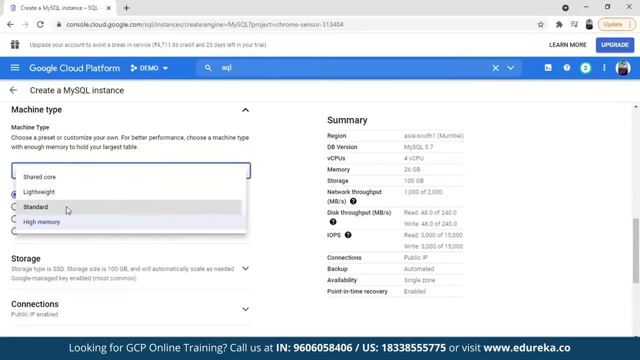 Okay, Then right now I will go with the standard one. So that's more than enough, because the more higher the features you will choose, the more it will cost. Okay, So remember that. So I will just remember the standard virtual CPUs: 3.75 GB, And then you can choose. 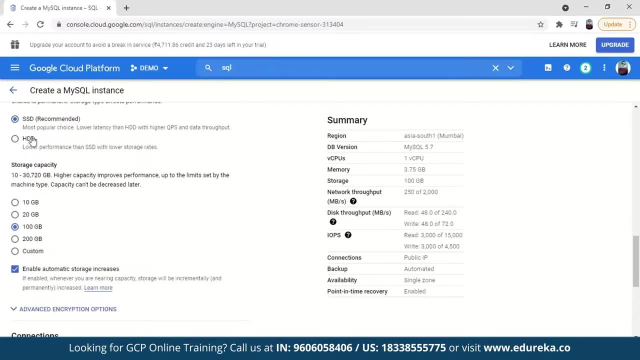 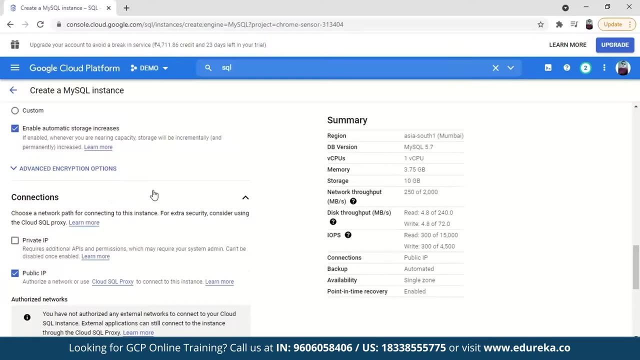 SSD or HDD, whatever you want to choose. So I will just choose 10 GB. That's more than enough for me right now. It was just for demo purpose. So yeah, Then we can also choose. also go for connections, public, private, whatever IP is there, you can choose for that. 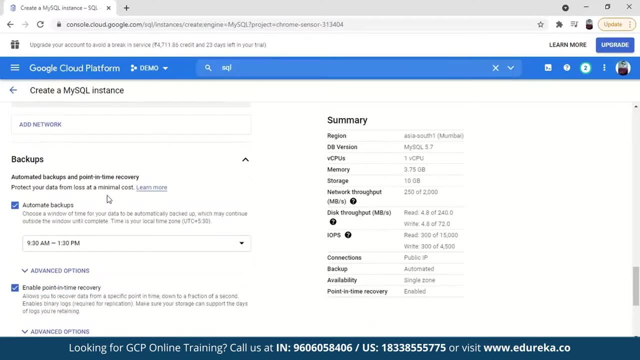 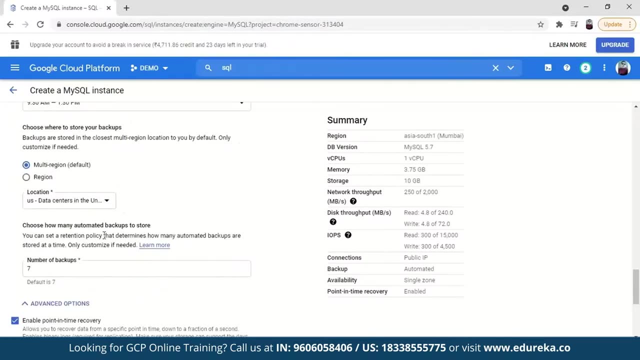 Select that, Okay, And you can then just go to backups, Like at what time you want to get your backup. So you choose the time. Yeah, You can select the region also. That's just okay. My region is okay. Then for maintenance purpose, you can like on which day it gets. 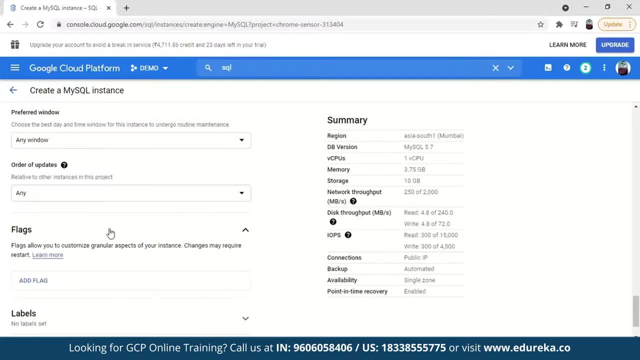 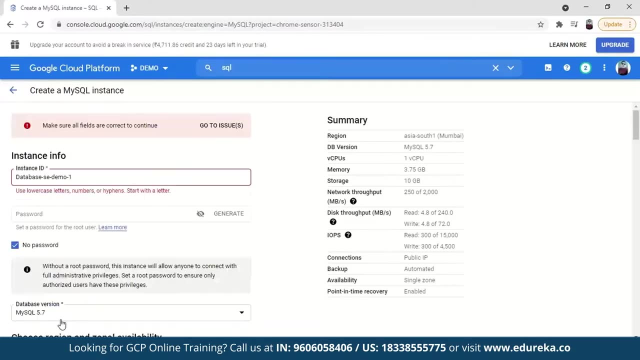 serviced. Okay For maintenance. So that's it. And also, you can select your flag, labels or whatever you want to choose. Okay, So everything is done now. So let's create the instance. Okay, Use lowercase letters. Okay, Remember that to use the lowercase letters. 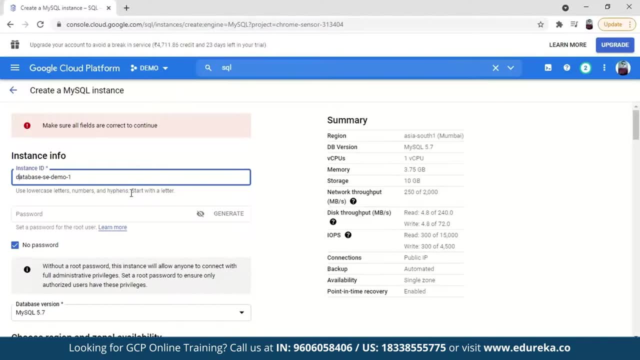 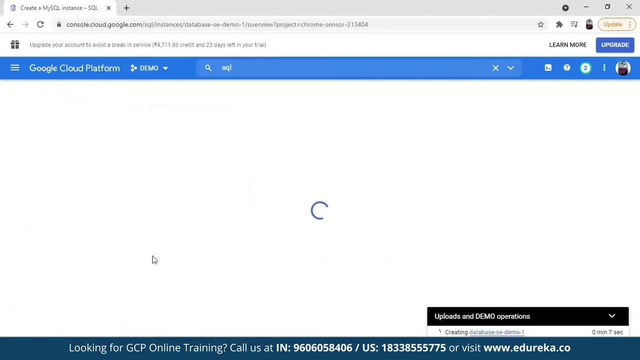 Okay. Also like use lowercase letters, numbers and hyphens. Start with the letter Okay. Strings are given. Keep that in mind. So let's create the instance now. So, as you can see here, The instance has been created. So here it is And here you can see the overview of it. 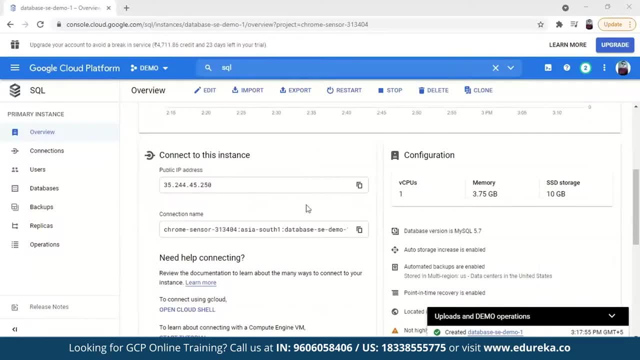 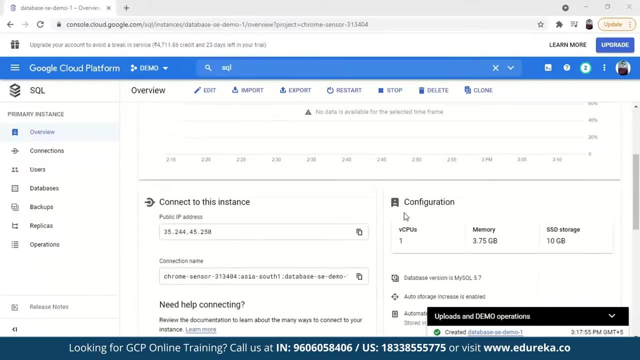 like the things are being given. You can see here like the public ID is given And this is just the CPU utilization. It's given And now, right now, it's not utilizing, So it's not showing anything. So the configurations are given and everything. One more like suggestion. 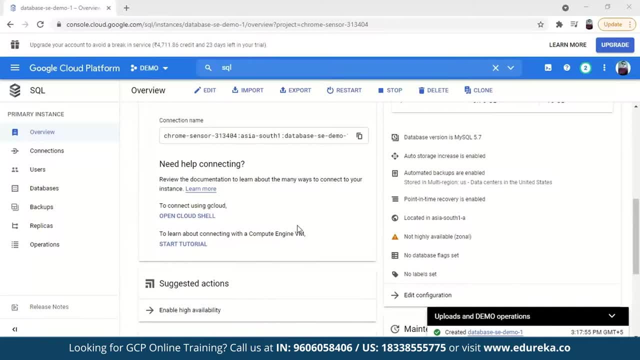 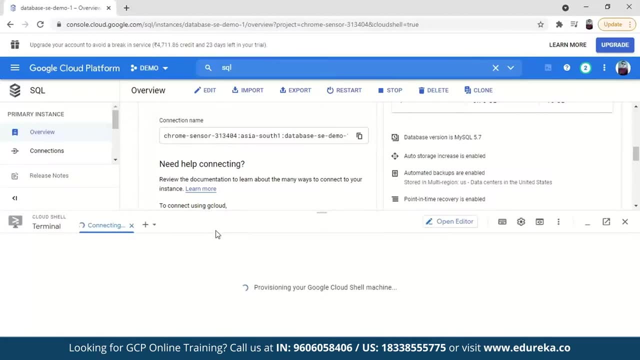 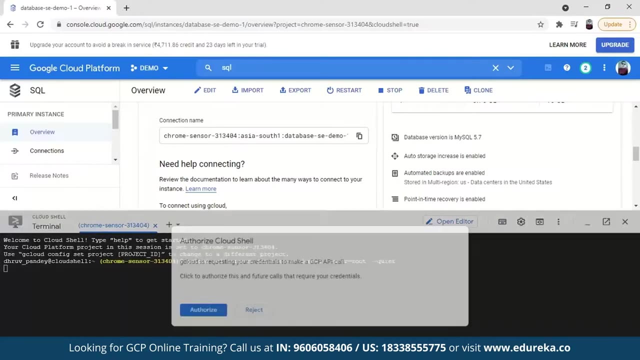 for a service account and everything is given. But one cool thing let you know about this instance is you can connect it through Cloud Shell. So just click here, So it's getting connected to Cloud Shell, So the cloud SQL connect database, So it will show here. Just enter, Authorize it. 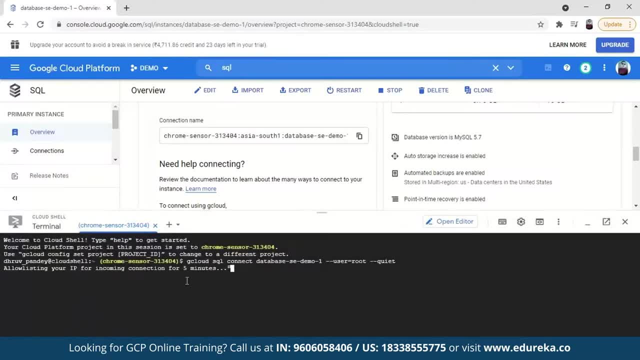 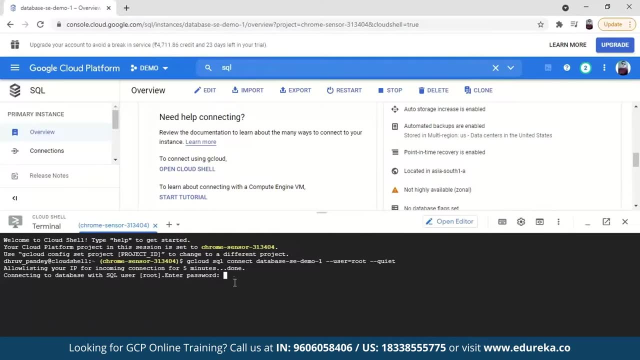 It will take some time. A few minutes it will take, Yeah, Not more than that. So you can see like it's asking for password, But I haven't created a password, So I will just enter. But if you created the password, just enter the password and go for the next step. So 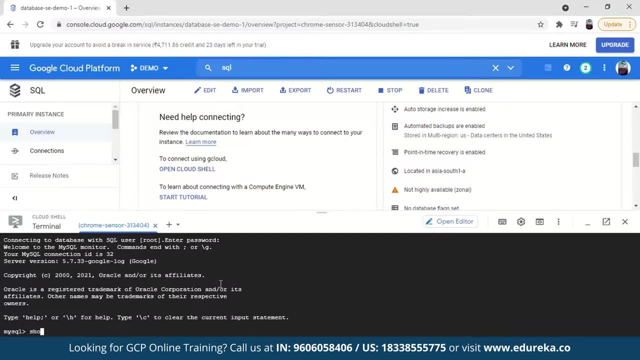 now you can see the databases, So just type for it: show databases. These are the databases And if you want to create a database in it, you can just type create database demo or you can just give test database service. Okay, So yeah, Okay. 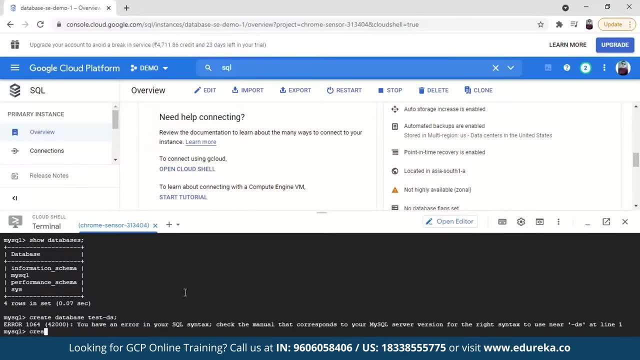 Just don't give hyphen or anything like that. Okay, Just say: create database test. Okay, Yeah, So it's got features. You can just show databases And you can see here test has been created. Okay, So now you can just exit from here. 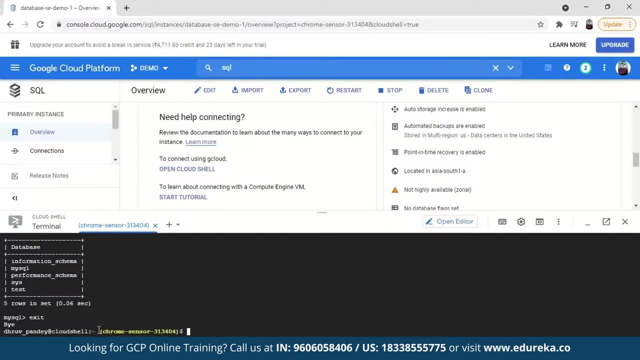 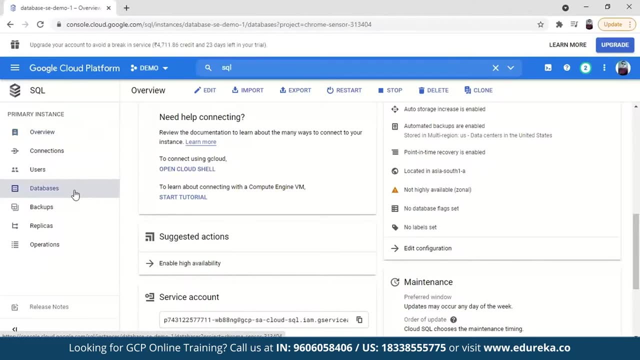 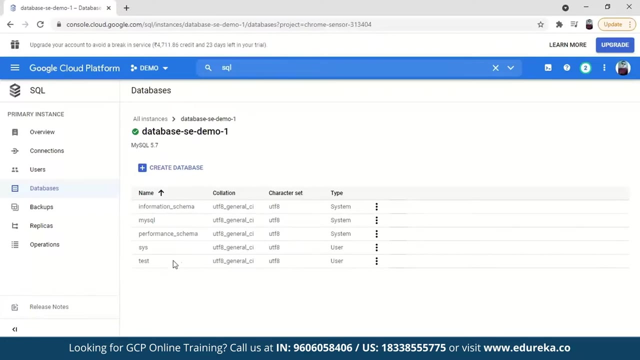 So exit. So you have to exit again Now it will be exited from Cloud Shell. Okay, So now you can come to databases. So under database se, demo one, That's the instance name of our SQL database. So yeah, You can see, like I mean, this is the name of our SQL. 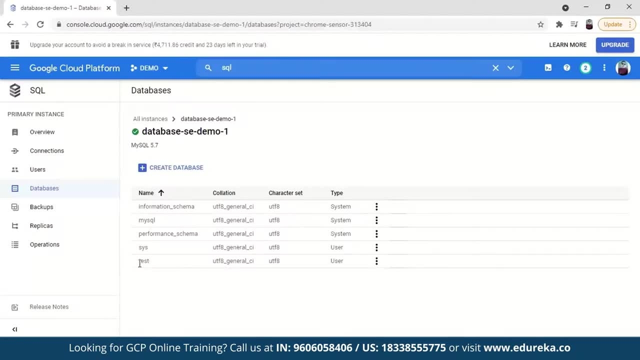 instance database, se demo one. So here you can see like test has also been created, Okay, And also like you can come to users also, Here also default one is there root, So you can create a database from here also Like just have to click here, create database Give. 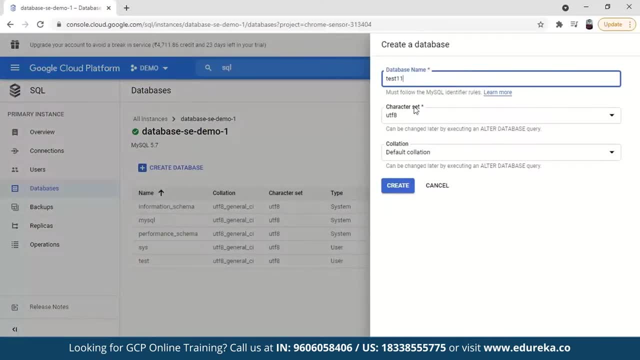 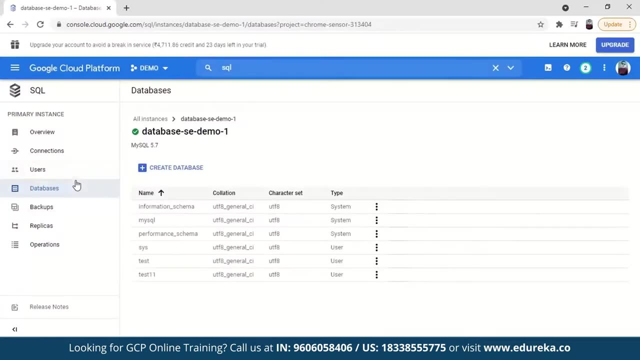 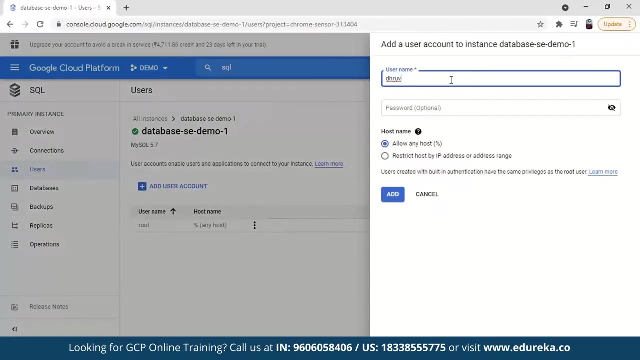 it a name. Test one one. Okay, Yeah, Just create it from here. Similarly, test one one is created. Okay. Similarly, you can go to users and create a user account with the name through 66. That's it. And give a password also. It's optional, But I mean just we can. 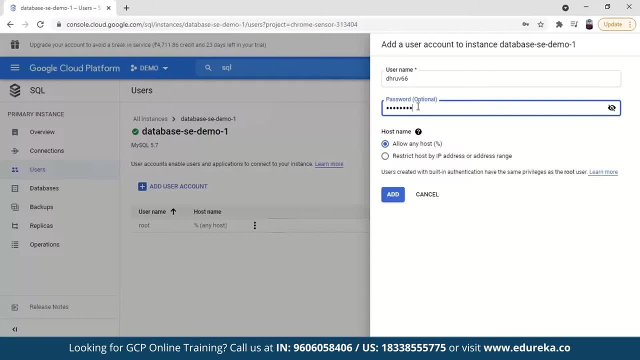 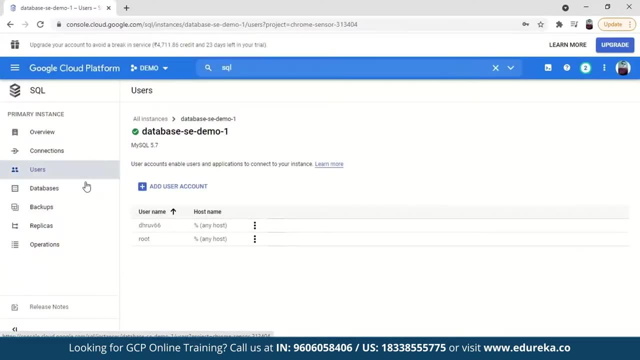 just give one. Go through 662.. Just create, So the user account will be created. Yeah, Okay, That's how users and databases have been created. I hope you have understood it now how to create it through Cloud Shell and everything. That's how the instance have been. 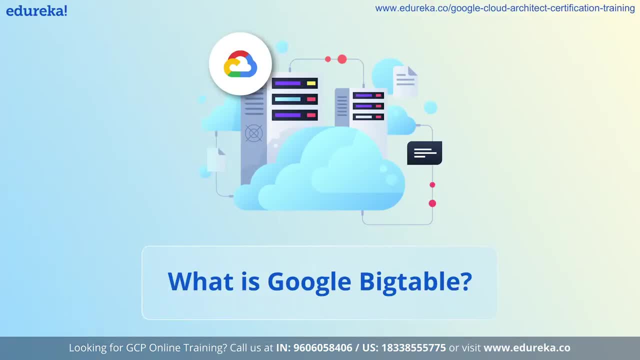 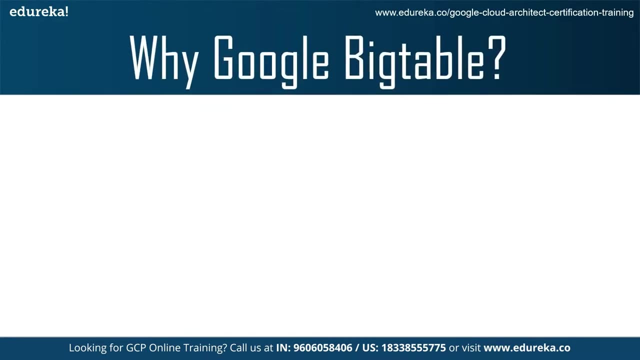 created through Cloud SQL. Why do we need Bigtable? In the age of Internet of Things, data is only going to get bigger and more complex. Having such a large amount of information requires an equally complex and powerful database, And Bigtable seems to rise to that occasion, Even with the presence. 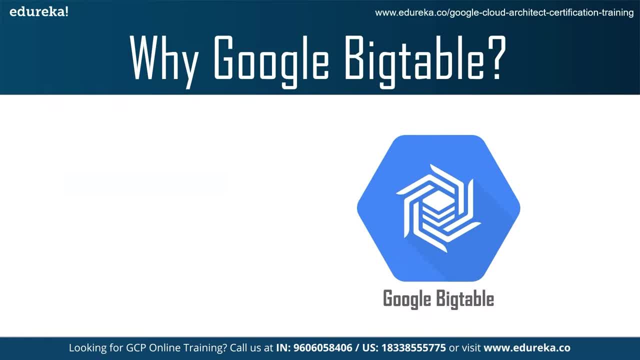 of other competitors in this space. here are some of the major reasons why you should consider Google's Bigtable for database needs at your organization. So first is lower costs. Google has introduced an interesting pricing strategy For Bigtable by separating the storage and computing needs of organizations. This makes 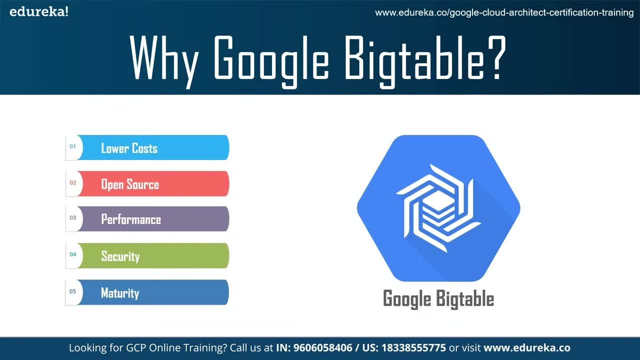 Cloud Bigtable a very useful proposition for companies who might need to store large amounts of data over an extended period of time, especially if they only require minimal access and manipulation of that information. This makes it more cost effective compared to competitors, who usually charge for each read or write operation on the data. Google has even claimed that charges. 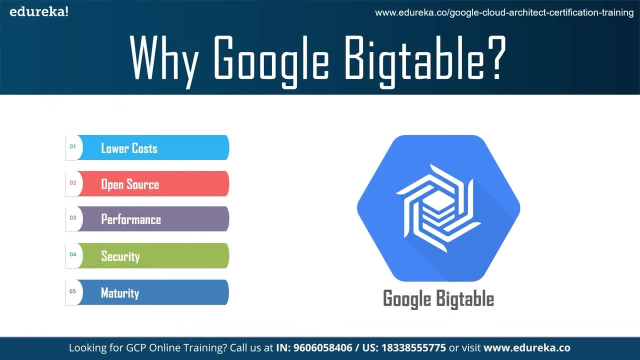 on Bigtable would translate to half the cost as compared to the cost of the data. Google has also claimed that the cost of the data is less compared to competitors, But this might depend on the required configuration, among other factors. Second is its open source. So Bigtable is available as open source, which is a major 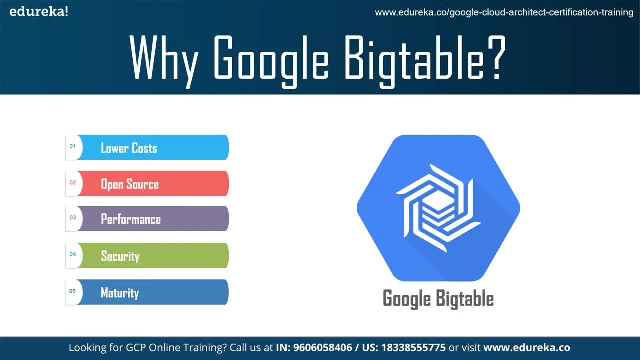 advantage, as it enriches the kind of comments and contributions it receives over time. Users are then assured a good degree of improvement and addition with an active developer base in the open source context. This also means that Bigtable would adhere to the required industry standards. 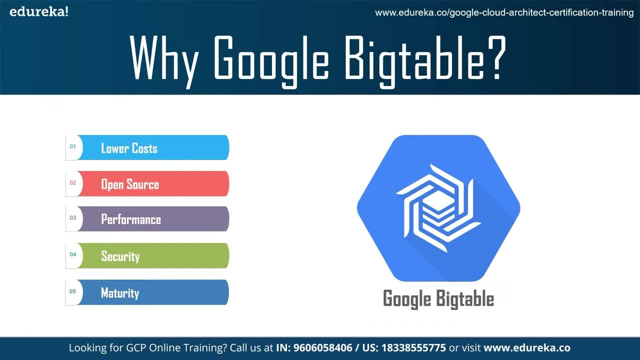 For example, the HBase API, which is one of the most popularly used bases, is seamlessly supported, and organizations that already use products like HBase would find it doubly simple to set up Bigtable for their data. Third is high performance. Google is no stranger. 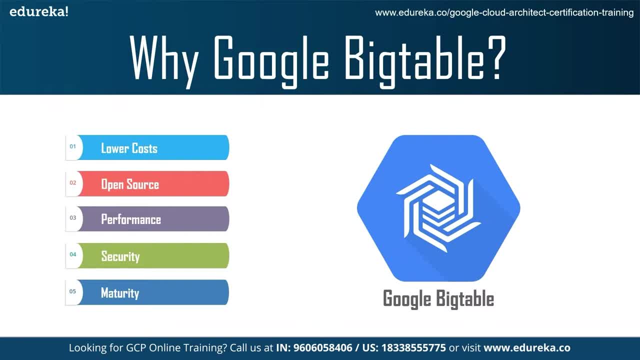 to high performance requirements and as Bigtable has already been used internally, there is not much doubt that it can provide the needful to external business customers as well. Much of the setup and initial storage calculation is done in an instinctive manner requiring minimal user inputs, which results in saving much time and effort. for new customers, Many 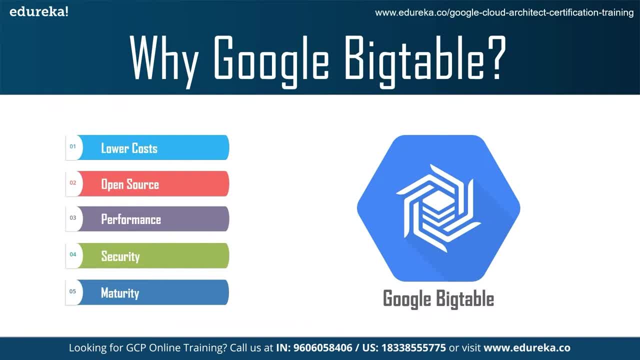 initial users, including SunGuard and Qubit, have been more than satisfied with Bigtable's ability to handle large volumes of data. that is supported by the ease of setting up and scaling as required. The analytics support provided by Google could also be invaluable for the needs of many data-heavy industries. 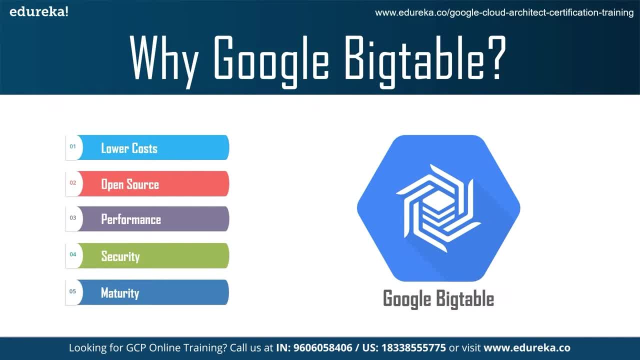 Fourth is it's highly secure. With large amounts of data, concerns for data security also escalate just as much, So Bigtable offers a replicated storage strategy with algorithms for encryption of data, something that is sure to help allay these concerns. Customers can also bank on Google's expertise in the area, with their long-standing experience of 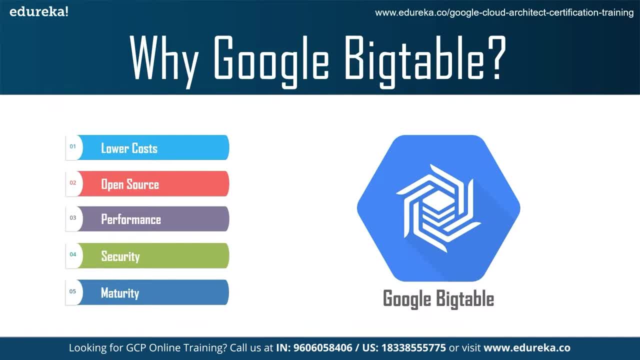 handling the privacy and security of large amounts of data. Fifth is maturity. Due to the simple fact that Bigtable has been used for a number of years and is used internally for a significant period of time by a data giant like Google, it can promise a high level of stability and maturity to its users. It is not at all comparable. 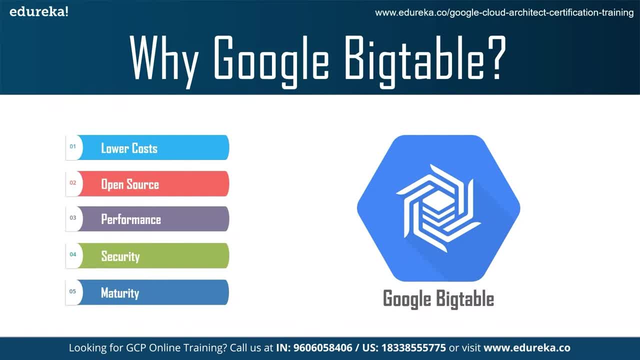 to a new and untested product and might probably score favorably on many fronts when compared to long-standing players in the arena as well. Due to its internal use, customers can also be sure of its continued availability and enhancement, Drawing on its strengths as an organization. 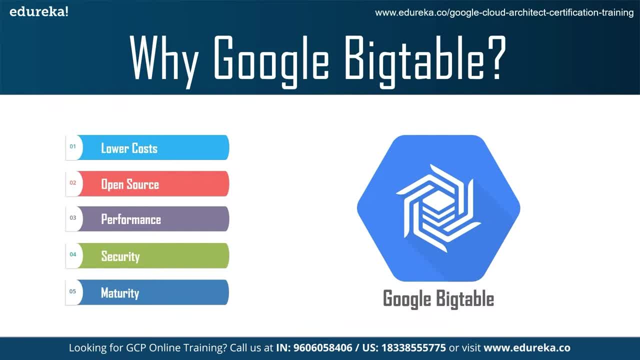 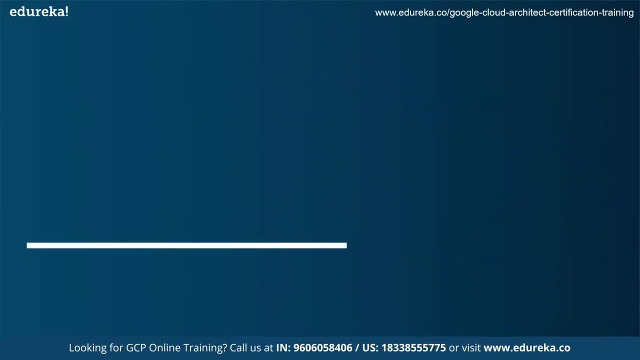 Google also lists many of its service partners as well. For example, Pythian, CCRI and Sengar are companies who can build platforms to help support a faster transition to Bigtable. Now, what actually is Bigtable? Let's understand that. 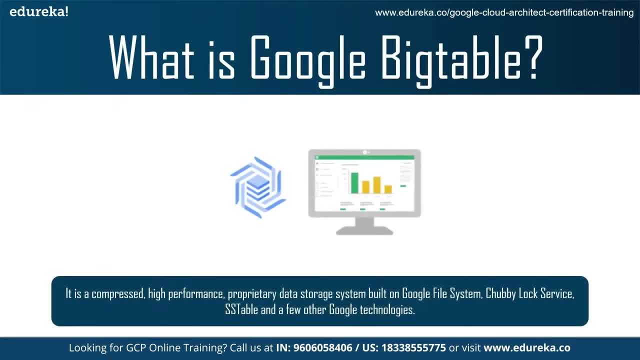 First of all, Google Bigtable is a key-value database. A key-value database is a data storage paradigm designed for storing, retrieving and managing associative arrays in a data structure more commonly known today as Dexterity or Hashtable. So Google provides the key-value. 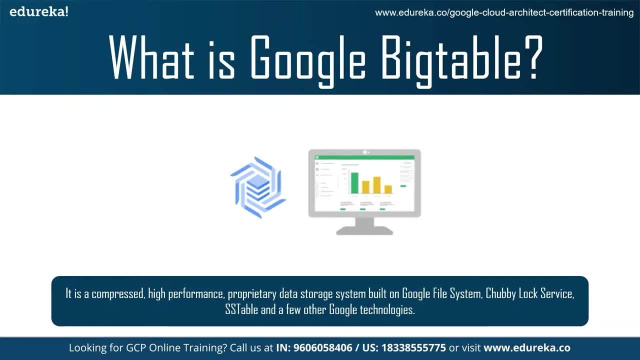 database service in the form of Bigtable. It is a distributed storage system for structured data. Also, it is a compressed, high-performance proprietary data storage system which is built on Google File System, Chubby Lock Service, SSTable and a few other Google technologies. 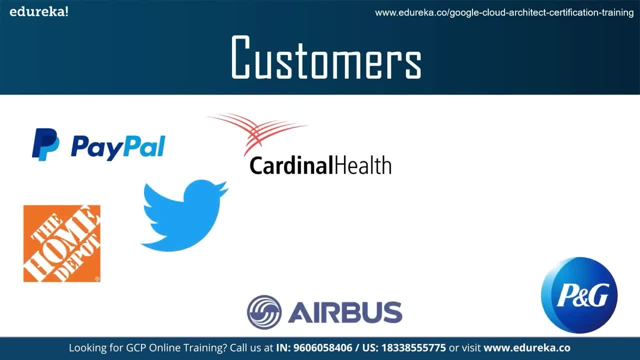 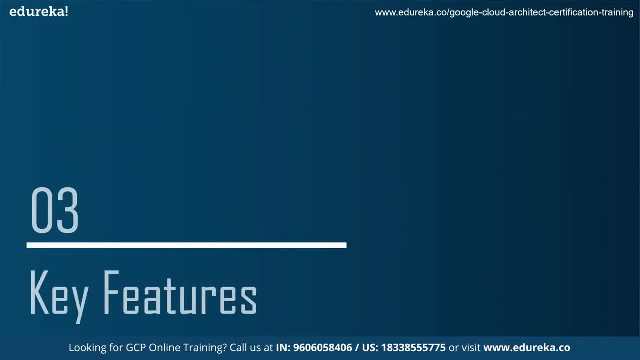 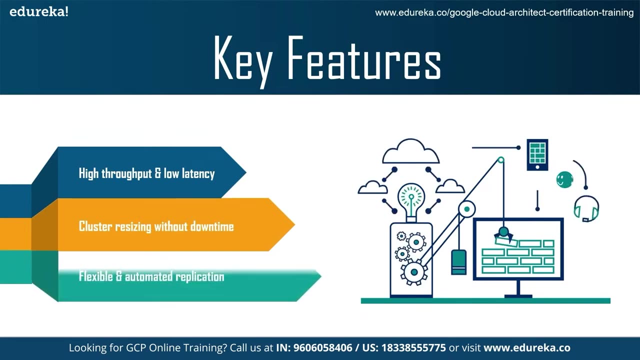 You can see here how many of the world's leading companies are choosing Google Cloud to help them innovate faster, make smarter decisions and collaborate from anywhere. Now moving ahead, let's understand some of the key features of Google Bigtable. First of all, it has high throughput at low latency. Bigtable is ideal for storing a very 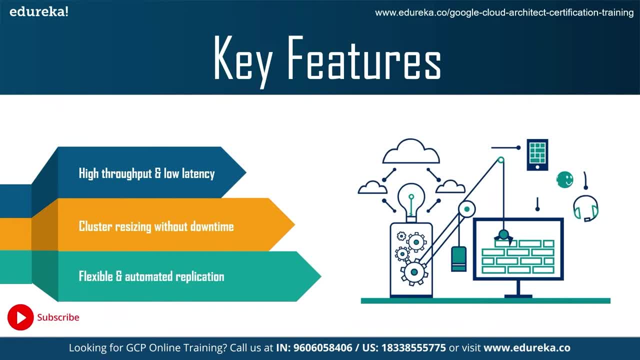 large amount of data in a key-value store and storage environment. It supports high read and write throughput at low latency for fast access to large amounts of data. Throughput scales linearly. You can increase QPS- means queries per second- by adding Bigtable. 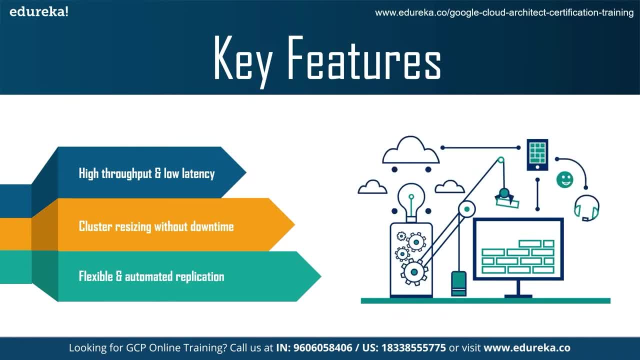 nodes. Bigtable is built with proven infrastructure that powers Google products used by billions, such as Search and Maps. Second is cluster resizing without downtime. It scales seamlessly from thousands to millions of reads and writes per second. Bigtable throughput can be dynamically adjusted by adding or removing. 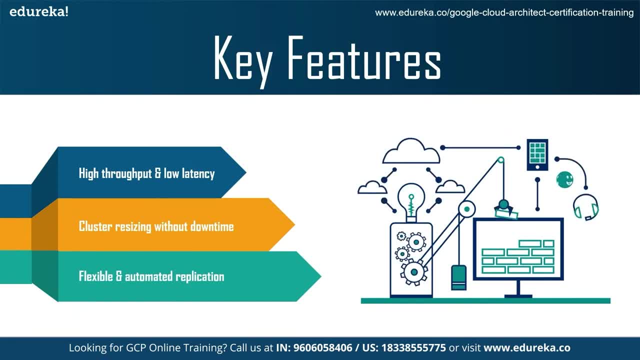 cluster nodes without restarting, meaning you can increase the size of a Bigtable cluster for a few hours to handle a large load, then reduce the cluster's size again, all without any downtime. Third is flexible and automated replication. to optimize any workload, Write data once. 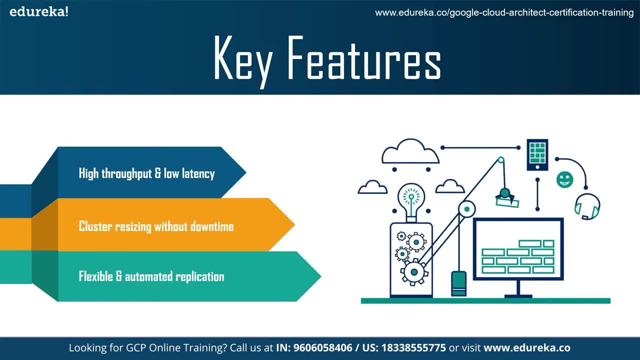 and automatically replicate where needed, with eventual consistency, giving you control for high availability and isolation of read and write workloads. No manual steps needed to ensure consistency, repair data or synchronize writes and deletes. Benefit from a high availability- SLA of 99.999% for instances with multi-cluster routines. 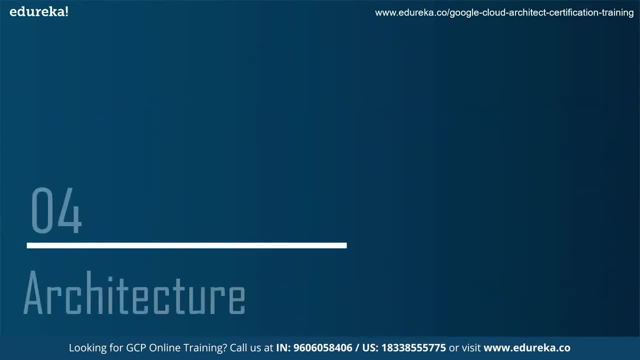 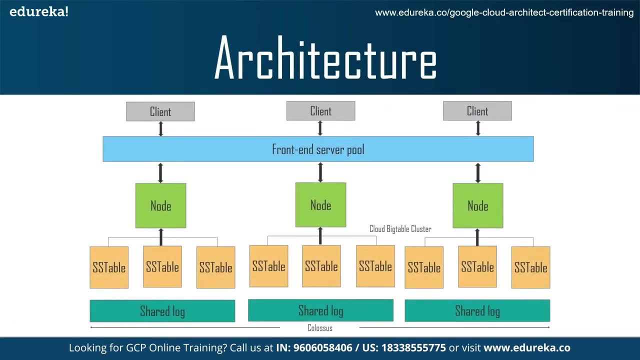 across three or more regions. Now let's understand the architecture of Cloud Bigtable. So we will understand it step by step. So first of all, you can see here like how client requests go through a front-end server and then nodes are organized into a Cloud Bigtable cluster of a Cloud Bigtable instance. 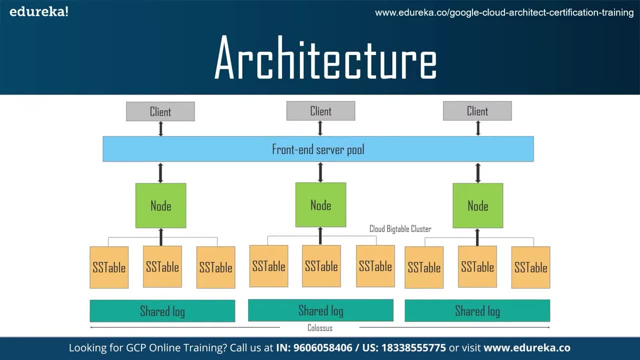 Each node in the cluster handles a subset of the request to the cluster and then a node is added to the cluster. The nodes are added to increase the number of simultaneous requests to handle maximum throughput. Then table is shredded into blocks of contiguous rows called tablets, Similar to edge-based. 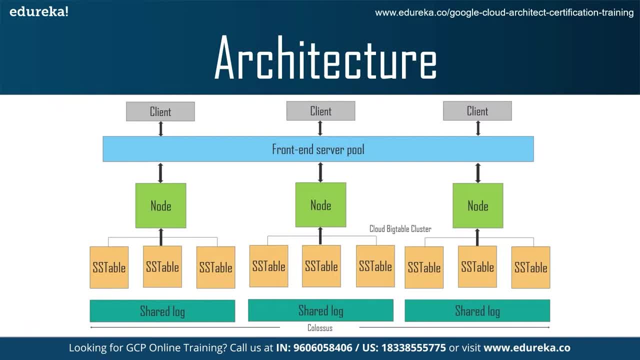 regions. tablets are stored on Colossus, Google's file system, in SSTable format. An SSTable is an ordered, immutable map from keys to value, and both are byte strings. Tablet is associated with a specific node, Like writes are stored in Colossus' shared log, as acknowledged. 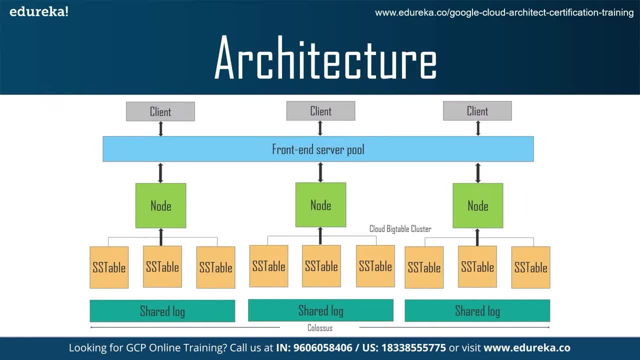 Then data is never stored in the cluster. Tablets are stored in nodes themselves. Nodes have pointers to a set of tablets stored on Colossus. Debalancing tablets from one node to another is very fast. Recovery from the failure of a node is very fast. 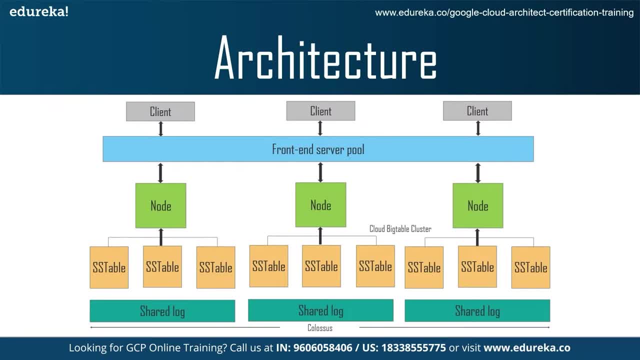 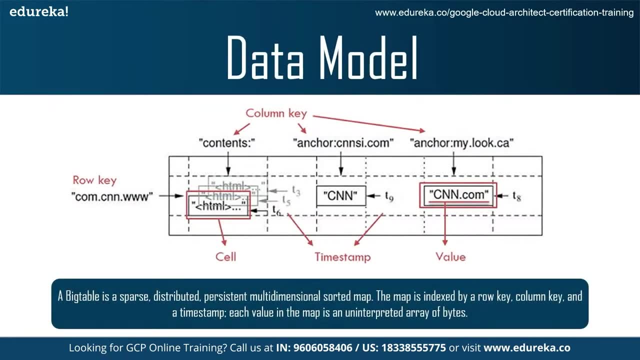 When a Cloud Bigtable node fails, no data is lost. I hope you have understand the architecture. Let's now have a look at the data model of Google Bigtable. A Bigtable is a sparse, distributed, persistent, multi-dimensional sorted map. 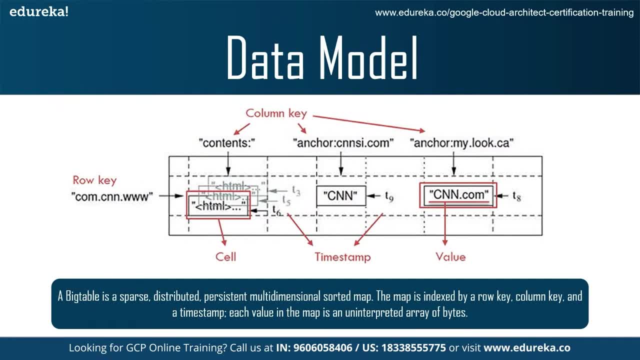 The map is indexed by a row, key, column, key and a timestamp. Each value in the map is an uninterpreted array of bytes. I settled on this data model after examining a variety of potential users of a Bigtable-like system, As one concrete example that drove some of our design decisions. 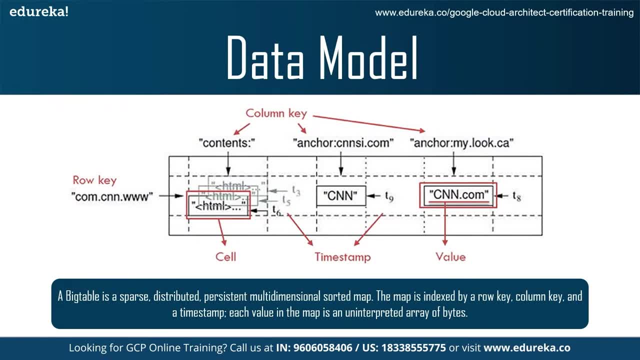 suppose we want to keep a copy of a large collection of web pages and related information that could be used by many different projects. Let us call this particular table the Webtable. In Webtable, we would use URLs as row keys, various aspects of web pages as columns. 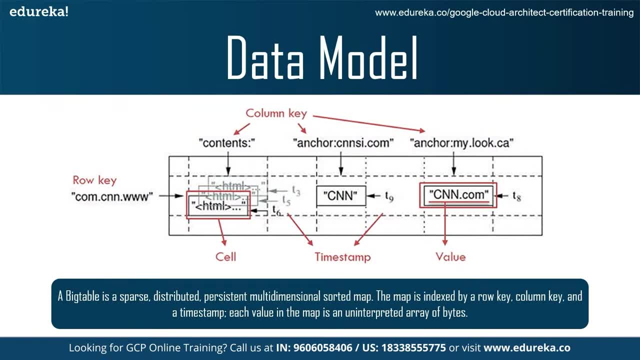 and store the contents of the web pages in the contents column under the timestamps when they are fetched, as illustrated in the figure. In this figure you can see a slice of an example table that stores web pages. The row name is a reversed URL. 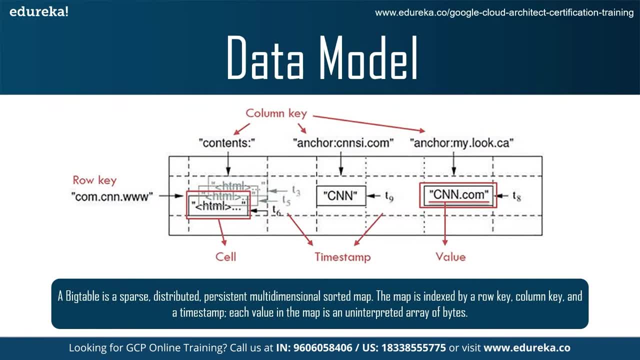 the contents column family contains the page contents and the anchor column family contains the text of any anchors that reference the page. CNN's home page is referenced by both the Sports Illustrated and the My Look home pages, So the row contains columns named anchor-cnn-sicom and anchor-mylookcm. 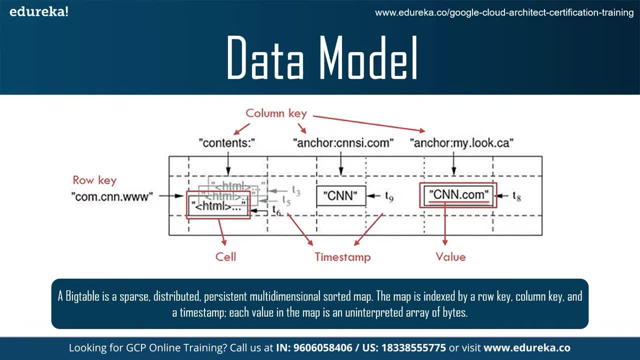 Each anchor cell has one version. The contents column has three versions at timestamps T3, T5, and T6.. Now let's understand the keys in the data model. So first is row key. So the row keys in a table are arbitrary strings. 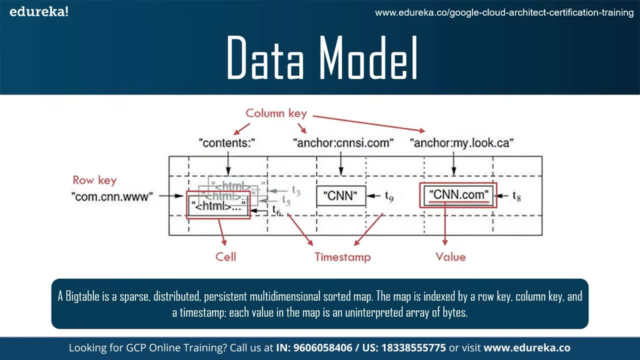 currently up to 64 KB in size, through. 10 to 100 bytes is a typical size for most of the users. Every read or write of data under a single row key is atomic, Regardless of the number of different columns being read or written in the row. 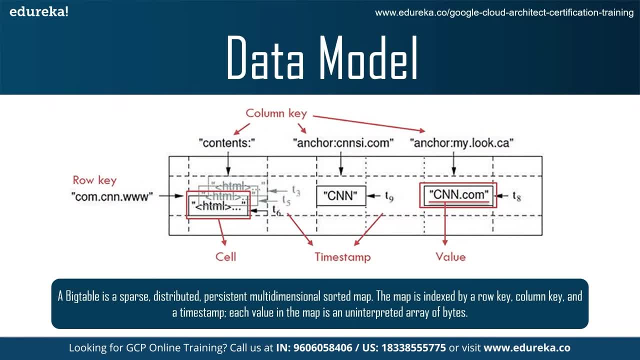 a design decision that makes it easier for clients to reason about the system's behavior in the presence of concurrent updates to the same row. Bigtable maintains data in lexicographic order by row key. The row range for a table is dynamically partitioned. 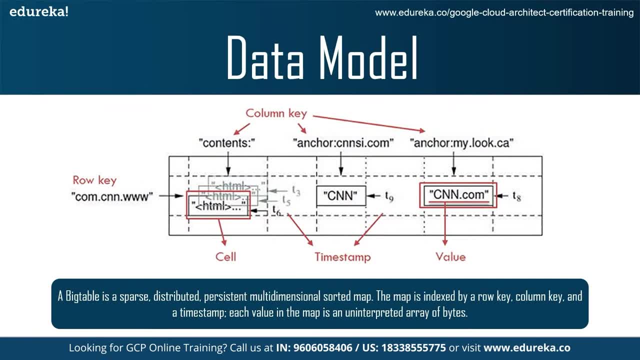 Each row range is called a tablet, which is the unit of distribution and load balancing. As a result, reads of short row ranges are efficient and typically require communication with only a smaller number of machines. Clients can exploit this property by selecting their row keys. 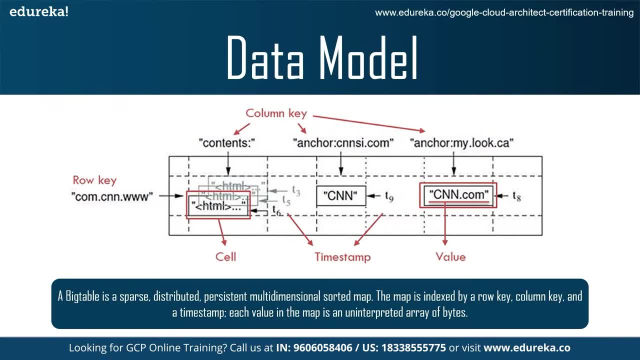 so that they could get good locality for their data accesses. Then the second key is for, like the column family, So column keys I mean. So column keys are grouped into set called column families, which form the basic unit of access control. All data stored in a column family is usually of the same type. 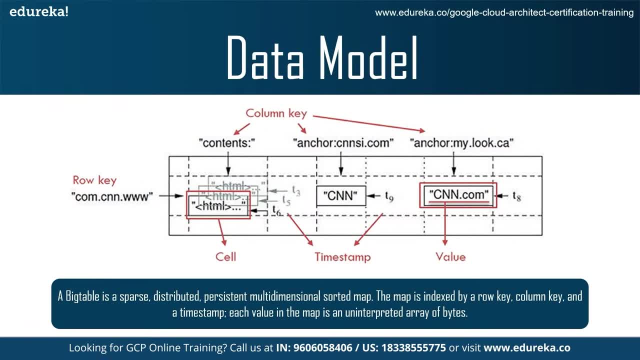 We compress data in the same column family together, So a column family must be created before data can be stored under any column key in the family. After a family has been created, any column key within the family can be used. It is our intent that the number of distinct column families in a table be small. 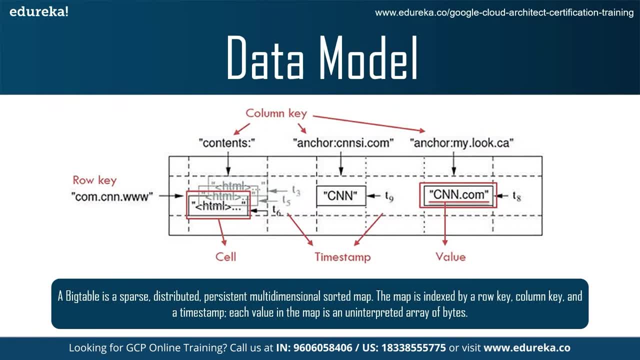 in the hundreds at most. okay, And that family is rarely changed during operation. In contrast, a table may have an unbounded number of columns. A column key's name under the syntax family is to qualifier, So column family names must be printable. 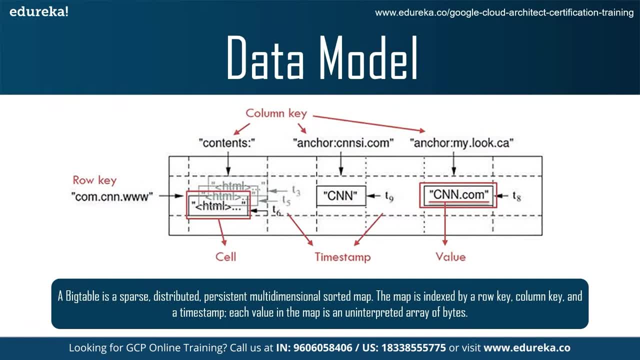 but qualifiers may be unbounded And they must be of arbitrary strings. An example for column family for the web table is language, which stores the language in which a web page was written. We use only one column key in the language family and it stores each web page's language ID. 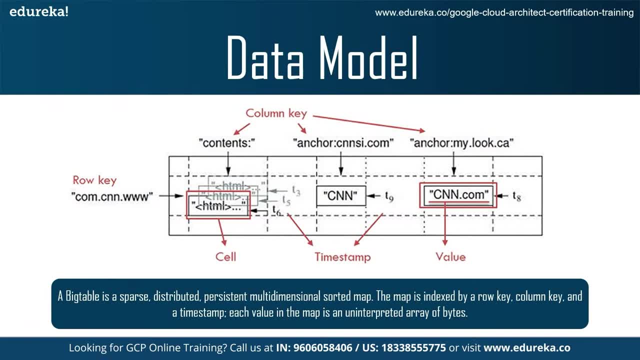 Another useful column family for this table is anchor. Each column key in this family represents a single anchor, as shown in figure. The qualifier is the name of the referring site. The same contents is the link, text, Access control and both disk and memory accounting. 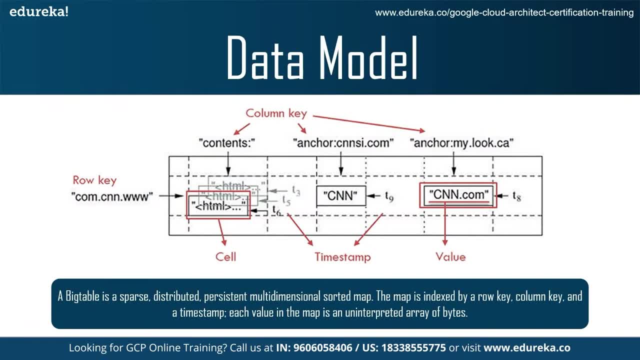 are performed at the column family level. In our web table example, we can see like their controls allow us to manage several different types of applications: some that add new base data, some that read the base data and create derived column families, and some that are only allowed to view existing data. 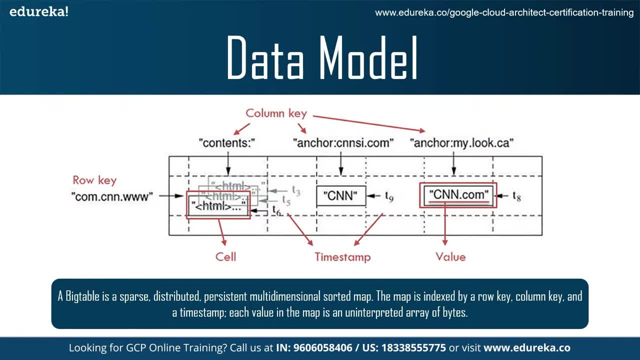 and possibly not even to view all of the existing families for privacy reasons. Now the third key is timestamps. Each cell in a table can contain multiple versions of the same data. These versions are indexed by timestamp. Big table timestamps are 64-bit integers. 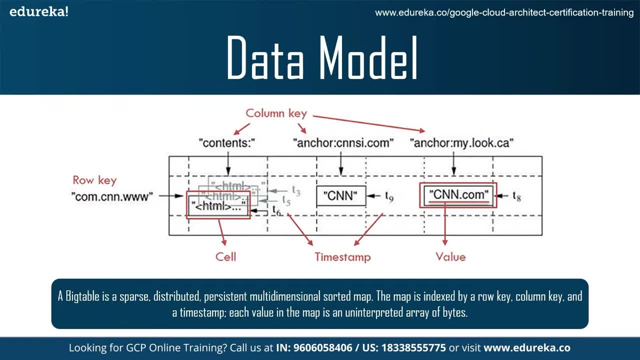 They can be assigned by big table, in which case they represent real time in microseconds, or be explicitly assigned by client applications. Applications that need to avoid collisions must generate unique timestamps themselves. Different versions of cell are stored in decreasing timestamp order so that the most recent versions can be read first. 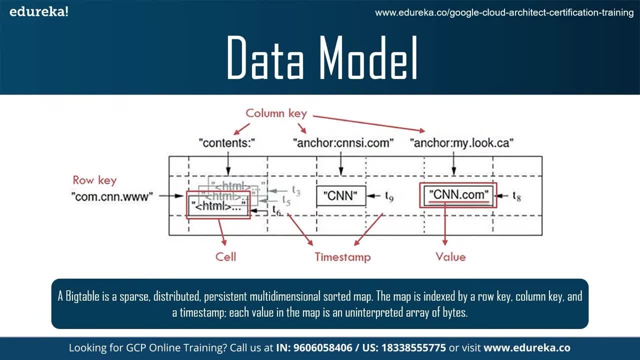 To make the management of version data less venerous, we support two per column family settings that tell big table to garbage. collect cell versions automatically. The client can specify either that only the last end versions of a cell be kept or that only new enough versions be kept. 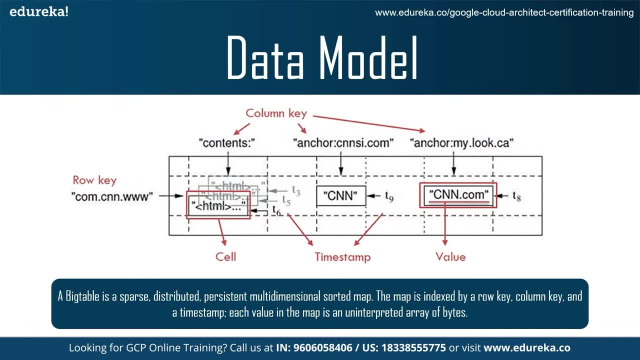 Example, only key values that were written in the last seven days. In our web table example, we set the timestamps of the crawl pages stored in the contents Column to the times at which these pages' versions were actually crawled. The garbage collection mechanism described above. 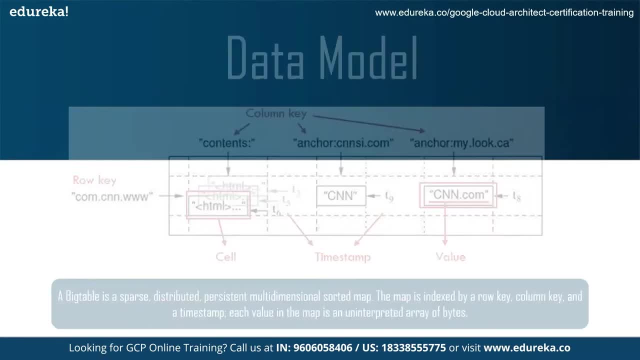 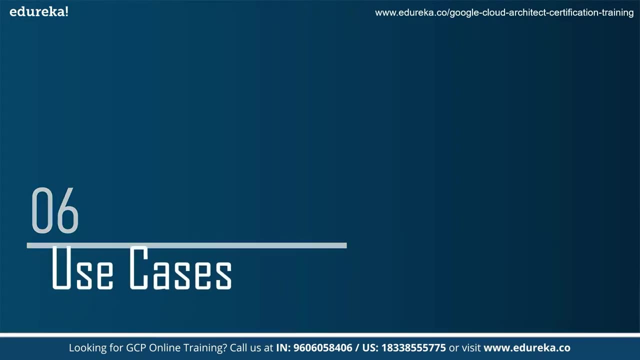 lets us keep only the most recent pages in three versions of every page. Now let's understand the use cases for Cloud Bigtable. You can use Google Cloud Bigtable to store and query all of the following types of data. The first is marketing data, such as purchase histories. 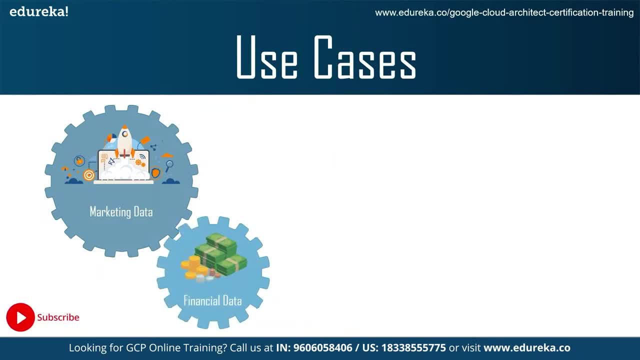 and customer preferences. Second is financial data, such as transaction histories, stock prices and currency exchange rates. Then Internet of Things data such as usage reports from energy meters and home appliances. Also the time series data, such as CPU and memory usage over time for multiple servers. 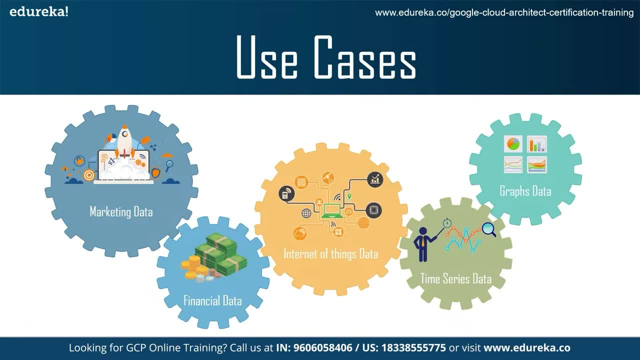 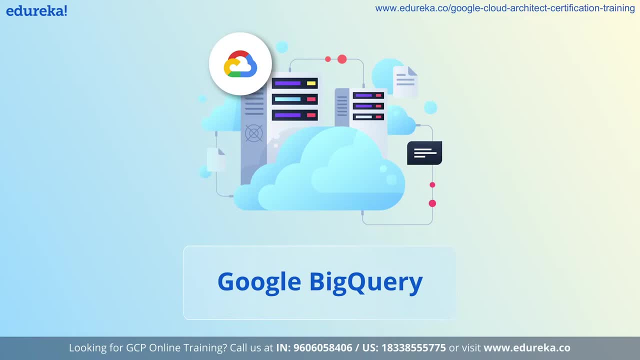 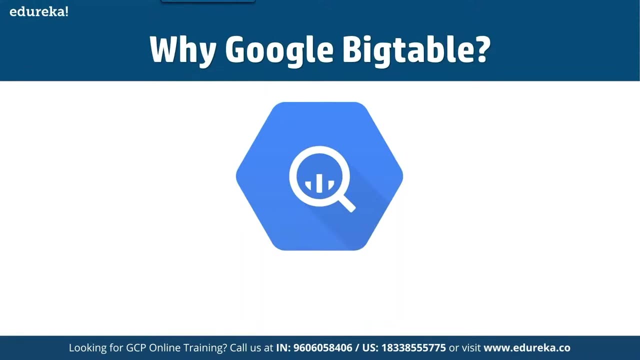 And last, like graph data, such as information about how users are connected to one another. Now, what is Google BigQuery? So basically, BigQuery. now we are talking about this guy. So basically, BigQuery is a fully managed, serverless data warehouse service. 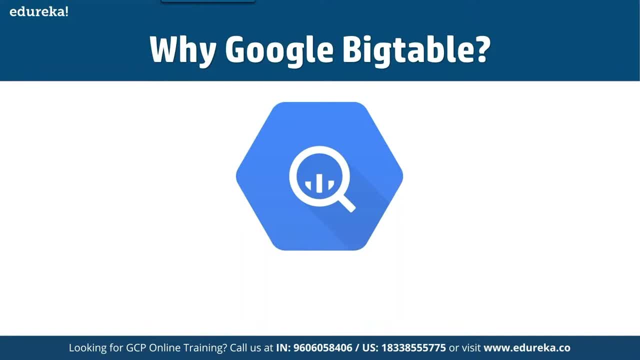 that enables scalable analysis over petabytes of data. So this is a pass which is platform as a service that supports querying using Ansys SQL, So you can, you know, store the data in a large storage and whatever you're going to consume. 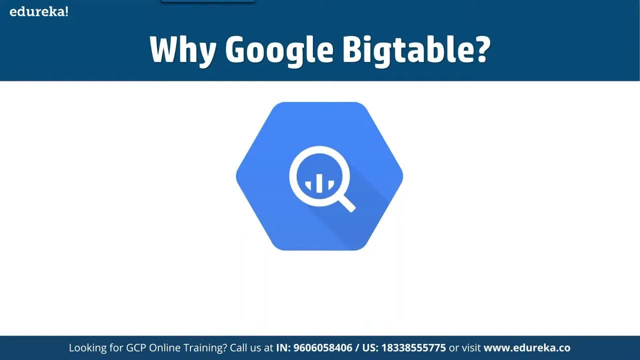 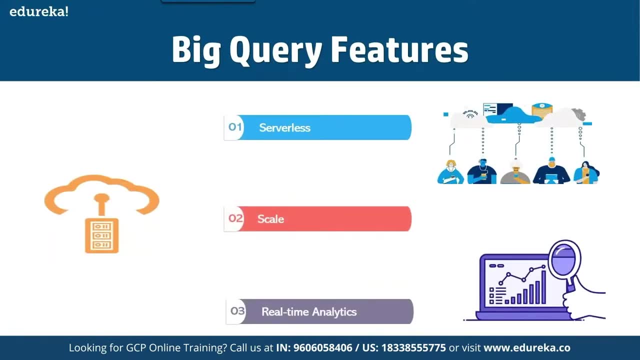 you're going to pay for it. Now, what are the different features of it? Now, coming to different features, it has various features, like: first is serverless. What serverless means? It means that, in order to run this, there is no dedicated server required. 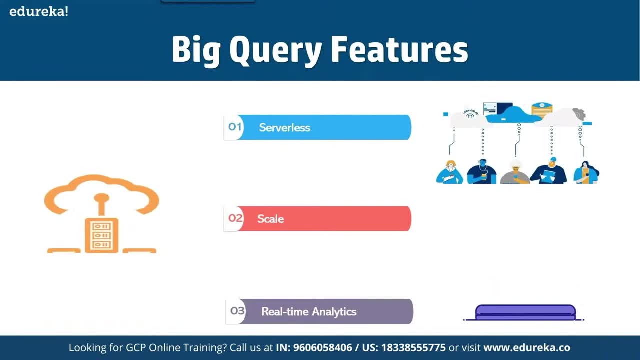 Now you know that if I had to basically run the resources, what I will need, I will need a resource, a virtual machine, basically that way that I will require to run those resources. right, So it's a serverless. You don't require the server without having the server. 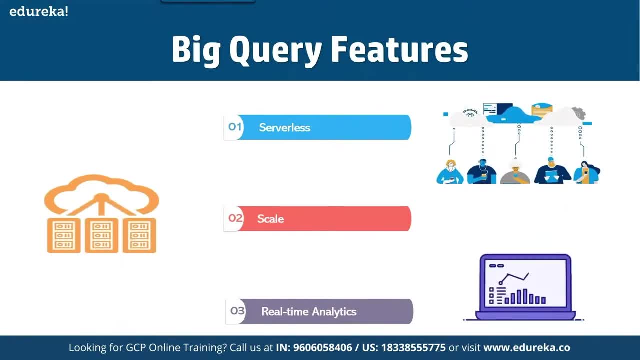 You basically can, you know, deploy your resources. You can access it, You can integrate with the application Plus, since you are not going to use a server, so having that overhead to manage the server, performing the patching, installing the updates. 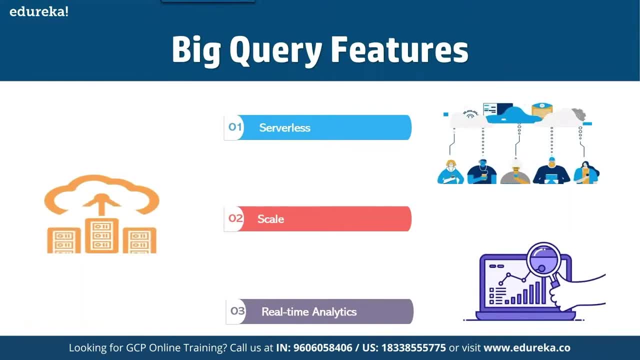 you know, even paying for that dedicated environment, you can just save the money on that. Second is scale. So it basically you can perform the scaling as well. You can basically perform automatic scaling At the same time. you know it basically supports petabyte of data. 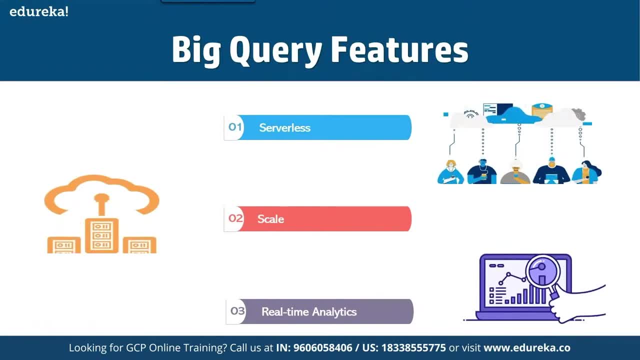 So if you want to basically scale with, let's say, you know, more CPU, more RAM, then you can do it very easily with this. In addition to that, in addition to scaling, let's say you want to increase the number of. 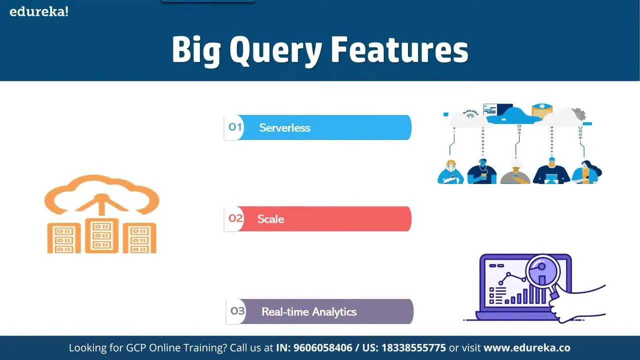 code processors as well. you can do If you want. you can write a script, You can write the criteria, For example, if your CPU utilization is going to go high at a certain, with a certain amount. So in that case, in such kind of scenario, 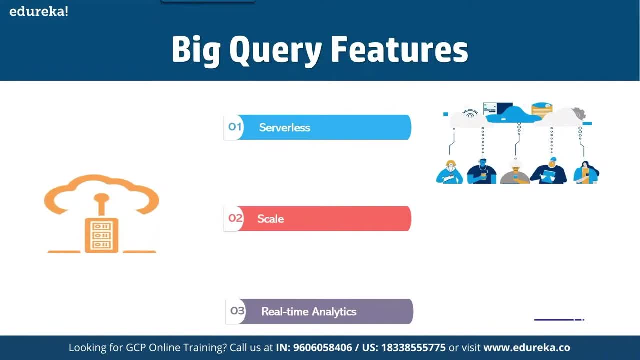 what you can do is it's going to automatically increase the resources. When the CPU utilization is going to go low, it's going to automatically decrease the resources. Next is real-time analytics, So wherein you can basically inject the data from video sources in this. 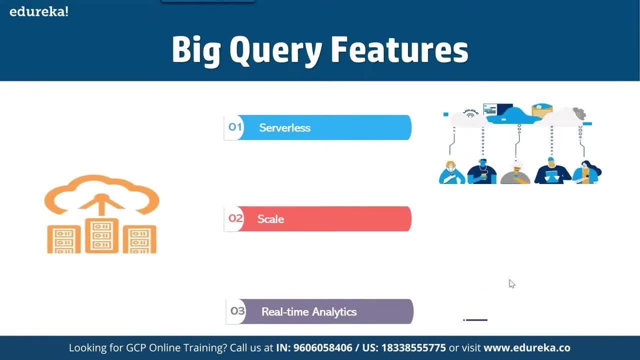 And, as you can see here, towards the right. you can see the progress, Like I want to see my company's going in profit, my company's going in loss, But each and every information is going to be available And you can get that information very, very easily. 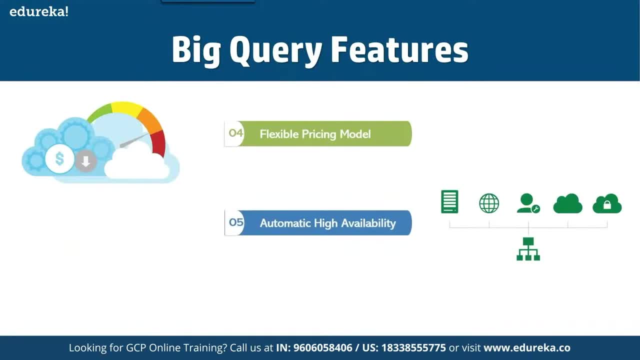 Now, next one is your flexible pricing model. So it basically provides you various type of pricing model that we are going to dive in more detail today. So it supports flexible pricing model where you can easily get the you know, I would say you can easily pick up the package. 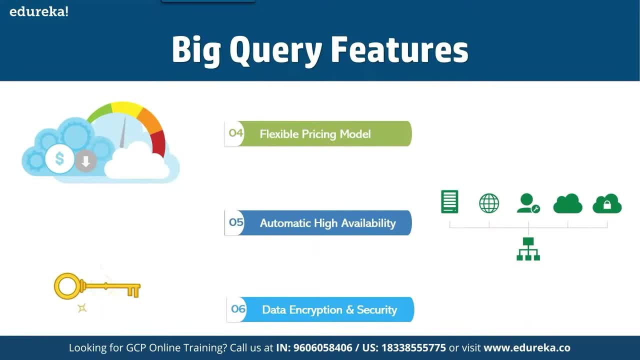 depending on your need, depending on your requirement. In addition to that, you have to also, you know, you can basically decide that I want to go with a monthly package, yearly package. I want to go with the services, the way the services I'm going to do. 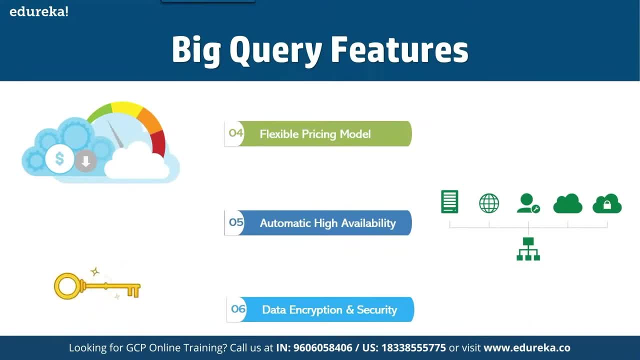 So that's something you'll be able to have. that entire, you know, flexibility with this. Plus, you have automatic high availability. So whenever you're going to create the resources- in this case, in the case of Google BigQuery- those resources basically are going to be you know. 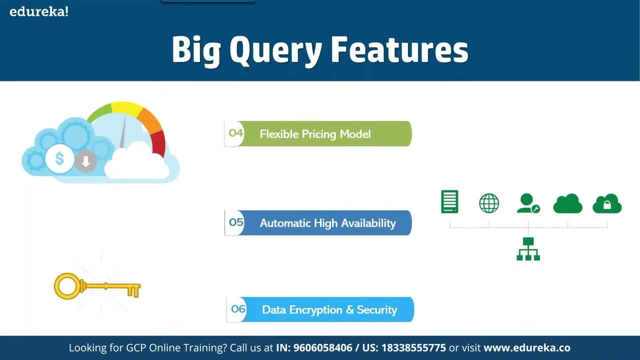 replicated at the different sites. Depending on the site model that you're going to use, those resources are going to be, you know, replicated automatically. at the same time, It also supports data encryption and security, So you know that nowadays, encryption is one of the biggest requirements. 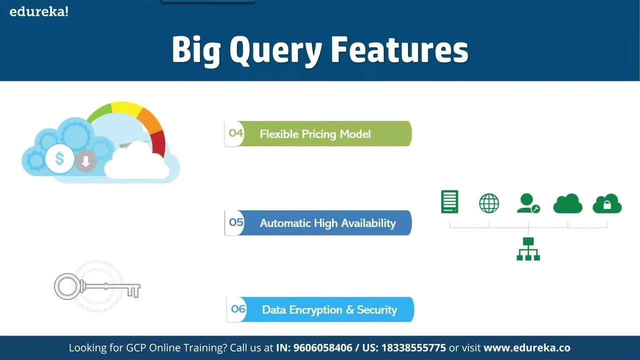 based on the ongoing hacks, So many companies were hit by the ransomware as well. So in the case of data encryption, what happens is your data is going to be encrypted automatically with the key, And that key you can store in a keyword. 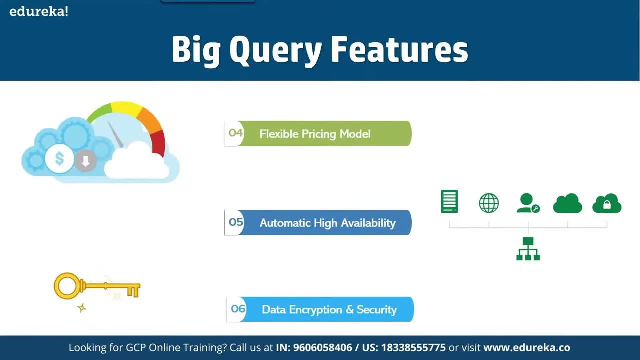 in an HSM, depending on the requirement that you have. So that also provides- And now, if I talk about the security, it basically supports. you know RBAC as well, which is role-based access, wherein you can basically define that. 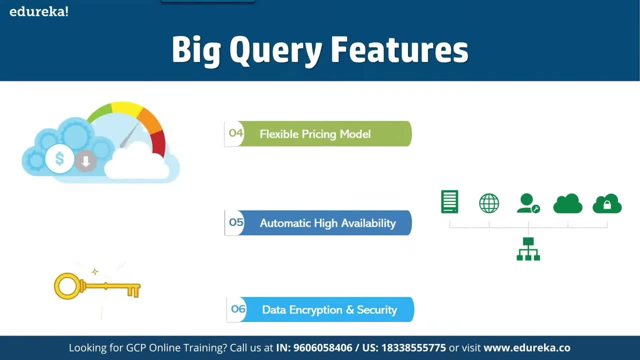 you know, like which user, what kind of role you want to assign. So all those things, basically, are available here as well, at the sake of this. Plus, there's no, you know, specific, complex implementation. Each and everything is designed in such a way. 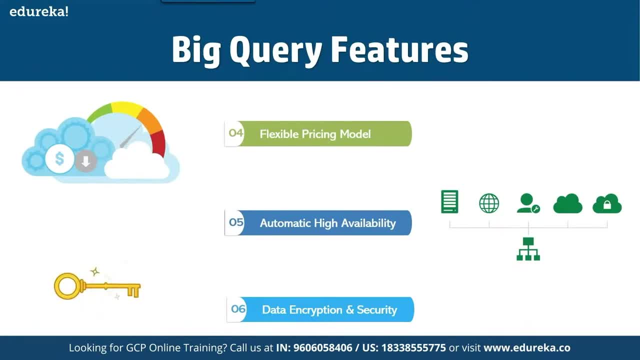 that you can get. you know easy interface with easy integrations as well. You can make a API call using different programming languages like Java, Python. different APIs are also available. You just have to change the. you know some variables over there. 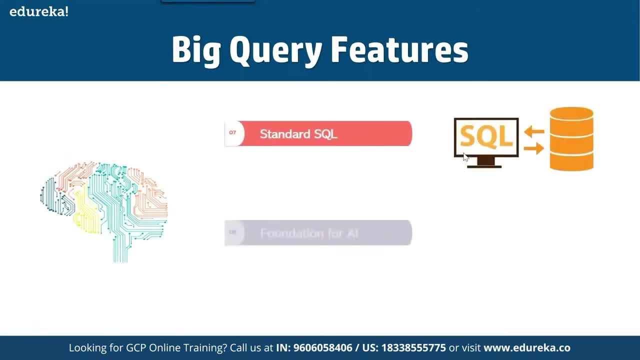 and you will be able to use it directly. Next one is standard SQL, So it automatically have inbuilt standard SQL. at the same time, You can also, you know, define your own database by, you know, creating a new resource in that you can also create your own database as well. 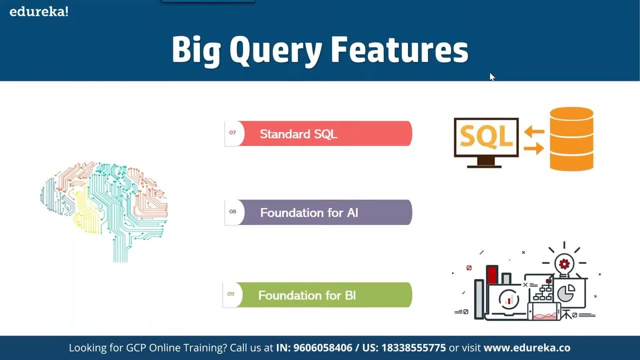 Next is foundation of AI, which is artificial intelligence. You can integrate with- you know artificial intelligence as well- And you can also integrate with DIA as well, which is business intelligence. Yeah, Now, moving on, let's talk about the BigQuery storage. 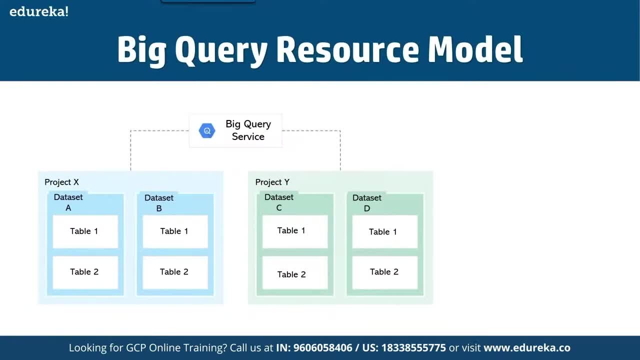 So in the case of BigQuery source model, it basically have five major components: the projects, the dataset, your tables, your views and the jobs. Now here, in this case, let me just use this highlighter. You know this is a project. 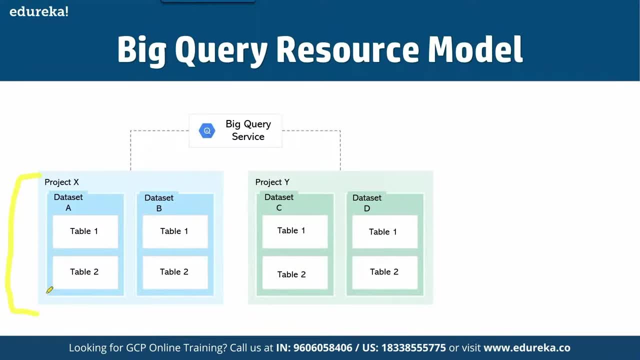 basically one project is found. In that project basically you have a dataset. In that dataset you can basically have, you know, tables. So now in those tables you basically can have different views and you can basically, you know, have different jobs for it. 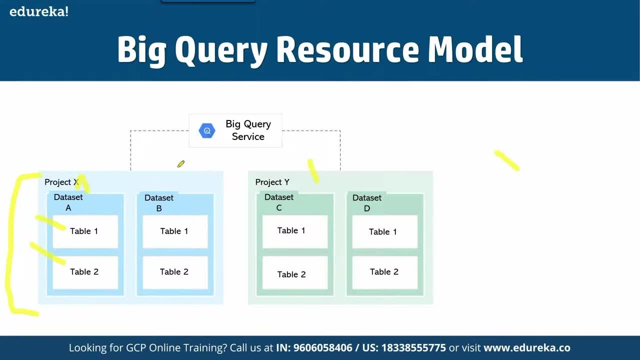 Now, this is a different project. Now, likewise, you can have different different projects here which can be integrated directly with your BQS, which is BigQuery service, wherein you can easily- you know- query the data. For example, 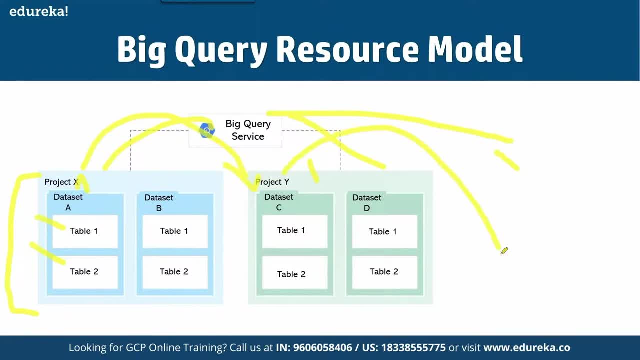 this project needs some data with you know this project, or this project needs data with this project, or some different project needs data with this project. So this entire management, that role-based access control, can be easily be done with your BigQuery service. 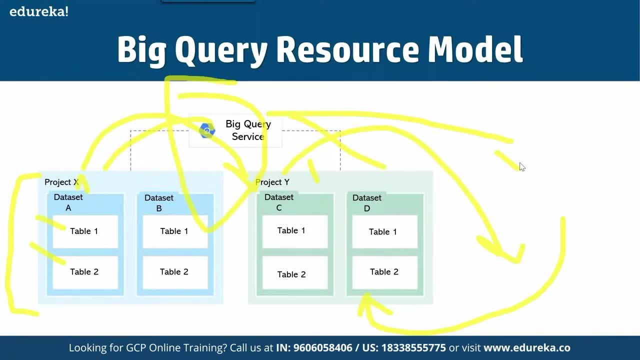 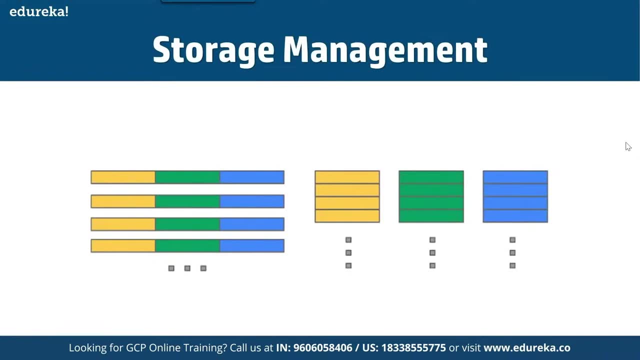 So that's again. you know a little bit over here at a higher level. Now, coming to the storage management that we have, let's take a look how storage management looks like of BigQuery and how it is different from others. 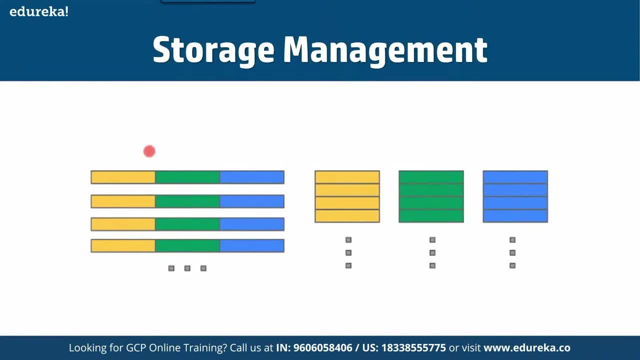 So this is towards the left that you can see. this is traditional RDA BMS storage where you are going to have record-oriented storage Like this is the one record, second record, third record, likewise On the right side. 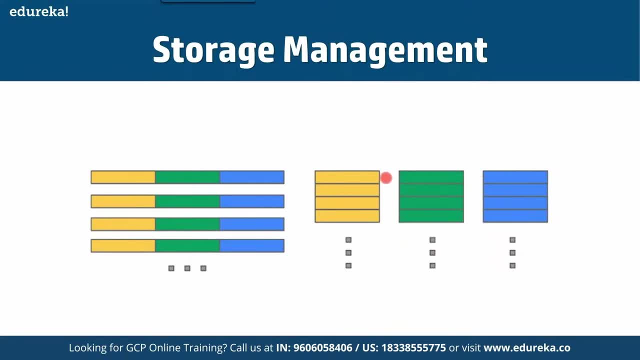 you see, this is BigQuery storage. So here it uses the column-level storage. Now, even if I want to perform encryption, I can perform encryption in one column. Maybe I have a data, let's say, you know, in one column. 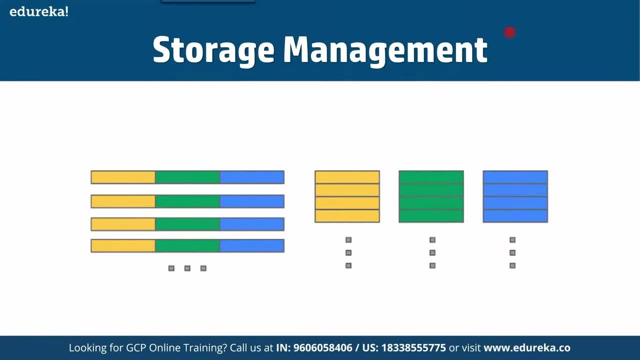 I have name. Second column: I have their- you know last name. Third column: I have their credit card number. Now, this blue one is sensitive for me, But if I go with the traditional RDA BMS storage, I have to basically encrypt the entire row. 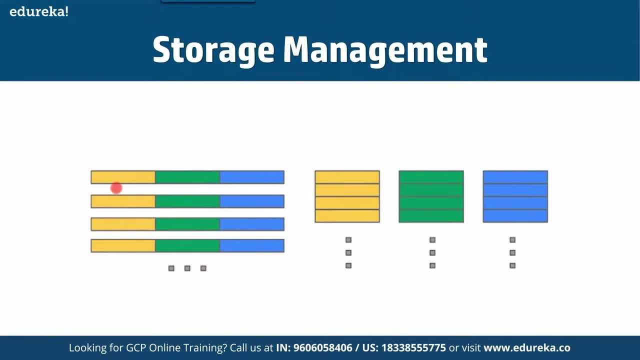 You know it's going to be difficult for me And, at the same time, encryption- decryption will take time. The operations execution will take time, So execution will take time, which is going to be difficult. Now towards the right. 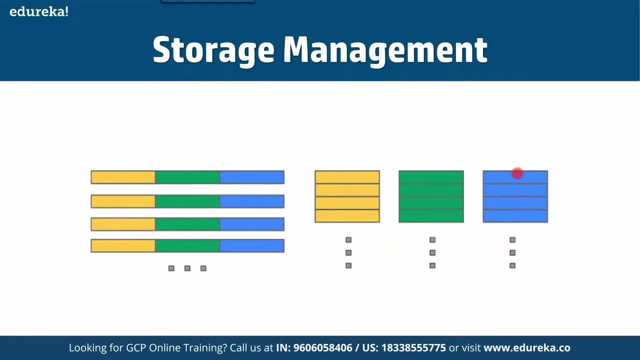 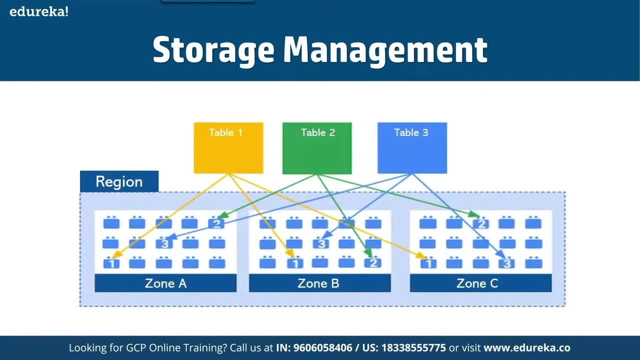 if you talk about, you know, BigQuery storage. we are going to have the column-level storage, where we are going to encrypt one column at the time, Clear Now coming to the other one, which is storage management Now. 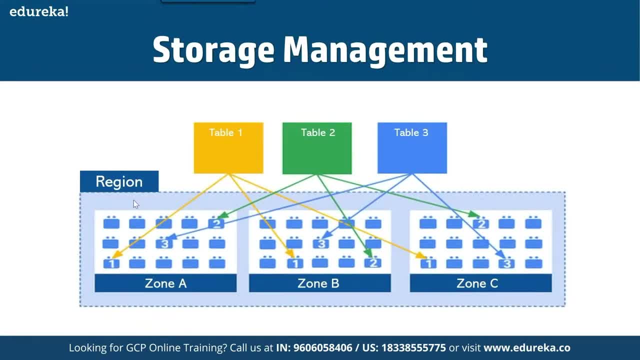 here. in this case, as you can see, like we have this table one, table two, table three In one region, we can have different zone, Different zones, basically like your different data center, Maybe in India? I have this data center in Bangalore. 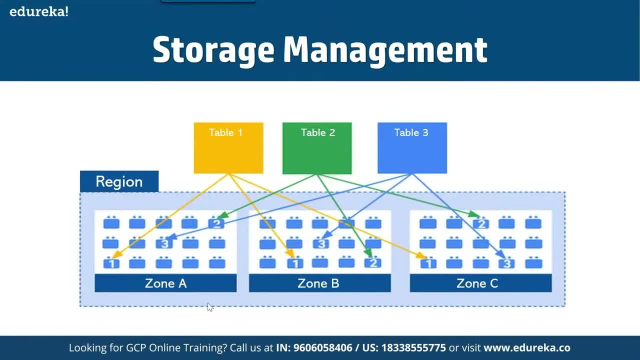 Second is Hyderabad, Third is Delhi. So if one zone is down, my data is still going to be there, at the second, at the third, Now here in this case, if you see, this second one is available here as well. 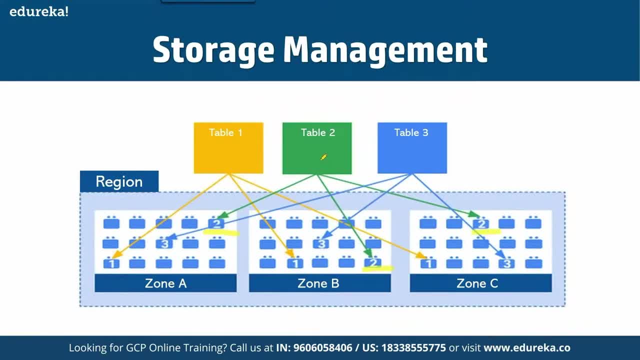 It's available here as well. It's available here as well. So the same data from table two is pointing out to this. The same data is copied at the second zone. Same data is also copied at the third zone, So even. 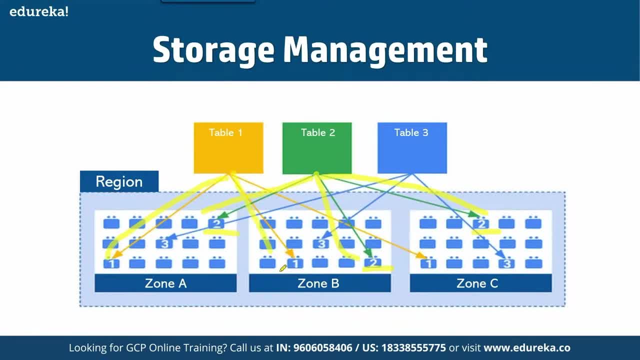 and similar in this table one. this is copied in the first, This is copied here in the second, This is copied here in the third. So we have this one, this one and this one Now in the third table. 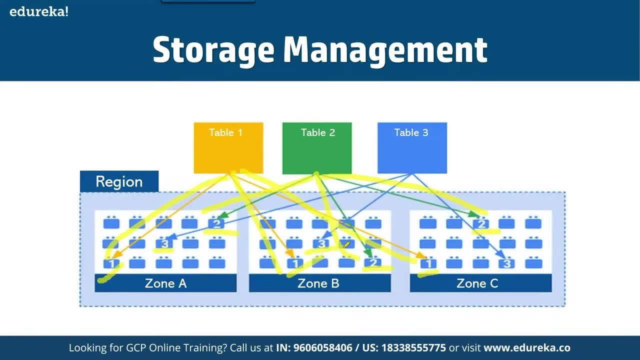 the same data you can see is copied here as well. It's copied here as well. It's copied here as well. Now, this one zone is going to go down. This is going to remain up. This is going to remain up. 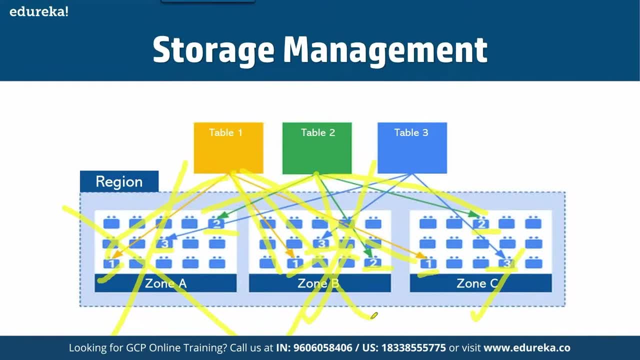 Let's say, this one also got down. There was a network issue, So in that case, the third zone will remain up. Now you can have multi-regions as well, wherein the data from one region is going to be copied to the other region as well. 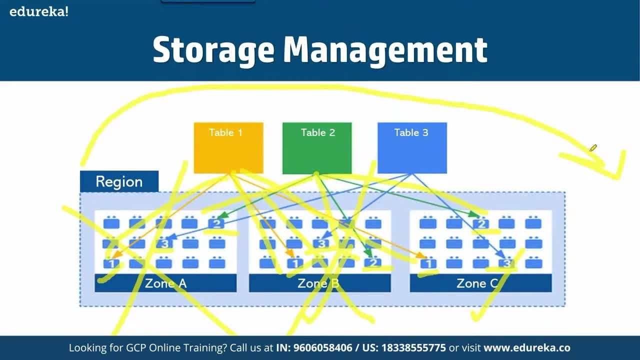 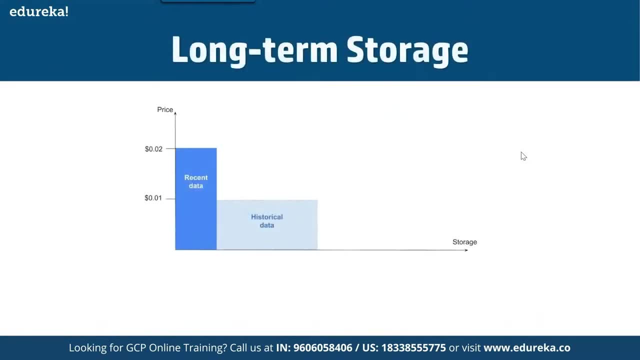 so that's why it basically provides you a very good resiliency and the data is going to be replicated automatically with the other data at the sake of ease. now coming to lts, which is long-term storage, so if you have a table or partition which is not modified for 90 consecutive 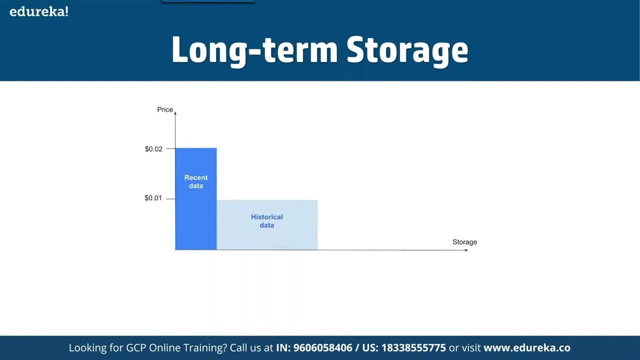 days, it is considered as long-term storage and for pricing for the storage for that table automatically gets dropped by 50 percent to the same cost as cloud storage in airline. so basically, discount is going to be applied on per table, per partition basis. that's the biggest beauty of it. 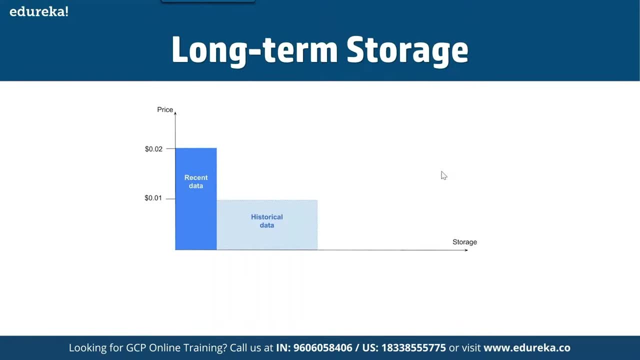 so if you are not using it, there is no need, there is no requirement that you have to, you know, change the storage type, it's automatically going to drop the you know price by 50 percent at the same cost. that's the biggest beauty of you know, the google cloud. if i were to say so that you're not spending, 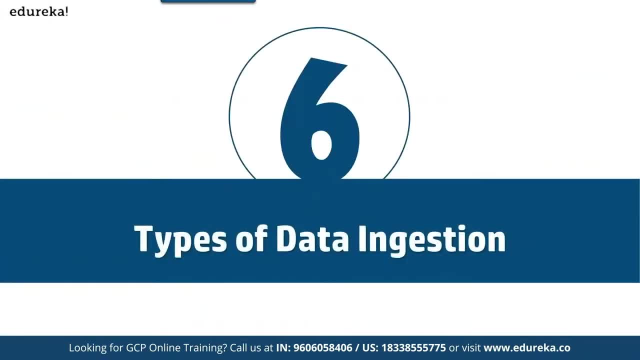 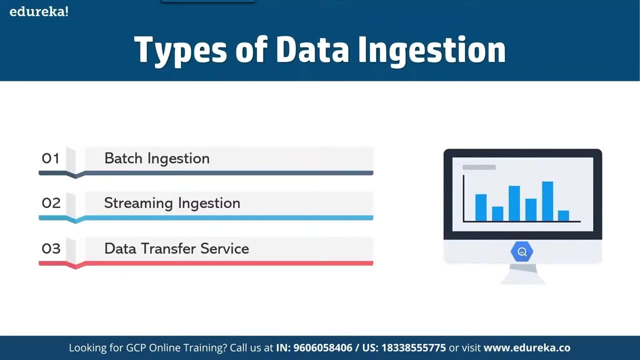 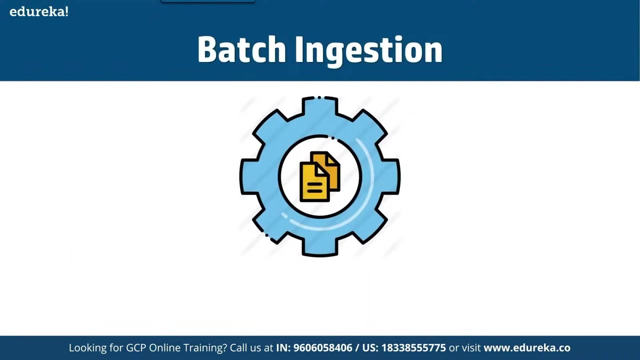 a lot of money on that. moving on, what are different types of data ingestion that we have? so we basically have a batch ingestion, we basically have streamlined, we basically have data transfer. now let's talk about. you know each of them one by one. what is the batch ingestion? so, batch ingestion basically. 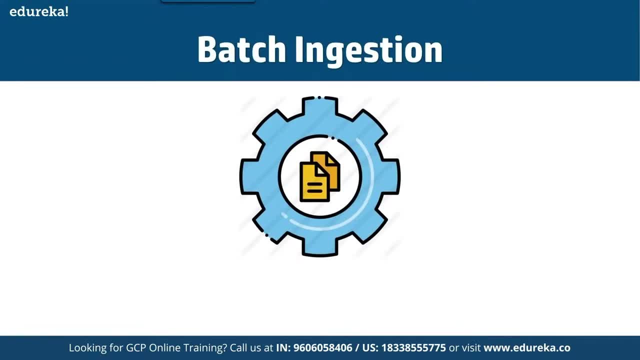 you know involves loading pages, you know, basically having data set that does not have to be processed in the real time, so they are typically ingested at a specific regular frequencies and all the data which is going to be processed in the real time is going to be processed in the real time. 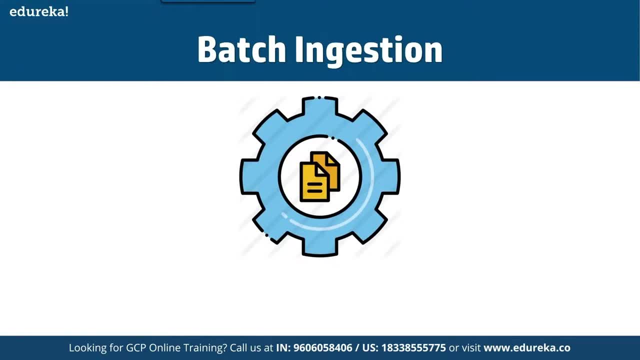 to arrive. it's going to arrive at one time or it's not going to arrive at all. so the ingested data is then queried for creating reports or combining with different sources, where it can have data from maybe different cloud providers. it can have data from your, you know, on-premise platform. it's 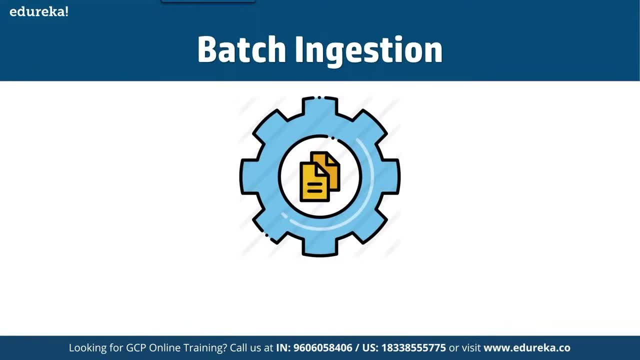 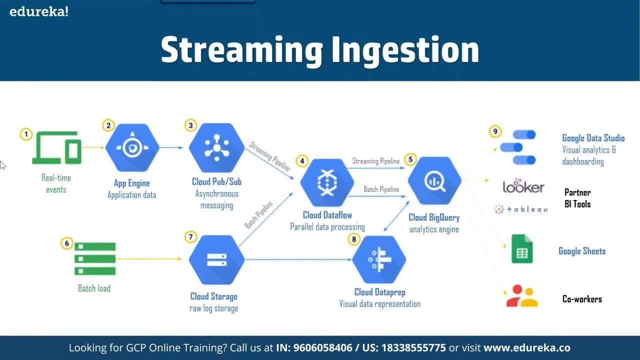 going to be appeared together and at the same time, it's going to be processed together. in the case of streaming ingestion, it's a bit different. in the case of streaming ingestion, or you can see in this diagram- um, you know, you are going to have your real-time events. maybe i have a streaming ingestion. 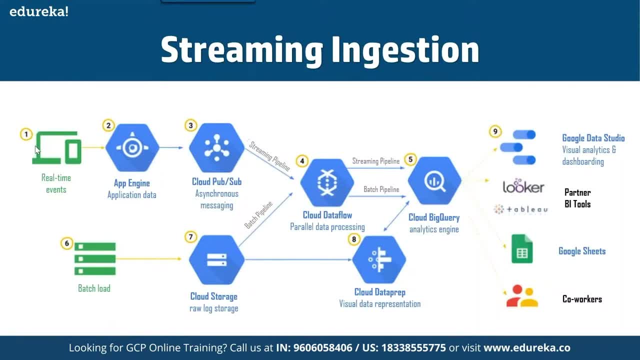 maybe i have a service running, so it's, uh, it's going to generate real-time events. you are going to have, basically the app engine which is going to be integrated with your applications can be on, for mines can be on. a google cloud can be on, uh, you know, any other third-party cloud as well. 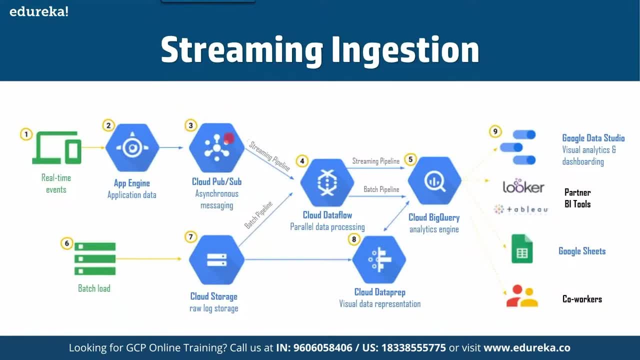 and uh, these events are going to be, you know, fed together into your uh messaging service. so any cloud model you talk about- for example, your uh, you know azure, you have your google or other- they provide the messaging services. so different type of messaging services they are providing. 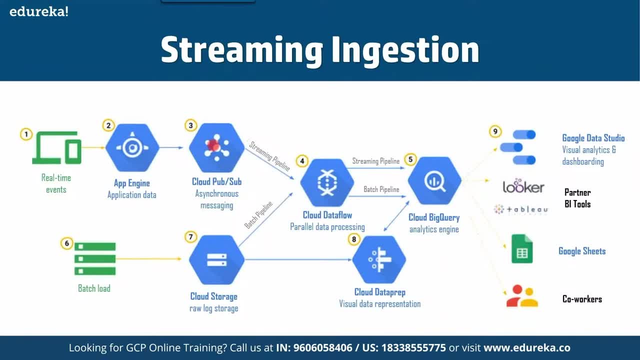 with the help of which you can have the request response protocol set up, based on which, uh, you can also set the acknowledgement. like the way tcp works: you send a request, wait for a response. if there is no response, you send another- uh, you know- same request again, because it will consider that your 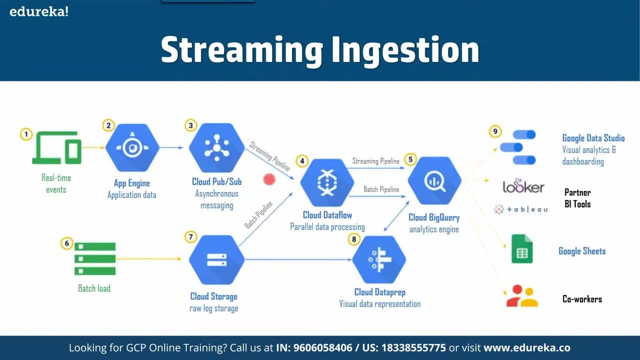 request has been dropped. so, with the help of stream pipeline, the request that you have received is going to be, uh, going to the, you know like like a queue, where you can have multiple pipelines all together because it supports parallel communication, and next, when you have a batch pipeline, wherein 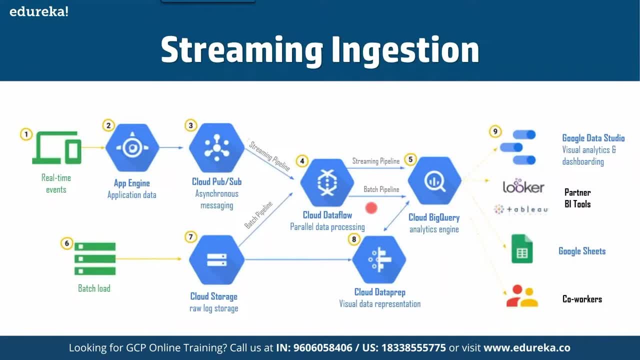 uh, you can basically create the batch of cds batches. you can basically create the batch of cds, batches of requests, which is going to be, you know, accumulated in the queue together and at the end it's going to process together. then after that, uh, you know, you are going to have again. this is a. 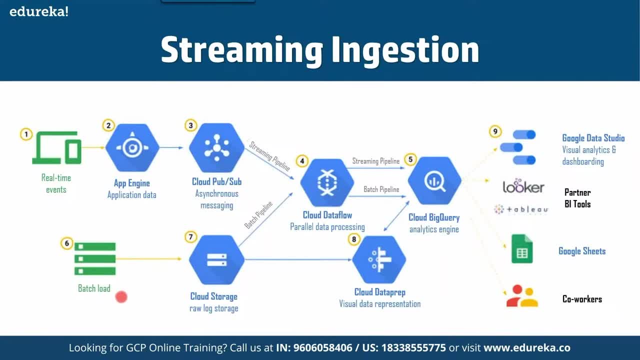 batch processing data which is coming from. you can have a batch load where the requests are accumulated and, uh, you know, at a specific storage it gets a certain use cases, like your services are running maybe 2 pm every day, 3 pm every day, so it's going to, uh, you know, ingest all the services. 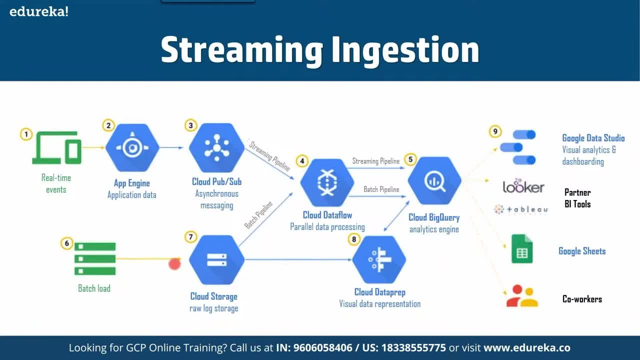 from different sources to your environment at the same time, which is going to be processed by the cloud data flow and it's going to process together. again, this is a very big topic, guys. uh, all three times. uh, we basically have a detail, even this in streaming and ingestion. we basically spend almost an hour on this. however, uh, based on the time constraint, that 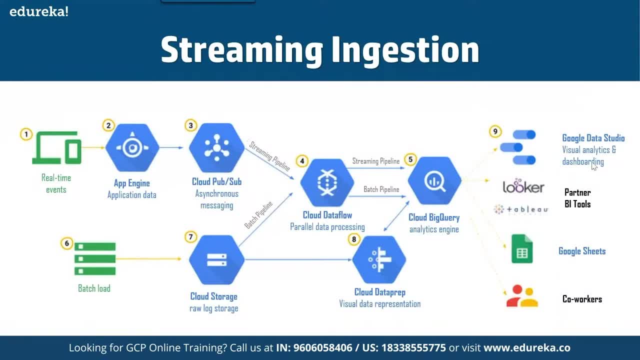 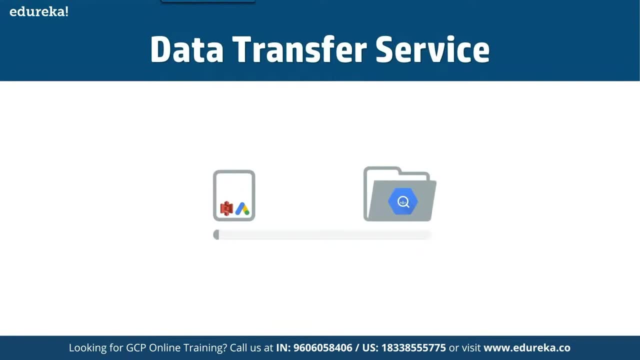 we have. that's why we're just talking about a bit overview of it. otherwise, in general, this is a very big topic that we cover in detail now. the third service that we have is dts, which is known as data transfer service. so your- uh, you know- big query. data transfer service is basically a. 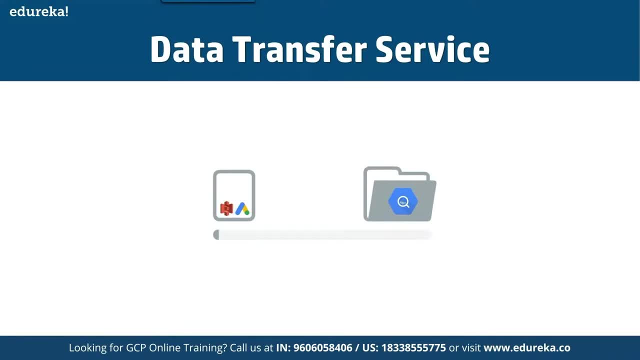 fully managed service to ingest data from your data transfer service so you can transfer the data from your data warehouse technologies like your google uh saas application. saas is software service applications like your google ad, your external cloud storage provider like amazon, you know, and different, different providers we have. 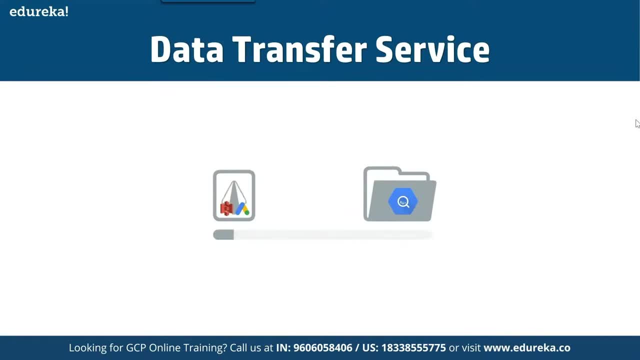 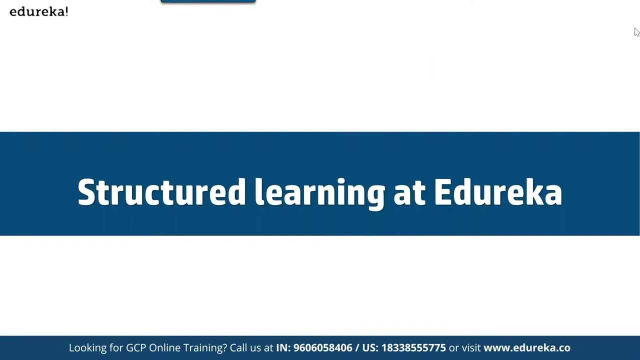 and you can transfer the data from data warehouse technologies like your tera data, your amazon red shift. so all this thing basically falls into this category, which is data transfer service here and out in this. now, um, coming on to the structured learning editor, you want to enroll for the course and you want to know what all the topics are. like you said, we 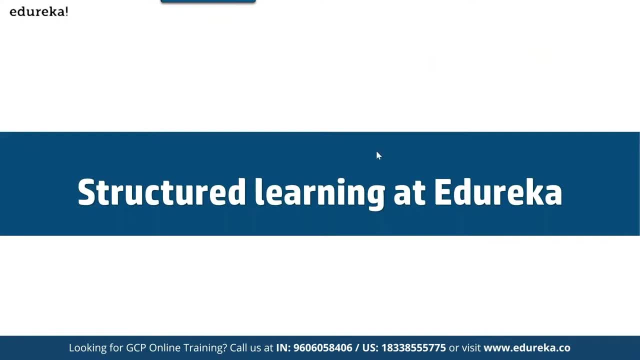 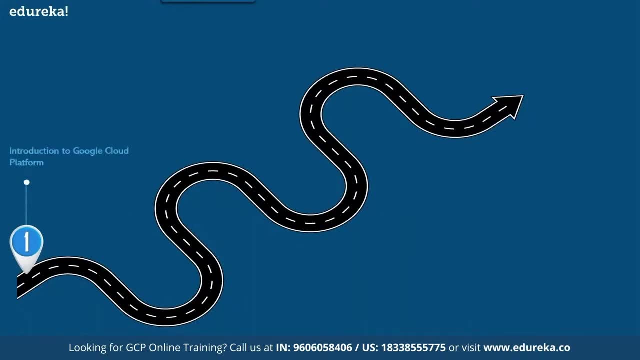 bring the transparency. so all this kind of topics, every information is available on our website. so let me just share the curve path, the learning path, how it's going to be there. so if you're going to enroll for the course, this is going to be the learning path in the first class you learn about. 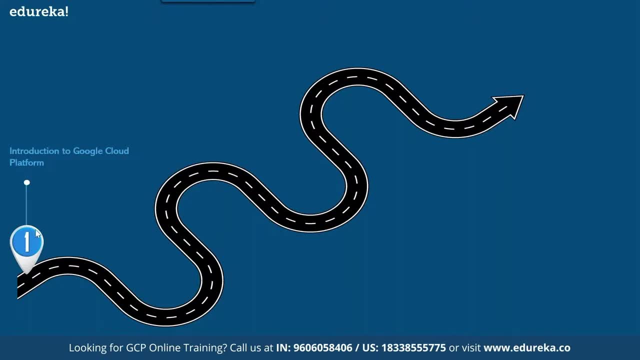 google cloud platform, how you can create your account, how you can set up the labs, its components, sub components, with the hands-on on different topics. then after that, in the second class, we will learn about how you can basically manage your google cloud platform, its services, its component and sub components, with the perspective hands-on. then in the third, 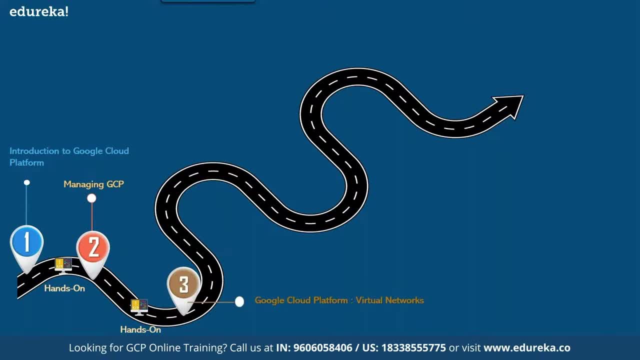 class you will learn about google cloud platform, virtual networks- uh, what are different type of networks that you can create with the perspective, and so on. then, in the fourth class, you will learn about security and identity fundamentals. um, you know how basically you can create different, different type of access you can. how basically you can control the entire access with you. how? 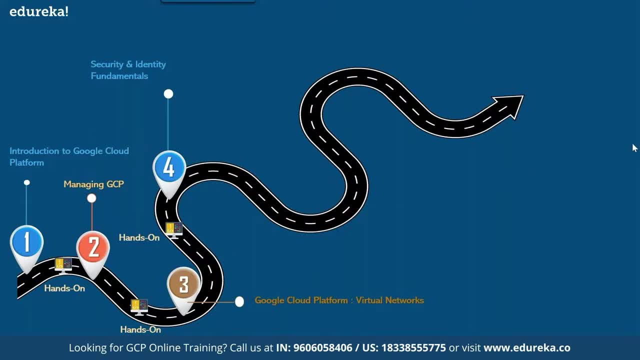 basically, you can give different permissions, how, what are the different roles that you can create? at the same time, you can also or define your own- uh, you know- structure like: uh, how many roles you want, how many users you want, because i don't want more than 15 users to access a resource. so all. 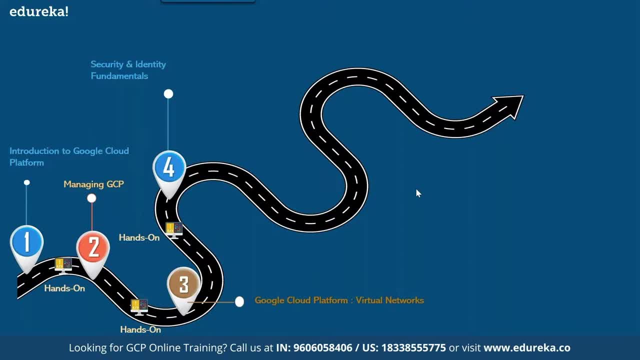 these kind of things can be restricted uh here that we are going to learn, uh with practicals, hands-on. then after that you will learn about compute services, different type of storage that you have, different type of, um, you know, services, uh that you can leverage, including the case of cloud. 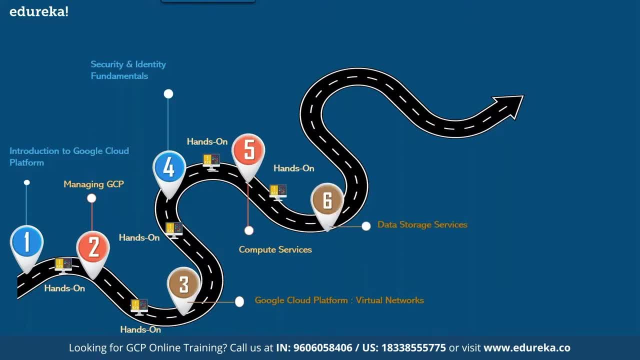 and the hands-on. in the sixth class you will learn about data storage services. what are different? database that it supports, the different ways of storing it, what are the proprietary of? you know google? google has provided you know various type of different storage services which are their own proprietary. what are they? what is the difference between them? 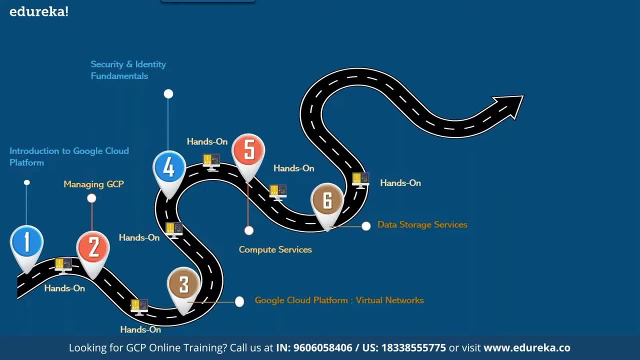 how you can select which storage service is based depending on the use case. with the practical hands-on, then in the next class you will learn about architecting with google kubernetes, engine docker. what is how you can integrate kubernetes? uh, you know how basically kubernetes look like. 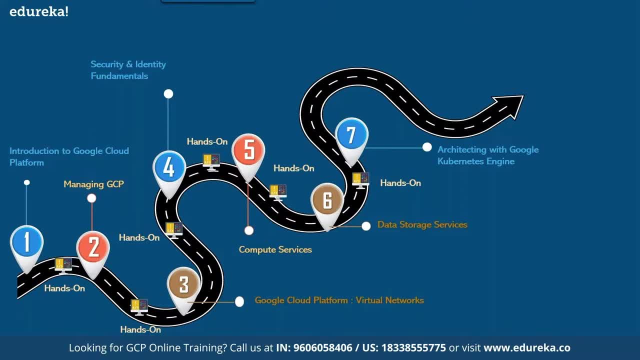 in gcp, how it is different from normal kubernetes. uh, how you can integrate with docker. each and everything you're going to learn in detail with the practical hands-on after that we are going to learn about in the eighth class. you'll learn about application development, if you. 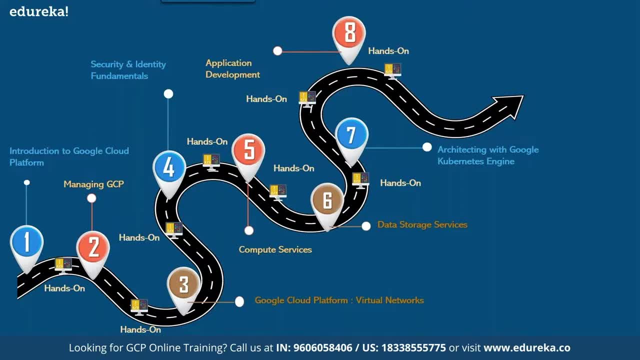 want to write the code, you want to develop the application. you know how you can do it. it's components of components. with the practical hands-on. then you will learn about data and ai services with the practical hands-on and then, in the last class, you will learn how you 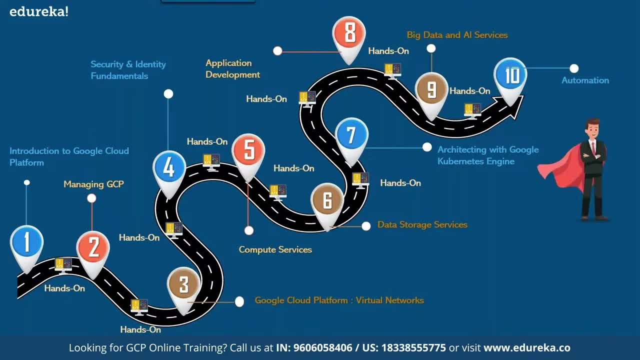 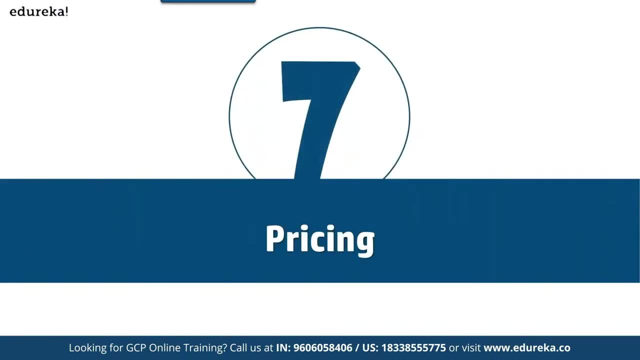 can perform automation on the components with the practical hands-on. so this is the entire career path, i would say the training path for your certification if you're applying to take. now, coming to the pricing if we talk about, we basically have a two pricing model in the case of 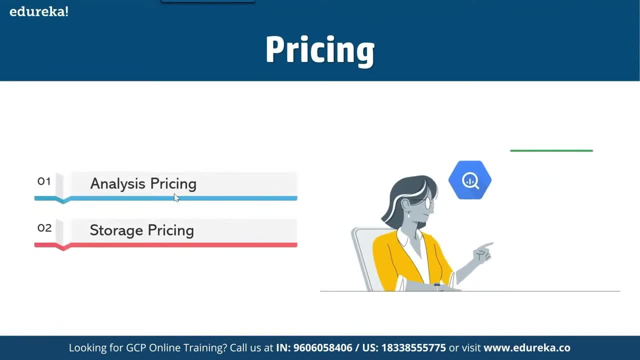 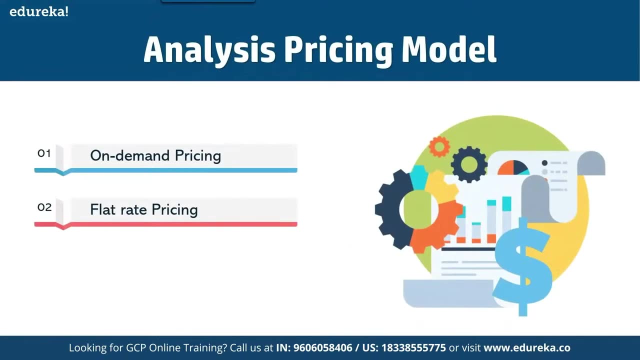 you know google that it provides. one is analysis pricing. second is storage pricing. now, if we talk pricing, this is basically on-demand pricing. uh, basically it has flat rates pricing. in this we have three model. first is: you are going to have the annual model. you are going to be basically. 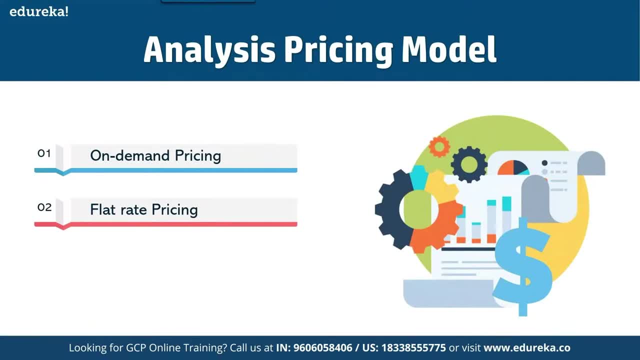 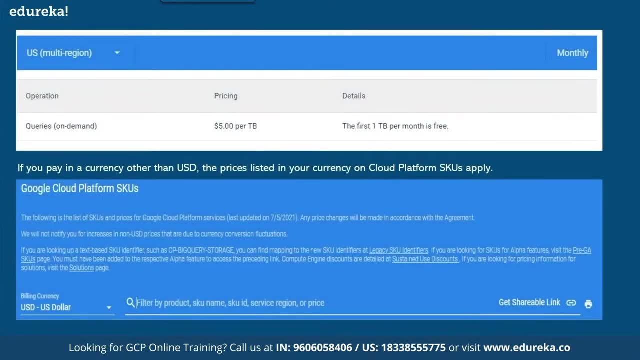 billed and paid annually. second is on a monthly basis. third is basically the flexible store slots that you can choose. so this is again one of the example of the pricing model, the way it looks like. for example, queries on demand, you have to pay five dollars per tb. so first tb is going to be free. 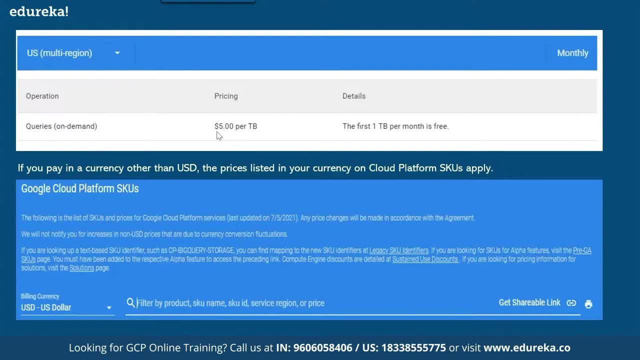 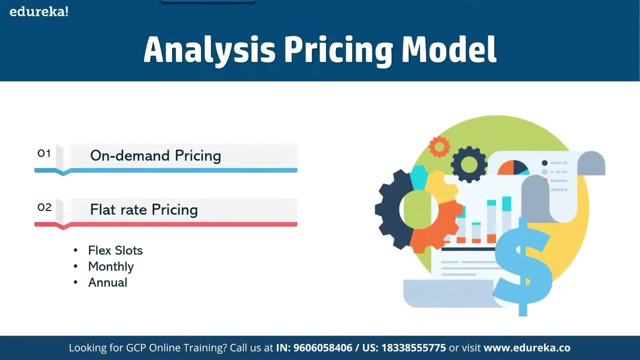 uh, but after that you have to pay five dollars every tb, which is a- you know a good deal as compared to other cloud vendor providers. again, the same thing that i shared a moment ago: a different pricing model that it supports. now, if we talk about the cost of a flexible slot commitment, like i said, we have three times the. 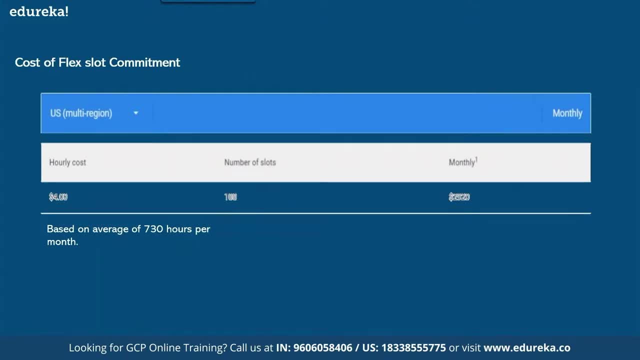 flexible monthly and the annual. so if you, if you basically take a look at flexible slot, you know you're going to get uh, this much slots and uh, you know, basically average of this is 7- 30 hours per month, depending on your requirement. you can decide if you're using heavily. 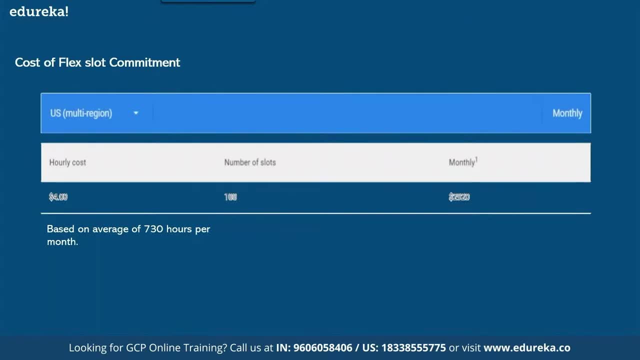 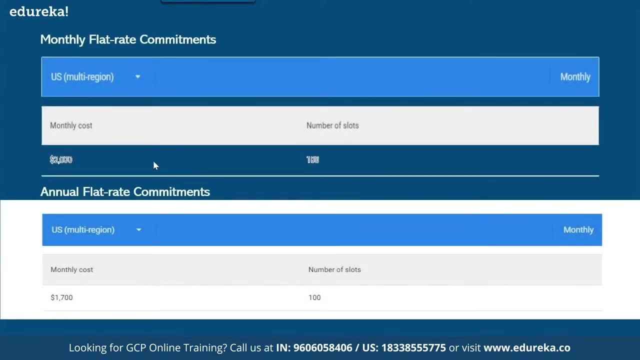 uh, you want to go with the flexible, or your monthly is going to be best or annually is going to be best. likewise, if we talk about, you know, monthly. in the case of monthly, number of slots that you get is 100. you have to pay two thousand dollars for that. in the case of annually, the amount 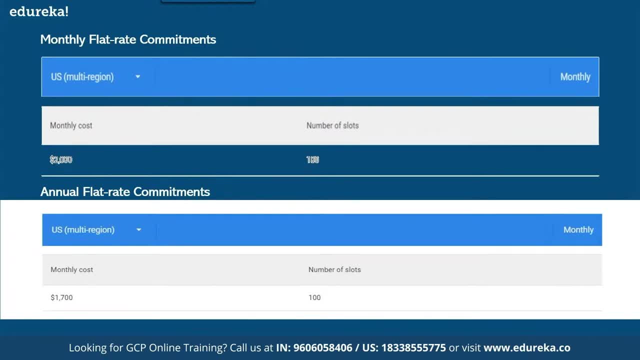 is less, so where you're going to pay less, which is seventeen hundred dollars now, if you look at the cost in the case of flexi, it's uh, you know a bit more now. you basically look at the cost of your- uh, monthly it's high. annually is less, so you can save the money on that now in the terms of so. 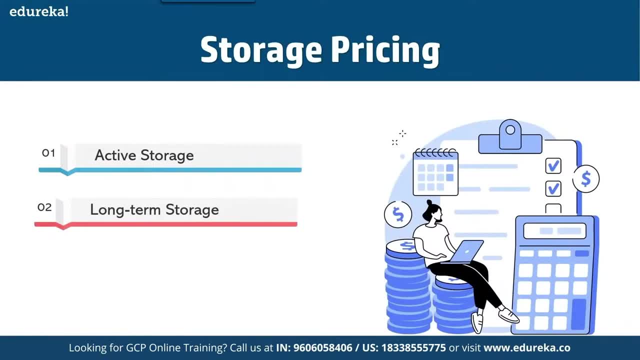 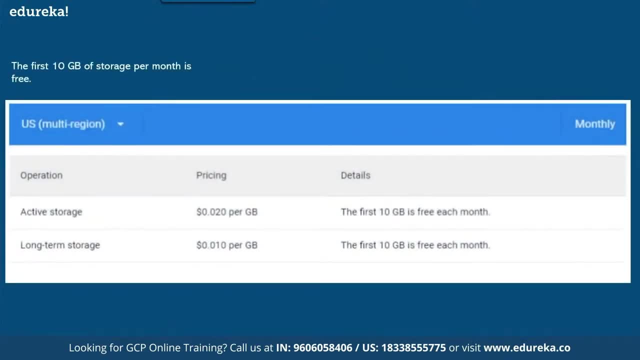 if you talk about, it has two types of storage pricing. one is active storage. second is lts, which is long-term storage. so you have seen that in the case of long-term storage, what will happen? that we even talked about a moment ago, which is, which has a benefit, that, if your 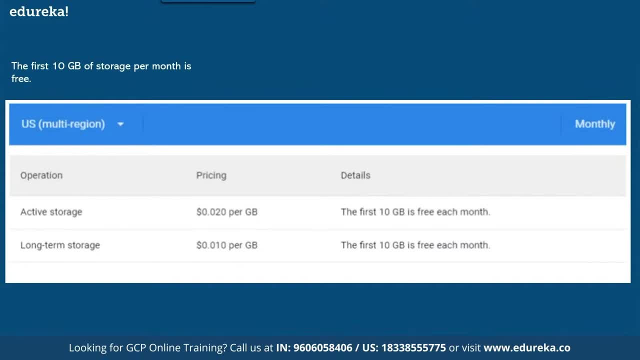 table or partition is not modified for 90 consecutive days, that is going to be considered as a long-term storage and price of that storage is going to be automatically dropped by 50 percent. that's why, in this case, you see, for active storage- uh, it's uh- the cost is 0.02. 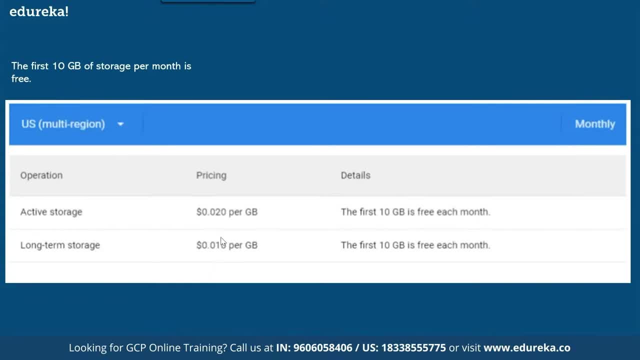 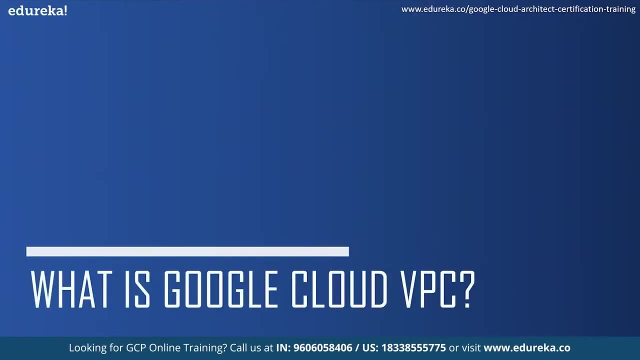 dollars 0.02 and for long term is 0.01, which is half, because the price get taught by 50 and in both the cases the first 10 gb are free. what is google cloud's virtual private cloud? google cloud virtual private cloud provides network functionalities to compute engine. 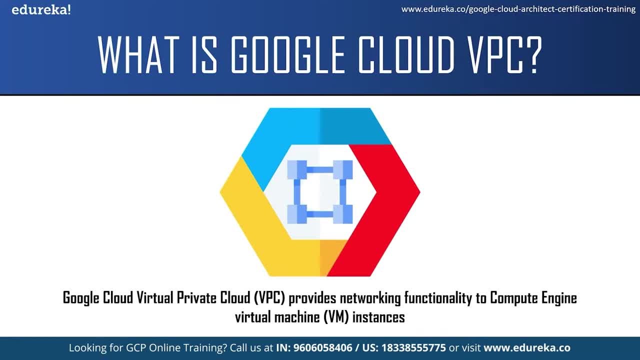 virtual machine instances such as google kubernetes, engine containers, app engine, flexible environment and other good capabilities, such as the cloud cloud virtual machine option and the cloud cloud. virtual private cloud provides network functionalities to compute engine virtual Google Cloud products which are built on compute engine virtual machines, basically VPC. provides 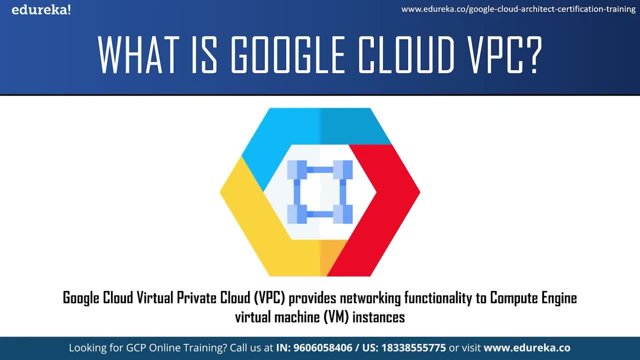 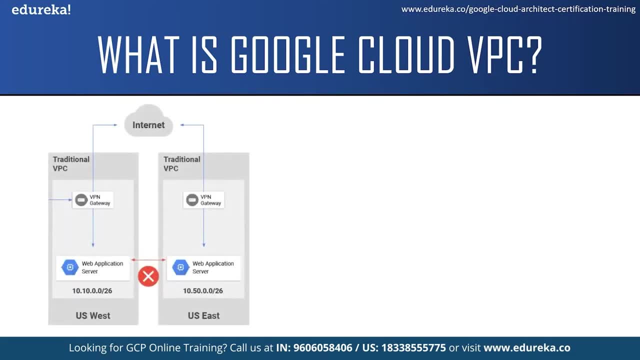 networking for your cluster-based services that is global, scalable and flexible. Now, Google VPC is quite different from the VPC of other cloud service providers. Now, in the traditional VPC, or the VPC provided by other cloud service providers like AWS, the architecture would look something like this: 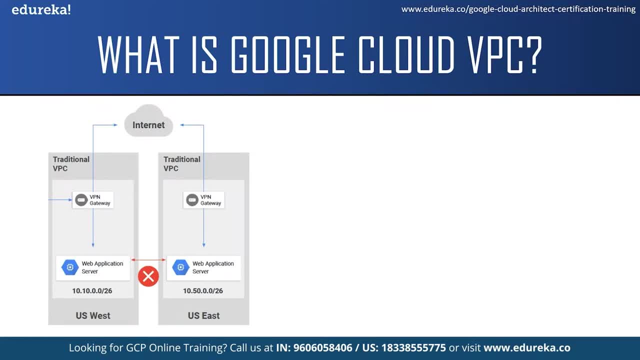 Now here in the first diagram, we can see that there is two VPC built with two different subnets in two different region, which are us east and US West. Now the virtual machine in one region can access the internet and communicate with the other virtual machine only through the VPC gateway, which acts as an interface in the 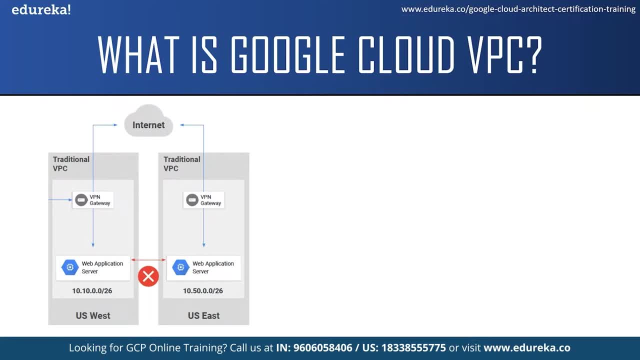 traditional VPC, one virtual machine cannot directly communicate with the other virtual machine. Now, in the Google version of the virtual private cloud, it is a global construct, which means instead of creating a VPC in US West and the other one in us east region. 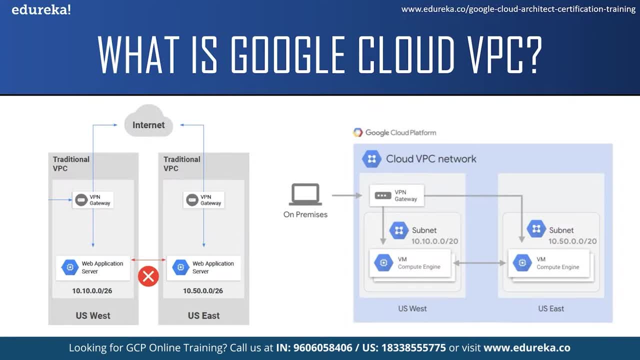 We just create one VPC and put the subnets in two different regions, which are us east subnet, in different region within that VPC. now, in this case, the virtual machine present in one region can directly communicate with the virtual machine in the other region without the help of the VPN Gateway. 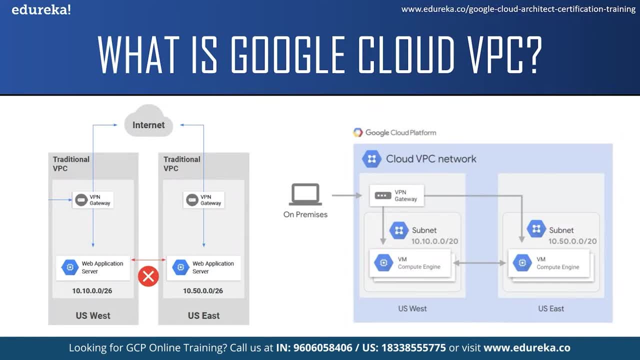 Now the communication between the virtual machines is handled by Google underlying Network. This is the same Network that Google users for a search engine, YouTube, Gmail and its other applications. Now the Google version of VPC can be very helpful. Let's say, for a large project you use the traditional. 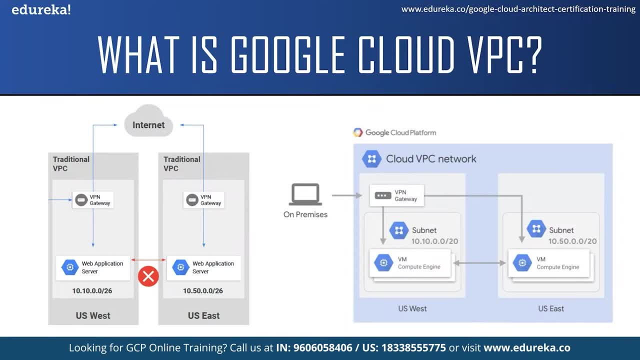 approach, then you have to build multiple VPC and multiple Gateways, which would be very hard to maintain and to keep a track of. now, with Google VPC, You just have to create one VPC and a Gateway and can create multiple virtual machines in multiple subnet. 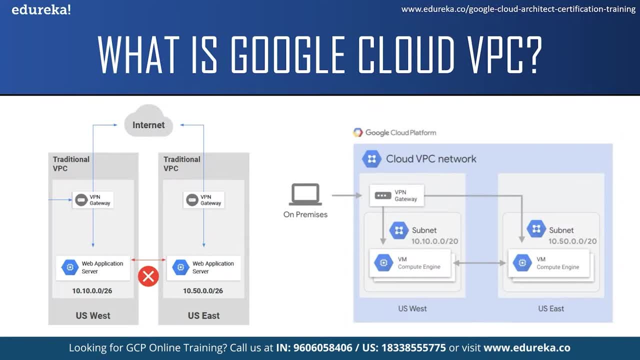 It is much simpler and easy to maintain. also, if something goes wrong with the traditional Network infrastructure, It would take a lot more time and cost to identify and resolve the issue. in Google VPC There are fewer Network construct to break and troubleshoot. this would help in identifying the problem faster and 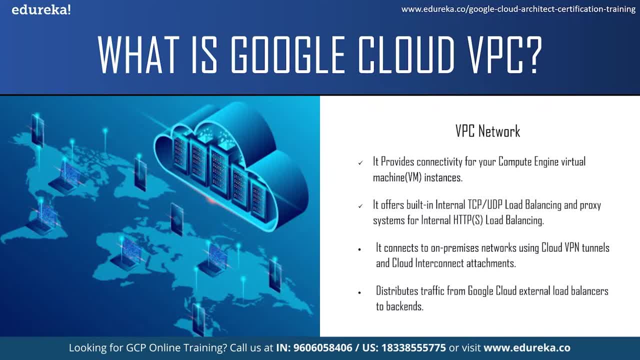 faster And solving it. now let us understand VPC Networks. You can think of VPC Network the same way as a physical Network, except that is virtualized within the Google Cloud. a VPC Network is a global resource that consists of a list of regional virtual sub networks in data centers. 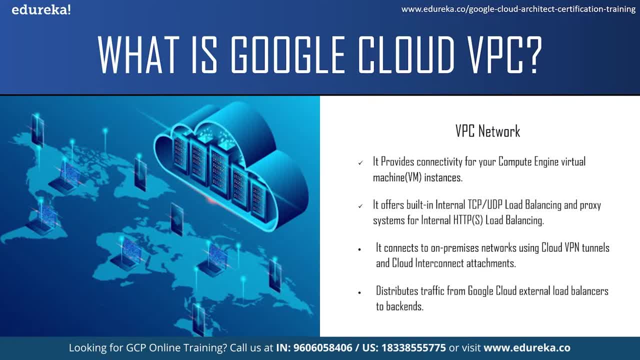 which are called as subnets, and all these are connected by a global wide area Network. Also, VPC Networks are logically isolated from each other in the Google Cloud. Now some of the functionalities offered by Google Cloud VPC Network Are: it provides connectivity for your compute engine virtual. 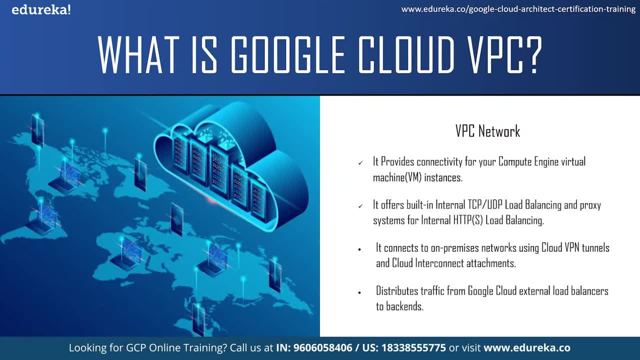 machine instances, including Google Kubernetes, engine clusters, app engine instances and other Google Cloud products built on compute engine virtual machines. It offers built-in internal TCP UDP load balancing and proxy system for internal HTTPS load balancing. It can also help in connecting to on-premises Network using 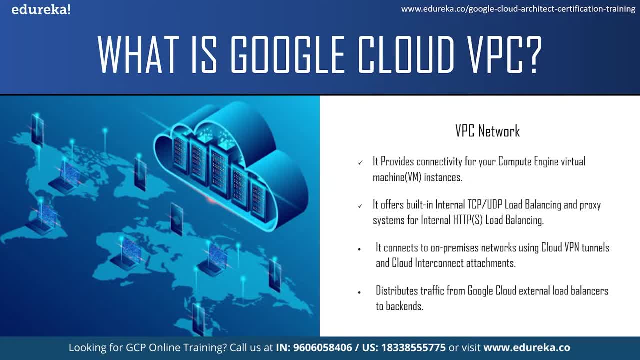 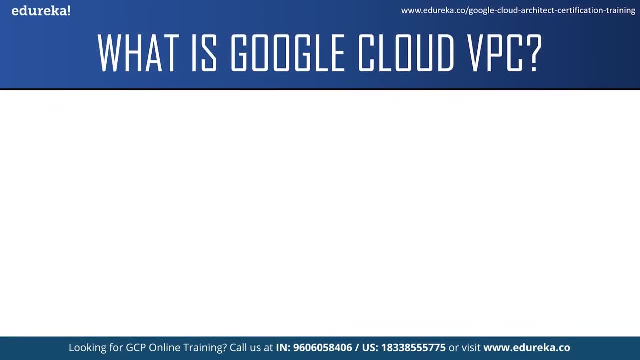 cloud VPN tunnels and cloud interconnect attachments. It distributes traffic from Google Cloud external load balancer to the back end. Now to understand VPC Network better, Let us take a look at its architecture. Now. here you can see, we have two regions: us-west one and 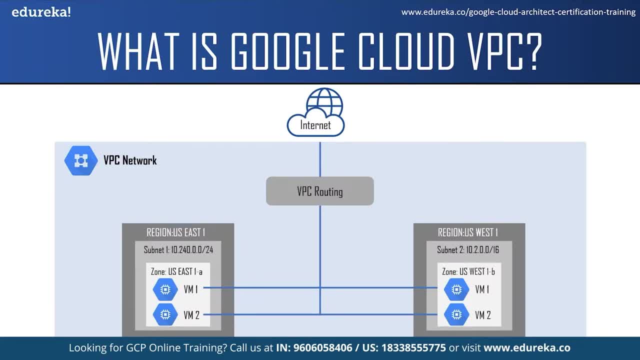 us-east one in a VPC Network. Now, a region is nothing but a specific geographical location where you can host your resources, and a region can have three or more zones. For example, us-1 region has three zones: us-east 1a, us-east. 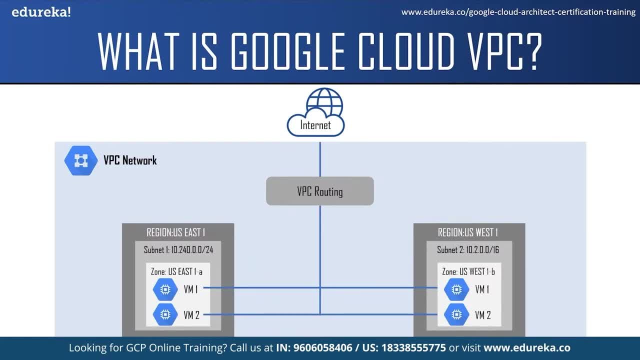 1b and us-east 1- 3. now talking about zones, zones are independent of each other. They have completely Physical infrastructure, networking and isolated control planes. This is to ensure that typical failures event only affect that zone. now coming to subnets: a subnet or a subnetwork is: 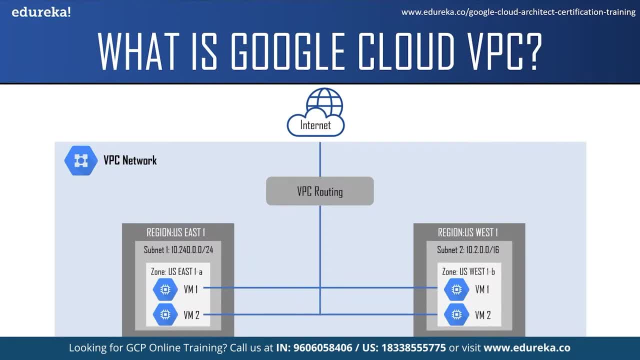 a segmented piece of a larger network. The virtual machine instances can be created in the subnet and the instances can communicate with each other in the same VPC Network using the private IP addresses. here You can see there are two virtual machines in us-east subnet. 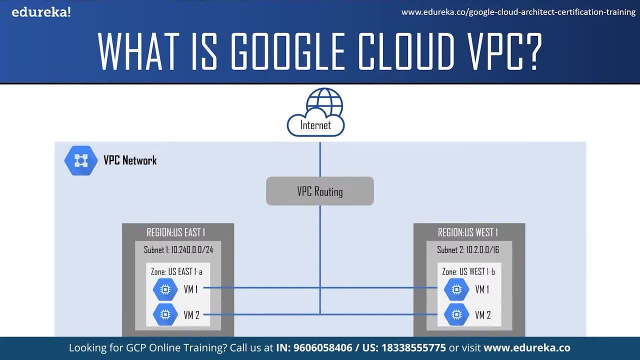 and there are two virtual machines in us-west subnet. now these virtual machines can access the internet through the VPC routing. VPC routing decides how to send traffic from the virtual machine instances to the destination. The destination could be either the other virtual machine instances or the internet. moving on. 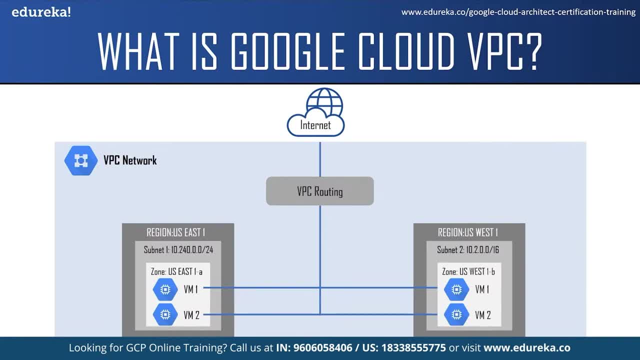 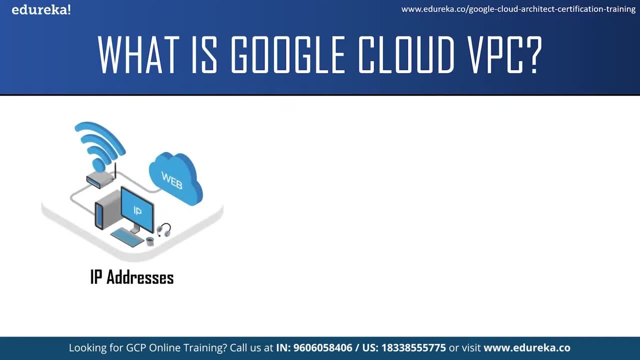 Let us understand a few important concepts in VPC, like IP addresses, routes and firewall rules. You will find all this concept in Google Cloud VPC console. So first let us talk about IP addresses. Now each virtual machine instances in GCP will have an internal 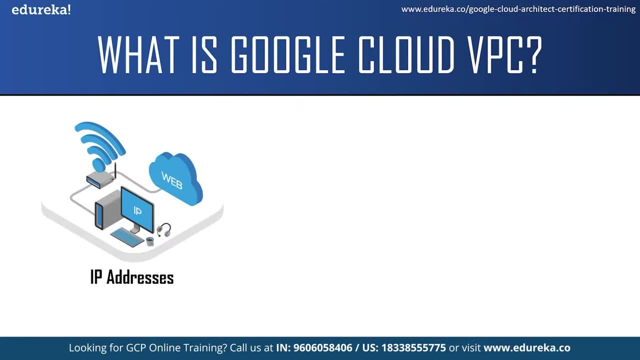 IP address and typically an external IP address. The internal IP address is used to communicate between instances in the same VPC network, while the external IP address is used to communicate with instances in other networks or the internet. These IP address are ephemeral by default, but can be statically. 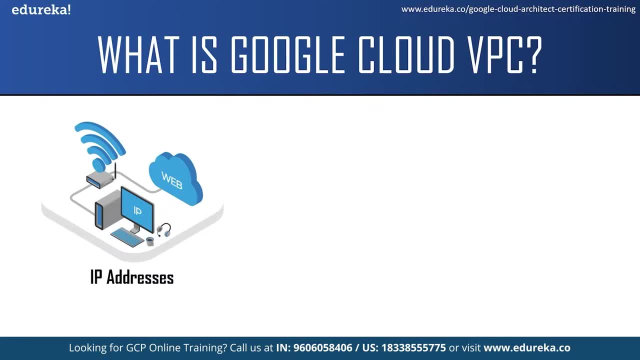 assigned to ephemeral means. the IP address will keep changing every time the virtual machine research- now talking about the VPC routes route tells virtual machine instances and the VPC network how to send traffic from an instance To the destination. The destination can be either inside the network or outside. 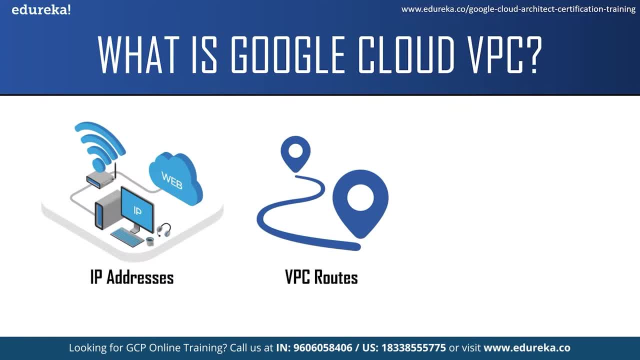 of Google Cloud, which is the internet. You can also create custom static routes to direct some packets to specific destination. Now, each VPC networks comes with some system-generated routes. There are two different system-generated routes. First is the default route. This route defines a path for the traffic to leave the VPC. 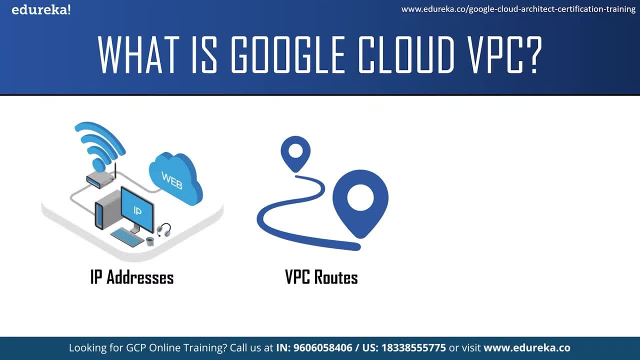 network. It provides general internet access to virtual machines that meets the requirement. It also provides the typical path for private Google access. Next, for communication within the network, There is subnet routes. It defines the path for sending traffic among instances within the network by using internal IP addresses. 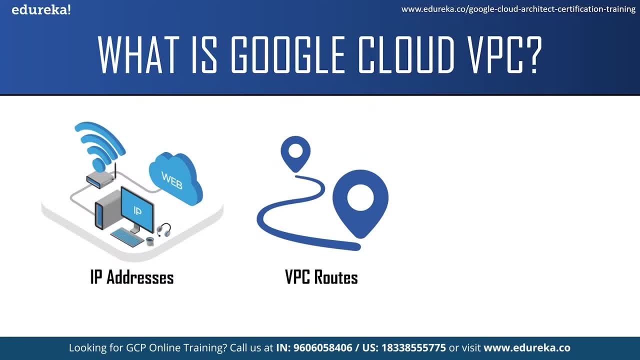 But for one instance to communicate with another, you must configure appropriate firewall rules, because every network has an implied deny firewall rules for English traffic. Now talking about firewall rules, each VPC network implements a distributed virtual firewall that you can configure. firewall rules allow you to control which packets can traffic. 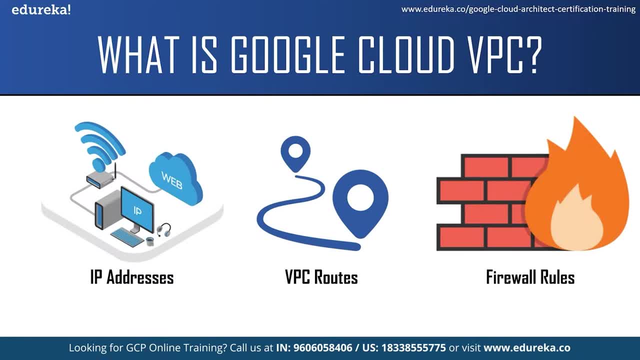 Travel to which destination. it lets you allow or deny connection to or from your virtual machine instances based on configuration that you specify. Now, when you're creating a VPC firewall rule, you must specify the VPC network and a set of configuration that defines what 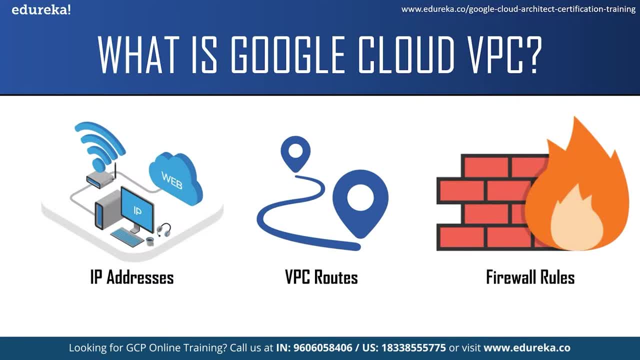 the rule does. the configuration enables you to target certain types of traffic based on the traffic protocol, destination, port sources and destination. You can create a modify VPC firewall rules by using a Google Cloud console, gcloud command line And rest api's. now, these were some of the important topics. 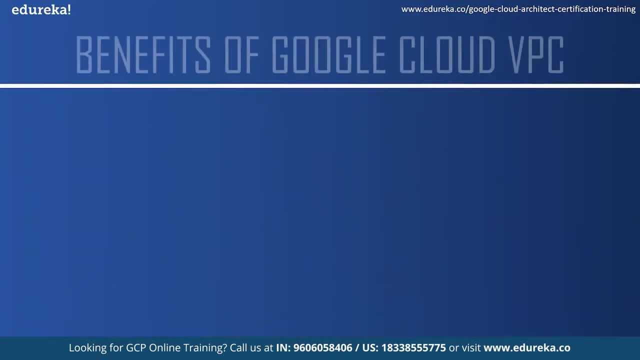 in Google Cloud VPC. Now let us move on to the next topic and see some of the benefits of Google Cloud VPC. first is it is global. using a VPC gives you manage global networking functionality for all your Google Cloud resources through subnetworks known as. 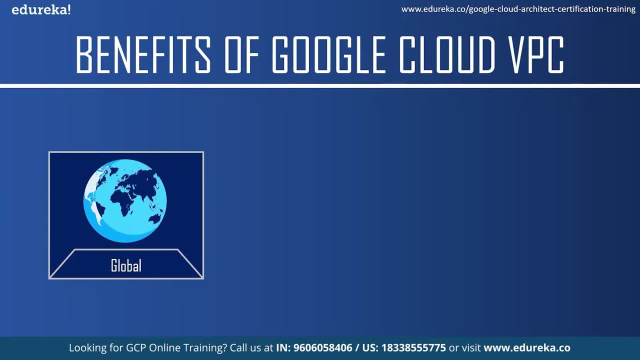 subnets which are hosted on Google Cloud data centers. a single Google Cloud VPC and its subnets can span across multiple region without ever connecting to the public internet. It remains isolated from the outside world And it's not associated with any specific region or zone. 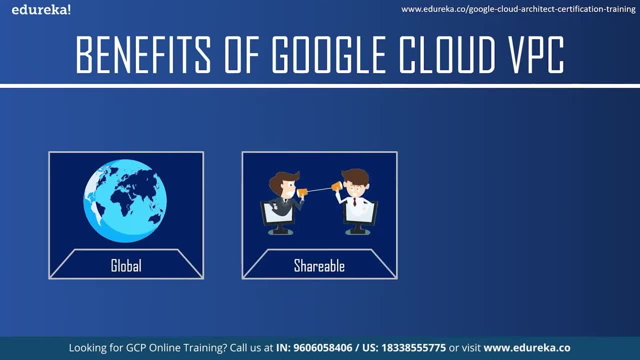 second benefit is it is shareable. now an entire organization can use one VPC and share it across the various team. different team can be isolated within projects with different billing and quotas, yet They can still maintain a shared private IP space and access to commonly used services. 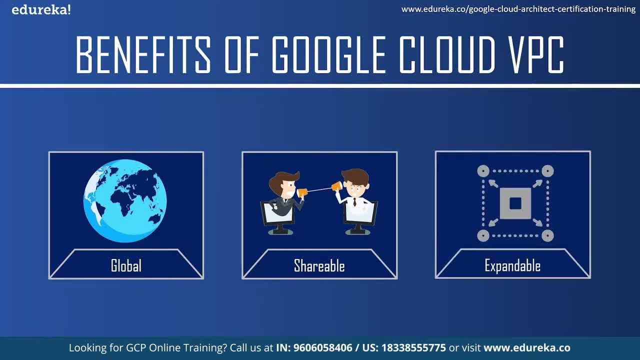 The next advantages. it is expandable. Google Cloud VPC lets you increase the IP space of any subnet without any workload shutdown or downtime. This gives you flexibility and growth option to meet your needs. Now I guess you have some idea about VPC. 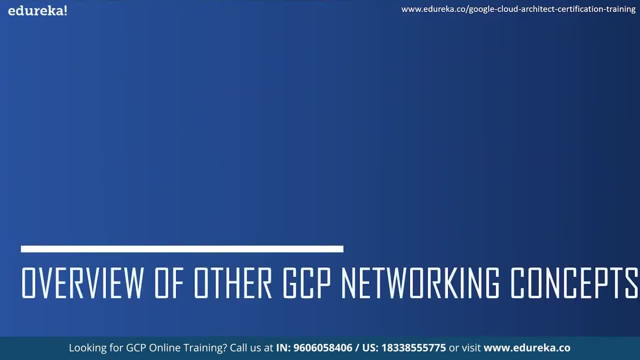 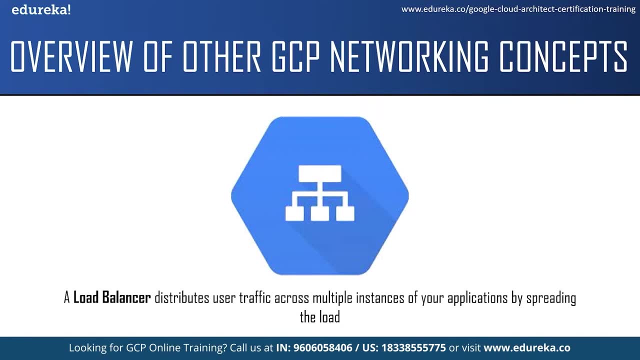 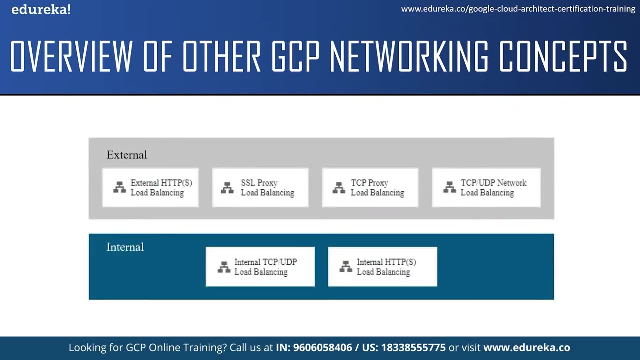 Now let us move on to the next topic and see what is Google Cloud load balancer. Basically, a load balancer distributes user traffic across multiple instances of your application. by spreading the load, load balancing reduces the risk that your application experience performance issues. Google Cloud offers six types of load balancer, which are: 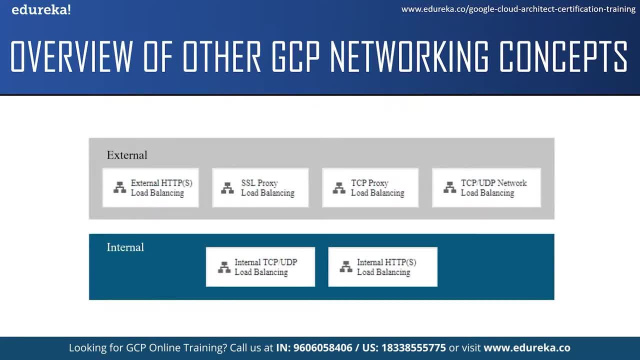 external HTTPS load balancing, SSL and TCP proxy load balancing. External TCP UDP network load balancing. internal HTTPS load balancing and internal TCP UDP network load balancing. not to decide which load balancer best suits your implementation, consider factors such as global and regional load balancing. You can use global load balancing when your back ends are. 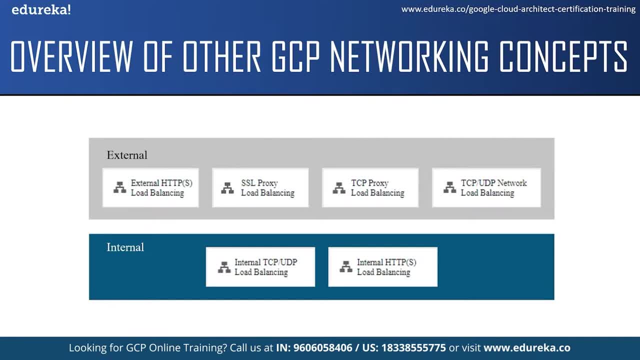 distributed across multiple region. your user needs access to the same application and content and you want to provide access by using a single IP address. You can use regional load balancing when your back ends are only in one region. The next factor is external and internal load balancing. 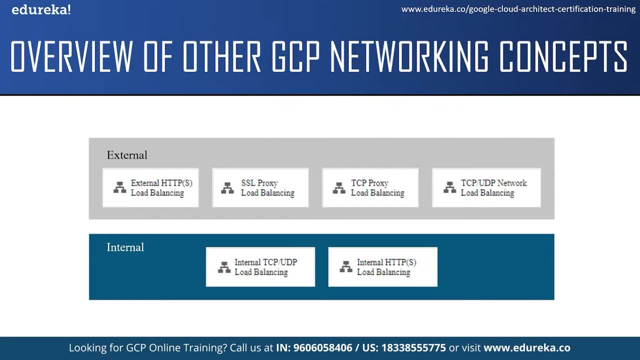 Now, external load balancer distributes traffic coming from the internet to Google Cloud VPC network, and internal load balancer distributes traffic to instances within the GCP network. and the last factor you need to keep in mind is the type of traffic that you need a load balancer to handle. such 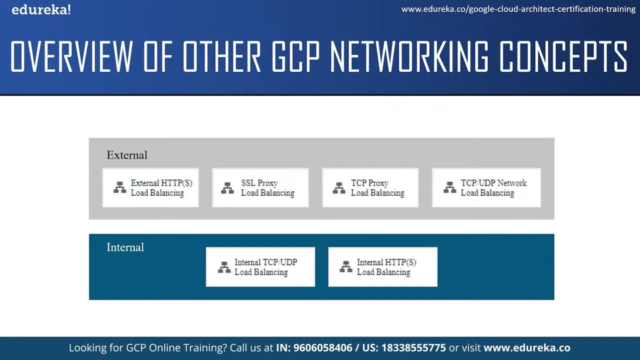 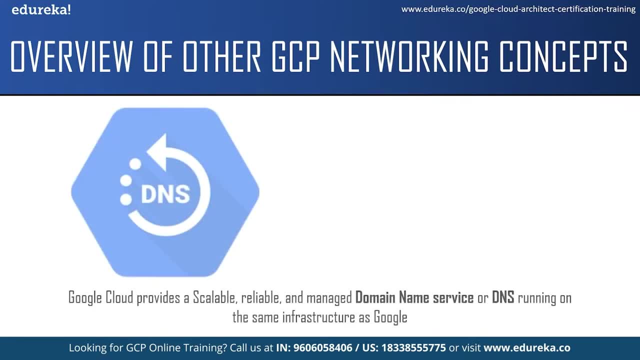 as HTTPS, TCP or UDP traffic. Now, this was a brief information about Google Cloud load balancing. Let us move on to the next topic and understand what is cloud DNS service. Cloud provides a scalable, reliable and managed domain name service, or DNS, running on the same infrastructure as that of 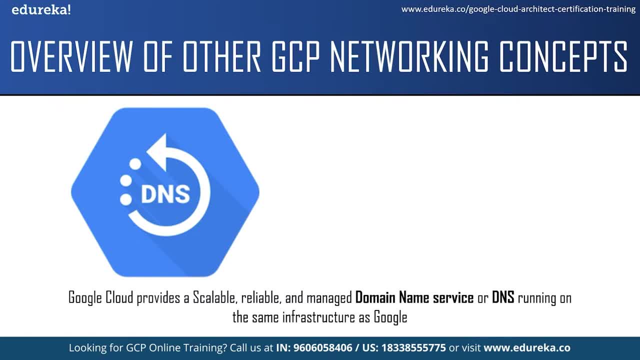 Google. But before we get into cloud DNS, let us understand what DNS is. So DNS is a hierarchically distributed database that lets you store IP addresses and other data and look them up by names. In other words, DNS is a directory of easily readable domain. 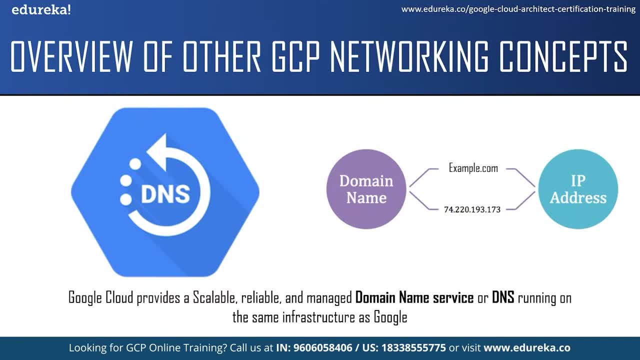 name that translate to numerical IP addresses which are used by computers to communicate with each other. For example, when you type URL into a browser, DNS converts the URL into an IP address of a web server associated with that name, like wwwexamplecom. is translated to IP address. 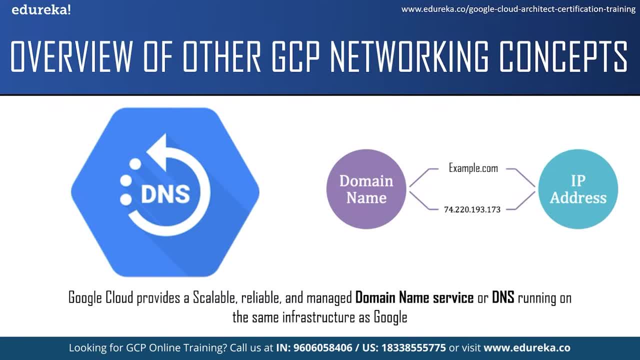 of 72.2, 20.193.173. then the DNS directories are stored and distributed around the world on domain name servers that are updated regularly. Now, cloud DNS is a high-performance, resilient global DNS service that publishes your domain name to the global DNS. 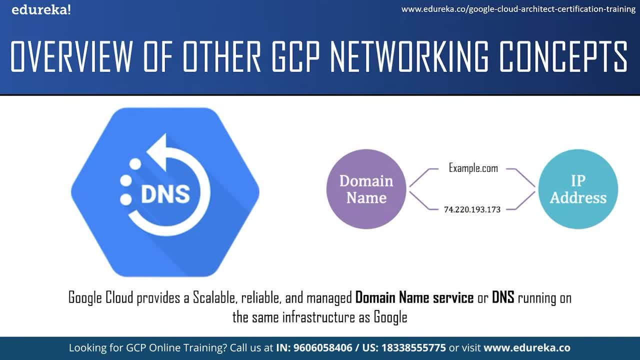 in a cost-effective way. Cloud DNS lets you publish your zones and records in DNS without the burden of managing your own DNS servers and software. cloud DNS offers both public zones and private managed DNS zones. Now, public zone is visible to the public internet, while a 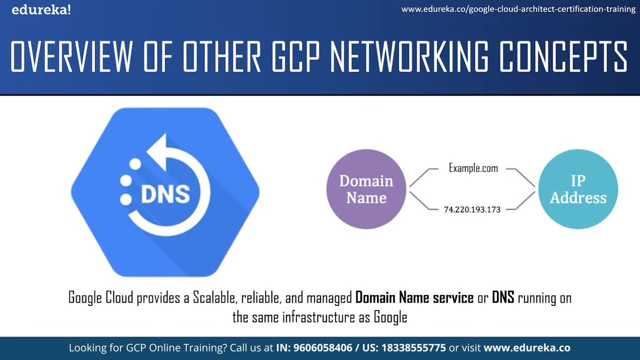 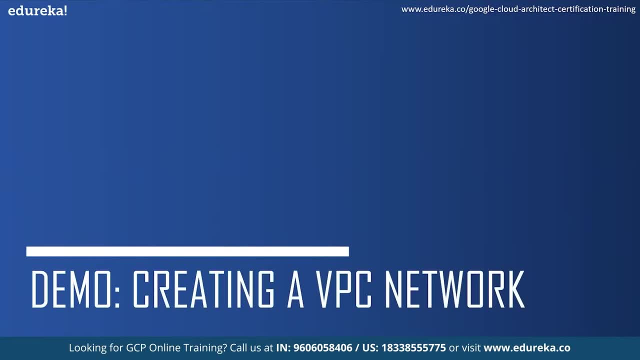 private zone is visible only from one or more virtual private cloud networks that you specify. this was about cloud DNS. Now let us move on to a demo part, where I will show you how to create a VPC network in Google Cloud. So for a demo, I've logged in into a GCP account. 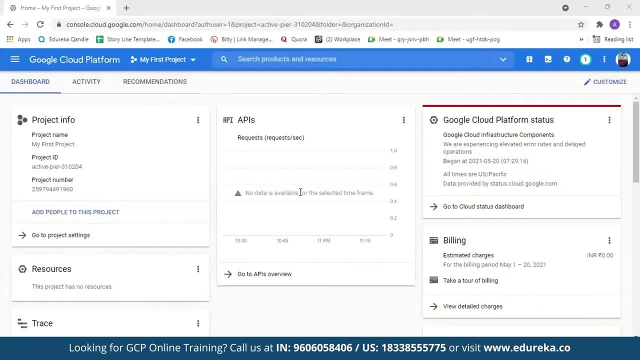 For people who are new to GCP, This is what the GCP console would look like now. It is very simple to create a GCP account. All you have to do with enter your debit card or your credit card details and your address. then you might be charged maybe. 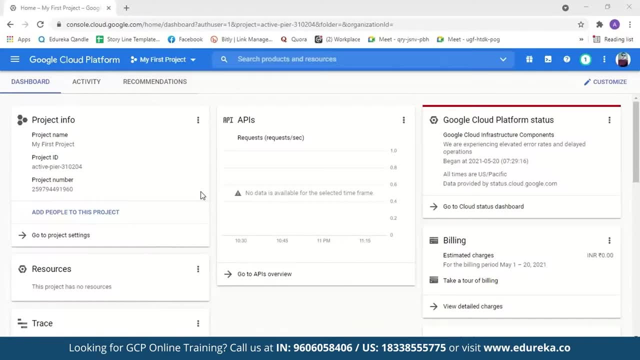 a rupee, but even that would be refunded later. and after you sign into a new account, GCP will provide you $300 free credits. You can use this amount to explore Google Cloud Services. You won't be charged until you choose to upgrade, and it will. 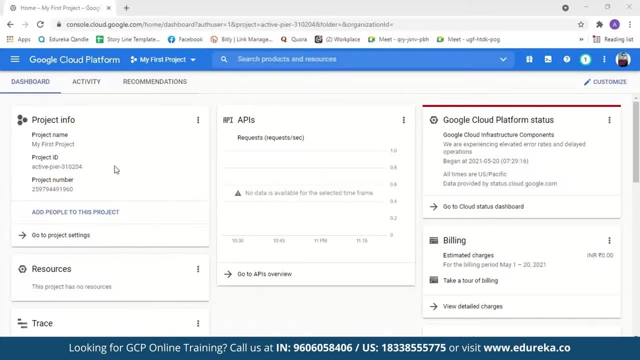 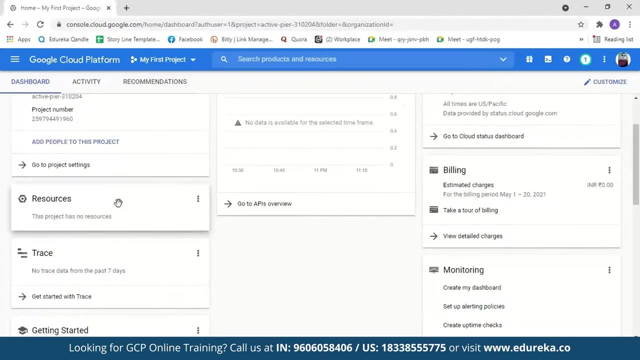 be valid for 90 days. now, coming back to a GCP console, You can see we have the project Info over here. Now you must have a project in order to use the GCP resources, and here will be the list of resources that your projects. 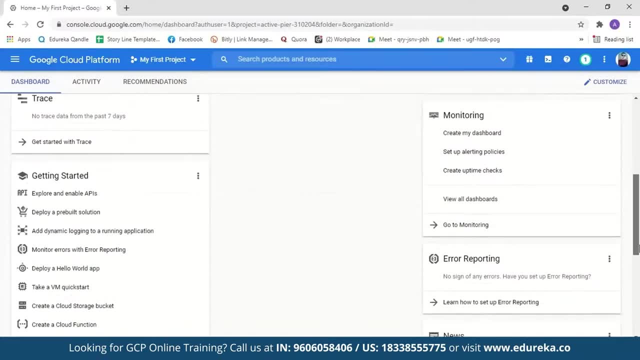 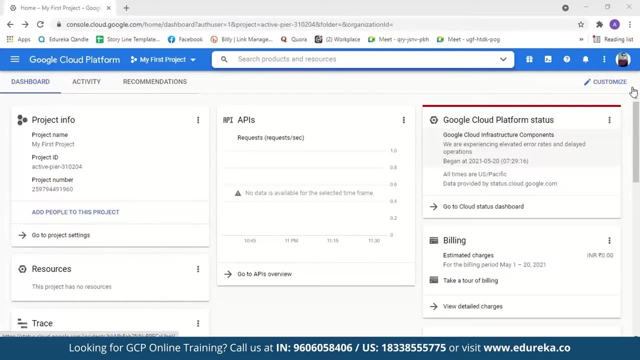 use here will be the billing, the monitoring dashboards. If you're new to GCP, you can explore the various services provided by Google Cloud. So demo is going to be very basic, where I will explain how to create a VPC and subnets. 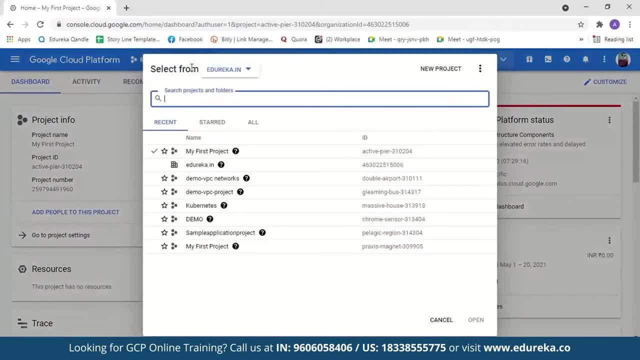 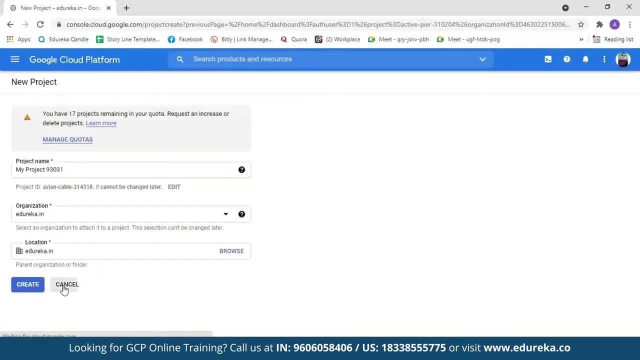 So the first step is to select a project. Now, if you're using GCP for the first time, you can just create a new project from here. click on new project, name your project anything you like and just created. Now for this demo, I'll just select from an existing project. 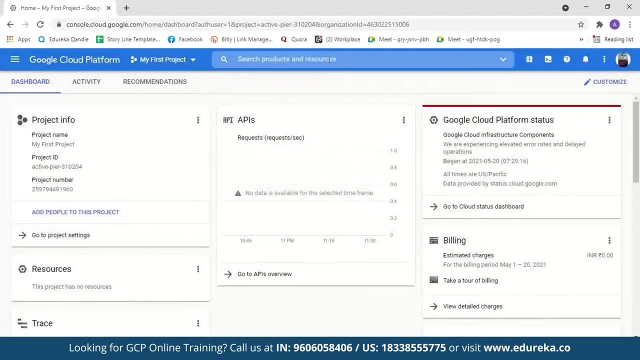 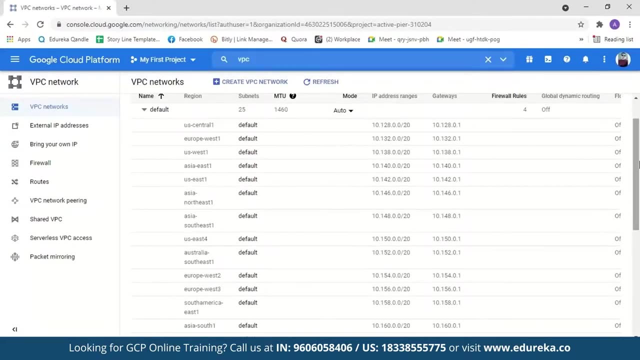 So I'll let this be, and now let us search for VPC over here. We'll select the VPC network. Now you can see here that Google Cloud comes with the default VPC, and this VPC has 25 subnets, each subnet having its own IP. 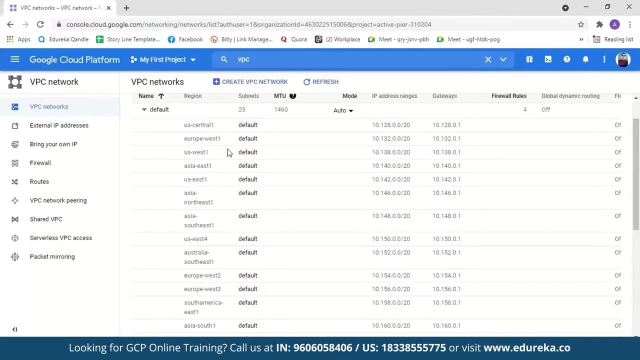 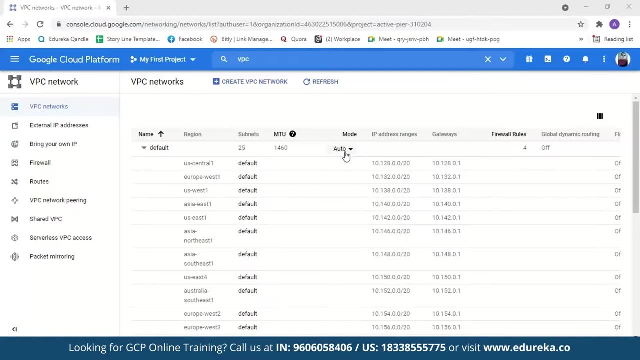 address and in a different region. as I mentioned before, GCP has 25 region and 76 zones, So each subnet is created 25 different zones. Next, you see something called mode over here and you can see there are two types of mode: custom and Auto. 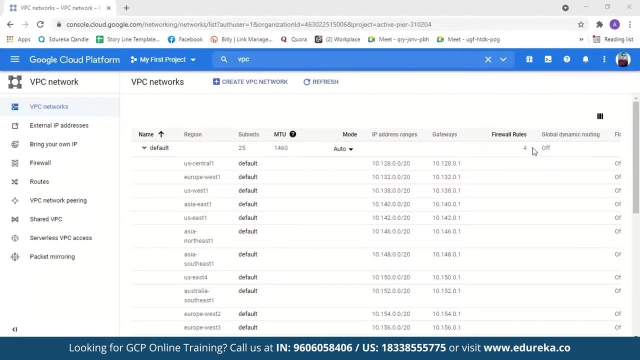 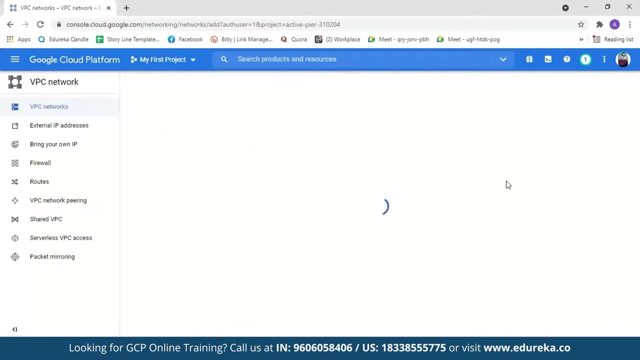 We will talk about this when we're creating a VPC and there are four default firewall rules. So let us now create a new VPC. So just go to create VPC Network And we can name a VPC anything we want. So I'll just name it demo VPC. 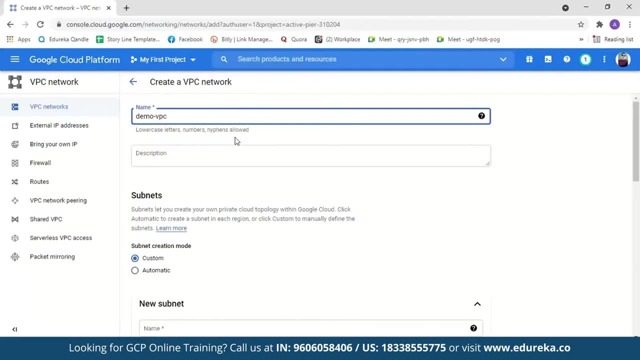 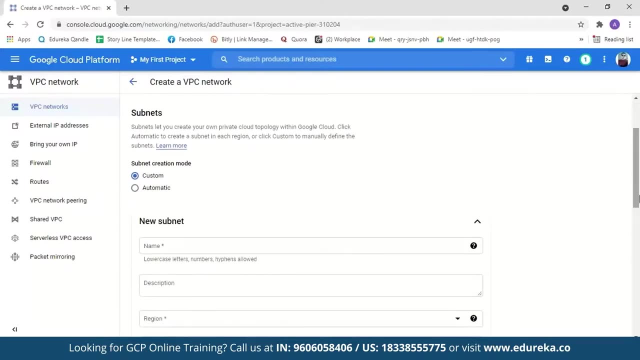 And you can see only lowercase letters. numbers and hyphens are allowed. Next, you can describe your VPC, but this is optional, So I'll just skip it. Now, coming to subnets, We can create a subnet with two different methods. 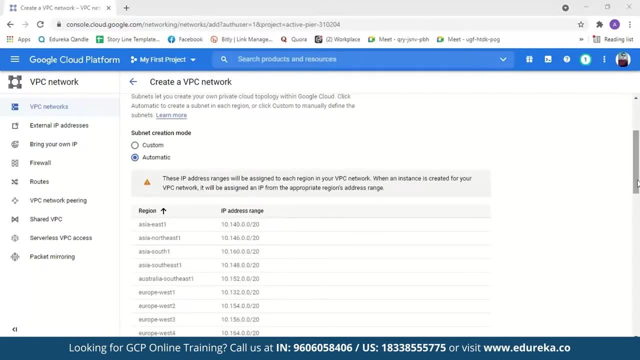 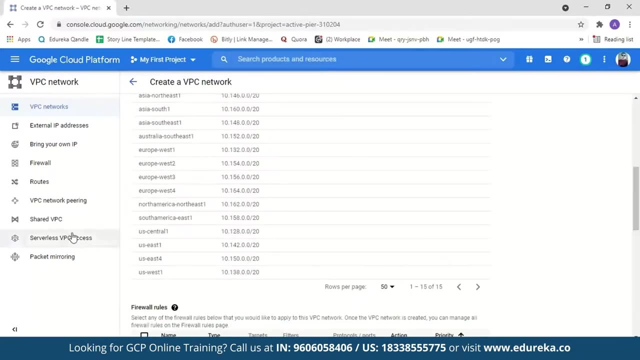 One is custom and the other one is automatic. If you select automatics, subnets are automatically created with different IPs in different regions. Now you can see an automatic: 15 subnets are created in 15 different regions. If you want, you can select any firewall rules from here. 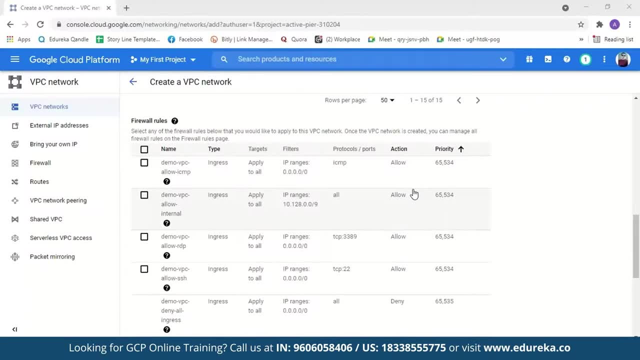 Now, as I mentioned before, firewall rules allow you to control what packets can travel to which destination. with the demo VPC, allow ICMP, It will allow only ICMP traffic from any source to any instances in the network and with the allow internal firewall rules, It will allow connection for all protocols and ports among: 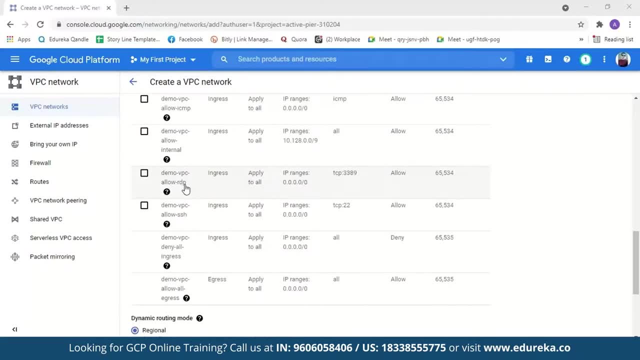 instances in the network. Next, the allow RDP firewall rules allows RDP connection from any source to any instances on the network using port 3389.. The port is given over here. Next is the allow SSH Pick rule. This allows TCP connection from any source to any instances. 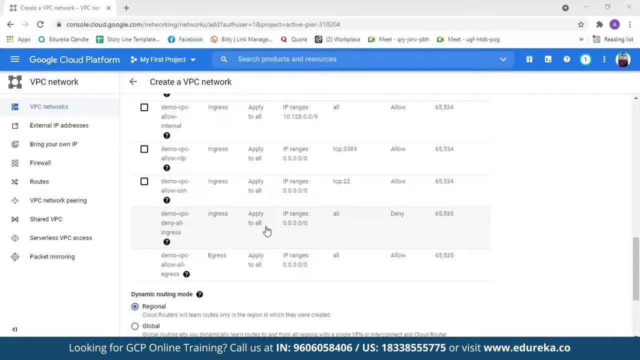 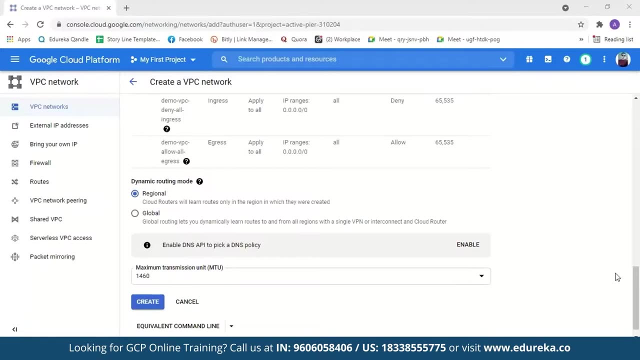 in the network with the destination port 22 next. These two are the default firewall rules and the default routing mode is set to regional. you see, Google Cloud makes it very simple for you to create a VPC. All you have to do is just name your VPC, select automatic. 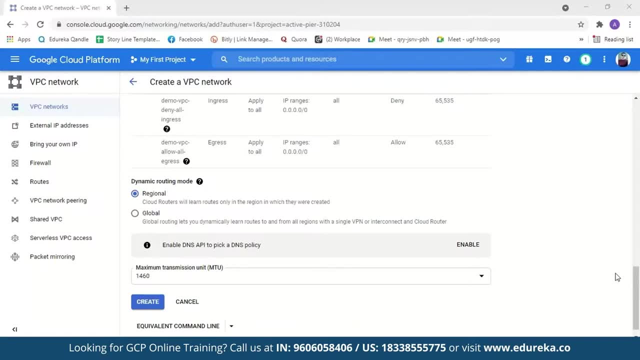 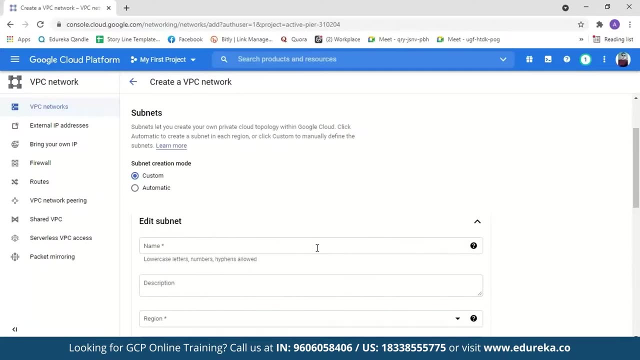 and click on create button and then your VPC will be created. But for this demo we're going to select the custom subnet and create only a few subnets, So we'll just go to custom. Now we can name a subnet anything we want. 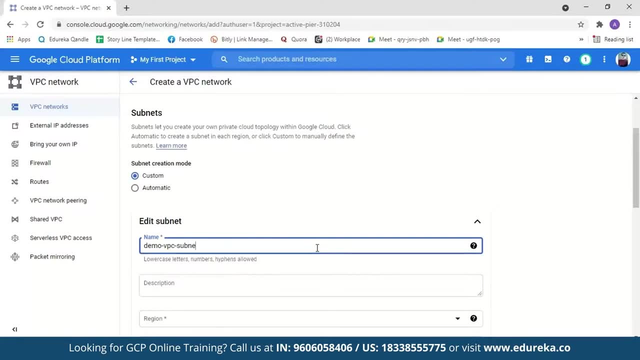 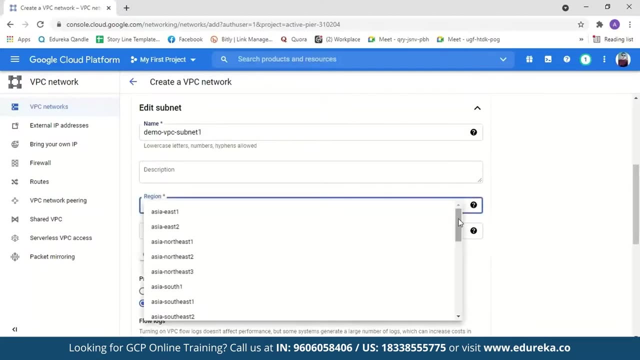 We'll just name it Mo VPC subnet. If you want, you can add description about your subnet next up to select a region. So these are the available regions. So we'll just select us East one and have to mention the IP address range. 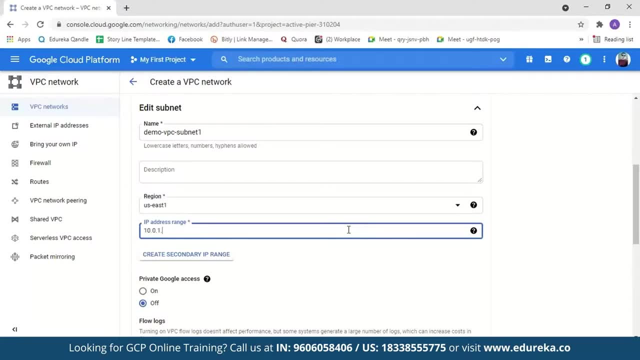 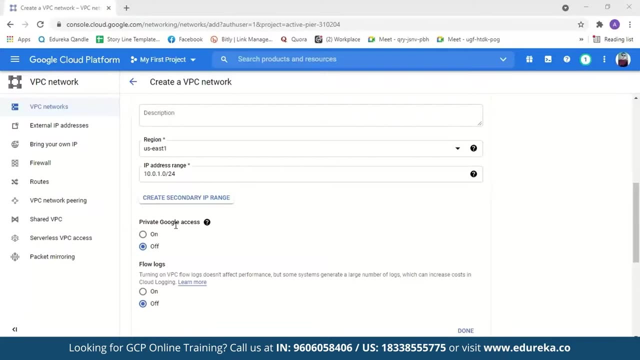 So I'll just mention 10, 0, 1.0, 24.. Next, we have something called private Google access. This means I can set my virtual machines in the subnet to access Google services without assigning an external IP address. So I'll just on this. so now my virtual machines will be able. 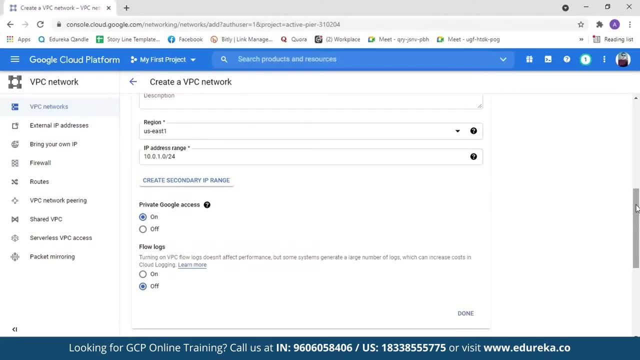 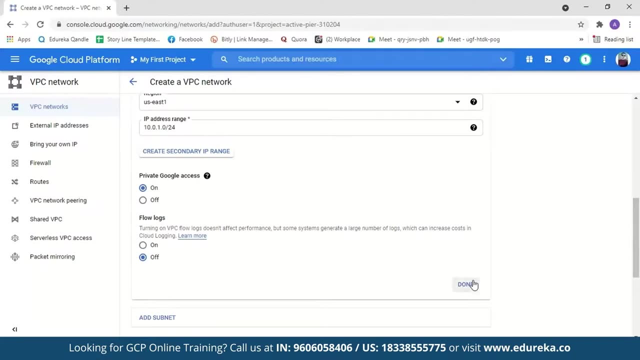 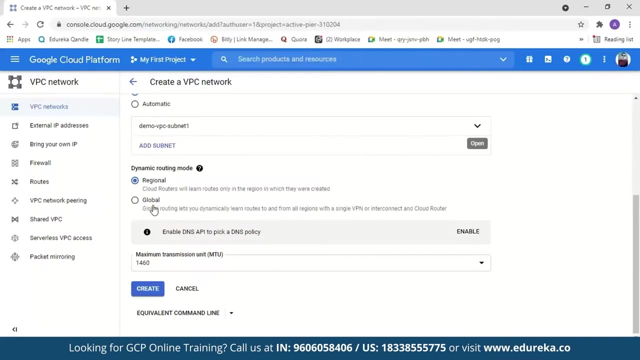 to access Google services without an external IP address. I will let the flow logs be off. flow logs are just to record the network flow. if you want, you can own it as well. I'm just going to click on done. Next we can select regional or global routing mode. regional: 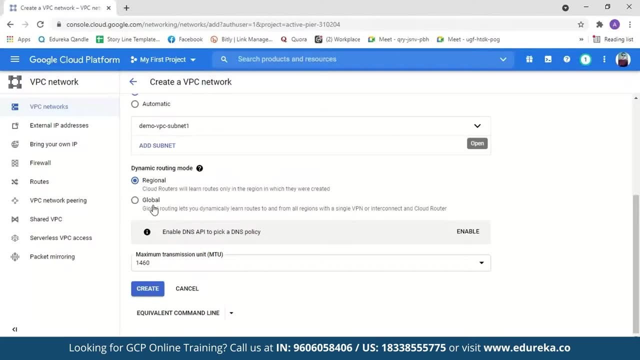 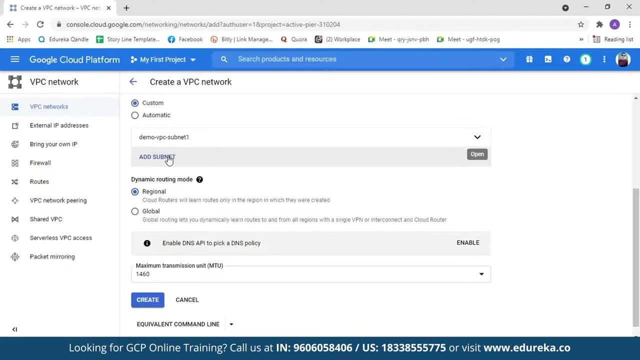 routing will route only in the region They were created, and global routing will route to and from all the regions. So let it be default regional. Now let us create another subnet. We just name it demo VPC subnet 2.. And the region will select us: West one. 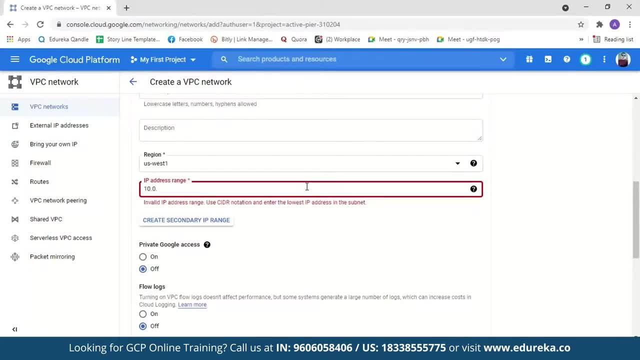 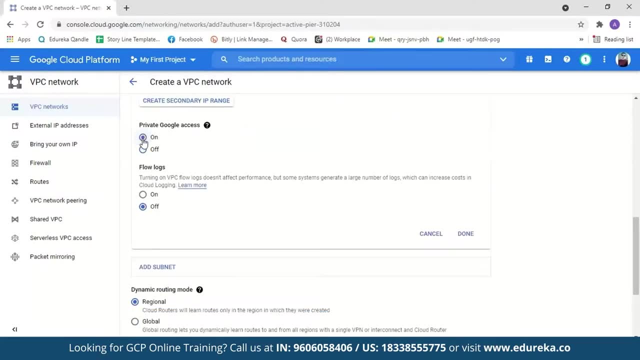 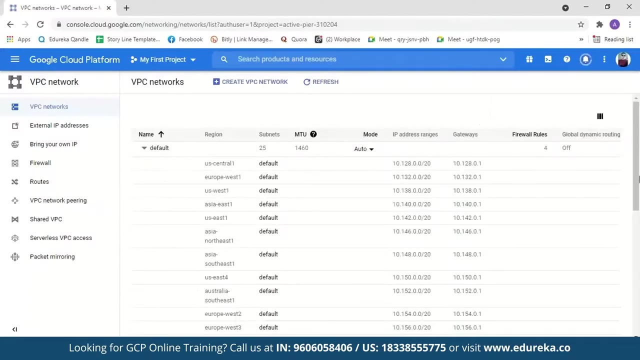 We give the IP ranges 10.0.2.0, slash 24.. We'll let the private Google access be on And click on done. I'll just create my VPC Now. VPC is being created. This might take a couple of minutes. 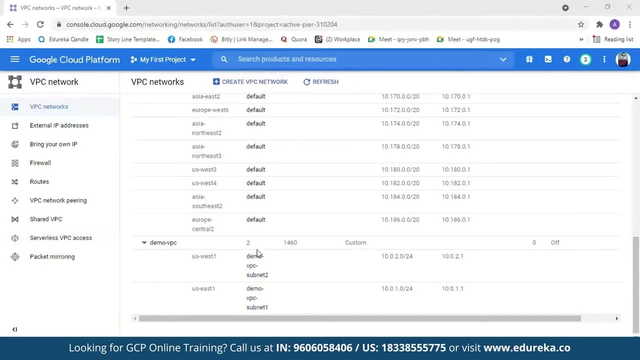 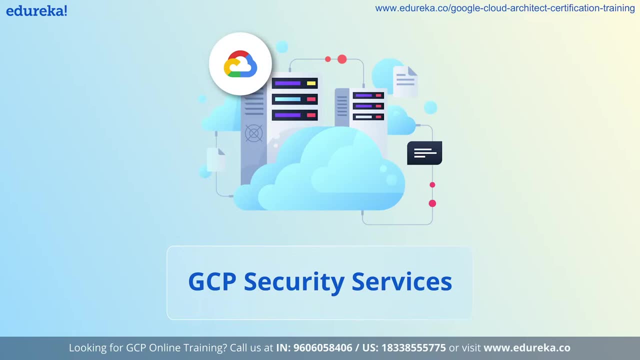 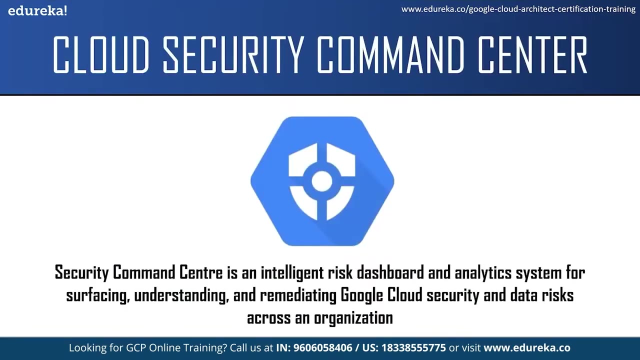 Now you can see a VPC successfully created and two subnets are created, in us West one and the other one in us East one. What exactly is GCP security command center? security command center is a security and risk management Platform provided by Google Cloud. 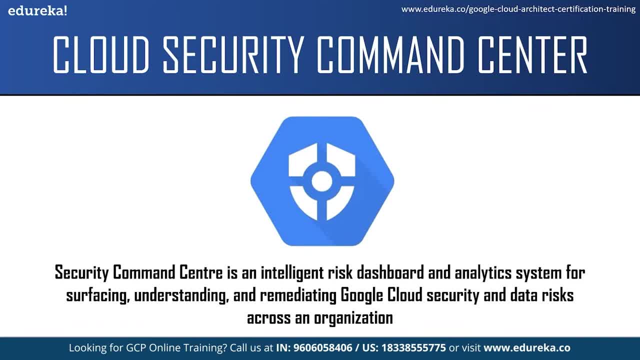 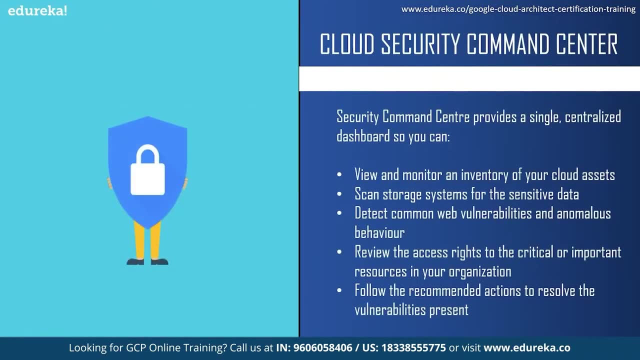 It is an intelligent, rich dashboard and analytics system for surfacing, understanding and remediating Google Cloud security and data risk across an organization. in simple words, It is an established security and risk database for Google Cloud. Now the security command center have security teams gather. 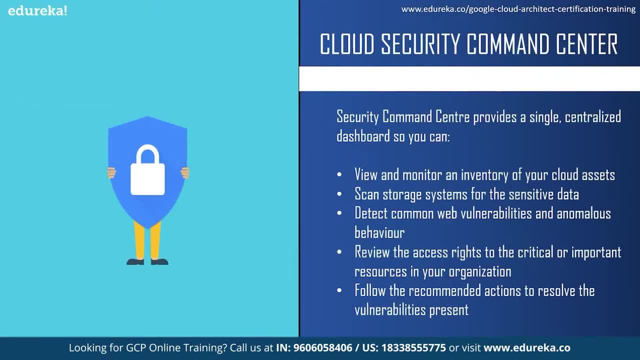 data, identify threats and act on them before the result in business damages or loss. It offers deep insight into application and data risk so you can quickly reduce the threats to your cloud resources across your organization and evaluate the overall health security command center provides a single, centralized dashboard so you 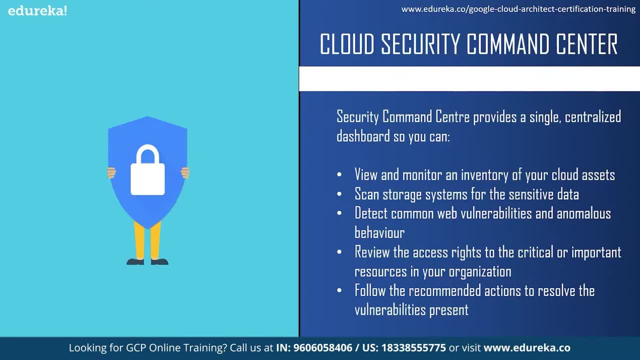 can view and monitor an inventory of your cloud assets. now, assets are nothing but your resources, like organizations, your projects, your instances and your applications. It can also help in scanning storage system for the sensitive data. It can be used to detect common web vulnerability and anomalous. 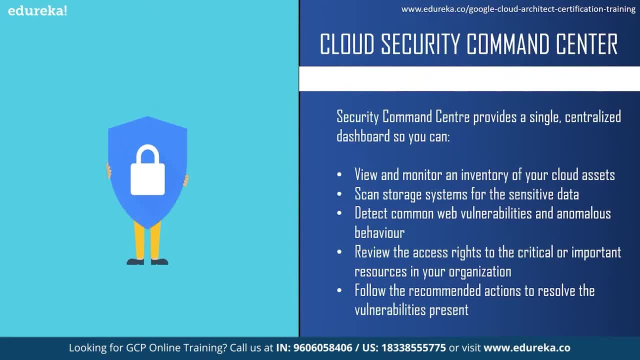 behavior, But security Command center. You can also review the access right to the critical or important resources in your organization and along with that, you can follow the recommended actions to resolve the vulnerability present. Now I guess you have some idea about what exactly is the. 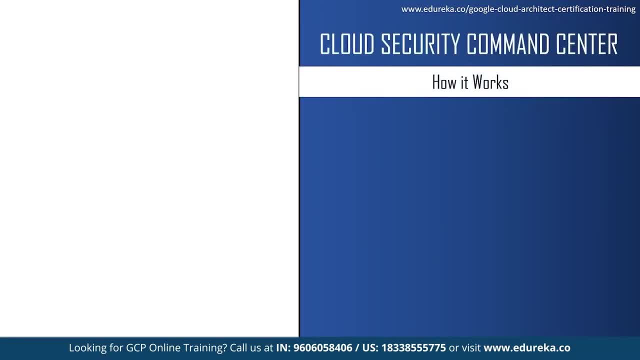 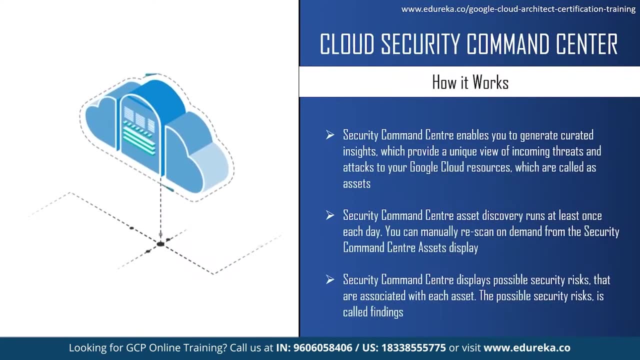 security command center. So now let us see How does the security command center work in order to understand it better. security command center enables you to generate curated inside, which provides a unique view of incoming threats, and, attached to a Google Cloud resources which are called as. 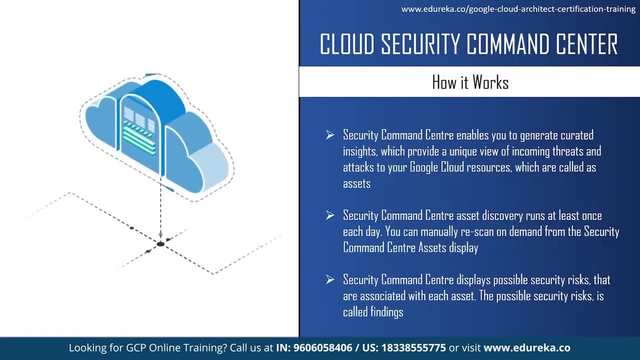 assets. now, assets are nothing but resources like organization, projects, instances and application. the security command center asset Discovery runs at least once a day. You can also manually rescan on-demand from the security command center assets display. then the security command center displays possible security risks that are associated with each asset. 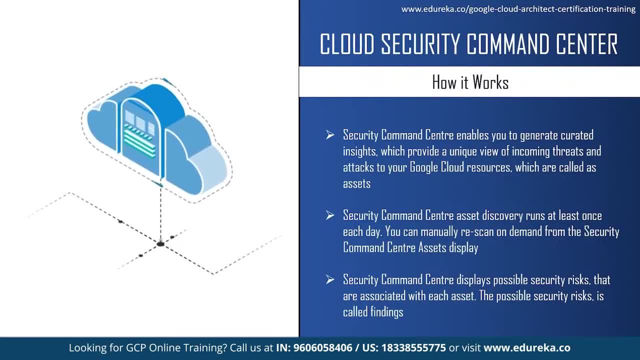 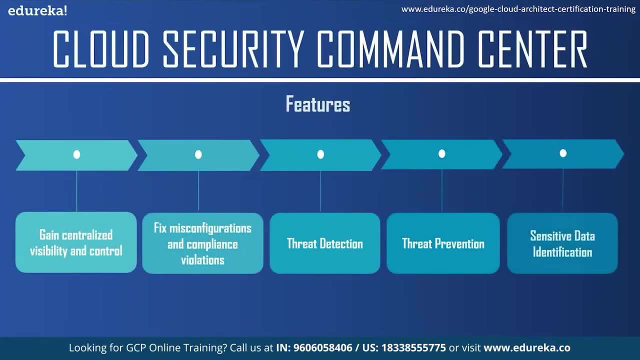 The possible security risk is called as findings. Now, this finding comes from security sources that include security command centers, built-in services, Third-party partners and your own security detectors and finding sources. Now, this was the working of security command center. Let us take a look at some of his prominent features. 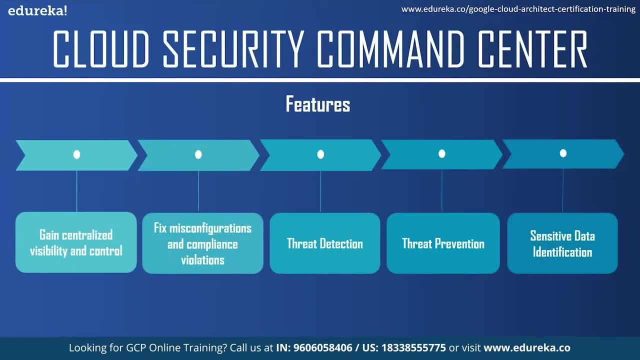 The first one is you can gain centralized visibility and control. security command center gives you a centralized visibility of the number of projects are using, what resources are deployed, and you can also manage which service account has been added or removed. The second feature is you can fix misconfiguration and compliance. 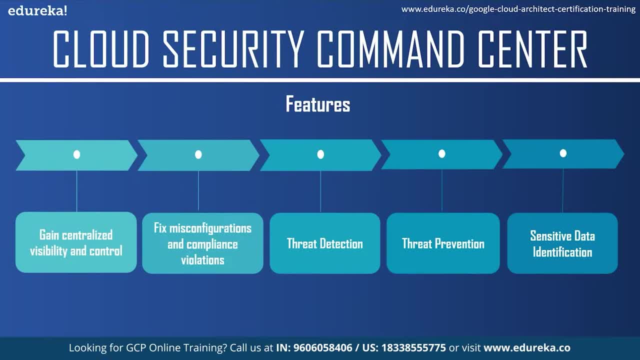 violation. with security command center, You can identify security misconfigurations and the compliance violation in a Google Cloud assets. After you've identified this vulnerabilities, you can resolve them by following the actionable recommendation which is provided by Google Cloud platform. The third prominent feature is threat detection. 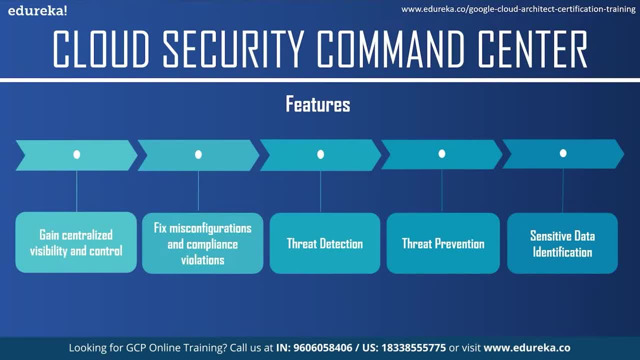 You can detect threat using the logs running in the Google Cloud. at scale, You can detect some of the most common container attacks, including suspicious binary, suspicious library and reverse shell. You can also identify threats like cryptography, mining anomalies, reboots and suspicious network traffic with built-in anomaly detection. 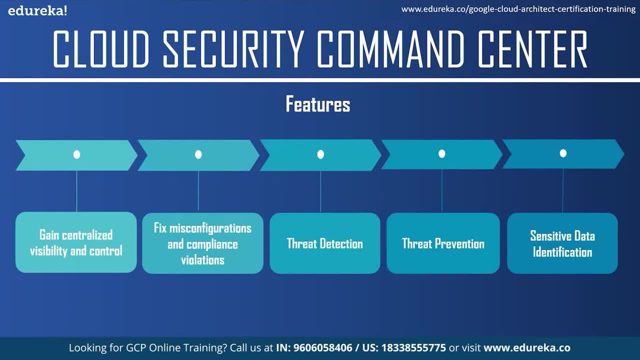 technologies which are developed by Google itself. Next, after threat detection, we have threat prevention with security command center. You understand the security state of a Google Cloud assets. You can uncover common web application vulnerabilities, such as cross-site scripting or outrated libraries in a web application. 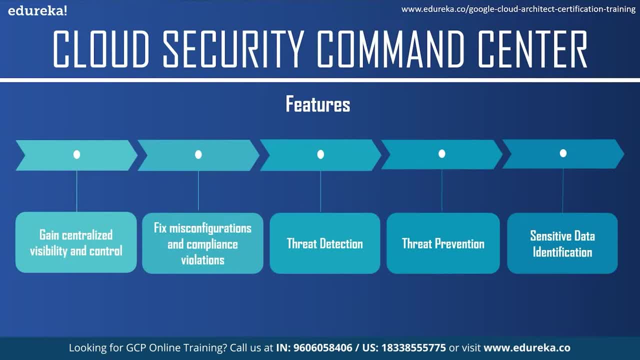 that are running on either Google App Engine or Google Google Kubernetes engine or Google compute engines, Then you can quickly resolve this misconfiguration by clicking directly on the impacted resources and following the procedure steps on how to fix it. The last feature is sensitive data identification with security. 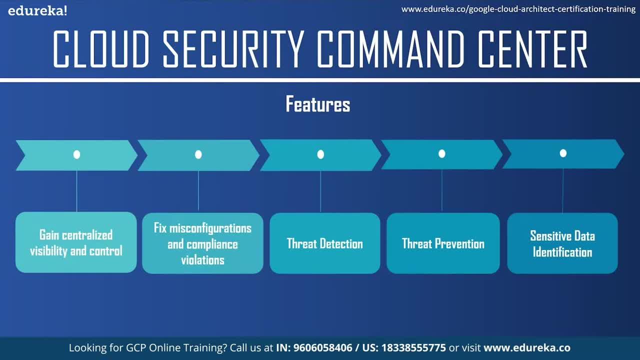 command center, You can find out which storage bucket contains sensitive and regulated data. using cloud DLP, You can also prevent unintended exposure to this storage buckets and let only the authorized person access it. So these were some of the features of cloud security command center. 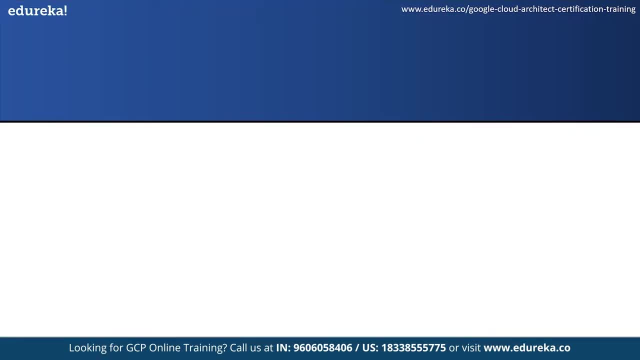 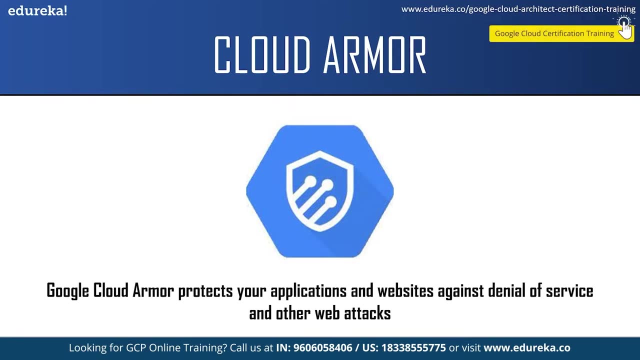 Let us move on to the next topic and see what is cloud armor. Google Cloud Armor protects your application and website against denial of service and other web attacks. You can use Google Cloud Armor security policies to protect your application running behind a load balancer from distributed 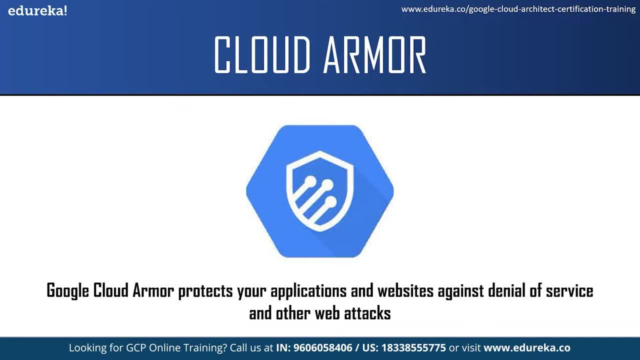 denial of service or DDOS and other web-based attacks, and your application could be deployed anywhere, whether on the Google Cloud or in a hybrid deployment or in a multi-cloud architecture. So this was the definition of cloud Armor, and let us understand how this cloud armor works. 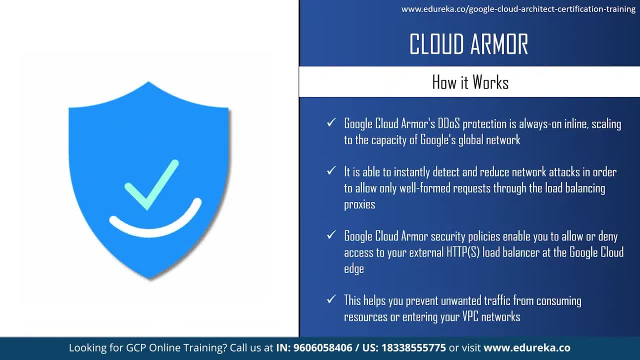 Google Cloud Armor's DDOS protection is always on inline scaling to the capacity of Google's global network, So it is able to instantly detect and reduce network attacks in order to allow only well-formed request to the load balancing proxies with Google Cloud Armor security policies. 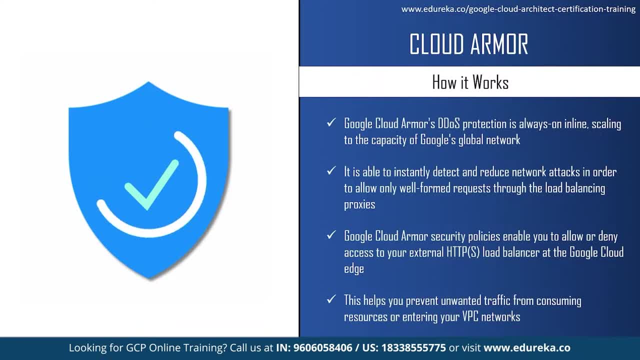 You can also allow or deny access to an external HTTPS load balancer at the Google Cloud Edge, which is as close as possible to the source of incoming traffic. This helps you prevent unwanted traffic from consuming resources or entering your VPC network. Now let us take a look at some of the features of Google Cloud. 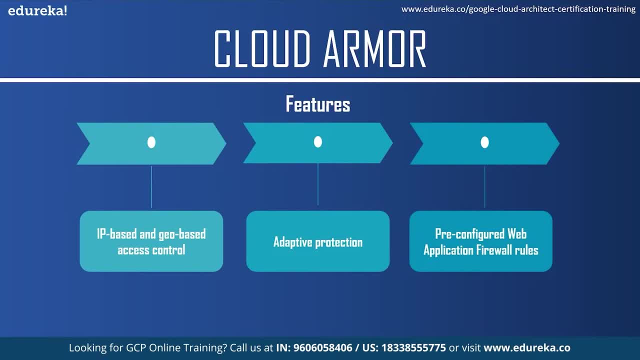 Armor. The first feature is IP waste and geo-based access control. You can filter your incoming traffic based on IPv4 and IPv6 addresses, or CIDRS. We can also enforce geographic based access control to allow or deny traffic based on source geographical location using. 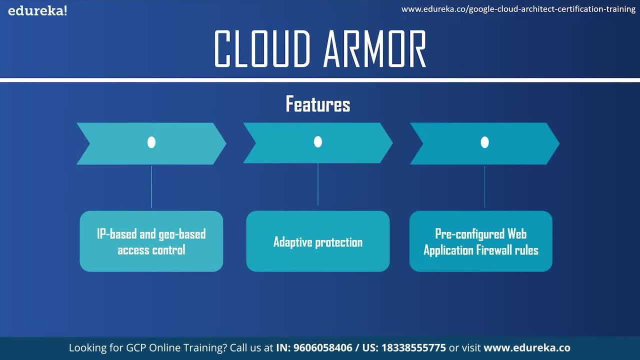 Google geo IP mapping. The next feature: Adaptive protection. Cloud Armor automatically detects and help reduces high-volume DDOS attacks with a machine learning system trained locally on your applications. The last feature is pre-configured web application firewall rules. Cloud Armor comes with the out-of-the-box rule set based on. 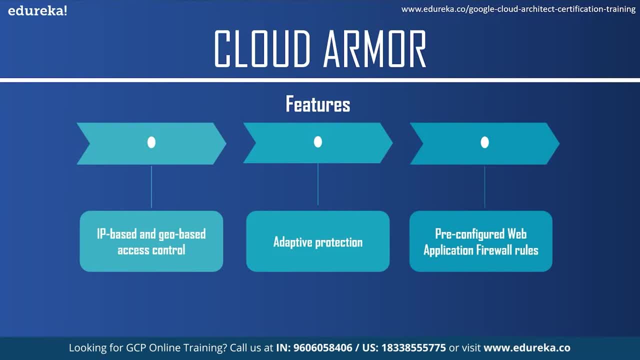 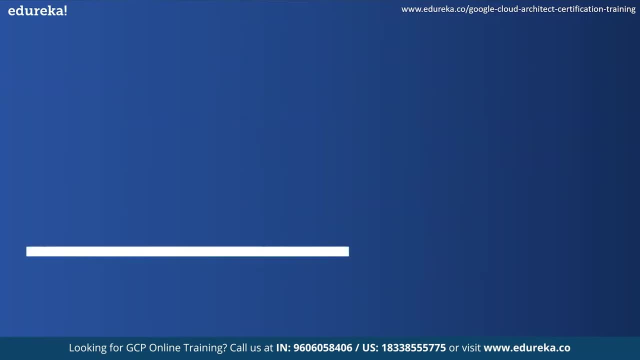 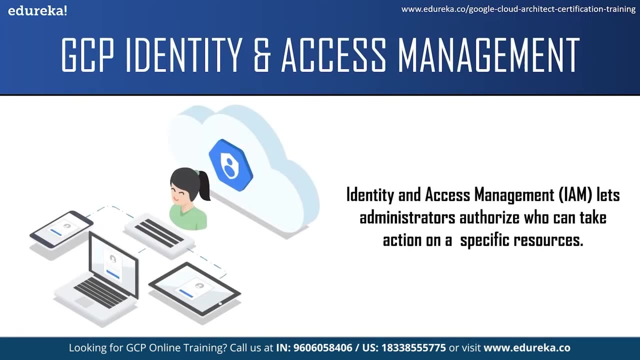 industry standard to reduce the common web application vulnerabilities and help provide protection from various web attacks. So this was about Cloud Armor. Let us move on to the next topic and talk about identity and access management. Identity and access management: that's administrator authorized who can take action on a specific resources which will help. 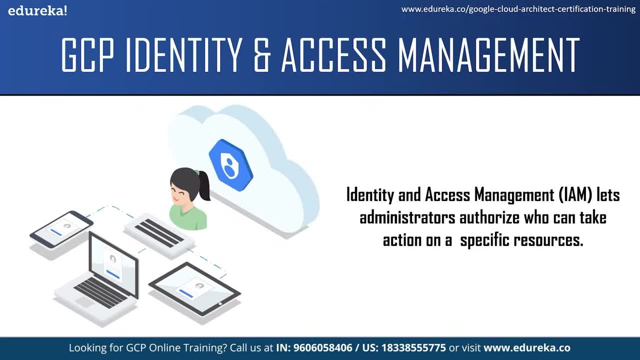 you have full control and visibility to manage your Google Cloud resources centrally. IAM provides tools to manage resource permissions with minimum confusion and high automation. You can map job function within your companies to groups and roles so that the user gets access only to what they need. 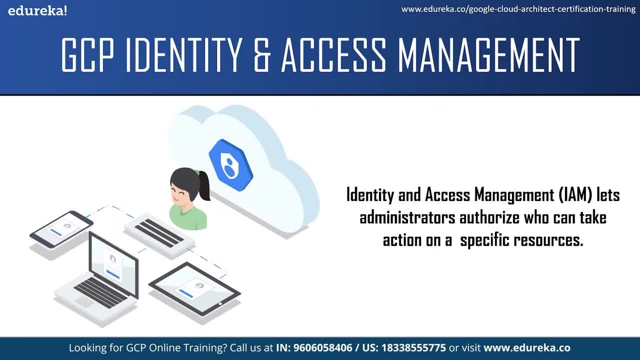 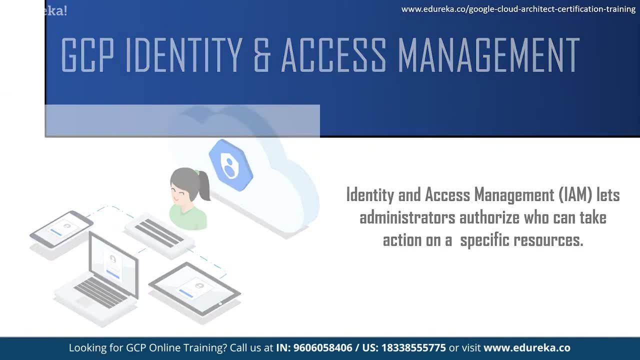 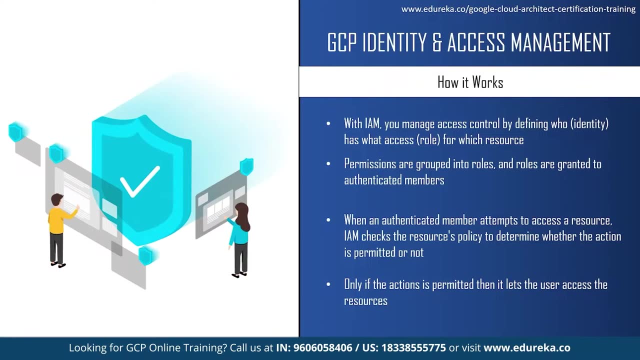 to get the job done and the admins can easily grant default permission to enter group Of users. So this was the definition of identity and access management in GCP. Let us understand. How does it work. with identity and access management, You can manage access control by defining who has what access. 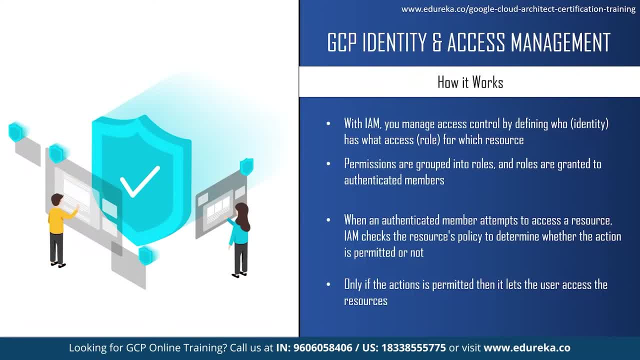 for which resources? now resources are nothing but your compute engine virtual machine instances or your Google Kubernetes engine clusters, your cloud storage bucket and so on. in IAM, permission to access a resource is not granted directly to the end user. instead, Permission of group into roles and rules are granted to. 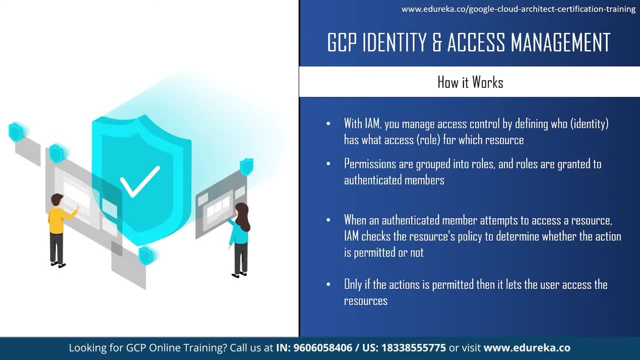 authenticated members. Now, an IAM policy defines and enforces what roles are granted to which members, and this policy is attached to a resource. So when an authenticated member attempts to access a resource, I am checks the resource policy to determine whether the action is permitted or not. 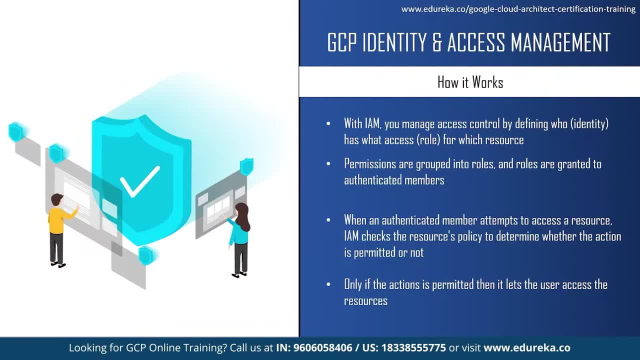 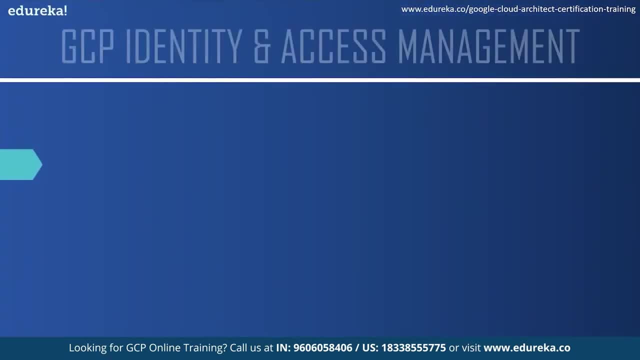 So only the action is permitted. then it lets the user access the resources. So I guess you have some idea about how this cloud identity and access management works. Now let us look at some of the features of IAM. The first feature is smart access control, actually permission. 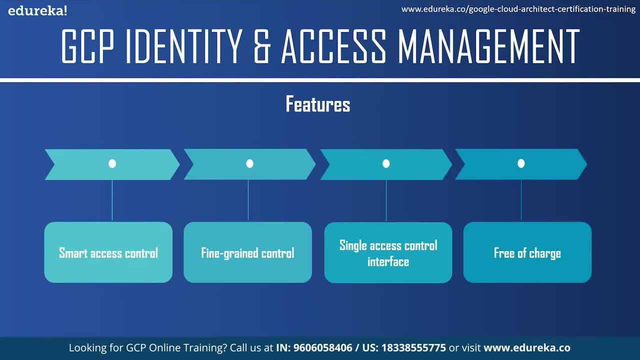 management can be a time-consuming task. So Google I am provides recommender, which helps admin remove unwanted access to Google Cloud resources for using machine learning to make smart access control recommendations. with recommender, security teams can automatically detect overly permissive access and make them right based on the similar. 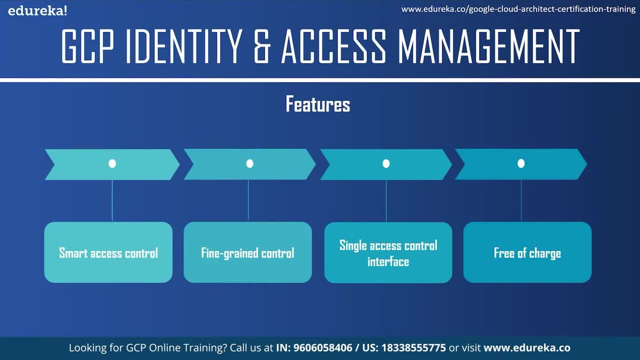 users in the organization and their access. The next feature is fine-grained control, which means you can set I am policy at any level in the resources hierarchy. It can be either in the organization level or the folder level, the project level or the resources level. I am enables. 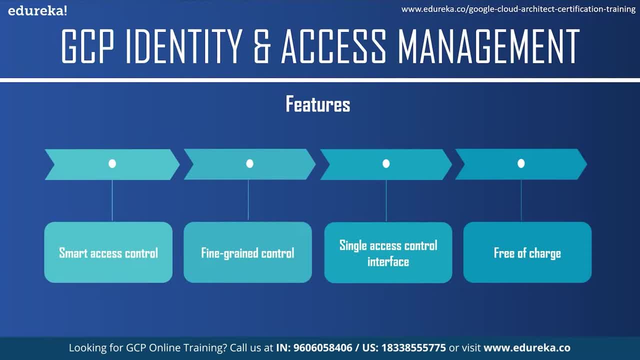 you to grant access to crowd resources at a fine-grained levels. You can create more granular access control policies to resources based on attributes like device security, status, IP addresses, resource types and date and time. moving on to next feature, Which is single access control interface. 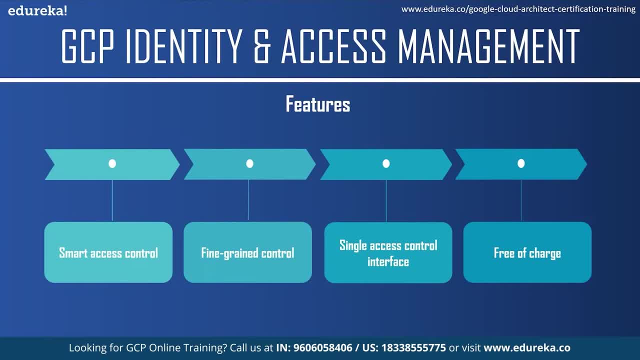 Now what this means is: I am provides a simple and consistent access control interface for all the Google Cloud Services, So you can just learn one access control interface and apply that knowledge to all the Google Cloud resources. The last feature is it is free of charge. 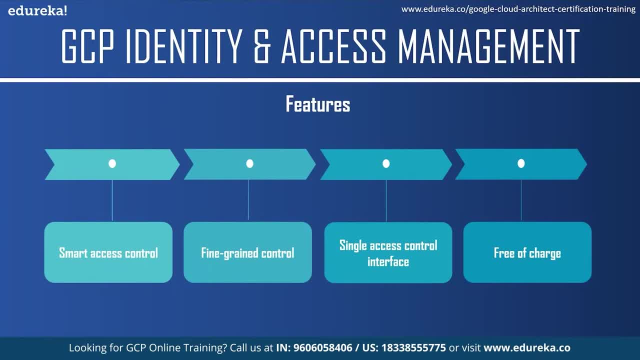 Now I would say this is more of a benefit. Google Cloud identity and access management is offered at no additional charge for all the Google Cloud customers, So you will be charged only for the use of other Google Cloud services. not I am. this was about GCP identity and access. 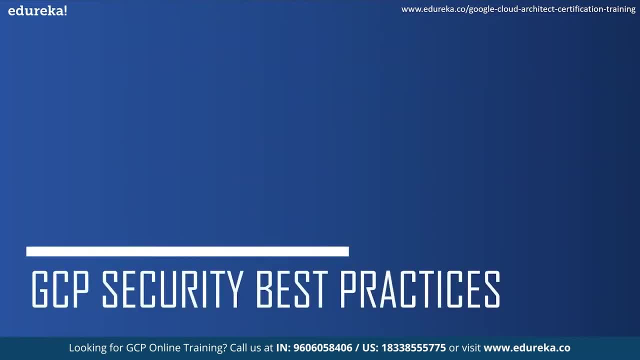 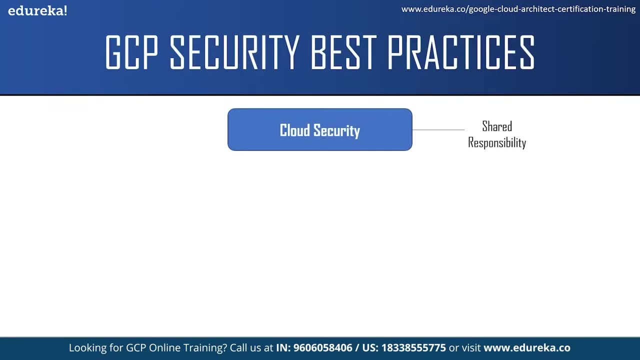 management. Let us move on to a final topic and see what are the best GCP security practices. now, before we dive into the best practices, I want you to know that cloud security is a shared responsibility, which means you and your cloud service providers are both. 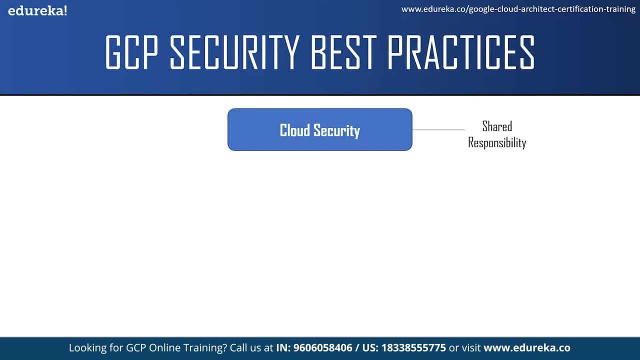 responsible for securing your resources and applications, while your cloud service provider, which is, in this case, Google Cloud, is responsible for platform security, which would include managing the physical machines and data centers, your application and data users. on the other hand, the users, that is, you- are responsible for application security, which includes setting. 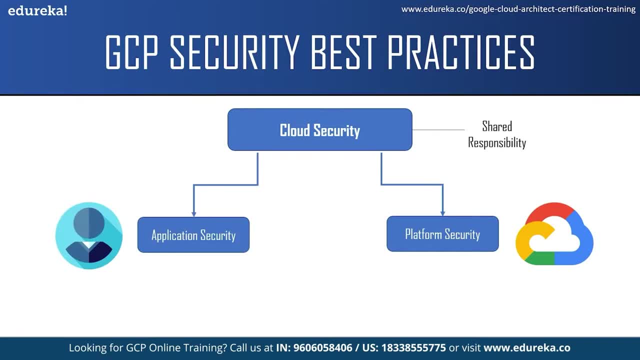 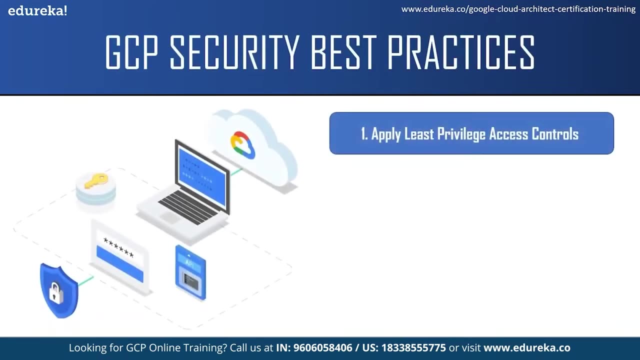 up proper authentication, authorization and identification for users in their system. next, the infrastructure security can be managed by users with the help of various tools which are provided by Google Cloud. So this is managed by you with the help of Google Cloud platform. now, talking about the best practices, the first best practices: 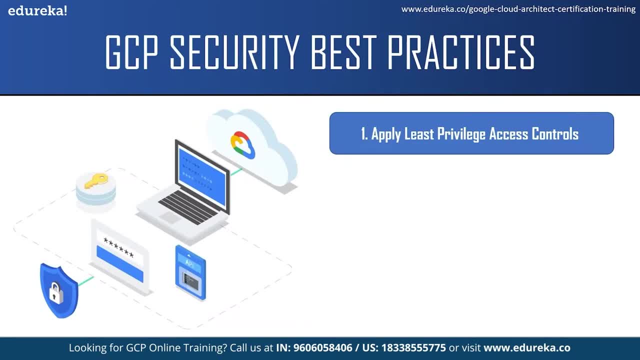 apply least privilege, access control or identity and access management. The principle of least privilege is a critical foundation element in GCP security. This concept is of only providing employees with the access to application and resources They need to properly do their jobs. only the selected users. 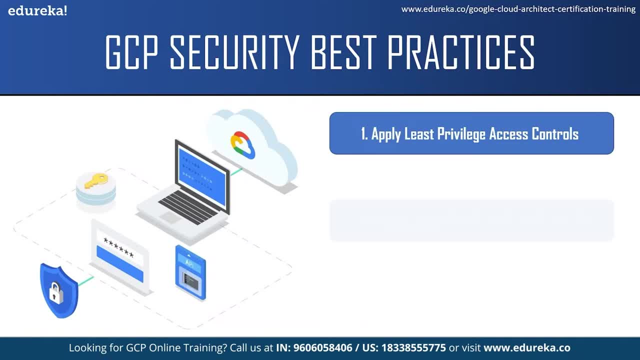 should be authorized to take action on a specific resources. The next best practices manage unrestricted traffic and firewalls. you should limit the IP ranges that you assigned to each firewall and only allow the network that need access to those resources. GCP's advanced VPC features allow you to get very granular. 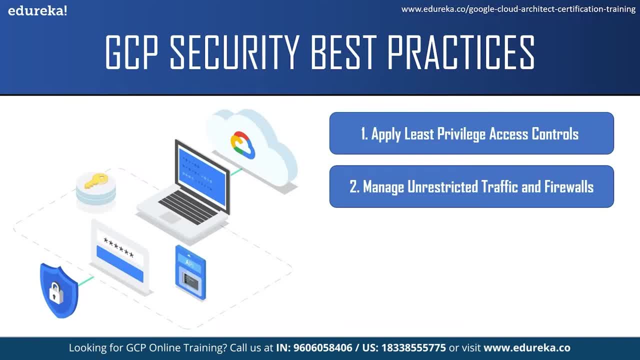 with traffic by assigning targets by tag and service accounts. The next best practices: ensuring your bucket name are unique across the whole platform. Now it is recommended to append random characters to your bucket name and not include the company's name in it. an example for your bucket name could be: product logs- b7, b12, b365, something. 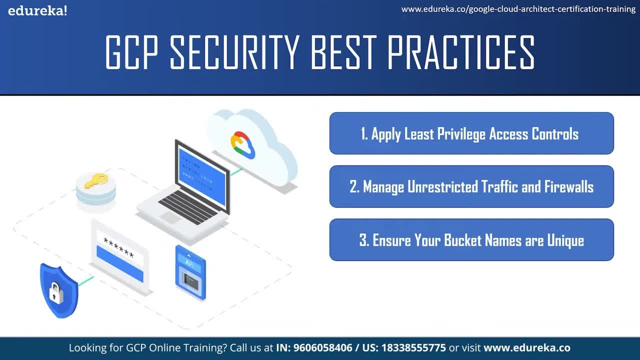 like that. This will make it harder for an attacker to locate bucket in a targeted attack. The next best practice is setting up a Google Cloud organization structure. When you first login into a Google Cloud admin console, everything will be grouped into a single organization unit, any settings. 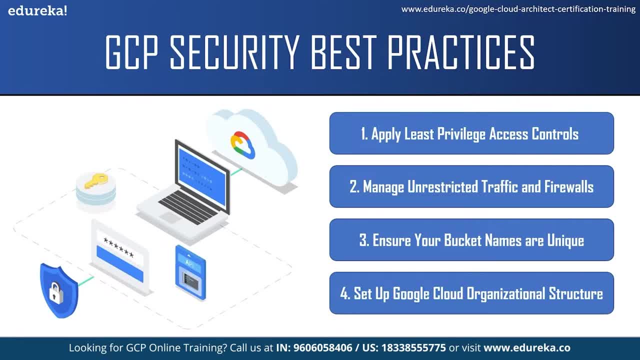 you apply to this group will apply to all the users and devices in the organizations, So you should plan out how you want to organize your units and hierarchy before diving into what will help you save time and create a more structured security strategy. Now These are some of GCP security best practices. 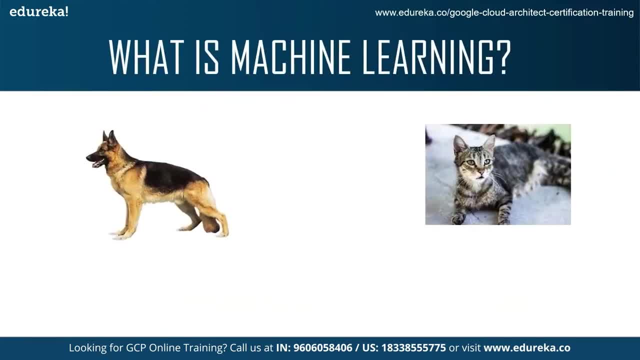 What is machine learning? So suppose you have a picture of a dog and a cat, right? So how does a computer understand the difference between which is which right? How can the computer tell which is a dog, which is a cat? so to do that you have to do certain processes. 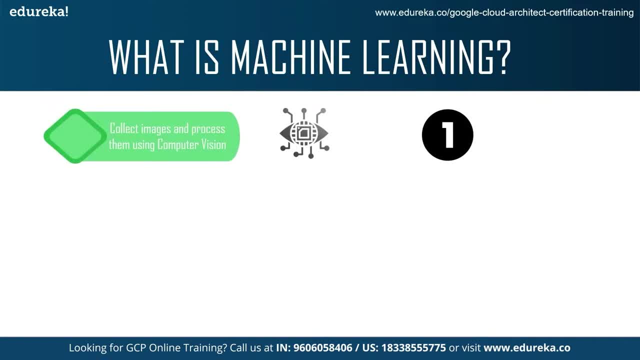 The first thing you do is you collect the images and process them using computer vision, Which is again a machine learning service that is there. So computer vision will basically understand what kind of image that you are processing, right. Then you convert all the images in the same format. 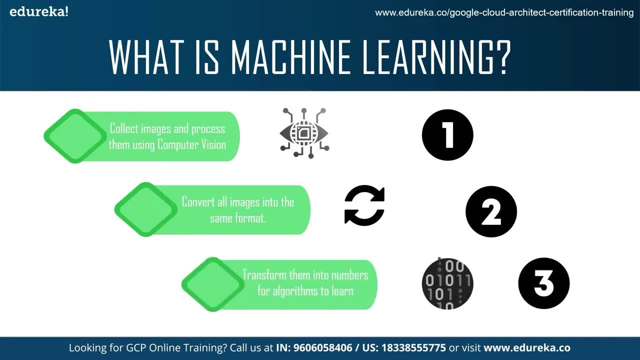 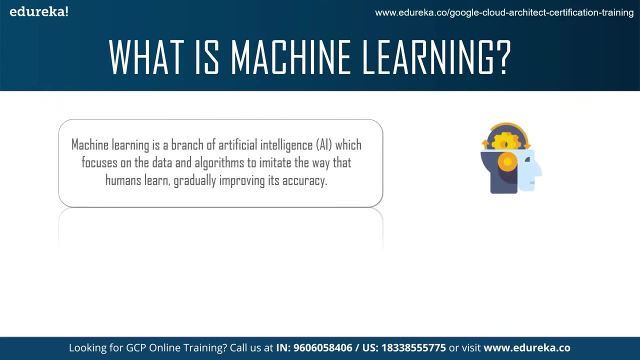 So it's easier for your computer to understand. and finally, you transform them into numbers for algorithms to learn, right. So the main aim for you to teach a computer what a certain thing is so that it can imitate you, right. So machine learning is a branch of AI which focuses on the data. 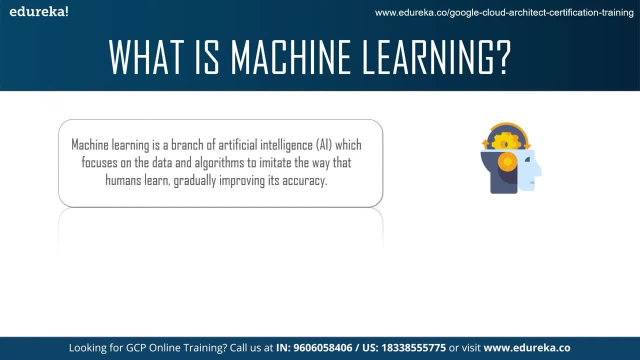 and algorithms to imitate the way that humans learn, gradually improving the accuracy right. So machine learning is always data driven and the main aim is to imitate human learning techniques as best as possible. and there is the opportunity for continuous improvement for the accuracy right. 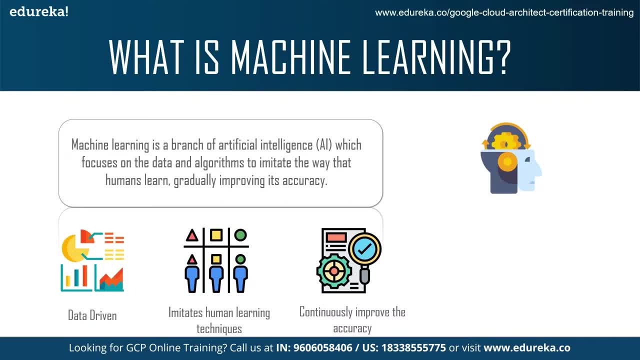 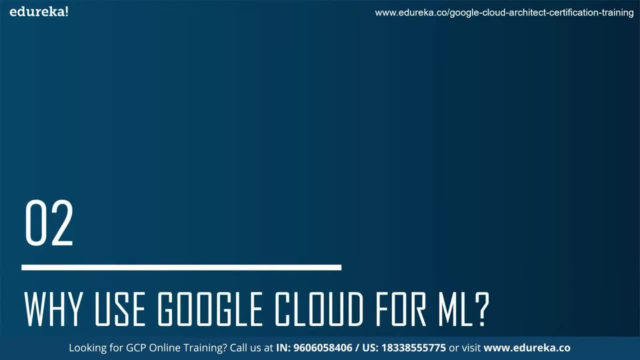 So it is always possible to create a perfectly copying model. So this is what machine learning is. Then we talk about why use Google Cloud for machine learning. So the basic reason why people use Google Cloud for machine learning is because it improves efficiency is. 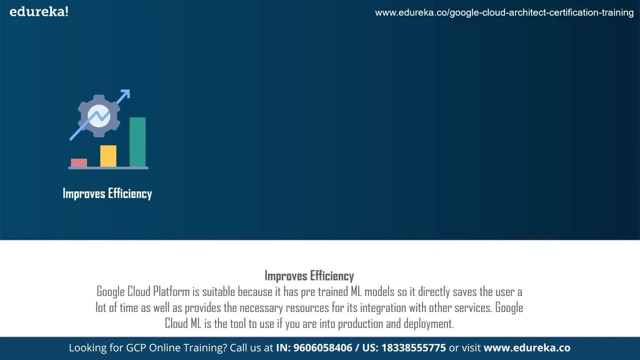 suitable because it has pre-trained models right, So it directly saves the user a lot of time, as well as provide necessary resources required for the integration of the model with other services. So Google Cloud ML is one of these tools that is used for production and deployment of machine learning models. 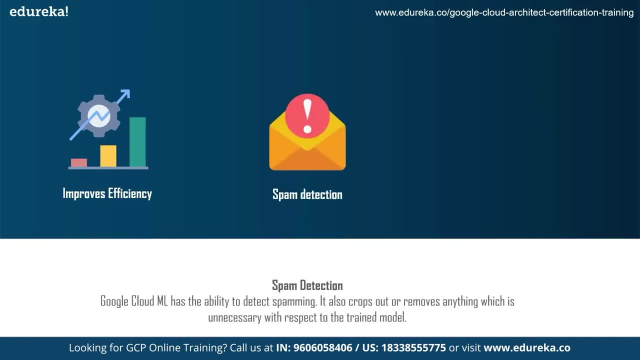 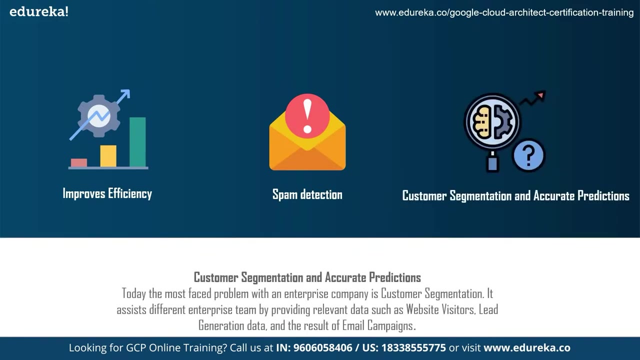 Then we talk about spam detection. Now, when it comes to spam detection, we talk about the fact that Google Cloud has the ability To detect spamming right, So it crops out or removes anything which is unnecessary with respect to the trained model. Then we talk about customer segmentation and accurate predictions. 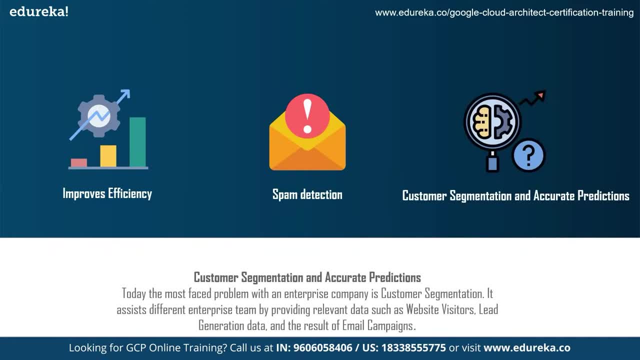 So the most faced problem today that we have is the enterprise company in customer segmentation. So different enterprise teams provide relevant data, such as website lead generation and all of that, and the result is basically a big segmentation of what people want, And that is how you divide customer based on their needs. 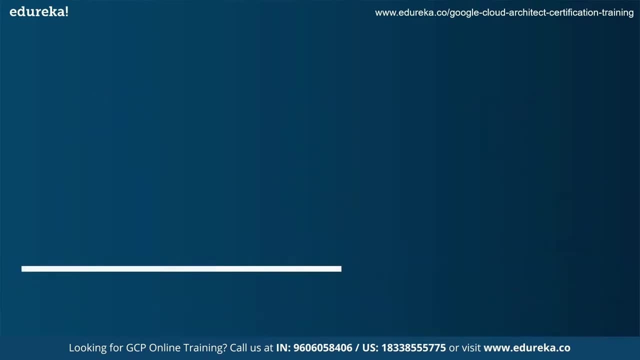 So that's what customer segmentation is all about. Then we talk about the different services that Google Cloud machine learning has. So, of the many services that Google Cloud ML machine learning has, we're going to discuss a few of them here. The first one we talk about is your Cloud Auto ML. 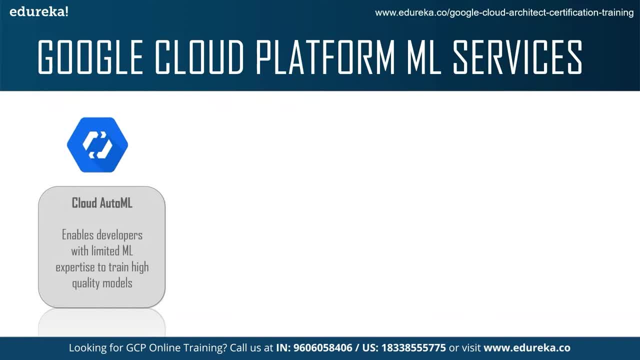 Now the Cloud Auto ML will basically enable developers with limited ML expertise to train high quality models, followed by we talk about the Google Cloud text-to-speech. So text-to-speech or speech-to-text is another service which basically enables developers to generate human-like speech. 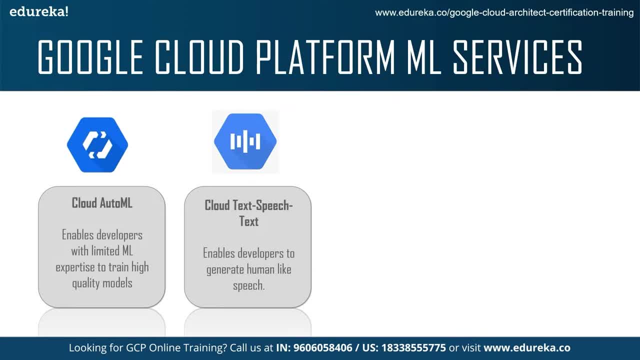 A very good example is your Google Translate. So when you basically give a certain input, let's say type in a certain word, Google Translate will say that word in a certain human-like voice format. So basically, for a certain given text you will get a certain voice. 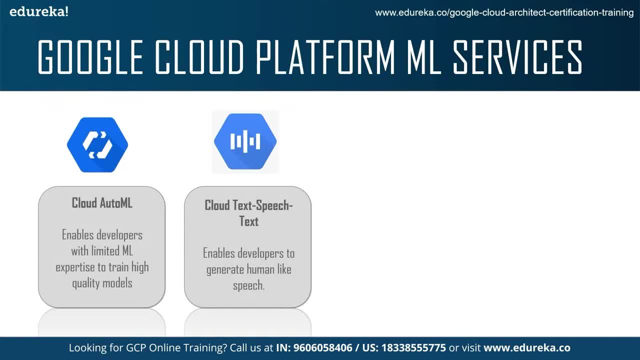 output or for a certain voice output, You'll get a certain text. That is what Google text-to-speech does, and the aim is to generate as much as human-like voices as possible. right Next up, we have the Cloud Vision API. Now, the Cloud Vision API allows developers to easily integrate image. 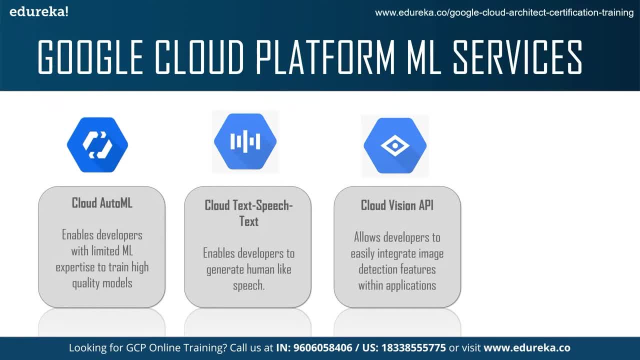 detection features within applications, For example, let's say, the optical character recognition. Optical character recognition is something which helps you detect text in images. So if there is, let's say if there's- an image and it says No parking, so you will. Google Cloud Vision will basically help you. 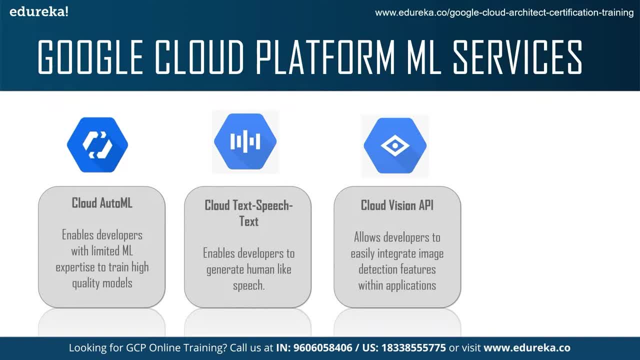 detect that text and print out. no parking over there because of its capabilities for optical character recognition. Then we talk about the natural language processing API. So the cloud natural language API is an interface to several other NLP models which are working on bigger data sets right. 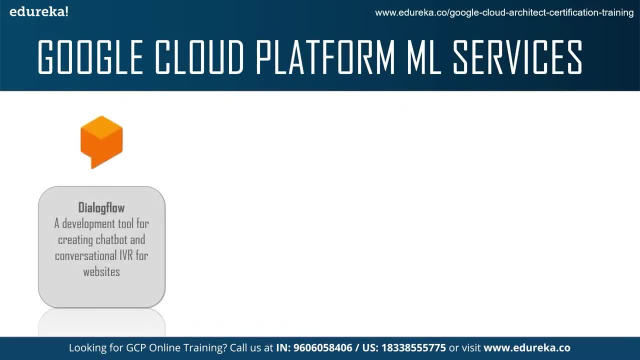 Then we talk about dialogue flow. So dialogue flow is basically a development tool for creating chat bots. So the main aim for creating chat bots in a website is so that you make the user interface much more interactive than it already is, And if the users of that website have concerns, they can directly. 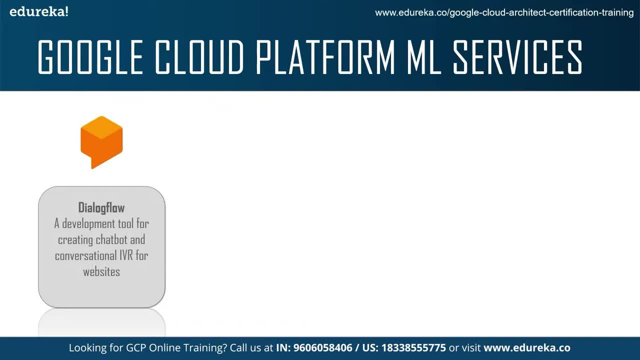 converse with the chat bot, So it makes the entire user experience much more seamless and better. Then we talk about the vertex AI, which is one of the most important Cloud ML services provided by Google Cloud. So vertex AI is basically an environment for scientists to experiment. 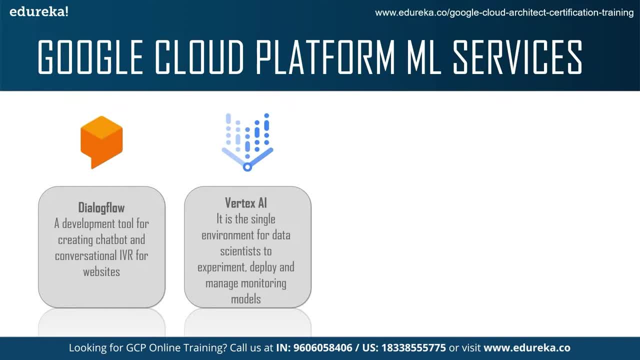 deploy And manage the models that they create. right. Then we talk about the cloud machine learning engine. Now, the cloud machine learning engine is a managed Google infrastructure for training and serving large scale models. right, So it is used mostly on larger training models, unlike AutoML. 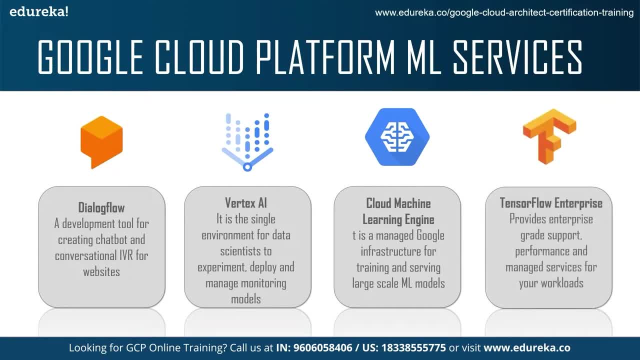 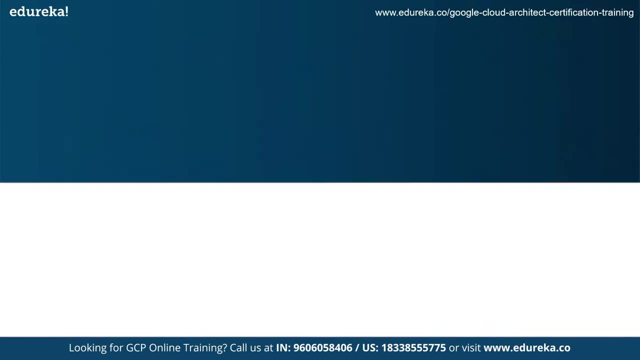 And finally, we talk about the TensorFlow Enterprise. Now TensorFlow Enterprise performs enterprise grade support, performance and manage services for your workloads, Right? So this is basically the services that Google Cloud provides. We'll talk about some more a bit later. So next up, we talk about Google Cloud machine learning features. 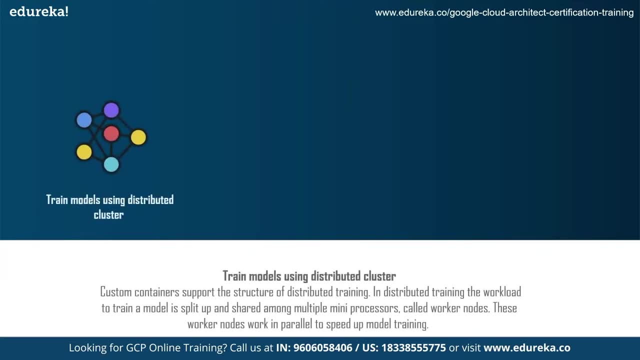 The some of the features that Google Cloud machine learning offers us are the capability to train models using distributed clusters, And what this means is that a distributed training cluster will have the workload to train a model, which is split up into different processes- right, So these small processes which take up a part of the workload are called. 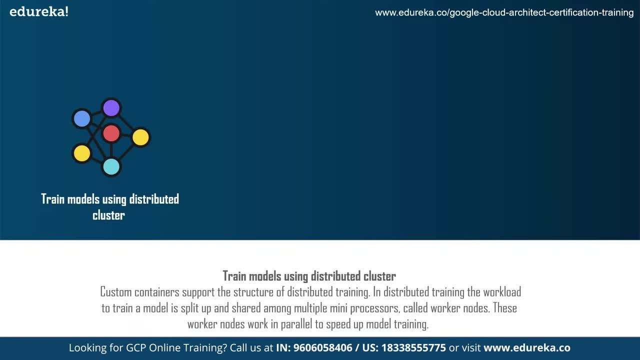 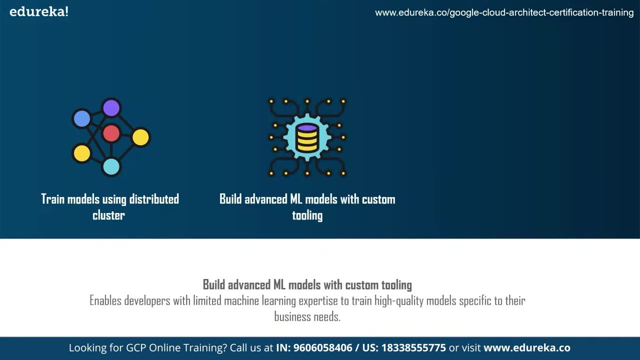 worker nodes, And these worker nodes work in parallel so as to speed up the process of model training. right Next up, we talk about the fact that Google Cloud ML allows you to build ML models with custom tooling. Now, what this means is that it enables developers with limited machine 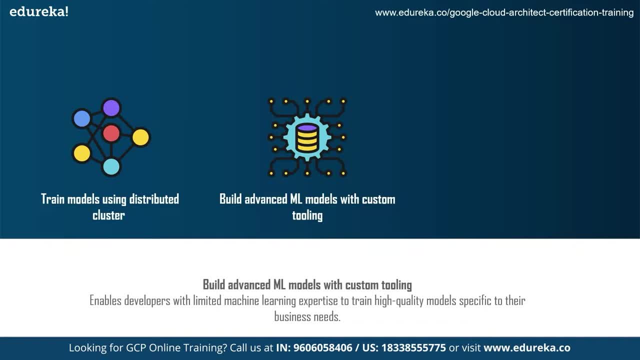 learning expertise to train high quality models specific to their business needs. And even if you aren't really not someone who is into AI, it will help you build high quality trained models with ease right. And finally, we talk about the enterprise-level compute infrastructure. 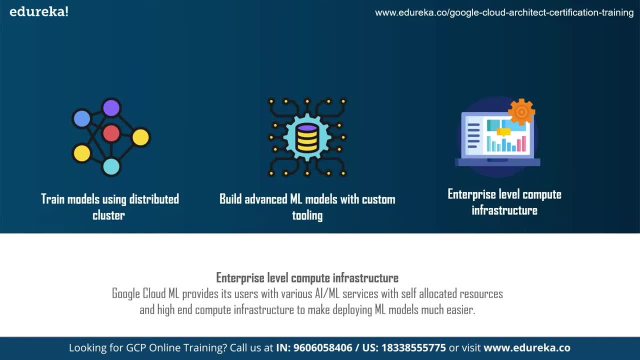 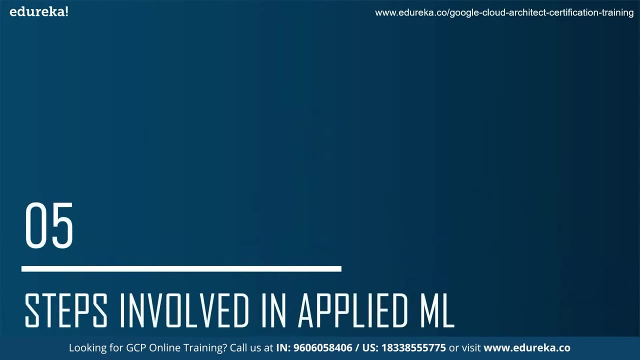 that Google Cloud machine learning provides, And this is basically something where you can see that the ML services have self-allocated resources and high-end compute infrastructure to make the deployment of the model much more easier. right, Then we talk about the steps involved in applied machine learning. 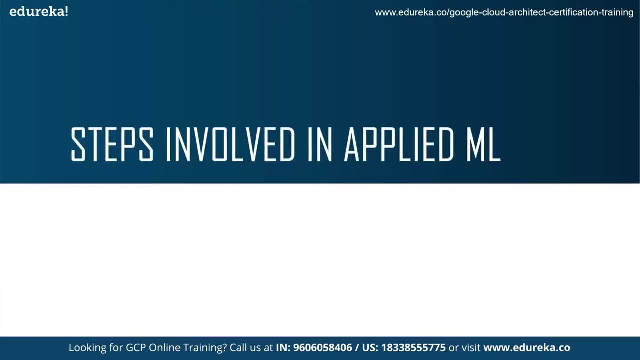 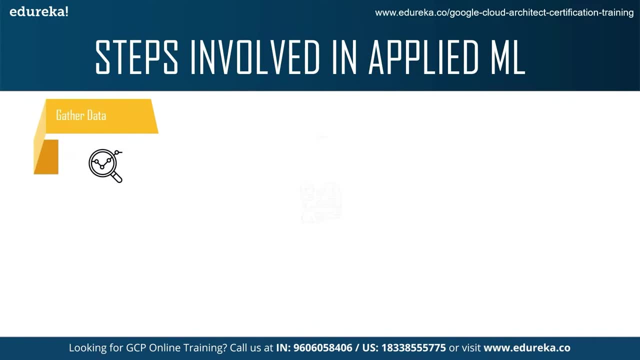 So let's suppose you want to train your own Machine learning model. What do you do? The first thing you do is you gather the data that you need to feed your model right, And after you gather the data, you basically structure it in such a way. 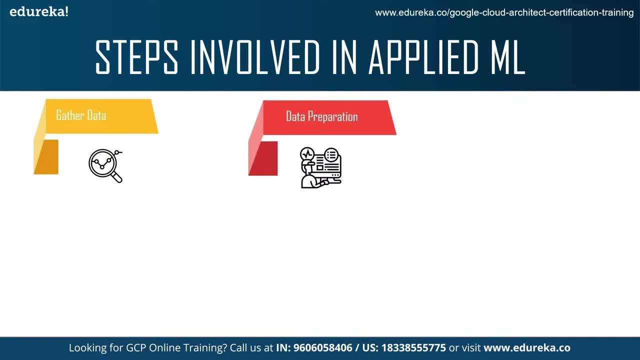 so that it's easier for your model to understand. So you prepare it. The next thing, and one of the most important things, is choosing a model for your deployment- right Model that you can train. So what you have to do here after this is evaluate the different. 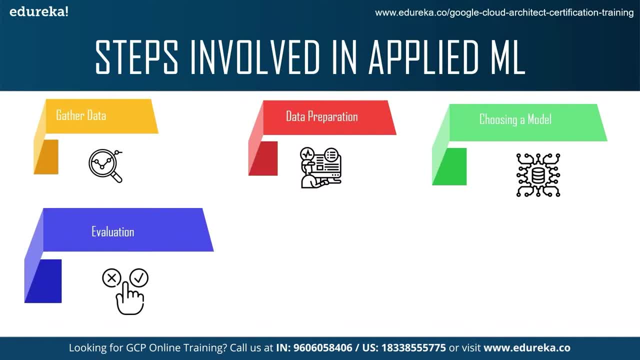 configurations that are available and choose what is best for your model and what you want according to your business needs. After that, you go to parameter tuning, where you can again fine-tune your configurations for your model so that you get your best possible prediction, because the aim is to get the highest accuracy right. 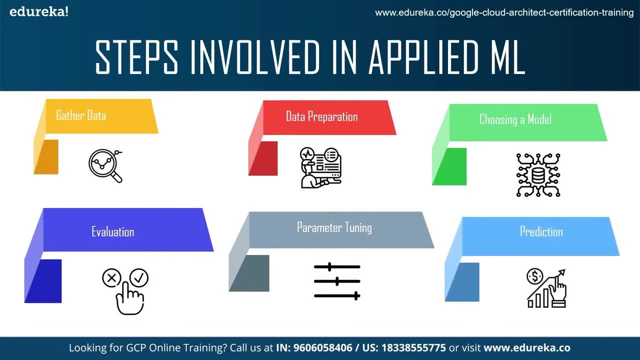 And the final part is the prediction part. So the prediction part basically tells us how accurate our machine learning model is or how well we have predicted it. Now, this is basically the higher the prediction, the better the learning capability of your model. So these are the different steps in applied ML. 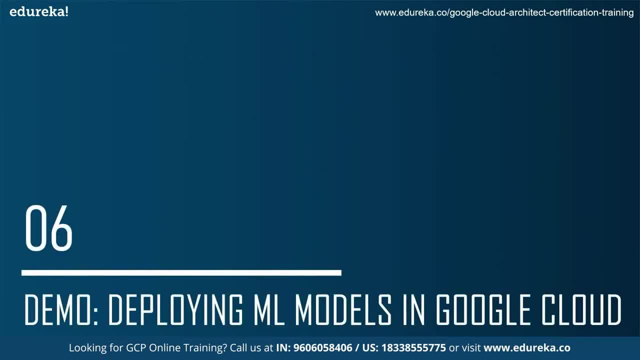 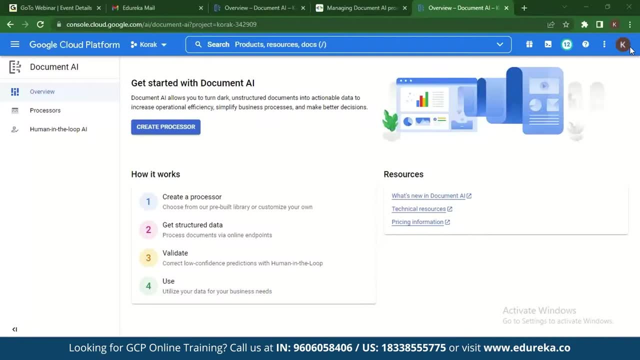 So now we come to the demo, which is managing Document AI processors using Python. So Document AI is a service provided by Google Cloud Platform, which is basically a technology that uses NLP and machine learning to train computers to simulate human review of documents. So, basically, what Document AI does is it extracts information from 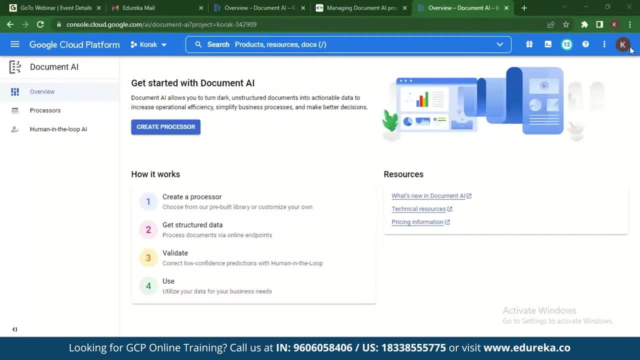 documents in digital or print form right. It is able to accurately identify text, characters and images as well, in different languages. So this is basically what Document AI is used for. Now, what we will be doing here is we will be creating processors and 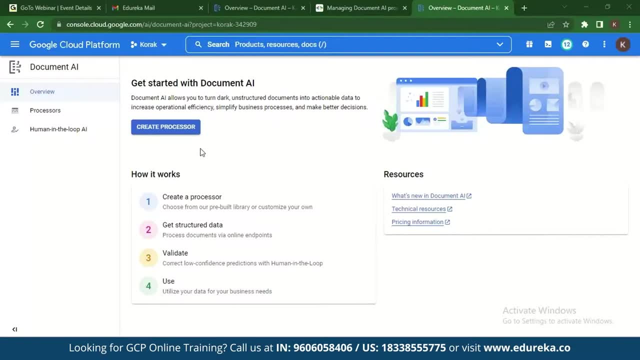 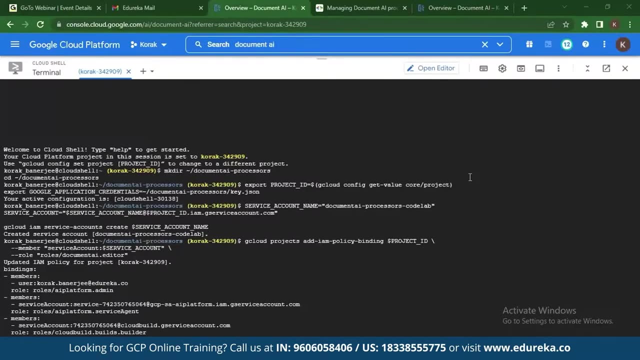 managing those processors using Python. right, Let's get started. So the first thing you need to do is make sure that you have a project created on Google Cloud Platform and on that project you have Document AI enabled. Now, once you have Document AI enabled, you can just go to the cloud shell. 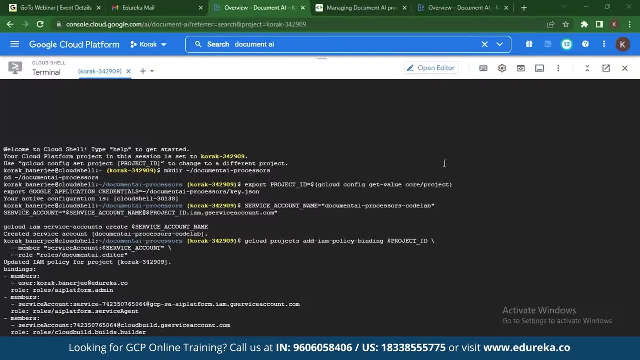 and do the following. So once you've basically enabled Document AI, you can just first thing you do is make a directory called Document Processors. So once you've made the directory, you will have to export your project ID and your Google application credentials with that as well. 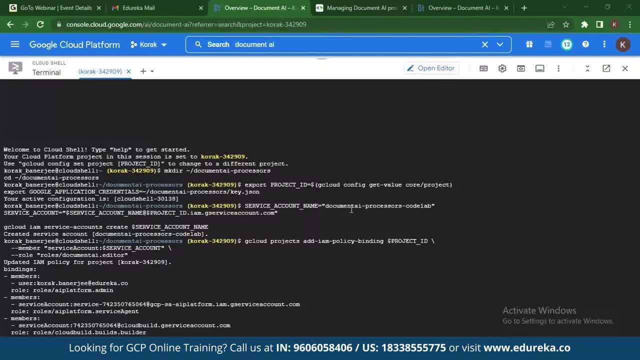 And once you've done that, make sure that you make a new service account Here. the service account's name is Document: AI processors code lab, right? So once you create the service account, you can see that the service account has been created, right here. 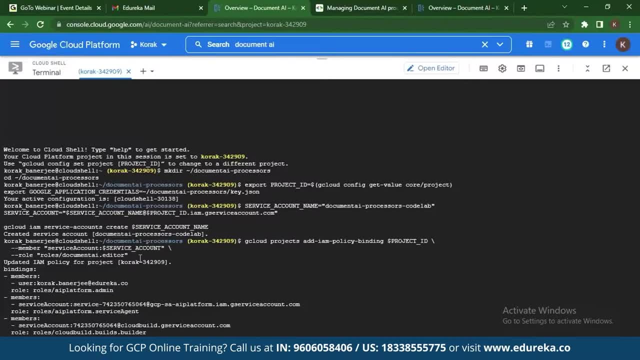 The next thing you do is you change the IAM policy and you add the editor access. So you need editor access to manage your processors that you create. So once you've done that, it will update the IAM policy And, as you can see, this is all being updated. 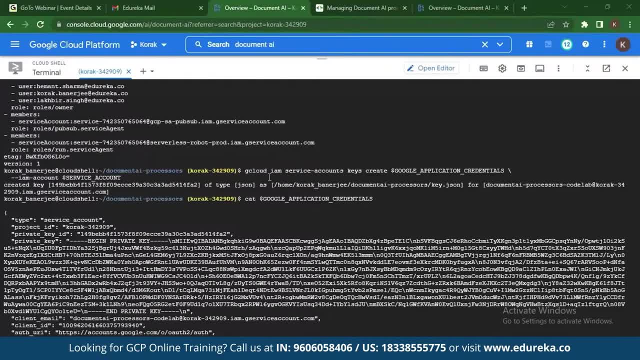 So once after you've created your service account and you've made the changes to the IAM policies so that you have entered access, you have to create and download a JSON key- Service account key Key that you have. So this is basically the service account key that I have and it's 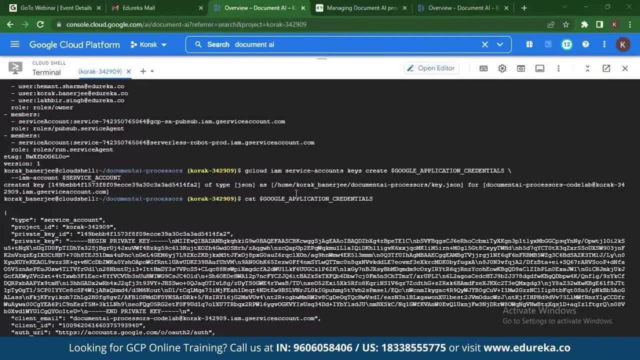 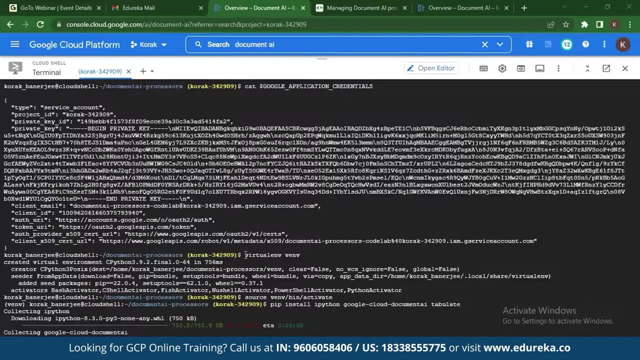 being downloaded, And after that I'm just checking for the entire path of my service account. And this is the entire path of my service account, which shows me the project ID, the private key and the public key as well. right After this, what you do is you create a virtual environment on cloud. 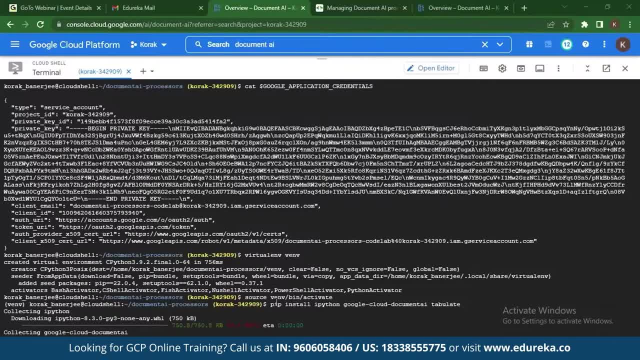 shell, And once you've created a Python virtual environment, what you need to do is that you need to activate it using source, And we've been slash activated, So now your virtual environment has been created and activated. So once you've done that, since you're using document AI, you need to 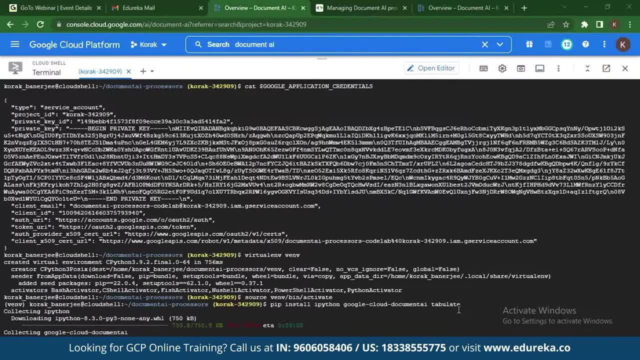 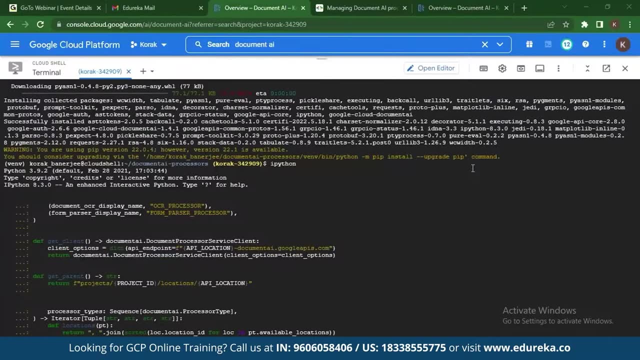 basically install this, which is the cloud document AI tablet. Now, what document AI tablet does is it basically makes your data that you have in the document look much prettier when you have to print it right. So now that you have your document AI tablet installed, what you have- 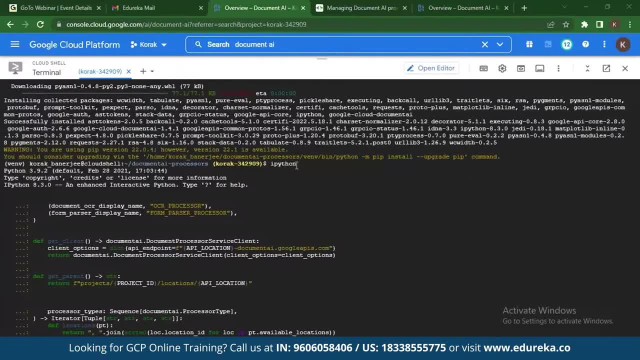 to do is create a Python session, So command IPython. now you've created a Python session, which is basically an interpreter for Python, And for that you'll have to put all your functions and all your code in this IPython file, right? 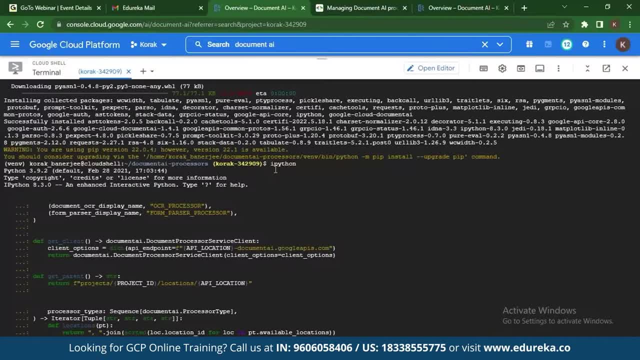 After you've basically downloaded the document AI tablet file, you'll see that it's been installed. Now what you have to do is get a Python interpreter. Now you can log into this Python interpreter by the command IPython right, After which you can just put in your functions inside that IPython file. 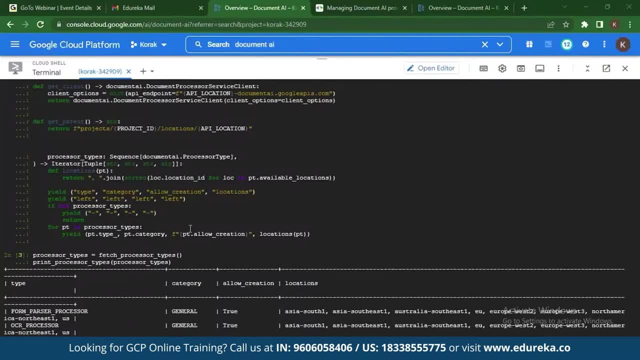 So you have the code Now. the code basically shows you the kind of processors you have and the processor type, and basically you have to print the processors that you have. So if you do that, you'll see that you'll have something like this: 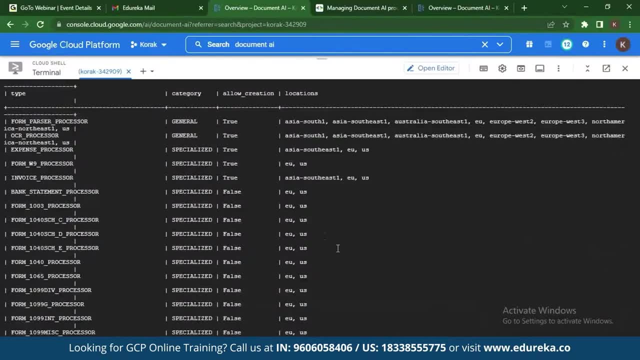 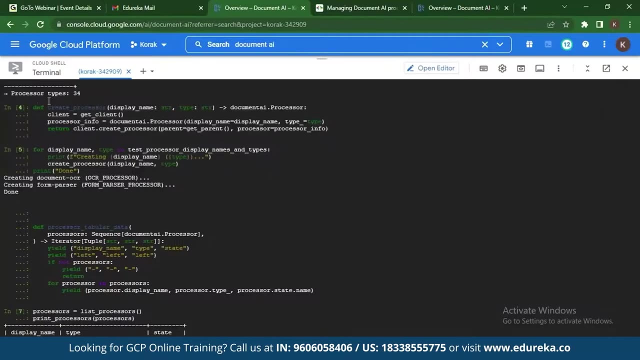 Let's go down here. As you can see, this is basically all the processors that we have, and this being shown using a tabular format, using document AI, right, So we'll try something Else out as well. Let's just see the number of processors that we have here has been typed. 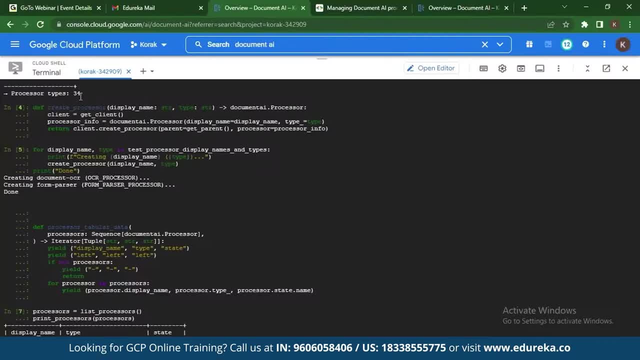 out to be 34.. Now, this is all because that we want to know the number of processors that are present. So this is basically nothing but listing the Python and processor types that you have. So these are basically the processor that was already present. 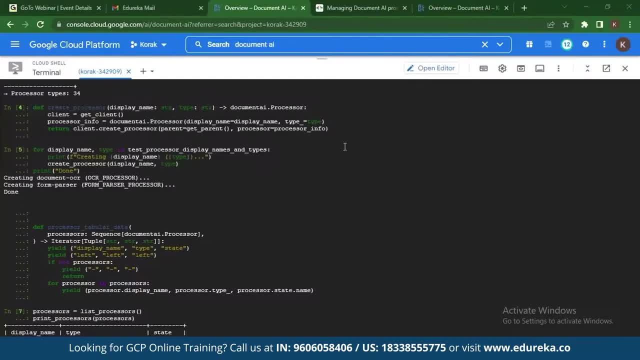 Now let's just try creating our own process and basically print that as well. So what you see here is a data frame where we're creating a processor and displaying it As well, And this is the same. So what we're doing is we're creating another data frame, which is the. 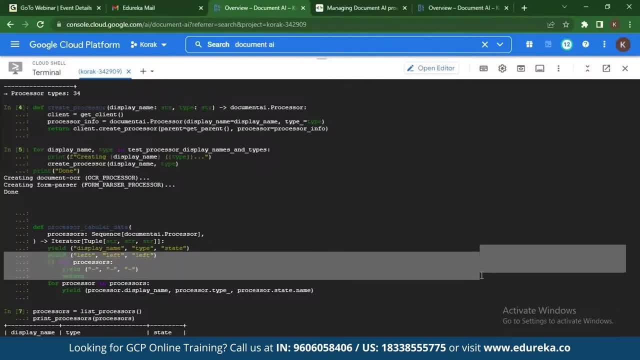 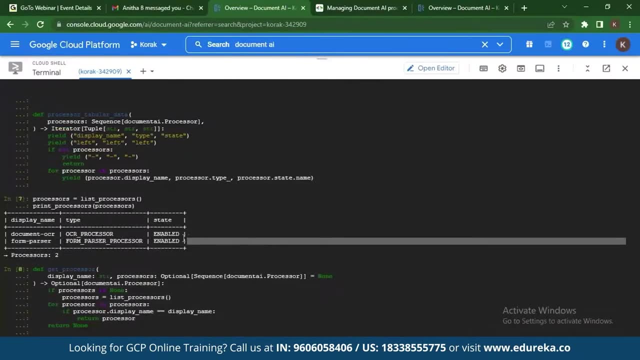 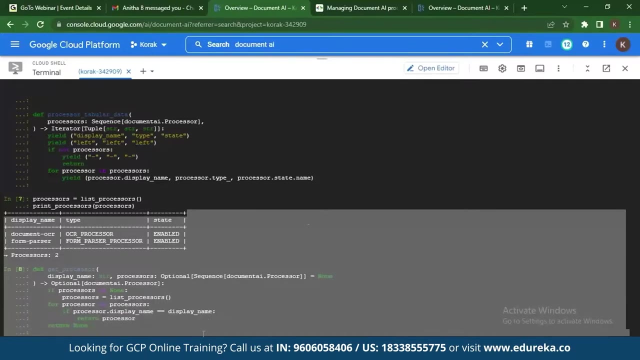 tabular data function which will show us our new processors printed in the tabular state. And if you run this command, this is what you see: that these two processors have already been created and enabled. right after this, There's another function which is basically showing us: there's another. 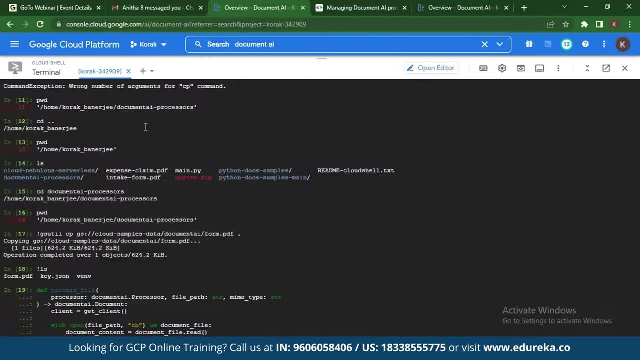 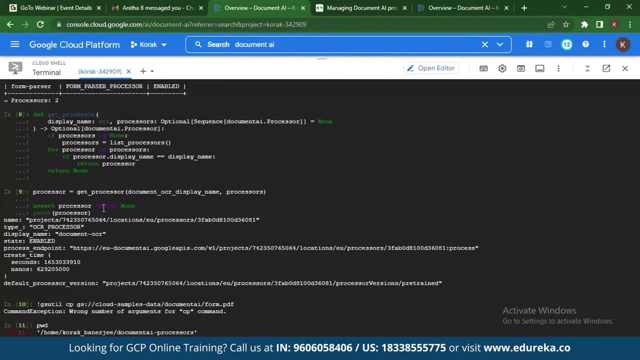 processor and we'll have to get that processor if it exists, right, So let's just go Back here. Yeah, So let's just check out if a certain processor is already there existing, For example, in this function. we'll basically go check out if the OCR. 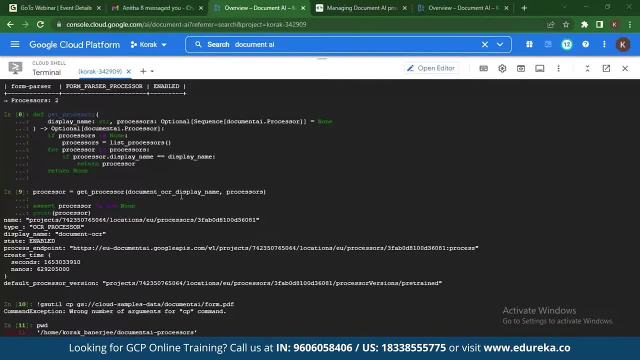 processor exists, right, And we'll have to go check it out and display the name of the processor and the OCR name as well, right? So the type of processor that we have is the OCR processor. This is a processor that we created and it's called document OCR and it's 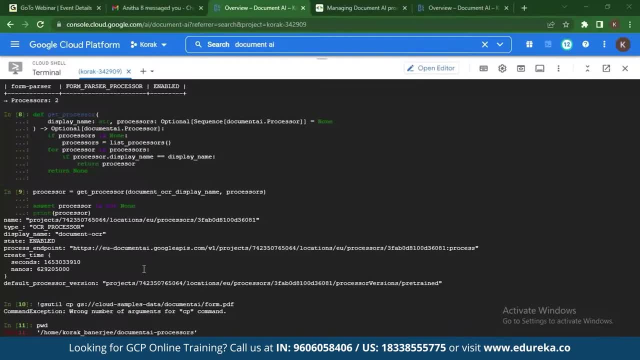 So this is a different command that you can use for getting the processors that you've created, right? So, basically, it also shows you the version of the projects that you've created and the processors that you've created as well. right? So let's try out something else now. 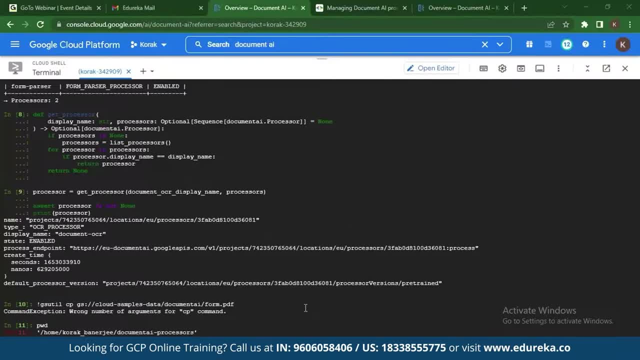 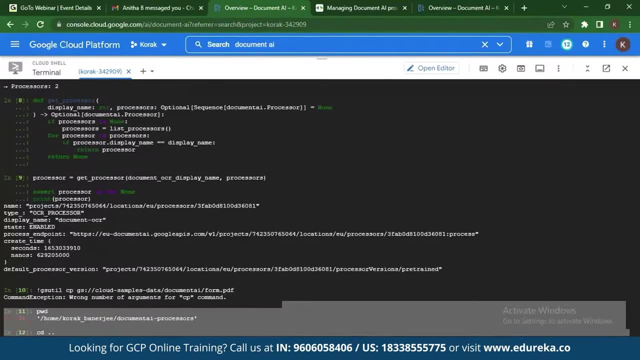 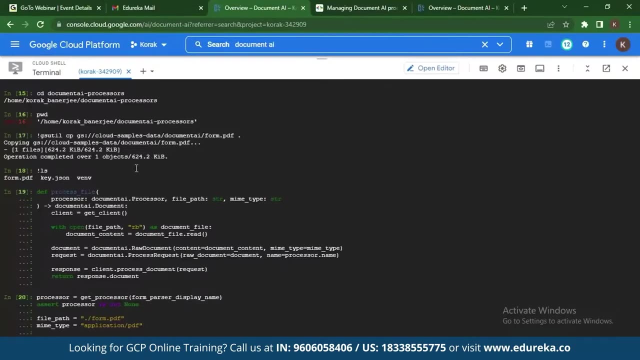 So the next thing we're going to try is we're going to try and analyze the document. in this document It's basically called form dot PDF, right? So we'll have to, just Right. So if you go here, you'll see that the form dot PDF file has been downloaded. 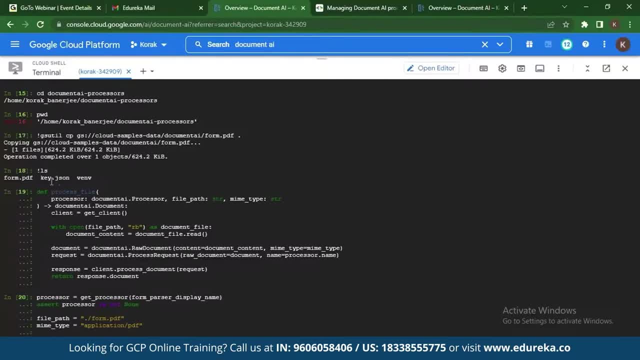 and basically, when you LS into it, you'll see the files that are there to perform dot PDF, the JSON and the python environment. right Now there's a function called process file, which will basically process your document and analyze it and print the path of the file and the document. 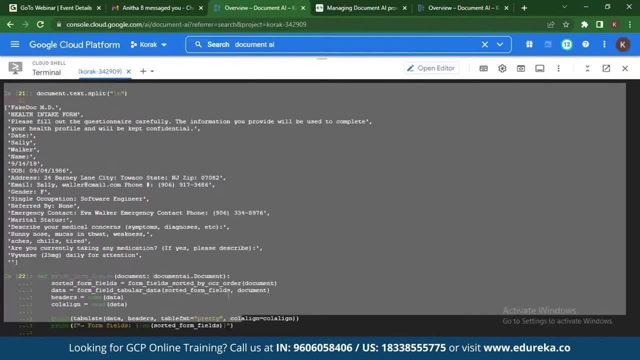 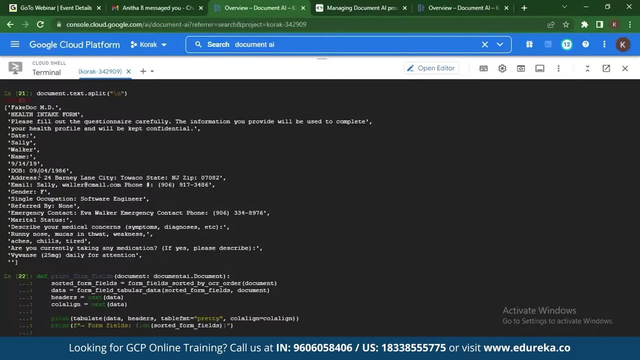 as well. So, basically, after that, what you have to do is create the file. So, once you print the file, this is what you see, that it's a health intake form and this is the data that you have in there, right? So this is not in tabular format, because we did not mention it, but you 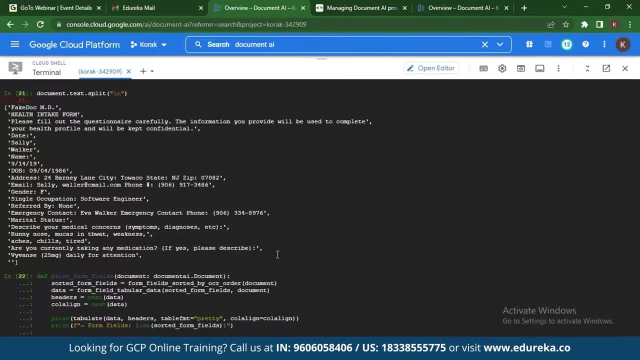 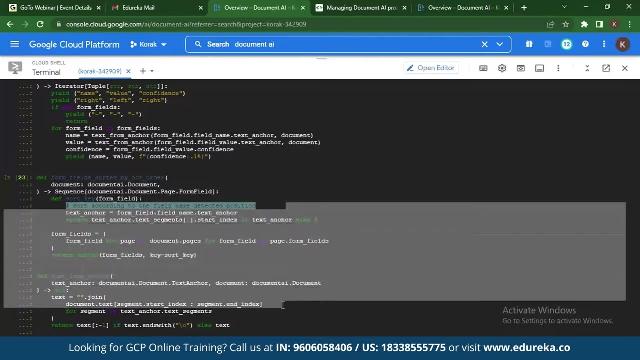 want to, you can, and after this you'll have to check out the fields in the document that you have. So do that. We have another function called print form fields. You should print the tabular data form fields and do that. So this is basically the fields that you will select, and 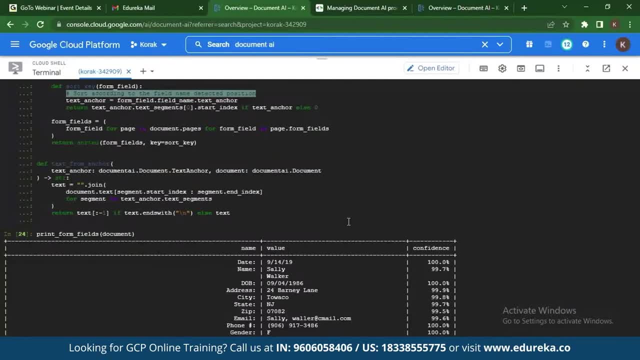 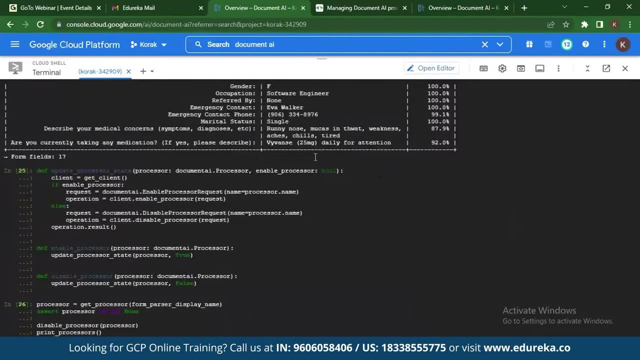 Once you select those fields that you want and print the same document, you'll see that the entire part where you wanted it to be tabulated and shown has been shown here, like this right. So there are 17 fields and this is what you have as your document. 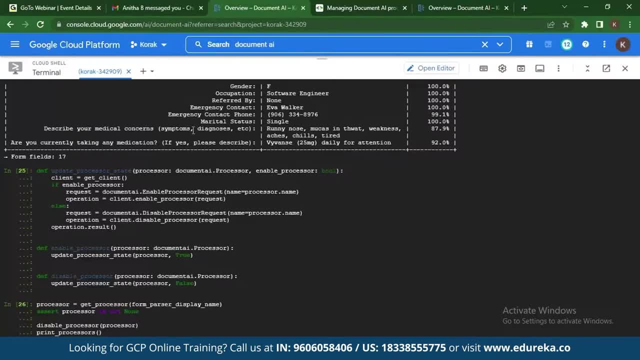 So document AI can read and show you tabular data, which is not redundant. So now you're going to update the processor state after this. now, to basically update the processor state, What you need to do is delete the processor right, So you will have to disable the processor first. 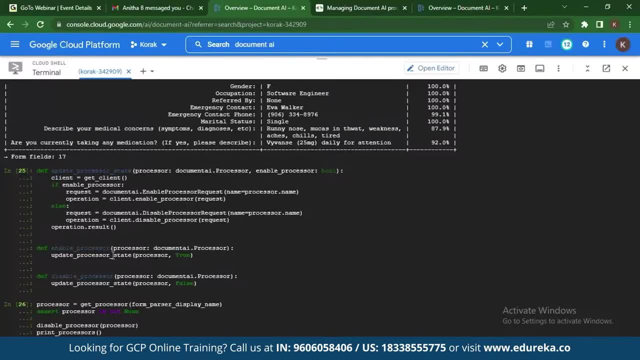 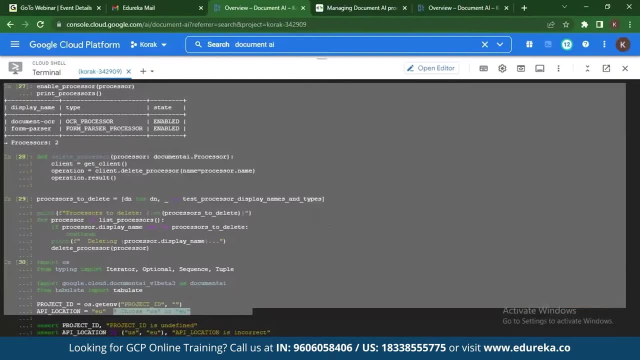 So to disable the processor. This is the function for disabling the processor and this is also a function for enabling as well. So if you want to enable it from disabling, you can check that out. What you need to do is you need to print out all the enabled processors. 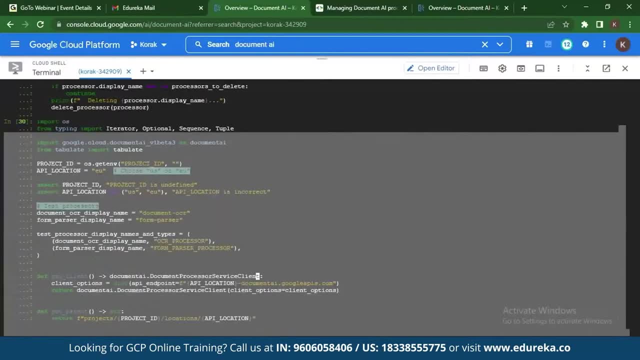 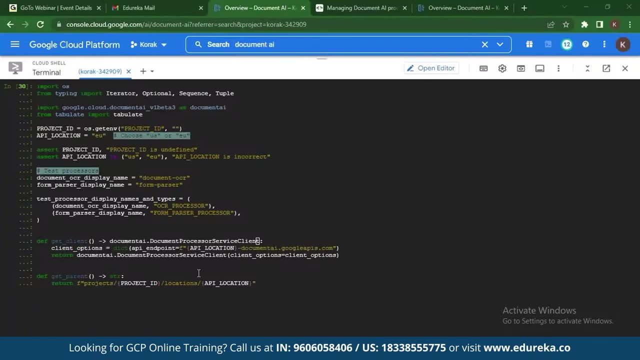 here and, once you've done, you can just delete them, because this is a function which shows you how to delete the processors that you already created. before this, We saw how to create the processor. We saw how to get fields from a certain document. 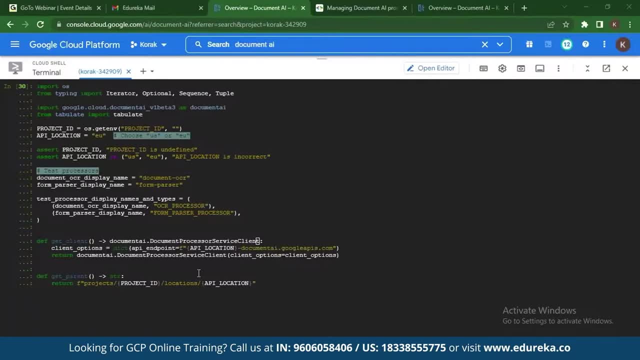 We saw how to analyze the document. We also saw how to enable and disable the processors- which is extremely important- before you delete it, right? And this final part is showing us how to basically delete them. So, once a file is deleted, we are done and you've cleaned up all the data. 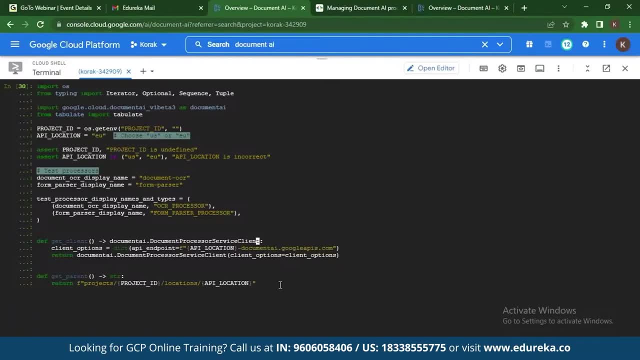 that you've already used, right? So you don't want to keep instances or processors keeping on running because you say, if you exceed the free tier limit it will basically cost you money, right? So you don't want to do that. So make sure you always delete your instances and processors, right? 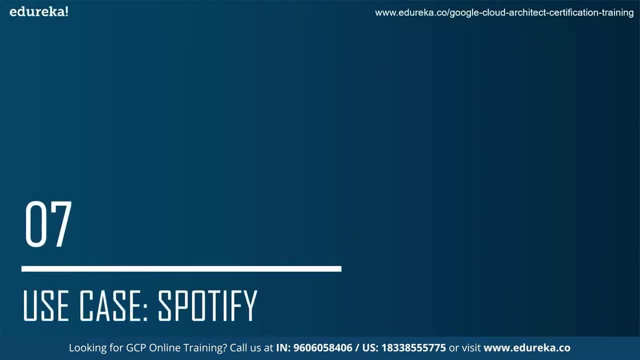 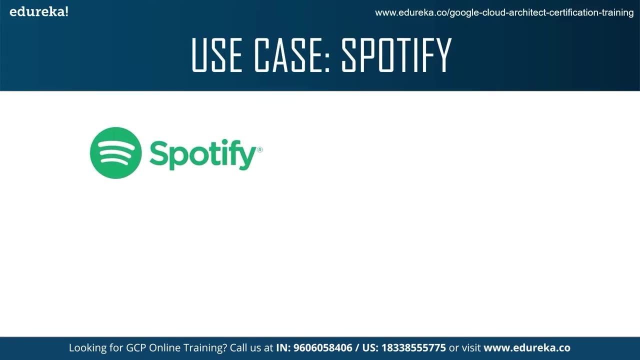 So with that, we come to the end of the demo. Finally, we come to the use case, which is Spotify. Now, Spotify is the world's leading music streaming service, all across the world, and what you can see here is that Spotify have actually turned. 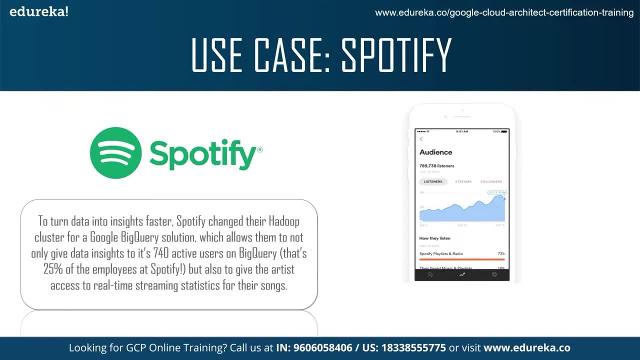 their data insights much faster. Now, how has this happened? Spotify uses their Hadoop cluster, and then they change the Hadoop cluster into a big query solution. Now, what this does is it allows you to not only give data insights as well. 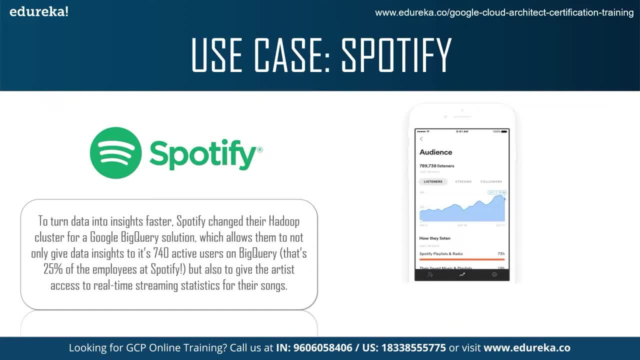 but also have around 740 active users on big query right. So that's around 25% of the employees at Spotify, which is a pretty huge percentage. So not only this, but this also gives direct and real-time insights to the artists so that they can access the live real-time streaming statistics. 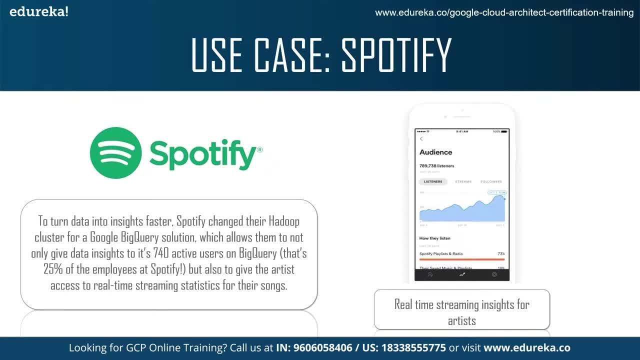 for their songs, right? So this is how Spotify has Use Google Cloud in their functionality, And this is why I think Spotify is still going to be one of the leading music streaming companies for years to come, and Google Cloud has been integrated into literally every aspect of our life. 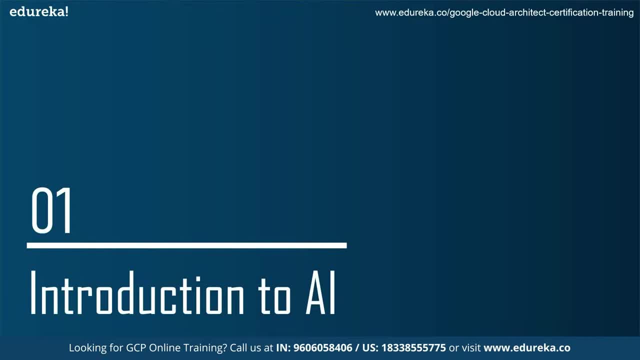 So you might have heard a lot about the term AI. There are a lot of devices in the market which are powered by AI that we use on a daily basis, So the term AI sounds very alluring, right, But what actually is AI? 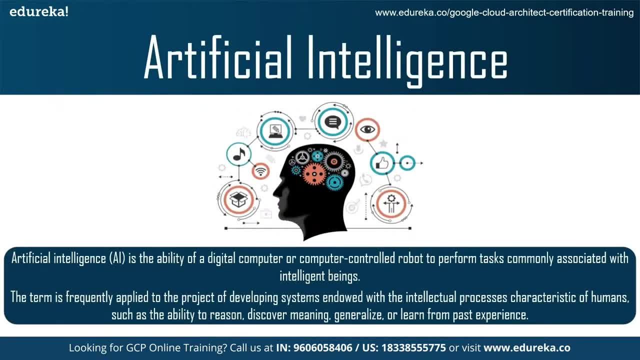 So now let's have a little introduction of it. So AI stands for artificial intelligence, which is an intelligence demonstrated by machines, unlike the natural intelligence displayed by humans and animals, which involves consciousness and emotionality. The term is frequently applied to the project of developing systems. 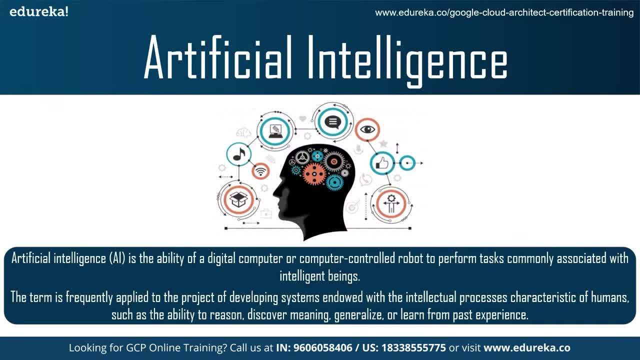 provided with intellectual processes, characteristics of humans, such as the ability to reason, discover, meaning, generalize or learn from past experience. Since the development of the digital computer in the 1940s, it has been demonstrated that computers can be programmed to carry out various complex tasks, as, for example, discovering proofs for mathematical theorems or 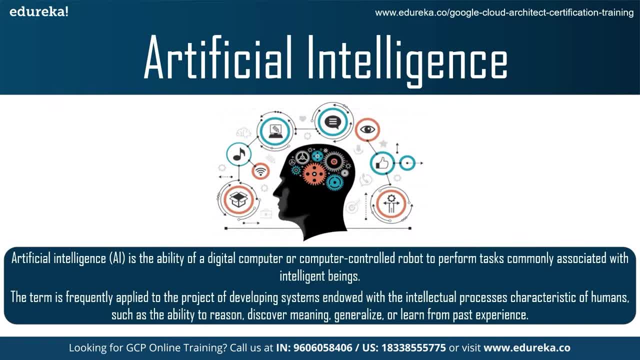 playing chess with great proficiency. Despite continuous advances in computer processing speed and memory capacity, There are yet no programs that can match human flexibility over wider domains or a task requiring everyday knowledge. On the other hand, some programs have attained the performance Level of human experts and professionals in performing certain specific 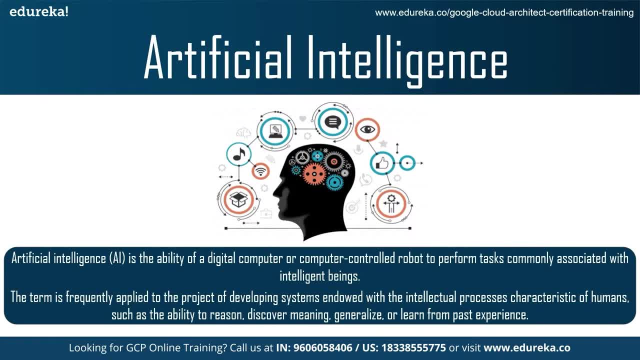 tasks, so that artificial intelligence in the limited sense is found in applications as diverse as medical diagnosis, computer search engines and voice or handwriting recognition. Now let's have a look at some of the major domains which have been eased out with the help of AI. 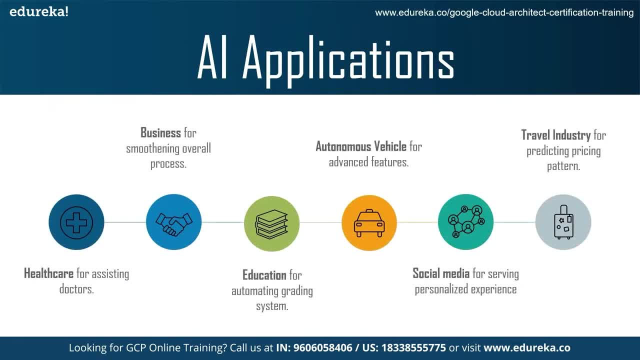 So AI and healthcare has simplified the lives of patients, doctors and hospital administrators by performing tasks that are typically done by humans, but in less time and at a fraction of the time. The cost in the business domain, If you see, in the present time, at least 30% of the companies globally use 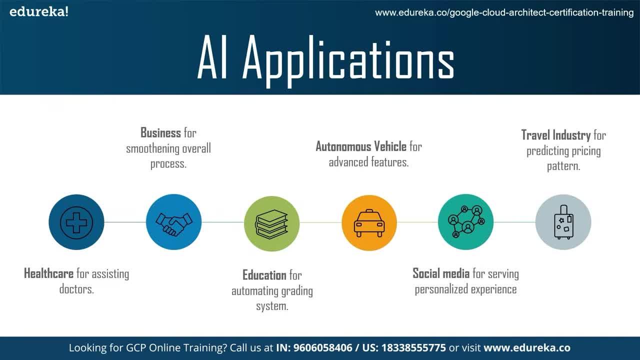 AI in at least one fragment of their sales processes. today, businesses across the globe are leveraging artificial intelligence to optimize their process and reap higher revenues and profits. AI and education is used to develop smart school scheduling tools for scheduling individual student timetables using machine learning, which 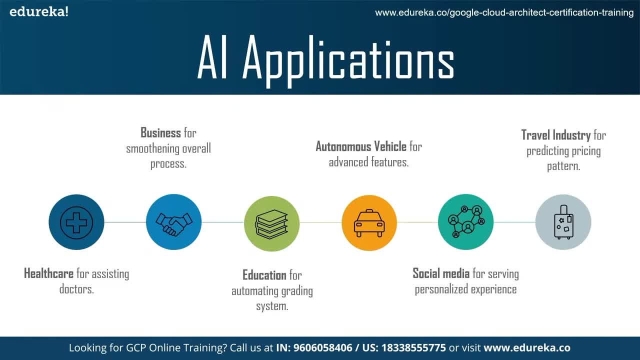 is an AI based assessment process helps in many ways, like it helps in faster grading, Testing and performance monitoring of the students quickly with board accuracy. Now moving on to AI in autonomous vehicle. So with every car manufacturer and their mother racing to develop artificial intelligence and self-driving technologies. 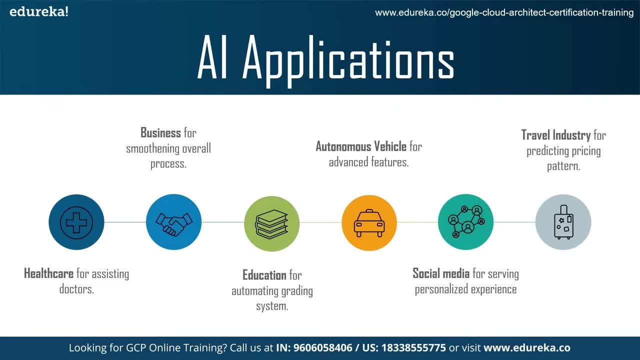 There are also a few of tech companies and startups with the same purpose, though many believe personal autonomous vehicles are the future, but there are multiple ways in which AI and machine learning are being implemented in how vehicles are built and how they operate on the road. 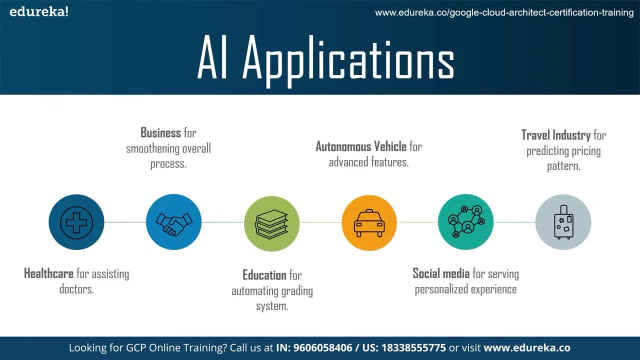 So, if you see, in AI powered social listening tool can deliver insights from your brand's social media profiles and audience. This often involves using the power of AI to analyze social data at scale, understand what's being said in them, then extracting insights based on that information. 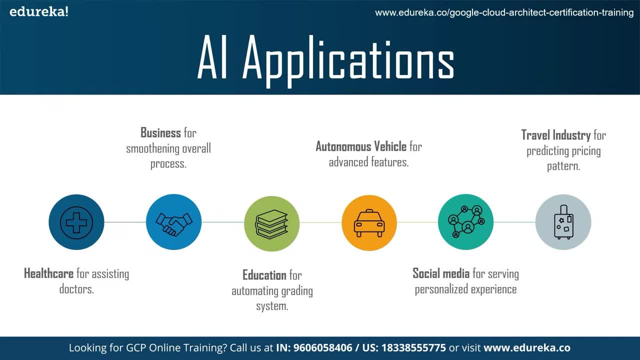 So now moving on to the last industry, that is, Trevor industry. So, if you see, like most hotels and results rely heavily on delivering excellent customer service to build their reputation, and AI technology can assist with this in a variety of ways. For example, artificial intelligence can be used to improve personalization. 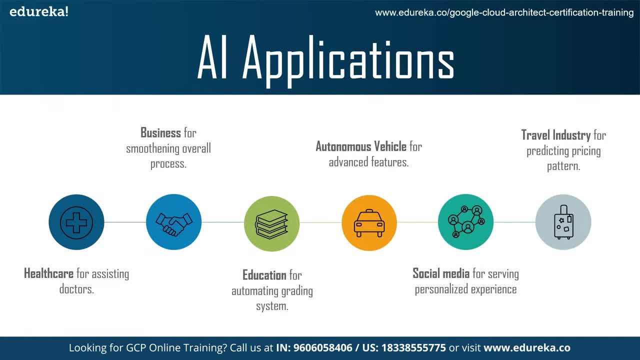 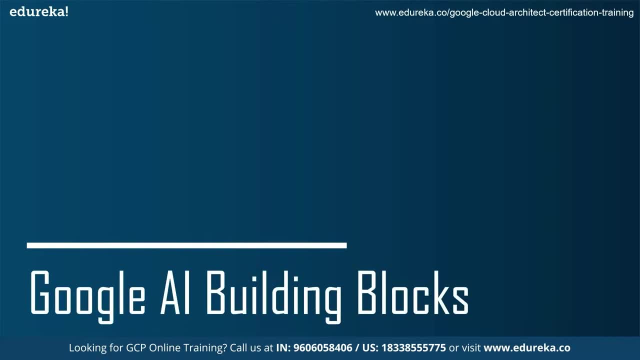 dealer recommendations and guarantee fast response times given in the absence of stuff. Now let's take a look at some building blocks of AI in Google Cloud. So they have four major building blocks. first one is site, second is language, then conversation and structured data. 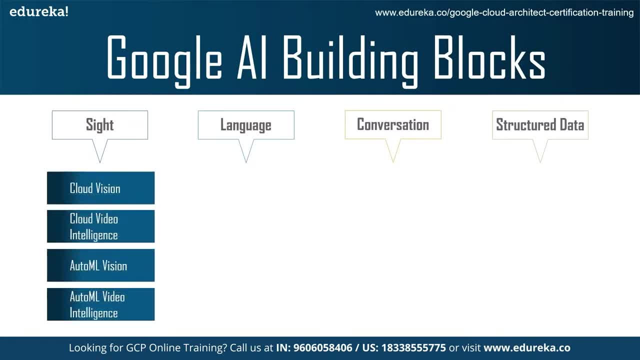 So on the side we have multiple products. that is first. one is vision API, with vision API and machine learning model which helps you reading images. Suppose, if I upload an image, Vision API, by just reading that image, the Google Cloud platform can help you identify the data points which are related to the particular. 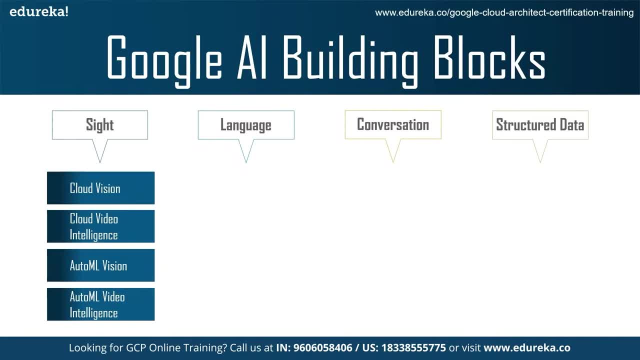 image, So it's very efficient for data processing. I mean image data processing. now the next one, that is, cloud video intelligence, which has, like pre-trained machine learning models that automatically recognize a vast number of objects, places and actions in storing and streaming video, which offers like exceptional quality out. 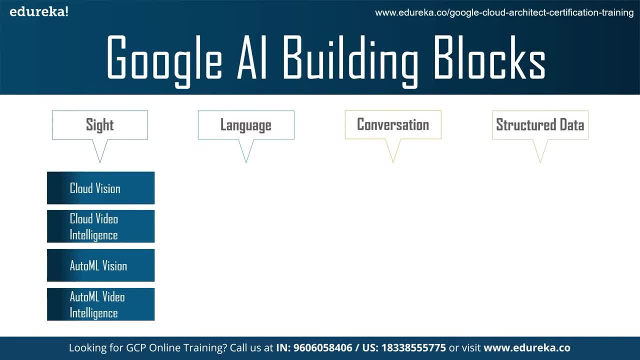 of the box. Also, it's highly efficient for common use cases and improves over time as new concepts are introduced. Now the next is AutoML Vision, which enables you to train machine learning models to classify your images according to your own defined labels. then 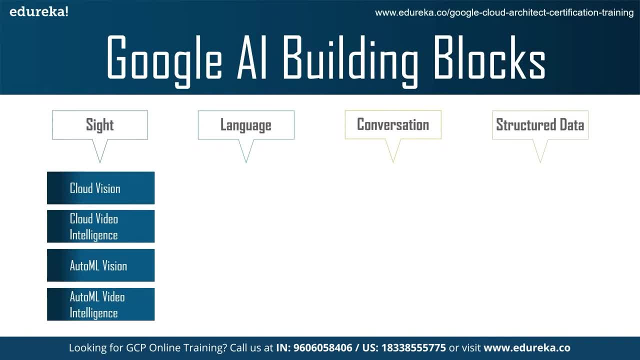 AutoML video intelligence, which has a graphical interface that makes it easy to train your own custom models to classify and track objects within videos. Even if you have like minimal machine learning experience also, then also it can work very efficiently. It's ideal for projects that require custom labels that are aren't 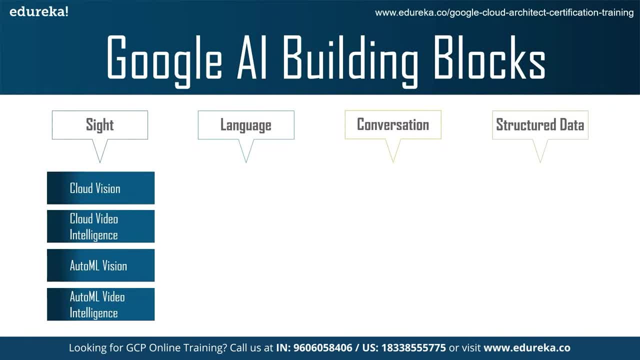 covered by the pre-trained video intelligence API. second category is language. So under language we have the first product as a cloud translate which, like, helps you in convert one particular language to another. Okay, suppose you have something written in Japanese. You can feed that in cloud translate and it can get converted into. 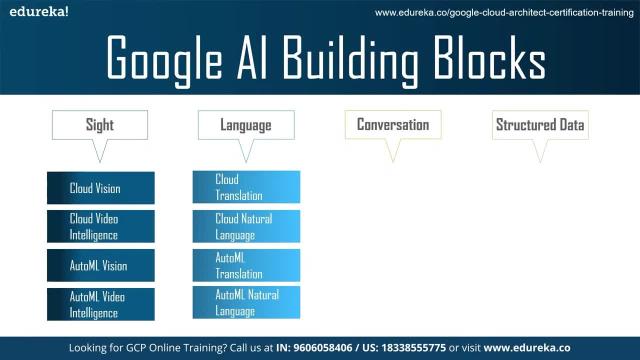 English or like any other language of your choice. So the next one is like cloud natural language, which is like a very famous product to send for doing sentiment analysis. Okay, then we have with the AutoML translation. like AutoML translation, So with AutoML translation developers, translators and localization experts. 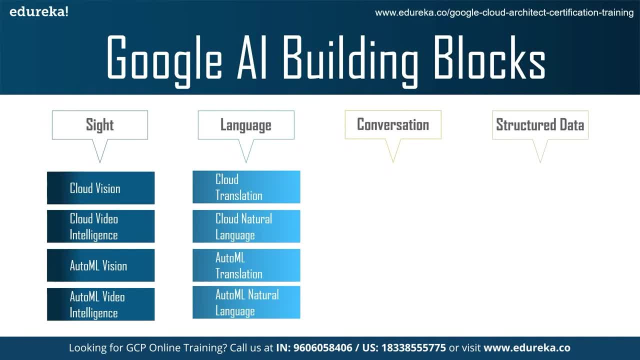 with limited machine learning expertise, can quickly create high quality and production duty models. So the software translated image pairs and, like AutoML translation, will train a custom model that you can scale and adapt to meet your domain specific needs. Last is AutoML natural language, which enables you to build and deploy 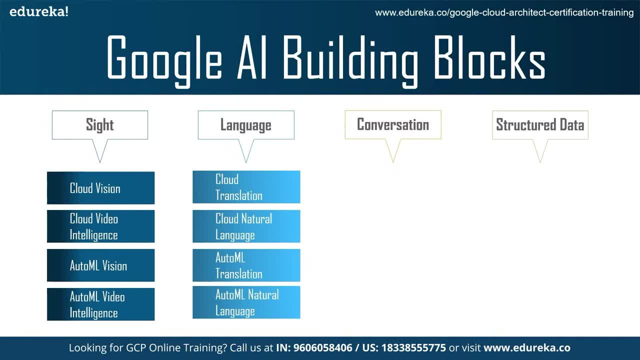 custom machine learning models that analyze documents and like, categorize them, identify entities with them or assessing attitudes with them. Now the third main category is conversation. So under conversation we have the first product is dialogue flow, which is a natural language understanding platform that makes it easy to design and integrate a 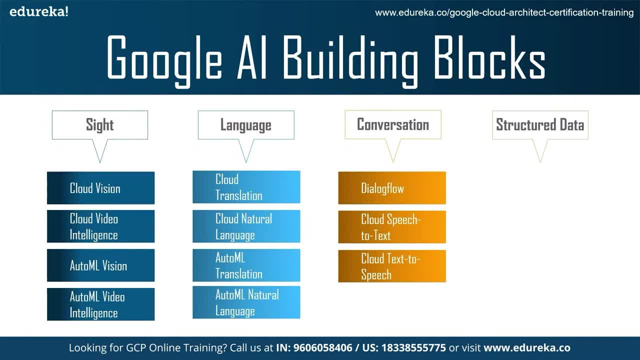 conversational user interface into your mobile app, web application or device, bot, interactive voice response system and so on. So, using a dialogue flow, you can provide new and engaging ways for users to interact with your product, and dialogue flow can analyze multiple types of input from your customers, including text or audio inputs, like 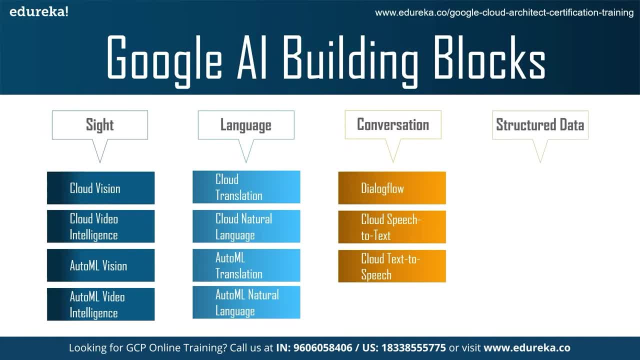 from a phone or voice recording, So it can also respond to your customers in a couple of ways, Either through text or speech. Then we have a speech to text API in under conversation which helps in converting your speech, So suppose someone is speaking at the same time. 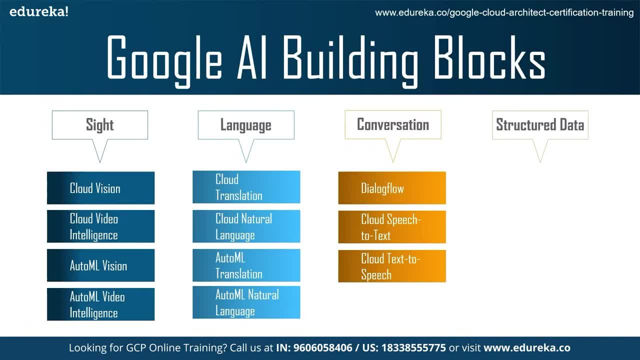 You wanted particular speech to be converted into text, Then that case this particular API and machine learning model comes handy and it helps you do that analysis. Similarly, we have text-to-speech API, which helps in converting given text to the speech at the same time. now comes to the last building block, that 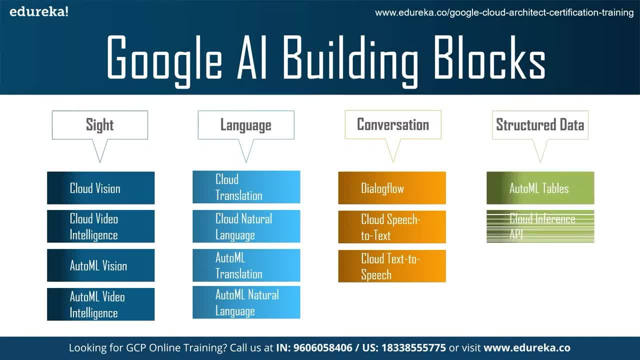 is the structure data. So first product in the structure data is AutoML tables, which enables your entire team of data scientists, analysts and developers to automatically build and deploy state-of-the-art machine learning models on structured data at massively increased speed and scale, which in turn transform your 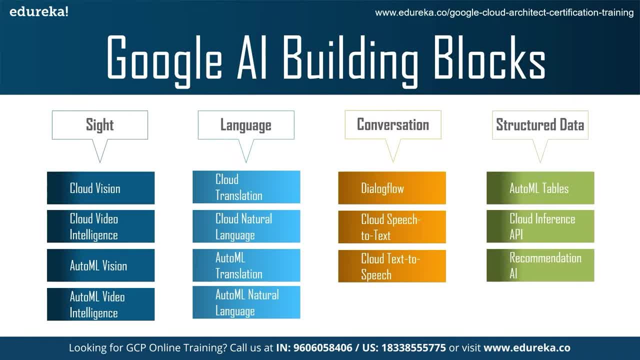 business by leveraging your enterprise data to tackle mission critical tasks like supply chain management, fraud detection, late conversion, optimization and increasing customer lifetime value. now coming to cloud inference API, So if you see time series analysis, essential for day-to-day operation of many companies, Most popular use cases, including analyzing foot traffic conversion for 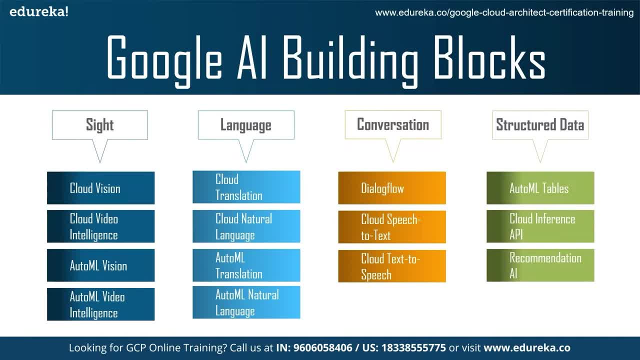 retailers, detecting data anomalies, identifying correlations in real time over sensor data or generating high quality recommendations. So with cloud inference API, you can gather insights in real time from your type to time series datasets. So, moving on to the last product, that is, the recommendations AI, which draws 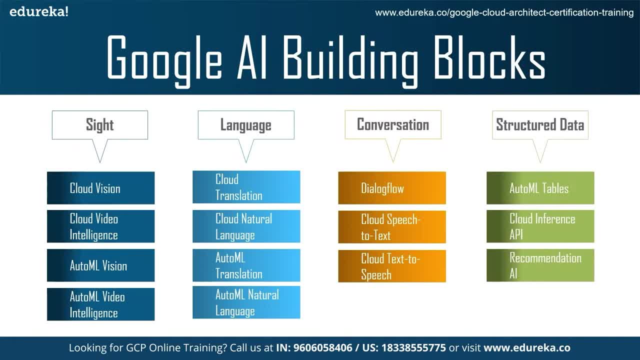 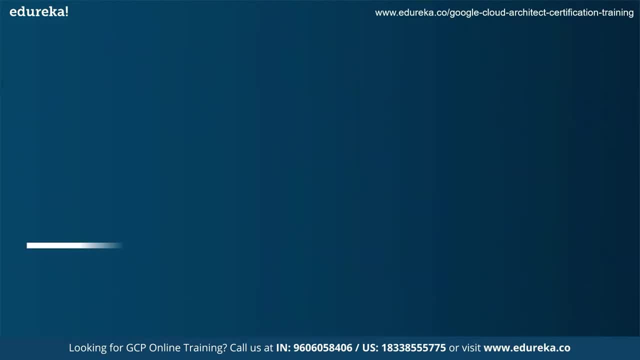 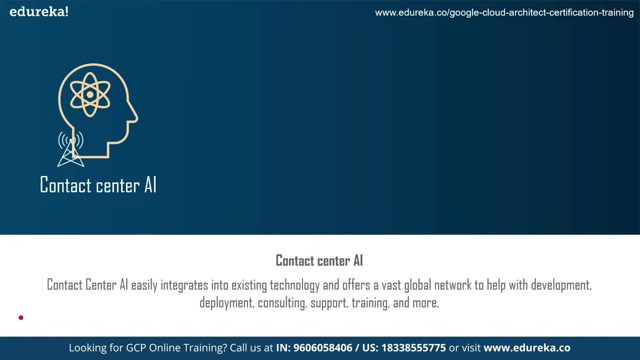 on the experience and expertise in machine learning to deliver personalized recommendations that suit each customer's taste and preferences across all your touch points. Now, finally, let's look at some of the solutions of AI provided by GCB. The first one is contact center AI. with this, you can lower cost and 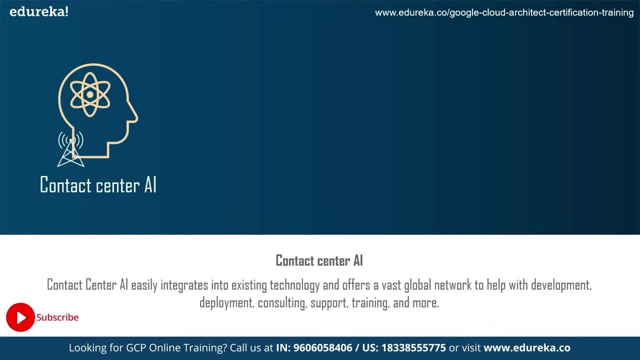 increase customer satisfaction with the best of Google AI technology. So customer service is being improved with AI that understands, interacts and talks. So with contact center AI, you can create agents that are superheroes of your customers. Also, you can enable natural interactions with virtual agents and empower. 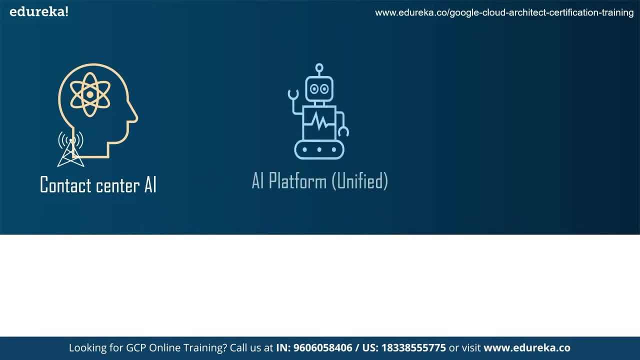 your teams with actionable insights. Moving on to the next one, that is, AI platform unified. So AI platform unified brings AutoML and AI platform classic together into a unified API client library and user interface. with AI platform unified, both AutoML training and customer training are available options. 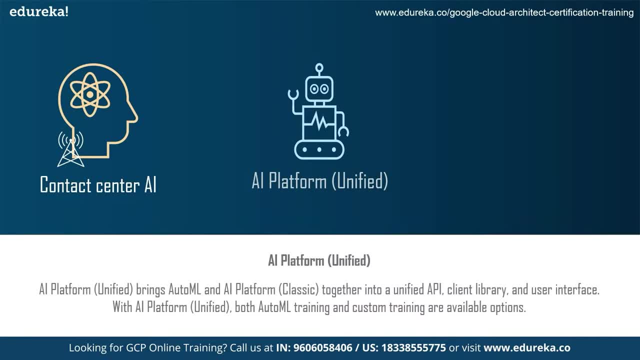 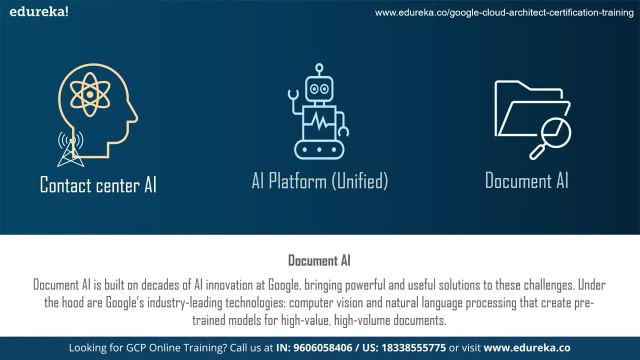 So, whichever option you choose for training, you can save models, deploying models and requests predictions with AI platform unified. Now the last major solution, that is document AI. with document AI you can automate data capture to scale to reduce document processing costs. It is built on decades of AI innovation at Google. 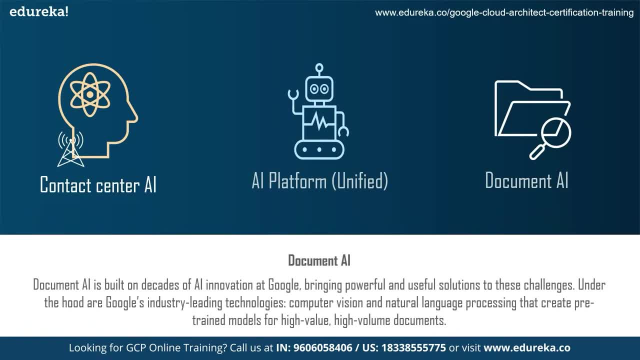 So you can create powerful and useful solutions to these challenges. under the hood are Google's industry-leading technologies like computer vision and natural language processing that create pre-trained models for high volume documents. Document AI has already like process 10 billions of tens or billions of. 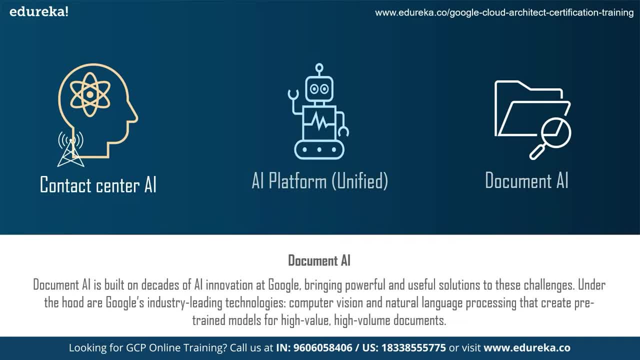 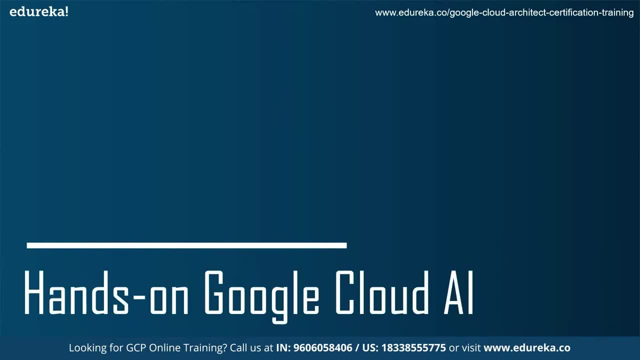 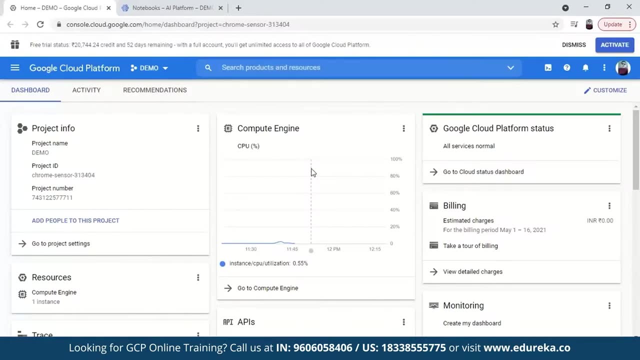 pages of documents across landing, insurance, government and other industries. So now let's have a better understanding of Google Cloud AI platform, but trying our hands on it. If you don't have an account on Google Cloud platform, then create one. GCP is like a really good platform to have your account on. it will ask for your like. 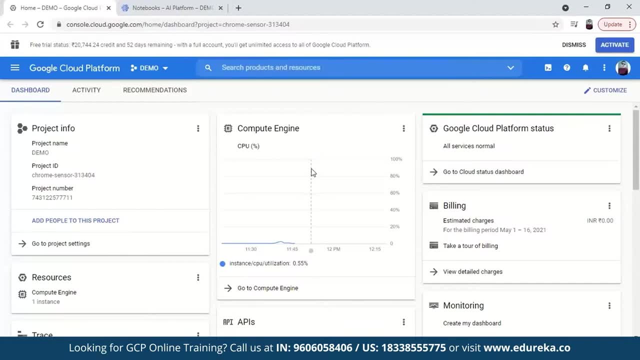 credit and debit card details just for the verification purpose and you will get a free trial for 90 days with $300 credited in GCP account and you can use that for the like demo I'm showing you know for exercises. I'm showing you practice with that. 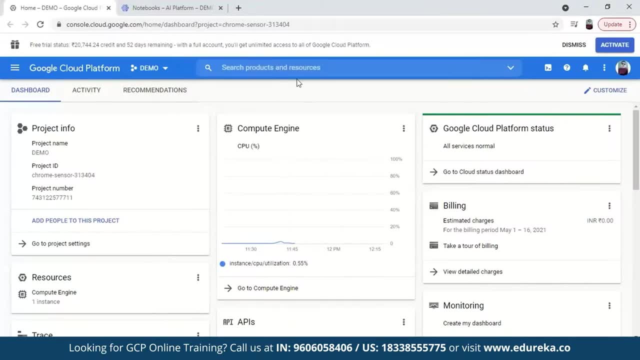 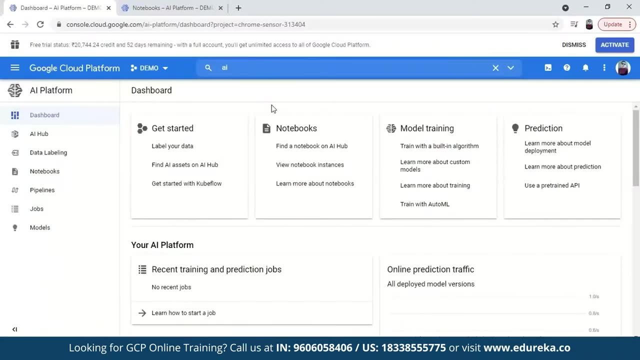 So this is the dashboard of Google Cloud platform and we have to go for AI platform, So you can just type here AI platform. So basically, AI platform is used to train your machine learning model and then scale your machine learning model And then you can like take your train model and deploy it on your AI. 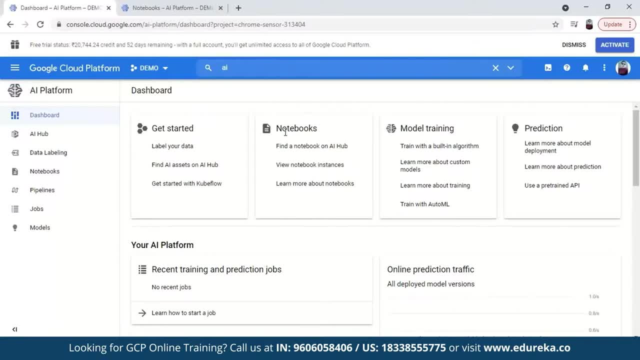 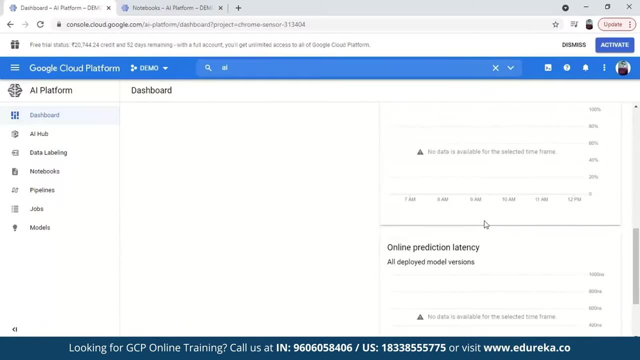 platform. This is the dashboard where you can- if you upload your model or anything, So it will show all the predictions for it. Also, the. it will predict traffic on it and everything. error rate will also show prediction latency. It will also show these kind of things out there right now. 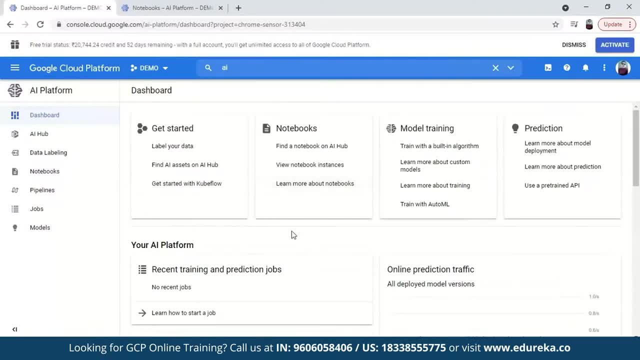 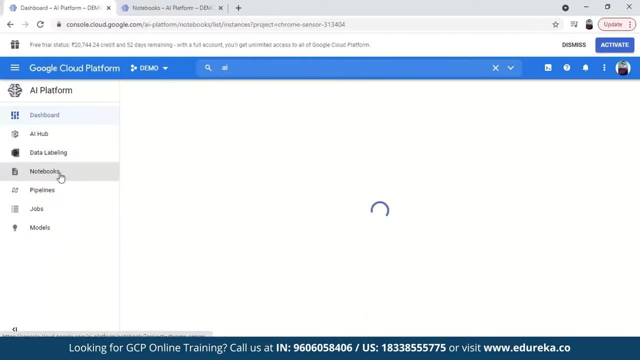 The way there's no model uploaded, So just showing the basic headings for it. So the first one, the first feature in this one is: you can say of we can come to note notebooks, It is how to generate a notebook instance, Just like you have no Jupiter notebook right in that way, only you can. 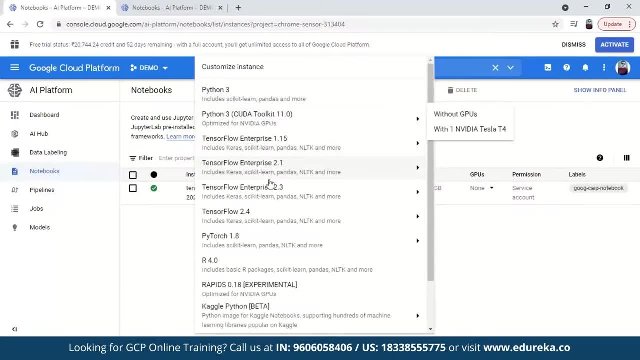 just go to new instance here and you can go to TensorFlow. these kind of options are there. like you can upload your simple python notebook also which have like scikit-learn or pandas or numpy, anything simple visualization or things are done, data analysis done. under that you can upload or you can 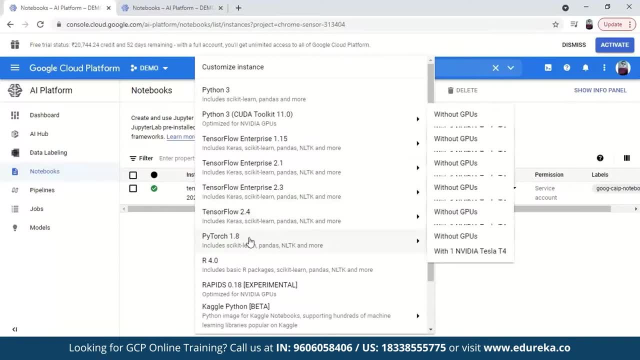 go for the happy heavy notebooks, also like TensorFlow or PyTorch, another like gaggle bit, like this ID and gaggle python also you can use a different kind of GPS. You in that, and here we are going with TensorFlow, like Enterprise with 2.1. 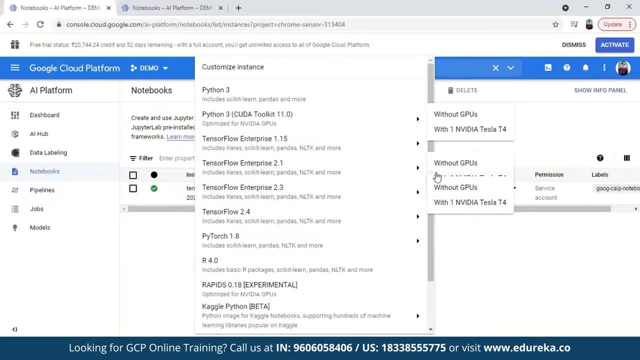 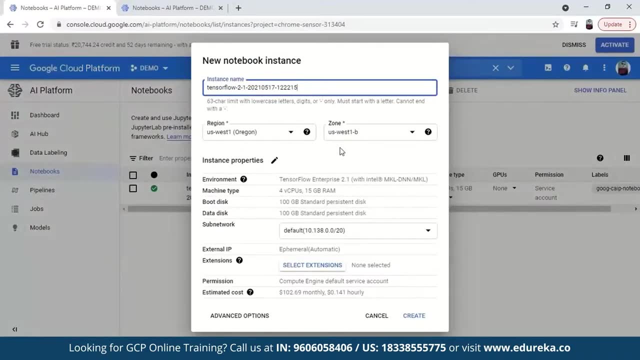 with like without GPU, and you also have option of Nvidia Tesla. Okay, So without GPU, and we did this- or Nvidia Tesla you can go for, but right now we are going with without GPUs. So here you can create your instance name and everything, or you can also. 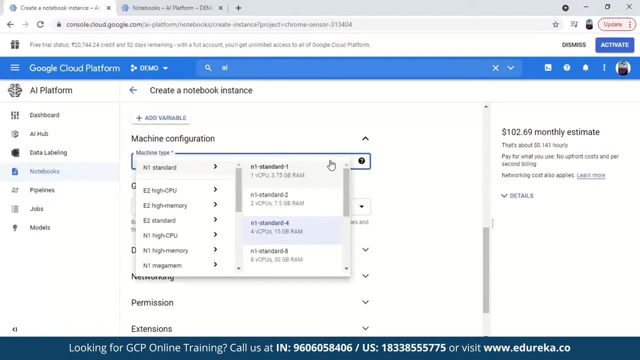 go to the advanced options. Here you can choose. the default one have like four virtual CPUs, and the standard one. I mean standard one has four virtual CPUs, 15gb ram and if you like want more, you can select more ram. And if you want the less, when you can select for the plus one and then 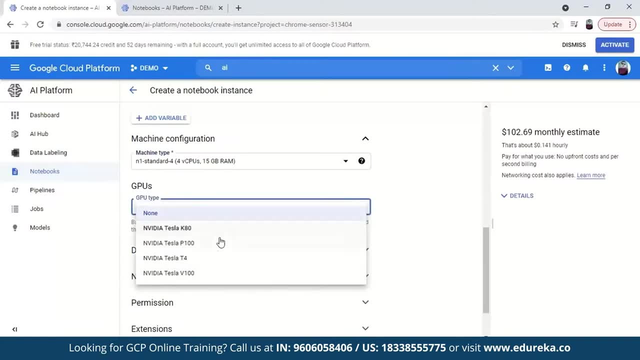 you can also select for GPU whichever you want. Okay, like it's like 80, p100, 300, like various options are there, Okay, and you can just and then create it. Okay, it takes time. So what I did is: I already created one, so we can just go back and launch. 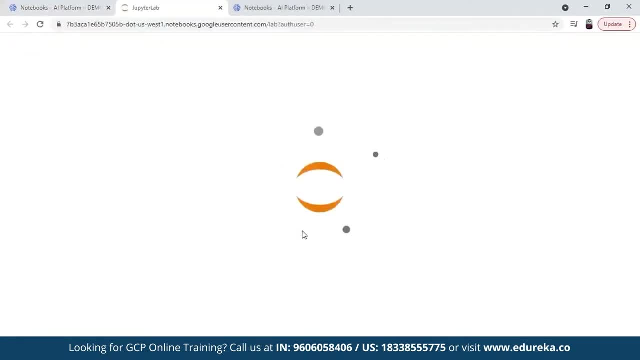 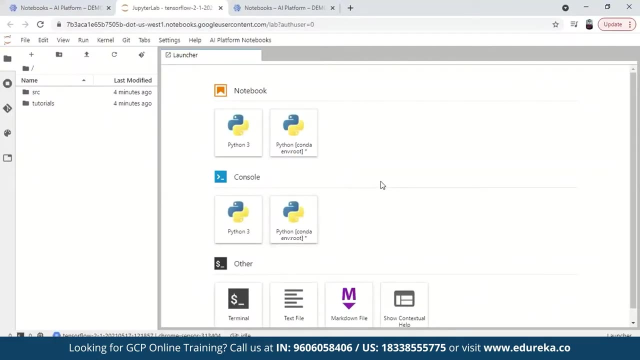 from here in this open Jupiter notebook here. So naturally it comes with all the built-in packages of TensorFlow and everything. but if you want to like install some Specific package, you can just go to terminal. here You can type like: pip- install XGBoost. you can install like: okay. 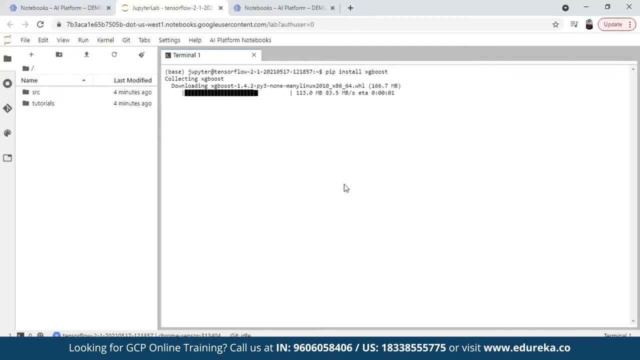 So it's downloading, install that. Okay, We have this. multiple options here, launching a notebook or a simple python console or everything. So we can just go to notebook. right now, You can select, or they are like multiple languages, You can select. Okay, you can also set python to other languages also, right now. 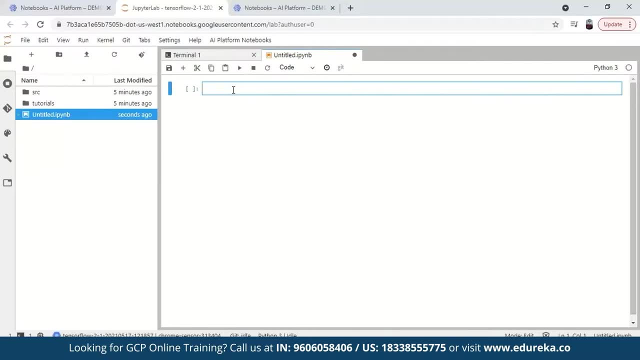 I've chosen python So we can check the version of XGBoost we have installed. Okay, so we can type just: you can import XGBoost as XGB, Then XGB, for checking the version XGB dot. double underscore. version Double underscore. 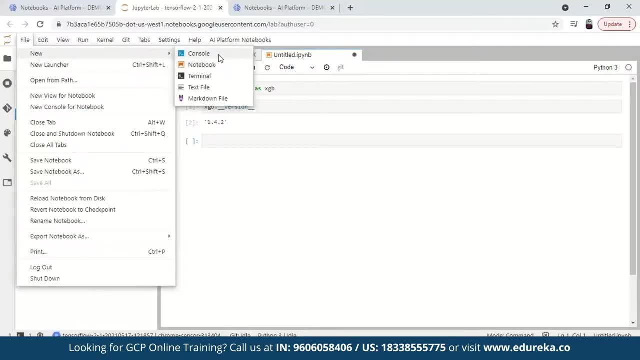 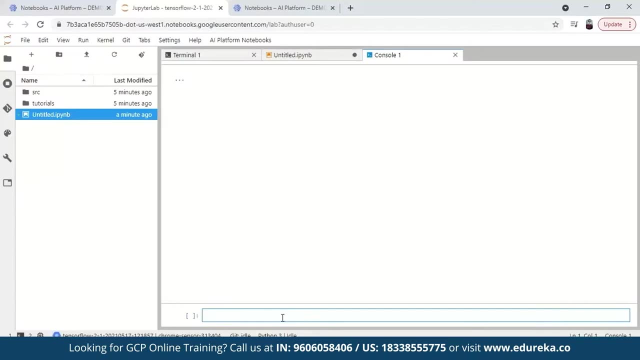 Okay, then we can also launch like simple python console also. So what you can do here is: come as a simple python. So what you can do, you can go for like checking the XGBoost version also. So just import XGBoost. 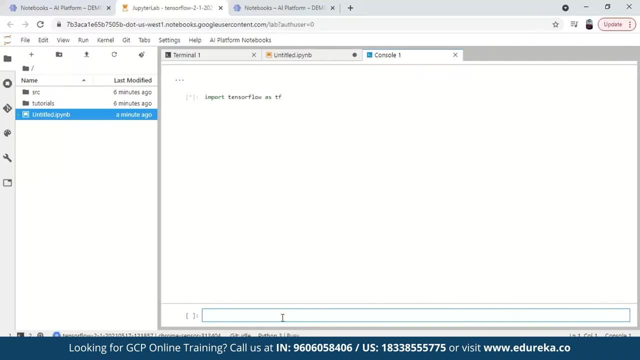 As a TF And then for checking the version, same TF dot, underscore, underscore version. So this is the 2.1.3 version of XGBoost. So this is how you can play with your jupyter with this notebook, Just like you play with a manual jupyter notebook, right? 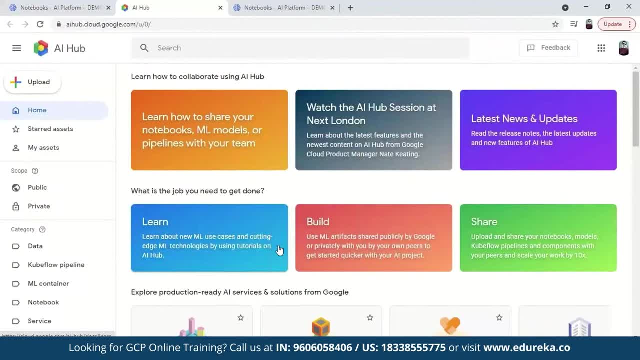 So, yeah, now coming to the next service, that is, AI hub. So what AI hub will generally does is if there is a like Google Cloud, AI team is there and Google Cloud team, They just post the content here, the latest contents of whatever kind of content, whichever is useful for you can take that and you can like if you. 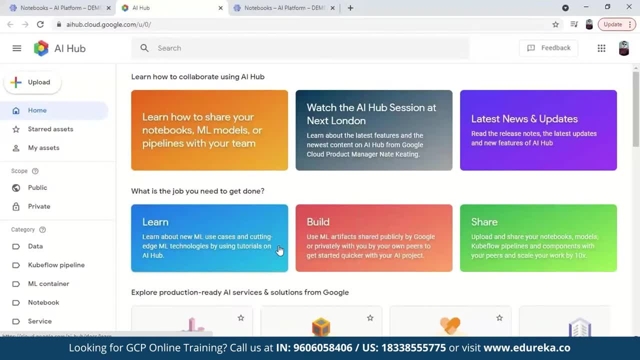 want to understand any model, you can get it from here. or if you want to run any RNN or something, you can understand and get a research content from here. So that's just one thing. second thing AI hub does is if you working in an organization, they have separate teams or something you can share your. 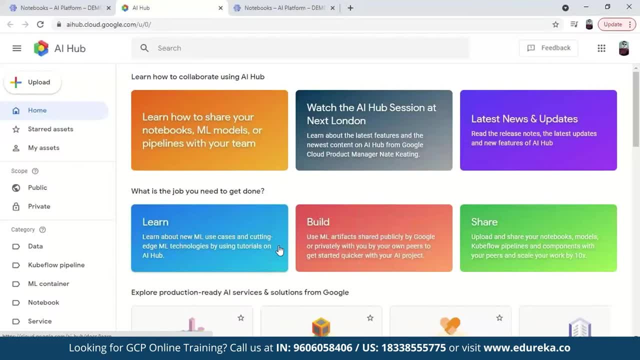 model here and it will be. you can put the limitation of it. It will completely be private to your team or certain to multiple teams. If you want to share your model with, That will be completely private. So that's a very good thing with AI hub. 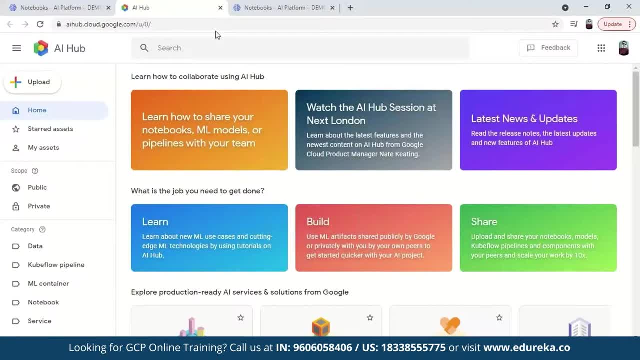 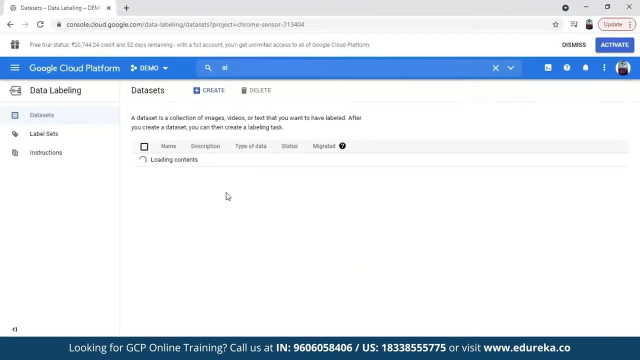 Okay, you can get your model uploaded here and share it with the people you want to, with your customizations. Okay, so that is AI hub. Then we have data labeling. So in data labeling, what happens is you put your data set, bit of image of. 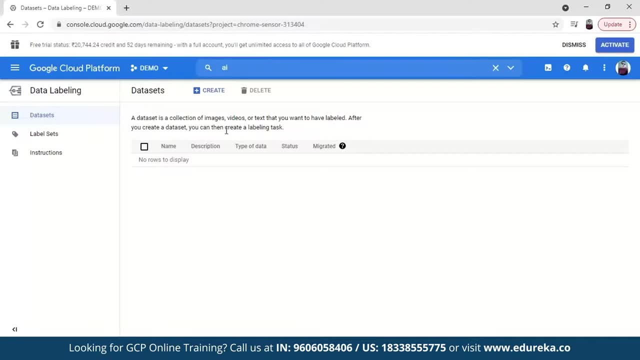 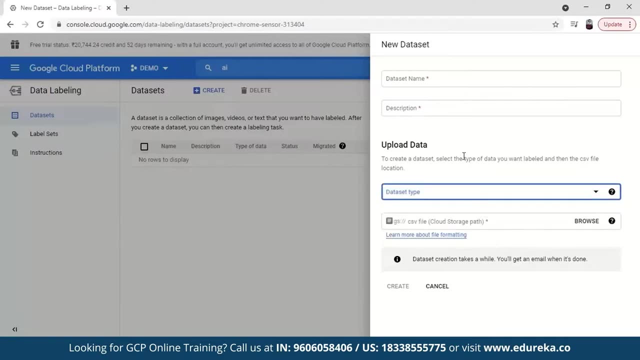 videos, in whichever manner it gets annotated by the human annotators, So you can just create it here. You can insert your data, set whichever like- image, video, text, or you can create- and then you can give your parameters or descriptions, whichever way you want your data to get annotated. 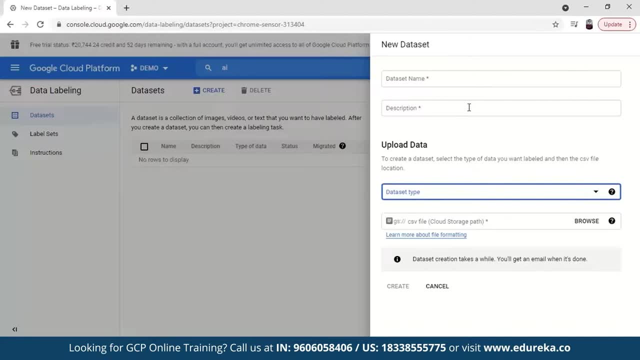 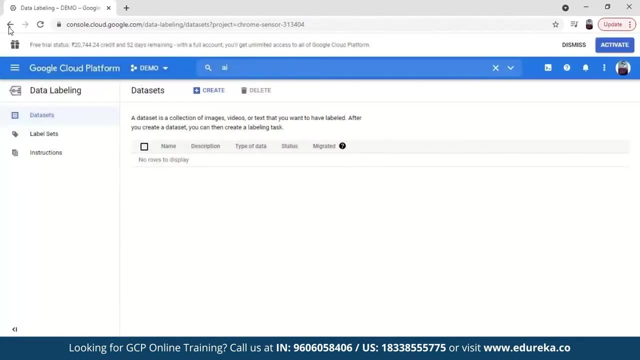 So you can give a better description. It will give you a better results on the basis of that. The more your description is accurate, the more accurate will be the annotations. Okay, so that's how it can be done. Then we can go back to the other service. 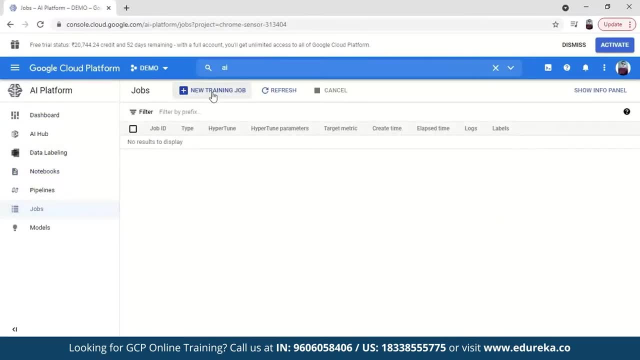 That is, you can go to jobs. the jobs here is: you can like create a new training job from here. We have option of built-in algorithm training, then a custom code training. a custom code training. You can write your model, create your model and you can upload it here and 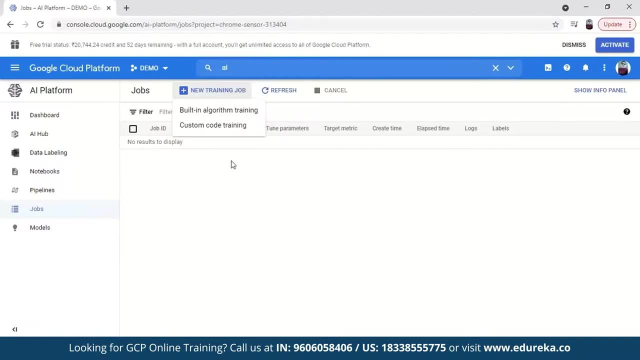 whichever way you want- You upload or you want to give any kind of model. that is custom code. but it's plus point is in built-in algorithm training. with built-in algorithm training We get the option of: like: you can select any kind of algorithm. these 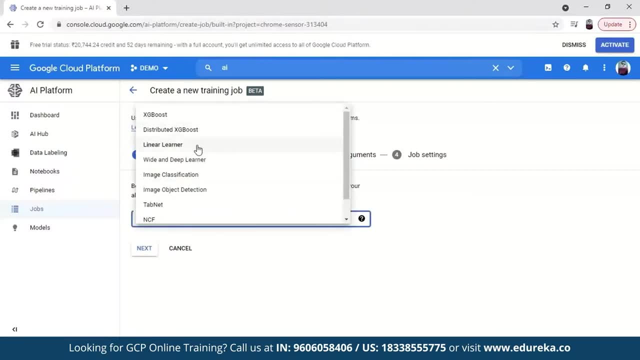 option. all the algorithms are given: XGBoost distributed XGBoost linear learner, wide and deep learner, image classification, image object detection. These are the new ones which are Google Cloud introduced, like tabnet and ncf. all these things you choose your algorithm, then you can give your. 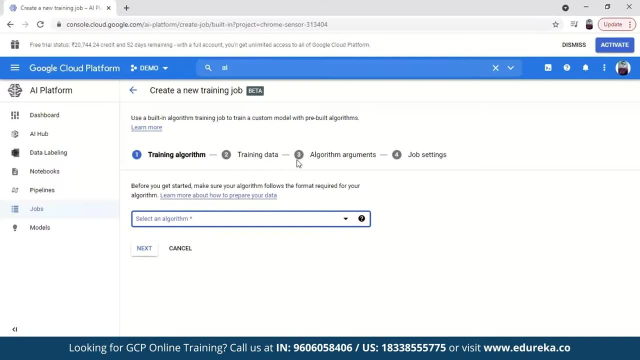 training data you can give, and then you can give your algorithm arguments Also, and you can provide the split ratio Also. Also you can give other parameters also. on the basis of that parameter, The model will be analyzed and prepared. So that's a very plus point. 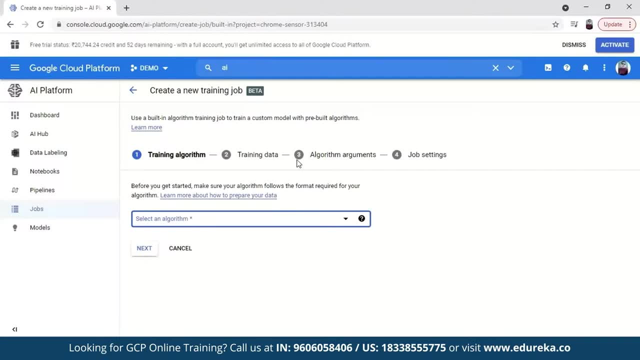 Is it like? saves a lot of time. instead of making the whole model, It just directly creates a model for you. You don't have to code and do everything, So that's a very plus point. and then we have pipelines. So what pipeline does is pipeline addresses all your mlops lifecycle. 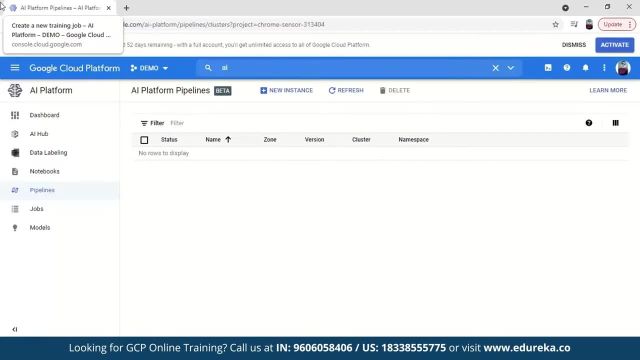 starting from acquiring data, preparing data, analyzing data and training the model. Analyzing the model, deploying the model and then tracking your like model artifacts, evaluating the model. It is like built on Qflow pipelines and tensorflow extended modules, So it basically allows you to build an end-to-end pipeline and, at the same, 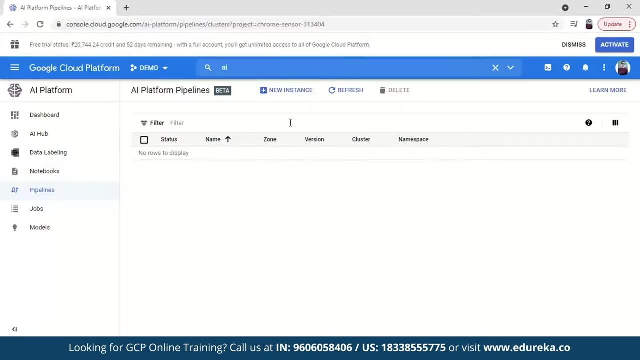 time deploying the end-to-end pipeline. So this is what the pipeline, a pipeline is. So then we have like models. models is something if you want to do code wise like command line programming, you have to do like command line model. You have to make or analyze it or deploy it. 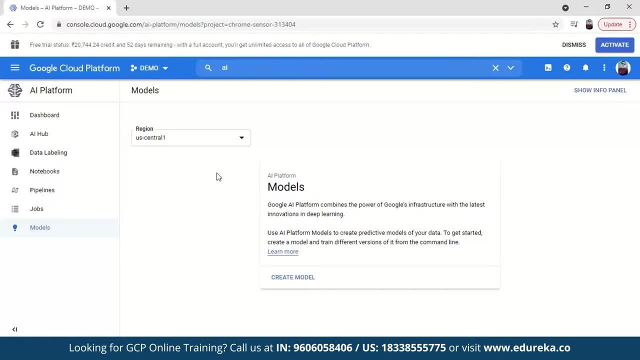 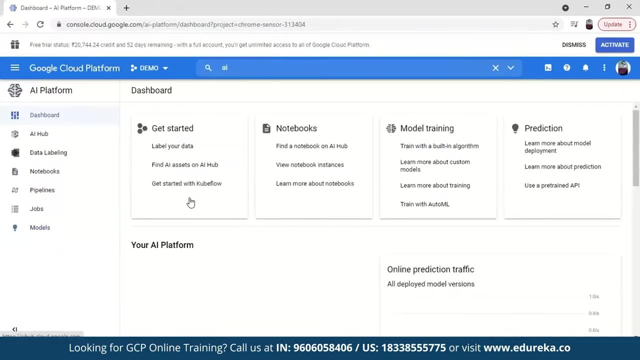 That's where model is used. We can discuss that later. That's actually a big process, So yeah, so I just wanted to show you the demo thing for this. So this is how the Google Cloud AI platform works. So this is the general description for it. 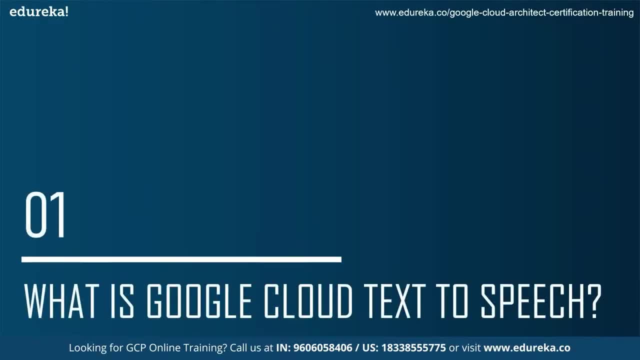 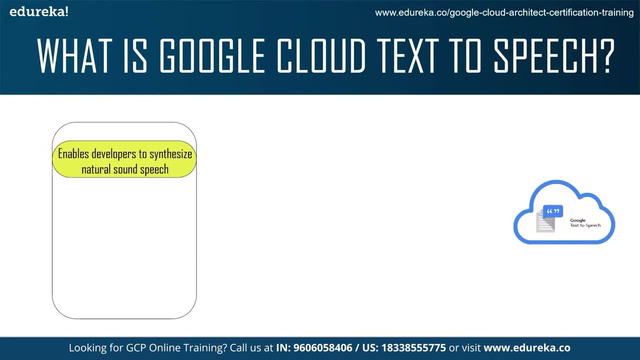 What exactly is Google Cloud text-to-speech? right? So Google Cloud text-to-speech is one of these services that Google Cloud platform offers. It's nothing but a service that enables developers to synthesize natural sounding speech from a certain text, So it offers over 30 plus voices that you can choose from and basically it's. 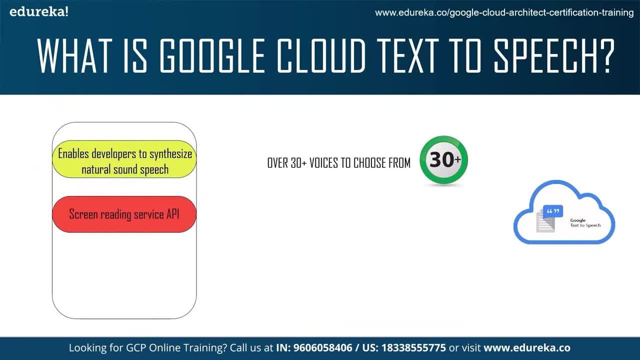 a screen reading service- API. So APIs are something that you can call to invoke a certain function or a service. right, So it's a screen reading service that Google Cloud provides its users with. right, So it's something that Google provides worldwide. and also the fact that 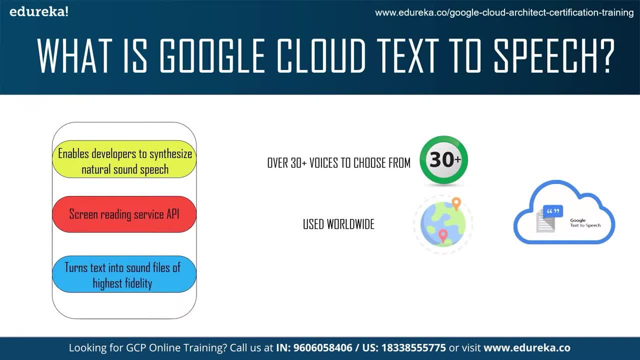 Google Cloud text-to-speech turns text into sound files with a high fidelity. So high fidelity is something that comes into play when you want to make the voice sound human-like. So if it is high fidelity, it means that it sounds very much like humans. 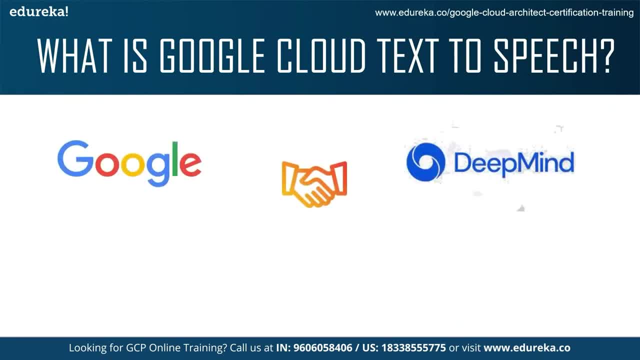 So next we come to the fact that Google Cloud text-to-speech- has been developed by Google and DeepMind. Now Google has helped with neural networks, whereas DeepMind is a company which focuses mainly on artificial intelligence. Now, these two have collaborated before in making the Google Maps API or the 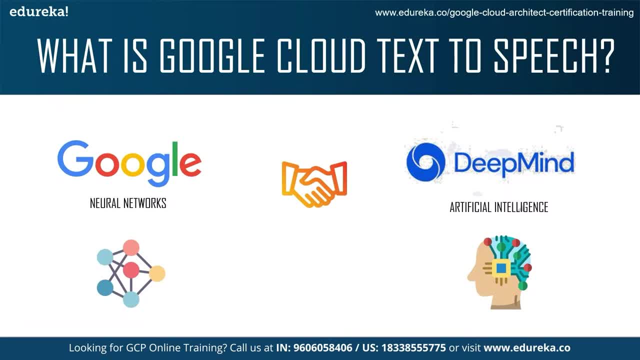 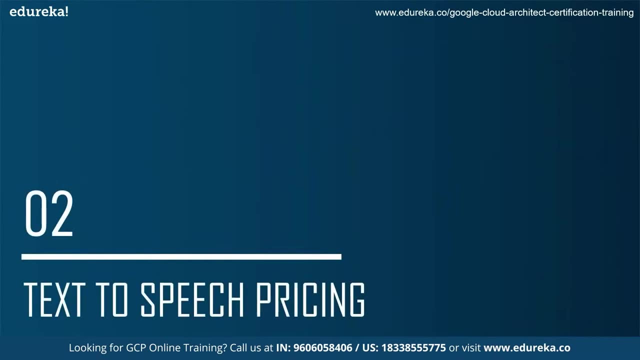 Google Assistant API that are there Now. both of them have combined with the neural networks and artificial intelligence services that there are and APIs that there are. Both of them have combined to create Google Cloud text-to-speech- right. So next we come to this pricing for Google Cloud text-to-speech. 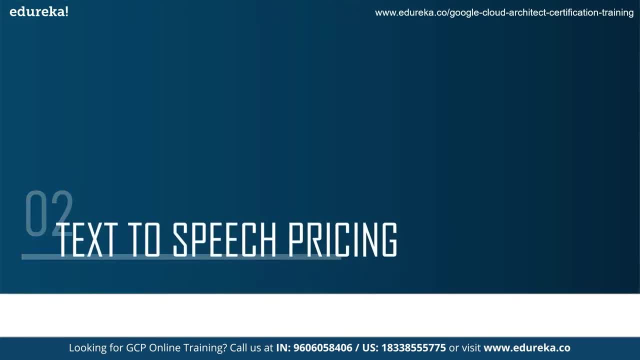 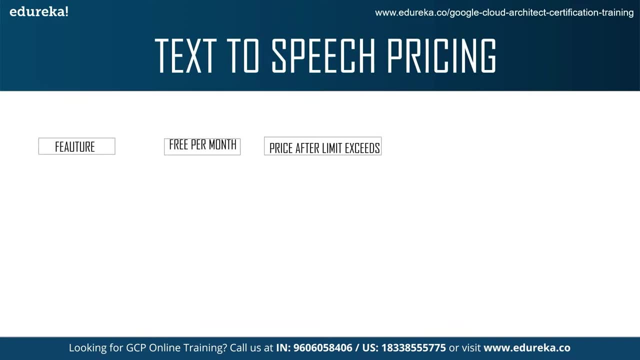 Now the first thing question that comes into mind is: is it free Now? Google Cloud text-to-speech is free for a certain amount of time, just like other AWS and cloud services and GCP services. So for a certain point of time, the standard Google Cloud text-to-speech 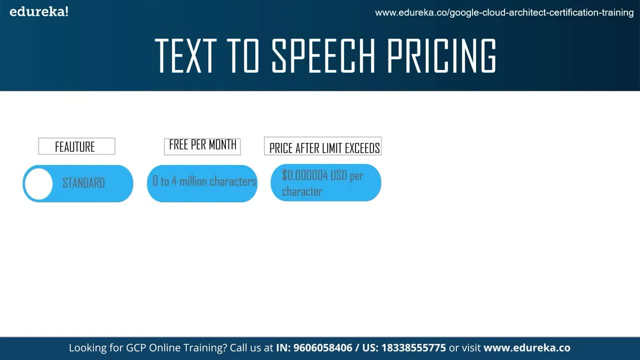 pricing is free for 0 to 4 million characters that you type, But after the 4 million characters have been crossed, this price limit exceeds to $0.00004 per character right. So that's a very small amount, or if you do not use the standard version. 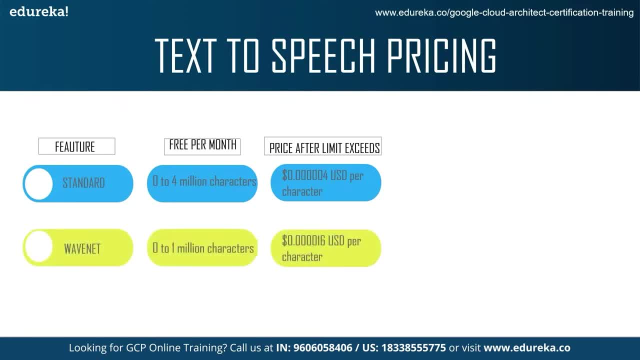 for pricing or speech. you have the WaveNet speech, which allows you to have 0 to 1 million characters to be spoken, And if you exceed that limit, you will basically have to 0.0001416 US dollars per character, right. 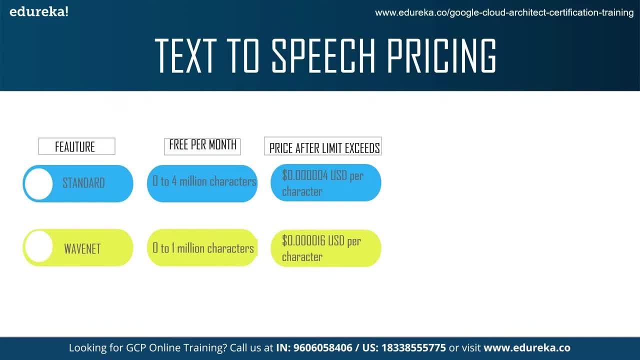 So this is the basic pricing valuation that Google Cloud provides its users with. Also, when it comes to pricing, you have to remember that SSML and Spaces are definitely counted when it comes to pricing your APIs and services that you use. Now, SSML is like HTML and any other language that you use to basically, 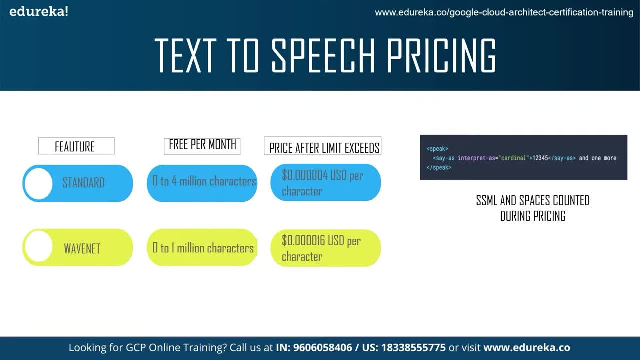 convert and synthesize The text you have into a certain synthesized voice, right? So, apart from the fact that SSML is counted during pricing, the price is based on the number of characters you have sent, right? So if it exceeds the free limit that you have, you will be charged. 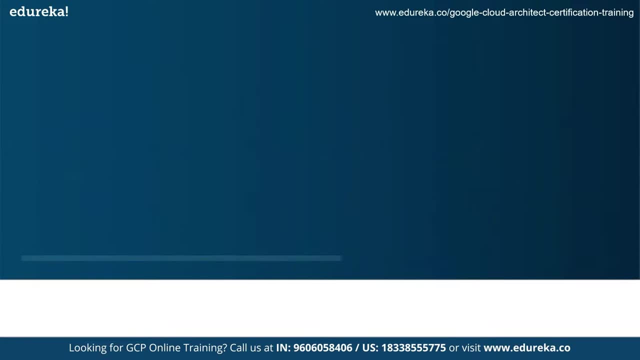 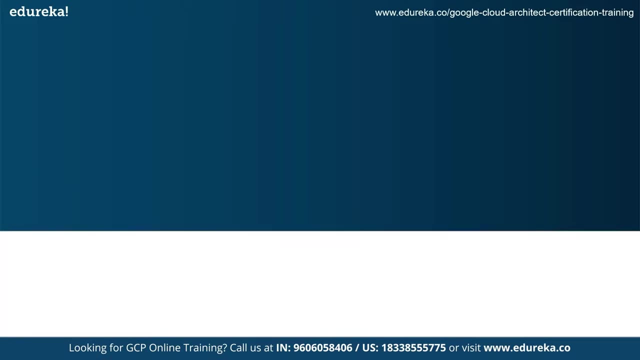 based on what the charges are right. Next up, we have the key features of Google Cloud text-to-speech. Now, when we talk about Google Cloud text-to-speech, first thing we talk about is creating Audio files. Now, audio files can be created using Google Cloud text-to-speech. 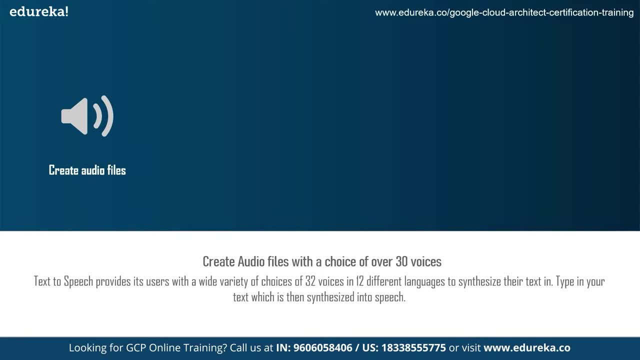 So this is where you have a choice of over 30 voices. So, and this is why this is a very in use tool. when it comes to Google Cloud platform, right Next up we can see that pitch tuning is another feature that Google Cloud text-to-speech provides its users with. 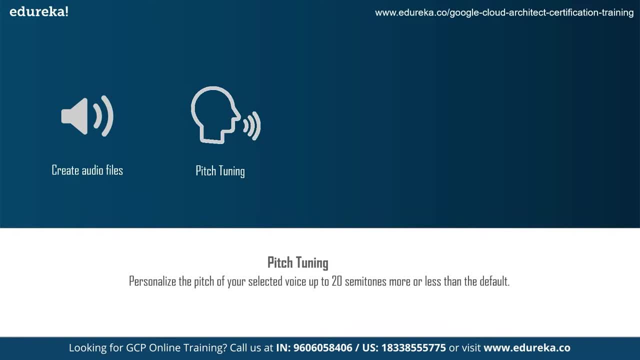 Now, pitch tuning is basically the ability for the user to personalize their pitch up to set 20 semitones right. So that is one Of the features that is there. Next up, we talk about the integrated REST APIs that are there. 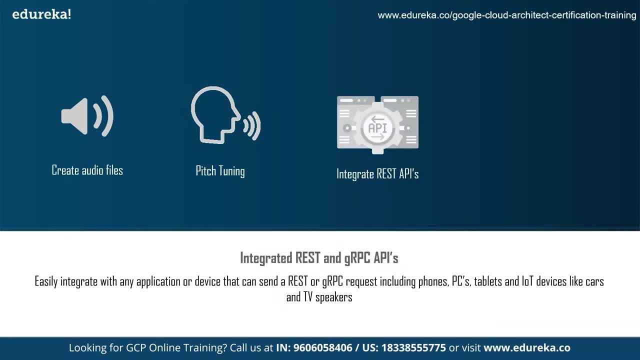 So Google Cloud text-to-speech allows you to use integrated APIs with Python, Java etc. So that you can make those function calls, deploy a program and then, using that program, use the Google Cloud features and services and get a text-to-speech right. 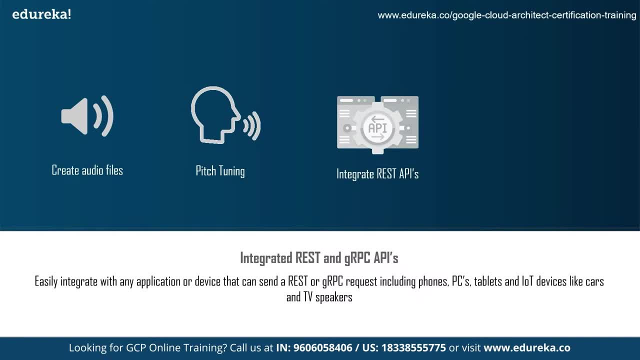 So you can integrate APIs easily with any application and the REST APIs or the gRPC requests right, So that can be done anywhere using PCs, tablets, let's say, IOT devices, etc. etc. And finally, last feature is the fact that Google Cloud text-to-speech 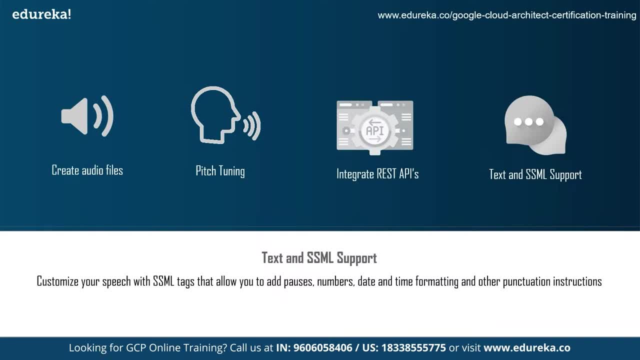 is text and XML supported. So, as someone basically allows you to customize the way you want the speech to be set, like, for example, if you want to add pauses or numbers or, let's say, date and time, you can do all of that using Google Cloud. 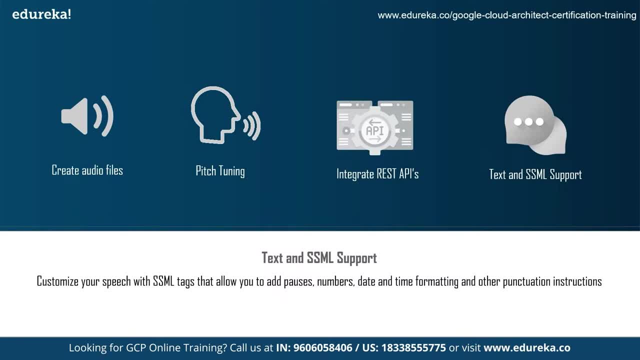 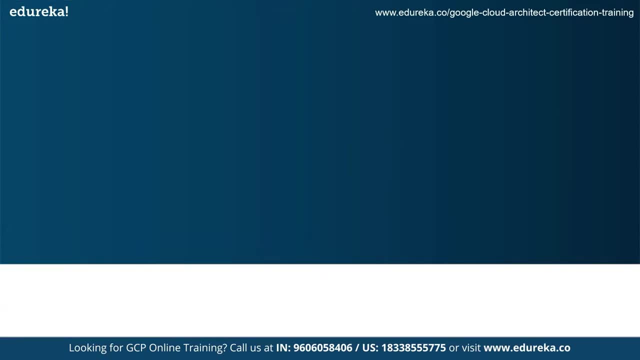 text-to-speech, And SSML is something that is used to do that right. Next, we come to the benefits of Google Cloud text-to-speech. Now, the first benefit is high-fidelity speech. Now, high-fidelity speech, like we talked about, is the fact that how? 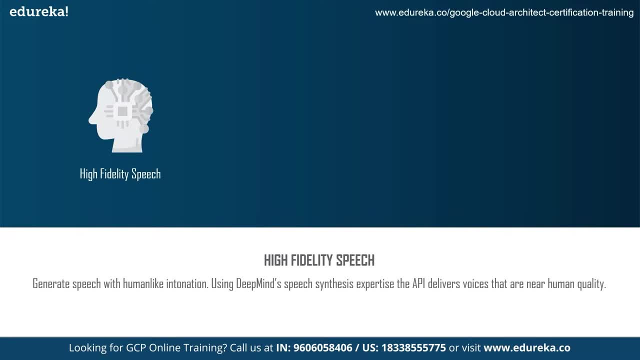 human-like can your voice get, and with Google Cloud text-to-speech, you can really get very human-like voices using DeepMind's WaveNet voices that are there, So that is something which is extremely efficient when it comes to high-fidelity voices. 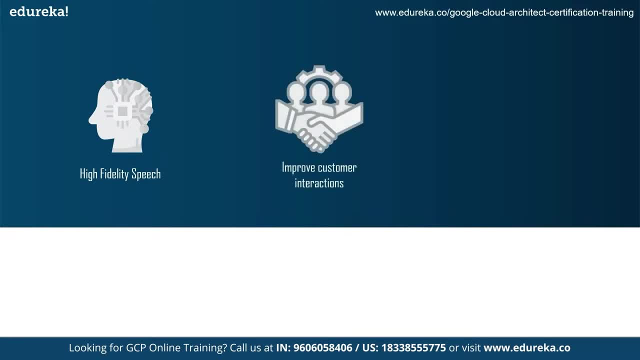 Next, we talk about improving user interactions and customer interactions. Now, Google Cloud text-to-speech will automatically improve customer interactions if it can basically get that engagement. Now, when you change- let's say, for example, you have a certain chatbot- 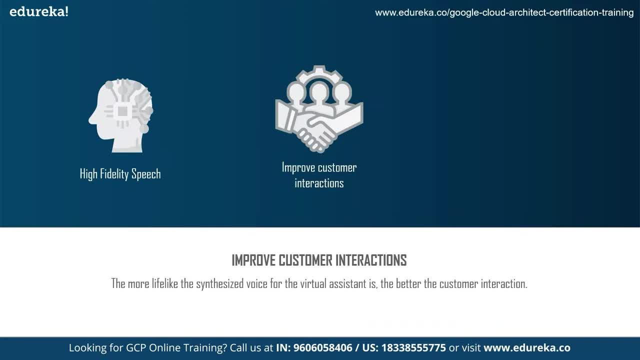 in a website. Now, the fact that the chatbot is typing whatever message it is delivering to you can get a bit tedious. So if you change the chatbot to, let's say, a Google Cloud text-to-speech enabled assistant that you might have. 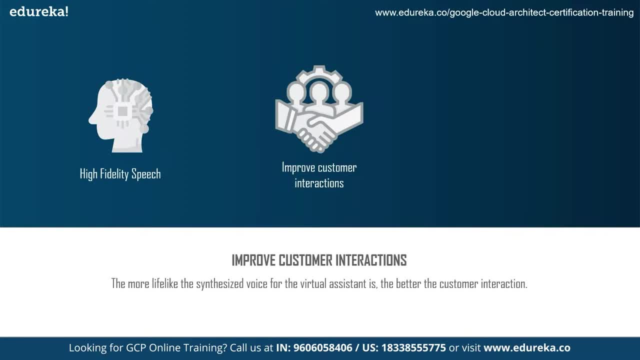 that assistant might be able to basically interact with you using Google Cloud text-to-speech, and it's much easier and faster for you to communicate, right? So that is why the main thing that Google Cloud text-to-speech does is it increases engagement for users based on the UI. 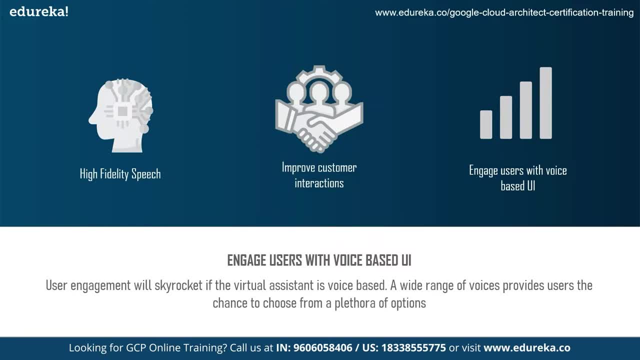 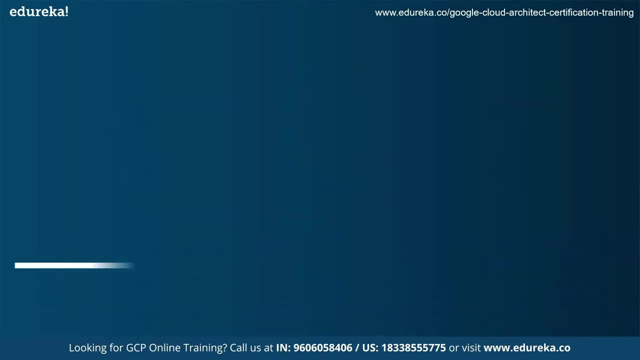 So the more the engagement of the users, the more is the customer interaction improvement. So these two are based on one another. So engagement will directly coincide with customer interactions, right? So next we come to the demo for Google Cloud: text-to-speech- right. 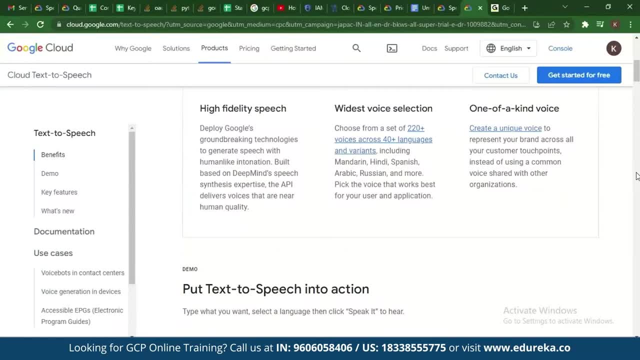 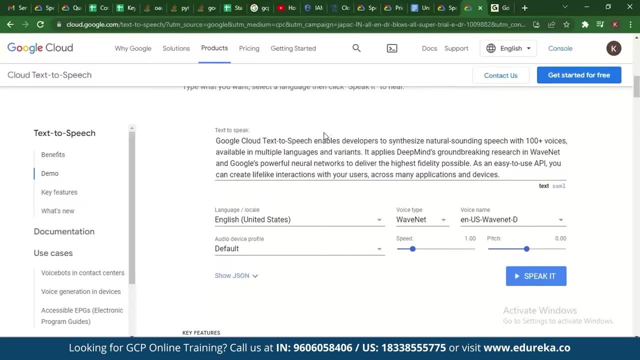 So when you go to Google and type Google Cloud text-to-speech, this is something that you can see, and here you can see that it has high-fidelity speech. So what you can do, we can just check out some basic things here. 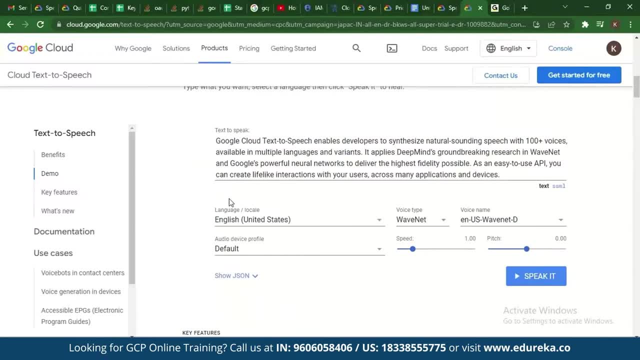 Let's say, for example, this is the text that you want to speak, right, And this is the language. So you can choose the language that you want the person to speak in, and I want him to speak in English, So I'll keep it as English, United States. and that is the speed at. 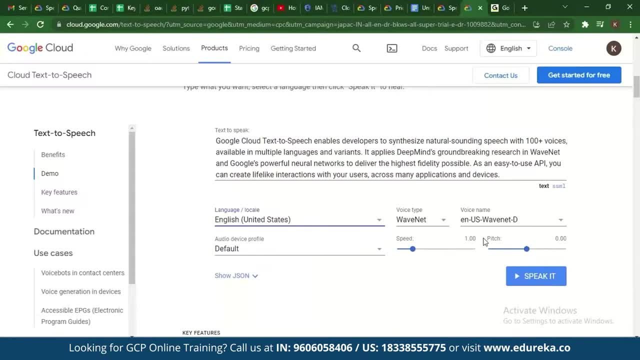 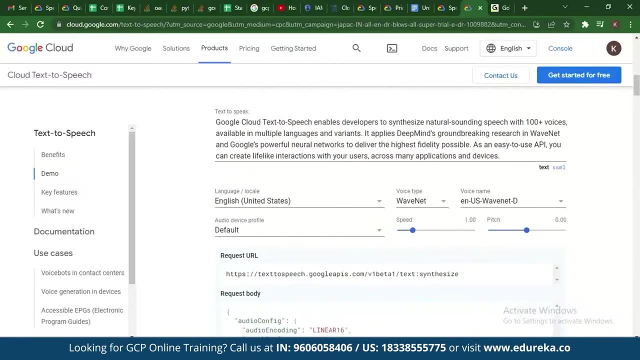 which he'll speak it and the pitch at which he'll speak- right, So you can change this and you can also see the JSON format of the file, Let's say of the audio file is here Now. this is done using an API which we will talk about in some time. 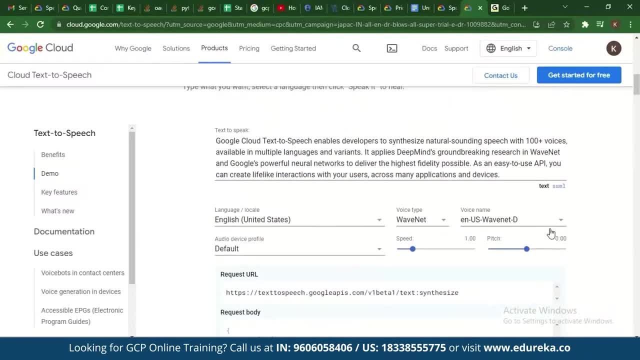 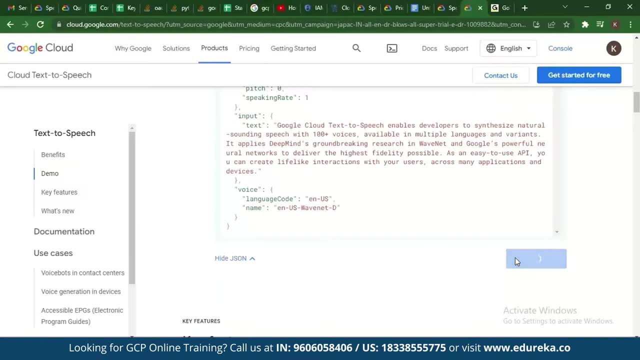 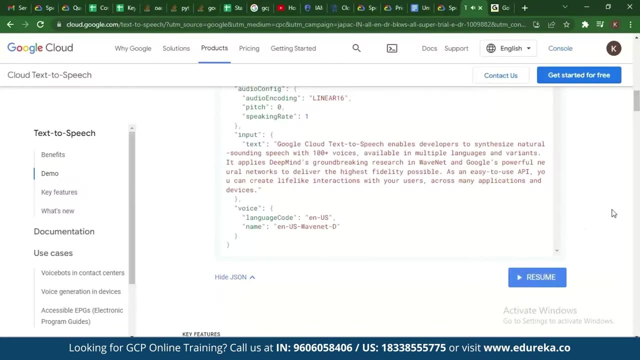 So let's say, this is the voice That is being used, the USB type voice. using WaveNets, You can use standard as well And after that, when you go to speak it. So this is basically showing you that this text that you have, it's being. 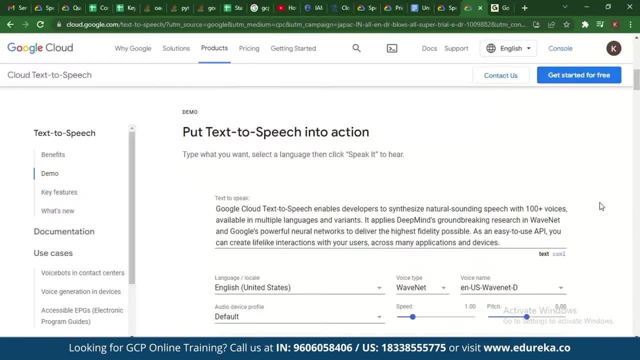 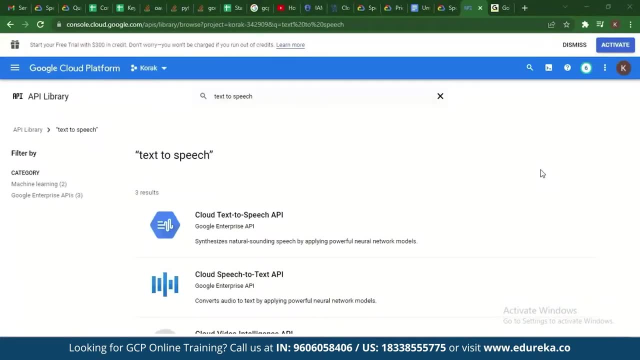 synthesized from text into speech. Now what we can do here is we can now go to the console and see how we can use APIs. So now that we basically want to use the Google Cloud text-to-speech API with Python, First thing we have to do is go to Google Cloud text-to-speech and try. 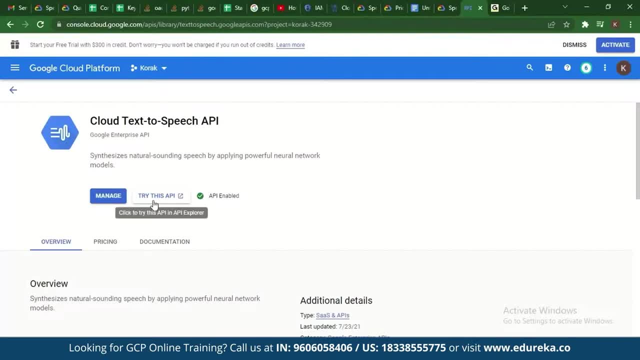 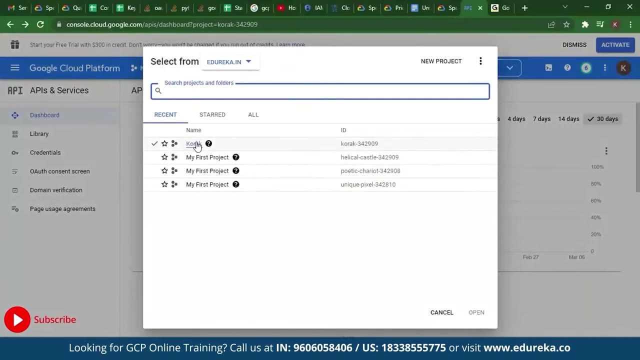 this API and enable it. firstly, So this is enabled. now We have to try this, right. So what we do here is, let's say, let's go back to the console, right, Yeah, so we go back to the console and basically go back to the project. 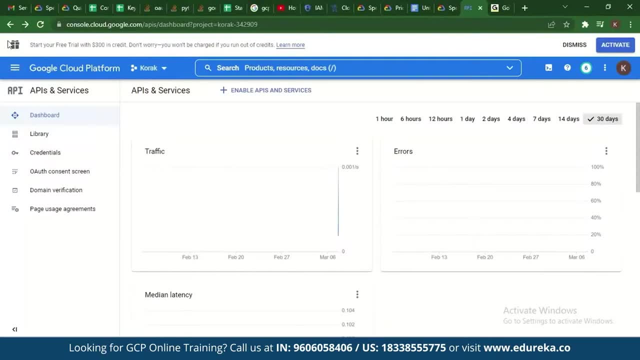 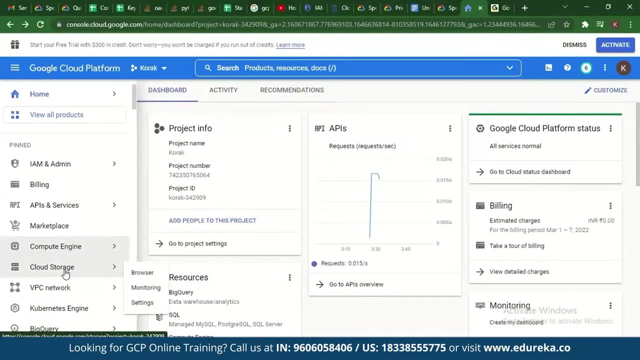 We created. this is a project that I created. What I can do here is go back from APIs to credentials, right. So here I would have to do is I have to launch an instance, a virtual instance, So I can go to- I am an admin- and go service accounts. 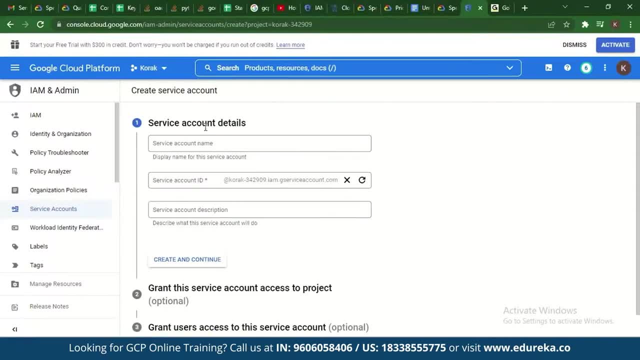 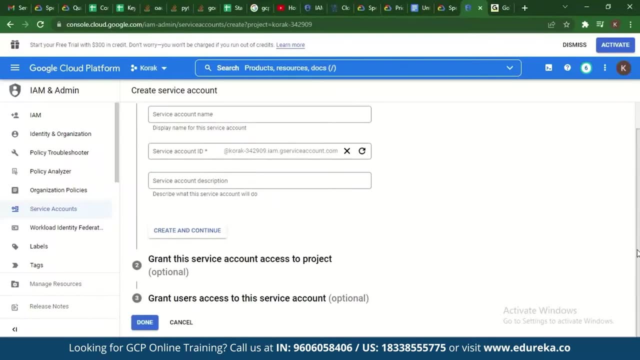 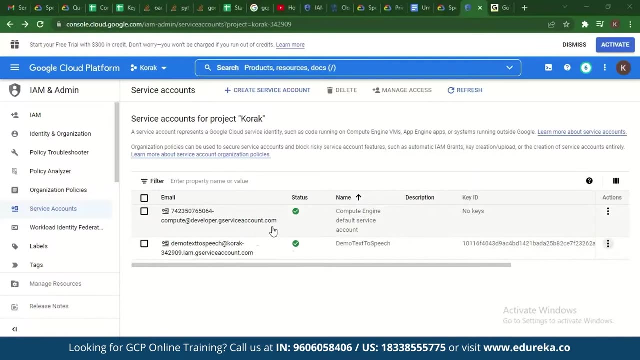 Now, when I go to service account, I can go create a service account and these are the information that I have to fill in for service accounts, right? So the name Is all you need to do here when you create service accounts. So once you basically made a service account, you can just see that the 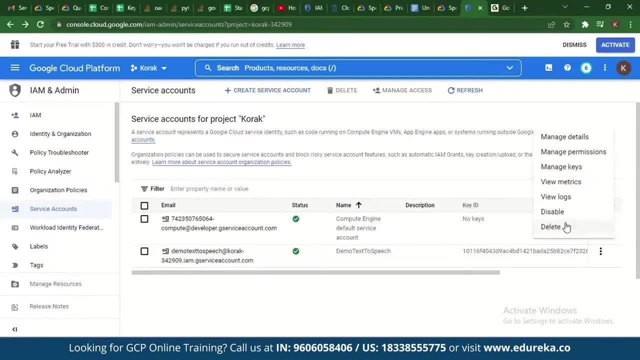 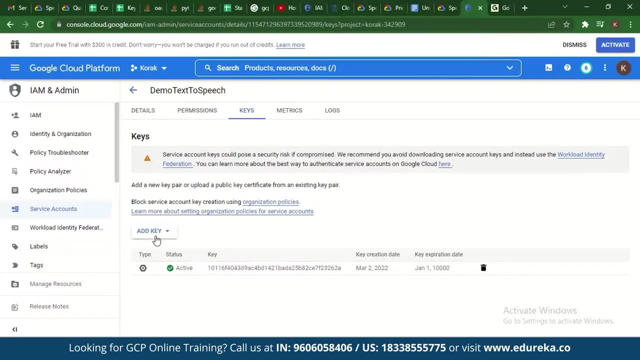 service accounts being made here. What you can do is go here and manage keys, right? So when you go to manage keys, what you can do is add another key, And when you go to add another key, you can go to select key and then go. 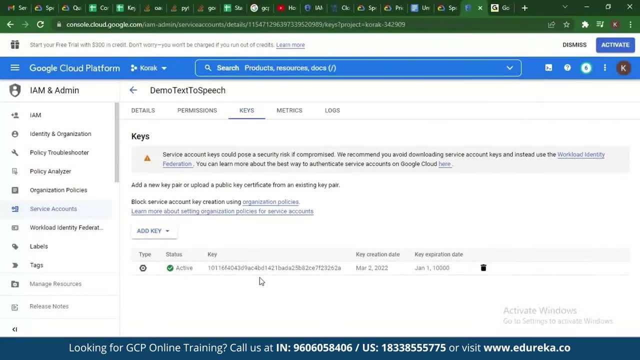 to Jason and download this. Now. I'll not be doing this because I've already done it and it's active. So, once all of this is done, what we need to do is go to, let's say, a Python environment, And first thing we need to do is create a python environment using 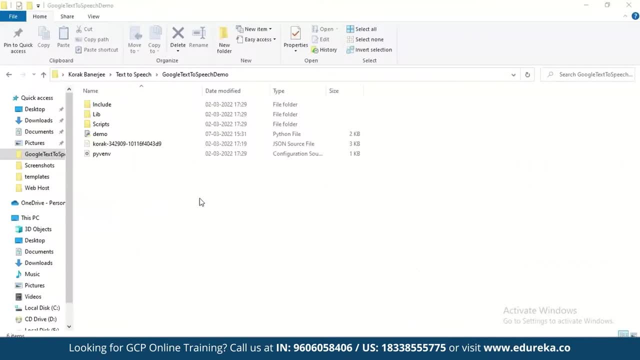 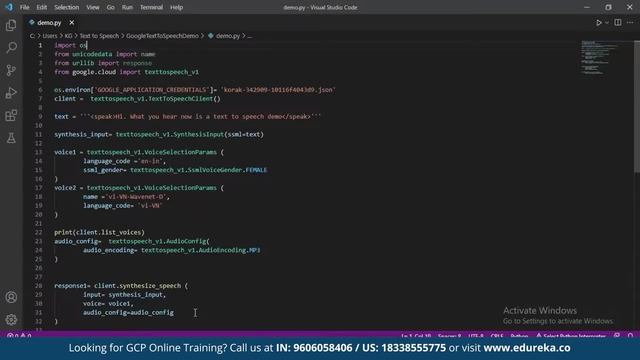 CMD, right? So basically, once you've created a python environment, you'll have files, which are the scripts, The libraries that are there, the packages that are there. the python environment has been created, So I'll show you how the entire process of using the API for text-to-speech 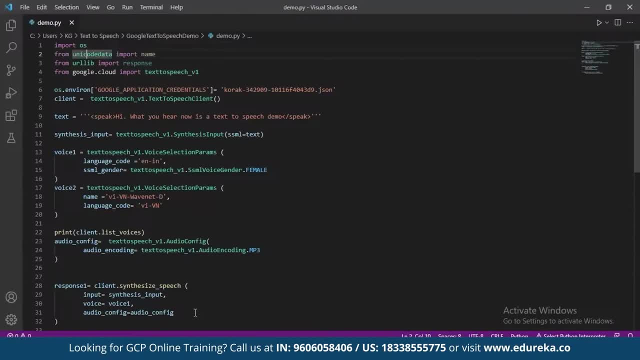 is happening here. So here we are basically importing the service services that are there using text-to-speech, And now what we need to do is cloud import text-to-speech. So this is something that we are importing and this will be used for. 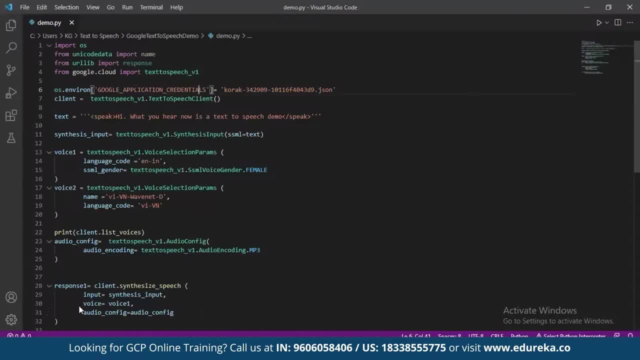 changing text into speech. Now, the second thing here we do is create a virtual environment, and I named the virtual environment Google application credentials. So what do you do after? this is the key that you Created, the json file that you created, So that file has to basically be in here. 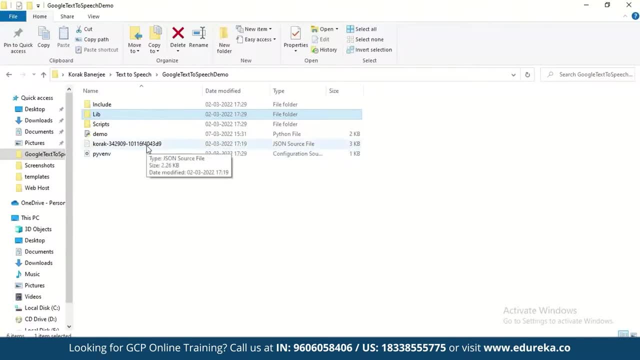 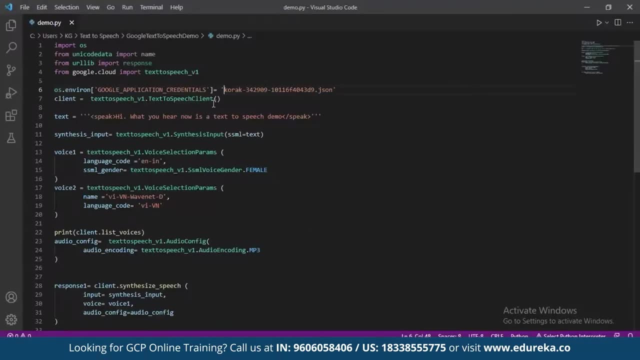 So let's go back here and you can see this is the name of my json file. And if you go back here you can see this file for the json is same and here I'm creating a client environment for python in the CMD right. 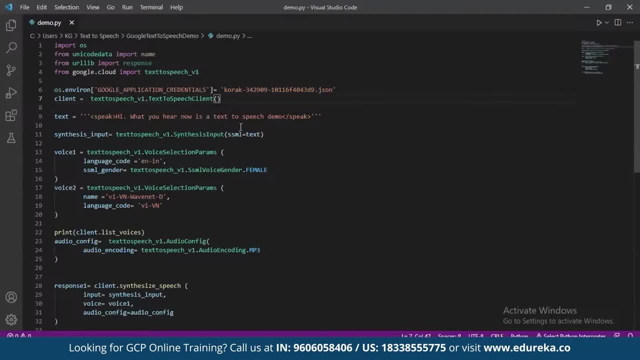 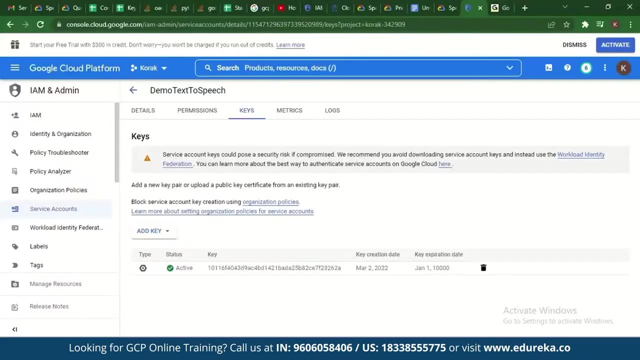 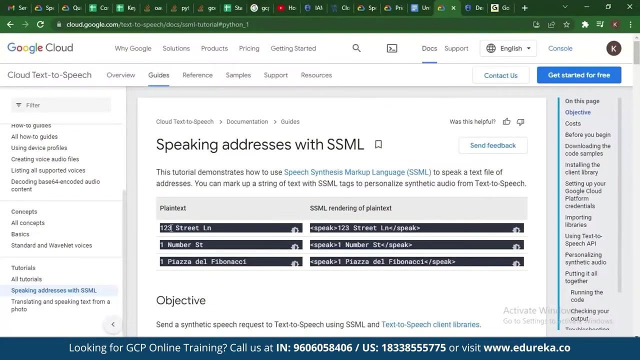 And this is the text that I want to speak. So since we are using SSML here, We want to use SSML syntax. Now let's just go back here and let's just see SSML rendering of plain text. So if you want to say something like 123 street lane, you have to, basically 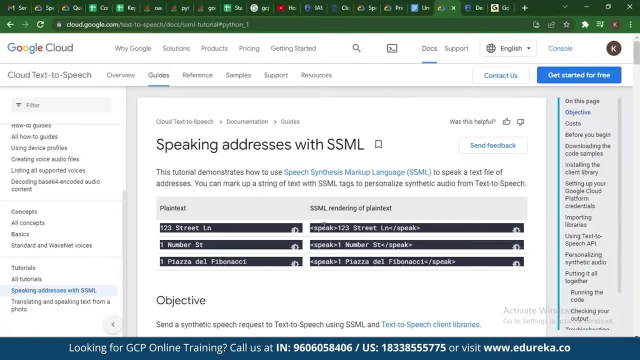 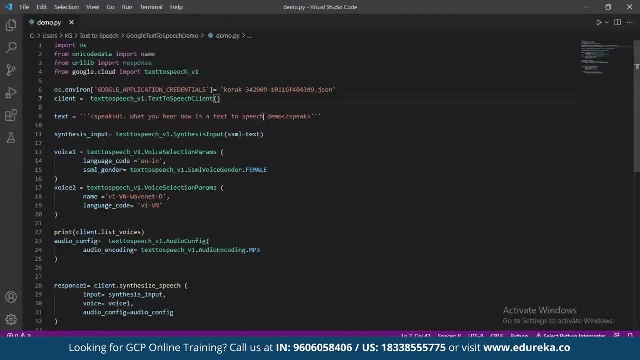 type in the syntax like this, using SSML: So you just add a speak tag here, right? So, similarly, what we've done here is added the speak tag and then added what we want to say. So this is basically Synthesis input, which is another variable that I have defined to. 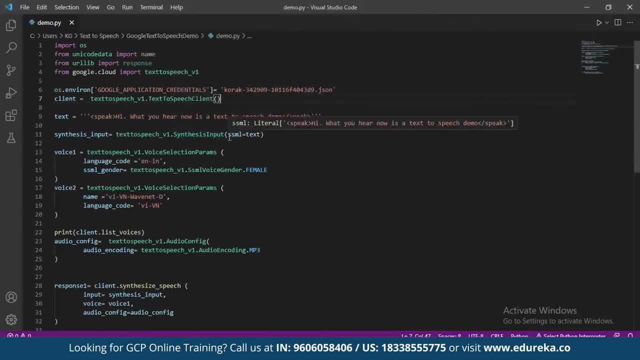 basically use this method right. So synthesis input method will basically use this as SSML and read out the text that I've done. And this is basically another variable where I've basically selected the parameters of the kind of voice I want in my virtual assistant. 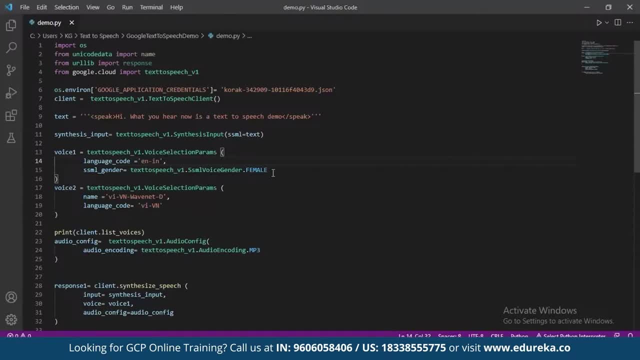 So language code wants you to basically select the kind of language you want your virtual assistant to speak, And SSML gender will basically help you to select the finer things. Let's say, when you want to add pauses, when you want to, let's say, change it. 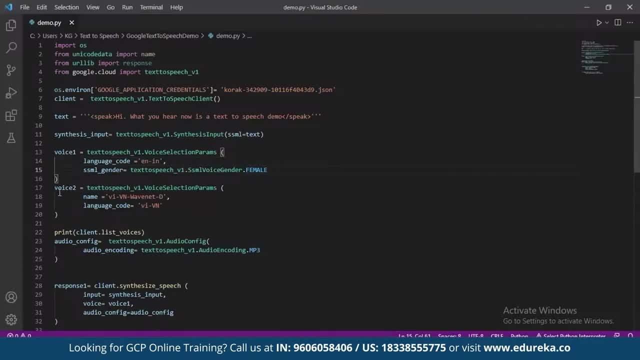 to male, from male to female. all of that and this is another voice that we have, so we can choose to do this or not do this as well. So let's just keep it for now, And what I've done here is since maybe some of these voices are not there in. 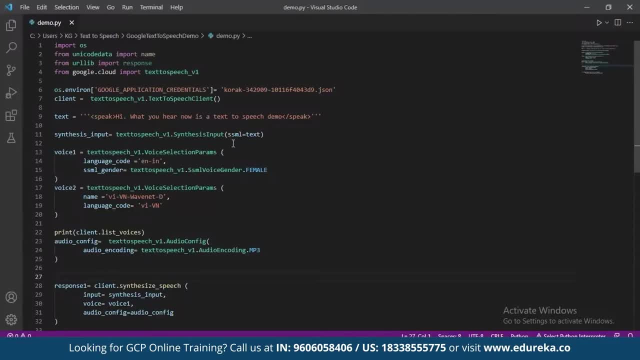 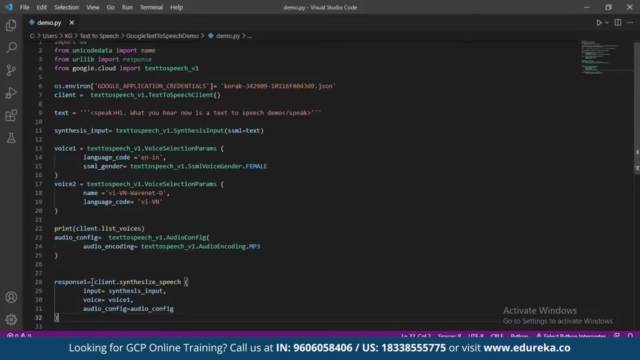 the list of voices that are available in Google Cloud text-to-speech. So we've done this: will Clinton to client and the list of voices that are available, and using that list of voices We are configuring our audio clip right. So there's another variable that I've defined where basically, we talk about. 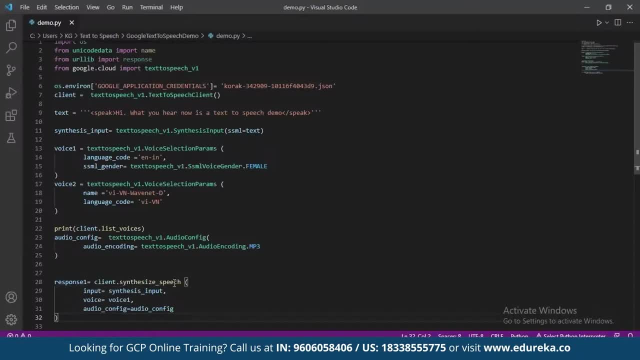 as response one. So this is basically the client response to the synthesized text, where the synthesis input variable in is basically put into the input variable and voice Variable is not the one which takes into account. first voice variable I've defined here in English and in female right so, and then the audio. 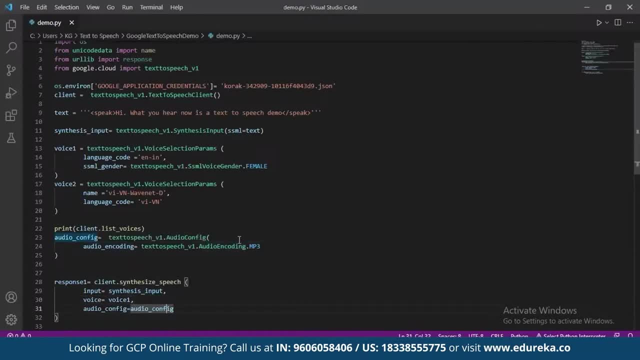 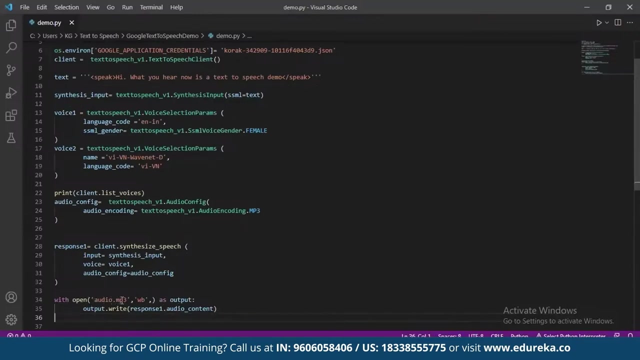 configuration is then seen here. So I've changed it to audio configuration and encoding. so encoding is something that is again used to change the text into speech, right? So, finally, what I've done is, when I basically run this python file, there will be a file called as audiofp3. 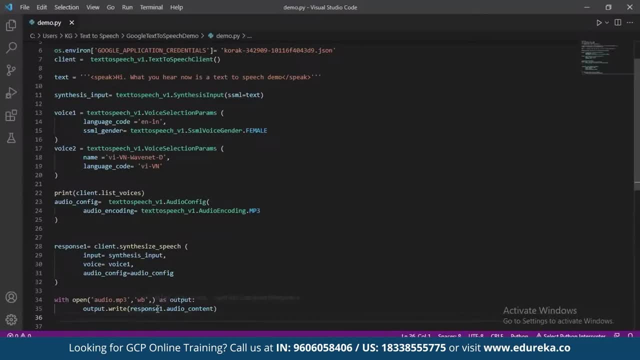 They'll be created, and when I open that audiomp3 file, the response that I'll get is based on this female voice speaking in English. So what I wanted to say is what, hi, what you hear now is a text to speech demo, right? 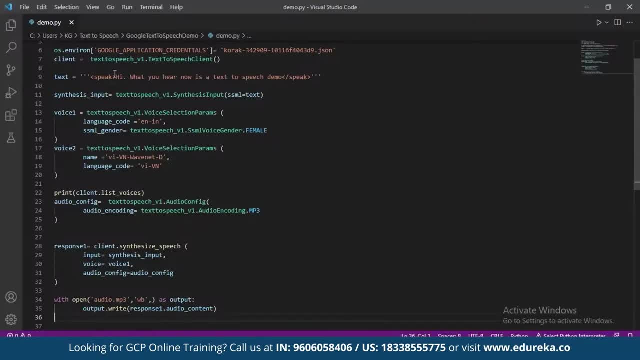 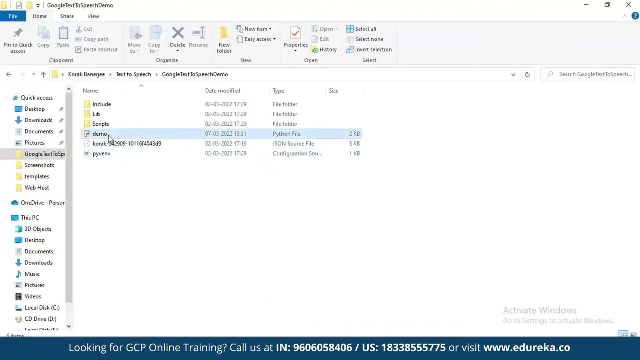 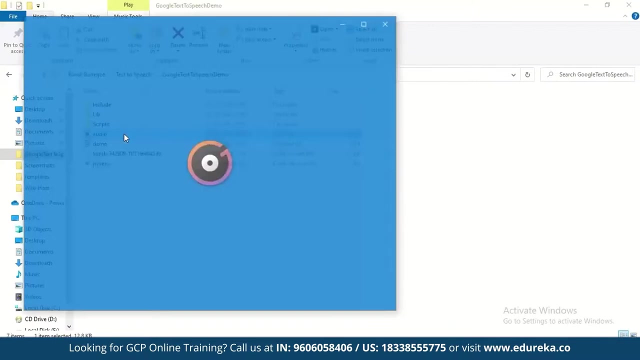 So let's try it out, Make sure that you save everything that you have, and so now just go and run this file and you can see, once you run this file, there should be an audio file. that's there and right. So let's go click on this audio file and hi. 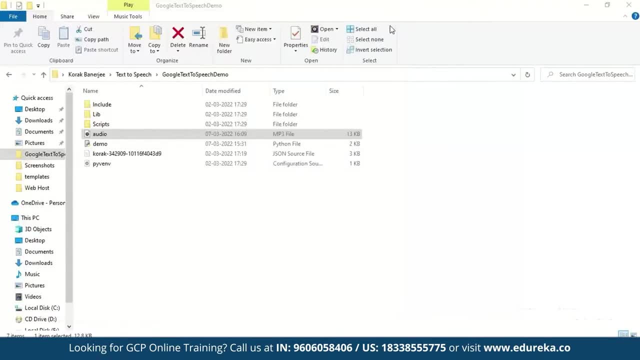 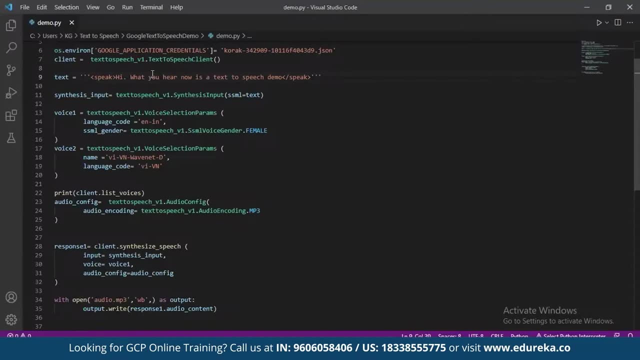 This is a text to speech demo. as you can see here, She's saying exactly the words that I've typed in here. Now what you can do is you can play around with this. You can change a bit. Let's say, you don't want it to be an SSML and you want it to be just plain. 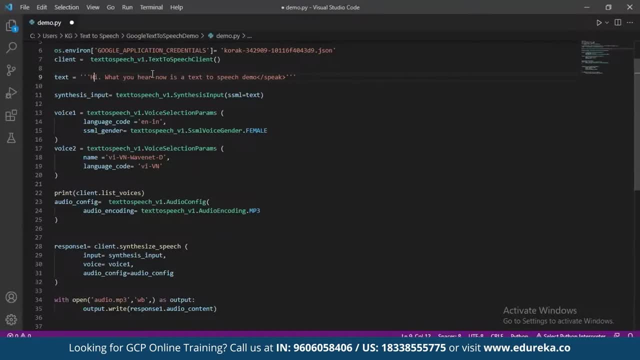 text that is being read out. So all you need to do is just change This and this. let's say hi, right, and here, since you're doing it as plain text, What you need to do here is change this to text Right. 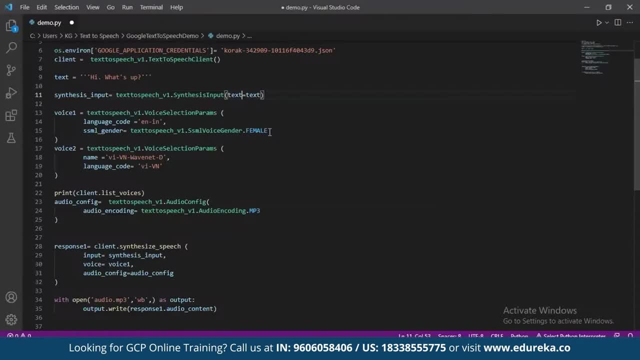 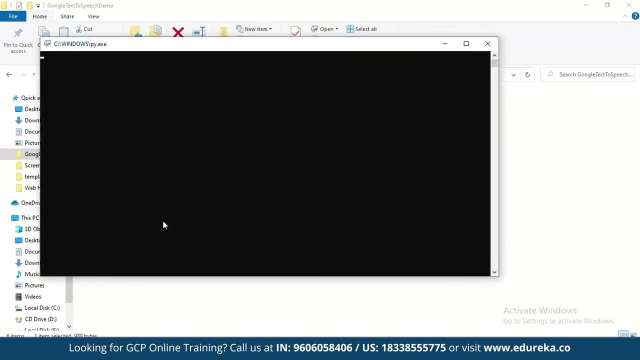 So when I do next, now change to text and let's say: I want a male voice, right, So change this back to male and save it. So now That you've saved it, go back here and let's say: run the file again, Right? 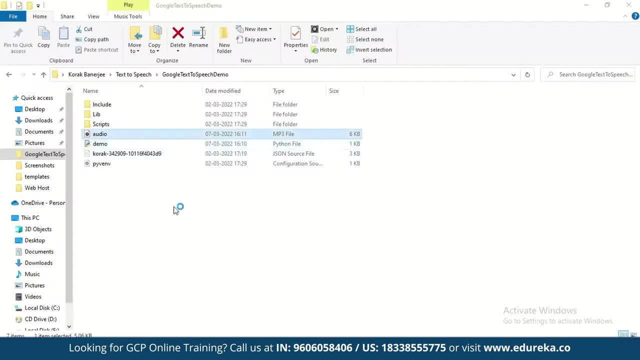 You've run the file and an audio file has been generated. Now Let's play this audio file and see if it's working. Hi, what's up? So, as you can see, the voice has changed to a male voice and it's again. 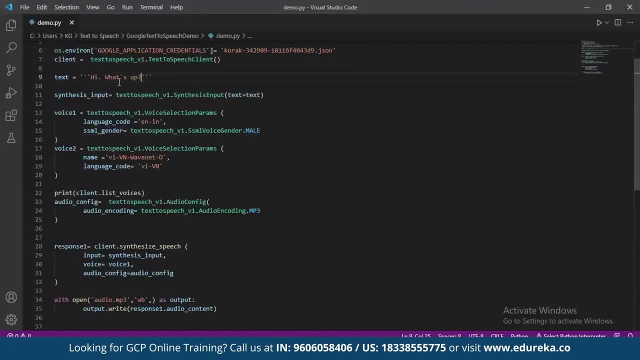 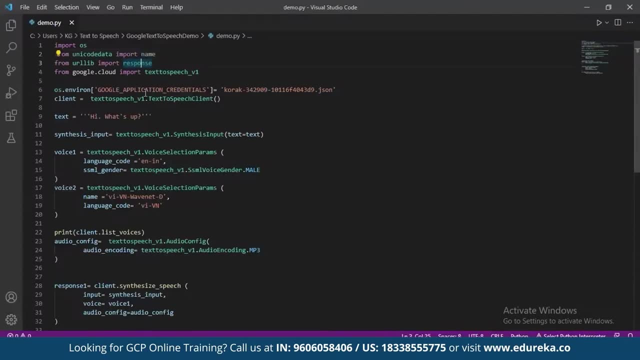 saying what I wanted to say. So since I've changed this, you can see it's saying hi, what's up and not what was written here before. So that is how you Basically use. Google Cloud text-to-speech API is using python, So that is basically the end of the demo. 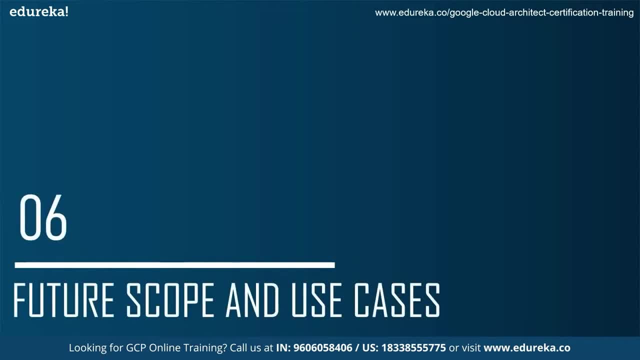 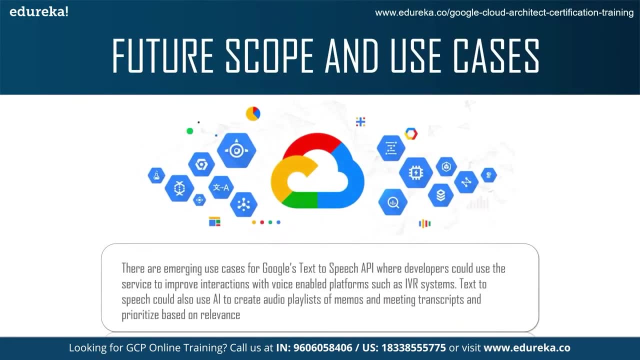 Right. So finally, let's talk about the future scope and this various use cases that Google Cloud text-to-speech has. so Google Cloud platform as a platform which provides its uses various cloud computing services, There are various emerging use cases right for the text-to-speech API. 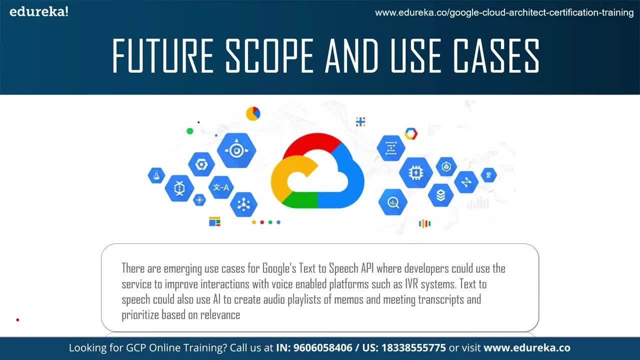 where the developers have used this service to improve interactions between Customers and voice-enabled platforms like IVR systems. So text-to-speech is also being considered with AI to basically create playlists of memos or transcripts, to prioritize data based on relevance of what has been spoken in meetings and other such things that go on in. 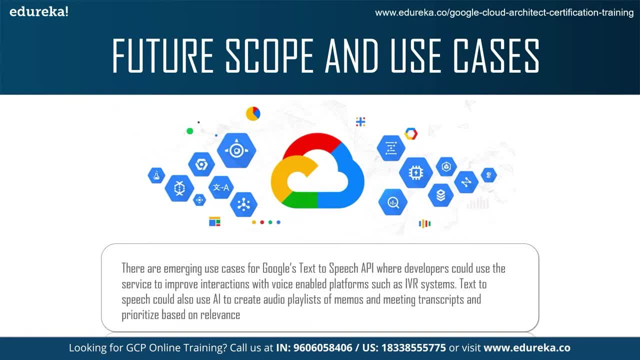 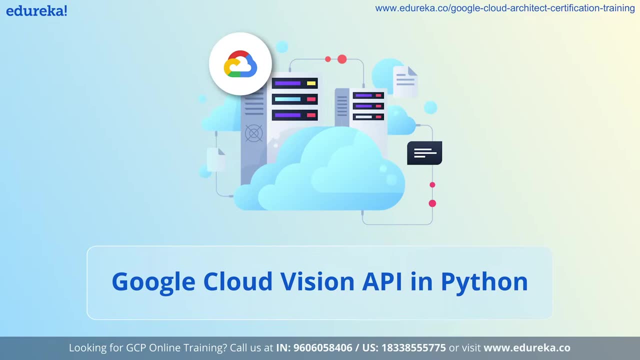 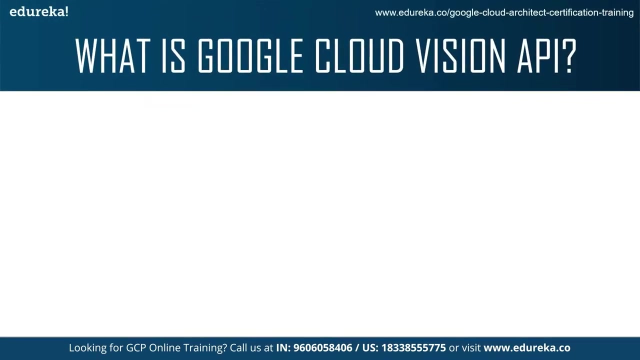 industries. So Google Cloud text-to-speech is really emerging as one of the most used features when it comes to cloud computing and Google Cloud, And it is something which makes has made life way easier. What exactly is Google Cloud Vision API? So Google Cloud Vision API is a machine learning service that is provided. 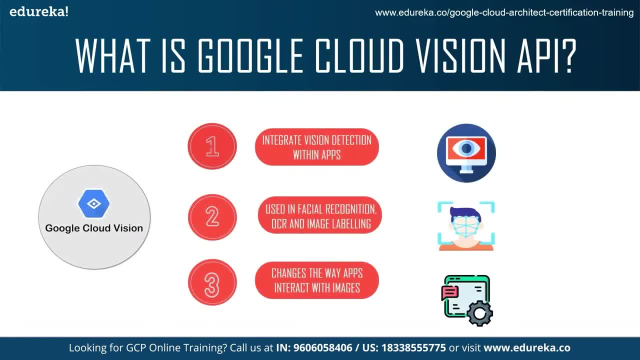 by Google Cloud platform, and this API allows developers to basically integrate vision detection features into their applications, right? So this includes labeling, you know, face detection, CR, which is basically optical character recognition, and it changes the way that apps integrate with images. 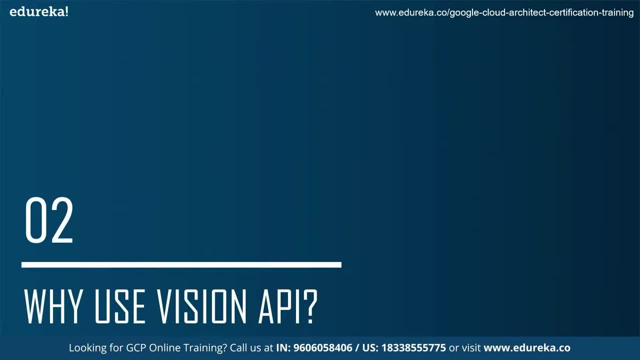 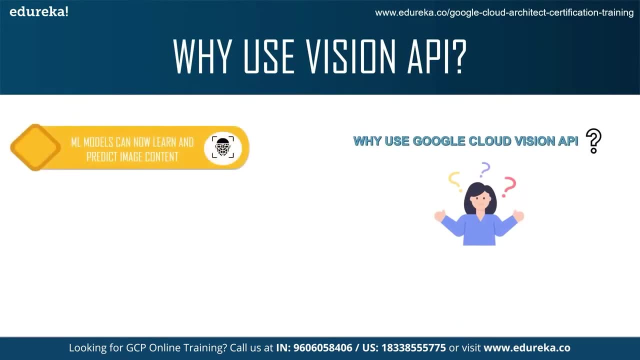 So, after that, what we talk about is: why do we need to use Vision API? So why do we need to use Cloud Vision API? So the first reason why we use Cloud Vision API is the ML models that it provides, because these models can be used, they can learn and predict. 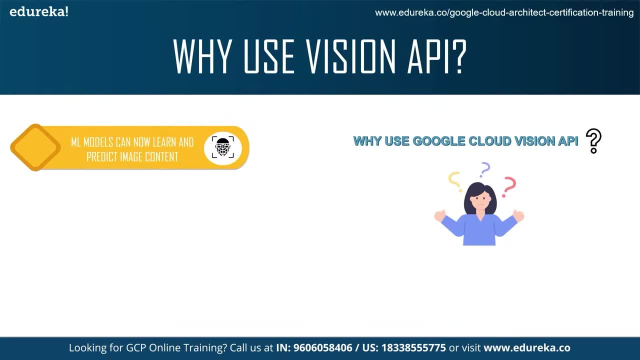 image content very easily, and then basically, the fact that it is a fairly easy to use rest API And you don't need to really do a lot of things and it's fairly easy to learn and, most importantly, it provides pre-trained ML models through the rest APIs that are there. 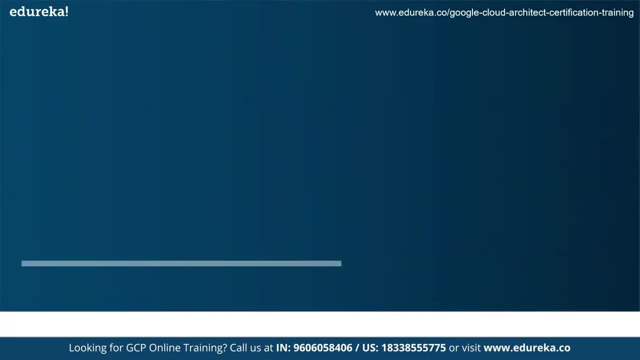 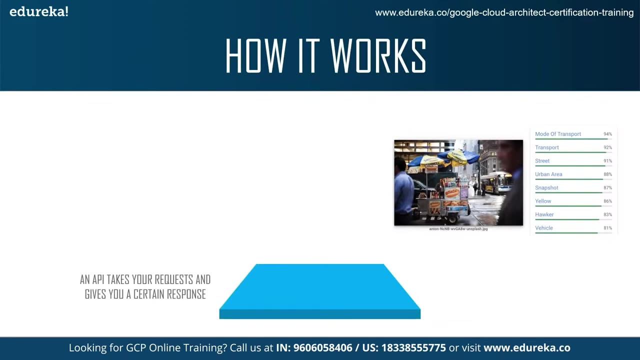 So this is why you need to use Cloud Vision API. Now we talk about how Cloud Vision API works. So, first thing, we see that an API takes your requests and gives you a certain response. So you've given a certain request, the API takes it and gives it to the 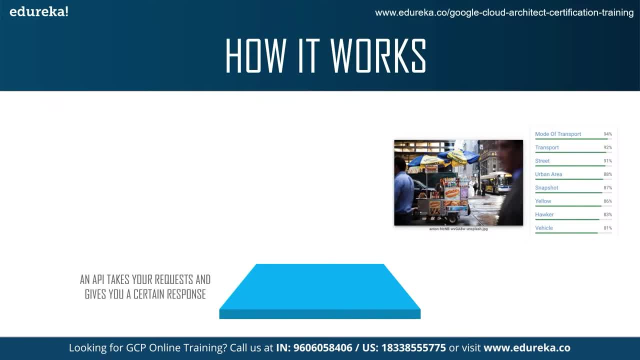 server. The server gives the API the response and then the API gives a feedback to you and next we see that Vision API then categorizes these images that you have. So it helps detect faces, objects, all of that and gives you certain insights on that right. 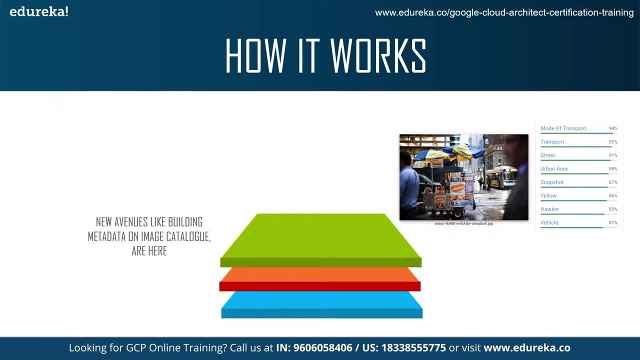 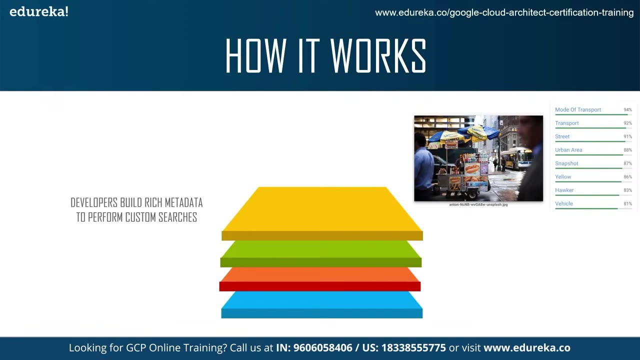 So new avenues like building metadata is basically something that is extremely important when it comes to image cataloging, and image cataloging is something that these developers do. and finally, we see that developers build rich metadata all around to perform custom searches and give good results, as you can see here. 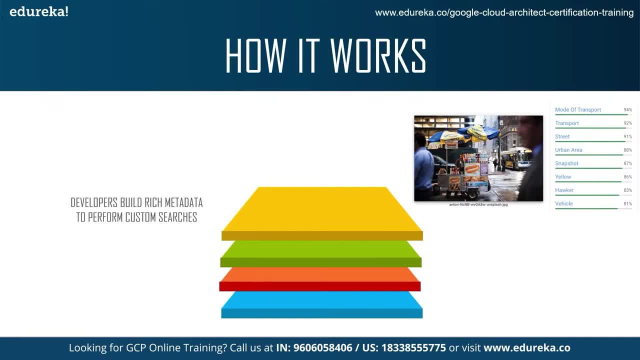 For example, we can see that, for this image that you see here, We have a search which basically gives it labels such as the mode of transport that you can see the transport that you can see the street, that you can see the urban area. So this is what it's detecting from the image that you've put right. 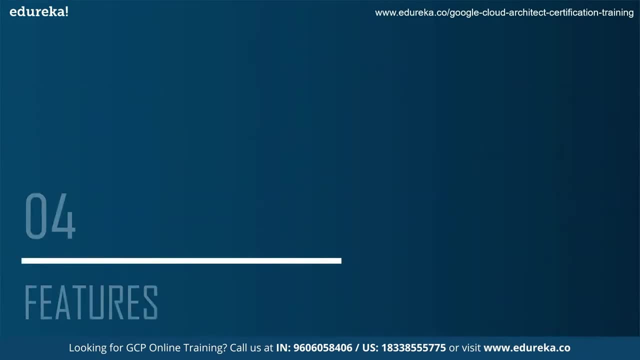 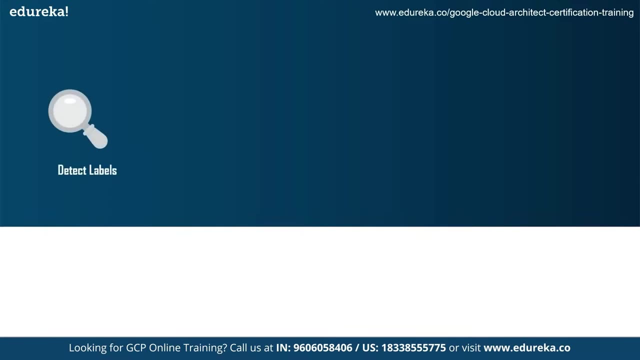 So this is how Cloud Vision API works. Next we come to the features of Cloud Vision API. First thing we talk about is the fact that Cloud Vision API Helps in detecting labels. now, detecting labels basically allows you to extract information about certain entities in an image and you 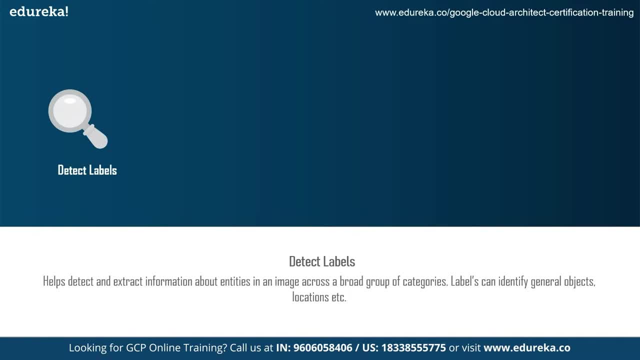 can basically group them in a broader category. So labels can identify general objects, locations etc. So this is one of the features of Cloud Vision API. Next we see optical character recognition, or OCR. now OCR is basically the electronic conversion of images of typed, handwritten or printed 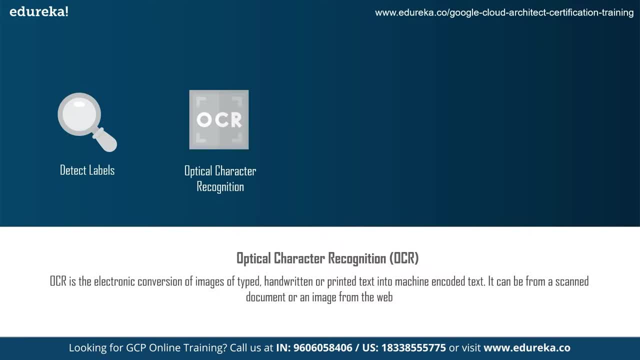 text into machine Encoded text. So what basically this means is that if an image has some sort of text in it, be it scanned, be it imprinted in the image, It doesn't matter. But if there is some sort of text in the image, OCR will help recognize. 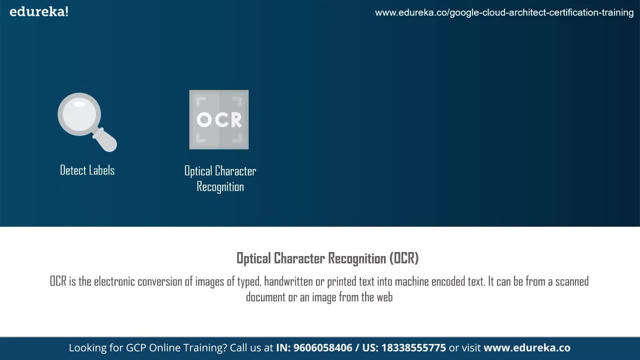 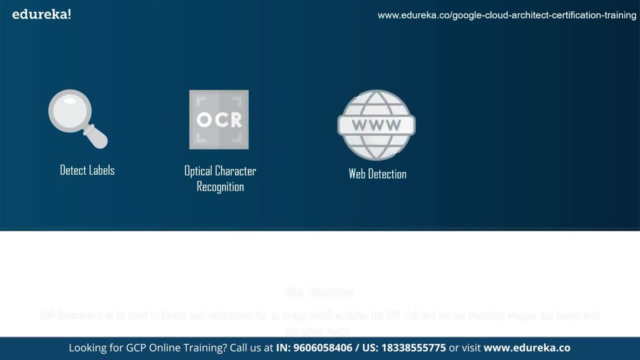 it and then change it into machine encoded text, So this can be from scanned documents or from the web as well. Next, we come to web detection. Now, when we talk about web detection, this basically can be used to detect web references for an image, for the Alexa, for example. 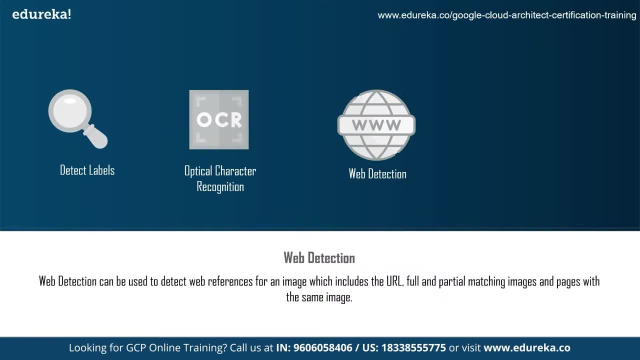 If you use an image from the internet, you can basically check out the URL, the full and partial matching images and the pages that use the same image that you downloaded. So this is what Vision API helps it right. and finally, we come to facial recognition is one of the key features, based on the image. 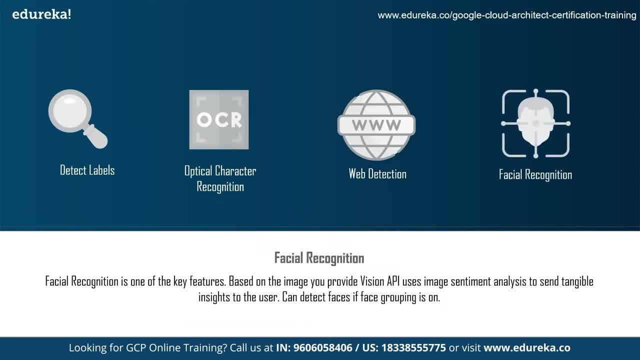 that you provide now. Vision API uses sentiment analysis to give tangible insights to users. Now, these insights can be, let's say, what kind of facial features and structure they have, the kind of person He or she is. you know, these are the insights for facial recognition. 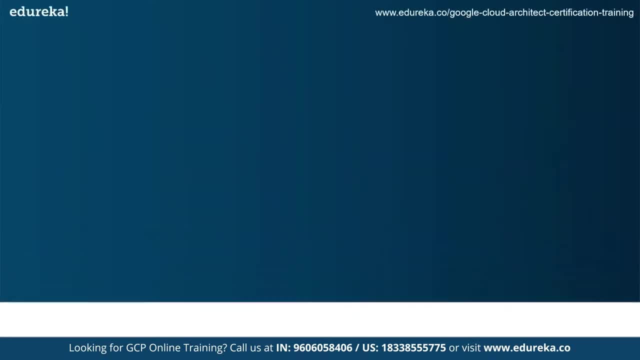 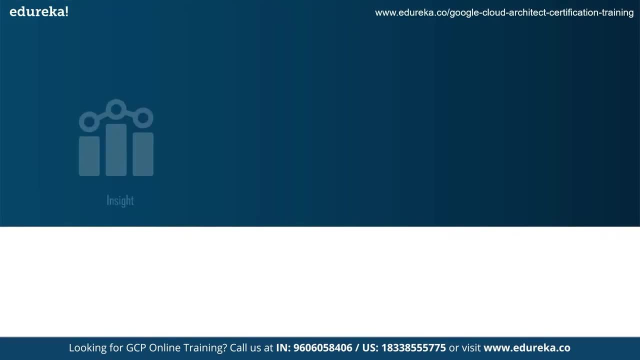 So, basically, this can detect faces of face. grouping is on. So next we come to the benefits of Vision API. Now, Vision API main benefit is that it gives you a lot of insights on any image that you provided with. let's say, for example, that cloud. 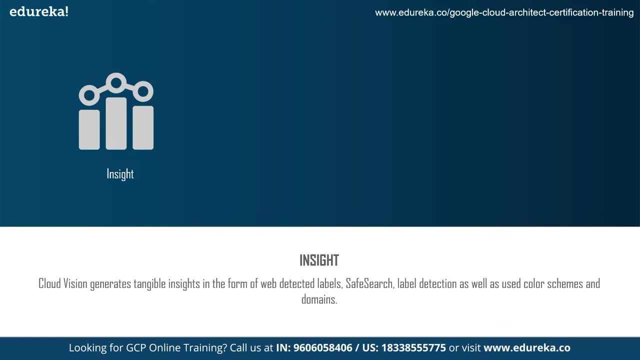 vision generates tangible insights, right. So safe search, label detection and color schemes: are all these different domains that you can use to basically Insights to a certain image. now, all of these are different. Let's say, labels basically tell you the type of image that can be safe. 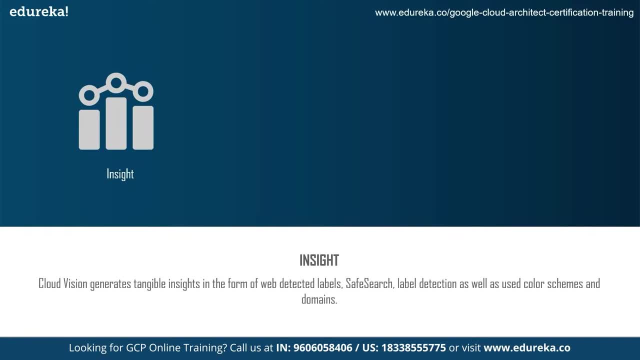 search tells you if your image is safe enough to be on the internet. next we come to in entity detection. Now, entity detection is basically the fact that you can identify web labels, text images within an image and other such entities for the user very easily, and that is a very important benefit as well as 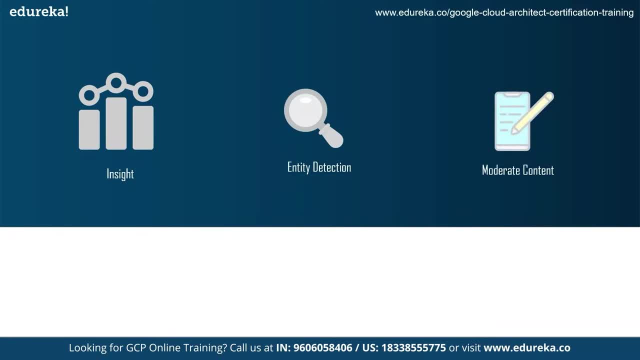 a feature. And then we come to moderation of content. now, which Vision API moderates your content? using safe search. like we talked about before, safe search is basically provided by Google, So exclusive content will be marked unsafe if safe search is on and content is based on user interaction. right. 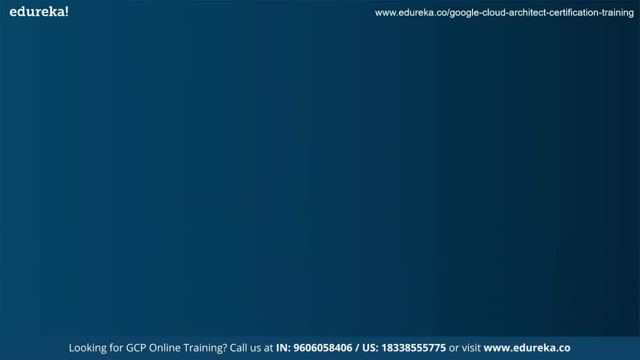 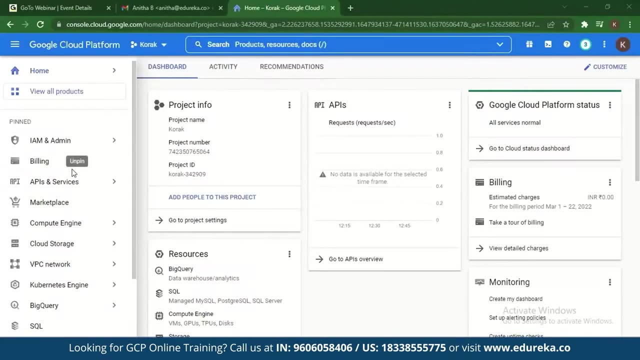 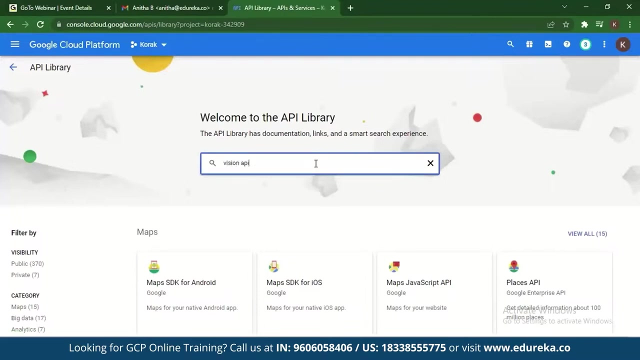 So these are the benefits of Vision API. Then we come to the demo for cloud Vision API. So you go to your Google Cloud Platform account Console and you go to APIs and Services, go library and just type in Vision API- We have cloud Vision API right here- and go to manage. 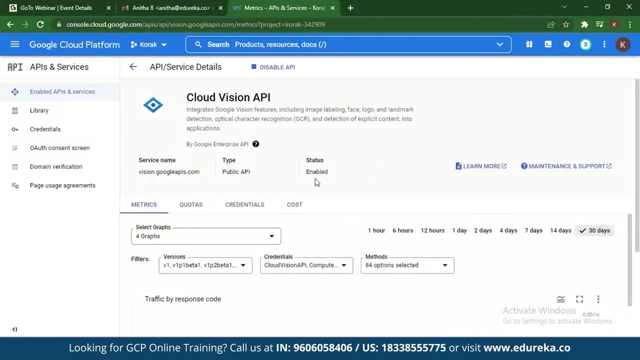 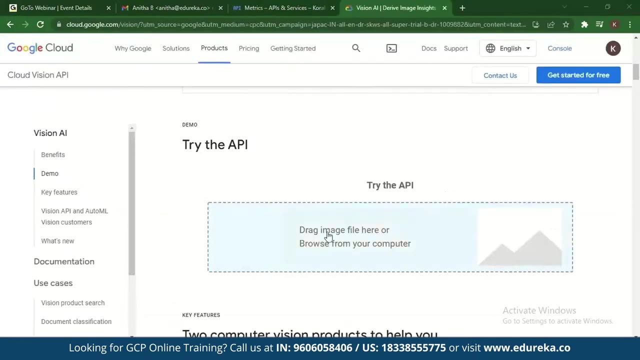 So this is cloud Vision API and this is already enabled, and you have to make sure that before you use any API on Google or platform, you have to enable it separately. So let's check out how Google Cloud Vision Basically gives you insights on certain images, right? 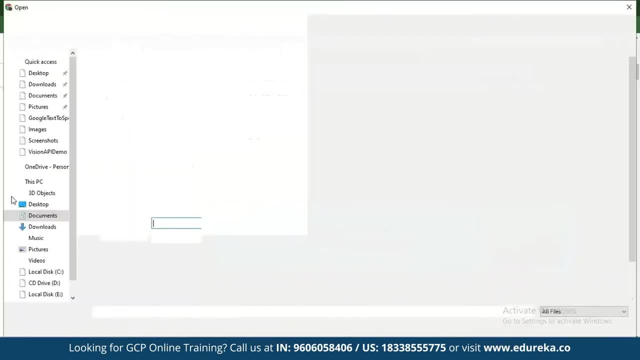 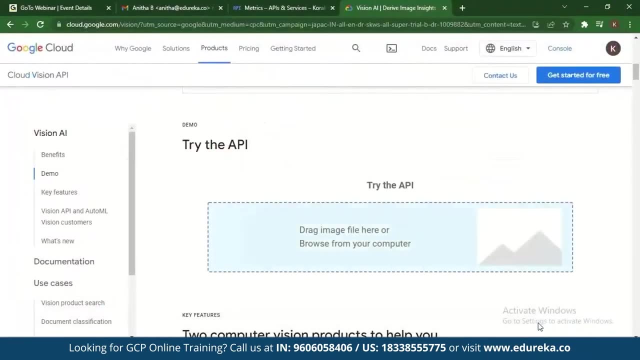 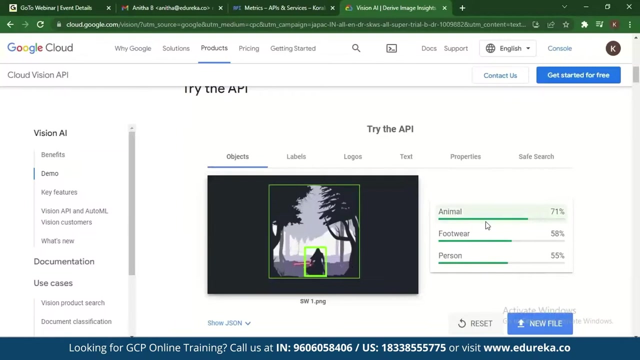 So you can just drag an image in here. Let's say, for example, go in here and check this out And click this as well. So, as you can see, what Vision API does is gives you insights on what the image might or might not be. now, 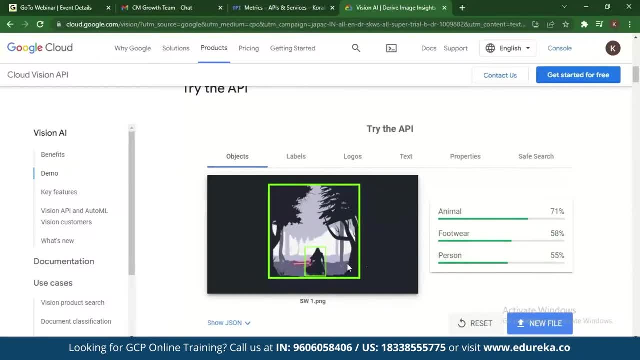 This gives you a chance that it might be a person there, some sort of footwear in the image, And there can be animals as well. So it is 71% share of this, 55% share of this. So there are labels then that it might be a mammal world and all of 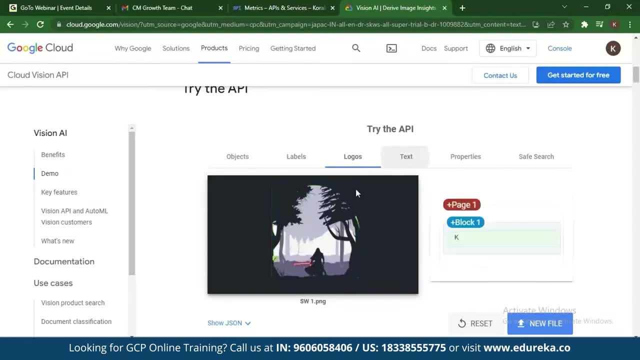 these are different. Next we come to logos text. if there are text, So there's no text here, So basically there is nothing in here, and the properties will basically tell you the different colors schemes that are there here and save search finally gives you the 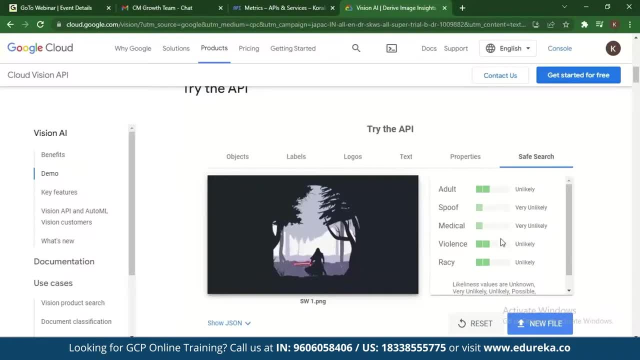 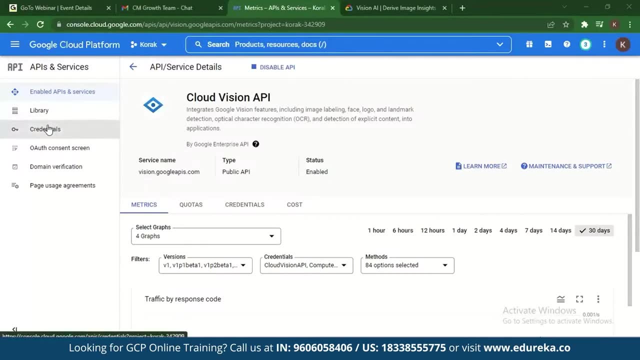 Kind of content the image has to provide. So this is a fair enough image for the internet. So let's check out how to use Google Cloud Vision API with python. So when you go to your console, what you have to do is enable Google. 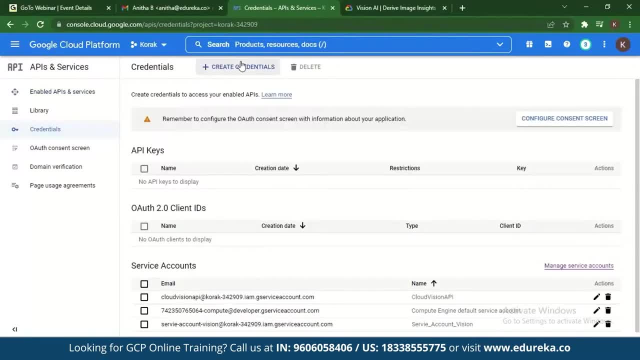 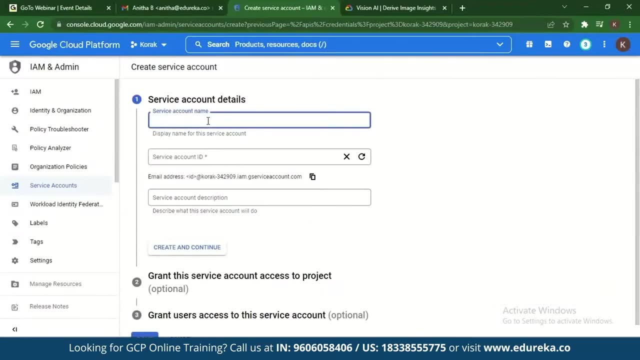 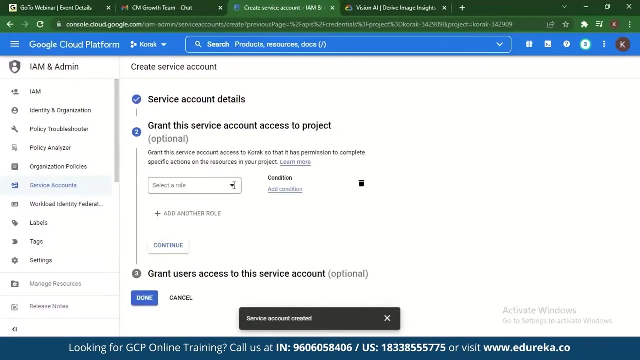 Cloud Vision API. then go to credentials and go to create credentials and go to service account. Now make sure you give the name to your service account, Let's say Vision API- and go to create and continue. Now, here you go, to search role. 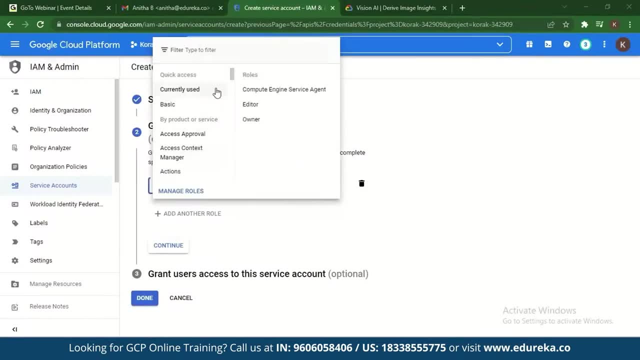 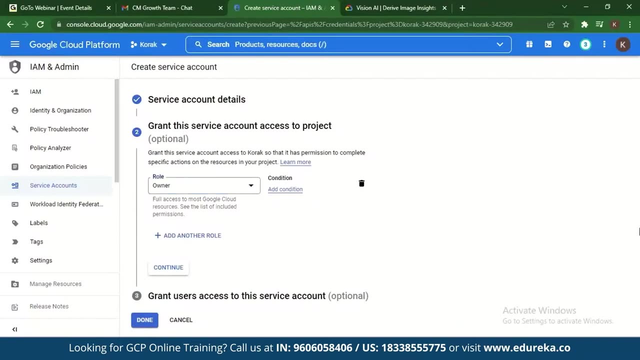 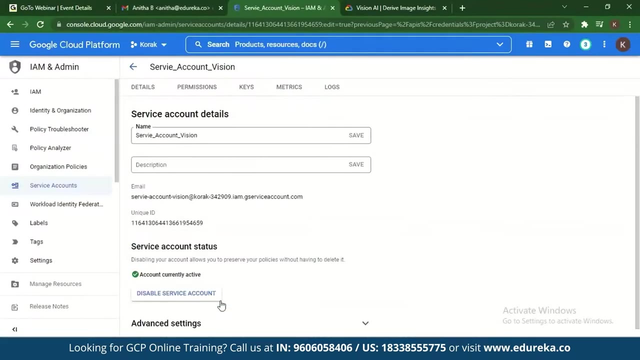 So you go here and you check currently used and you go to owner and this is basically you're granting the access and the role for your service account, right? And then after this, you click on done So. once you've created your service account, you can go check it out. 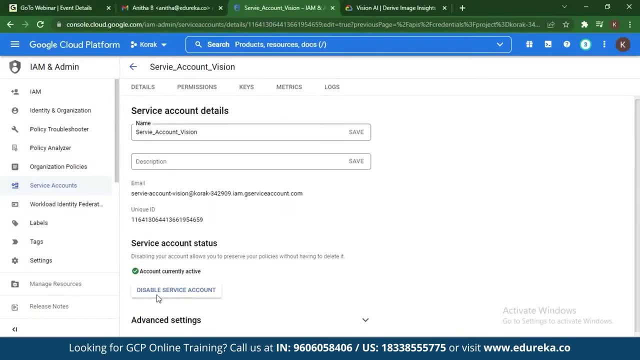 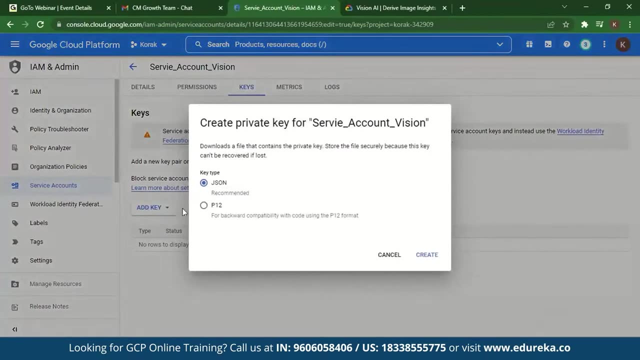 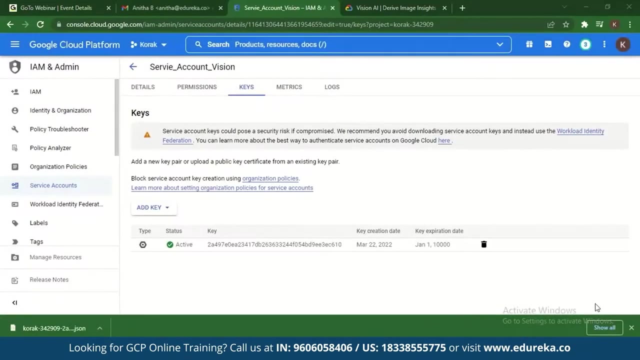 the description of it and basically just go and go to keys. So you basically Then go to key and create new key and download the JSON format and private keys now saved to my computer. So once you've downloaded your JSON file you can then go to your. 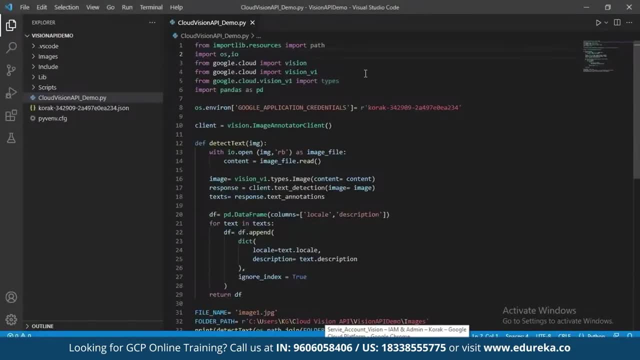 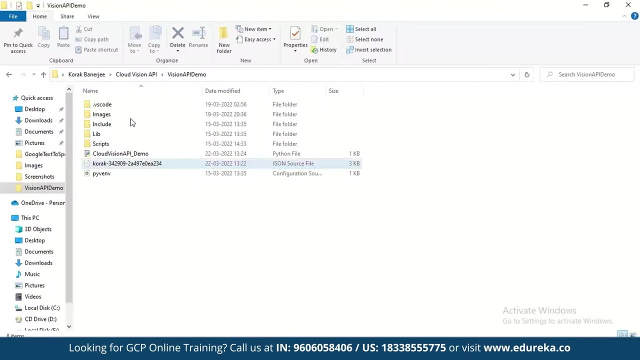 VS code editor and let me just explain this code to you. So before doing any of these, you have to make sure that you have made a python environment. I've named my python environment Vision API demo and this is it, and then you can go to your. 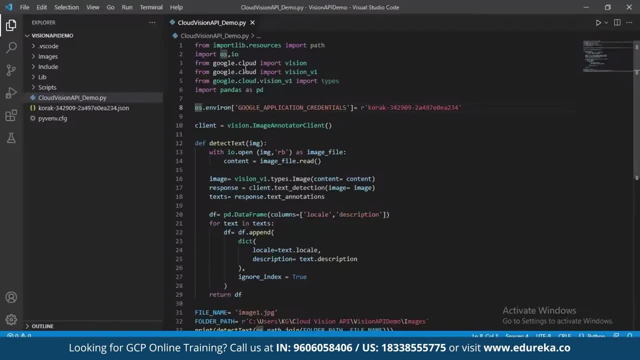 This code. So what you have to do is, before doing any of these, you have to make sure that, through CMD or any PowerShell, you have to install Google Cloud Vision and that once that is installed, you can go to your editor and let me just explain this code now. right, 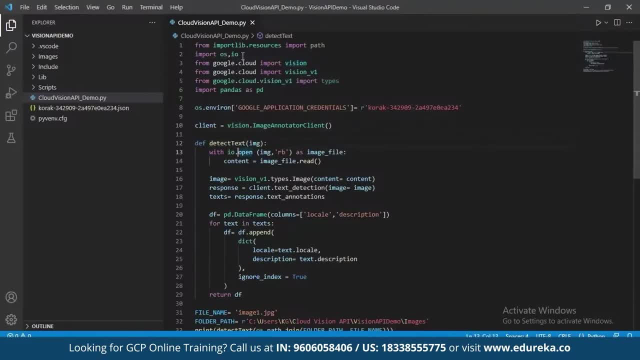 So first you import the OS and IO files. then, from the Cloud Vision API that you installed through CMD, you can import Vision and Vision B1 instances. So these are packages that you can import. So the difference, The difference between Vision and Vision B1 is that Vision B1 has to. 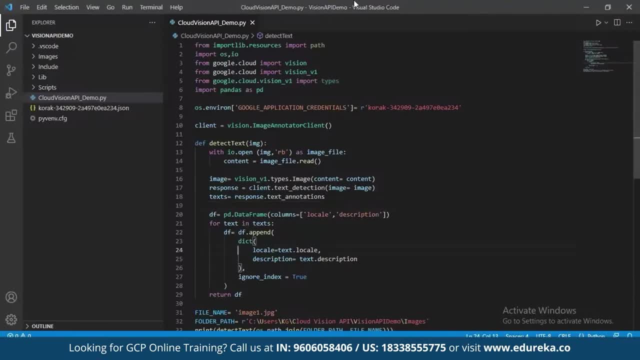 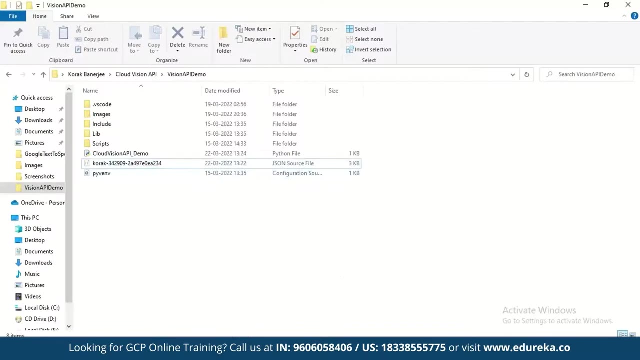 offer two more methods than vision, right? So the next thing we do is that we have to create Google application credentials and once that is created, this is what your JSON file is used for. So just go back here and use this as your name for the JSON file and 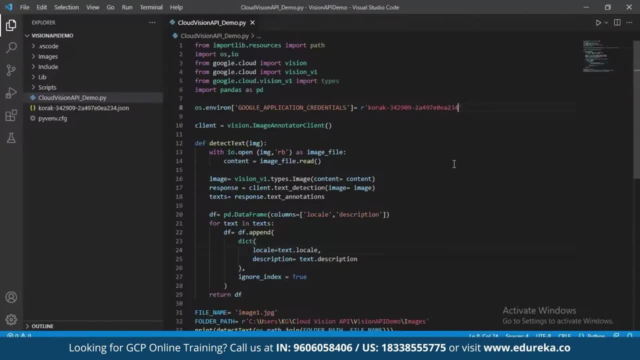 as you can see, this is the name of the JSON file, and you just have to put your name in here. So the next thing we do is go move to client Now. here we basically use the Vision Image annotated client method. Now, what we can see here is that we are defining a detect text method. 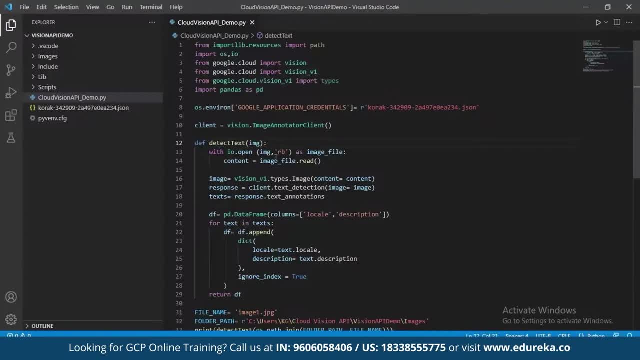 Now, detect text is one of the functions from Google Cloud Vision V1.. So here you can see: we have defined a function- detect text- and this is the code for it, and what this means is that detect text is one of the features of Vision V1 and that is where it's imported from and what 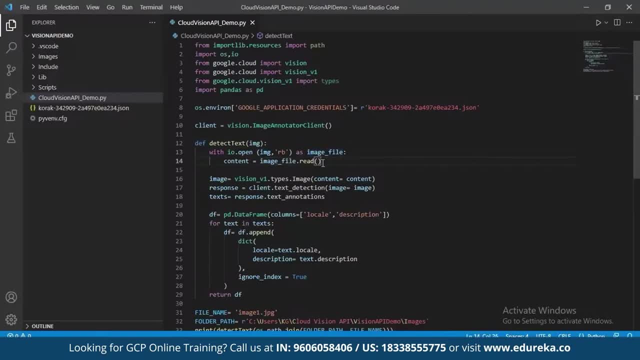 it does is reads content from the image file that you have, right, And after this what we do is that we have a response for the image that is being read, right. So whatever is being read is then responded as annotations to the user, right. 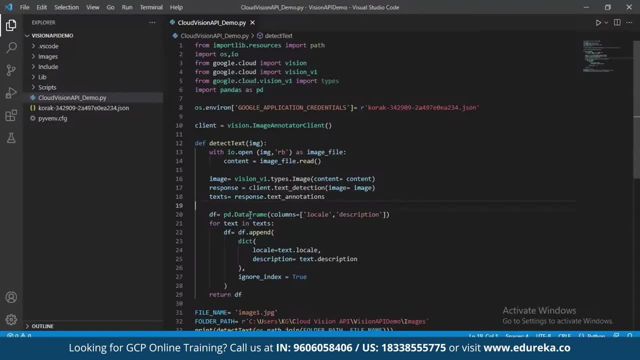 And here we've imported pandas. before now, pandas is basically used for dataframes- SQL And other such, let's say, Excel and all of that. now pandas will be used for dataframes, and this is the code for it: PD, or dataframe columns, and this will show me the location of any text that we have in the image. 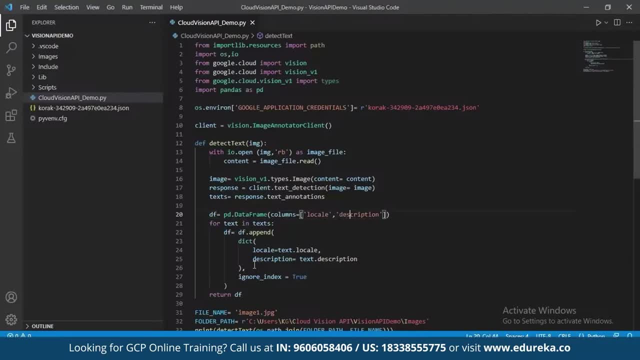 and the description that is there. that is description of the text that is there in the image. Now what we've tried to do here is another version of OCR where, basically, optical character recognition will happen. It will detect text from the image that is present there, right? 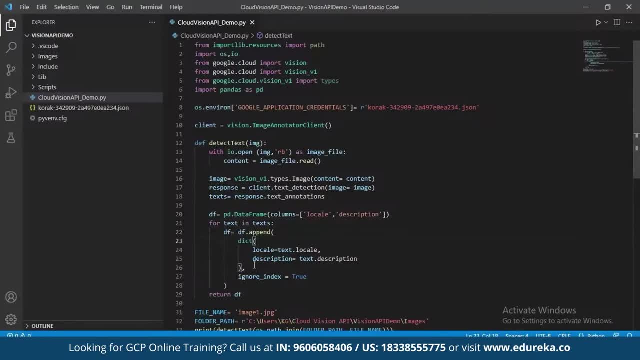 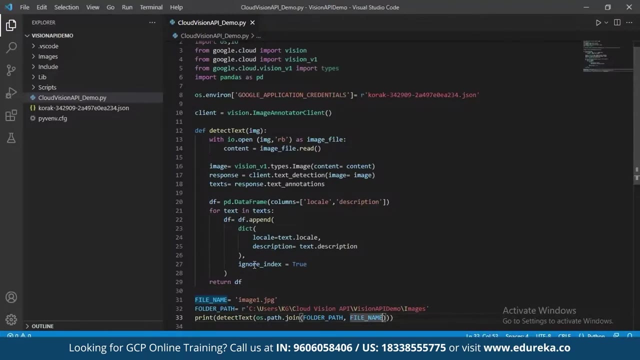 So the next thing we do is, after this, add the dictionary and add extra descriptions and look out right and then return the function for it. The last thing we do is print our file name and the image that you want now for this. views print, detect, text, OS, dot, path, join and the. 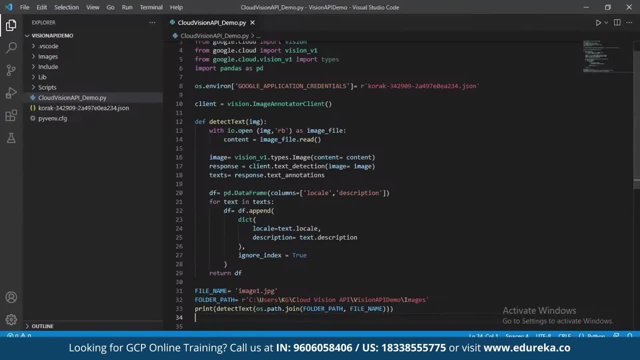 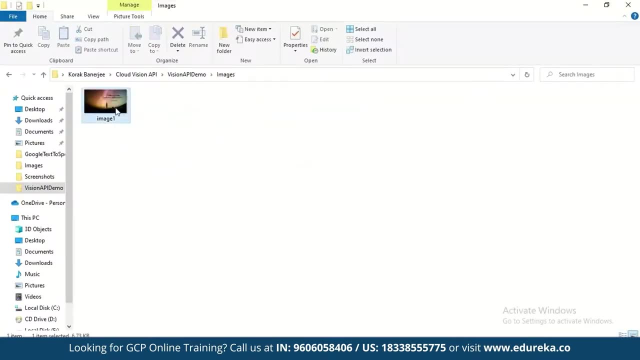 file name and folder path. Now what you need to do is run this. Now, before you run this, make sure that you have the image that you want open. Let's go and check out images, and this is the image, and you can see there is some text here. 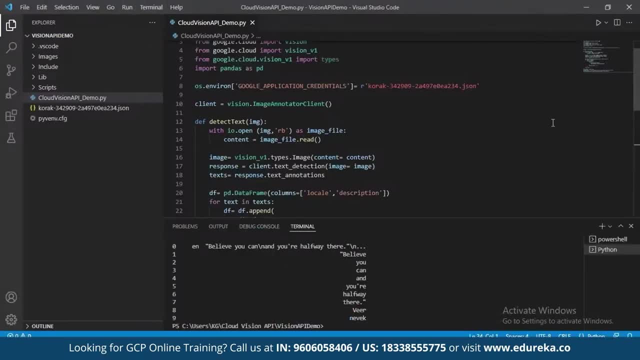 So let's go try and run this code right. So, as you can see, it's basically giving us an output and this is the text that you have here. If you go up here, you can check that. the location of the text in the 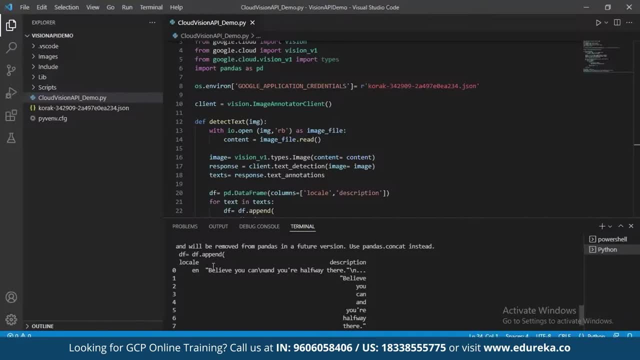 image and the text that is there has been Given the entire text You can see here in one line and here we talk about the locations. that is there for locale and description. Let's check the image Now. the image says: believe you can, and you are halfway there, right? 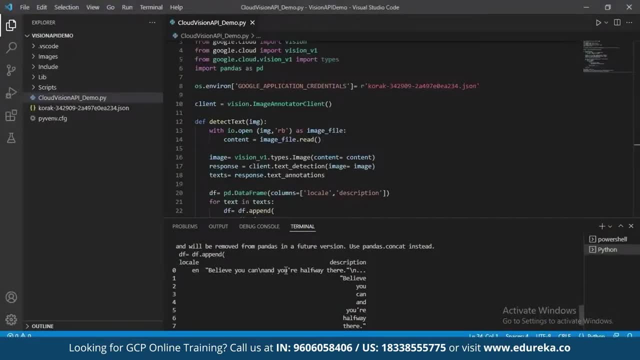 And let's go back here. So this is the image text that is present and for location one, We have believe this is true, that you can and, like this, you can see that Google Cloud Vision API is helping me detect the text that is there in. 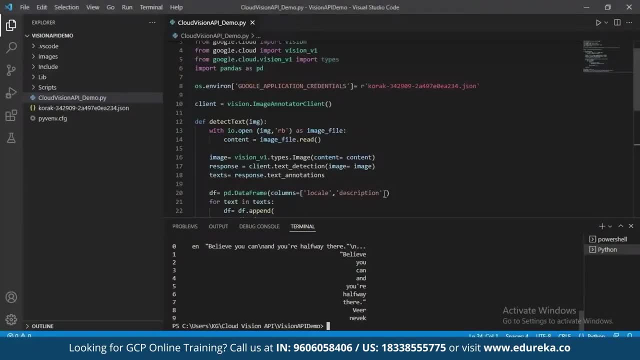 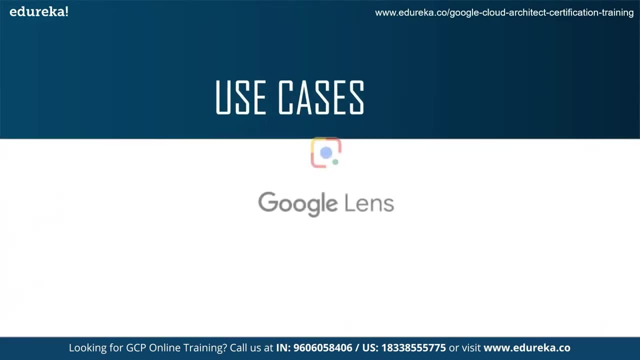 this image right. So this is how you basically use Google Cloud Vision API using Python. Finally, we come to the use case for Google Cloud Vision API, which is nothing but the Google Lens. Now Google Lens is the most popular and widely used case for Vision API. 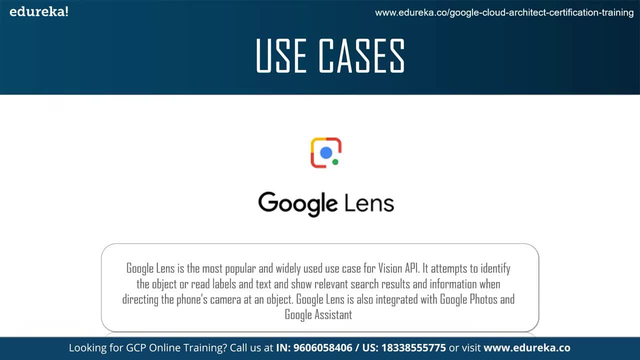 So Google Lens attempts to identify the object or delete labels and text and show relevant search results, right? So what you're doing is basically You're directing the phone's camera at an object and that, when directed towards the object, will basically give you insights on whatever you're. 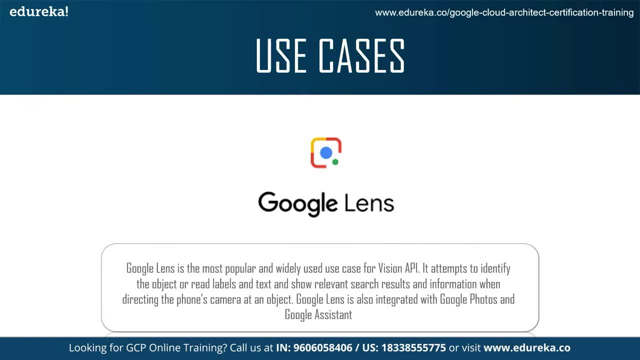 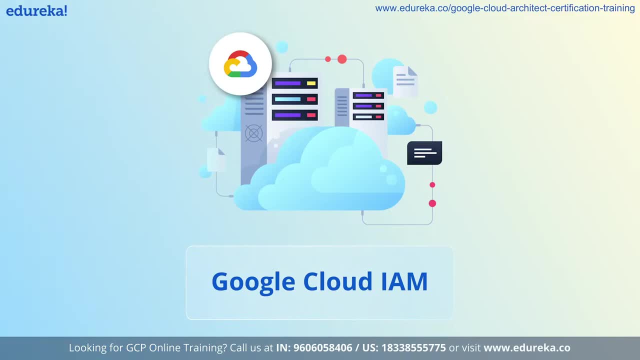 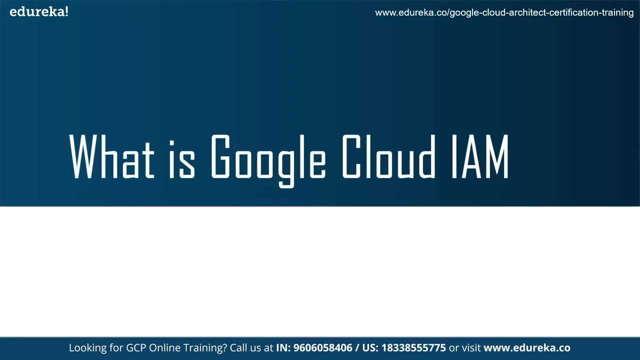 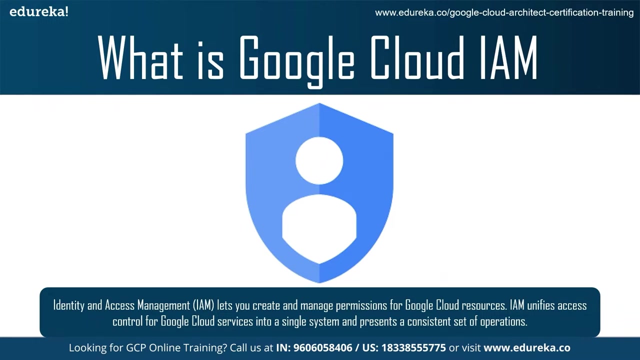 pointing it at right. So Google Lens is also integrated with Google Photos, Google Assistant and other internal Google services that are there present What Google Cloud IAM is. so IAM, which means identity and access management, lets you grant Granular access to specific Google Cloud resources and helps prevent access. 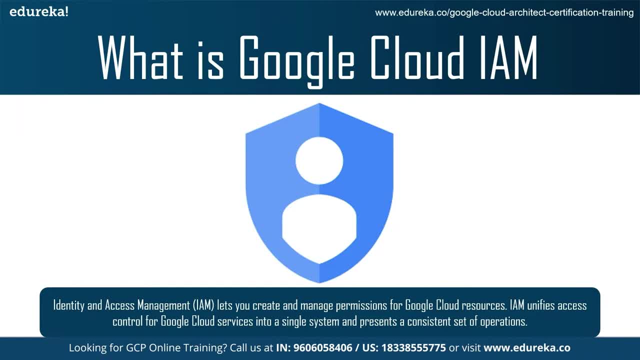 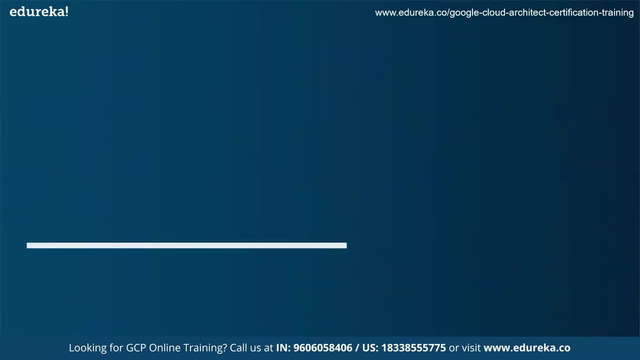 to other resources. I am lets you adopt the security principle of least privilege, which states that nobody should have more permission than they actually need. Let's now understand how Google Cloud IAM works. first, Let's take a real-time example, or say real-life scenario. 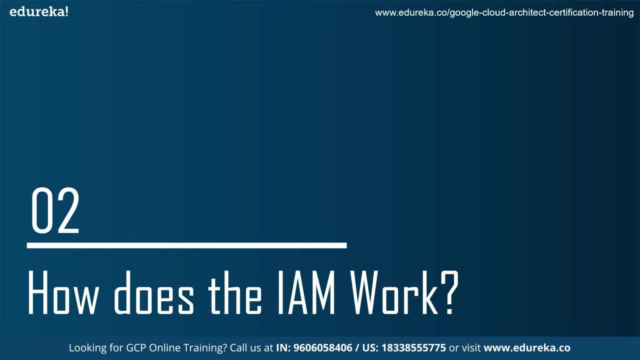 Suppose, if you enter a company and you got the visitor card, so you have a very limited access through it, Like, you can access reception, You can access cafeteria, You can access a lobby where you can rest. Okay, now suppose you got selected in that company. 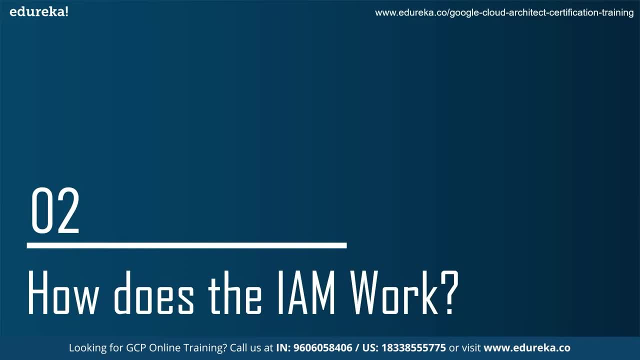 Okay, you got selected as a pressure in the position of junior analyst. You can say: now you have much more access than cafeteria, reception and Lobby. Now you have access to certain databases, You have access to certain- maybe cloud- resources also little bit better. whatever is required for you for analysis purpose. 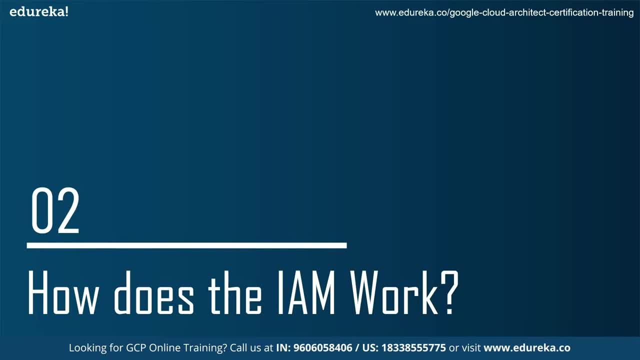 Also, you can have access to various analytical tools also, but you don't have complete access to all of them. Suppose now you are working under a senior research analyst. their senior research analyst- or you can say senior analyst- have much more access than you because you are a junior analyst. senior analyst have much more access. 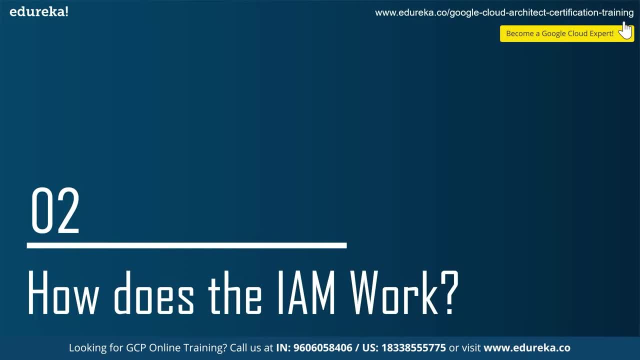 to more cloud resources. He has more access to much more Excel sheets. Also, you can say, and also like various other analytical tools also. now suppose there's another person who isn't an analyst team, He's in cloud team, say he's a cloud engineer. 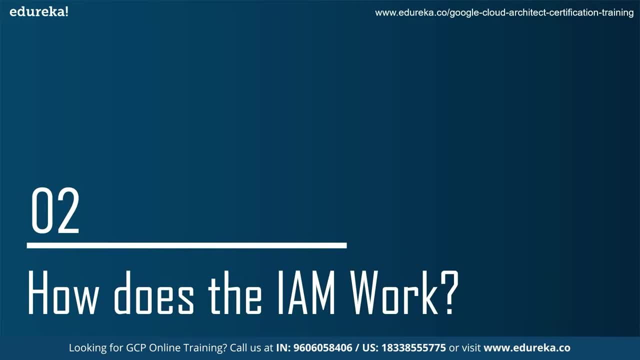 So now you can see, he might having the access of a lot of cloud resources compared to you, but he won't be having access to certain database services which you have access to, certain databases also which you have access to, a certain analytical tools also which you have access to. he might not be. 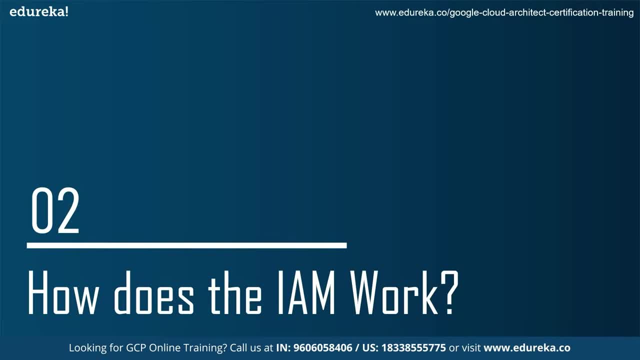 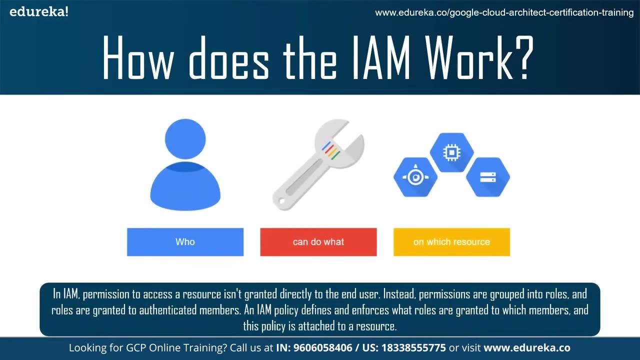 having that access. So that's how a certain rights and certain accesses are being provided to different teams and depending on their work. This is just. you can say it as a real-time example. Okay, that's how access and identity management works. So now let's understand how I am works in Google Cloud with. I am you manage? 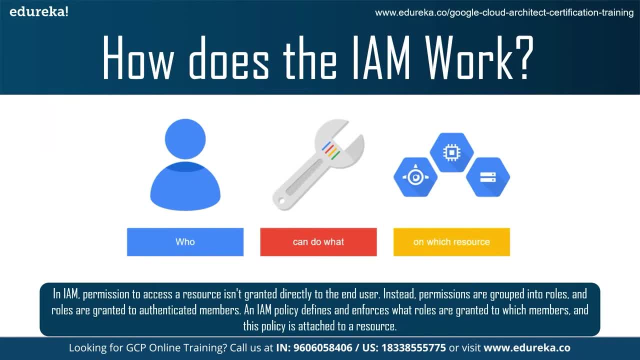 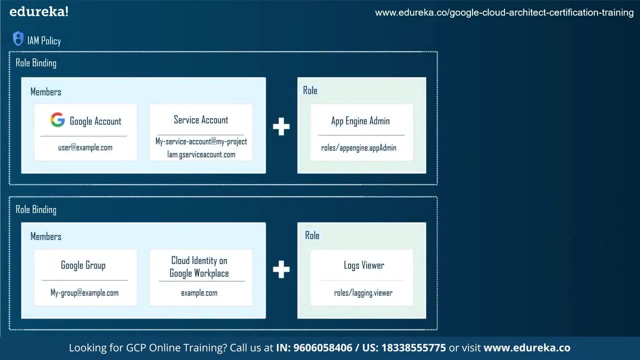 access control by defining who means identity, has what access means role for which resource. for example, compute engine, virtual machine instances, Google Kubernetes, engine clusters and cloud storage buckets are all Google Cloud resources. The organization's folders and projects that you use to organize your resources are also resources in I am permissions to access a resource. 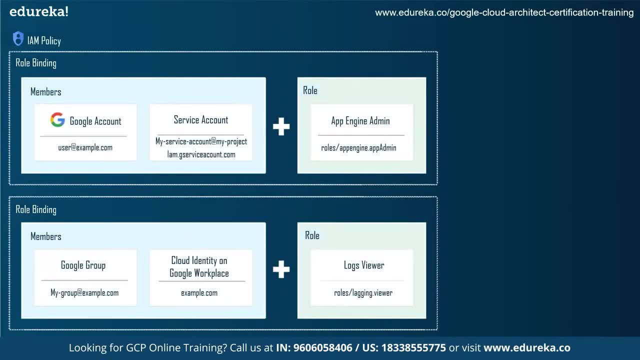 isn't granted directly to the end user. instead, permissions are grouped into roles, and roles Are granted to authenticated members and I am. policy defines and enforces what roles are granted to which members, and this policy is attached to a resource. when an authenticated member attempts to access a resource, I am. 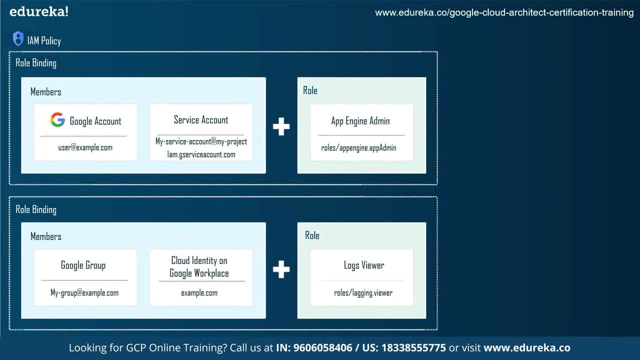 checks the resources policy to determine whether the action is permitted. You can see this following diagram illustrates permission management in I am. this model for access management has three main parts. The first part is member. So a member can be a Google account- You can say for end users- and a service account. 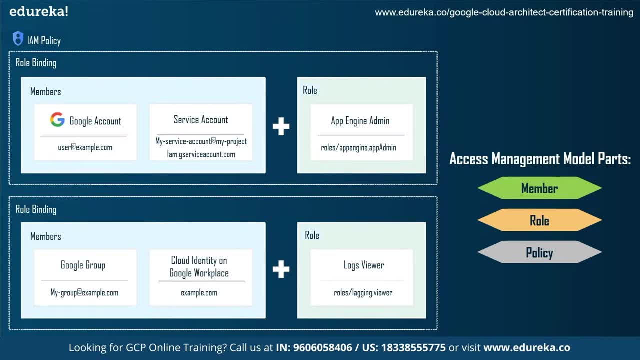 You can say for apps and virtual machines. and then there is a Google group or our Google workspace or cloud identity domain that can access the resource. The identity of a member is an email address associated with a user service account or Google group or a domain name associated with Google. 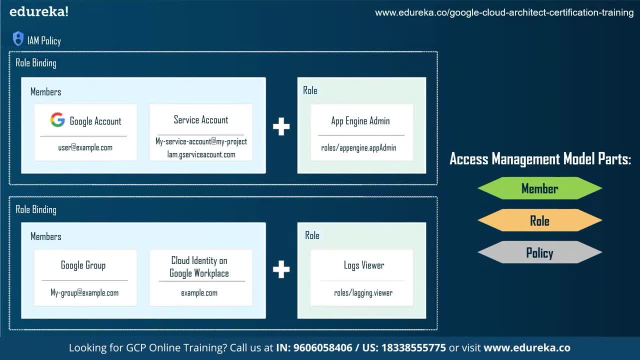 workspace or cloud identity domains. Then there is a role. So a role is a collection of permissions. permissions determine what operations are allowed on a resource. When you grant a role to a member, you grant all the permission that the role contains. Okay, and then there is policy. 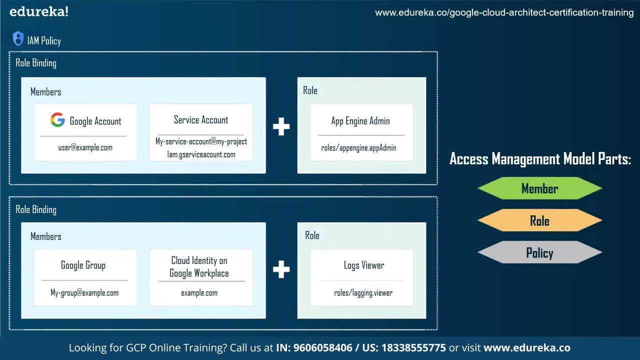 So the I am policy is the collection of role bindings that bind one or more members to individual roles. when you want to define who has what type of access means role on a source, create a policy and attach it to the resource. Now let's understand the concepts in I am first. 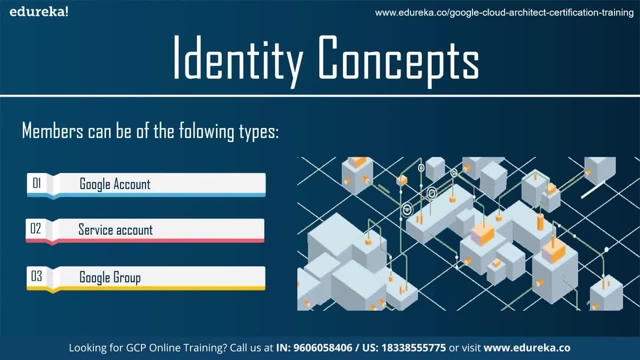 Let's understand the concepts related to identity. So in I am, you grant access to members and members can be Following types like: it can be a Google account which represents our developer and administrator or any other permission who interacts with Google Cloud account. can be an identity, including gmailcom or other. 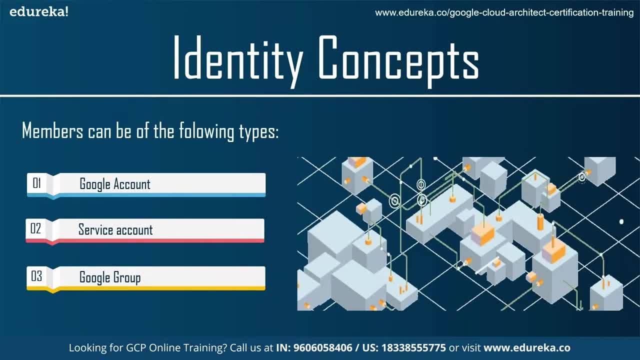 domains. new users can sign up for a Google account by going to the Google account signup page. Then there is service account. a service account is an account for an application instead of an individual end user. when you run code that's hosted on Google Cloud, the code runs as the account you specify. you can. 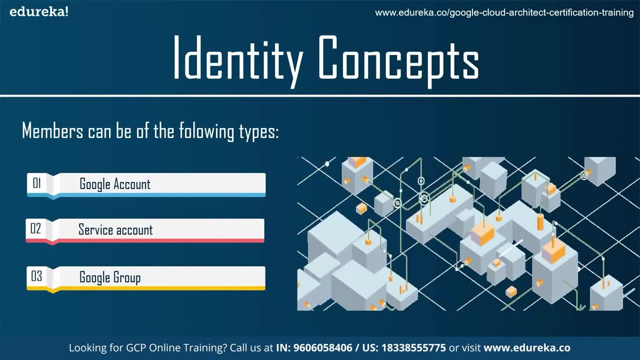 create as many service accounts as needed to represent the different model components of your application. Okay, then there is Google group. So a Google group is a named collection of Google accounts and service accounts. Okay, and every Google group has a unique email address that's associated. 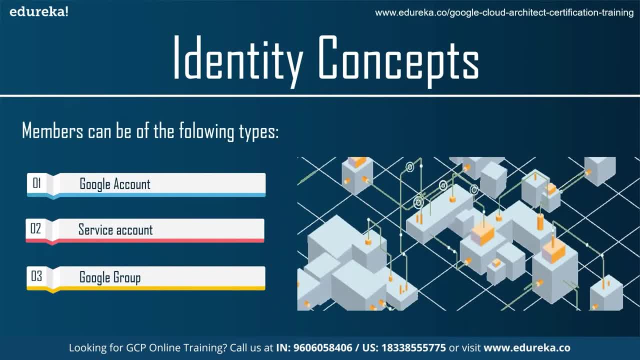 with the group. You can find the email address that's associated with the Google group by clicking about there. is this option about on the homepage of any Google group? Google groups are a convenient way to apply an access policy to a collection of users. You can like, grant and access access controls for a whole group at once. 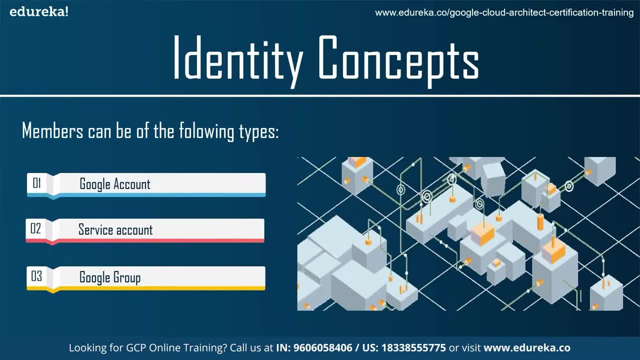 instead of granting or changing access controls one at a time for individual users or service accounts. You can also easily add and remove members from a Google group. instead of updating and I am policy to add or like remove users. Google groups don't have login credentials and you cannot use Google groups to establish. 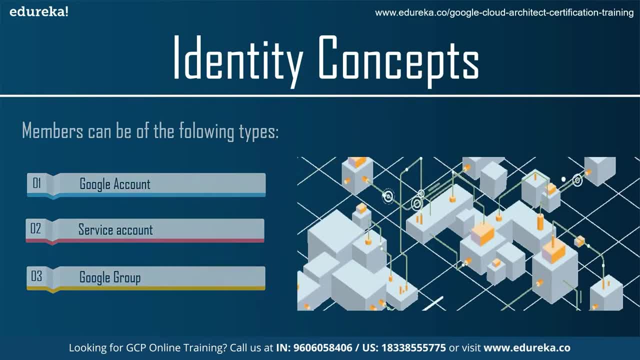 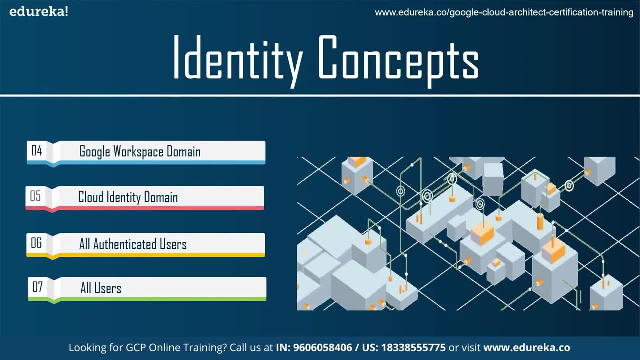 identity to make a request to access the resource. then there is Google workspace domain. Google workspace Domain represents a virtual group of all the Google accounts that have been created in an organization's Google workspace account. then Google workspace domains like represent your organization's internet domain name. 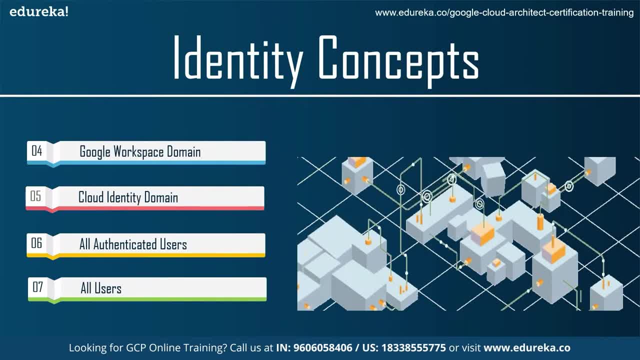 such as examplecom. You can just for example- so I'm just naming it as examplecom- and when you add a user to your Google workspace domain, a new Google account is created for the user inside the virtual group, such as, like you can take it: 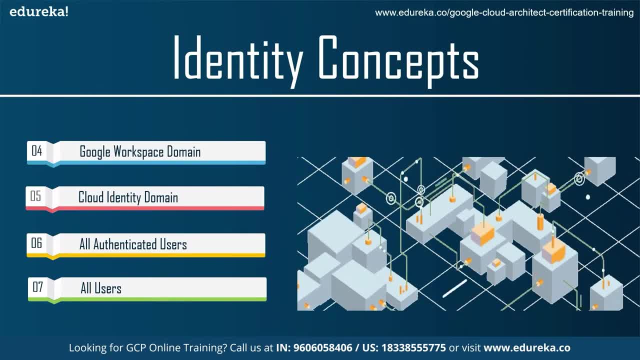 as user name at the rate examplecom. like Google groups, Google workspace domains cannot be used to establish I, But they enable convenient permission management. Then the fifth one is cloud identity domain. a cloud identity domain is like Google workspace domain because it represents a virtual group of all. 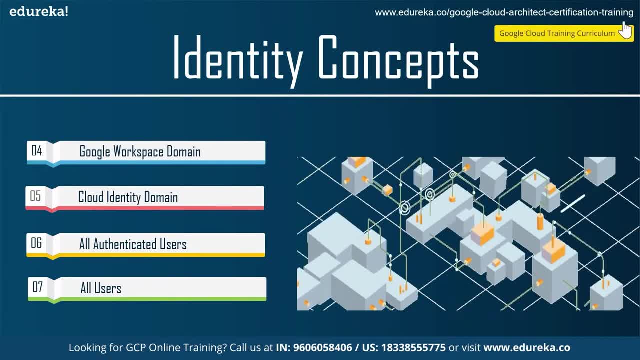 Google accounts in an organization. However, cloud entity domain users don't have access to Google workspace applications and features in the next one is all authenticated users, So the value all authenticated users is a spatial identifier that represents all service accounts and all users on the internet who have authenticated. 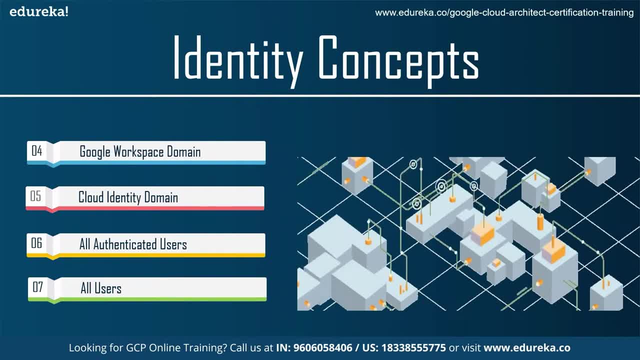 with a Google account, So this identifier includes accounts that aren't connected to a Google workspace or cloud identity domain, such as personal Gmail accounts. users who aren't authenticated, such as anonymous visitors, aren't included in. the last one is all users, So the value- all users- is a spatial identifier that represents anyone who. 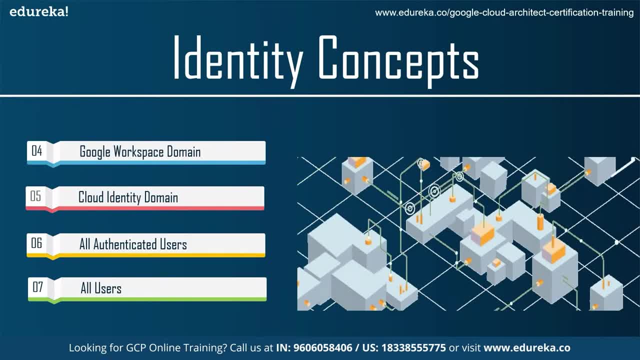 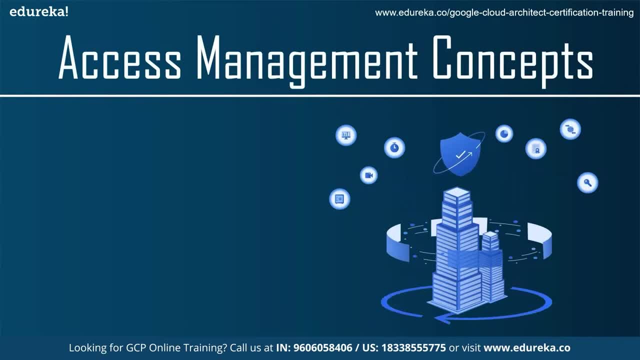 is on the internet, including authenticated and unauthenticated users also. Now moving ahead to the concepts related to access management. when an authenticated member attempts to access a resource, I am checks the resources for I am policy to determine whether the action is allowed or not. 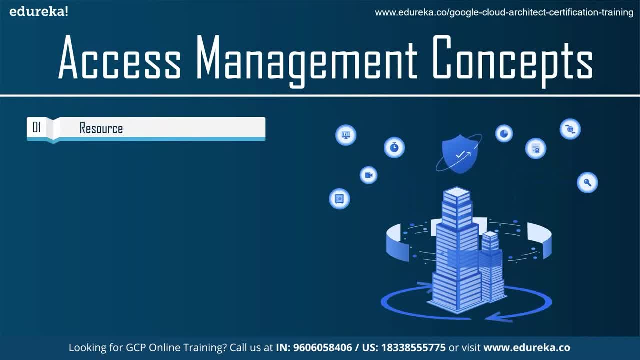 So the first one in this is resource. if a user needs to access to a specific Google cloud resource, You can grant the user a role for the resource. some examples of resources are projects, compute engine instances and cloud storage buckets. some services support granting, I am permissions at a granularity finer than 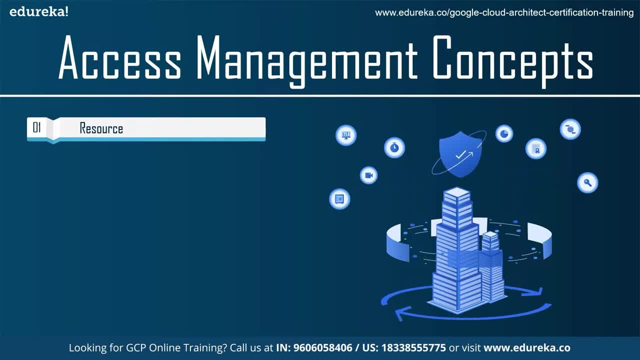 the project level. For example, you can grant the storage admin role to a user for a particular Cloud storage bucket, or you can grant the compute instance admin role to a user for a specific compute engine instance. In other cases you can grant I am permissions at the project level. 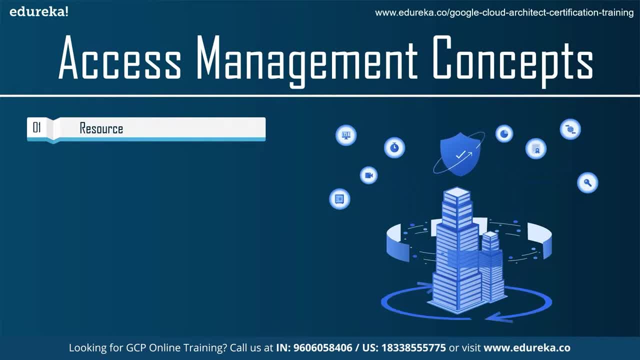 The permissions are then inherited by all resources within that project. For example, to grant access to all cloud storage buckets in a project: grant access to the project instead of each individual bucket. or to grant access to all compute engine instances in a project: grant access to the project rather. 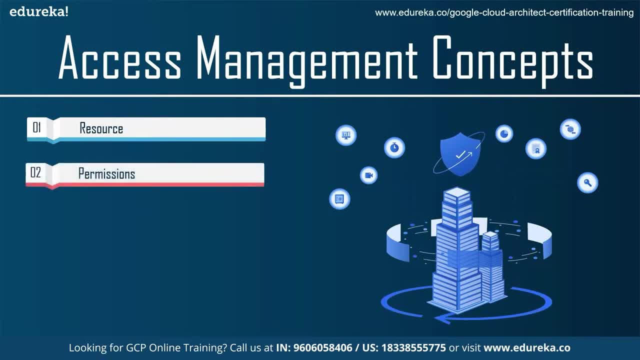 than each individual instance In the next one is permissions. So permissions determine what operations are allowed on a resource. in the I am world, permissions are represented in the form of service dot, resource dot verb. For example, if you are using pub sub, then you can give it as pub sub dot. 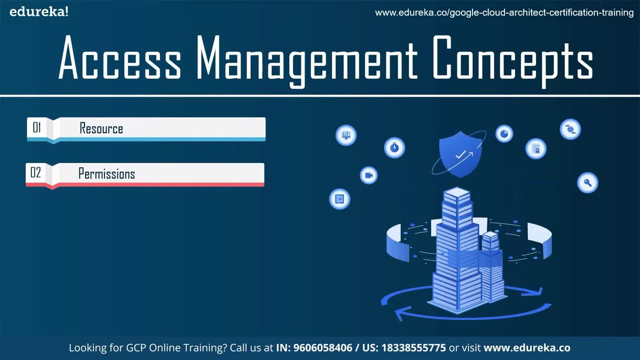 subscriptions dot consume. that becomes service, dot. resource, dot. verb right permissions often correspond one-to-one with rest API methods. that is, each Google cloud service has an associated set of permissions for each rest API method. It exposes the color of that method. needs those permissions to call that method. 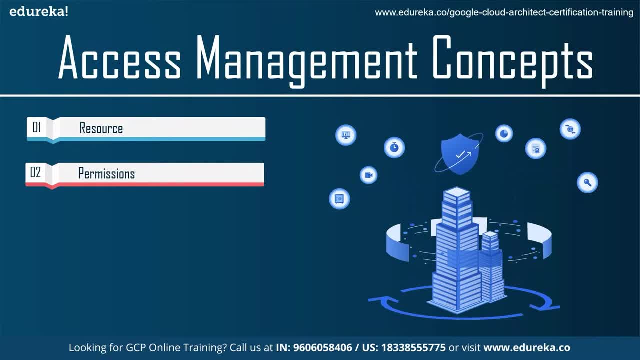 For example, if you use pub sub and you need to call the topics dot published method, you must have the pub sub topics published permission for that topic. You don't grant permissions to users directly. instead, You identify roles that contain their prepared permissions and then grant those. 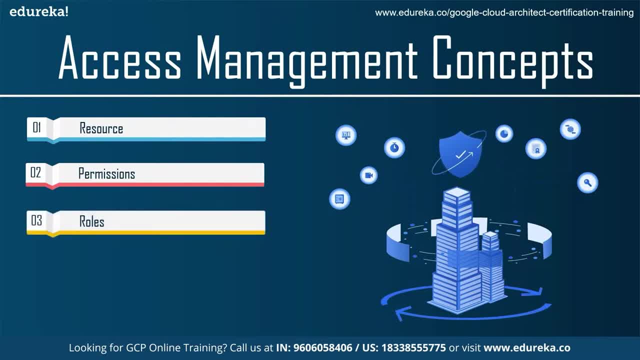 roles to the user. So the third one is roles. a role is a collection of permissions. You cannot grant a permission to the user directly. instead, You grant Them a role. then, when you grant a role to a user, you grant them all the permissions that they use. role contains: 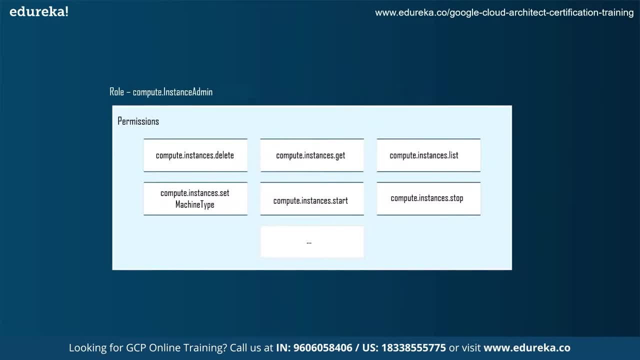 So there are several kinds of roles in. I am like the basic rules. rules historically believe in the Google Cloud console. These console are owner, editor and viewer. cautiously remember that basic roles include thousands of permissions across all Google cloud services in production environments. do not grant basic rules unless there is no. 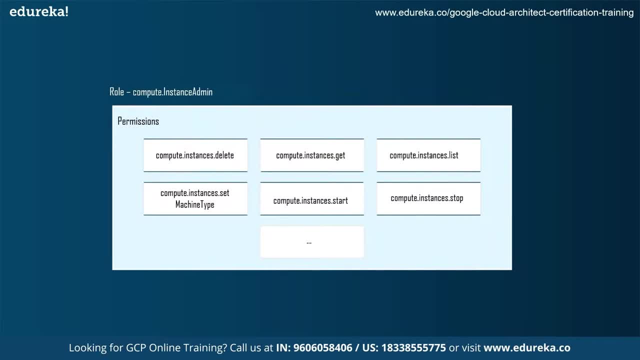 alternative. instead grant the most limited predefined roles or custom roles that meet your needs. Then there are predefined rules, So roles that give finer grained access control than the basic rules. For example, the predefined role pub sub publisher provides access to only publish messages to a pub sub topic only. then they are custom rules. 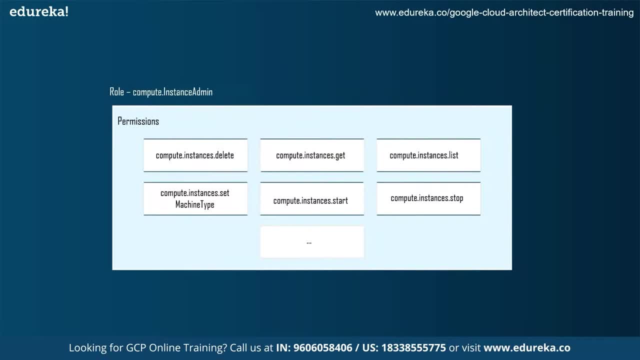 So roles that you create a tailor permissions to the needs of your organization when predefined roles don't meet your needs. like you can see here an example of role is given: like the role is assigned as a compute dot instance admins. like the role is assigned computer instance admin. 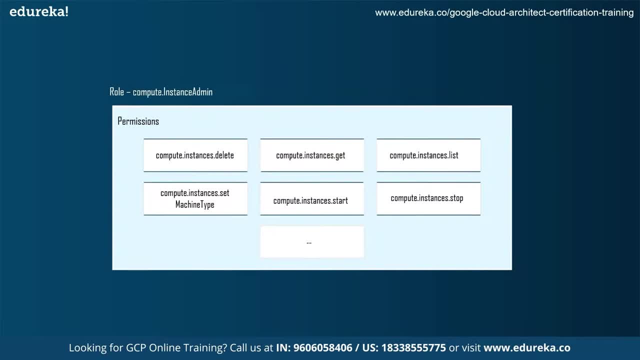 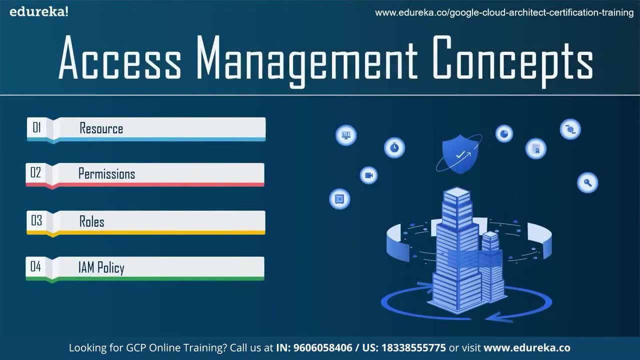 So under this role, you have permissions to access all the resources. under this role, like computer instance to delete, or like computer instance to get everything is you can access now. The next one is I am policy, so you can grant roles to users by creating an I am. 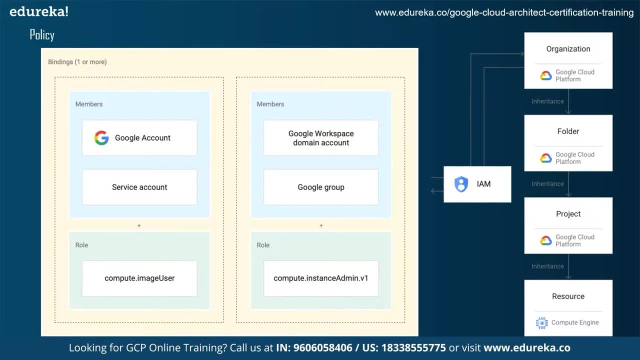 policy, which is a collection of statements that define who has what type of access. a policy is attached to a resource and is used to enforce access control whenever that resource is access, as you can see here. So an I am policy is represented by the I am policy object and I am policy object. 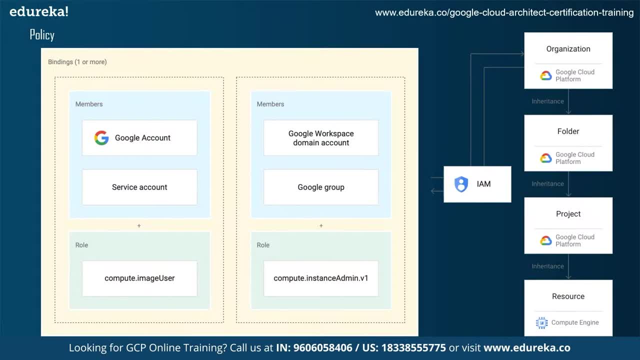 consists of list of role bindings. a role binding binds a list of members to a rule. I am provides a set of methods that you can use to create and manage access control policies on Google Cloud resources. These methods are exposed by the services that support. I am, for example, the: I am. 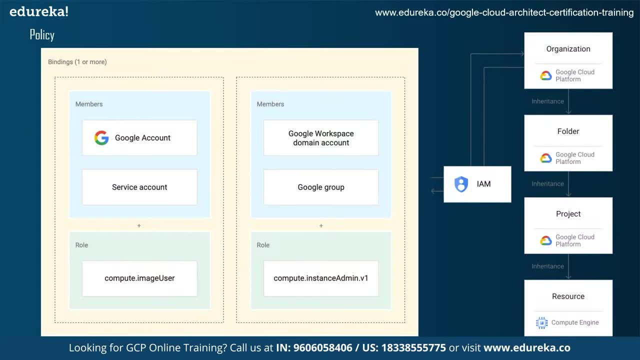 methods are exposed by the resource manager: pub, sub and cloud life sciences APIs, just to name a few. like the I am. methods are set I am Policy, which sets policies on your resources. Then there is get I am policy, which gets a policy that was previously said. then 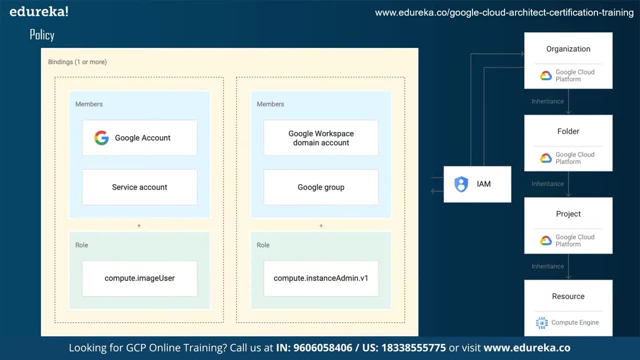 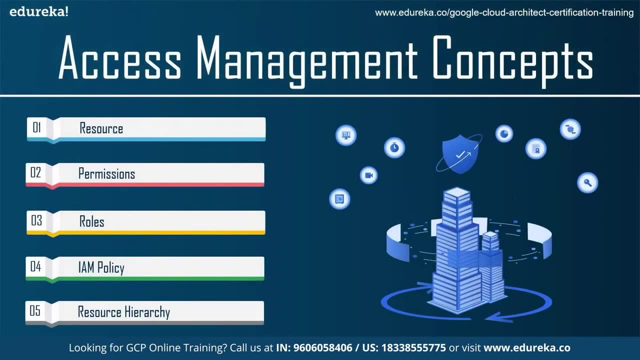 there is test I am permissions that sets. then there are test I am permissions which test whether the caller has the specified permissions for a resource or not. Now moving on to the next and the last one, that is, resource hierarchy. So Google Cloud resources are organized hierarchically, like the organization is. 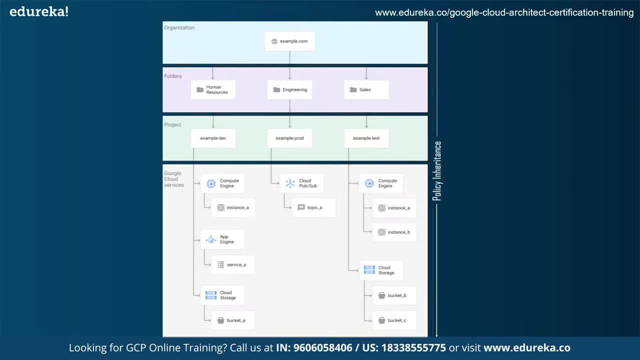 the root node in the hierarchy. Then there are folders, which are children of the organization, then projects are children of the organizations or of a folder. and the last one, like the resources for each service, are descendants of projects. Each resource has exactly one parent. So this following diagram is an example of a Google Cloud resource hierarchy. 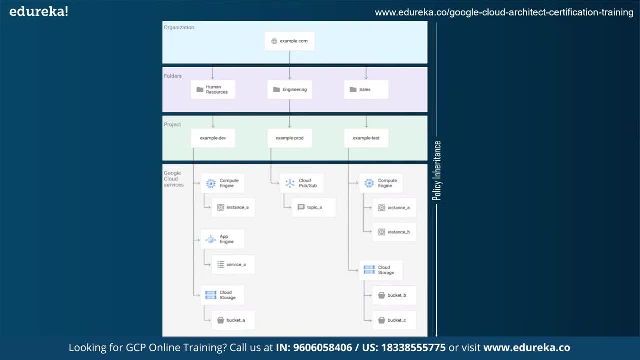 You can set an I am policy at any level in the source hierarchy: the organization level, the folder level, the project level or the resource level. resources inherit the policies of all their parent resources. the effective policy for a resource is the union of policy We set on that resource and the policies inherited from higher up in the hierarchy. 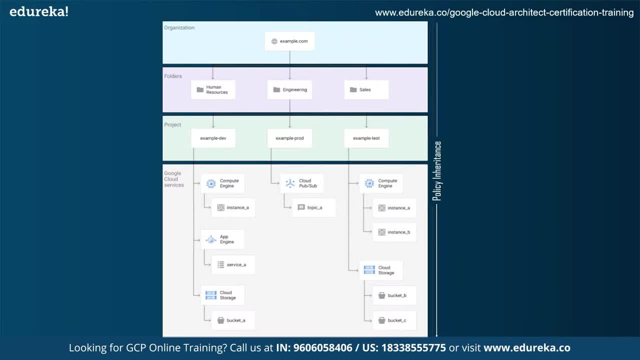 and this policy inheritance is transitive, in other words, like a resource inherit policies from the project, which inherit policies from folders, which inherit policies from the organization. Therefore, the organization level policies also apply to the resource level. For example, in this diagram, topic underscore a is a pub sub resource that lives under the 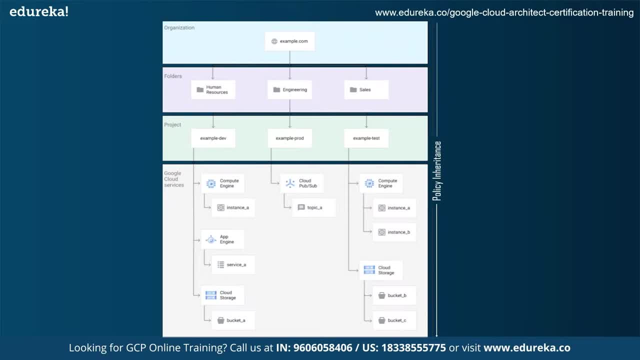 project example: prod. suppose there is a account name Mika at that example dot com. and if you grant the editor wrote to Mika at that example Com for resources, for example production, and grant the publisher role to song at that example Com for topic underscore a, you effectively grant the editor role for topic underscore. 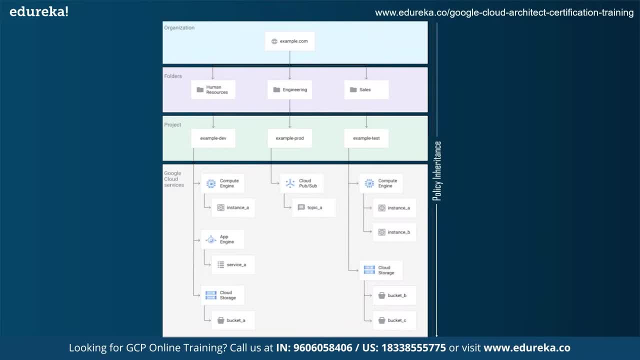 a to Mika at that example Com. and the publisher role to song at that example Com. the policies for child resources inherit from the policies for their parent resources. For example, if you grant the editor role to a user for a project and grant the viewer 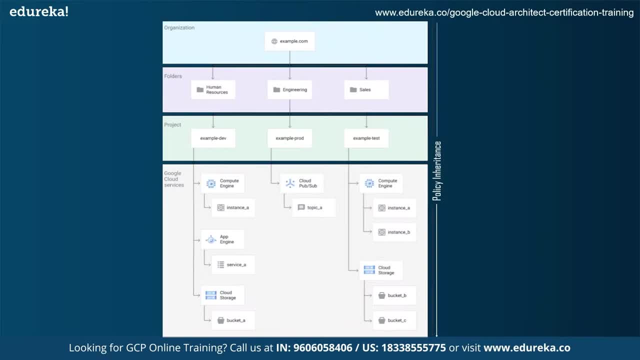 role to a same user for a child resource, then the user is still has the Editor role grant for the child resource. If you change the resource hierarchy, the policy inheritance changes as well. For example, moving a project into an organization causes the project to inherit from the organization's. 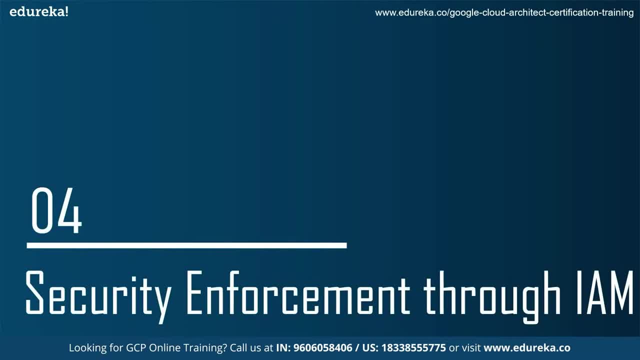 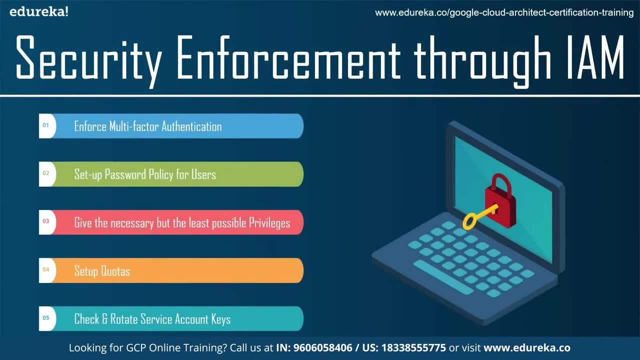 I am policy. Now let's understand the practical, actionable settings you can modify in the I am, which will greatly improve the security of your project. So the first one is you can enforce multi factor authentication. You can say it as MFA, which is a method where not only is one piece of information used. 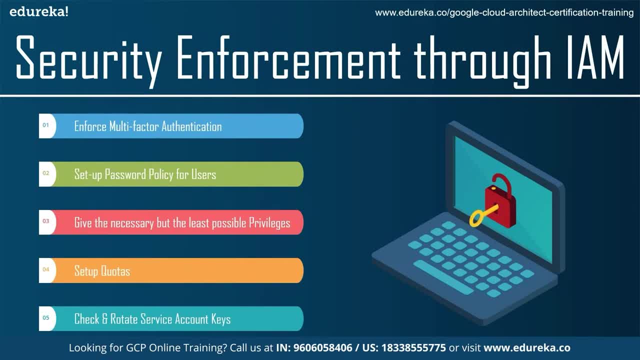 to authenticate a user, For example a password, but there's also at least one additional source of proof needed to establish that the right person is accessing a system. on Google Cloud platform, users authenticate themselves using Google accounts. These can be individual email addresses. is stirred as a Google account or, more commonly, 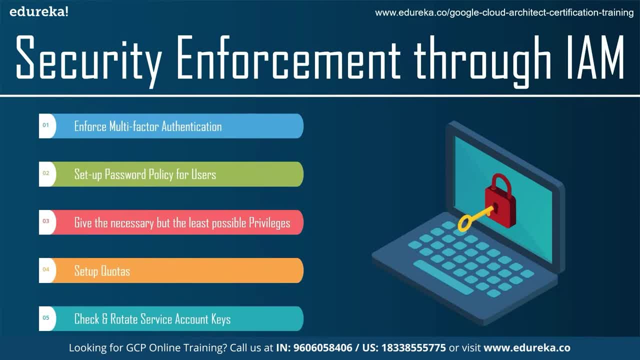 like accounts of a Google suit domain on the Google Cloud platform site. You cannot enforce that. the Google accounts that have access to your project must have multi-factor authentication enabled, means MFA enabled. But If you only grant access to users from your Google suit domain, then the Google suit domain 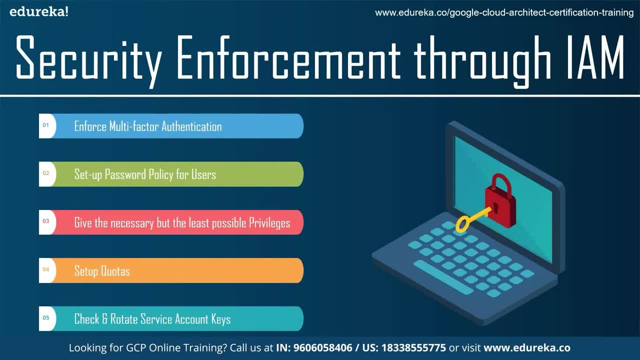 administrator can set up MFA on the Google suit domain in a way that forces everyone to use it. If you need to give access to people without accounts in your Google suit domain, then you can create accounts for them in your Google suit domain for the sole purpose of accessing. 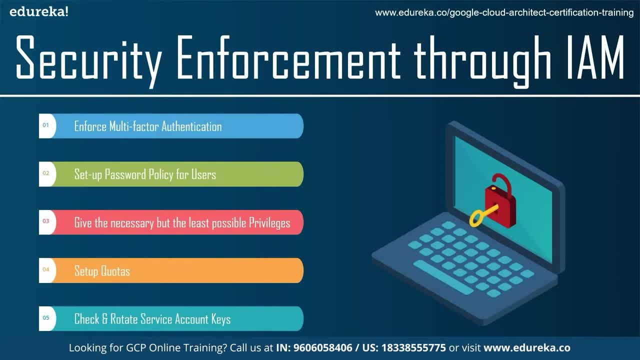 your project. This way, you can enforce settings on their accounts. If you combine both these rules, then you can be certain that every user who has access to the Google Cloud platform project needs to validate themselves. using MFA means multi-factor authentication. This makes it much harder to compromise your project. 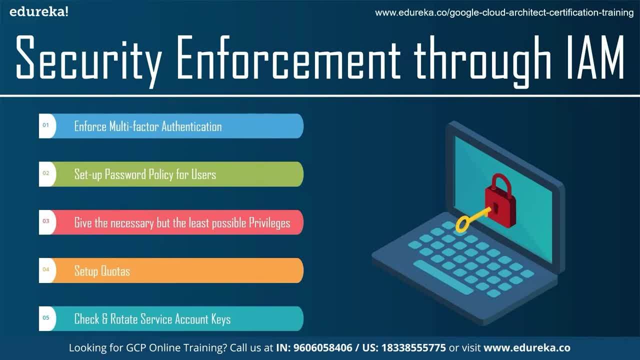 Even if the password for an email address leaks from another source. Second thing is, you can set up password policy for users. The password policy settings are technically not inside the Google Cloud platform but at the discretion of the Google suit domain administrator. If you only allow users from your domain and the domain is set up with the right password, 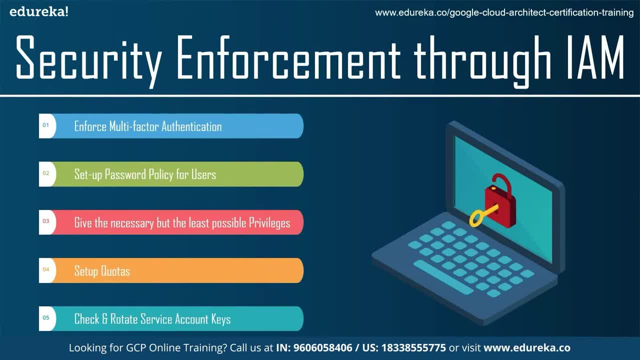 policy, Then these two things combined will result in the password policy being enforced on all your Google Cloud platform users. Third one is give the necessary but the least possible privileges. So it is a good practice in general to only give the minimum necessary privileges to all. 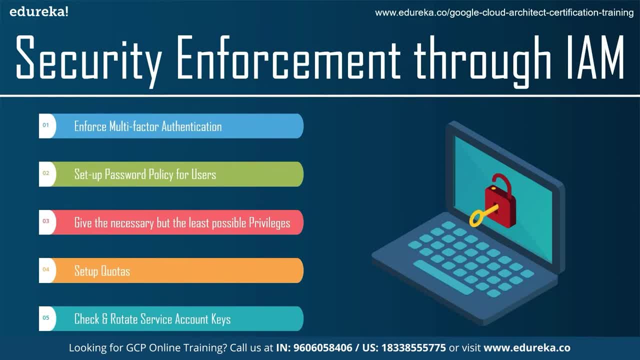 of your users. If all of the previously discussed account protection methods fail, your attackers will still have fewer services to break into or steal information from. The actual implementation of this principle will vary based on your usage patterns. For example, if you're dealing with a user who has access to the Google suit domain, 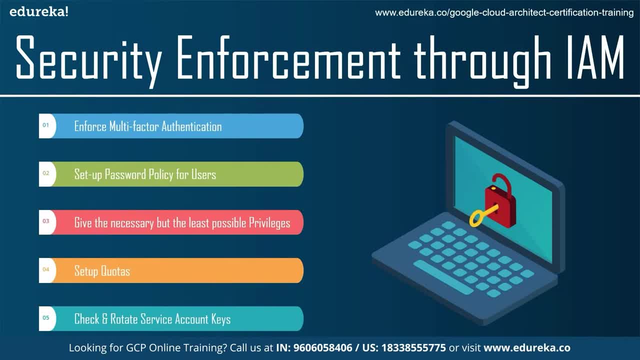 database. For example, if your database administrators only need to do Google Cloud SQL administration tasks, don't give them project editor role. give them a Cloud SQL admin role instead. Also, what you can do is you can set up quotas Like default. quotas are set for every newly created project on Google Cloud platform. 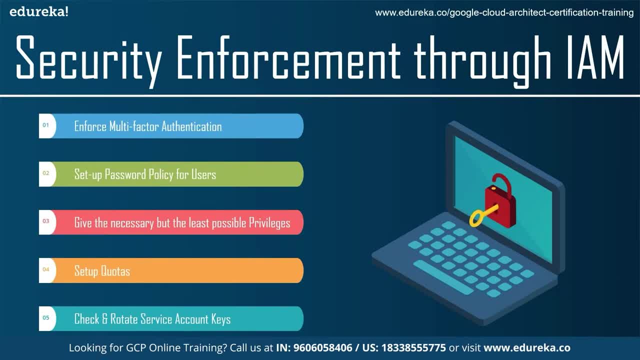 This is a least resort security control to avoid unexpected runaway spending. For example, if you have a faulty script creating resources in a recursive manner, it will only be able to create them. It can also protect against compromised account, creating a lot of new resources for the attacker's. 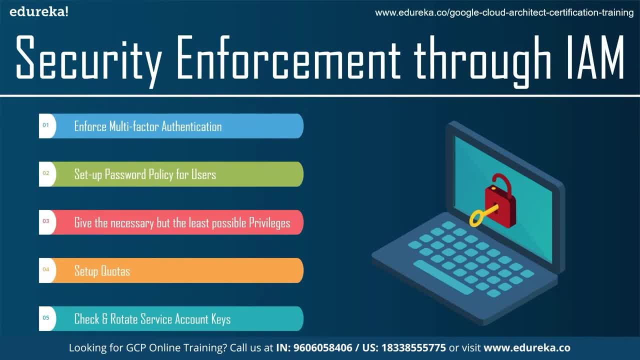 purposes. The quotas can be changed on the quotas page, but it requires the service usagequotasupdate permission, which is only included in the following predefined roles like owner, editor and quota administrator. So if a compromised account or faulty script does not have the permission, then the spending. 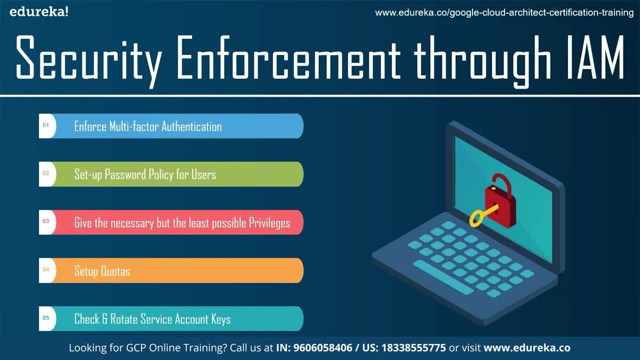 can only increase up to the quota limits. Last thing is check and rotate service account keys. There is another type of account on Google Cloud platform besides the user accounts, that is, service accounts. So service accounts are meant for programmatic use cases. They cannot be used to access the Google Cloud console because they are only valid for Google. 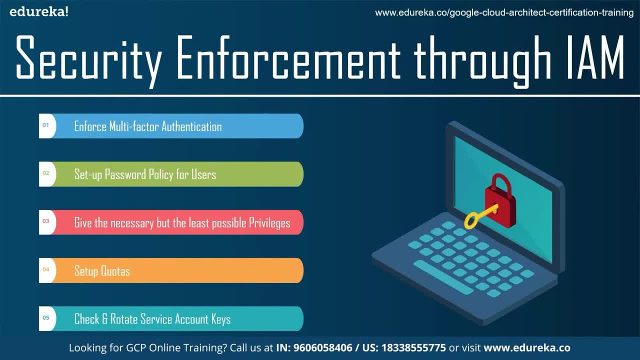 Cloud API access. The most frequent use case is to run applications or instances inheriting the rights of a specific service account so they can access other cloud service without extra authentication. Service account use cases are meant for programmatic use cases. Service accounts use keys for authentication. 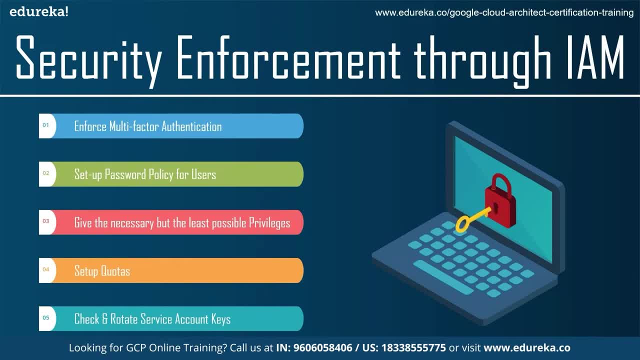 One service account can have multiple keys associated with it. It is a good practice to regularly rotate the keys of the service account. This can be achieved by creating a new key for the service account, then overwriting the current key with the new one, everywhere it was saved, and then deleting the old key. 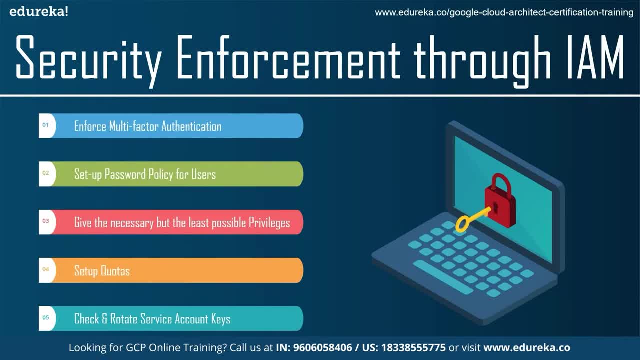 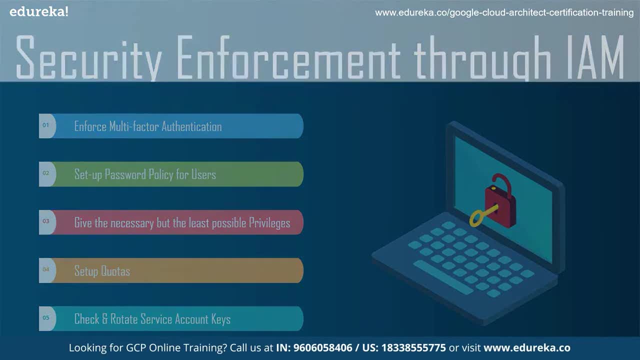 associated with the service account. This way, even if an application where the key was stored is compromised without your knowledge, the attacker will only have a limited time window to use the key. Now that you have a theoretical understanding of Google Cloud identity and access management. 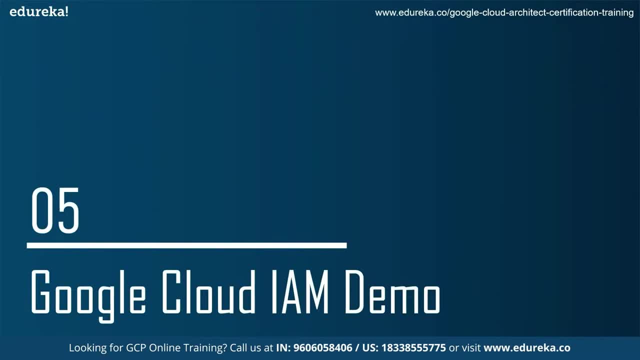 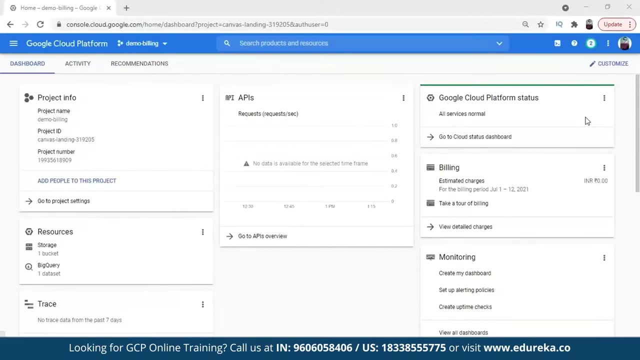 working in concepts. let's now see a practical demonstration of it on Google Cloud platform. So we are at Google Cloud console now. This is how the dashboard of Google Cloud platform looks like. means console looks like You can see the ID: dhruvpandeedurekaco. 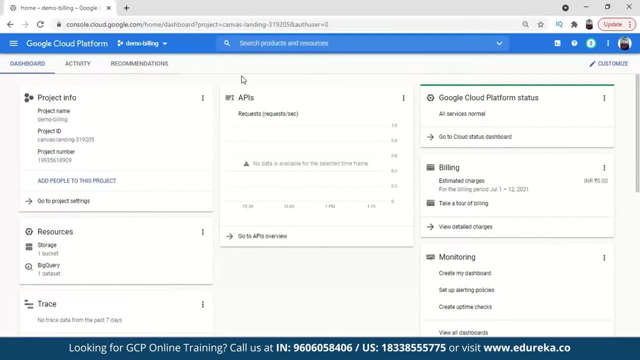 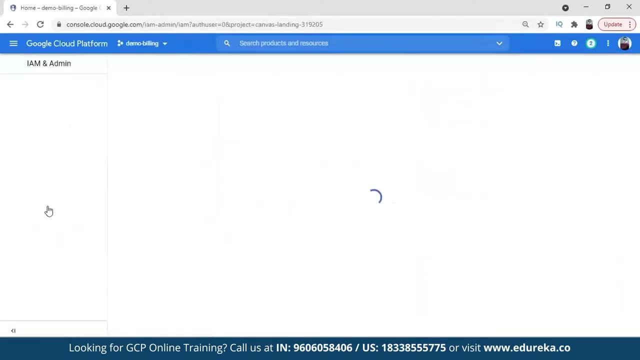 So what we are going to do is we are going to see the identity and access management. So let's move on to IAM. You can just click here and go to IAM and admin And here you can see all the permissions the accounts have. 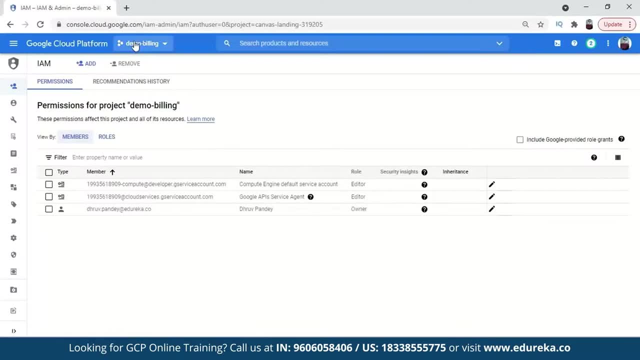 So we are going to provide a new access to that. Like you can also see the project here, It's demo billing, So from this project I will be giving the access. So let's add account So you can add it from here. 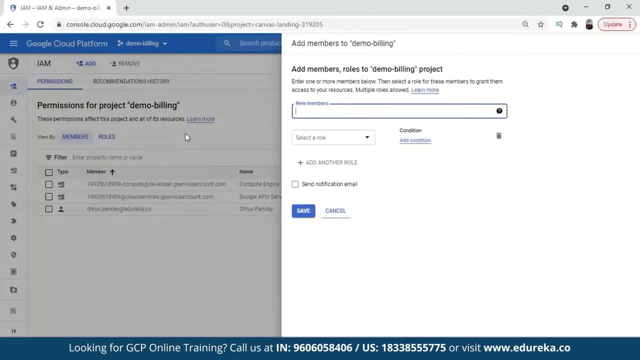 I'm going to add, like the other accounts of mine, in it. So yeah, it will be At project level. you are going to give a role now, So select it. Go to project. Give editor. As I have explained to you how we have to give the editor role here, 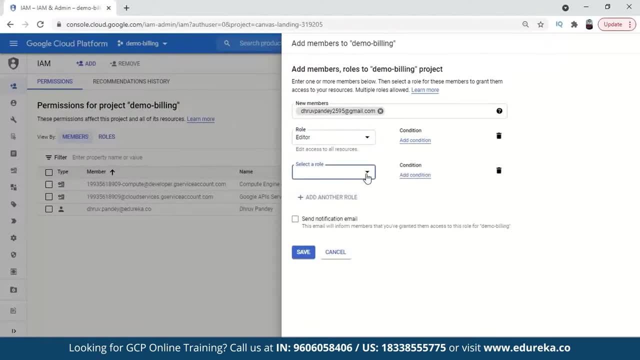 Editor. Now you have to give another role at resource level. That's how the that's what is given in the policy right. I have explained to you the policy of access management. Choose a resource for it. So you're going to choose cloud storage. 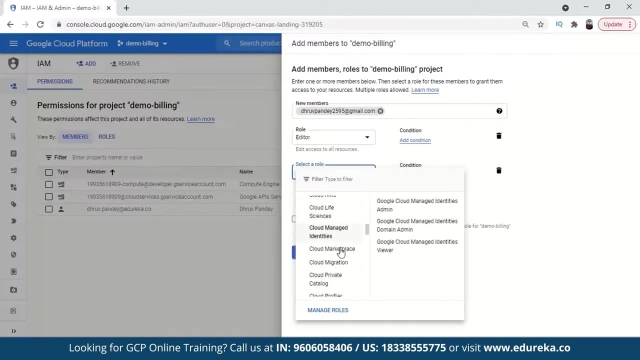 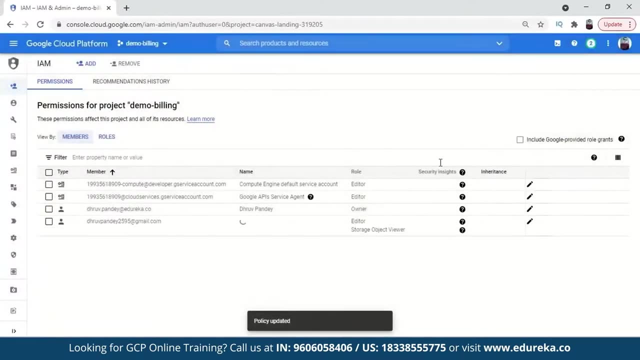 We can choose. So cloud storage Here it is. Yeah, So we are just going to choose the viewer option. Okay, So yeah, save it. But at the project level we have the editor option. Remember that? Okay So, yeah, it's been added now. 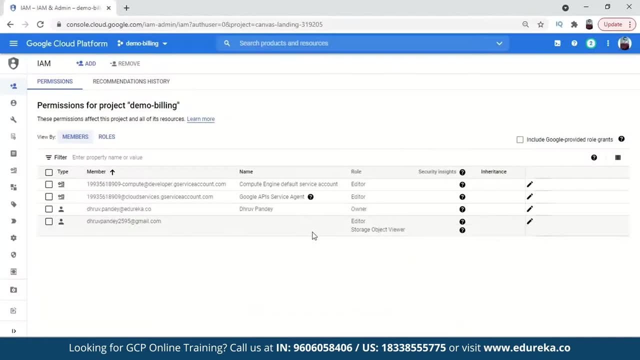 Now you can just go to like because you have the, the literal permissions at the project level. So you can just simply see how like we can go to virtual machine also. So here you can go and you can see if there is any virtual machine is there. 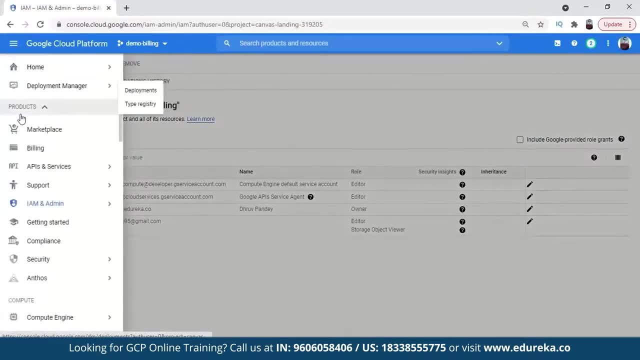 Oh, just a second. Right now I'm logging in my the same account, So what I can do is I can go to another account, that is. Oh, just a second. Right now I'm logging in my the same account. 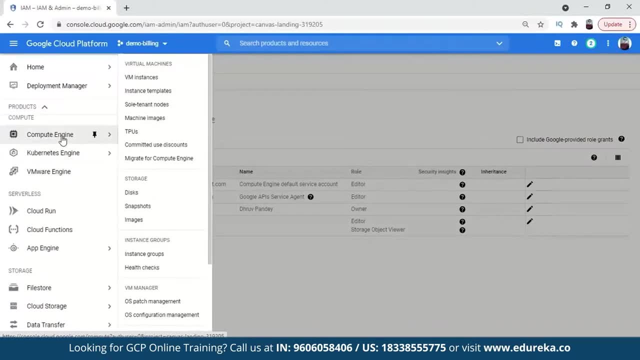 So what I can do is I can go to another account. that is Okay. So I can just go to this account and I can just go to this one. So I can go to this one, Okay, So I can go and you can see if there is any virtual machine. is there? 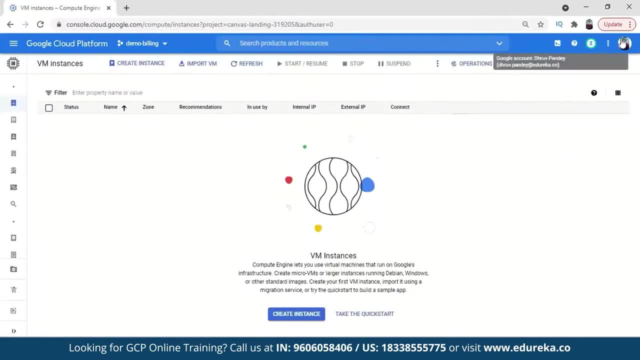 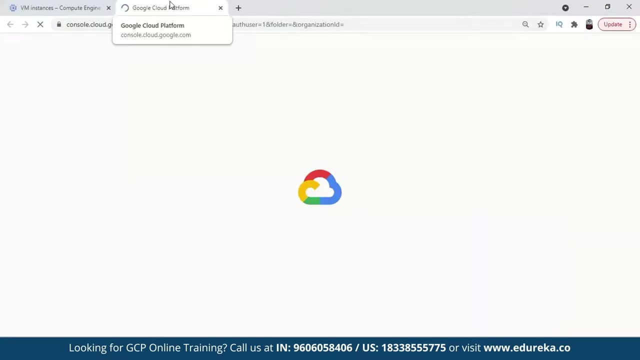 Oh, just a second. Right now I'm logging in my the same account, So what I can do is I can go to another account, that is which I've given permission to, right, So I'll go to this account, Sorry. 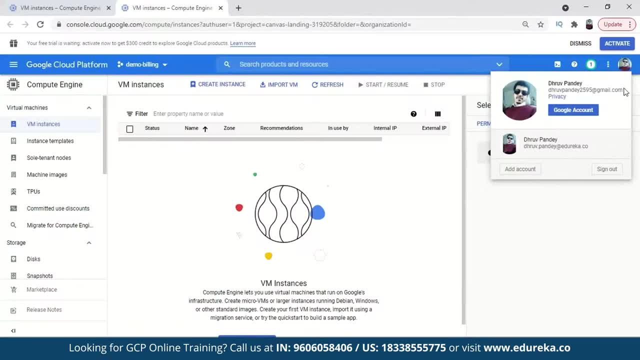 So now I'm logging into my other account. It is the bandit two, five, nine, five, eight, three made of come. You can see now. So in this account I have been to the VM stands now. So in this you can see like there's no VM created now. but I can create an instance. 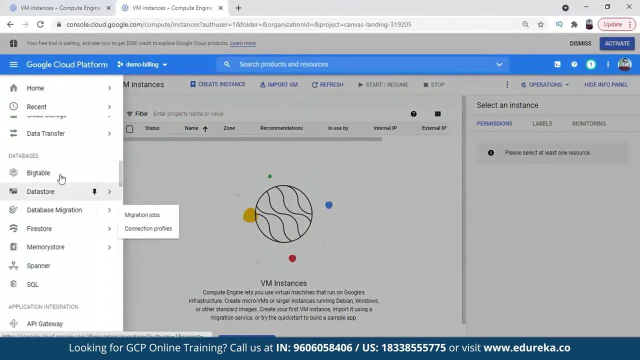 from here And, similarly, if you go to cloud storage, you can access other services also through this account because you have the editor option at the project level. Okay, Let's go to cloud storage and you can see there is this demo store. cloud is here. 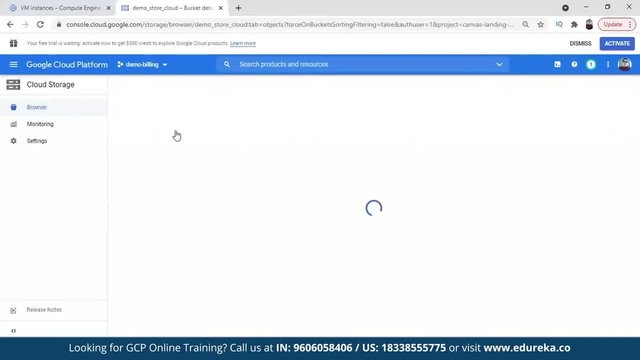 So you can even create a new bucket or you can just go to this one and you can upload any file into it. Also, like I'll show you how upload files say okay and this upload this, So you can see how upload has been done, because you have all the rights of editor. 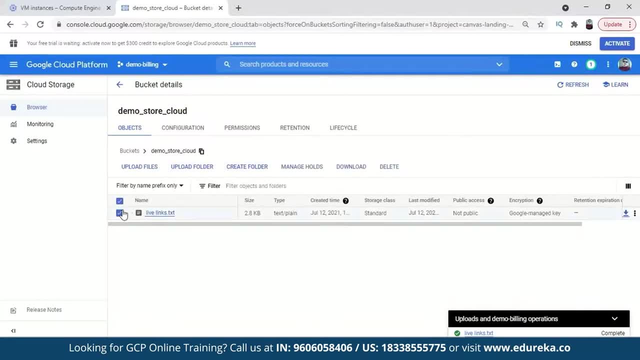 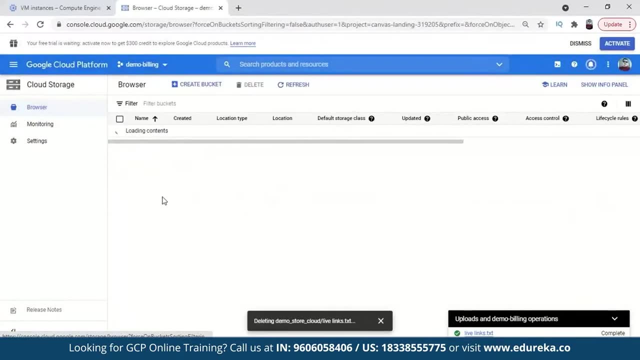 You can delete it also. So you just select this one, So you can just delete it from here. Yeah, That's just someone and it will get deleted. Now go back. You can even delete this one also. you can just select it and you can delete it from. 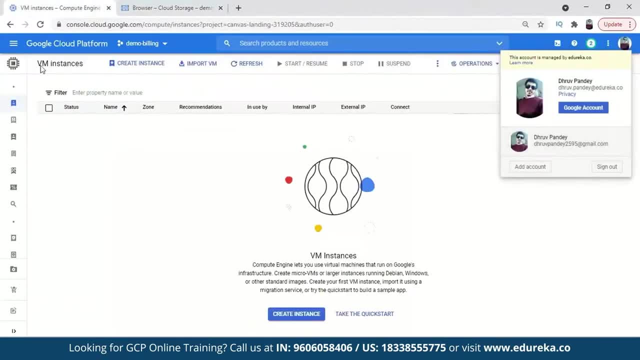 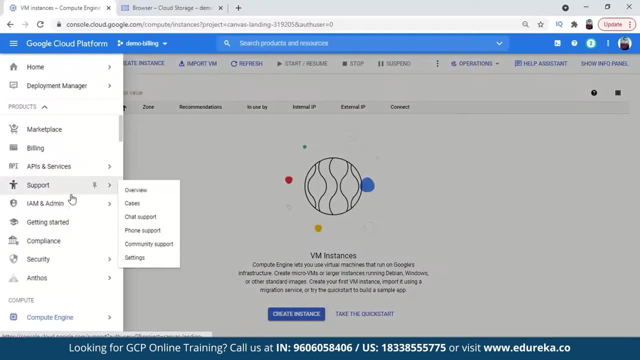 here. Okay, Now let's move back to our own IAM permissions. This is the main account I'm opening. You can see here. from here I will go to the IAM roles and everything. So IAM, access management means I, entity and access management. 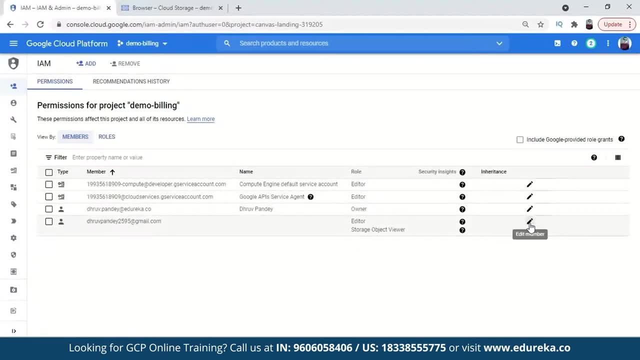 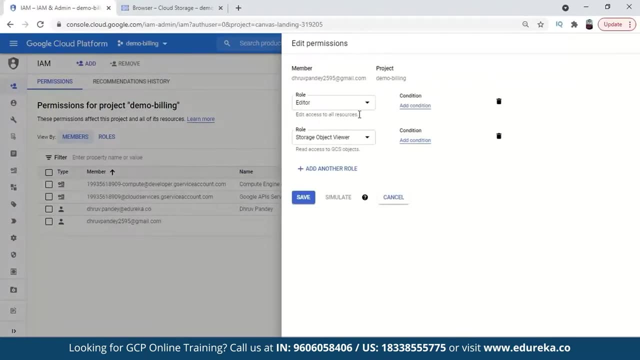 And what I'm going to do And what I can do here is I can edit the rules. So what I can do is I can delete it from here. Right, Okay, I will not delete it. Project level: No, no. 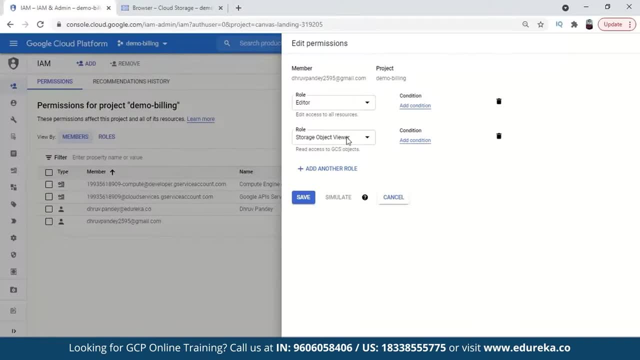 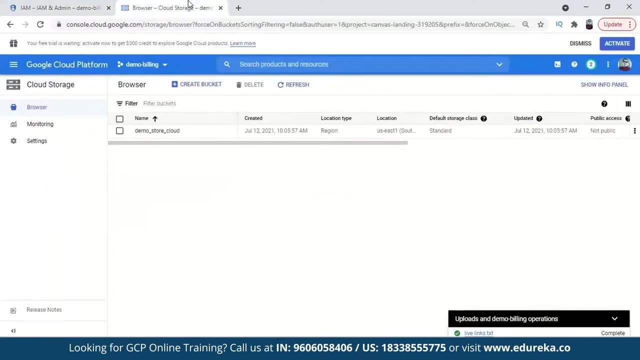 I will delete it. The editor, Okay, But the resource level it will remain, but it won't be completely deleted, Okay, So I'm just deleting this one. So just select here the troll one and save Okay. Now, if you refresh it, you will see like you won't be having access to it. 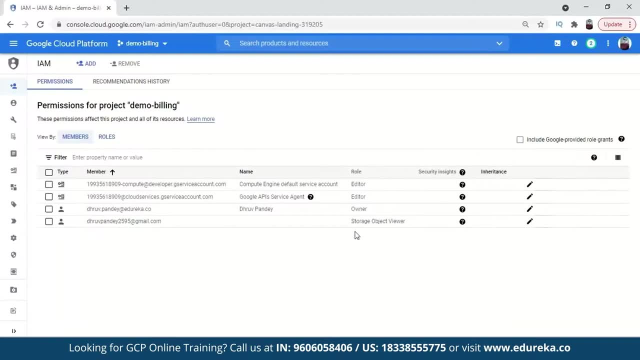 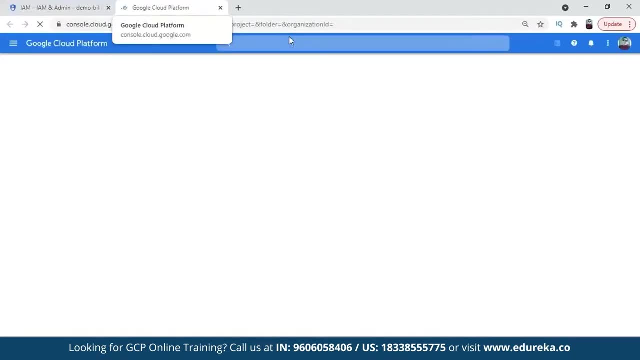 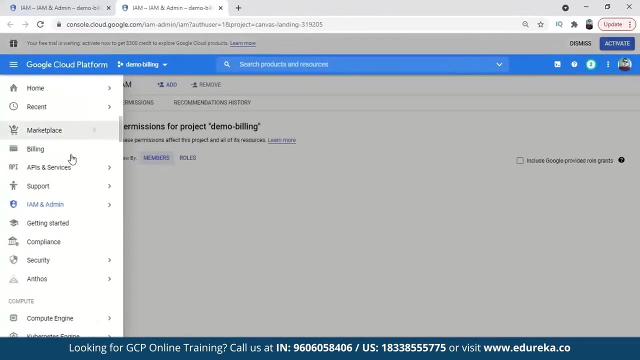 Now the we have deleted the Okay. Okay, We have deleted the editor role. What we can do is we can choose the other account- Okay, Access to the secondary account, And then we'll go to storage. but just to say, can cloud storage? 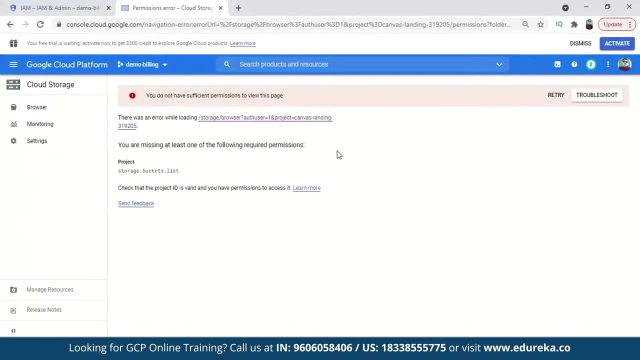 So you can see, the permissions are being limited, So you don't have sufficient permissions to view this, Even though the other way to view this is because you have the viewing option at- not at the project level level, but at the resource level, so you can view it from the cloud shell. there are certain codes. 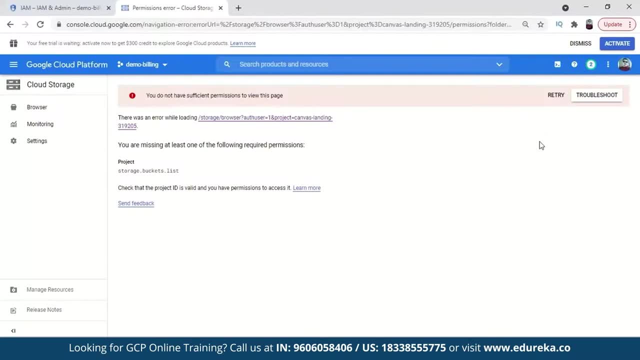 being given the documentation, part of identity and access management in google cloud and see the codes and you can just type it here at the command line interface of the google cloud. it is cloud shell, which is this. you can activate it from here and you can just access means. so you can view. 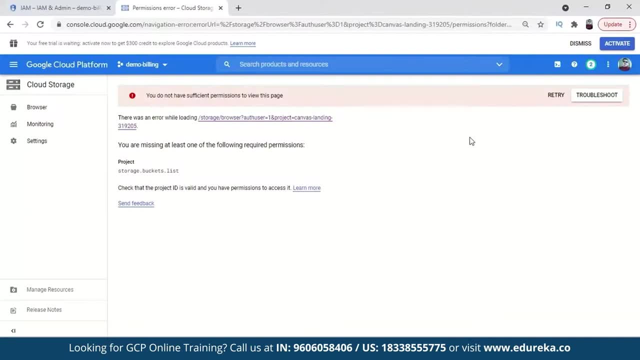 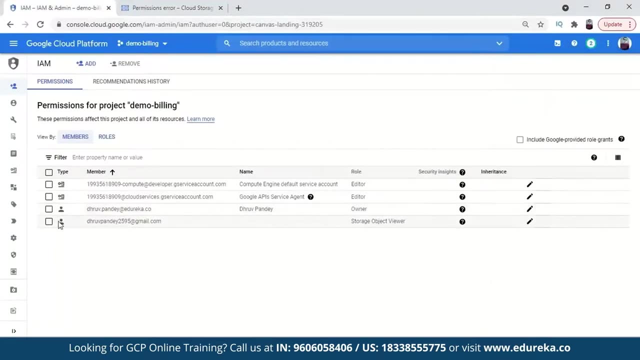 the files from here. okay, but not at the console. you can only be able to see it from command line interface. that is cloud shell. now let's go back to the. this is my main account. now i can even delete these roles, like the real roles i provided. so i can delete this role completely, okay. so i. 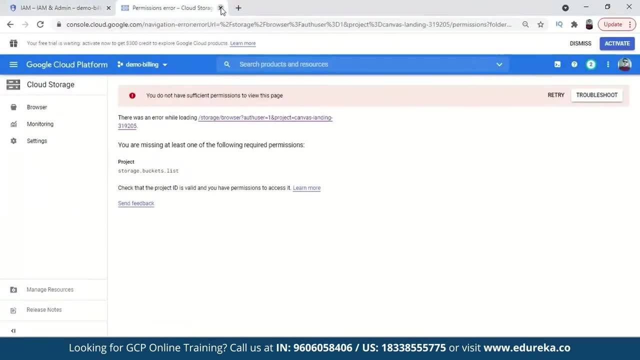 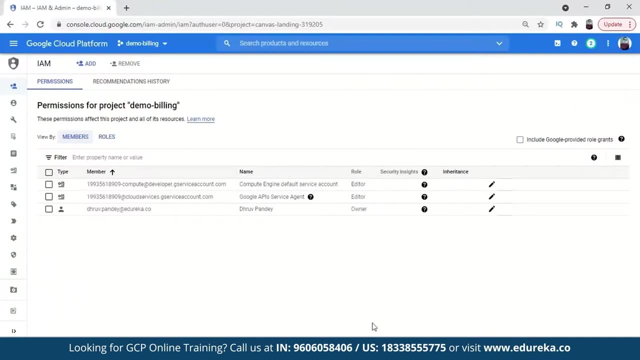 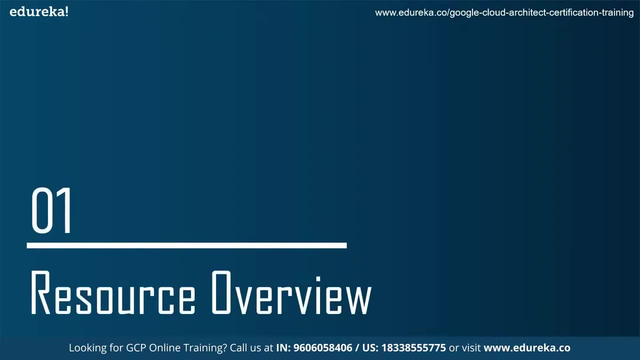 just remove it from here. confirm, okay. so that's how the role has been deleted. i hope you have understand how identity and access management in google cloud works. you can configure billing on google cloud in a variety of ways to meet different needs. so let's start with having a brief overview. 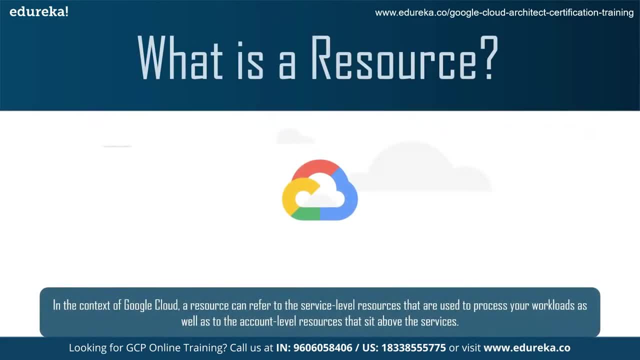 of a resource in google cloud. so the first question that arise while having an overview of a resource in google cloud is: what is actually a resource in the context of google cloud? a resource can refer to the service level resources that are used to process your workloads- virtual. 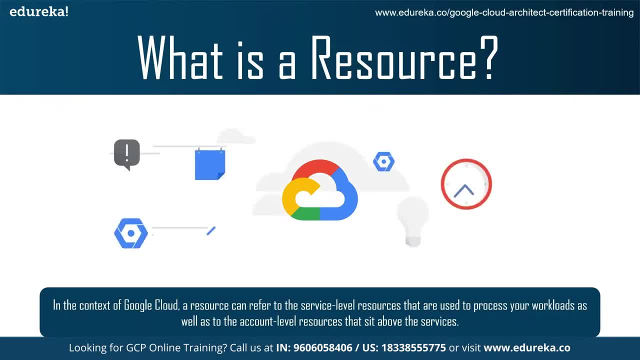 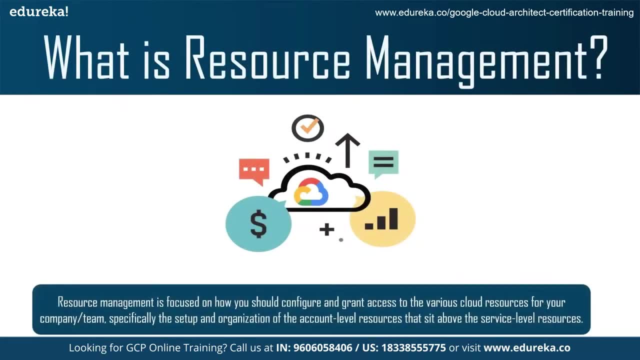 machines, databases and so on, as well as to the account level resources that sit above the services, such as projects, folders and the organization. now the next thing we need to understand, and the resource overview, is: what is resource management? resource management is focused on how you should configure and grant access to the various cloud. 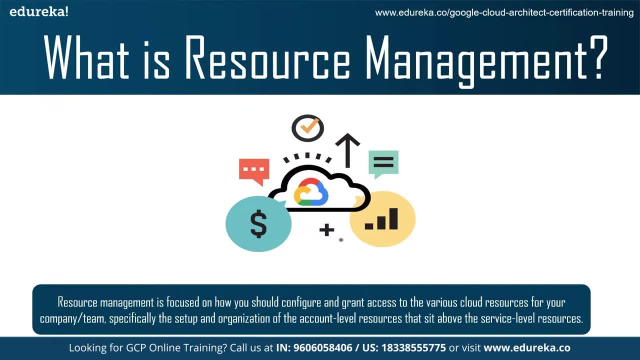 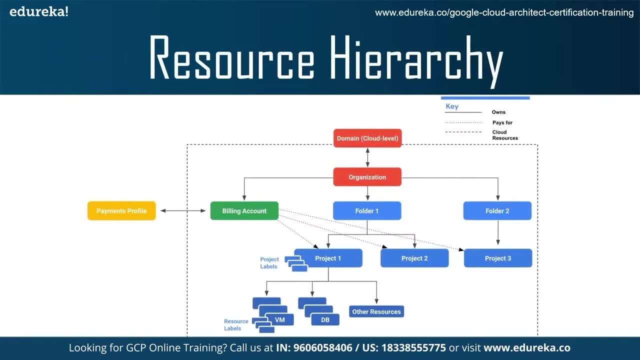 resources for your company or team, specifically, the setup and organization of the account level resources that sit above the service level resources. account level resources are the resources involved in setting up and administrating your google cloud account. the third and major thing is resource hierarchy. google cloud resources are organized hierarchically. 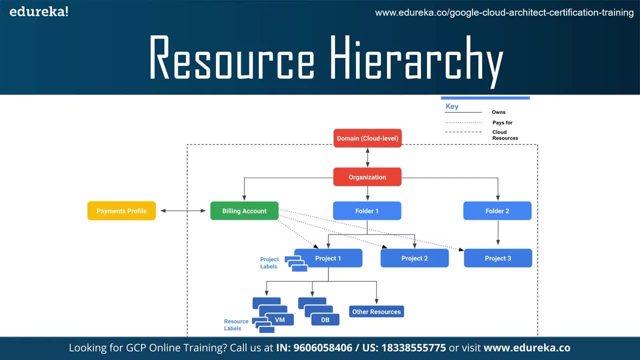 this hierarchy allows you to map your organization's operational structure to google cloud resources to manage access control and permissions for groups of related resources. the resource hierarchy provides logical attach points for access management policies like identity and access management and organizations policies- also both identity and access management and organization. 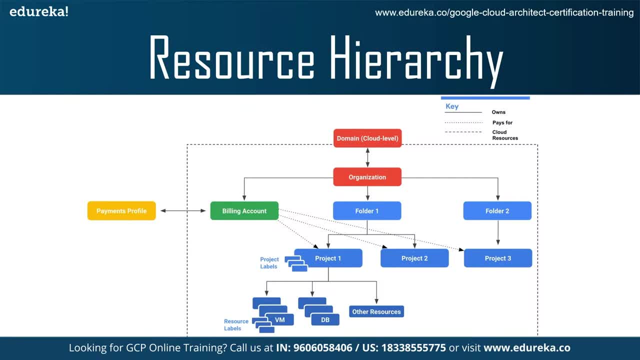 policies are inherited through the hierarchy and the effective policy at each node of the hierarchy is the result of policies directly applied to the node and policies inherited from its ancestors. so the results of the policy directly apply to the nodes and policies inherited from its ancestors. so this following diagram requires data and information to make an 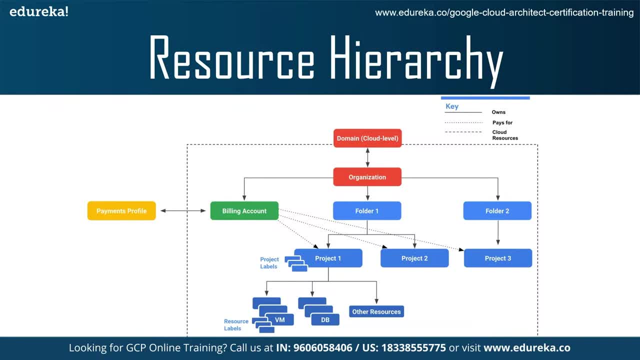 shows an example of resource hierarchy illustrating the core account level resources involved in administrating your Google Cloud account. so in this you can see, first is like domain, so your company domain is the primary identity of your organization. that establishes your company's identity with Google services, including Google Cloud, to manage the users in your organization at. 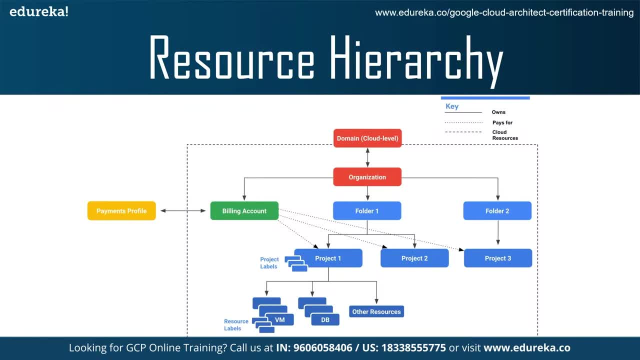 the domain level, you define which users should be associated with your organization when using Google. Cloud domain is also where you can universally administer policy for your users and devices, for example, enable two-factor authentication, reset passwords for any users in your organization. the domain is linked to either a Google workspace or cloud identity account. the Google 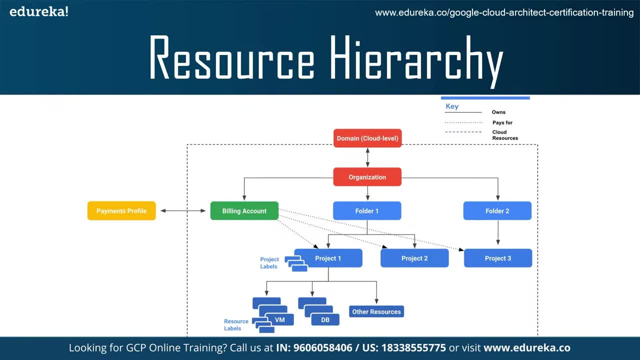 workspace or cloud entity account is associated with exactly one organization. you manage the domain level functionality using the Google admin console from like admingooglecom in. the second thing is organization. an organization is the root of your organization, node of the Google Cloud hierarchy of resources, all Google Cloud resources. 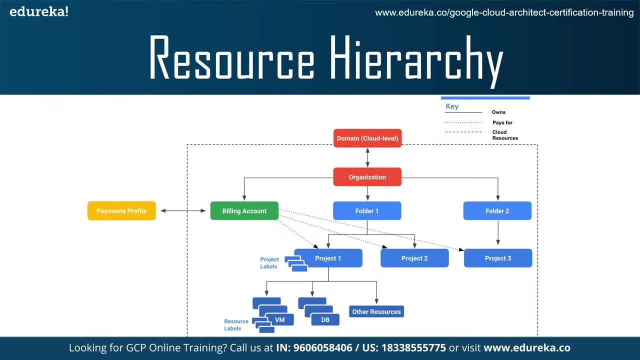 that belong to an organization are grouped under the organization node, allowing you to define settings, permissions and policies for all projects, folders, resources and cloud billing account parents. an organization is associated with exactly one domain established with either a Google workspace or cloud identity account and is created automatically. 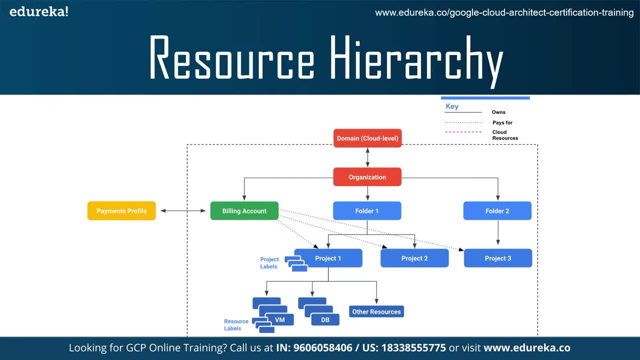 when you set up your domain in Google Cloud using an organization, you can centrally manage your Google Cloud resources and your users access to those resources. this includes proactive management and reactive management, so productive management is to reorganize resources as needed. for example, like restructuring or spinning up of a new division may require new projects and 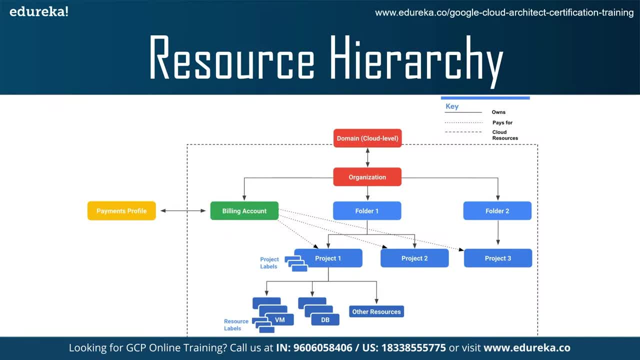 folders and reactive management is the: an organization resource that provides a safety net to regain access to lost resources, for example, if one of your team members loses their access or leaves the company. the various roles and resources that are related to Google Cloud, including the organization projects, folders, resources in cloud billing. 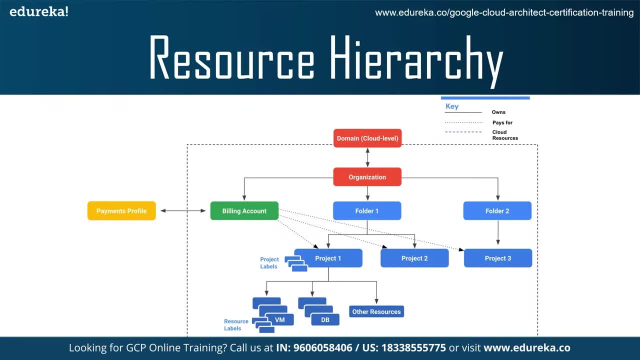 accounts are managed within the Google Cloud console. now the third thing is folder. the folders are a grouping mechanism and can contain projects, other folders or a combination of both. to use folders you must have an organization. node folders and projects are all mapped under the organization. node folders can. 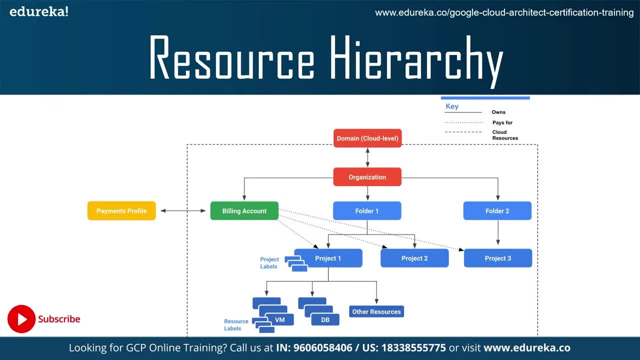 be used by group resources that share common identity and access management policies. while folder can contain multiple folders or resources, a given folder or resource can have exactly one parent. and the fourth one is projects, so projects are required to use service level resources such as compute engine virtual. 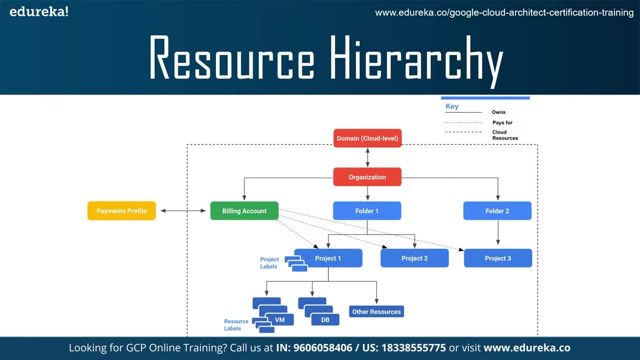 machines, pub subtopics, cloud storage, buckets and so on. all service level resources are parented by projects, the base level organizing entity in Google Cloud. you can use projects to represent logical projects, themes, environments or other collections that map to a business function or structure. projects form the basis for enabling services. api's and I am 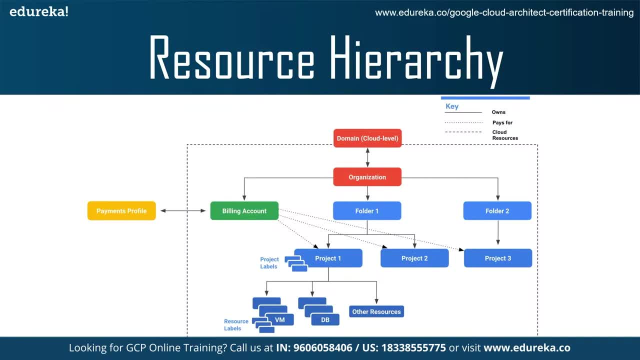 permissions. any given resource can only exist in one project, and then we have resources. so Google Cloud service level resources are the fundamental components that make up all Google Cloud services, such as compute engine, virtual machines, pub subtopics, cloud storage buckets and so on for billing and access control. 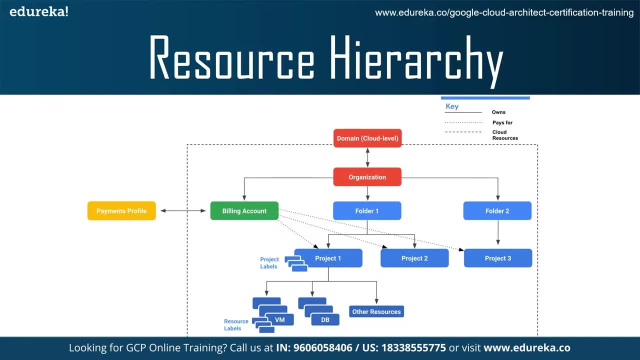 purposes. resources exist at the lowest level of a hierarchy that also includes projects and an organization. in the last one is label. the labels help you categorize your Google Cloud resources, such as computer engine instances. a label is a key value pair. you can attach labels to each resource, then filter the resources based on their. 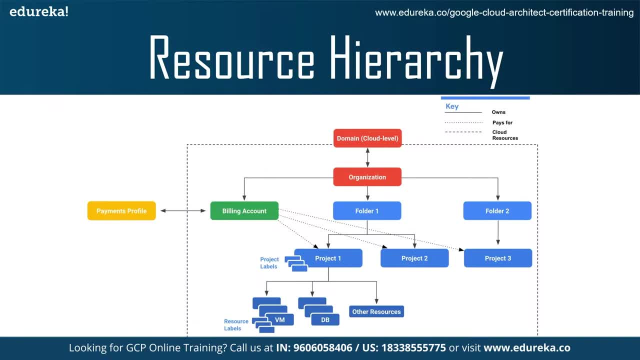 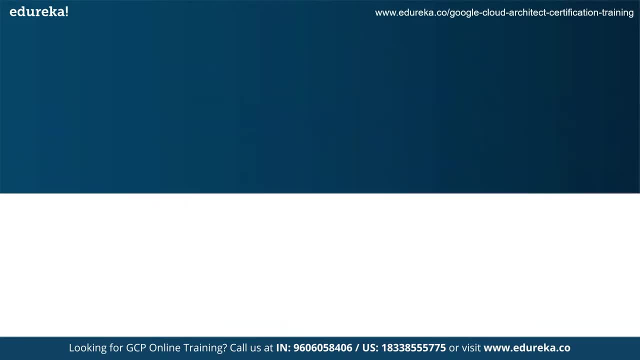 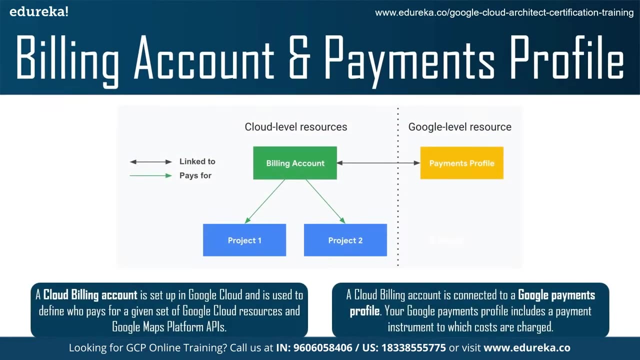 labels. labels are great for cost tracking at a granular level. information about labels is forwarded to the billing system so you can analyze your charges by label. now let's move on to understand cloud billing account and Google's payment profile, so we will understand them simultaneously. okay, so a cloud billing account is set up in Google Cloud and is used to define. 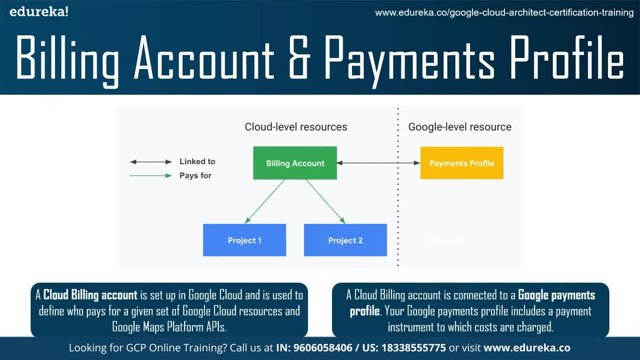 who pays for given set of Google Cloud resources and Google map platform. api's access control to a cloud billing account is established by identity and access management rules. then a cloud billing account is connected to a Google payments profile. your Google payments profile includes a payment instrument to: 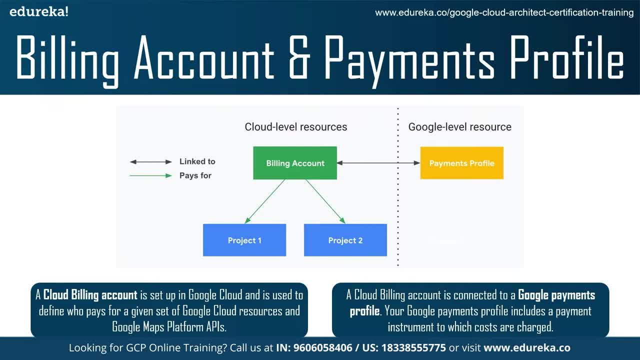 which costs are charged. so a cloud billing account is a cloud level resource managed in the cloud console, whereas Google payments profile is a Google level resource managed at paymentsgooglecom. a cloud billing account like tracks all the costs incurred by a Google Cloud usage. a cloud billing account can be linked to one or more projects and projects usage is. 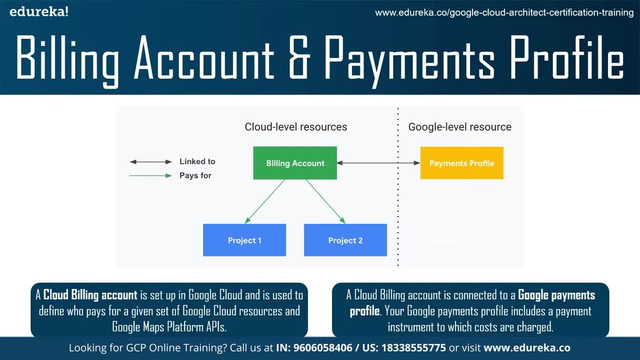 charged to the linked cloud billing account- okay, whereas a Google payments profile connects to all of your Google services, such as Google Ads, Google Cloud and five phone services. a cloud billing account results in a single invoice for a cloud billing account- okay, and a Google payments profile process. 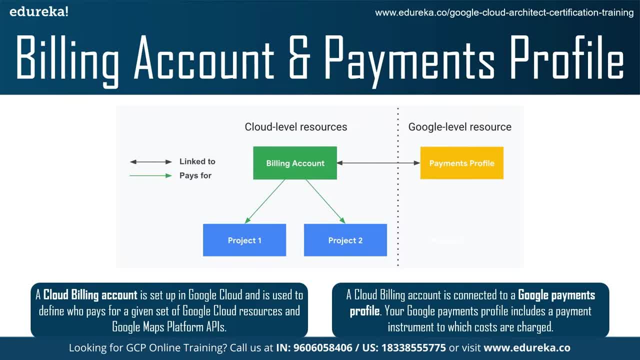 payments for all Google services, not just Google Cloud. a Cloud billing account operates in a single currency and defines who pays for a given set of resources. a cloud billing account is directed to a Google payments profile which includes a payment illustrating defining how you pay for your charges. 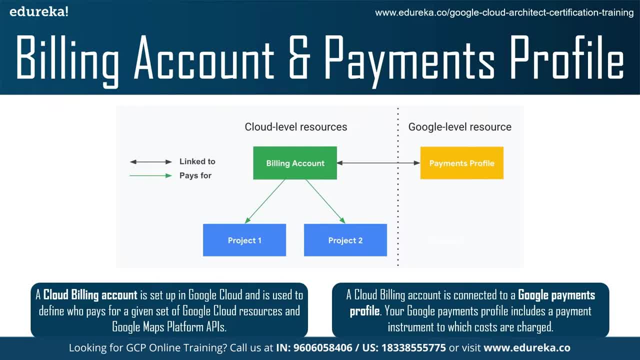 Google payments profile on the other side stores information like name, address and tax ID, when required legally and who is responsible for the profile. also, it stores your various payment instruments, like credit cards, debit card, bank accounts and other payment methods you have used to be able to pay for these own accounts. 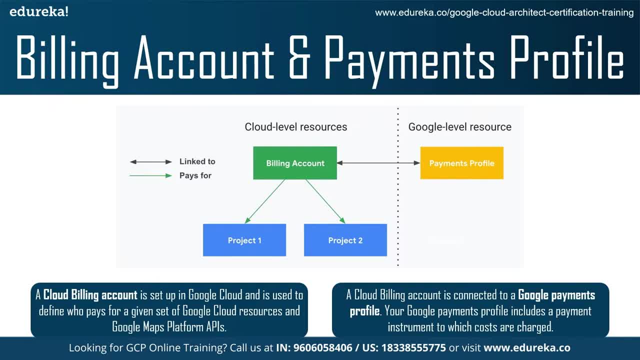 buy through google. in the past also, google payments profile functions as a document center where you can view invoices, payment history and so on. cloud billing account has, like billing, specific roles and permissions to control accesses and modifying billing related functions established by entity and access management roles, whereas google payments profile controls who can view. 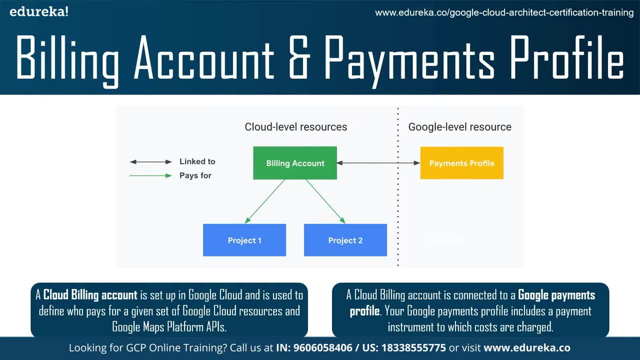 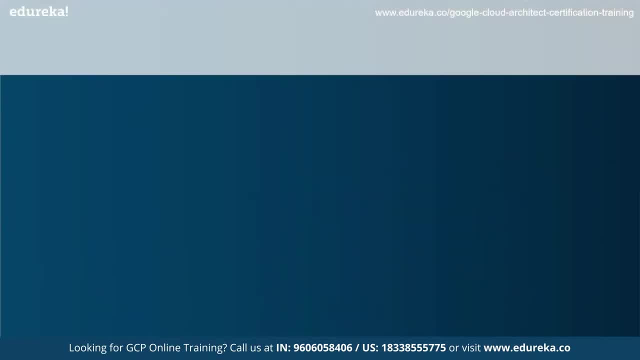 and receive invoices for your various cloud billing accounts and products. now let's understand the types of cloud billing accounts and profile. so there are two types of cloud billing accounts. first is self-serve account, so in which the payment instrument is a credit or debit card or 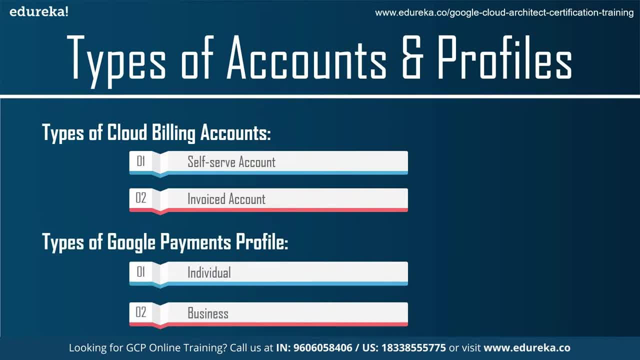 ach direct debit, depending on availability in each country or region, and in that the costs are charged automatically to the payment instrument connected to the cloud billing account. you can sign up for soil server accounts online. the documents are needed for self-serve accounts include statements, payment receipts and tax invoices, and are accessible. 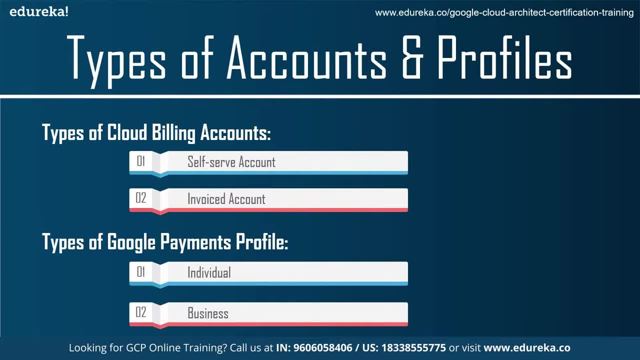 in the cloud console. and the second one is invoiced account, or you can say offline account. in this the payment instruments can be checked, or via transfer. invoices are sent by mail or electronically. invoices are also accessible in the cloud console as our payment receipts. you must be eligible for invoice billing, so for that, learn more about invoice billing. 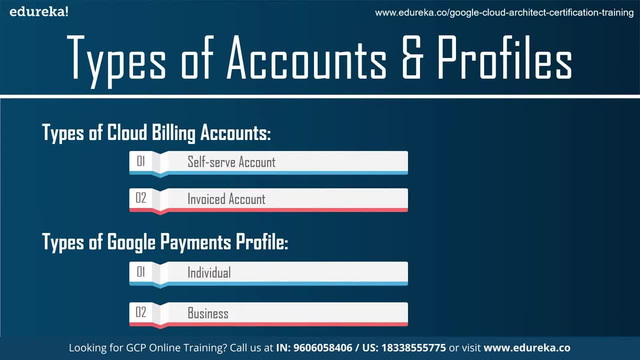 eligibility. you can learn that from the documentation of your gcb billing on a google platform documentation. okay, now coming to the types of google payments profile, when you create your information on cloud service, you need to set up your cloud service profile. in your execution. create your payments profile, you will be asked to specify the profile types This information must. 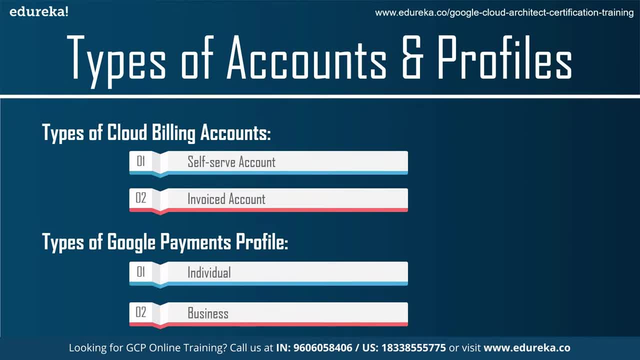 be accurate for tax and identity verification. This setting can't be changed. when you are setting up your payments profile, Make sure to choose the type that best fits how you plan to use your profile. There are two types of payments profile. One is individual and another is business. So in 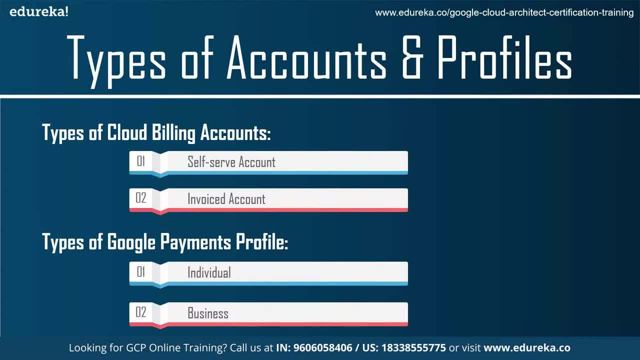 individual. you are using your account for your own personal payments. If you register your payments profile as an individual, then only you can manage the profile. You won't be able to add or remove users or change permissions on the profile And in business payment profile you are paying on behalf. 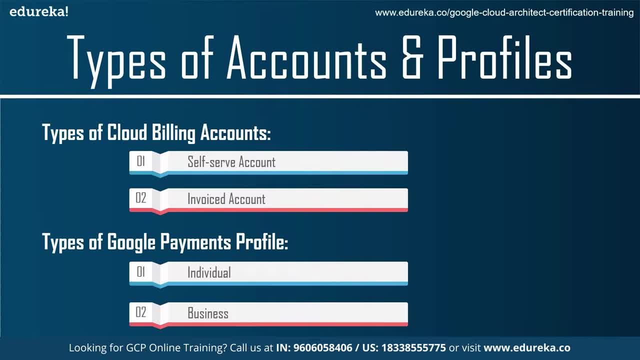 of a business, organization or partnership or educational institution. You use Google Payments Center to play apps and games and Google services like Google Ads, Google Cloud and Fire Phone services. A business profile allows you to add other users to the Google Payments profile you manage so that more than one person can access or manage a payments profile. 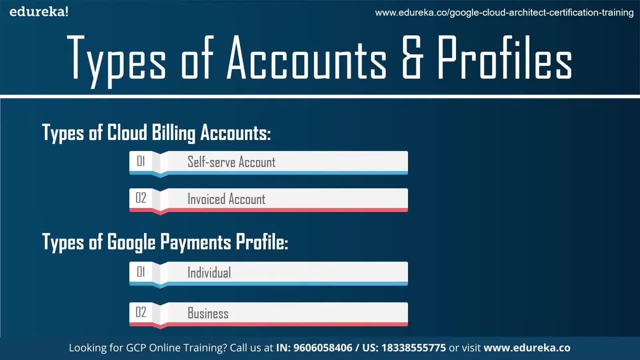 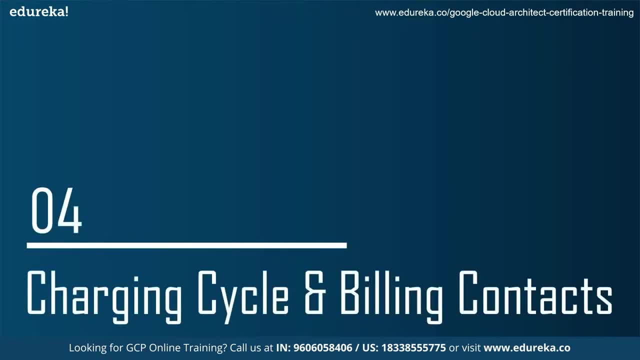 All users added to a business profile can see the payment information on the profile. Now let's understand the charging cycle and billing context in GCP billing criteria. okay, So first understand the charging cycle. So the charging cycle on a cloud billing account determines how and when you 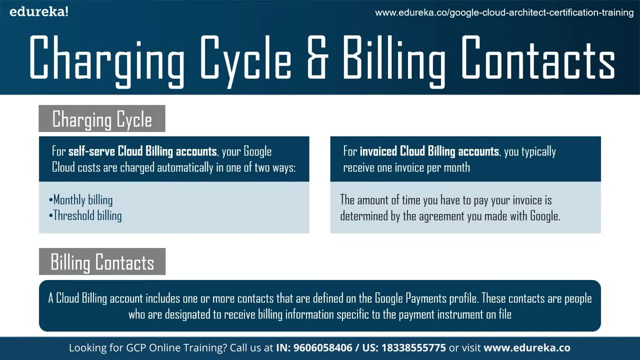 pay for your Google Cloud services and your use of Google Maps platform APIs For self-serve cloud billing accounts. your Google Cloud costs are charged automatically in one or the two ways You can see of like your monthly billing. which are your costs, and your billing costs You can see. 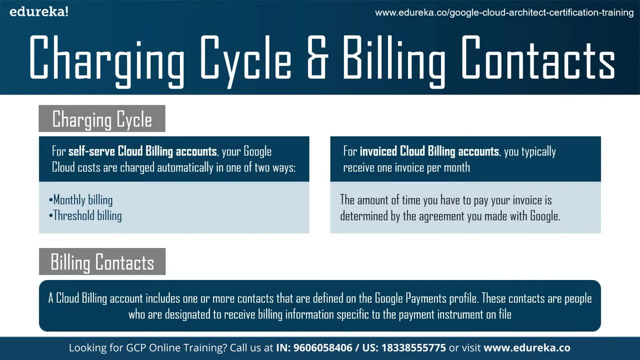 the costs are charged on a regular monthly cycle and the second is the threshold billing in which the costs are charged when your account has acquired a specific amount. For self-serve cloud billing accounts, your charging cycle is automatically assigned when you create the account. You do not. 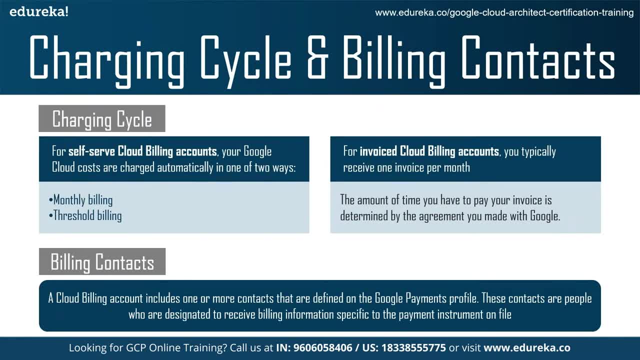 get to choose your charging cycle and you cannot change the charging cycle For invoice cloud billing accounts. you typically receive one invoice per month and the amount of time you have to pay your invoice means your payment terms is determined by the agreement you made with the Google. Now let's understand the billing context. A cloud billing account includes: 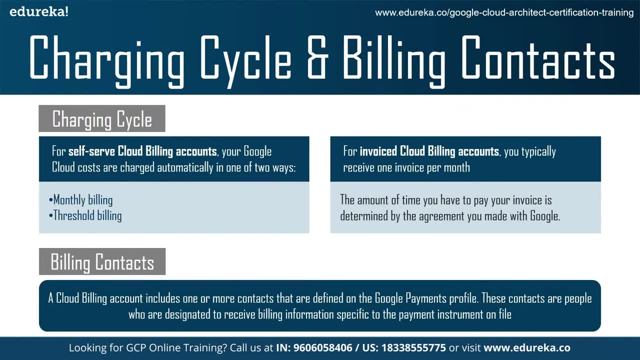 one or more contacts that are defined on the Google payments profile that is connected to the cloud billing account. These contacts are people who are designated to receive billing information specific to the payments instrument on file, For example, when a credit card needs to be updated To access and. 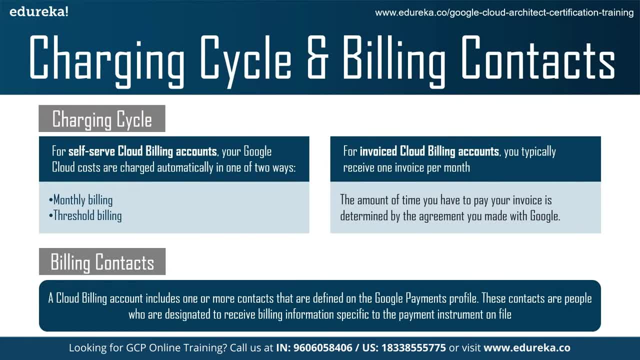 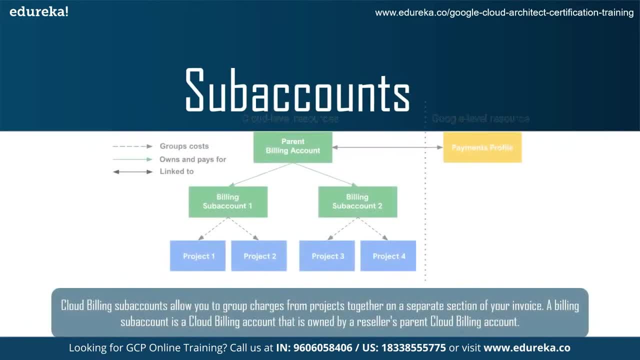 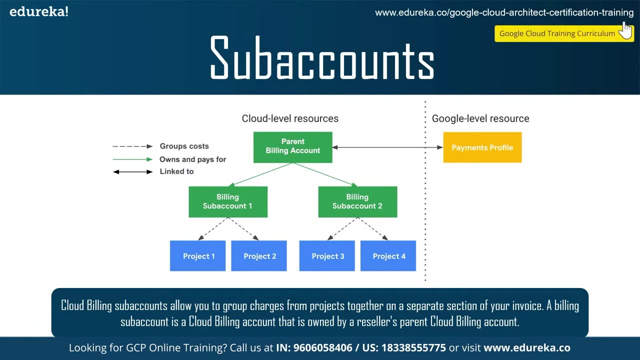 manage this list of contacts. you can use the payments console or you can use the cloud console. Now understand the billing sub accounts under cloud billing accounts. So subaccounts are intended for resellers. If you are a reseller, you can use subaccounts to represent your customers. charges for the purpose of charge. 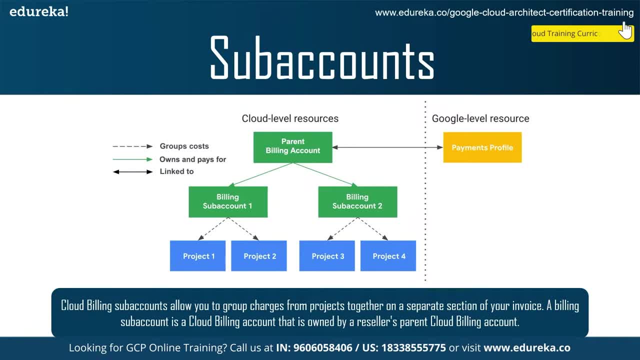 packs. Cloud billing subaccounts allow you to group charges from projects together on a separate section of your invoice. A billing subaccount is a cloud billing account that is owned by a reseller's parent cloud billing account. The usage charges for all billing subaccounts are paid for by the 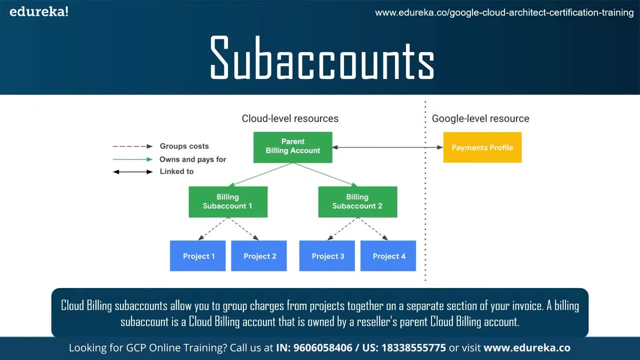 reseller's parent cloud billing account. Note that parent cloud billing account must be an invoice billing. a sub account behaves like a Where to request an application cloud billing account. in most ways. it can have projects linked to it, cloud billing data exports can be configured on it and it can have identity andxs management rules defined on it. Any charges. 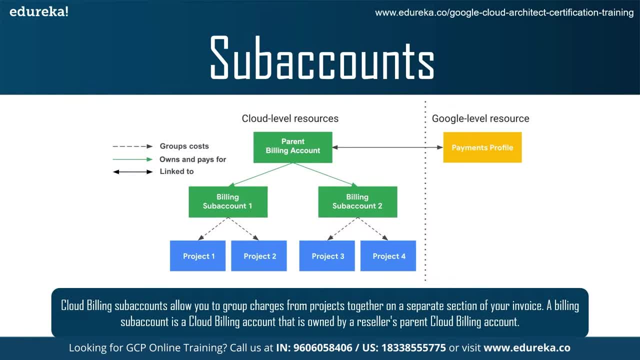 made to projects linked to the sub account or grouped and supported on the invoice, and the effect on resource management is that access control policy campaign entirely segregated on the sub account to allow these classes to be خ Nations streaming online is a subaccount, are grouped and supported on the invoice and the effect on resource management is that access control policy can be entirely segregated on the subaccount via subaccount are. so usd policy can be entirely aerodegradable to allow public application permission or other liability concerns that may resist against the company's financial support efforts. the access control policy can be entirely segregated on the subaccount to allow ple lukeruption". 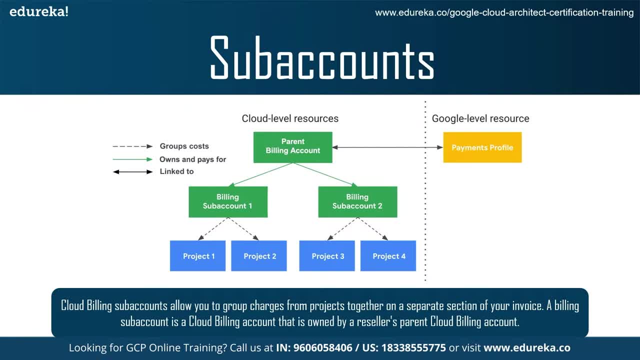 12. activity 8 nd. 11. segregated on the sub account to allow for customer separation and management. the cloud billing account api provides the ability to create and manage sub accounts. use the api to connect to your existing systems and provision new customers or chargeback groups. 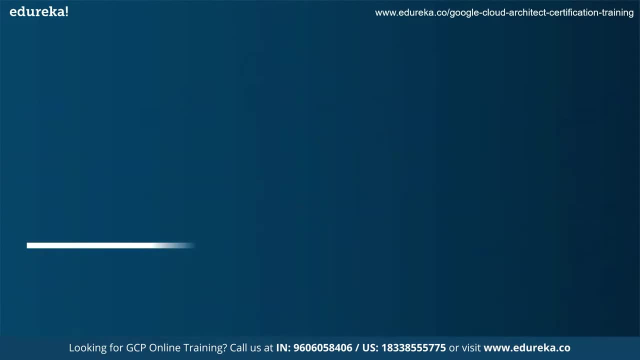 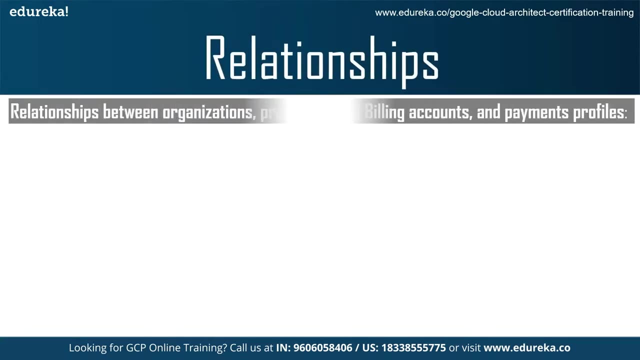 programmatically. now let's understand the relationships between organizations, projects and cloud billing accounts and payments profile. there are two types of relationships that govern the interactions between organization cloud billing accounts and projects, that is, ownership and payment linkage. so ownership refers to an identity and access management permission. 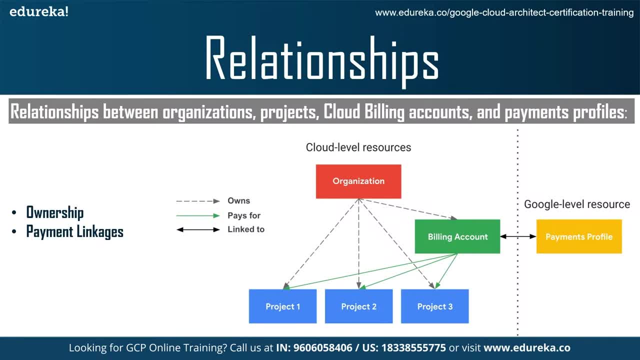 inheritance and payment linkage is defined which cloud billing account pays for a given project. ownership of a cloud billing account is limited to a single organization. payment linkage of a project linked to a cloud billing account is not limited by organization ownership. it is possible for a cloud billing account to pay for projects that belong to an organization that is different from. 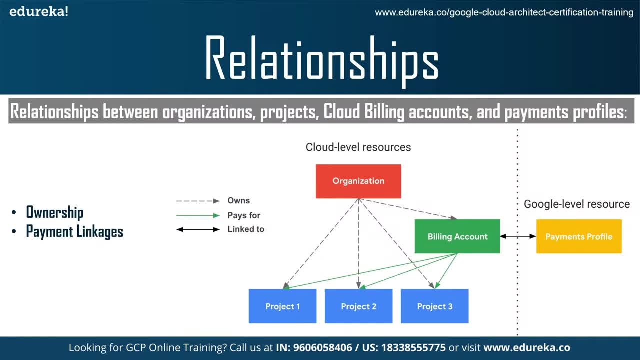 the organization that owns the cloud billing account. the following diagram you can see shows the relationship of ownership and payment linkages for a sample organization. in the diagram, the organization has ownership over projects one, two and three, meaning that it is the iam permissions parent of the three projects. the cloud billing account is linked to project one, two and three. 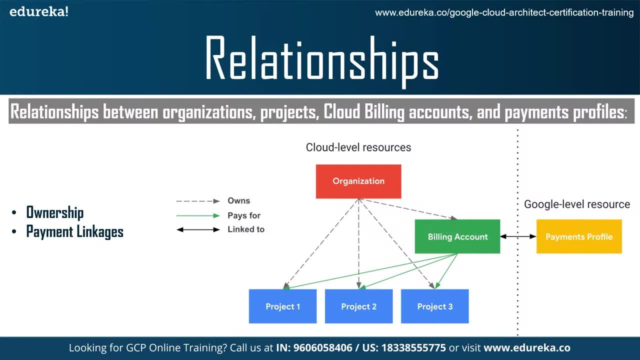 meaning it pays for costs incurred by the three projects. note that, although you can link cloud billing accounts to projects, cloud billing accounts are not parents of projects in an entity and access management sense and therefore projects don't have the ability to pay for projects. they don't inherit permissions from the cloud billing account. they are linked to the cloud billing. 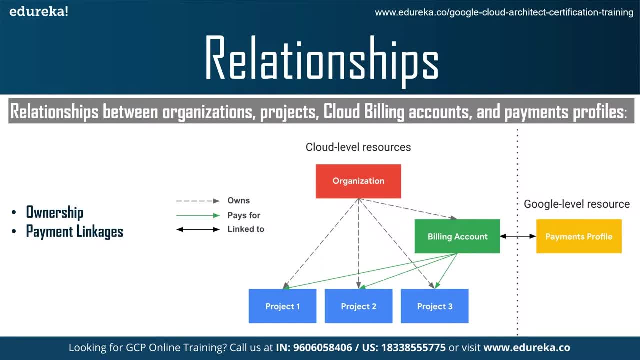 account is also linked to a google payments profile, which stores information like name, address and payment methods. in this example, many users who are granted entity and access management billing roles in the organization also have those roles on the cloud billing account or the projects, now that you have a theoretical understanding of billing criteria in google cloud platform. 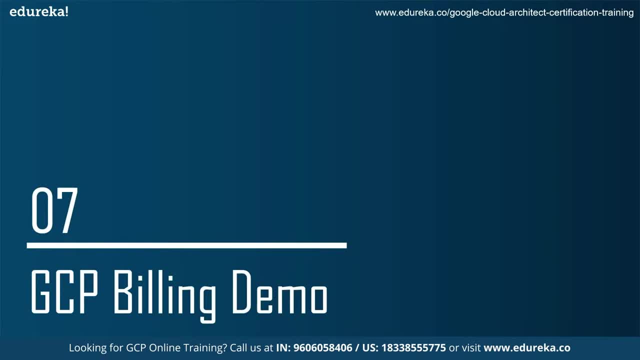 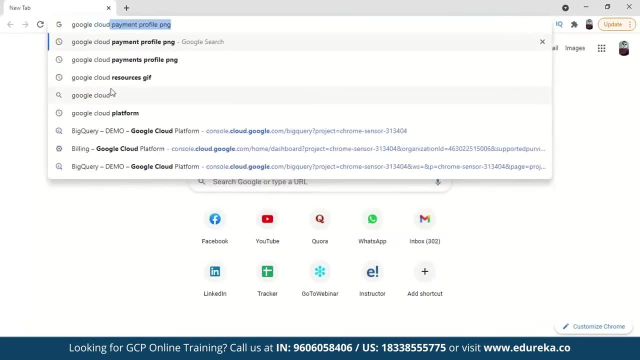 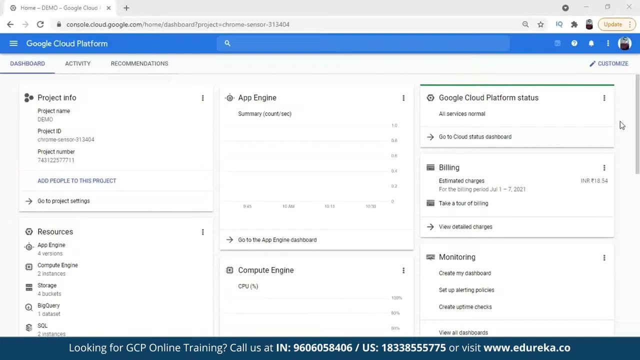 let's now see how it's been done practically by trying our hands on it. on google cloud platform, you can just guide directly, go to the google cloud console. so i already have my account login here. if you don't have an account on google cloud platform, create one. it's a very good platform to have your account on. you will just 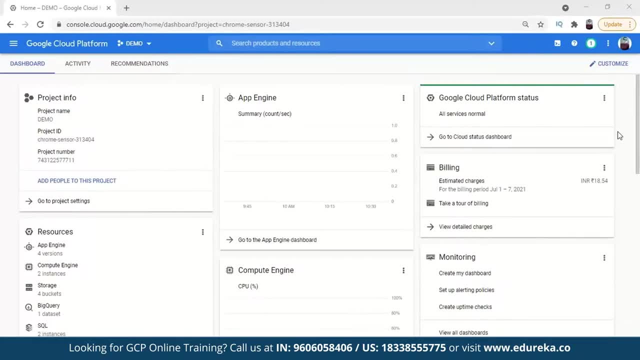 ask for a little bit of information, including debit, of credit card details, and it will just deduct a very like small amount of money- one or two rupees, that's it, and that will also be refunded, and what you will get is a. by creating a google platform account, you will 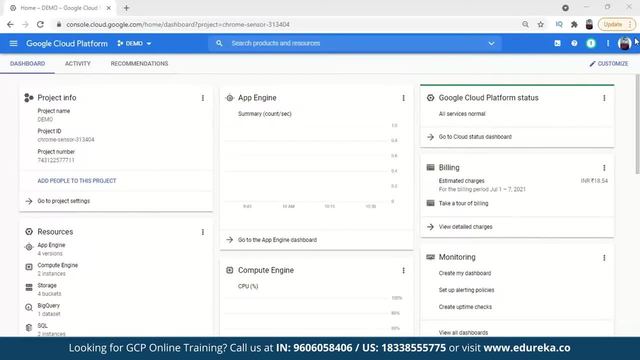 get a 90 days free trial in which you will get 300 of free credit and you can use that for certain demos of like big piri or big table or you can say of compute engine, virtual machine instances, launching any kind of service you can use using those free credits. okay, 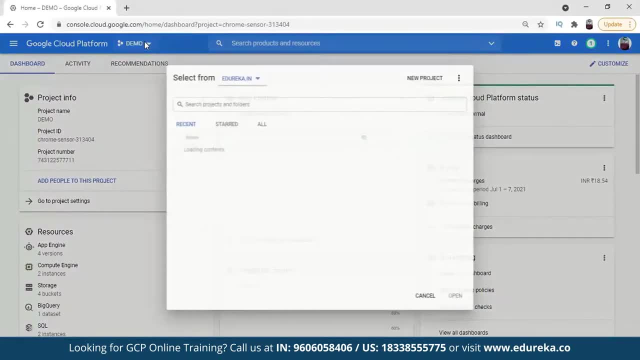 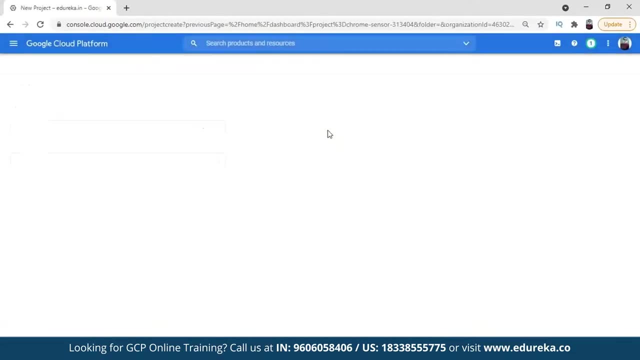 so this is the project i can show you, like you can go here and create a project, okay, or you can like- i have like certain projects here, but i will create one more new project, okay, so that I can show you how billing can be linked to this project. 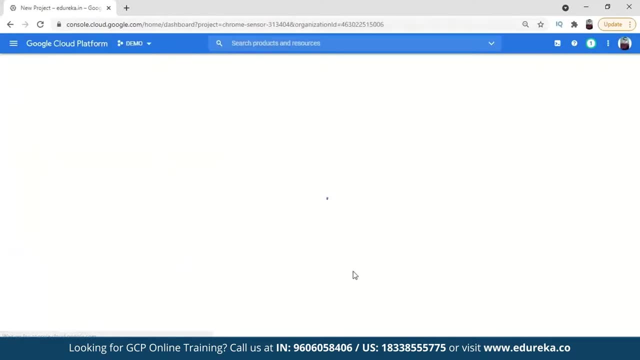 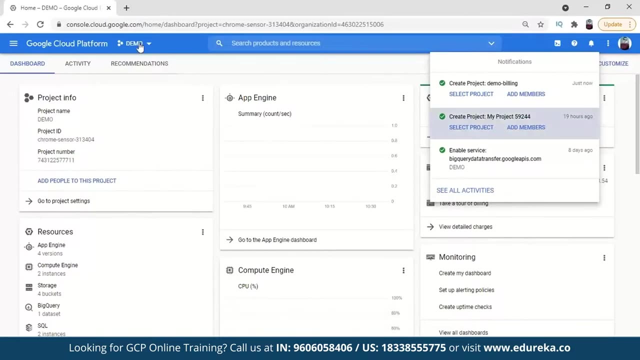 So I will just make. the project is getting created. You can see the project name. Okay, this is the older one, So we will just open the new one: Demo billing: Yeah, So now you can see the project name here. 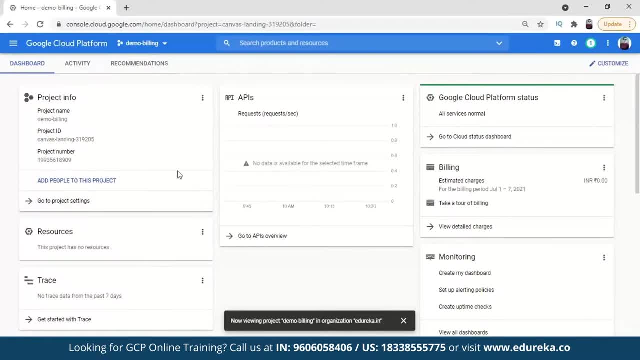 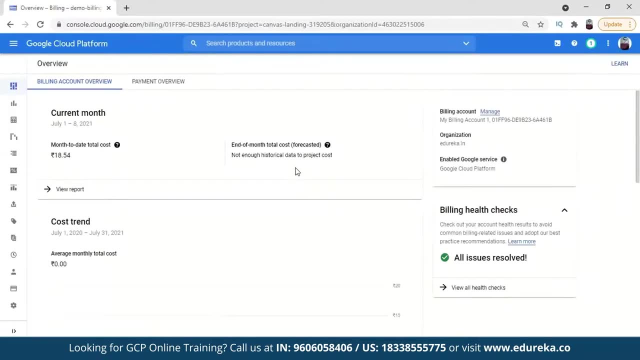 project ID has been shown and project number, everything is here. But right now the billing account has not been linked to it. So we can just go here and open billing from here, So we can manage from here. What you can do is you can create a new billing account. 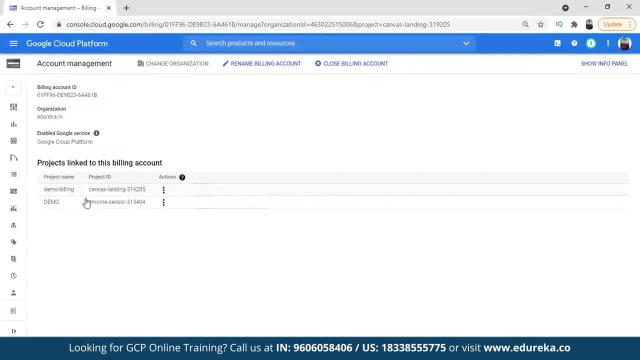 also, like for this, we can say, right now, it's because it's been linked, because there's a limit of three- like if you're making projects, so only three accounts can be linked to a billing account. And right now, before making this project, 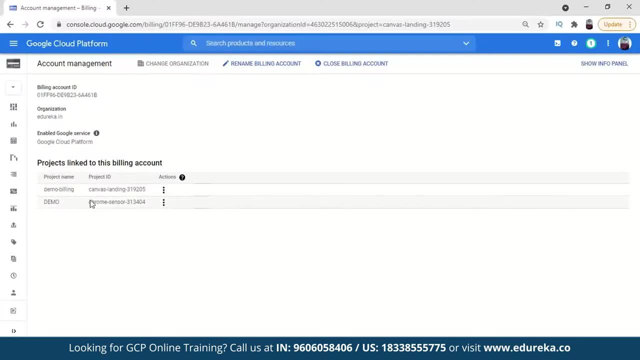 I only had one account linked to it, So I just created another and it got automatically linked to it. Okay, So it just got linked and means it got it linked by itself. but you can like if it don't get linked, you can if you open this from like billing section. 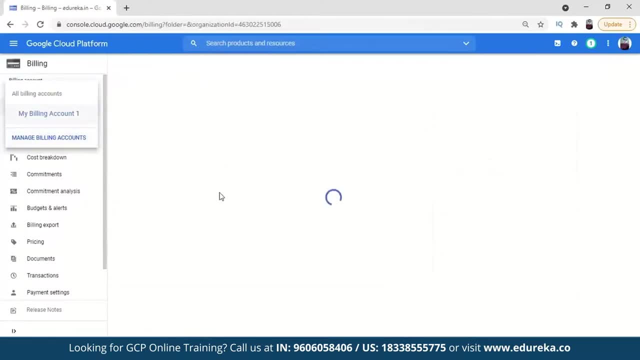 when you open up from there only you can link the account like: manage billing accounts is there, You can like go here, and if you don't have a billing account, you can create one billing account from here and then the account will be appropriated to it. 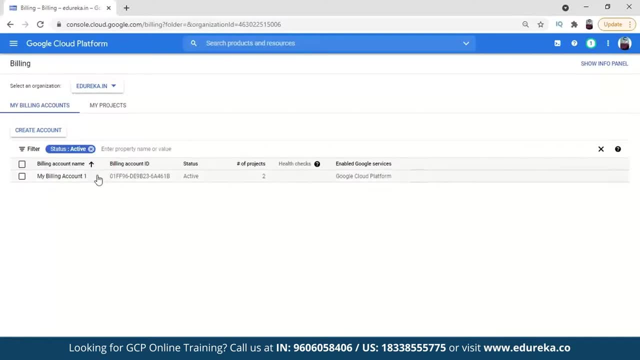 The billing account will be attached to your project. Okay, So we can see like there is one active billing account And if we close the active, then there are two account. This is the free tire account. Actually, my free tire is over. 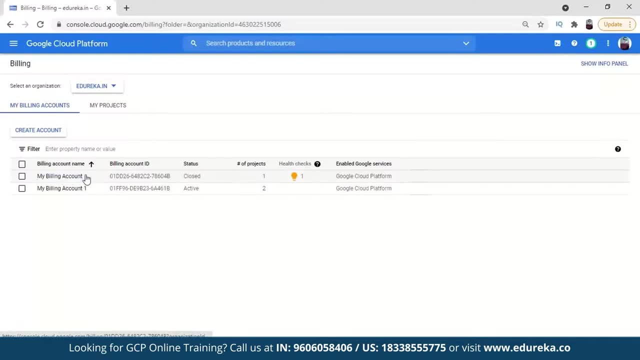 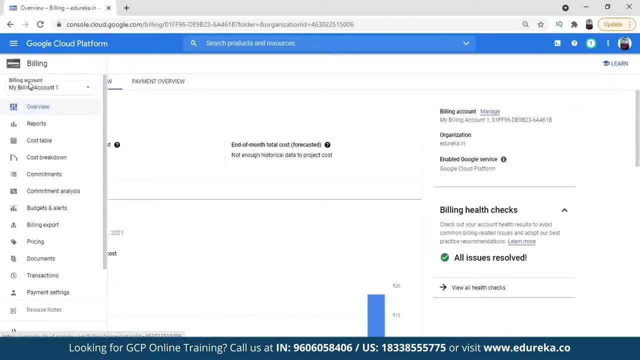 So it's closed. now That is my billing account. This is the free tire account And right now we are accessing is my billing account one. Okay, So that's how it's get linked And then what you can see here, like it's showing the billing account. 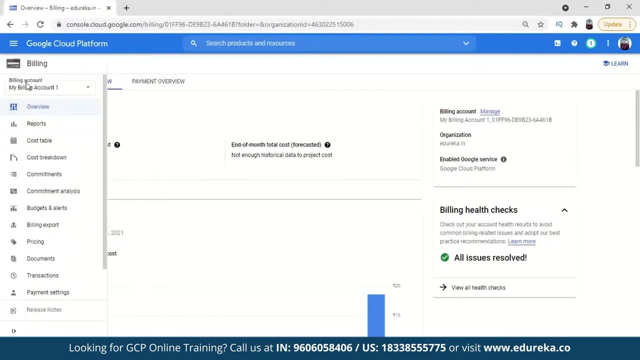 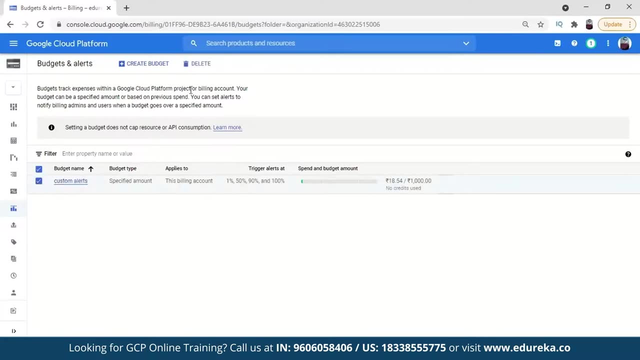 my billing account, one we are accessing right now. Now what we can do is we can set the budgets and alerts for it, So we can just go to budgets and alerts. Right now the budget is being created for that. We can delete this one. 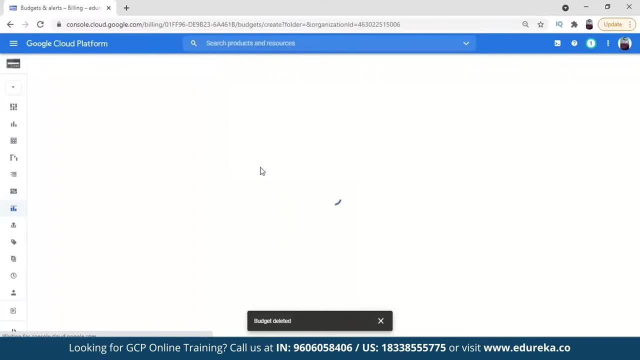 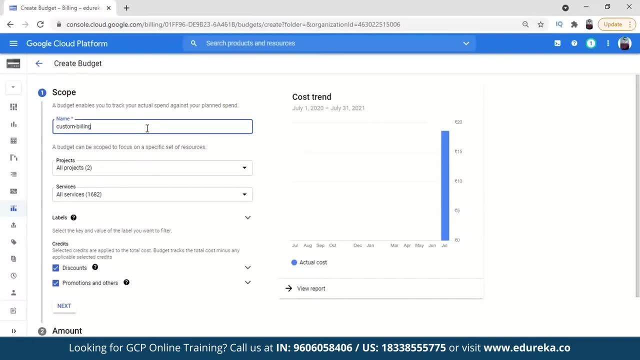 This is the older one, So we will just delete this one and we can create budget. So all you have to do is give a name. So we can say, like custom, and you can like select for which you want to give, Like there are, two are there. 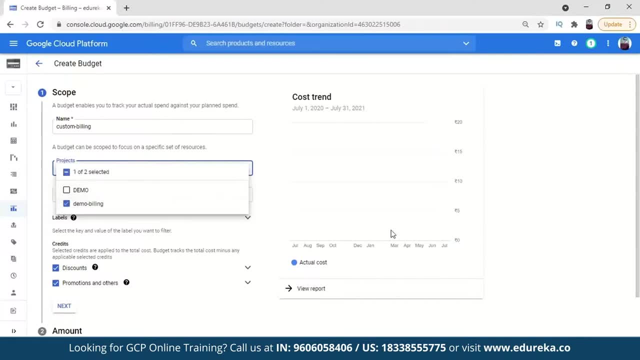 Two projects are there: demo or demo billing. But we have to choose the demo billing. So we are just going to choose demo billing Or we can choose all of them also. It's up to us, And then we can go for all services. 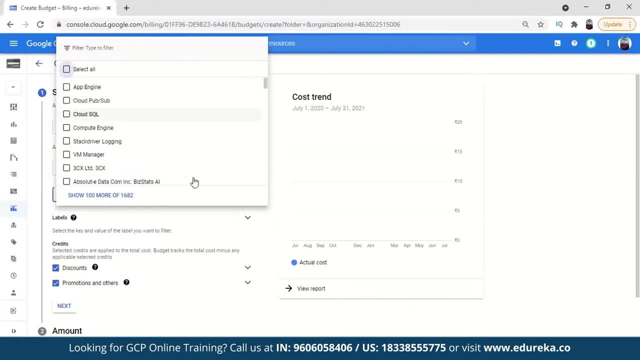 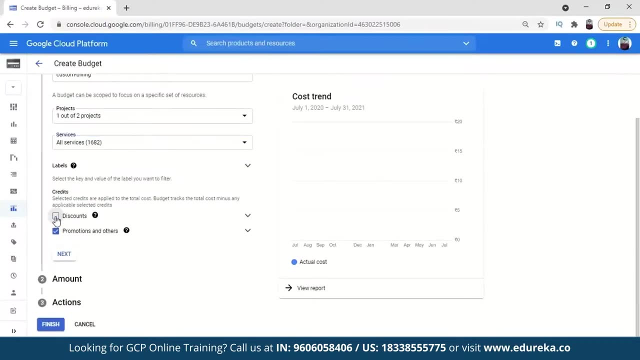 You can choose a specific service also, or you can choose all of them. So right now I'm choosing all of them. Yeah, And I've chosen all of them. And then I'm just right now I'm checking it because we want to see the price. 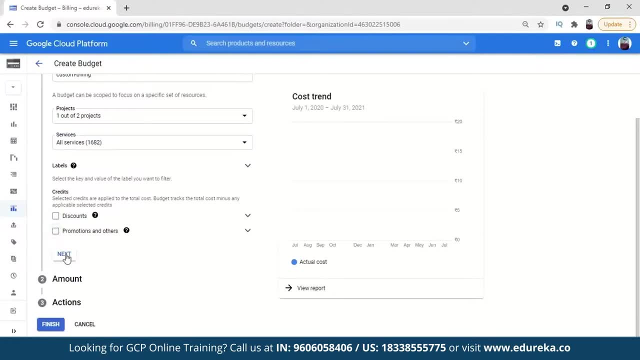 like without our discounts And promotion applied to it, So we can just go to the next thing. Then there are like two options here. You can see amount, Like if you want to give the last month's spend whatever you have spent last month. 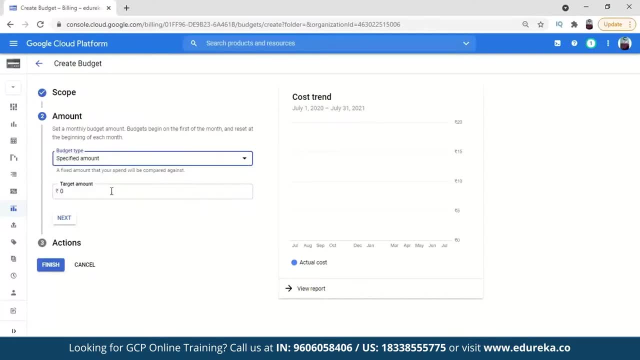 that will be applied here, Or you can just choose a specific amount, So I will just do the specific amount for it. Like I can give a thousand, Okay, And the maximum amount I'm going to choose, And that's thousand. Now you can see the. 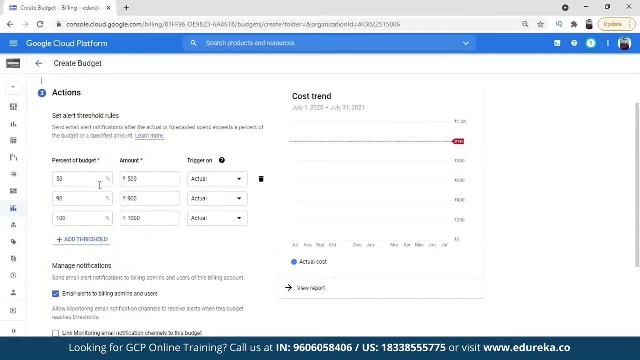 you can, like, put a threshold over it. If the Google will notify you, it will mail you or something, So that you get the alert that 50% of your budget is being spent, or 90% of your budget is spent, or a hundred percent of the budget is spent. 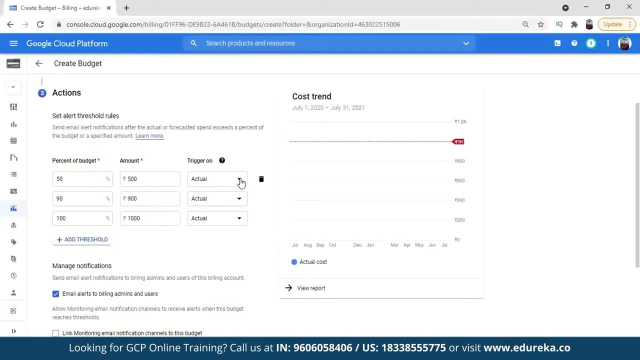 Okay, And from like: this is the amount on that basis, on the showing. Okay, So we can also go for actual or forecasted. So actual is like okay when it gets spent, I mean okay- And forecasted mean when it's. 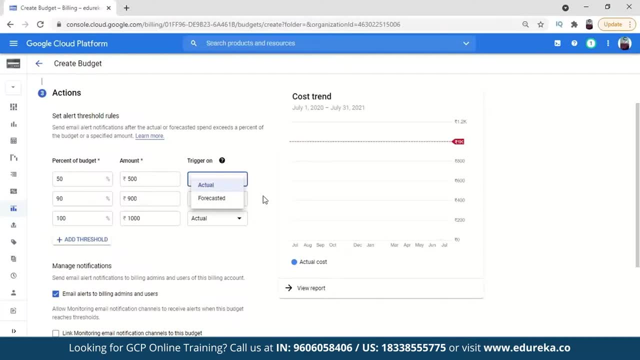 it will forecast that in how much time or in how much period of time it will get spent. It will notify you. Right now we are choosing actual and you can like create another threshold. if you want to like, I can give at 1% also. 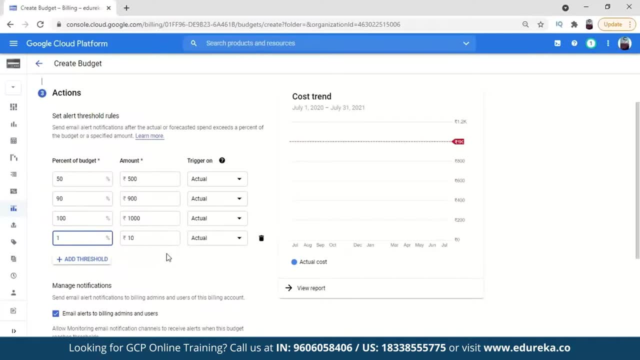 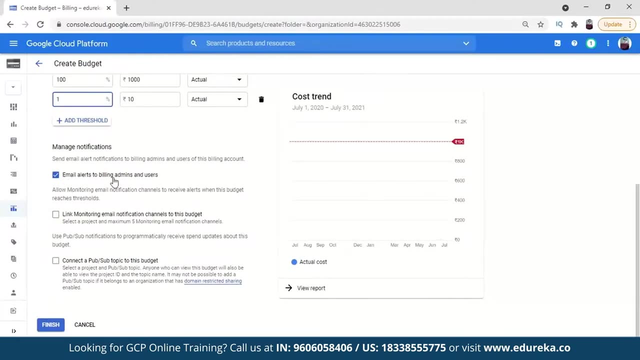 So 1%, that will be 10,. after 10 rupees will be spent, It will notify us, I mean, that this much amount has been spent. Okay, And you can like email alerts? Okay, It will email, So you can choose this so that you can get the email. 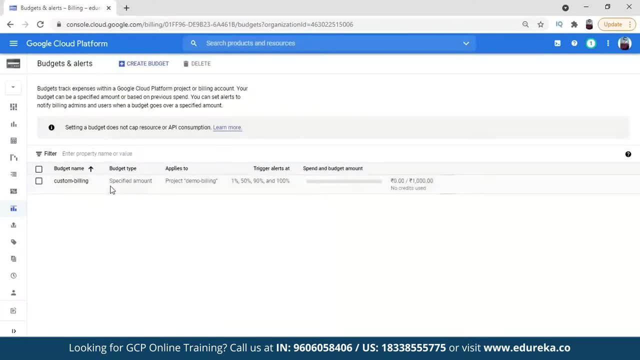 for threshold Okay, And you can just finish it. So custom billing has been made and zero credits are being used out of thousand That has been done, Then what we can do is go for billing export How you want to get it, export to your BigQuery. 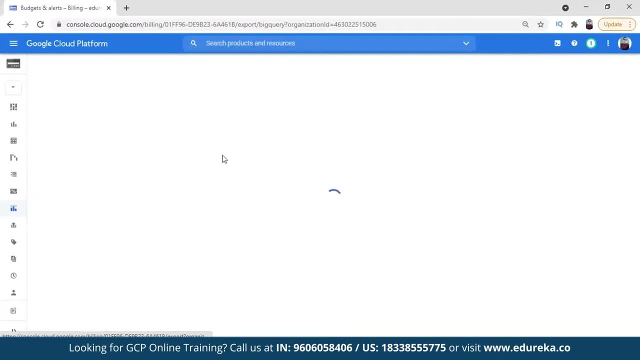 Okay, You can like export your billing, whatever you're billing amount and every information regarding billing. that will be exported to a BigQuery. It's enabled, actually, but it is enabled for demo right. It's not enabled for our demo billing project. 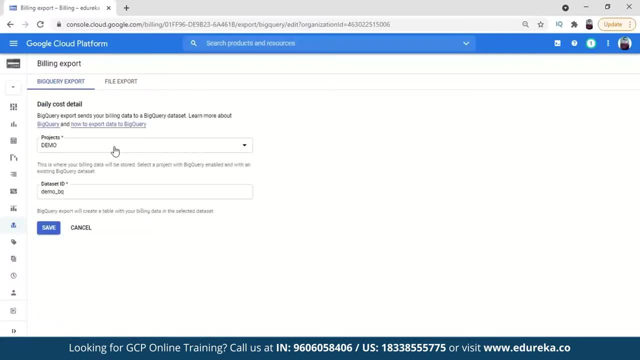 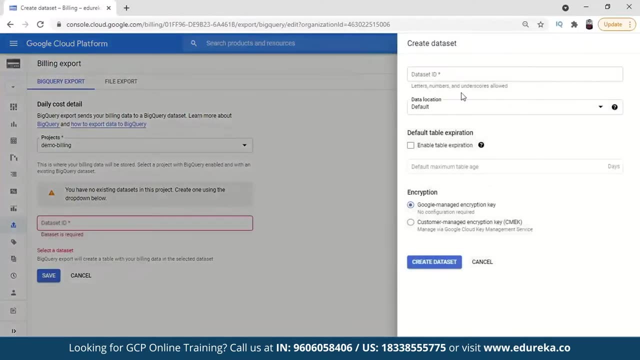 So what we can do is we can edit settings. We want to make it for demo billing, but right now we don't have a dataset, So create new dataset. we can do. This is getting created in BigQuery, under BigQuery only. 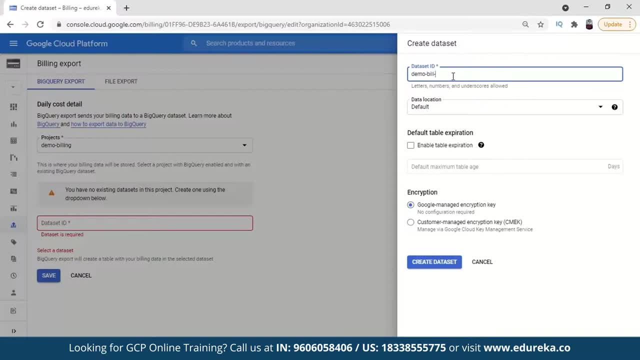 This dataset is getting created. So demo bill: underscore BQ: we can get. BigQuery, So data location default we can get. That's not a problem. So whichever location you want to choose and enable table expiration, Like it, is a very cool option. 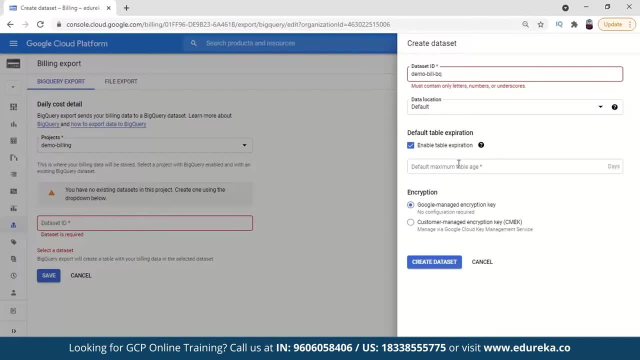 Like whatever data you are like getting saved in your table now under dataset. So for how many days should it retain, So you can get the number of days you want to retain, or if you don't want to delete it. So so, like just for a second you can understand. 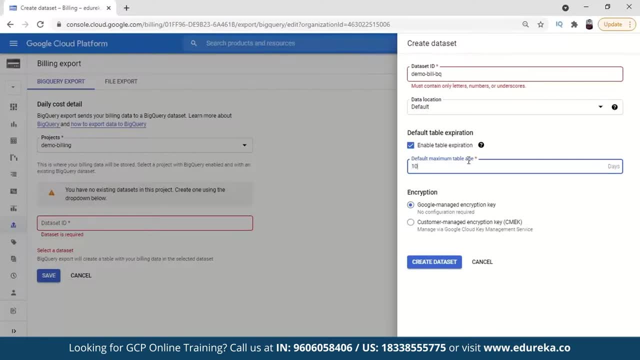 like you can give here 10 days. So if you give your 10 days after 10 days only, they're all the data under, under, under, under, under under data under table will get deleted. Even the table would get deleted. 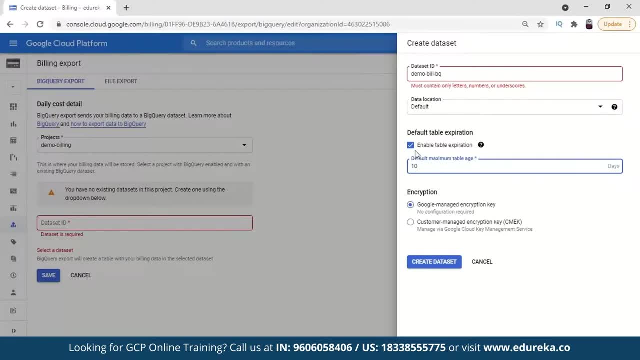 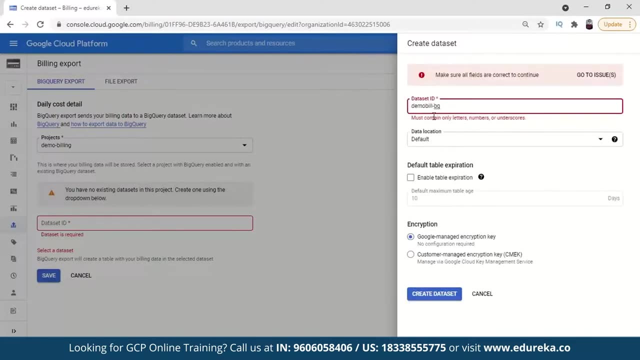 So in that sense, you can just give the days here or you can just remove it so that don't expires, Okay, So you can just create dataset. Okay, Must contain only letters. Okay. So demo bill BQ is okay, And just create dataset now. 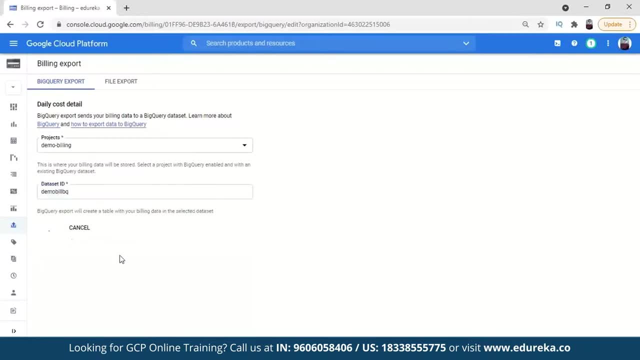 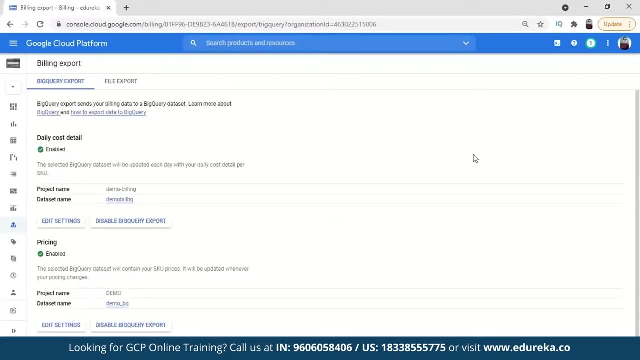 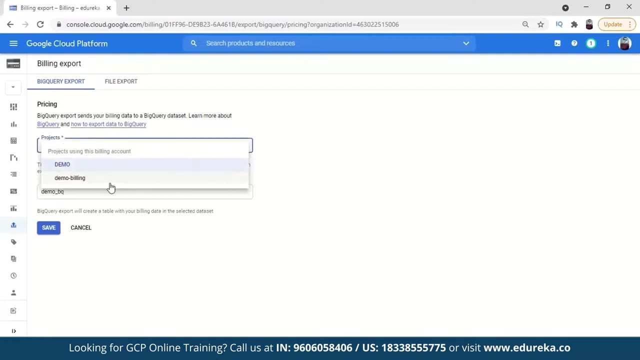 So dataset is being created, Demo bill BQ- we can choose and then we can save it. So BigQuery export has been getting created And then we can like also enable it for pricing. also, We can just go to edit settings. We can choose our project, that is, demo billing, and demo bill BQ. 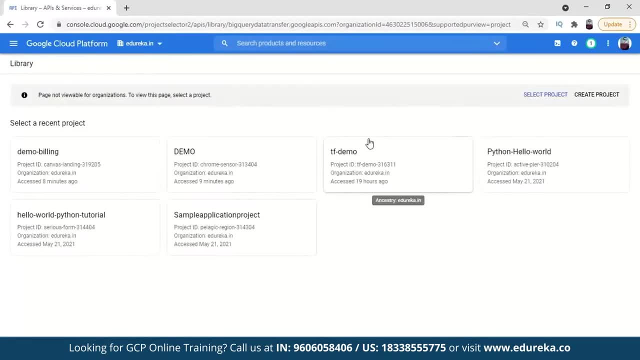 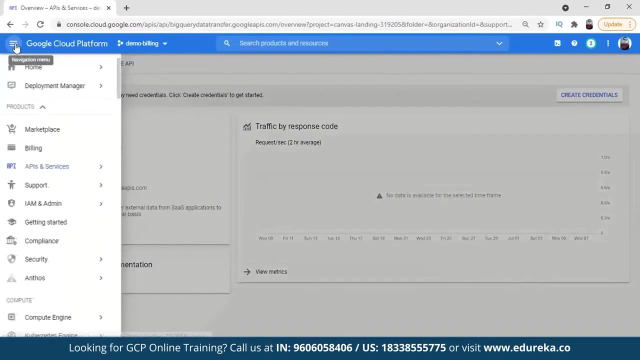 So we have to enable the data transfer API in BigQuery. So so we can just enable it, So we can just now go back to the billing, And then we can go back to the billing, And then we can go back to the billing. 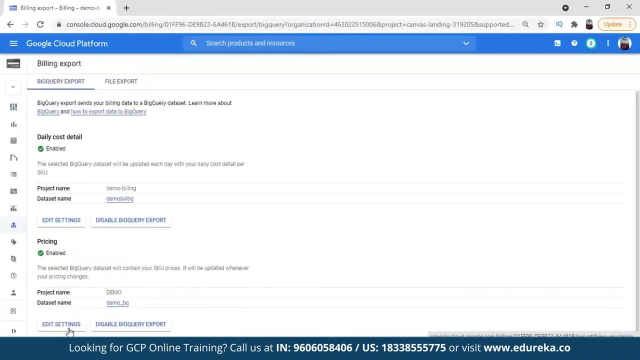 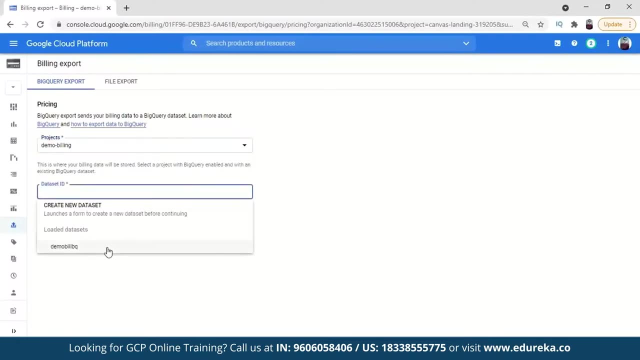 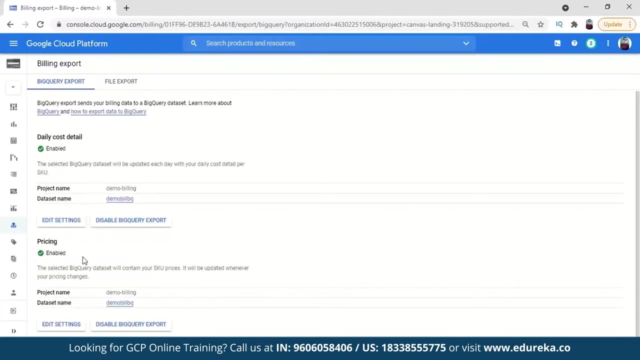 Export, And now we can do this As the data transfer API is being activated. Now we can go for demo billing and we can choose demo billing, IQ and save it. Okay, So the pricing has been enabled for demo billing And also the daily cost detail has also been enabled. 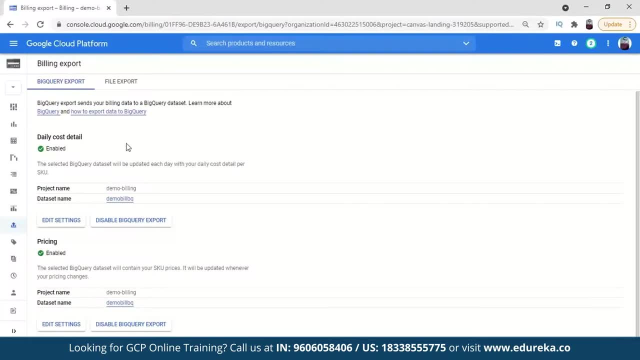 and that will be saved in your BigQuery dataset under the table- Okay, Whatever table it's been getting created under that So we can see the data set. So that will be there. You can see it in BigQuery also. Like, just go here. 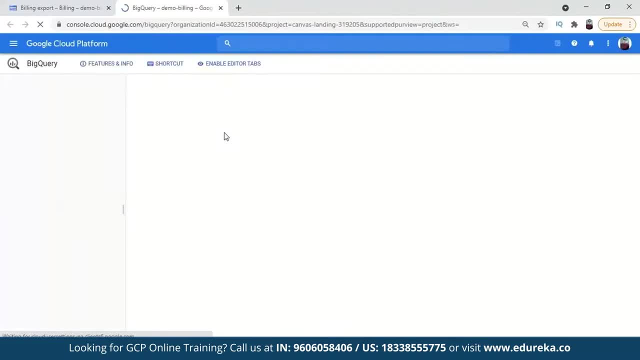 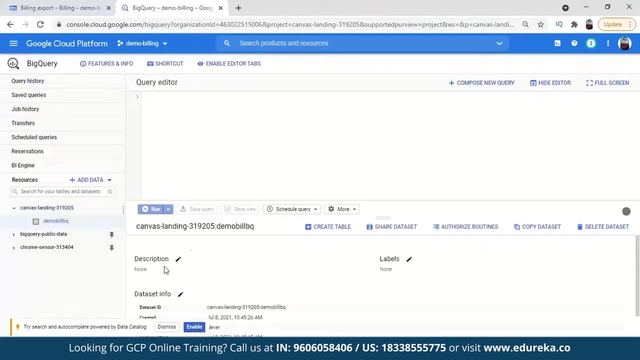 BigQuery: You can see the demo bill. IQ- You can see the dataset. So in this the table will be created. Right now it's not getting created, but it means when the data will be exported, at that time the table will be created. 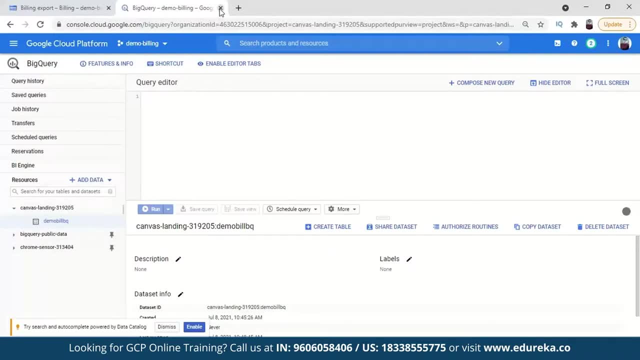 and the data will be saved here. So this has been showing in the BigQuery. Okay, I'm going to go back here. And now the last feature, that this is the main thing, that is, cost table. We can come to cost table. 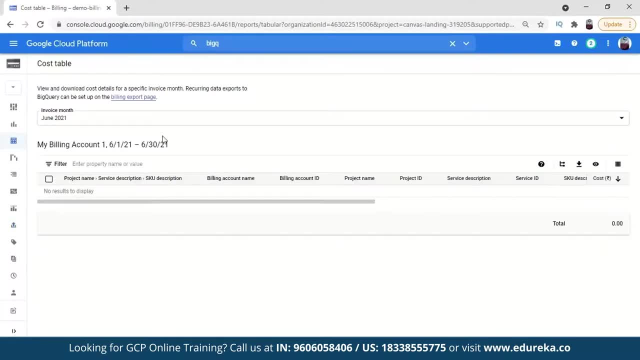 It will show you about the cost of your other sources you have used. So for this, like right now, I haven't made any resources in this billing account. What we can do is we can go to the data. I've told you Like I have that free direct account. 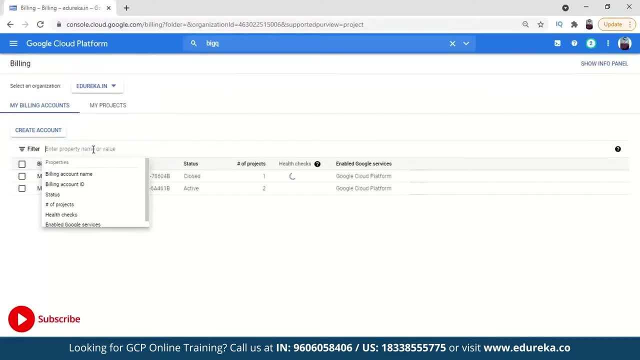 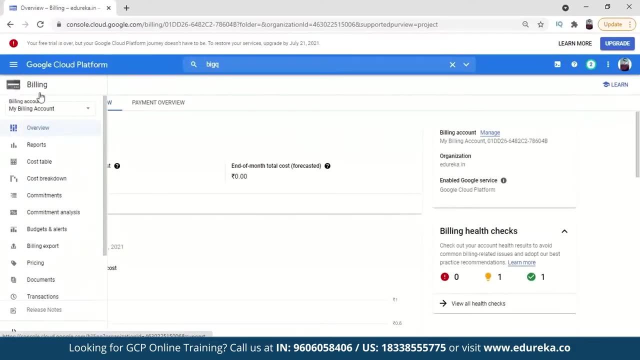 So we can go to that account. We can choose that account, Like we can remove and go to the older one, That is closed one, but we can choose this one. So we can just go to my billing account, this And now we can go to cost table. 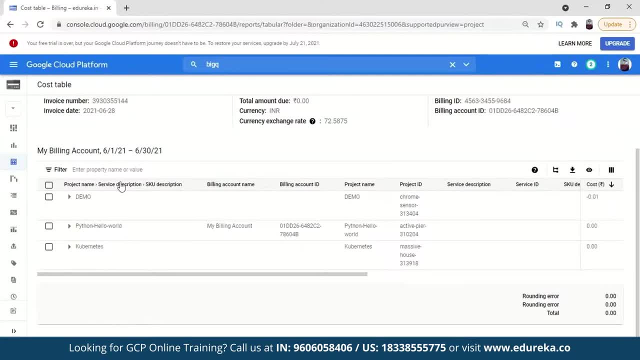 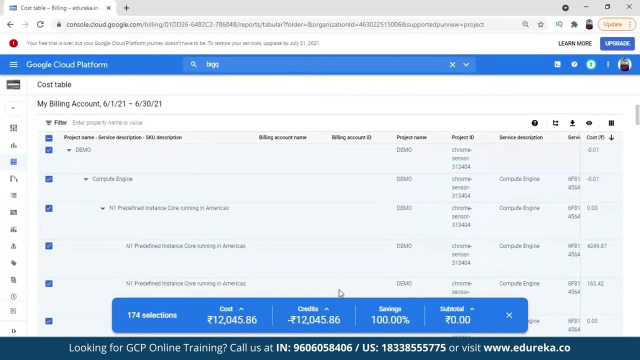 So here I have all the invoices for it, because I have used it, I have used resources in this, So we can choose this project. Okay, We will open this project demo Now. all the costs and everything which has been charged for this project, it's just showing here. 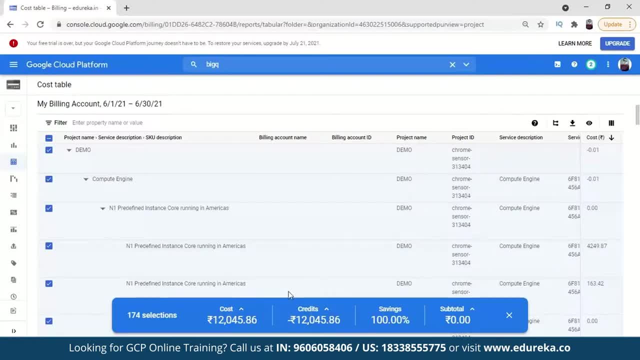 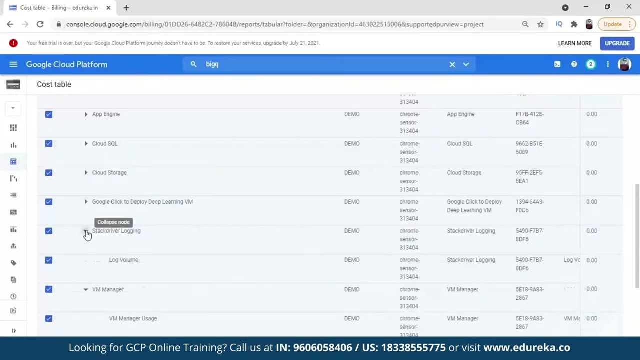 cost credit and everything, because this was a free entire account. So all of whatever is charged, it's been reimbursed at the same time. Okay, So you can choose for, like compute engine, Every resource has been elongated here So we can just minimize it, recover it, I mean. 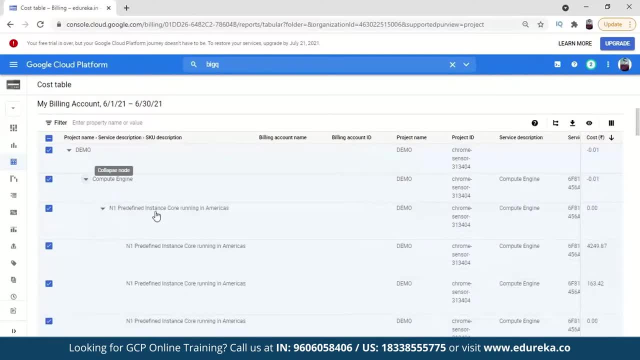 So in demo we have a compute engine. So in compute engine we can see like I have launched the instance and when predefined instance for America and everything, however it is being given. So you can see the prices for it, like the cost four to nine, seven. 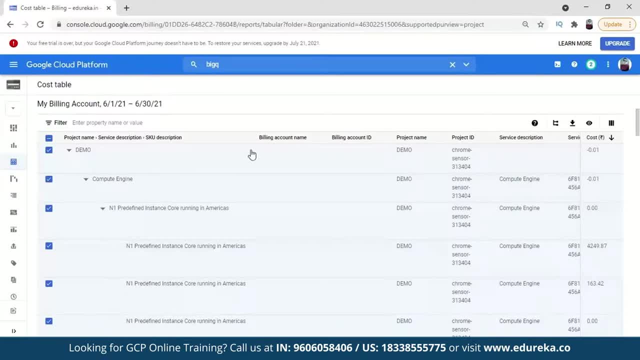 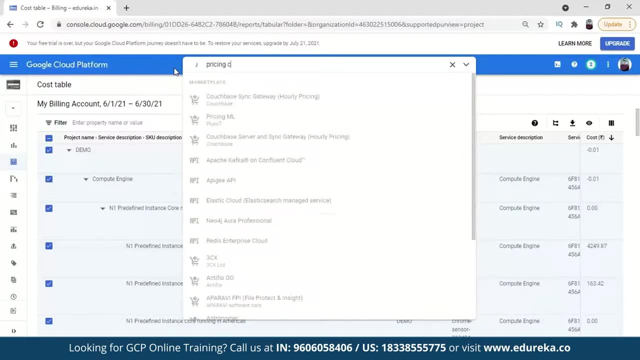 the virtual machine instance which I have launched. it is showing the cost four to nine seven. But we can check it from a pricing calculator also, like: how much does it cost Open from pricing calculator from here? So just open pricing calculator, okay. 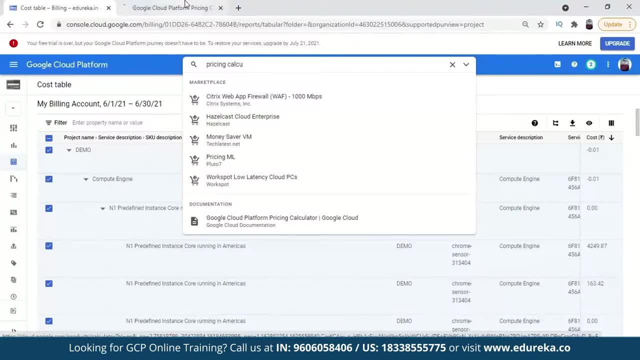 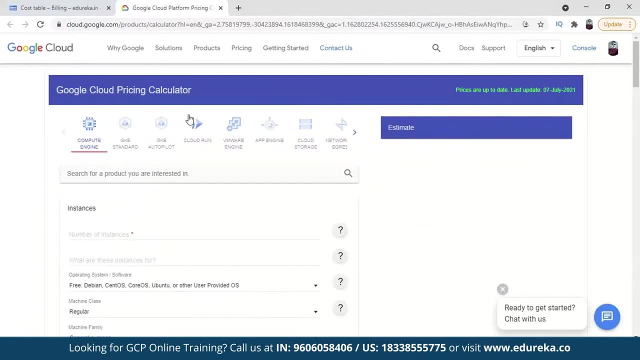 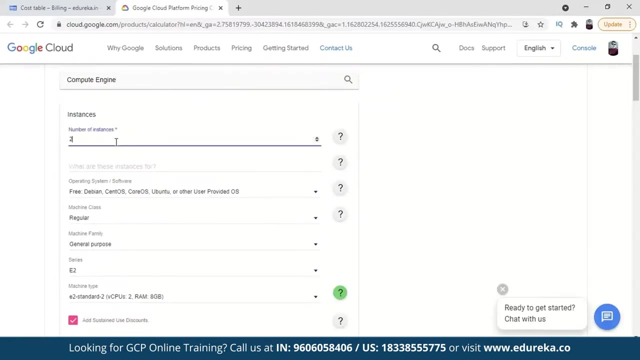 And we can just check, for instance compute engine instance like how much does it cost? I might have rendered for around a month, actually 20 days or a month. So in just compute engine and instances we are seeing so number of instances we can say like two instances. 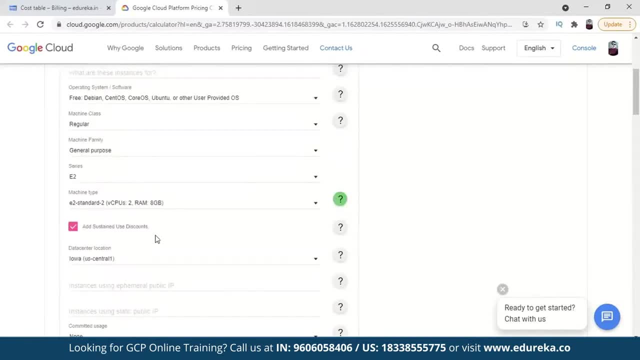 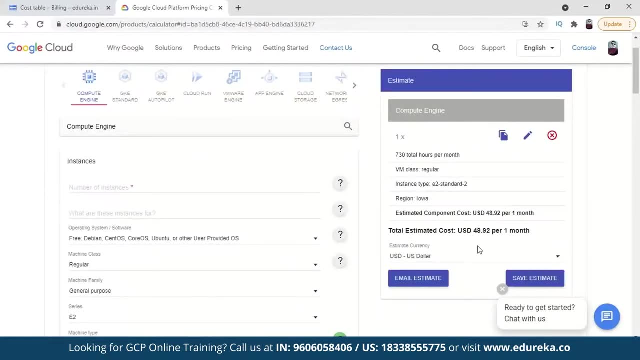 but we can okay check for one only. So, yeah, all these things are okay. okay, no problem. That's machine type standard only might have. I have chosen, so I have to estimate. So estimate cost: it's showing us $48.92 per month. 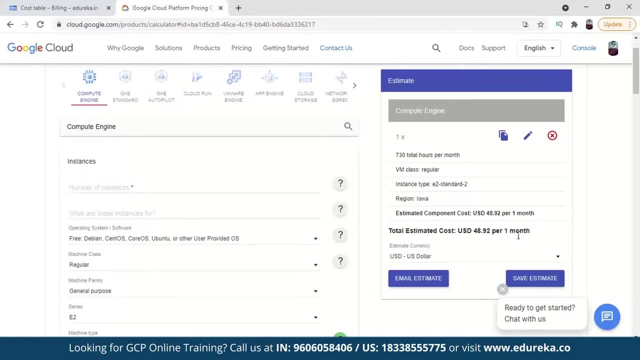 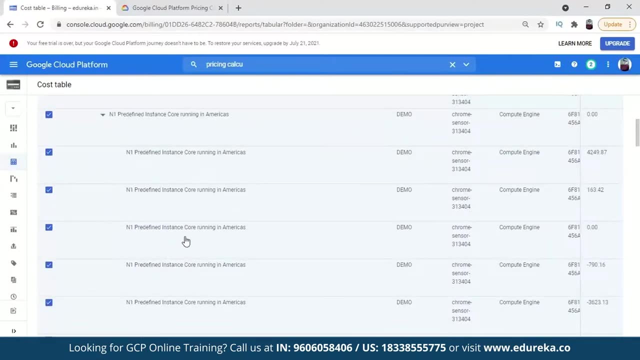 So that will come around around like 4,000, 5,000 only. So that's how I've been charged for it. Similarly, if you can see like there's a N1 Prefine instance score and N1 Prefine instance score running in Americas, 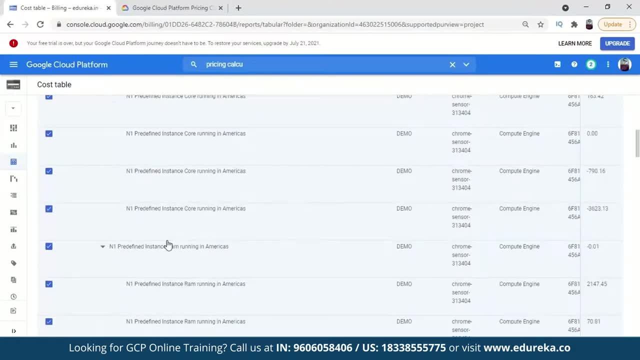 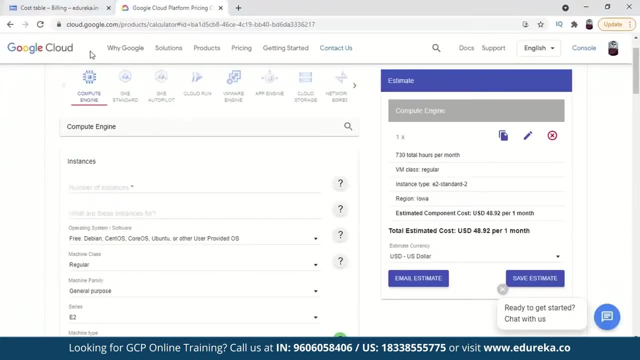 everything like how it has been charged: 163, other instance that might be. Then there's a RAM running, so for that also it's been costed around 2147.. That also you can check in pricing calculator only. So instance okay, it will come in instances only. 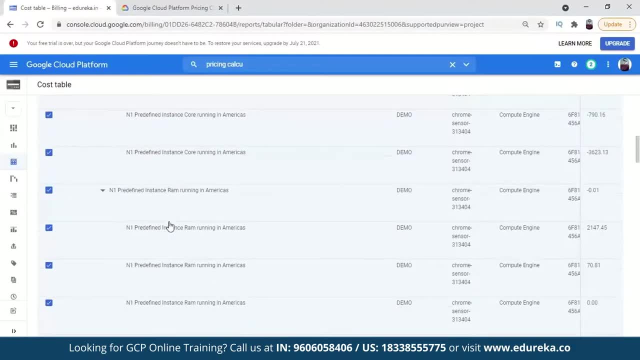 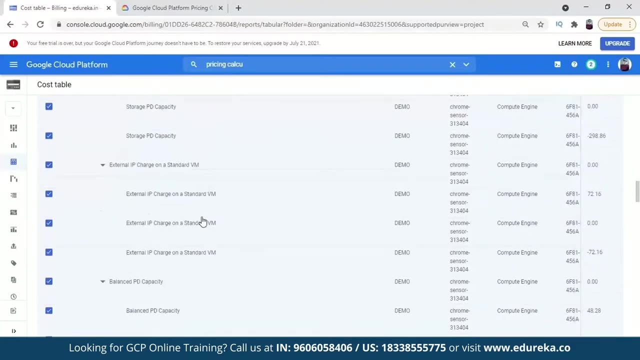 RAM and everything. So, for instance, for instance, RAM, So, and then we can see for you two instance score how it costed 756 rupees For everything. you can see like the cost is given for every resource. Similarly we can come for the App Engine also. 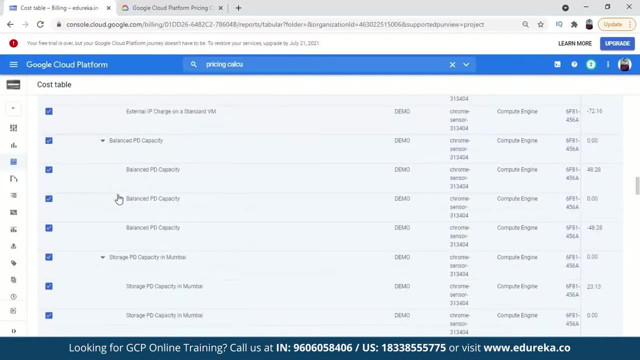 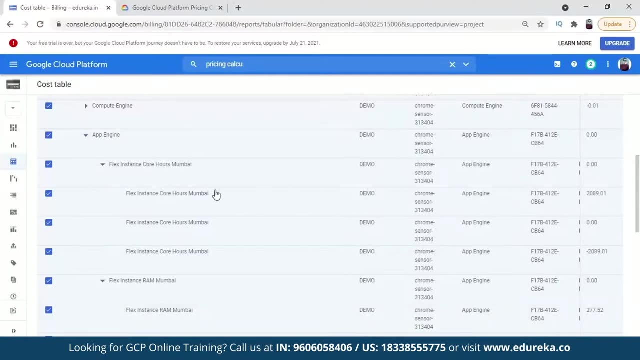 Just a second. What I can do is I can minimize it from here computing. So now there is App Engine. You can see similarly for the prices for it. The Flex instance score are from Mumbai, In Mumbai. I have launched it, so for Mumbai region. So it's costed 2089.. Flex instance RAM in Mumbai costed 277.. Similarly you can see it for Cloud SQL also. These are the prices And for those prices you can choose the like if you think it's really high. 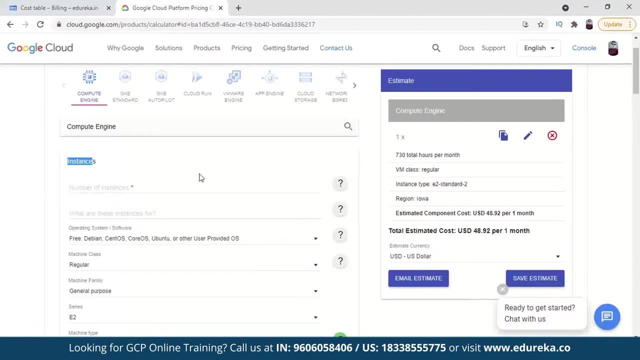 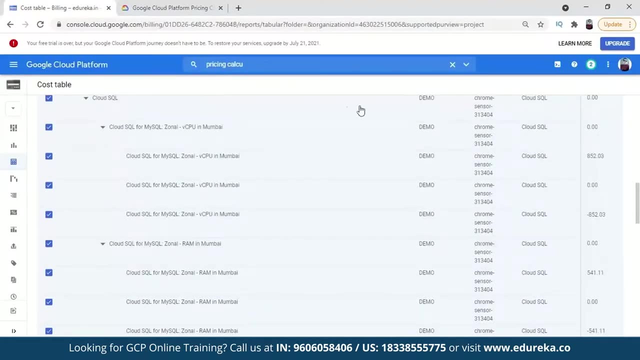 so you can check it for here, Like: what's the average price for the resource you are going to launch? okay, For whatever you are like using the resource you are using. So now you have understood, like, how it is costing And if it is not similar to the cost. 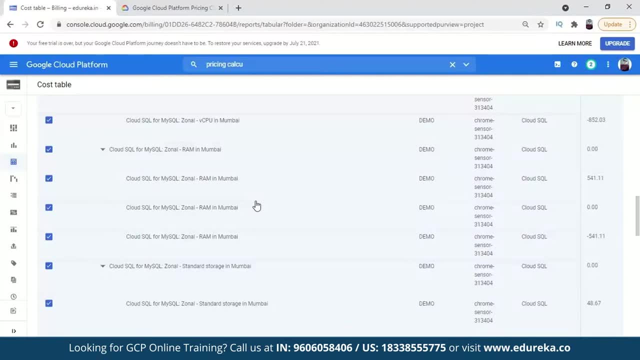 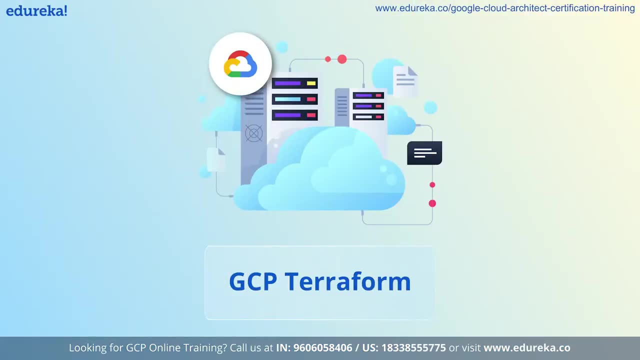 that has been showing in pricing calculator. then you can redefine it and make it more efficient by understanding the cost and everything. That's how the GCP billing prices works. Let us now see the reasons why one should consider Terraform. So Terraform lets you define infrastructure. 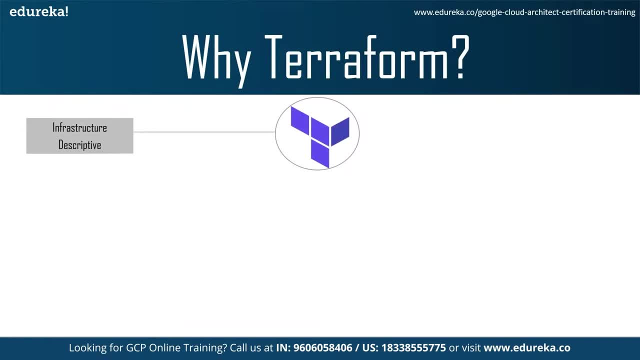 in configuration code and will enable you to rebuild and track changes to infrastructure with ease. So Terraform provides a high level description of infrastructure, which means it's infrastructure descriptive. Second, it has a lively community and it's open source. There is a massive community developing around this tool. 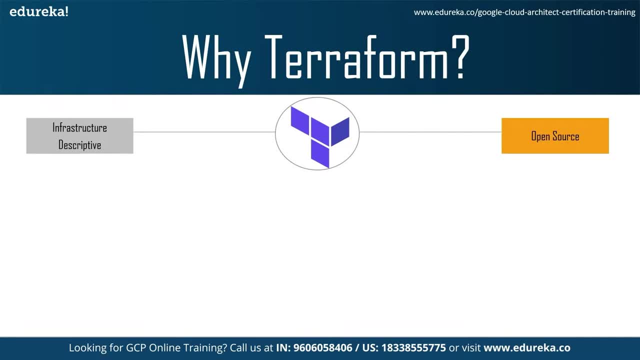 Many people are already using it and it's easier to find people who know how to use it, like plugins, extensions, professional support, et cetera. This also means Terraform is evolving at a much faster rate. They do releases very often. 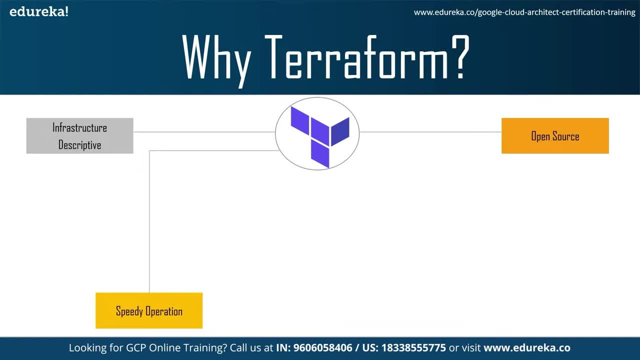 So third is like speedy operations. So Terraform's speedy operations are like exceptional. One cool thing about Terraform is its plan command lets you see what changes you are about to apply before you apply them. Code reuse features, and Terraform tends to make most changes. 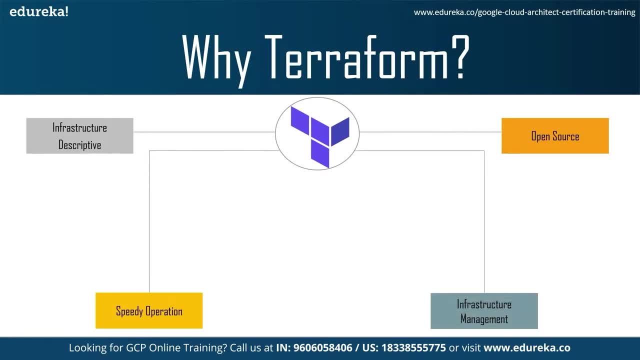 faster than similar tools like CloudFormation. Also, it is like the right tool for infrastructure management, as many other tools have a severe impedance mismatch from trying to wrangle an API design for configuring management to control an infrastructure environment. Instead, Terraform matches correctly. 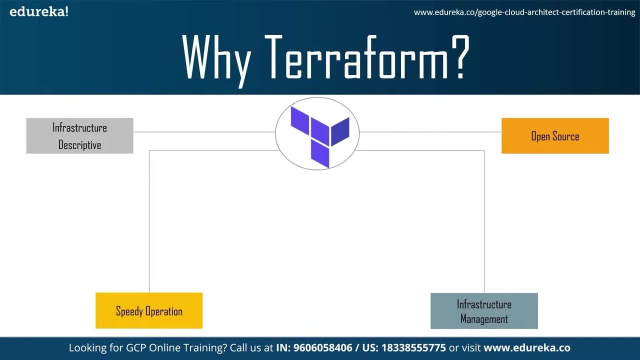 with what you want to do. the API aligns with the way you think about infrastructure. Also, like Terraform, is the only sophisticated tool that is completely platform agnostic as well as supports other services, while there are a few alternatives, but they are focused on a single cloud provider. 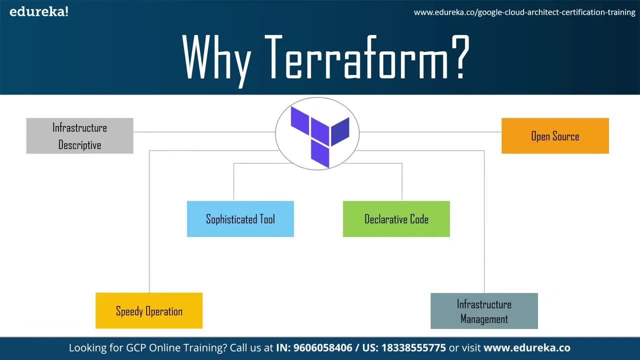 There's a declarative code, So Terraform enables you to implement all kinds of coding principles, like having your code in source control, the ability to write automated tests, et cetera. Now that we have understood why one must choose Terraform. 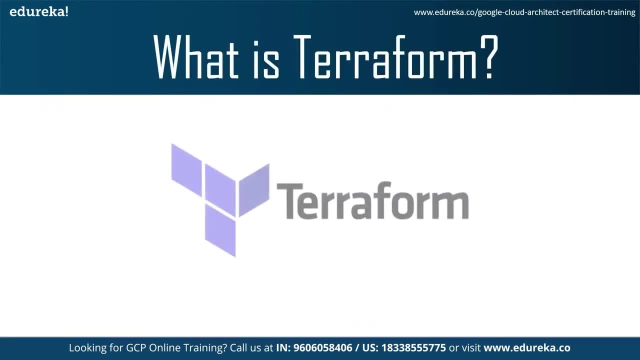 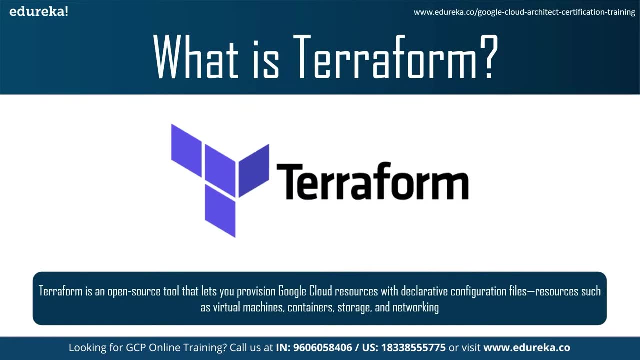 now let's briefly understand what Terraform actually is. Terraform is a configuration orchestration tool designed to provision the servers themselves. It refers to arrangement and coordination of automated tasks resulting in a consolidated process of workflow, So it is also in like open source tool. 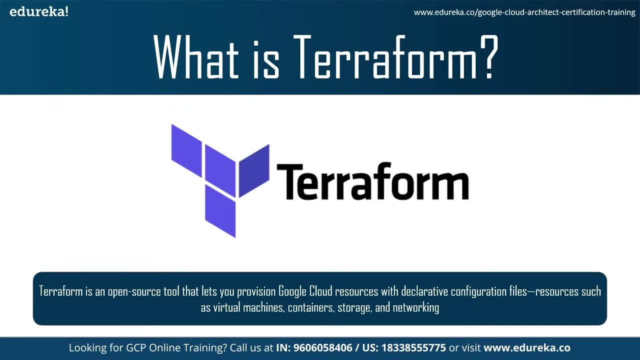 means open source software tool created by HashiCorp. So HashiCorp created Terraform to manage present as well as popular service, along with the custom in-house solutions. So Terraform lets you provision Google cloud resources with declarative configuration files, resources such as virtual machines, containers. 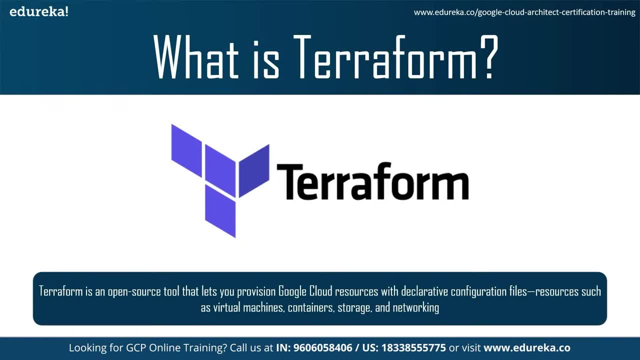 storage and networking. Terraform's infrastructure is a code that is an IAC approach. supports DevOps best practices for change management, which lets you manage Terraform configuration files in source control to maintain an ideal provisioning state for testing and production environments. 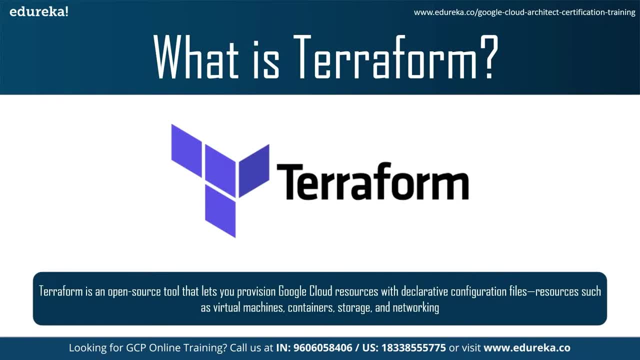 Terraform manages external resources with providers. external resources like public cloud infrastructure, private cloud infrastructure, network appliances, software as a service and platform as a service. HashiCorp maintains an extensive list of official providers and can also integrate with community developed providers. 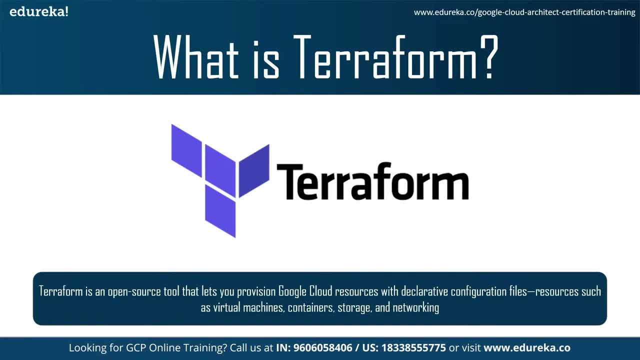 Users can interact with Terraform providers by declaring resources or by calling data sources, Rather than using imperative commands to provision resources. Terraform uses declarative configuration to describe the desired final state. Now let's look at some tools for using Terraform with Google Cloud. 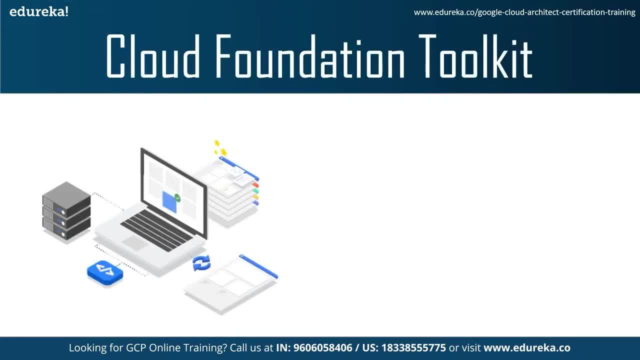 We will briefly understand these tools. So there are like variety of tools you can use to optimize your Terraform experience. So first let's explore the Cloud Foundation Toolkit, which provides a series of reference modules for Terraform. The modules reflect Google Cloud best practices. 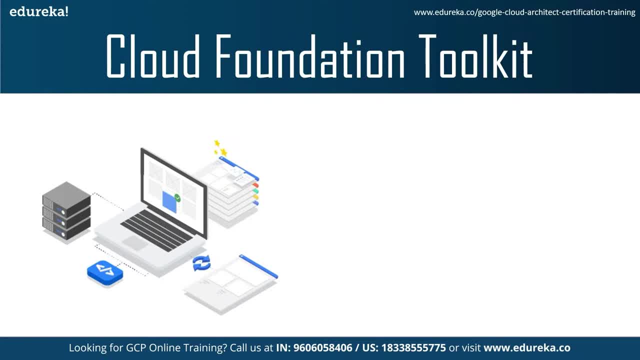 and using these modules help you get started with Terraform more quickly. The modules are documented in the Terraform registry and open sourced on GitHub. So these are some of the features of Cloud Foundation Toolkit. So first is ready-made templates. So the Cloud Foundation Toolkit provides a series 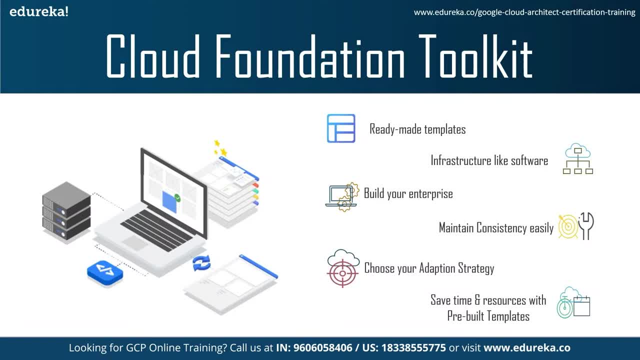 of reference templates for Deployment Manager and Terraform which reflect Google Cloud best practices. These templates can be used off the shelf to quickly build a repeatable enterprise ready foundation in Google Cloud. This frees you to focus on deploying your applications in this baseline secure environment. 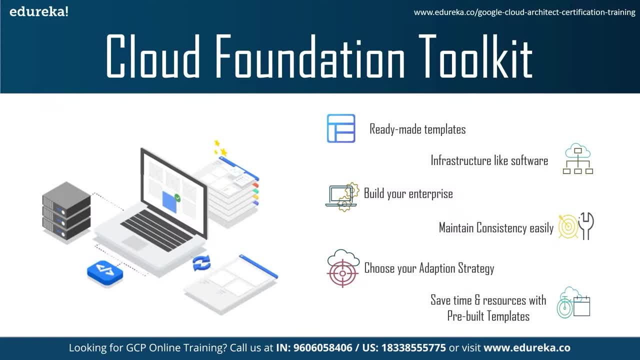 And with infrastructure as a code, you can easily update the foundation as your needs change. Second, like you can treat your infrastructure like software, So through the open source templates you can automate repeatable tasks and provision entire environments in a consistent fashion. 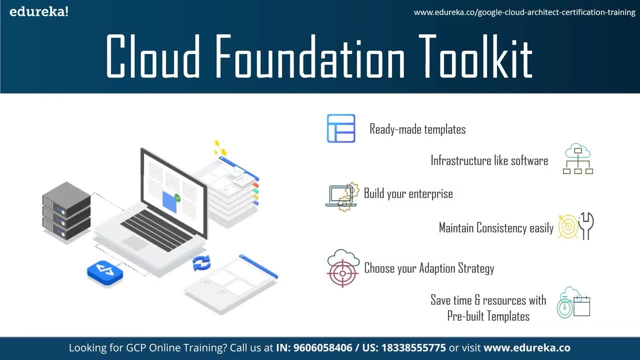 Plus, your teams can collaborate on the infrastructure by participating in code reviews and suggesting source code changes. Third, it's like a built for enterprise, So the Cloud Foundation Toolkit is designed especially to meet the compliance and security needs of enterprises By creating a foundational environment using these templates. 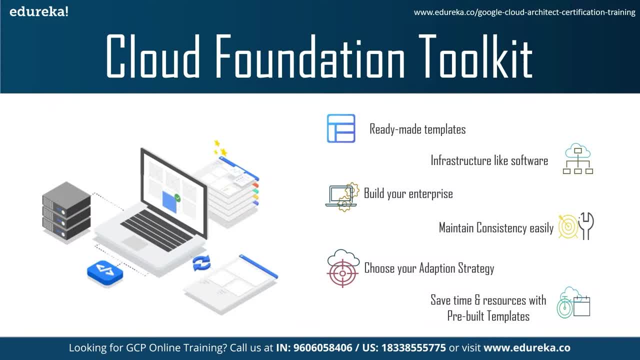 you can be confident that best practices are implemented out of the box, including key security and governance controls. Also, you can like maintain consistency easily by adopting the toolkit. you can be confident that different teams are deploying their applications and environments using a consistent set of tools and patterns. 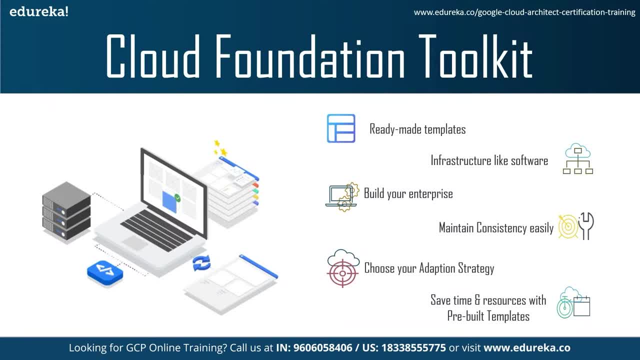 This reduces the potential for misconfigurations and inconsistencies, while allowing easier collaboration across different teams. Also, you can choose your adoption strategy. Each template from the Cloud Foundation Toolkit can be used independently. You can choose which patterns make sense for your organization and add new ones as your environment evolves. 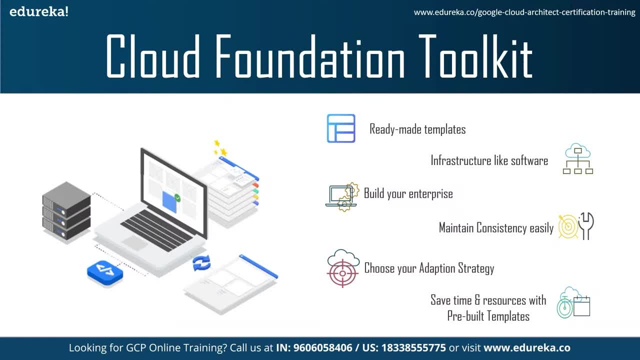 The open source templates can easily be forked and modified to suit your organization's needs. Lastly, you can save time and resources with prebuilt templates. With the Cloud Foundation Toolkit, you don't need to spend time developing your own templates and patterns for Google Cloud. 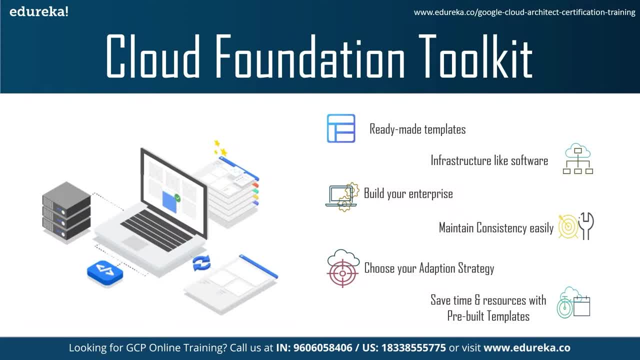 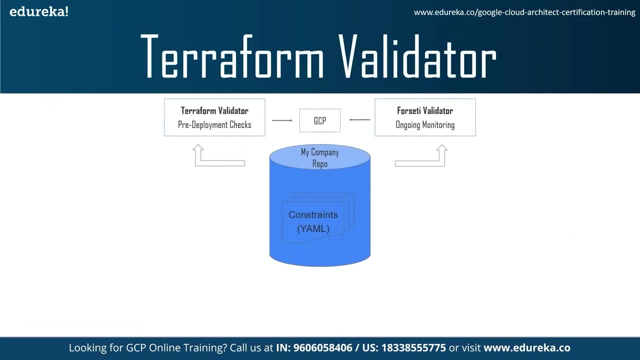 Instead, you can build an open source templates and focus only on the customizations which are required to your company and workloads. Developers can like, move faster and migrations are less time consuming because of it. So the second tool is Terraform Validator. So leverage Terraform Validator to enforce policies. 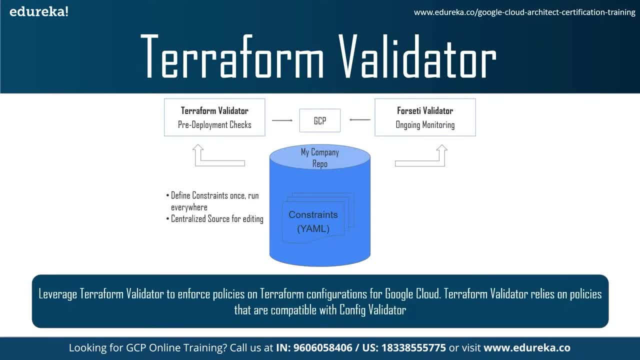 on Terraform configurations for Google Cloud. So Terraform Validator is a tool for validating compliance with organization policies prior to applying Terraform plan. It can be used either as a standalone tool or in conjugation with Forseti or other policy enforcement tooling. 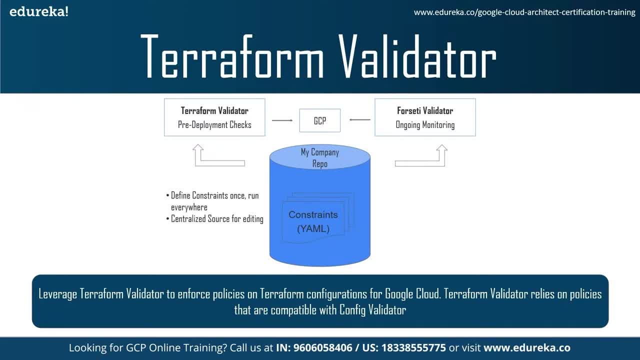 Terraform Validator relies on policies that are compatible with Config Validator. Note that using Terraform Validator does not require an active installation of Forseti. Terraform Validator is a self-contained binary, So you can see the Forseti Config Validator shown here. 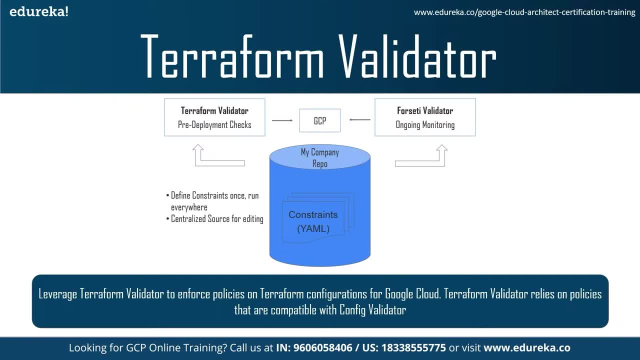 which is the newest addition to the Forseti Security Toolkit. So Config Validator helps Cloud Admins put guardrails in place to protect against misconfigurations in Google Cloud Platform environments. This allows developers to move quickly and give security and governance teams the ability. 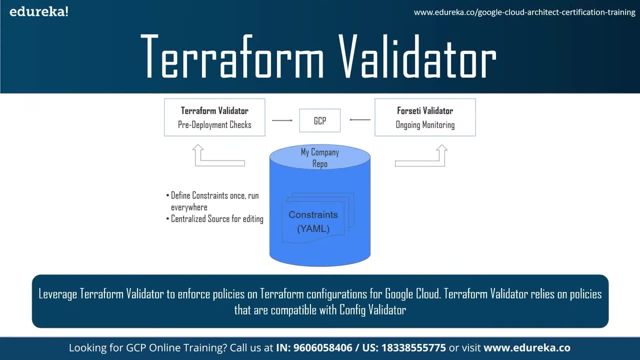 to enforce security at scale. So how does Terraform Validator works? So Cloud Admins write security and governance constraints as YML files once and store them within their company's dedicated Git repo as a central source of truth. Then Forseti ingests security and governance tools. 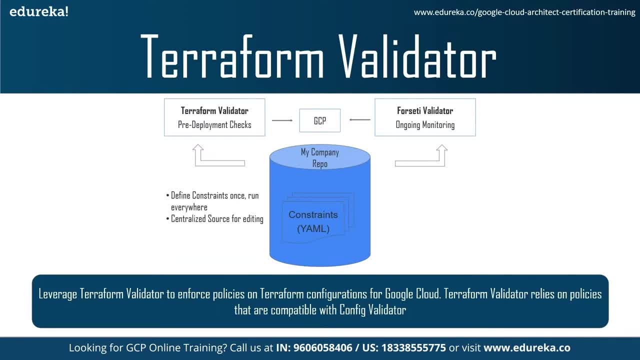 constraints and uses them as a new scanner to monitor for violations. Then Terraform Validator reads the same constraints to check for violations before provisioning, in order to help prevent misconfigurations from happening. That's how the whole process of Terraform Validator works. 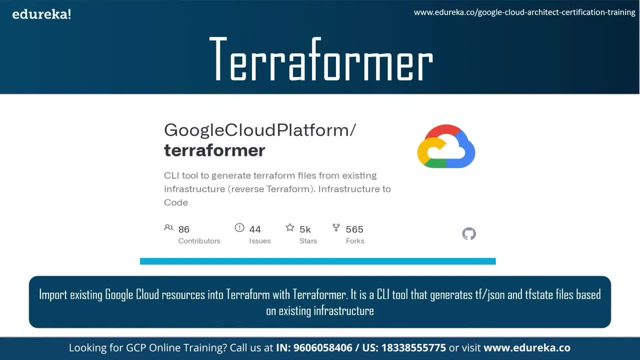 The next tool we have is Terraformer. So by importing existing Google Cloud resources into Terraform. with Terraformer, it is a command line interface tool that generates TF or JSON and TF state files. Terraform already has existing resources and it can be used to monitor violations. 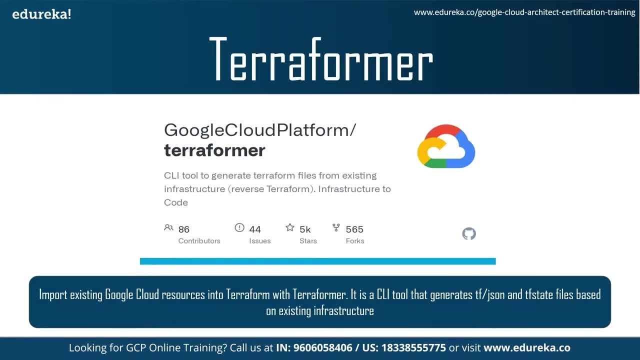 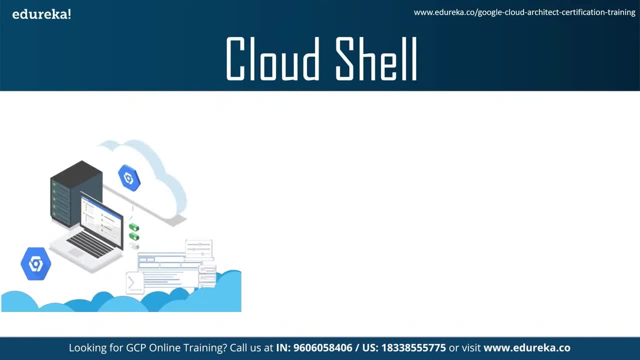 So, by importing existing resources in your environment, performing the reverse of what Terraform is designed to do, this tool can be thought of as infrastructure to code. Next, and the last tool is Cloud Shell, So Terraform is integrated with Cloud Shell. 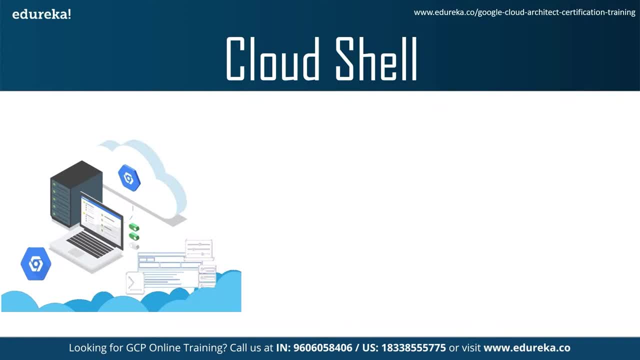 and Cloud Shell automatically authenticates Terraform, letting you get started with less setup. Using Cloud Shell, you can manage your infrastructure and develop your applications from any browser. Cloud Shell is an online development and operations environment accessible anywhere with your browser. You can manage your resources with its online terminal. 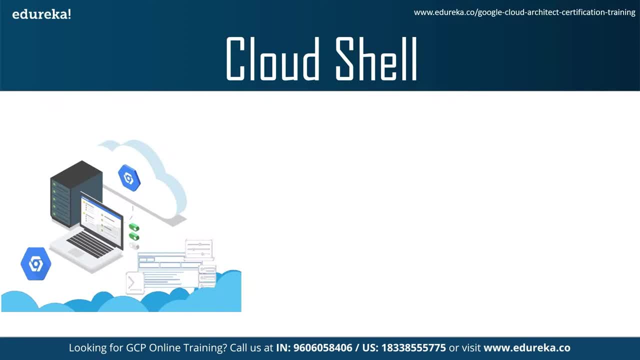 pre-loaded with utilities such as the gCloud command line tool. You can also develop, build, debug and deploy your cloud-based apps using the online Cloud Shell editor. So some of the features of Cloud Shell are like full power access from anywhere. 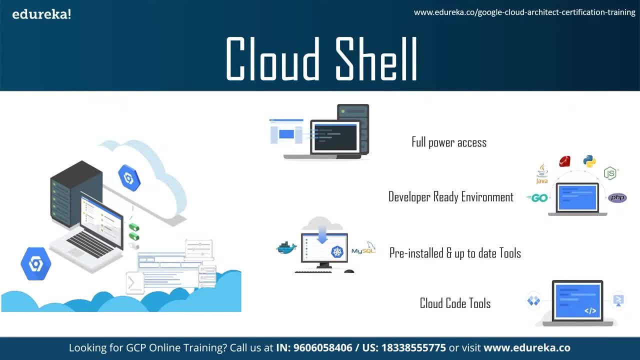 You can manage your Google Cloud resources with the flexibility of a Linux shell. Cloud Shell provides command line access to a virtual machine instance in a terminal window. Then it has a developer-ready environment so you can develop your apps directly from your browser. 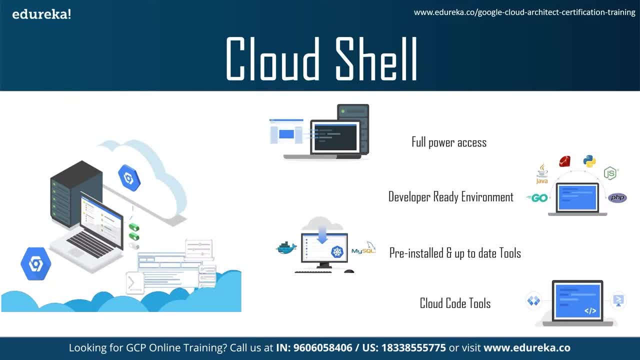 with a Cloud Shell editor streamlined to increase your productivity, with features such as Go, Java, Nodejs, Python and C language support, An integrated debugger, source control, refactoring and a customizable interface. Run your app on the Cloud Shell Virtual Machine. 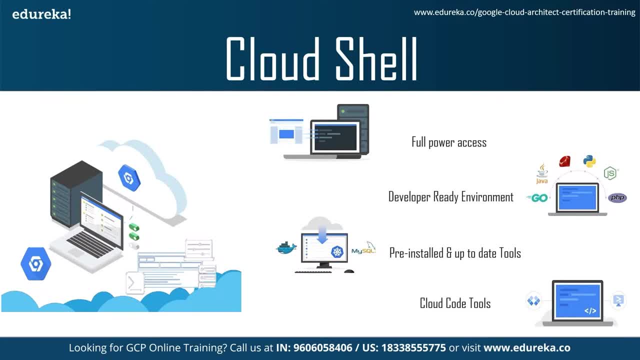 or in the Minikube Kubernetes emulator. review it directly in your browser. then commit changes back to your repo from your grid clients. Then the next feature is: like your favorite tools, pre-installed and up-to-date. So many of your favorite companies, like Microsoft. 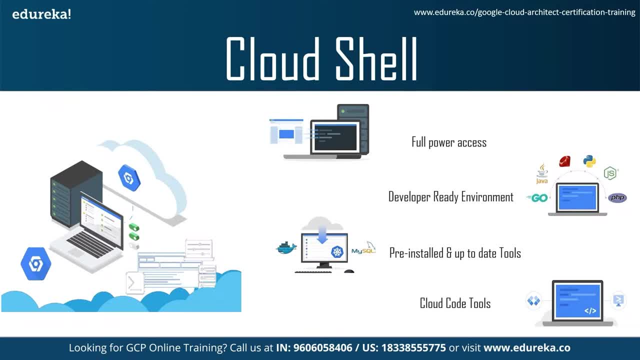 Command line tools, from Bash and SH to Emacs and Vim, are already pre-installed and kept up to date with Cloud Shell. Admin and development tools, such as command line tool, MySQL, Kubernetes, Docker, Minikube, are configured and ready to use. 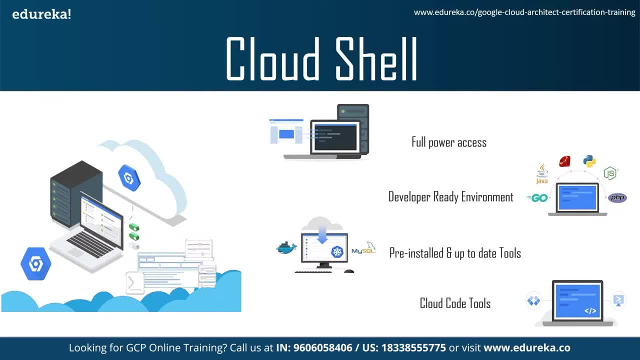 No more hunting around for how to install the latest version and all its dependencies. Just connect to Cloud Shell and go So. the last feature is a cloud port tools for maximizing development productivity. With this, you can easily develop cloud-based applications with the tools provided by our cloud code extensions. 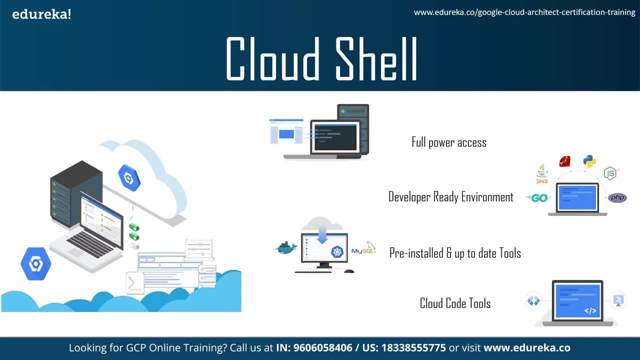 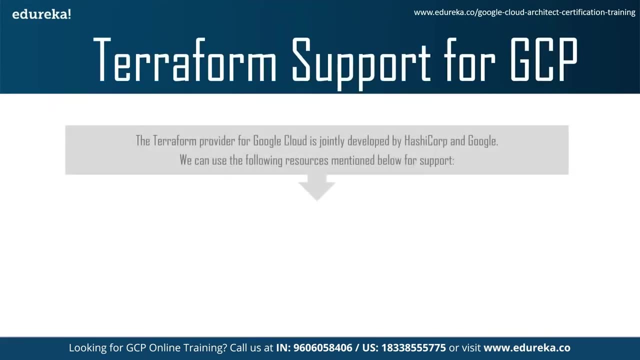 Allowing you to develop and deploy your Kubernetes and Cloud Run applications, manage your clusters and integrate Google Cloud APIs into your project, All directly from the Cloud Shell editor. So now let's understand the support that Terraform provides for GCP. The code Terraform command line interface is developed by HashiCorp. 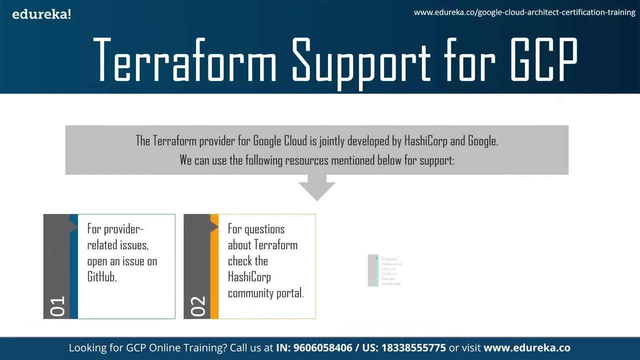 Use the following resources for support, Like for provider Related issues. open an issue on GitHub for questions about Terraform in general and common patterns. check the HashiCorp community portal for general troubleshooting advice. see Terraform's debugging documentation and joining the Google Cloud Community Slack Terraform channel. 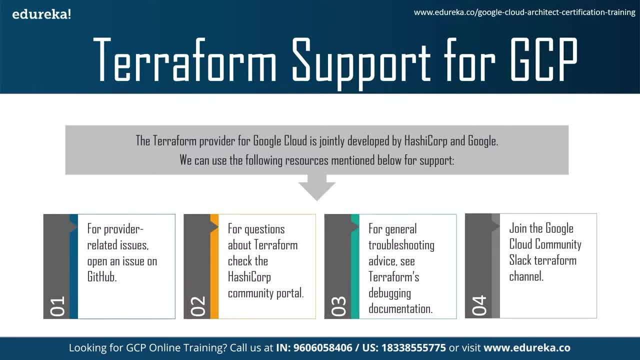 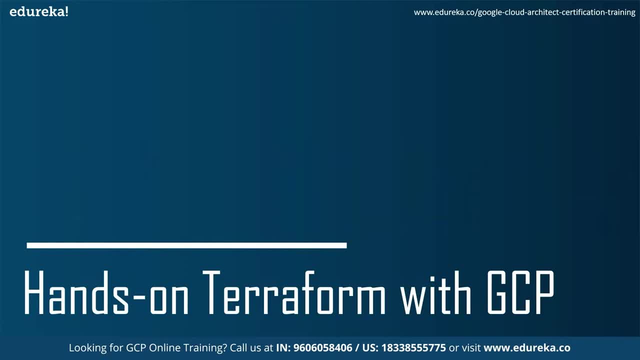 If you haven't already, you can like register for the Google Cloud Community Slack. Now that you have a theoretical understanding of Terraform with GCP, let's demonstrate it practically with an example of launching a virtual machine instance in GCP through Terraform. 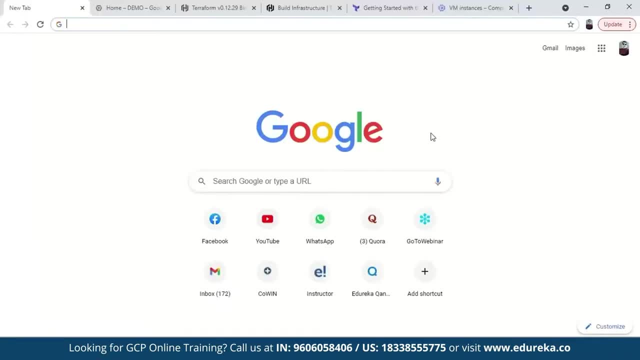 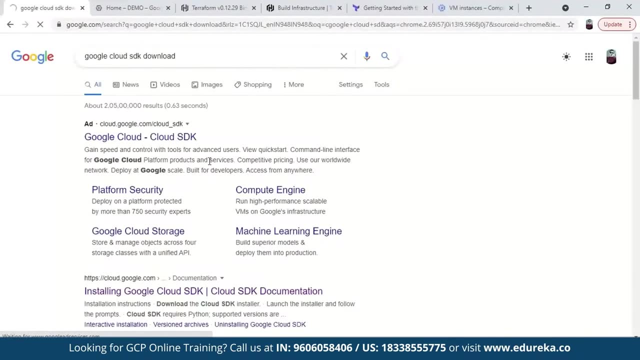 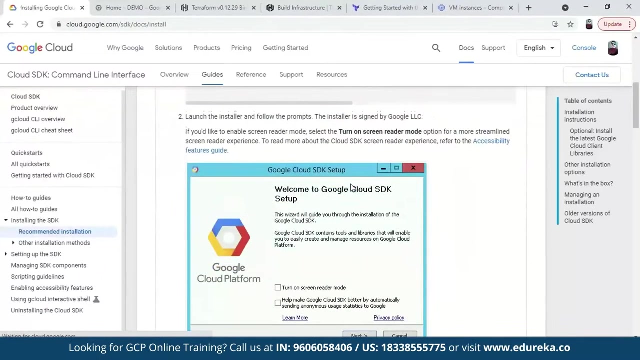 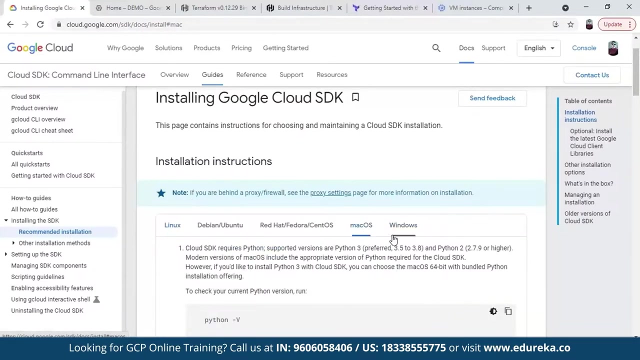 So let's start. So the first step is to download the Google Cloud SDK installer. So just search out Google Cloud SDK So you can just directly go to the install section here. Yeah, yeah. So yeah, here, like if you have a Linux OS, you can go to Linux and follow the steps to download, or you can go for Mac OS also, because I have Windows. 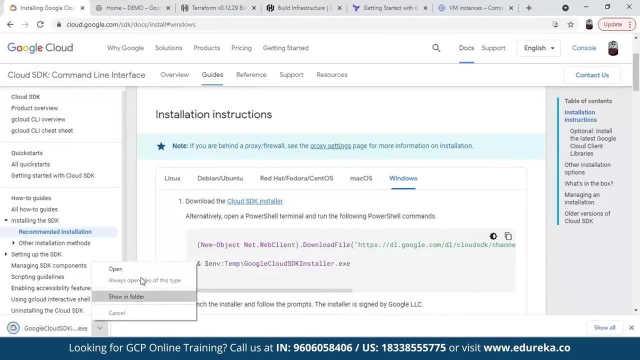 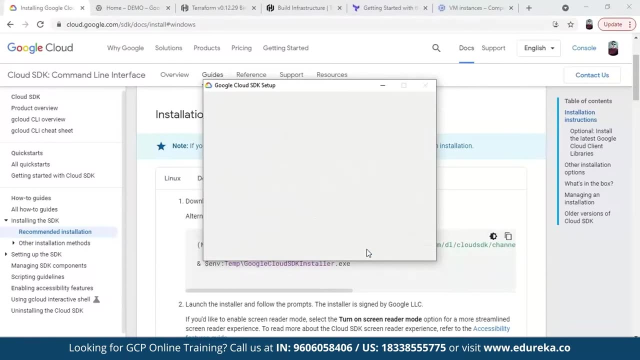 So I will start download directly from here. So I got it downloaded. Okay, Open takes a few seconds. Yeah, let's go next. next, next. So I already have a SDK installed so I don't have to continue. but if you don't have SDK installed, so to go, continue like get the installation complete. 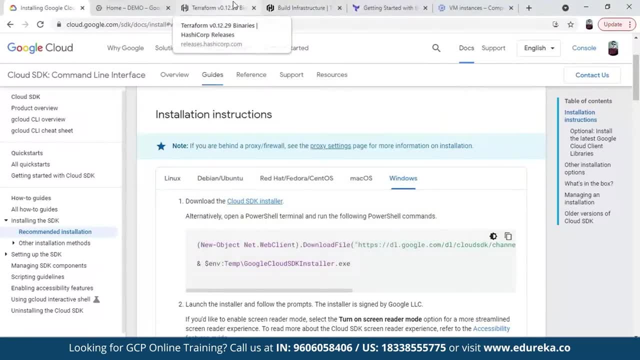 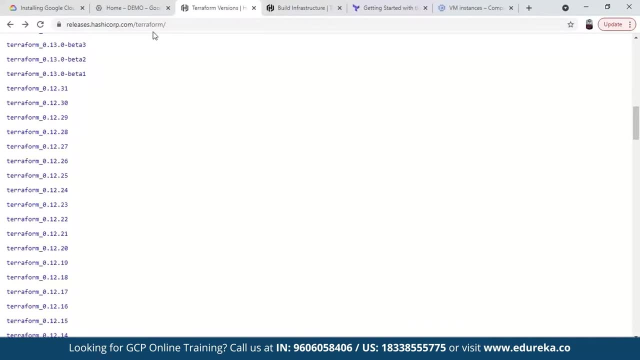 So yeah, the next step is to download your Terraform, So you can just directly go to releaseshashicorpcom slash Terraform. So HashiCorp, as I've told you, is the company that created Terraform. So from here, like all the versions are given. 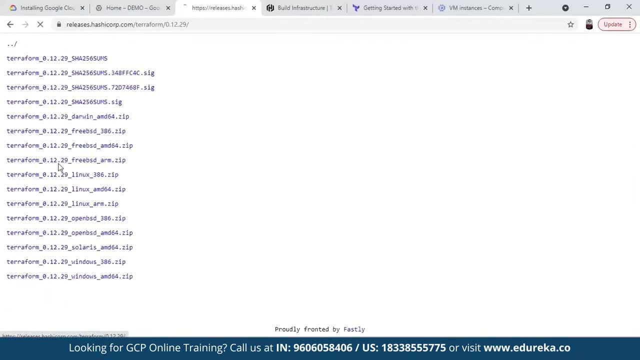 A lot of versions are there, so you can just go and download one. Yeah, If you have a Linux OS, you can just copy the address from here and unzip it. Okay, That's what you have to do. So if you're a Windows user, you can just download it from here. 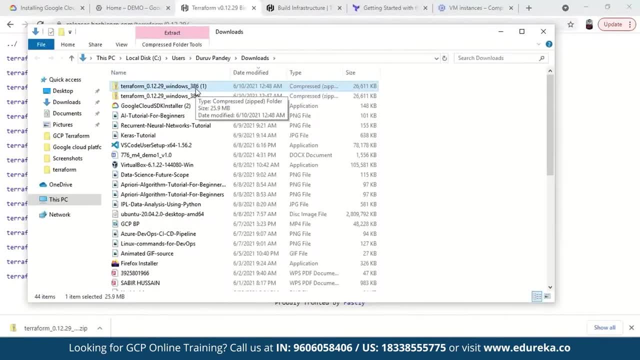 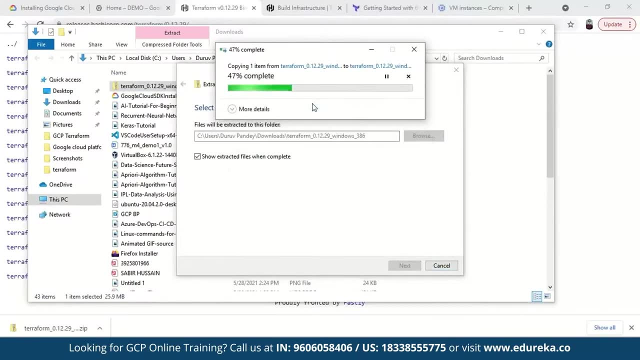 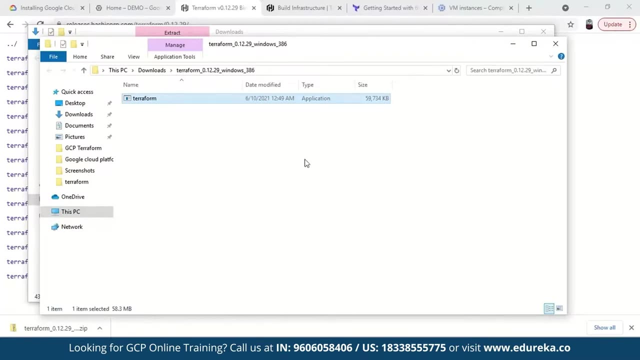 Yeah, It got downloaded. Download it twice So you can get this one. Yeah, So you can just extract it from here. Yeah, Yeah, Just copy it and paste it somewhere where you are going to like place other files, like separately. 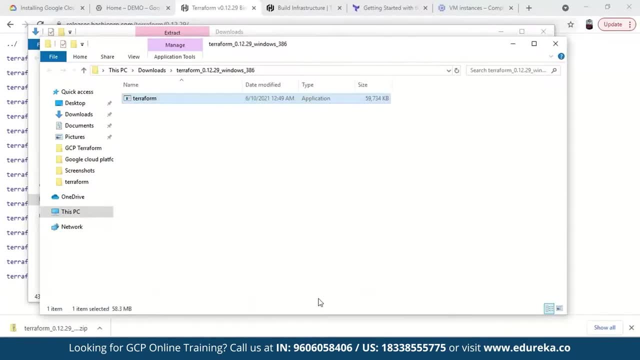 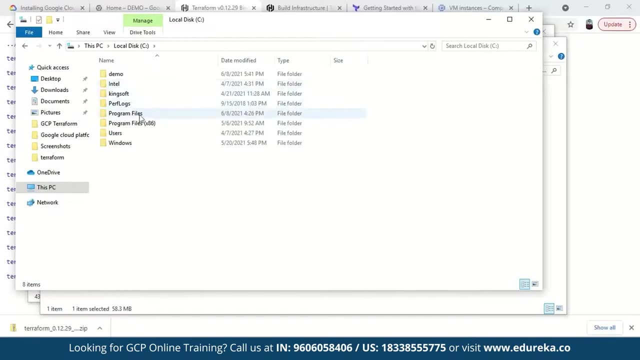 Like I have a different place to copy, So I will just go to my section. like not here, Just a second. Okay, I will just go to my place, Right, Because I am going to provide the path. also, I'll keep that in mind to place it separately. 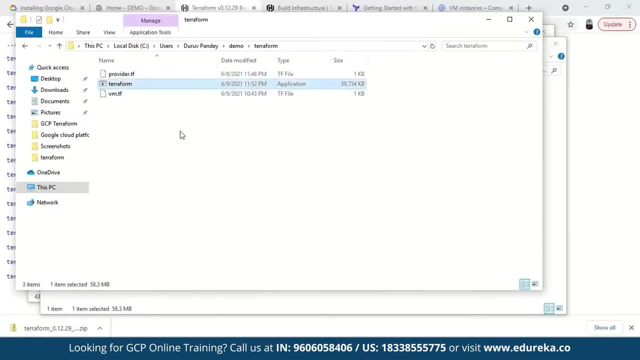 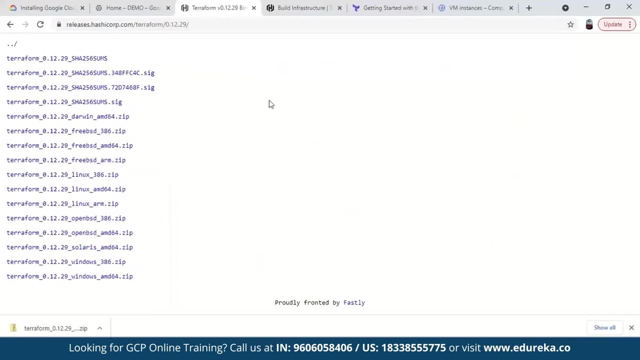 In demo section, the Terraform. Yeah, Like this one. I have got it before, So I will delete this one and I will paste the new one. Yeah, And I will name it as Terraform only. So the next step is to go to the build infrastructure. 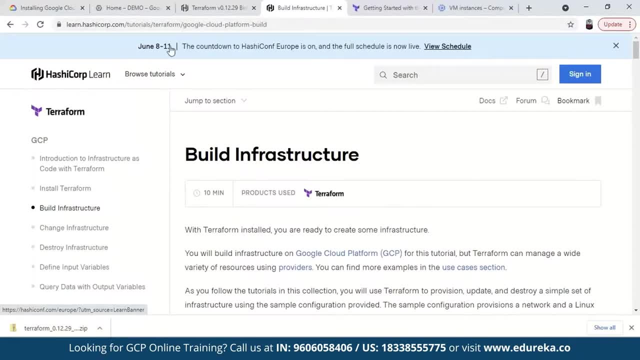 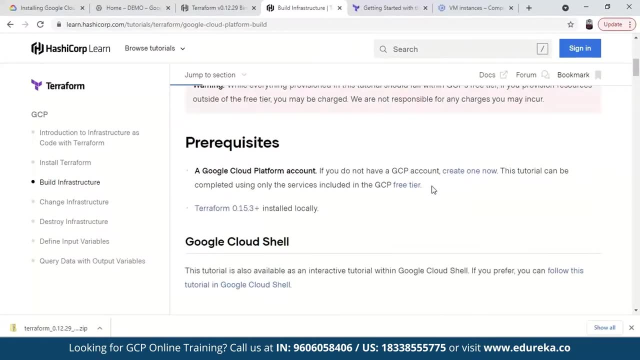 So here go to the HashiCorp website. From here you will go to the tutorial section of Google cloud. Okay, The prerequisites are given. Like you can create, you have to create the account on Google cloud platform. So if you don't have an account, create one. 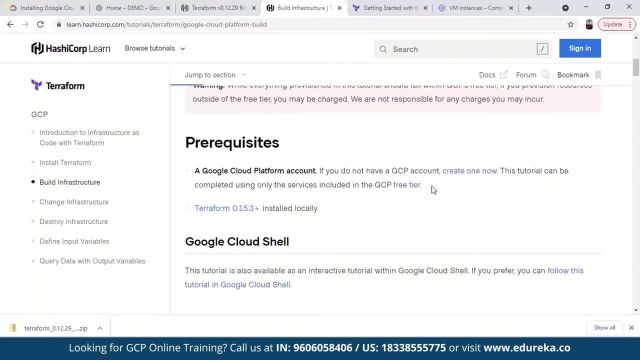 It's a like. it's a very good platform to have your account on and it provides a free trial Like. it's given the free trial. So free trial account is provided for 90 days with $300 credits And when you're going going to register it. 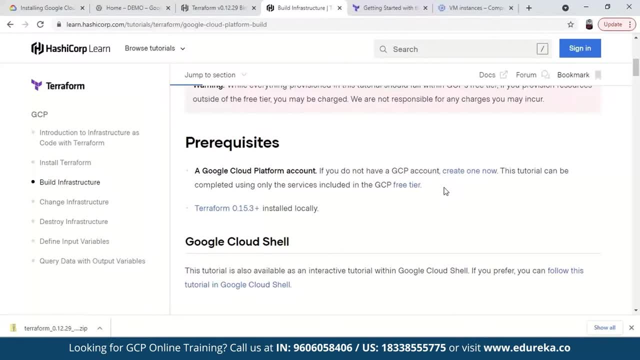 Plus for your debit or credit card details and it will just have it one rupee And it will also be refunded very soon. Also, like $300 credit is provided, So there is like a lot of credits, even means the exercise which I'm going to provide you. 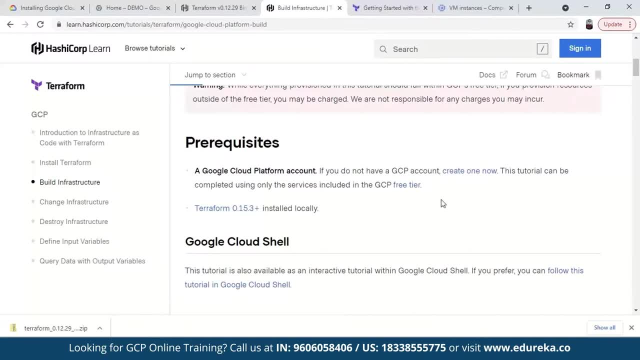 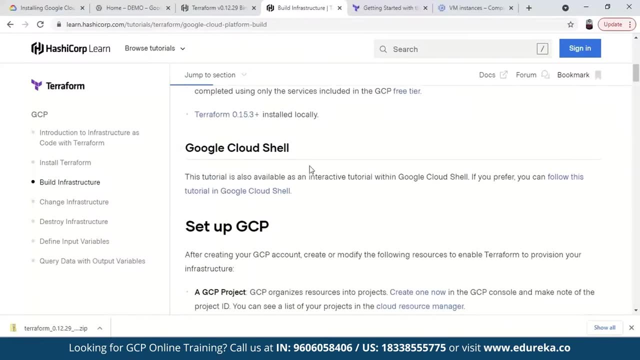 It's like it doesn't cost anything. It will only cut $15, $20,, not more than that, or maybe make some $50.. That's it, So that's how you can use it. So next, uh, I've already explained you how it works and what are its features. 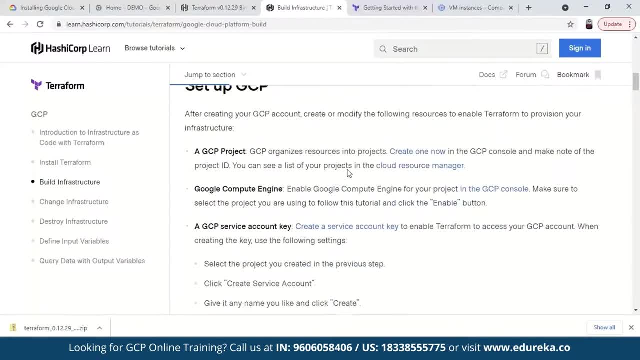 Then as a set of the GCP. So what do you have to do in the GCP? Yeah, You have to create a project, then you have to create a service account and you have to generate a key. Okay, So let's go to the GCP console. 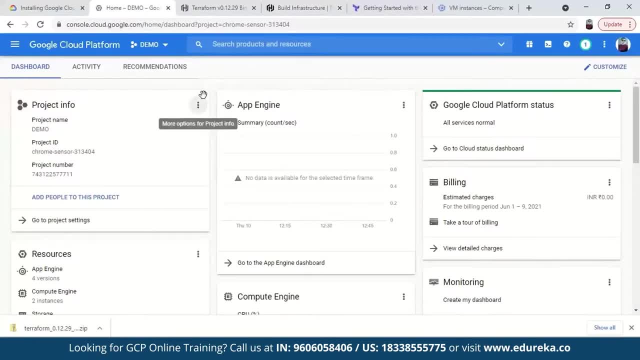 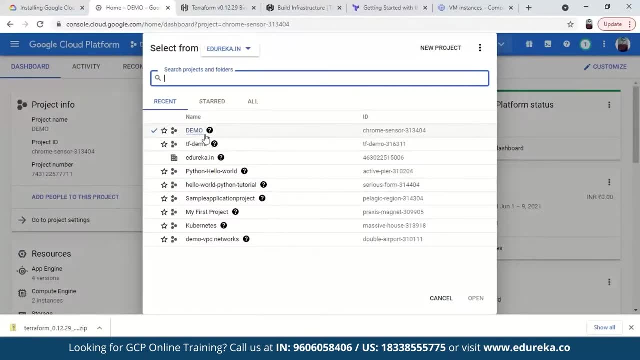 So this is how the GCP console, like Google cloud platforms console, looks like. Okay, From here, you go here and create a project, So you can create a project for me, but I already had like created the project. My project name is demo. 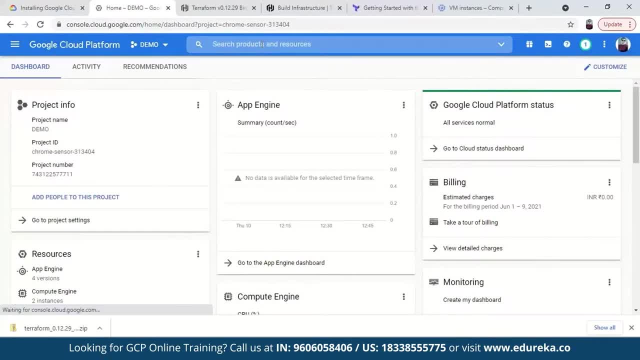 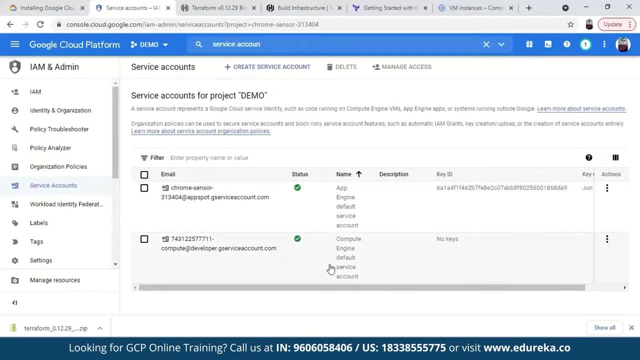 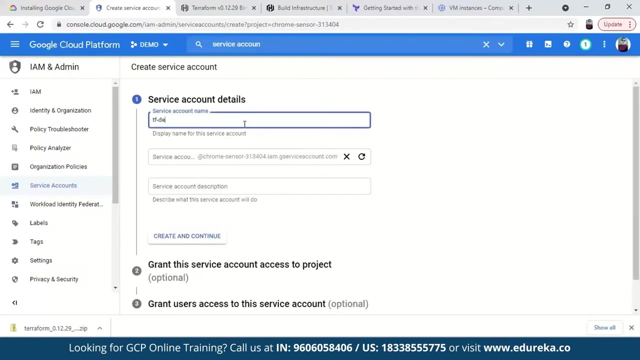 So I will use this project only. So now what I have to do is I have to make a service account. So I will type service account and, yeah, this is the default one and this is the one I have created recently, So I will create a new one with the name TF- demo service account. 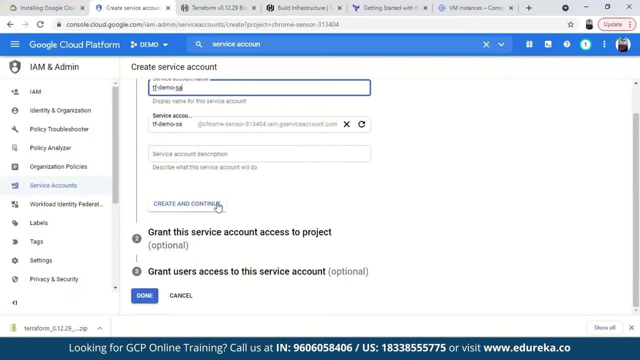 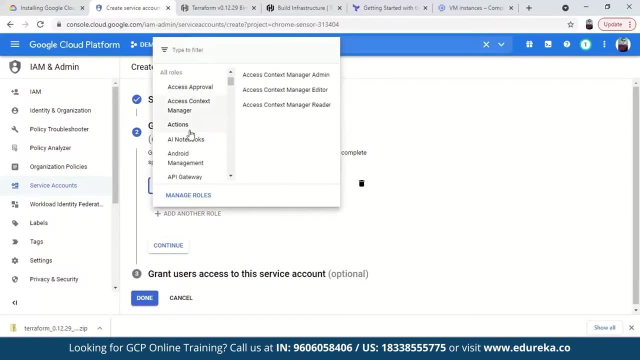 We're going to name it as S S A. Okay, So creating continue. now for access purpose, you have to do the role. So, like, different access options are provided for, like different services, Again, you can provide like for a specific service, you can provide the. 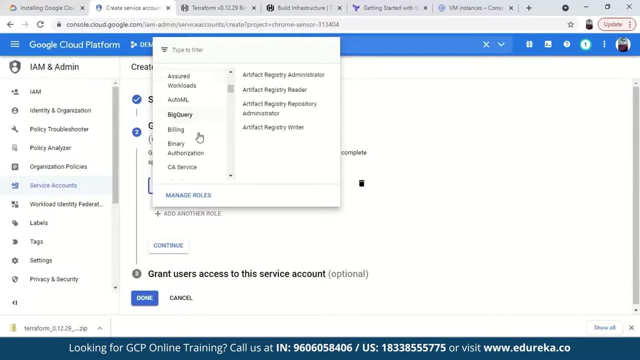 access like app engine or air notebooks and everything. auto ML, CSL with cloud asset, cloud data Labeling for specific service. whichever. whatever purpose you want to give, you can give it specifically for this service account. I want to complete access. 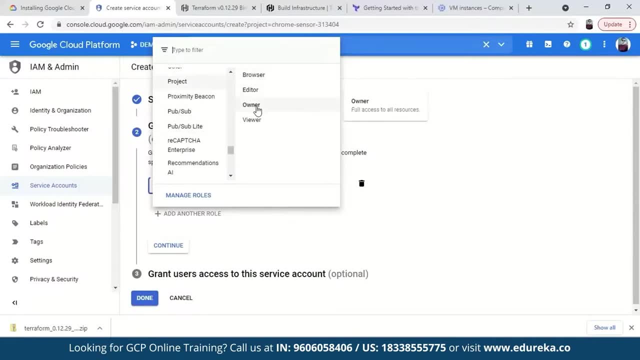 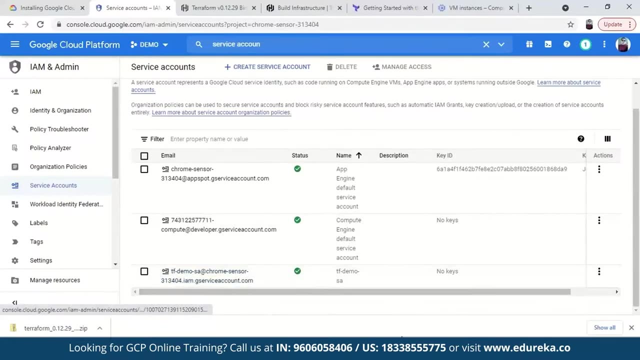 So I will just go to the project and in project I will give the owners to get the complete access. So yeah, continue that. So yeah, the service account is created for TF demo. I say okay for the next step, you can go to the registry. 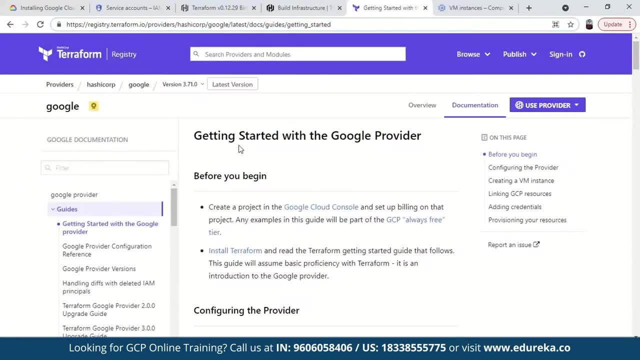 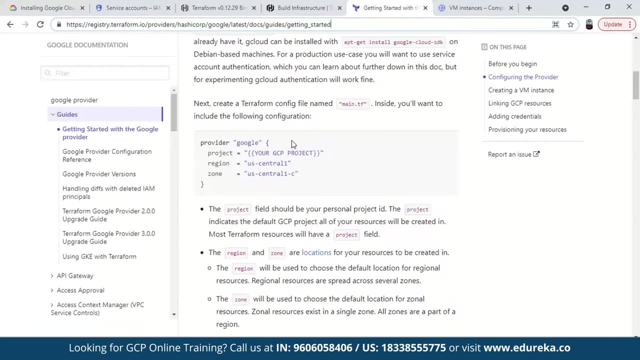 platform that I've already opened. Okay, In this way, you have to go to the getting started with cloud provider. You will get the code for here at the basic code, for What's the machine launching this simple, This one? I think it's a basic code of a Terraform. 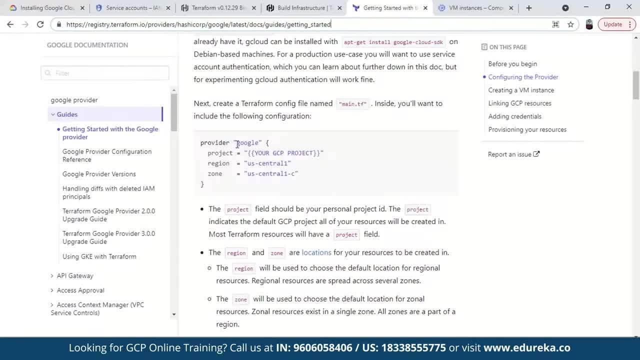 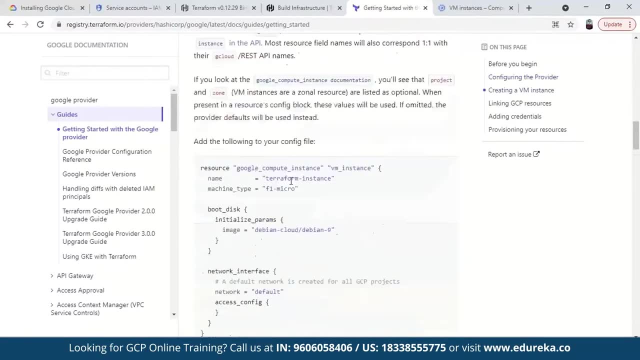 Okay, So if you're going to use AWS now, so in AWS you will just use instead of Google you will use. all the things will be same And similarly, the provider code is provided below, So just copy this code also and make a provider file. 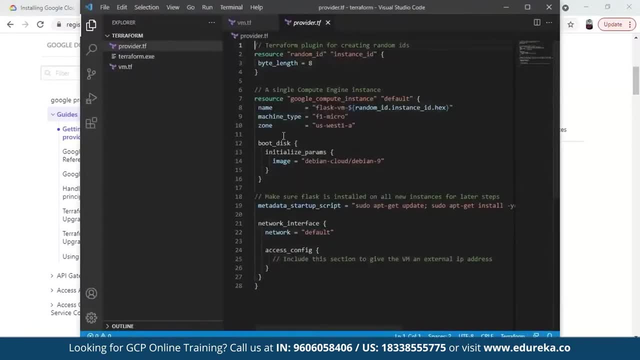 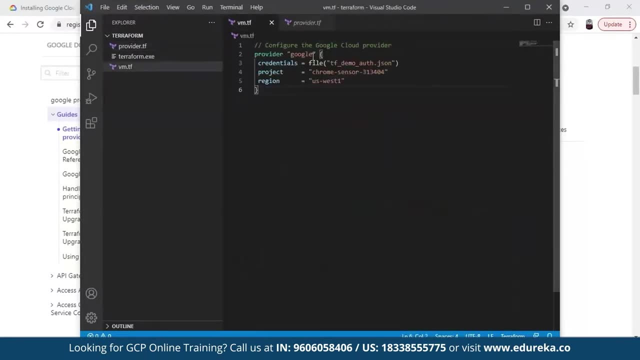 And for this creative VM file, like I have created one, So this is how I have copied it here. Like this is the VM, the basic codes and then the provider code is provided here. So you can see in VM like the credentials are given: project and. 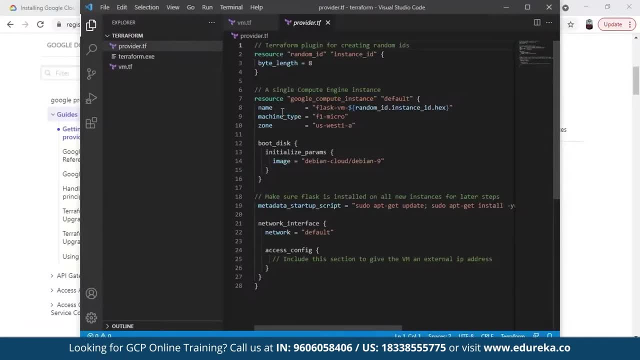 then region is given everything And similarly, like the provider, in this, the name, like with the virtual machine instance that will be created now that will be named by flask VM and whatever the ID it will be there. So in that name the virtual machine will be created. 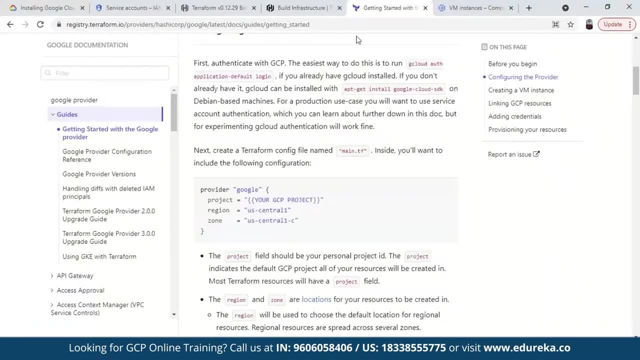 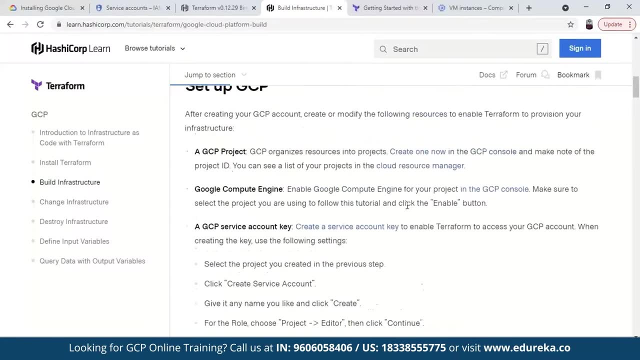 Similarly, machine type is given and zone is given. also one more thing. So I have to generate a key in this, like this I have created. now I have to generate the key I have, like I remember I told you in this, like the third step is: 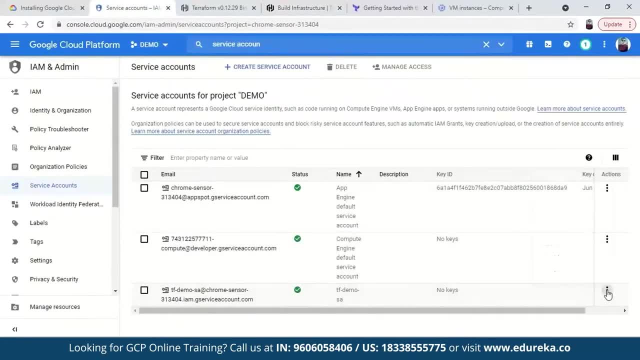 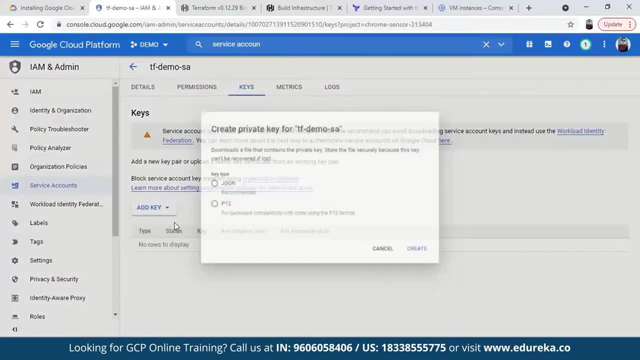 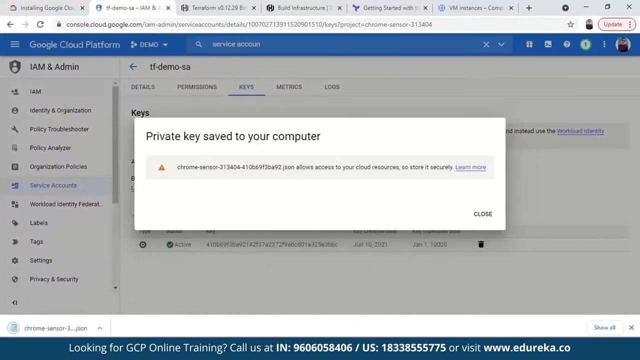 to create a service account key. So In go here like the service account we have created, in that we have to create a key. so manage keys and add a key, create new. So in, Jason, failure will be created from here. So, yeah, got created. 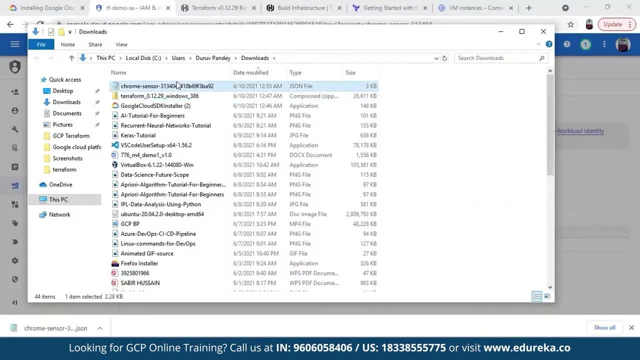 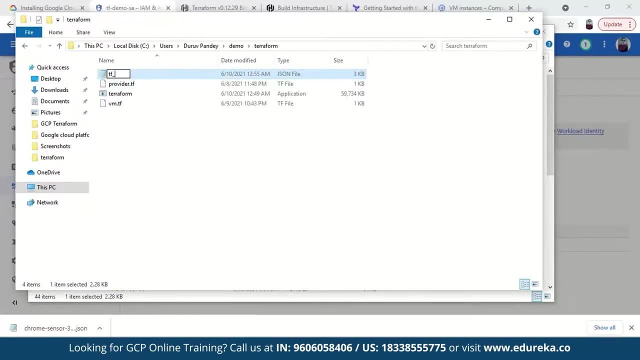 So we can just go to downloads. Yeah, So it is here. So we can just copy here and you will just paste it to where we have on the platform files and name it as a tier. underscore. position, underscore: Okay, Yeah, That's good. 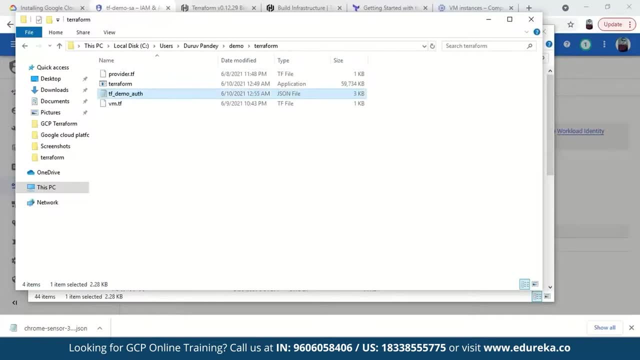 And that's good authorization. This is what I named in the code. Also, there's time naming this. So yeah, even just put them on the spot, or Jason, So that's what it is Same. So coming back. So yeah, all the quotes and everything is done. 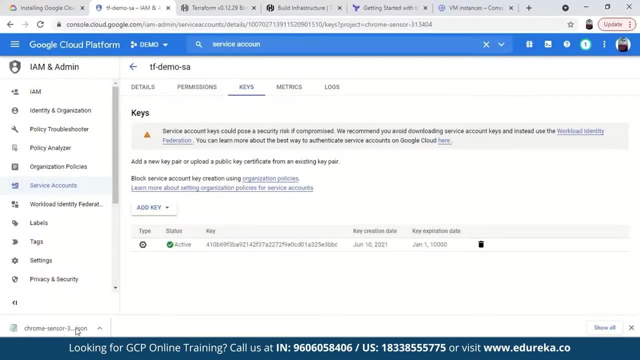 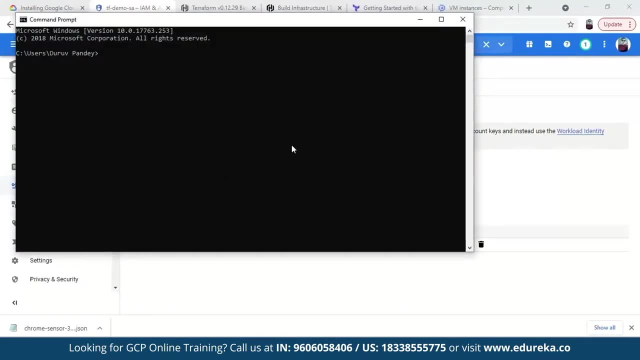 So now what we have to do is take that. So it's, the key is active. Now you can see. So what we have to do is now open the command prompt. You just have to provide the path first. So the path is a CD. 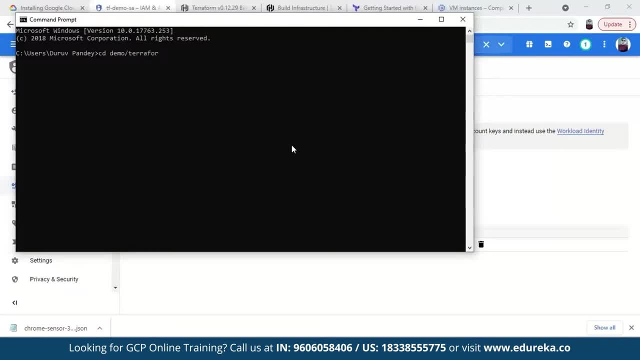 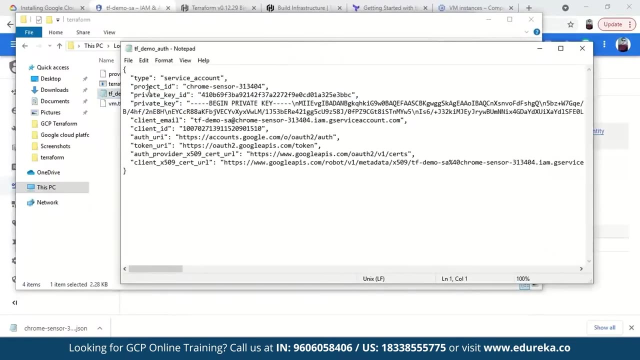 Demo slash telecom. So yeah, the path is here. Then we have to revoke the authorization. So G cloud authorization: purpose for G cloud authorization. revoke One more thing. I will show you the Jason file. If you see, everything is given like privately for project ideas. 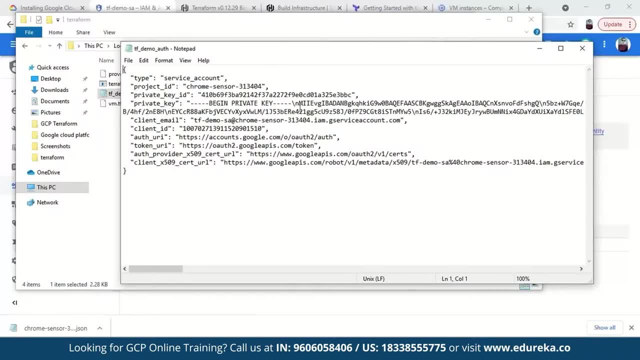 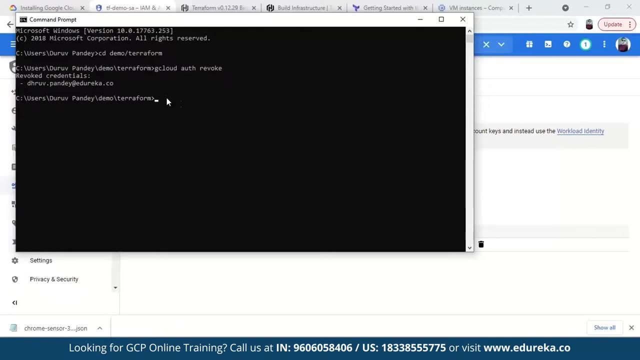 game. private EID is also given from the name that virtual machine will be launched. Now the key will begin. this blast ID in the key and private keys given in client email. Client ID authorization token. Everything is given this. Okay, So we've got this. authorization to book. credentials are here. 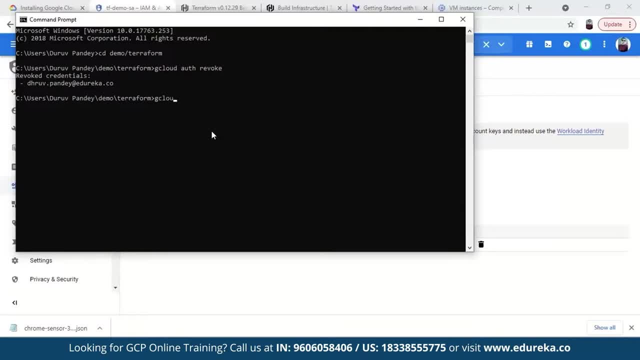 So after that we have to configure So G cloud config configurations list. So yeah, though, everything is right in my account, but if you want to change, so what you can do is you can initialize this. So let's clear this one. 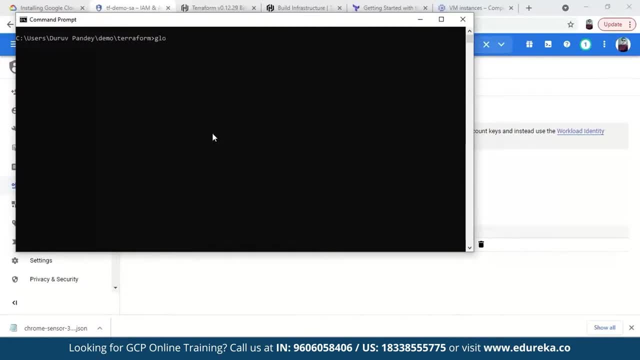 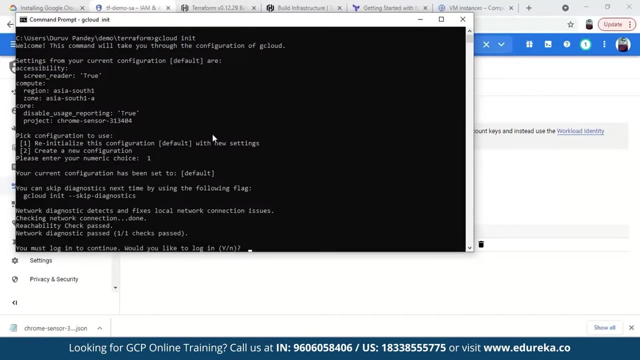 So you can initialize it for changing Anything in your configuration list. Okay, So G cloud. Oh, sorry, She cloud. initialize I N I T. So yeah, for initialize. give the one choice. It's been done Then. would you like to log in? 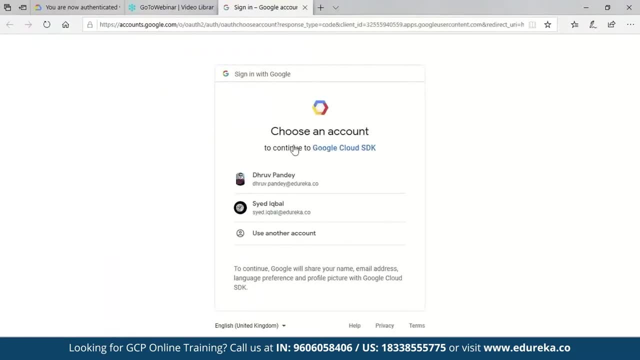 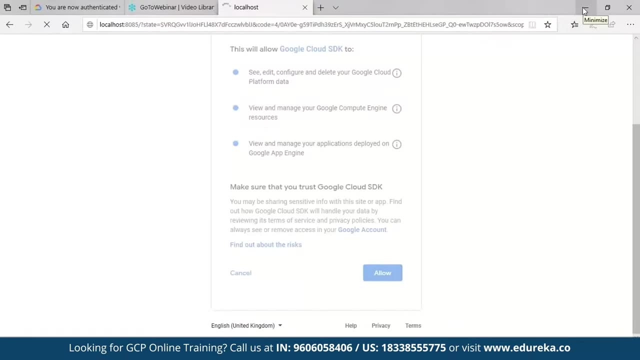 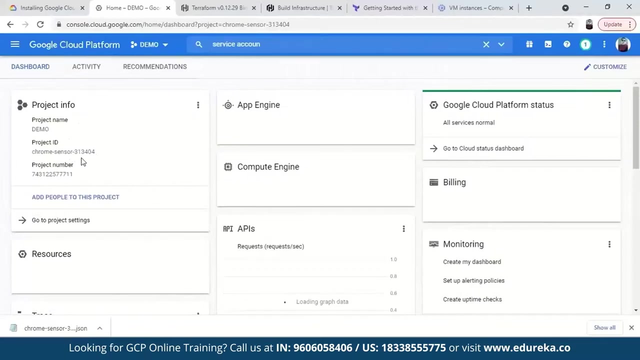 Yes, I want to log in. Just have to log in from authenticated to be done now. So in this comeback you can choose The project from here. So your project name is, if you remember it's, Chrome sensor 3, 1,, 3, 4, 0, 4.. 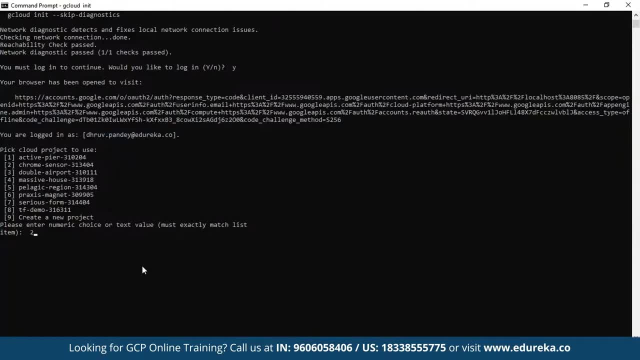 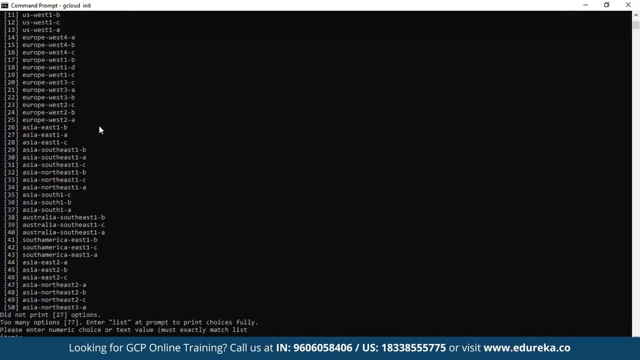 Okay, So there's Chrome sensor, So it's second, And I think then the zone and region we have to select. So, yeah, we want to select. So my region is South Asia. Yeah, So I will select 37: South Asia. 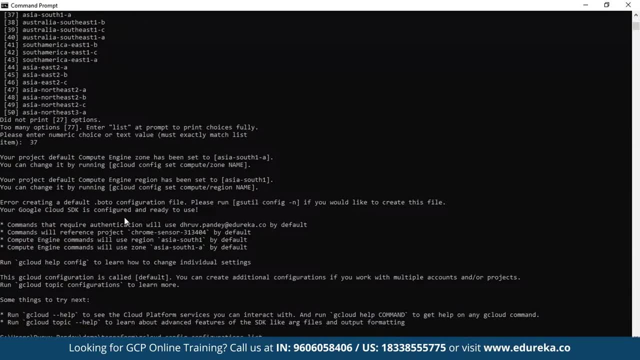 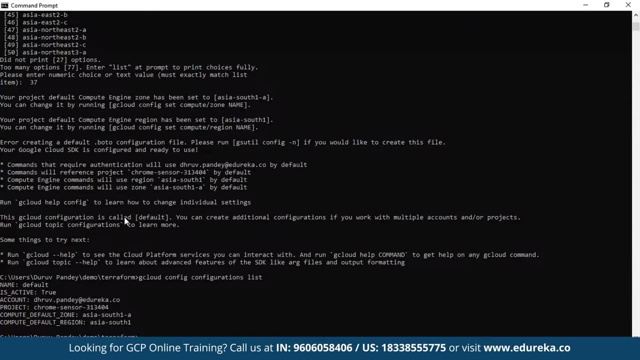 So, yeah, everything is done now, So we can just again configure now. So, yeah, everything is at place, Account: Yeah. So last time, if you see, like I was saying like everything is there, but last time also, 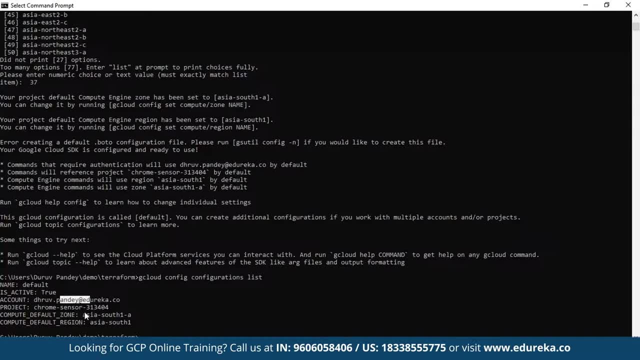 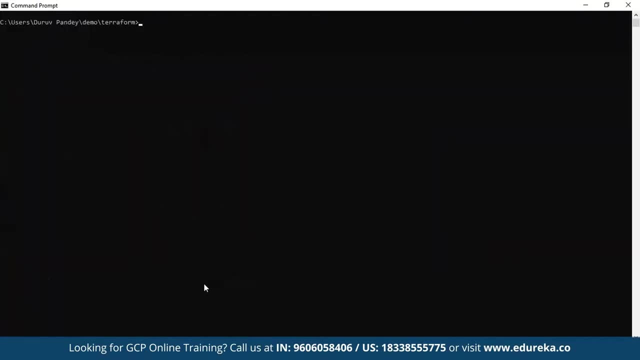 like everything wasn't right because in the place of the account, my account wasn't selected, So it wouldn't have worked. Do check it properly. Then let's clear this. Then let's start with the telecom initialization. There's a form in it. 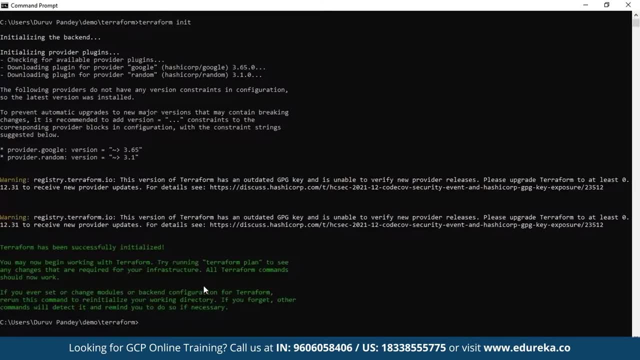 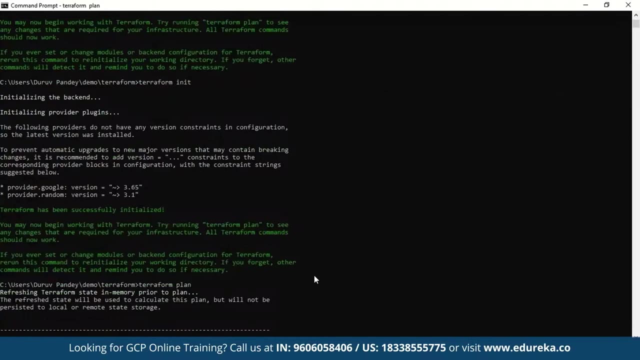 We have to go with. I think it's getting initializing. So yeah, it's got initializing it with plan. So the phone. sorry, you can't stop Please. I have already initialized that, Sorry. So telephone plan now. So yeah, 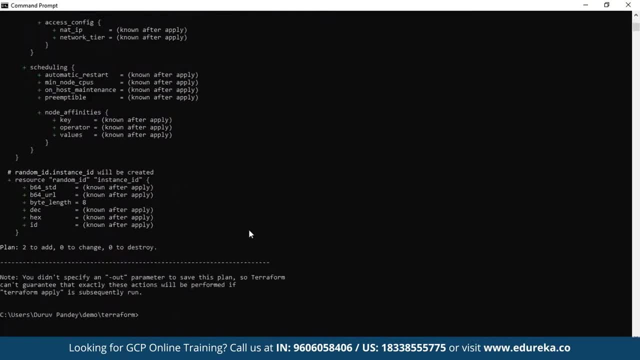 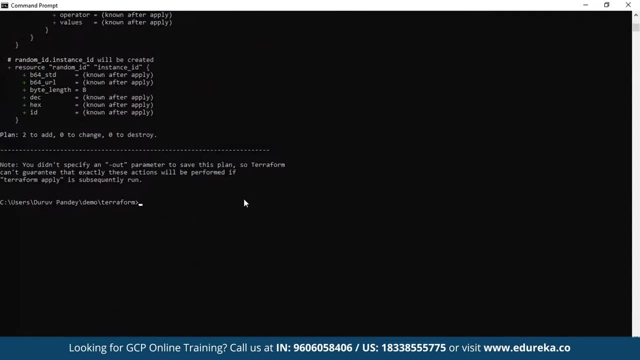 So it will be like the create, So if you got done but you can go, so you can see, like full compute instance will be created now, Okay, So what we have to do is we just have to apply. So the command is telephone apply. 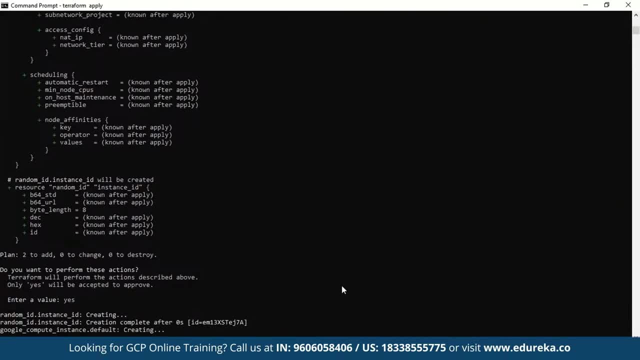 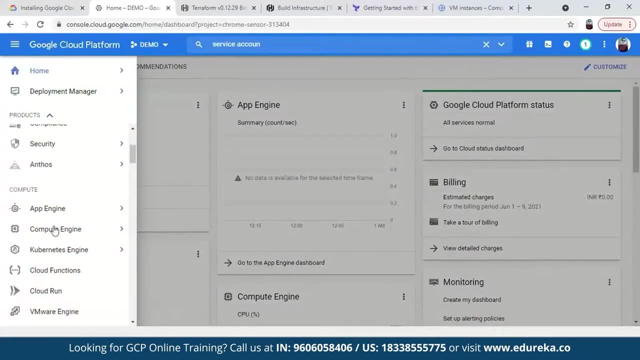 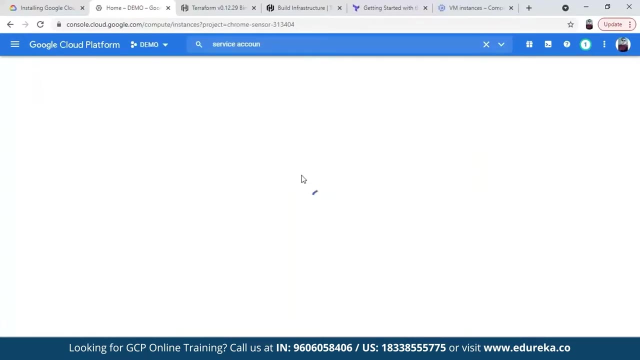 Only yes will be accepted. So, yeah, Yes, Yeah, So it's got. So let's check. let's go to the virtual machine instance, your engine, virtual machine instances. the flask will be created with the name flask or some ID will be given again flask, VM ID- something I hope it get created will be created because it's showing. 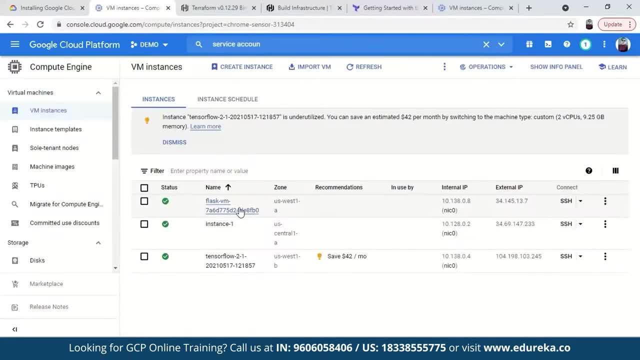 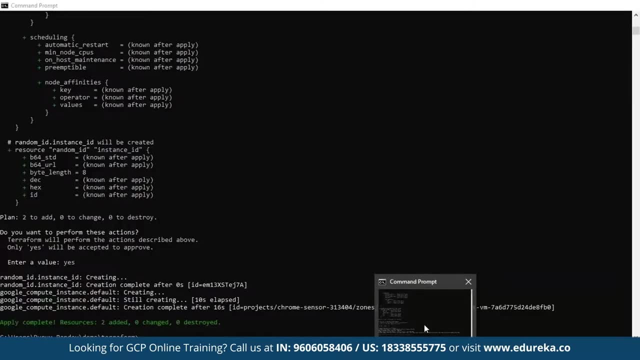 So cause it got created: Yeah, Last VM in the private hacky. So, yeah, that's how it got created. And if you want to delete it and just to get the command of destroy, Okay, So you can just come here. 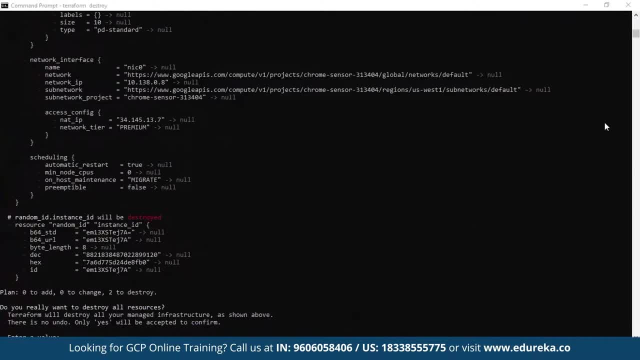 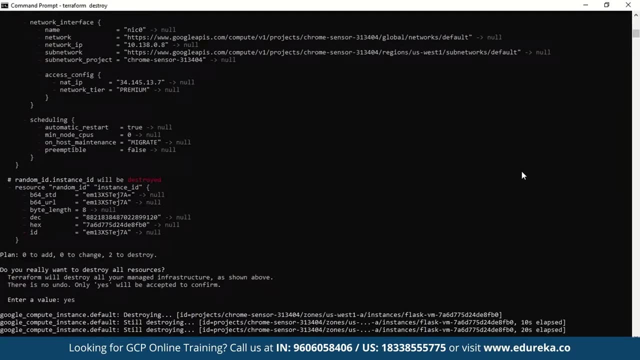 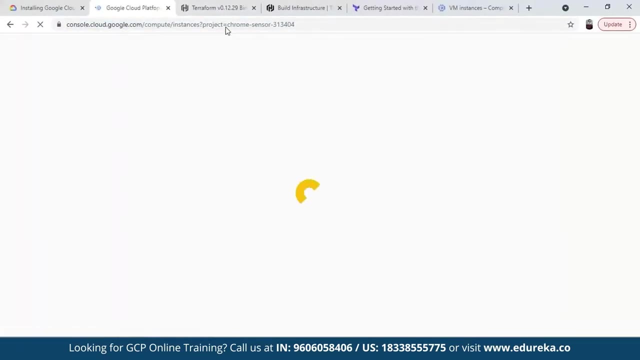 You can give. You can give the command of destroy. Only yes is accepted. So yes, it takes a few seconds. So yeah, So it got destroyed. Let's check Now. it is here, So we will just refresh it. We'll find that it will get deleted from here. 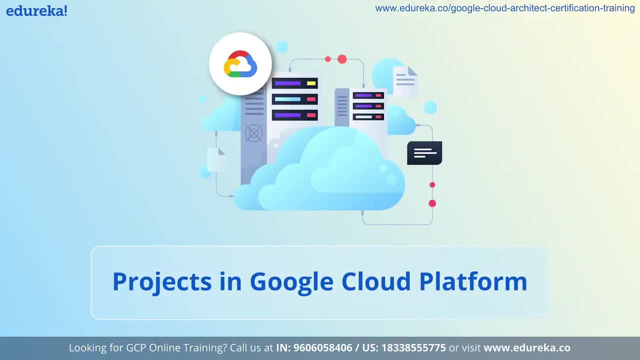 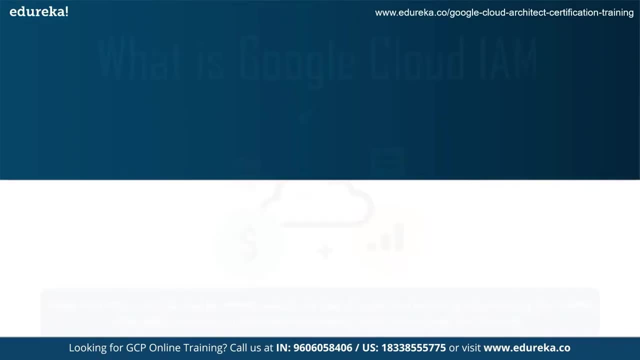 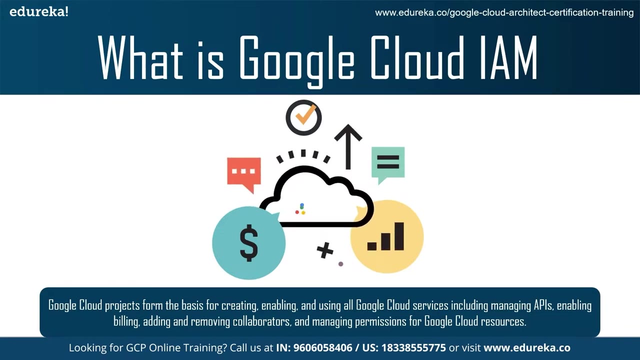 Yeah, So it got deleted. What is a project in Google cloud? A project consists of a set of users, a set of API's and billing, authentication and monitoring settings for those API's, like, for example, all of your cloud storage buckets and objects, along with user permissions for accessing them, reside in a project. 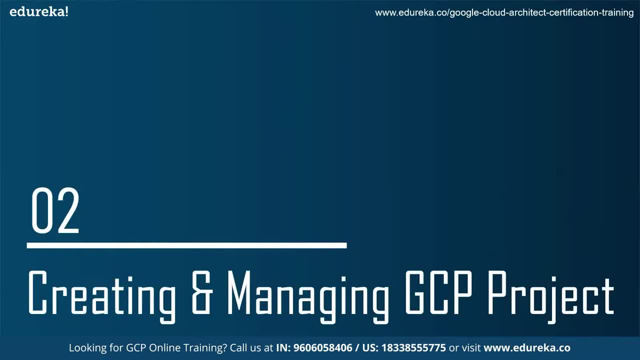 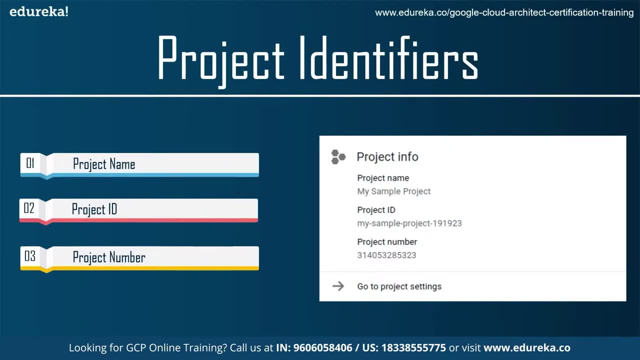 Let's now understand how to create and manage projects in Google cloud platform. Before we begin, keep in mind that in order to interact with Google cloud resources, you must provide the identifying project information For every request. So the following are used to identify your project: 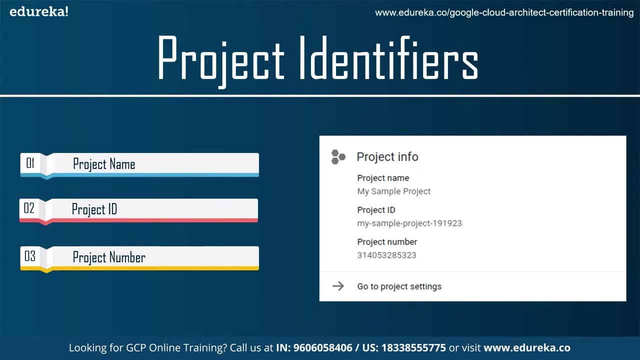 First is a project name, which is a human, readable name for your project. The project name isn't used by any Google API's. You can edit the project name at any time during or after project creation. Project names do not need to be unique. 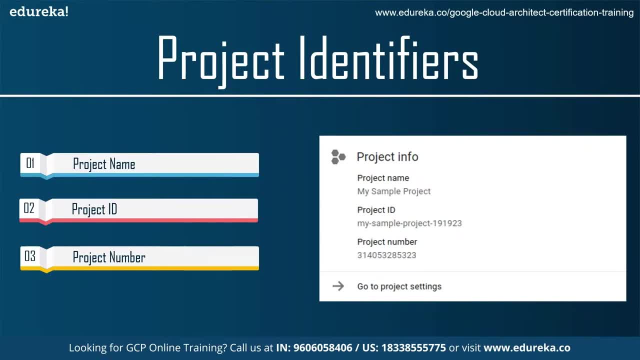 Now the next one is a project ID, which is a customizable unique identifier for your project. So you can see this in the project name. my sample project is given, which is the project name. Then the second thing is project ID, Which is a customizable unique identifier for your project. 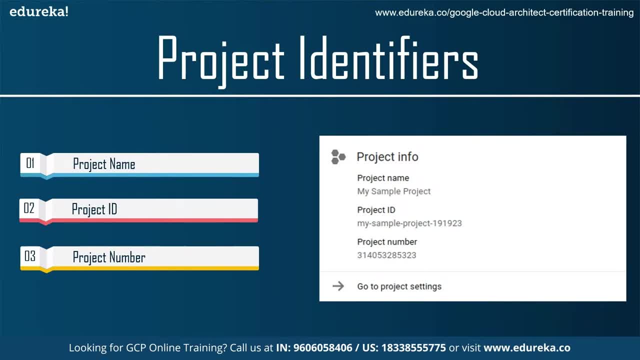 The project ID is a unique user assigned ID that can be used by Google API's. If you do not specify a project ID during project creation, a project ID is assigned automatically. The project ID must be a unique string of six- 30 lowercase letters, digits or hyphens. 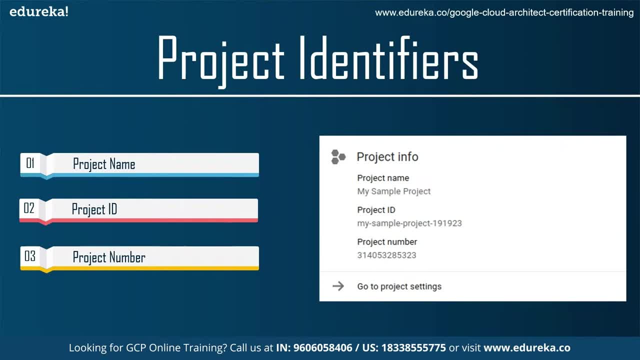 It must start with a letter and cannot have a trailing hyphen. You cannot change a project ID Once it has been created. cannot reuse a project ID that is in use or one that has been used for. Some words are restricted from use in project IDs. 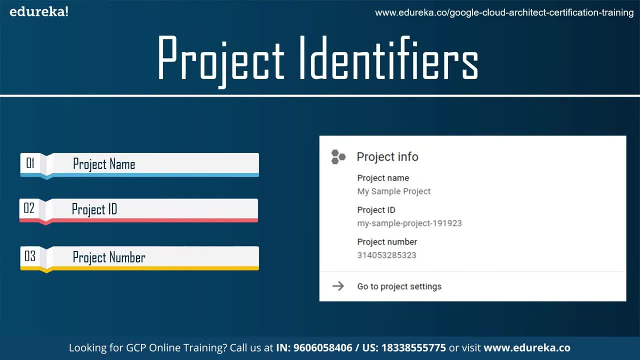 If you see restricted words in the project name, such as Google or SSL, the generated project ID excludes these words. Now, the last one is a project number, which is an automatically generated unique identifier for your project. The project number and project ID are unique across Google Cloud. 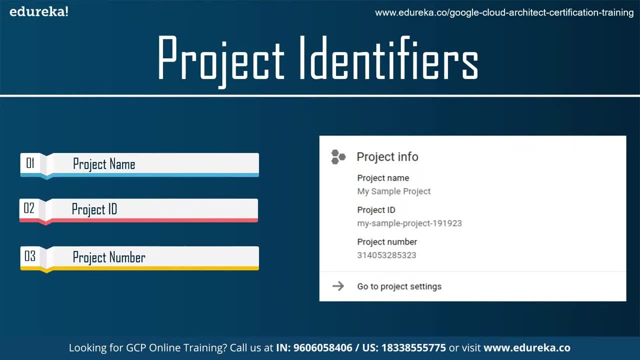 If another user owns a project ID for their project, you won't be able to use the same project ID. You can't reuse the project ID of a deleted project as well. So when you choose your project ID, don't include any sensitive information in your names. 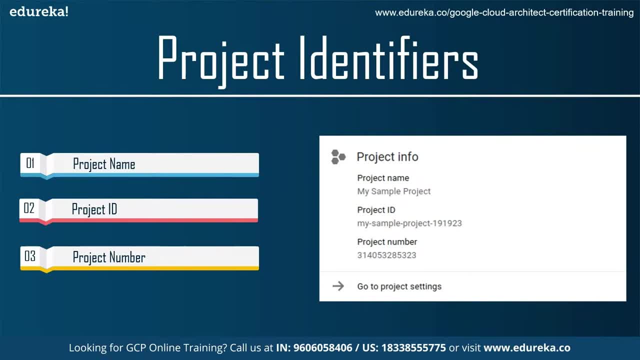 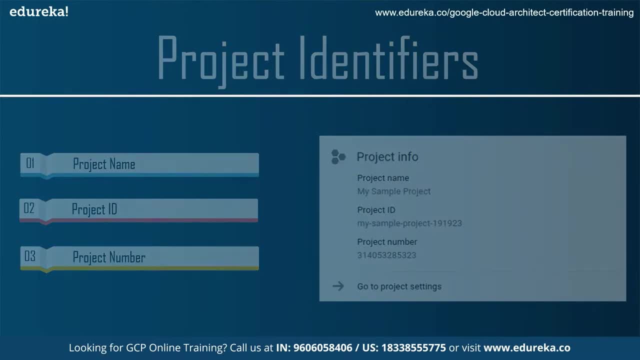 Like you can see here, the project ID is given as a MySampleProject191923 and project number. This is just a for example. I'll show you project number that is also automatically assigned. Now let's get started with understanding how to create a project. 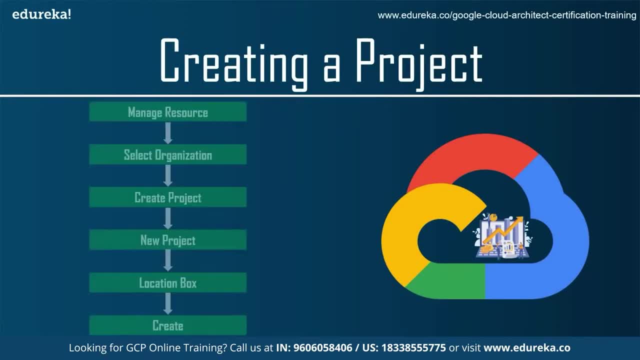 This permission is included in the project creator resource manager. project creator role, which is granted by default to the entire domain of a new organization and to free trial users as well. If you do not specify the parent name, you will not be able to create a project ID. 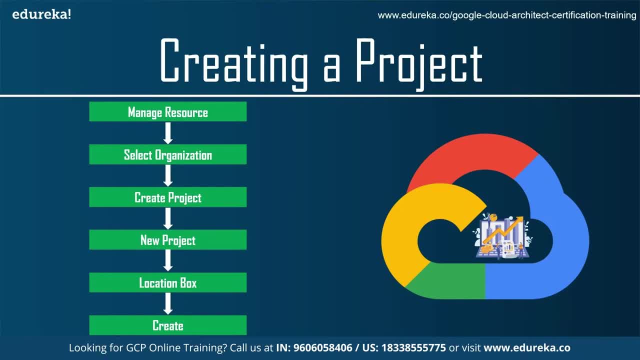 The parent resource is selected automatically based on the user accounts domain. You can create a new project using the cloud console, the Google Cloud command line tool or the project create method as well. So to create a new project, do follow these steps Like: go to the manage resource page in the Google Cloud console. 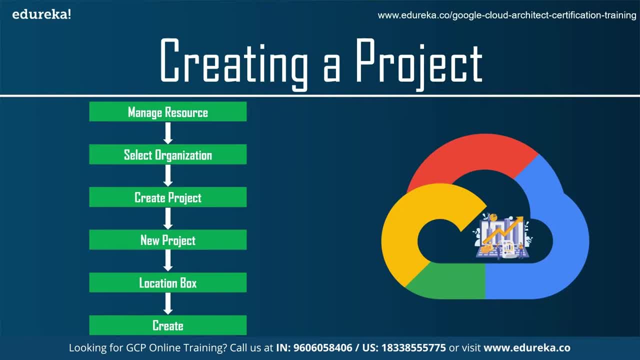 On the select organization drop down list at the top of the page, select the organization in which you want to create a project. If you are a free trial user, skip this step. as this list does not appear, Then click create project. in the new project window that appears, enter a project name and select billing account as applicable. 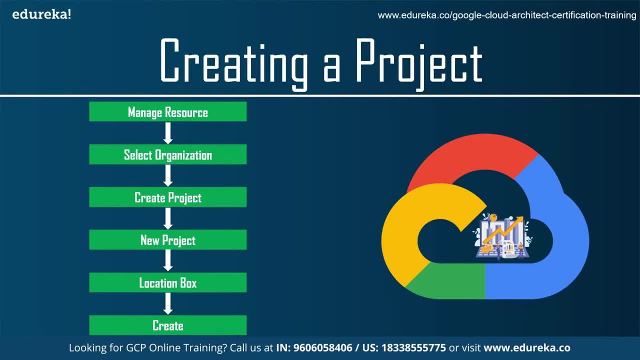 A project name can contain exclamation points and must be between four and 30 characters. Then enter the parent organization of folder in the location box. That resource will be the hierarchical parent of the new project. When you are finished entering new project details, click create. 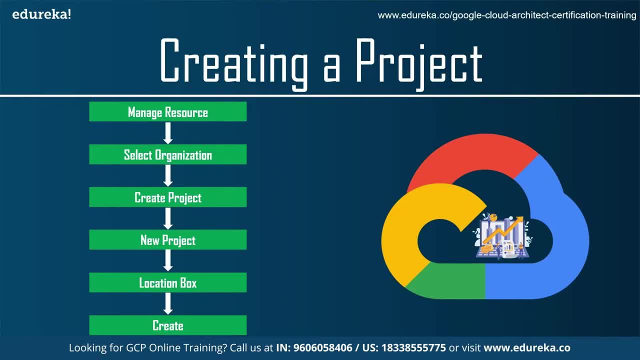 Also, you can create a project using a service account. You can use a service account to automate project creation. like user accounts, Service accounts Can be granted permission to create projects within an organization, and service accounts are not allowed to create projects outside of an organization and must specify parent resource when creating a project. service accounts can create a new project using the cloud tool or the project create method. 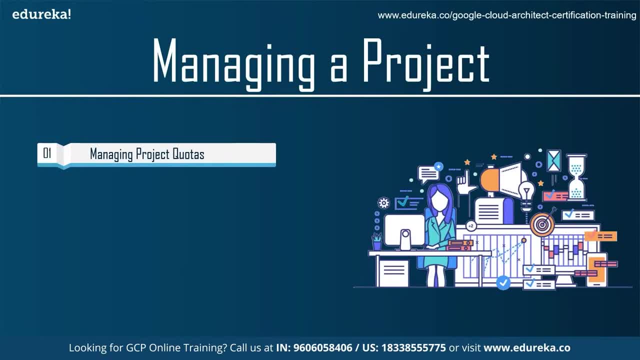 So now let's understand how to manage a project. So the first step is to like manage project quotas. So if you have fewer than 30 projects remaining in your quota, notification displays the number of projects remaining in your quota on the new project page. 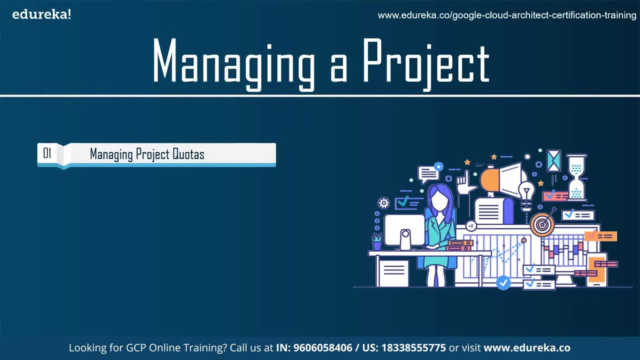 Once you have Your project limit to create more projects you must request a project limit increase or alternatively, you can schedule some projects to be deleted after 30 days on the manager to source page. projects that users have a soft deleted count against your quota. 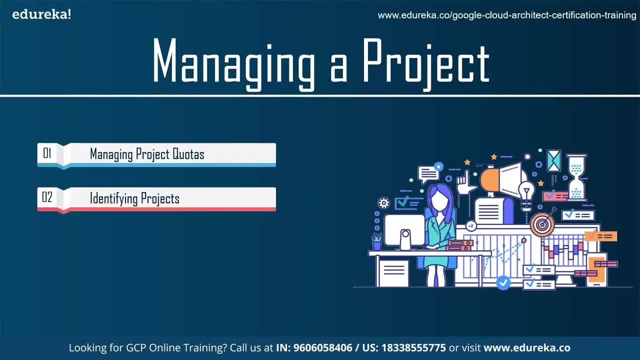 So these projects get fully deleted after 30 days only. And the second thing is identifying projects. So to interact with the Google cloud resources, you must provide the end thing, project information, for your request. A project is identified by its project ID and project number, as I have like already explained you what is project ID and project number. 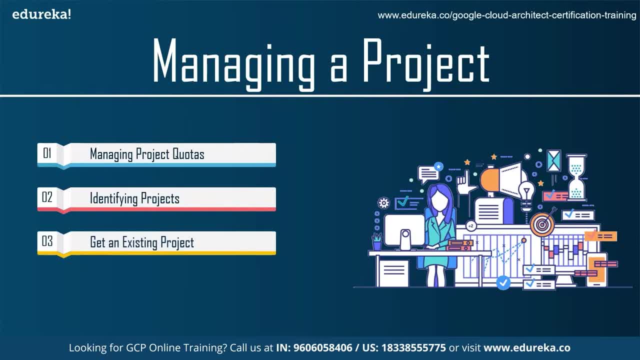 And how to get them. Also, you can like get an existing project. You just have to go to the project list and choose your existing project. Then you can also like go for listing projects, which can be done in two ways. That is, a list all projects under resource, or search for a project for managing the project. 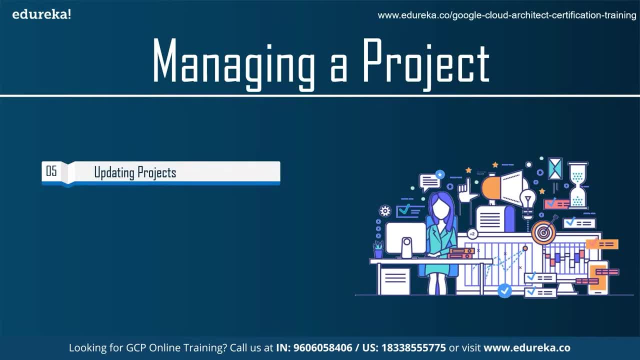 The updating of the projects can also be done, Like you can update projects using the cloud console or the projects dot patch method. Currently, the only fields that can be updated are the project name and labels. You cannot change the project ID value That you use with the Google cloud command line tool or API request. 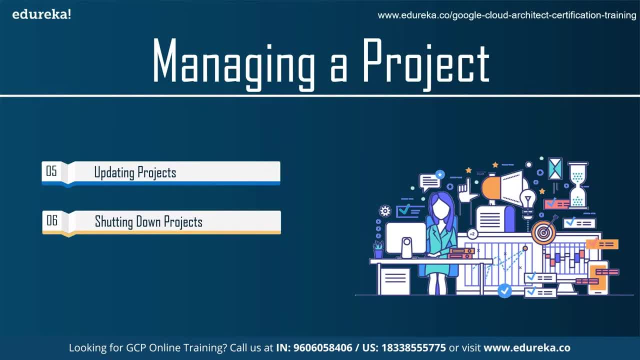 Next thing is shutting down. or can you can say, like the rating the projects, So you can shut down projects using the cloud console or the projects dot delete method? A project must have a life cycle state of active to be shut down in the way. 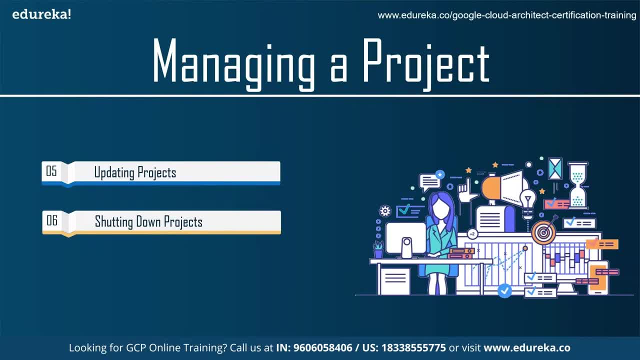 This method immediately marks a project to be deleted. A notification email will be sent to user who initiated the delete operation and the technical category contracts that are listed in his initial contacts. Project that is marked for deletion is not usable If the project has a billing account associated with it. that association is broken and isn't restrained if the project delete operation is cancelled. 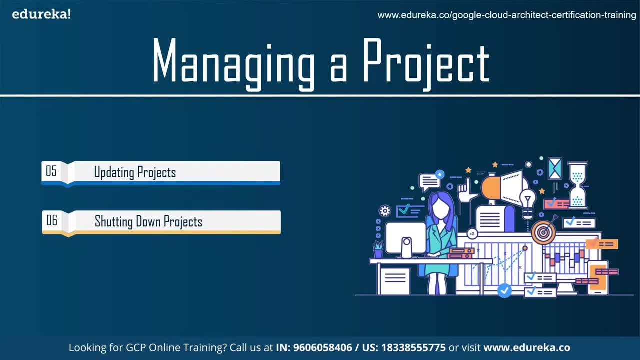 After approximately 30 days, the project is deleted. at the end of the 30 day period, The project and all of its resources are deleted and cannot be recovered. until it is deleted, The project comes towards your project quota. If you have set up billing for a project, it might not be completely deleted until the current billing cycle ends and your account is successfully charged. 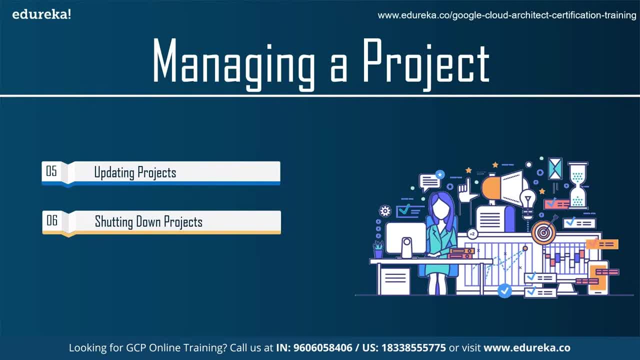 The number and types of services in use can also affect when the system permanently deletes a project. If the process to shut down a project fails, you can go for troubleshooting project duration, And the last thing in managing a project is restoring a project. Project owners can restore a deleted project within the 30 day recovery period that starts when the project is shut down. 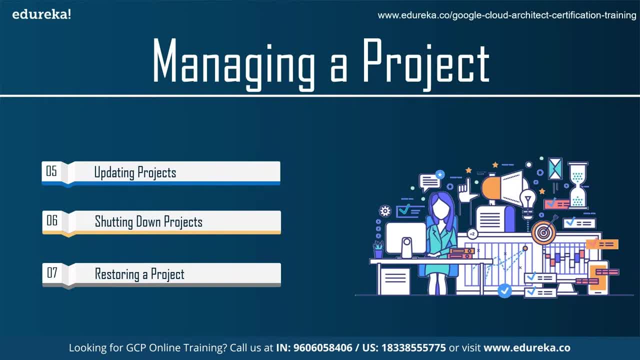 Restoring a project returns it to the state it was in before it was shut down. So some resources, such as the cloud storage or PubSub resources, are deleted before the 30 day period. So some resources, such as the cloud storage or PubSub resources, are deleted before the 30 day period ends and may not be fully recoverable. 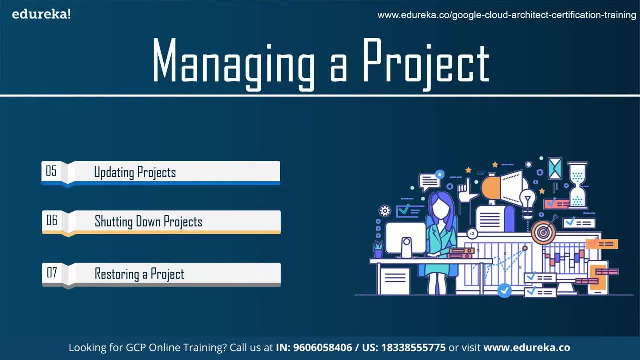 To restore a project using the cloud console, you just have to go to the manage resources in the Google Cloud console and in the project picker at the top of the page select your organization. Below the list of organization folders and projects, click resource pending deletion and then check the box for the project you want to restore. 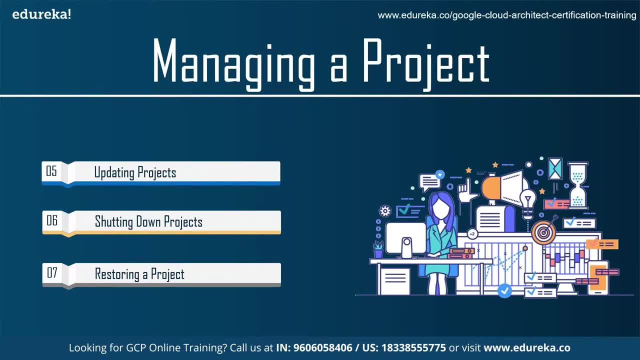 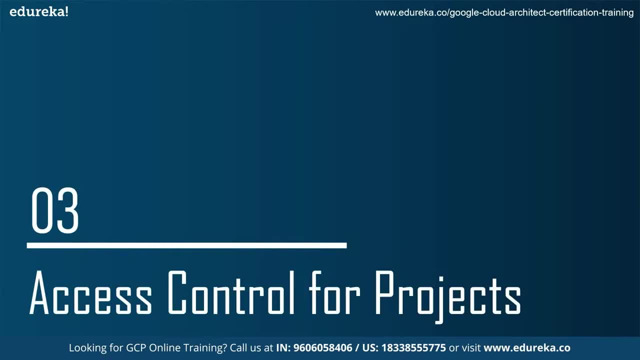 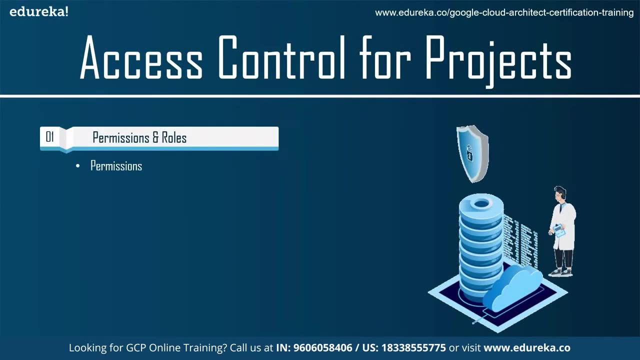 Then click just restore and the dialog that appears confirm that that you want to restore the project. Now that we have understood how to manage and create a project, let's understand how we can provide access and control for projects using identity and access management. So Google Cloud offers identity and access management, which lets you give more granular access to specific Google Cloud resources and prevents unwanted access to other resources. 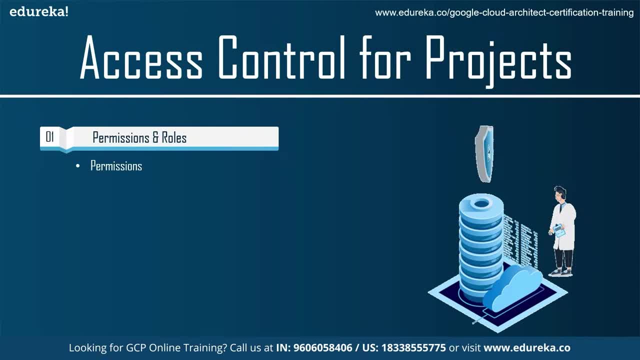 So IAM lets you adopt the security principle of least privilege, So you grant only the necessary access to your resources. IAM lets you control who has what access to which resources by setting IAM policy which grants specific roles that contain certain permissions. So the first thing. 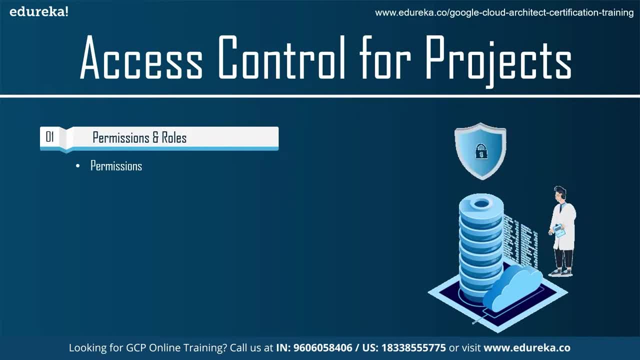 in access control is permissions and roles. so to control access to resources, google cloud requires that accounts making api requests have appropriate iam roles. iam roles include permissions that allow users to perform specific actions on google cloud resources. for example, the resource manager organizations list permission allows a user to list the organizations they own while resource 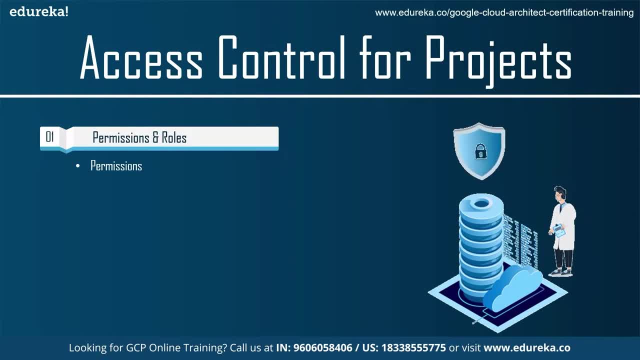 manager projects delete. allow a user to delete a project. you don't directly give users permission state. you grant them roles which have one or more permissions bundled with them. you grant these roles on a particular resource but they also apply to all of that resources. descendants in the. 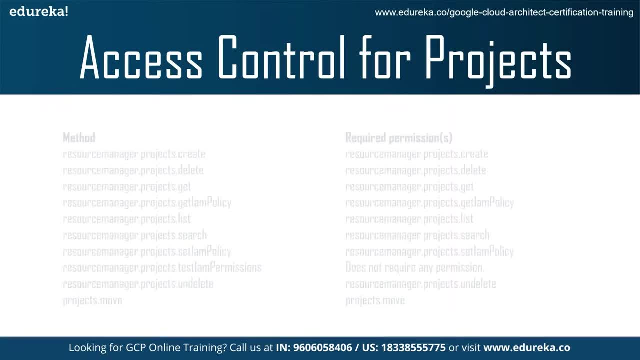 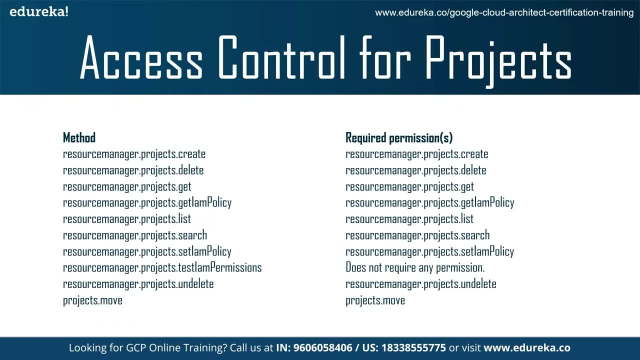 resource array. so let's understand it briefly, so fastest permissions. so to manage projects, the caller must have a role that includes these. following permission, the role is granted on the organization or folder that contains the projects. so you can see the method and required permissions for it. you can see for 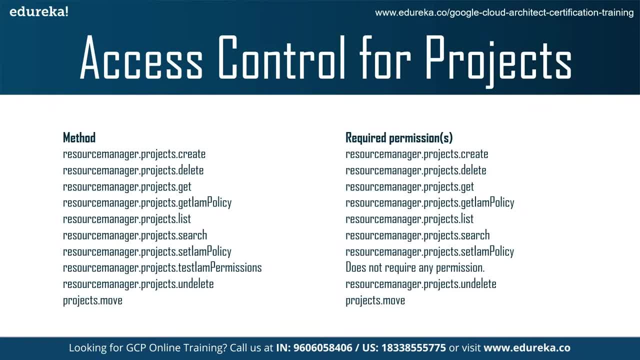 create permission. there is a resource manager projects create. you can see all the same, but you can see the third, last one, which is resource manager projects dot test. i am permissions. that doesn't require any permission. then there are user predefined roles as well, so i am predefined. 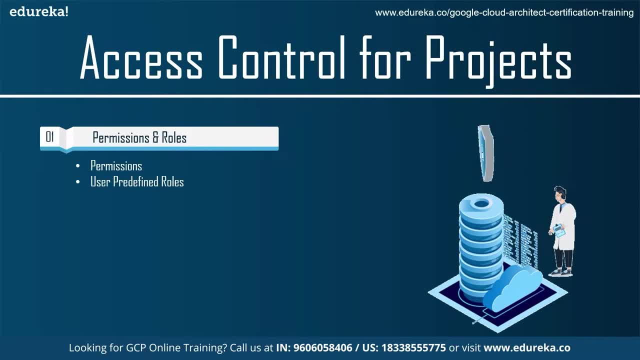 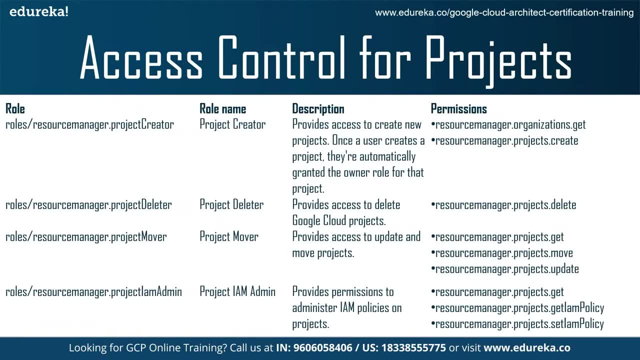 roles allow you to carefully manage the set of permissions that your users have access to. the following table is the predefined rules that you can use to grant access to a project. each role includes description of what the role does and the permissions included in that role. so you can see the role and the name for it, then also the description, like you can see for role name. 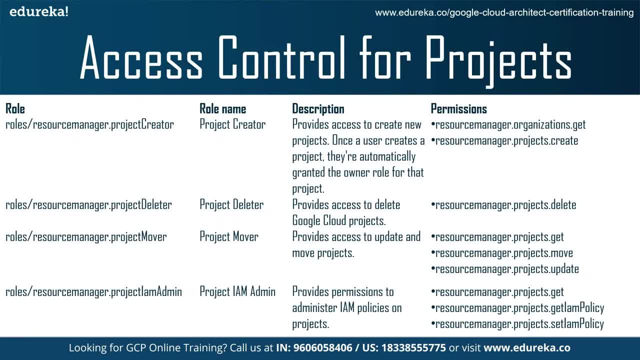 project creator. you can see that it provides access to create new projects. once a user creates a project, they are automatically granted the owner role for that project. then you can see the permissions for it, the specific permission for it. like resource management organization start get to get the permissions similarly for project deleter and project move and project. i am admin. 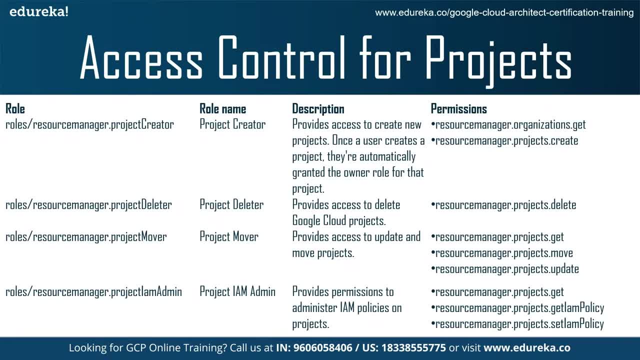 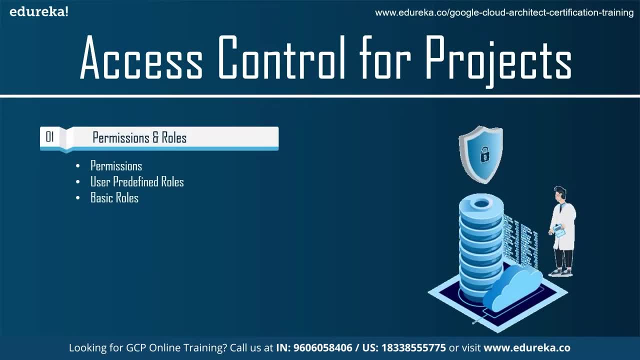 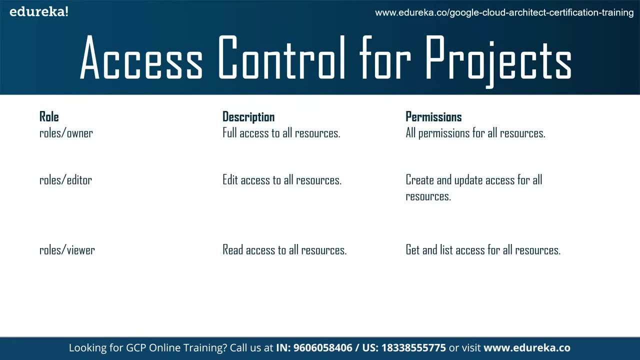 specific permissions are there and you can select. see the descriptions also for it. then there are basic roles. these roles are very powerful, include a large amount of permissions across all google services, like you can see, for owner, editor and viewer. these are, like you see, in resource hierarchy, they are the highest roles. you can see, like how, for owner. 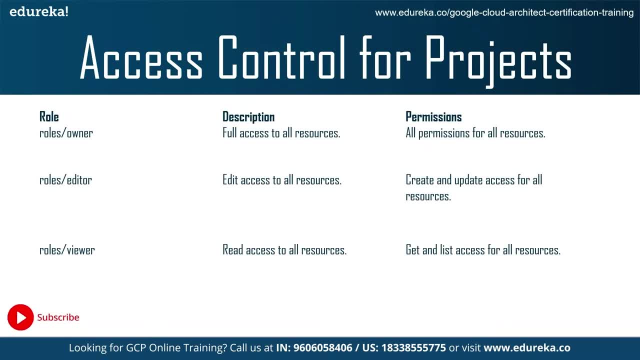 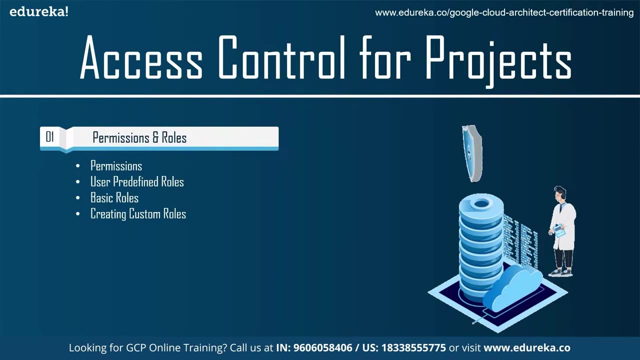 all permissions for all resources are given. then for editor: create and update access for all resources. and then, with the viewer role, you can like, get and list access for all resources. also, like can create custom roles. so, in addition to the predefined roles described in the top, you also create custom roles that are collections of permissions that you tailor to your needs. 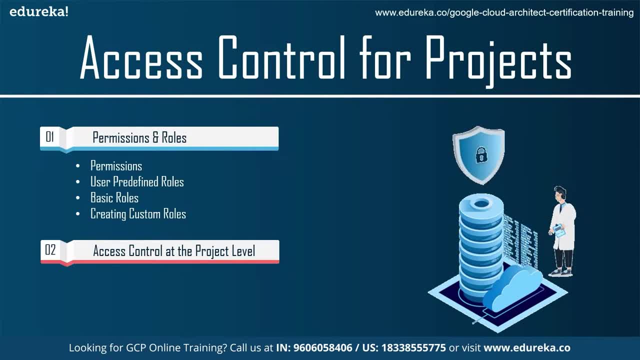 then the second thing in access control at the project level. so you can like grant roles to users at the project level using the google cloud console, the resource manager api in the google cloud command line tool. so there's a default role, also like when you create a project. 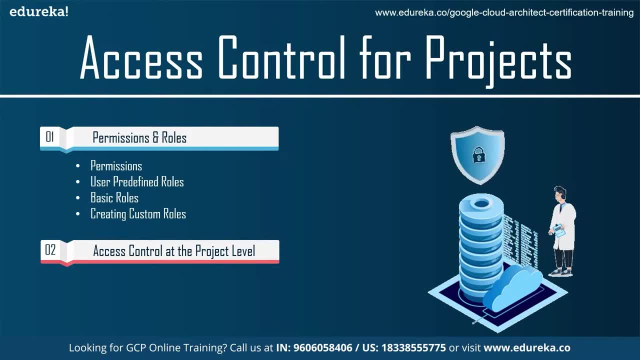 you are granted the owner role of for the project to provide you full control as the creator. this default role can be like changed as normal in an iam policy as well. then there are like vpc service controls, so vpc service controls can provide, like additional security when using the resource manager api. so vpc service controls improves. 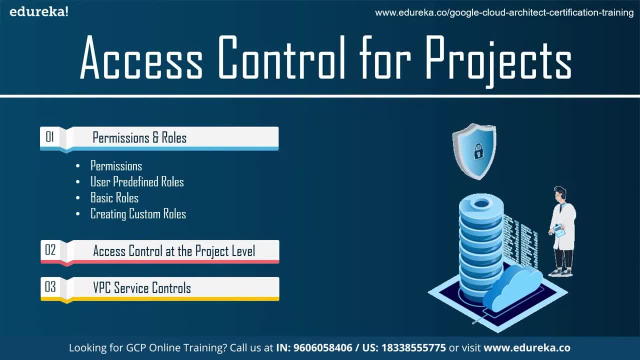 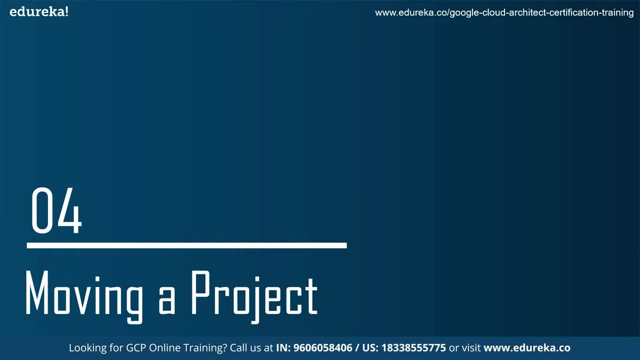 your ability to mitigate the risk of data exfiltration from google cloud services, such as cloud storage and bigquery. you can use vpc service control to create parameters that protect the resources and data of services that you explicitly specify. now let's move on to understand how to move a project within the resource hierarchy. so the project resource is the. 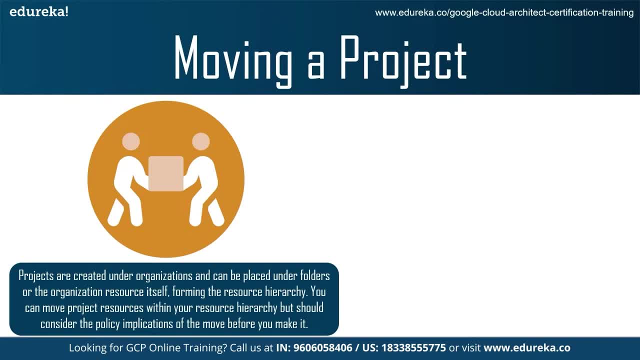 entity in a Google Cloud organization. Projects are created in organizations and can be placed under folders, so the organization resource itself forming the resource hierarchy. You can move project resources within your resource hierarchy but should consider the policy implications of the move before you make it So. when you move a project, any identity and access management policies. 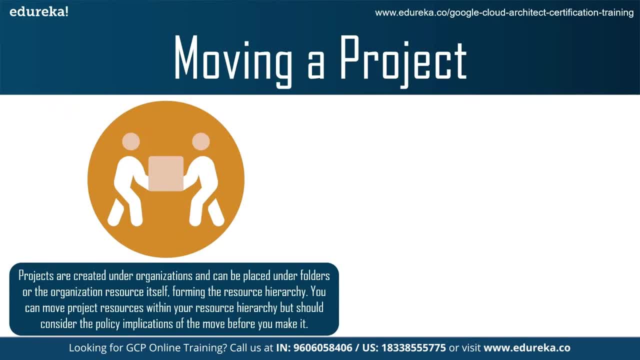 or organization policies that are directly attached will move with it. However, a project in your resource hierarchy is also affected by the policies that inherits from parent resources. So if a project inherits an IAM role that provides user permissions to use a particular service, Users will. 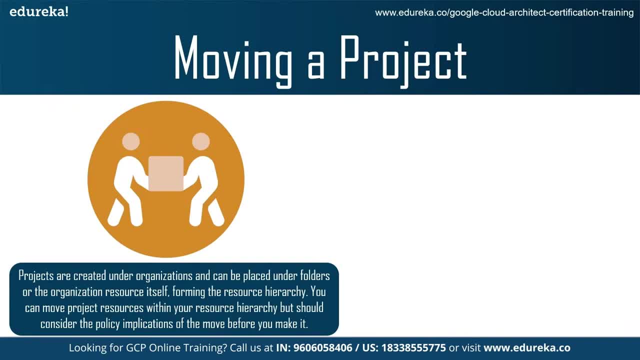 not have access to that service at the destination unless it would inherit the permision at the destination as well. So like, for example: consider a service account as the storage object creator role bound to a user or a folder, You can consider the folder as folderring, So the service accounts. 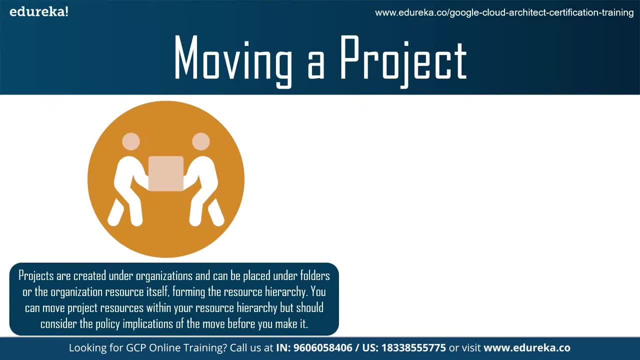 permissions to upload data to cloud storage in any project in folder a. if you move one of these projects to folder b, which does not have the same inherited permission, the service account for that project loses the ability to upload data, resulting in a service outage. these same considerations. 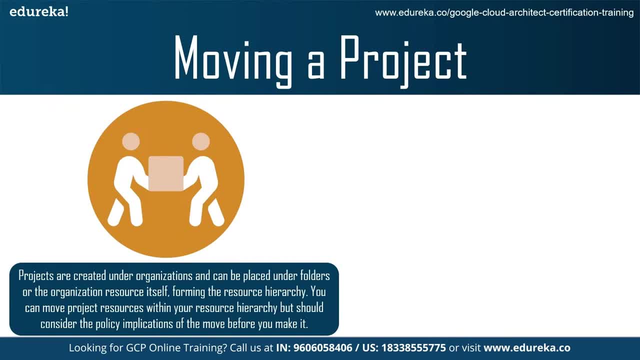 apply if organization policies are defined at the source and destination folders, like im policies. organization policies are inherited. consequently, you must ensure that your organization policies are consistent between source and destination folders. to move a project, you need the following im rules, like having the resource manager dot projects, update permission on the project which 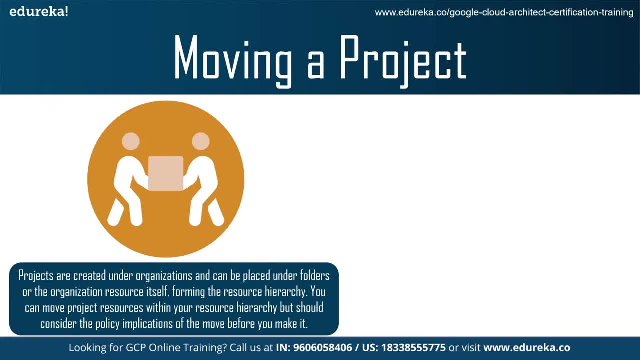 typically comes from having either the project editor or project owner rules on the project. so the second permission is have the resource manager project move permission on both the source folder and the destination folder. this permission is typically part of the project owner, project editor or folder admin or folder mover rules if the resource is not in a folder. 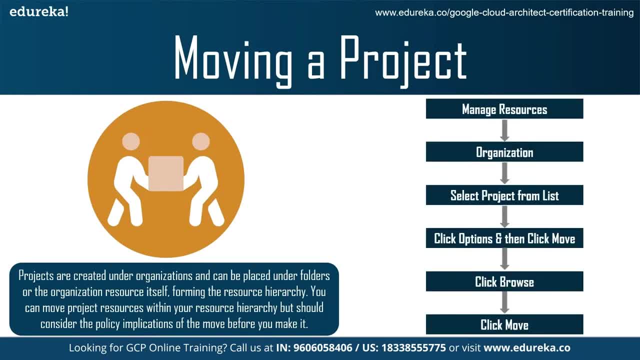 you will need the permission on organization node. you can follow these step to move a project. so in the google cloud console, go to the manage resource page. select your organization from the organization drop down on the top left of the page. third is the like: click on your projects row to select your project role. 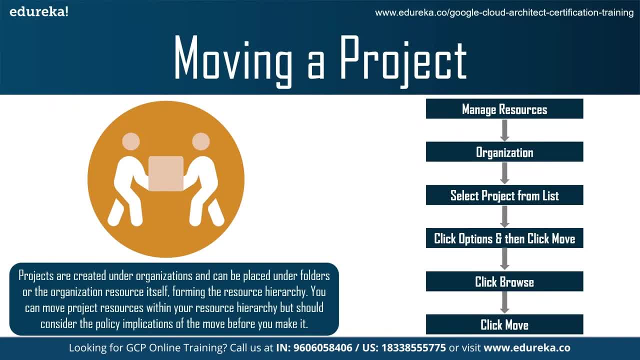 from the list of resources. note that you must not click on the name of the project which takes you to the projects iam page. then next you have to click on the options menu in the row and like click move. then click browse to select the folder to which you want to move the project. 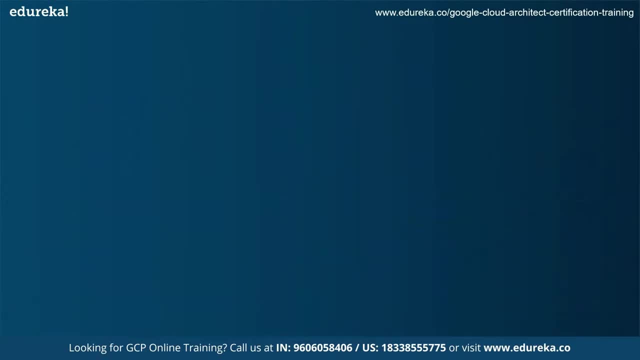 and then finally click move. now that you have understood how to move a project, let's now understand how to migrate a project between organizations. we will understand it quite briefly. so the project resource is the base level organizing entity in a google organization. projects are created in organizations and can be placed under folders or the organization resource. 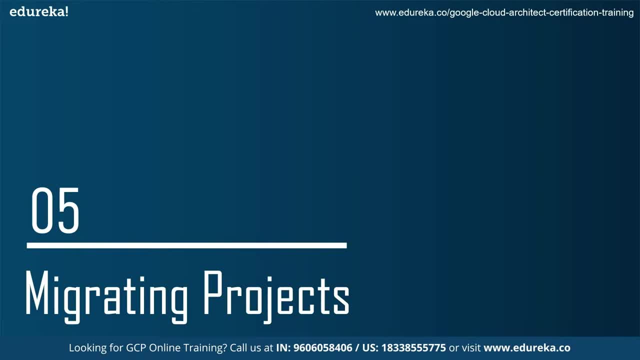 itself forming the resource hierarchy. you may need to migrate projects between organizations due to acquisitions, regulatory requirements and separation between business units, among other things. you can resource manager API to move projects across organizations or to another place in the resource hierarchy of its current organization. The resource manager API also lets you roll back. 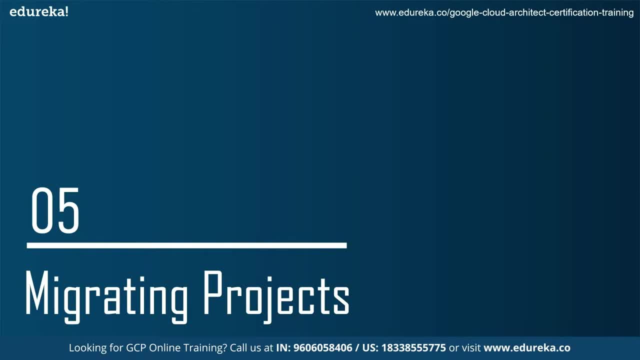 the migration, moving the project back to its original place in the resource hierarchy. Note that it generally takes less than a minute for the project move to complete. After moving a project, it may take several minutes to reflect this change in the Google Cloud console. So in migrating, 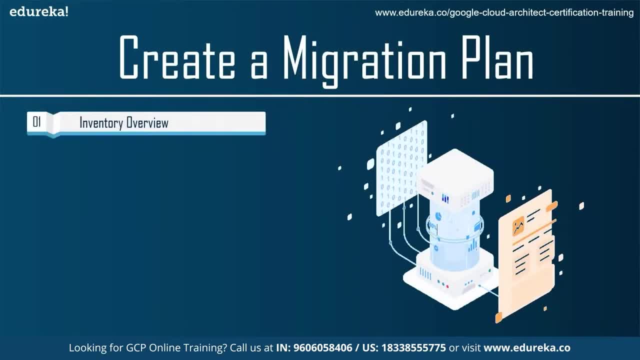 projects. first we need to create a migration plan. So the most important thing to consider during a project move is how the migration will impact the services running inside the project. The resource manager API treats the project resource and all services running underneath it as a single unit, meaning that no configuration changes will be applied inside the project. 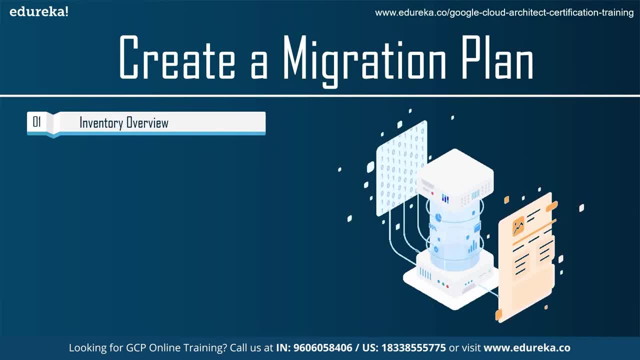 While migration will not make direct configuration changes to the project, the change in the resource hierarchy is likely to have an impact on the function of the project and its running services: inherited policies, such as identity and access management or organization policies. While migration will not make direct configuration changes to the project, 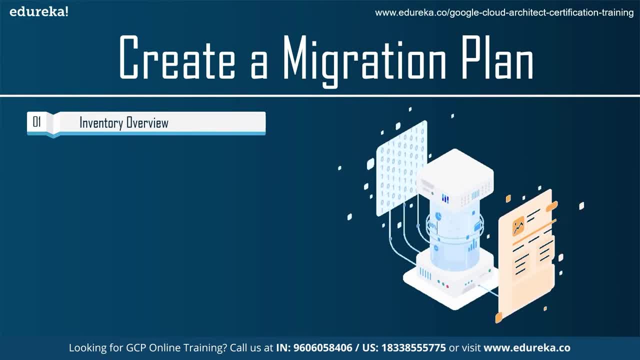 change in the resource hierarchy is likely to have an impact on the function of the project and its running services. So inherited policies such as identity and access management or organization policies will not move with the project during migration, Only policies and serve accounts that are attached directly to the resource. This may cause unintended behavior after the migration is. 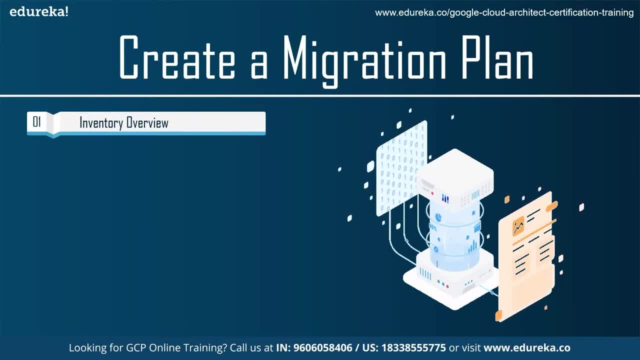 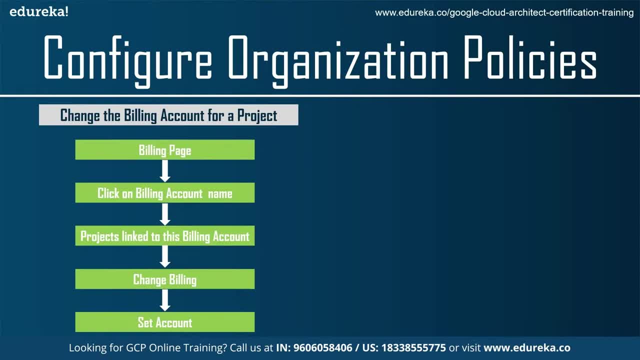 is that the resource manager API will not move with the project during migration. So the third thing in configuration is that the resource manager API will not move with the project during migration. So the third thing in configuration: follow these steps and you can like change the billing account for a project Charges already. 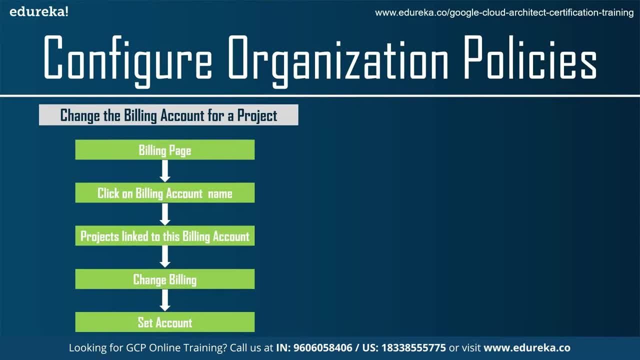 incurred that have not yet been reported in the transaction history will be billed in the former billing account. This can include charges from up to two days prior to when the project was moved. Also, you can move a billing account between organizations, So a billing account can be moved. 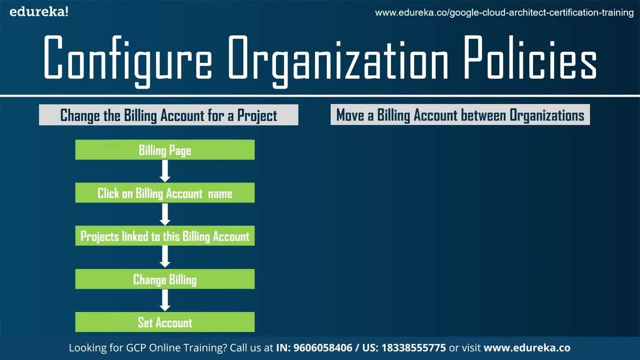 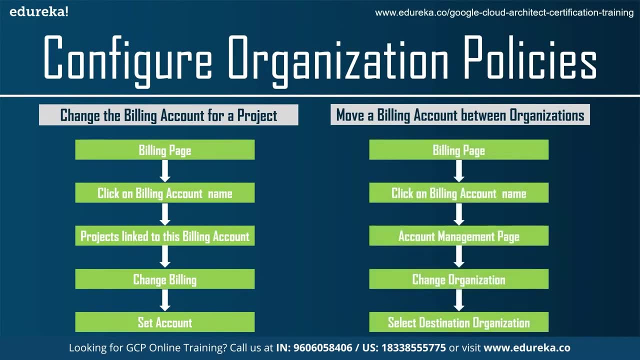 from one organization to another. although this isn't often a necessary step, Most existing organizations will already have a billing account. that should be used instead. If you need to migrate an existing billing account, get the billing admin role on the source and destination organizations. then go to the billing page in the cloud console. Click on the name of the billing account you want. 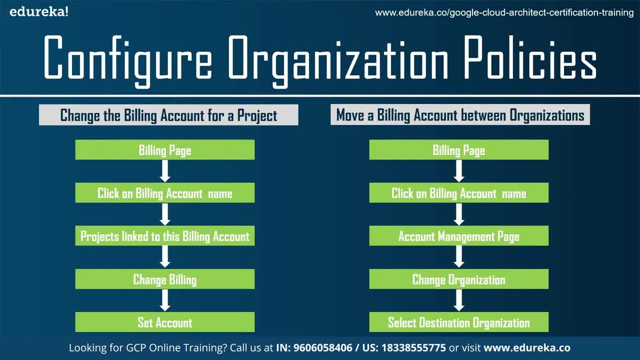 to move. At the top of the account management page, click change organization, Then select the destination organization and then click ok. The billing account is now associated with the specific organizations. Note: if you move a billing account that has active Google Cloud Marketplace subscriptions, those subscriptions are automatically cancelled. Then the last step in migrating a. project is to move a billing account from one organization to another. If you move a billing account that has active Google Cloud Marketplace subscriptions, those subscriptions are automatically cancelled. Note: if you move a billing account that has active Google Cloud Marketplace subscriptions, those subscriptions are automatically cancelled. Then the last step in migrating a project is to 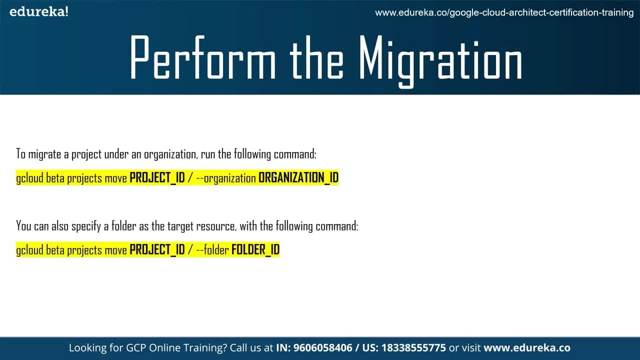 perform the migration. So if you have the appropriate IAM permissions and the required organization policies are imposed, you can use the resource manager API to move a project resource. The following instructions are only for migrating a project from one organization to another. To migrate a project under an organization, run the following command: 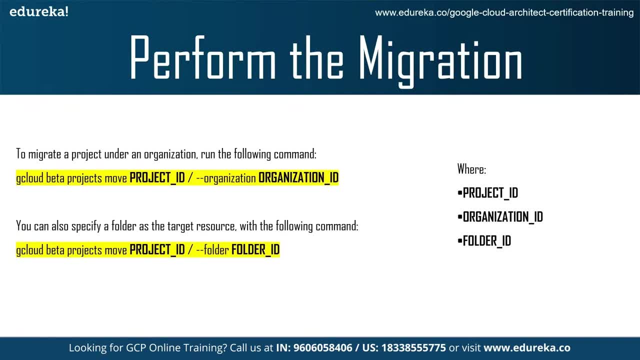 Then you can also specify a folder as the target resource with the following command: So where it will happen? So you need to understand the project ID, for that, Like, project ID is the ID or number of the project you wish to migrate, And then there's organization ID, which is the ID of the organization to which you want to move the project. 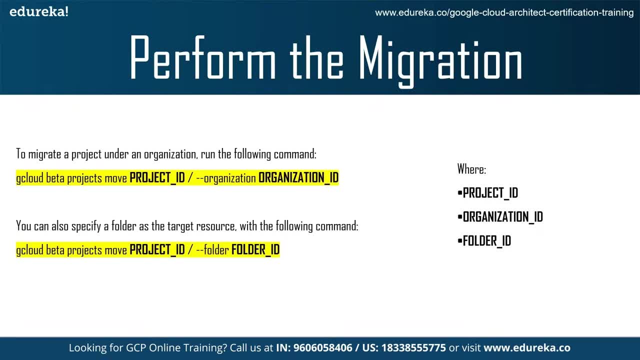 You can only specify one target, either an organization or a folder. And then there is folder ID, which is the ID of the folder to which you want to move the project. You can only specify one target, either a folder or an organization. 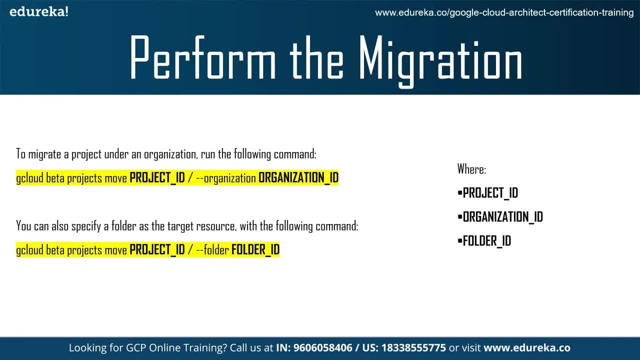 Also, you can roll back a migration. So if you have mistakenly moved a project, you can roll back the operation by performing the move again, With the old source as the new destination and the old destination as the new source. you must have the necessary IAM permissions and organization policies enforced to allow this, as if this were an entirely newer migration. 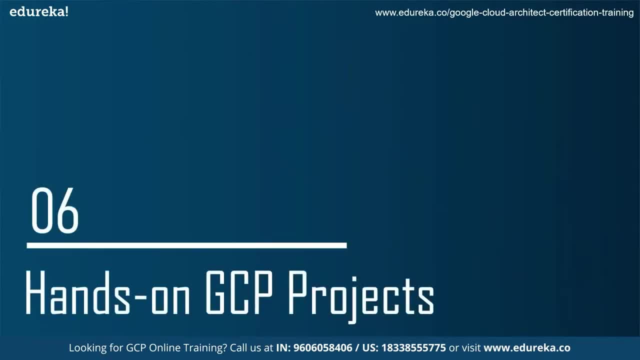 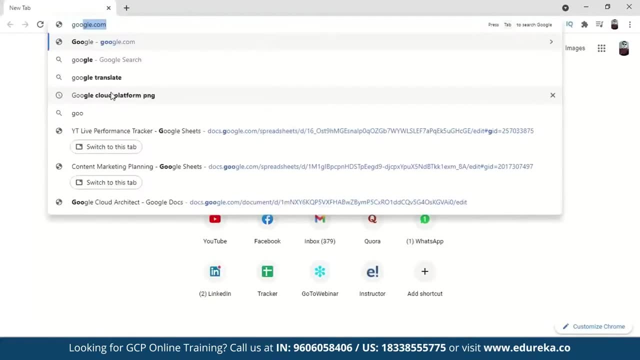 So now that you have a theoretical understanding of projects in GZB, let's now see how it's been made practically by trying our hands on it. on Google Cloud Platform, You can just directly go to Google Cloud Platform console. So this is how the Google Cloud Platform console looks like. 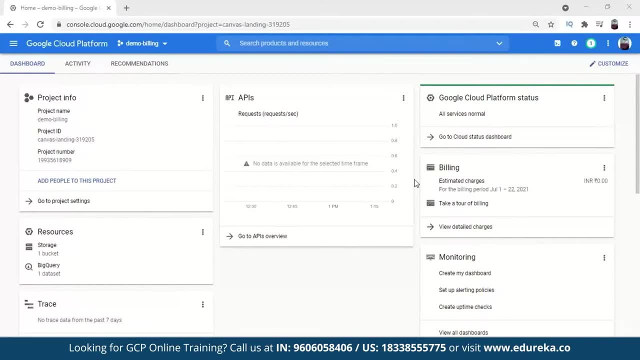 So if you don't have an account on Google Cloud Platform, create one. It's a very good platform to have an account on. While making the account, it will ask for a credit and debit card details. It will just deduct one rupee and that will also be refunded soon. 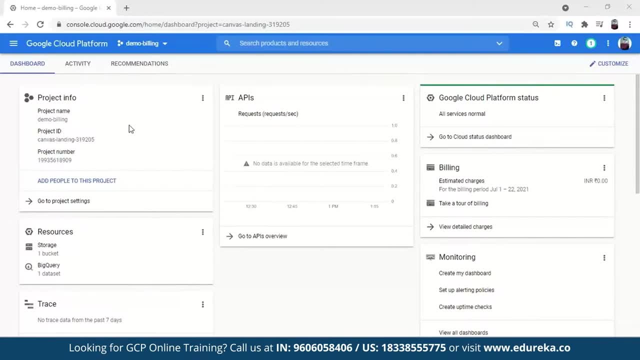 So here you can see like the project name, project ID and project number is given. Dashboard looks like so and you just have to go here. This is from where you can choose your project. Like I have created a number of projects, So this is how the project looks like. 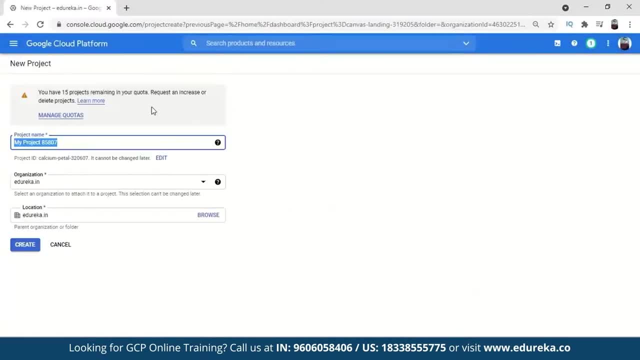 So this is how the project looks like. So you can also like go and create a new project from here. This gives a project name. You can give it like project list So you can see the project ID is getting created with this, the name and then this number. 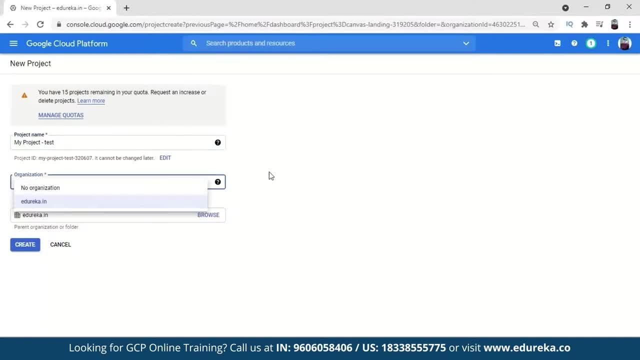 It cannot be changed later. okay, Then you can also choose your organization. If you are using a free account and you don't have an organization, then you can choose no organization also and create a billing account like this, Or you can just simply choose the organization. 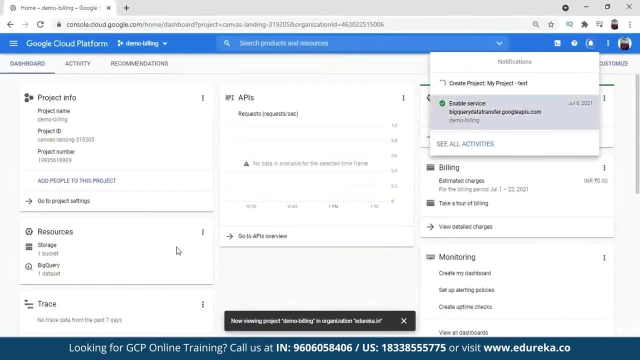 I will choose it from here, So I will just create it. It will take a few minutes. one few minutes like one or two minutes. yeah, So you can see like it got created. I will just select this project. So now you can see like the project name and project list, project ID and project number. 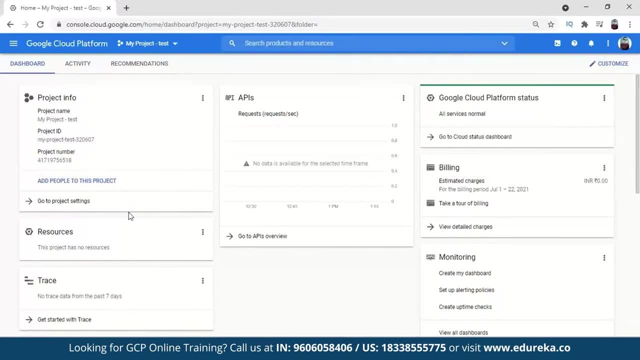 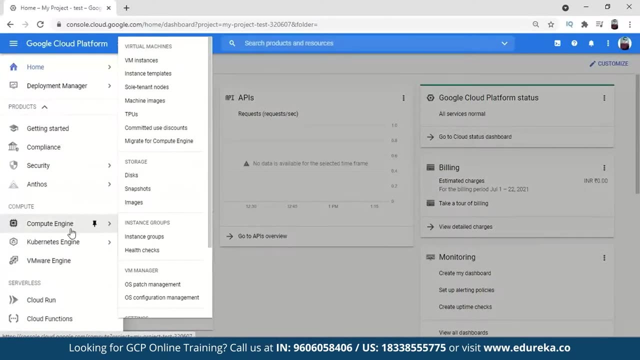 Everything is given here. That's how easy it is to create a project in Google Cloud Platform And from by making this project now you can like use all its services that you can see. You have the access to use a compute engine, Kubernetes, engine storage services also. 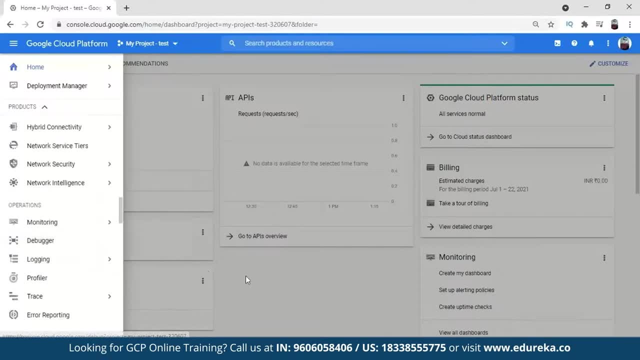 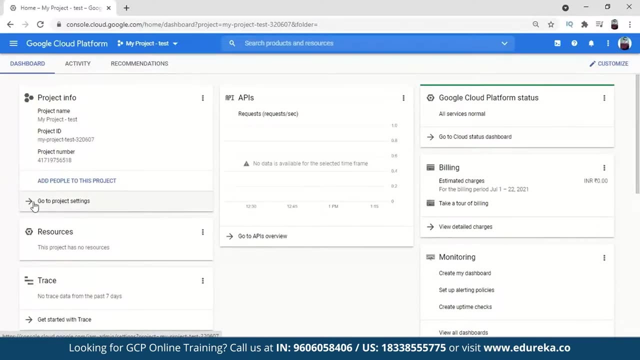 database services. also application integration As well. all these services you can use once you create a project. Under the project, you get the access to use these services. If you want to delete the project, you can just go to this settings. go to the project settings. 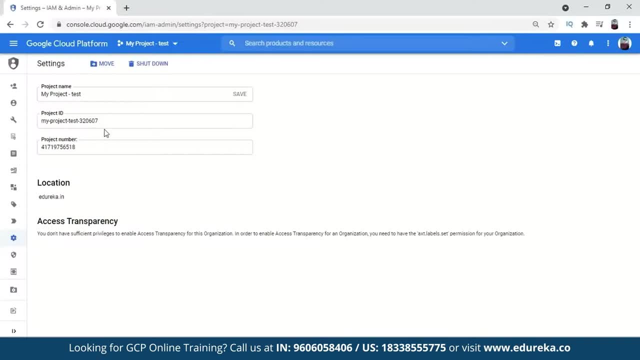 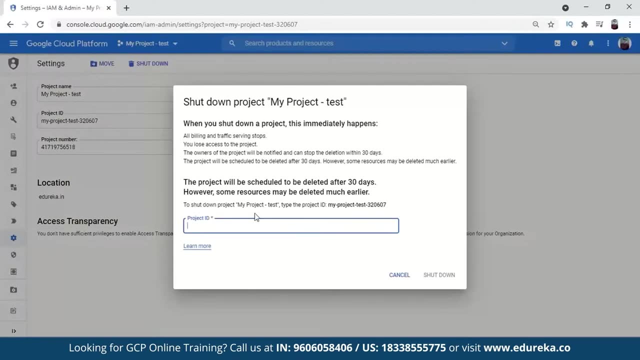 You can see. you can like choose the project name. This one only we have created, So we will just delete this project. You just have to shut down for that, You just have to type the name for it. So project ID with this, okay. 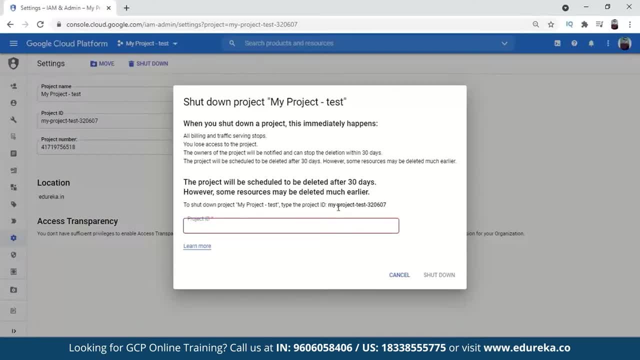 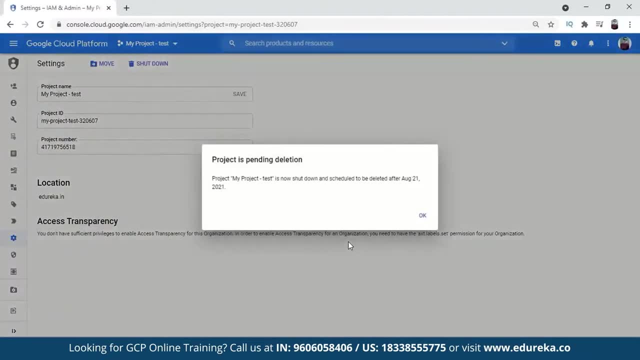 You shut down project, You just have to type the project ID. So this is the project ID. I'll just copy it, Paste it here And shut down. So, as I've told you, like, it takes at least one month to get the project shut down. 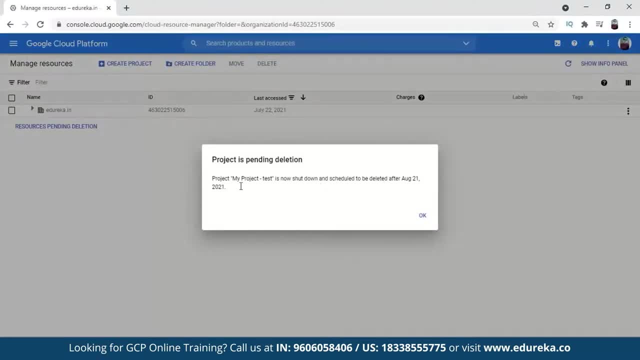 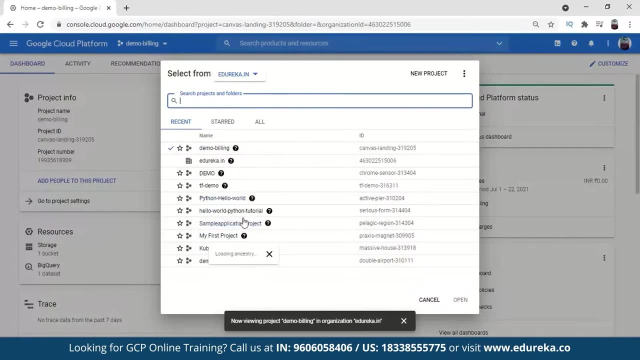 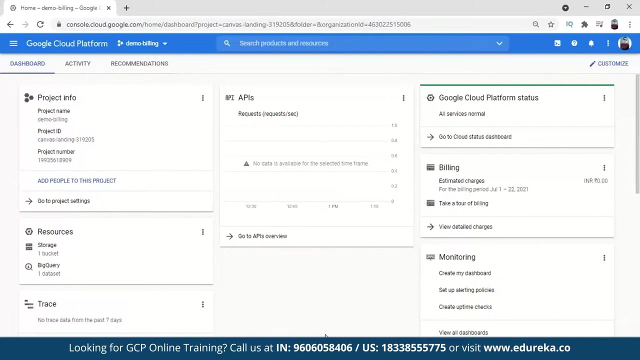 So you can see, today is like 22 July, So by 21st August we'll get shut down. That's how it's been shut down. Now you can see my project test does not exist here anymore, right? So I hope you have understood how to create a project and how to delete the project in Google Cloud Platform. 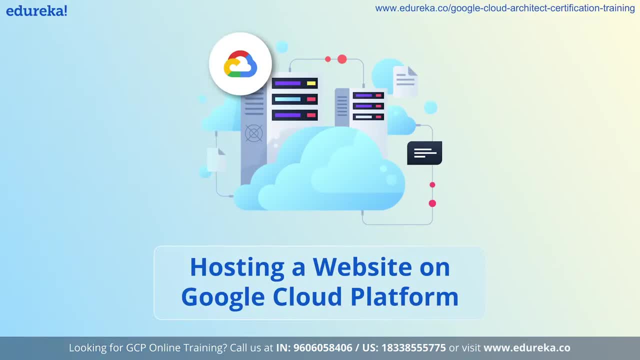 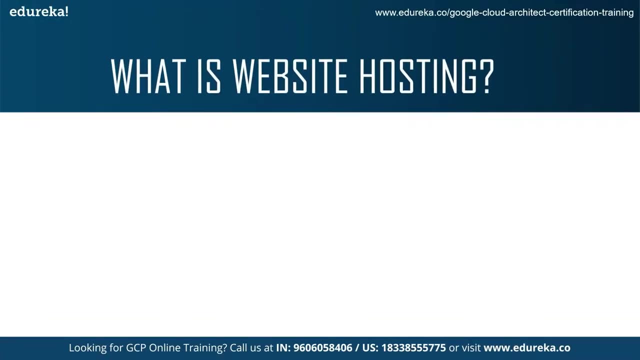 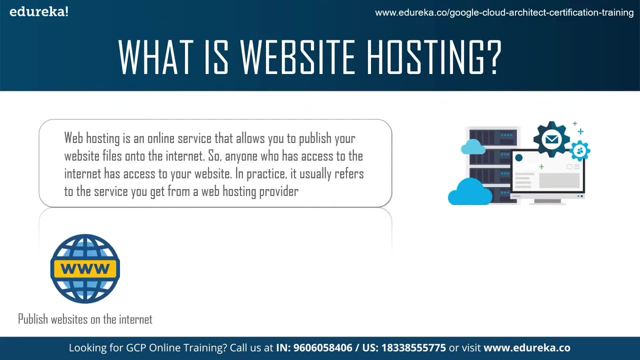 These are the concepts of Google Cloud Platform projects. What is Website Hosting? Now, when we talk about Website Hosting, we can see that Website Hosting is basically an online service that allows you to publish your website on the internet, So anybody who has access to the internet has access to your website. 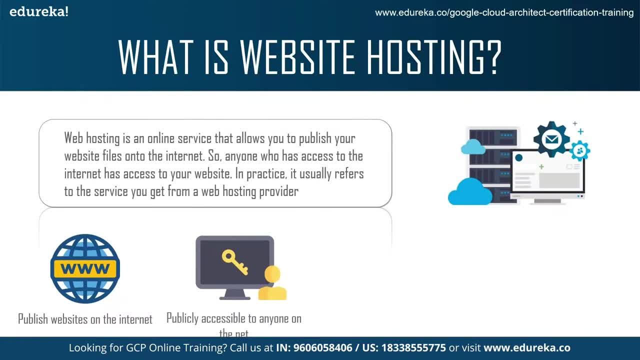 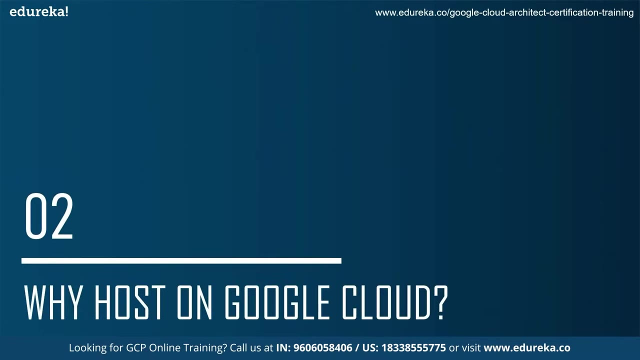 And basically in practice, it refers to service you get from a web hosting provider. So a hosting provider is somebody who is a third party and basically helps you host your website for you and maintains them. right, so hosts are responsible for maintaining the site. next up, we talk about why host on Google Cloud, right? so there are 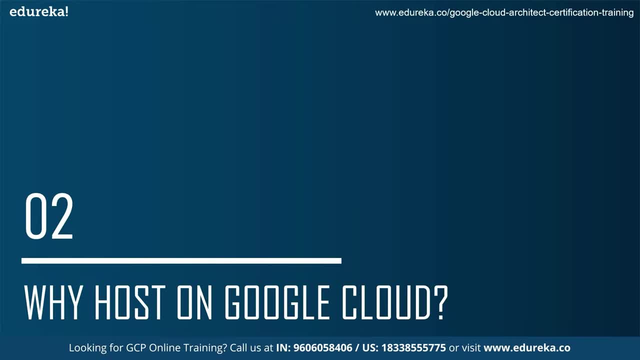 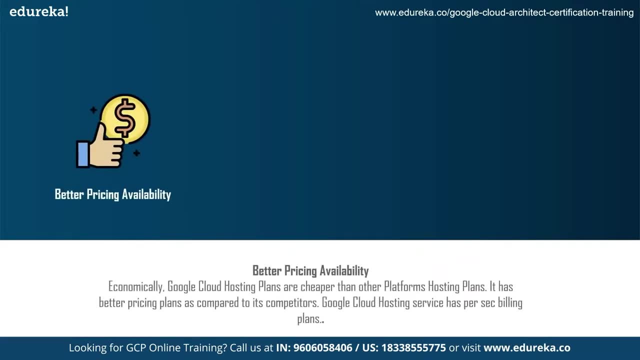 various reasons why you should host on Google Cloud. there are various advantages as to why people use Google Cloud platform for hosting. the first reason is the fact that it has a bit of pricing availability right. so when it comes to better pricing availability, economically, Google Cloud hosting plans. are much cheaper than the AWS or, as your hosting plans like, Google Cloud platform is definitely at least five percent cheaper than Azure and at least eight percent cheaper than AWS hosting plans. right, so this better pricing plan is basically something that keeps Google Cloud platform hosting services ahead. 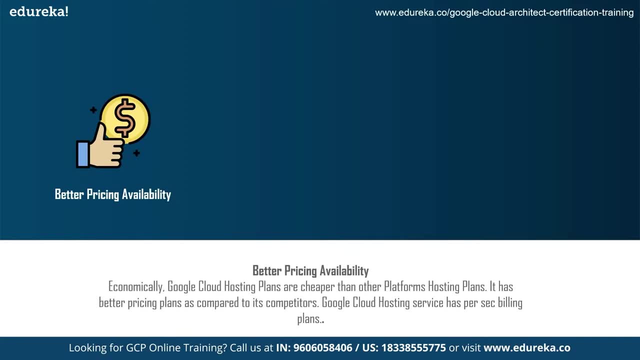 and it is built per second. so that is why Google Cloud platform is better pricing. next up, we talk about the enhanced execution that Google Cloud platform offers us. so when we talk about enhanced execution, we see that the enterprise level Google Cloud has enhanced the performance of its hosting services. right, so an individual can access the data from any. 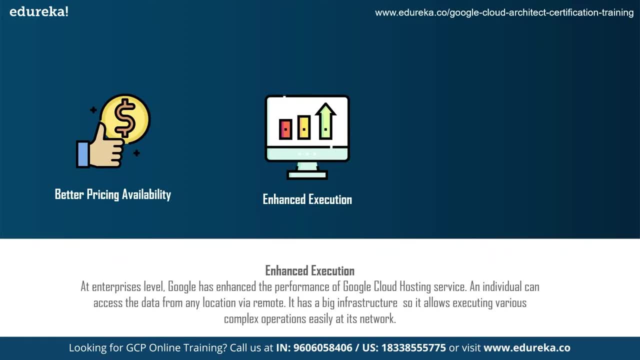 location via remote or a big infrastructure right, so that big infrastructure allows Google Cloud to basically execute various complex operations and enhance its own resources and services. right next up, we talk about the commitment to constant development. so when we talk about this, we talk about the fact that when Google is developing, 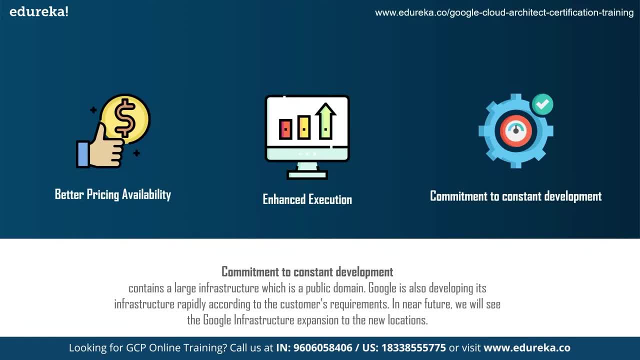 its infrastructure rapidly right. that is, according to its customers requirements. so when, in the near future, we'll see that the customers requirement has changed, it will be based on the Google infrastructure based on new locations- right. so it's continuously evolving based on your requirements. next up, we 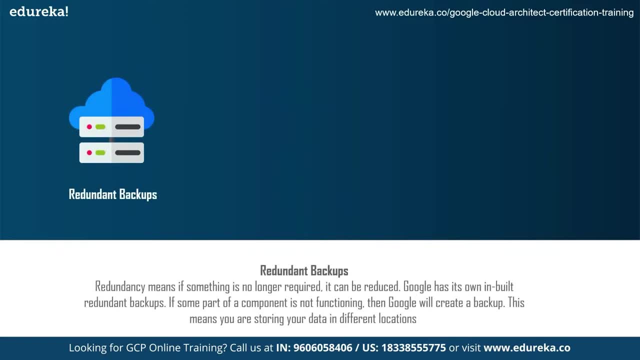 see that Google Cloud hosting with, basically, something where you can have redundant backups. now, redundancy, basically, is something where you do not have an extra copy of certain data, right so every data is unique to itself, right so? Google has its own built-in redundant backups, right so if some component is not, 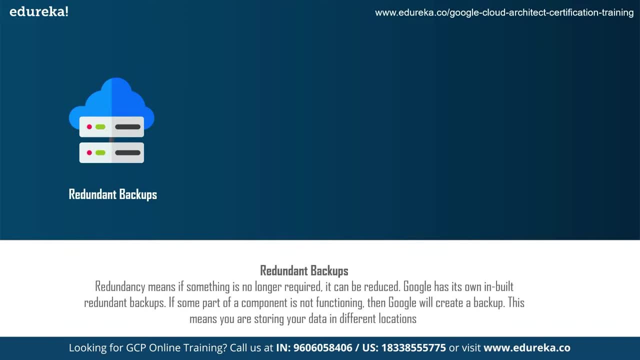 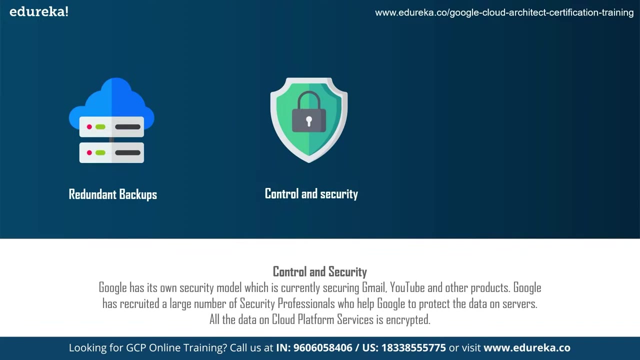 functioning, then Google will create a backup automatically, because you are storing the data in different locations, right? so that is why there's a backup. next up, we talk about the control and security that Google Cloud platform hosting will provide us. this is because that Google has its own security model. 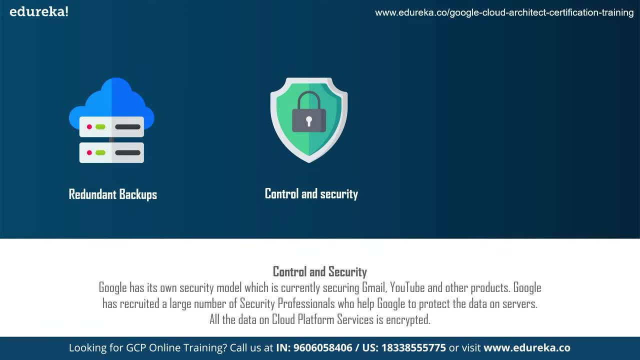 so when it has its own security model which is again used in other services provided by Google, such as Gmail, YouTube and other such products? Google has a included a large number of security professionals just to basically protect the data of the servers, right? so all the data on the Google Cloud platform is? 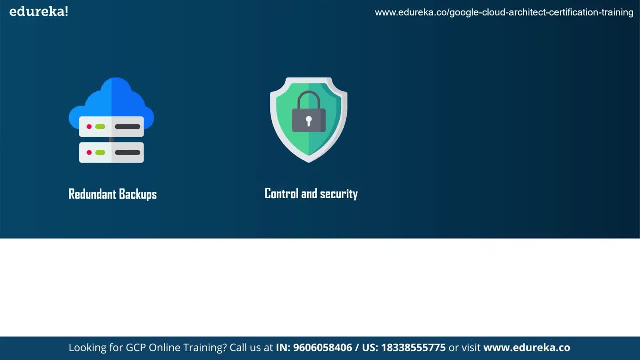 encrypted, so it is extremely secure. and finally, we come to the fact that live migration of data is possible. so one of the top advantages of Google Cloud hosting is live migration. right, it is the biggest advantage, because AWS and Azure both do not provide this benefit. right, so it only consists of. 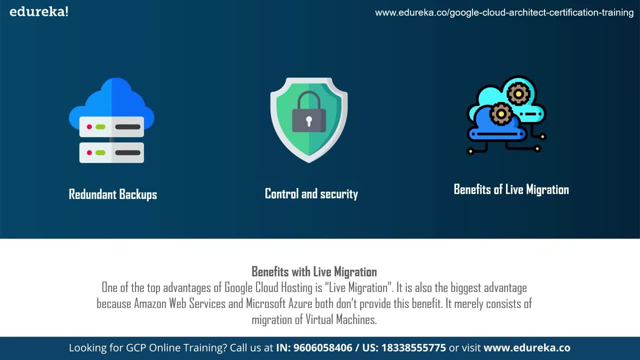 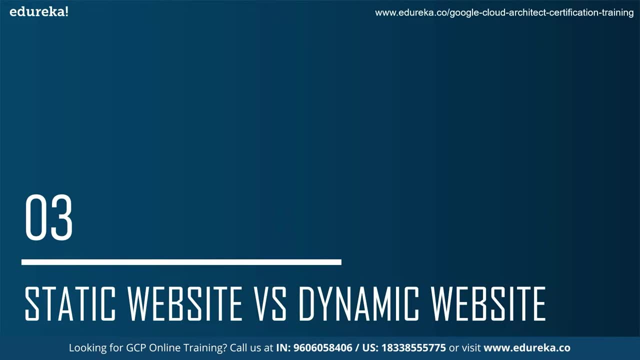 migration of virtual machines. when it comes to AWS, next up, we talk about static website versus dynamic website. so when we talk about hosting in cloud, that is basically cloud hosting, which is one of the various kinds of hosting available, such as VPS hosting as well. so, when it comes to cloud hosting, there are 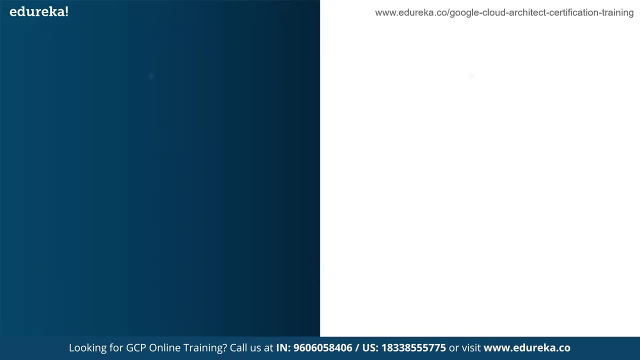 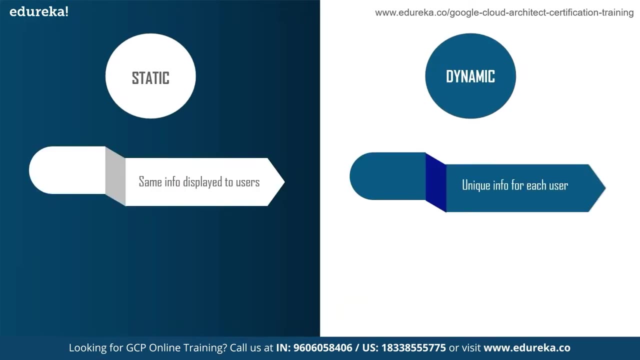 two kinds of websites that can be hosted, right? so one of the websites is a static website and the other is a dynamic website. so when it comes to a static website, it is basically the same info displayed to every user that is there, while a dynamic website will be unique for each user, for example, your Gmail. 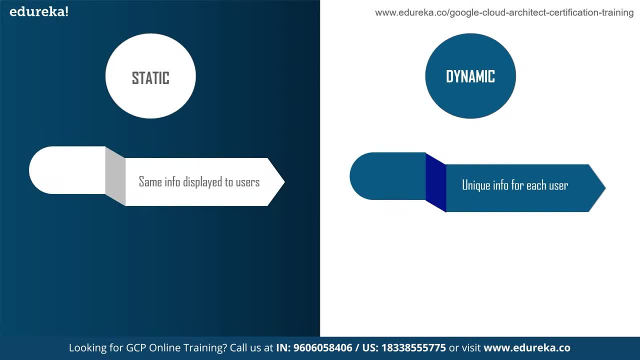 login page and your Gmail home page will be different for every user because it's customized to you and you can customize it as well, whereas a basic HTML hello world page will be the same for everybody, and that is an example of a static web page. next up, we talk about the fact that static web page does not. 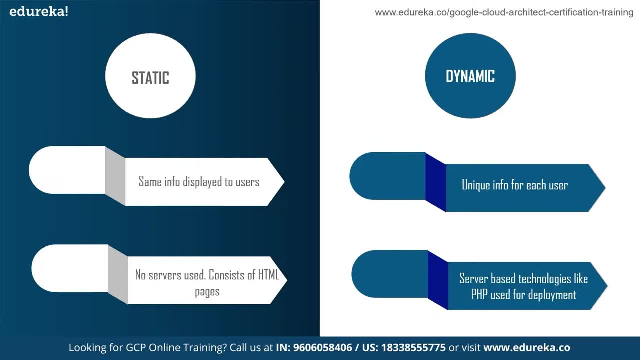 have. any servers that are in cloud are used right, so it consists of basic html pages which can be stored in buckets, and these buckets can then be hosted on google cloud using the endpoints, right, whereas dynamic websites need server-based technologies like php, and that is basically something that is necessary for. 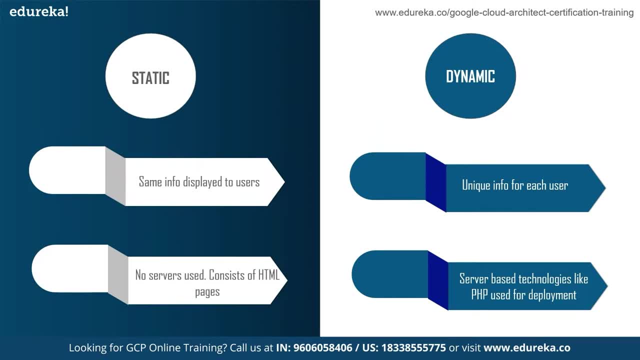 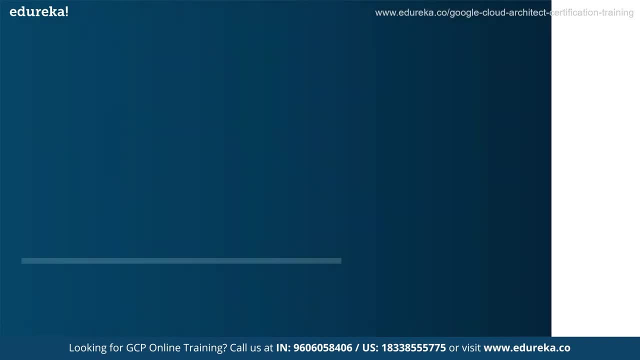 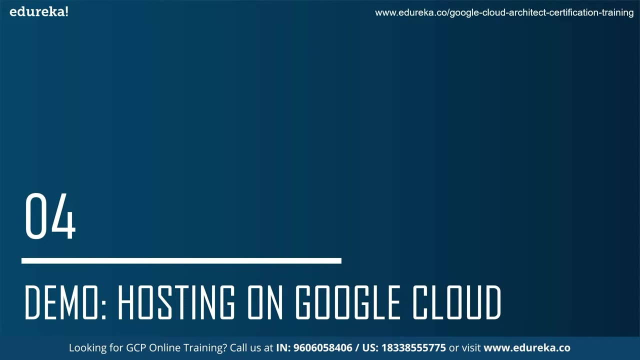 deployment: web apps are used for the deployment of dynamic websites, so these are the two different kinds of websites that are present. when it comes to hosting, next up, we have a demo on basically how to host a static and a dynamic website on google platform. so once you've basically logged, 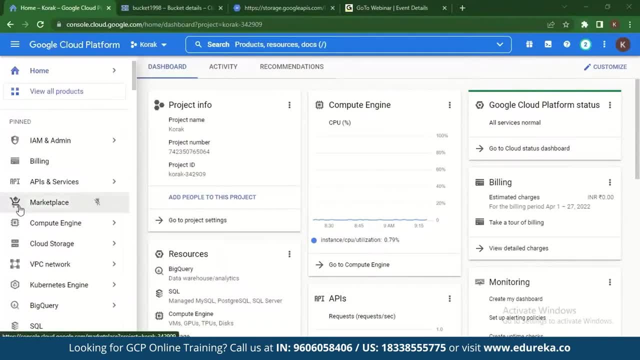 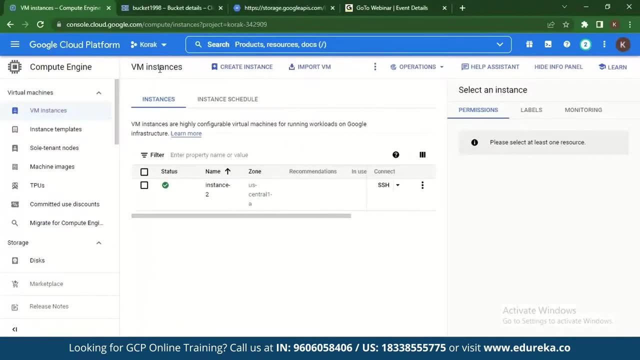 into your google cloud platform console. you can go to compute engine and go to vm instances. we're going to basically talk about how to host a dynamic website on google platform, so the first thing you need to do for this is create your own project and in that project you'll have to go to compute engine. 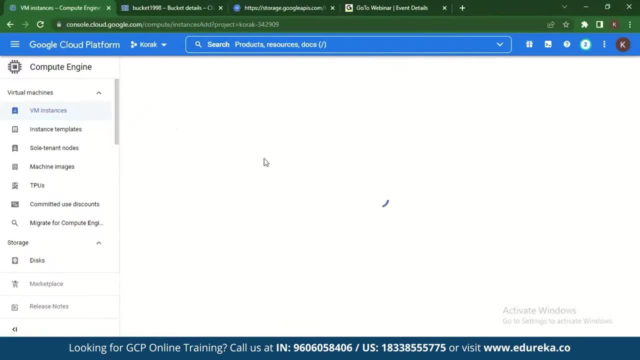 and then create an instance. make sure that you have a service account as well, but in this demo we'll be using the default service account. that's there. so let's get started. so let's see, there's an instance name here and it's named as instance 3. 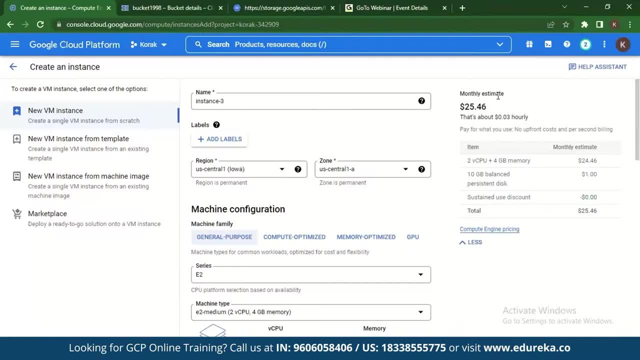 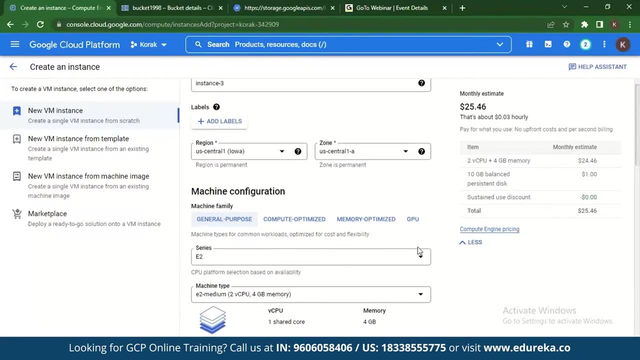 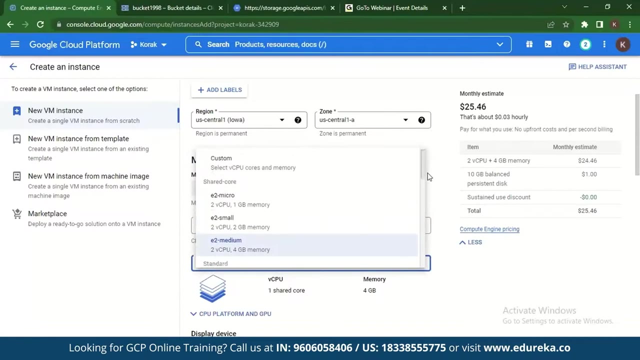 so we can keep that as is. and on the right hand side you can see that the pricing for the estimate pricing for our machine is given right. so the pricing depends on the amount of resources you use, the kind of machines you use, and what you have to do here is just get it, change it to. 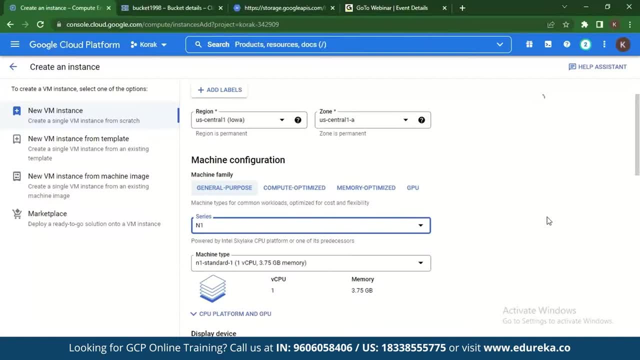 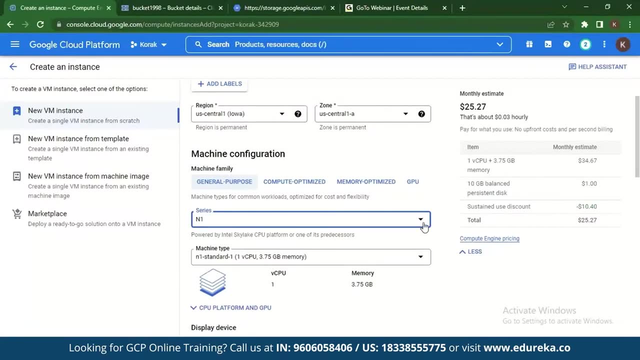 n1. so when you change it to n1, you can see that the price has just reduced or it's the same, because you don't need a lot of users to be logging into your instance right now. it's just you, so you'll be the one logging in, so you don't need a very powerful. 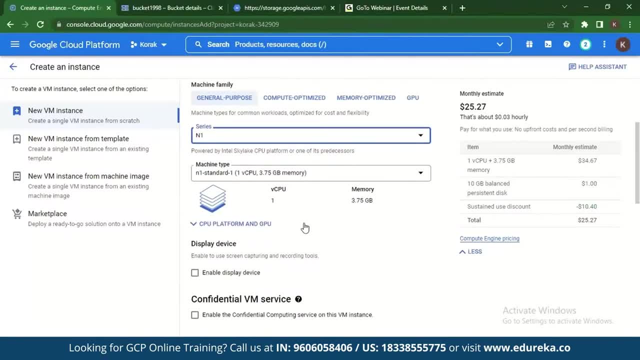 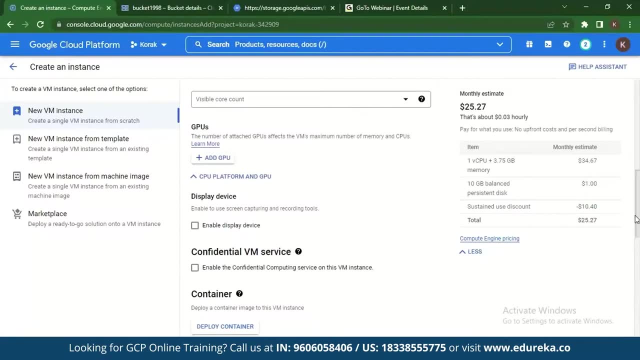 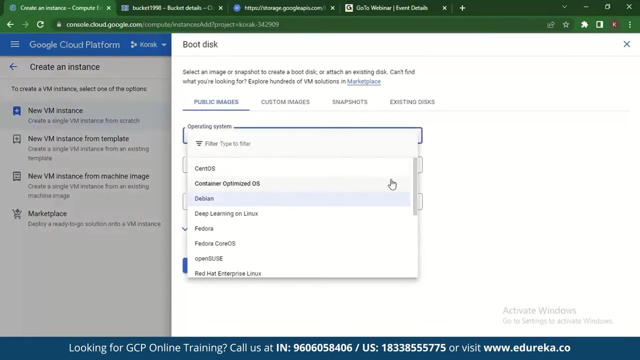 machine that's n1, and what you have to do here is the platform gp, configure all this, it's done and come here and change the boot disk. now you can keep it as you wish. you can keep it as devian as well, if you want. i'll be keeping it 2.2. 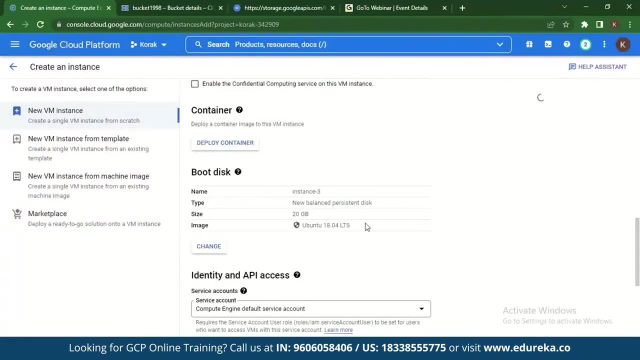 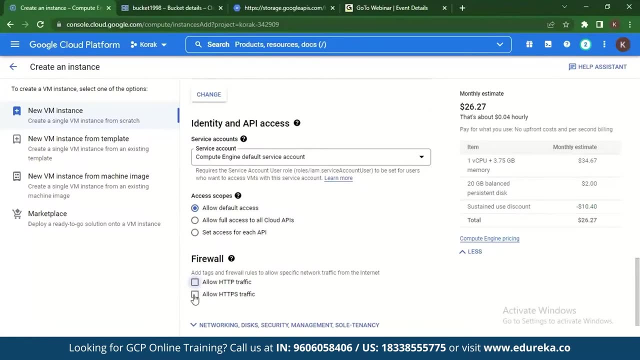 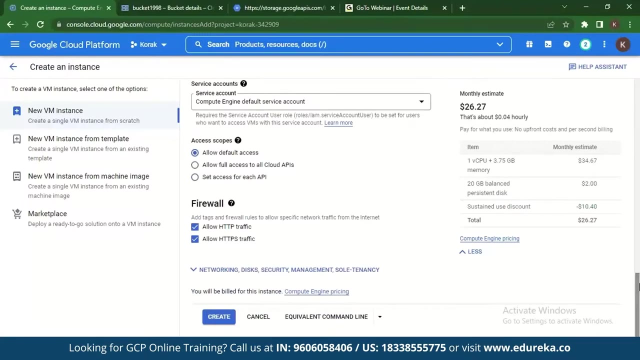 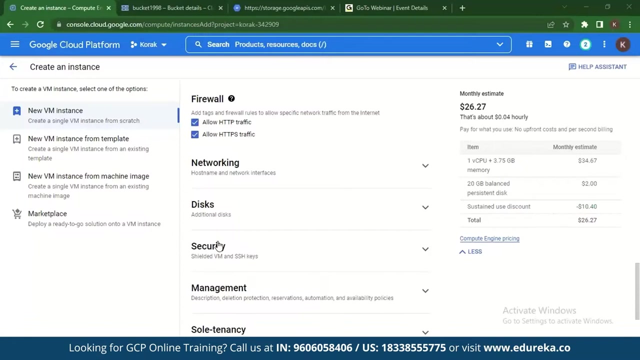 to 20 gb. that is changing my boot disk- and after that you'll have to allow http and https traffic, because you need public access for your website. so when you basically go onto the internet, you want your website to be shown right. so after this, what you have to do is basically go to security, and here what you have to do is manage. 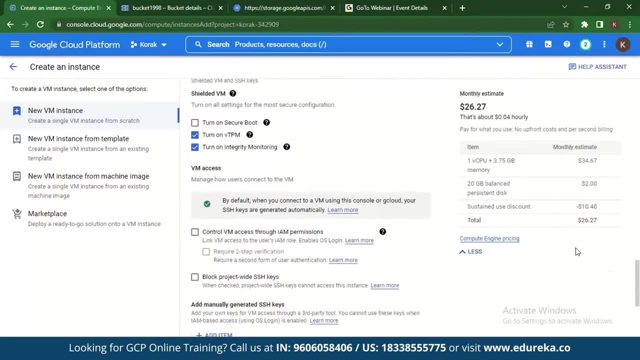 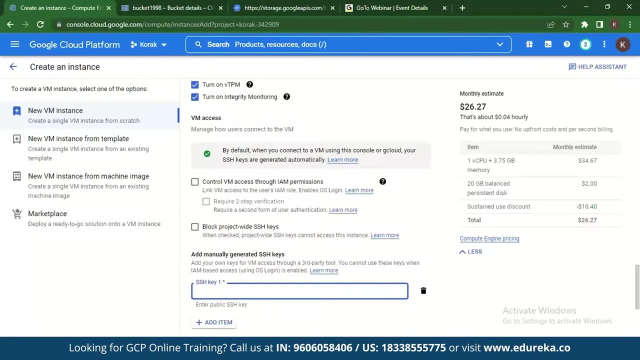 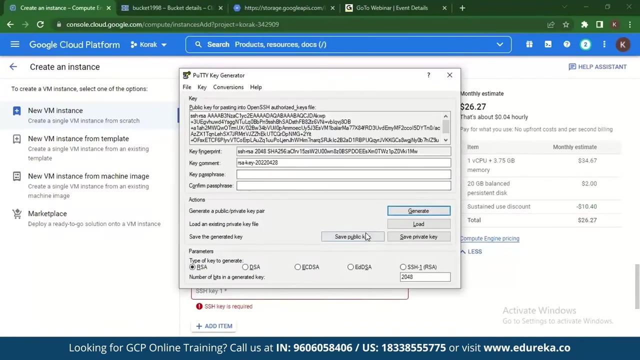 your access for the vm right. so for this, what we need to do is create a public key, and you'll have to add the public key separately, and for that we'll be using puttygen. generate your key, save it as private key, right, so you'll have to make a passphrase. 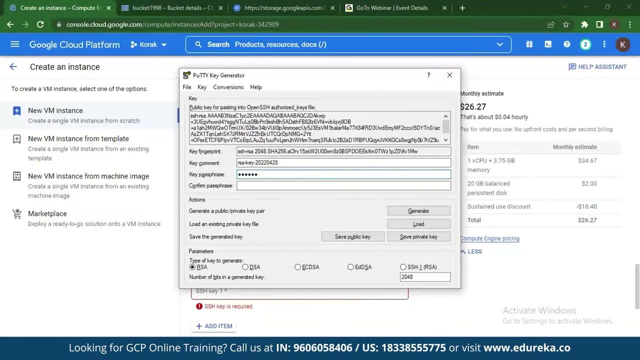 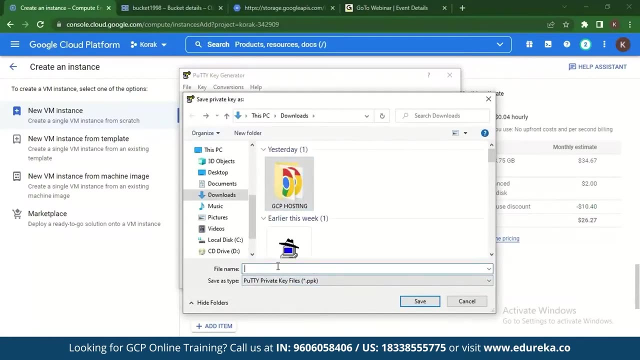 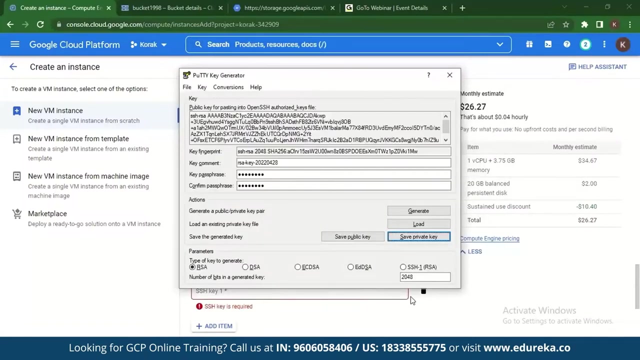 and that passphrase is for basic authentication and improving the security right. so you can keep this passphrase whatever you want to and save it as a private key. so let's just name this private and dot ppk. save that and after this what you need to do is load this. 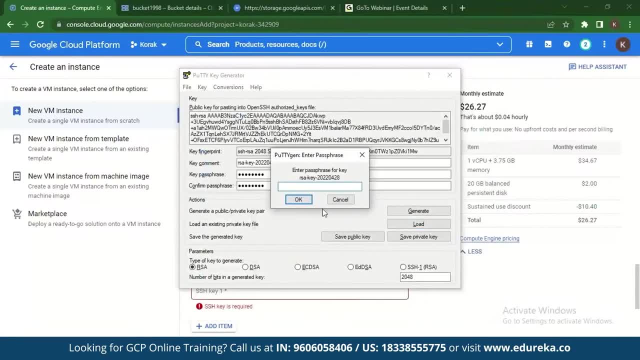 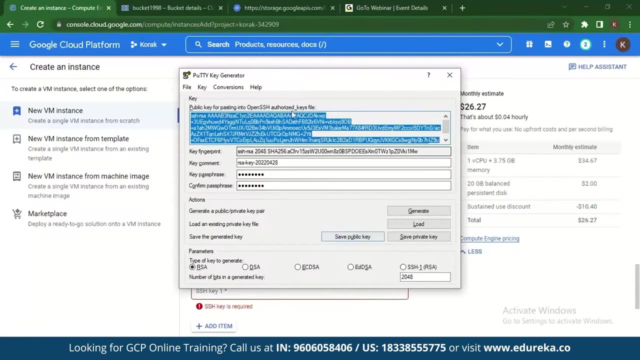 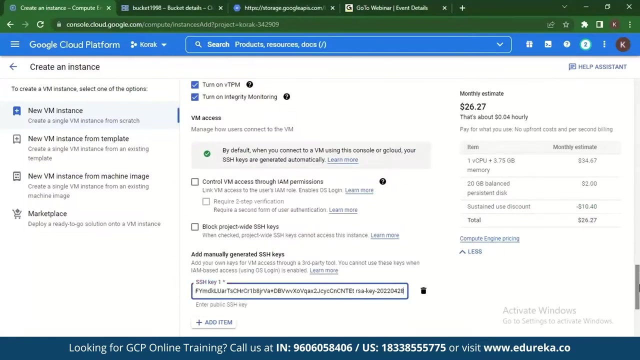 go to privateppk it and open this up. open up your with your passphrase and you'll have your public key that you can copy. you can just copy this and we can now go back here and paste this here and after this just create the instance. then you can just admissions. 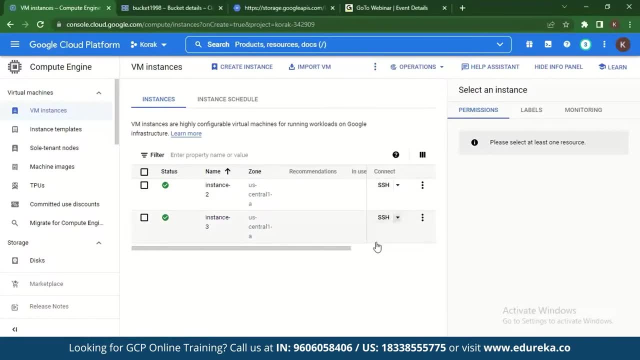 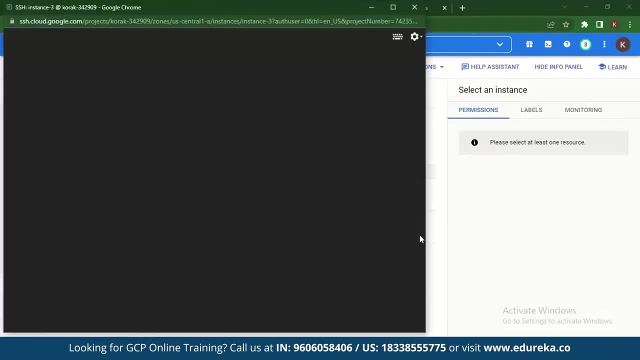 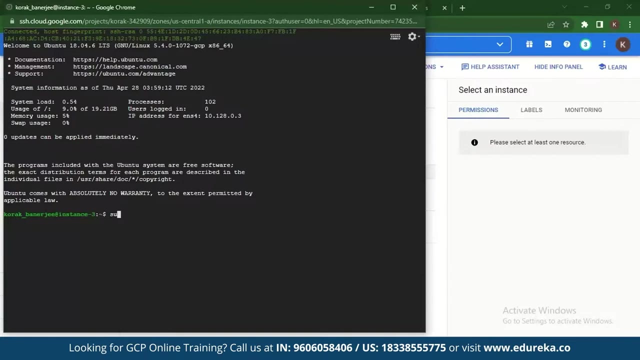 right. so your instance is now created. what you need to do now is connect to the ssh and open it, upplant the window. once connection to your ssh has been established, type in sudo su and you can just CD and just type apt-get- right. so this is what you have to write and you can see your Apache 2 is being. 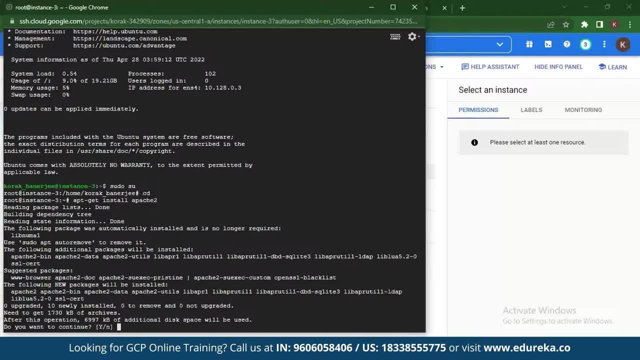 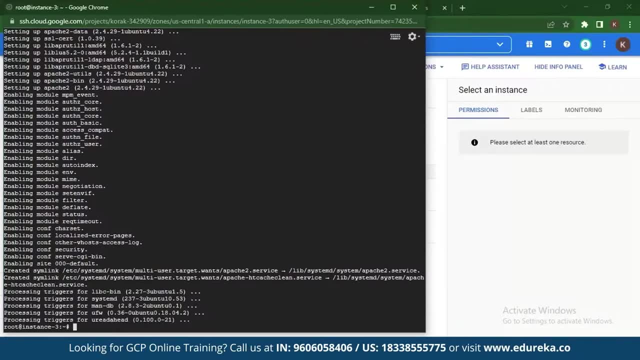 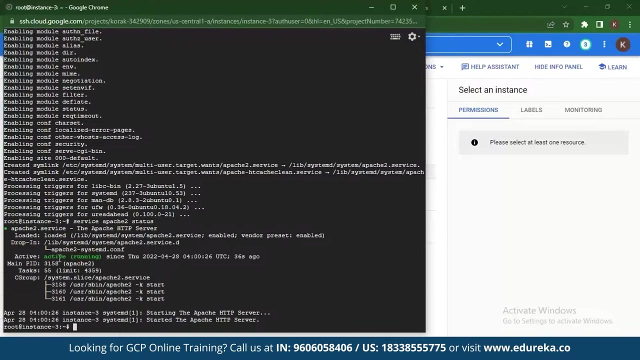 installed- now Apache 2 is basically going to be the server- and just type in y, right, so this is now done. so what we can do is just check if our Apache is running, so that we just have to do this. as you can see, basically this is running. so basically what you have to do now is 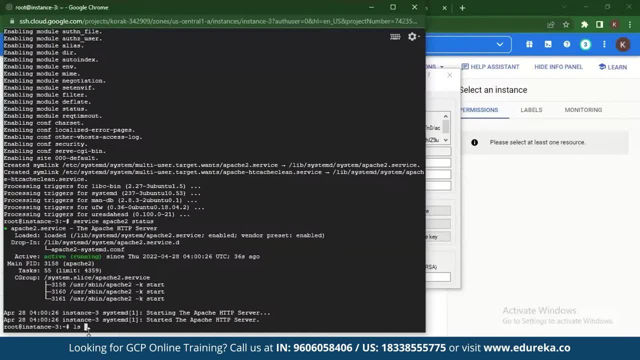 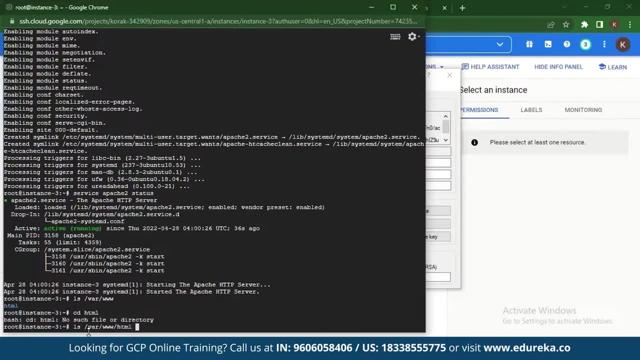 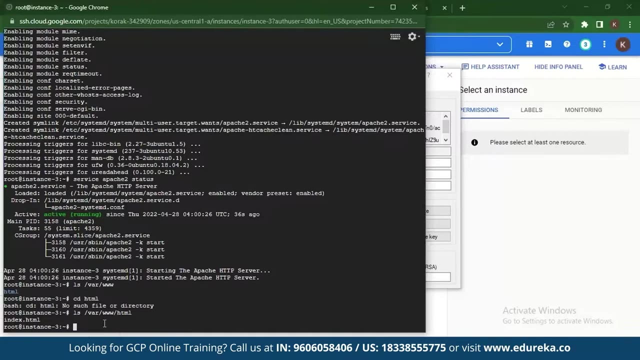 go back in here- I've been- and s and then add HTML here to go into the directory. you can see there's an index dot HTML page. now, when we talk about the index dot HTML page, what we have done here is the index dot HTML page is supposed to be the Apache server page. 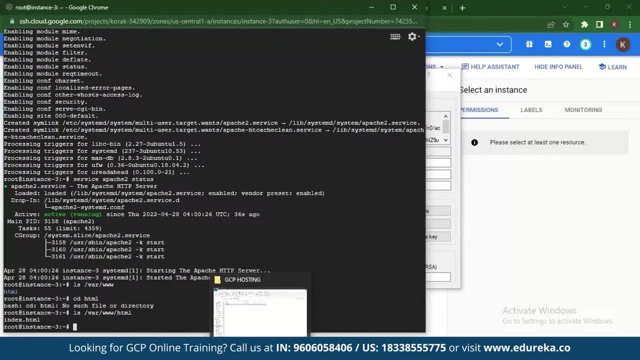 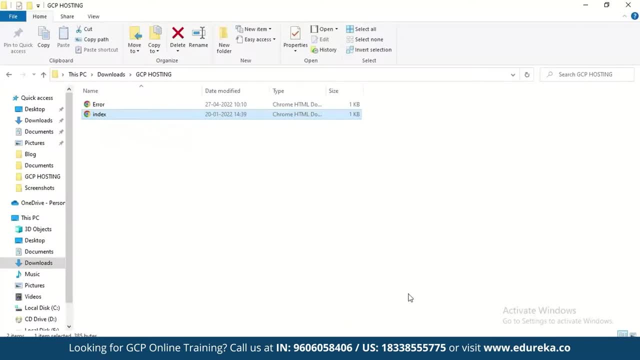 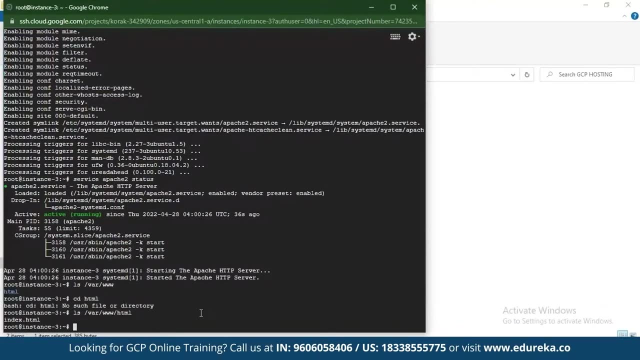 but we need to host our own website, right? or our own dynamic website. so what we've done here is had our own index dot HTML web page which is going to replace the apache server web page, right? so let's try that out. go into LS, let you backslash. 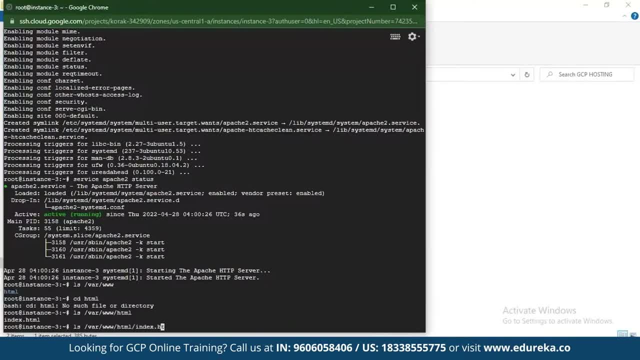 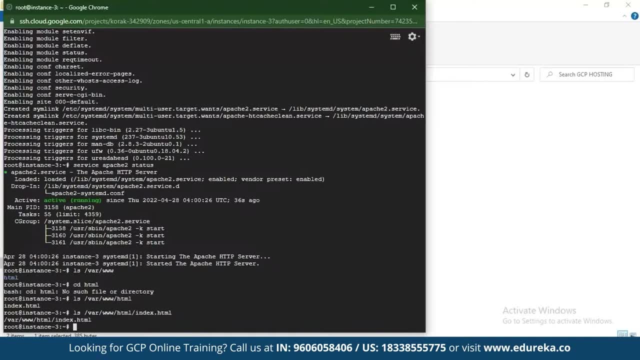 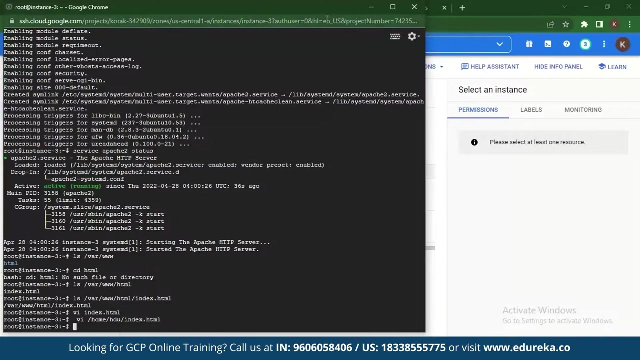 and index right. so now you're in here and basically what you have to do after this is: I index dot end. you know the index dot HTML page. you take this code in and you change it in the index dot HTML, and let's now go back and copy this. and when you're done, 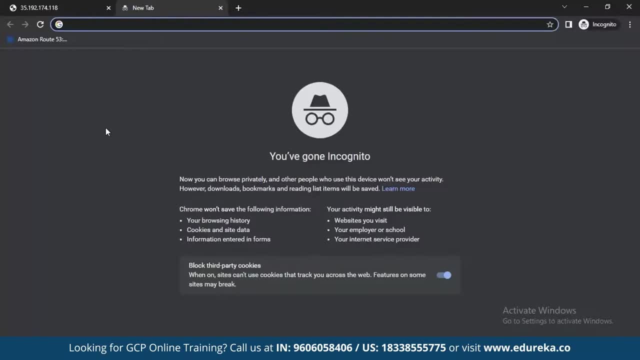 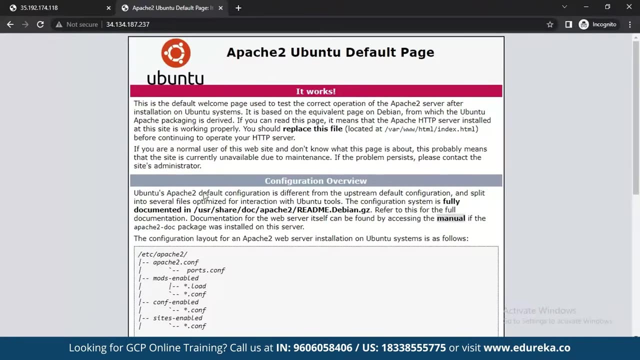 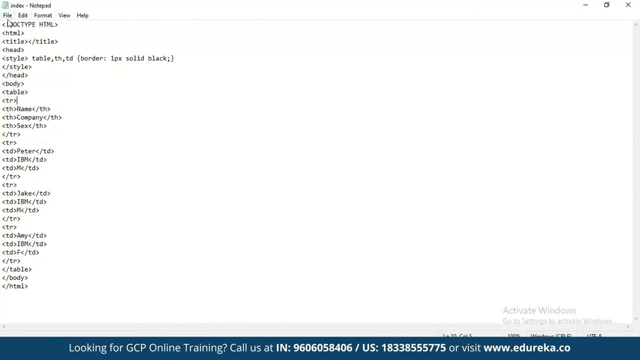 copy. just go back to your incognito what you can see- a partially server default page, right? so you can see that this page has bit and it's running. what you need to do is change this. this is your code. this is the web page with which you will change this page, right? so basically what you 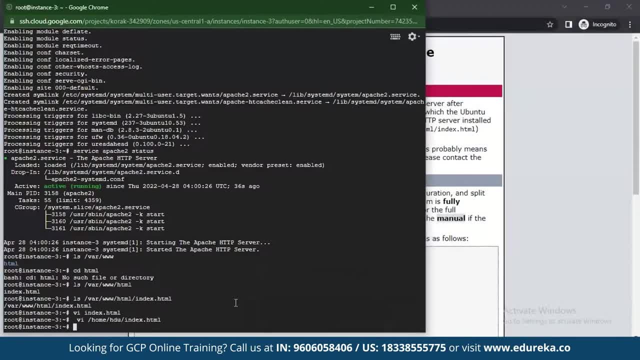 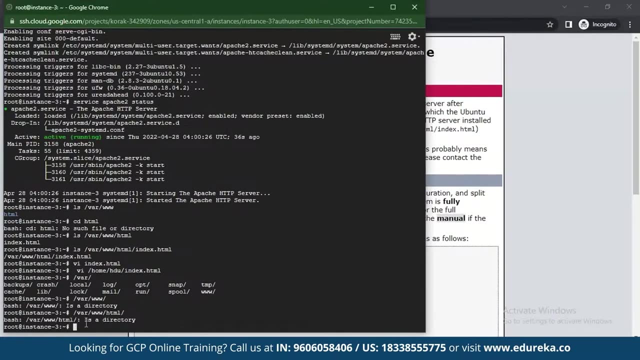 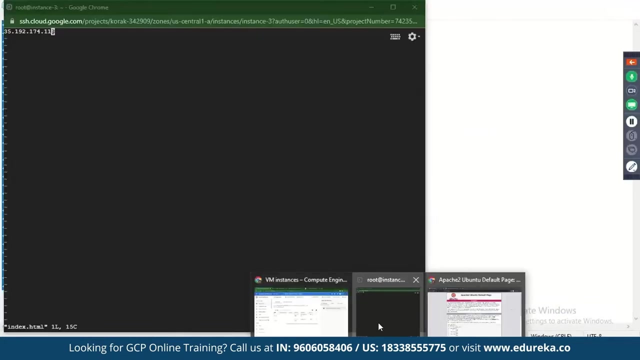 have to do is go back into your SSH and into your index dot HTML, which is basically just right. so just go back to. so basically, you can see that HTML is already a directory, right? so you just have to VI into the index dot HTML, right? take your code here, copy it and add in here. so right now you have your code and 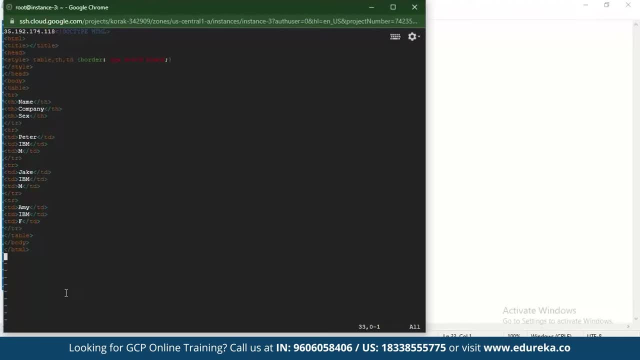 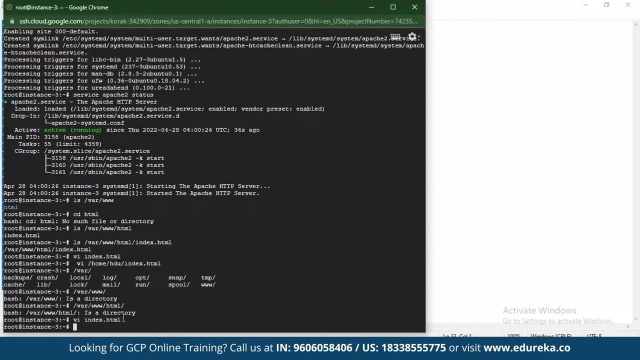 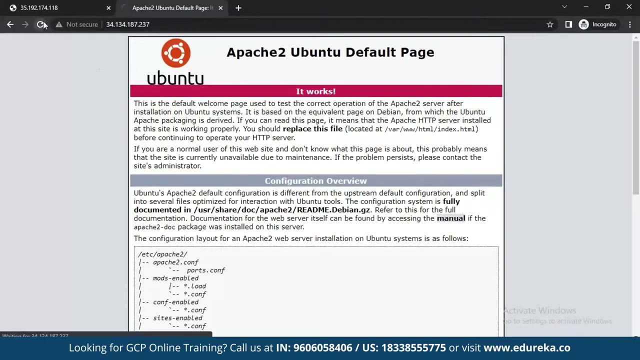 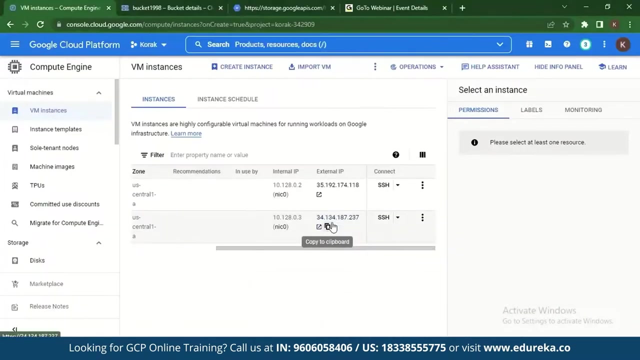 it's changed from the original code to the new code and it's changed from the Apache page to your very own that page, right? so you can basically go back using the command column wq. so now, when you refresh this, let's just try refreshing this. it's still the same and let's go back. why, right? so copy this up. 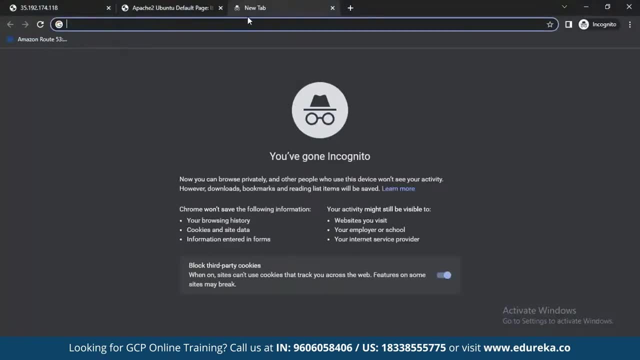 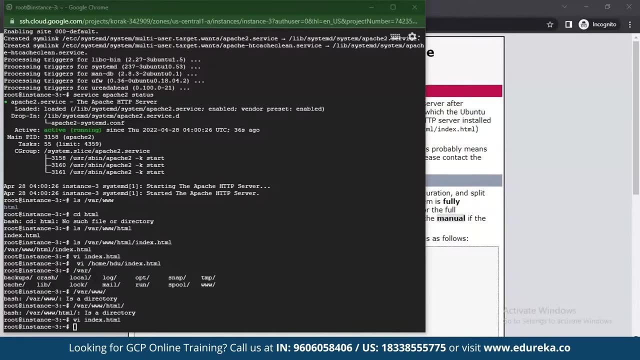 yes, this add it go back to�� MERRY CHRISTMAS, and so what you have to do here is starting from change the html code. so now that you've changed the html code, what you need to do is move it in somewhere else. let's try this: mv. index dot html. 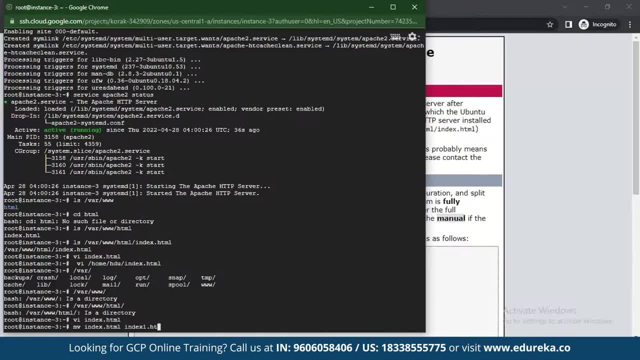 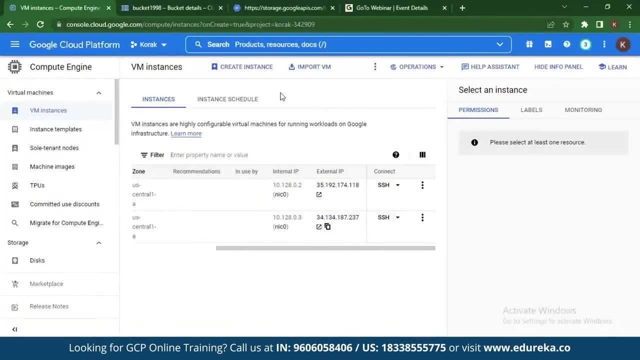 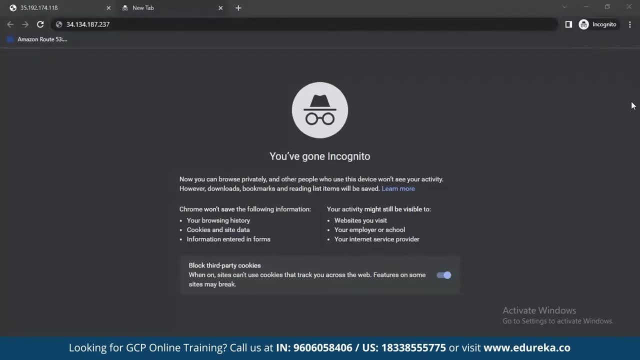 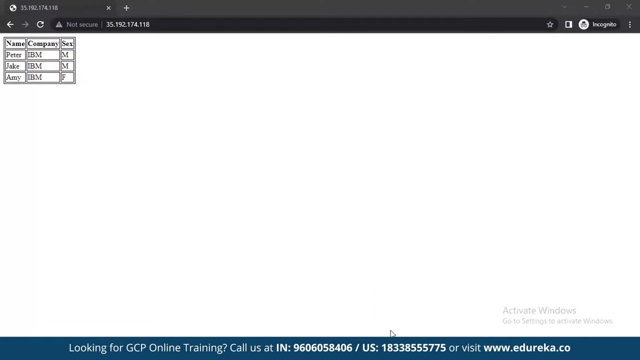 index one html. so now let's try it out. go back here. this and this is this, and basically what you'll see is that you have your own web page in here, which you've replaced with the apache web page, and that is because you went into the ssh. 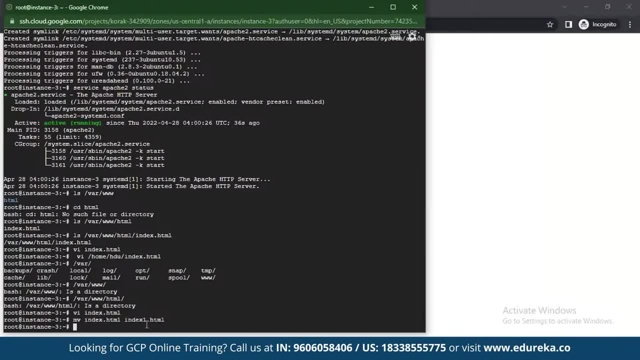 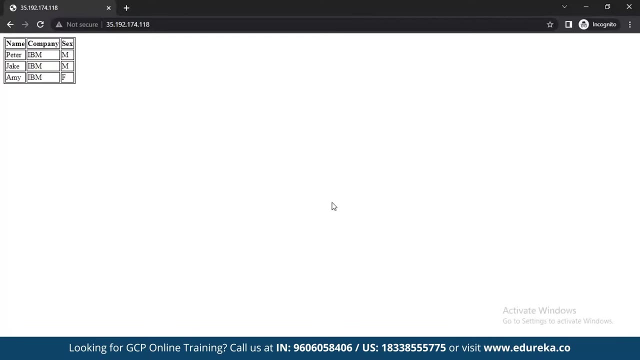 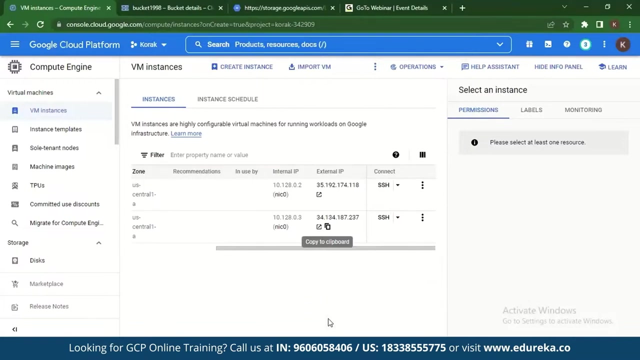 changed the code in indexhtml and moved it from index to index one dot html. so that is basically how you host a dynamic website using servers and vms on google cloud platform. there's another way you can host dynamic websites on google cloud platform, but that is through app engine, if you would like. 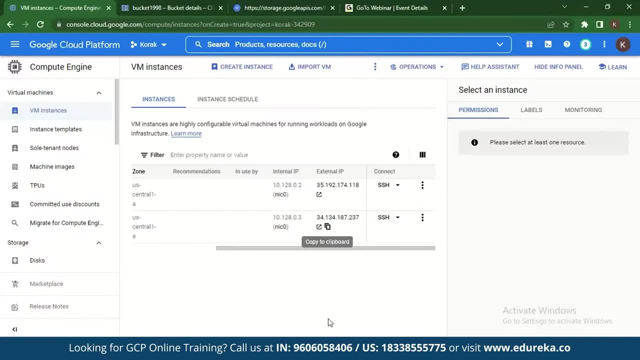 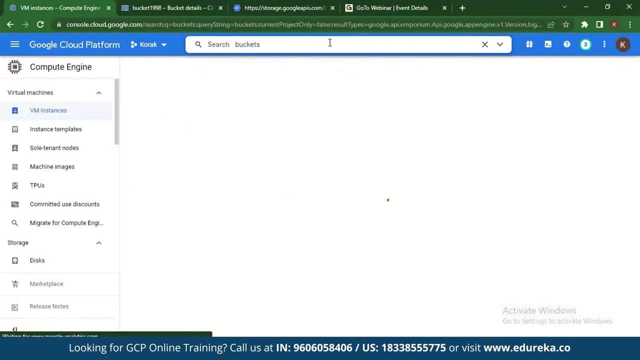 us to make a video on google cloud app engine. please do let us know in the comments below. and now let's go back and check out what it's like to host a static website, right? so when you create a static website, you need buckets and what you need to do is just go to cloud storage. 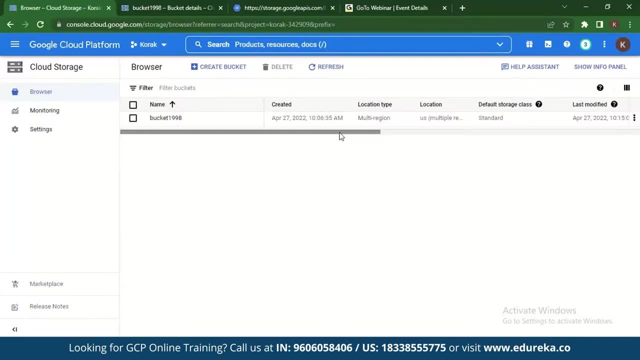 so, when you're talking about hosting a static web page, you basically need only a storage service, because you're going to basically get the html code in these storage buckets and these buckets have then got a url which are publicly accessible and you'll have hosted a static web page. so let's. 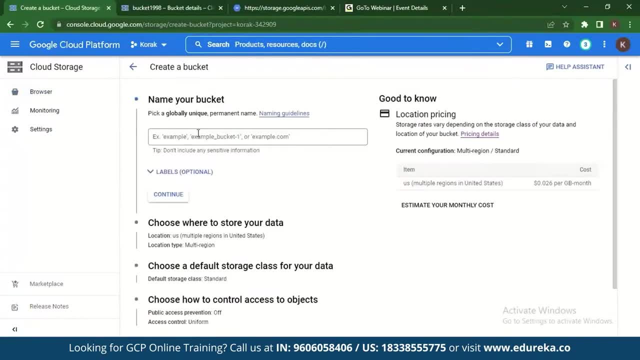 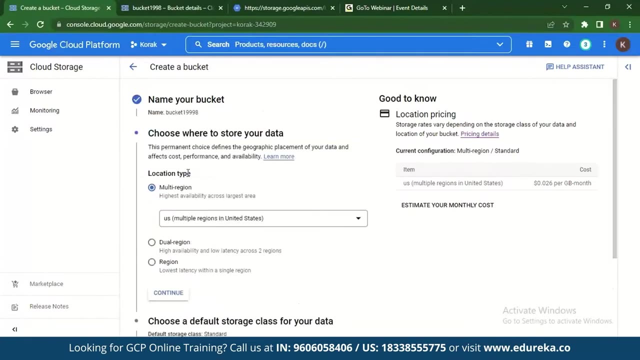 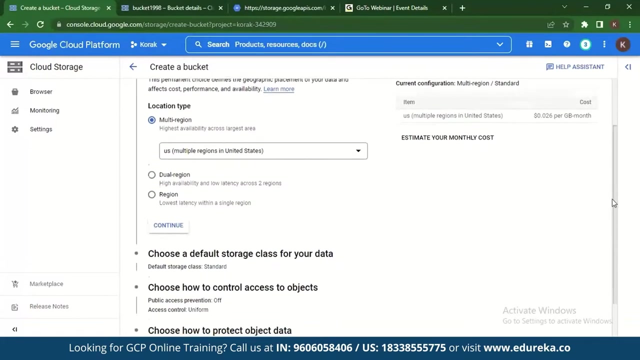 start it. we'll try and create a bucket sign, name it anything we want. let's say bucket 997. right, continue. okay, so this is taken. so let's try this out. right, so we want it to be multi-regional because it will be publicly accessible. right, so this is going to be multi-regional and us multiple. 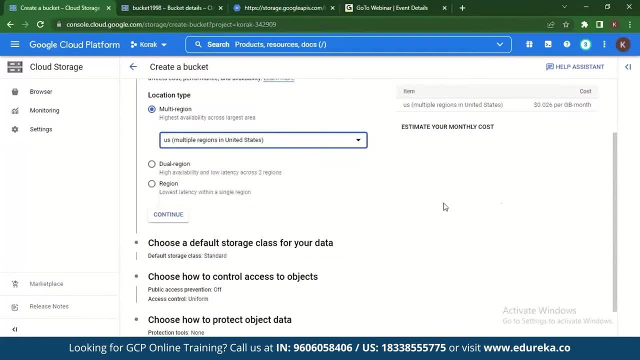 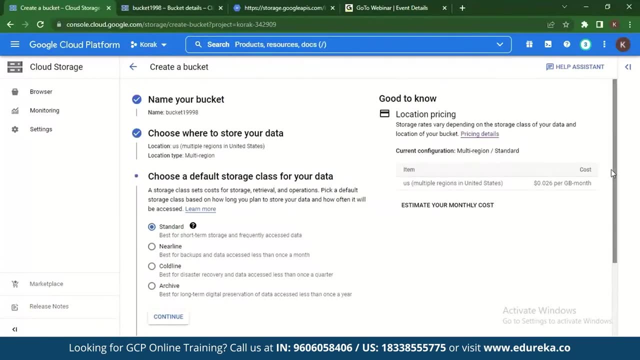 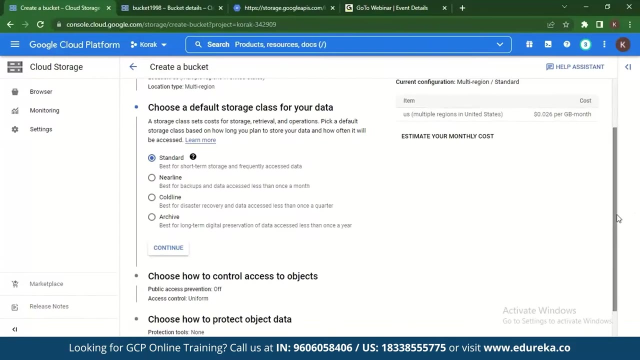 regions in the united states. right, so you can change it to europe if you want. next, go to continue again. you get to choose your default storage class for your data, and these are divided into standard, nearline code line and archive, standard being the most short term and archiving the most long term. and then let's go to continue so. 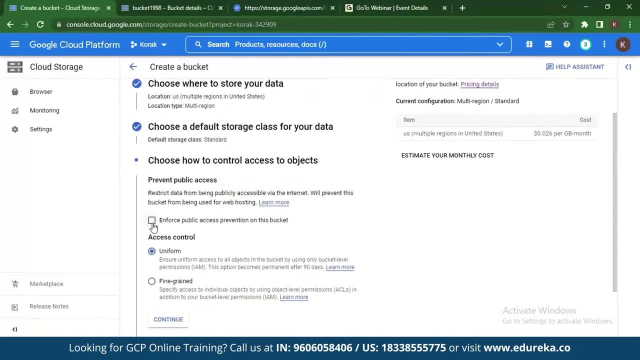 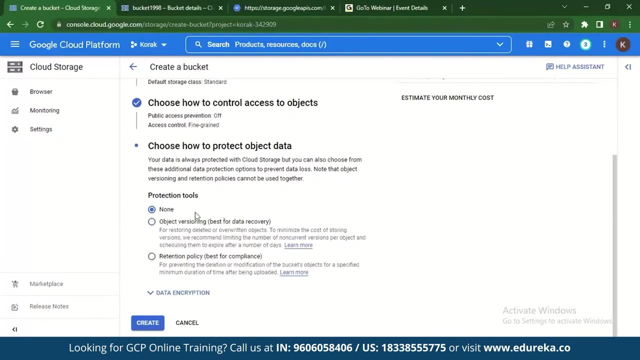 what we want to do here is: we don't want to prevent public access, right, so we will not take on this. what we'll do is give it to fine grain. uh, as we're not going to do that, we'll just choose the static where we have ACL permissions and go to continue, and what we do here is have. 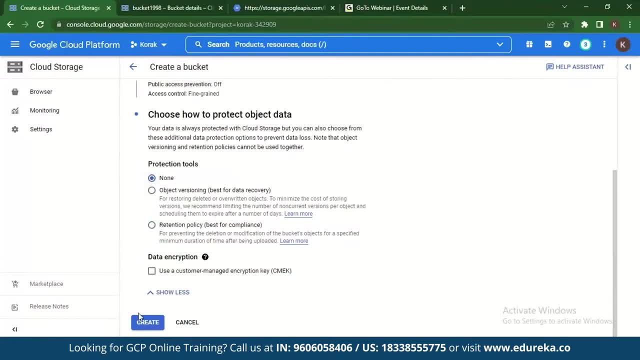 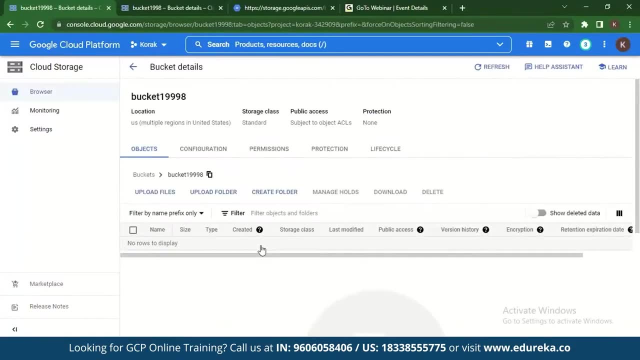 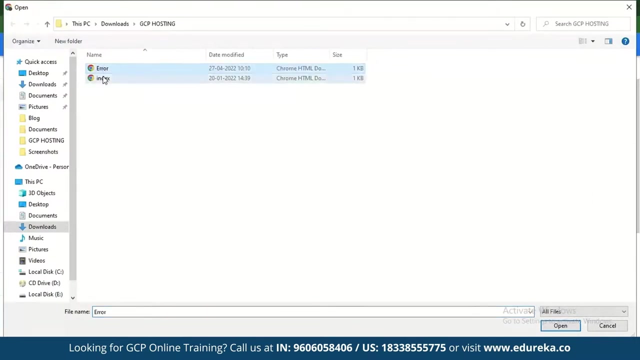 none of the protection tools. but we have none of the protection tools and right after that, we basically create a bucket. right, so a bucket is created. now what we need to do is upload our HTML pages in the bucket. on this bucket. let's do this. there's an error file I have and there's an indexhtml file I have. let's. 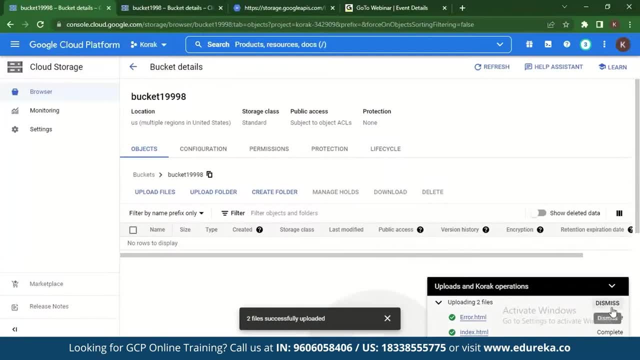 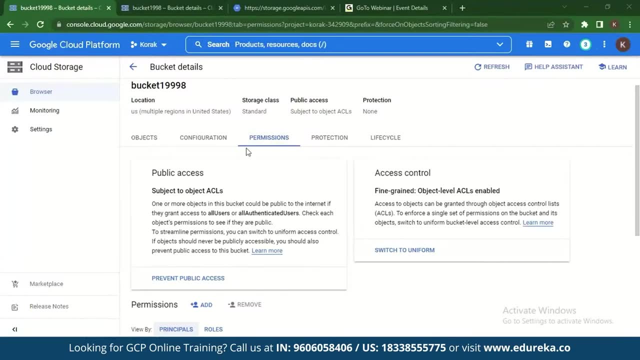 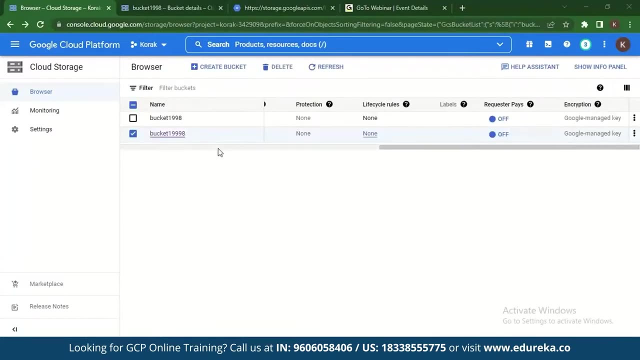 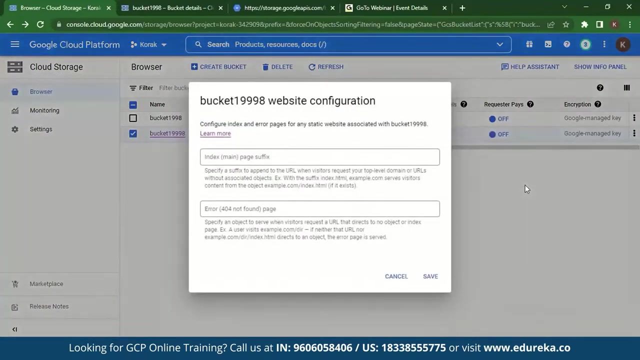 upload both of these. so we've uploaded both these files. so basically what we have to do now, after we've created the bucket, is change its permissions and allow public access. so once you basically made the bucket, you have to change the configurations, that is, basically edit website configuration and you have to add your 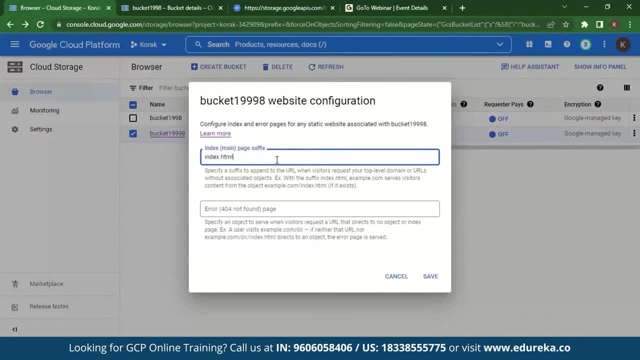 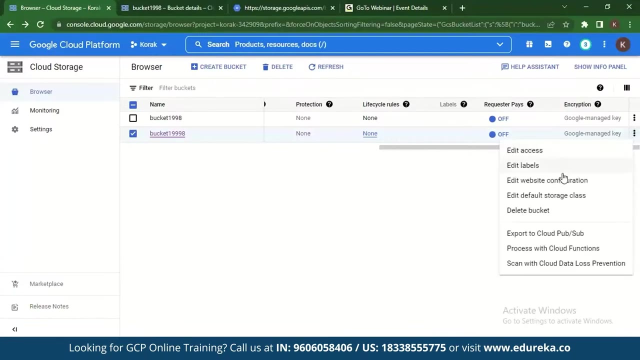 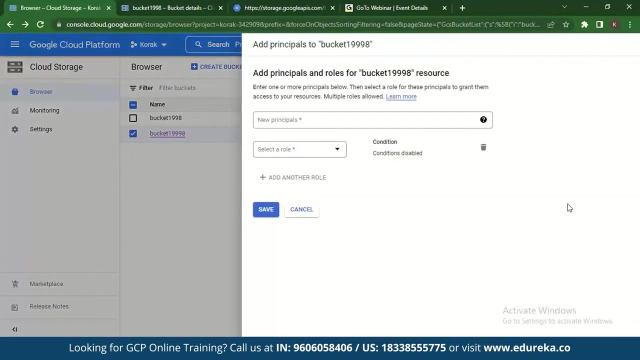 indexhtml and errorhtml and save it right. so, right after you've done that, what last thing you need to do is you have to create a bucket and you have to edit the access. now, when you're editing the access, you need to. public access is subject to a CLS. now what we have to do is add a new principle, and here we'll. 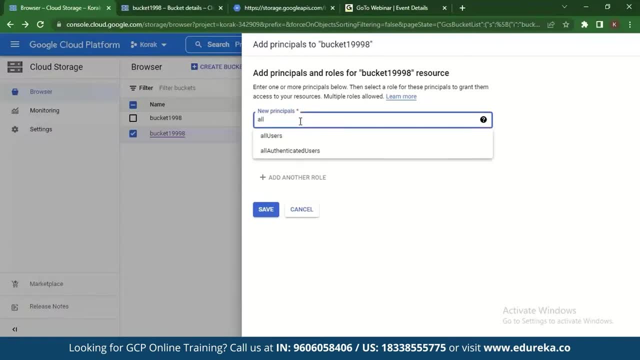 have to select all users right, and here too, here we'll have to select a role which is the object view storage object is equal to the company name of the project. it is an item called a public access. which is the object view storage object is equal to the company name of the project. it is an item called a public access. 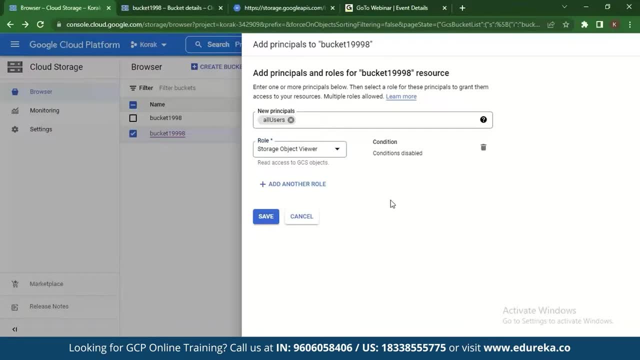 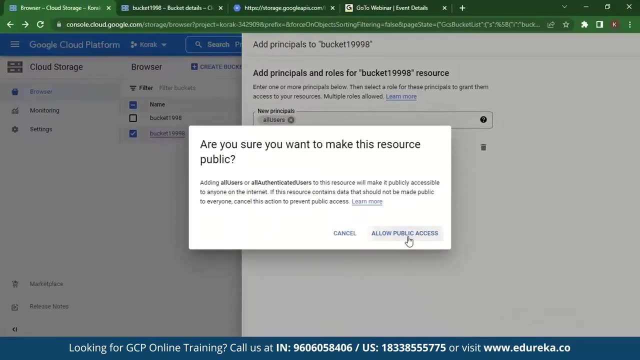 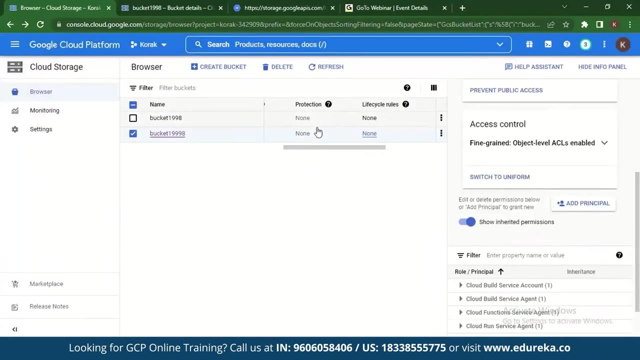 viewer, which basically gives you the view access to the website only, and you have to save that. so, basically, this is asking if you want to make it public. so we just have to update this. and now a bucket has public access. let's just check. right, so there is public access to the internet, right? so now that we have 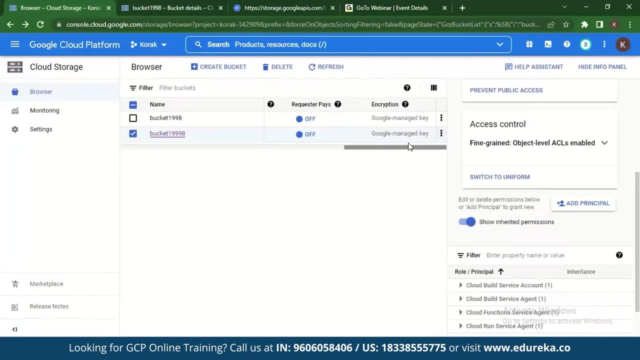 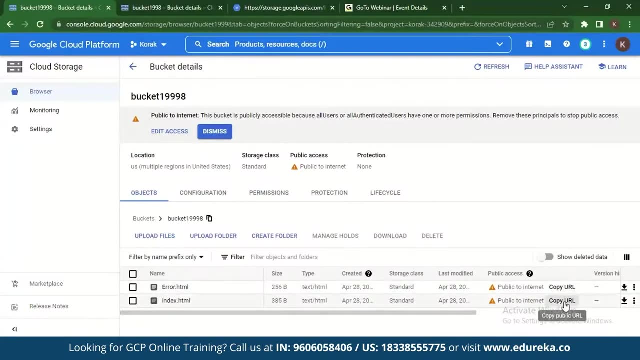 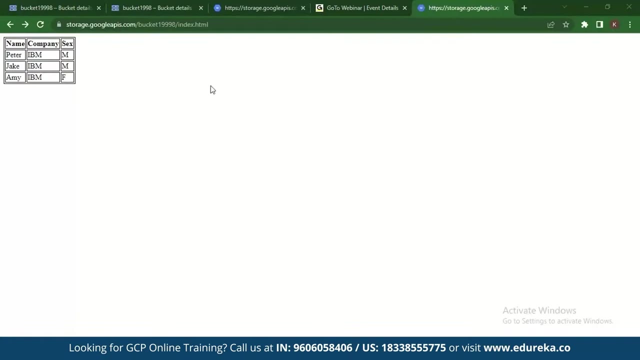 public access to the internet. let's just go check out our URL, so enter your bucket, copy the URL and paste it in here, so, as you can see, our indexhtml page has been posted on this endpoint, which is basically googleapiscom, with this bucket name: indexhtml, and that is how you host a. 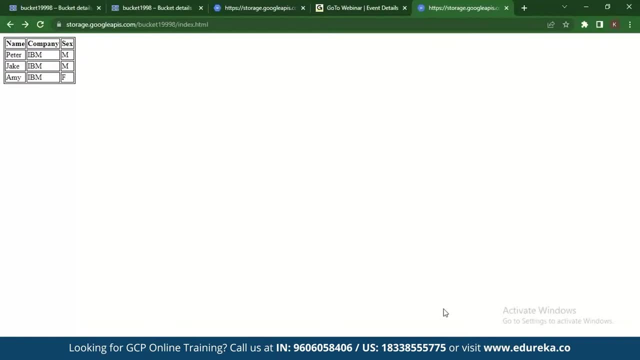 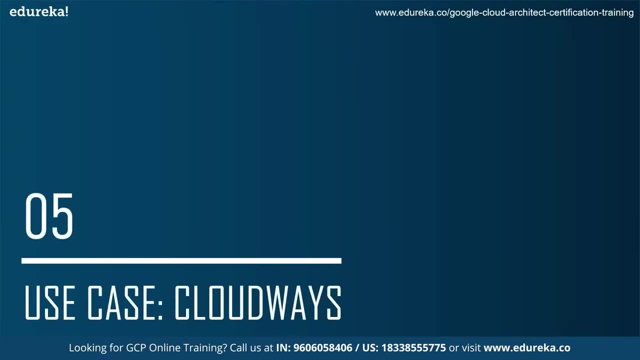 status website on google cloud platform. so we've seen how to host a static website and we've seen how to host a dynamic website. so the last thing we talk about is the use case. so, when it comes to the use case we talk about, we're going to 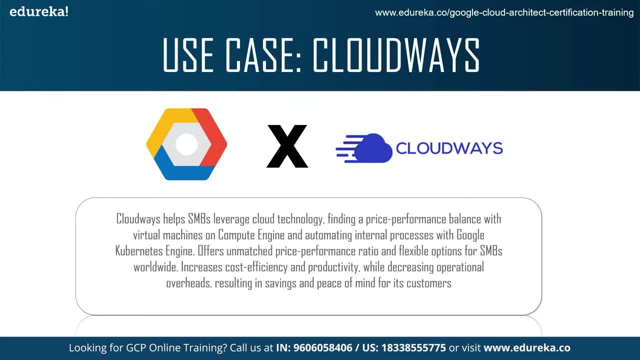 talk about one very popular use case, which is the cloudways use case. so cloudways is basically in partnership with google cloud platform and what happened is the price performance balance for the virtual cloud is basically in partnership with google cloud machines. cloud computing engines, automatic compute engines, are repeat. 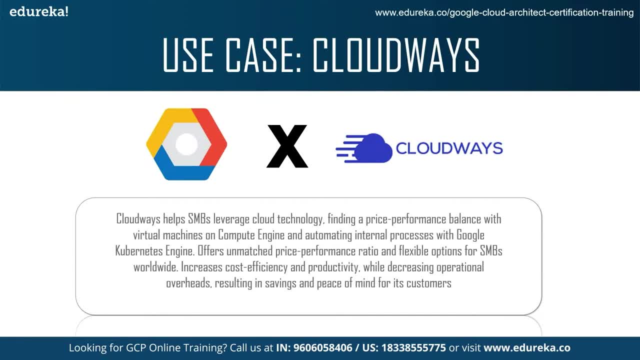 automating compute engines, internal processes. so cloudways, in collaboration with GCP, has improved, in fact, a lot of Google cloud platforms already existing services, such as the kubernetes engine, the compute engine and other such performance ratios, and this basically increases a lot of cost, efficiency and productivity. right, so this is how hosting using a cloud google platform has 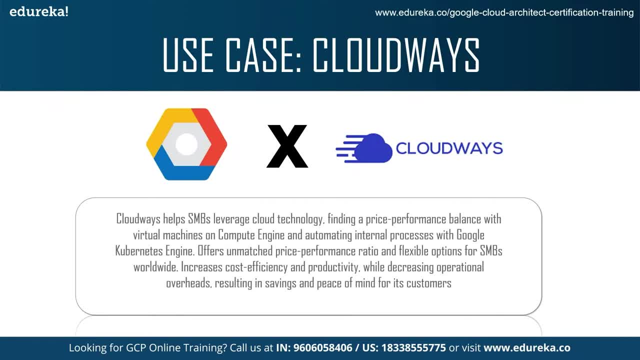 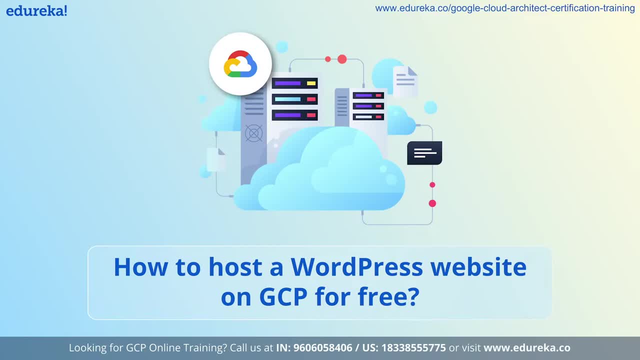 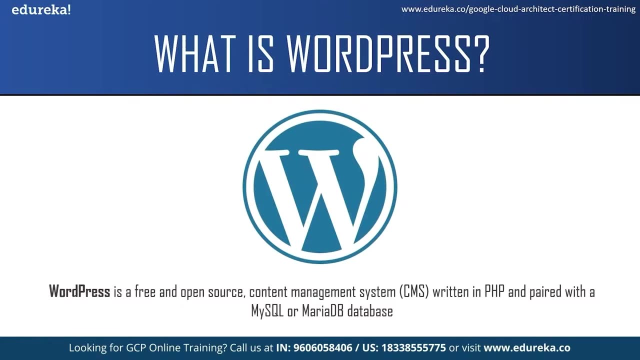 made cloudways much more scalable and cost effective. what is wordpress? wordpress is a web publishing software you can use to create a website or a blog. technically, it could be defined as a free and open source content managing system written in php and paired with mysql of maria db database. it can be used to not only create 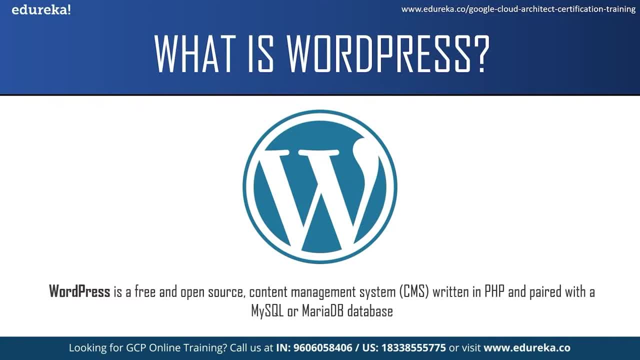 blogs and website, but can also be used to create directory, forums, galleries, business website, online e-commerce website and many more. it is the most popular website building platform in the world. just to give you an idea about how popular wordpress is, wordpress powers about 35 percent of all internet websites. bloggers, small businesses and fortune 500 companies use wordpress. 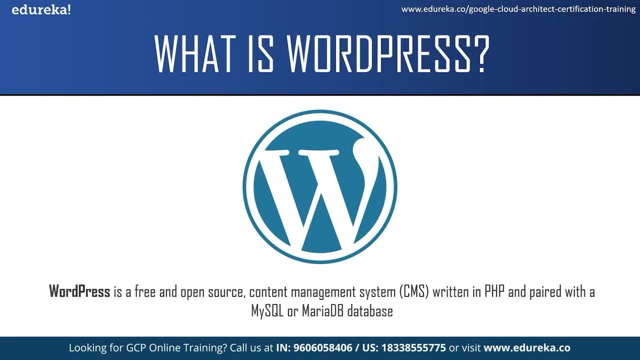 then all your options combined. now you do not need any coding knowledge to use wordpress. it enables you to build and manage your own full featured website only by using your web browsers. now, what makes wordpress so famous? to answer this, let us look at some of its features. the first: 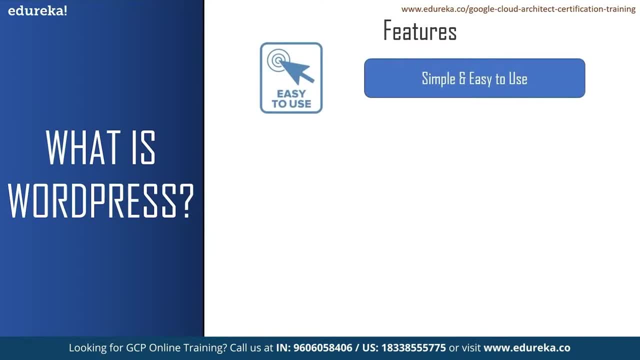 feature is it is simple and easy to use. creating content with wordpress is as simple as creating and using ms word document. you can create posts and pages, format them easily, insert media and with your content is live and on the web. and also wordpress is available in more than 70 languages. 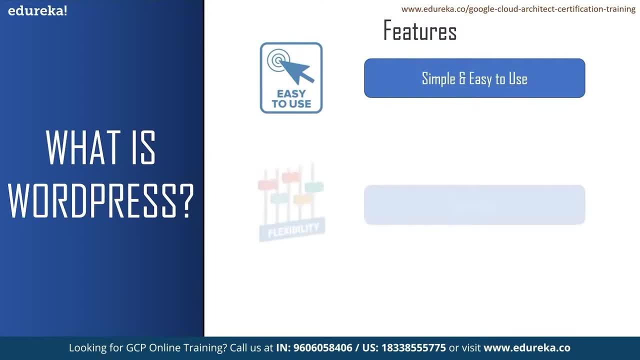 so you can choose and create content with the language you're most comfortable with. the next feature is it is flexible. now, with wordpress, you can create various types of website, like a personal blog, a website, a photo blog, a business website, a professional portfolio, a government website, a magazine, a new website, an online community and many more. you can make your 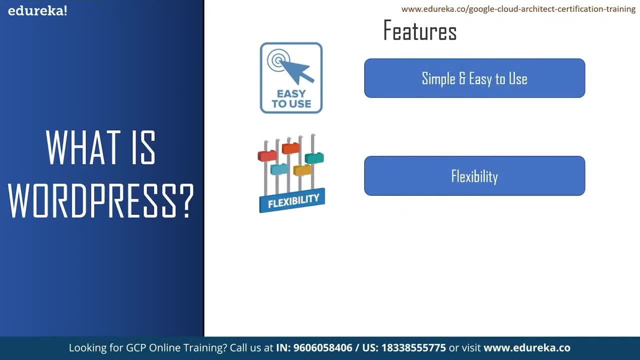 own content using themes and extend it with plugins. with wordpress, you can also build your very own applications. the next feature is user management. wordpress uses a concept of roles, which are designed to give the site owner the ability to control what users can and cannot do within the 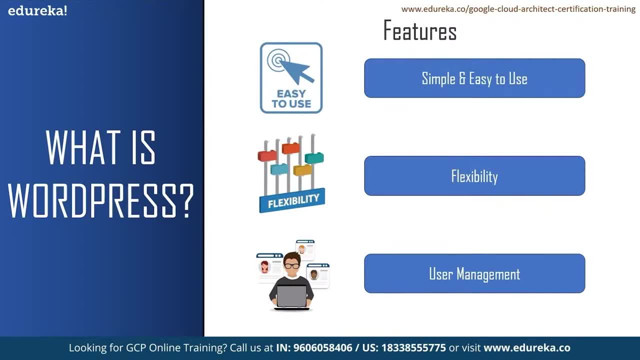 site. the site owner can assign different roles to different set of users. generally, wordpress has six predefined roles: the super admin, administrator, editor, author, contributor and subscriber. the super admin role allows a user to perform all possible capabilities or functions. the administrator manages the site. editor works with the content. author and contributor write the. 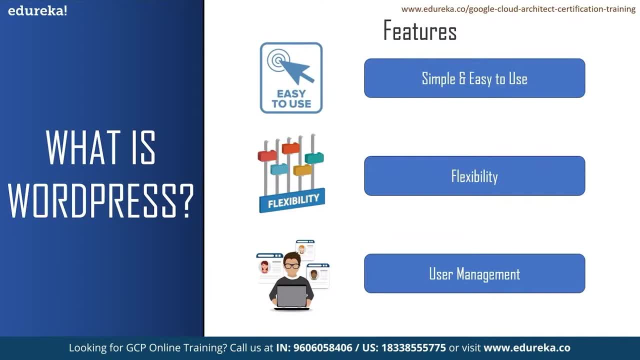 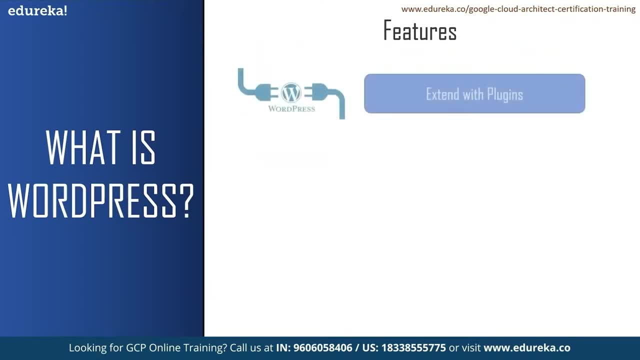 content and subscriber has only the read capabilities. this lets you have a variety of contributor to your website and let others simply be a part of your community. the next feature is you can extend it with plugins. wordpress comes packed with a lot of features for every user, for every feature that is not in the wordpress core. 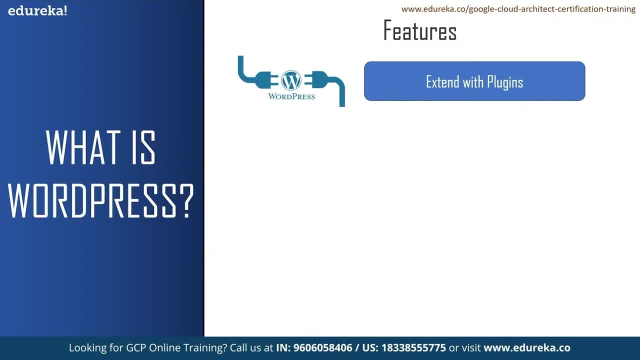 there is a plugin directory with thousands of plugins. you can add complex galleries, social networking forums, social media widgets, spam protection calendars, fine-tune controls for search engine optimizations and forms. these were just some of the plugins which you could use with wordpress. the next feature is it has a easy theme system. you can select from thousands of. 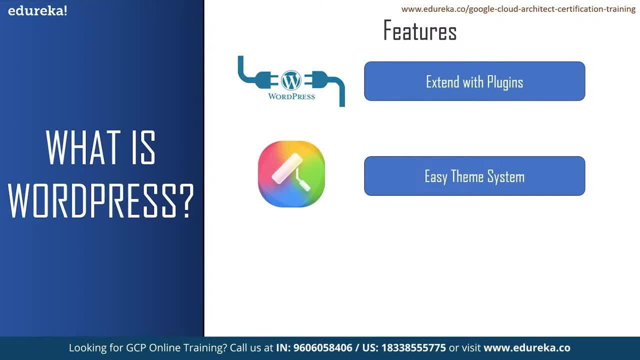 themes to create a beautiful website from the theme directory. but default wordpress comes bundled with three default themes. but you can upload your own website from the theme directory with a few clicks. now it only takes a few seconds for you to completely customize your website. the next feature is search engine optimization. wordpress is optimized for search engines, right. 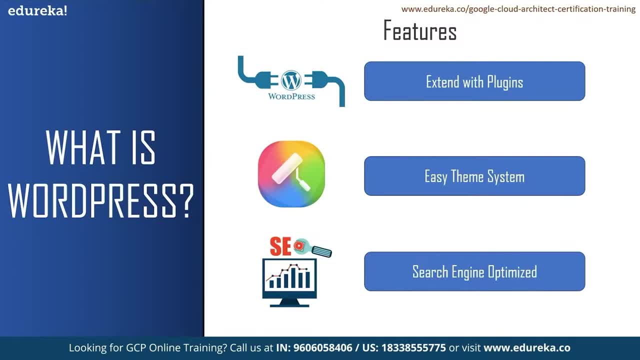 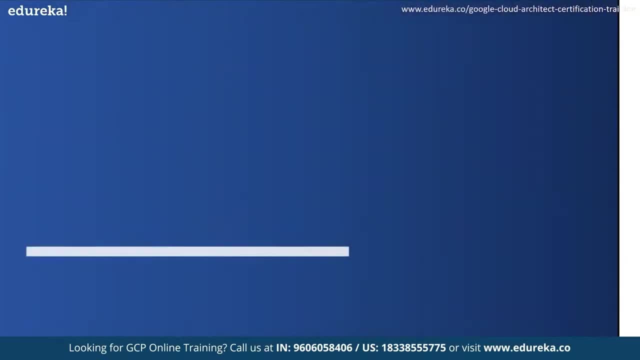 out of the box. if you want more fine-grained seo controls, there are plenty of seo plugins to choose from now. these were just some of the features of wordpress. let us move on to our next topic and see what is google cloud platform. google cloud platform is a suite of cloud computing services. 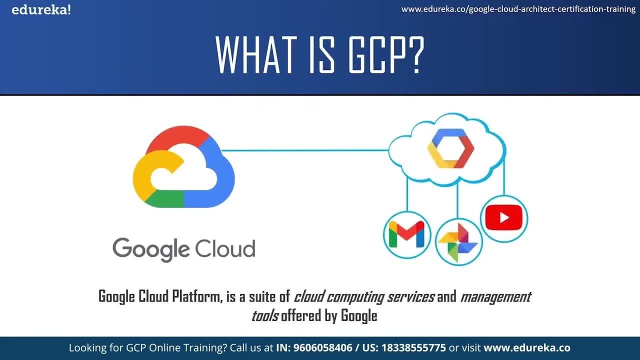 and management tools offered by google. gcp runs on the same cloud infrastructure that google uses internally for its end user products such as google search, gmail, google photos and even youtube. it is one of the leading cloud service providers, along with amazon web services and microsoft azure cloud, and owns seven percent of 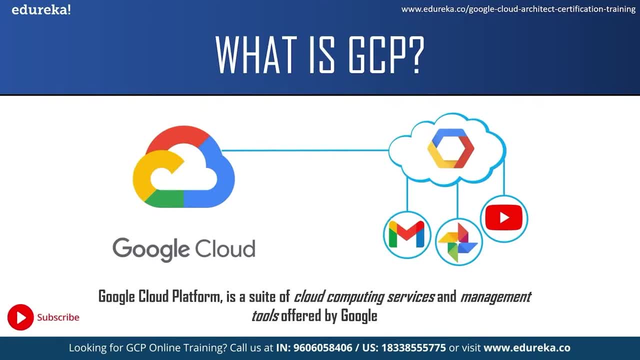 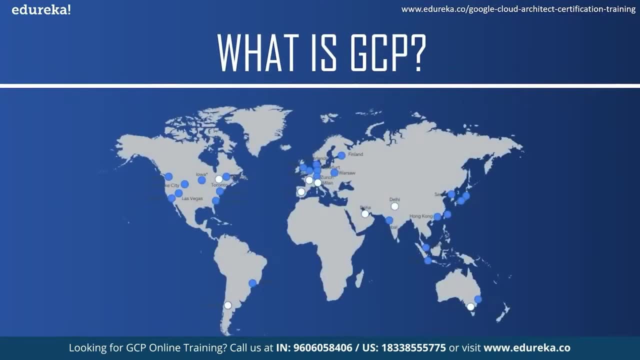 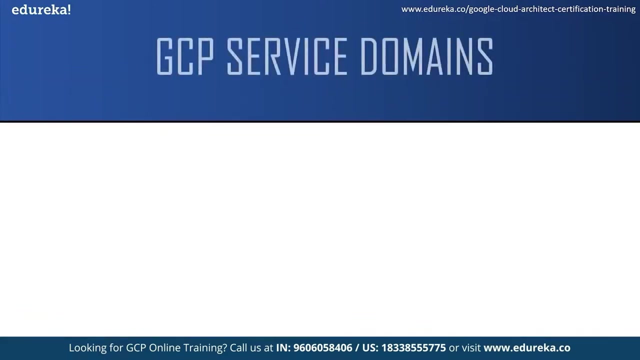 the total cloud market share, gardner has positioned google as a magic quadrant leader among the furthest three position vendors. google cloud's global network spans across 25 regions, with 76 countries now. the region is a specific geographical location where you can host your resources, and a region can have three or more zones. now what are the resources? 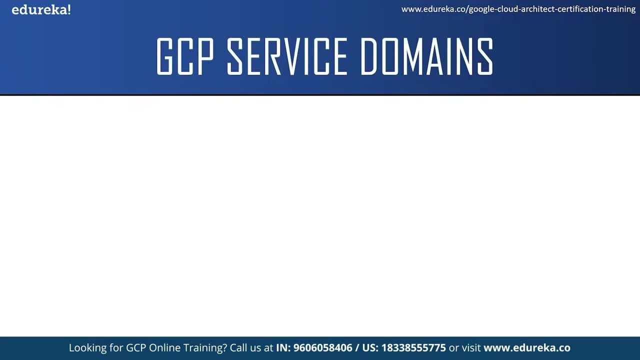 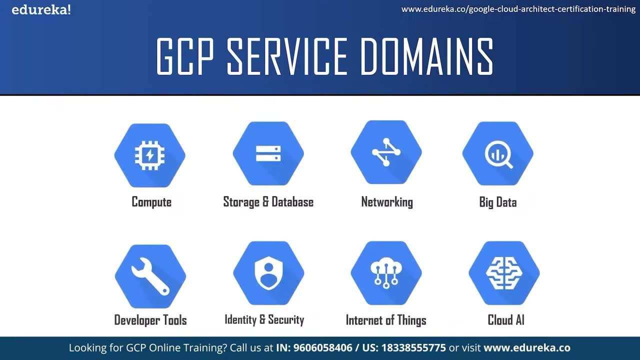 gcp provides us google cloud platform provides various services in different domains. let us take a look at some of the core gcp service domain. first is the cloud compute engine. this service is where we can create instances or virtual machines on gcp. second is the storage and database. 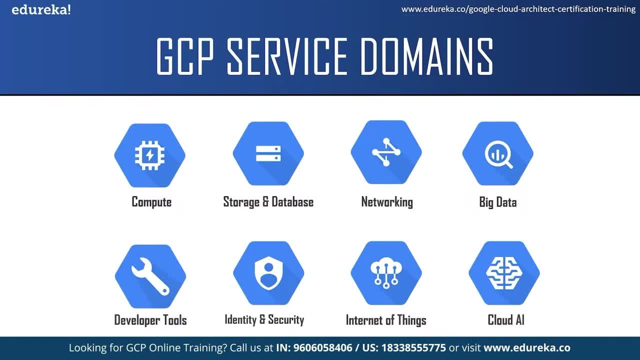 offers highly durable, available and scalable storage solution for different types of data and access methods. next is the networking service. GCP provides a fast, reliable, securing networking that scales, based on user demands. next we have big data: GCP provides several services like data flow, data procs and data fusion to help you create a complete cloud. 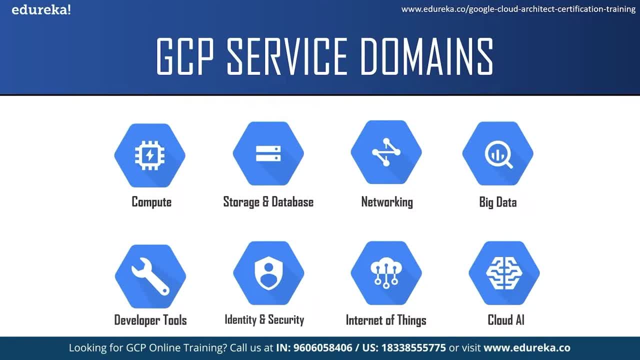 based big data infrastructure. next GCP, provides all the tools developer and development team needs to be productive while writing, deploying and debugging application hosted on the google cloud. the next service domain is identity and security. this domain lets administrator authorize who can take actions on specific resources, giving you full control and visibility. 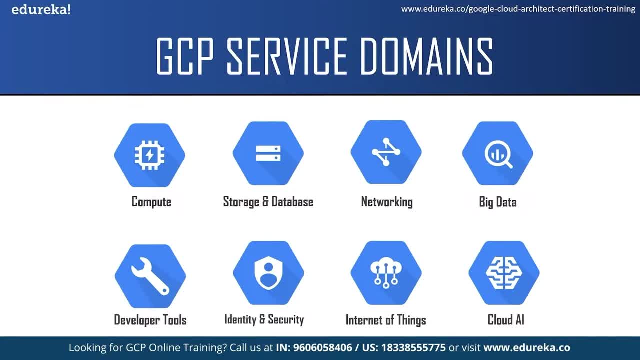 to manage google cloud resources. next, we have internet of things. GCP provides you with an intelligent iot platform which is scalable, fully managed and integrated. it lets you connect, store and analyze data at the edge and in the cloud. GCP provides you with an intelligent iot platform which is scalable, fully managed and integrated. it lets you connect, store and analyze data at the edge and in the cloud. 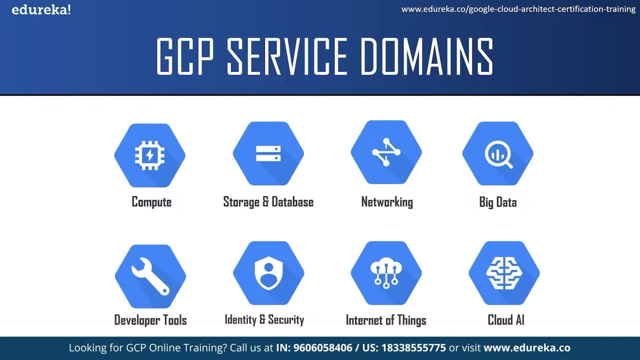 the next service domain is cloud ai. GCP provides fast, scalable and easy to use ai offerings, including ai platform, video and image analysis, speech recognition and multi-language processing. these were some of the core service domains in GCP. now google also provides free trial to all its new customer. it provides $300 in free credit to fully explore and conduct an. 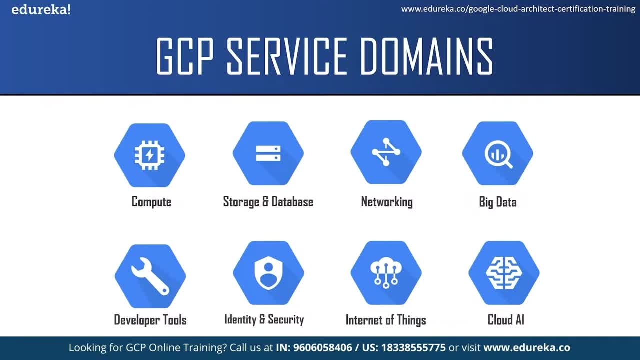 assessment of google cloud platform. you can use the $300 to try various google cloud products and learn how to use them. you won't be charged until you choose to upgrade and it is valid for 90 days. GCP also has free tier in which all google cloud customers can use selected. 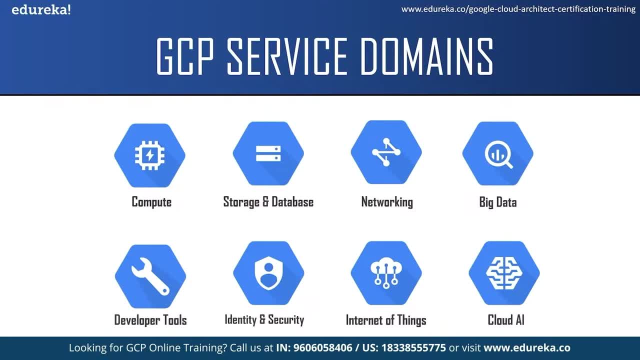 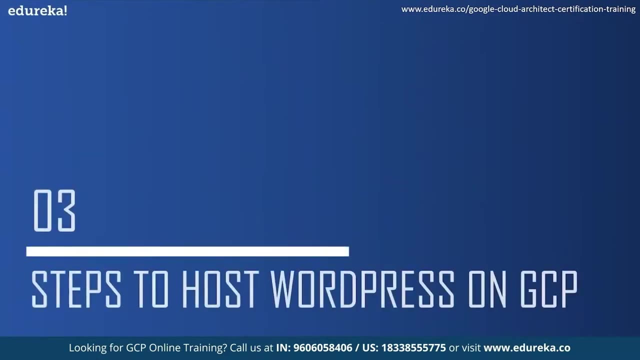 google cloud products like compute engine, cloud storage and bigquery, free of charge within the specified monthly usage. now, until you stay in your free tire limits, these resources will not be charged. now we are talking about GCP free tires because we're going to use it for our demo. now let us move on to our next topic and see the steps to host wordpress. 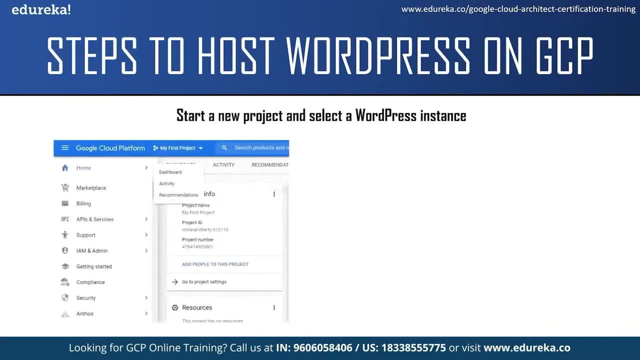 on GCP. the first step would be to sign in into your google cloud console. if you're new to google cloud, you can just sign up for an account by providing your address and your credit or debit card details. it is a very simple process and it won't take you long. 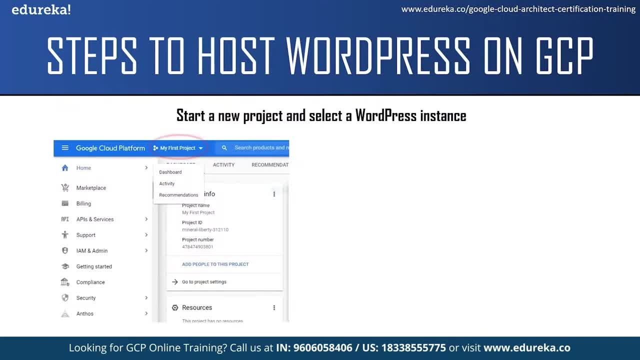 next. after that, you have to first create a new project in the google cloud. you will find first project on the top left corner. from there you can create your project. the next step is selecting a wordpress instance. for this you have to go to the navigation menu, which is on the left hand side, and under that select marketplace. 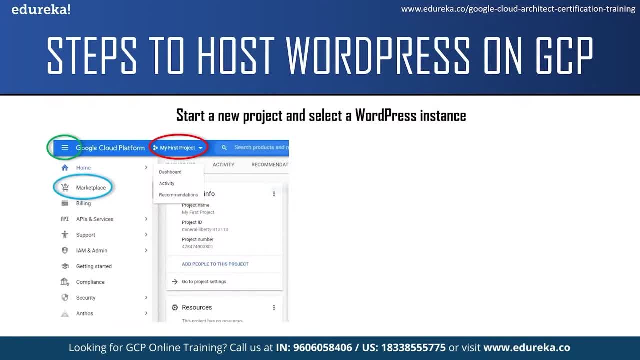 now google cloud marketplace will allow you to quickly deploy functional software packages that run on google cloud. even if you're not familiar with services like compute engine or google cloud storage, you can start up with familiar software packages without having to manually configure the software or the virtual machine, the storage or network settings. 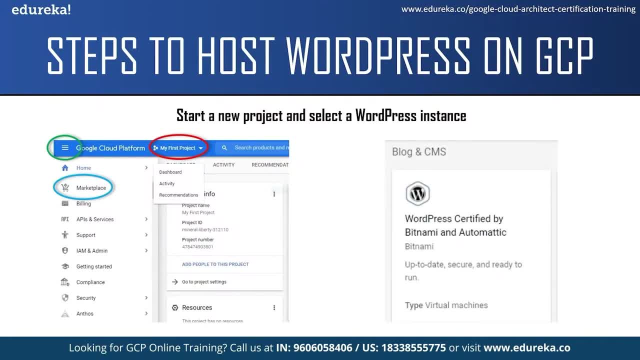 next you have to select your wordpress instance from the GCP marketplace. now there are various deployment of wordpress in GCP. i will show you in the demo part. so in today's session i will be explaining you guys how you can easily start things up in google cloud with. 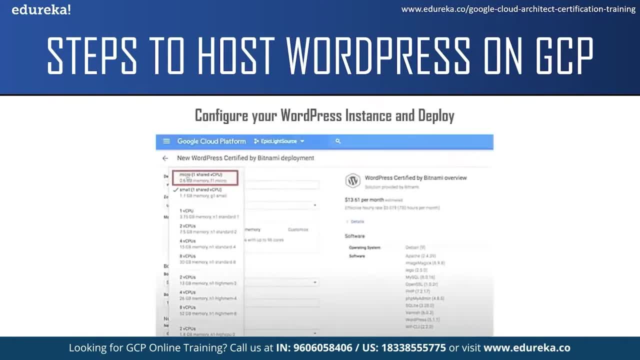 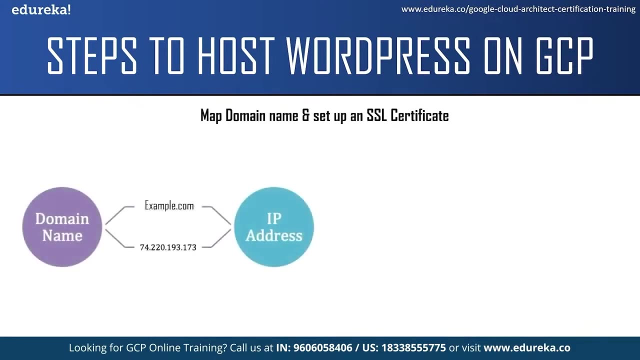 the help of a website. it's really nice because it is quite simple and straightforward to install. you will find this under blogs and cms column. next it will ask you to configure your wordpress instance. you can make changes according to your convenience. after the configuration is done, you can simply click on deploy and, after a few moments, your wordpress website. 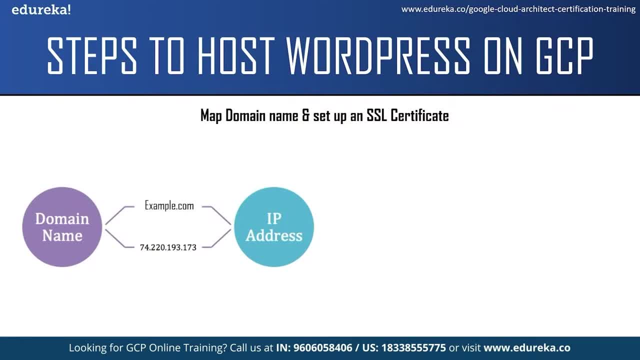 is deployed on google cloud platform. but this is not the end. your site is only accessible via an ip address, so you'll have to map a domain to the ip address. this step is important because to enter the domain name to a website rather than the IP address, You can just register. 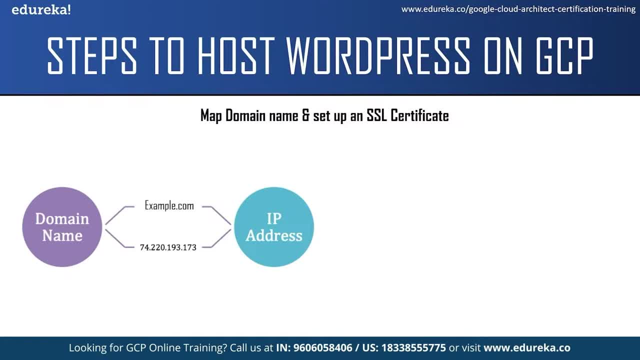 for a new domain name, if you do not have one, and link it to your WordPress website. Next, you have to set up an SSL certificate, which stands for secure socket layer. Now, this is a type of digital certificate that provides authentication for a website and enables an. 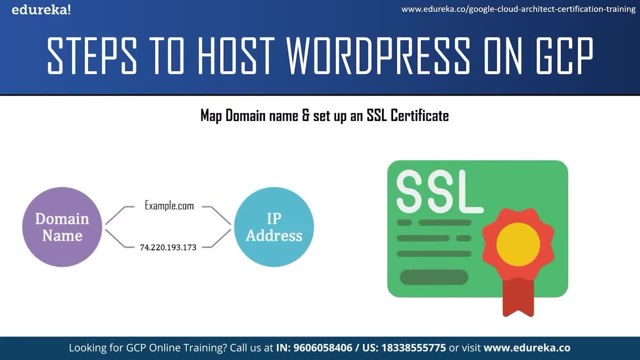 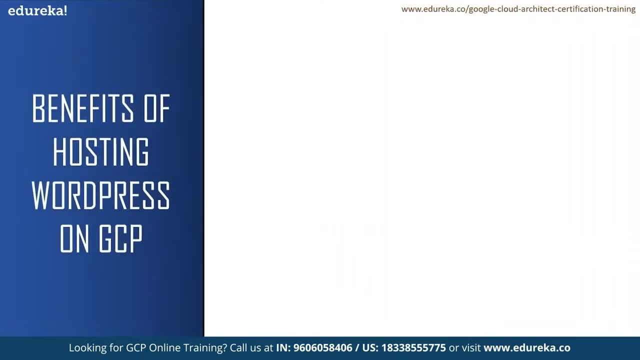 encrypted connection. This step is not mandatory, but it is recommended. Now let us move on to the next topic and see some of the benefits of hosting WordPress on Google Cloud platform. The first benefit is uptime. Businesses such as big e-commerce stores, trading sites and 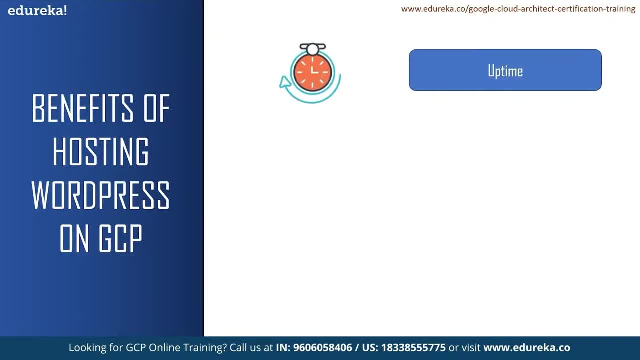 new site rely heavily on optimal server uptimes. They would want the servers to be up and running always, because even with a slight interruption in the service it can cause them a lot of financial damage. But Google Cloud engine is available for more than 99.9% of the time. 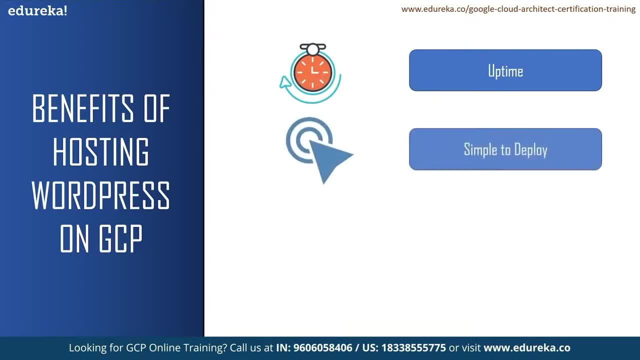 So companies can be assured they won't have this problem. Next, it is simple to deploy. As I've told you in the previous topic how simple it is to deploy WordPress on the Google Cloud, I will also show you how simple it is. It also gives you complete liberty to make changes. 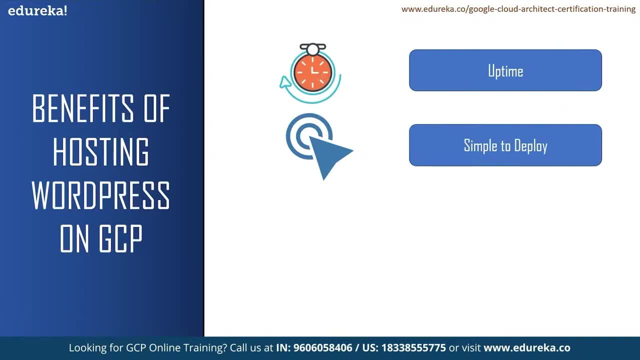 to any of your root files. With GCP hosting, you will get high performance consistently, no matter how much traffic you receive. The third benefit is reliability. Google Cloud engine uses the same infrastructure as other Google apps like Gmail and YouTube, which means your website is hosted on the most well-maintained hardware, which is controlled by Google. So 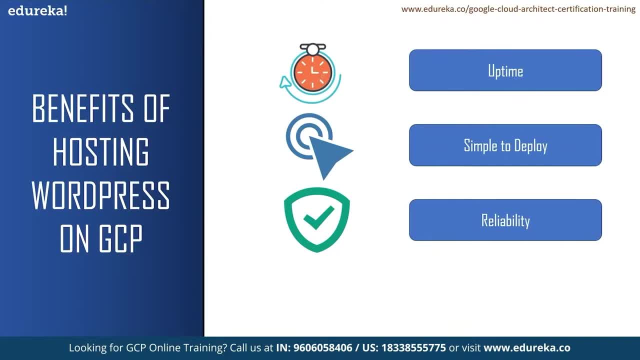 you can be assured there would not be much downtime to your website. Google constantly works on improving the services So they can provide a better customer experience. The next benefit would be scalability. Google Cloud engine servers are highly scalable and can handle unexpected traffic spikes with. 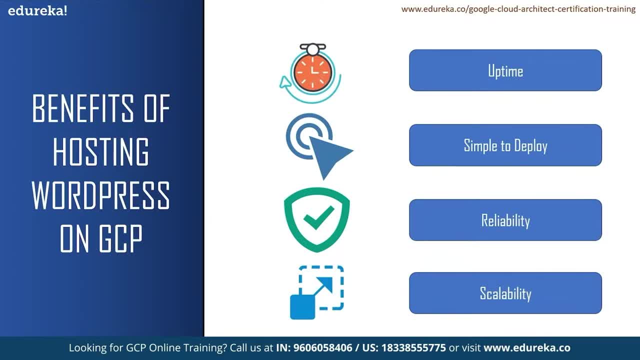 ease. So imagine there is a peak time and a lot of users are trying to access your website. Now, as the website is hosted on the Google Cloud, it will scale its servers up in order to match the incoming traffic. With GCP, you can also upgrade or downgrade a server size. 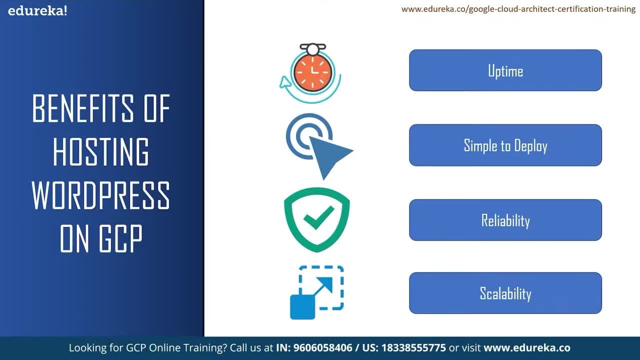 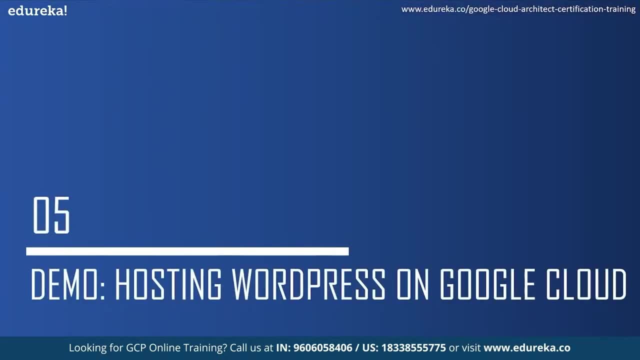 without changing the IP address. Now, these were some of the advantages of hosting a WordPress website on GCP. Now let's move on to a demo part, where we'll host a WordPress website on the Google Cloud platform. So for our demo, I've logged in into a GCP account. It is very simple to create. 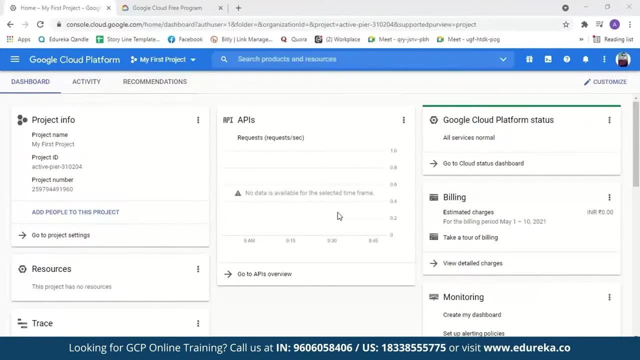 a GCP account. All you have to do is enter your debit card or your credit card detail and your address. Then you might be charged maybe one rupee, but even that will be refunded later. Now, as you sign in into a new account, GCP will provide you $300 free credit Now. 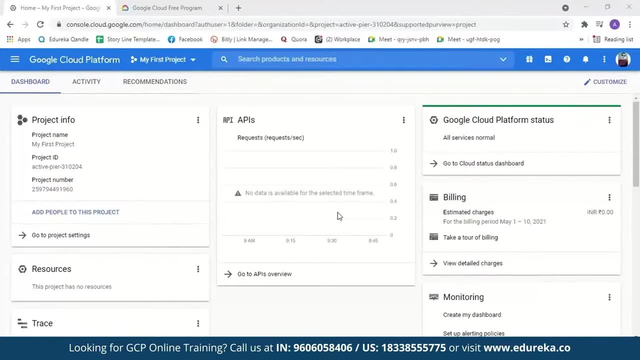 you can use this $300 to explore Google Cloud services. You won't be judged until you choose to update and it will be valid for 90 days. So the first step is creating a new project. So we'll go to my first project over here. 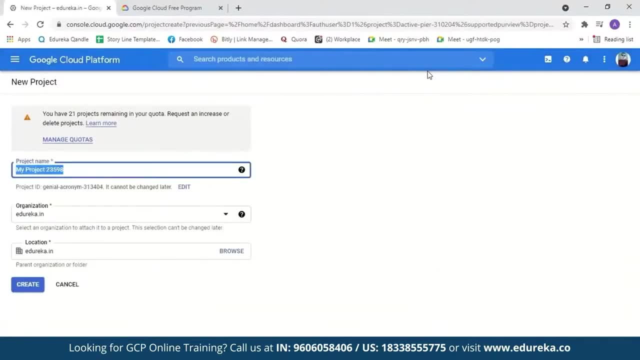 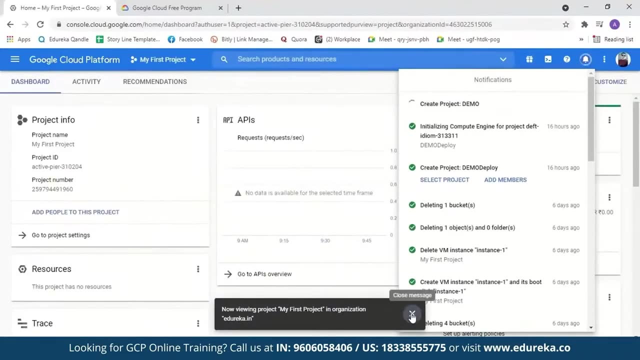 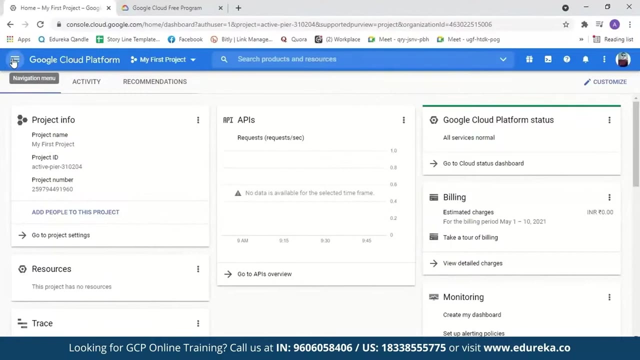 I will just select a new project from here. We can name a project anything, So let us name it demo. We'll just create it Now. you can see our demo project is created. Now let us move on and select a WordPress instance. So for that we'll go to navigation menu. 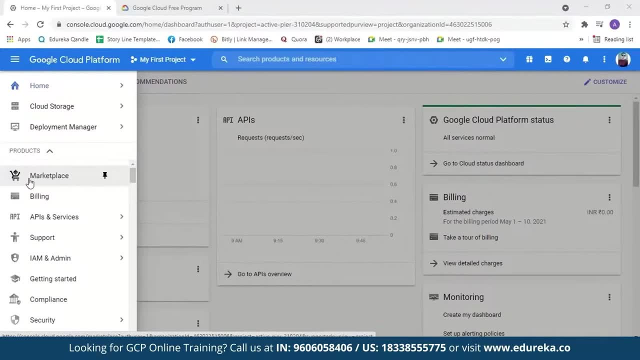 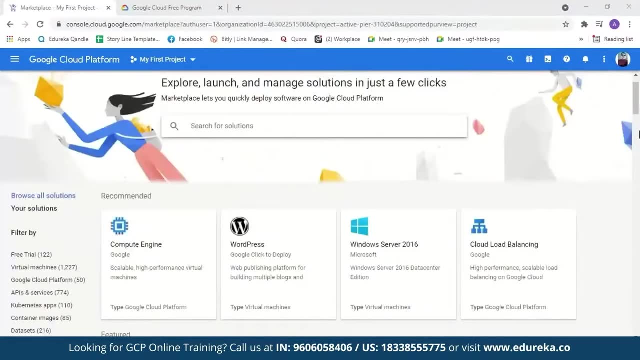 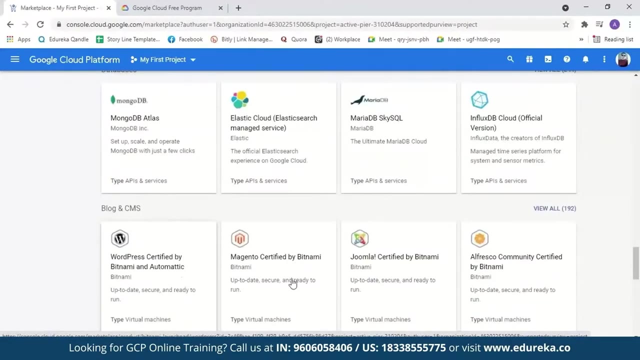 Now here you have something called a marketplace. Now, marketplace will allow you to quickly deploy functional software packages that run on Google Cloud. So go to marketplace. Here you can see there are a few WordPress instances, But in today's session we're going to use WordPress certified by Bitnami and automatic. 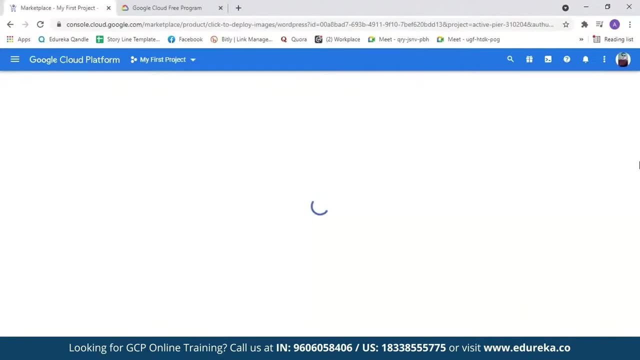 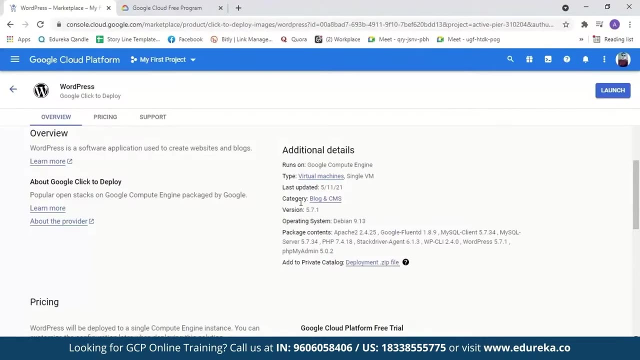 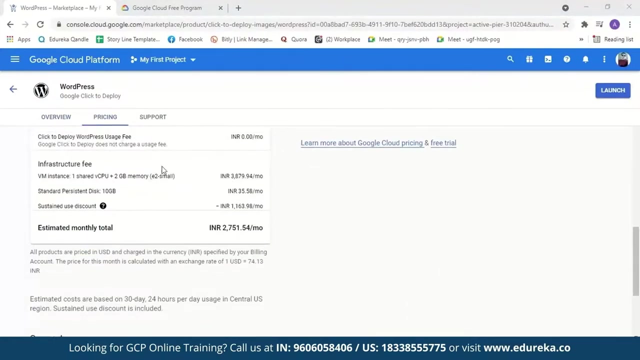 But let us take a look at WordPress: Google click to deploy. So we select this. Here you can see the overview of the instance and its details: the type of virtual machine, the version, the operating system, The packages it contains. here, when we go to pricing, you can see how much will it cost. 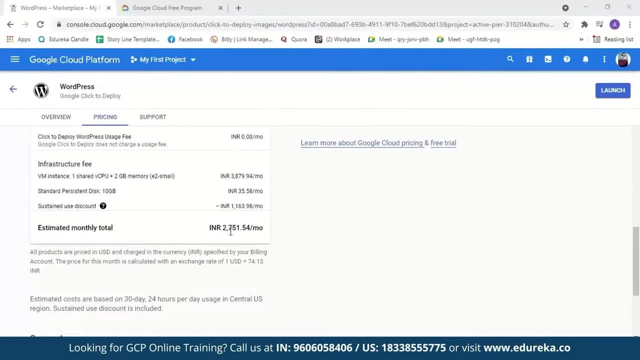 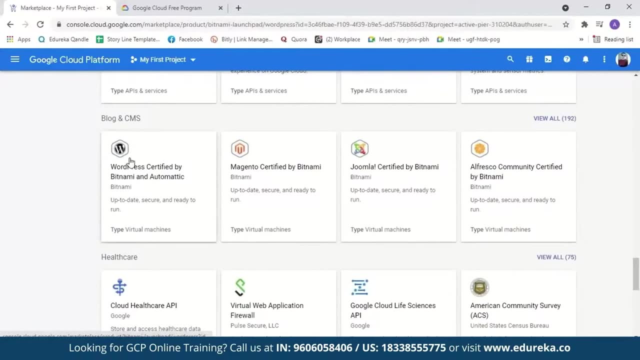 you per month to the cost us 2751 rupees per month. Now let us go back and see WordPress by Bitnami. It will be under blocks in CMS, So just click on this. So here is our overview of our instance. 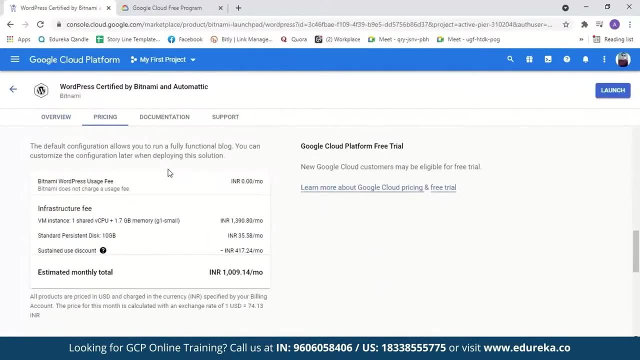 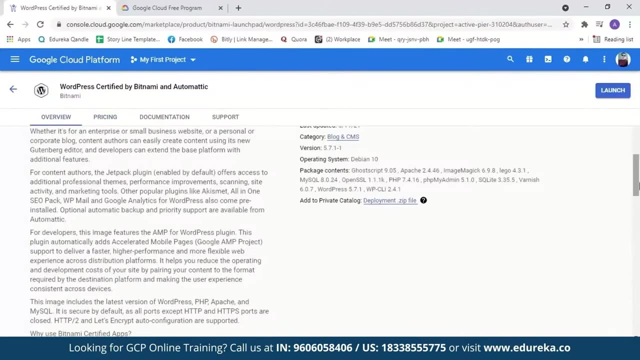 its details And the pricing and you can see the pricing is 1009 rupees. It is way more cheaper and it is very simple and straightforward to deploy. It also comes with a lot of pre-loaded packages which are very helpful for a WordPress website. 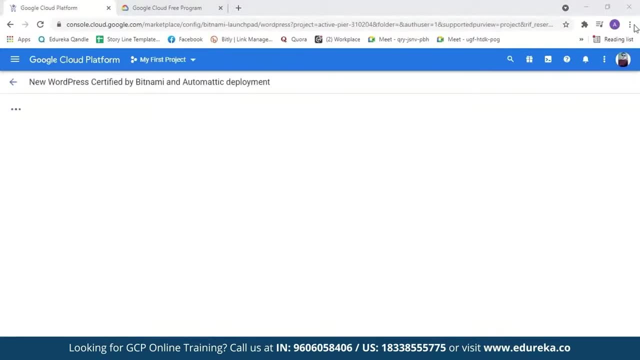 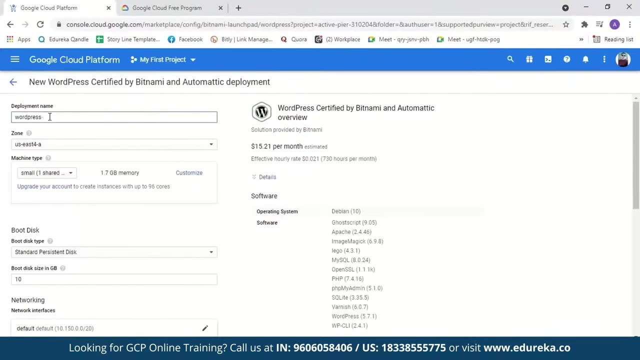 So now we will go ahead and launch it. Now we have to configure our instance. first We have to name our deployment, So just name it WordPress demo. next We have to select a region. So for this, if you're using a free tire account, you should select a particular region only if you go to the DCB free tire. 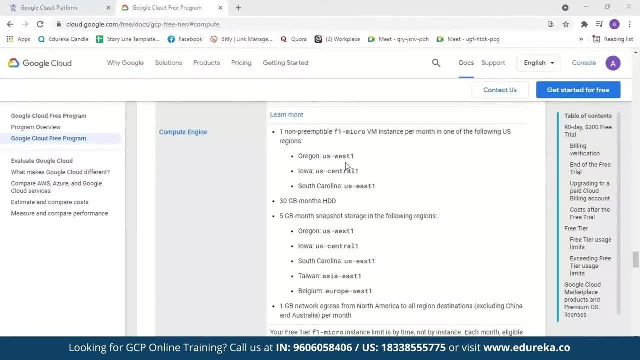 page, We can launch a F1 micro virtual machine for free only in this region. So for this, if you're using a free tire account, you should select a particular region. only if you go to the DCB free tire page, We can launch a F1 micro virtual machine for free only in this region. 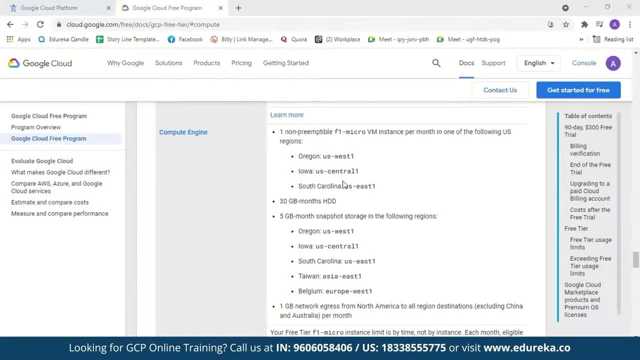 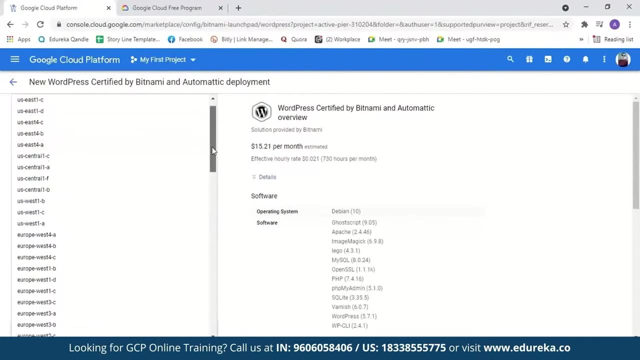 Which is Oregon, us-west one, or lower us-central one, or South Carolina, which is us-east one. So we'll go back and we just select us-east one. Now you can select anything from BCD. These are just the zones available. We'll just select this. 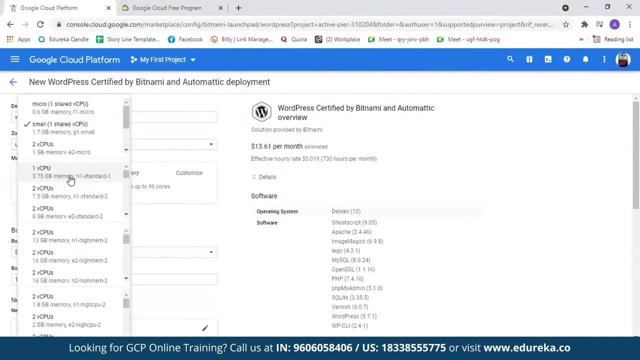 Next we have to select the machine type. So for this demo I won't be needing too much of compute capacity. Now. here the default is small, with one shared virtual CPU And 1.7 GB memory. but for this demo I'll go with micro where I get one shared virtual. 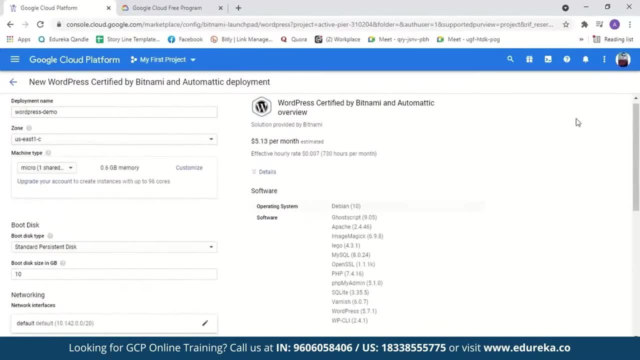 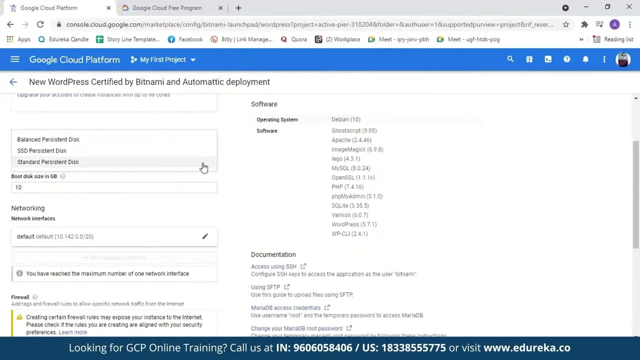 CPU and 0.6 GB memory. You can select a compute capacity according to your website needs. now the micro machine type will only cost me $5.13 per month. Next we have boot disk. The boot disk type can be either standard persistent or SSD persistent or balance persistent. 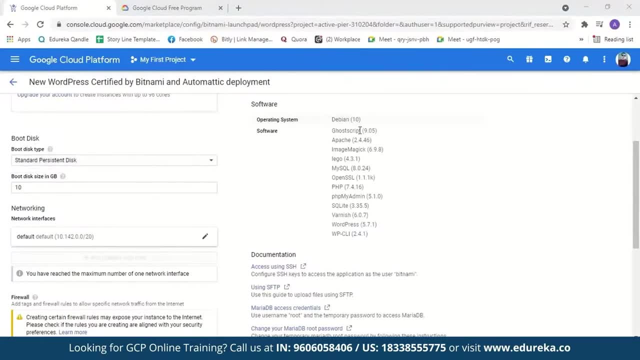 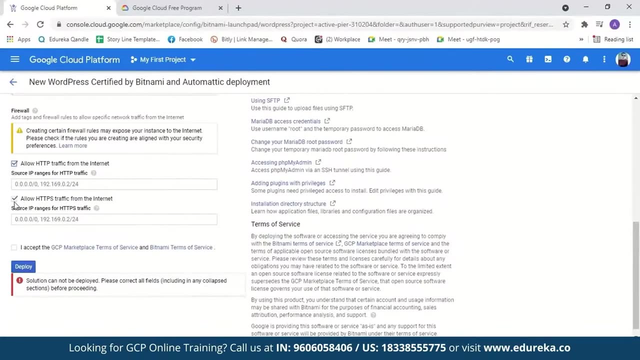 So let us just go with the standard persistent disk And the boot. We'll keep the 10 GB will keep the networking at default itself. Next, we'll select both HTTP and HTTPS traffic from the internet. This basically means allowing network traffic to your website. 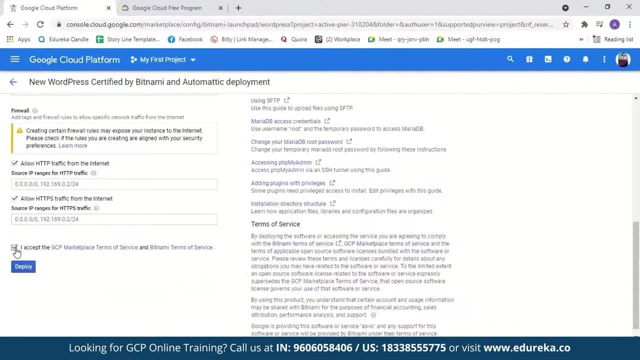 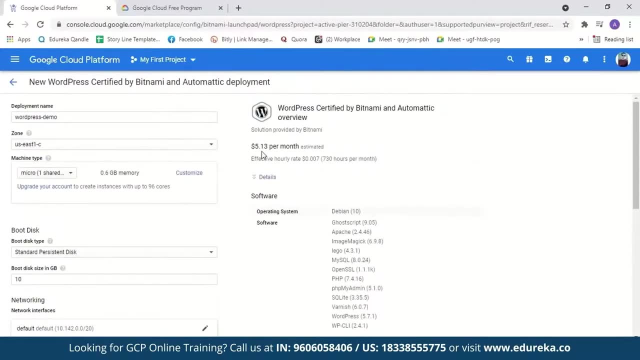 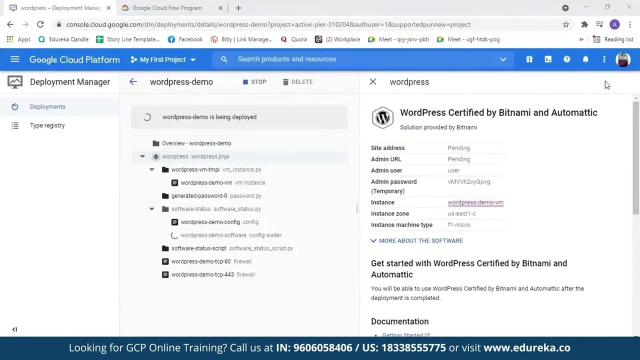 This means anyone with the access of internet can visit your website, will accept the term and condition and just click on deploy. now You can go back and check how much would it cost you per month. for me It would cost $5.13 per month. will just go ahead and deploy it. 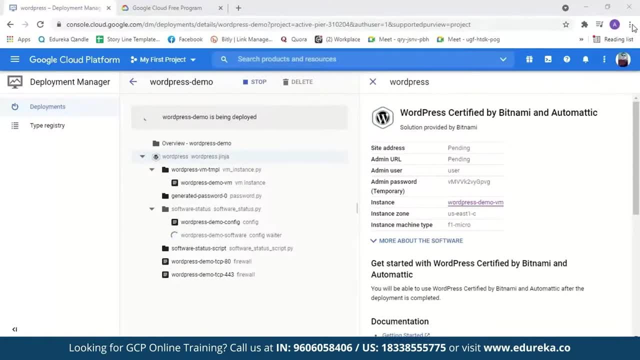 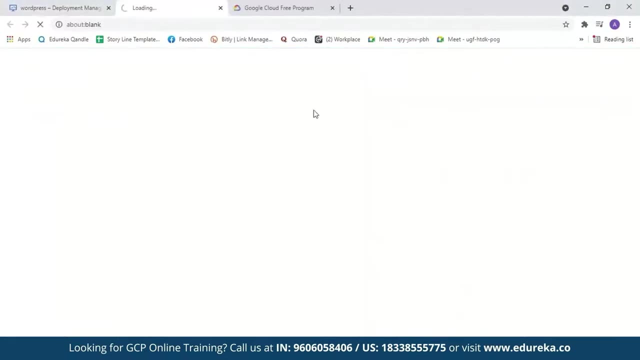 It will just take a few minutes For Google to deploy your WordPress website. During the process, software scripts is run, WordPress is configured. the username and password for your WordPress account is generated. Now you can see. a WordPress website is successfully deployed. Now let us log into a WordPress website. 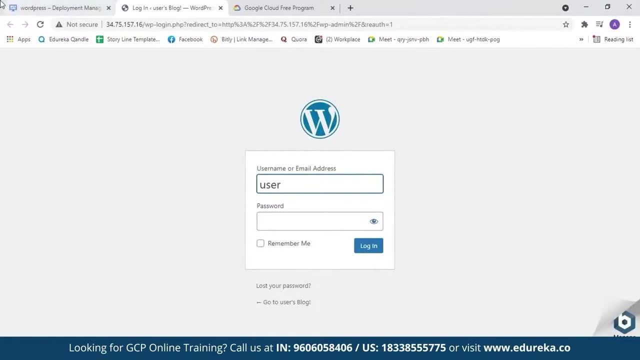 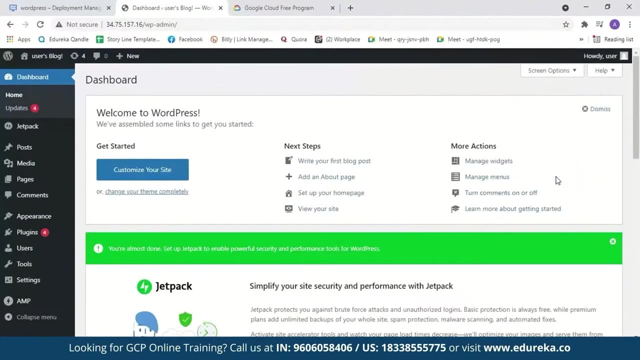 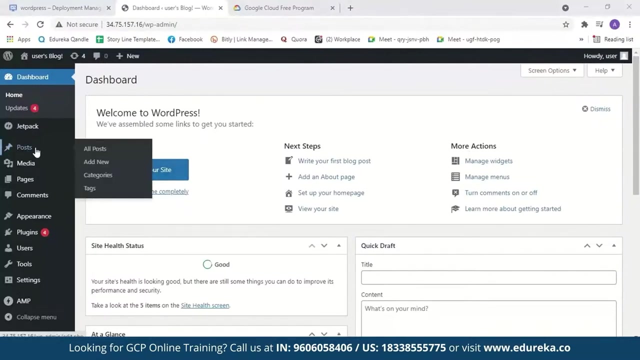 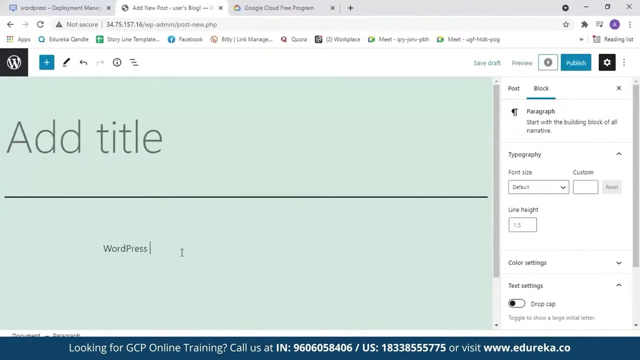 We'll just click on admin URL. Our username is user. just copy the password from you And we log in. And now we are in Our WordPress website. Now let us just post. something would post and you will just type WordPress on GCP. 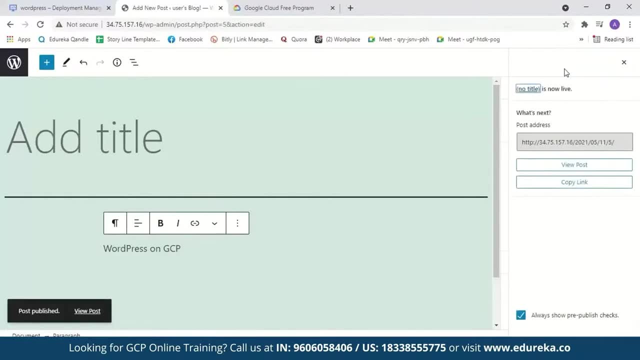 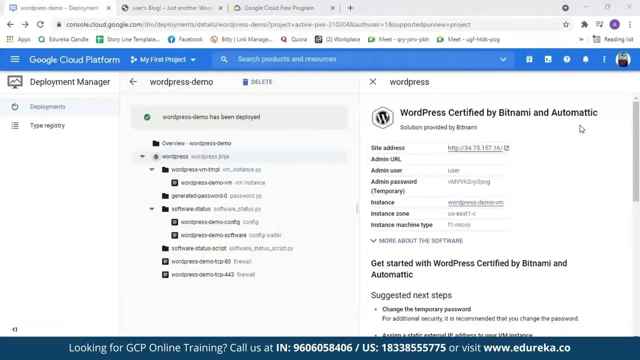 And we publish it Now. let us view our website Here: WordPress on GCP. Now going back to a Google Cloud platform, You will see the IP address which we used to login will keep changing every time I restart my virtual machine. Now we have to make that static, so for that will just go to navigation menu. 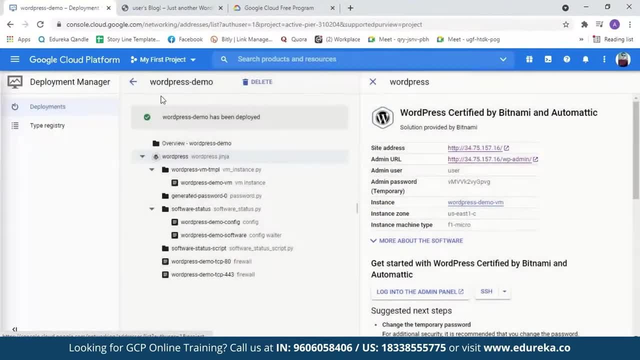 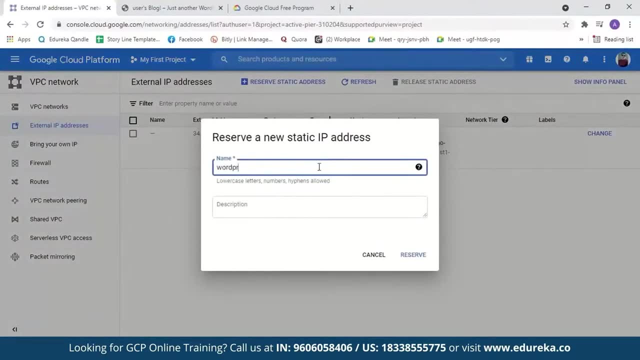 And we select VPC network and from here will go to external IP addresses. Now, the type here is ephemeral, will make it static, will just name it. I will just resolve this now. the IP address will be static and it won't change every time. 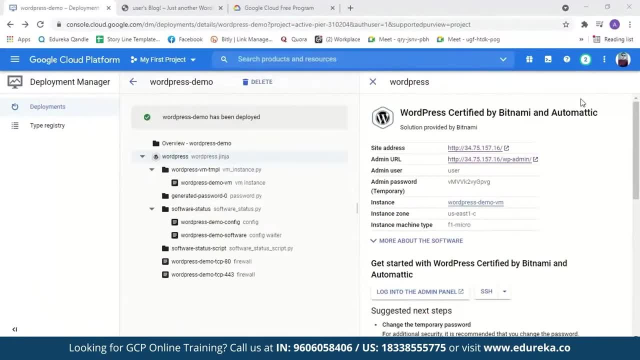 I restart my virtual machine, So this was today's demo. but after this, you still have to link a domain name to a static IP address and also set up a SSL certificate. Now, SSL certificate is a bit of code on your web server that provides security for online. 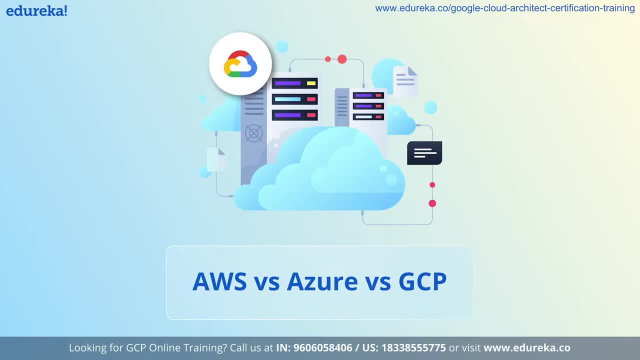 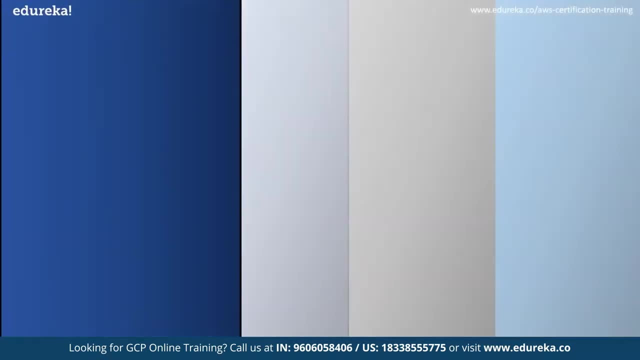 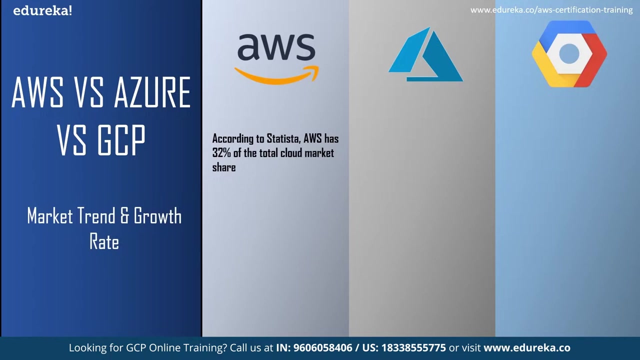 communication. Let us compare this three cloud service providers. Let us first compare them based on the market trends and growth rate. Now, according to statista, AWS owns 32% of the total cloud market share. Amazon reported that Amazon web service Revenue was $13.5 billion in the first quarter of 2021, which actually exceeded the analyst. 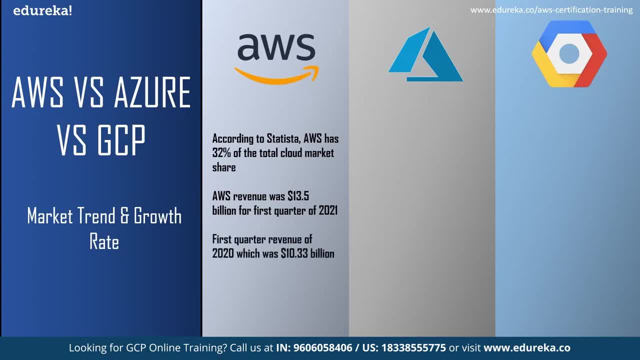 prediction of $13.1 billion, and when you compare this to the first quarter revenue of 2020, which was 10.33 billion, we can see AWS revenue grew more than 30% in a year. in the first quarter of 2021, AWS revenue accounted for 12% of total Amazon's revenue and nearly 47%. 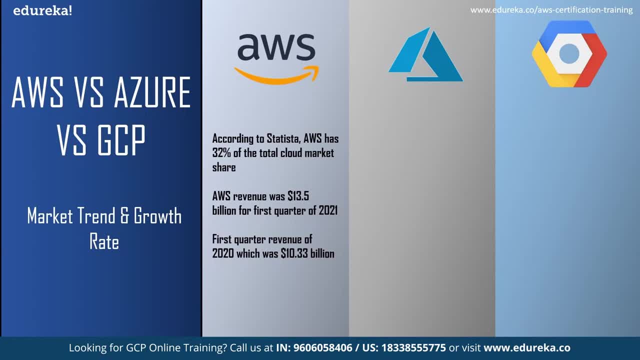 of Amazon overall operating income. Amazon CEO Jeff Bezos has said AWS has an unusual advantage of a seven-year head start before facing like-minded competition. as a result, The AWS services are by far the most evolved and most functionality rich. next, Let us take a look at the market trend for Azure. according to statista, Microsoft Azure. 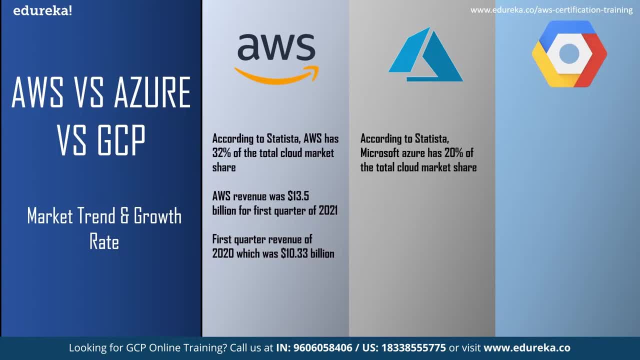 owns 20% of the total cloud market share. now, unlike Amazon, Microsoft only reports the growth rate and not the revenue. it reported 50% revenue growth over the previous quarter, Which was better than the 46% growth the analyst expected in 2020. Microsoft reported that. 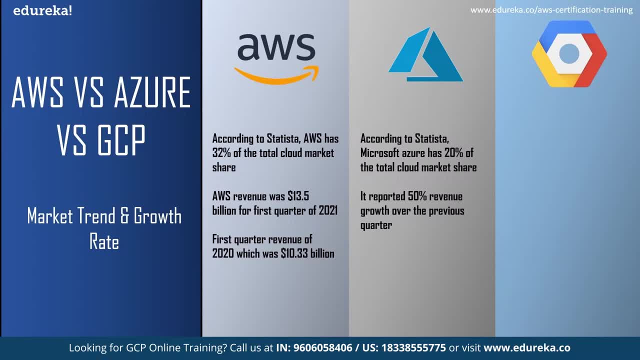 its commercial cloud officially hit the 50,000 billion mark for its annual run rate. next, looking at the market trend for GCP: according to statista, GCP owns 9% of the total cloud market share. in the first quarter of 2021, Google Cloud reported revenue of 4.0 billion. 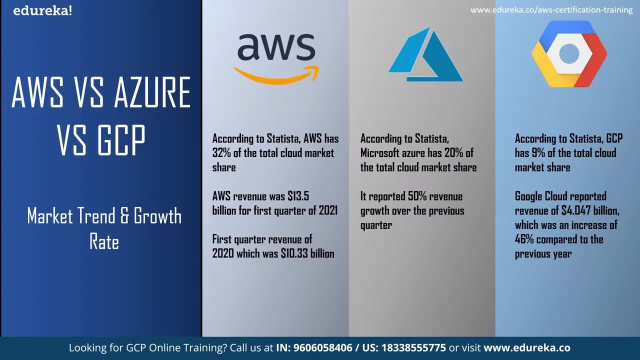 dollars, which was an increase of 46% compared to the previous year. also, the operational losses: It was reduced to 974 million dollars this year, compared to the losses of 1.73 billion last year. Now, this was the market trend and growth rate of AWS, Azure and GCP. 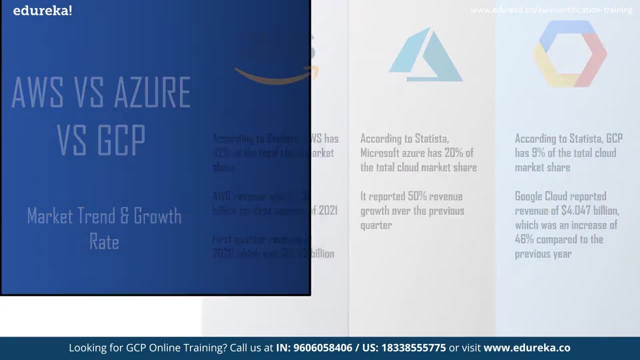 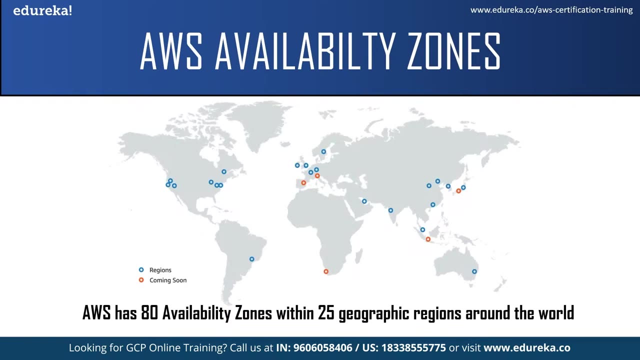 Now let us move on and compare them based on the availability zones. But before we compare their availability zones, I would like to define water availability zones and regions Now. region is a specific geographical location where you can host your resources, and availability zones are distant location within the region that are engineered to be isolated from failure. 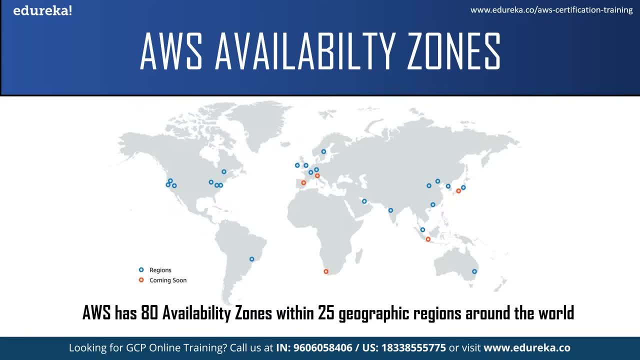 from the other availability zones. Now, talking about the availability zones of AWS, It has the most extensive global cloud infrastructure is multiple availability zones are connected by a low latency, high throughput and highly redundant networking. AWS, as 80 availability zones within 25 geographical location around the world, has also announced for 15 more availability. 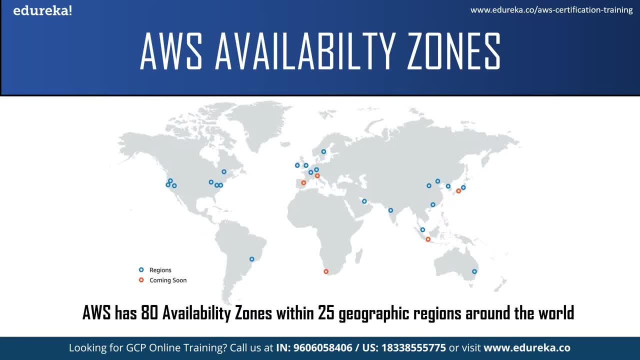 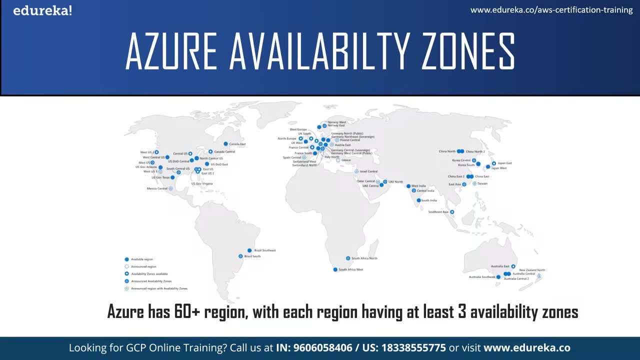 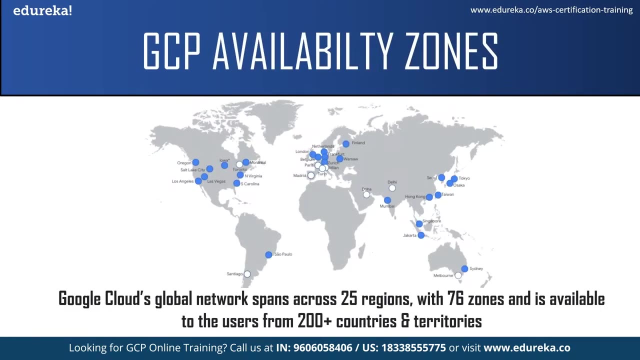 zones and five more regions in Australia, India, Indonesia, Spain and Switzerland. now comparing it to the Availability zones in Azure, Azure as 60 plus region, with each region having at least three availability zones, next coming to GCP availability zones. its global network spans across 25. 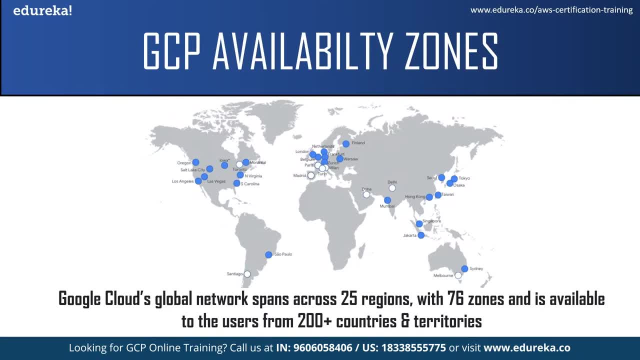 regions with 76 zone and is available to user from 200 plus countries and territories. GCP has recently announced new regions in Seoul, Salt Lake City, Las Vegas, Jakarta and Warsaw and will also expand its networks to nine more regions. now, this was about the availability zones. next, 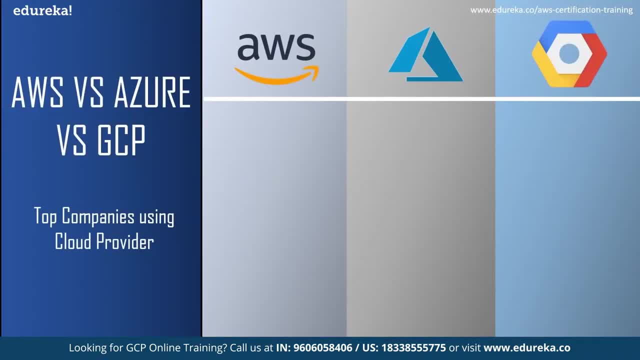 Let us see what are the top companies using this cloud service providers. first, talking about AWS, its services are used by top companies like Netflix, coca-cola, McDonald's, Unilever, ESPN and Adobe. next, coming to Azure, It is used by many Fortune 500 companies and some of the companies which use Microsoft. 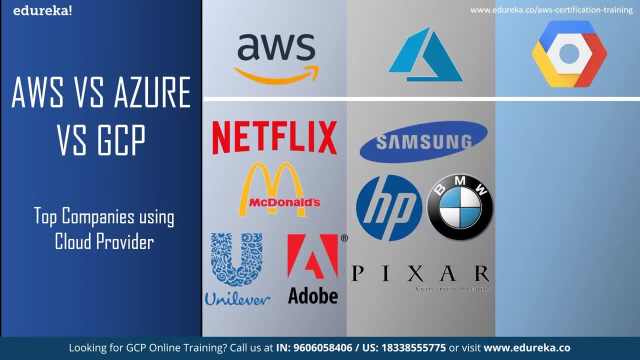 Azure clouds are Samsung, HP, BMW, FedEx and Pixar animated studio. moving on to GCP, the top companies who use their services are PayPal, Twitter, 20th Century Fox, PNG and King Digital Entertainment. Now that we have seen what are the top companies which uses cloud service providers, 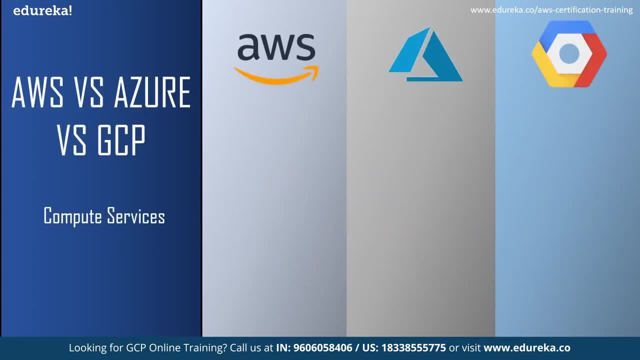 Let us compare them based on the compute services. compute services are one of the core services when it comes to cloud computing. compute services helps to create instances of virtual machines in minute and also scale up instances instantly if needed. So in today's session We're going to compare this. 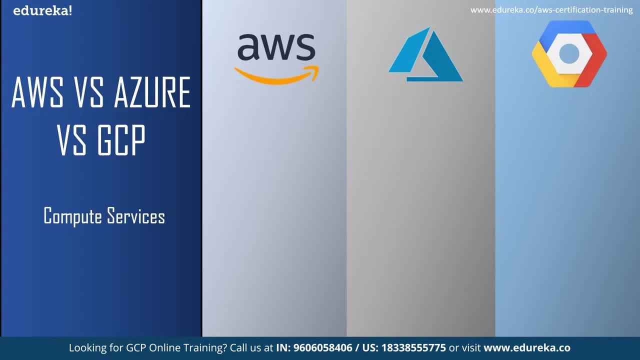 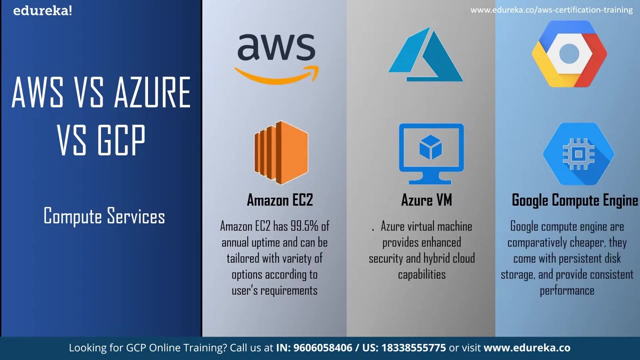 Three cloud service providers based on the compute service and storage service. The primary compute service for AWS is Amazon easy to. the primary compute service for Azure- Azure virtual machine, and for GCP is Google Compute Engine. Now, all the three services are equally powerful, but unique in their own way. 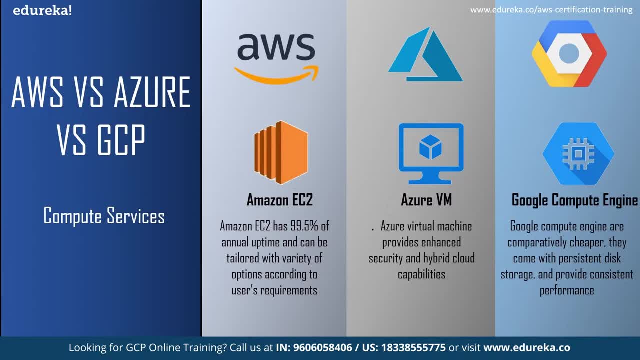 Each one has its own advantages and disadvantages. like Amazon, easy to as 99.5% of the annual uptime and can be tailored with variety of options According to users Requirements. on the other hand, Azure virtual machines provides enhanced security and hybrid cloud capabilities. but when you compare the cost, Azure instances tend to get costlier. 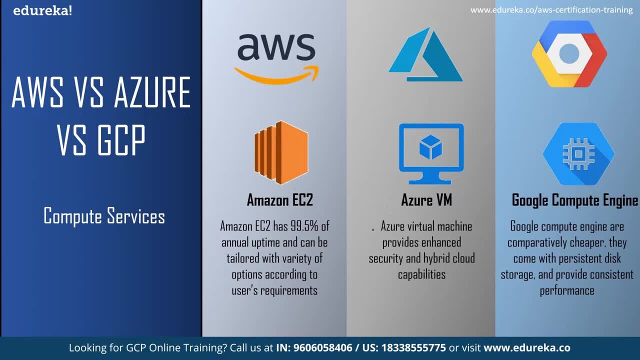 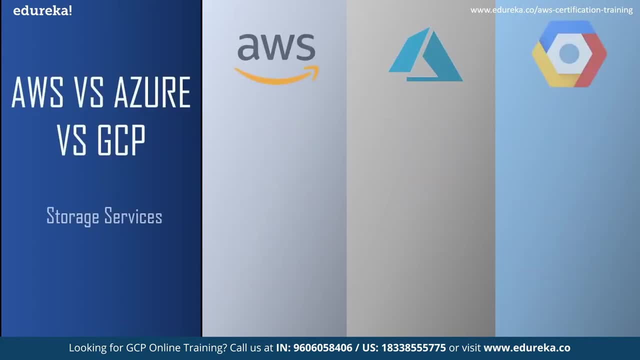 as a compute size increases. next, talking about Google Compute Engine, the comparatively cheaper they come with a persistent disk storage and provide consistent performance. next, talking about the storage services, AWS offers a variety of storage option, like s3 for object storage, EBS for block storage, EFS. 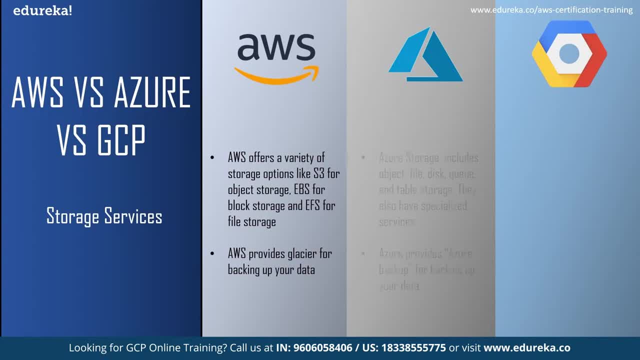 For file storage and a few other storage services. next, talking about Azure cloud storage, This also includes object file disk queue and table storage. They also have specialized services for data rich applications and many data backup services. now talking about GCP cloud storage, They have a fewer storage as compared to the other two, but they're more targeted for object. 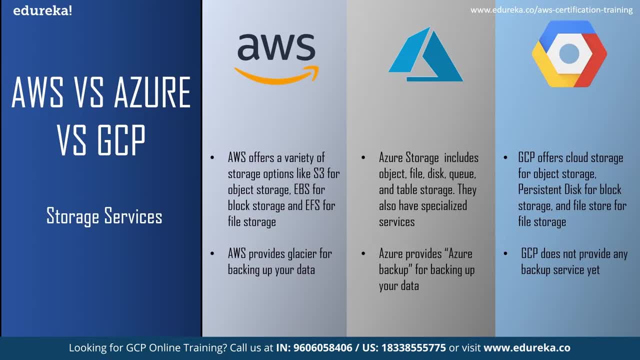 storage. GCP offers cloud storage. It offers persistent disk for block storage to be used with virtual machine And file storage for storing the files for backing up your data. AWS provides a service called as AWS Glacier and Azure provides a service called as Azure backup, but Google 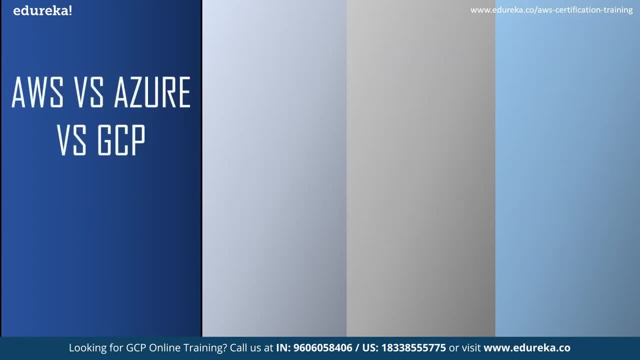 does not yet have any backup services. next, Let us compare this three cloud service providers according to the pricing. now, all the three cloud service providers offer a pay-as-you-go structure, which means you only pay for the services you use. now pricing would vary for different services. for compute services, one: 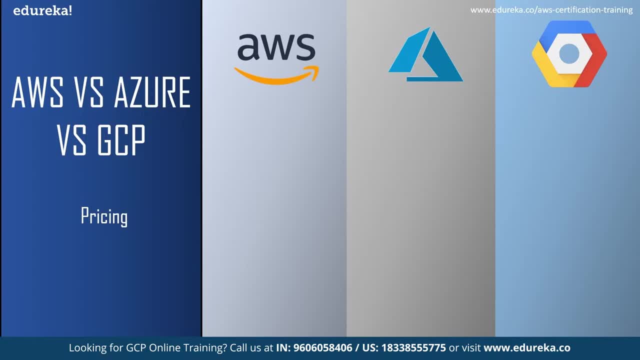 cloud service provider could be cheaper, but it could be costlier for database services and so on. So just to give you in general overview of the pricing among the three cloud service providers: GCP offers a slightly cheaper pricing model and has a flexible cost control which. 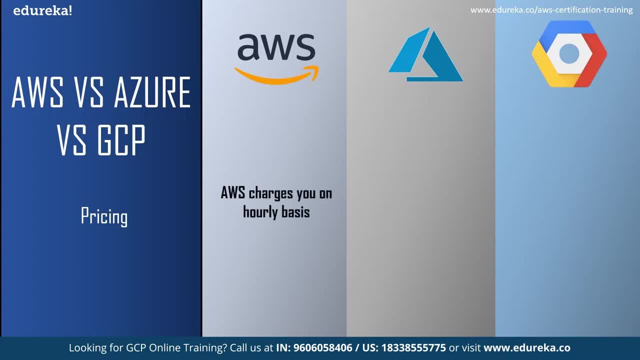 allows you to try the different services and features. AWS charges you on hourly basis, Whereas Azure charges you on a per minute basis and GCP provides per second billing for its resources. when it comes to a short-term subscription plan, Google Cloud and Azure gives you a lot more flexibility, but in certain services, Azure tends to be. 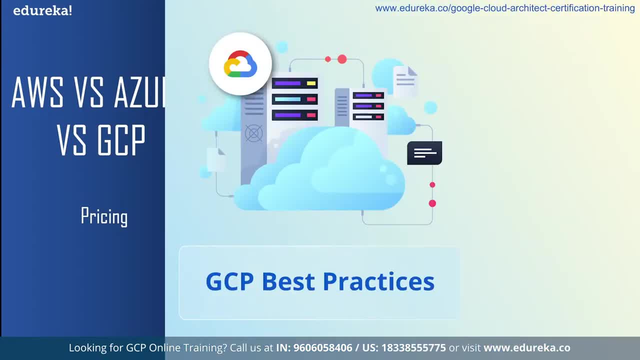 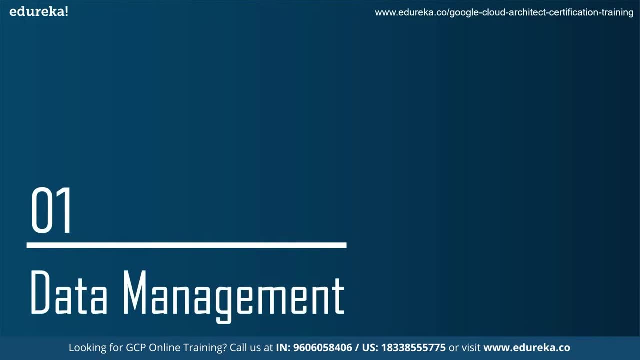 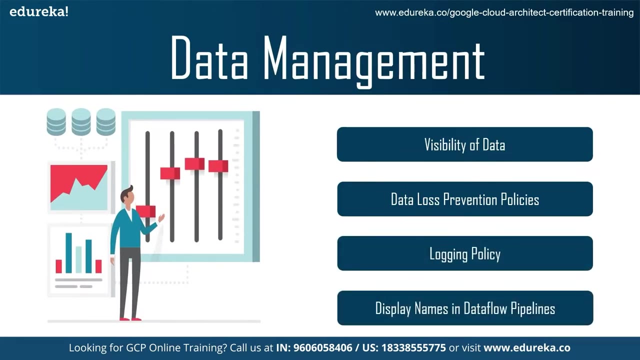 costlier when the architecture starts scaling up. Let's understand the best practices under data management. So first you have to ensure a total visibility of data. without a holistic view of data and its resources, It can be difficult to know what data you have, where data originated from and what data. 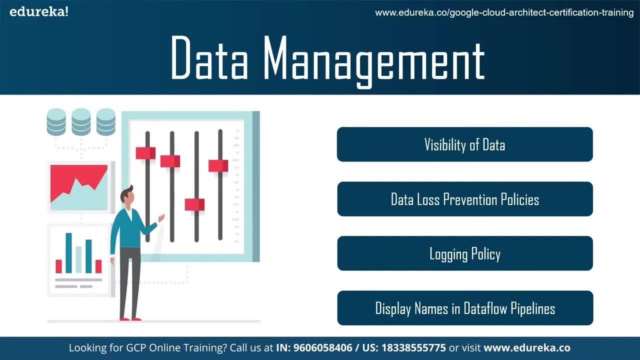 is in the public domain. that shouldn't be second. So the first step is to design data loss prevention policies in G Suite. So data loss prevention in G Suite is a set of policies, processes and tools that are put in place to ensure your sensitive information won't be lost during a fire or natural disaster. 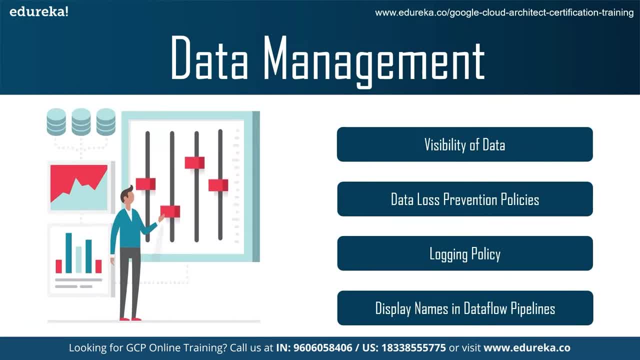 or break-in. You never know when tragedy will strike. That's why you should invest in prevention policies before it's too late. Third is have a login policy in place, So it is important to create a comprehensive login policy within your cloud platform to 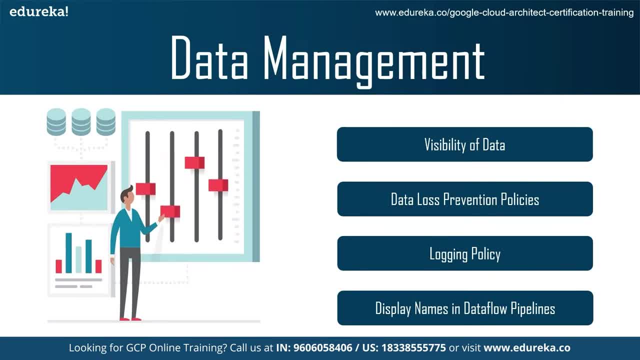 help with auditing and compliance. Access logging should be enabled on storage buckets so that you have an easily accessible log. object: access Administrator. audit logs are created by default, but you should enable data access logs for data rights in all services. Also, use display names in data flow pipelines. 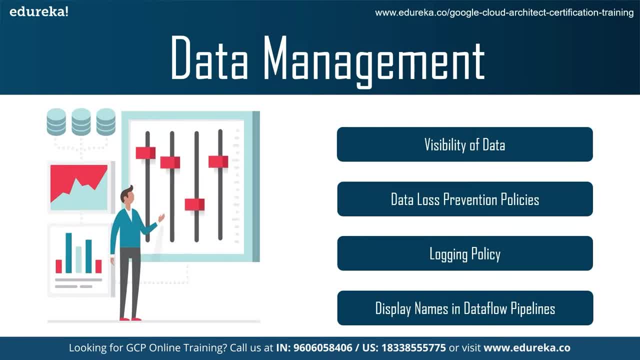 So always use a name field to assign a useful at a glance name to the transform. This field value is reflected in the cloud data flow monitoring UI and can be incredibly useful to anyone looking at the pipeline. It is often possible to identify performance issues without having to look at the code. 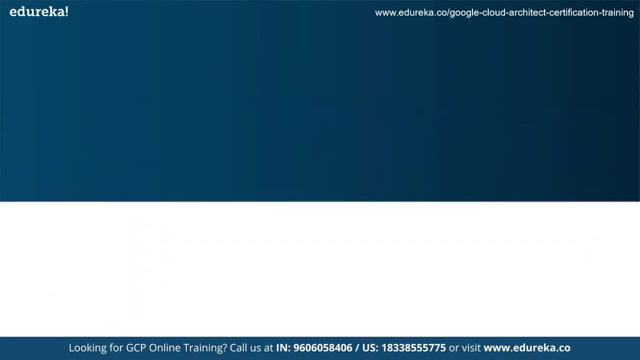 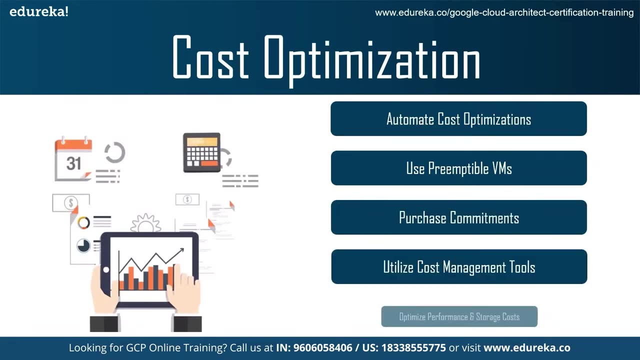 using only the monitoring UI and well-named transforms. Then, moving on to the second category, that is, cost optimization. So one of the best practices for cost optimization is to automate it, like automating the task, and reduce manual intervention. Automation is simplified using a label, which is a key value pair applied to various Google. 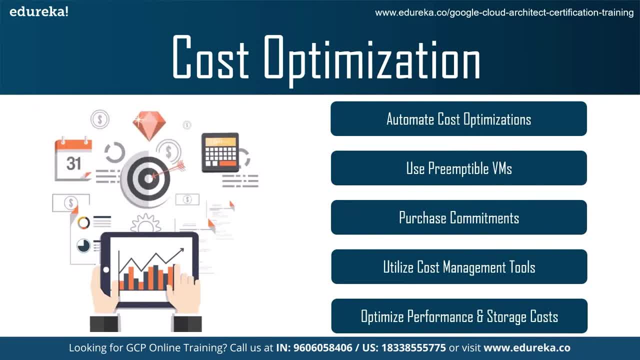 cloud services. You can attach a label to each resource, such as compute instances, then filter the resources based on their labels. So the second best performance under cost optimization is using preemptible virtual machines. As with most trade-offs, the biggest reason to use a preemptible virtual machine is cost. 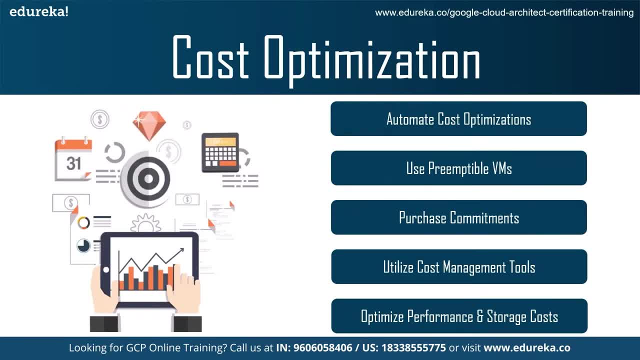 So preemptible virtual machines can save up to 80% compared to a normal on-demand virtual machine. This is a huge savings if the workload you are trying to run consists of short-lived processes or things that are not urgent and can be done anytime. 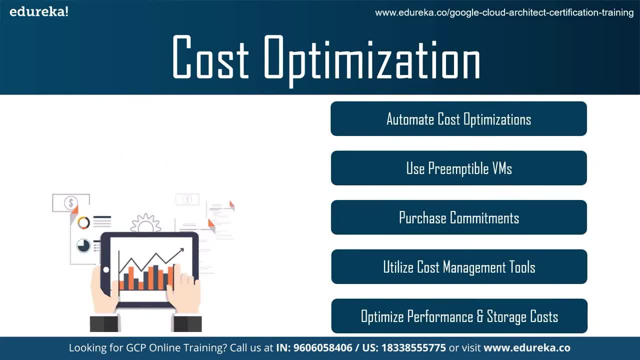 The third one is purchase commitments. The sustained usage Customized discounts are a major differentiator for GCP. They apply automatically once your instance is online for more than 25% of the monthly billing cycle and can net you a discount of up to 30% depending on instance type. 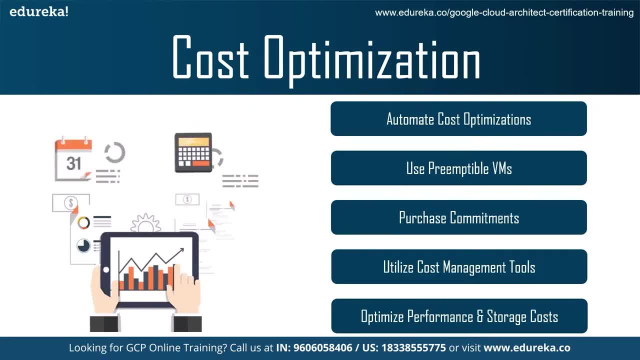 You can combine sustained and committed use discounts, but not at the same time. Committed use can get you a discount of up to 57% for most instance types and up to 70% for memory optimized types. Fourth is: utilize cost management tools that take action. 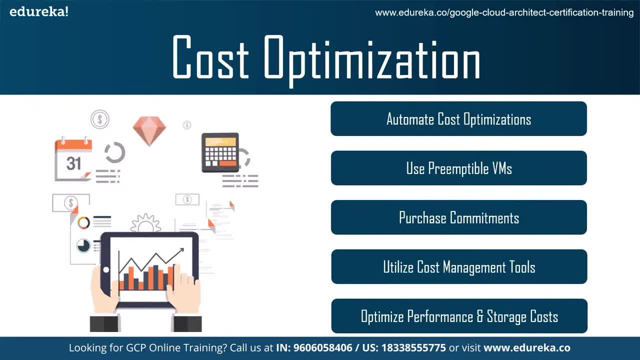 Using third-party tools for cloud optimization helps with cost optimization. Make sure you aren't just focusing on cost visibility and recommendations, but find a tool that takes the extra step and takes those actions for you. This automation reduces the potential for human error and saves organization time and 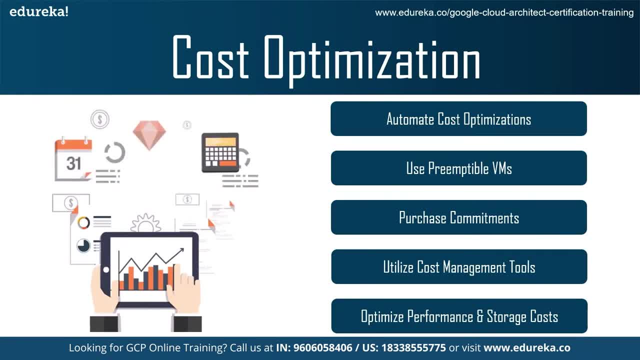 money by allowing developers to reallocate their time to more beneficial tasks. The last best performance in cost optimization is optimized performance and storage costs In the cloud, where storage is billed as a separate line item. paying attention to storage configuration and configuration can result in substantial cost savings and storage needs. 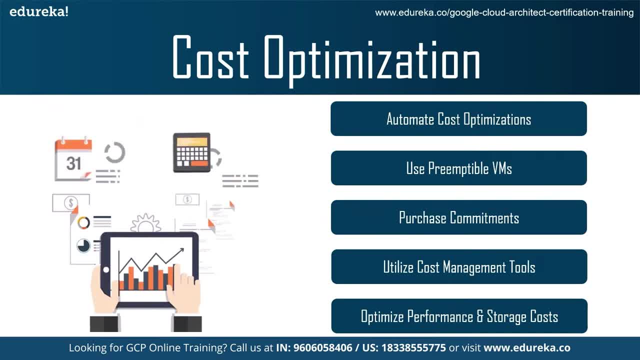 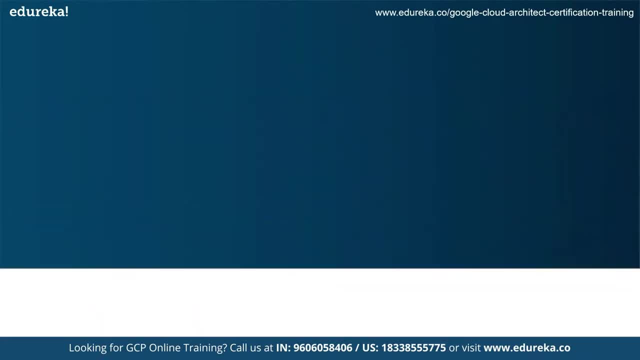 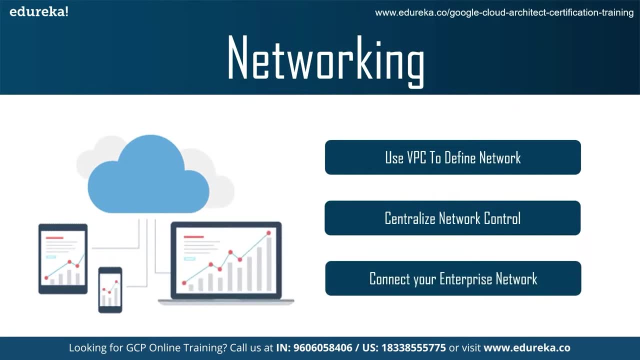 like compute, are always changing. It's possible that the storage class you picked when you first set up your environment may no longer be appropriate for a given workload. Moving on to the next category, that is networking. So the first best performance in networking is use virtual private cloud to define your 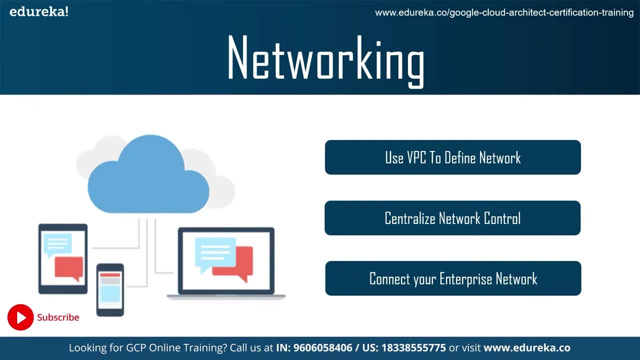 network. So use VPCs and subnets to map out your network and to group and isolate related sources. Virtual private cloud is one of the best performance in networking. Virtual private cloud is a virtual session of a physical network. Virtual private cloud networks provide scalable and flexible networking for a compute engine. 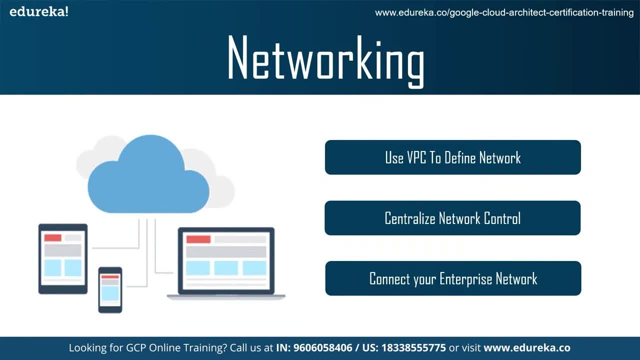 virtual machine instances and for the services that leverage virtual machine instances, including Google Kubernetes, engine, data proc and data flow, among others. VPC networks are global resources. A single VPC can span multiple regions without communicating over the public internet. This means you can connect and manage resources distributed across the globe from a single. 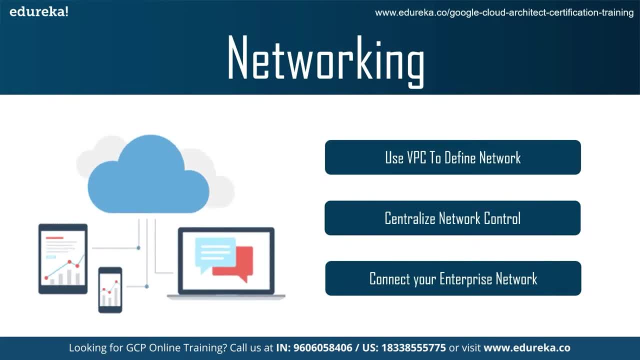 Google cloud project, And you can create multiple isolated VPC networks in a single project. VPC networks themselves do not define IP addresses ranges. Instead, each VPC network consists of one or more partitions called subnetworks. Each subnet in turn defines one or more IP address ranges. 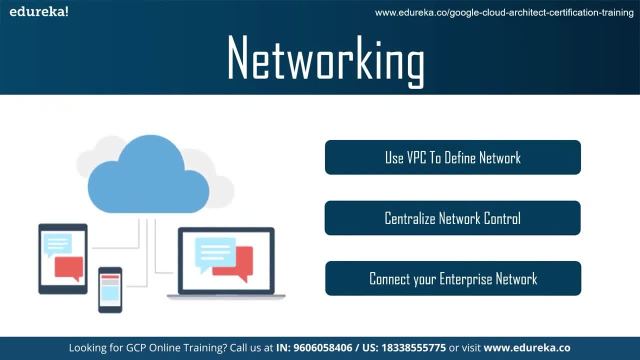 Subnets are regional resources. Each subnet is explicitly associated with a single region. Then we have centralized, like you have to centralize, the network control. So use shared VPC to connect to a common VPC network. Resources in those projects can communicate with each subnet. 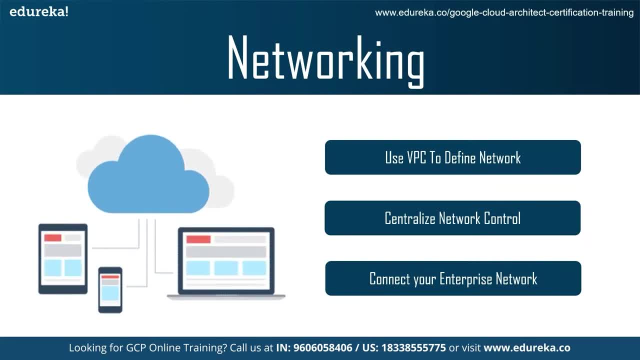 Each other, security and efficiently across project boundaries. using internal IPs, You can manage shared network resources, such as subnets, routes and firewalls, from central host project, enabling you to apply and enforce consistent network policies across the projects. With shared VPC and IAM controls, you can separate network administration from project. 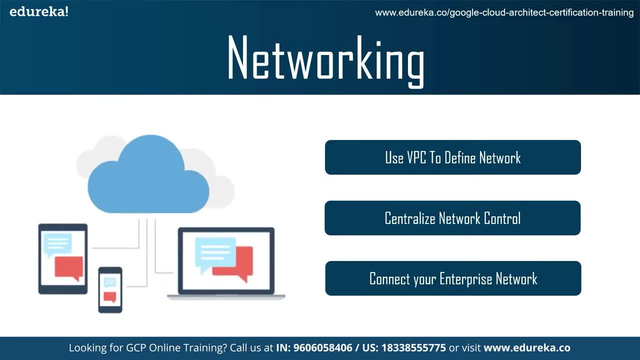 administration. This separation helps you implement the principle of least privilege. For example, a centralized network team can administer the network without having any permissions into the participating projects. Similarly, the project admins can manage their project resources without any permissions to manipulate the shared network. 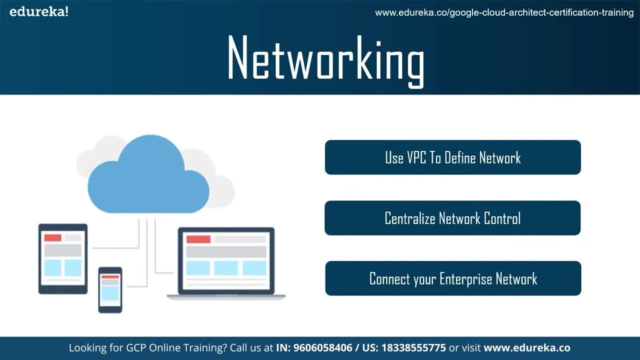 Then connect to your enterprise network. So many enterprises need to connect existing on-premises infrastructure with their Google cloud resources. Evaluate your bandwidth, latency and SLA requirements to choose the best connection option If you need low latency, highly available, enterprise-grade connections that enable. 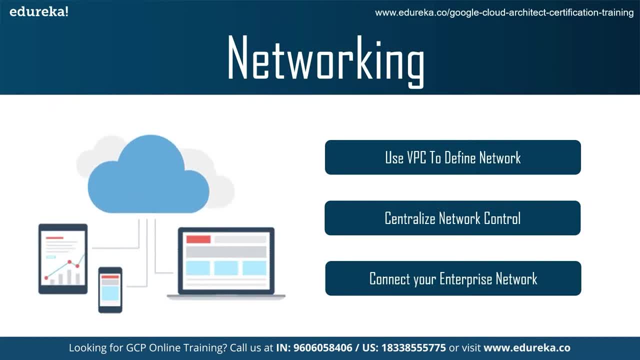 you to reliably transfer data between your on-premises and VPC networks without reversing the internet connections, Then use cloud interconnect. and if you don't require the low latency and high availability of cloud interconnect or you are just starting on your cloud journey, then use cloud VPN. 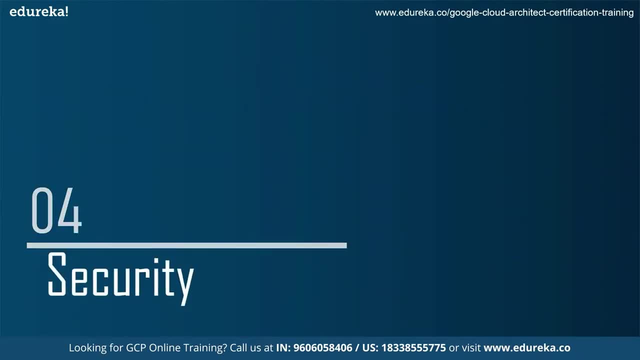 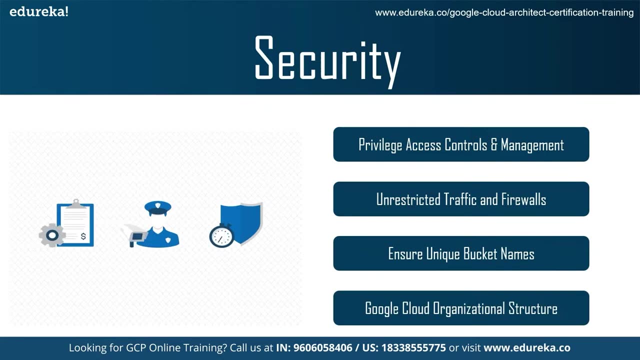 Now moving on to the next category of best practices, that is, security. So under this first one is like: apply least privilege, access controls or identity and access management. The principle of least privilege is a critical foundation element in GCP security. The principle is the concept of only providing employees with access to applications and 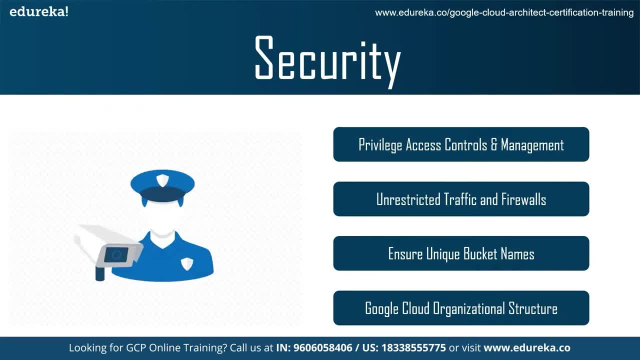 resources they need to properly do their jobs. Second is the manage unrestricted traffic and firewalls. Limit the IP ranges that you assign to each firewall to only the networks that need access to those resources. GCP's advanced VPC features allow you to get any granular with traffic by assigning targets. 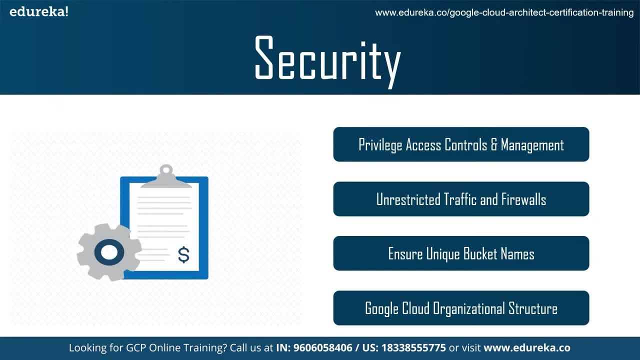 by tag and service accounts. This allows you to express traffic flows logically in a way that you can identify later, such as allowing a front-end service to communicate to virtual machines in a back-end service or service account. And the third one is ensure your bucket names are unique across the whole platform. 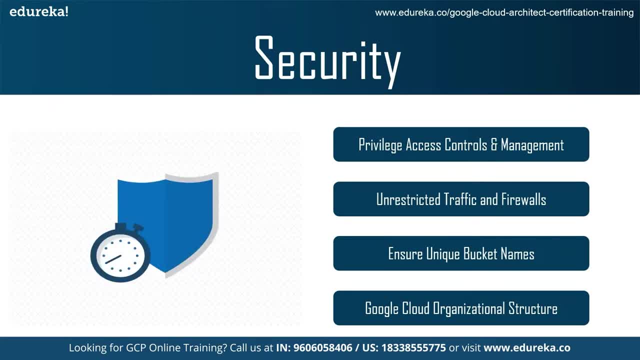 It is recommended to append random characters to the bucket name and not include the company name in it. This will make it harder for an attacker to locate buckets in a targeted attack. Fourth is set up a Google Cloud organizational structure. When you first log into your Google admin console, everything will be grouped into a. 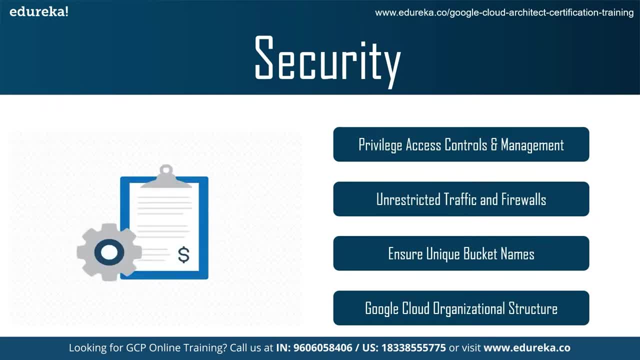 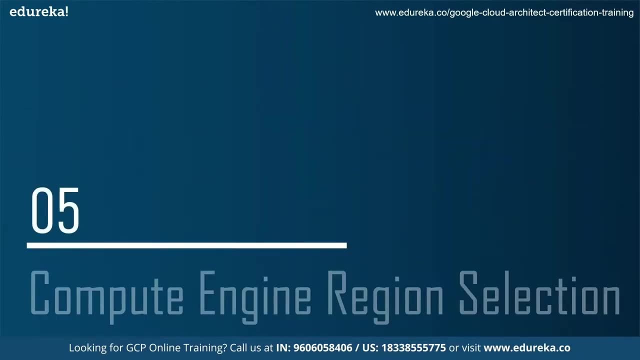 single organizational unit. Any settings you apply to this group will apply to all the users and devices in the organizations. Planning out how you want to organize your units and hierarchy before diving in will help you save time and create a more structured security strategy. Moving on to the next category: compute engine region selection. 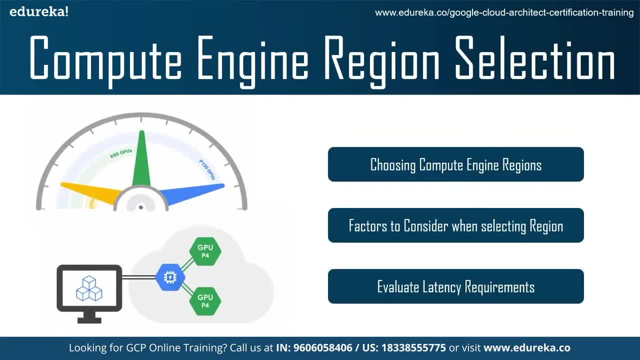 The first one in this is when to choose your compute engine region. So early in the architecture phase of an app, decide how many and which compute engine regions to use. Your choice might affect your app. For example, architecture of your app might change if you synchronize some data between. 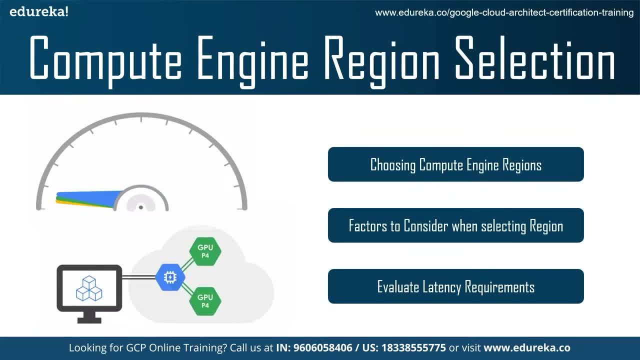 copies because the same users could connect through different networks. This is important. Also, the process to move an app and its data between regions is cumbersome and sometimes costly, So should be avoided once the app is live. Second is we need to see the factors to consider while selecting regions. 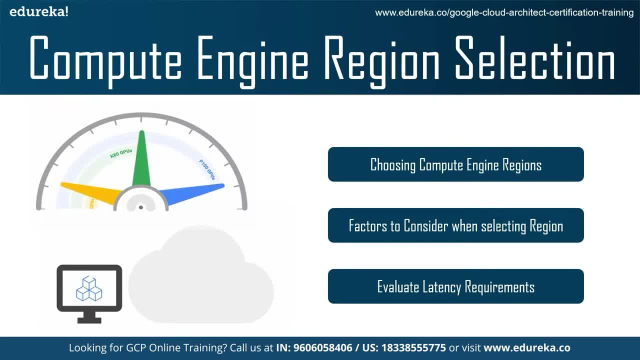 There are multiple factors where you decide to deploy your app. So first factor is latency. However, this is a complex problem because the user latency is affected by multiple aspects, such as caching and load balancing mechanisms. In enterprise use cases, latency to on-premises systems is a very common problem. 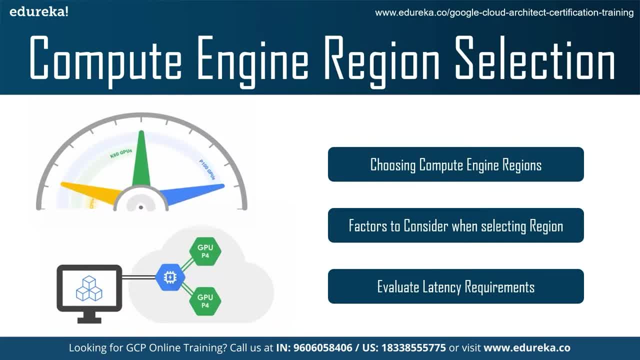 This is because the user latency is affected by multiple aspects, such as caching and load balancing mechanisms. In enterprise use cases, latency to on-premises systems is very common. This is because the user latency is affected by multiple aspects, such as caching and load. 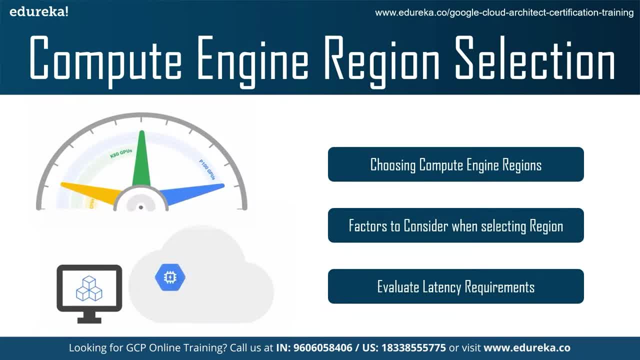 balancing mechanisms. So this is because the user latency is affected by multiple aspects, such as caching and load balancing mechanisms, and the second factor affecting is price. Google cloud resources is cost different by region, So all resources available to estimate prices are the compute engine pricing calculator. 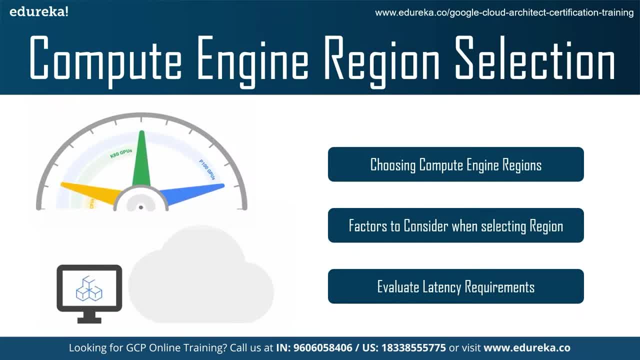 the billing API, Google Cloud, SKU, and so on. So the second factor affecting is price. If you decide to deploy in multiple regions, be aware that there are network charges for data synced between regions. and the third factor affecting is co-location with other Google cloud services. 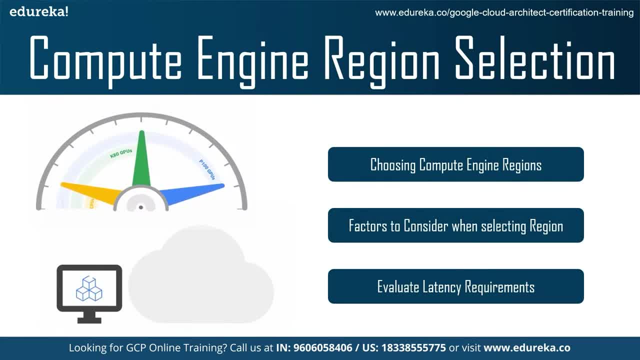 The third factor affecting is co-location with other cloud services, So color Google cloud services wherever possible. While mostly sensitive services are available in every region, some services are available only in specific locations. Fourth factor affecting is machine type availability. Not all CPU platforms and machine types are available in every region. 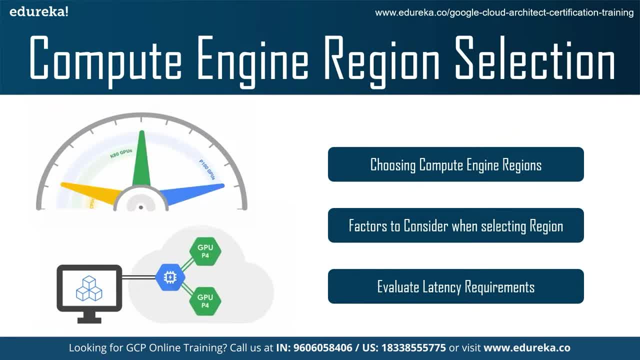 The availability of specific CPU platforms or specific instance type differ by region and even zone. The fifth factor affecting is resource quotas. Your ability to deploy compute engine resources is limited to regional resources quotas, So make sure that you request sufficient quota for the regions you plan to deploy. in Moving on to the third best practice, that is, 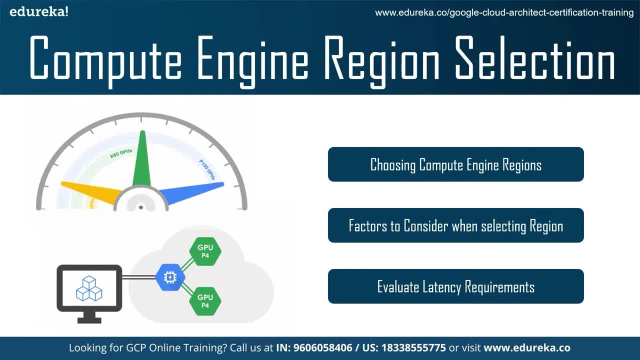 evaluating latency requirements. So latency is often the key consideration for your region selection, because high user latency can lead to an inferior user experience. You can affect some aspects of latency but some are outside of your control. Region selection can only affect the latency to the compute engine region and not like entirety of the latency. So the first one in this: 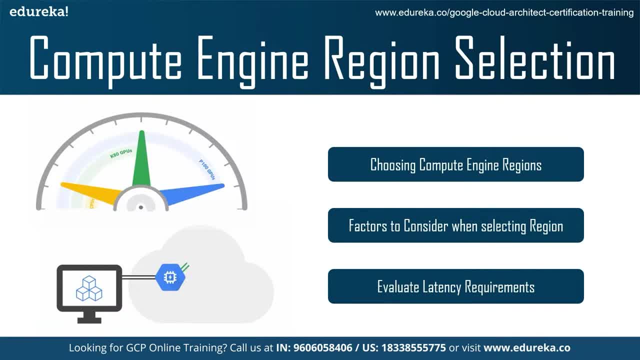 is a last mile latency. The latency of the segment differs depending on the technology used to execute the latency. So the first one in this is a last mile latency. The latency of the segment is the internet. Then the second one is a Google front-end and edge pop latency. These are like 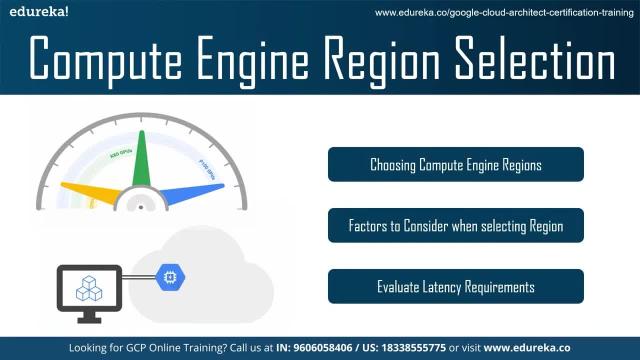 subcategories under: evaluate latency requirements, best practices. So second subcategory I mean is Google front-end and edge pop latency, Depending on your deployment model. the latency to Google's network edge is also important. This is where Google load balancing products terminate TCP and 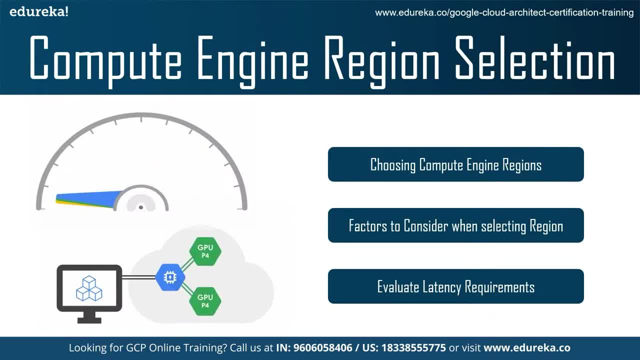 SSL sessions and from which cloud Syrian delivers cache results Based on the content serve. many round trip might already end here because only part of the data is available. So the second one in this subcategory is the network latency of the segment. So the third subcategory is the network. 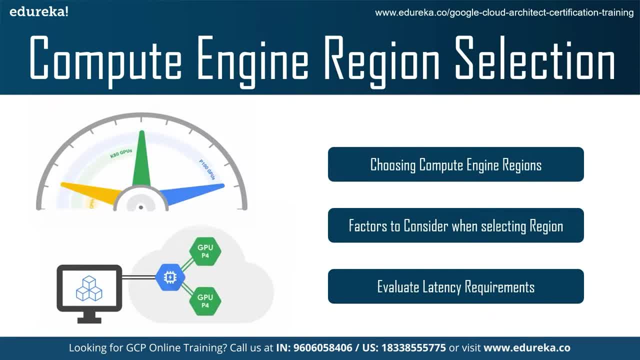 latency of the segment. So in the data data we have, the data needs to be retrieve the whole way. So moving on to the third subcategory is compute engine region latency. So in compute engine region latency the user request enters Google's network at the edge, pop, the compute engine region is. 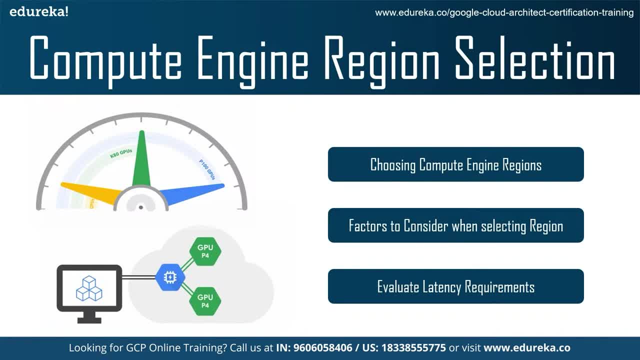 where Google cloud services are handing request are located. This segment is the latency between the edge pop and compute engine region, and it's so wholly within Google's global network. So the four app users are more forgiving of latency issues, apps that interact asynchronously or mobile apps. 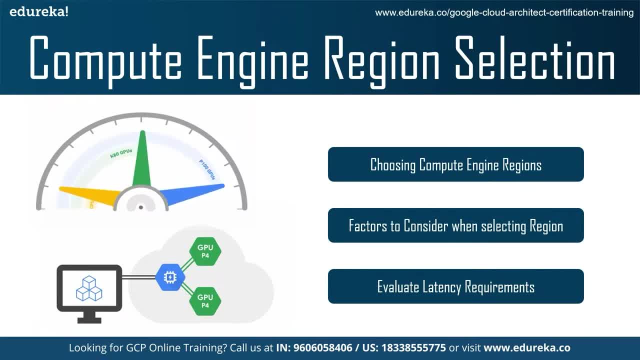 with a high latency threshold- 100 milliseconds or more- can be deployed in a single region without degrading the user experience. however, for apps such as real-time games, or a few milliseconds of latency can have a greater effect on user experience. deploy these types of apps in multiple 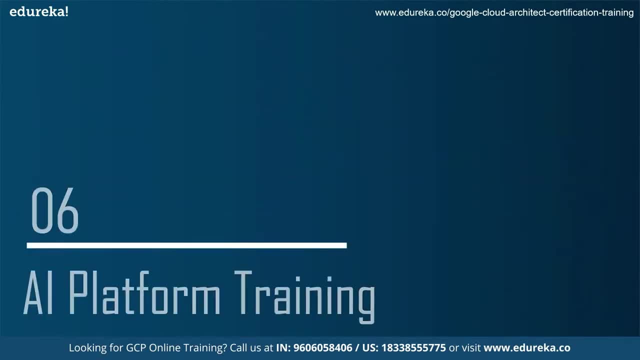 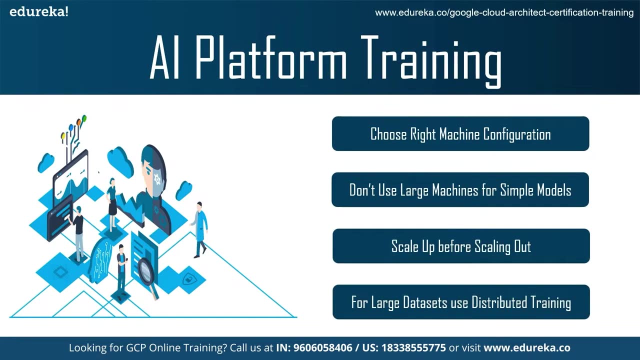 regions close to the users. now moving on to the next category, that is, ar platform training. we have different best practices under ar platform training also, so the first one is choose the right machine configuration for your training characteristics. you can choose arbitrary machine types and various gpu types. the machine configuration that you choose depends on your data. 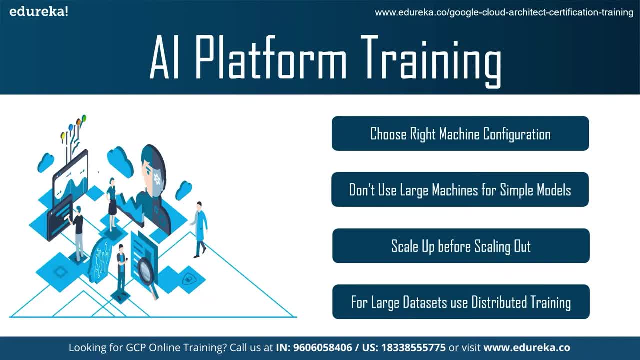 size, model size and algorithm selection. for example, deep learning frameworks like tensorflow and pytorch benefit from gpu acceleration, while frameworks like scikit-learn and xgboost don't. on the other hand, when you are training a larger cycle model, you need a memory optimized machine. 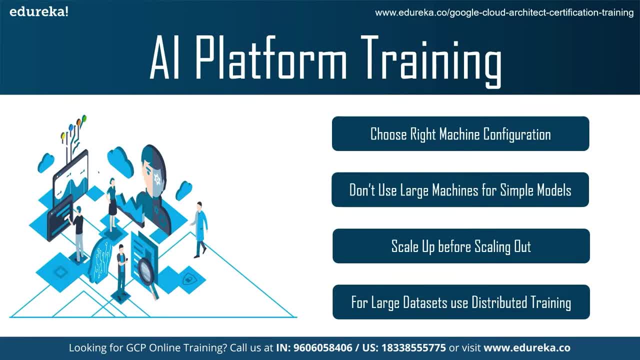 okay. so the second one in this is: don't use large machine for simple models. simple models might not train faster with the gpus or with distributed training, because they might not be able to benefit from increased hardware parallelism, because the scikit-learn framework doesn't support distributed 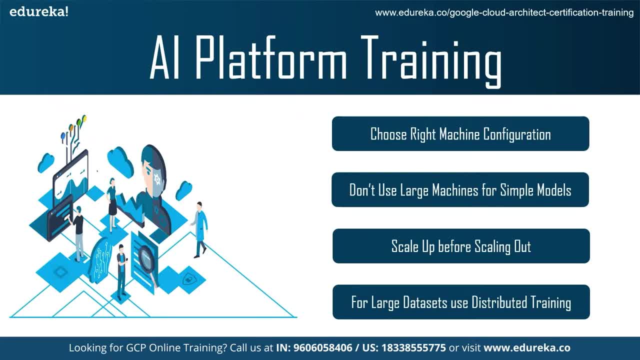 training, make sure that you use only the scale tire or custom machine type configurations that correspond to a single worker instance. and the third: best performance is scale up before scaling out. so scaling up instead of scaling out while experimenting can help you identifying the configurations that are performant and cost effective. for example, start by using a single worker that has a 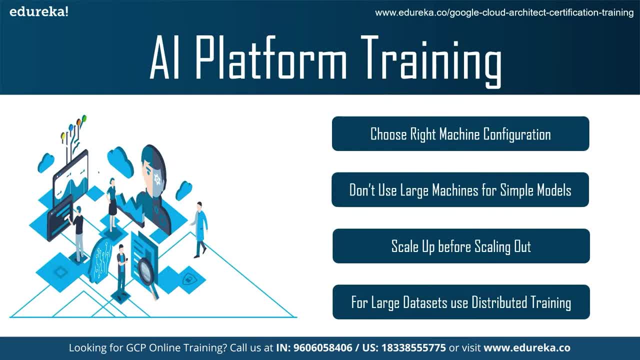 single gpu and then try a more powerful gpu before you use multiple gpus. after that, try distribute training, as discussed later in the section. scaling up is faster than scaling out because network latency is much slower than the gpu interconnect. and the fourth best performance under ar platform training is for large data sets. use distributed training. so if a gpu has high buffer and can be used for simpleدistributed training. you need to be more flew, better than TCP orícioverumu, and you cannot use multiple audios. that should be up to allillar easy. and the fourth: best performance under platform training is: forge data sets. use distributed training, so 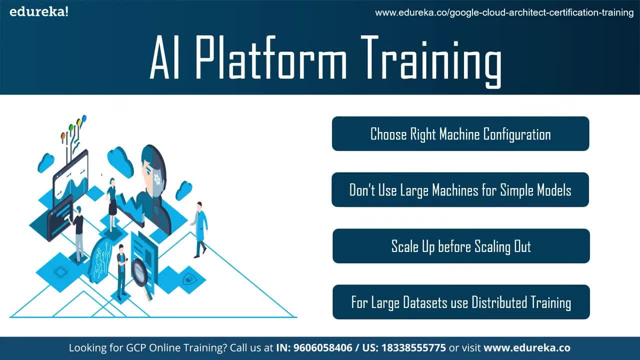 fourth, best performance under ar platform training is a: for large data sets. use distributed training, so distributed training, So distributed training platforms. data parallelism on a cluster of nodes to reduce the time required to train a TensorFlow model. when you use a large dataset, Make sure that 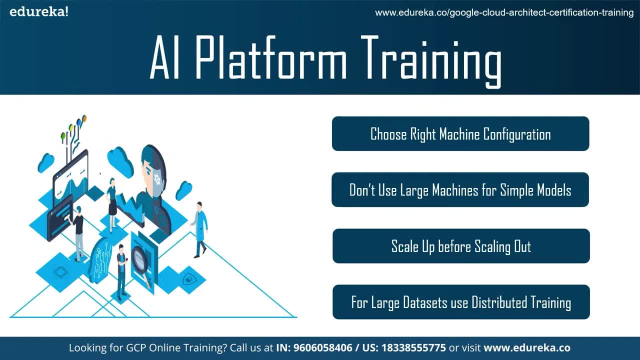 you adjust the number of iterations with respect to the distribution scales. That is, take the total number of iterations that are required and divide the total by number of GPUs multiplied by the number of work nodes. I hope you have understood all the best practices under Google Cloud Platform. 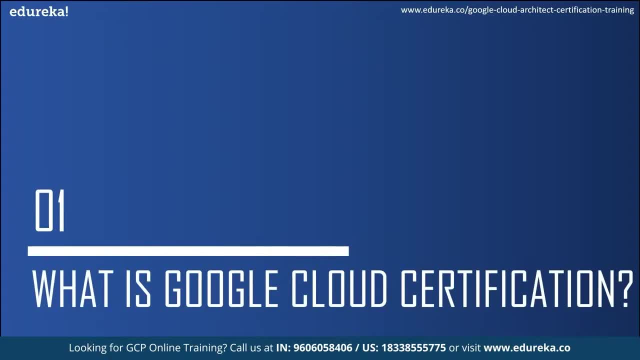 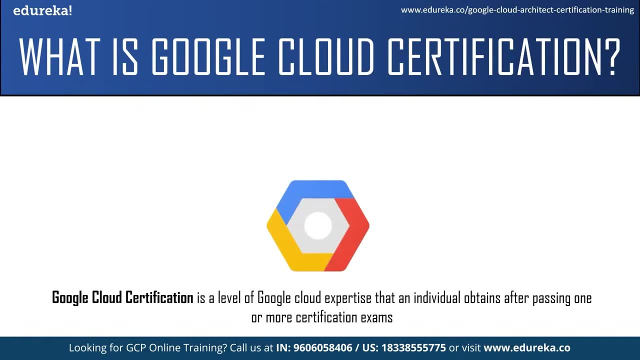 What exactly is Google Cloud Certification? Well, Google Cloud Certification is a level of Google Cloud expertise that an individual obtains after passing one or more certification exam. The certification validates your cloud expertise and helps you showcase your ability to help company and businesses with Google Cloud technology. Now some of the reasons to get a Google Cloud. 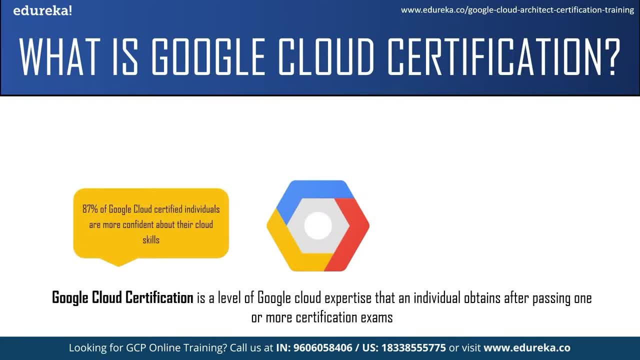 Certification would be. you will be more confident about your cloud skills. According to the survey response from the 2020 Google Cloud Certification, you will be more confident about your cloud skills Next, the professional cloud architect was the highest paying certification of 2019 and also. 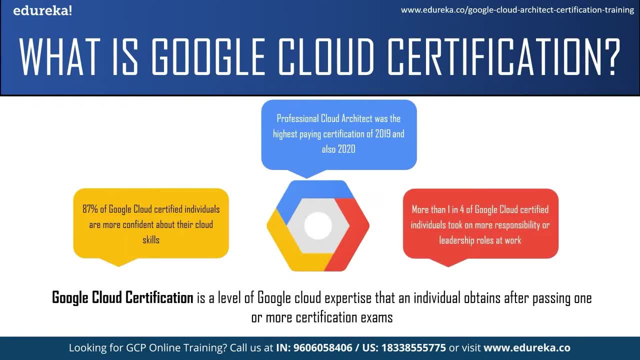 2020.. Next, more than one out of four Google Cloud Certified individuals to call more responsibility and leadership roles at their work. Now, a company or an organization is more likely to work with an individual who is certified rather than a person who isn't. Now, a company or an organization is. 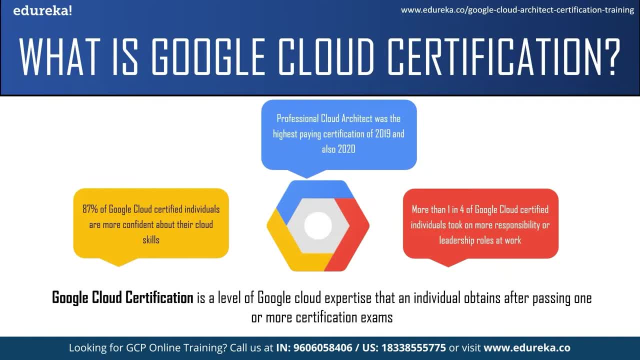 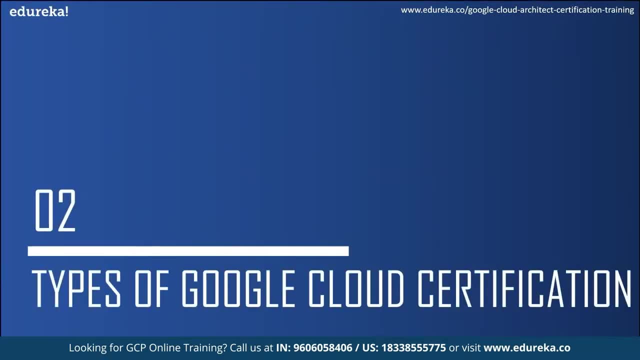 more likely to work with an individual who isn't. This is because the certification acts as a proof that you have knowledge about Google Cloud and you have worked on it. before Now, this was about Google Cloud Certification. Now let us move on to our next topic and see the types of certification There. 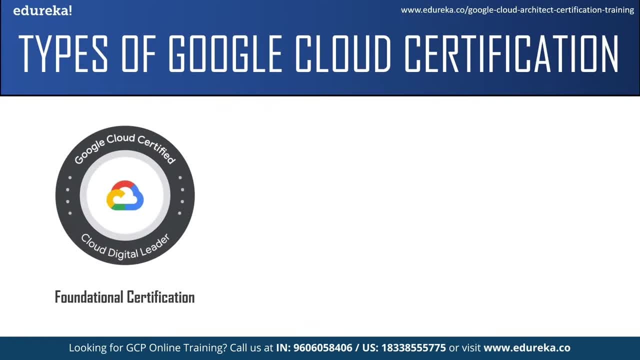 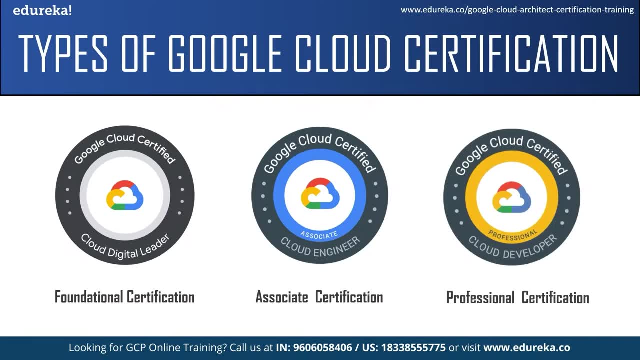 are three levels of Google certification. First is the foundational certification, Next is the associate level certification and then comes the professional level certification. Now let us discuss about them one by one. The fundamental level of certification validates broad knowledge of cloud concepts, customer practices and information about cloud Through the interpretation and the 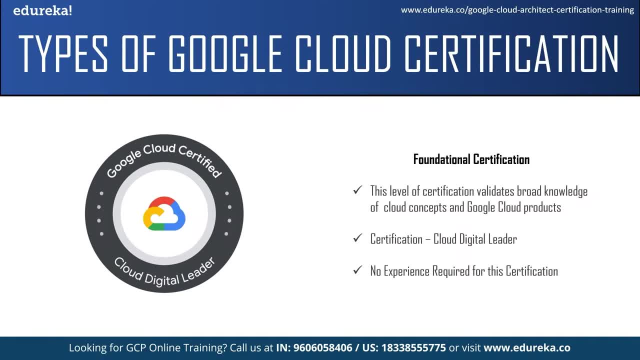 and Google Cloud products, services, tools, features, benefits and use cases. To sum it up, you should basically understand the capabilities of Google Cloud. Now, in this level of certification, there is only one certificate, which is the cloud digital leader. 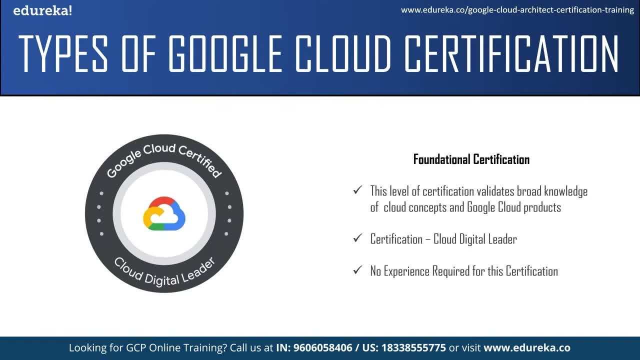 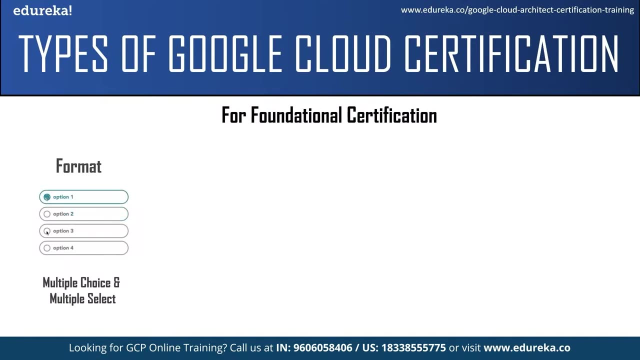 This certification is appropriate for individuals in a non-technical job role who wants to add value to their organization by gaining cloud knowledge. This certification is also for someone who has little or no hands-on experience working on the Google Cloud. In the foundational certification, multiple choice and multiple select types of questions are asked. 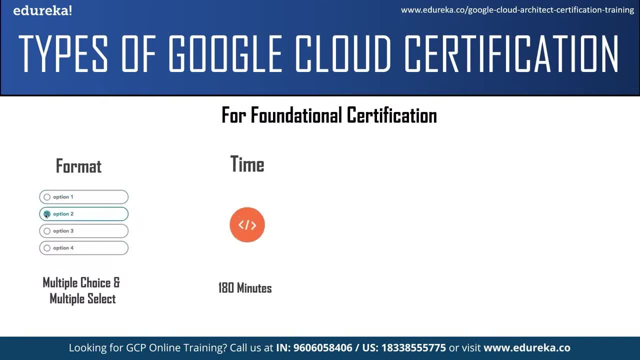 You will have three hours to complete this examination and the registration fees for this examination is $99.. You can write this examination in English. You can either write it online or in a test center near you. The next level of certification is the associate level. 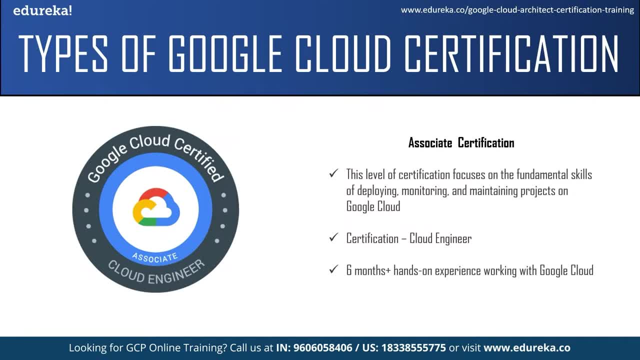 This level of certification focuses on the fundamental skills of deploying, monitoring and maintaining projects on Google Cloud. In this level of certification also, there is only one certificate, which is the cloud engineer. Now, this certification is a good starting point for those who are new to cloud. 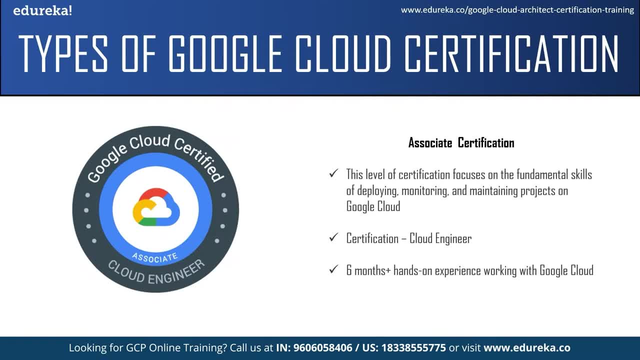 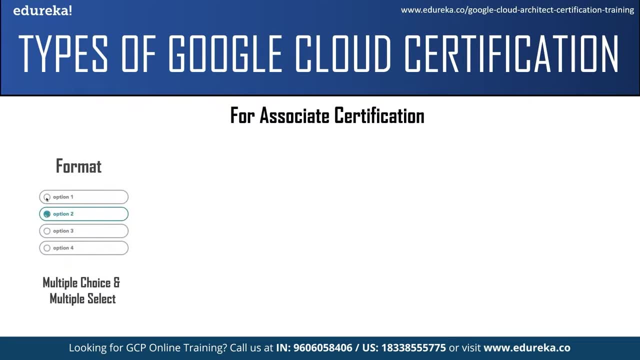 and can be used as a path to professional level certifications. It requires at least six months of work experience working on the Google Cloud. The types of questions which are asked in the associate examinations are also multiple choice and multiple select. But you will have only two hours to complete this exam and the registration fees for this examination is $125 plus taxes. 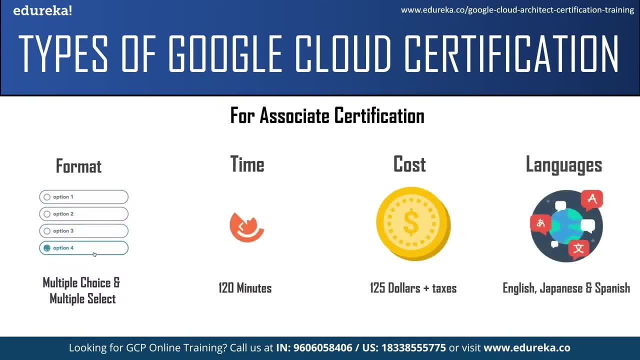 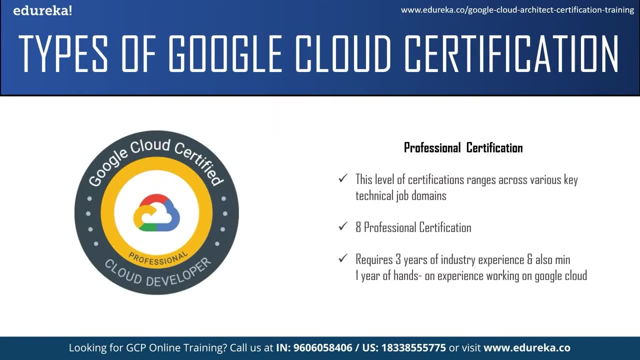 You can write this examination in English, Japanese or Spanish. The last level of Google certification is the professional level. This level of certification ranges across various key technical job functions and accesses advanced skills in design, implementation and management. The certifications are recommended for individuals with industry experience and familiarity with Google Cloud products and solutions. 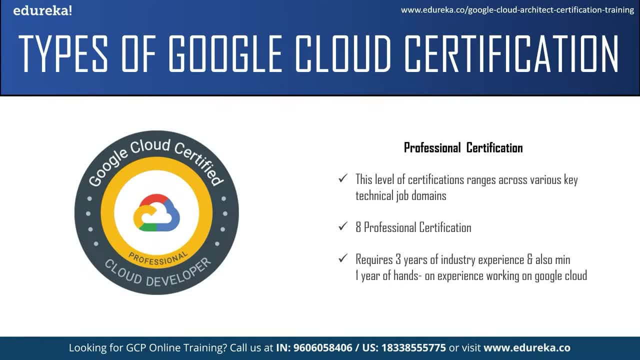 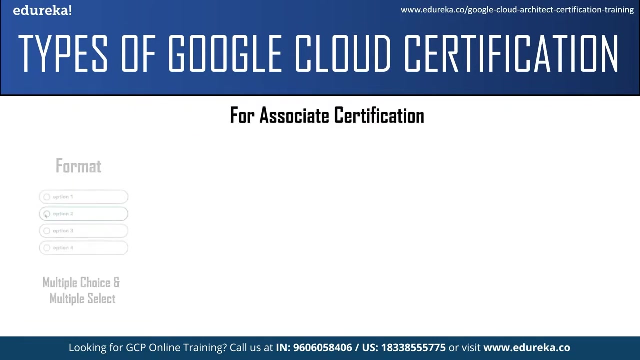 There are eight professional cloud certifications in Google, which are the cloud architect, cloud developer and cloud engineer, Cloud engineer, cloud machine learning engineer, Cloud network engineeruckle engineer, cloud devops engineercollaboration engineer and machine engineering engineer. 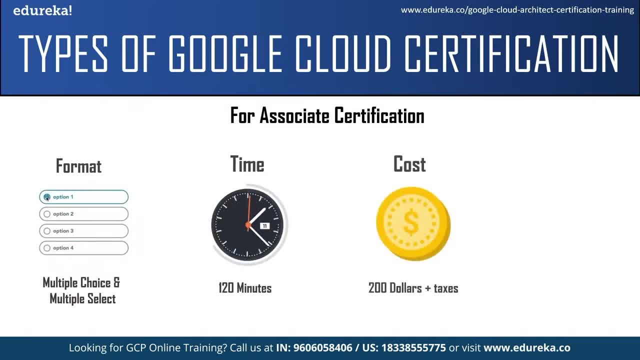 This certification level requires three years of industry experience, more than one year of hands-on experience working on the Google Cloud. The types of questions which are asked in the associate examinations are also multiple choice and multiple select. this examination in English. Now some of the professional certification exam can also be. 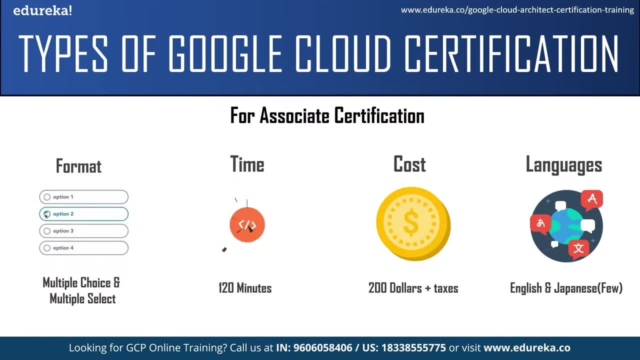 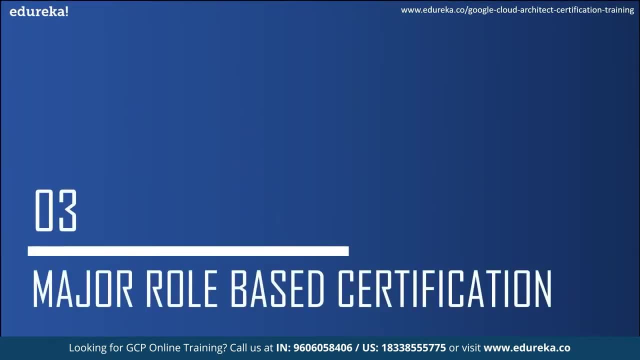 written in Japanese. You can either write this examination online or in a test center near you. Now, these were the types of certification. Now let us move on to the next topic and see some of the major role-based certification. We will start by knowing the fundamental level certification. 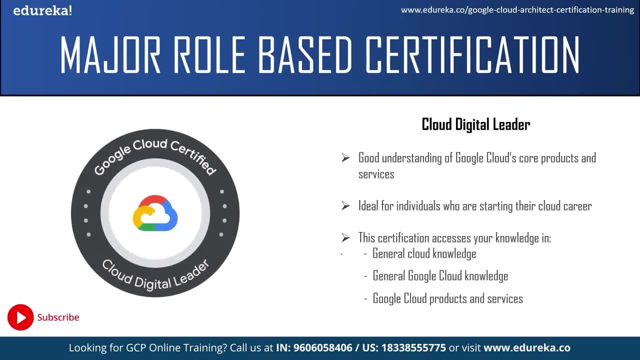 which is cloud digital leader. A cloud digital leader should have good understanding of Google Cloud core products and services and how they benefit the organizations. The cloud digital leaders should understand how the services can be used in real time to solve business problems and how cloud solutions support an enterprise, making it more efficient. This is the only Google 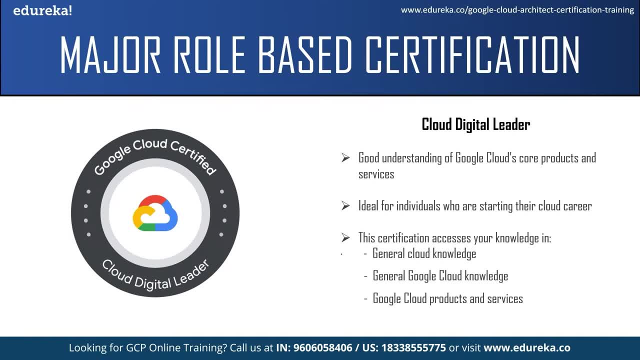 Cloud certification that does not require any previous cloud experience or requires hands-on experience with Google Cloud. So if you're just starting your cloud career and do not know where to begin, while preparing for the certification should be your first step step. The cloud digital leader exam accesses your knowledge in three areas. The first is 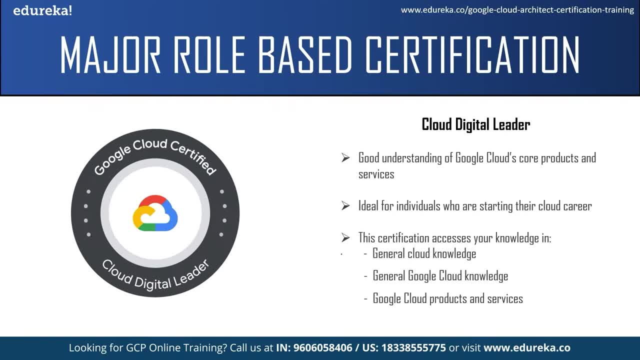 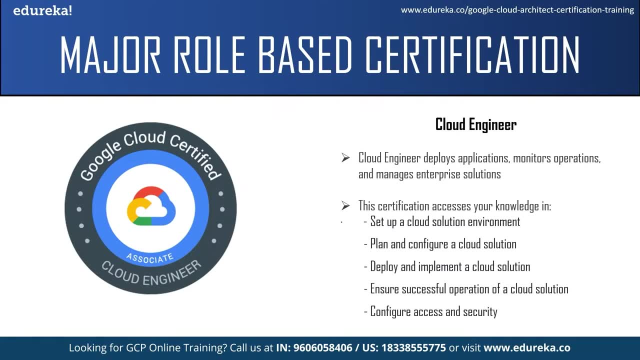 general cloud knowledge. Second, general Google Cloud knowledge and Google Cloud products and services. The next certification we'll talk about is the associate level cloud engineer certification. An associate cloud engineer is expected to deploy application, monitor operations and manage enterprise solution. An individual appearing for the certification. 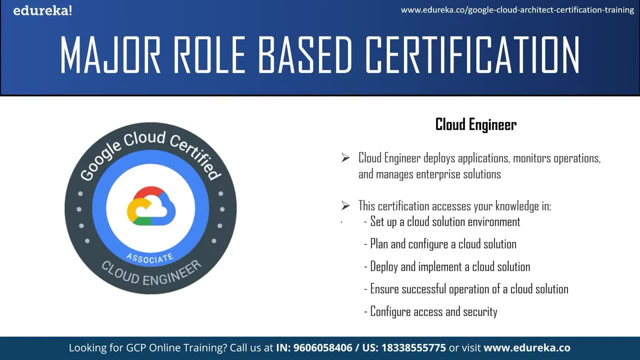 should be able to use Google Cloud console and command line interface to perform common platform based tasks to maintain one or more deployed solution that leverages Google managed or self managed service on Google Cloud. Now for this associate level certification, you will need more than six months of hands on experience working with Google Cloud. The 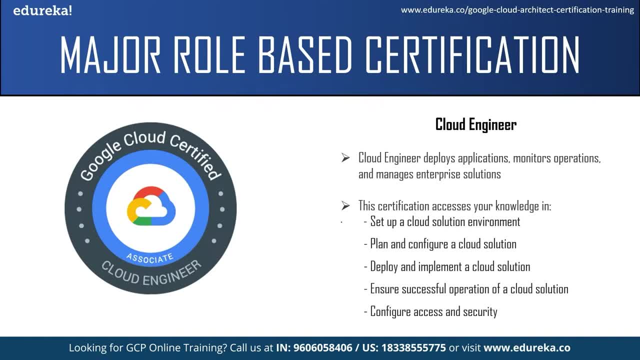 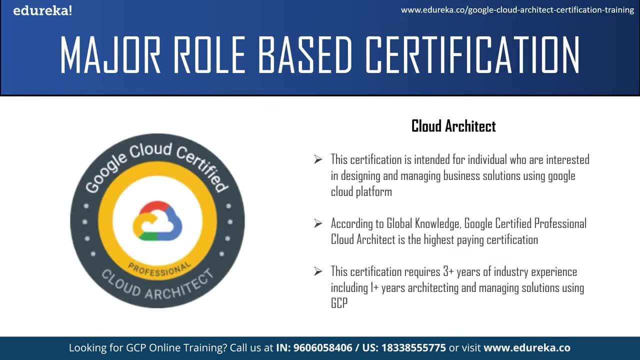 associate cloud engineer exam examines your ability to set up a cloud solution environment plan and configure a cloud solution, deploy and implement a cloud solution and manage a cloud solution and ensure successful operation of a cloud solution, and also configure access and security. The next certification we'll talk about is the professional level cloud. 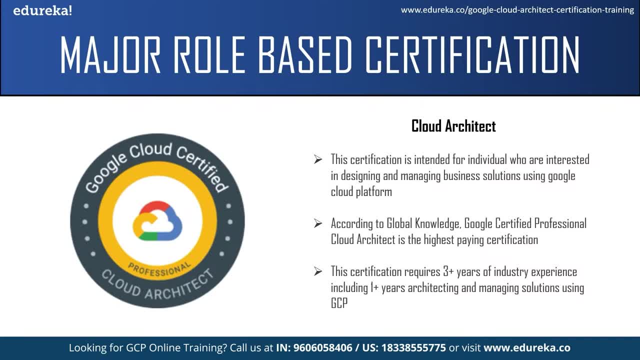 architect certification. The certification is intended for individuals who are interested in designing and managing business solution using Google Cloud platform. According to Google knowledge, Google certified professional cloud architect is the highest paying certification Now. the professional cloud architect should be able to use cloud technologies to manage. 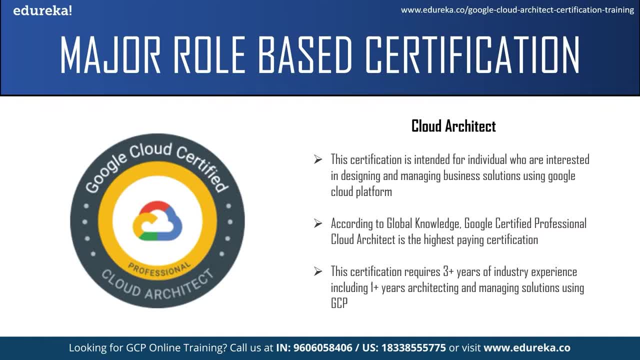 and maximize the benefit for their organization. They should have a thorough understanding of cloud architect and Google cloud platform. They should be able to design, develop and manage robust, secure, scalable, highly available and dynamic solutions to drive business objectives. For this certification, you should have more than three years of industry experience and 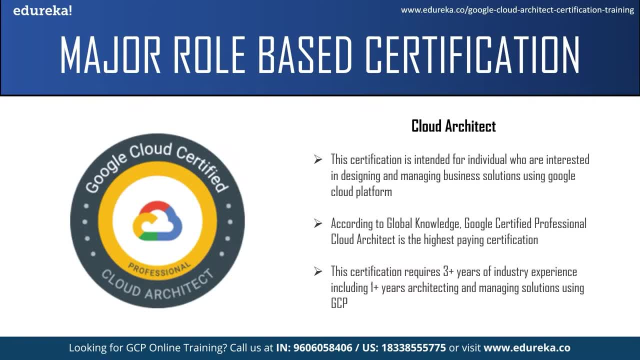 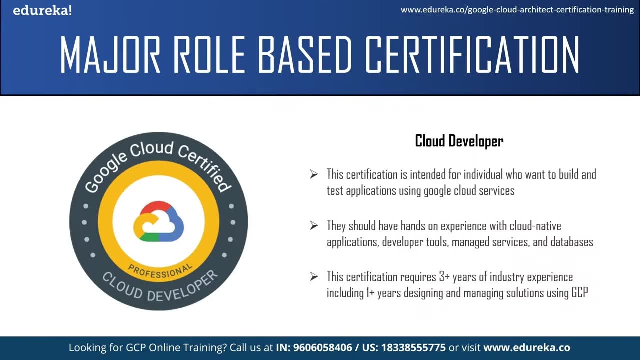 also have one or more year experience architecting and managing solution using GCP. The next certification is the professional cloud developer. This certification is intended for individual who want to build and test application using Google cloud service. A professional cloud developer should be able to build scalable. 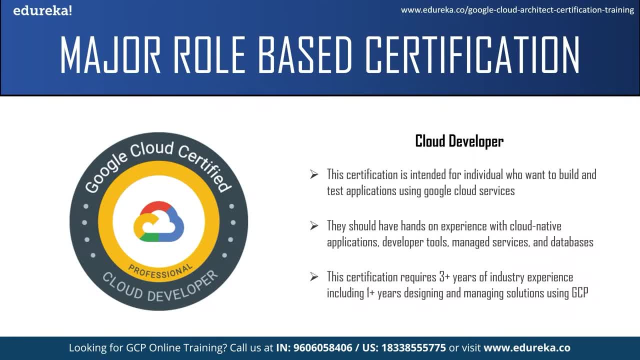 and highly available application using Google recommended practices and tools. It should have hands on experience with cloud native application developer tools, managed services and databases. A professional cloud developer should be skilled with at least one high level programming language and skilled at producing meaningful metrics and logs to debug and trace. 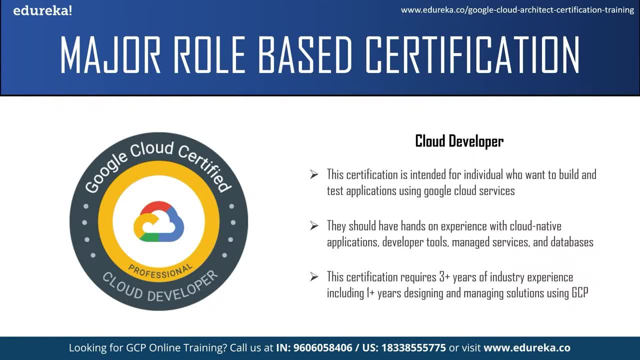 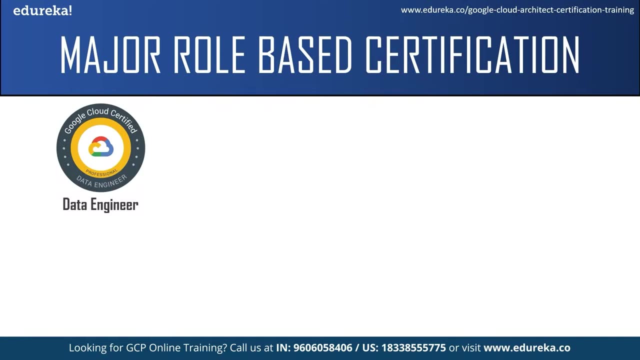 code For this certification. also, it should have more than three years of industry experience and more than one year of experience designing and managing solution using Google cloud. The rest of the professional certifications are the data engineer: This certification is intended for individual who want to design and build data collecting and processing machine. 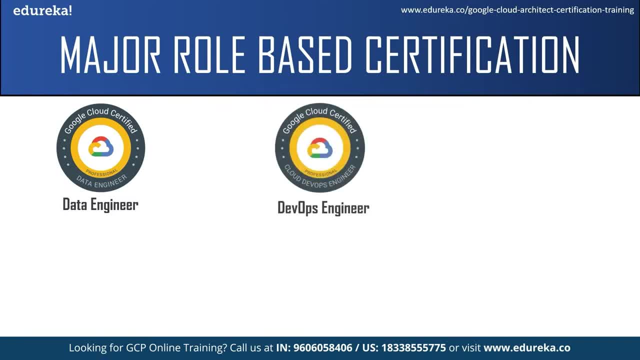 learning models on Google cloud platform. Next, we have cloud DevOps engineer. This certification is intended for individual who want to work as a DevOps engineer. They should be efficient in both and operation and should have good knowledge of various devops tools. 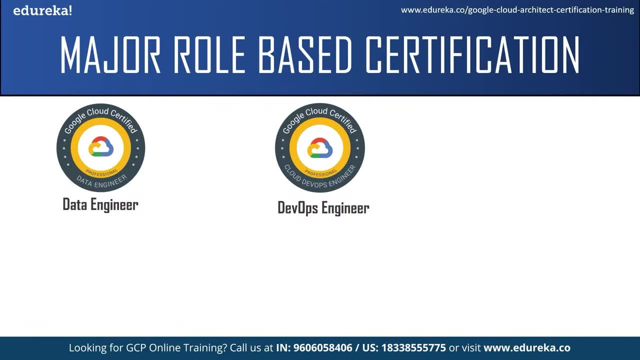 You should build software delivery pipeline, deploy and monitor services. The next certification is cloud security engineer. This certification is intended for security engineer who have good understanding of security best practices and the current industry security requirements. They have to design, develop and manage a secure infrastructure using Google security services. 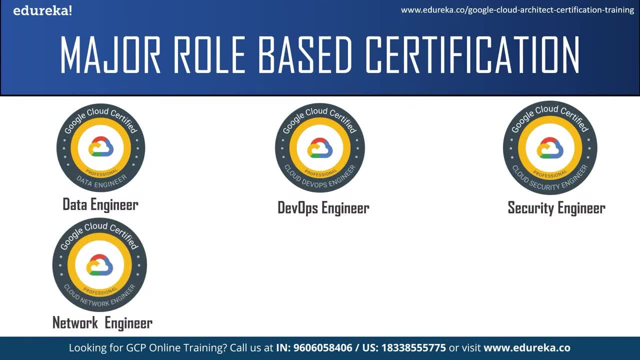 The next professional certification is a cloud network engineer. The certification is intended for individuals who want to design, implement and manage network architecture on Google Cloud Platform. Next is a collaboration engineer. This certification is intended for individual who can understand an organization's main routing and identify management infrastructure and be able to efficiently and securely establish. 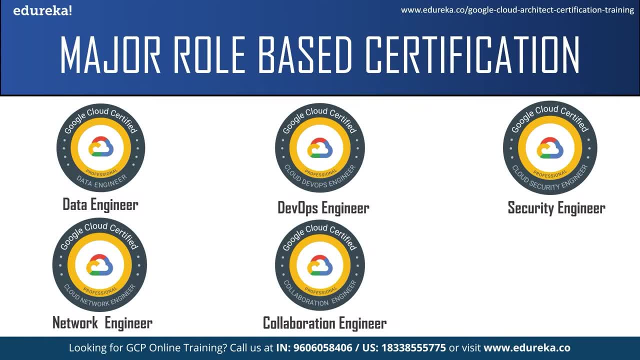 communication and data access. You should have at least one year of Google workspace administration experience. The next certification is the machine learning engineer. This certification is intended for individual who want to design, build and product and eyes ML models to solve business challenges using Google Cloud technologies. 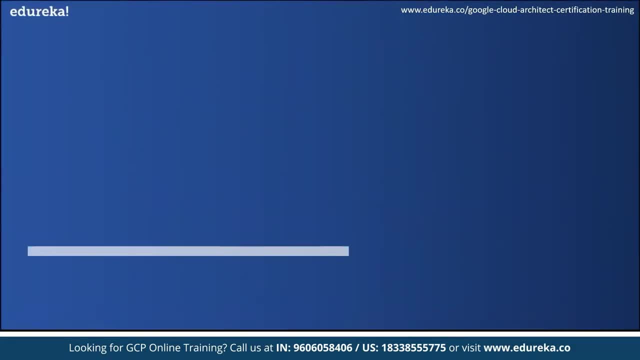 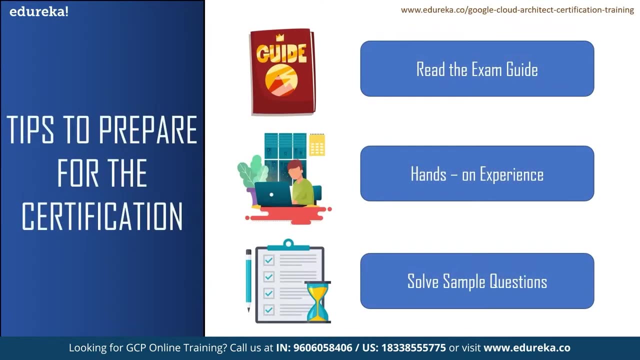 Now, these were the professional level certification. Now we will move on to a final topic for today where I will give you a few tips to prepare for the certification. The first point is: read the exam guide for the certification. Now, before you start practicing for the certification, I would suggest you to go through the exam. 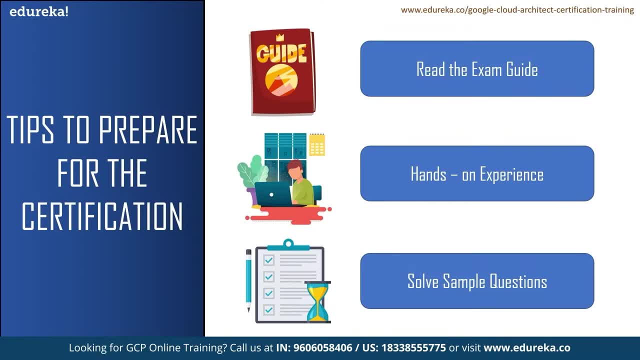 guide. This will give you a clear idea about what topics you should focus on in order to pass the examination. You will find the exam guide in the Google Cloud certification official website. Next, the most important step is hands-on experience. If you are writing any certification examination except the cloud digital leader, you should 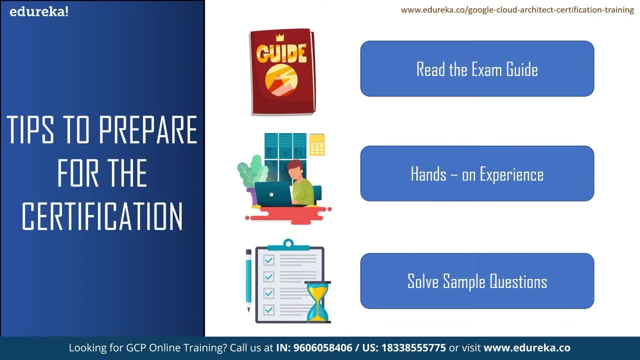 have at least 6 months of hands-on experience working on the Google Cloud. But if you are just starting your career in Google Cloud or want to start your career with Google Cloud, I would highly recommend you using the GCP free trial account. Now Google provides all its new customer with free trial, which offers $300 in free credits. 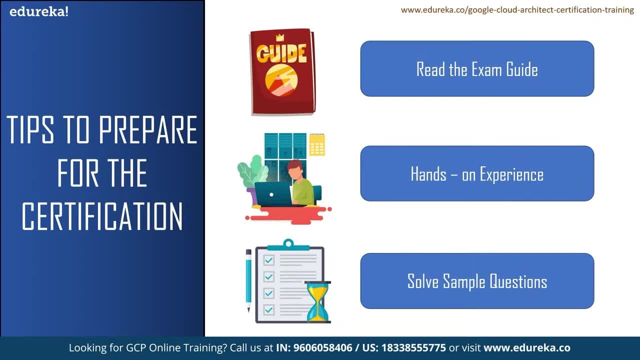 Now. they do this because they want you to fully explore and conduct an assessment on Google Cloud platform. You can use this $300 to try various Google Cloud products and learn how to use them. You won't be charged unless you choose to upgrade and it will be valid for 90 days. 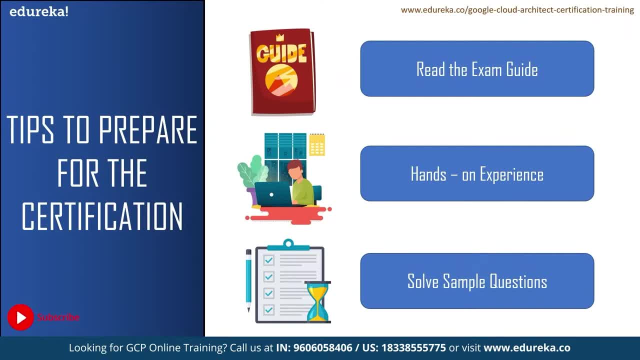 My next suggestion would be solving the sample. The sample questions will familiarize you with the format of the exam question and example content that may be covered on the exam. Now solving the sample questions will help you improve your confidence. We can also refer Google white papers, which will give you technical knowledge about various 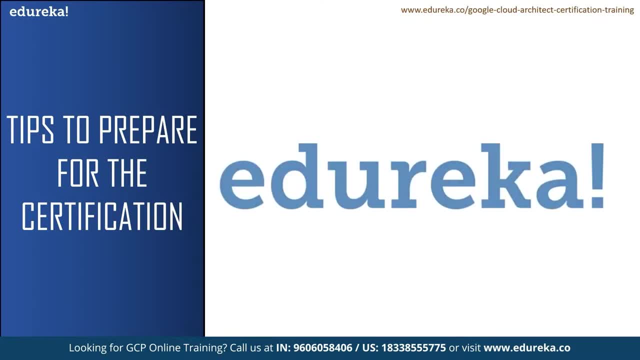 Google Cloud concepts and services. If you want to follow a structured approach, then I would highly recommend you to opt for an online training certification. I would highly recommend Edureka certification training, Which is curated by top industry experts. The certification course consists of demonstration assignments, MCQs and a certification project. 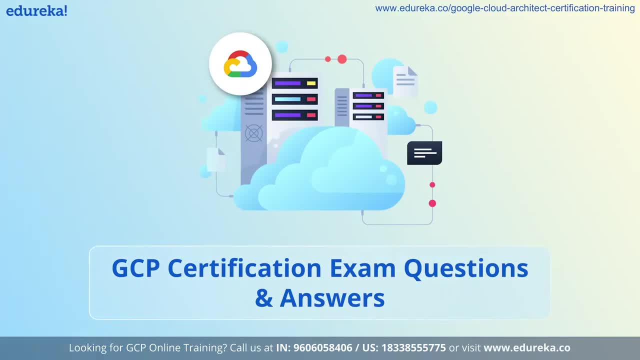 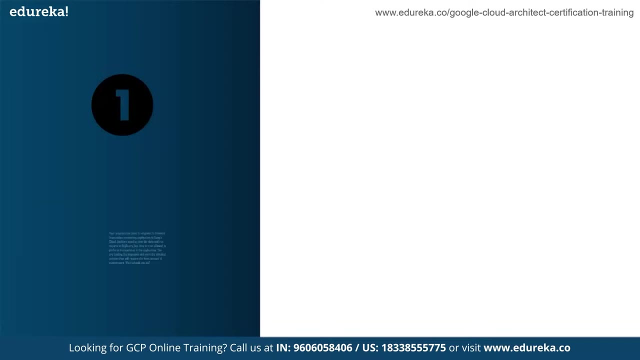 which will help you master the concepts. Let's go through certain exam questions that have been coming for Google Cloud Platform associate certification over the past few years. First up, we have your organization plans to migrate its financial transaction monitoring. Let's go through some of the questions that have been coming for Google Cloud Platform. 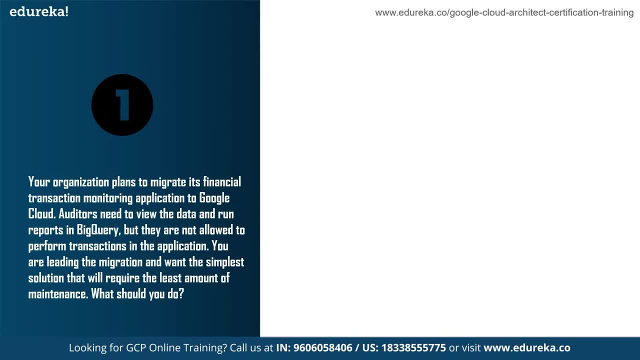 First up, we have your organization plans to migrate its financial transaction monitoring. Let's go through some of the questions that have been coming for Google Cloud Platform associate certification over the past few years. First up, we have your organization plans to migrate its financial transaction monitoring. 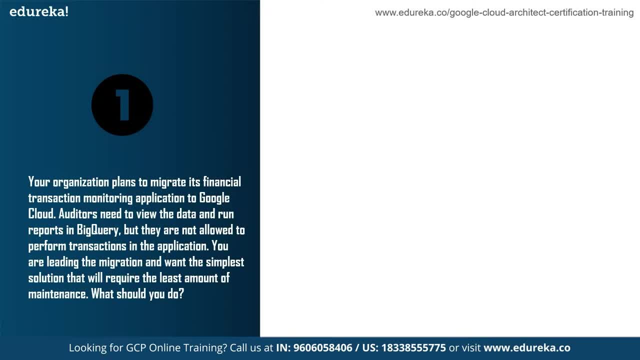 application to Google Cloud. Auditors need to view the data and run reports in BigQuery, but they are not allowed to perform transaction in the application. So you are leading the migration and you want the simplest solution, And what is it that you should do? 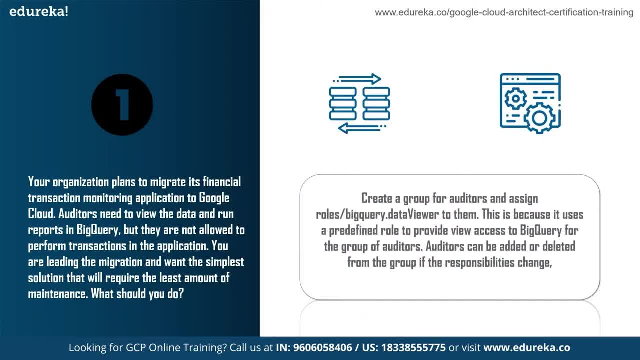 So the answer to this is fairly simple. What you need to do is, since you're working with BigQuery and there are a lot of auditors, what you need to do is create a group of auditors and assign roles to each BigQuery data viewer. 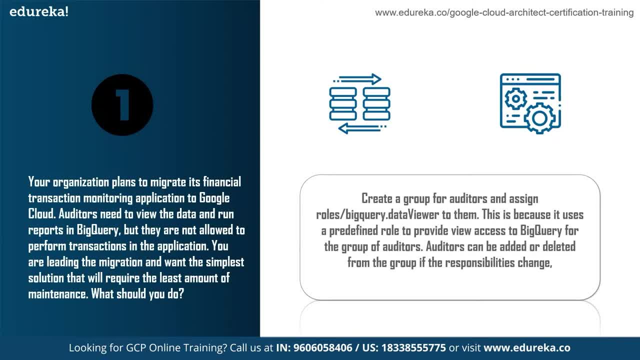 So the answer to this is fairly simple. What you need to do is, since you're working with BigQuery and there are a lot of auditors, what you need to do is create a group of auditors and assign roles to each BigQuery data viewer. 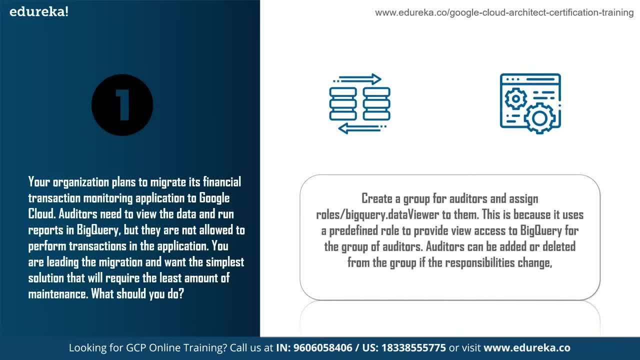 So this is because a predefined role is always used to basically provide access to BigQuery for the group of auditors. Now, auditors can be added or deleted from the group right according to your responsibilities, So you can always have a group of auditors working on certain data sets at all times. 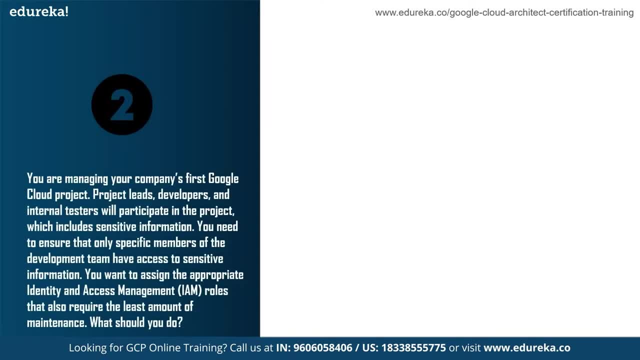 Next up we have. you are managing your company's first Google Cloud project. Now project leads developers and internals. They can be an organization, They can be a gardener, They can be a designer, They can be an engineer, They can be a team leader. 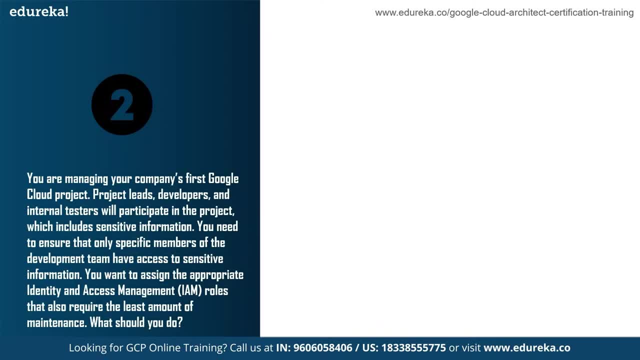 They can be a team leader or a development manager, And they can be things like H- abdominal heavy duty items, fitness items or things like that. Now, they can be various things. For that reason, group of auditors or third party auditors or team leaders. 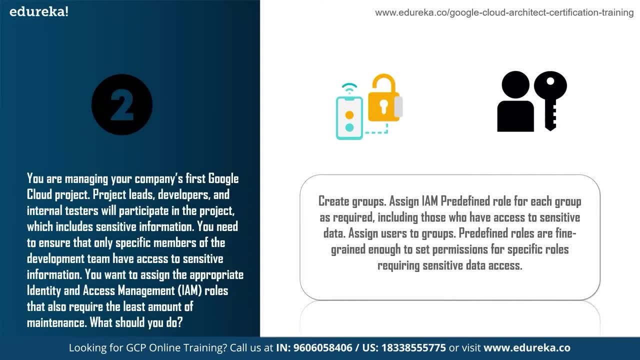 They can all be associated with that group of auditors. What they cannot be is the first group of auditors. For them, it's the first group of auditors. They cannot be single, in other words, because they are just batches. 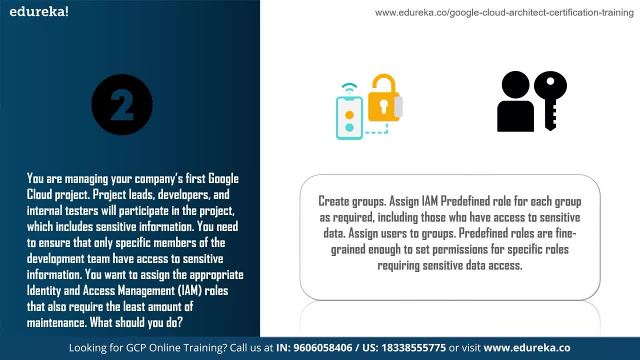 They cannot be different from each other, And so, right now, your group of auditors is represented by a group of auditors who are involved in a group of auditors, for every project is specific and you have to make sure that you don't want if 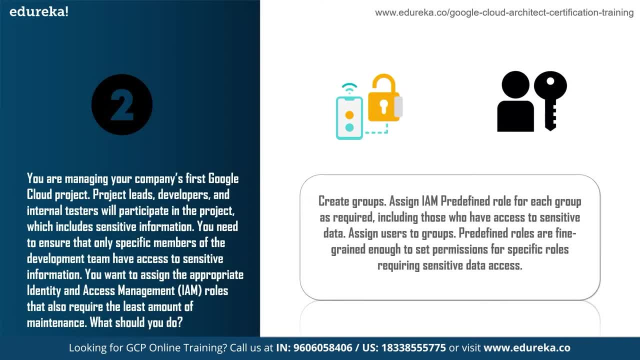 you don't want everybody in the team to know, then you will have to assign roles for specific users who can access these projects. so you have to create the groups and then assign the pre- I am predefined- rules for each group, right? so this is included for those who will have access to the data that you have, right? 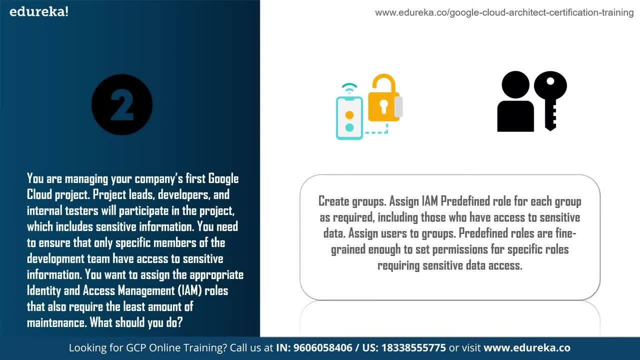 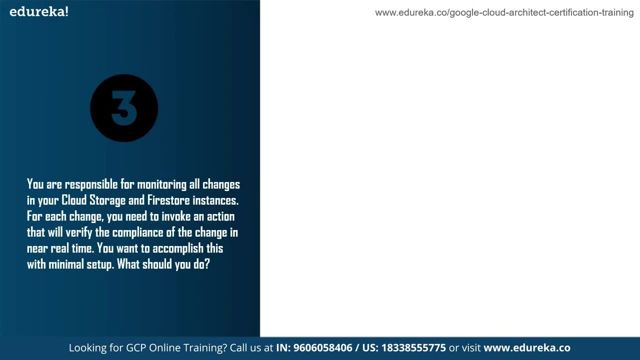 so predefined rules are fine-grained enough to set permissions for specific rules, and that is how you basically make sure that your sensitive data is only accessed by people you want them to see. the next question is: you are responsible for monitoring all the changes in your cloud storage and Firestone instances. 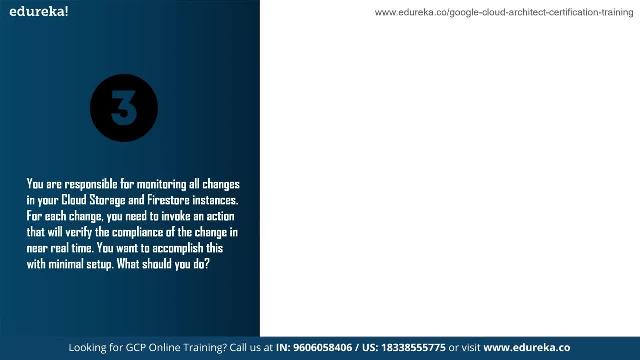 for each change, you need to invoke an action that will verify the compliance of the change in near real time, so you want to accomplish this with minimal setup. so when it comes to compliance and real-time application of Firestone and storage, you have to make sure that you have to use Google Cloud Function events. 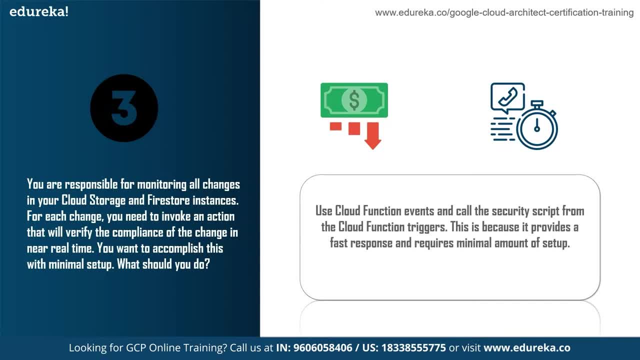 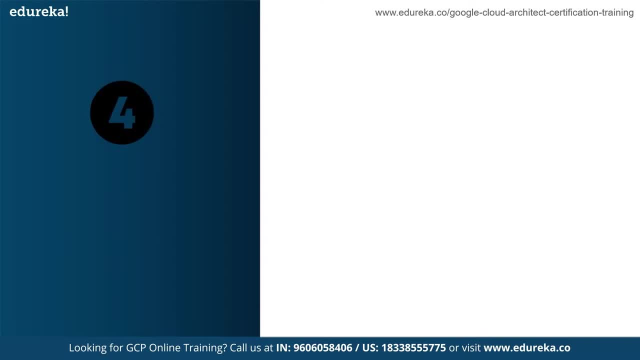 and call the security scripts for the function event figures. this is because Google Cloud Function provides a fast response and requires minimal amount of setup. the next question is: your application needs to process a significant rate of transactions. the rate of transactions exceeds the processing capabilities of a single virtual machine. 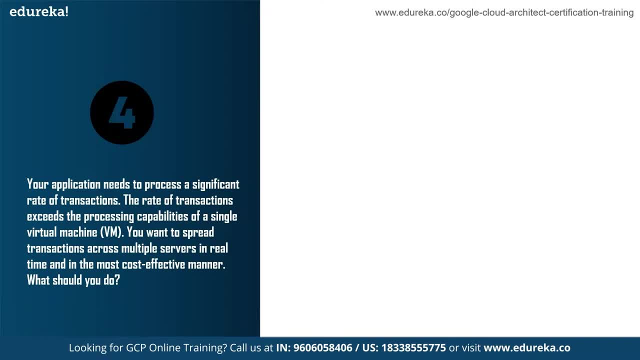 you want to spread transactions across multiple servers in real time and in the most cost-effective manner, so how do you do that? so the answer to this will be that you have to send transactions to PubSub. now, PubSub is another search API that is present in Google Cloud Platform, and you can use this to process the 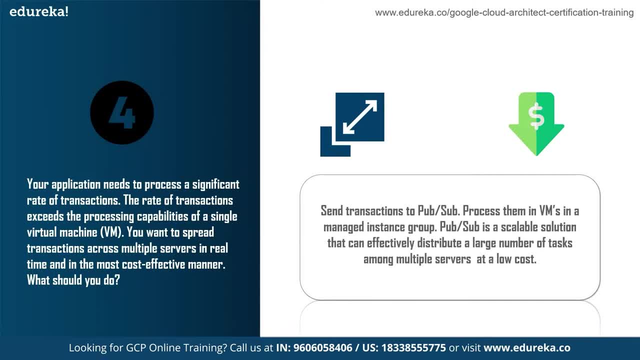 transactions in the VM in a managed instance group right. so PubSub is a very scalable solution that can be effectively distributed in a large number of tasks in a group at a very low cost. so this is why PubSub is the best option when it comes to assigning large number of tasks effectively in a group. next up, we have 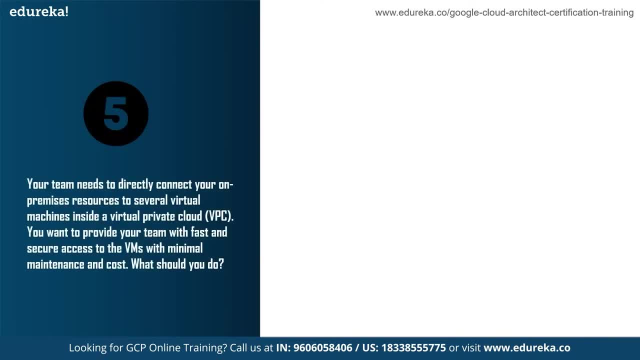 your team needs to directly connect your on-premises resources to several virtual machines inside a virtual private cloud. you want to provide your team with fast and secure access to the VMs with minimal maintenance and cost. how do you do that? so here we see that we can use cloud VPN to create a bridge. 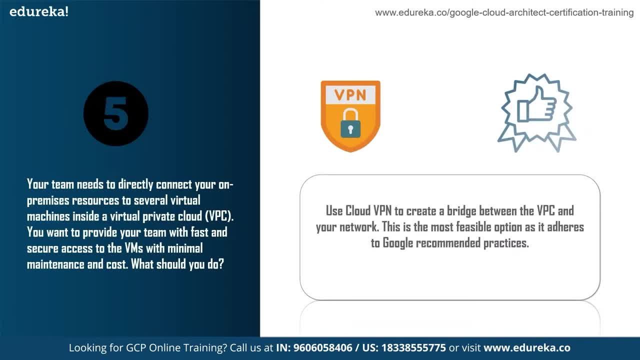 between the virtual private clouds and your specific network. so this is the most feasible option as it adheres to Google's recommended cloud practices, and if you follow Google's best practices, you will basically make sure that you can have the minimal cost and the maximum amount of maintenance with no 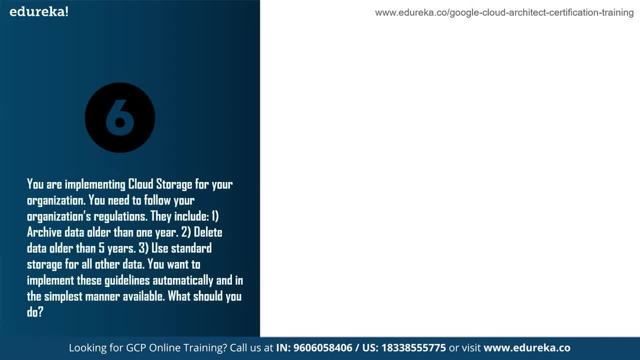 cost next up we have. you are implementing cloud storage for your organization and you do need to follow your organization's regulations now. these in include that you have to archive data older than one year, you have to delete data older than five years and you have to use standard storage for all other. 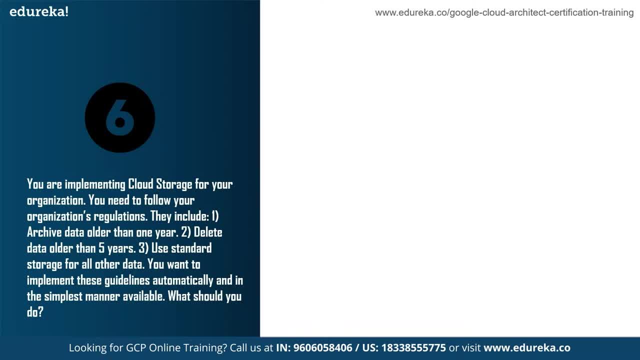 data. now you want to implement these guidelines automatically and in the simplest manner available, so to do this, what you have to do is you have to set up a project lifecycle management. so these are policies that allows you to basically automate the entire implementation process of the organization's data policy. and next up, we 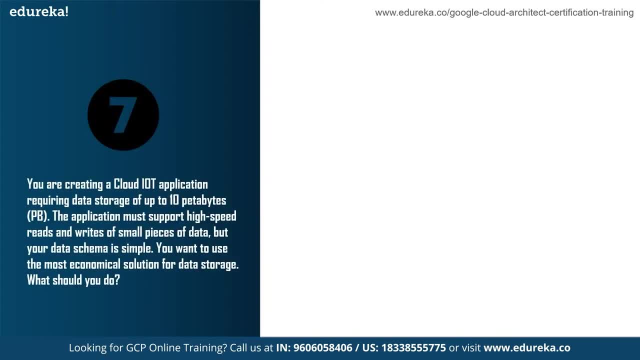 come to the next question, number seven. now, here you can see that you are creating a cloud IoT application requiring data storage for up to 10 petabytes. right, the application must support high-speed reads and writes of small pieces of data, but your data schema is simple. you want. 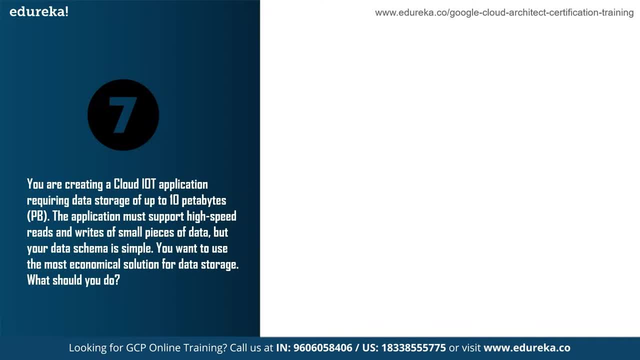 to use the most economical solution for data storage. now, in this case, when you have to use data storage for your private application that you need for continuous cedar eyes, you want to use different types of data. have to make sure that you want economical data storage capabilities. 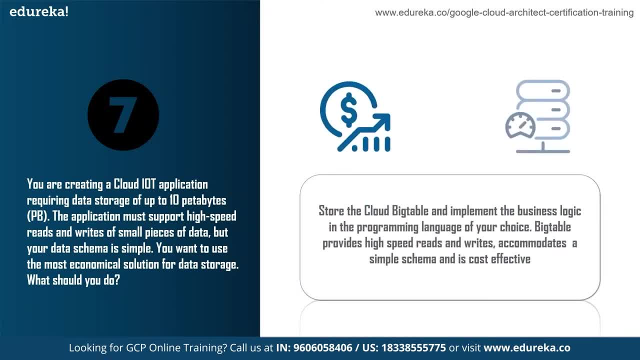 So here what you do is you store it in the cloud, Bigtable, and implement the business logic in the programming language of your choice. Now what Bigtable does is: Bigtable provides high speed reads and writes and accommodates a simple schema, which basically makes it very cost effective. 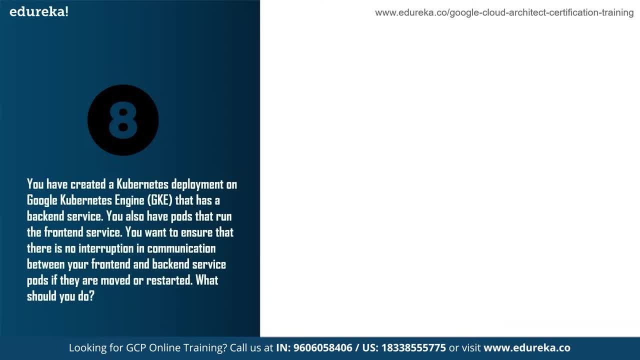 Next question is: you have created a Kubernetes deployment on Google Kubernetes engine that has a back end service. Now Google Kubernetes engine is an ML service provided by Google and you also have pods that run on the front end service. Now you basically do not want any interruption in the communication between the front end. 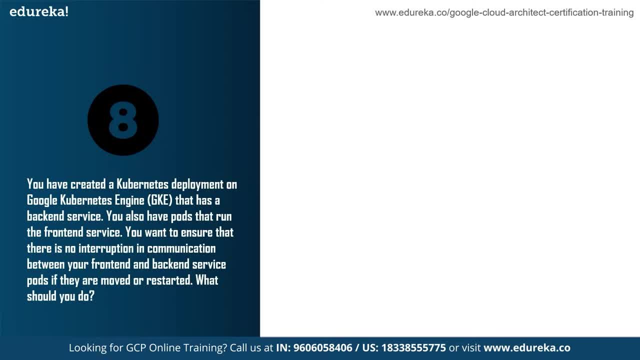 and the back end, even if these pods are removed or restarted. Now, what should you do when there is a case like this? Now, it's a very simple answer: You have to create a service that groups your pods together in the back end service. 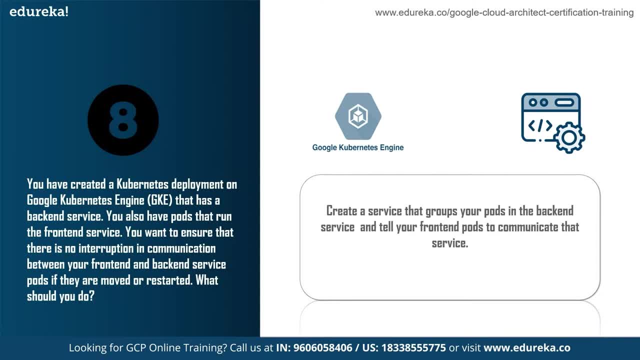 And tells your front end pods to communicate to that service. So you basically have a middle intermediate service that connects both to your back end and front end. Next we have question number 9.. You are responsible for the user management service of your global company. 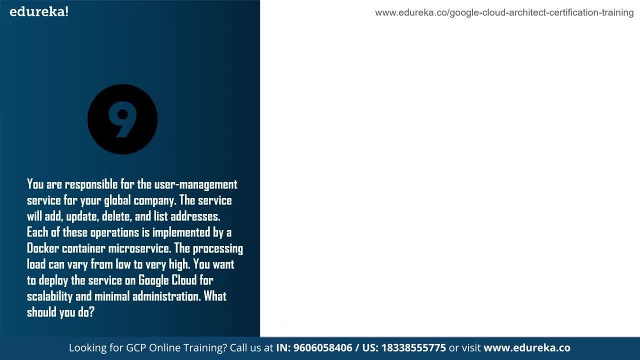 The services will add, update, delete and list addresses. Each of these operations is implemented by a docker container microservice. The processing load can vary from low to very high. You want to deploy a service. You want to deploy a service on good cloud for scalability and minimal administration. 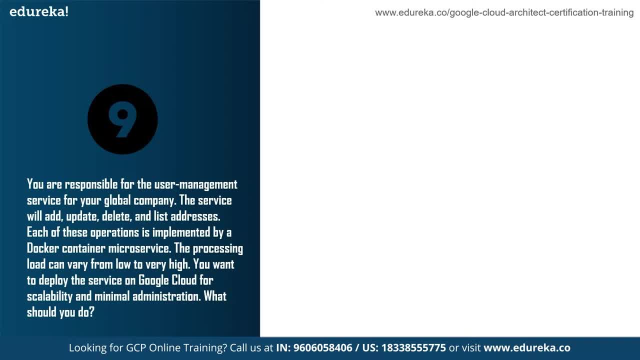 What should you do Now here? what you have to do is you have to deploy your docker containers into cloud run. Now, cloud run is a managed service that basically helps you with minimal administration of your docker containers. And finally we come to the last question. 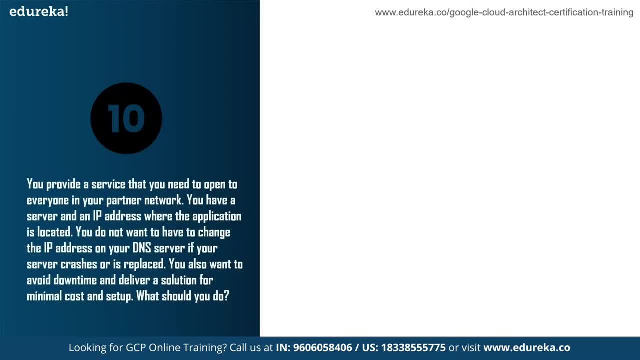 Question 10. You provide a service that you need to open to everyone in your partner network. You have a server and an IP address. That's where the application is located, But you do not want to change the IP address of your DNS server if your server crashes. 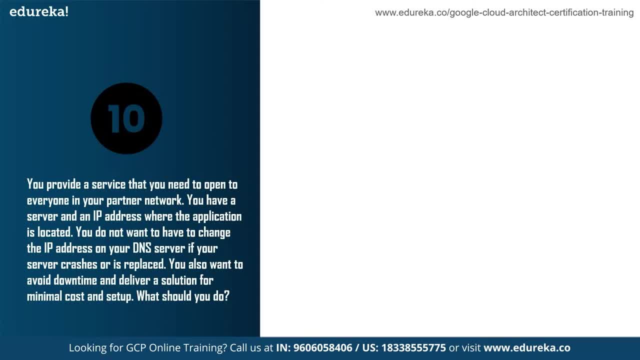 or it's replaced. You also want to avoid downtime and deliver a solution for minimal costs and setup. What should you do now? So, when it comes to making sure that you do not have to change your IP address on your DNS server when your server crashes or is replaced, what you do is you reserve a static 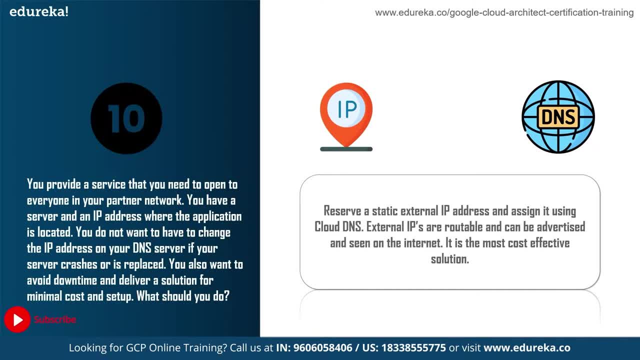 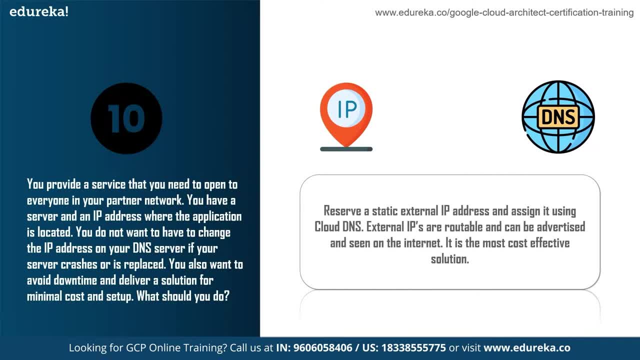 has a server, that has a server. It's also simple and can be quickly advertised and seen on the internet easily, and it is the most cost effective solution as well. Now, starting with our interview questions, we are first going to see some general cloud. 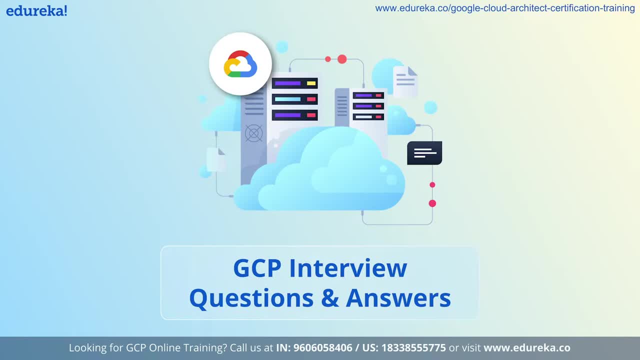 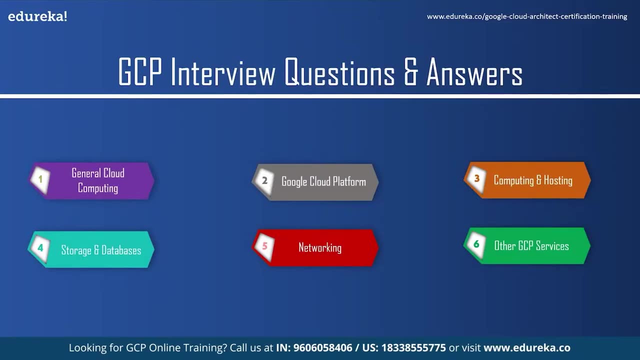 computing and Google Cloud Platform questions and questions on compute and hosting domains than storage and databases. Next, networking, followed by big data, machine learning and cloud artificial intelligence. So I guess it is clear what are we going to talk about today. So we will make a couple of instances in new frameworks for you to find out what you are. 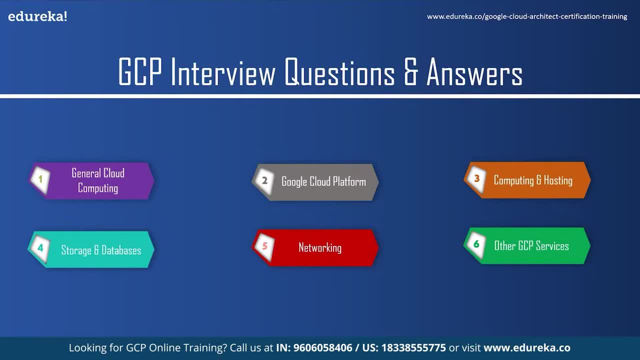 interested in. We will link there wreck for this session and we are going to talk about UBI and online plugins, So let's head into this session. In this episode, we are going to have an interview with Abdul Wad Luc crm and nncom Sungmi steel. 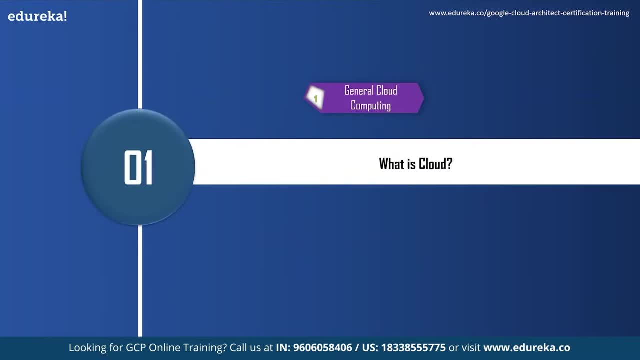 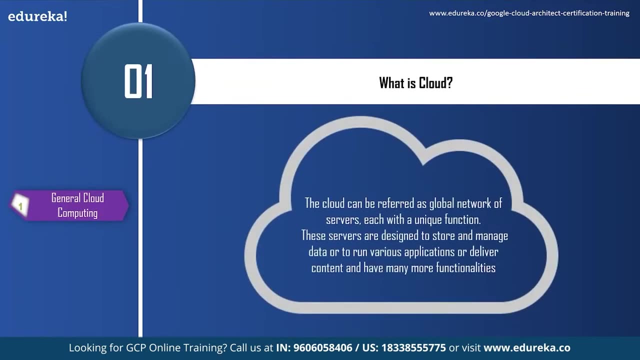 Okay, So let's get started. So the first question we're going to discuss is: what is cloud? now, there are various way to answer this. one of them could be: the cloud can be referred as global network of servers, each with a unique function. The servers are designed to store and manage data, or to run various application or deliver. 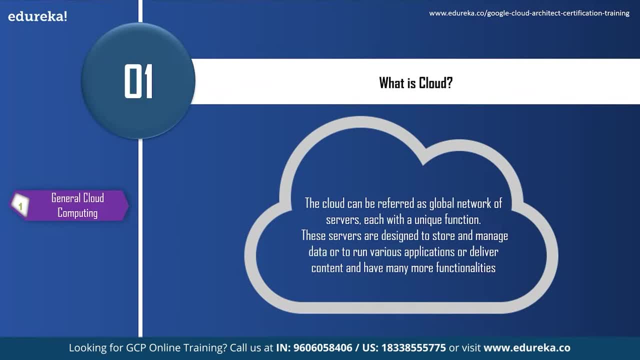 content and have many more functionalities. You can also mention that the servers are located in data centers across the world. You can also talk about the various service cloud offers, such as compute storage, databases, networking and so on. I want you to understand the concept and frame the answer in your own words. moving on to 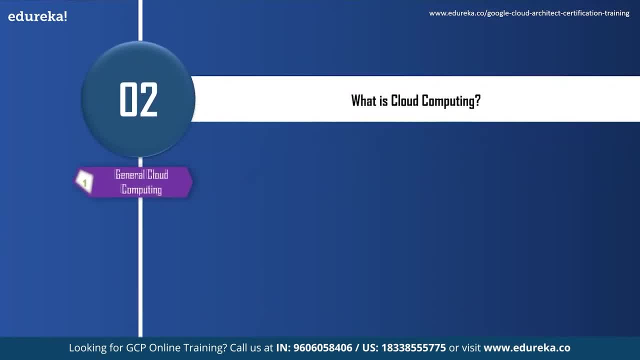 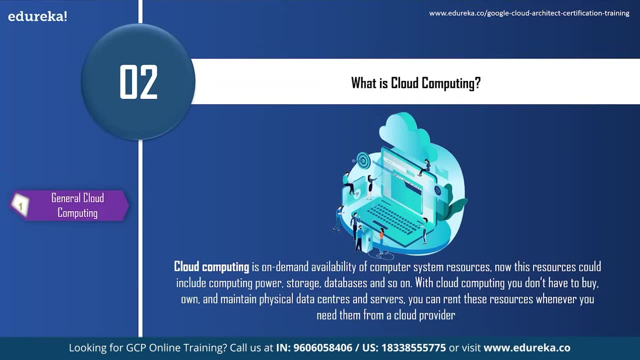 a next question: What is cloud computing now? like the previous question, even this question can be answered in many ways. So to answer this question, I would say: cloud computing is an on-demand availability of computer system resources. Now this resources could include computing power, storage, databases and so on. with cloud. 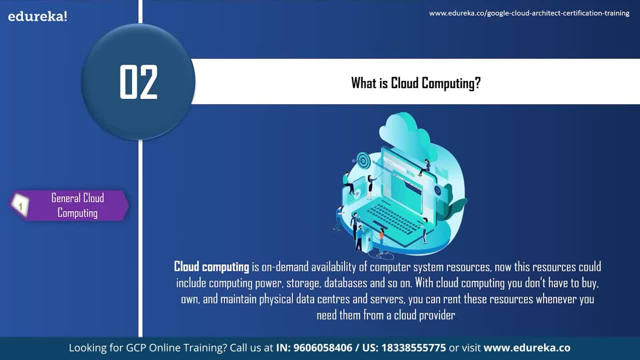 computing. You don't have to buy or own or maintain physical data centers and servers. You can just rent this resources whenever you need them from a cloud service provider. Now here you can also mention what a cloud computing used for, like it can be used for. 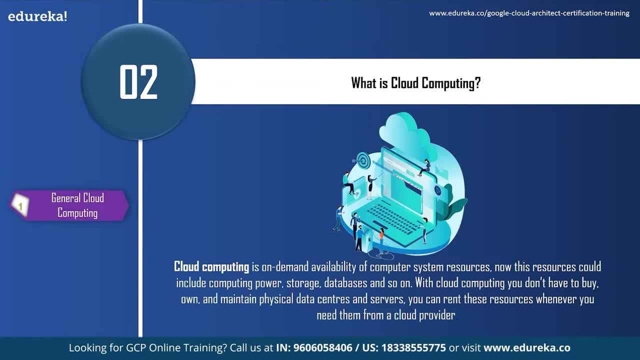 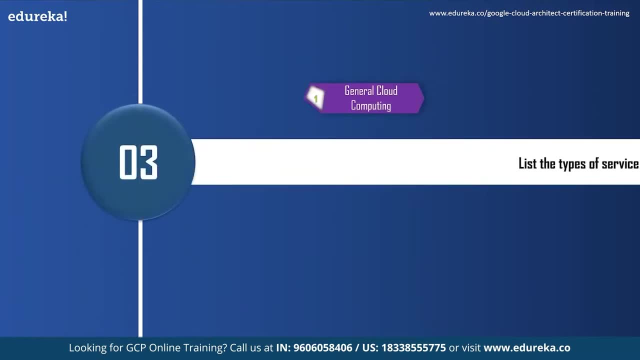 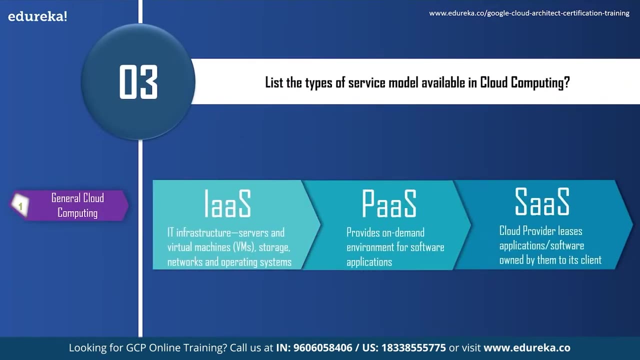 data backup, disaster recovery, virtual desktops, software development and testing, big data analytics and customer facing web applications. So now, moving on to a third question list: the type of service model available in cloud computing. So there are three types of service model available In cloud computing, that is, IaaS, PaaS and SaaS. IaaS stands for infrastructure as a service. 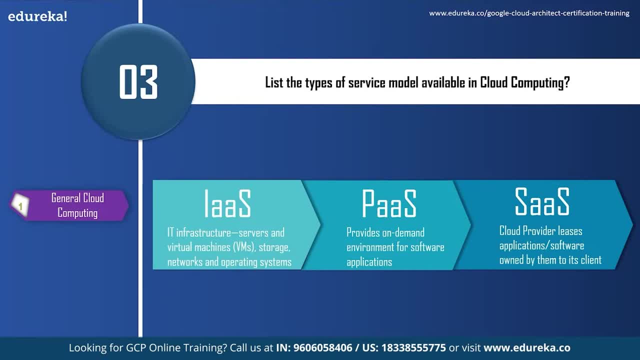 in this service model You can rent IT infrastructure such as servers and virtual machines, storage networks and operating system. Let's say a user wants to use a Linux machine. He can access the Linux machine using IaaS service model without worrying about the physical machine or the networking of the system on which the OS is installed. 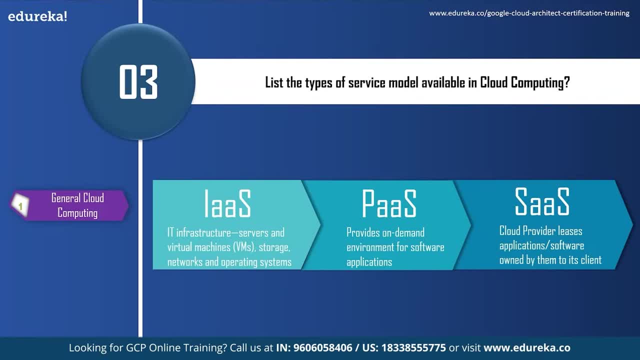 The next service model is platform as a service. This service model provides an on-demand environment for developing, testing, delivering and managing your software application. The users don't have to worry about setting up or managing the underlying infrastructure of servers, storage networks and databases which are needed for development. 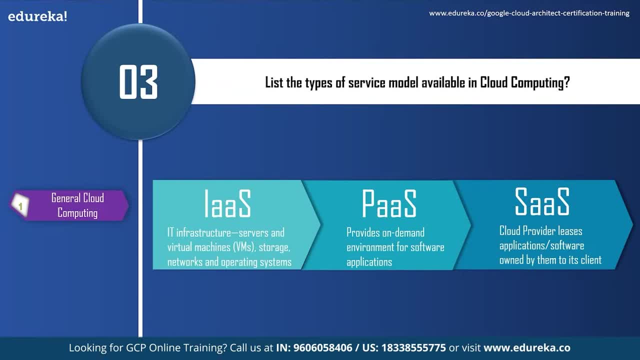 This is taken care of by the cloud service provider itself. The next service model is software as a service. In this service model, the cloud providers leases application and software which are owned by them to its client. The client is the provider. The client is the provider. 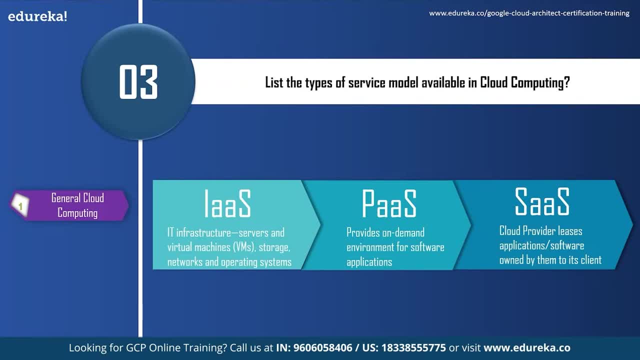 Clients can access this software on any device which is connected to the internet, using tools such as web browser or an application. Now, to summarize this answer, just think of it as this way: Infrastructure as a service provides you with an infrastructure such as virtual machine or 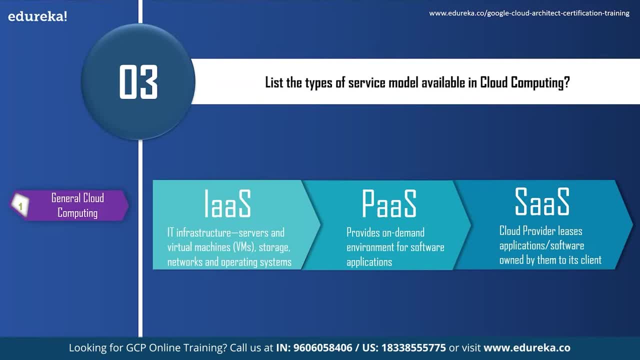 a servers, Whereas platform as a service provides you with a platform where you can develop, test and run your application, And software as a service provides you with the software itself. Now, I guess you have some idea about service models which are available in cloud computing. 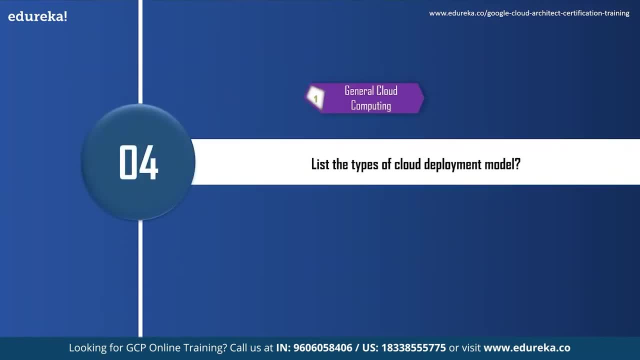 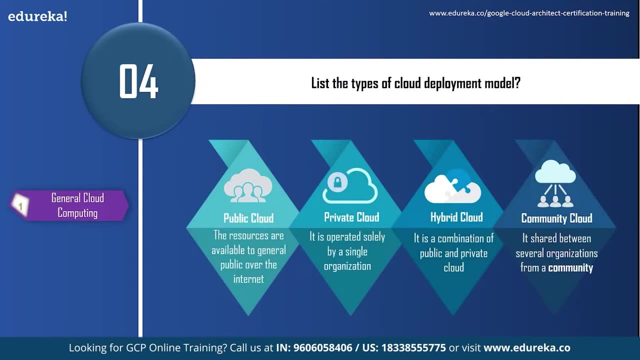 Let us move on to our next question. The next question is list the types of cloud deployment model. So there are four types of cloud deployment model, which are public cloud, private cloud, hybrid cloud and community cloud. in public cloud deployment model, the resources, such as application and storage, are available to general public over the internet. 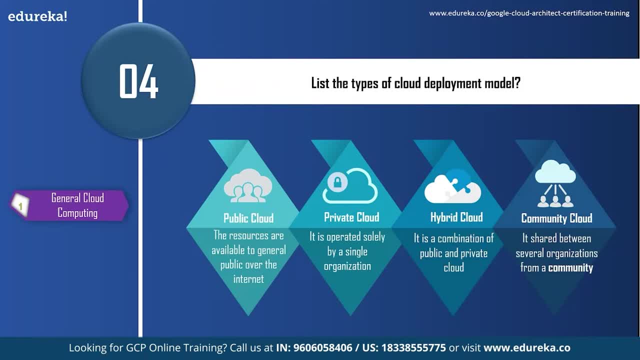 These resources can be free or sold on demand, which will allow users to pay only per usage for the CPU cycles, storage of bandwidth, the use. Now, when we talk about private cloud, It is operated solely for a single organization. It offers services over a private internet network, which is typically hosted on premises. 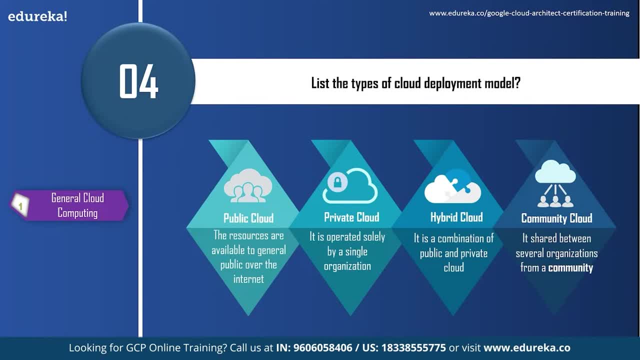 Now, this private cloud is costlier, but there is high level of security. Next, the hybrid cloud deployment model can be defined as a combination of public and private cloud. It can share services between public and private clouds, depending on the purpose. The fourth cloud deployment model is a community cloud. 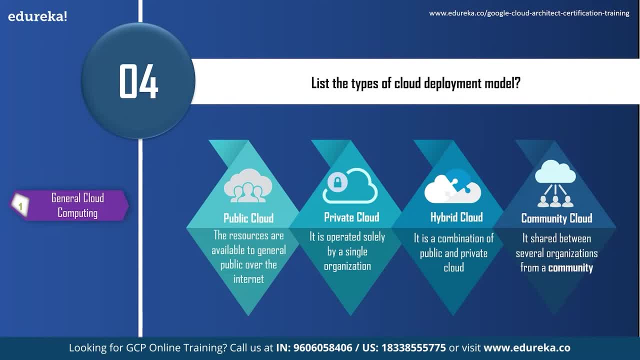 Now the community cloud infrastructure is shared between several organizations From a specific community with a common concern. educational University that are cooperating in the same area of interest as that of a research Institute can use the same community cloud. Now, these were the four types of cloud deployment model. 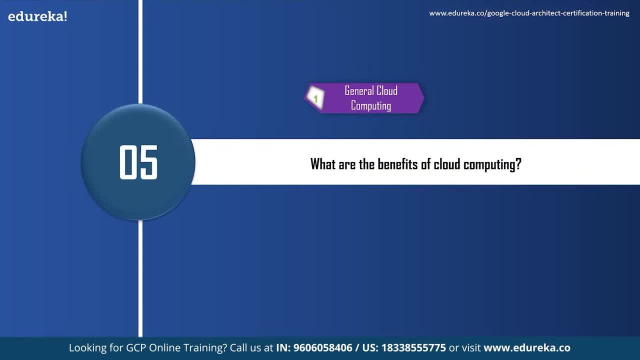 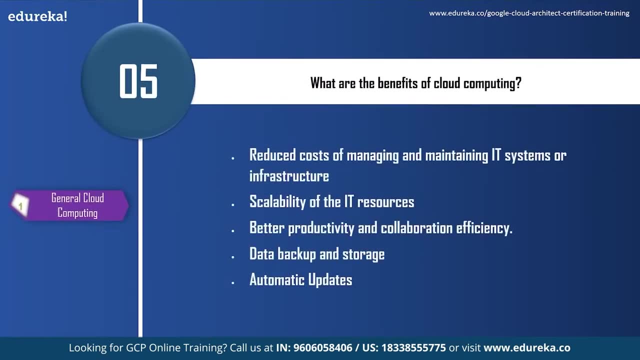 So now let us move on to the next question and see what are the benefits of cloud computing, or why companies are increasingly adopting cloud computing. So now, here you can mention some of the benefits of cloud computing, such as there is reduced cost of managing and maintaining IT systems. So now here you can mention some of the benefits of cloud computing, such as there is reduced cost of managing and maintaining IT systems. So now here you can mention some of the benefits of cloud computing, such as there is reduced cost of managing and maintaining IT systems. 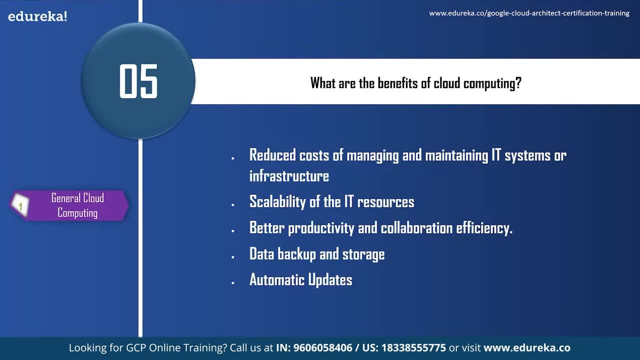 The next benefit is靠 the quality of the IT resources. You can scale up or scale down your operational and storage needs according to your convenience. the next benefit is it provides better productivity and collaboration efficiency. For example, if your team is working on a project across different location, you can. 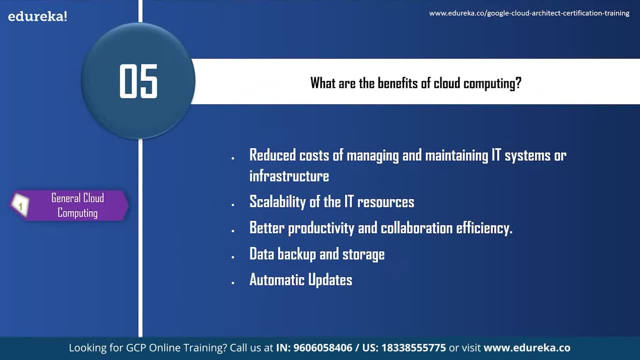 use cloud computing to give your employees, contractors and third party access to the same fight. The next benefit is data backup and storage. you can elaborate this by saying your data backup and storage. You can elaborate this by saying your data backup and storage. You can elaborate this by saying your data backup and storage. 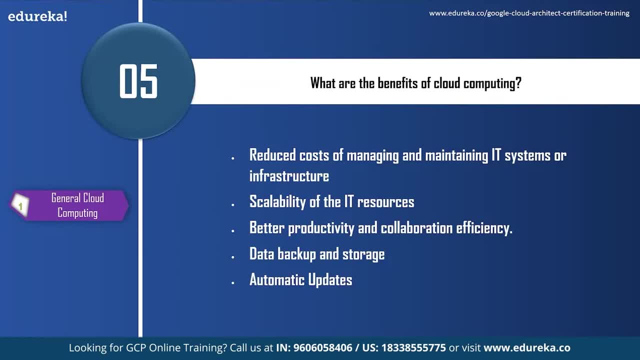 So you can create your own cloud computing as a state. The next benefit is you can eat, move your data andissue your data and share your data by following other entities saying your data is backed up, so you don't have to worry if your data is lost or deleted. 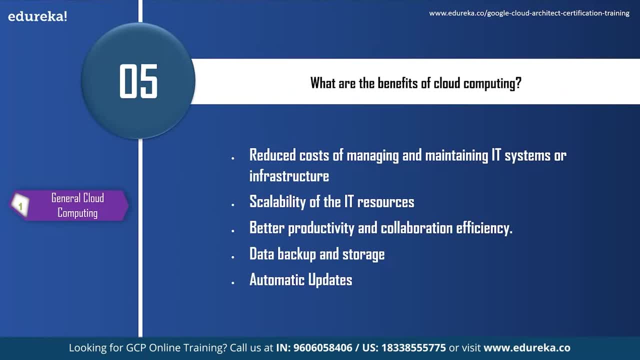 The next advantage is cloud service providers provide automatic updates. This would include up-to-date version of software, as well as upgrades to servers and computer processing power. Now, these were just some of the benefits of cloud computing. We can also mention some more benefits of cloud computing. 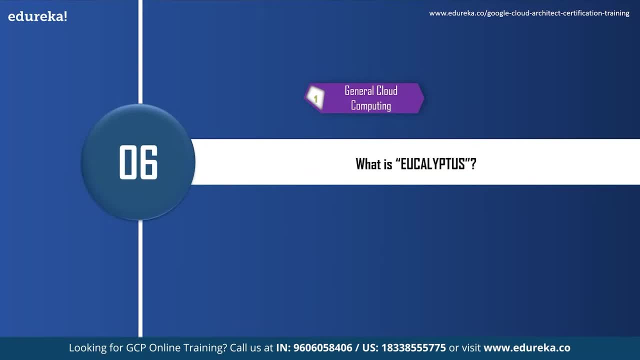 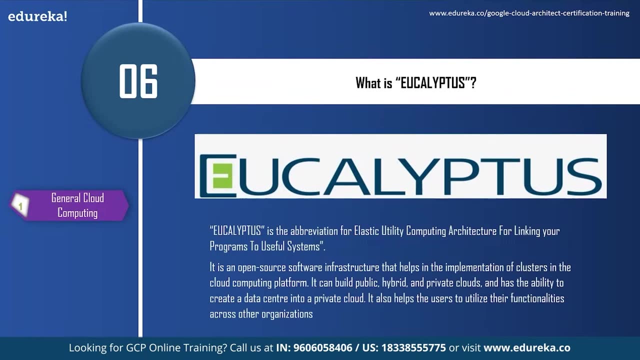 So now let us move on to the next question. So the next question is: what is eucalyptus? eucalyptus is the abbreviation for elastic utility computing architecture for linking your program to useful systems. It is an open source software infrastructure that helps in implementation of clusters in 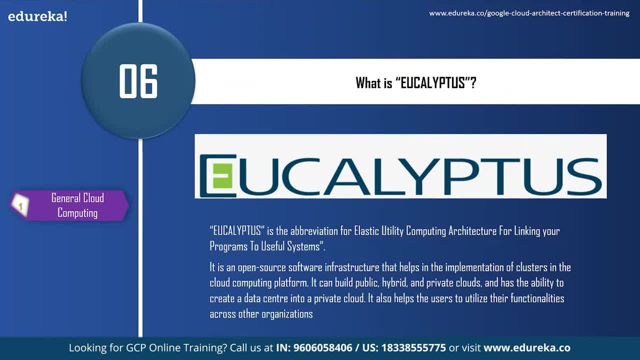 the cloud computing platform. It can build public, hybrid and private cloud and has the ability to create a data centers into a private cloud. It also helps the user to utilize the functionalities across those other organizations. Now these were some of the general cloud computing questions that can be asked in a GCP interview. 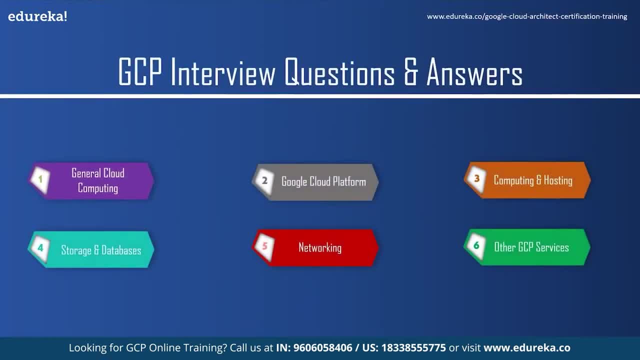 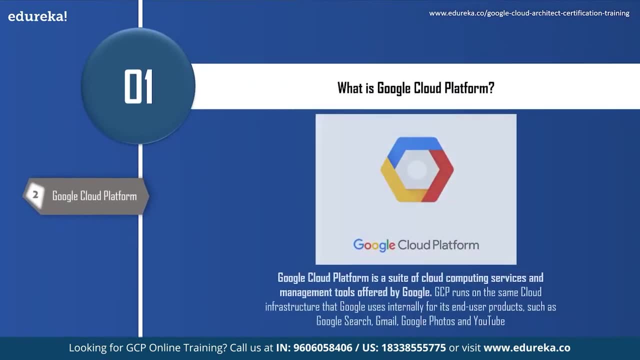 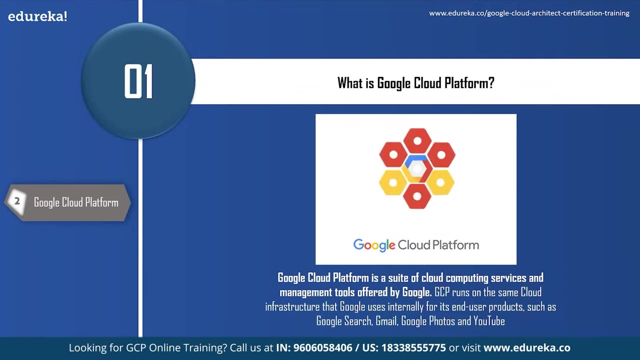 So now let us move on to a next set of questions on Google Cloud Platform. So first question is: what is Google Cloud Platform? We all know Google Cloud Platform is a cloud service provider, But just to define it, Google Cloud Platform is a suite of cloud computing services and 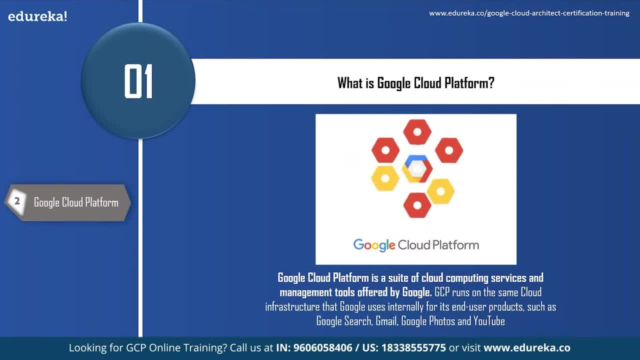 management tools offered by Google. It runs on the same cloud infrastructure that Google uses internally for its end user products, such as Google search, Gmail, Google photos and YouTube. Now, this is a very basic question, But even this can be asked in your interview. 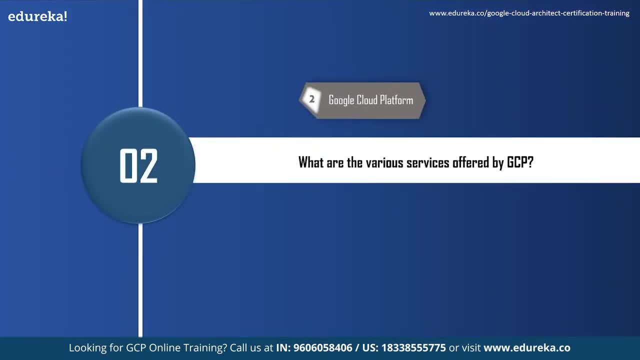 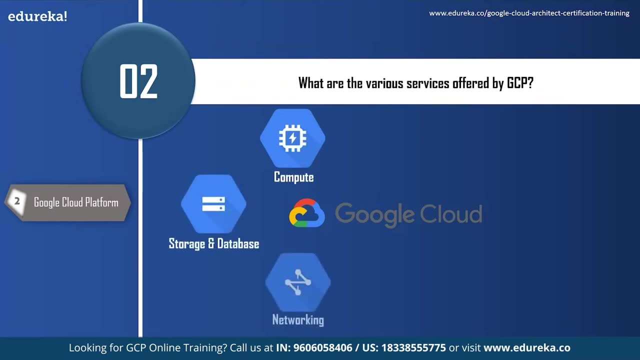 The next question is: what are the various services offered by GCP? The various services offered by Google Cloud Platform are compute services, storage and database services, networking services, big data services, identity and security services, Internet of Things services, then machine learning and cloud artificial intelligence. 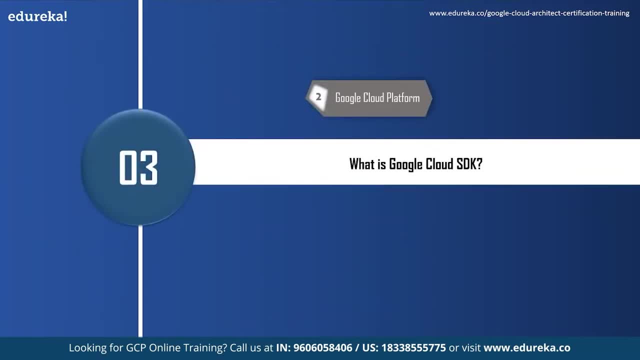 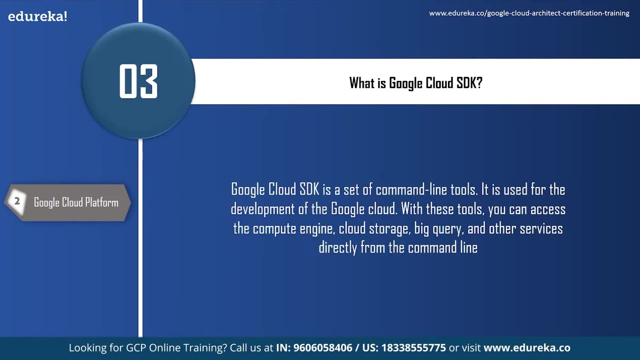 services. Moving on to our next question: what is Google Cloud SDK? Google Cloud SDK, Our Google Cloud software development kit, is a set of command line tools. It is used for the development of Google Cloud. With these tools, you can access the compute engine, cloud storage, BigQuery and other. 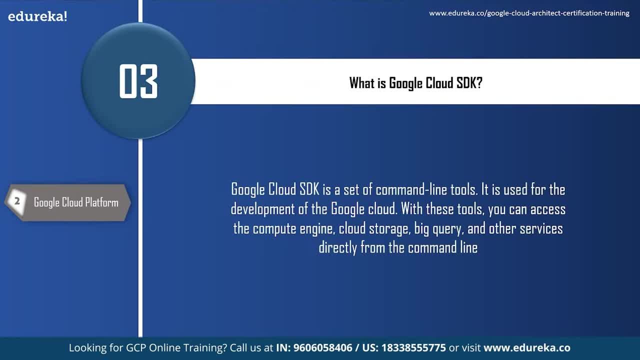 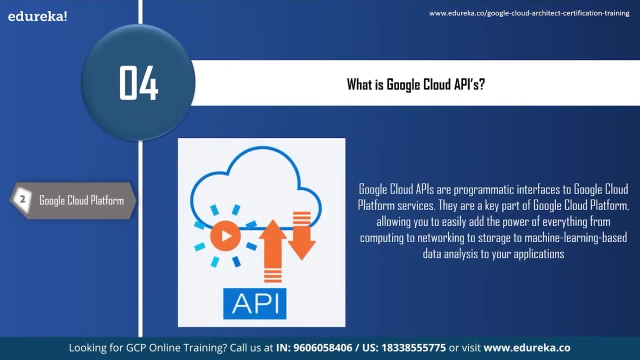 services directly from the command line. So now I guess you have understood what is Google Cloud SDK. So let us move on to the next question and see what is Google Cloud APIs. Google Cloud APIs are programmatic interface to Google Cloud Platform services. They are a key part of Google Cloud Platform which allows you to easily add the power of 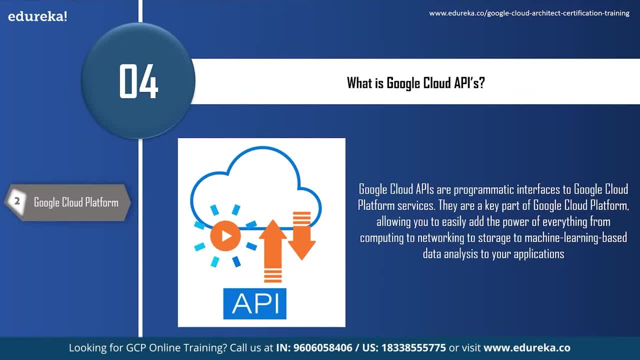 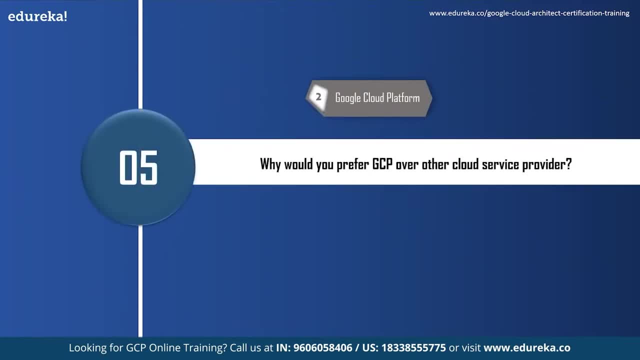 everything from computing to networking, to storage, to machine learning based data analysis, to your applications. Now, moving on to our next question: why would you prefer GCP over other cloud service providers? Well, here you are expected to say the benefits of GCP. 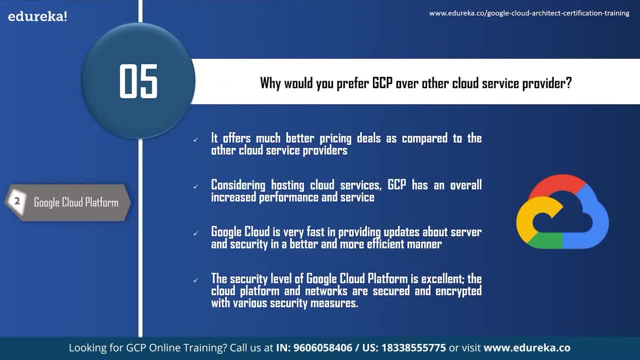 We can start the answer by saying: well, each cloud service provider has its own pros and cons, But what makes Google Cloud Platform unique is it offers a much better pricing model compared to the other cloud service providers. Next, GCP has an overall increased performance and service. 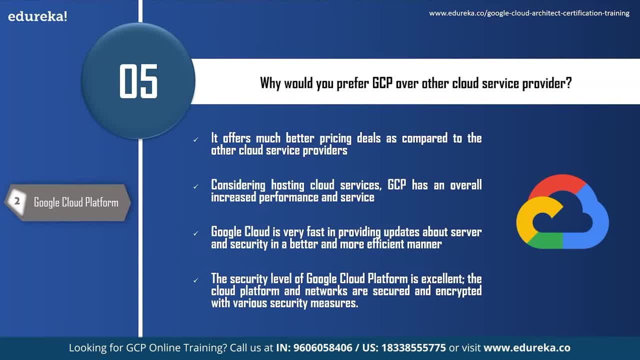 You can also mention Google Cloud is very fast in providing updates about servers and security in a better and more efficient manner. You can also mention the security level of Google Cloud Platform is excellent. The cloud platform and the networks are secured and encrypted with various security measures. 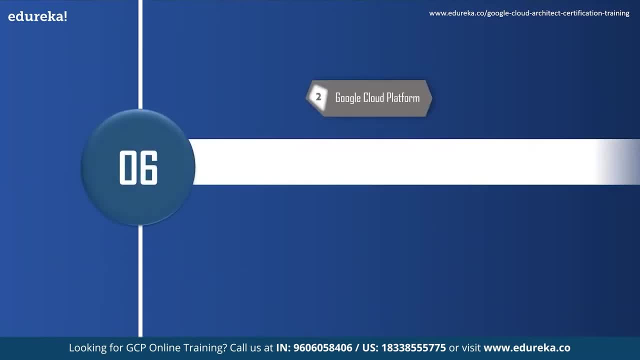 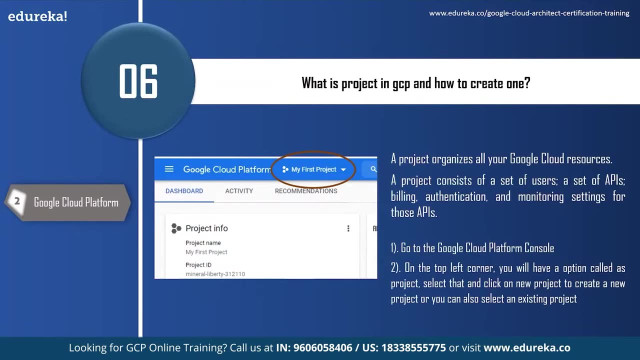 So I guess you got some idea about how to answer this question, So now let us move on to the next question and see what is projects in GCP and how to create one. A project organizes all your Google Cloud resources. A project consists of a set of users, a set of APIs and billing, authentication and monitoring. 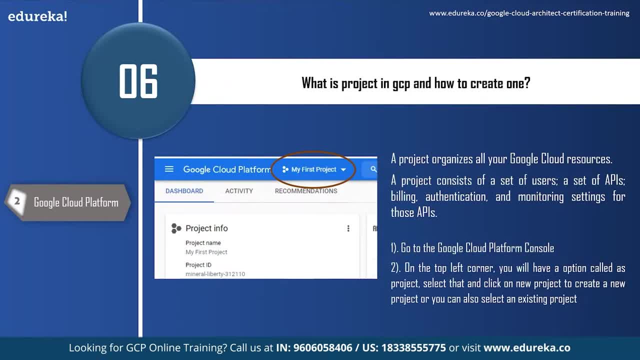 setting for those APIs. So, for example, all of your cloud storage buckets and objects, along with the user permission for accessing them. all this resides in a project. So in order to create a project, you have to sign into Google Cloud Platform console. 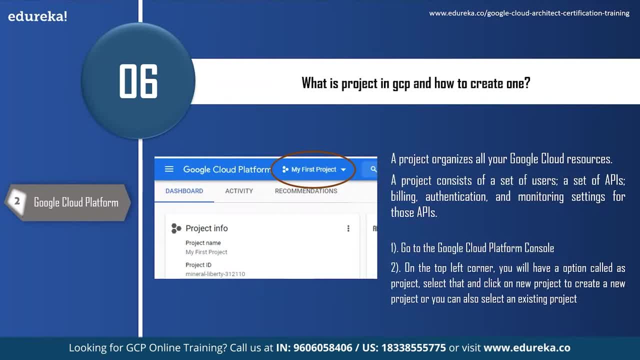 Then on the top left corner you will have an option called as project. Select that and click on new project to create a new project, or you can also select an existing project from the list. So now I guess you have some idea about projects in GCP. 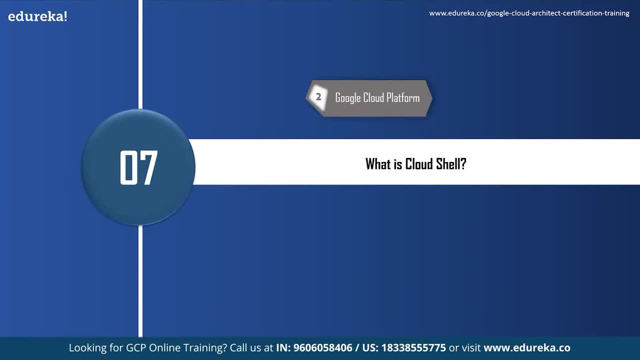 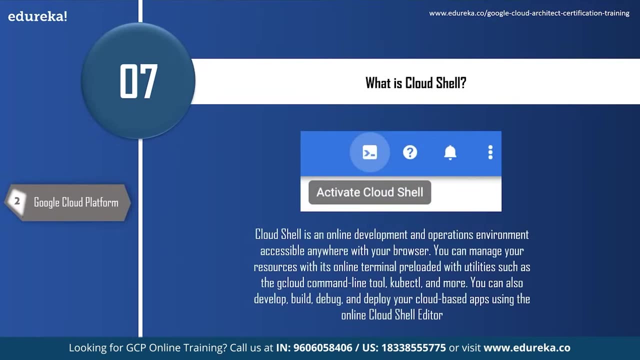 So let us move on to the next question. Our next question is: what is Cloud Shell? So if you have been using GCP, you will know what is Cloud Shell. So, for people who don't know what Cloud Shell is, Cloud Shell is an online development and 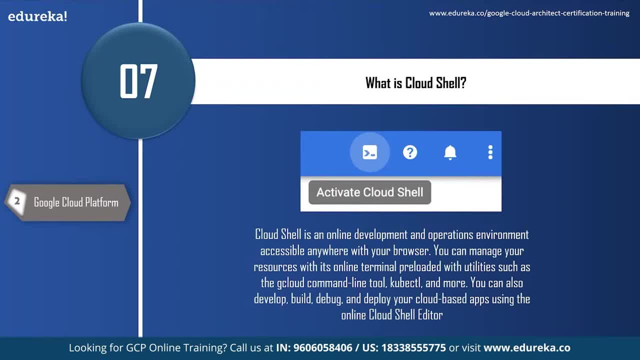 operational environment which is accessible anywhere with your browser. You can manage your resources with its online terminal, which is preloaded on your cloud. So you can manage your resources with its online terminal, which is preloaded on your cloud. So you can manage your resources with its online terminal, which is preloaded on your cloud. 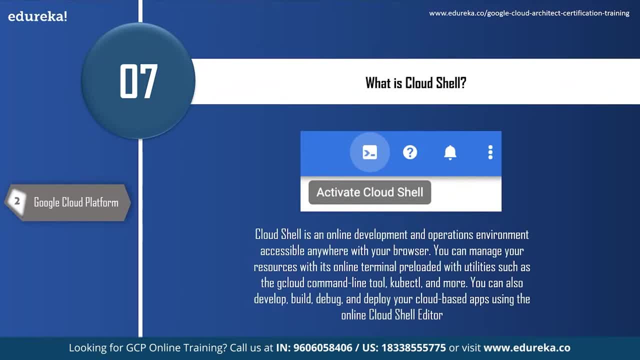 You can also be used with utilities such as G Cloud command line tool, cube, CTL and many more. You can also develop, build, debug and deploy a cloud based application using the online cloud shell editor. So this was our cloud shell. 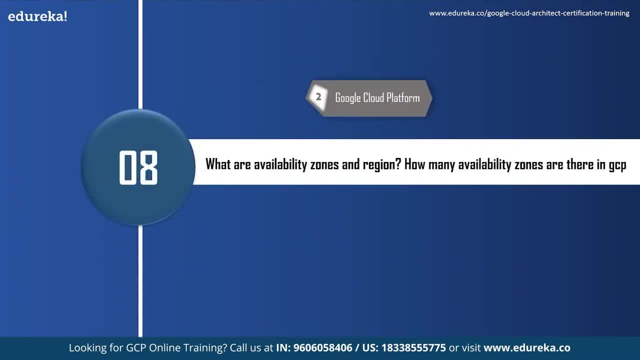 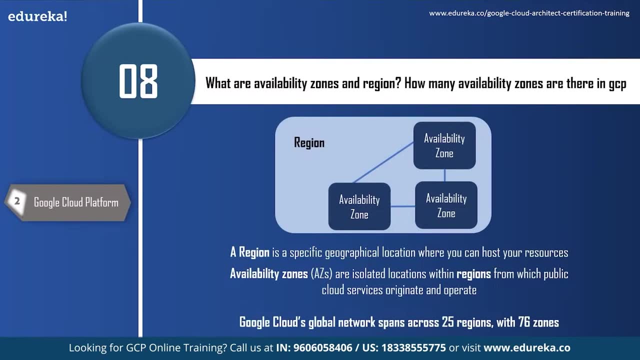 Our next question is: what are availability zones and region, and how many availability zones and regions are there in GCP? So region is a specific geographical location where you can host your resources, And availability zones are isolated location within the regions from where public cloud cloud services originate and operate. and then talking about Google Cloud Platform, 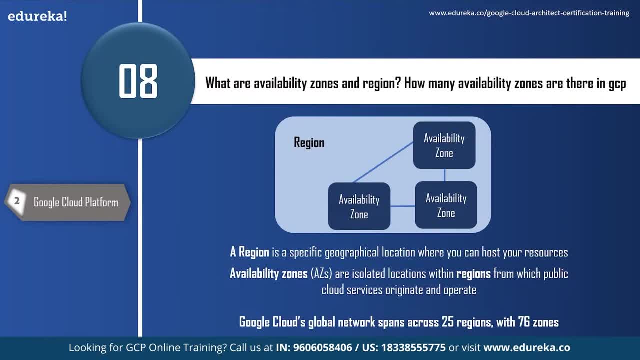 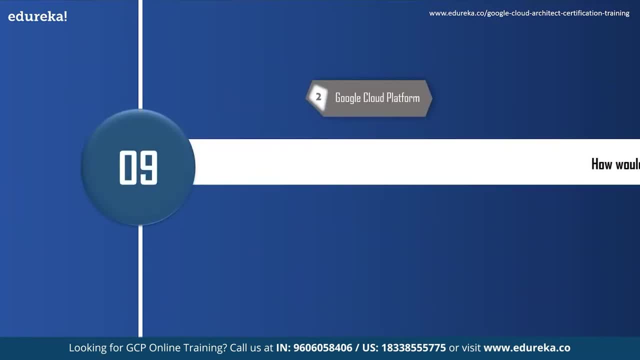 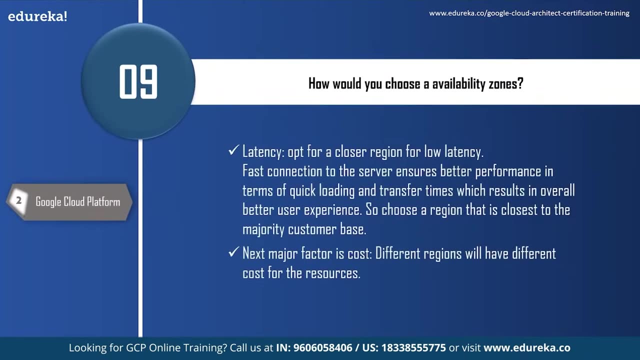 availability zones and region. it has 25 regions with 76 zones. each region has at least three or more zones. the next question, right after this, could be: how would you choose an availability zone, or what all parameters would you consider while selecting an availability zone? so you can answer this by saying you have 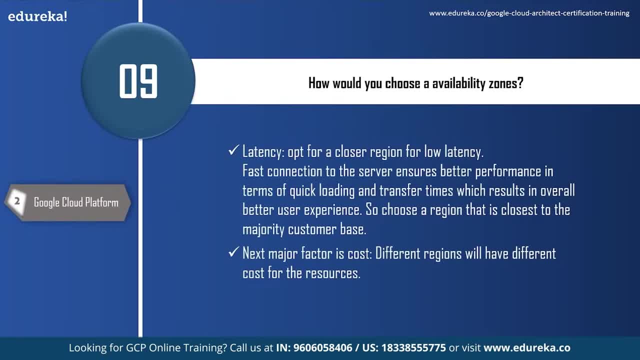 to select the availability zone based on the following factors. the first factor is latency. opt for the closest region for low latency. fast connection to the servers ensures better performance in terms of quick loading and transfer time, which results in overall, better user experience. so choose a region that is closest to the majority customer base. and then the next factor you should consider is the cost. different region will have different costs for the resources. for example, if I want to use an easy to instance virtual machine in the US central region, which cost me somewhere around $40 per month, 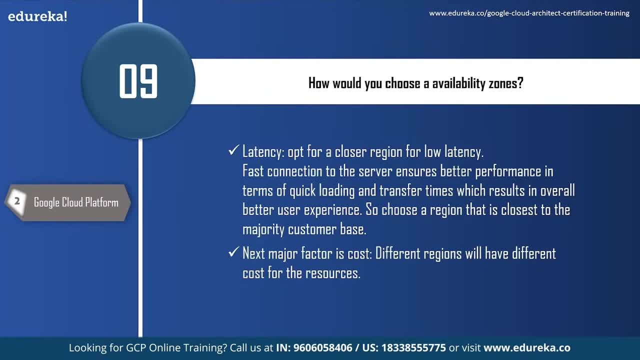 you should consider the cost for the resources. for example, if I want to use an easy to instance virtual machine in the US central region, which cost me somewhere around $40 per month, but the same virtual machine in Mumbai region would cost me $58. so you can see. 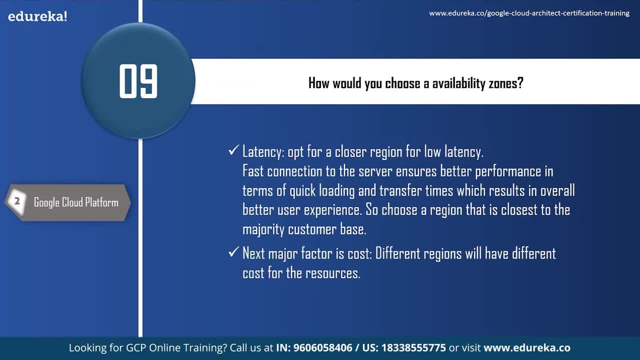 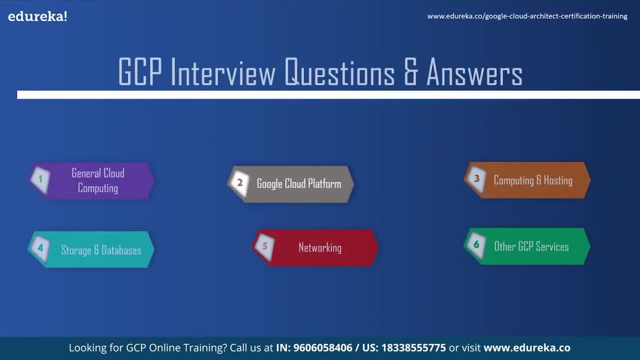 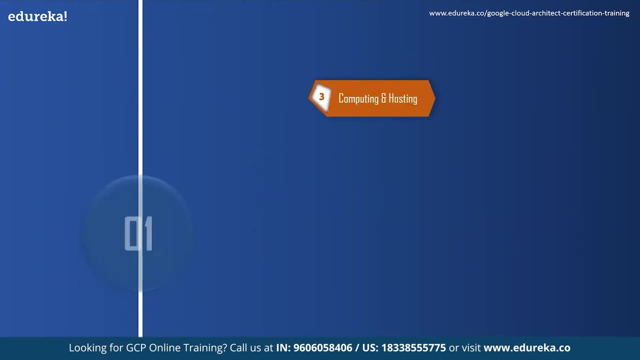 there is $10 difference per month in these two regions. so these are the factors you need to keep in mind before selecting an availability zone and region. so these were some of the general Google Cloud Platform questions, so let us move on to a next set of questions on compute and hosting services, on GCP. so 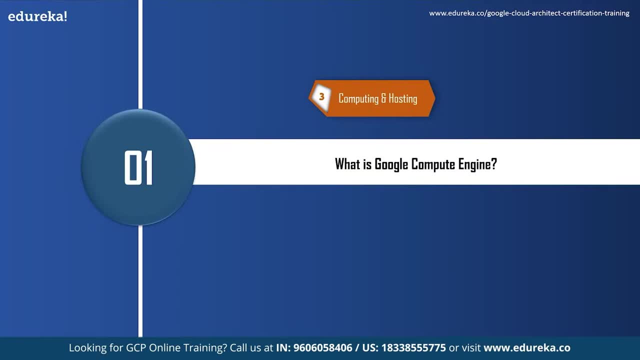 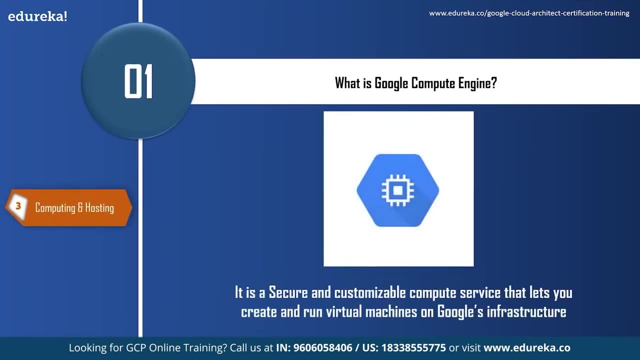 the first and basic question they could ask is: what is Google Compute Engine? because Google Compute Engine is a primary Compute Engine in GCP. so you can explain this in a very simple term: it is a secure and customizable compute service that lets you create and run virtual machines on Google's infrastructure. so now, moving on to a 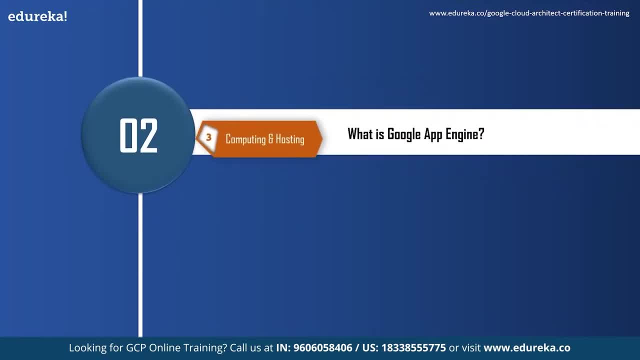 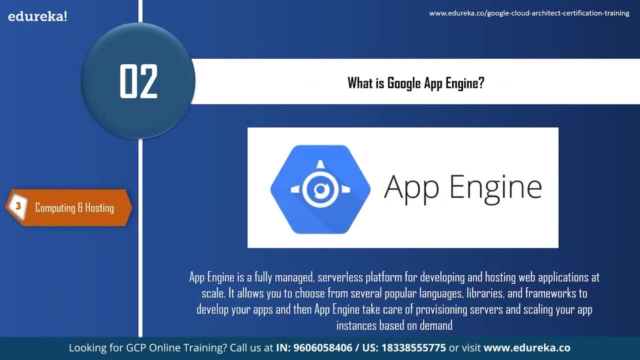 next question: what is Google App Engine? so App Engine is a fully managed serverless platform for developing and hosting web application at scale. it allows you to choose from several popular languages, libraries and frameworks to develop your application, and then you can use Google Compute Engine to build your application, and then the App Engine takes care of provisioning. 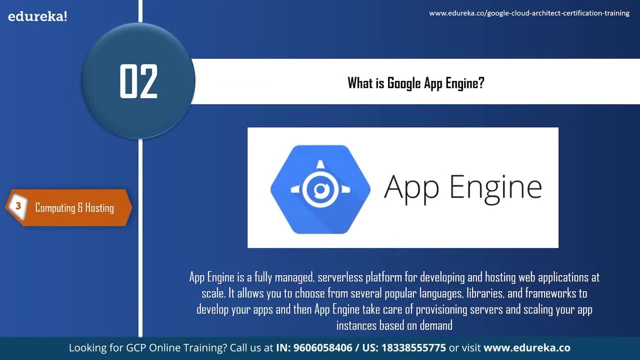 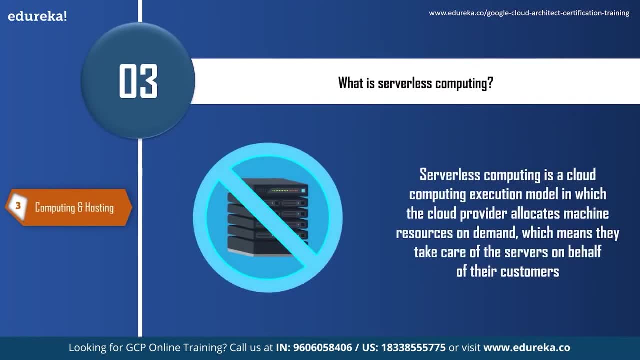 servers and scaling your application instances based on the demand. so now, when you answer this question, they might ask you: what is serverless computing? so serverless computing is nothing but a cloud computing execution model in which the cloud provider allocates machine resources on demand, which means they. 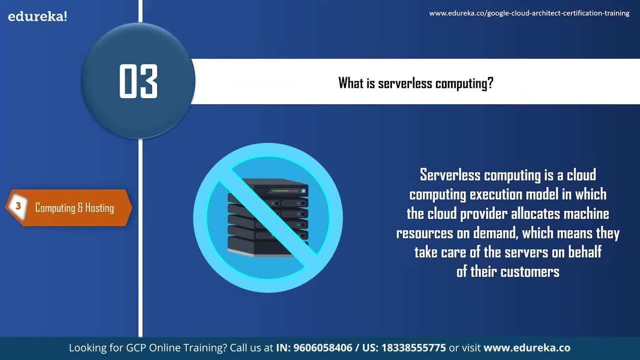 take care of servers on behalf of the customers, so the customers can only focus on building your application, where the servers and all that is taken care of by the cloud service provider. so this is an example of a serverless application, where the servers and all that is taken care of by the cloud service provider. 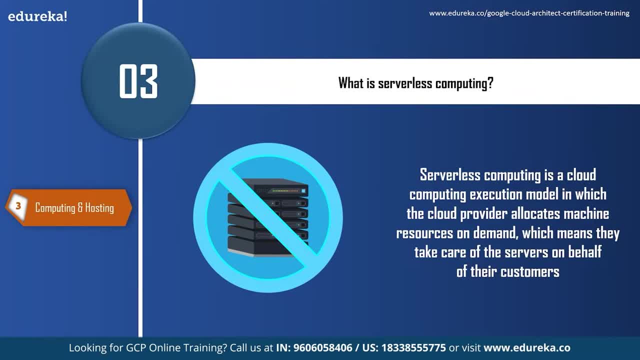 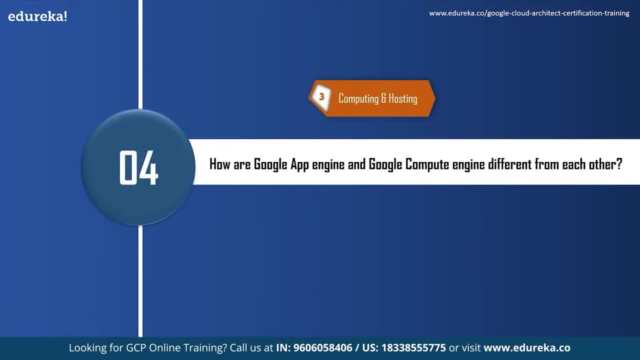 so I guess you have some idea about serverless computing. so now let us move on to our next question. now this question is a frequently asked question: how are Google App Engine and Google Compute Engine different from each other? you can answer this by saying: Google Compute Engine and Google App Engine are. 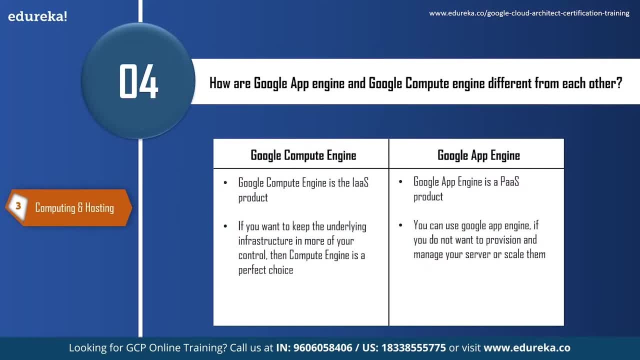 complementary to each other. Google Compute Engine is an infrastructure as a service product, whereas Google App Engine is a platform as a service product of Google. so now, if you want the underlying infrastructure in more of your control, then Google Compute Engine is a perfect choice. for instance, you can use: 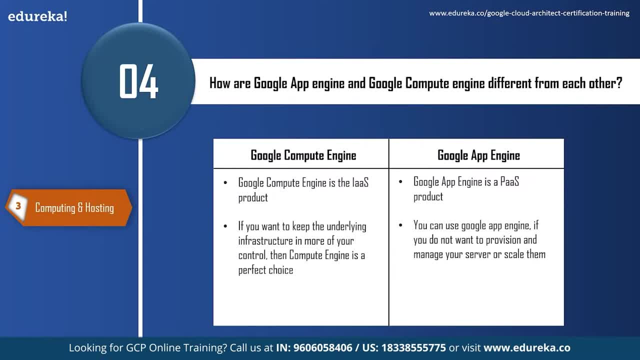 Compute Engine for the implementation of customized business logic or in case you need to run your own storage system. on the other hand, you can use Google App Engine if you do not want to provision and manage your servers or scale them. now I guess you have understood the difference between Google Compute Engine. 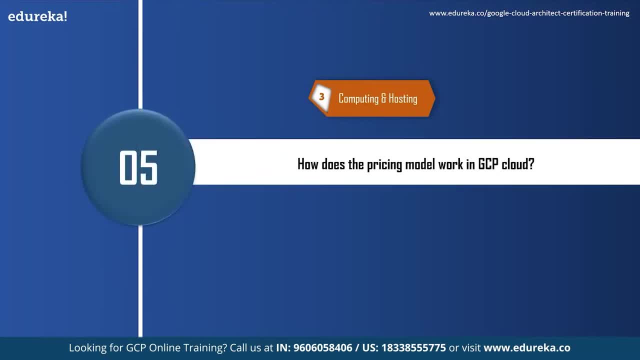 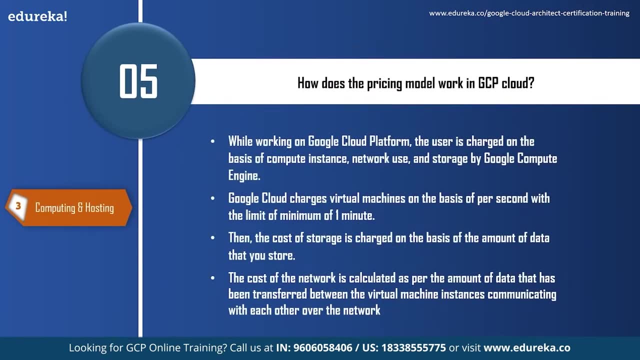 and Google App Engine. so now let us move on to our next question, which is: how does the pricing model work in GCP cloud? so to generally answer this question, you can say: while working on Google Cloud Platform, the user is charged on the basic of compute instances, network use and 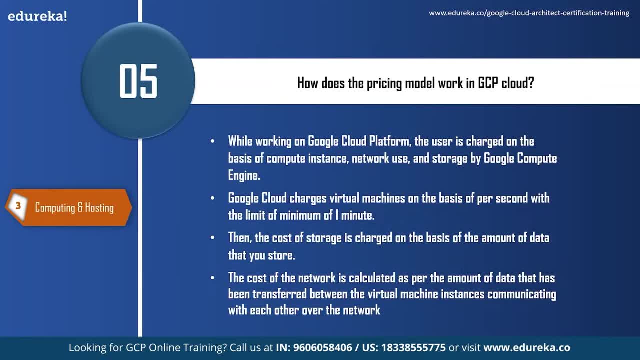 storage by Google Compute Engine. now you can see here I'm not specifically talking about a particular service, this is just an general overview. Google Cloud charges virtual machines on the basis of per second, with a limit of minimum of one minute. then the cost of the storage is charged on the basis of the amount of. 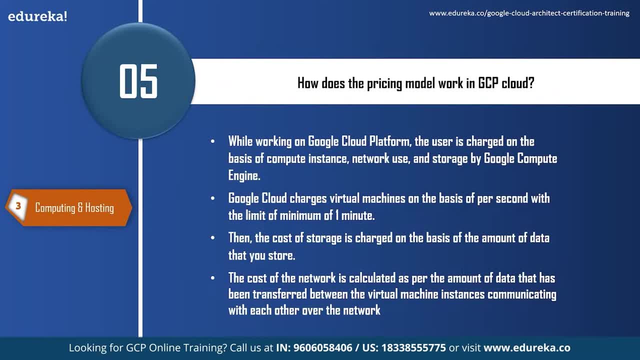 data that you store. the cost of the network is calculated as per the amount of data that has been transferred between the virtual machine instances and the overall location of the virtual machine instances between the virtual machine instances, with what. all those options work in the plugin user. so those two. 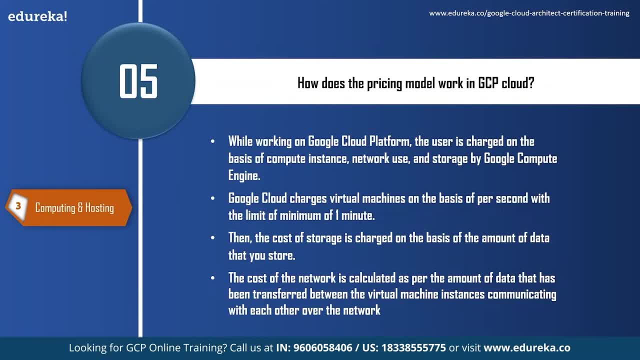 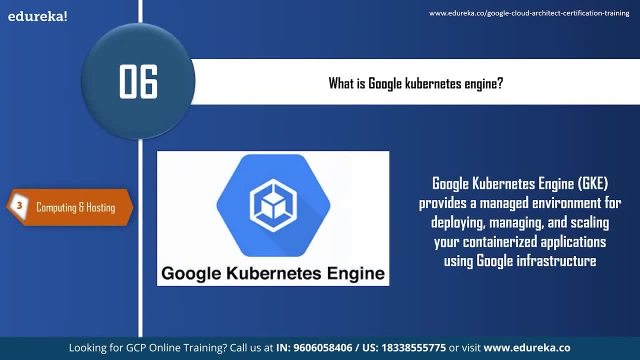 purposes, I'dminv for team user. so if you want to make your lives easier by הר, Community or Anchorage, but with the watts that baller, specifically while communicating with each other or over the network- over the network means the internet, if you prepare yourself with the questions on Google Cloud, 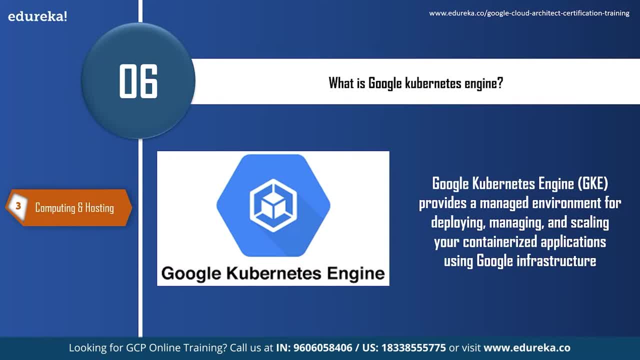 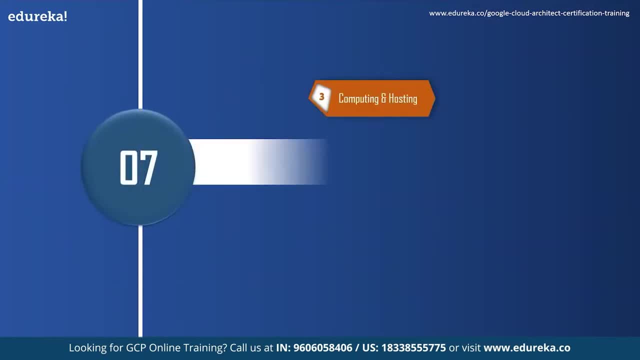 Platform pricing models at these arm on the most common Google cloud interview questions and manage containerized applications. So this was the definition of Google Kubernetes Engine. The next question is a scenario based question. So if I want to run my application on GCP, 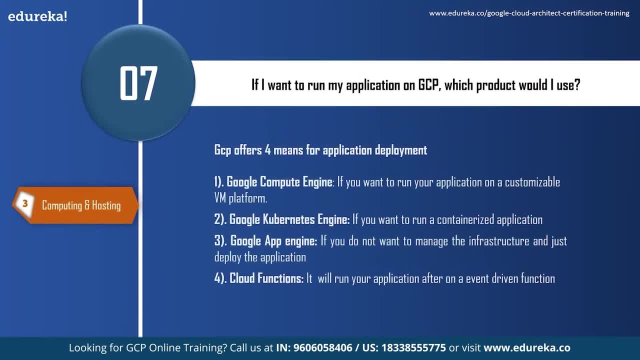 which product would I use? You can answer this by saying it depends on the application requirements. GCP basically offers four means for application deployment, such as Google Compute Engine, Google Kubernetes Engine, Google App Engine and Cloud Functions. You can use Google Compute Engine. 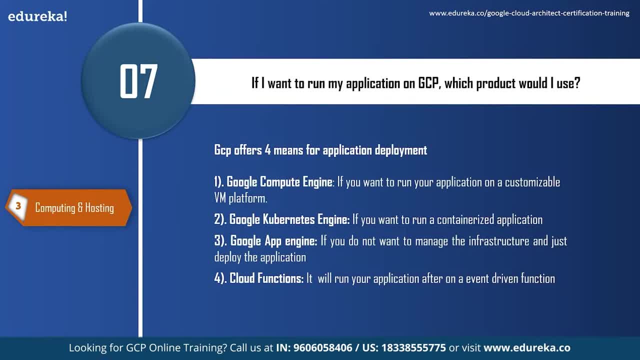 if you want to run your application on a customizable virtual machine platform. Next, if you want to run a containerized application, you can use Google Kubernetes Engine. You can use Google App Engine if you do not want to manage the infrastructure and just deploy the application. 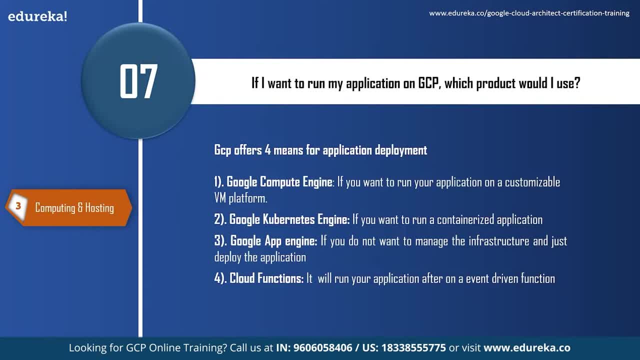 without worrying about scaling your servers. Next, with Cloud Function, it will run your application after an event-driven function. That means only after a particular event occurs your application will be deployed. So these were the four primary means for application deployment model. 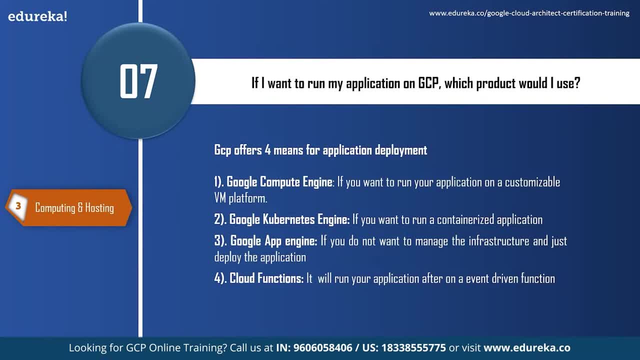 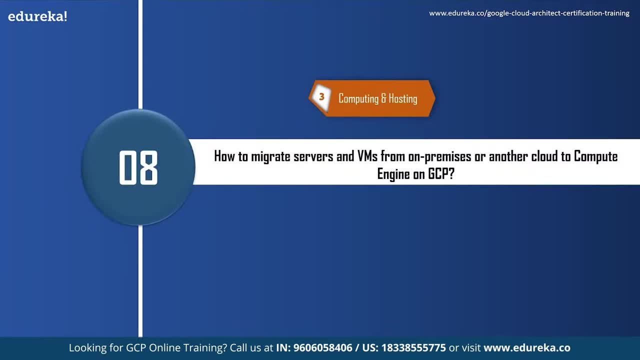 You can also tell the interviewers you can use a combination of these services. So let us see the next question. The next question is how to migrate servers and virtual machines from on-premises or another cloud to Compute Engine on GCP. So if the interviewer asks you this question, 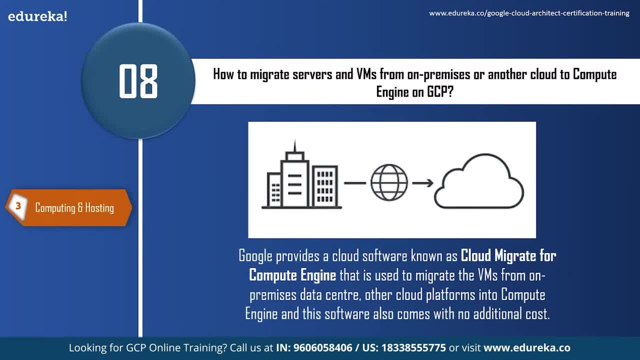 you can just say. Google provides a cloud software known as Cloud Migrate for Compute Engine. The software is used to migrate the virtual machines from on-premises data centers or any other cloud service providers into Compute Engine in the GCP platform. You can use the cloud service provider on GCP platform. 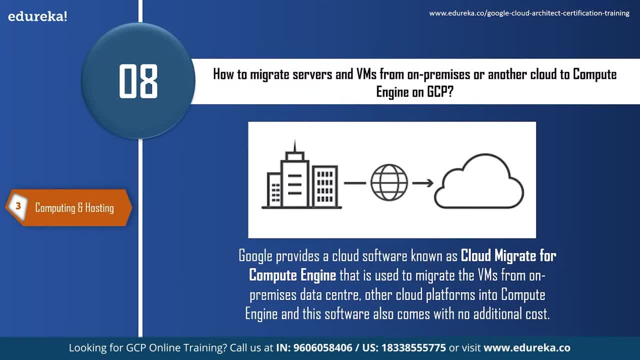 You can also mention, the software is provided by Google itself, and it comes with no additional cost. Now they can also ask this question as: what is Cloud Migrate for Compute Engine sensors? The answer would be the same. So now let us move on to the next question. 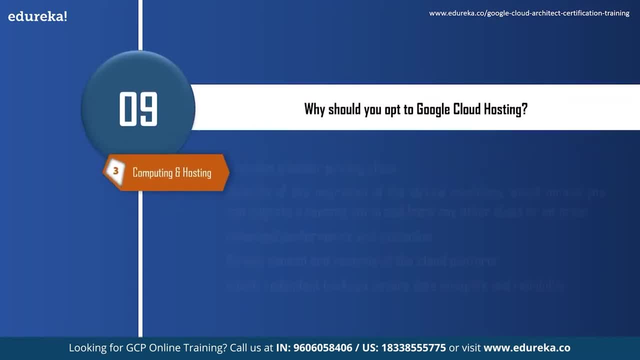 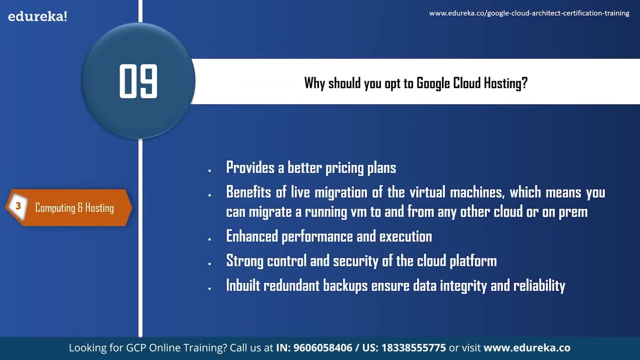 and see why should you opt for Google Cloud hosting? This question is usually asked in Google Cloud consultant interviews. The interviewer may ask this question to check your knowledge and explanation skills about Google Cloud. So here talk about the advantages of choosing Google Cloud hosting. 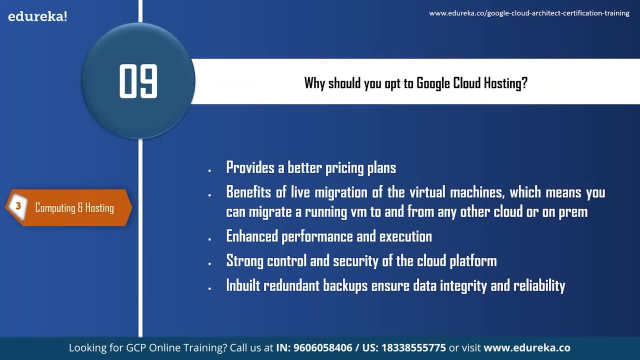 The first advantage is it provides a better pricing plans. Next, there's the benefit of live migration of virtual machines, which means you can migrate a running virtual machine to and from any cloud service providers, or on-premises also. The next benefit is it provides enhanced performance. 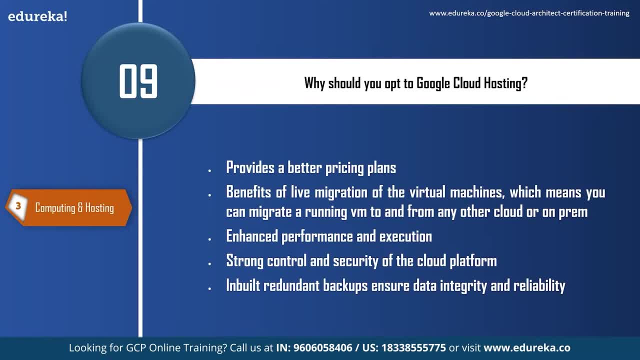 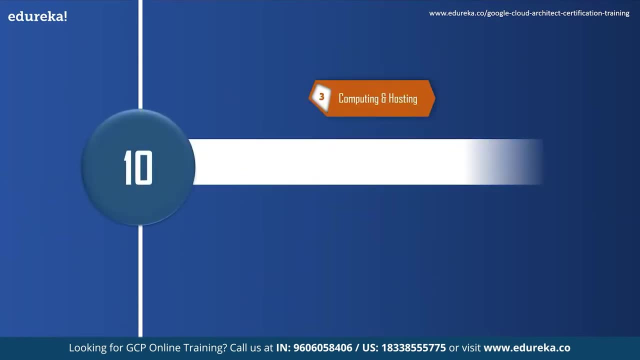 and execution. It also has strong control and security of the cloud platform. The next benefit is it has inbuilt redundant backup, which will ensure data integrity and reliability. So these were some of the benefits of Google Cloud hosting. Let us move on to our next question. 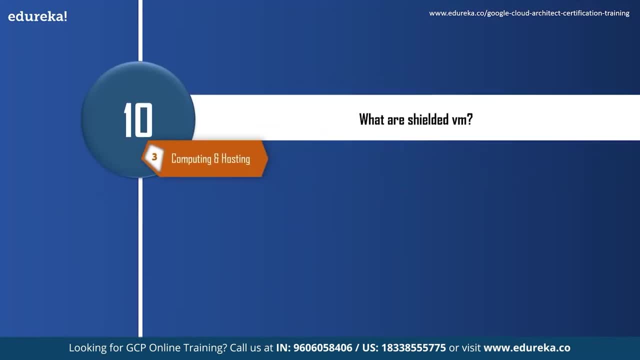 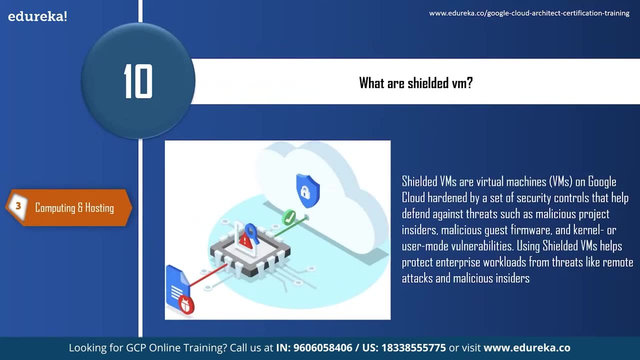 and see what are shielded virtual machines. Shielded virtual machines are virtual machine on Google Cloud which are hardened by a set of security control that helps them defend against threat such as malicious project insiders, malicious guest firmware and kernel or user mode vulnerability. 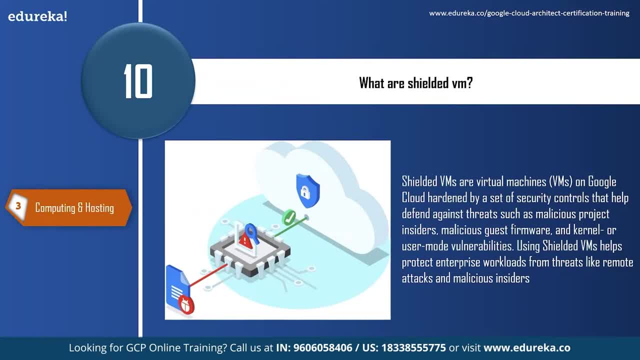 Using shielded virtual machines help protect enterprises workload from threats like remote attacks and malicious insects. So these were some of the questions on compute and hosting services in GCP. So now let us talk about the interview questions in storage and database services in GCP. 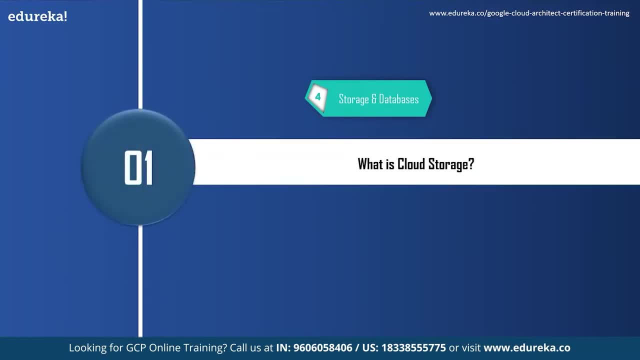 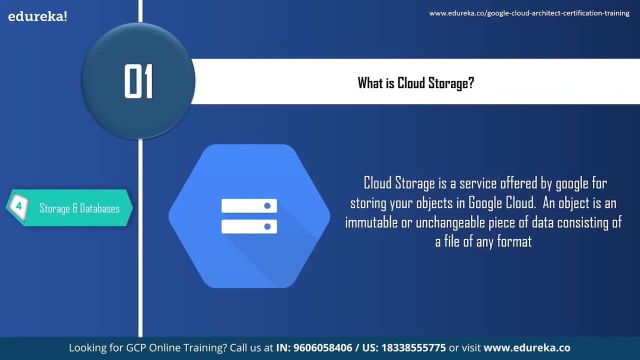 So our first question in storage and database section is: what is cloud storage? Well, cloud storage is a primary storage service in GCP. It is a service offered by Google for storing your objects in the Google Cloud. Now, an object is an immutable or unchangeable piece of data. 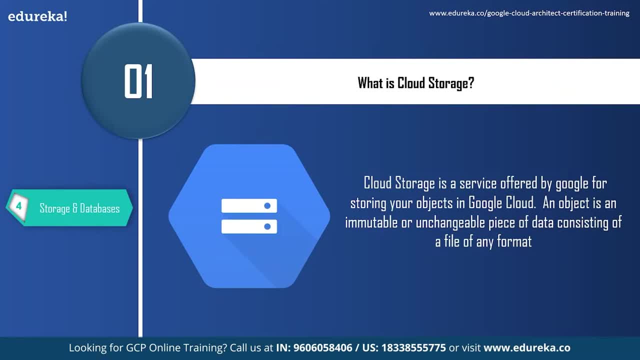 consisting of files of any format. Now, object can be unstructured data, such as music images, videos, backup and log files or archive files. Also, objects have two components, which are object data and object metadata, While object data is typically a file that you want to store, 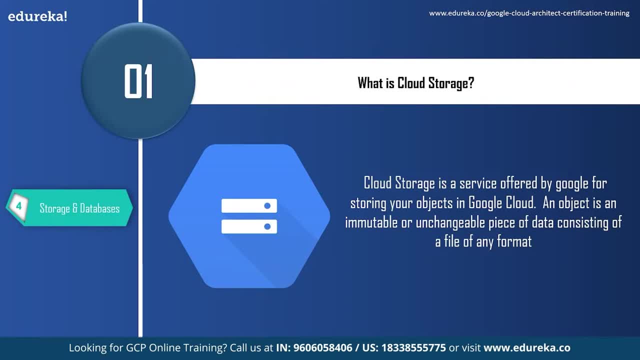 and object metadata is a collection of name value pairs that describes the various object qualities. Now you store these objects in containers called buckets. So when you mention about buckets, there is a high probability of the interviewer asking you: what are buckets in cloud storage? 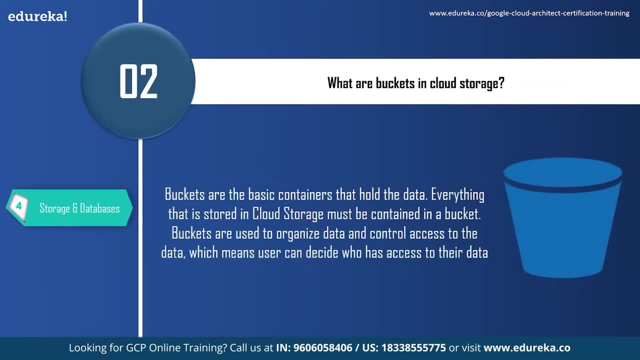 Well, buckets are nothing but a basic containers that hold your data. Now, everything that is stored in cloud storage must be contained in a bucket. You can use bucket to organize your data and control access to your data, which means you decide who has access to your data. 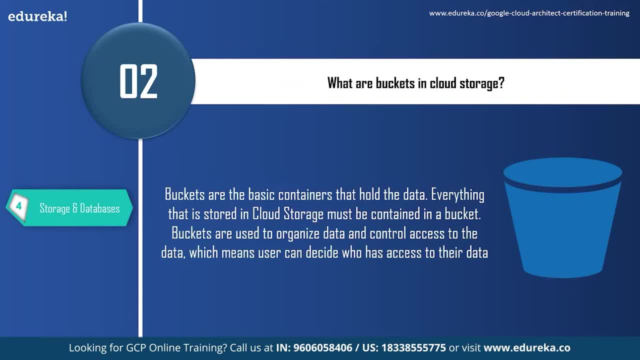 You can create a bucket by specifying a globally unique name for your bucket, Also specifying a geographical location where the bucket and its contents are stored and also a default storage class. So this was about buckets in cloud storage. The next question we're going to discuss is: 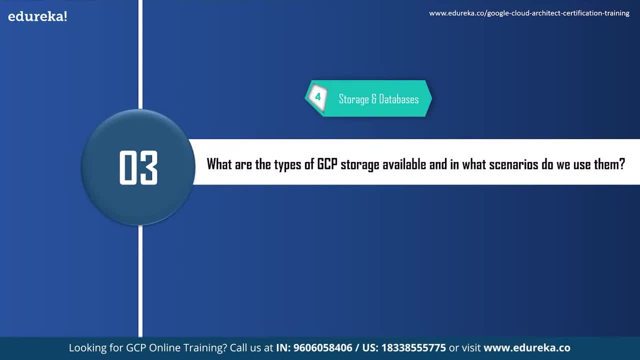 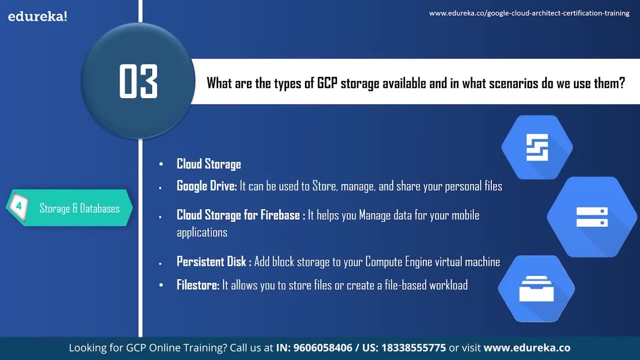 what are the types of GCP storage available and in what scenarios do we use them? Now, here we've already talked about cloud storage, so we move on to the other GCP storage services. Now it offers Google Drive, which can be used to store, manage. 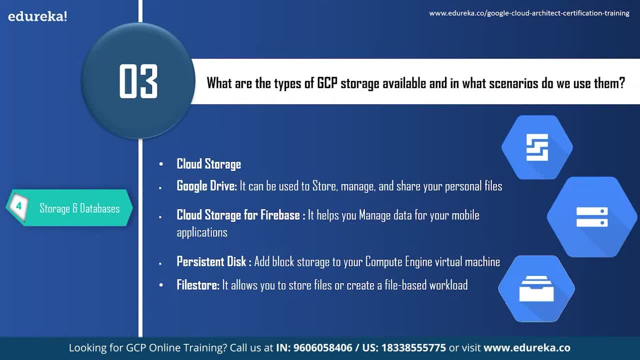 and share your personal files. Next, we have cloud storage for Firebase, which helps you manage data in your mobile applications. The next storage service is persistent disk. Now, this is a block storage which can be added to your compute engine, virtual machines. And last, we have file store. 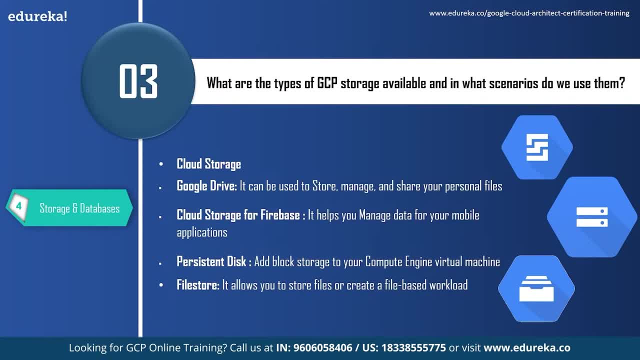 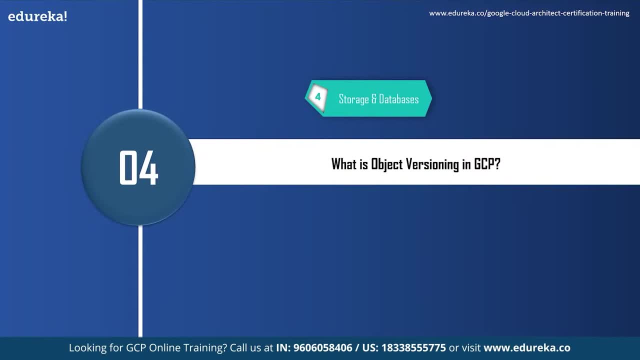 which allows you to store files or create a file based workload. So these were the GCP storage services. Our next question is: what is object versioning in GCP? Well, object versioning is used to retrieve objects which are overwritten or deleted. 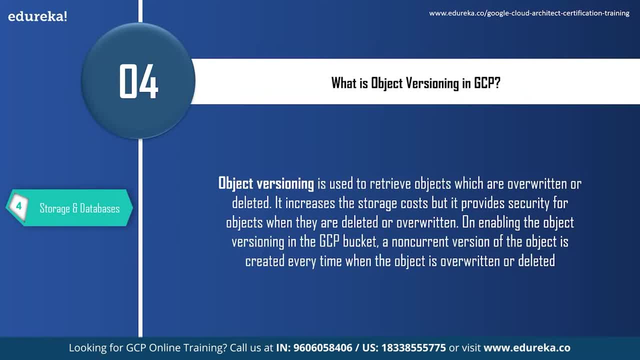 So let's say I have updated a file in cloud storage. Now the updated file and the file before updating, both version will be available to me. So if the updated file gets deleted by mistake or I want to check what other file before they update, 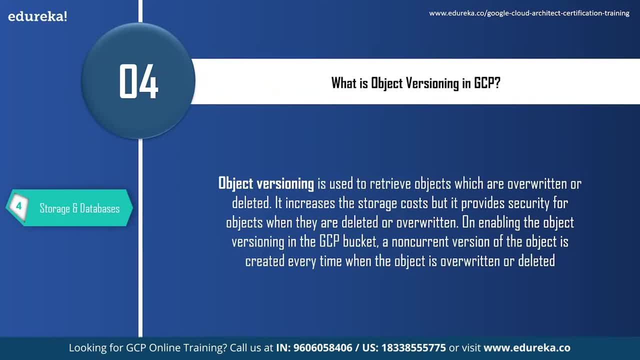 I can do that with the help of object versioning. One disadvantage of this would be it increases the storage cost, But it would provide me security for objects when they're deleted or overwritten. And on enabling the object versioning in GCP bucket. 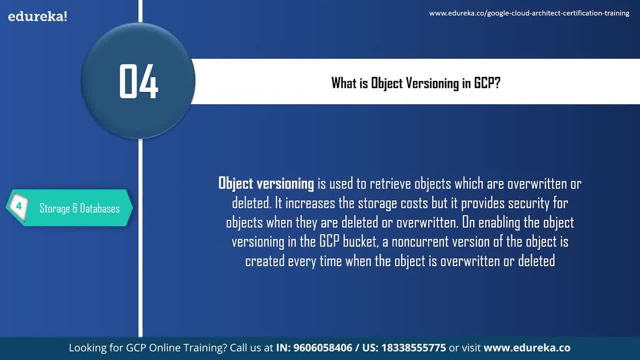 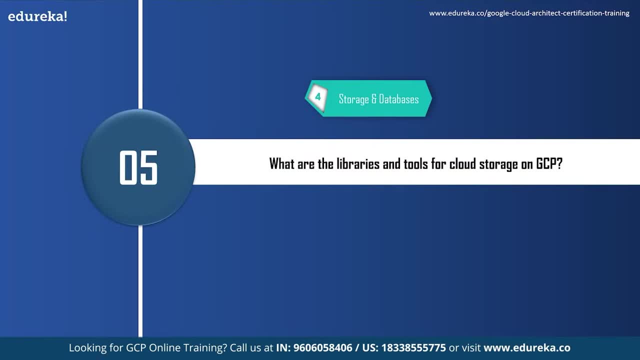 a non concurrent version of the object is created every time when the object is overwritten or deleted. So the next question in storage and database section is: what are the libraries and tools for cloud storage on Google Cloud Platform? Well, you can answer this question by mentioning 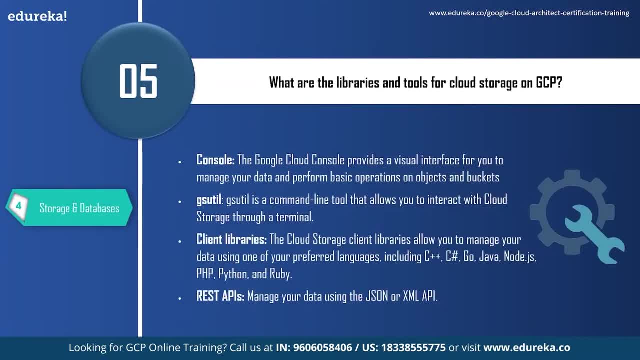 the libraries and tools such as console, gsutl, client libraries and rest apis. Now, console is nothing but the Google Cloud Console, which provides a visual interface for you to manage your data and perform basic operational on objects and buckets. Next, gsutl is a command line tool that allows you to interact. 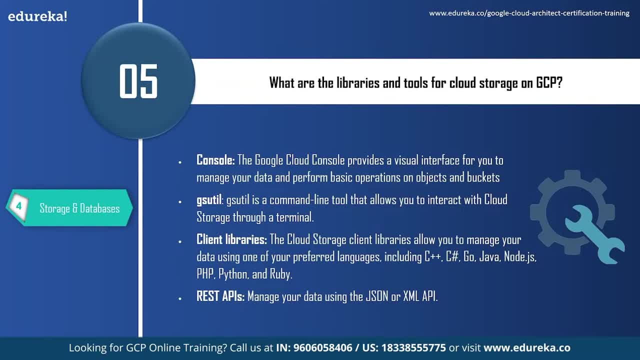 with cloud storage through a terminal. Next, we have the cloud storage client libraries, which allows you to manage your data using one of the preferred language, which would include C++, C, hash, Go language, Java, NodeJS, PHP, Python or Ruby. 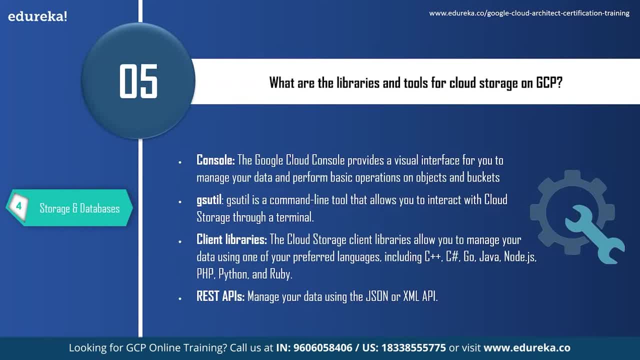 The next tool for accessing cloud storage on GCP is rest apis. Now you can manage your data using the JSON or XML apis. So these were the libraries and tools for cloud storage on Google Cloud Platform. So now moving on to our next question. 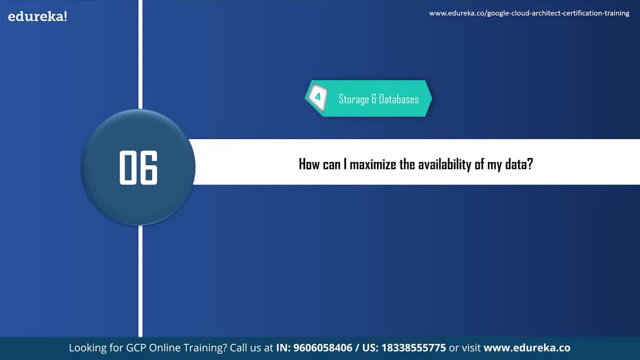 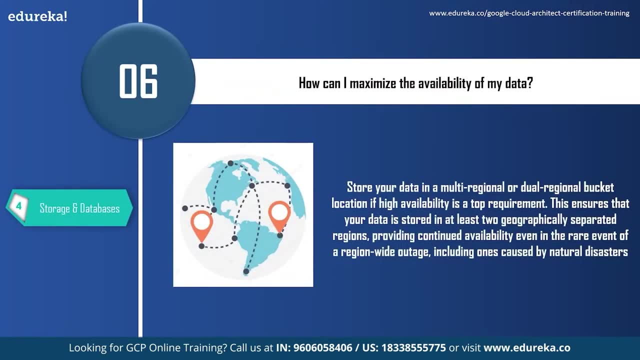 how can I maximize the availability of my data or how can my important data be more secure and available to me? You can answer this by saying you can store your data in multi-region or dual region bucket location if high availability is a top priority. This ensures that your data is stored in at least two geographical. 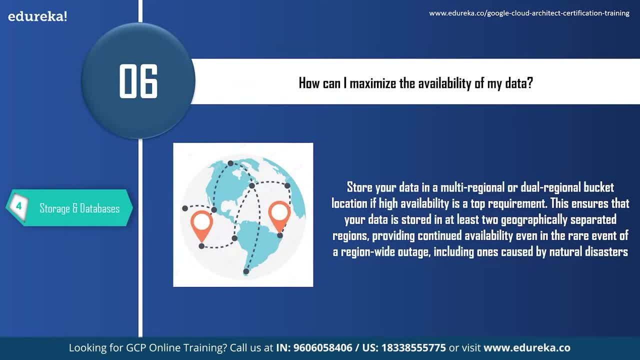 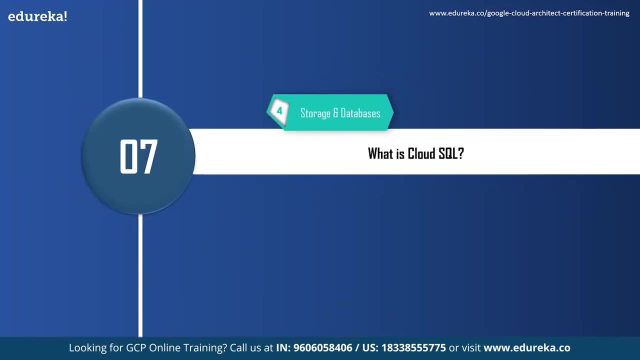 separated region which will provide you continued availability even in the rare event of a region-wide outage, which includes anything caused by natural disasters. So this is what GCP offers for more availability of their data. Moving on to our next question: what is Cloud SQL? 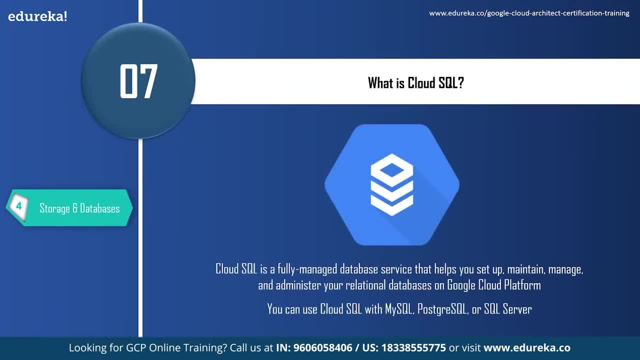 Well, Cloud SQL is a fully managed database service that helps you set up, maintain, manage and administer your relational database on the Google Cloud Platform. We can also mention you can use Cloud SQL with MySQL, PostgreSQL or the SQL Server. Well, Cloud SQL is one of the core database service. 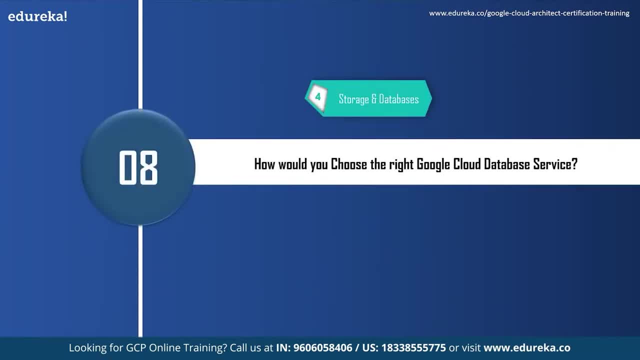 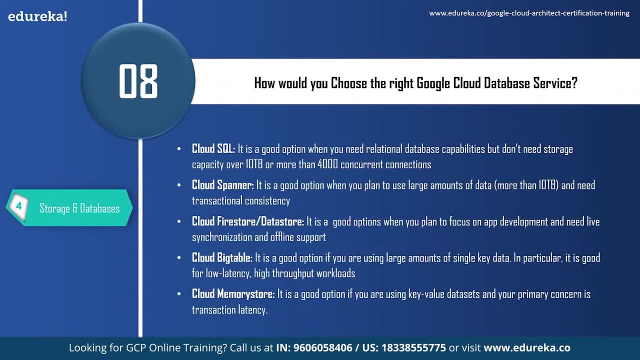 in Google Cloud Platform. The next question is: how would you choose the right Google Cloud database service? Well, this would definitely depend on the requirement. You can select from any of these options. You can select either Cloud SQL, Cloud Spanner, Cloud Firestore Data Store, Cloud Big Data or Cloud Memory Store. 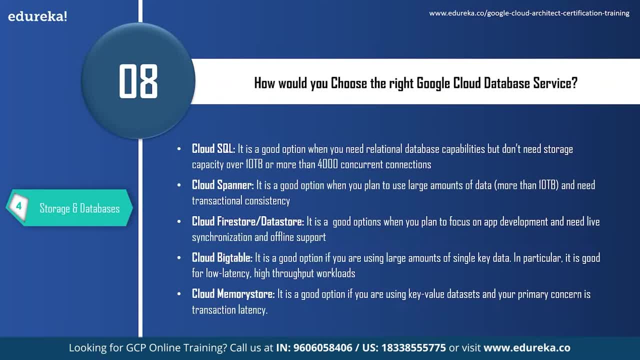 You can choose Cloud SQL when you need relational database capacity but do not need storage capacity over 10 TB or more than 4000 concurrent connections. Next, you can select Cloud Spanner when you plan to use large amount of data, which is typically more than 10 TB. 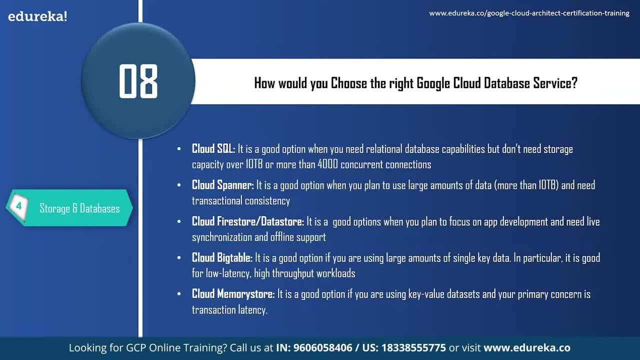 and need transactional consistency. Next, you can use Cloud Firestore or Data Store when you plan to focus on application development and need live synchronization and offline support. The next option is Cloud Bigtable. Now, Cloud Bigtable is a good option if you're looking for large amount of single key data. 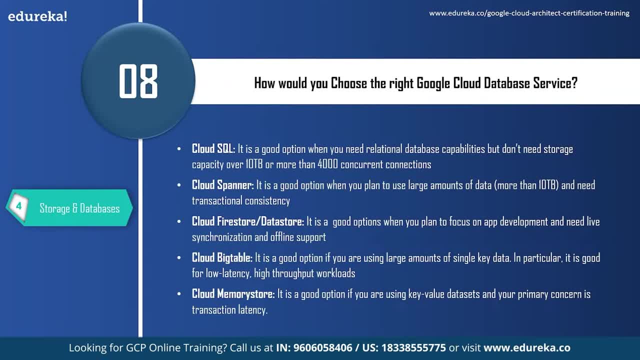 in particular, which is good for low latency and high throughput workloads. And the last option is Cloud Memory Store. Now, this would be a good option if you're looking for key value data sets and your primary concern is transactional latency. These were some of the Google Cloud database services. 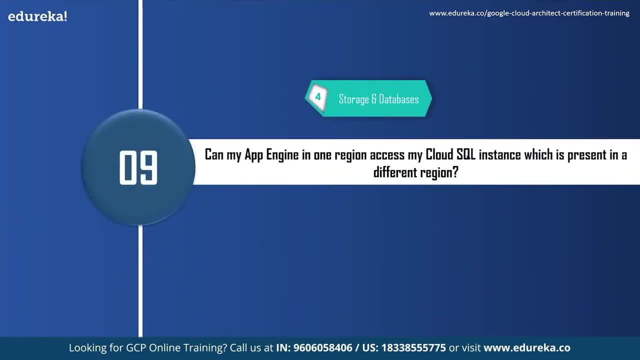 So now let us move on to our next question, which is a scenario-based question. So the question is: can my App Engine in one region access the Cloud SQL instance which is present in a different region? Well, the simple answer for this question: 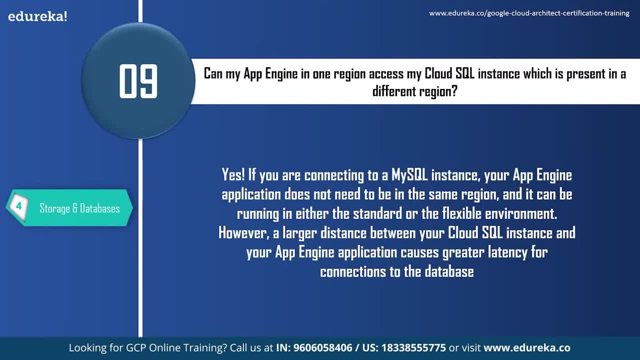 is yes. If you're connecting to a MySQL instance, your App Engine application does not need to be in the same region, and it can be running in either the standard or the flexible environment. However, a larger distance between a Cloud SQL instance and your App Engine application causes greater latency. 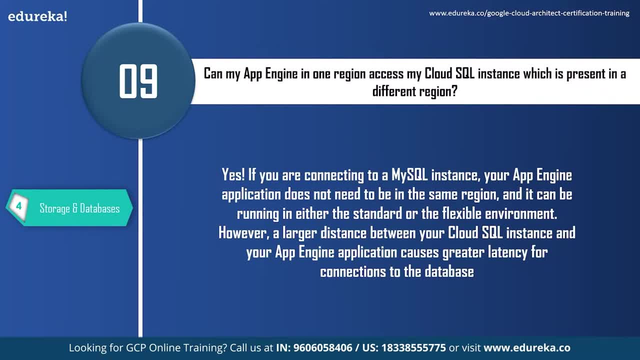 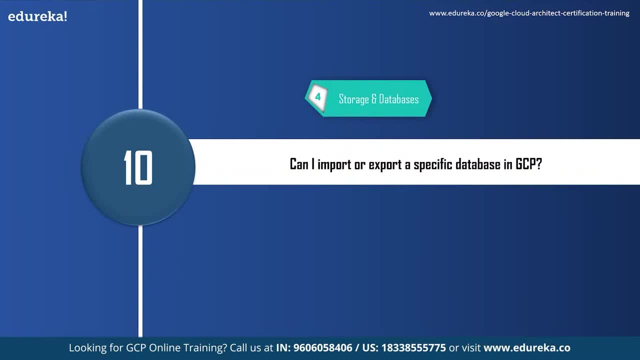 for connection to the database. Now, latency is nothing but a delay in the transmission of data. So next question in the storage and database section is: can I import or export a specific database in Google Cloud Platform? Well, the answer for this is also yes. 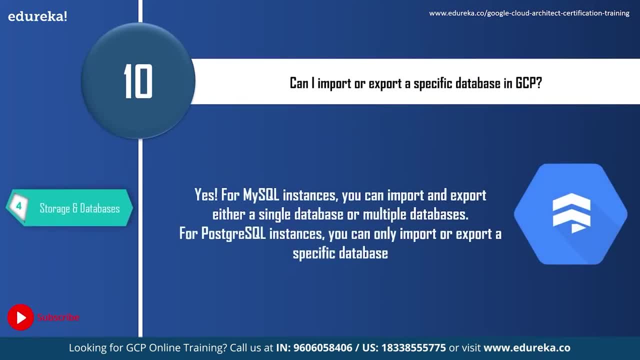 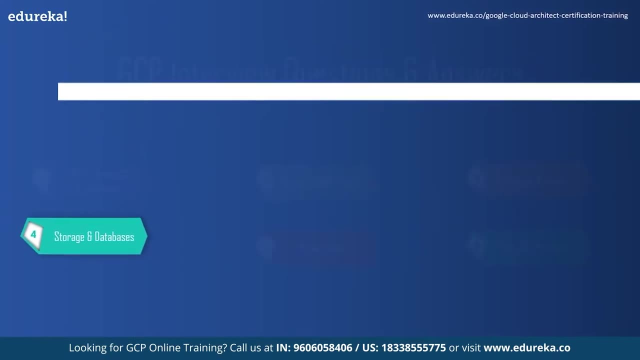 For MySQL instances, you can import and export either a single database or multiple database, And for PostgreSQL instances, you can only import or export a specific database. Now, these were some of the questions in storage and database service in GCP. Now let us move on to our next set of questions. 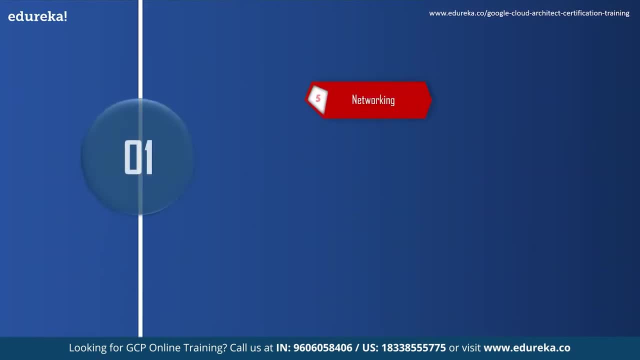 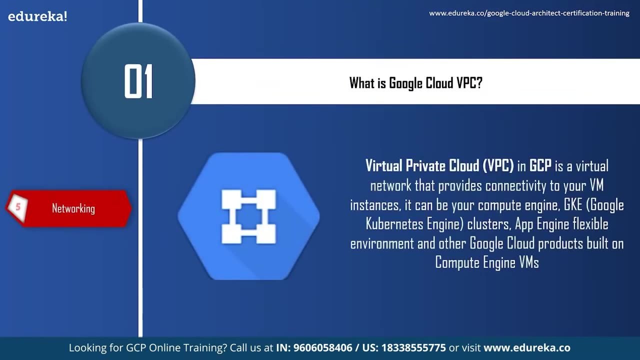 in networking. So the first question in this section is: what is Google Cloud VPC? Now, if you're applying for any Google Cloud VPC, you're expected to know this answer. Virtual Private Cloud in GCP is a virtual network that provides connectivity. 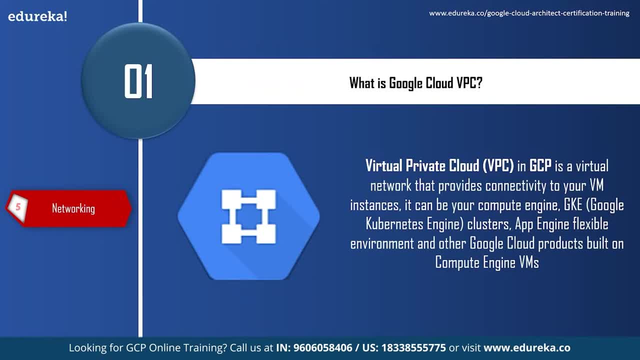 to all your virtual machine instances. It could be your compute instance, Google Kubernetes, Engine clusters or your App Engine, flexible environment and any other Google Cloud products which are built on the compute instances. So you don't have to talk in detail about VPC. 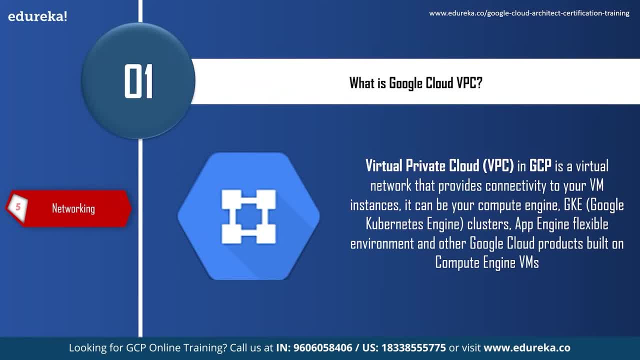 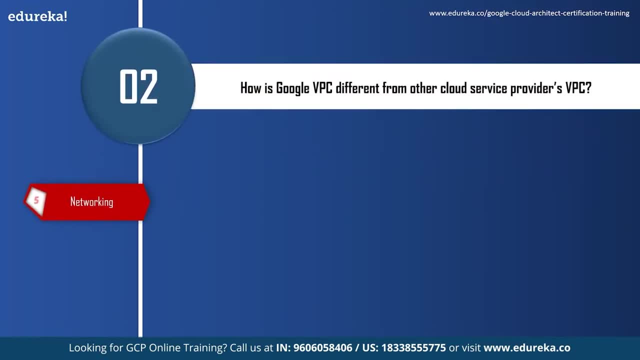 You can just define it. so the interviewer knows that you have some knowledge about VPC. So the next question is: how is Google VPC different from any other cloud service providers? VPC So, as you can see in the diagram, in the traditional VPC or the VPC provided, 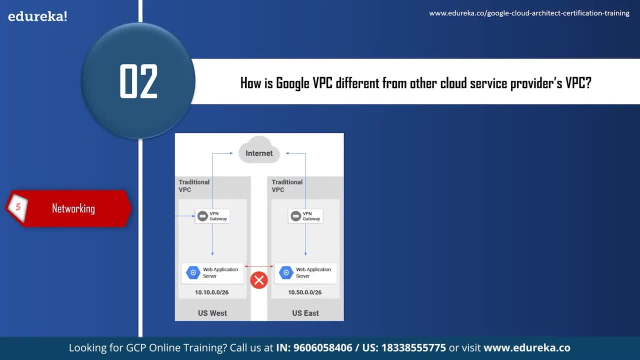 by other cloud service providers like AWS. the architecture would look something like this. Now, here in the first diagram, you can see there are two VPC built with two different subnet in two different regions, which are US West and US East. Now the virtual machine in one region. 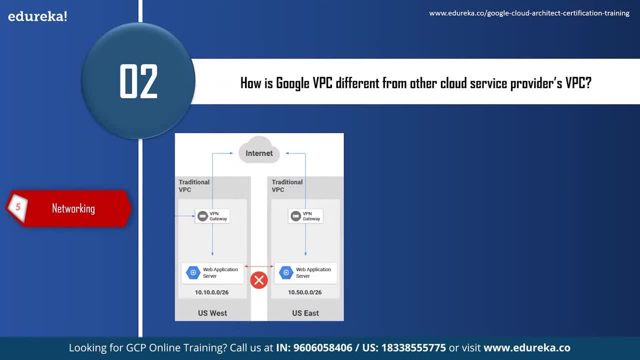 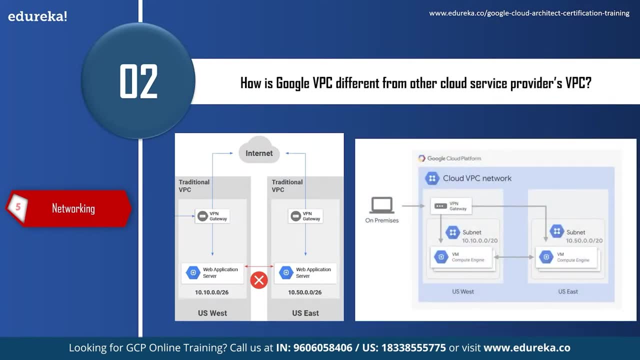 can access the internet and communicate with the other virtual machine only through the VPC gateway. Now this gateway acts as an interface. So now in a traditional VPC, one virtual machine cannot directly communicate with the other virtual machine. Now in Google version of Virtual Private Cloud, 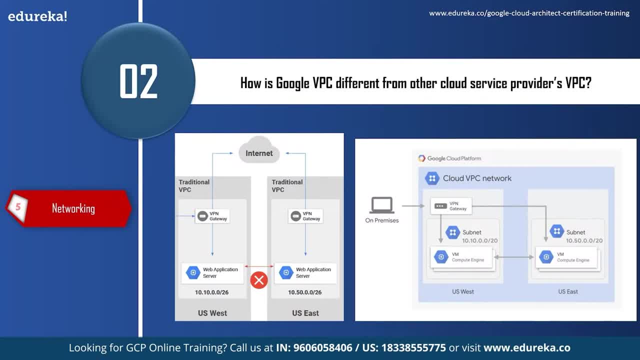 it follows a global construct, which means, instead of creating a VPC in US East and US West, you can just create one VPC and put the subnets in different region within that VPC. Now, in this case, the virtual machines present in one region. 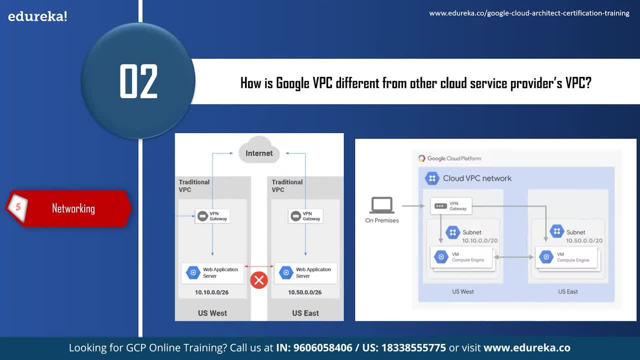 can directly communicate with the virtual machine in the other region without the help of VPN gateway. Now I guess you have some idea about how Google VPC is different from the VPC of other cloud service providers. Now, if you have understood the concept, 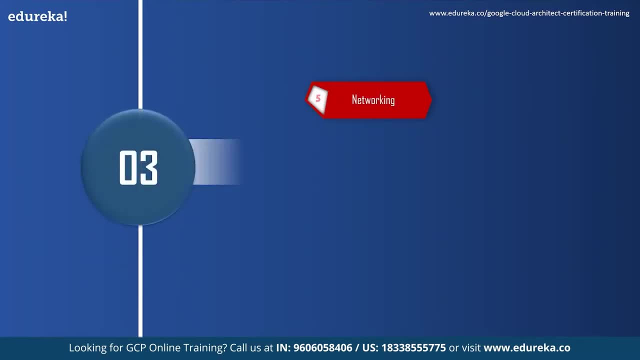 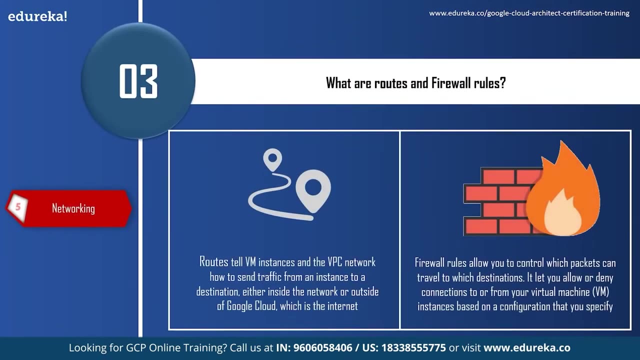 you can put the answer in your own word and explain it. The next question in networking is: what are routes and firewall rules? Now, when we talk about VPC, this question comes tagged along. Now, route tells the virtual machine instances and the VPC network how to send traffic. 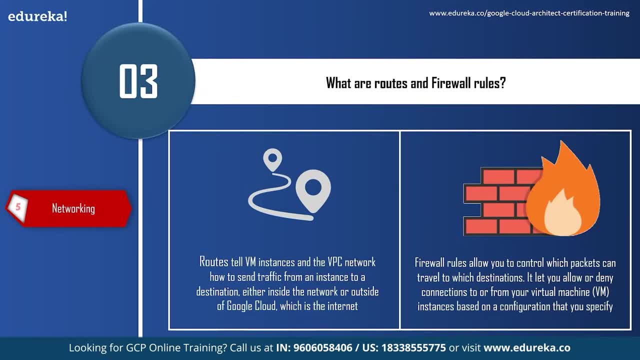 from one instance to the destination. This destination can be either inside the network or outside of the Google Cloud, which is typically the internet. Next, firewall rules are rules which allow you to control which packets can travel to which destination. It lets you allow or deny connection. 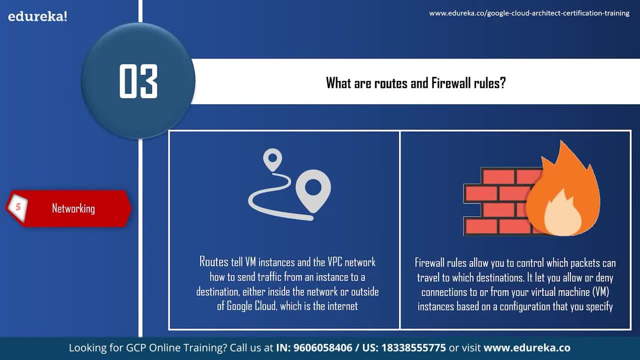 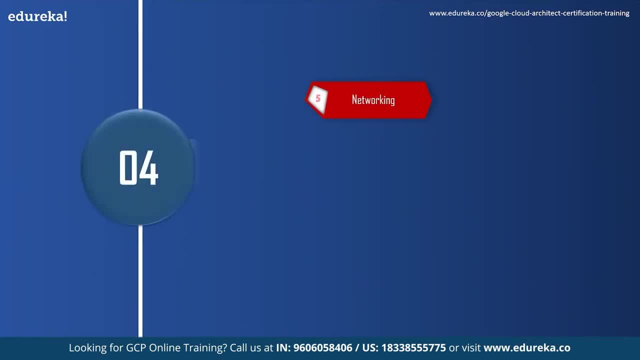 to and from your virtual machine instances based on the configuration that you specify. So this was about routes and firewall rules in Google Cloud networking. So our next question is: what is load balancing? Now, this is a frequently asked question in many GCP interviews. 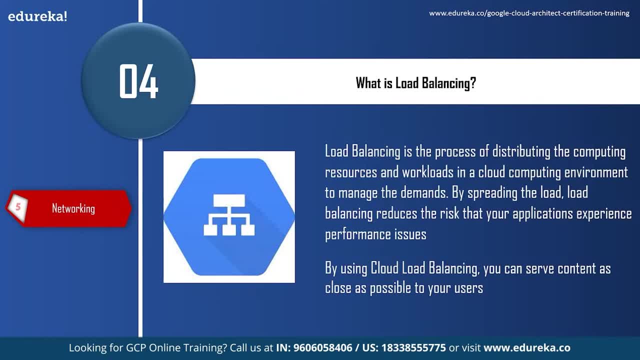 Load balancing is a process of distributing the computing resources and workload in a cloud computing environment to manage the demands. By spreading the load, load balancing will reduce the risk that your application will experience performance issues. By using cloud load balancing, you can serve content as close as possible to your users. 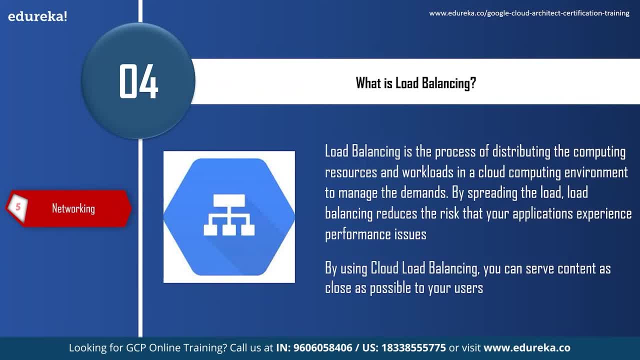 We can also mention this point that cloud load balancing is a fully distributed, software-defined managed service. It is not hardware-based, so you don't have to manage a physical load balancing infrastructure. So this was about load balancing. Our next question is: 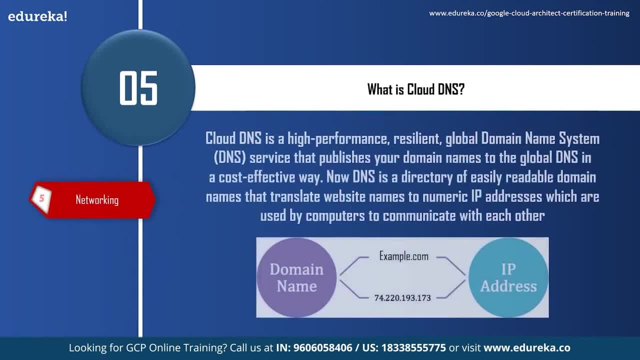 what is cloud DNS? Well, cloud DNS is a high-performance, resilient global domain name system service that publishes your domain name to the global DNS in a cost-effective way. Now, DNS is nothing but a directory of easily readable domain names that translate website names. 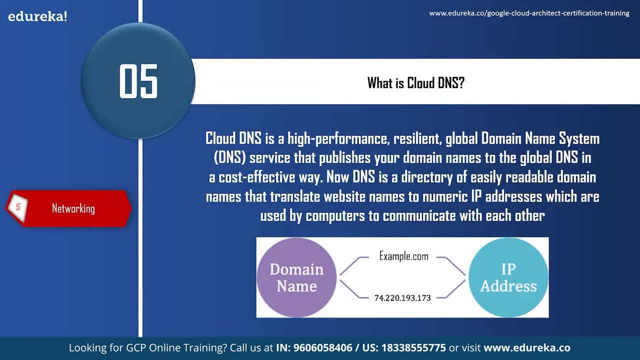 into numerical IP addresses which are used by computers to communicate with each other. For example, when you type a URL in your browser, DNS converts the URL into an IP address of a web service associated with that name, Like wwwexamplecom. is translated to the IP address of 72.220.193.173.. 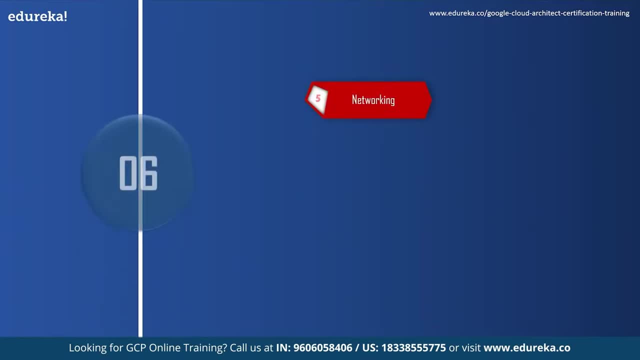 Now I guess you have some idea about DNS. Now let us move on to our next question. Now next question is a scenario-based question: How can I connect my existing network to Google Cloud resources? You can answer this by saying: Google provides four options to do this. 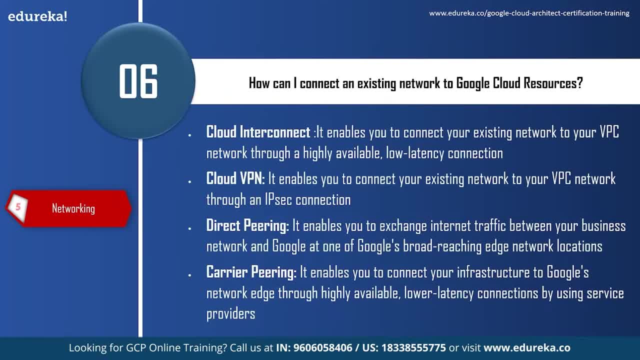 The first one is through cloud interconnect, The second one is through cloud VPN, The third is through direct peering And the fourth one is through carrier peering. Now, cloud interconnect enables you to connect your existing network to a VPC network. 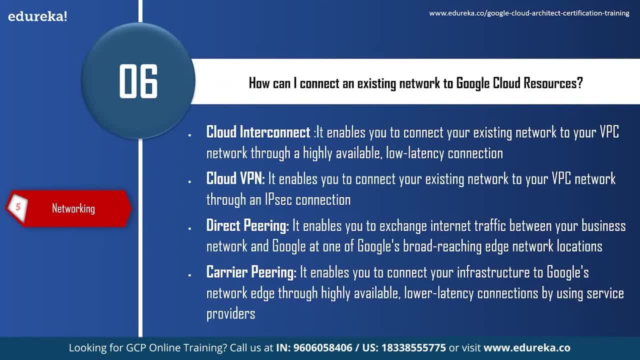 through a highly available low latency connection. You can choose cloud VPN, which will enable you to connect your existing network to a VPC network through an IPsec connection. Next, direct peering enables you to exchange internet traffic between a business network and Google. 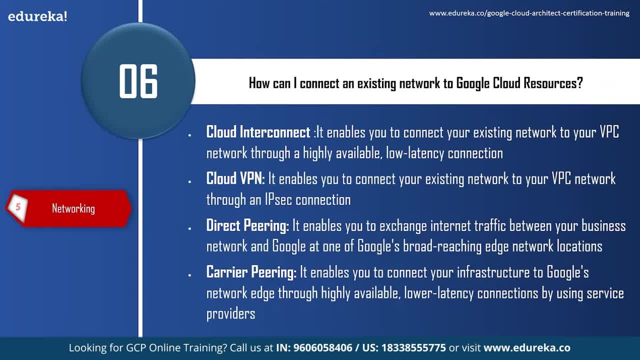 at one of Google's broad reaching edge network locations. And the fourth option is carrier peering, which allows you to connect your infrastructure to Google's network edge through highly available low latency connection which is provided by the service providers. Moving on to our next question, 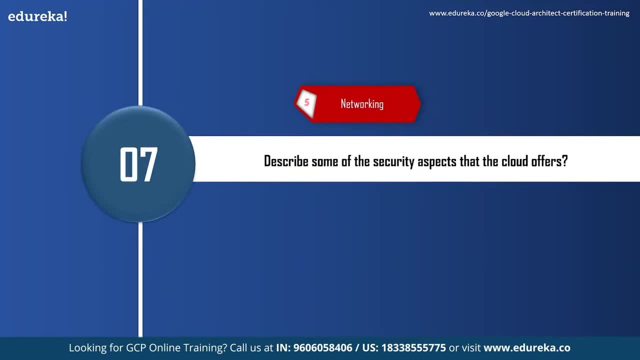 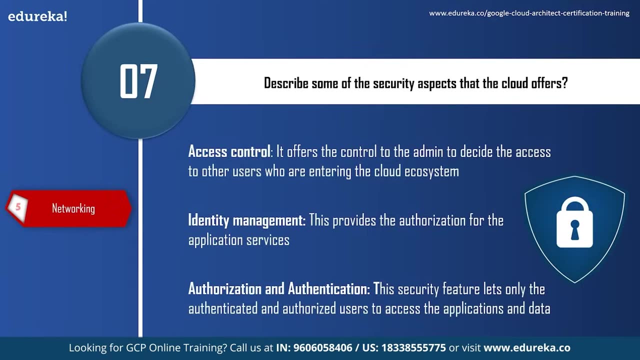 describe some of the security aspects that a cloud offers Well. some of the important security aspects that a cloud offers is access control. It offers the control to the admin to decide the access of other users who are entering the cloud ecosystem. The next security aspect is identity management. 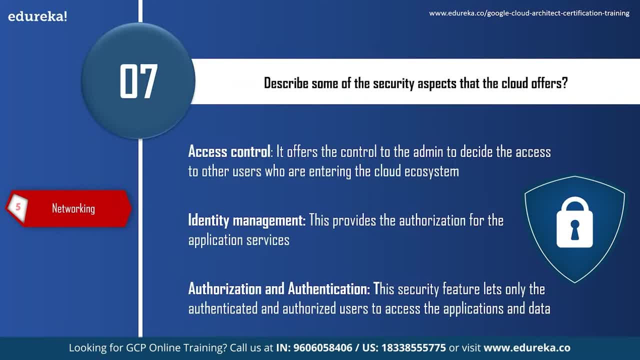 This provides the authorization for the application services. And third is authorization and authentication. This security feature lets only the authenticated and authorized users to access certain applications and data. These were some of the important security aspects that a cloud offers, Moving on to our next question. 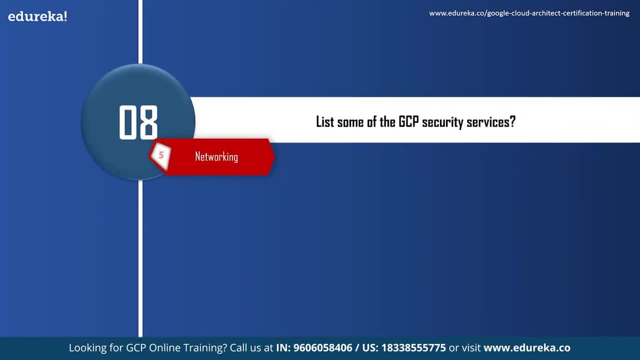 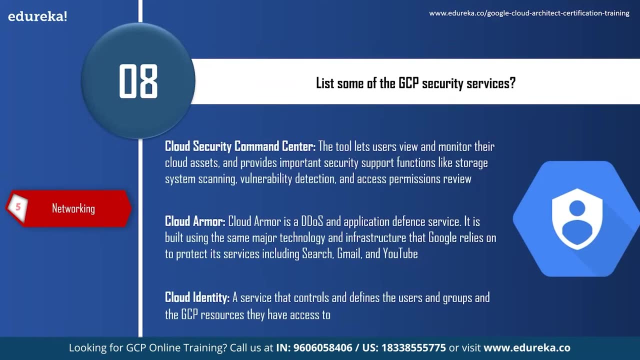 list some of the GCP security services. GCP security services include Cloud Security Command Center, Cloud Armor and Cloud Identity. Cloud Security Command Center is a tool that lets users view and monitor the cloud assets and provides important security support functions like storage system scanning. 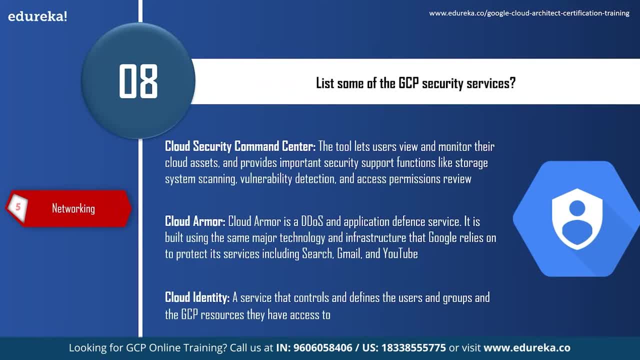 vulnerability detection and access permission reviews. Next, Cloud Armor is a DDoS and application defense system. It is built using the same major technologies and infrastructure that Google relies on to protect its services, including Google Search, Gmail and also YouTube. 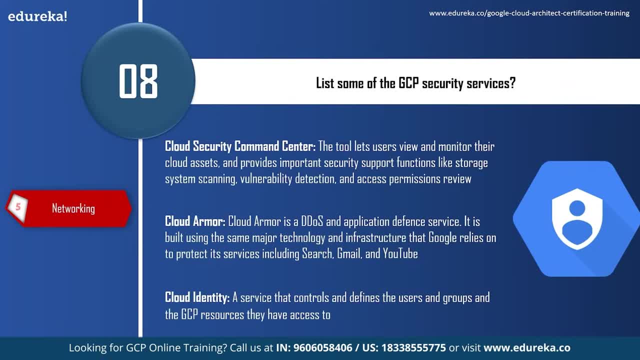 The third security service is Cloud Identity. Now, this service controls and defines the users and groups and the GCP resources they have access to. Now these were some of the GCP security services. So now let us move on to our last set of questions. 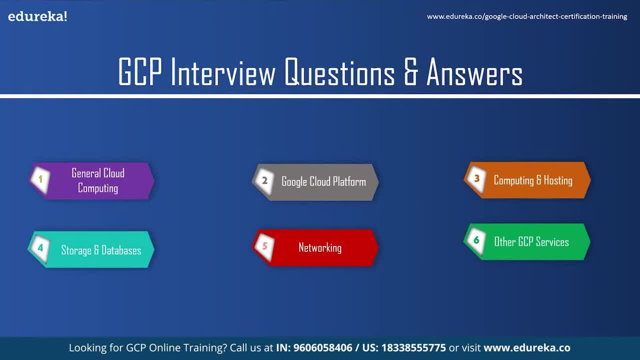 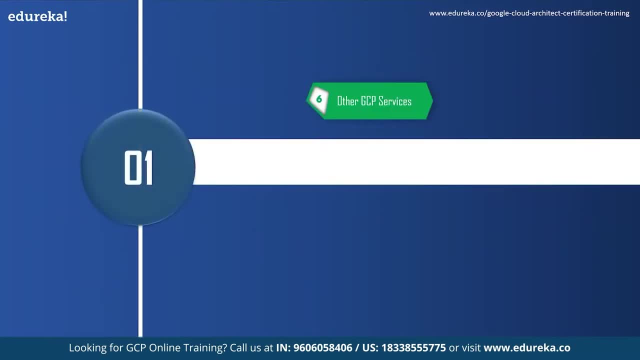 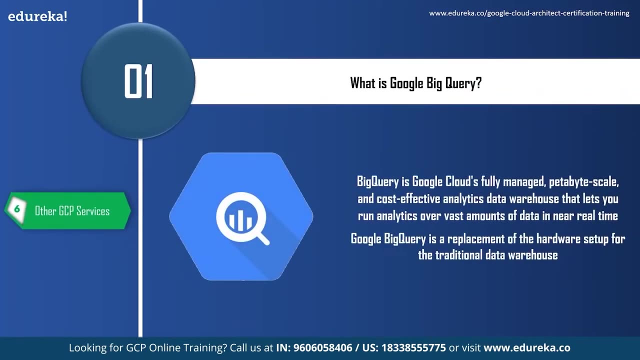 on other GCP services. Now, these other GCP services would include Big Data, Internet of Things and Google Cloud Artificial Intelligence. So the first question in this section is: what is Google BigQuery? BigQuery is a Google Cloud's fully managed petabyte scale and cost effective. 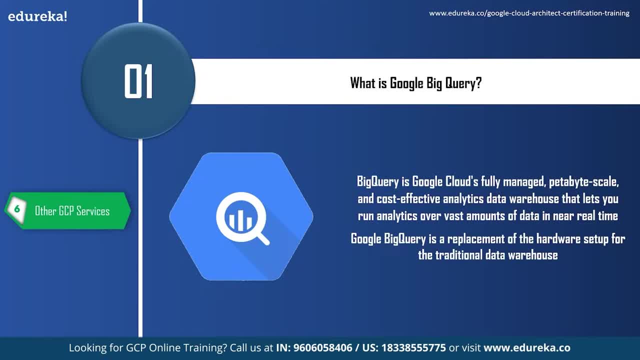 analytics data warehouse that lets you run analytics over vast amount of data in near real time. You can say: Google BigQuery is a replacement of the hardware setup for the traditional data warehouse. You can also mention how the BigQuery organizes its data. We can also mention the BigQuery organizes the data table. 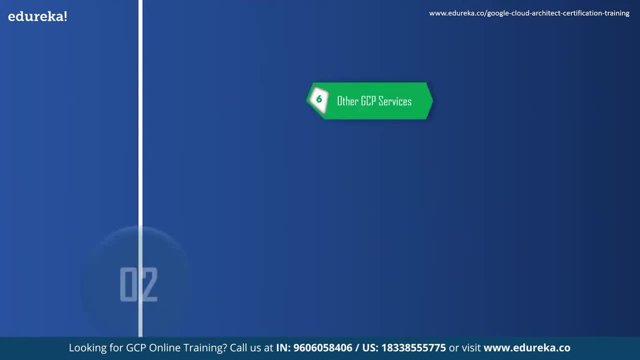 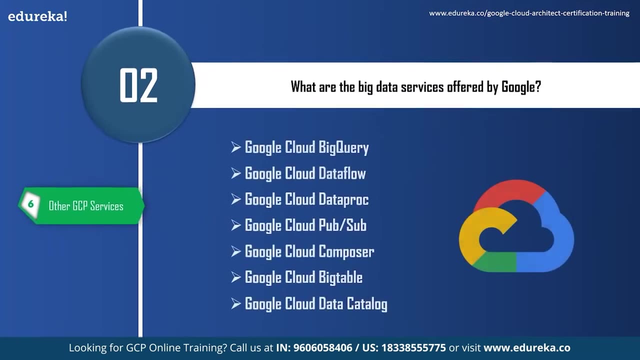 into units that are known as datasets. Moving on to our next question: what are the big data services which are offered by Google Cloud Platform? Well, some of the services are Google Cloud BigQuery, Google Cloud Dataflow, Google Cloud Dataproc. 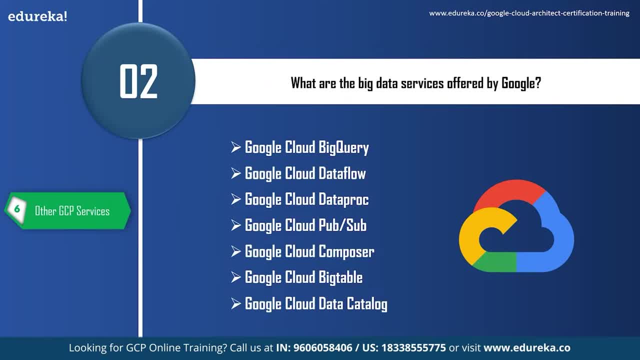 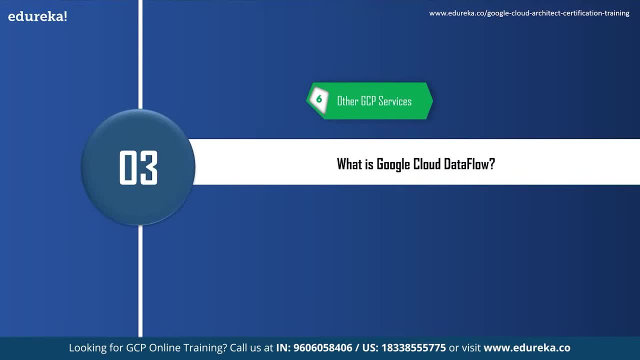 Google Cloud Pub or Sub Google Cloud Composer, Google Cloud Big Data and Google Cloud Data Catalog. Moving on to our next question, what is Google Cloud Dataflow? Well, this is one of the important GCP's big data service. You can answer this question by saying: 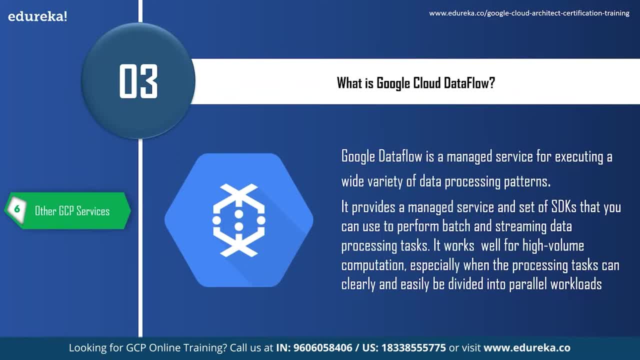 Google database is a managed service for executing a wide range of data processing patterns. It provides a managed service and a set of SDKs that you can use to perform batch and streaming data processing tasks. It works well for high volume computation, especially when the processing tasks 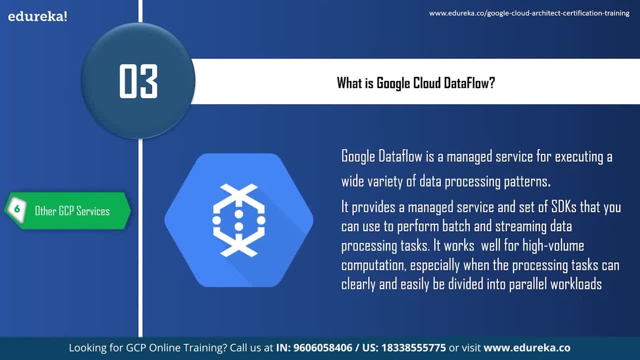 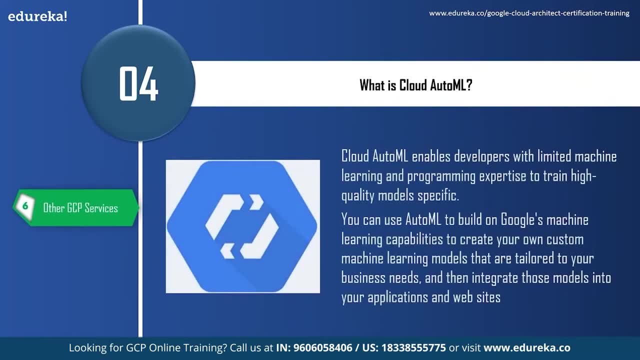 can clearly and easily be divided into parallel workloads. Next, moving on to our next question: what is Cloud AutoML? This is one of GCP's machine learning service. Well, Cloud AutoML is a service that enables developer with limited machine learning. 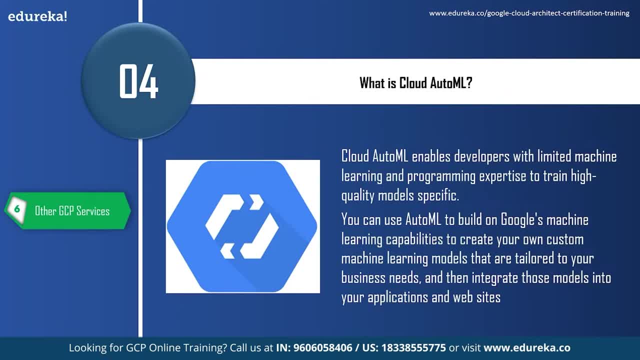 and programming expertise to train high quality model specific. You can use AutoML to build on Google's machine learning capabilities to create your own custom machine learning models that are tailored to your business needs and then integrate those model into application or website, or both. So this was about Cloud AutoML. 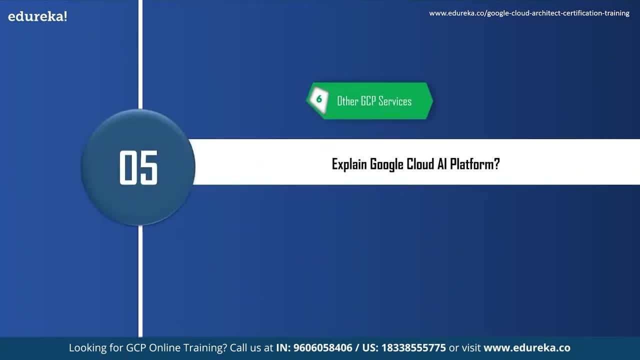 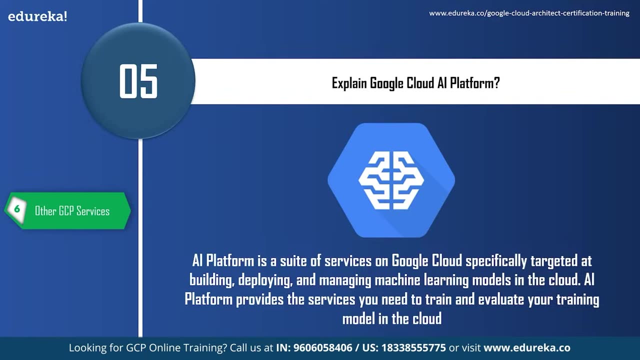 Let us move on to our next question. Our next question is explain Google Cloud AI Platform. Well, AI Platform is a suite of services on Google Cloud which are specifically targeted at building, deploying and managing machine learning models in the cloud. AI Platform provides the services. 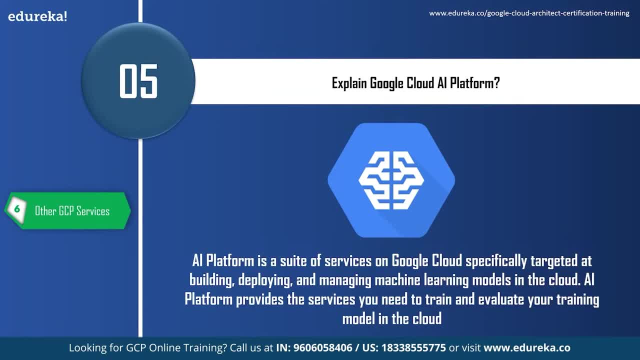 you need to train and evaluate your training model in the cloud. It is integrated with several easy to use tools like BigQuery and data labeling service to help you build and run your own machine learning models and machine learning applications quickly. You can store and manage the large amount. 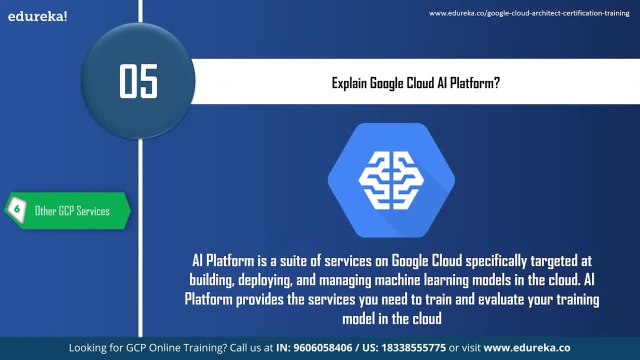 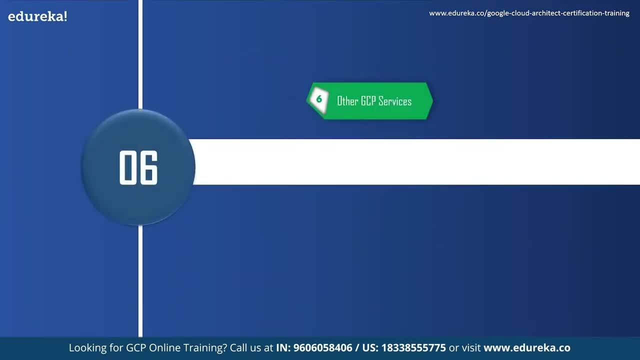 of data with BigQuery and then prepare or label this data for model training using data labeling service. So this was about Google Cloud AI Platform. Now our next question is: what is Cloud IoT Core? Well, Cloud IoT Core is a fully managed service that allows you to easily. 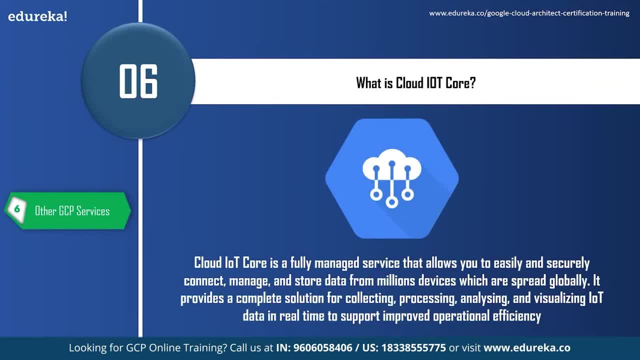 and securely connect, manage and store data for millions of devices which are spread globally. It provides a complete solution for collecting, processing, analyzing and visualizing IoT data in real time to support improved operational efficiency. So this was about Cloud IoT Core. 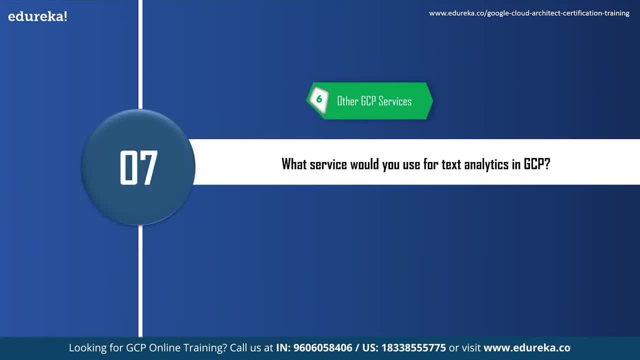 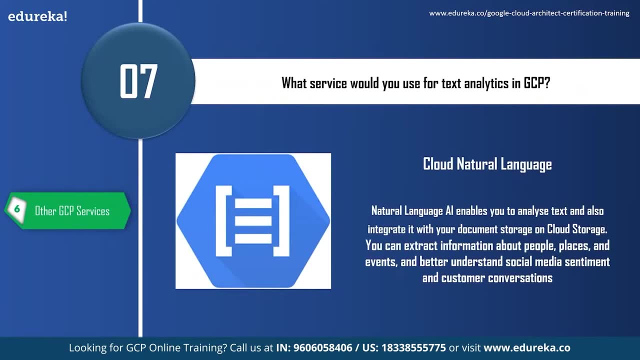 Now let us see the next question. Our next question is: what service would you use for text analytics in Google Cloud Platform? So the service which is used for text analytics in Google Cloud Platform is Cloud Natural Language. Natural Language AI enables you to analyze. 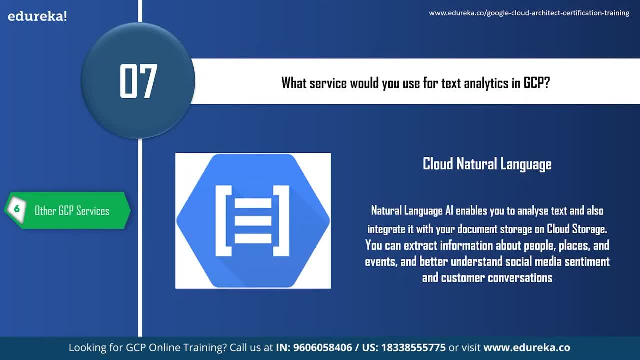 text and also integrate it with your document storage. on cloud storage, You can extract information about people, places and events and have a better understanding about social media sentiments and customer conversations. So these were some of the important and frequently asked GCP questions. 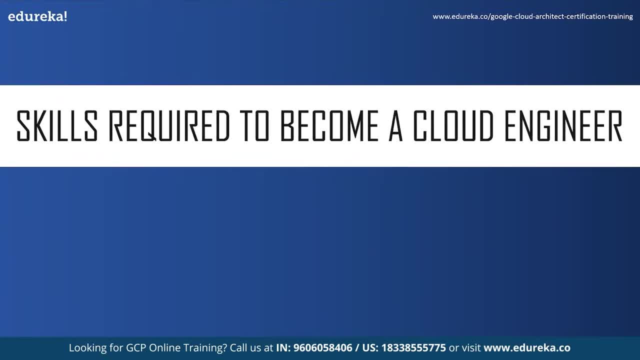 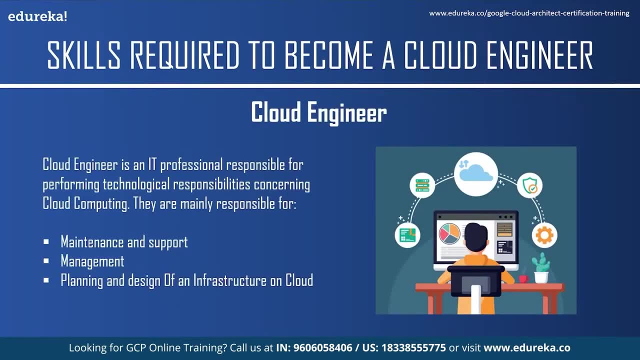 So now let us move on to our next topic and see what are the skills required to become a cloud engineer. So a cloud engineer is an IT professional responsible for performing technological responsibility concerning cloud computing. They are mainly responsible for maintenance and support management planning. 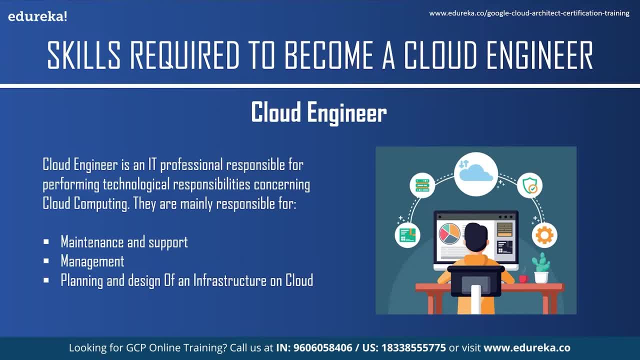 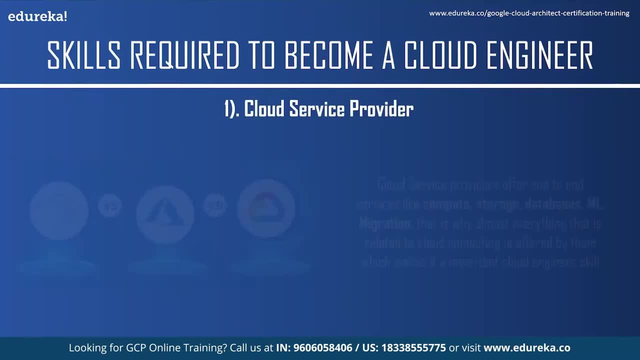 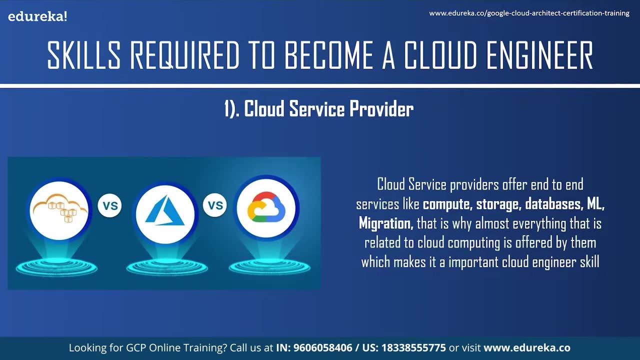 and designing of an infrastructure on the cloud platform. So now talking about the skills required to become a cloud service provider, the first skill is having knowledge about cloud service provider. So if you are thinking of taking the cloud computing career path, spend some time familiarizing yourself. 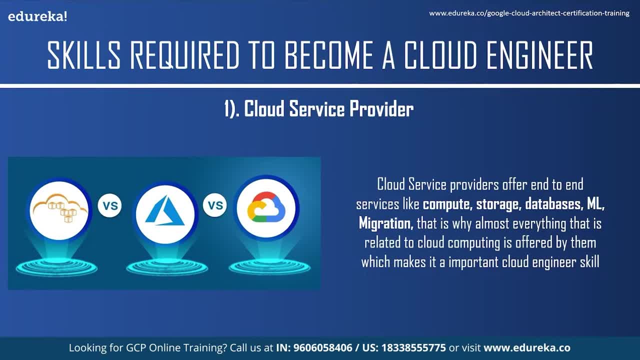 with at least one of the cloud service provider. The top three cloud service providers are Amazon Web Services, Microsoft Azure and Google Cloud Platform. Now, if you want to see a comparison between the two, I will leave a link to that video in the description box below. 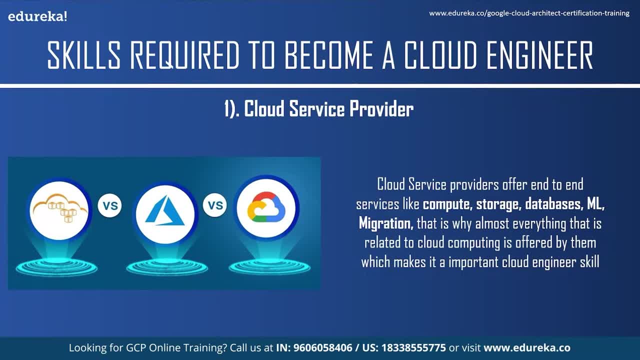 Now these cloud service providers offer end-to-end services like compute storage, databases, ML, migration and many more. It includes almost everything that is related to cloud computing, and this makes it one of the important cloud engineer skills. The next skill is: 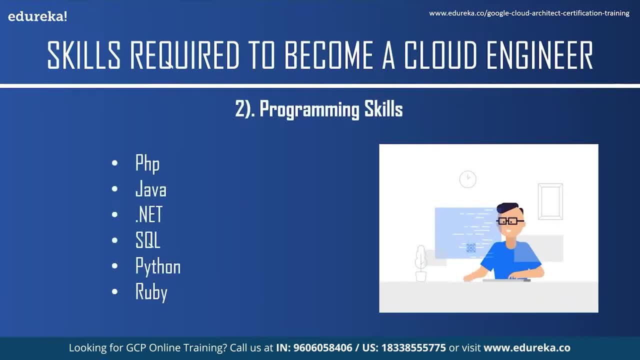 programming skill. This is one of the important cloud engineer skills. Proficiency in programming language is essential for scaling web application. Some of the programming language should be familiar with are PHP, Java, NET, SQL, Python and Ruby. You can learn all of these languages. 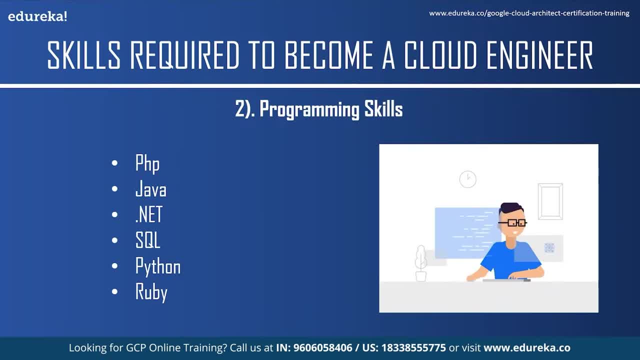 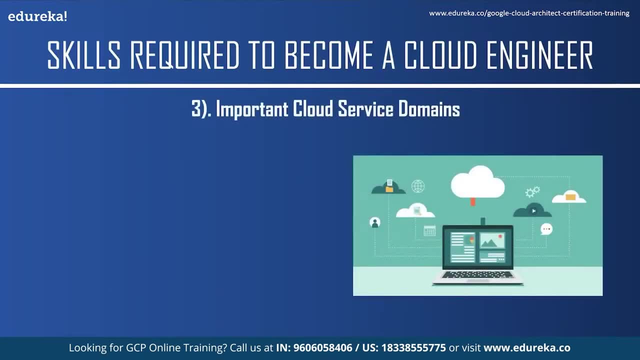 with the help of blogs, online videos or either offline or online classes, but the most important of all is hands-on practice. Now talking about the third skill required to become a cloud engineer is having knowledge about the important cloud service domains. Now, this cloud service domain would include: 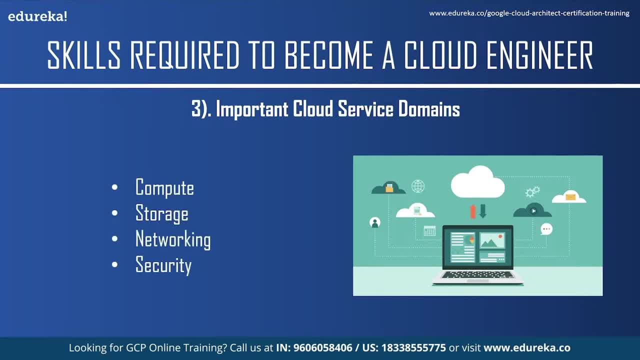 compute, which involves virtualization and serverless computing. Cloud engineers are also familiar with data storage, which deals with data and information which is stored in the cloud. After that, we have networking and security. Now cloud engineers should be familiar with the basic cloud networking concepts. 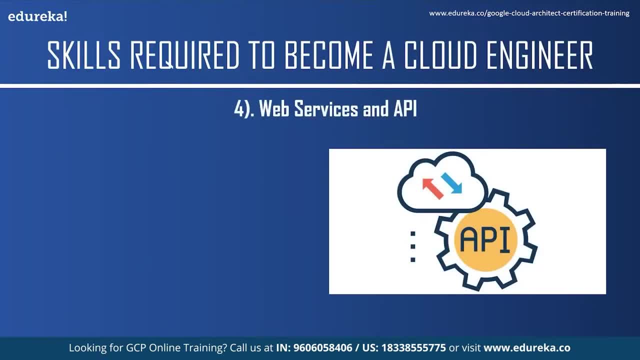 and network security, which includes encryption, authorization and different protocols. Moving on to our next skill, it is web services and APIs. Cloud architects are heavily based on APIs and web services, because web services provides developers with a lot of information: XML, SOAP, WSDL and UDDI open standards. 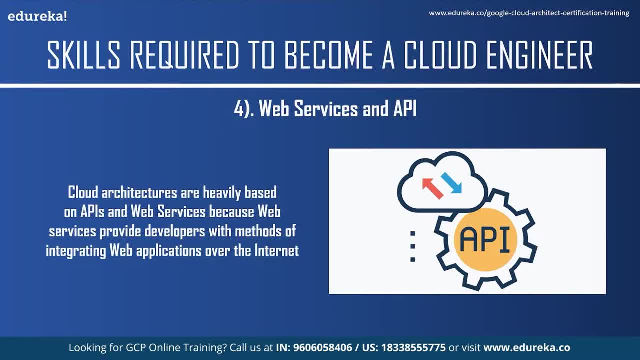 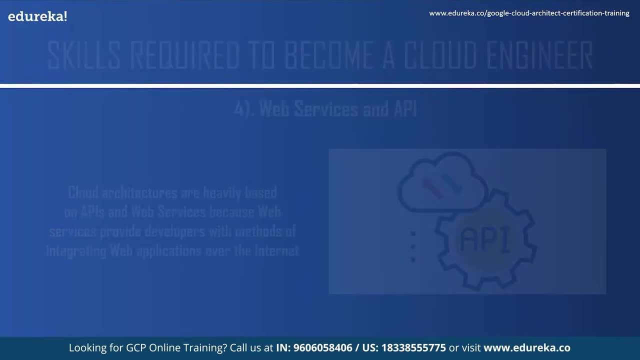 are used to tag data, transfer data, describe and list services available. Plus, you also need APIs to get the required integration done Now. having experience of working on websites and related knowledge would help you have a strong core in developing cloud architectures. The next skill is Linux. 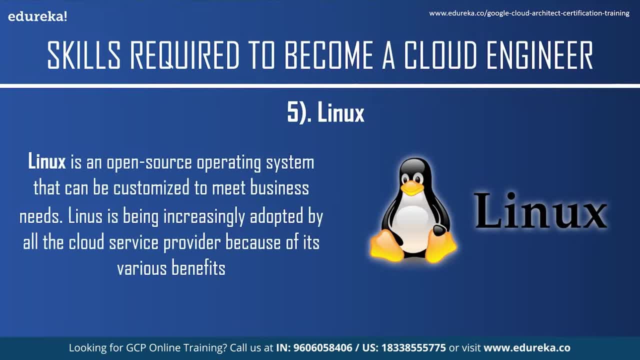 Now, Linux is an open source operating system that can be customized to meet business needs. Linux has been increasingly used by many cloud service providers because of its various benefits, So, as a cloud engineer, you should be able to architect, administer and maintain Linux-based servers.